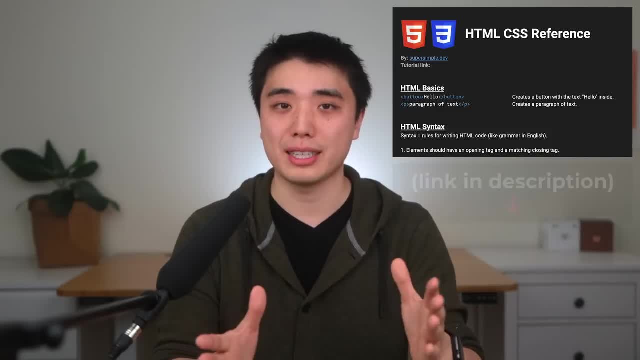 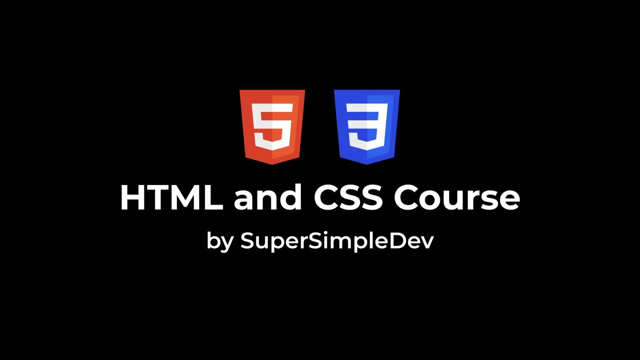 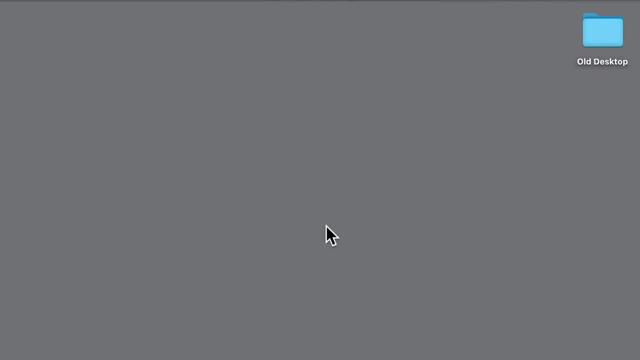 about taking notes. I created an HTML and CSS reference that will list everything that we learn in this course. With that set of lessons said, let's get started. I'm going to be doing this course on a Mac, but everything is the same for a Windows computer. 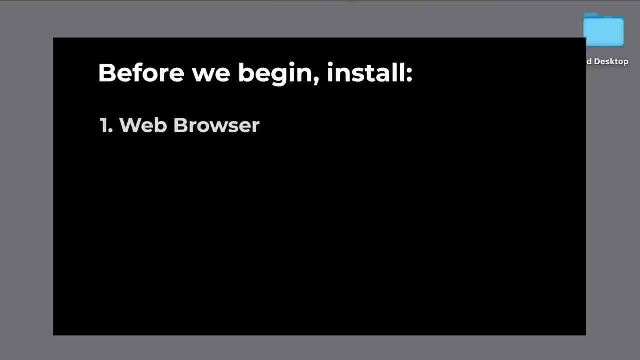 Before we begin, we're going to need two pieces of software: a web browser and a code editor. A web browser lets us view websites on the internet. It's also going to let us view the website that we create in this course. The most popular web browser for web development is Google Chrome. A code. 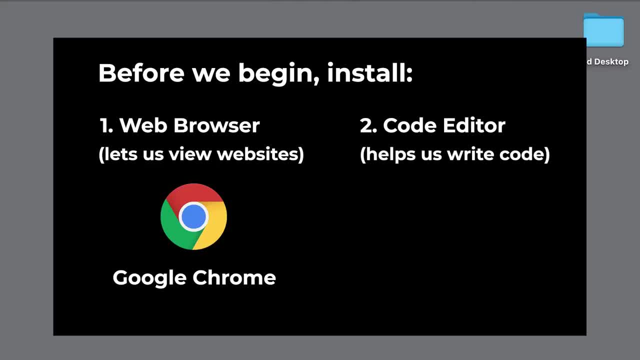 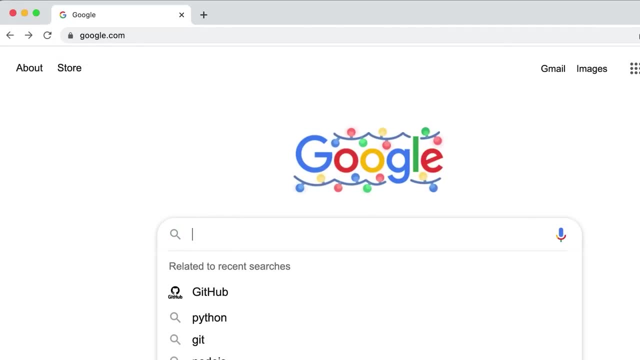 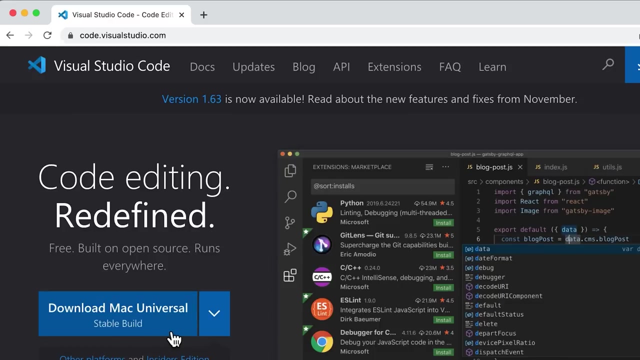 editor helps us write our HTML and CSS code. The most popular code editor for web development is called VS code or Visual Studio Code. To install both of these, we can go to googlecom and then search for Google Chrome or for VS code and then open the first result and follow the instructions to download and install. Once we have those two installed, we can start the course. 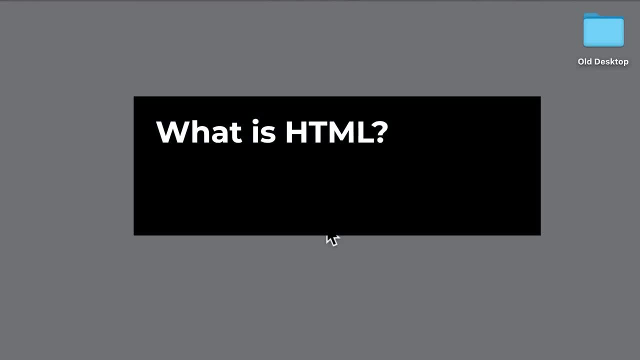 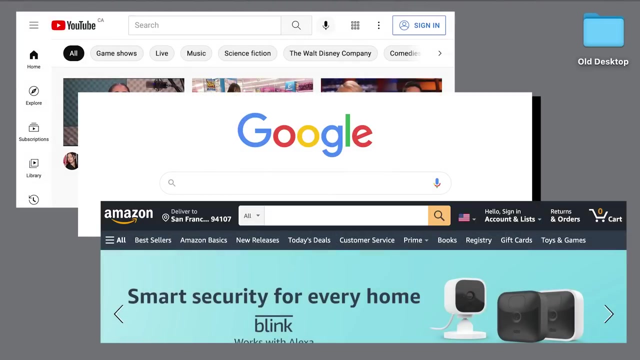 We'll begin by learning what is HTML. HTML stands for Hyper Text Markup Language. You don't have to worry about what that means, just know that it's a tool that we use to create websites. Every website, from YouTube to Google to Amazon, uses a combination of HTML and CSS to create. 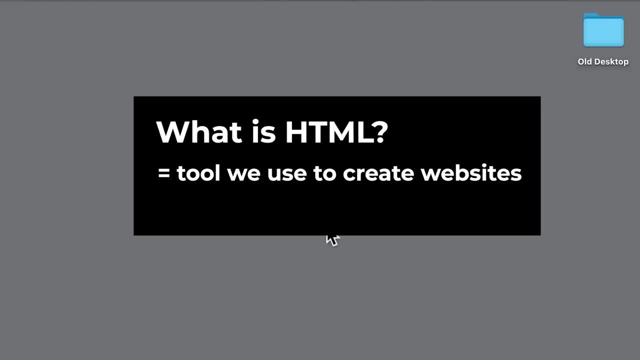 everything that we see on the website. The easiest way to understand what HTML is is that we're simply giving instructions to a computer. We're telling the computer what to do, step by step. The computer will then follow our instructions to create our website. 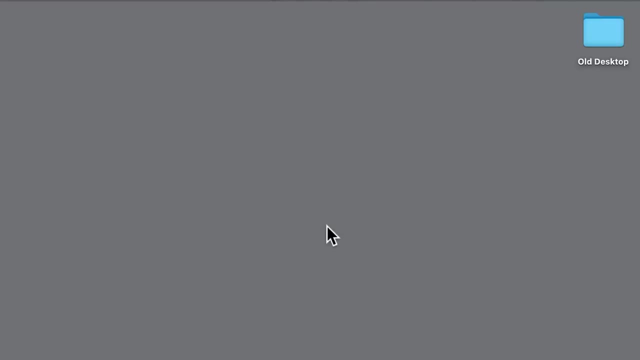 So I find the best way to learn HTML is to jump in and give it a try. So we're going to create our first HTML file and our first website. Let's go to our computer and we're going to create a new folder. 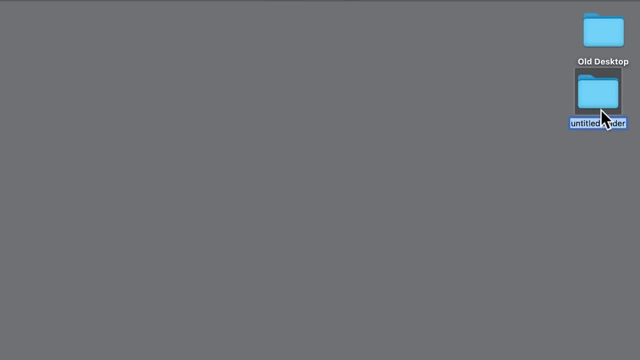 So this folder is going to contain all the code for this course. I'm going to call this HTML-STP. Next, we're going to open this folder in our code editor. So I'm going to open VSCode And then I'm going to click file open. 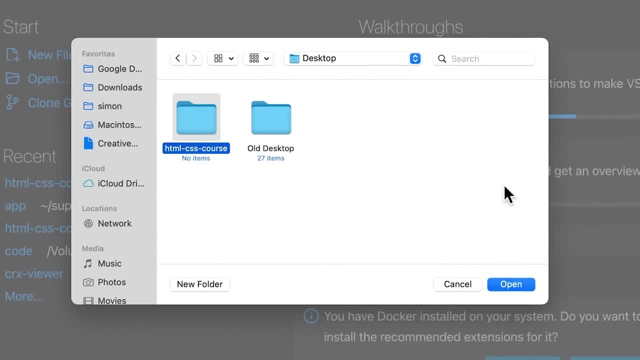 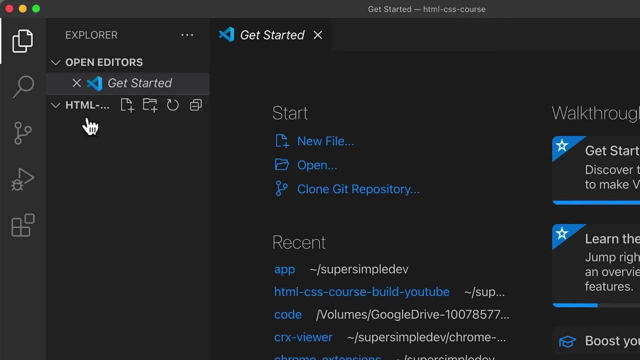 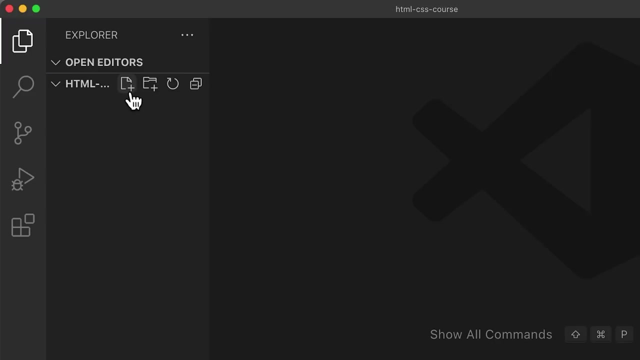 And I'm going to find the folder that we just created, which is this one. Now, once that's opened, you should see the folder name at the top here and on the side here. Now let's create our first HTML file. We're going to click this icon to create a new file. 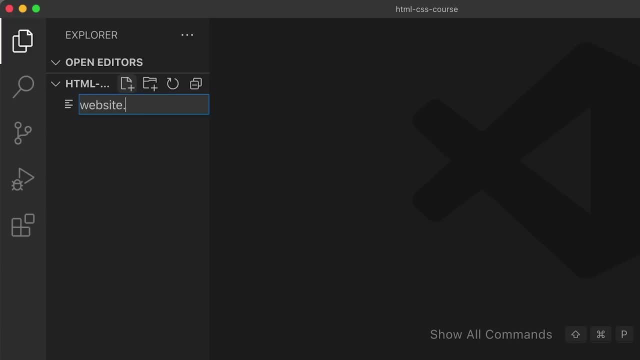 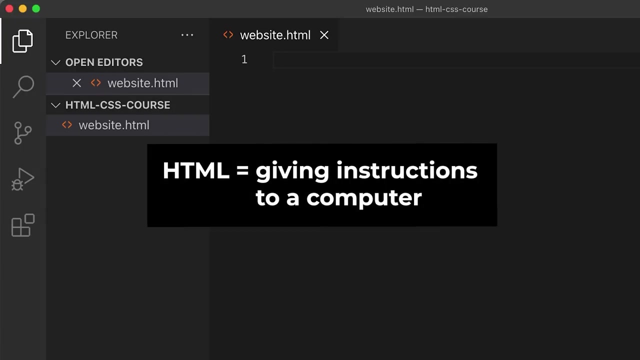 And we're going to call this file websitehtml, So we have to make sure that this file ends with html. This tells the computer that this file contains HTML code rather than just text. So, as I mentioned, HTML is basically some instructions you give to the computer. 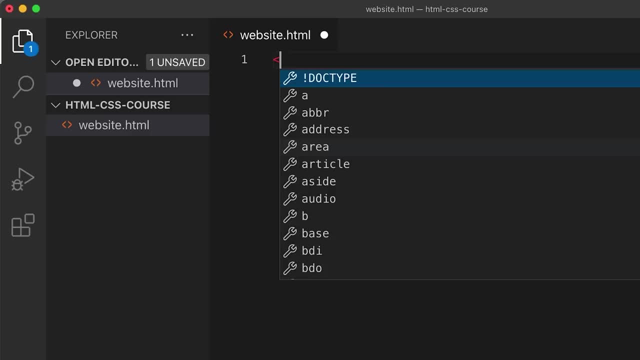 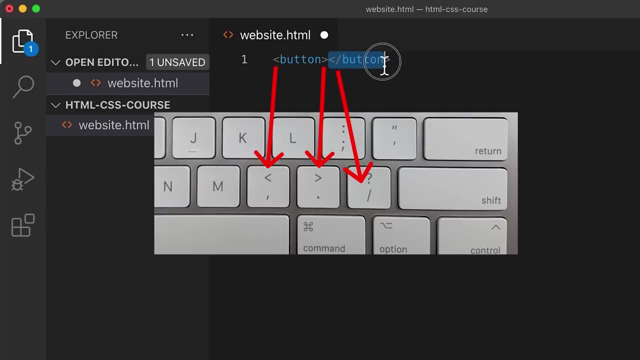 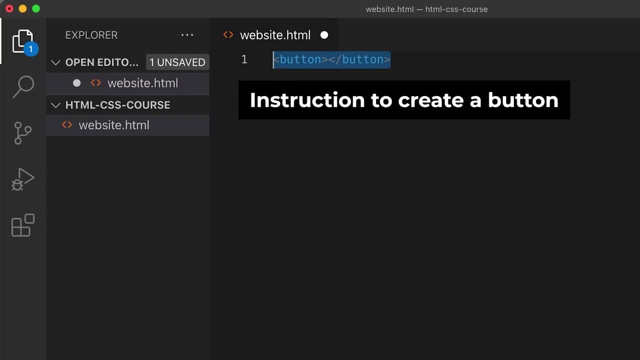 We're going to learn our first instruction: html. Now here's an example. So in a new folder we're going to create our website. That file is called html. Once we create our website, we're going to need to create a button inside the button. 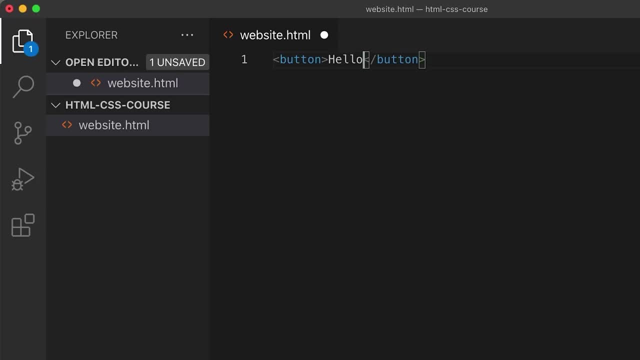 And inside this button we're going to have the text hello. Now let's save our file and we're going to learn how to open this in our web browser. To open our new website, we're going to go to the folder that contains our code and 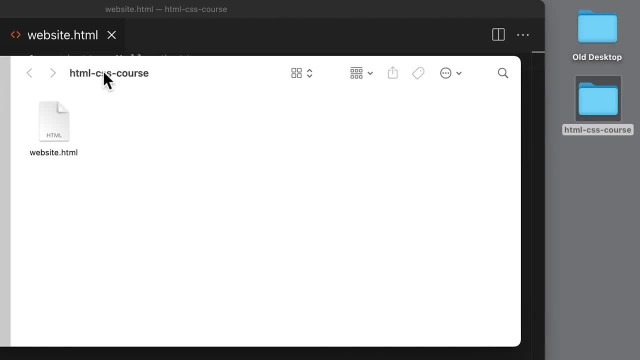 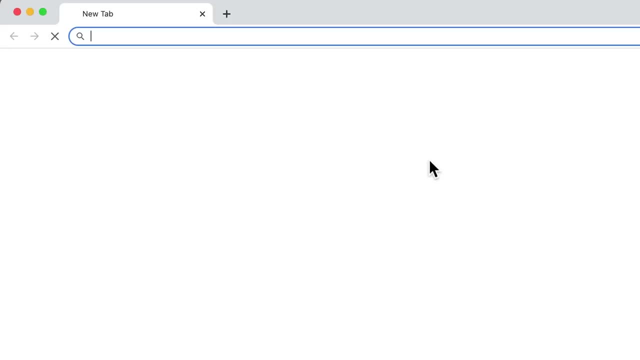 we're going to click this button. Click on this button code. we're going to find our HTML file. we're going to right click open with Google Chrome. Now you can see that we have our first website that has a button with the text hello inside. 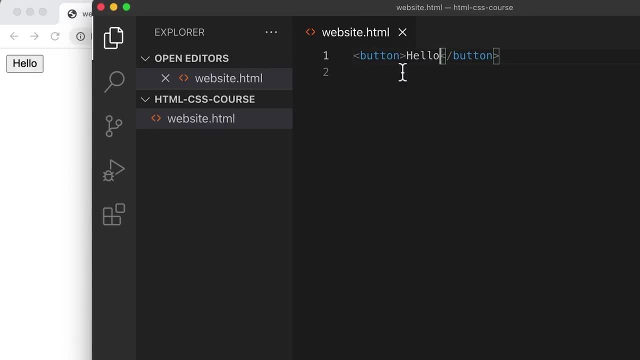 And if we look back to our code, that's exactly the instruction that we gave to the computer. So, as you can see, HTML is pretty straightforward. It's pretty easy to understand what's going on. Now let's try another instruction we can give to the computer. 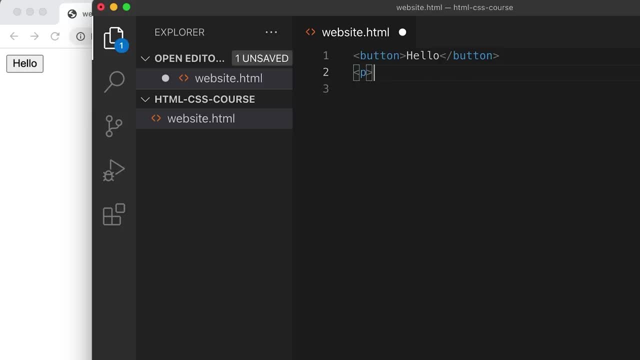 On a new line. we're going to type less than p greater than, And we also need to type less than slash, p greater than, And our code editor might autocomplete this for us too. So the p here stands for a paragraph. This is a paragraph of text. 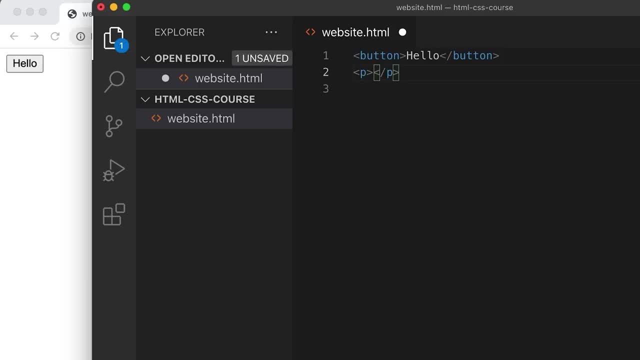 Inside a paragraph we can put some text, So let's put the text: paragraph of text. Now we can save this And to get our website To reflect our most current code, we're going to go to our webpage and refresh. 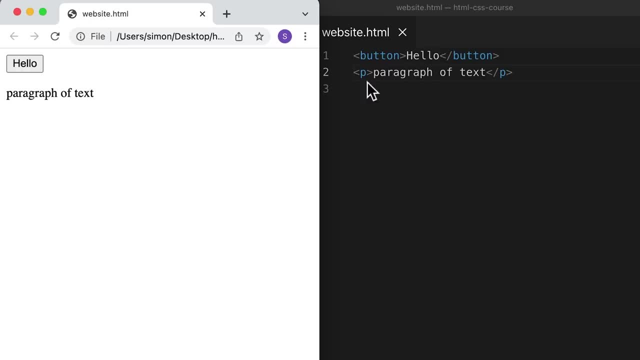 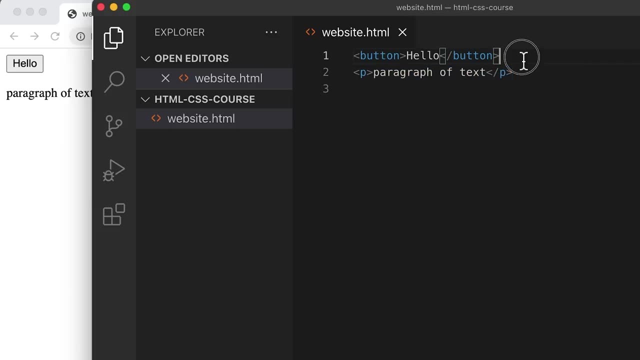 And now you can see that our website is displaying a paragraph of text, just like we told the computer to do. So that's basically how HTML works. The computer reads our HTML code from top to bottom and then follows those instructions and creates a button and a paragraph of text. 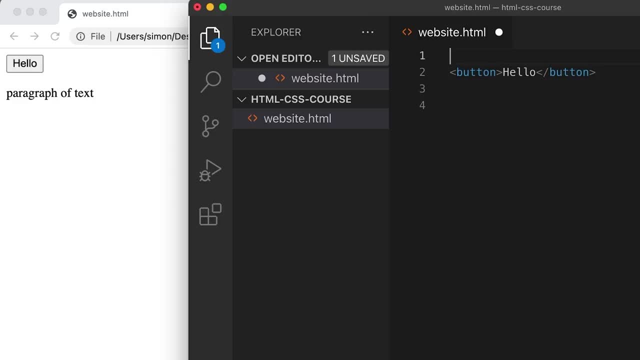 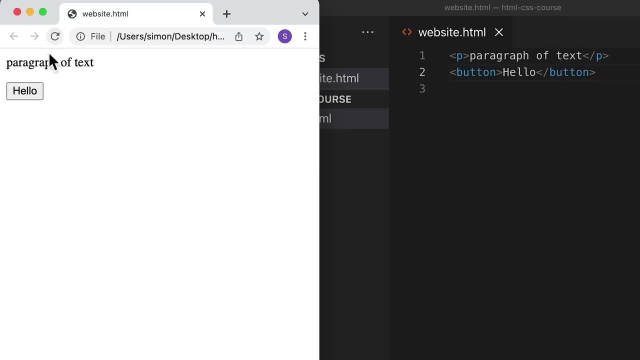 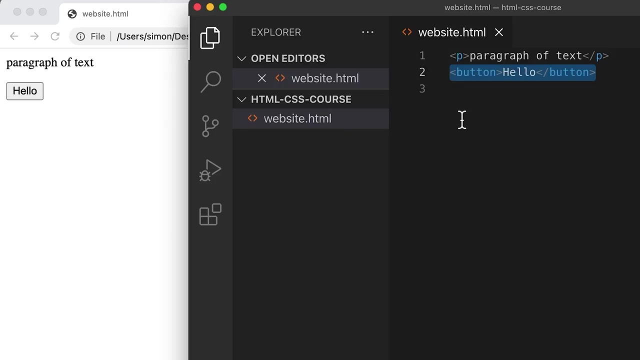 If we reverse the order of these lines, For example, if I put the paragraph up here And I save it and refresh the page, then the paragraph will appear on top Because, again, the computer is just following our instructions one by one. 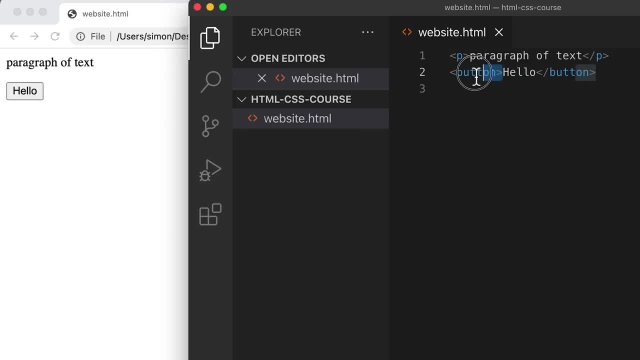 Now I'm going to introduce some terminology. So each of these things that we're displaying on the webpage is called an HTML element. So a button is a type of HTML element And a paragraph is another type of HTML element. So we're going to go ahead and do that. 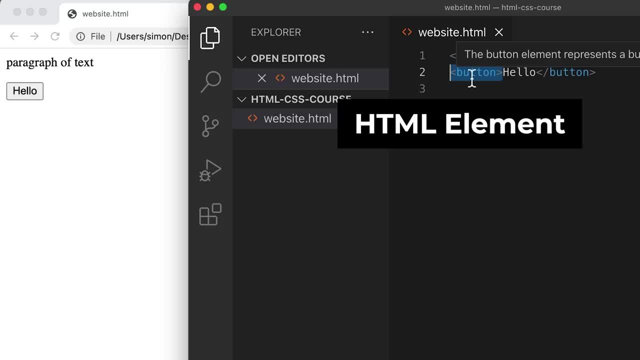 So we're going to go ahead and do that. So element is just a generic term that we use to describe anything that we can display on the webpage, And we're going to be using this term- element- throughout this course. So now I want to explain why we have to write all of these symbols. 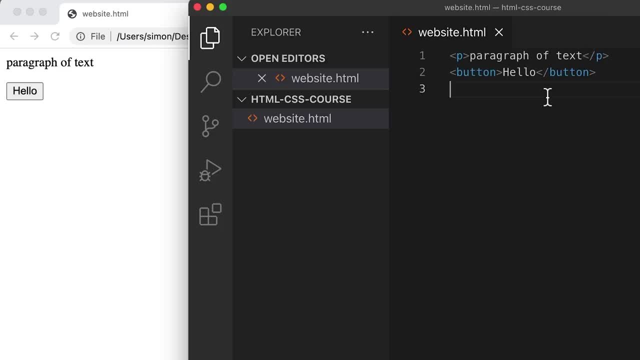 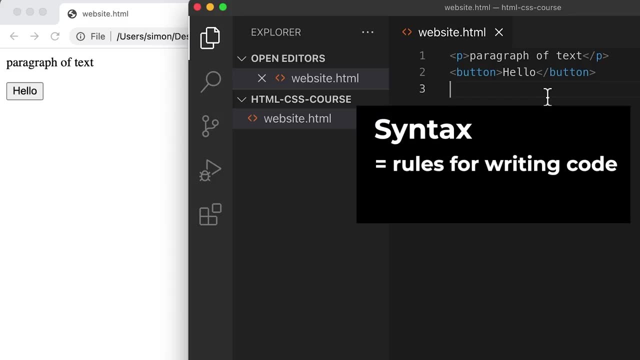 This less than this greater than and this less than slash. This is something called syntax. Syntax are the rules for how a coding language like HTML should be written. If you think of a language like English, we have something called grammar, which is the 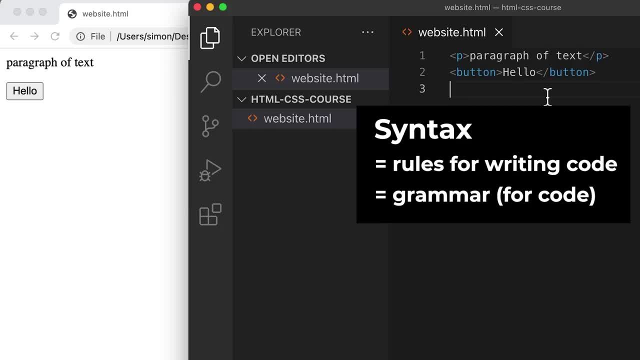 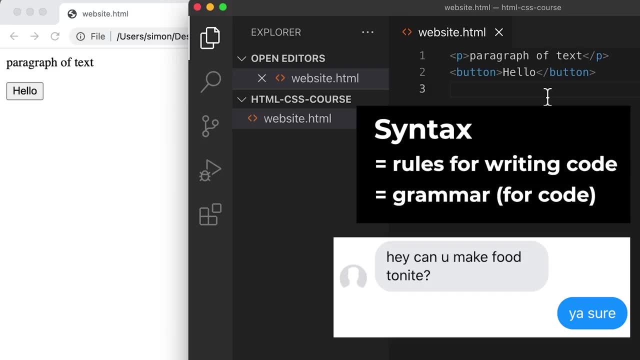 rules of the language. Syntax is basically the same thing, except for coding languages. Now, the biggest difference between a language like English and a coding language is that in English, you don't have to follow the rules of grammar perfectly. People can still understand you. 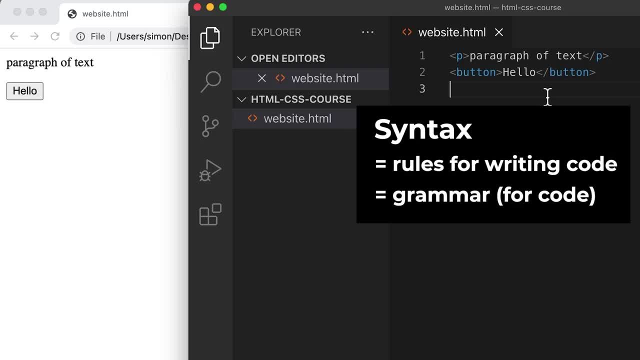 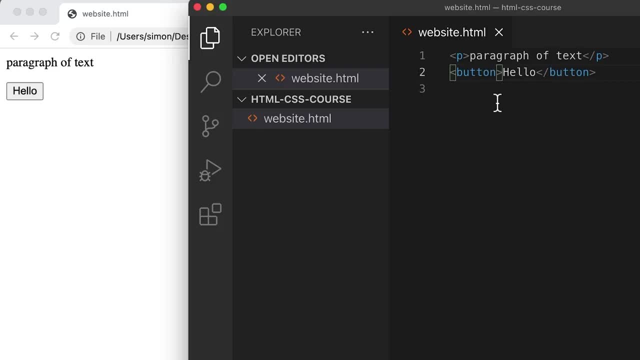 But in a coding language, if you don't follow the rules of syntax, the computer won't understand your code. For example, let's break the rules of syntax by deleting this greater than symbol, And now we're going to save our file. 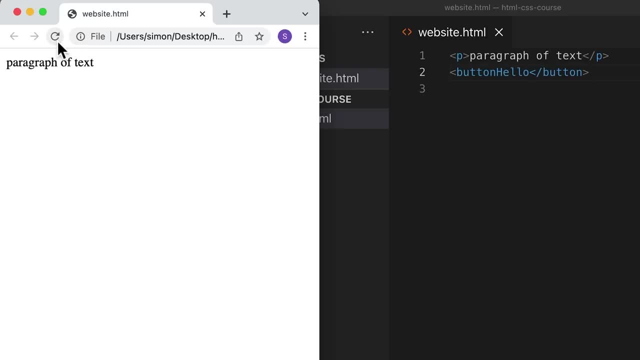 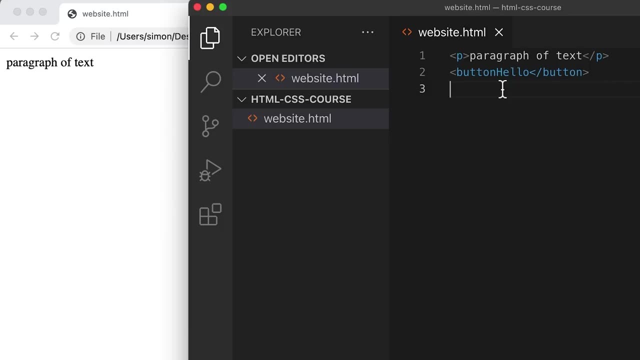 And we're going to go to our website and refresh, And now you'll notice that our button is gone, And that's because we're not following the proper syntax. so the computer doesn't understand our HTML code anymore. So let's put that greater sign back so that we're following the proper rules of syntax. 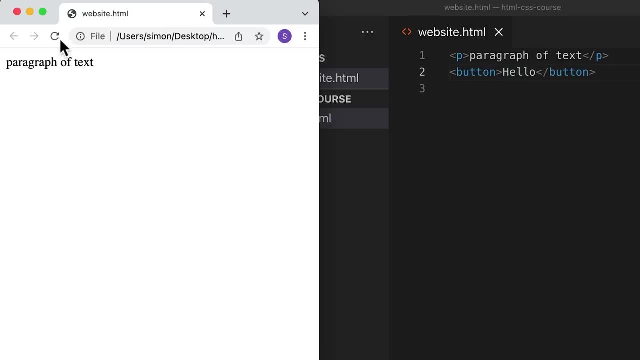 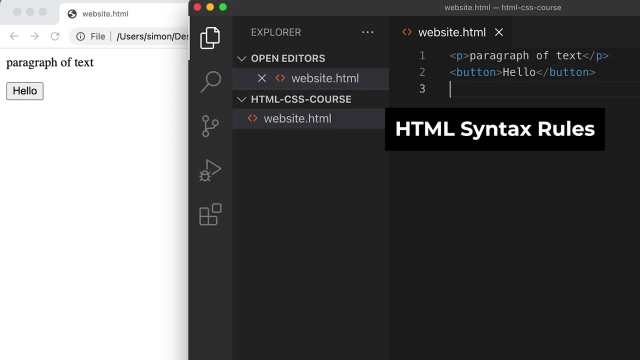 And we don't need this. So let's save and refresh our page. And now our button is back because we're following the rules of syntax. So what exactly are the syntax rules? Let's look at the syntax for HTML. So this part of the code is called an HTML tag. 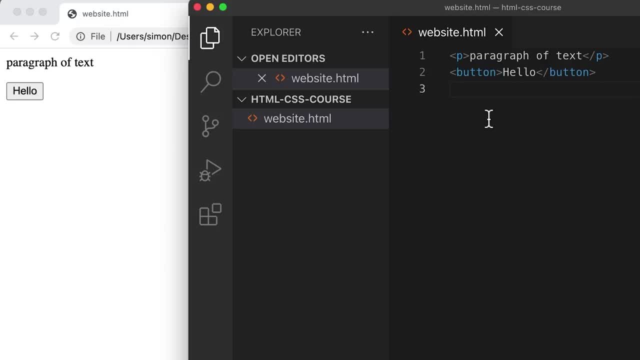 It basically tells the computer what we're trying to create. We write a tag by writing the less than symbol- This is the tag name, which tells the computer what kind of element we're trying to create- And then the greater than symbol. So every element consists of two tags: an opening tag and a closing tag. 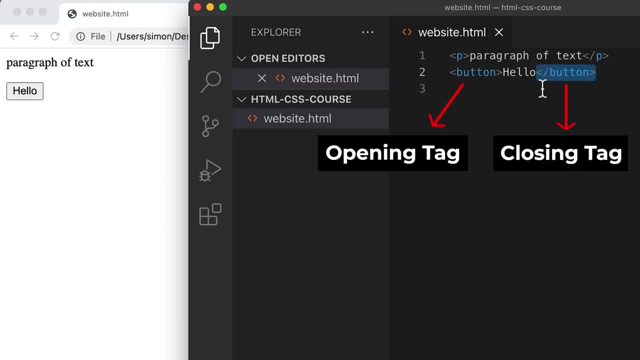 The closing tag is the same as the opening tag, except it has a slash in front of the tag name. That's how you can tell it is a closing tag. You can think of the opening tag as the start of the button and the closing tag as the. 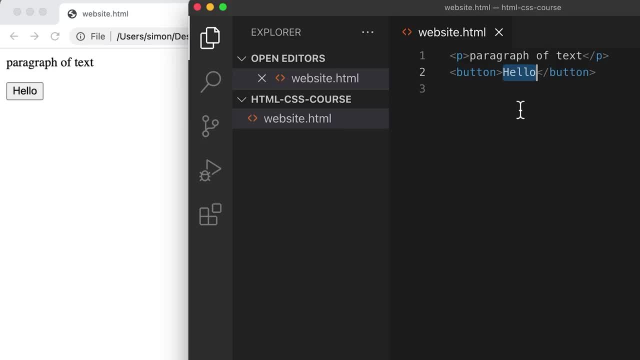 end of the button and then in between is the content or the text inside the button, And the same thing for the paragraph. The paragraph has an opening tag, a closing tag and some content inside the paragraph. So, as long as we follow these syntax rules for HTML, we have an opening tag and a closing. 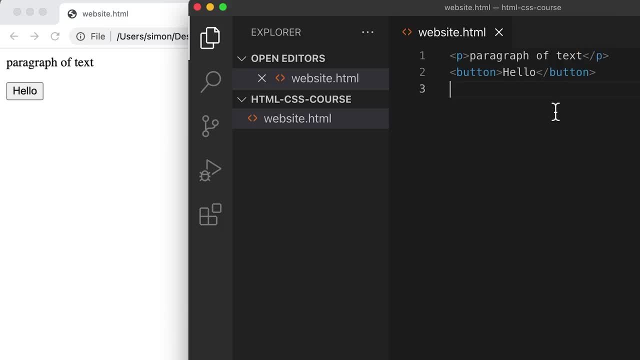 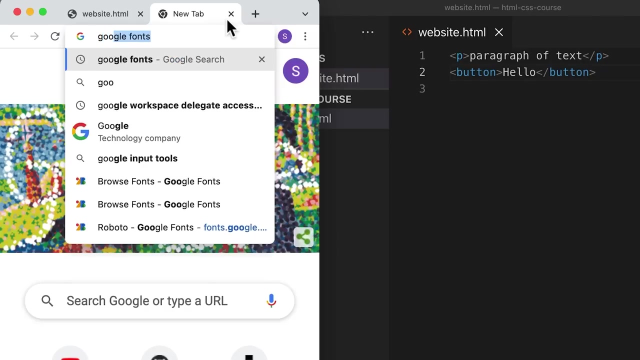 tag And the closing tag starts with a slash in front of the tag name. Then our computer will know what to do and display our elements on our web page. The next element that we're going to learn is a link to another website. For example, if we go to Google and we search for something on Google, it will give us a. 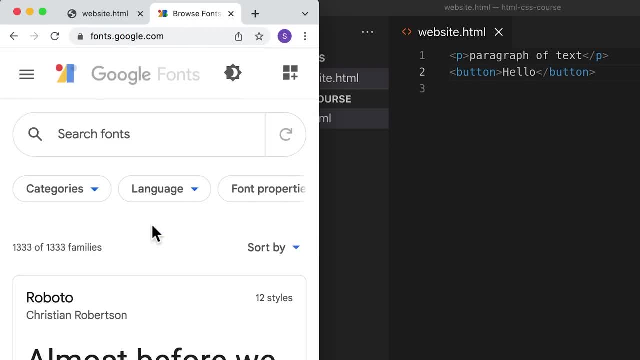 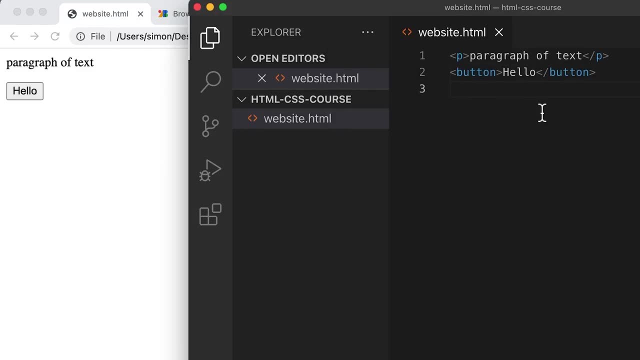 bunch of links And when we click these links it will take us to another website. So we're going to learn how to do that in our HTML code. So we'll go back to our website here And in our code we're going to type less than a greater than. 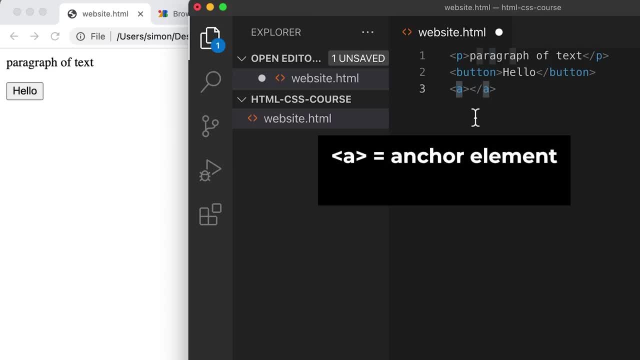 So this a here represents an anchor element. An anchor is basically a link to another website. So inside this anchor we're going to put the text of our link. So let's put the text as link to YouTube. We're going to save this and then refresh. 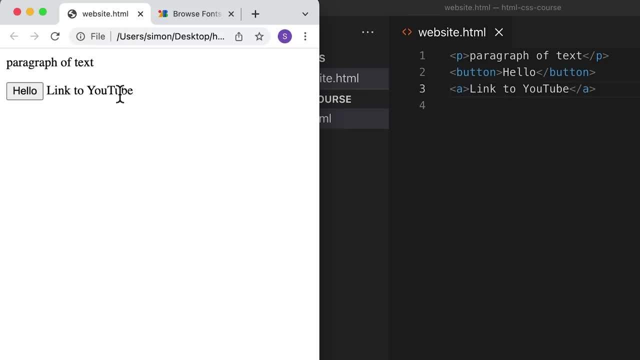 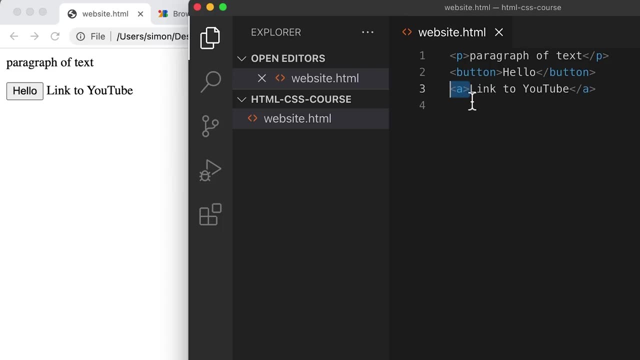 And now we have a link But It doesn't actually take us to YouTube, and that's because we haven't told the computer where this link is supposed to take us. Right now we just have a link without a destination. So to set a website to link to, we have to learn a little bit more HTML syntax. 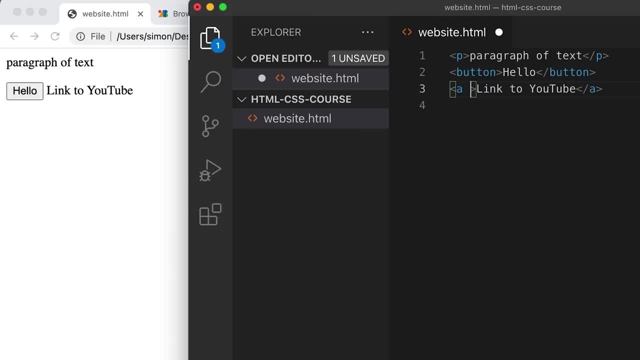 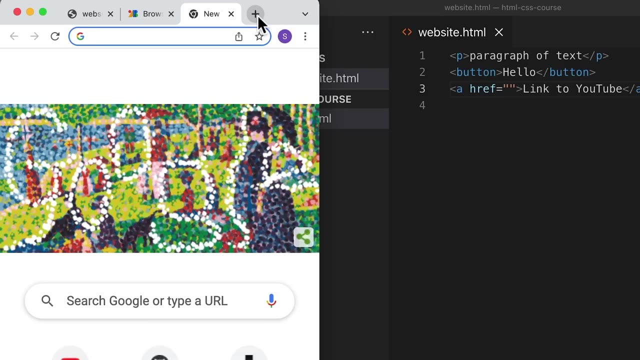 So we're going to go into the opening tag and we're going to type space: href equals double quotes, double quotes. So inside these quotes we're going to copy and paste YouTube's website URL. So to get that we can go to our web page and then type in youtubecom. 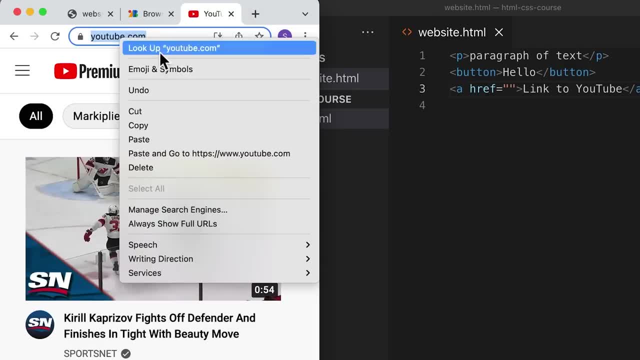 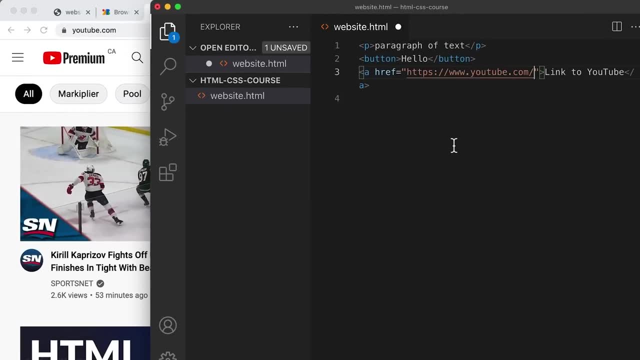 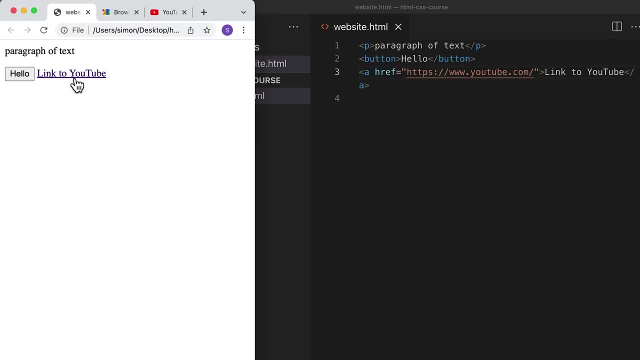 And at the top here we have the URL. So we're going to copy this and paste this into our quotes, And now we're going to save our file. We're going to go back to our website and refresh, And now we have a link that we can click. 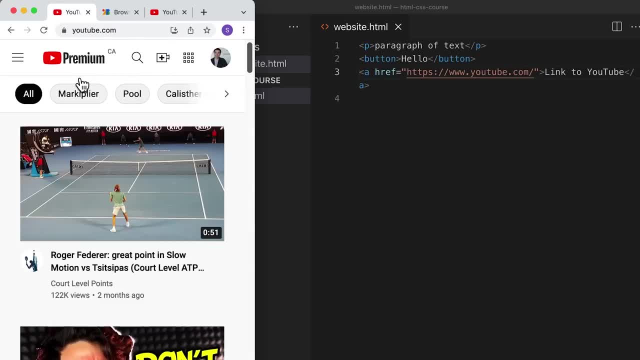 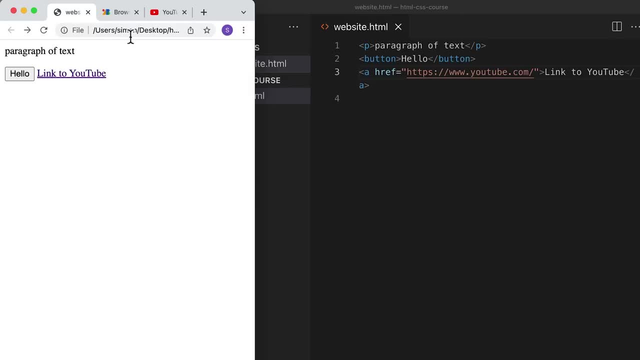 So when we click this link, it's now going to take us to YouTubecom. So that's how we create a link to another website with HTML. Now let's go back here and explain what this syntax means. So this is called an HTML attribute. 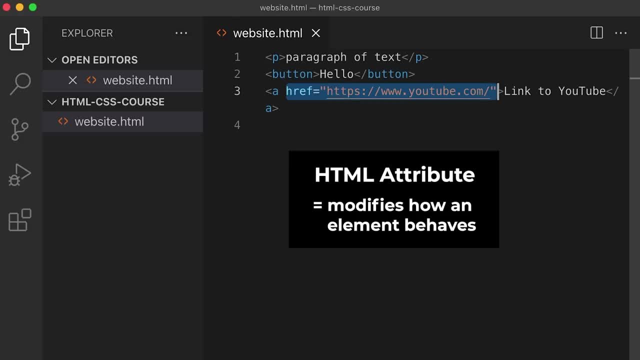 An attribute basically modifies how an element behaves. In this example, we're using the href attribute and it determines where this link element will take us when we click it. Right now it's going to youtubecom, but if we change this, it will take us to a different. 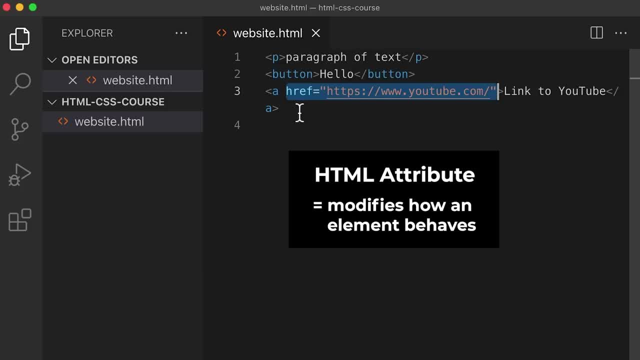 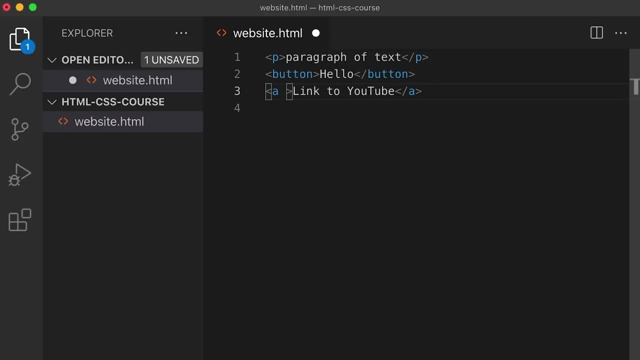 website. So this attribute is modifying how the link element behaves. So the syntax rules for an attribute are: we have to have a space between the attribute and the tag name. Otherwise if I write href here, the browser is just going to think that this whole thing. 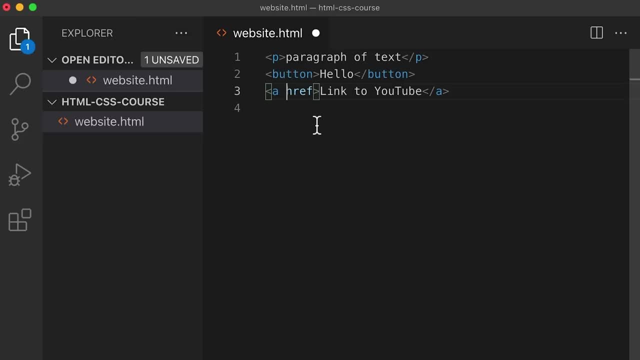 is a tag name, So that's why we have to have a space. So then we're going to have an equal sign and double quotes. So the text to the left of the equal sign is known as the attribute's name And on the right side is the value. 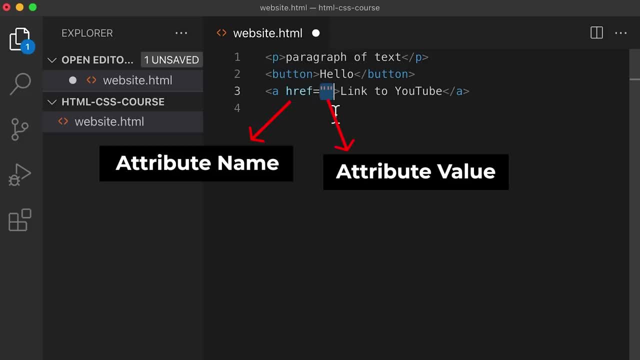 The value must be surrounded by double quotes, as you can see here. So you can kind of think of it like this: The name tells us what we're modifying. The value tells us what we are modifying it to. So the href tells us we're modifying the destination of this link and we're modifying it to youtubecom. 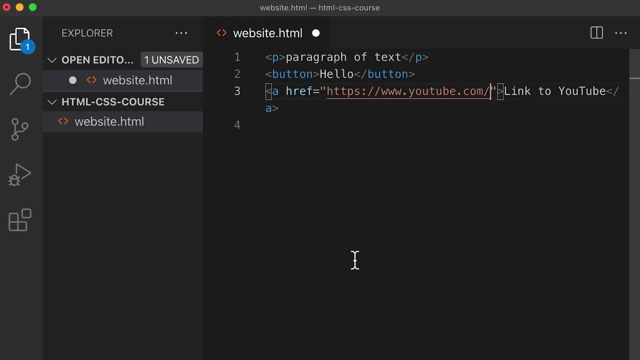 We can also have multiple attributes on an element. To add another attribute, we just separate it with a tag, Just a space like this. And now we're going to add another attribute to our link element, And this one is called target. 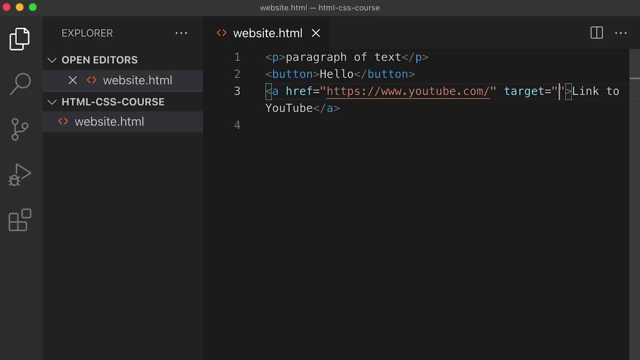 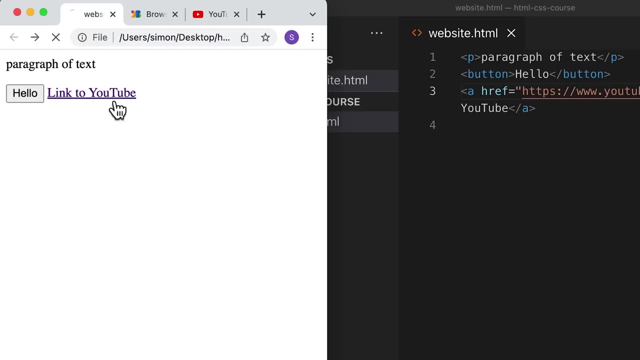 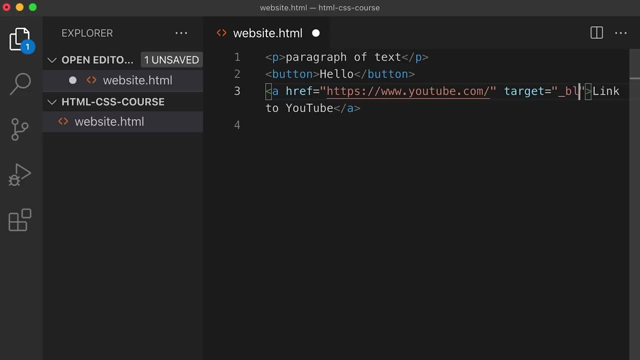 So the target attribute determines whether this link opens in the current page or in a new tab. So by default, if we don't have a target attribute, it opens in the current page like this. But if we set the target attribute to underscore blank, now this link element will open in a 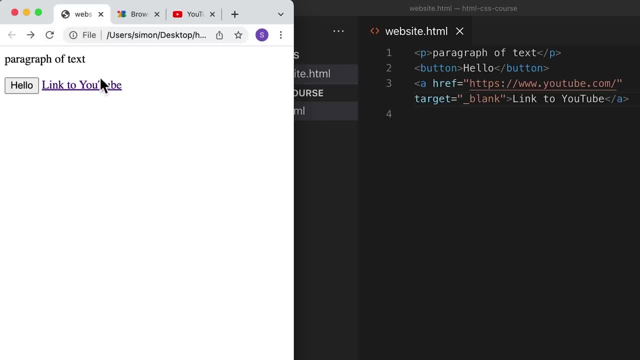 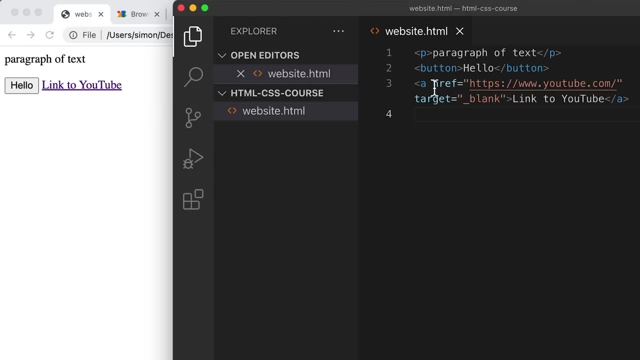 new tab. So let's go to our webpage and refresh And click this link. youtube will now open in a new tab. So by using attributes, we can modify different parts of this element's behavior. The href attribute modifies where this link goes and the target attribute modifies whether. 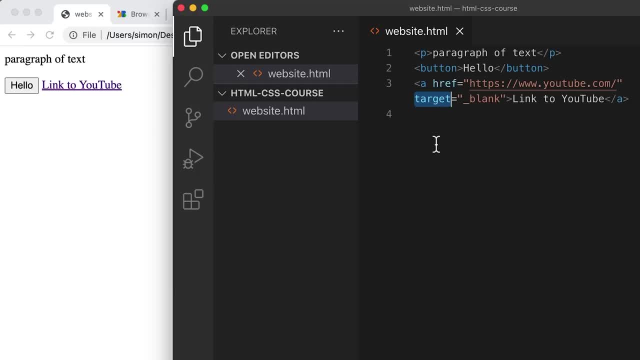 this link opens in a new tab or in the current page. Keep in mind that the href and target attribute only work on the link element. The button and the paragraph elements have their own set of attributes that we can modify and we're going to learn these later on in the course. 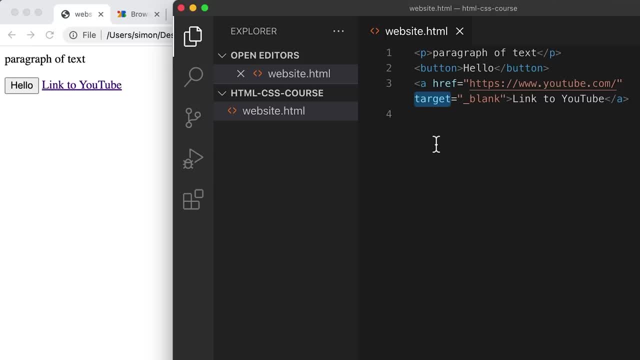 But for now, I just wanted to introduce you to the idea of using attributes to modify our HTML elements. The last thing we're going to learn in this lesson is some weird quirks of the HTML syntax. So something that a lot of beginners have trouble with is that in HTML, if you have 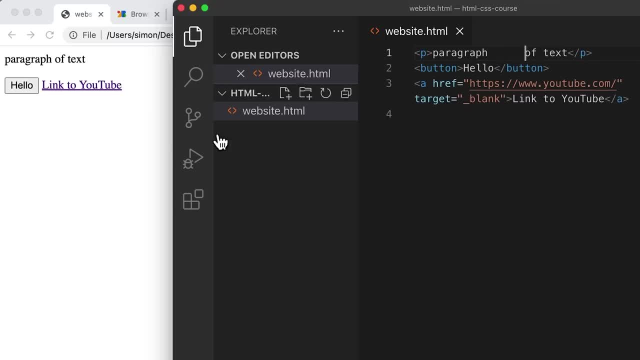 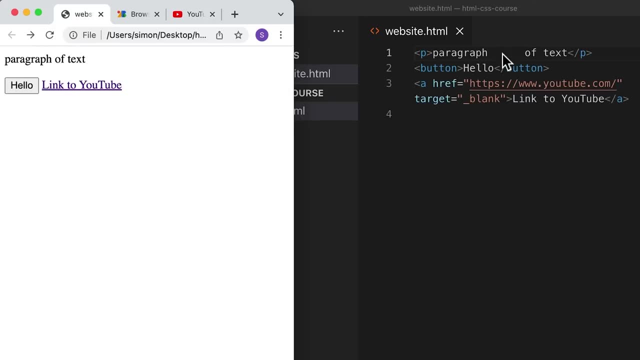 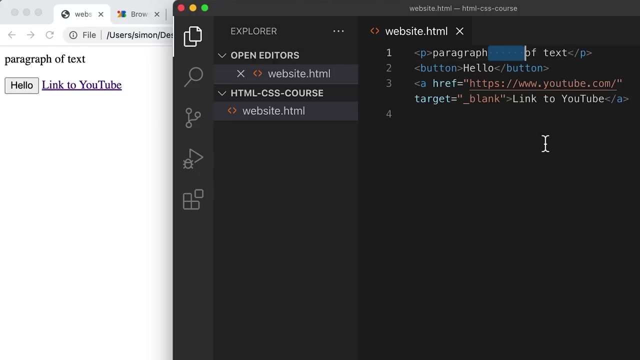 multiple spaces like this, For example: if we save this file And we reload, You'll notice that all of these spaces just appear as one space on the website, And that's because, according to the syntax, extra spaces are essentially ignored. So beginners usually have trouble with this because, for example, if they want to add space, 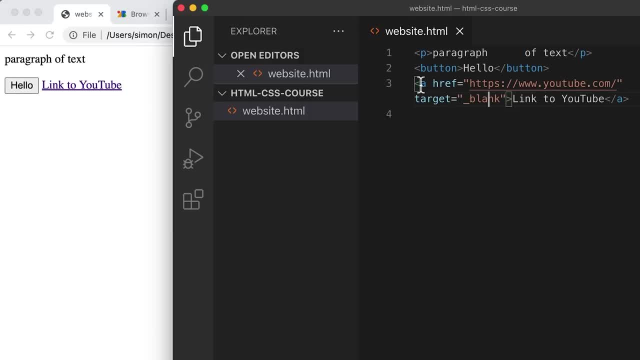 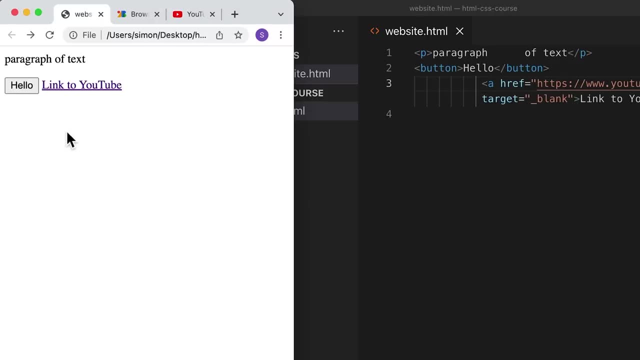 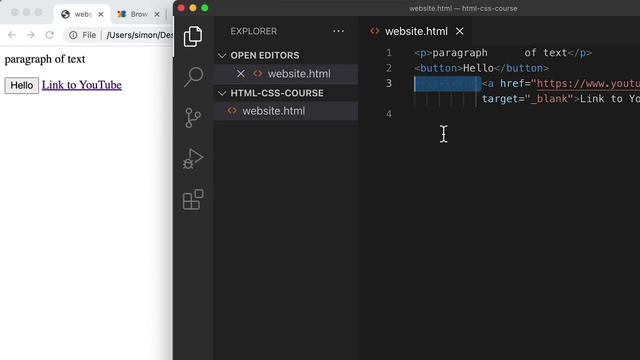 between this button and this link, they would start adding spaces in front of the link, thinking that it will move it away from the button. So if we save this and we refresh, nothing happens, And that's because all of these spaces are essentially ignored in HTML. 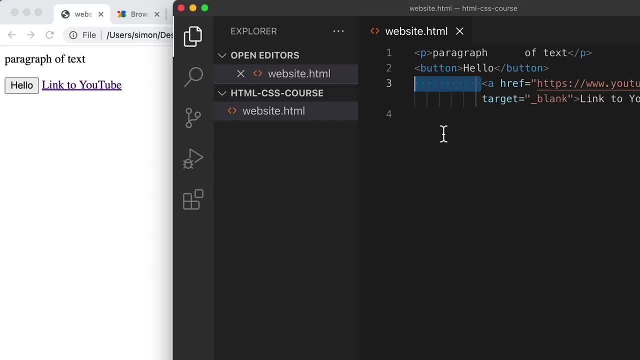 So later in the course we're going to learn how to deal with these situations, But for now just keep this in mind. So let's get rid of these extra spaces for now. And another weird quirk of this syntax rule is that if I put my cursor here and I press, 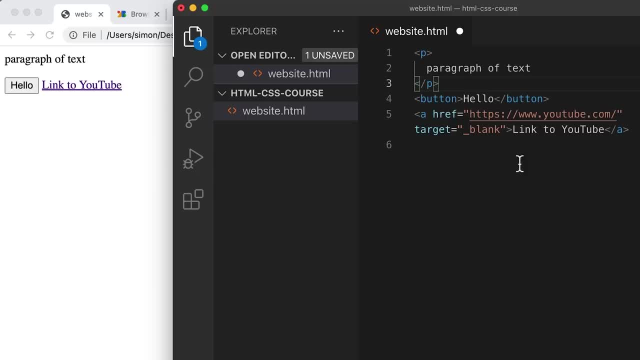 enter to create a new line and I put my cursor here again. these new lines also count as spaces, So the browser essentially ignores them. If I save the file and reload, you'll see that the new line doesn't do anything. So this actually makes organizing our HTML code very flexible. 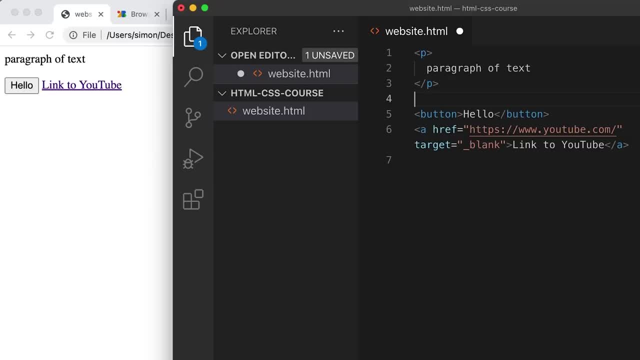 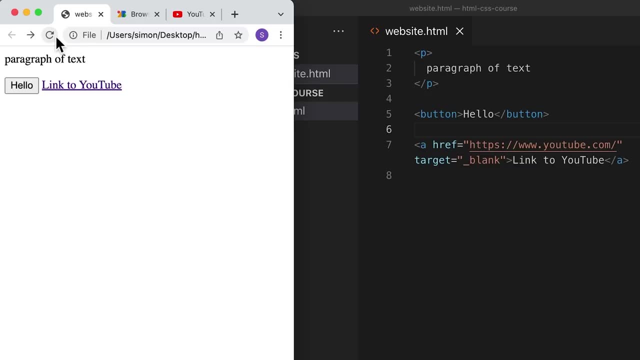 For example, if I wanted some more space between these elements so that it's easier to read in my code I can just add as much spaces as I want, and it won't get reflected in the website, because extra spaces like these new lines are just ignored. 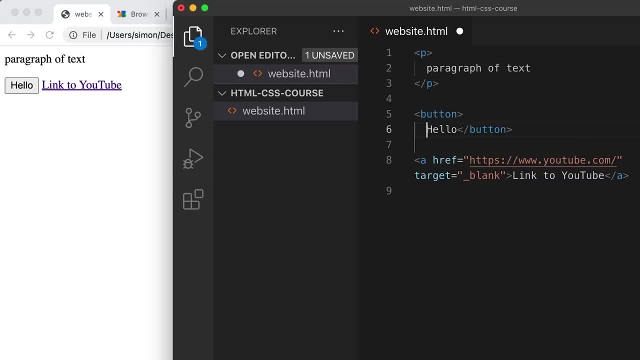 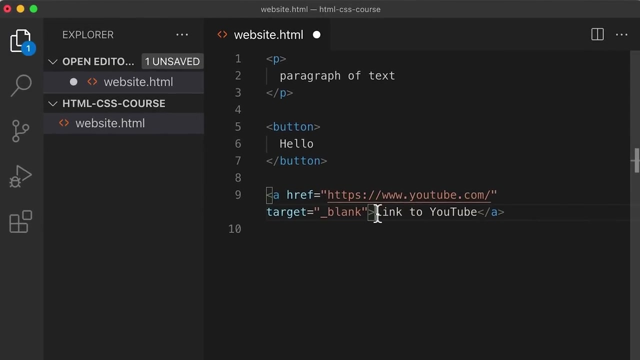 A lot of people like to put the content of the element on its own line like this, so that the tags basically align with each other in the same column And same thing. for here. You'll notice that this line is really long. We can actually add new lines here to make our code easier to read. 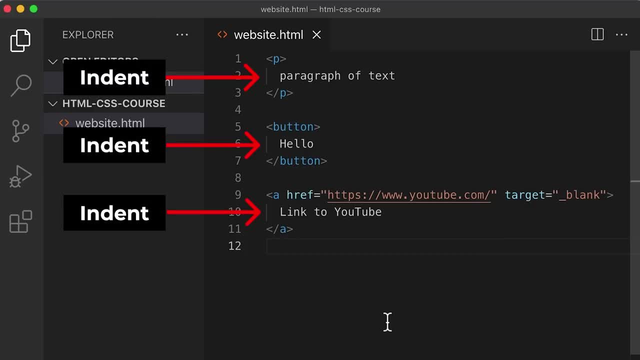 So when we organize our code like this, we generally indent or add spaces in front of these lines. This helps us clearly tell the difference, So let's go ahead and do that. If we didn't have this indenting, then it's pretty hard to tell where this element starts. 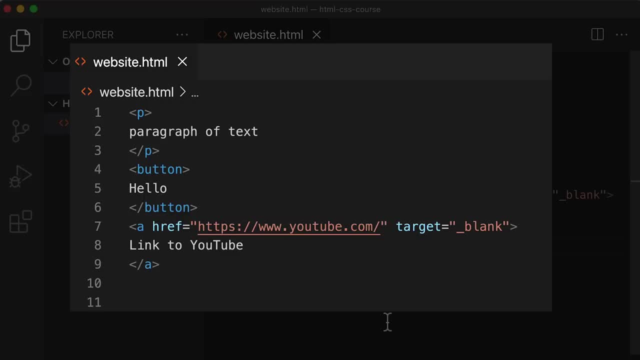 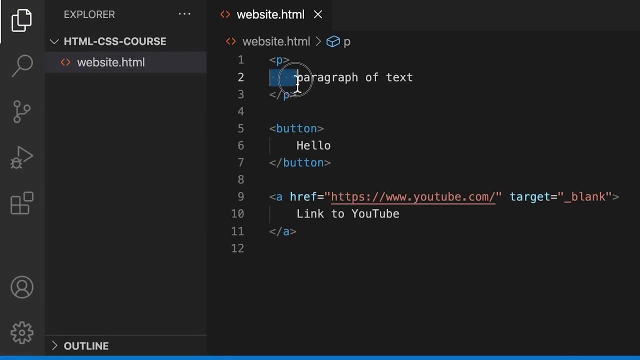 and where it ends, especially when we have a lot of code. Now your indents might look a little different from mine. It might look something like this: where you have more spaces than I do, This happens because, by default, VS Code uses 4 spaces per indent. 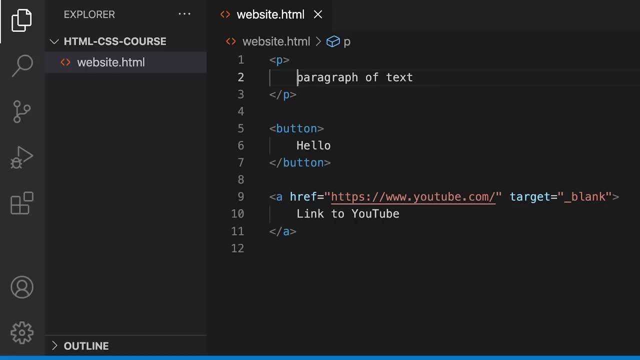 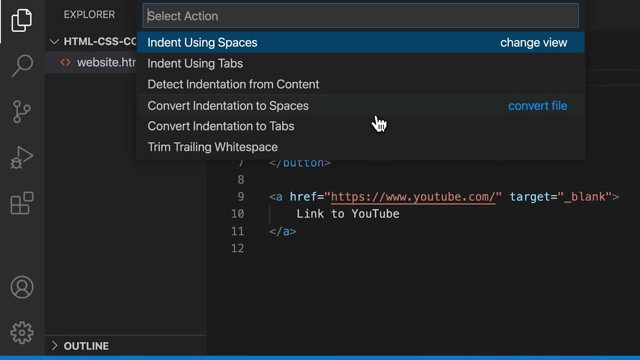 Generally in HTML and CSS, we use 2 spaces per indent. To update this, we're going to go down to this bottom toolbar and click this section And then we're going to click indent using spaces and we'll change this from 4 to 2.. 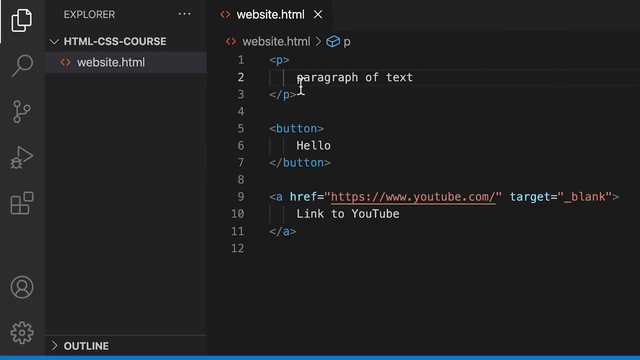 So now this file is going to use 2 spaces per indent, So we can get rid of this and press tab to have proper indenting. Now that only affects it for the current file. we can change it for every file going forward by going to the bottom left here. 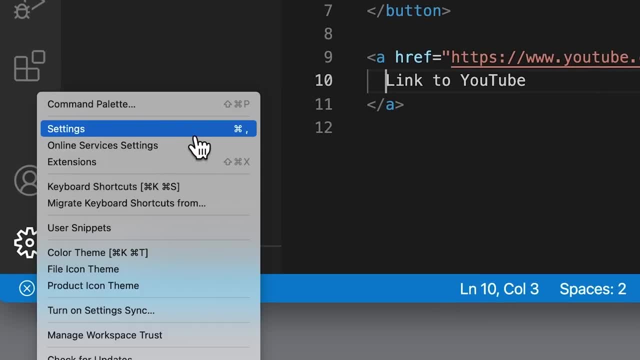 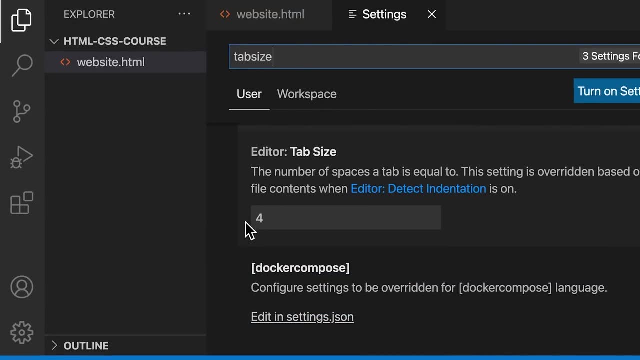 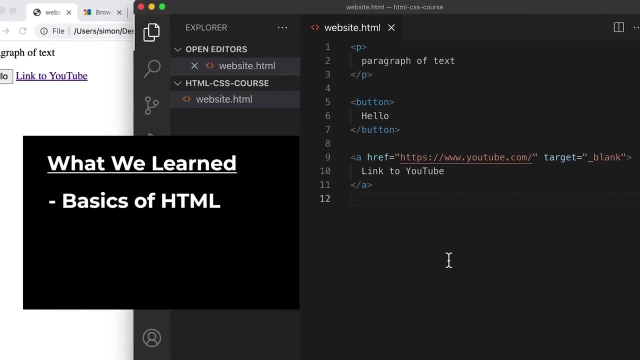 And clicking this icon and then going into settings, And in here we're going to search for tab size and we're going to scroll down and we'll change the tab size from 4 to 2.. Alright, so we just learned the basics of HTML: how to write HTML code and then turn. 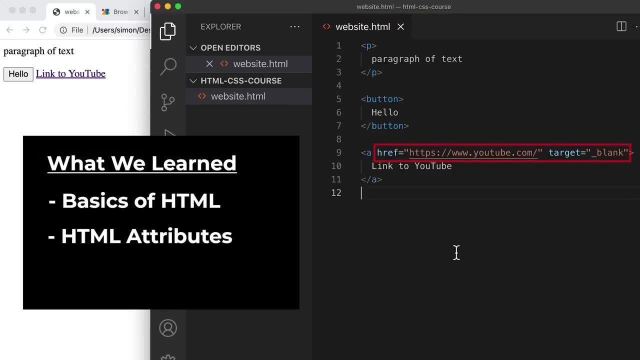 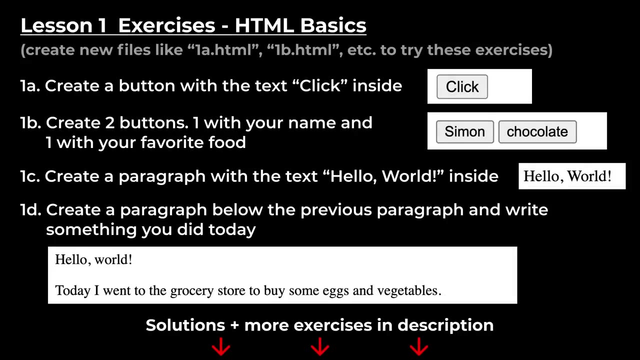 that into a website. We also learned how to write HTML attributes which modify the behavior of an element, And we learned about syntax, which are the rules that we have to follow when writing our code. Here are some exercises that you can try on your own to practice what we learned in this. 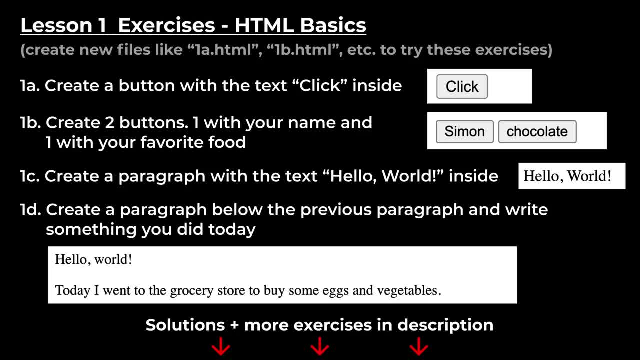 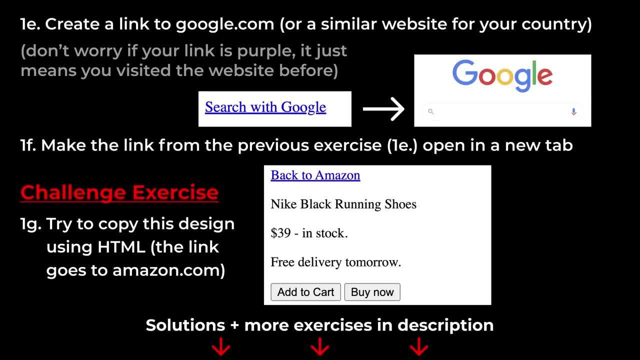 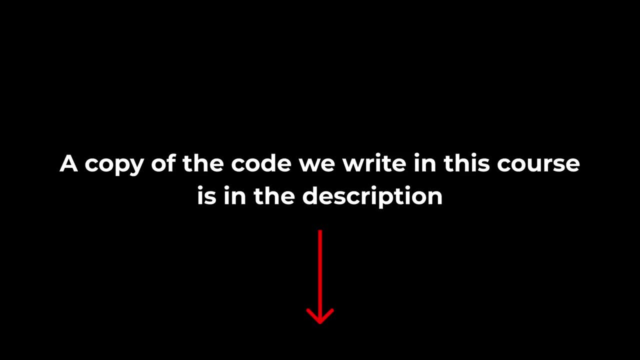 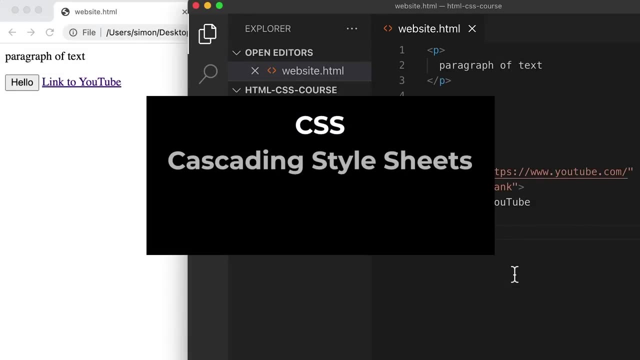 lesson. Feel free to pause the video here if you need to. You can find these solutions, as well as more exercises, on my website, supersimpledev. the link is below the video. In this lesson, we're going to learn CSS, or cascading style sheets. 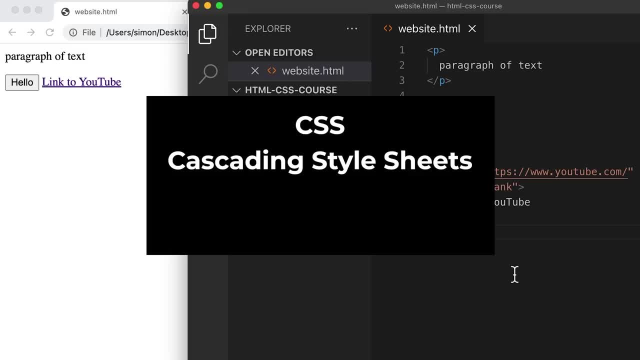 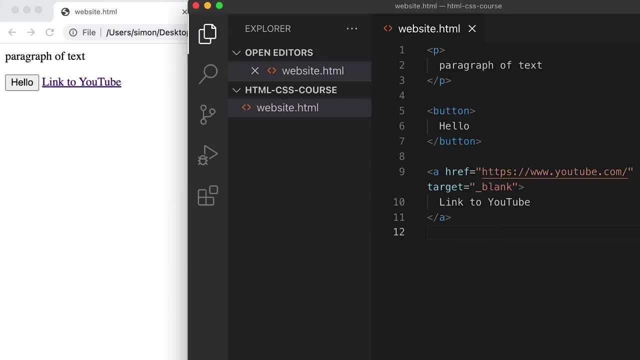 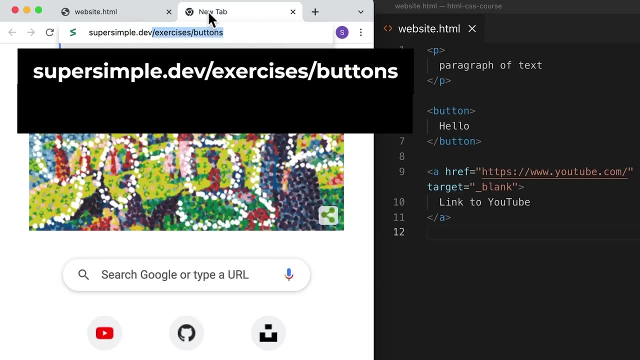 Based on the name. it's used to style our webpage, So it's used to change the appearance of our HTML elements. So I've actually prepared a project that we can do in this lesson. So we're going to open this project by going to supersimpledev: slash exercises- slash. 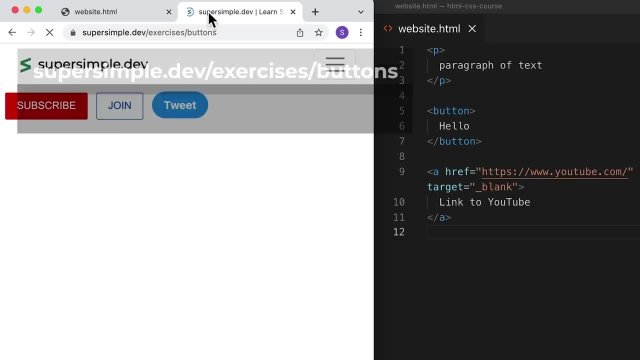 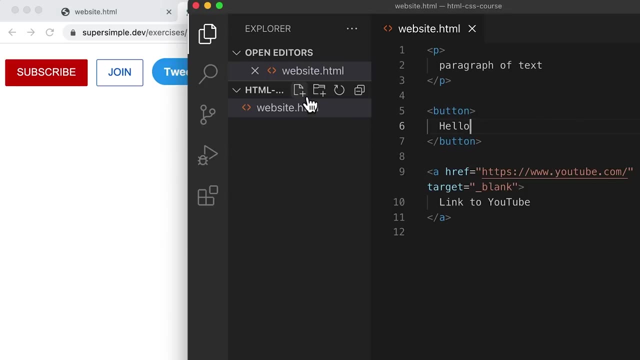 buttons. So on this webpage I have some really nice looking buttons from famous websites, namely YouTube and Twitter, that we can copy and practice our CSS with. So we're going to go into our code and we're actually going to create a new file for this. 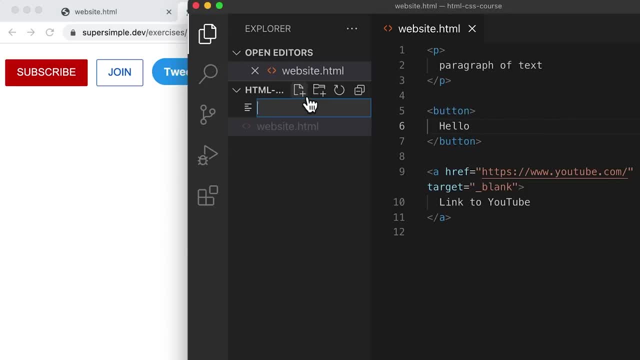 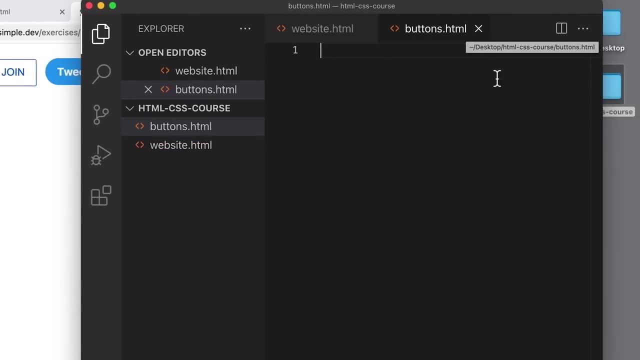 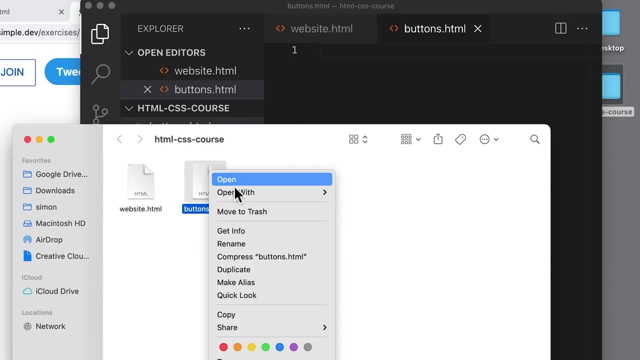 exercise. So let's create a new file and let's call it buttonshtml, And we're going to open our new HTML file. So let's open the folder that contains our code. we're going to right click open with Google Chrome. 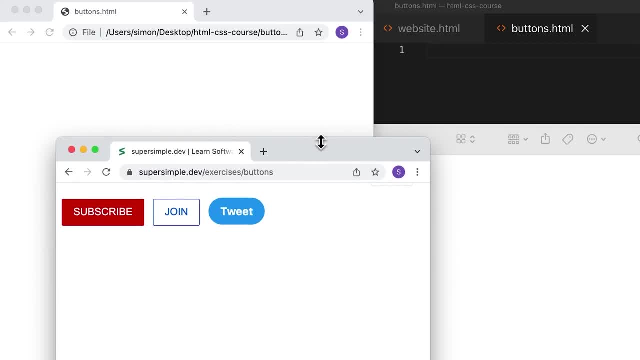 And now I'm going to set this up by moving our reference design to the bottom like this, so that it's easier for us to copy it with CSS. I'm just going to move that to the corner and then we can work here. 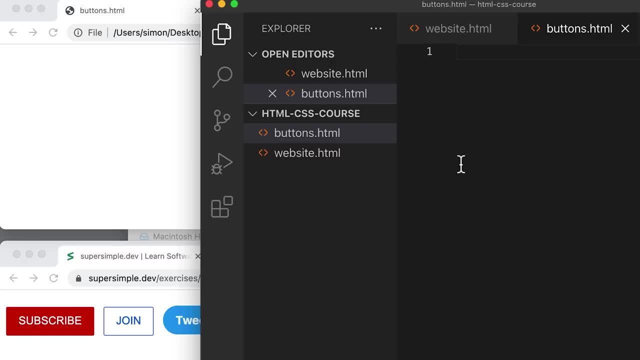 So first let's work on creating the software. So we're going to create a button using HTML. So, just like we learned before, we're going to create a button using HTML. So less than button, greater than, And then inside our button we're going to have the text subscribe. 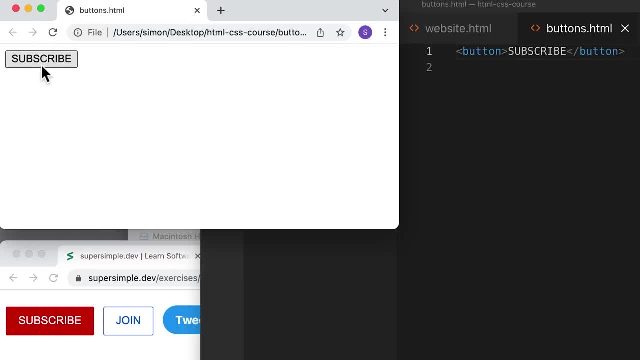 And now let's save and refresh our page And now we have our button. Next, we're going to start changing the appearance of this button so that it looks like the subscribe button from YouTube. Let's go into our code and we're going to start writing some CSS to change the appearance. 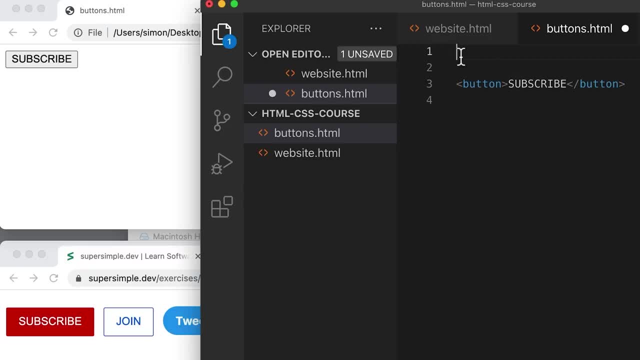 of this HTML element. So to write CSS we have to create a new element called a style element. So this style element is unique in that it doesn't appear visibly on the page. So, for example, if we save our file and then we reload the page, the style element doesn't. 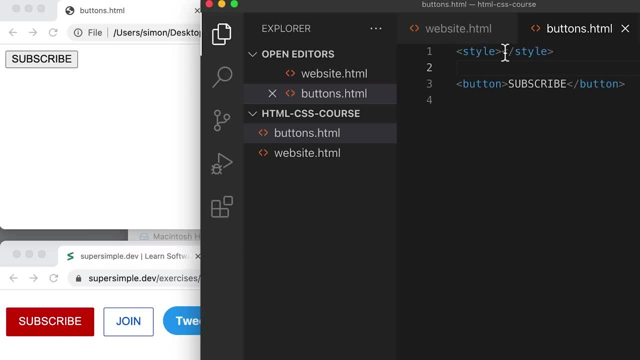 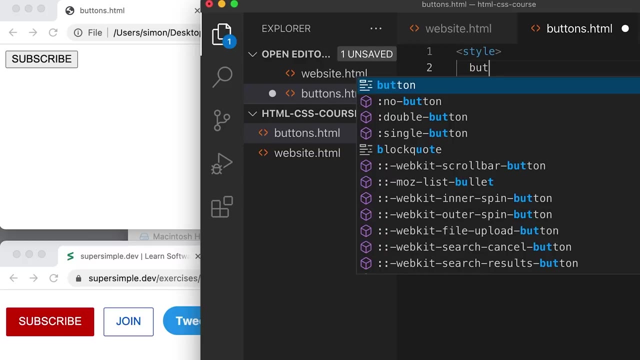 actually create anything. So the purpose of this element is that inside this element, we can write CSS code which modifies the appearance of other elements. For example, let's write our first bit of CSS code. We're going to type button: open- squiggly bracket. close squiggly bracket. 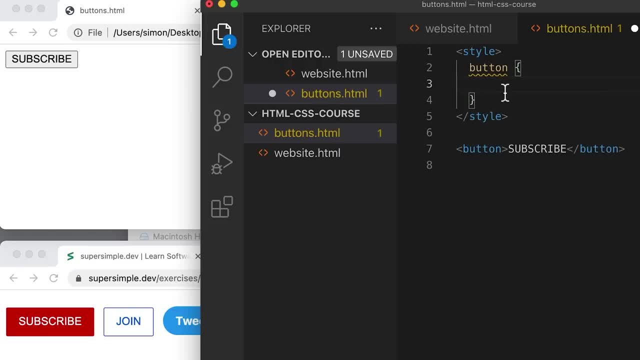 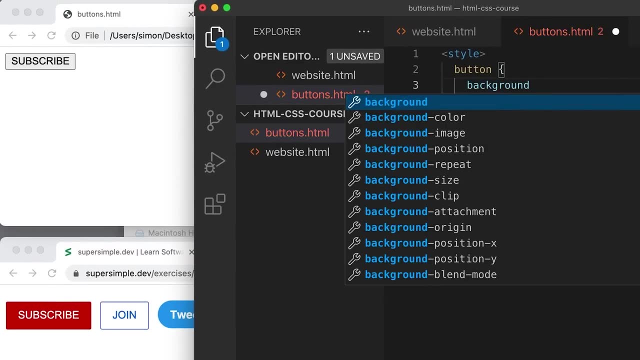 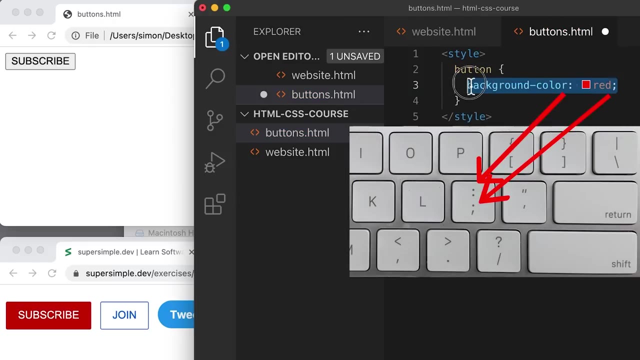 And then, inside these brackets, we're basically going to give instructions to the computer on how to modify the appearance. For example, Let's set the background dash color, colon, red and semicolon. So make sure that you write this out exactly as I have it here, so that we're following. 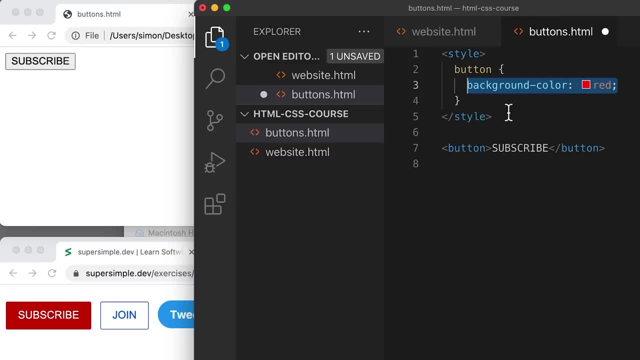 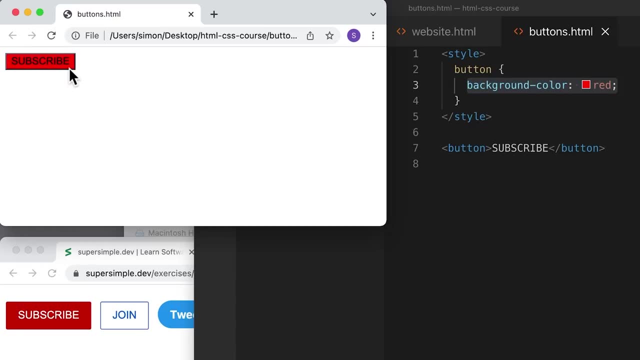 the syntax rules for CSS. Let's save this file and refresh our page, And now you can see that we set the background color of the button to red. So, as you can see, CSS is similar to HTML. We're simply giving instructions to the computer. 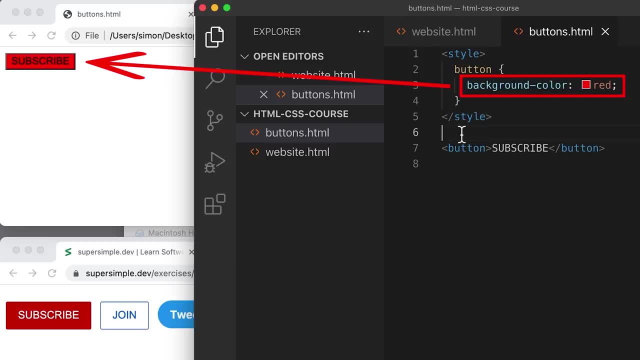 And then the computer follows our instructions step by step. And just like HTML, we have to follow certain syntax rules when writing our CSS so that the computer understands our code. So what are the syntax rules for CSS? How does this code work? 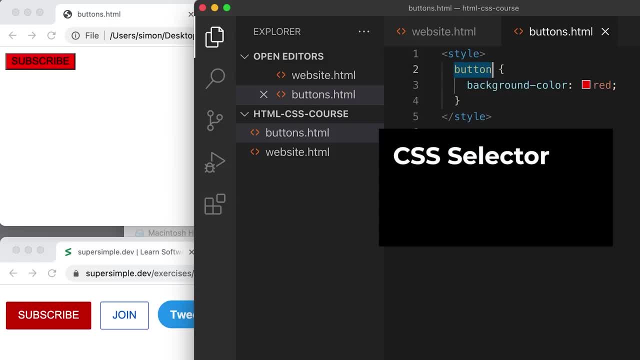 So the word at the front here is called a CSS selector. It tells the computer which elements on the page we are targeting with our CSS code. In this case We are targeting All buttons on the page and we're going to change the background color of all buttons. 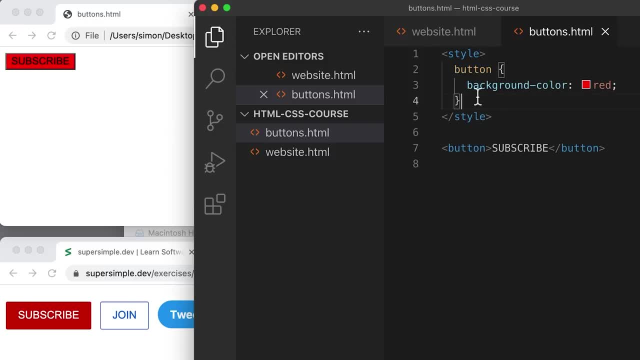 on the page to red. Now, inside these brackets, there are other rules that we have to follow. The text to the left of this colon is called the CSS property. It tells the computer what we are changing. To the right of the colon is the CSS value. 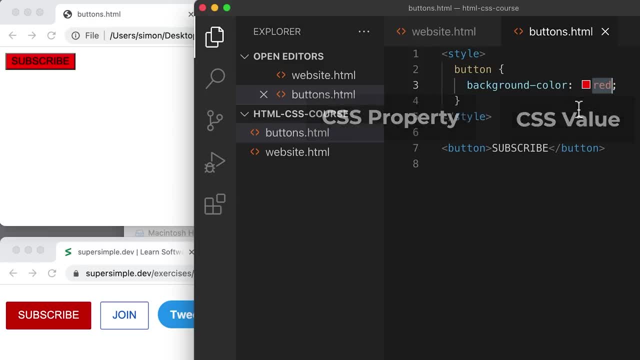 It tells the computer what we're changing the property to. In this case We're changing the property From background color to red, And that's exactly what the computer did. The colon is here to just separate the property and the value, And the semicolon here is just like a period in English. 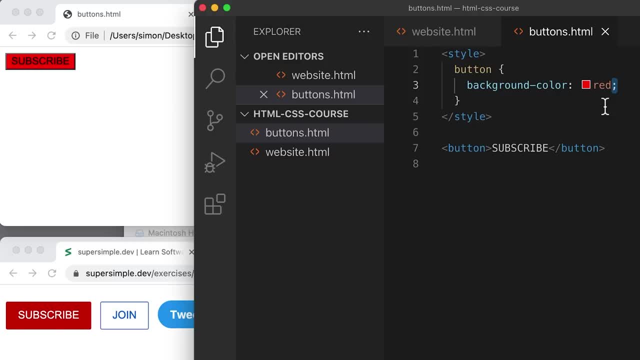 In English, you end sentences with a period. In CSS, you end a style with a semicolon. So that's what all of this syntax means. So we can actually add multiple styles inside these brackets. So let's go ahead and add another style. 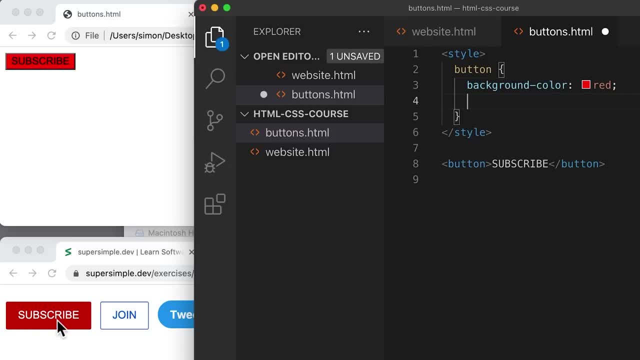 We're going to change the text color to white to match this design. So the property for changing the text color is called color. So notice that it's not called text color. it's just something that we have to remember. We're going to change it to white. 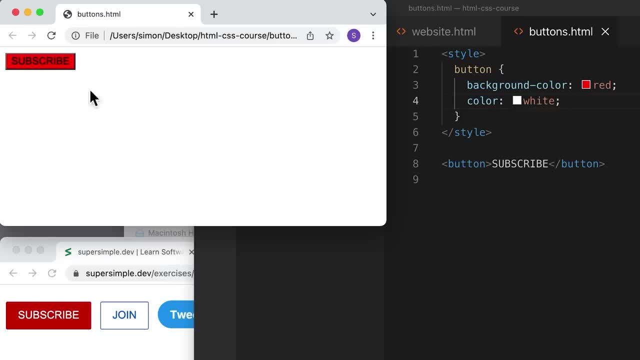 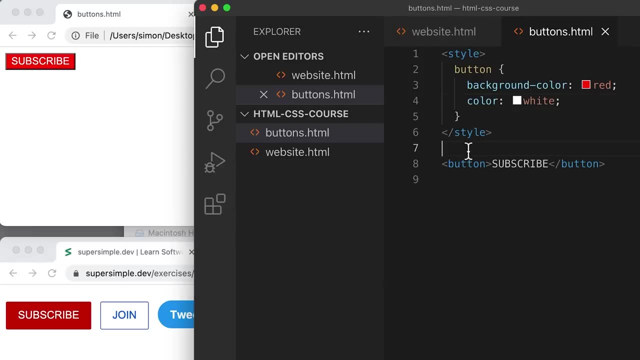 And we'll end it with a semicolon. Let's save and refresh, And now you can see that we changed the text color of this button to white, And that's basically how CSS works. We tell the computer that we want to change the text color to white. 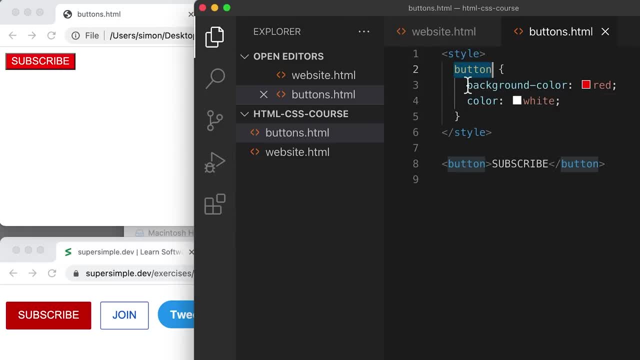 And that's basically how CSS works. We tell the computer what we're targeting And then we give some styles And the computer is going to apply these styles one by one. So let's do another example. This time we'll set the border property. 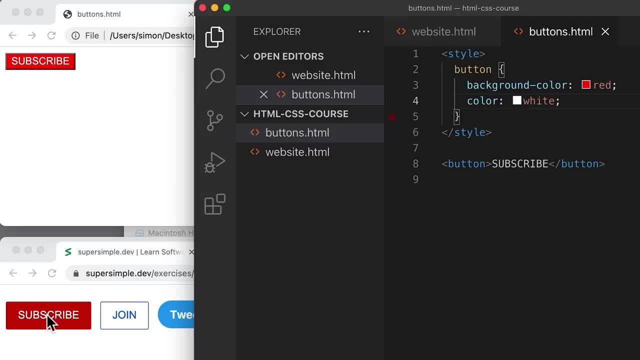 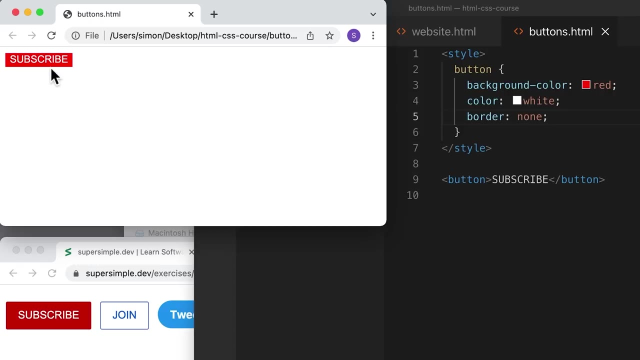 So notice that our button has a border, while the subscribe button here doesn't have a border. So we're going to set the border property colon to none, We're going to save this file and refresh, And now we just remove the border. So if you look at our styles here, it's actually pretty straightforward. 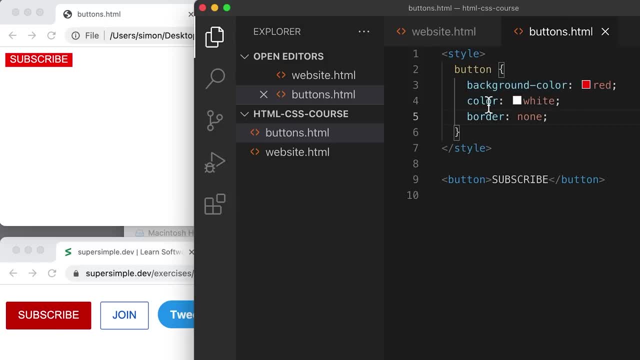 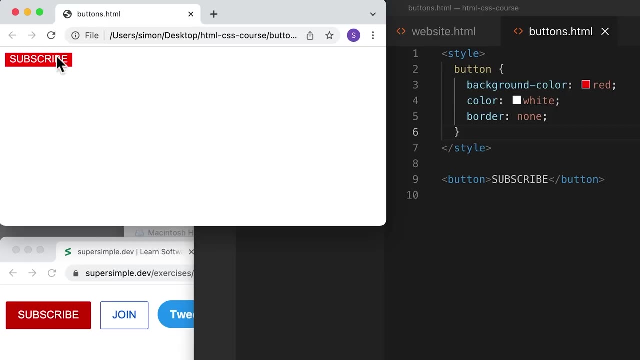 They're pretty easy to read. We set the background color to red, text color to white and border to none. So, just like HTML, CSS is pretty straightforward. We're essentially just giving the computer instructions. So the general technique for going from something that looks like this to something that looks 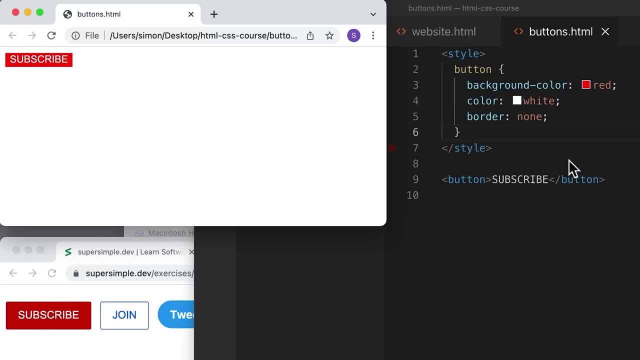 like this is to just change the styles one by one, So we're going to continue changing styles one by one Until we get our design here. The next style I'm going to change is the height, So our button is a little bit short. 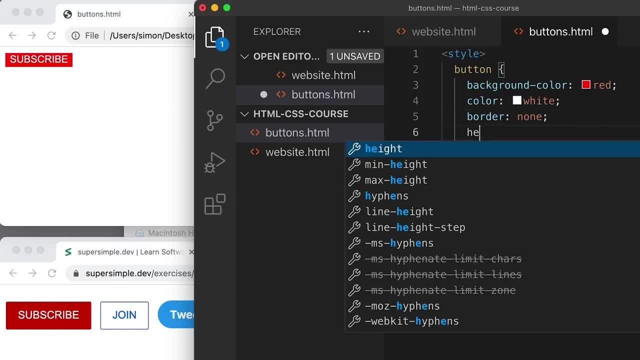 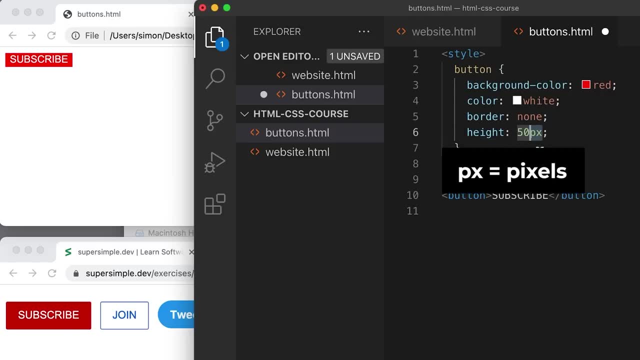 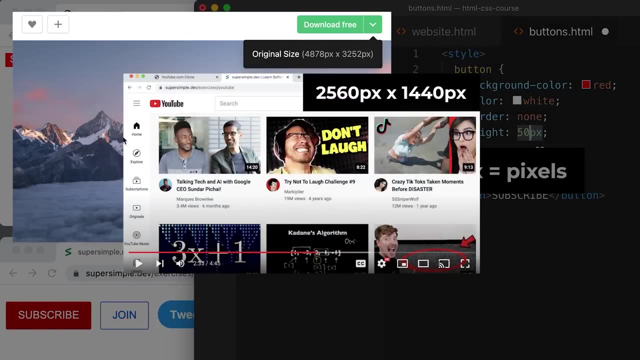 I'm going to make it taller, So I'm going to set the height to something like 50px. The px here represents pixels. Pixels are a very common unit of measurement in the digital world. Image sizes are measured in pixels. Video sizes are measured in pixels. 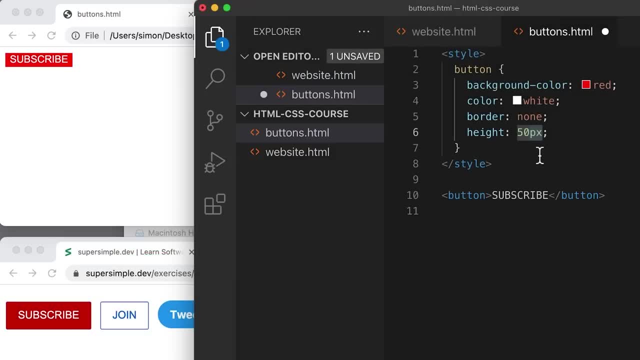 And your screen size is also measured in pixels, And your screen size is also measured in pixels. In this case, we're going to set the button height to 50px, And don't worry too much about knowing what 50px looks like. 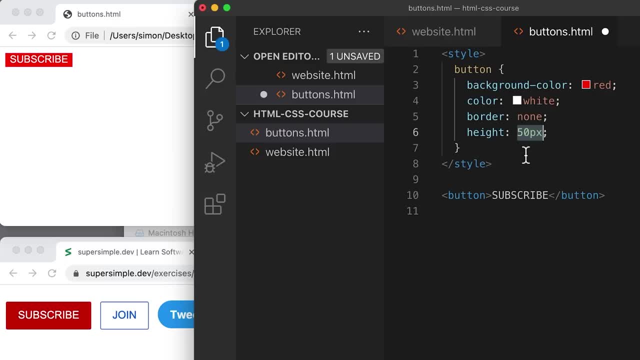 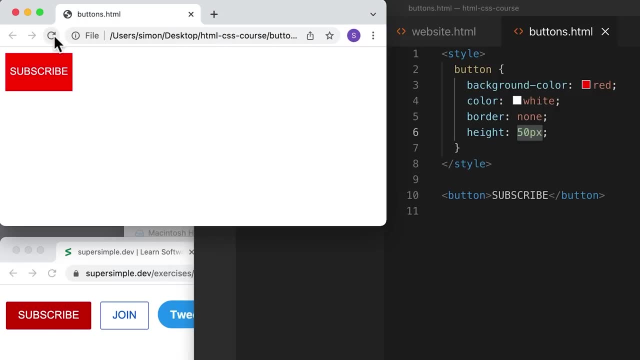 The more that you write CSS and work with pixels, the more you get a sense for how big these measurements turn out to be. So, for now, let's save this file and refresh the page, And now we have a button that is 50px tall. 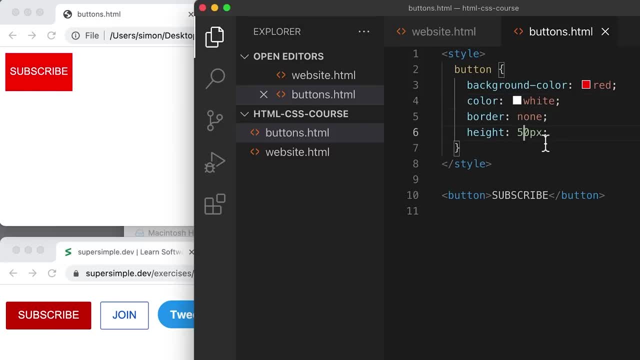 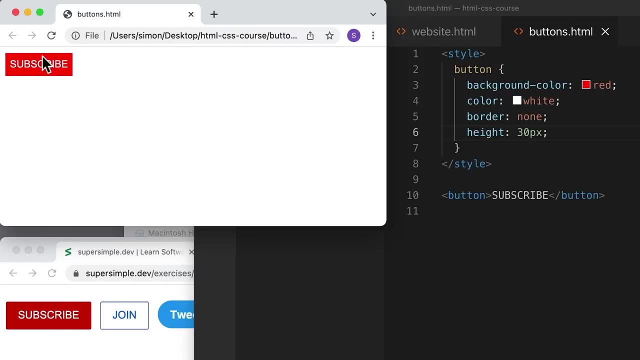 But it actually looks like it's a little too tall. So I'm going to change the height to something like 30px And we're going to refresh the page again And I actually want it to be a little bit taller, So I'm going to change it to maybe 36.. 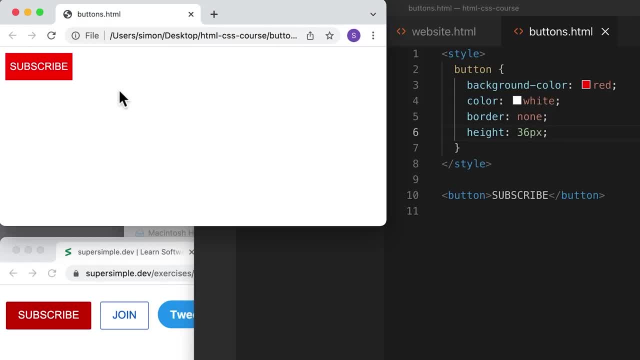 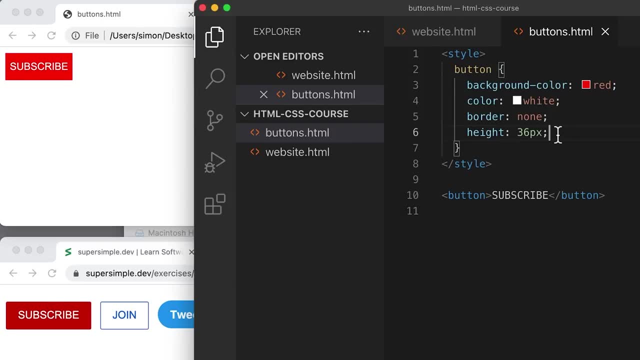 I'm going to refresh And I think that looks pretty good to me. So you see that in CSS we do a lot of trial and error to get our measurements right. Now let's keep working step by step to get to our design. 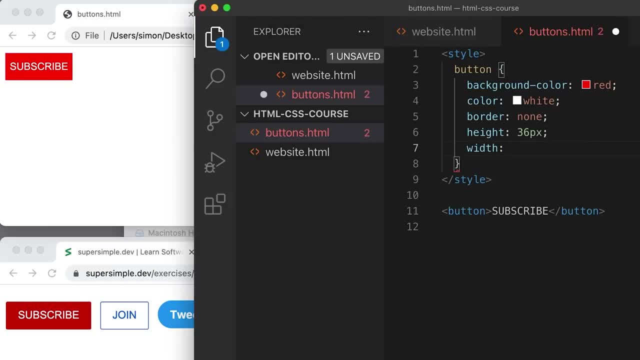 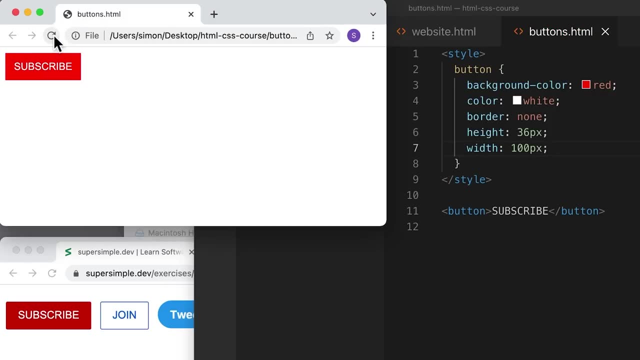 Next, we're going to adjust the width, So let's change this to something like 100px. Okay, Let's see how that looks. I'm going to save it, refresh, And I think it looks a little bit too small, so I'm going to increase it just a little. 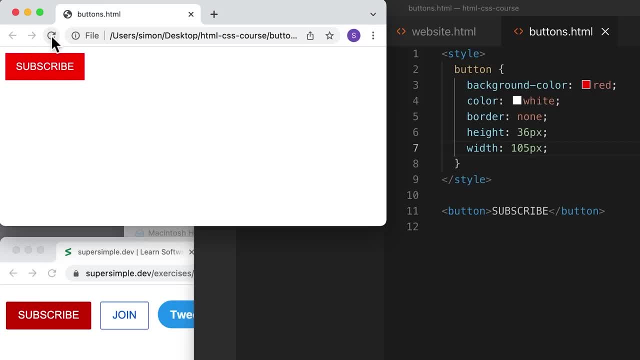 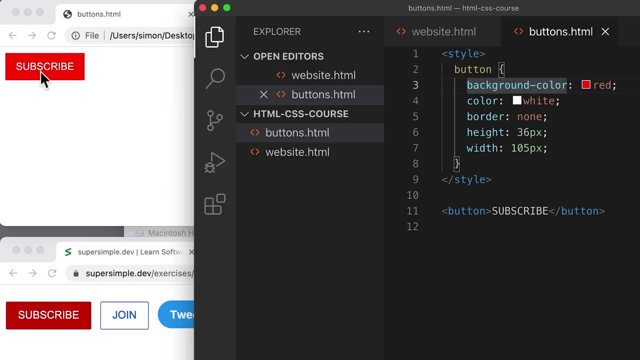 bit 105. And refresh. Okay, I think that looks good enough for me. Next, we're going to change the background color, Because currently our red is not the same as our design. So VS Code has a really nice feature, which is a color picker. 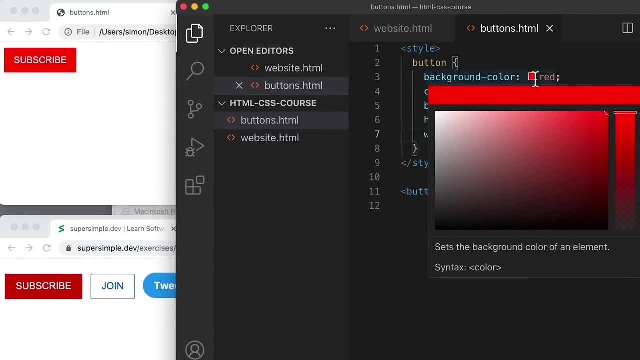 So if we hover over this color box here, It gives us access to a color picker that we can pick another color with. So I'm going to pick something that's a little closer to what I see at the bottom And, don't worry, it doesn't have to be perfect. 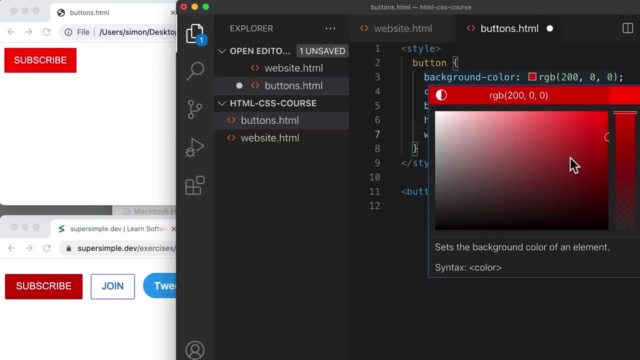 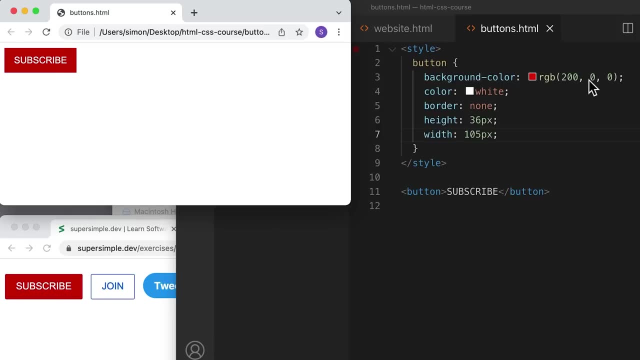 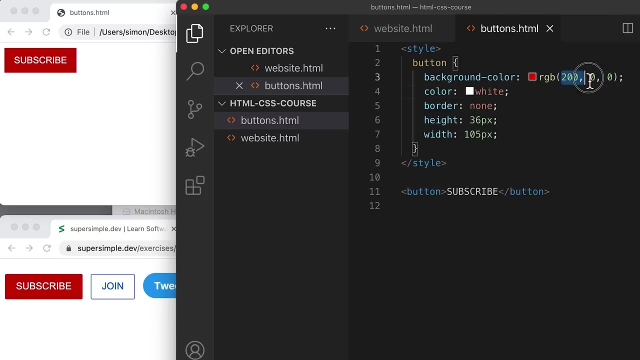 I'm going to pick something like 200.00.. I'm going to save this And refresh. Okay, so that looks. I think that looks close enough. So you might be wondering what this value means. We went from a color of red to RGB 200.00. 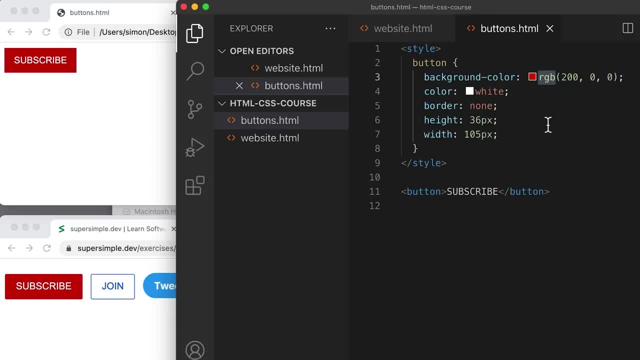 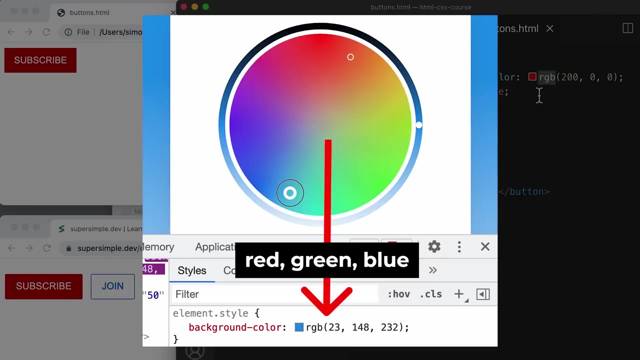 So this RGB value is another way of measuring color. It's a more precise way of measuring color than just using a word like red or white. So the way that RGB works is that pretty much every color can be created using a combination of red, green and blue. 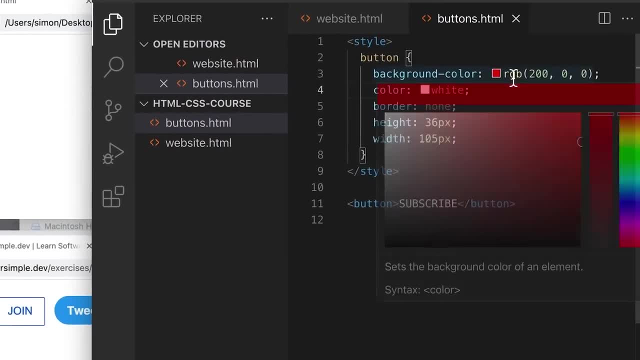 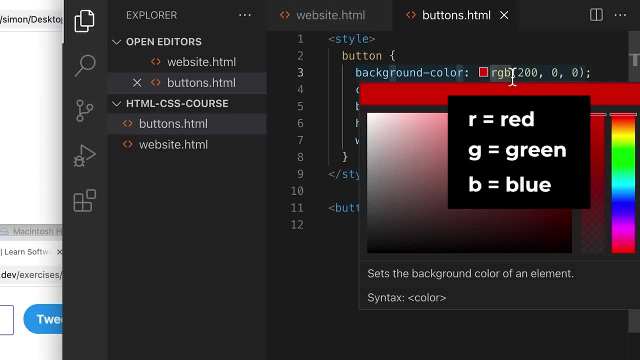 So that's what this syntax represents. The R represents how much red we have in this color, G represents how much green And B represents how much blue. And these three numbers represent how much red we have, how much green and how much. 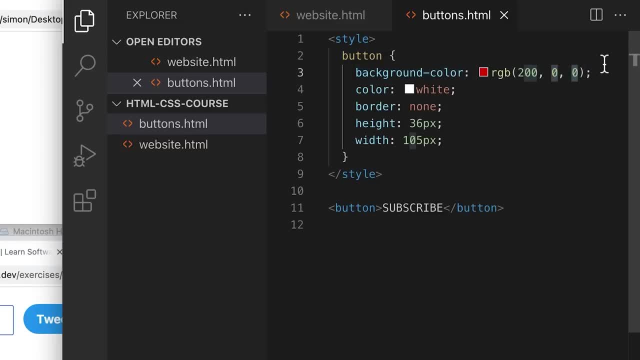 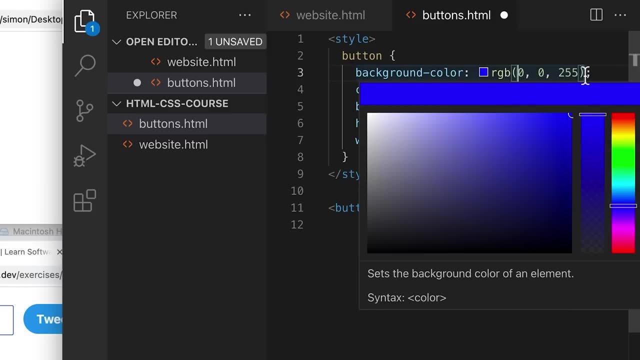 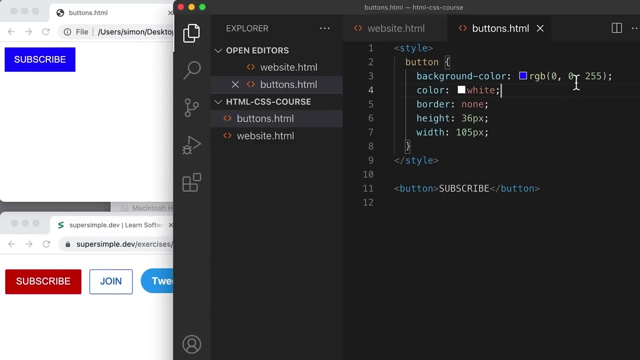 blue. The minimum value is 0, and the maximum value is 255.. So if we removed all the red and green and we just have maximum blue and we save, that's going to get us a blue color. On the other hand, if we have all green color and we get rid of the blue, we're going to 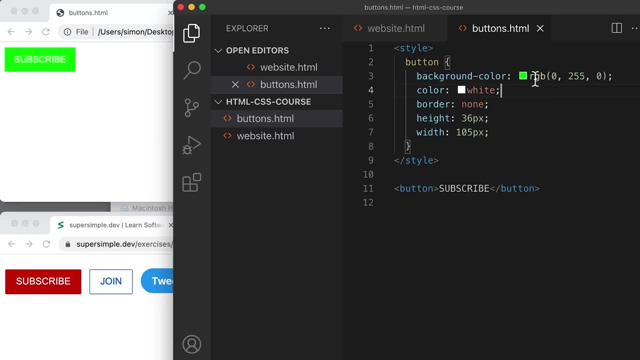 have a green color. So this is basically how RGB works. It's a combination of red, green and blue to create any color that we want. Now, don't worry too much about knowing what an RGB value looks like, For example, if you have a random value like this: if you gave this to me, I wouldn't even 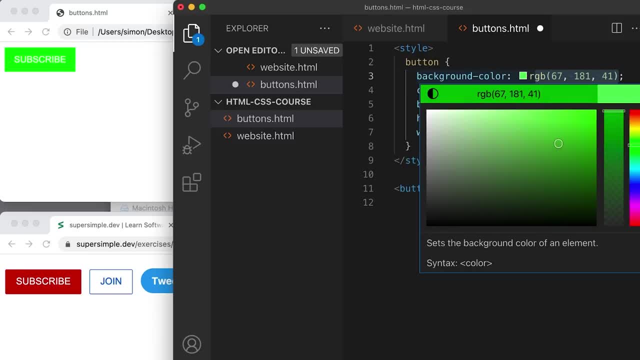 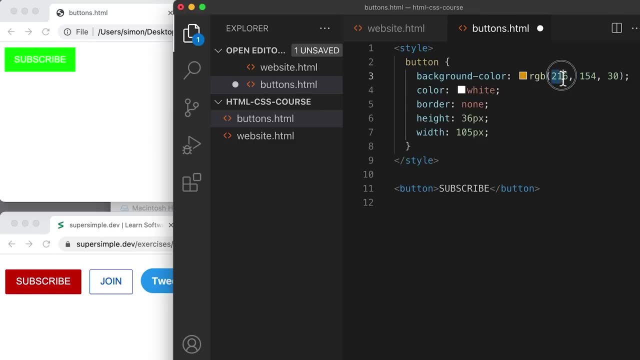 know what this color was. Usually I just use the color picker to pick the color that I want and then it will give me the RGB value that I need. The only RGB values I suggest you remember are if we set all, If we set all the colors to the maximum value, so 255,, 255, and 255, this creates white. 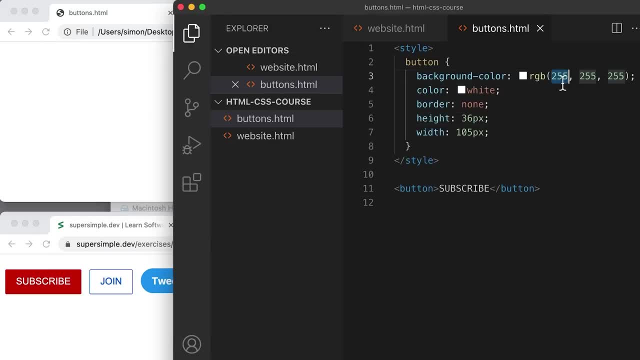 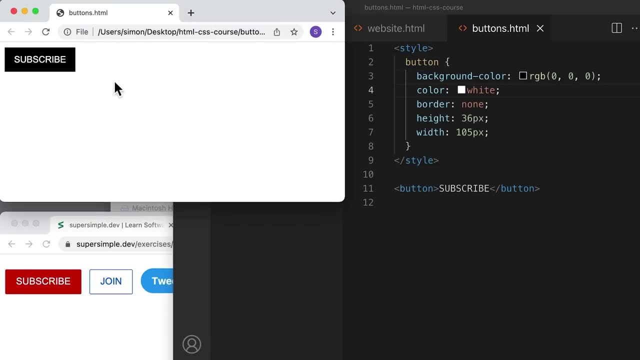 So we save it and refresh. that creates white. We set all of these three to 0, that creates black. We refresh that creates a black color. So now let's go back to what we had before, which I think was 200, 0, 0. 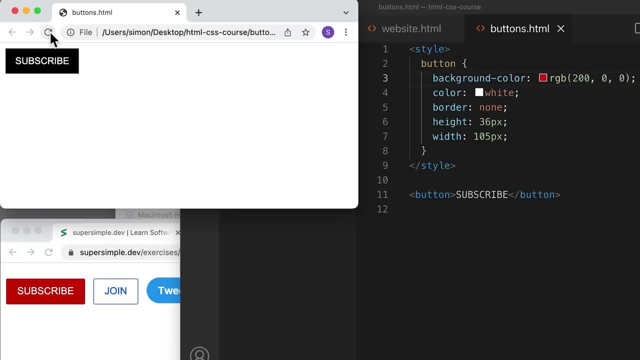 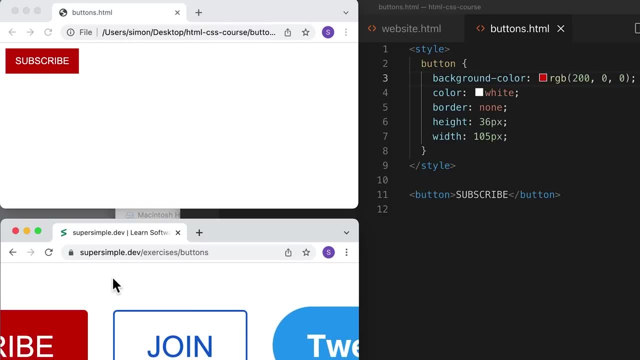 And we'll save, And we'll save, And we'll save and refresh. And the next thing we're going to change is: you might not be able to see it, but if we zoom in here, this button has rounded corners, while our button has pointy corners. 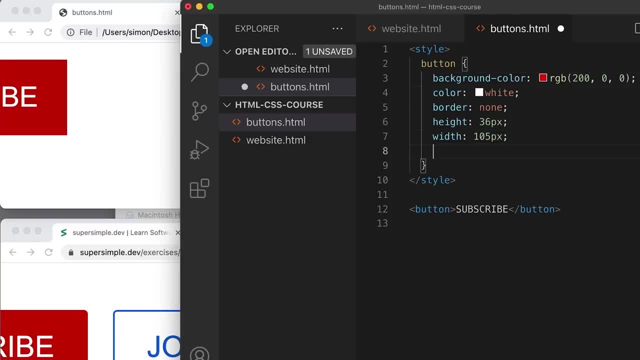 So to make rounded corners, the CSS property for doing that is border-radius, and the border radius takes a pixel measurement. The higher the pixels, the more round the corners will be. So for now let's try colon-2-pixels and save. 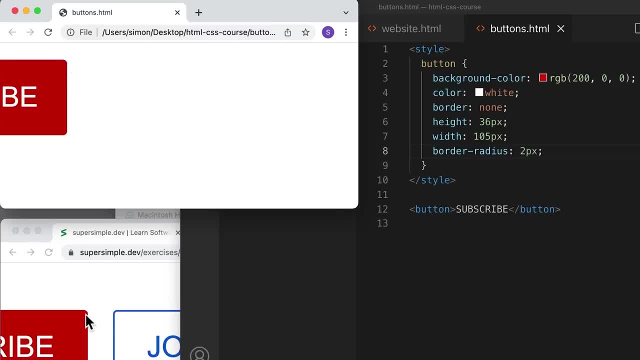 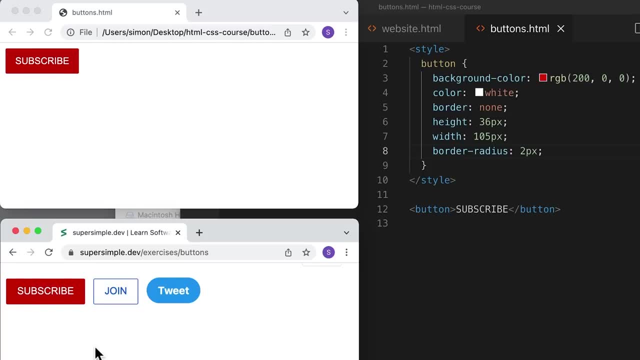 Now, if we refresh the page, our button now has rounded corners, just like our design. I'm going to zoom back out and zoom back out. So the last thing I'm going to change is, if we hover over this button, you'll notice. 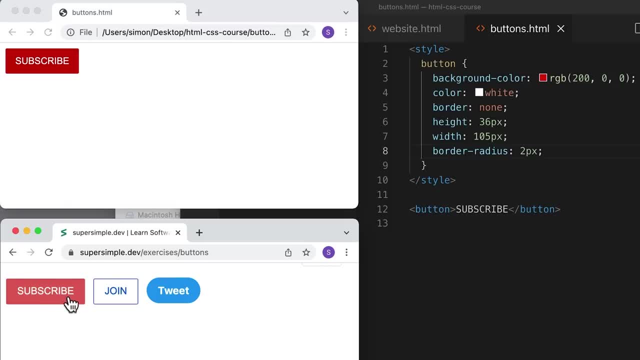 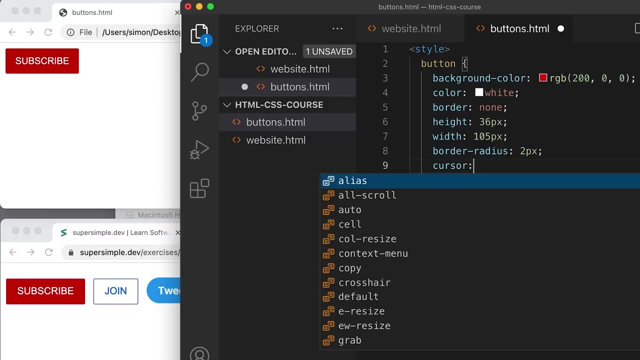 that our mouse turns into this sort of hand. This hand is called a pointer, So we're going to change the cursor. The mouse… that you point around is usually called a cursor, and we're going to change the cursor to a pointer. 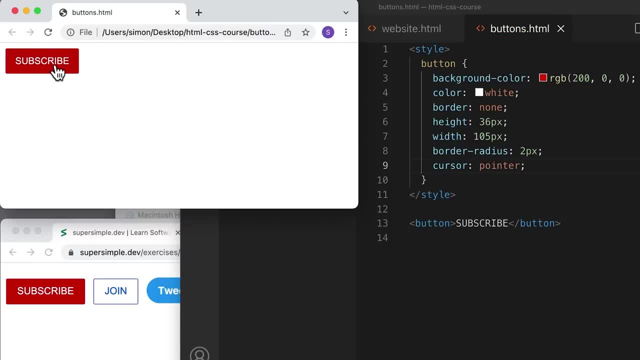 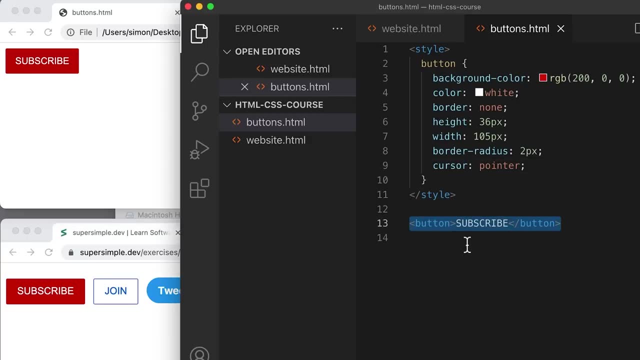 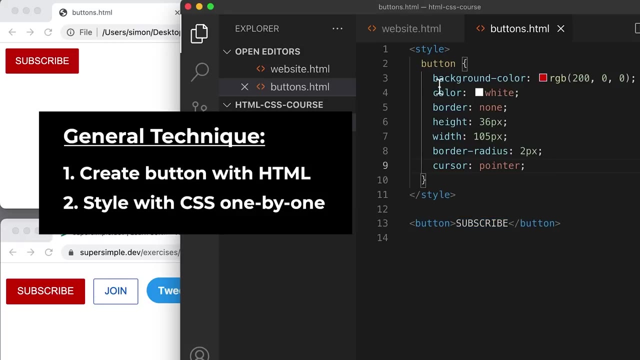 Let's save and refresh, and that's how you get this hand whenever your mouse is over this button. So that's basically how we go from a basic HTML button to something that looks more professional. We create the button with HTML and then we set the styles one by one. 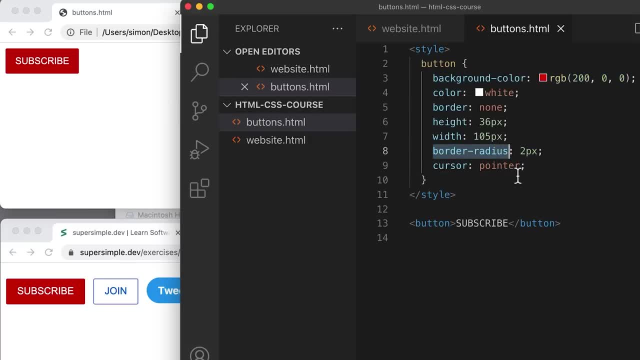 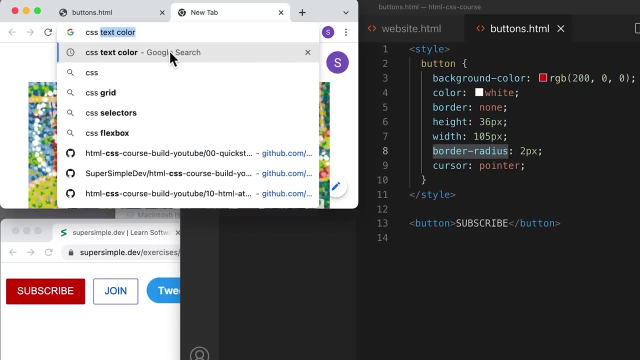 Now you might be wondering: how do I know all of these CSS properties? How are you supposed to memorize all of these? So usually when I don't know the CSS property for something- for example, if I want to create rounded corners- I would go to Google and search something like CSS and what I want. 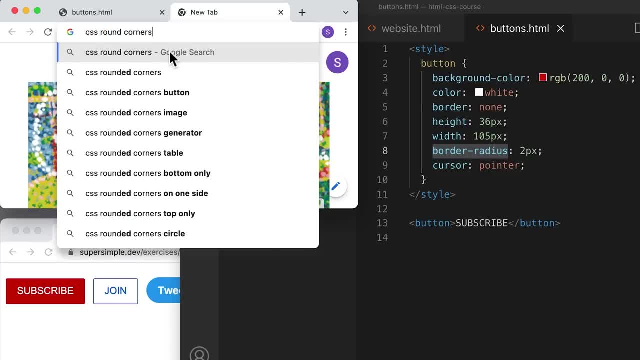 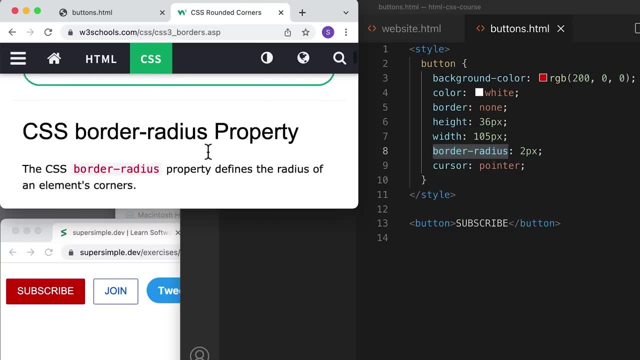 to do So. let's say, I want round corners, And usually the first few links give some really good suggestions on what the property is. So here, right away, we have the border-radius property in the first link and it gives us some sample code that we can use. 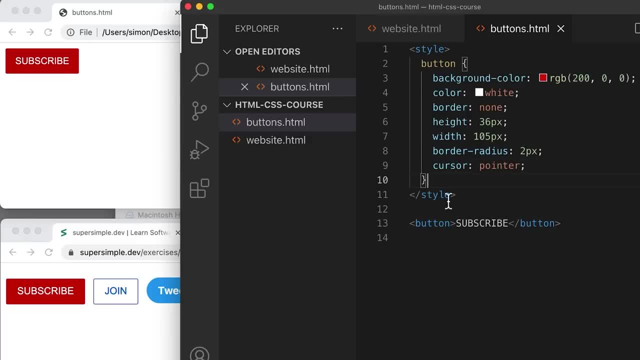 So that's how I discover all of these CSS properties. I look at a design and I ask myself: okay, what do I need to achieve this design? And then I search for it in Google. So don't worry, as you use CSS more and more, you're going to have to Google things that. 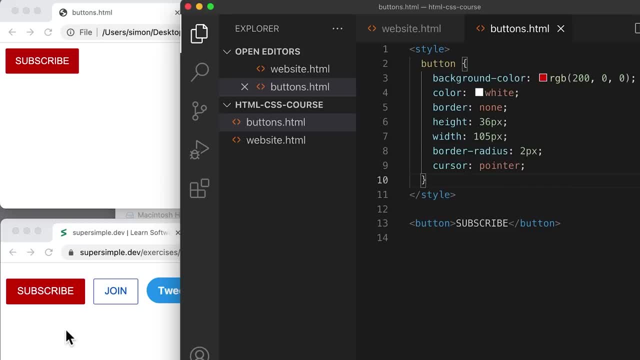 you don't know and you'll just get used to the process of finding answers by searching for them. But for this example, I'm going to go to Google And, for the purposes of this course, I'm going to give you a lot of these CSS properties. 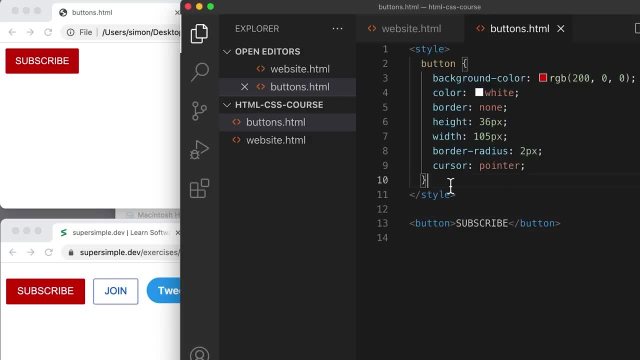 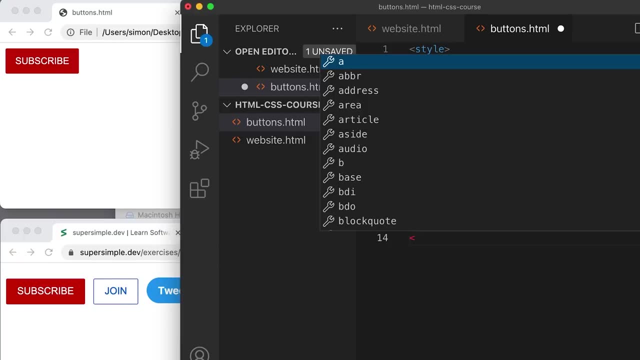 so that you can get some good practice with them. The next step we're going to do is to copy this Join button. So let's create a new button on our page with HTML And this is going to be the Join button. So we're going to put the text Join inside this button. 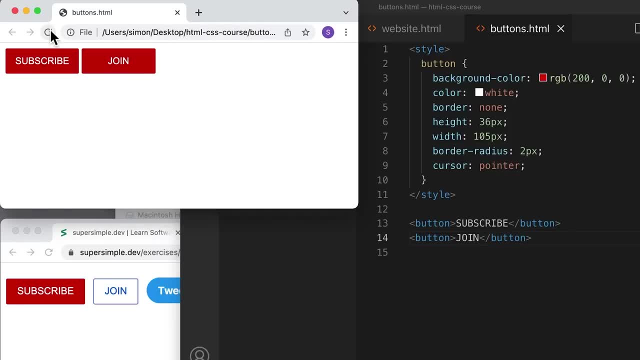 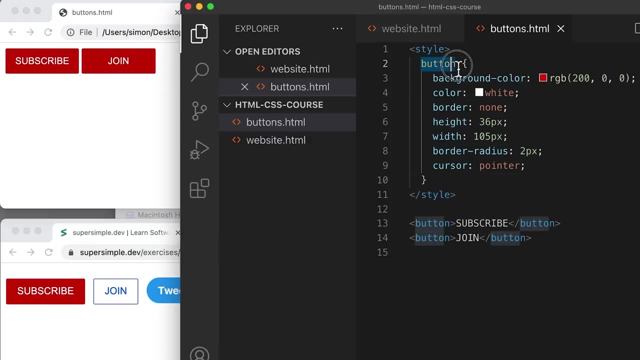 Let's save it and refresh And unfortunately it looks like our Join button. looks like this: So let's go ahead and add a button And if we click on the button, it looks like the Subscribe button. And that's because in our CSS this word button means that all of these styles are targeted. 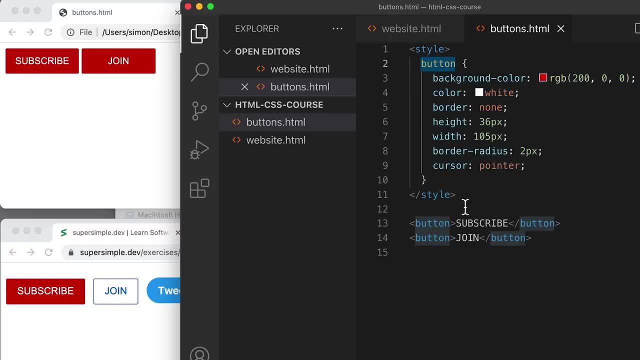 to all buttons on the page. So how do we get these styles to only target the Subscribe button? So we're going to learn a new HTML attribute that we can use for this. So remember, in the previous lesson we learned that attributes modify the behavior of elements. 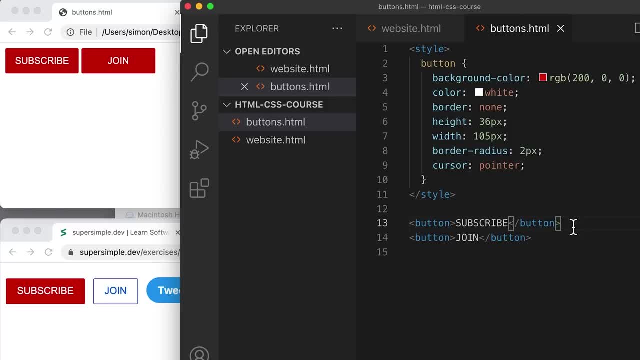 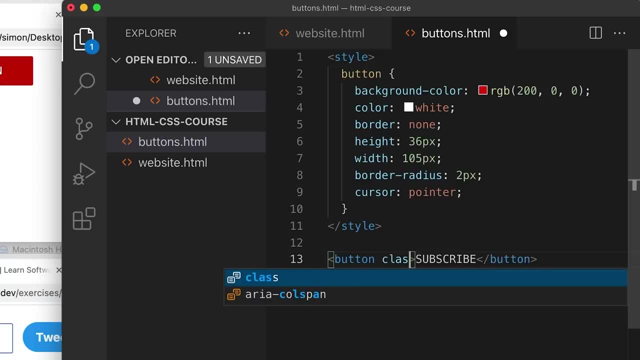 In this lesson we're going to learn a very useful attribute that is used a lot in the CSS. We're going to go to the opening tag again and we're going to add a new attribute called the class attribute. So I'm going to type: class equals quotes, quotes. 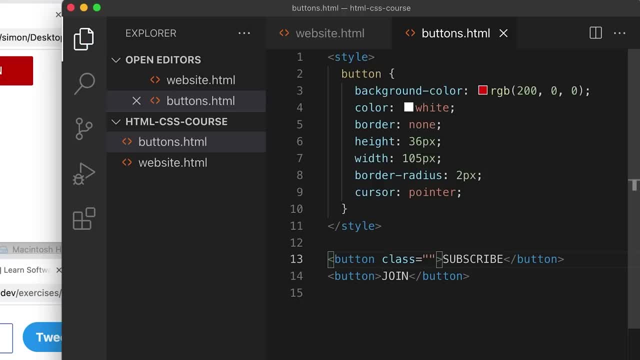 So the class attribute basically lets us label HTML elements. For example, let's label this button, the Subscribe button, And also my code is getting a little long for this line. Let's put the text on a new line to make it easier to read. 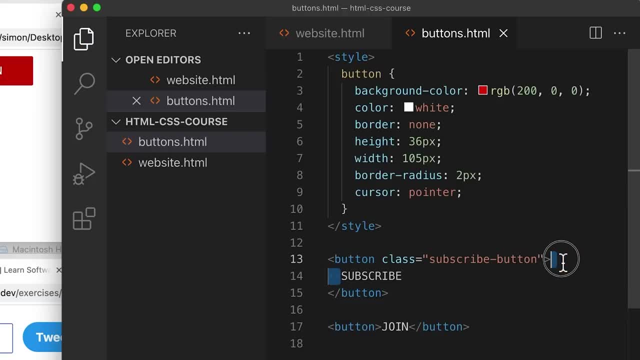 So remember, according to HTML syntax, these extra spaces don't matter, They're ignored. So now that we set the class attribute, we've essentially set a label to this button And we can target this label in our CSS. So to target a class in CSS, we can start with a dot. 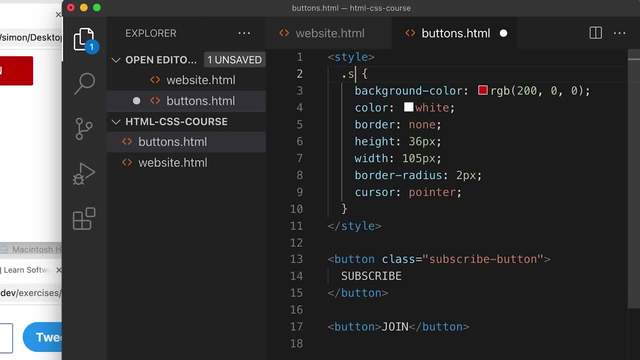 And then we're going to type out the class name. So we're going to type out subscribe-css. So according to CSS syntax, if we start this code with a dot, that means we're going to target a class name instead of an element name like button. 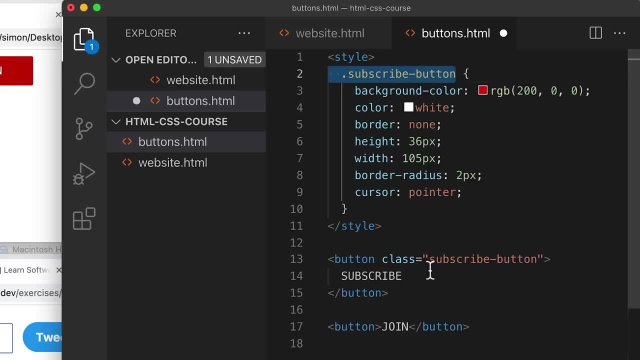 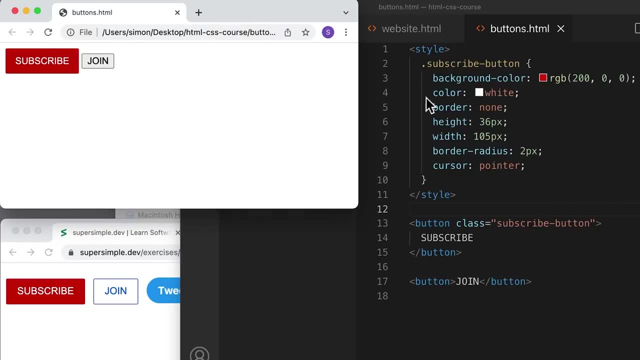 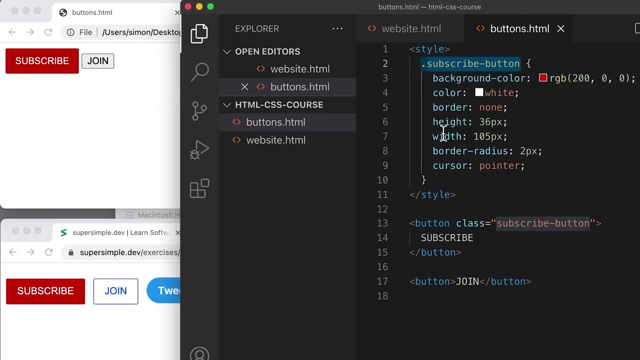 So here we're going to start targeting just any element that has the class subscribe button. So if we save and refresh now, you'll see that all of these styles only apply to elements that have the class subscribe, And our join button does not have any of these styles. 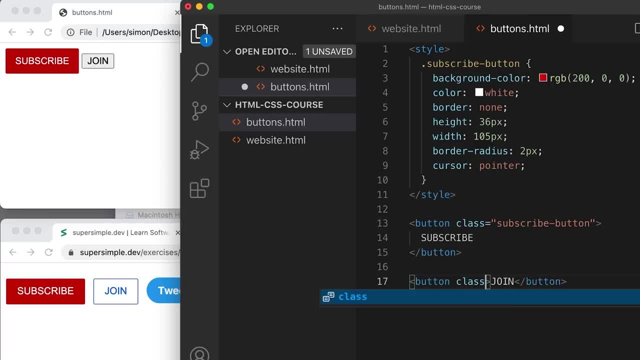 Now, multiple elements can have the same class. So, for example, if I set the class of the join button to subscribe-button, all of these styles will be applied to any element with the subscribe-button class. That's what this dot means, And that means these are going to be applied to this and this. 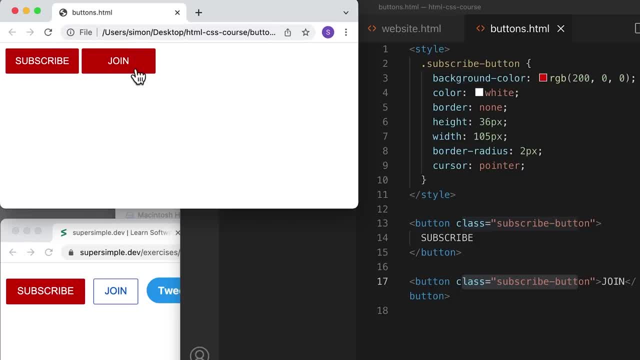 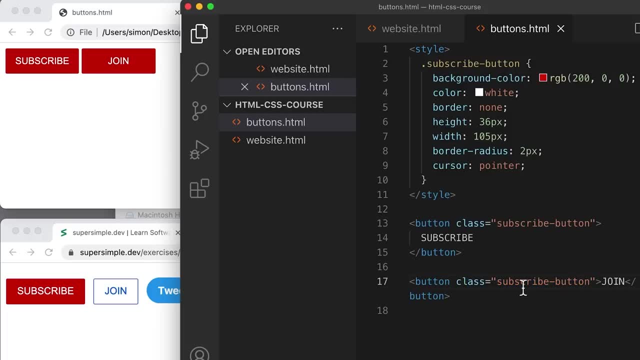 So if we save and refresh Again because it has a class of subscribe-button But for our purposes we actually want this to have a different set of styles, So let's give a different class to the join button. We're going to give the class join. 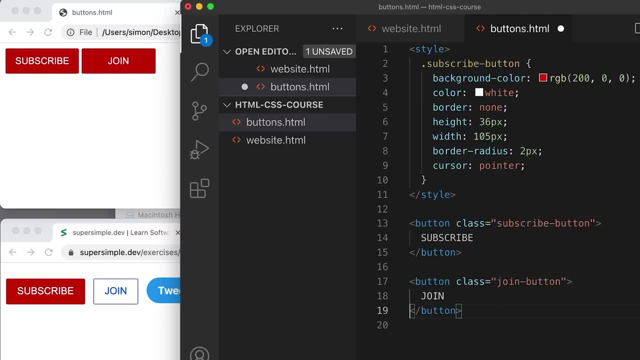 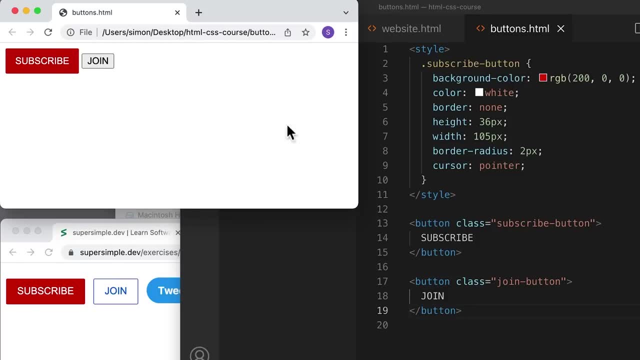 And I'm also going to reformat my code a little to make it easier to read. So let's save and refresh. And now we're back to where we can start modifying our join button. Now let's start styling our join button to match our design. 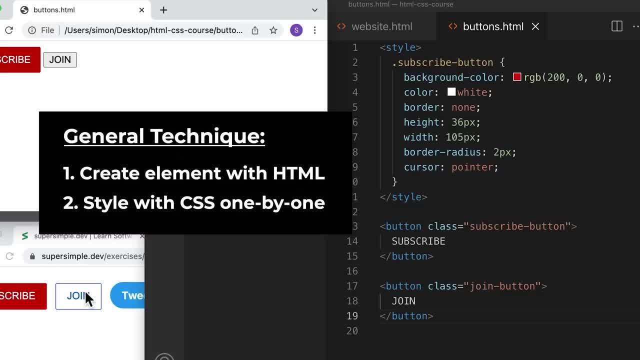 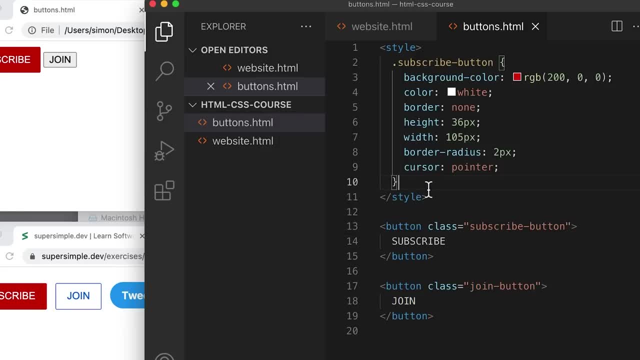 So, remember, the general strategy is to create the element with HTML like this and then style it one by one until you match your design. So first we're going to target the class. That's what this dot means. We're going to target the class join-button. 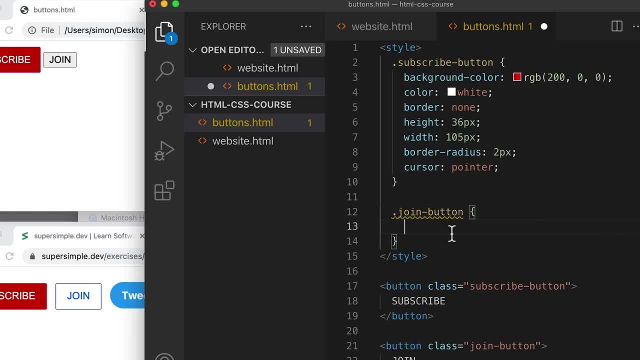 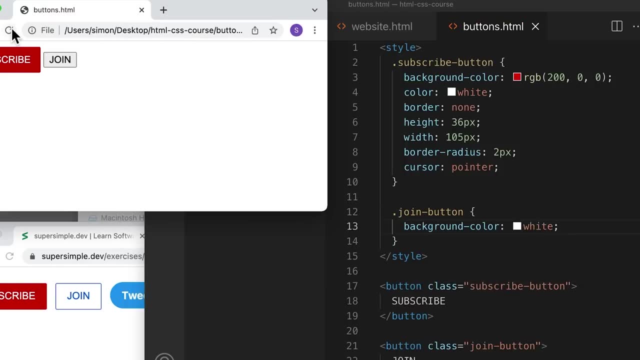 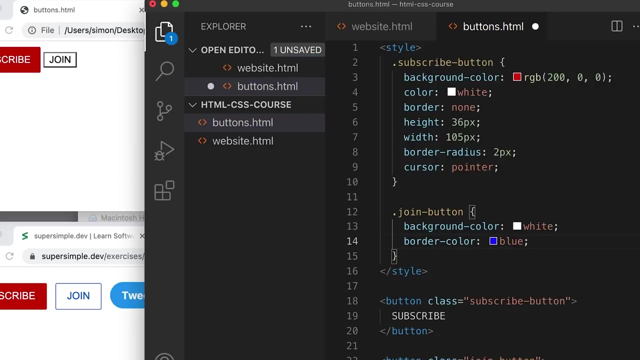 Okay, so let's set the background-color to white, Let's save it and refresh, And next Let's deal with the border. So our border is a little bit gray. We can set it to maybe border-color to blue, And let's see how that looks. 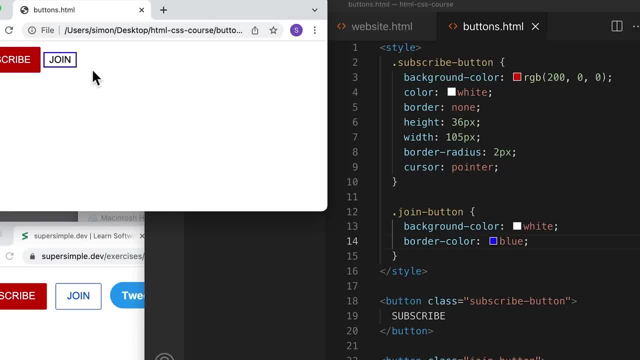 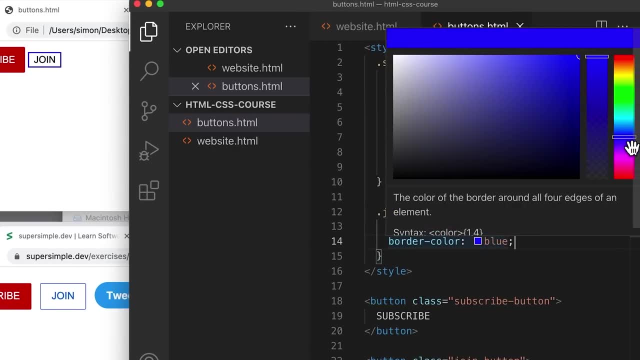 Let's save it and refresh. Okay, so it looks a little darker than what we have in our design. Let's go into our color picker and pick a more accurate color. I'm just going to do this by eye, Don't worry if it's not totally accurate. 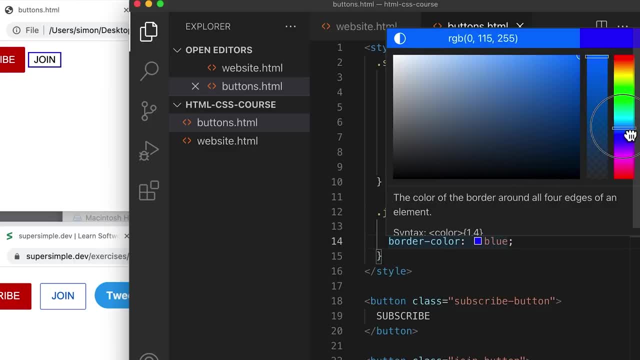 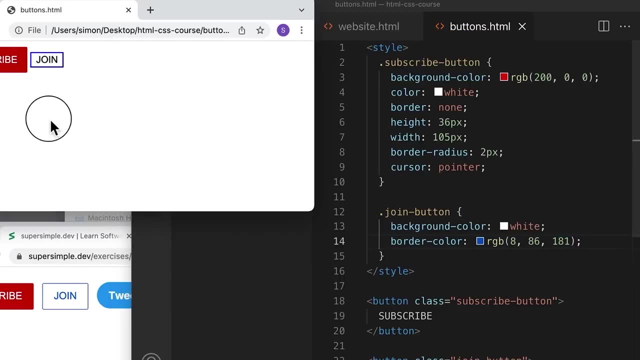 We're just trying to get something that's close enough. I'm going to go over here and I'm going to pick something like: maybe something like this: Let's save it, refresh, and that's a little bit too dark, so I'm going to pick something. 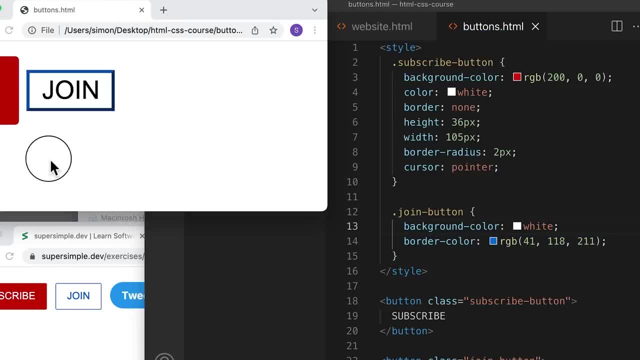 a little bit lighter, Save it and refresh. Okay, I think that's pretty good. But we also noticed that our border is a little weird. So on the top it looks like it's a darker, it's a lighter shade of blue, and at the bottom 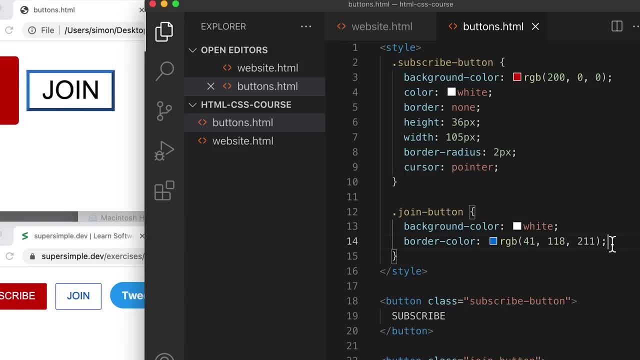 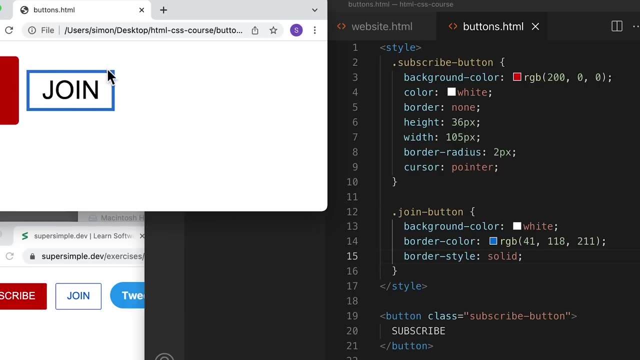 it's kind of a darker shade of blue. So to fix that, we're going to set the border style to be a solid color. Let's save this and refresh, And now we get a solid color all around. The next thing we can change is our border looks a little bit thick compared to the design. 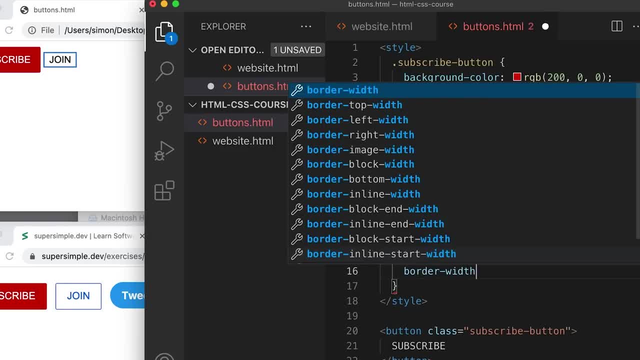 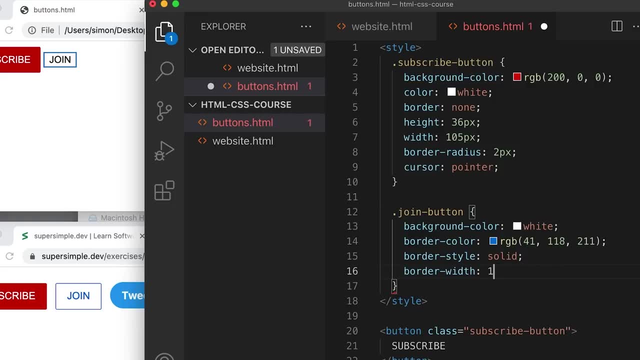 So we're going to change the border-width. So you'll see that a lot of these styles- Okay, A lot of these styles- are pretty self-explanatory. So we're going to set the border-width to, let's say, one pixel. 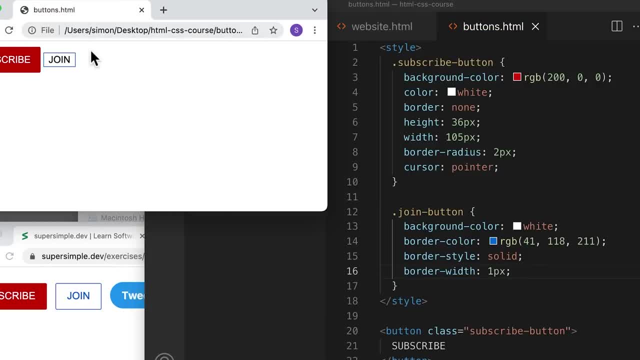 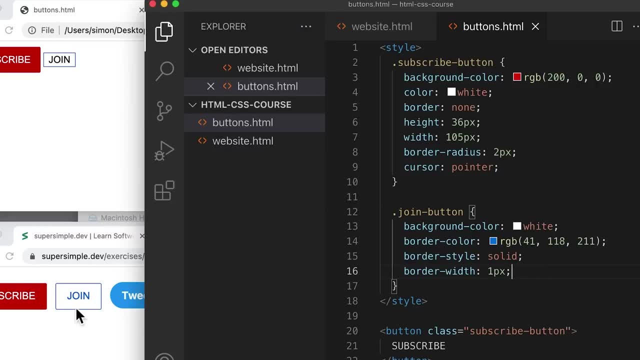 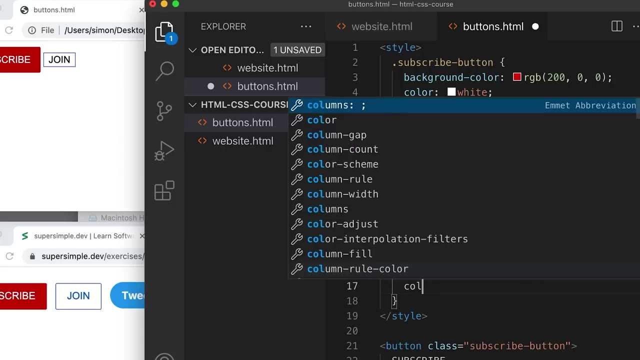 Let's save it and refresh. Okay, so that looks pretty good. Next, we're going to set the text color. So we're going to set the text color to blue and have it the same as our border. So remember, the property to set text color is called color colon and we're going to 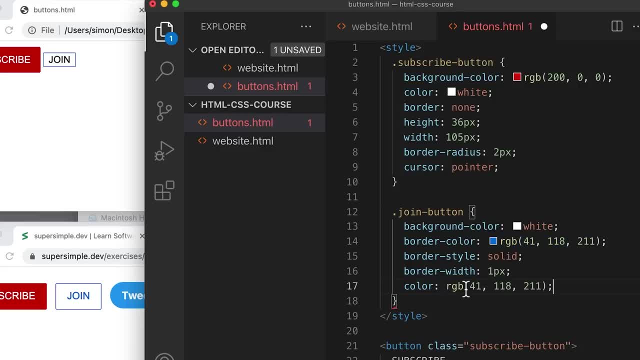 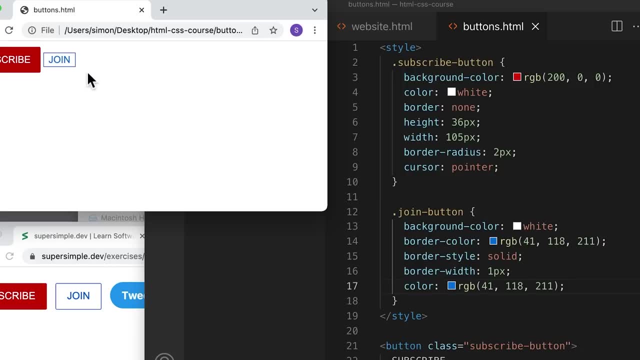 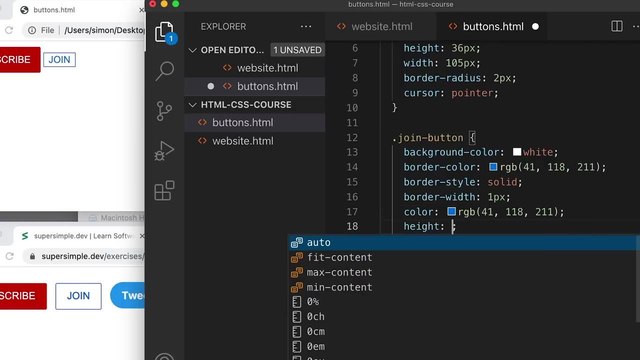 copy this color down here, Save it and refresh. Okay, so that looks a little light, but I think it's okay. Now we're going to set the height and the width. Let's set the height to be something like 36 pixels to match our subscribe button. 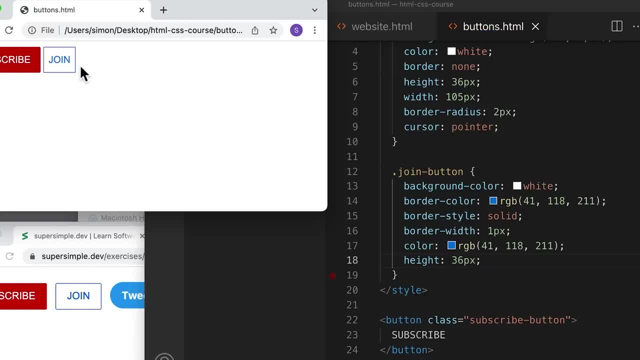 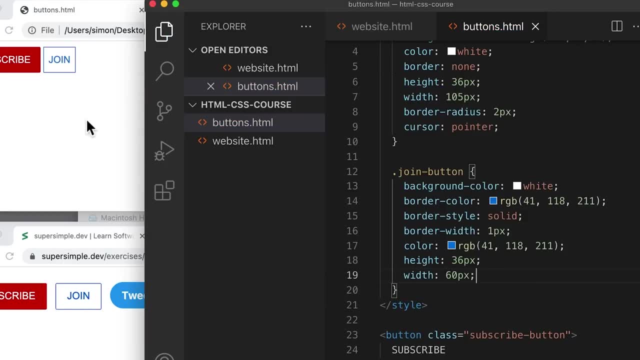 Refresh. And now we're going to set the width. So let's try. I don't know. 60 pixels. Okay, 60 pixels, Let's see how that looks. Save and refresh. Okay, I'm going to set it to maybe 62.. 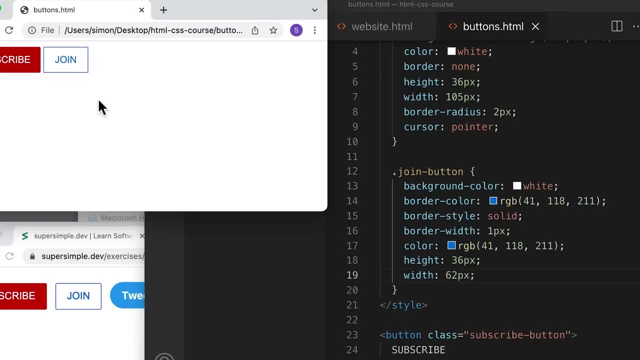 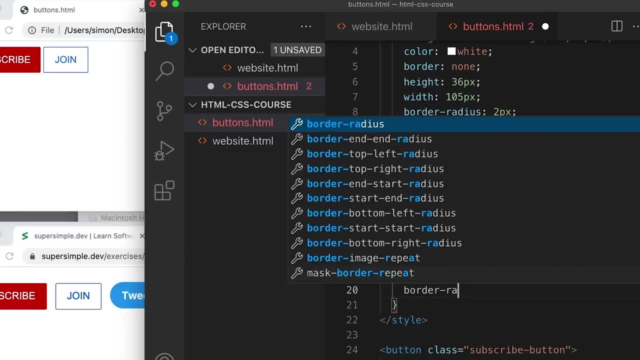 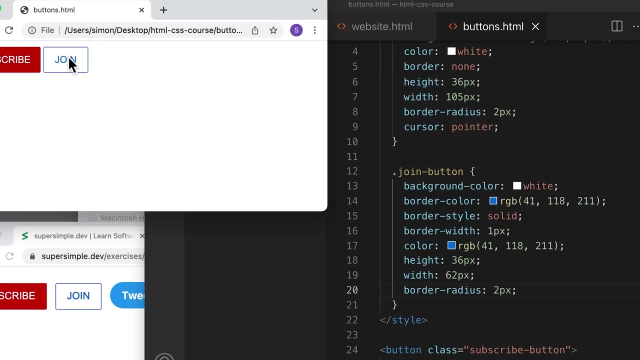 Okay, let's save and refresh, And again we're going to set some rounded corners. So that is border-radius: 2 pixels. We're going to save it and refresh, And now we're almost there to matching this design. The last one. 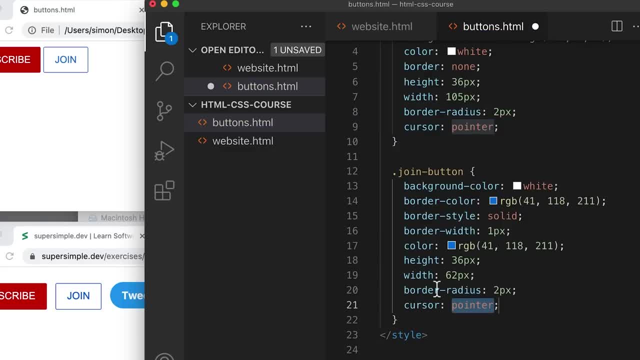 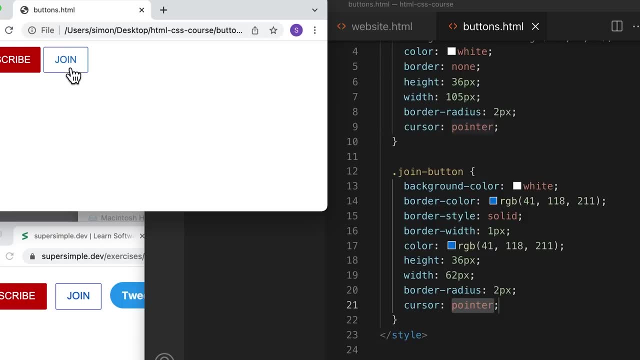 We're going to set the width, We're going to set this cursor pointer to get that nice hand pointer when we're hovering over the button. So refresh. Now, when we're hovering over the join button, we have this nice pointer icon. So another thing we notice is that there's a lot of space between these two buttons. 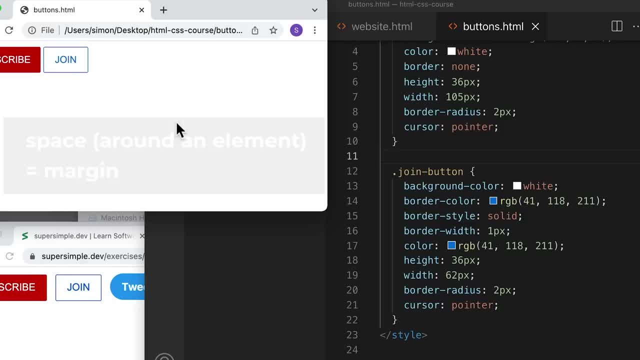 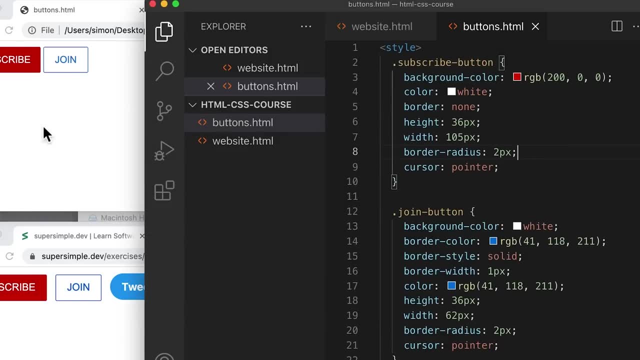 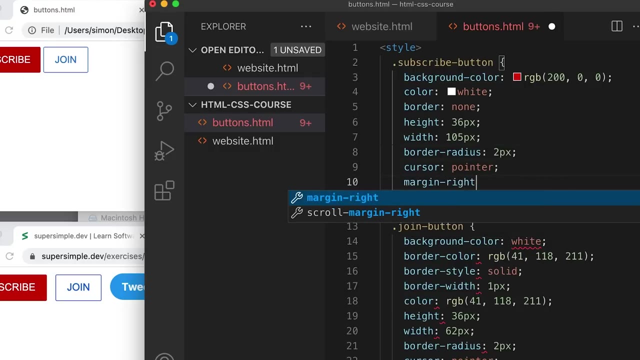 and there's not a lot of space between ours. So in CSS space is called margin. So to add space, we're going to add some margin. So let's go to the subscribe button styles And we're going to add some margin-right. 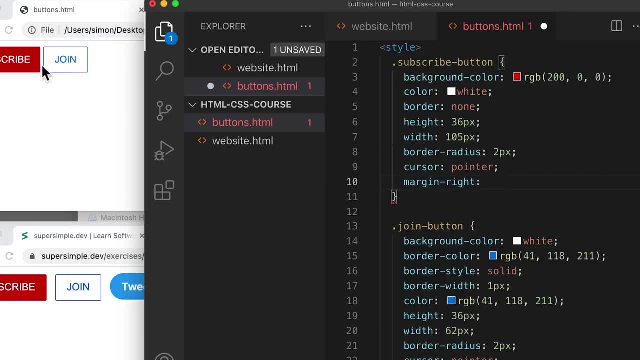 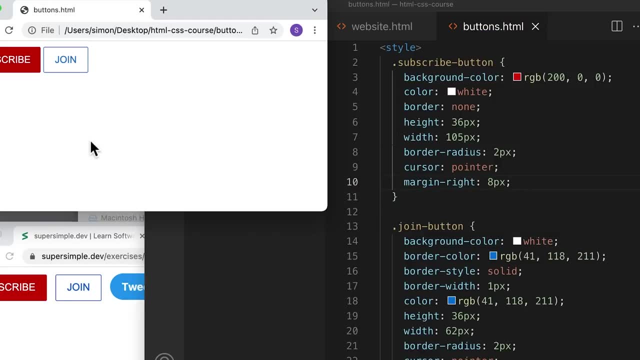 So we're going to add some margin or some space to the right of this button And we're going to set the space to maybe 8 pixels. Let's see how that looks: Save and refresh, And that looks pretty good to me. 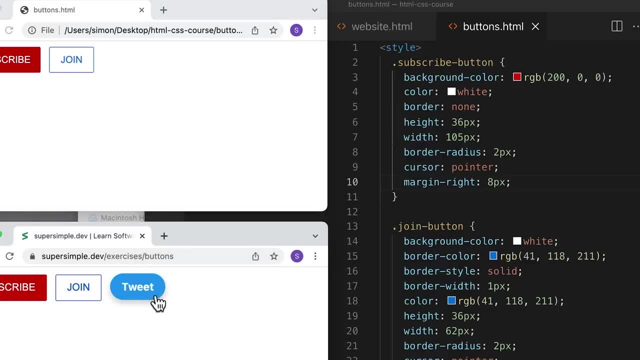 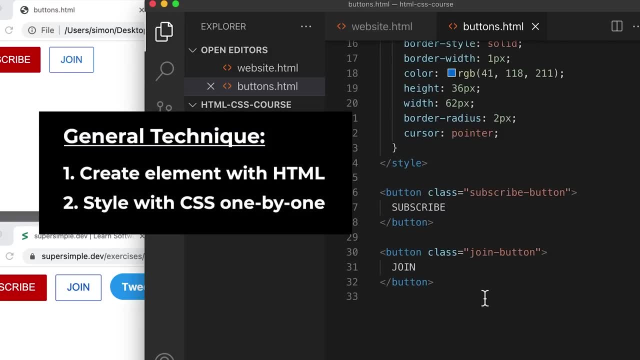 So now we're done with the join button. Lastly, we're going to create this tweet button. Let's go back into our code And remember: Our general technique Is to, number one, create the element with HTML And then, number two, style it with CSS, one by one. 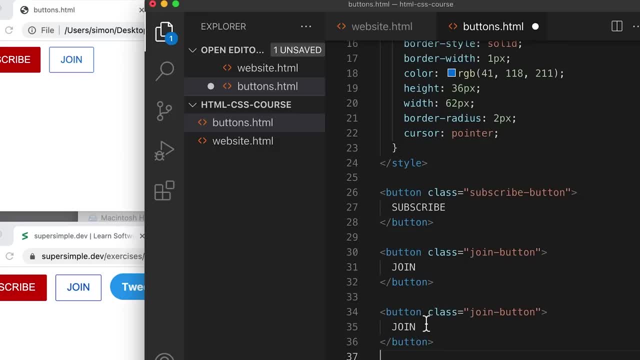 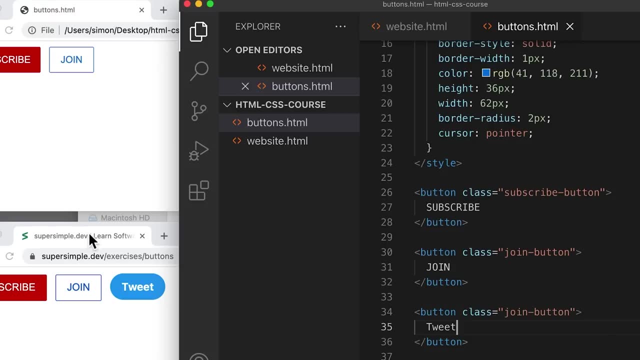 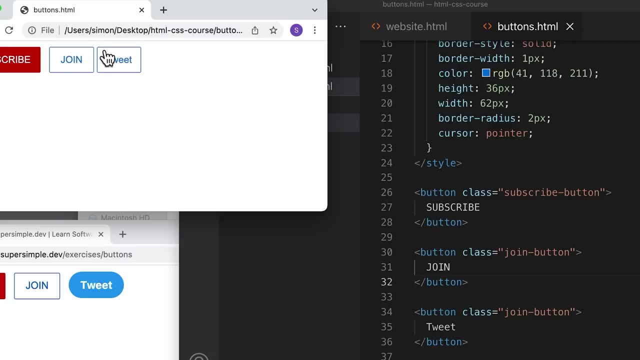 So we're going to create a button with a text tweet. I'm going to move my editor a little bit to the right here so we can see it. I'll move this here as well And let's refresh our page. So now this button has the same style as the join button because it has the join button. 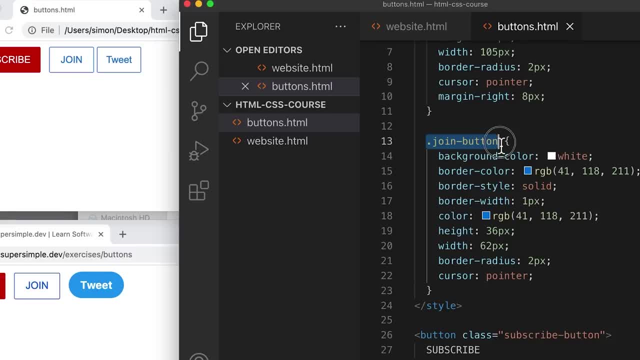 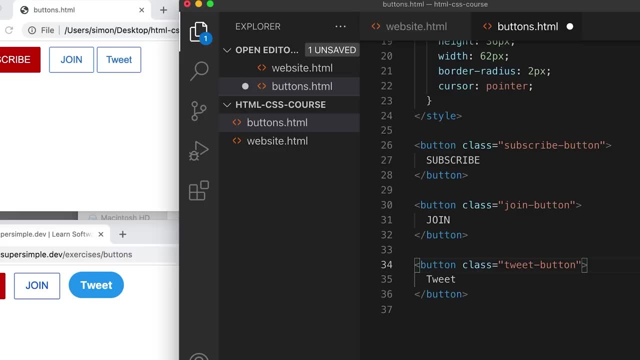 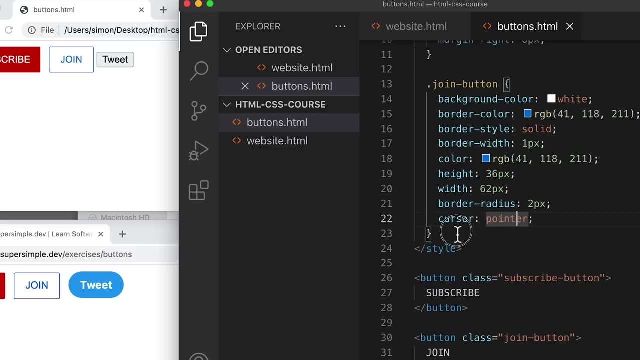 class That's being targeted up here. So instead of the join button we're going to give a class or a label of tweet button. Now save and refresh. And now we're back to the default styles. So in our CSS we're going to write some code. 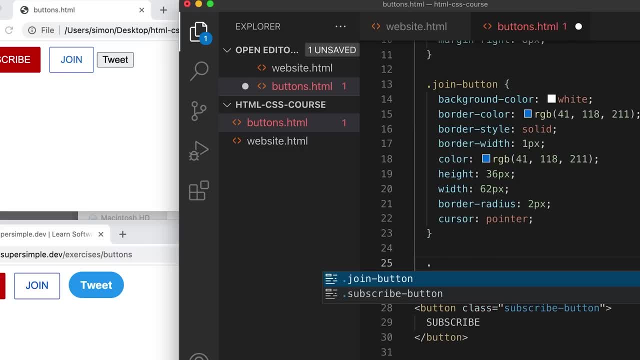 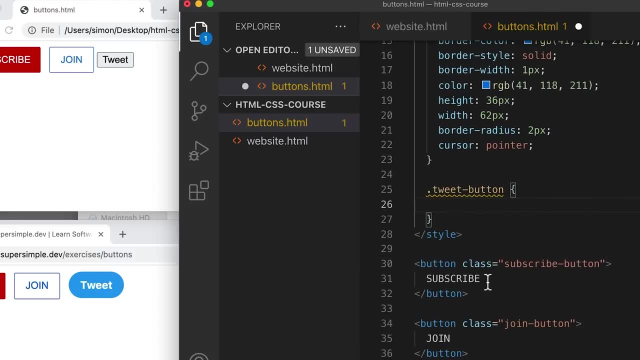 We're going to target the class, So we start with a dot to target a class. We're going to target the tweet button class. So, just like our other button, We're going to adjust the style of this button one by one until we match our design. 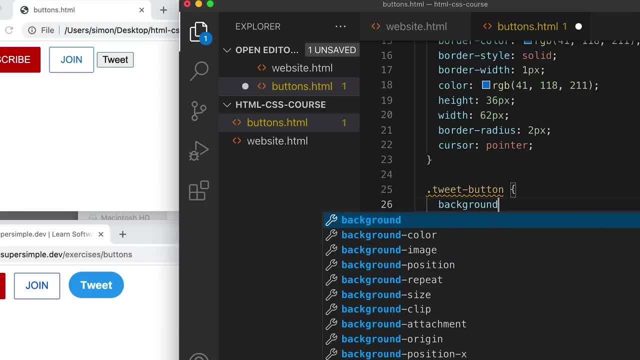 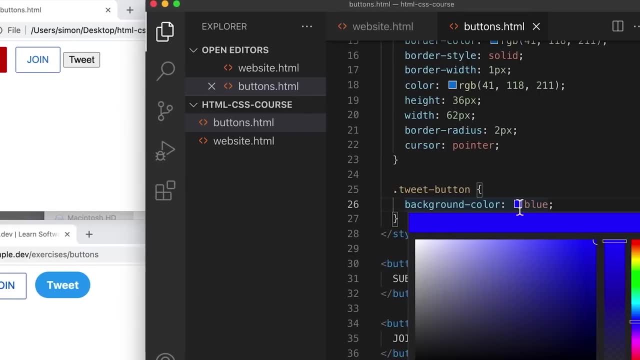 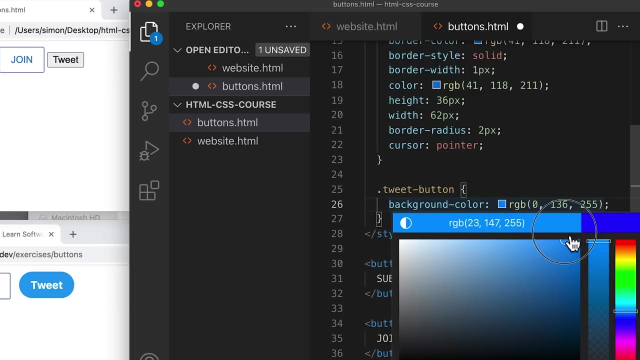 So let's start off with the background dash color. Let's set this to blue to start off with. Now I'm going to try my best to match the Twitter blue that we have here, So I'm going to pick something like this, And I think that looks pretty good. 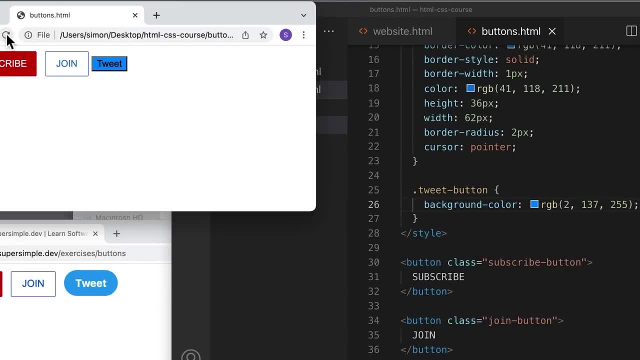 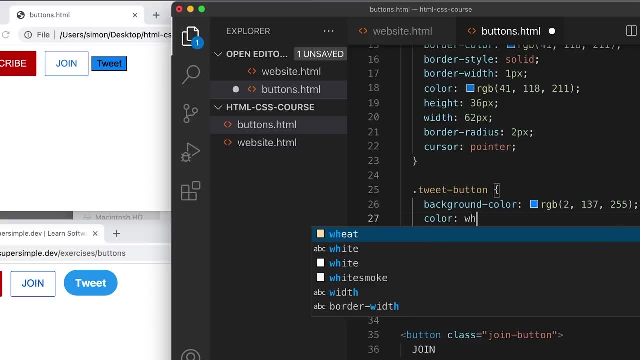 Save it And refresh. OK, We'll leave it like that for now. We might adjust it later. Let's change the color now to white, So that'll change the text color. OK, Let's get rid of the border. Refresh and save. 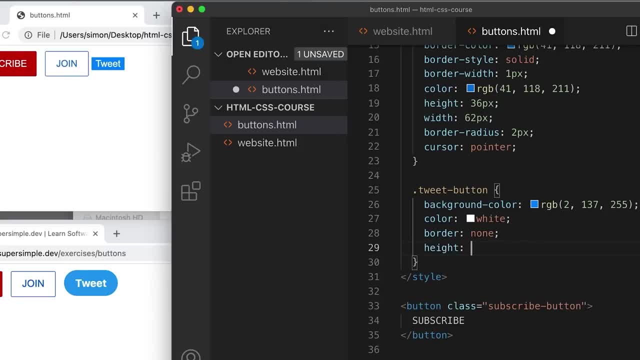 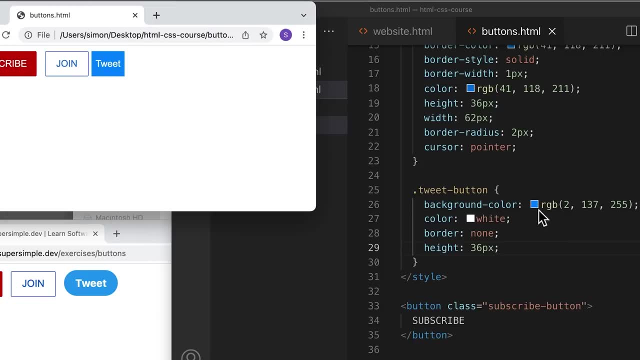 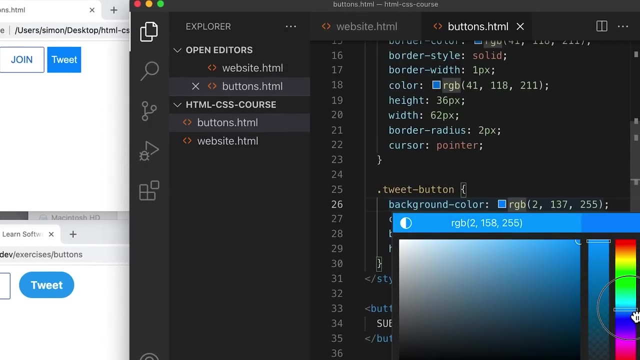 Let's give it a height of 36 pixels to match our other buttons, OK, And the color is a little bit off, So I'm going to adjust it just a bit. Maybe it should be a little more like this: Save it. 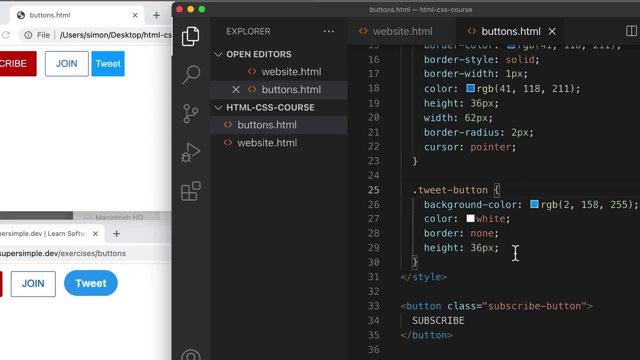 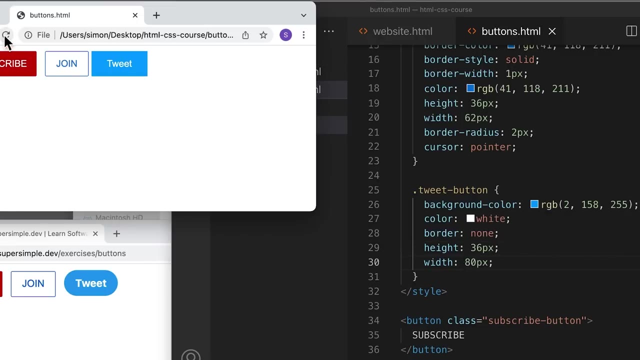 Refresh. OK, I'm pretty happy with this. Now we're going to adjust the width to maybe 105.. Let's see how that looks. OK, That's a little too much. Let's adjust it to 80.. Let's adjust it to 70.. 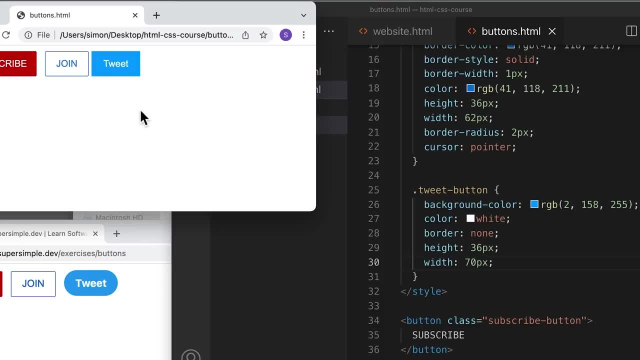 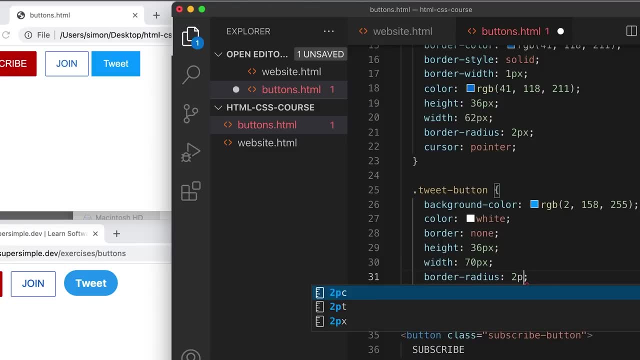 So, as you can see, there's a lot of trial and error when we're working with CSS. Now, to get this rounded effect, we can set a border radius. Let's start with 2 pixels. If we refresh, we get rounded corners. 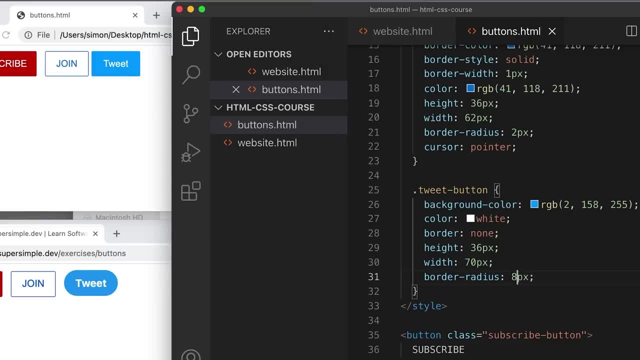 If we start increasing the pixels for the border radius- let's save and refresh- it starts getting rounder and rounder. So the trick to getting these round buttons is we have to set the border radius to half the height or the width, whichever is lower. 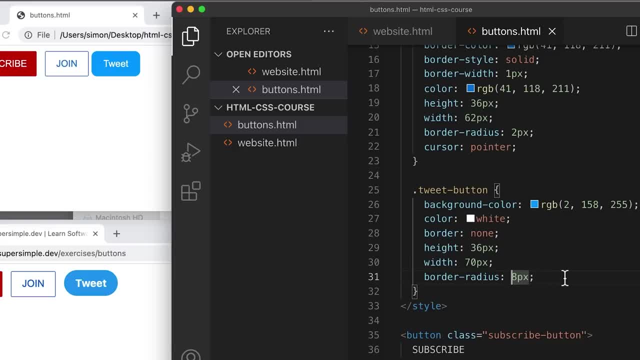 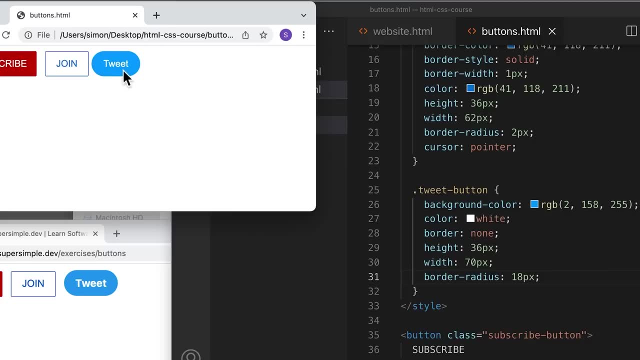 So in this case the height is 36.. If we set the border radius to half of that, which is 18, save and refresh. that's how we get this rounded color. The last thing we're going to do is to bold the text in here. 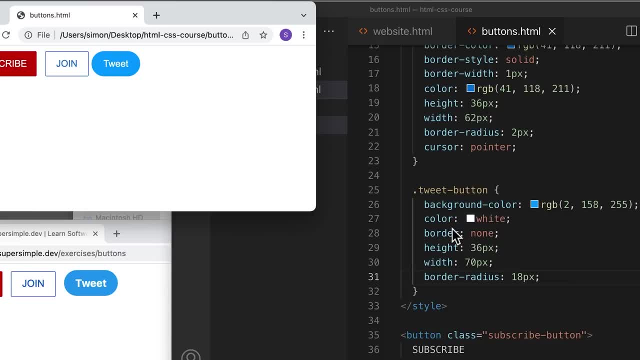 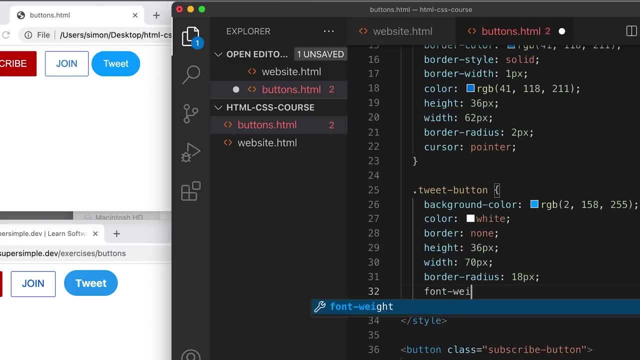 So in our design, this tweet text here is very bold. We're going to make our font bold as well. So to do that, we're going to set this property called font-weight. I'm going to set it to bold. Save and refresh. 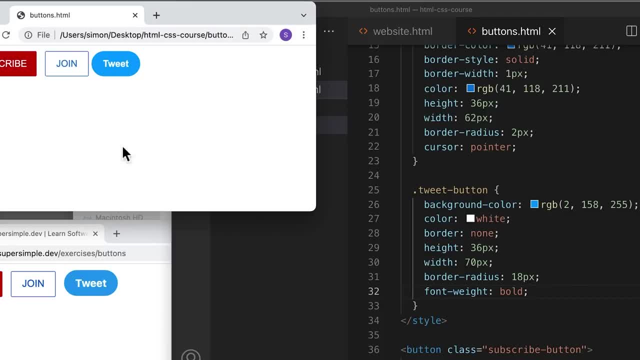 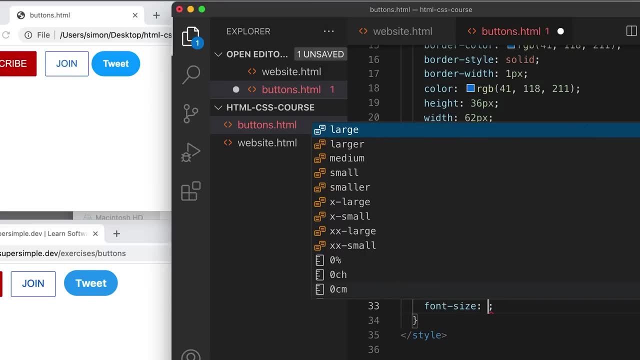 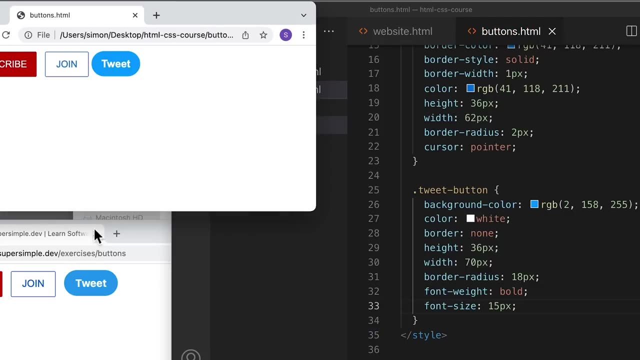 Okay, it looks pretty good. It looks like this font is actually a little bigger than ours, So let's actually set the font-size. Set it to maybe 15.. Let's see how that looks. Save and refresh. Okay, I think that looks pretty close. 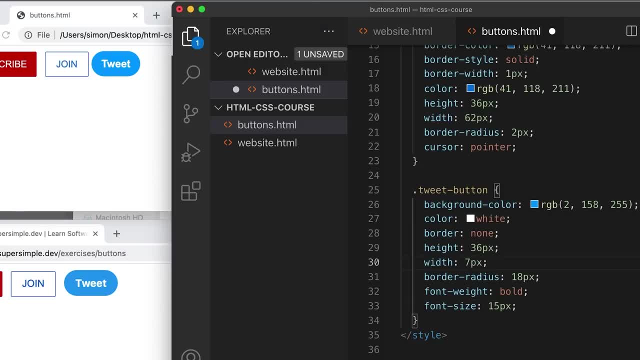 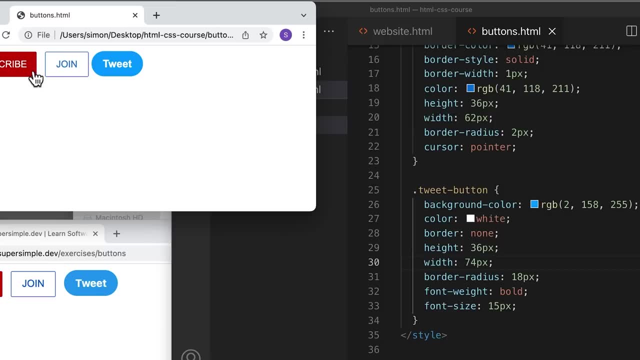 I'm going to change the width to maybe 74.. See how that looks. Okay, so I think this is good enough. Currently we're just trying to copy things by eye. Later I'll show you a technique of how to copy these colors and measurements exactly. 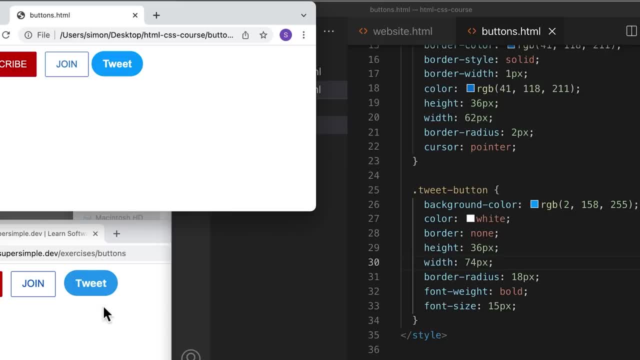 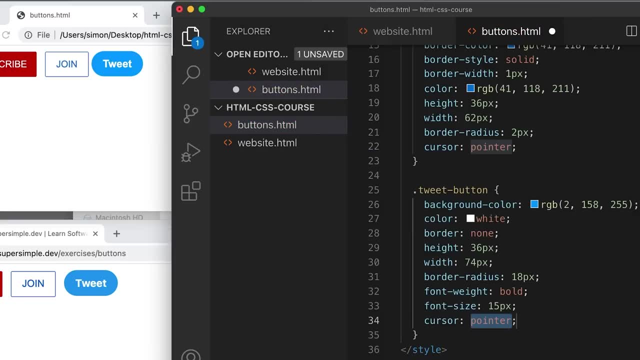 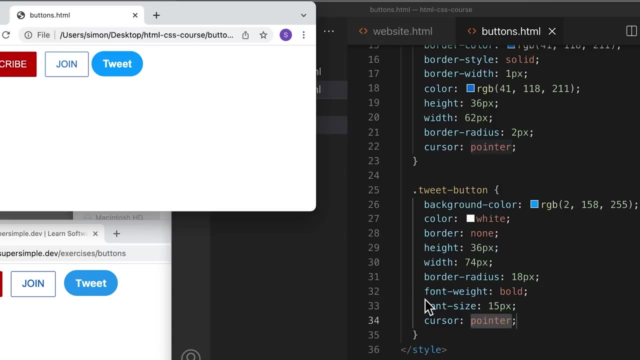 But for now it's good enough to be able to achieve these designs just by looking at them. So the last thing for this button is to add the cursor pointer. Let's save it and refresh. So if we hover over this button, we now get a nice pointer for our cursor. 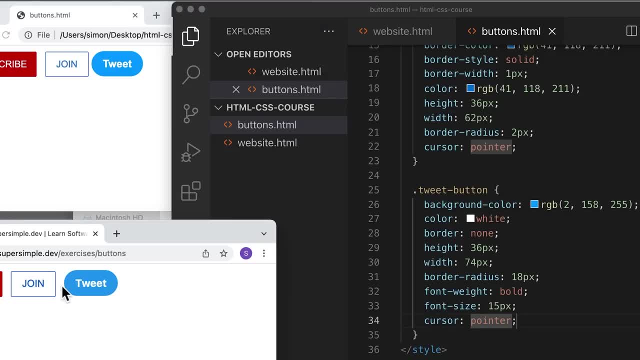 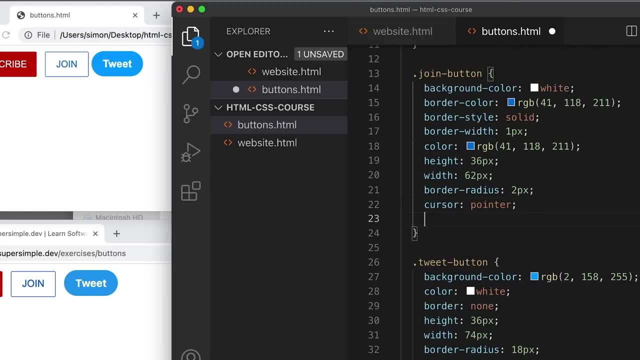 So the last thing I'm going to adjust here is the spacing between these two buttons. Remember, spacing in CSS is called margin. So we're going to add to the join button. Actually, let's add it to the tweet button, just for practice. 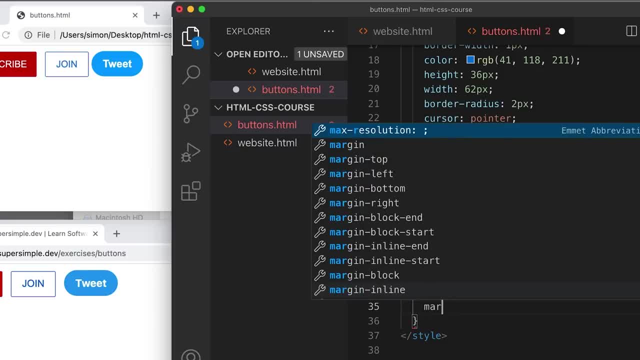 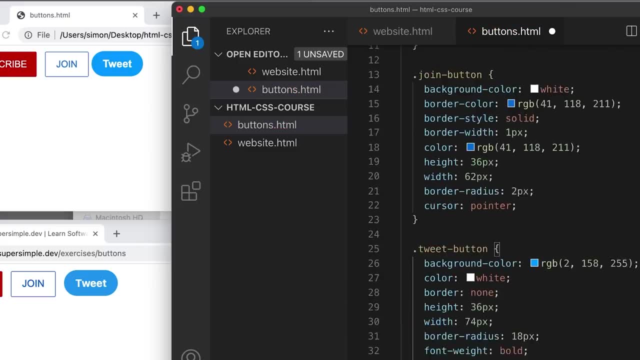 We're going to add spacing, So we're going to add margin to the left Colon And let's make it 8 pixels, like we had it for the subject, And we're going to add it to the subscribe button. Let's save it and refresh. 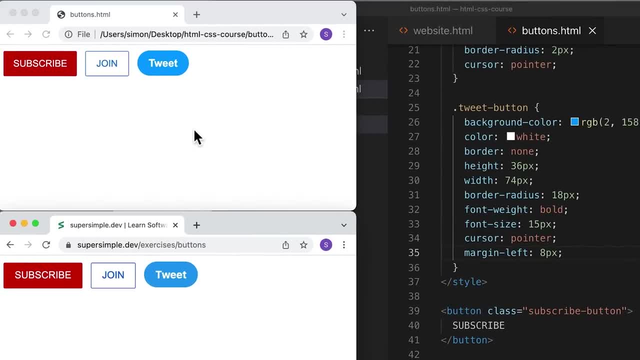 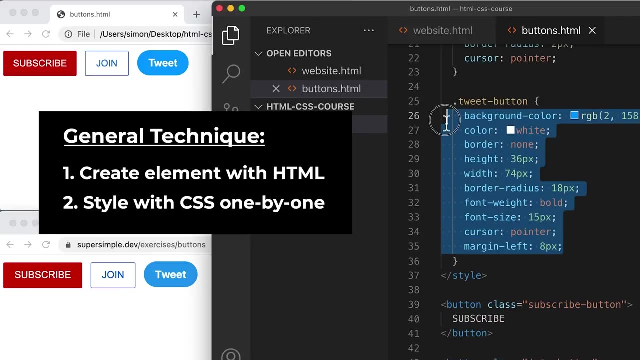 And there we go. So we took our basic buttons and we were able to copy these really nice looking designs just by looking at them. And the technique that we use for doing this is first we create the element with HTML and then we style it with CSS, one by one, until it looks close enough to our design. 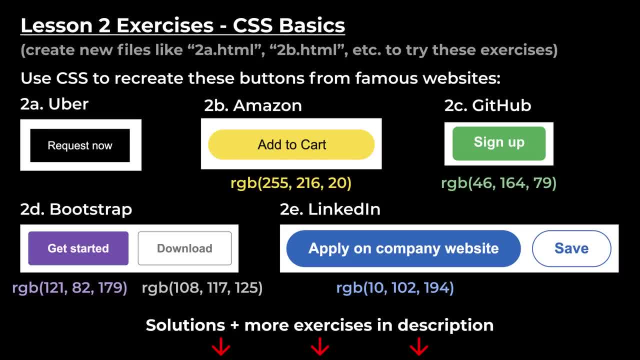 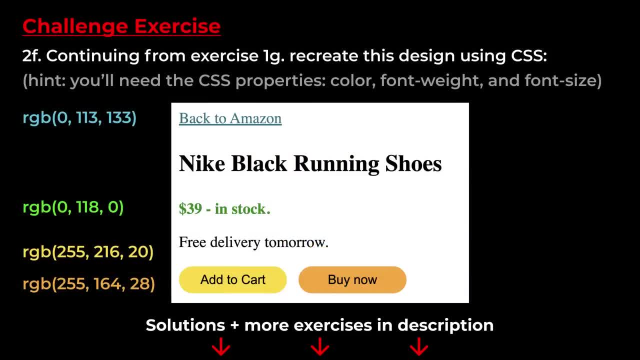 So here are our basic buttons. Let's go ahead and add them. So here are a bunch of exercises from other popular websites that you can try out for yourself. This is a good challenge for you: to be able to look at a website by eye. 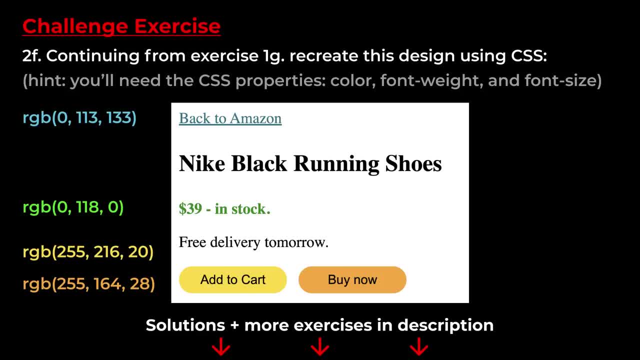 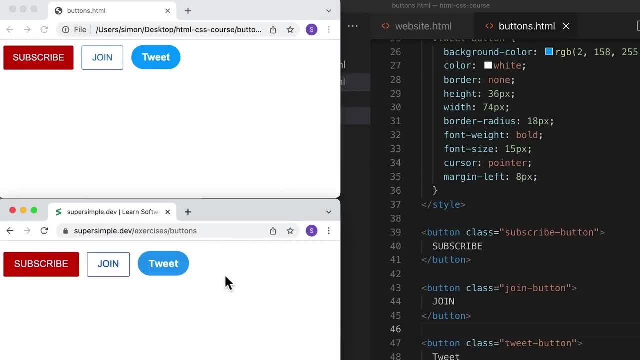 and use CSS to copy the styles that you see. In this lesson we're going to learn some intermediate CSS skills, such as how to create hovers, transitions and shadows For most buttons you see on the internet. if we hover over them with our mouse, they change their style slightly. 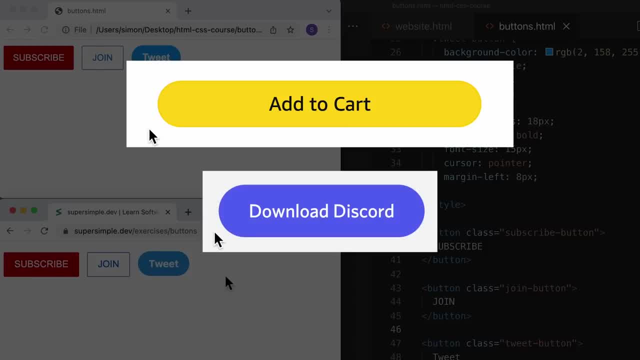 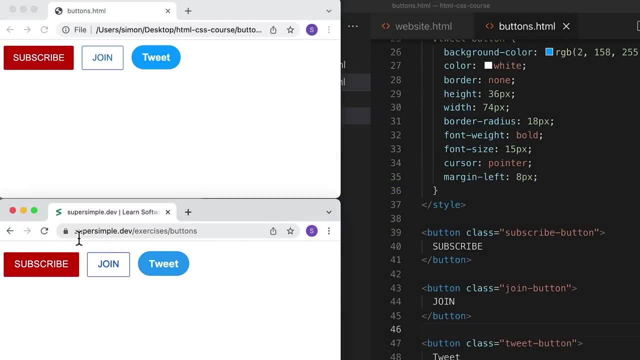 Some of them get darker, some of them get lighter. We're going to learn how to do that in our code, So we're going to use the same exercise as before. As a reminder, you can find it at supersimpledev. slash exercises- slash buttons. 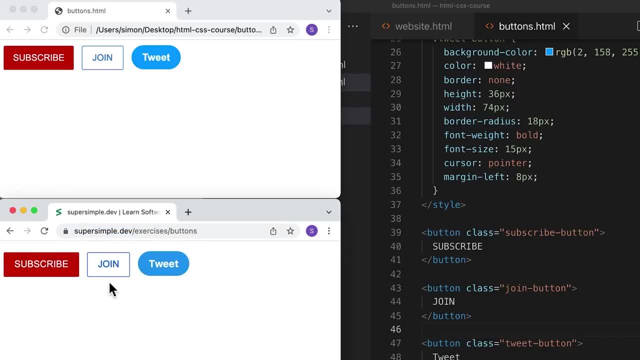 These buttons. when we hover over them, they actually change their style, So this is going to help us practice learning about hovers. In addition, you'll notice that if we hover in and out, they change their style smoothly, So we can also learn about transitions. 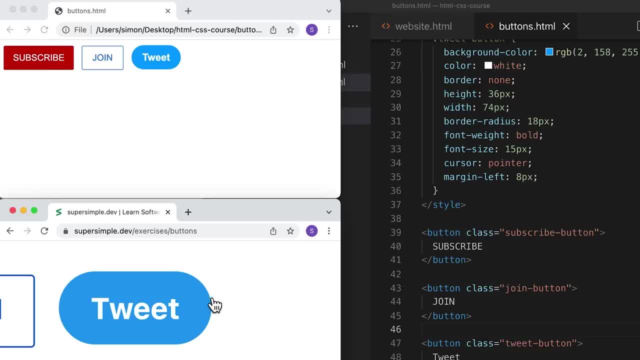 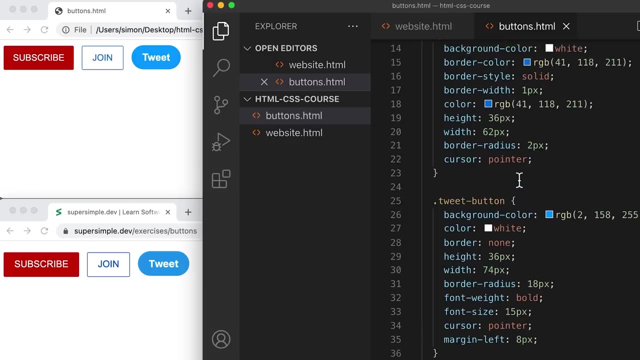 And lastly, this tweet button. if we hover over it it casts a little bit of a shadow, So that'll help us practice shadows. But first let's work on the hover styles for the subscribe button. Let's go into our code and find the styles for the subscribe button. 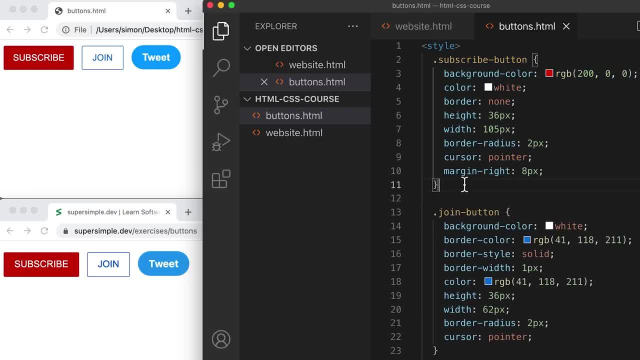 which is everything here And now. to create a hover effect, we're going to create a new block of CSS. We're going to use a dot to target a class. So this time we're still targeting the subscribe dash button, But this time we're going to add colon hover. 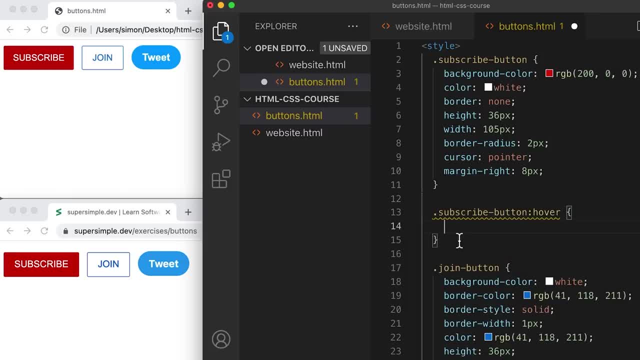 Open bracket, close bracket. So inside, these are styles that will apply only when we hover over the button. That's what this colon hover means. For example, we can set the background dash color to green. Now let's save our file and refresh the page. 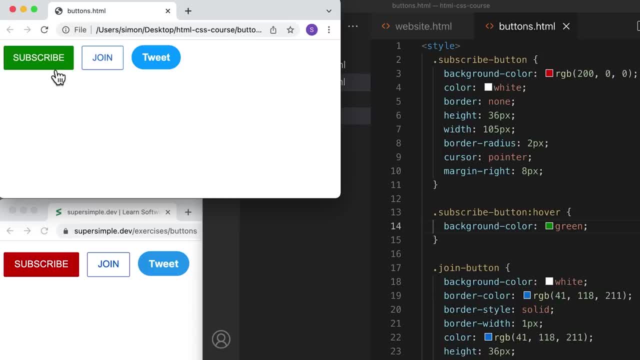 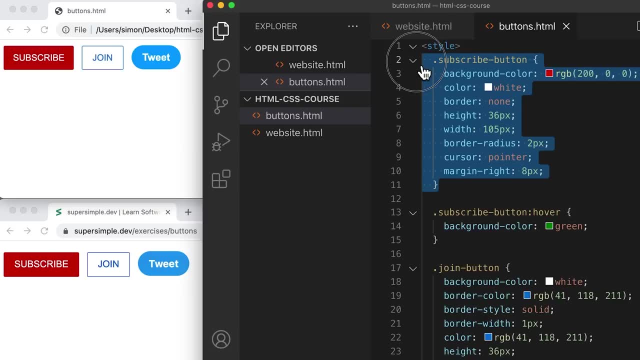 And when we hover over this button, you'll notice that it's green. So the way that this works is that if we are not hovering over, all of these styles apply. So the background color is red If we are hovering over the button. 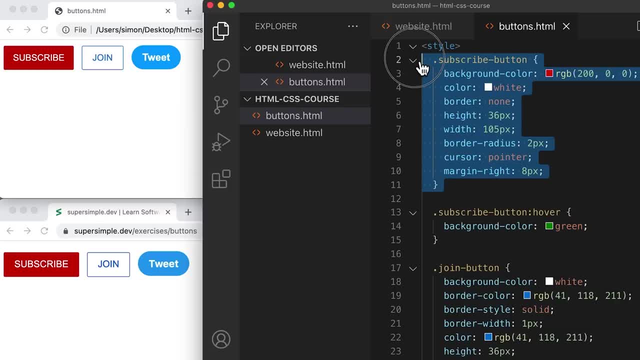 these styles now apply in addition to these styles. So we're essentially adding extra styles when we hover. So this colon hover is known as a pseudo class. It basically adds extra styles in a certain situation. So in this case it's going to add extra styles when we hover. 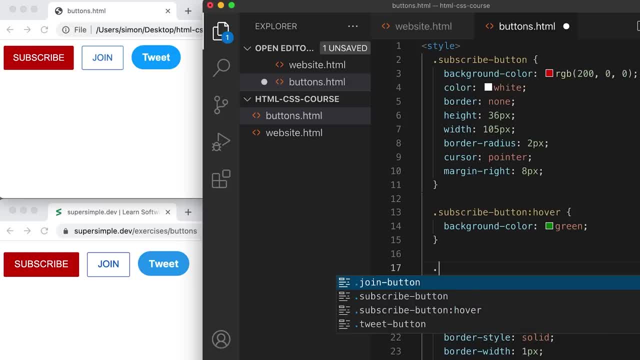 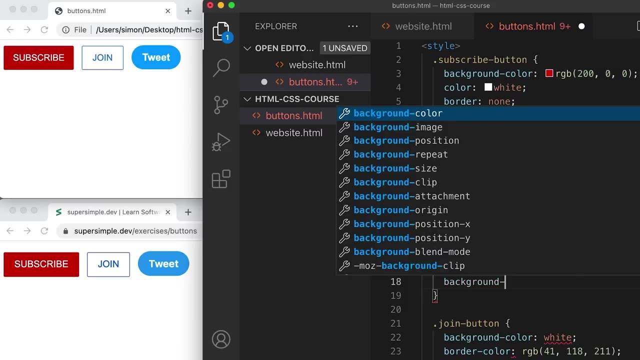 Another example of a pseudo class is dot subscribe button, colon active. So the active pseudo class activates when we click on the element. So when we click on the button we can set the background dash color to blue. Let's save this and refresh. 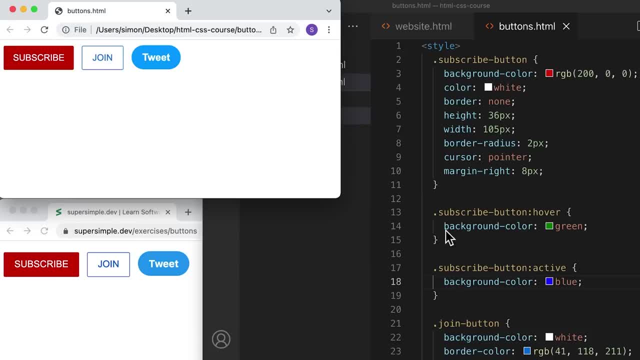 Now, when we hover over, we're going to apply these styles, So the background color is going to be green. And then, when we click, we're going to apply the active styles, And then the background color is going to be blue. So let's look at our design. 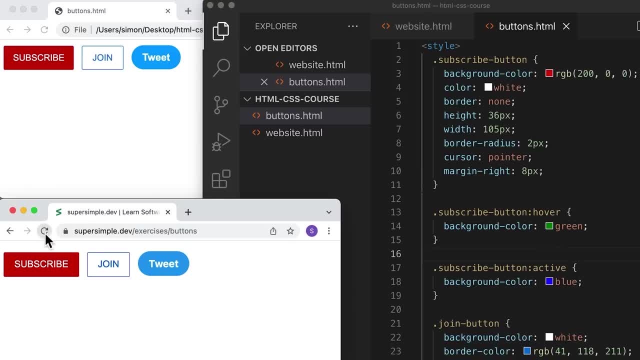 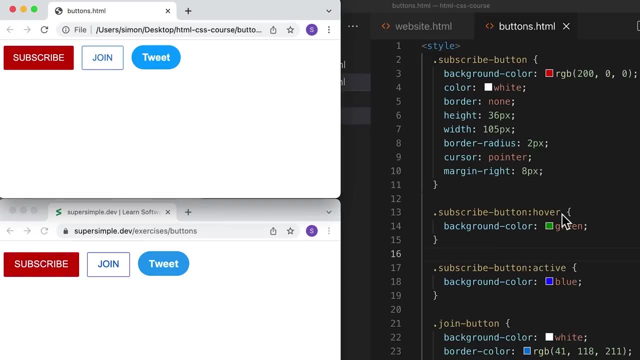 and see what kind of hover styles we have Refresh. So when we hover over our subscribe button, it seems to turn a little bit more light, And if we click it it becomes even lighter. So the way to make our button lighter is using a new property. 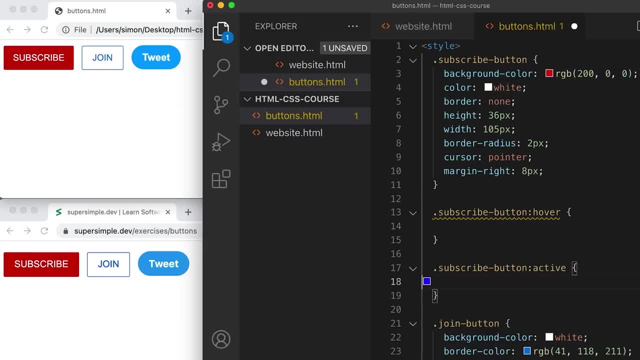 that I'm going to introduce. So let's get rid of these. for now, Let's save and refresh. So we got rid of those pseudo class styles. We're going to set a CSS property called opacity, So opacity tells us how see-through an HTML element is. 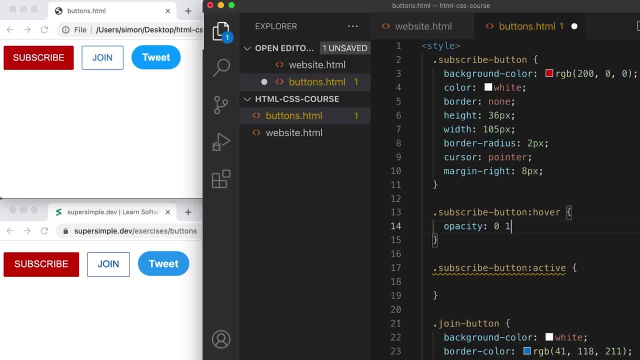 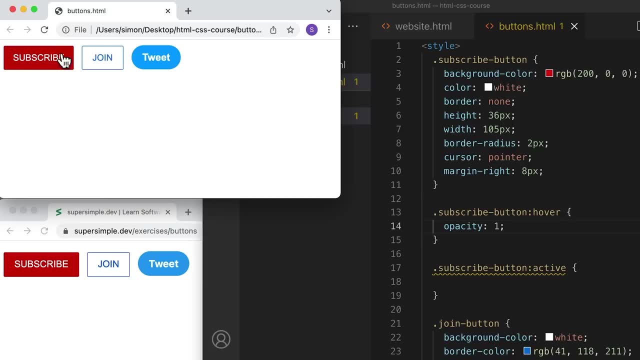 It takes a value between 0 and 1.. A value of 1 means that this element is completely normal. So if we save this and refresh, you can see that if we hover over it, it's completely normal. And as we decrease the opacity, 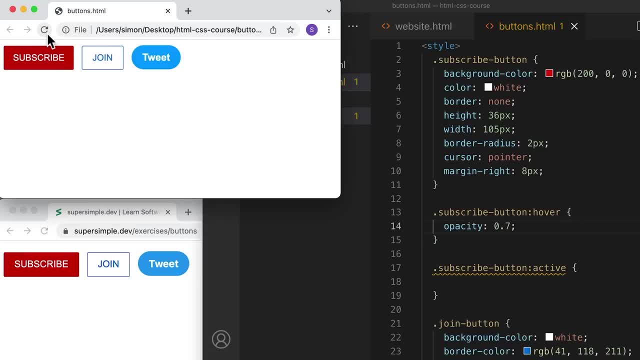 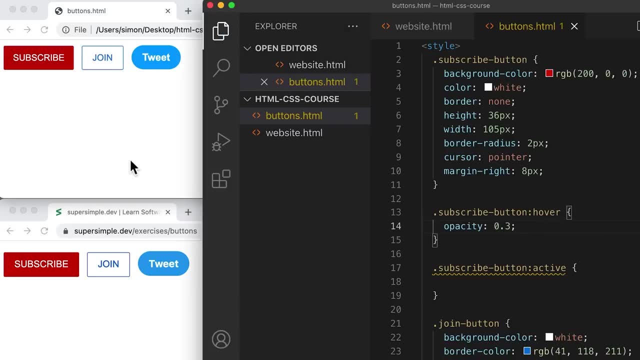 let's decrease it to 0.7, the element starts to fade. So if we decrease it even more to 0.3, refresh now- it's even more faded. So the opacity is used to fade out an element. If we go from 1 to 0,. 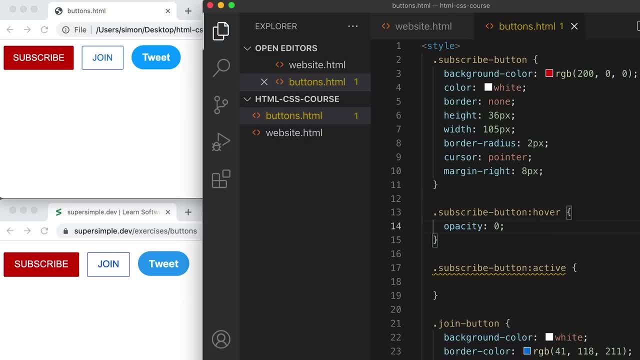 the element is going to fade out. So if we set it to 0, refresh. now. it's basically completely transparent and see-through. If the opacity goes from 0 to 1, that means the element is going to start to fade in. 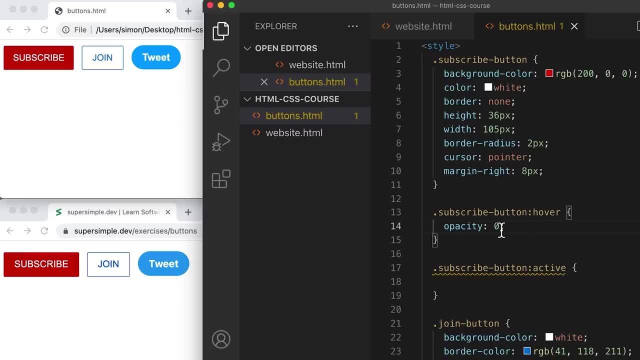 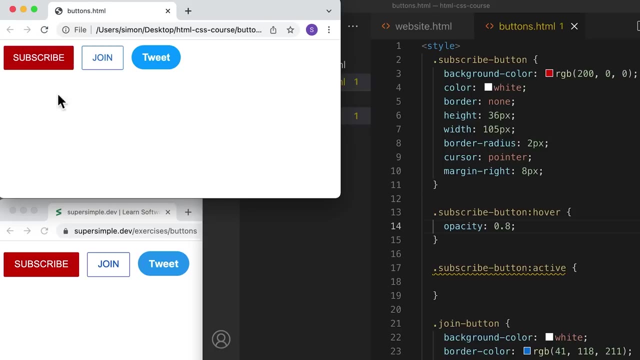 So that's how opacity works For now, if we hover over it, let's set the opacity to maybe 0.8.. So it's going to be a little bit see-through, but not totally see-through. So let's refresh and hover over it. 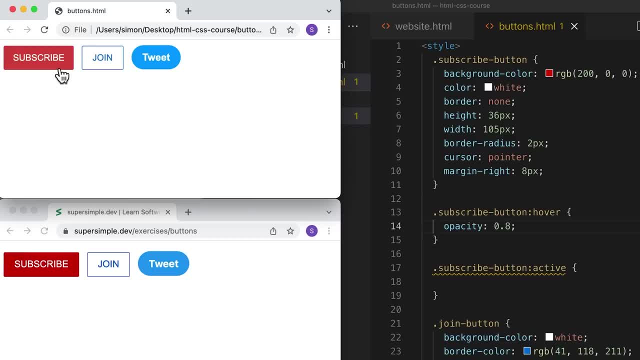 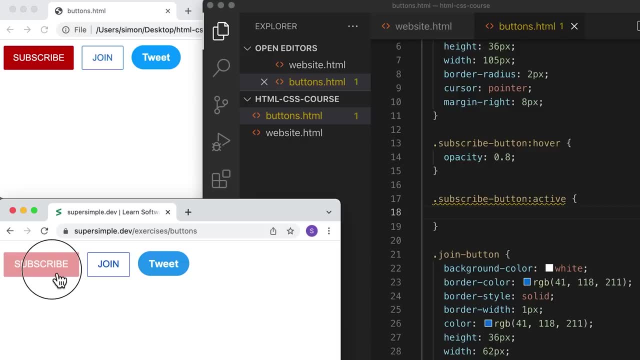 Okay, let's look at our design. So that looks pretty close to what we have. Next, let's set the active styles. So in our design, if we click on this, it gets even lighter, So we're going to set an even lower opacity. 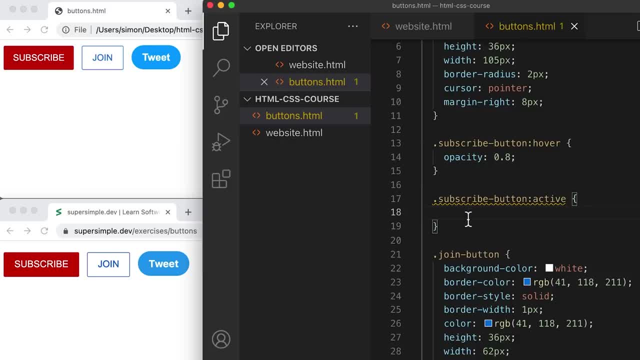 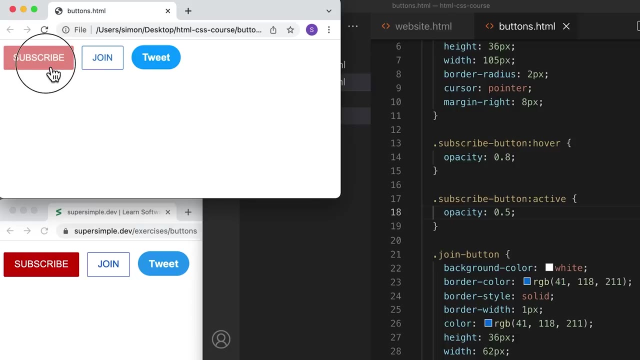 to make our button fade out even more when we click on it. Let's set it to something like 0.4.. Or 0.5, let's say, Save it and refresh Now when we hover over it, now when we click. 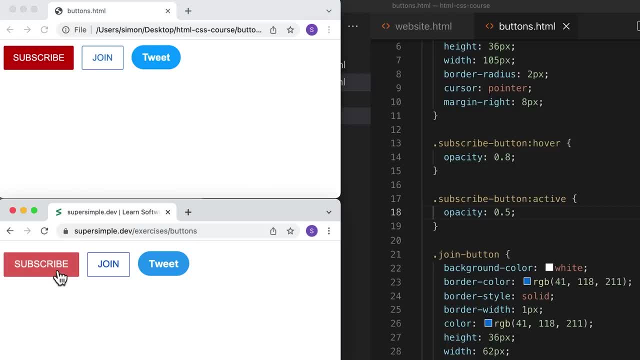 the button gets lighter And we can compare that to our design And that looks pretty good to me. Now we're going to work on the hover styles for our join button. So if we look at our design, the colors for this join button sort of inverts. 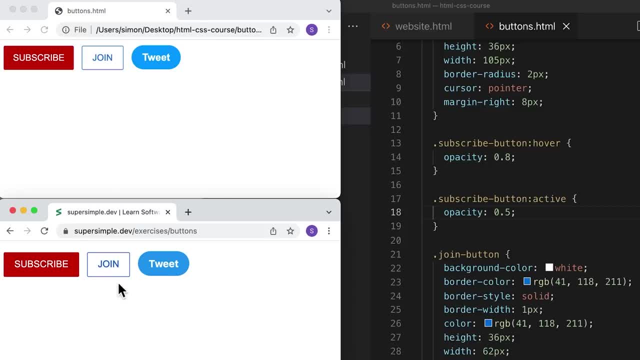 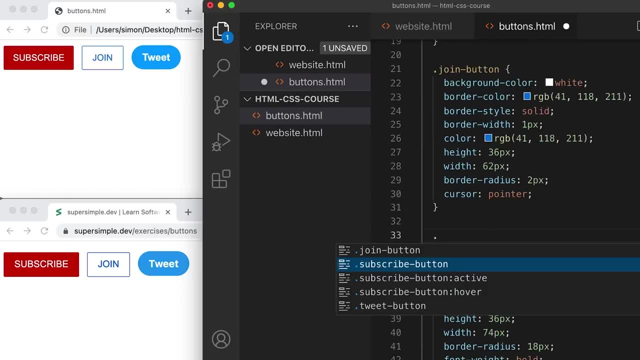 So the background color and the text color they reverse. So to do that, we're going to go into our code And again we're going to target the join button with a dot join button And we're going to add a pseudo class. 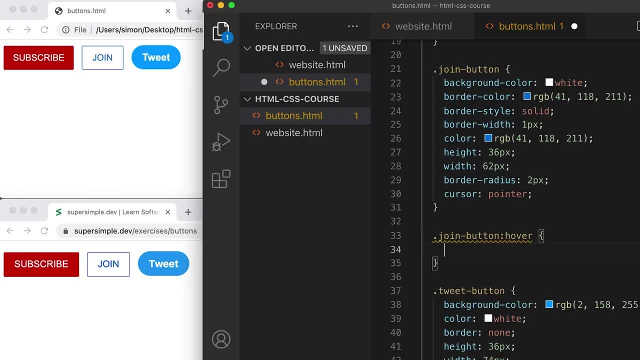 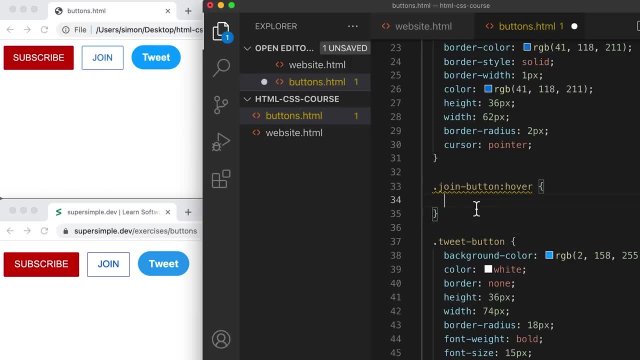 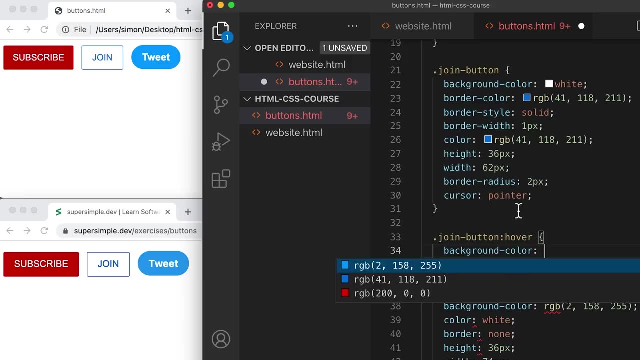 called colon hover, And now all the styles inside here will apply when we hover over this button. So when we hover over it, we want to invert the colors. So we want to set the background dash color to our text color, which is this: 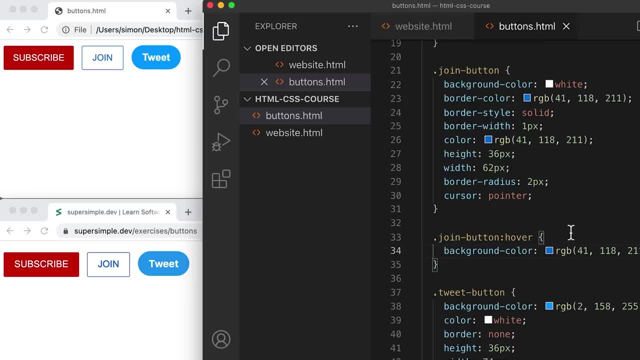 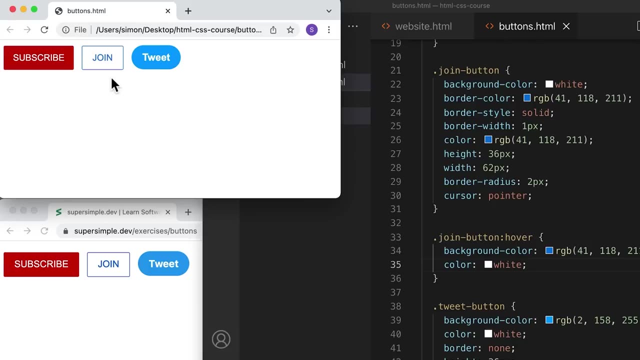 Copy and paste. And we also want to set the text color to our background color, So we're going to switch them up: Copy and paste here, Save it And refresh. And now, when we hover over our join button, that looks pretty good. 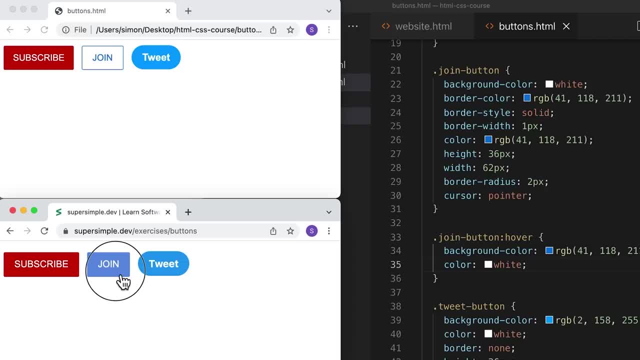 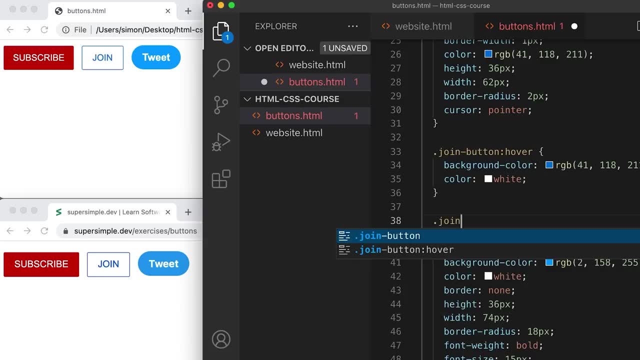 The next thing is, when we click the join button, you'll notice that it also fades out. So we're going to add an active pseudo class to this button as well. So target the join button class and add a pseudo class called active, So these styles will activate. 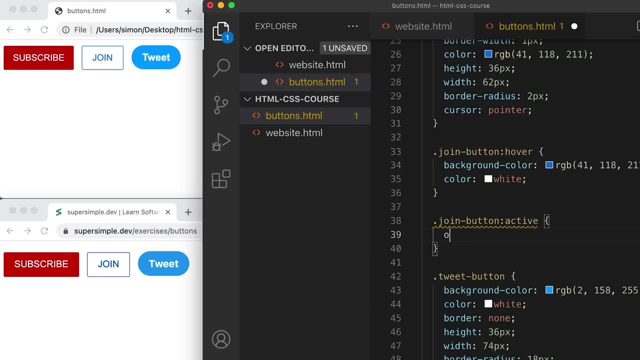 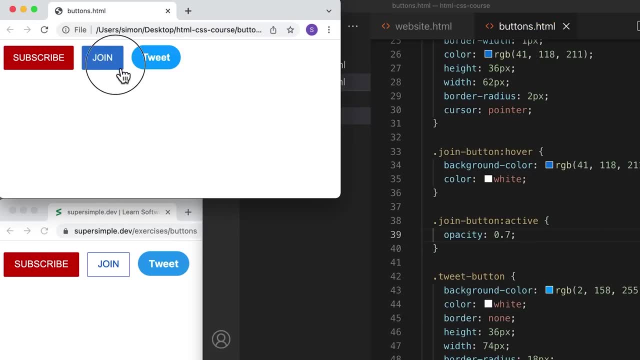 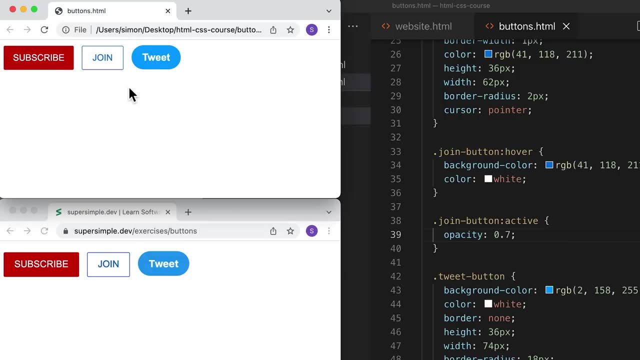 when we click this element. So let's set the opacity to maybe 0.7, maybe Save it, Refresh, Click it. Okay, So I think that looks close enough. So 0.7 looks pretty good. So that is how we set hover styles. 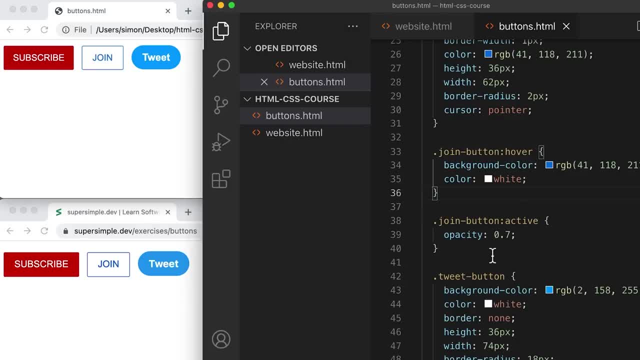 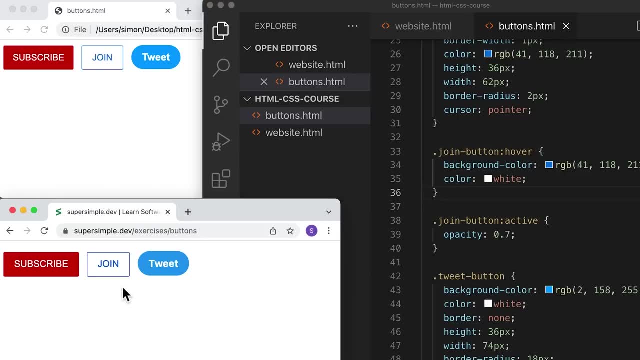 and other pseudo classes with our CSS code. Next, we're going to learn how to transition smoothly between these two styles. So, for example, if we go back into our project and we hover over this button, you'll notice that the background color and the text color change. 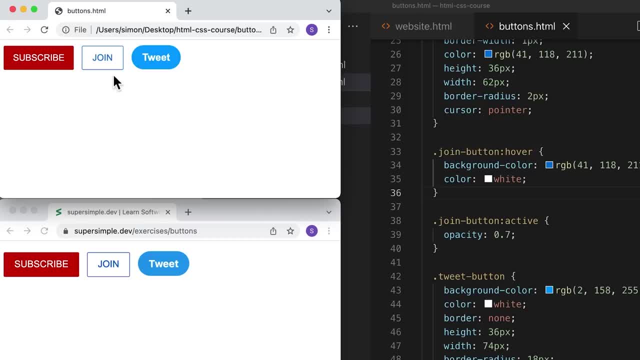 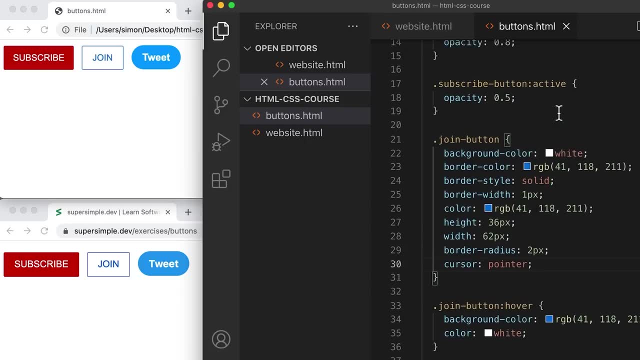 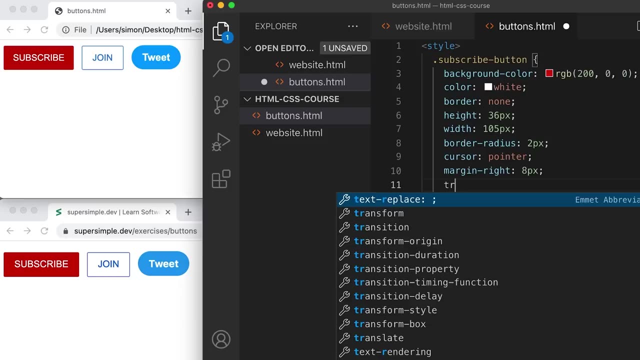 smoothly, But for our colors it changes almost instantly. So how do we make this transition? So to do that, we're going to scroll up to our subscribe button first. We're going to add a property called transition. So transition property takes. 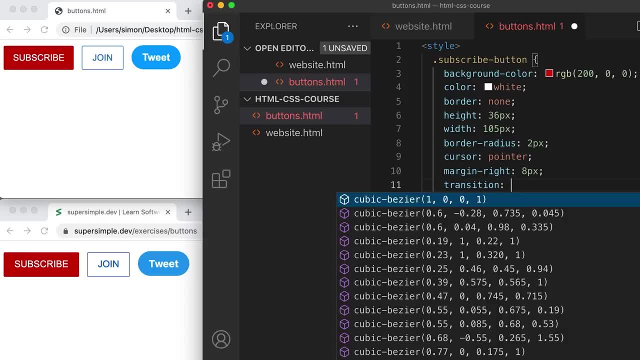 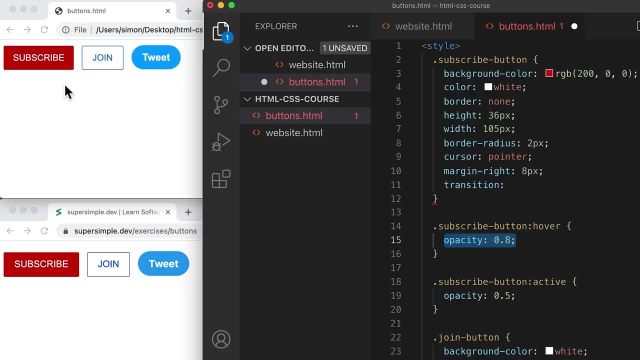 two values. The first one is what we want to transition. So in our case, we want to transition the opacity smoothly. So we want to smoothly fade out the button when we hover over it, instead of instantaneously. So let's transition the opacity. 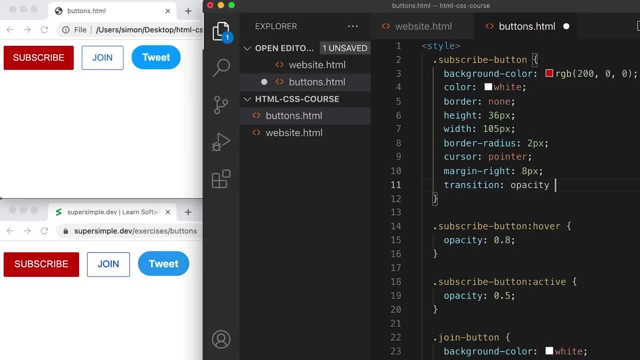 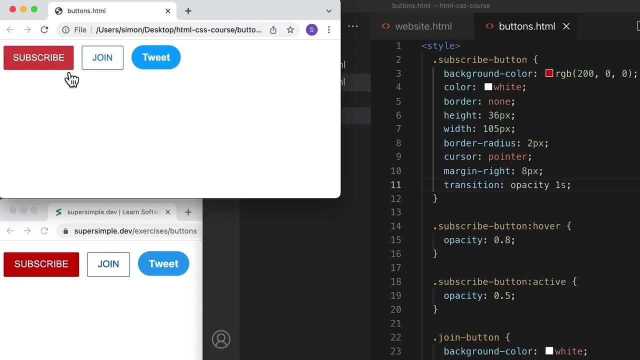 And the second value is how long this transition will take. For example, let's set it to 1s, which is one second, End it with a semicolon and save. Let's go back and refresh. And now, when we hover over our button, you'll notice. 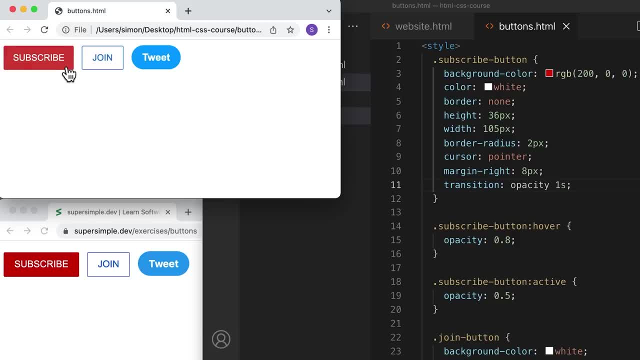 that the opacity changes smoothly. Now it might be a little bit hard to see, so let's change this to 0.1 to show you the effect. Refresh. So now you can see that the opacity is changing smoothly over one second. So this is how you transition between. 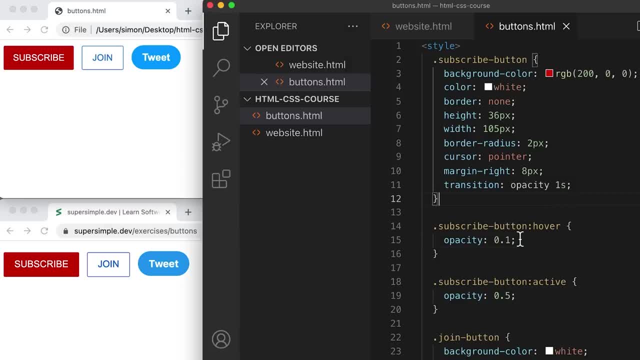 different styles when you're hovering over them. Now let's set it back to 0.8 and we're going to change one second because it's a little bit too long. So usually a good transition duration is something like 0.15 seconds. 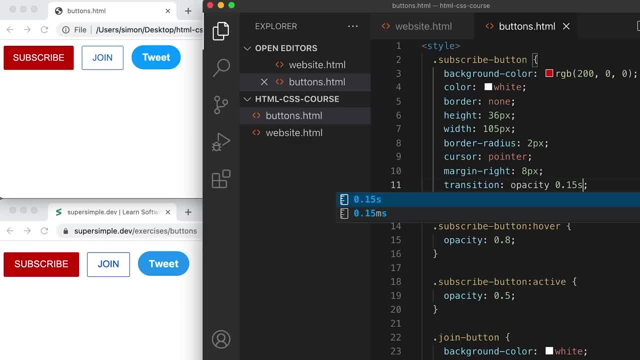 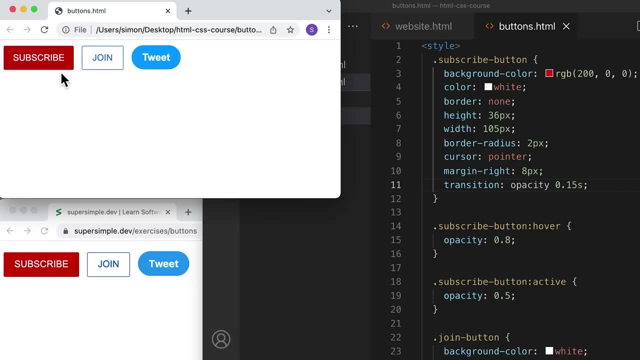 So it's pretty fast, but it's not too fast and it's not too slow. Let's go to our webpage and refresh. Now, when we hover over it we get a nice smooth transition. It might be a little bit hard to tell, but we do get a nice. 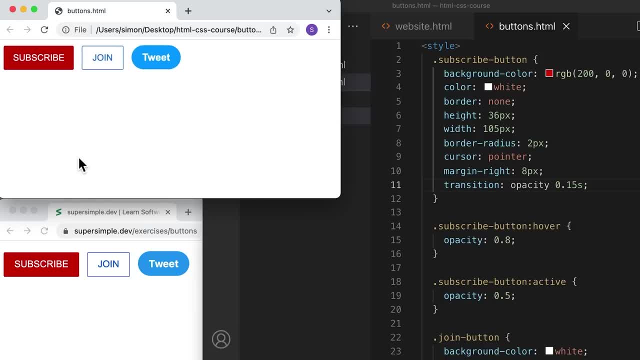 smooth transition instead of what we had before, which transitioned immediately. Let's work on the Join button now, So this one is a lot easier to see the difference. Let's scroll down to the Join button and again we're going to add a. 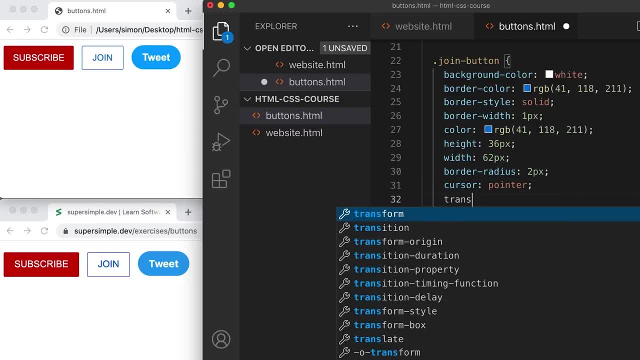 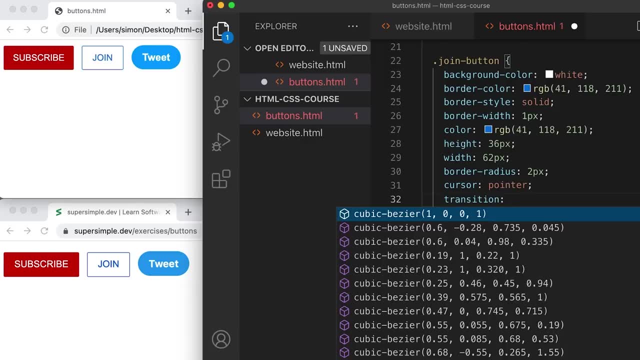 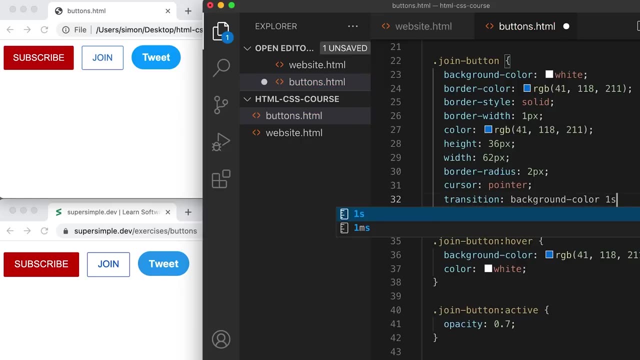 transition. So we're going to add transition and we're going to give it two values: What we want to transition and how long. First, let's transition the background-color and how long we're going to transition for one second. as an example, Let's save our file. 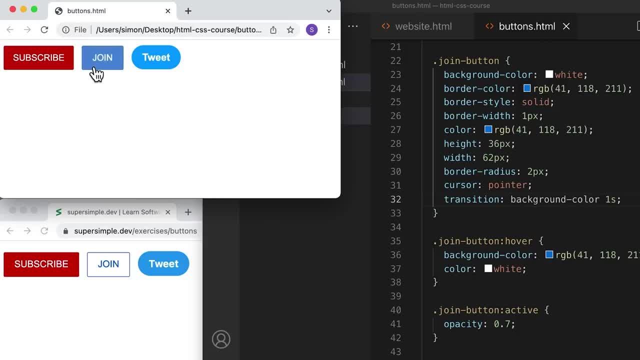 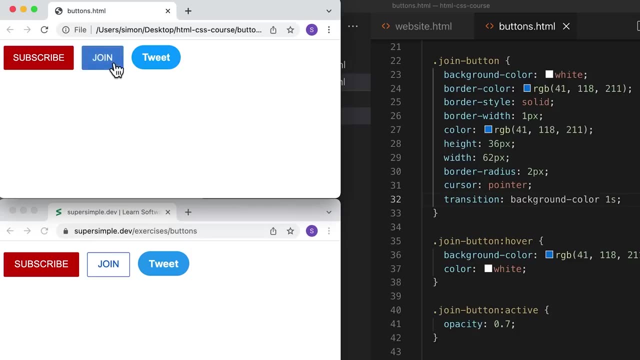 and refresh. Now, when we hover over the Join button, the background-color changes smoothly over one second, But you'll notice that the text-color changes immediately, whereas the text-color here also kind of transitions. So to make the text-color transition as well, we need to add another. 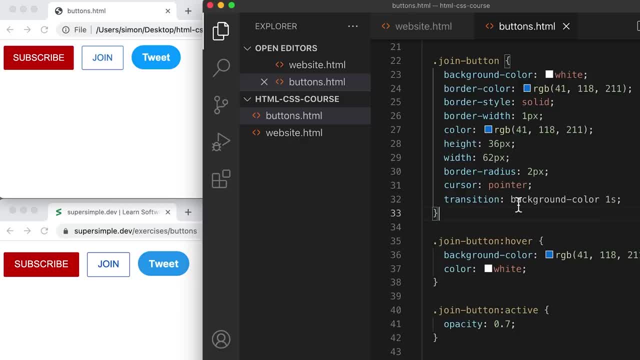 property to transition So we can actually transition multiple properties. we just have to separate it with a comma. So if we have a comma here, we can add another property to transition. This time I'm going to transition the color and we're also going to give it a. 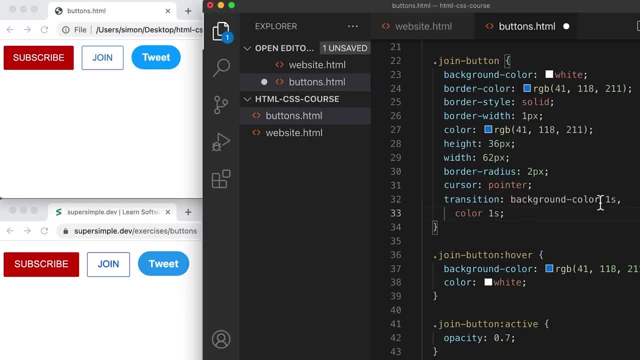 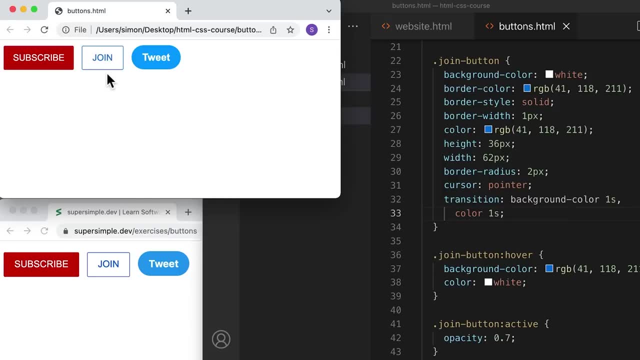 duration, which is one second. So how long it takes to transition this property, Save it and refresh. Now, when we hover over this button, it will transition both background-color and the color smoothly over one second, And that's basically how transitions work. So sometimes you 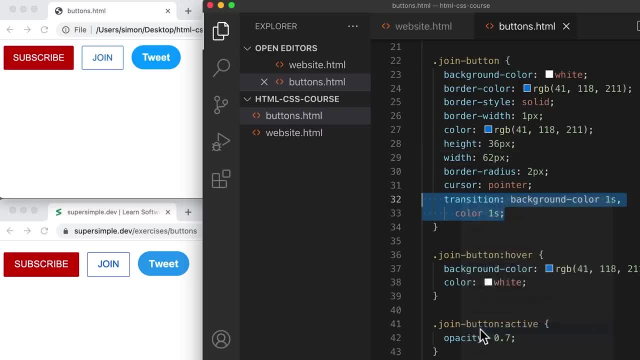 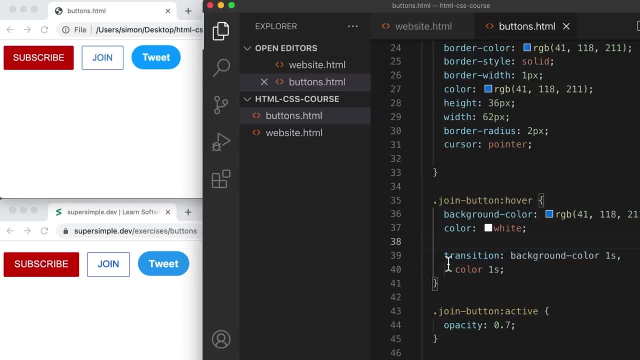 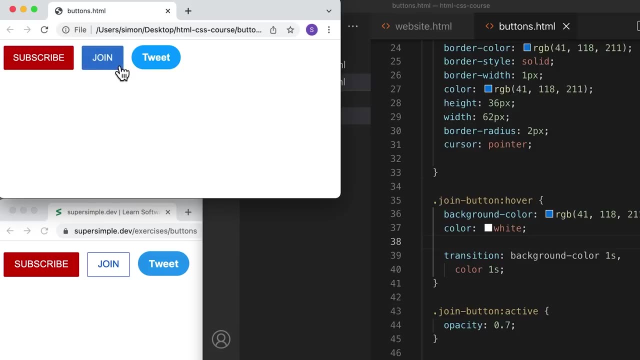 might be tempted to put this transition property into the hover, Because you think that we want to transition when we hover, So we have to put it here Now. the problem with this is that if we refresh when we hover over the button, everything looks good, But as soon as we hover, 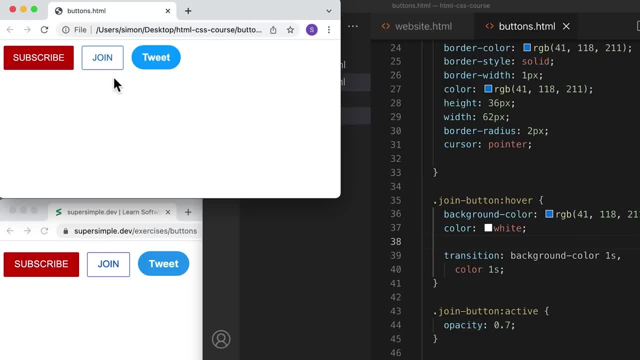 out. these styles change immediately And that's because, remember, these styles only apply when we're hovering. So if we are hovering, then we have a transition, But as soon as we take off the hover, it's the same thing as having no transition at all. 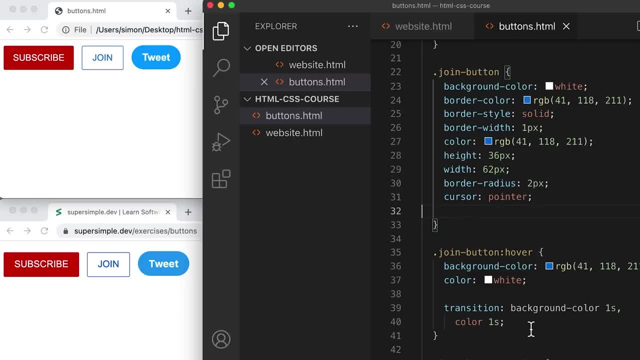 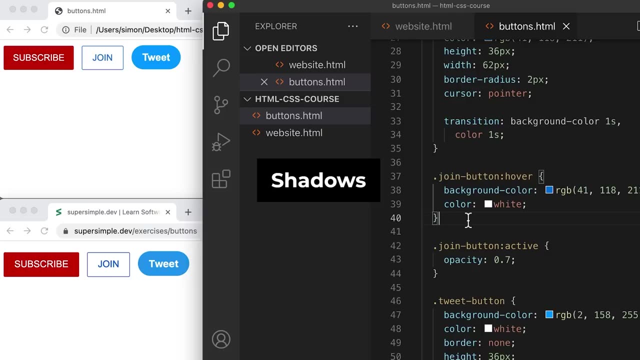 That's one common pitfall of the transition property, So let's move it back here where it should be. Just make sure that you put the transition always in this sort of base CSS style. The last thing we're going to learn in this lesson is how to create shadows. 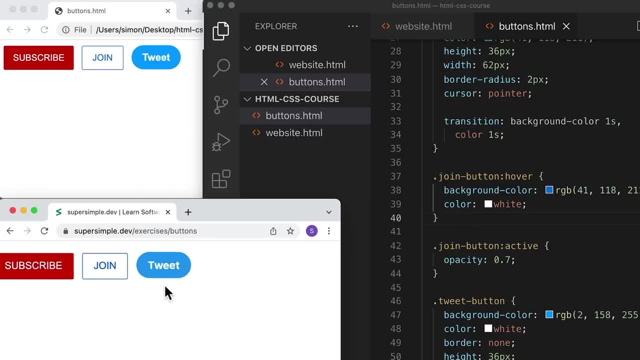 If we go to our project and we look at our design- I'm going to zoom in here- When I hover over the tweet button, it creates a faint shadow under the button. We're going to learn how to create this, So let's zoom out for now. 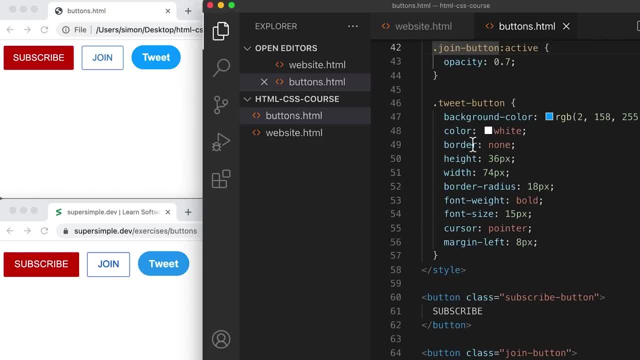 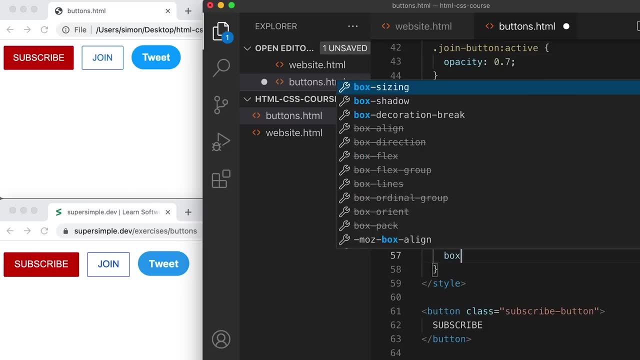 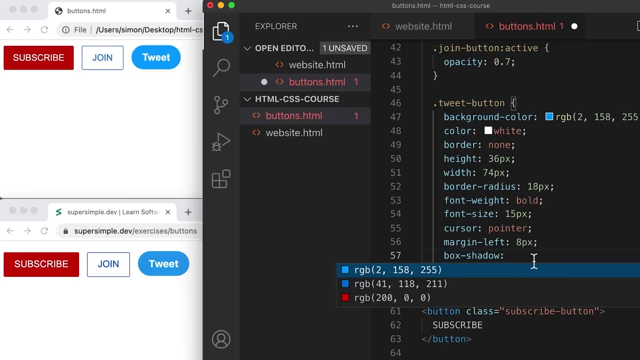 We're going to go down to the tweet button styles, and the shadow is just another CSS property. So the property for a shadow is box-shadow colon. Now, box-shadow actually takes four values, So I'm going to set the values to zero. 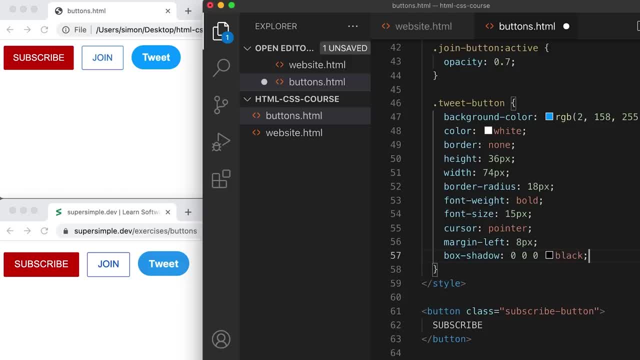 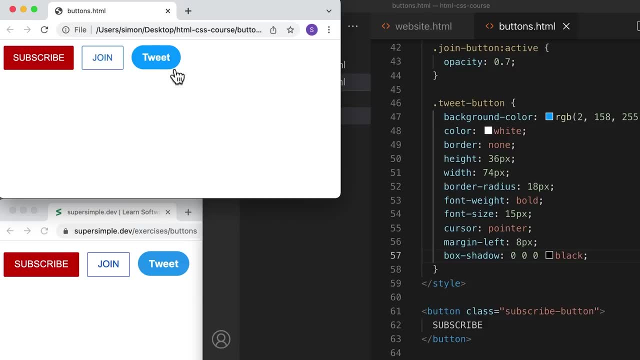 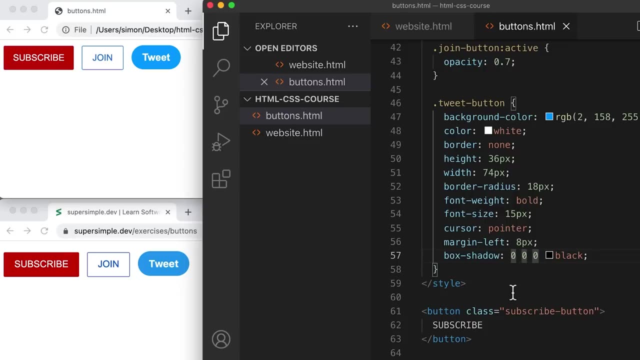 for now, and then we're going to change them one by one to see how they work. Let's save this and refresh. And now we do have a shadow, but we can't see it because it's right underneath the button. So the first value here determines the 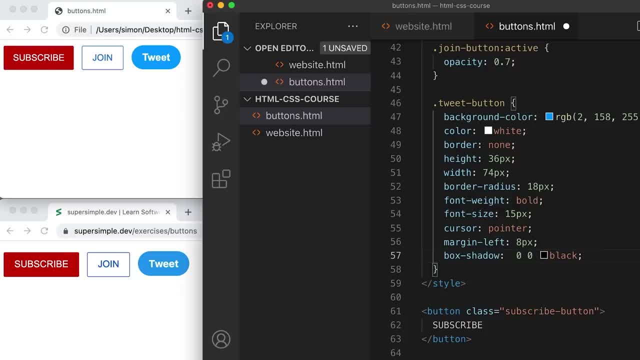 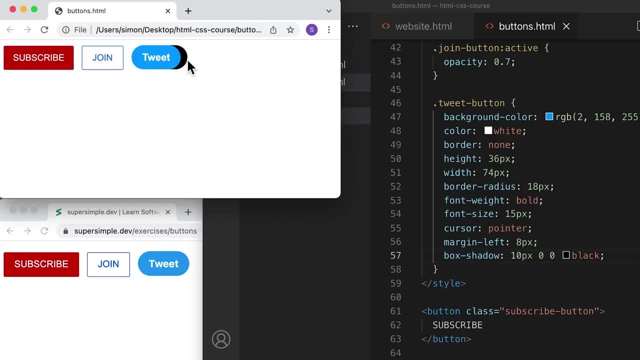 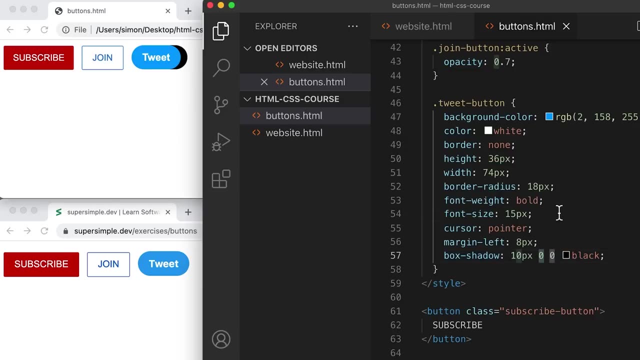 horizontal position of the shadow. For example, I can set it to 10 pixels and if I save, the shadow will appear 10 pixels to the right. The second value sets the vertical position of the shadow, For example, if I set it to. 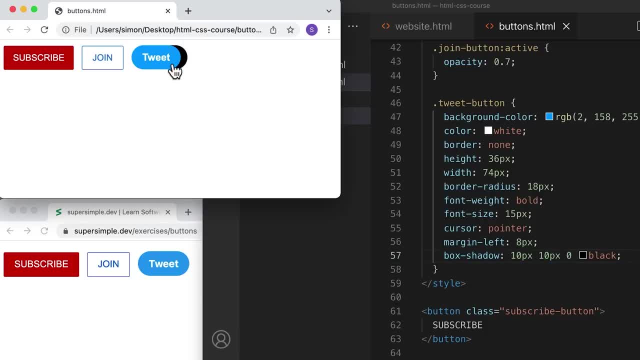 10 pixels in the second value, it will push it 10 pixels down. So now you can see we actually do have a shadow: 10 pixels to the right and 10 pixels down from the button. Now the third value here is the blur. 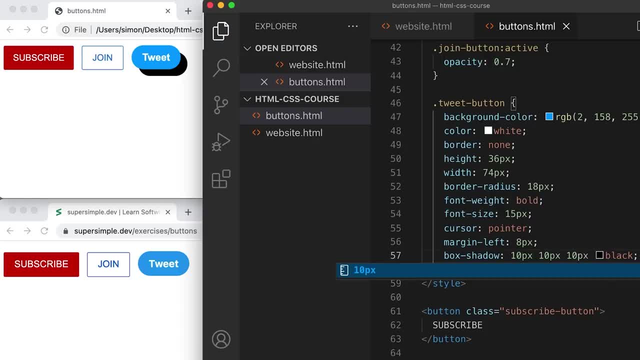 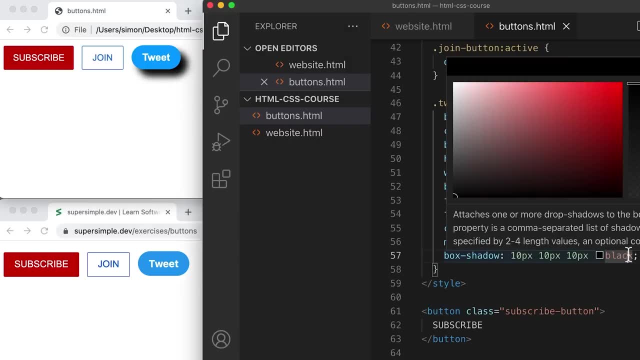 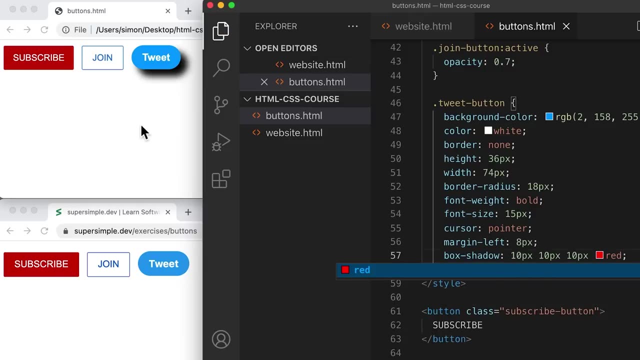 So if we set the blur to maybe 10 pixels, save refresh. now the shadow becomes blurred And the last value is obviously the color, So we can actually change it to whatever we want. We can actually change it to something like red. 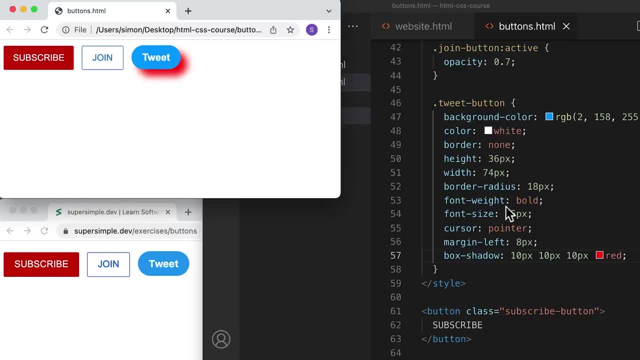 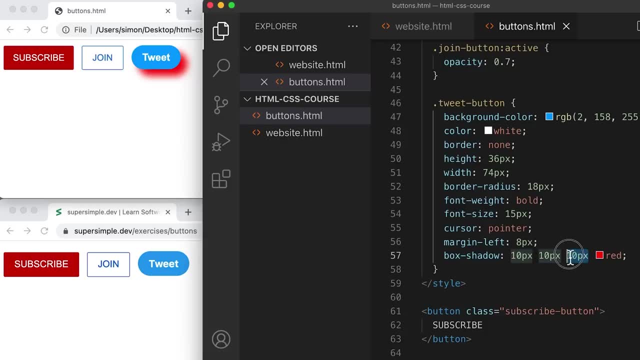 Save it, refresh and we get a red shadow. So this is basically how shadows work. We have a horizontal position, a vertical position, blur and color. So don't worry, the more that you work with shadows, the more you'll get familiar with. 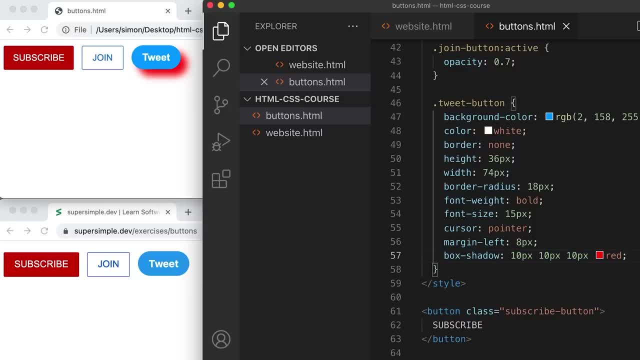 what these four values can do. So let's try creating a more realistic shadow. Usually, shadows aren't red or any color. They're usually kind of a darker shade of whatever they're covering. So to create a color like that, we're going to need a. 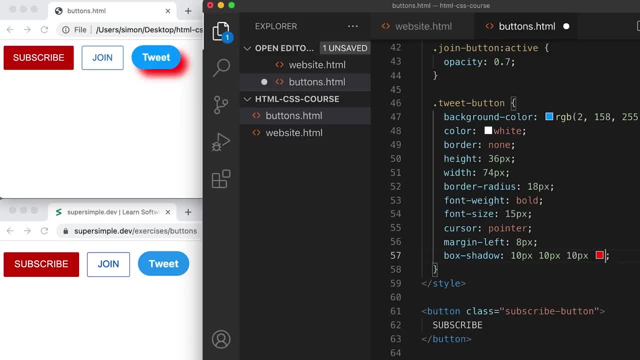 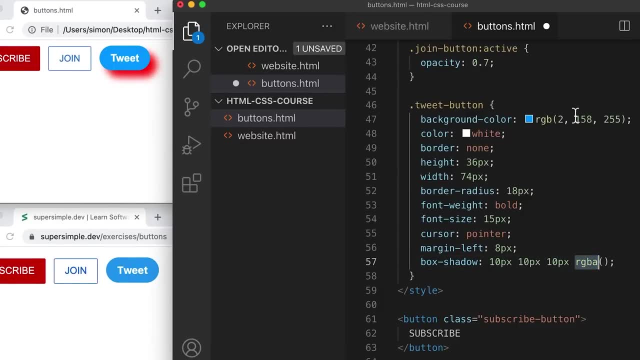 new way of measuring color. So let's get rid of this and we're going to use something called RGBA. RGBA is the same thing as RGB, except there's an A value. So this A value essentially means the opacity of the color. how? 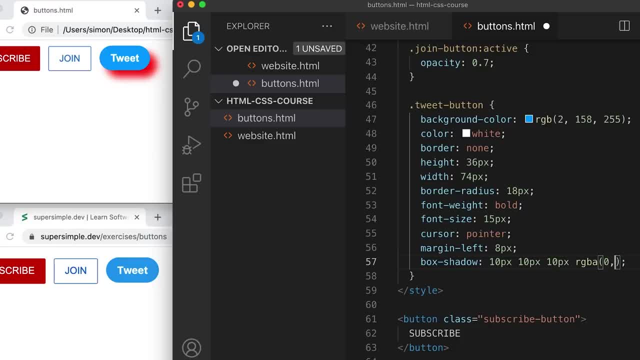 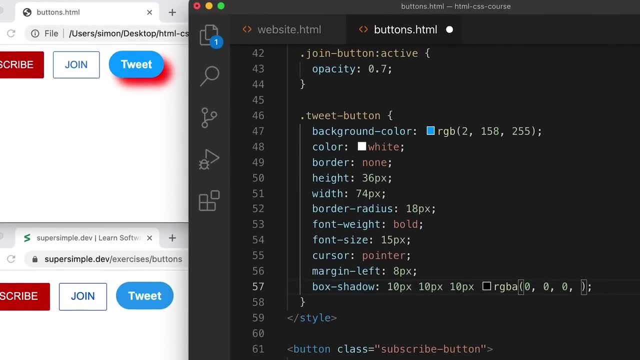 see-through it is. You can set the RGB to 0, 0, 0.. That gets us to black, as we learned. And then the fourth value is our A value If we set it to 1, and save. 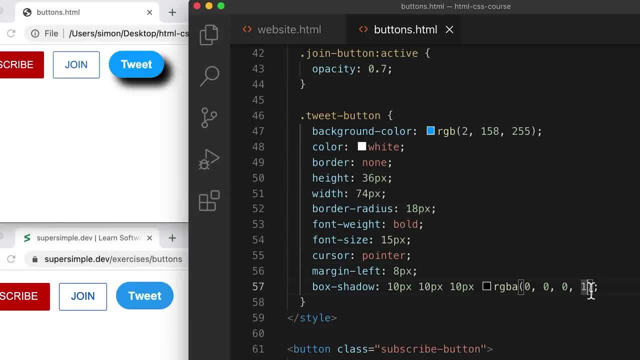 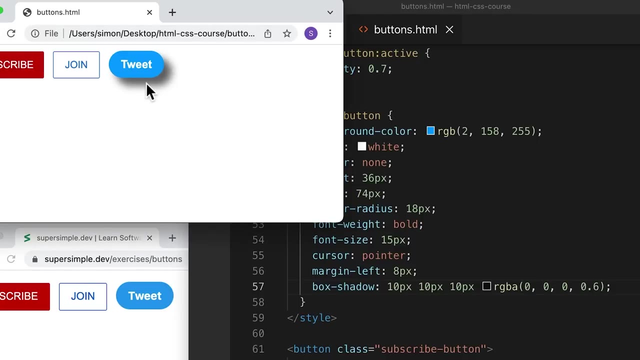 this is going to be pure black, But as we decrease the A value, the color is going to get more and more faded out and more and more transparent. So if we decrease it to 0.6, save and refresh now, this color is getting more. 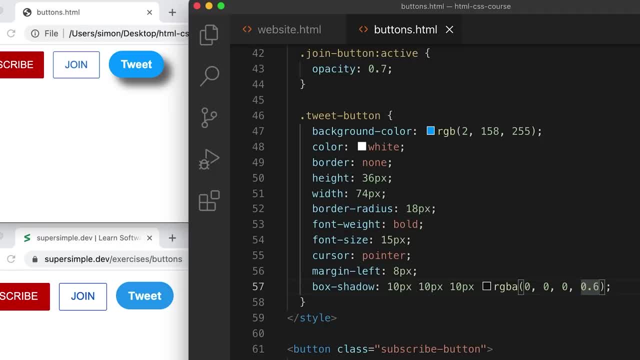 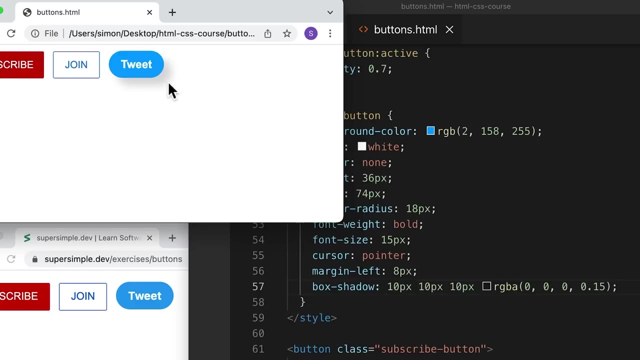 transparent and faded out. So a pretty natural color for a shadow is something pretty faint like 0.15.. So for shadows we usually don't want it to be too noticeable. Shadows are best when they're very subtle, And now we kind of want to. 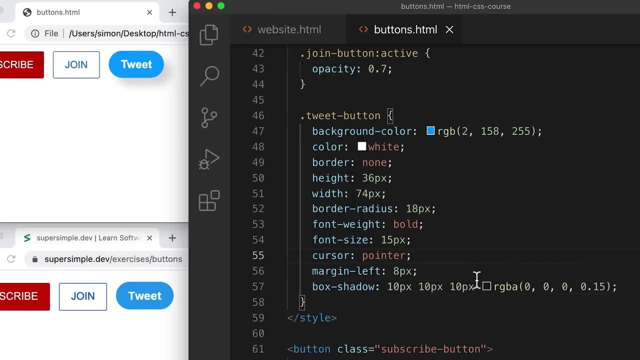 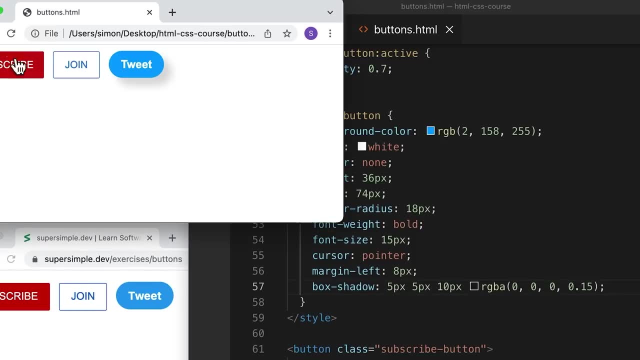 move the shadow a little bit closer to the button so it looks a little more natural. So let's actually move it, maybe 5 pixels and 5 pixels, Let's see how that looks. Save it and refresh. I think that looks pretty good. 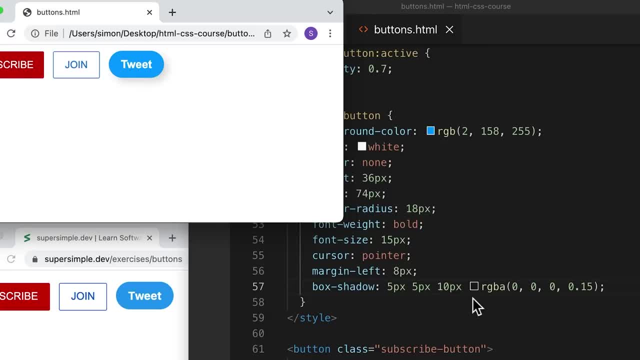 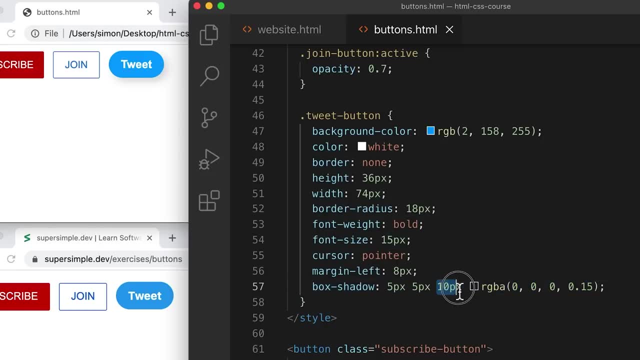 So that's how we create a natural looking shadow. with the box shadow property, We have 4 values: the horizontal position, vertical position, the blur and the color measured with RGBA. The A value means opacity, or how see-through this color is. 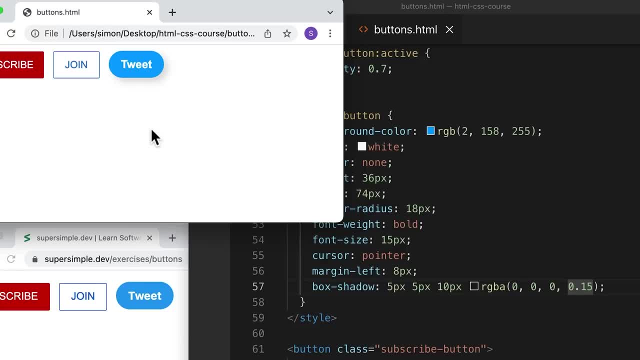 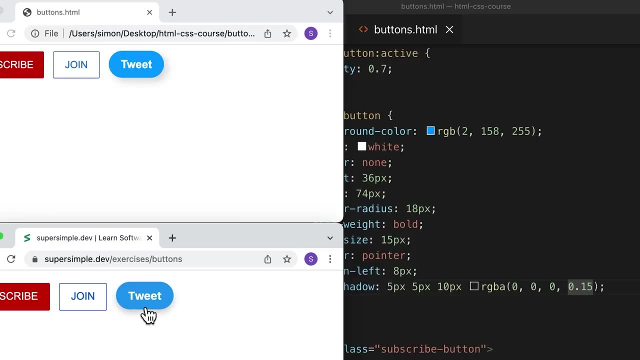 The final step of this lesson is to only make this shadow appear when we hover over the button. So for example, for here, if we hover over, we can see the shadow. If we're not, the shadow's gone. So this is another style. 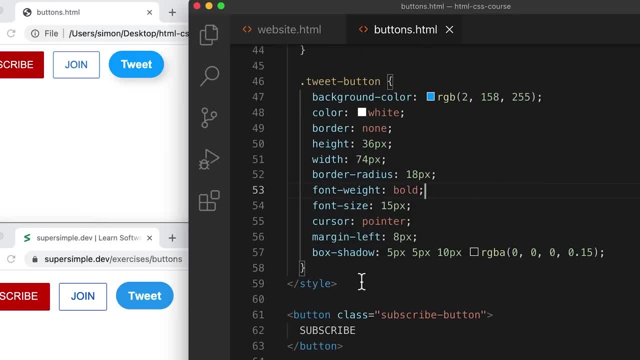 of button that we can create. So let's use what we learned so far. Remember: we first use a dot to target the class. So we're going to target the tweet-button class. We're going to add a pseudo class here called hover. 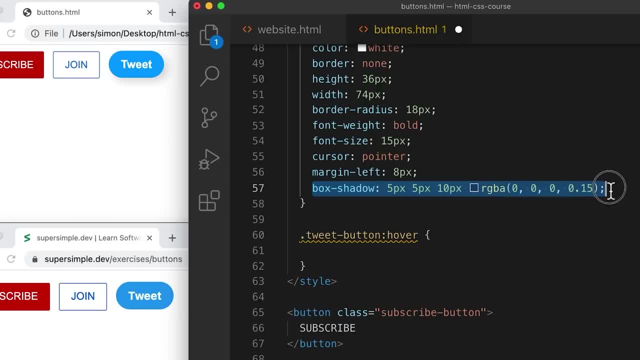 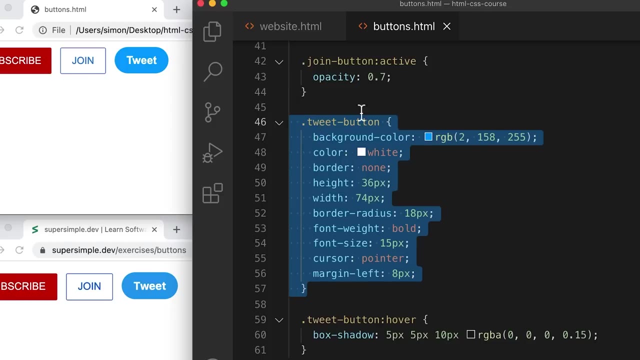 And then we're going to move our shadow into the hover pseudo class. We're going to cut and paste in here. So remember: the way this works is that let's refresh first. If we are not hovering over the button, we get all of these styles. If we are. 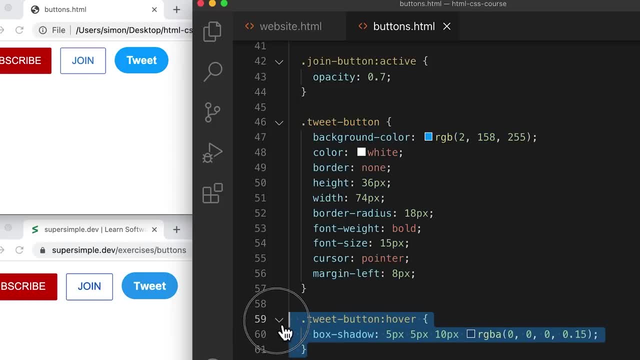 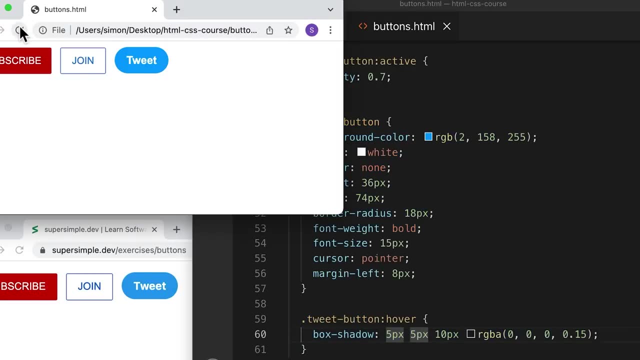 hovering over the button, we're going to get these styles, these hover styles, as well as all of these. So these styles get added on when we hover. So now, when we refresh and we hover over this button, we're going to get. 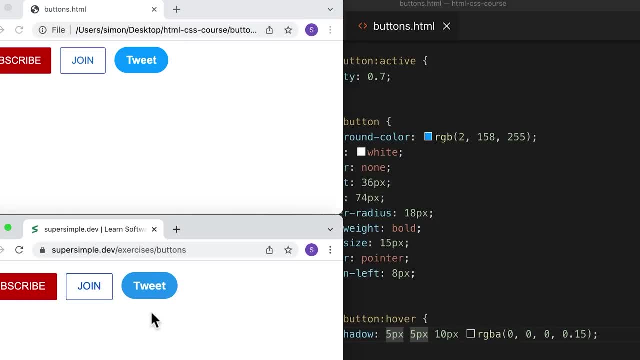 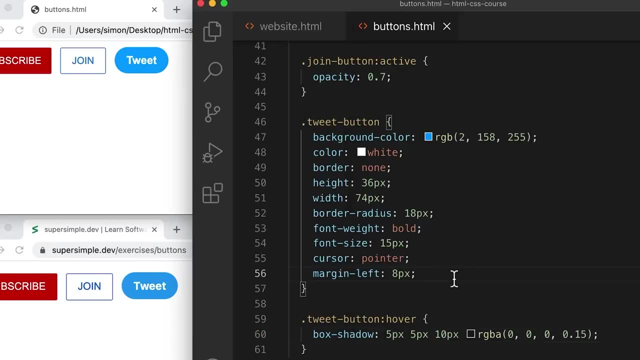 a pretty subtle shadow. It's not perfect, but I think it's close enough to what we want. Now the last thing we're going to do is to transition the shadow, So we can actually transition the shadow pretty easily by just adding the transition property. 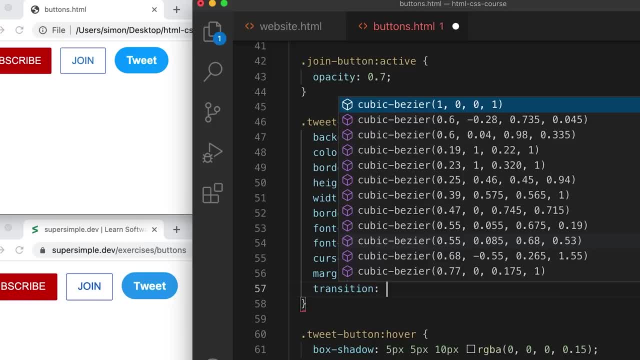 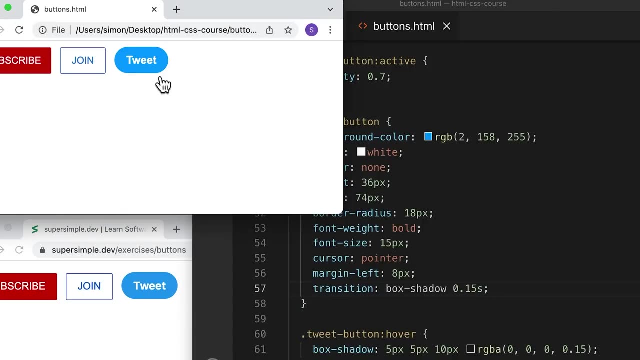 And we're going to tell it what we want to transition and how long. So we want to transition the box-shadow And let's transition it to something natural like 0.15 seconds. So let's save and refresh Now when we hover over. 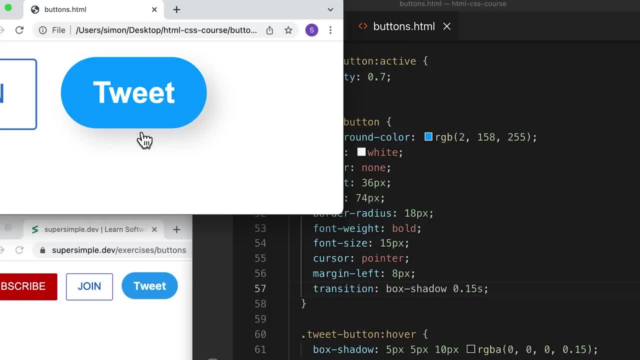 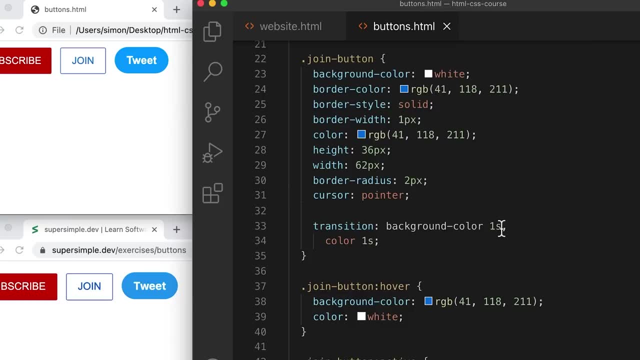 this button, we get a nice transition on the shadow like this: Alright, so the last thing we're going to do is: I realize I forgot to change the durations here, So let's change it to 0.15 and 0.15. 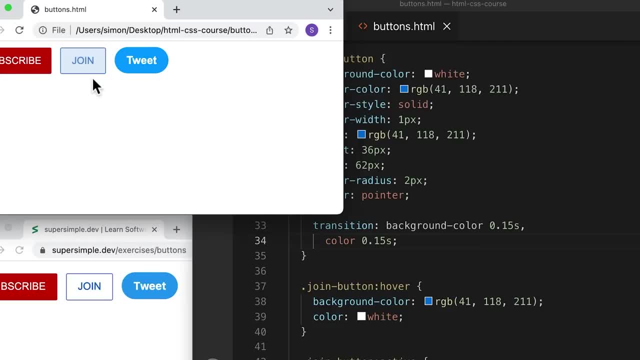 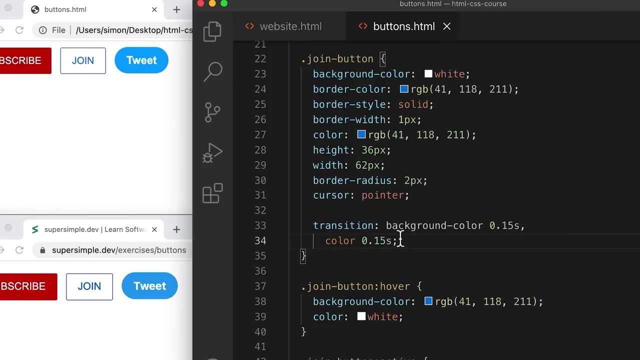 Let's save it and refresh, So now this looks something like what we have in our designs. So we just learned some intermediate HTML skills, such as creating hover effects, other pseudoclasses, transitions and shadows. Here are some more exercises from famous 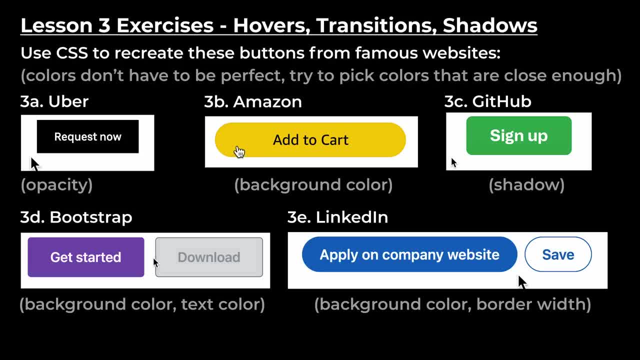 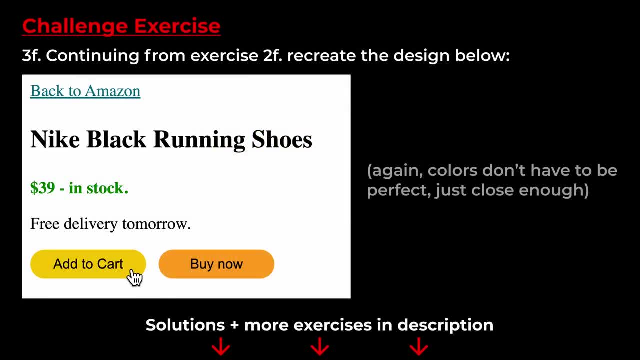 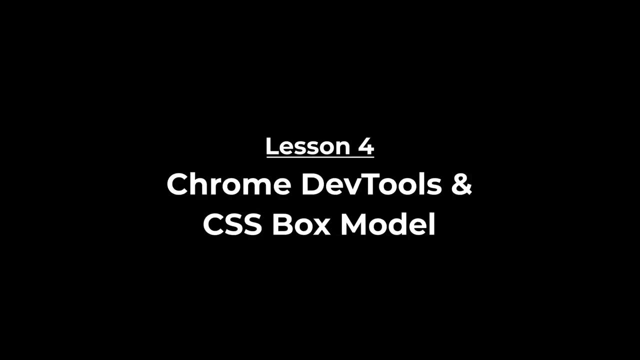 websites that you can try to copy. This time, we're also going to copy the hover styles. As always, you can find the solutions and more exercises below the video. In this lesson, we're going to learn about one of the most useful tools for web development called. 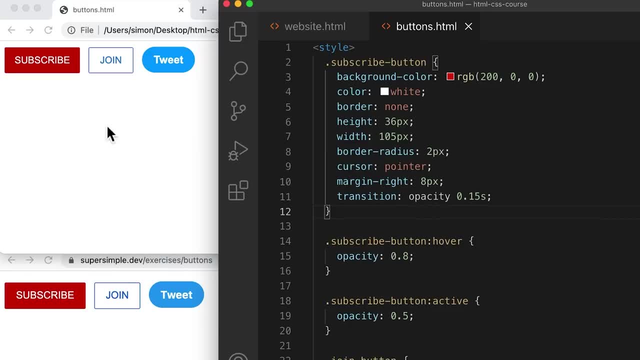 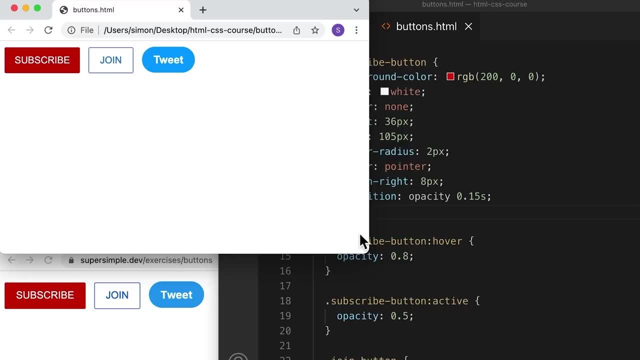 the Chrome DevTools, And we're going to use the DevTools to get perfect colors for our buttons. So, first of all, what are the Chrome DevTools? So I find that it's a lot easier to demonstrate it than to try to explain it. 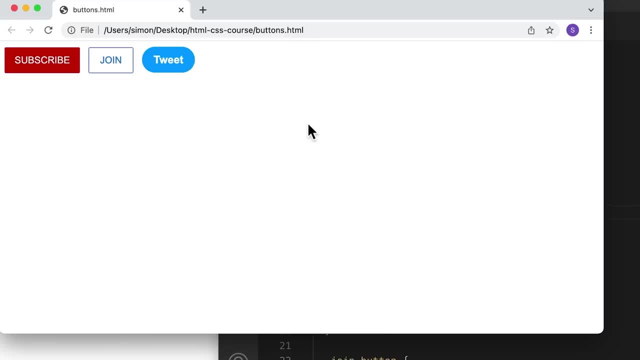 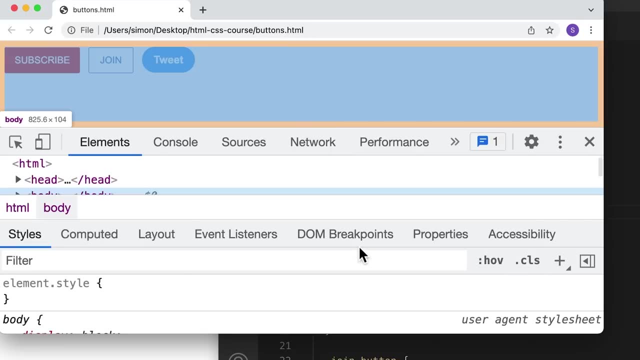 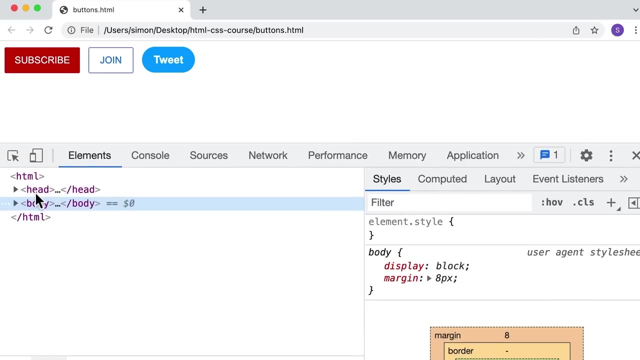 So let's go to our website and we're going to right-click in an empty area and we're going to click Inspect And this will open up the Chrome DevTools. So the cool thing about this is that we can now see all the HTML. 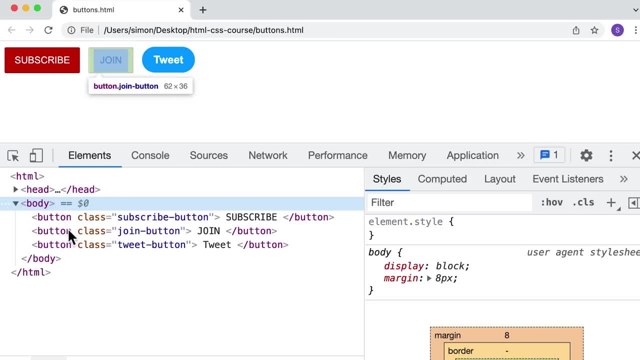 on our page. If we drill down here, we can see all the buttons, So this is a great way to visualize the HTML as well as the CSS on our page. If I click into one of these buttons, I can see all the CSS that is applied to this. 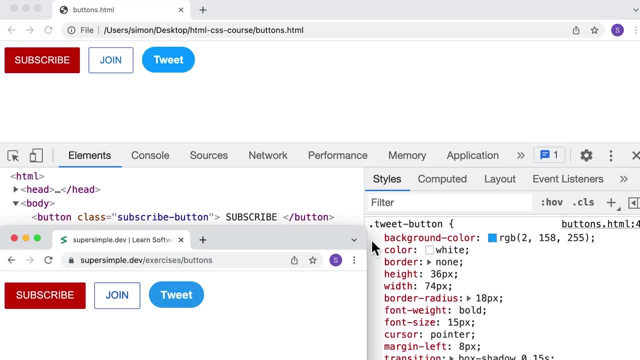 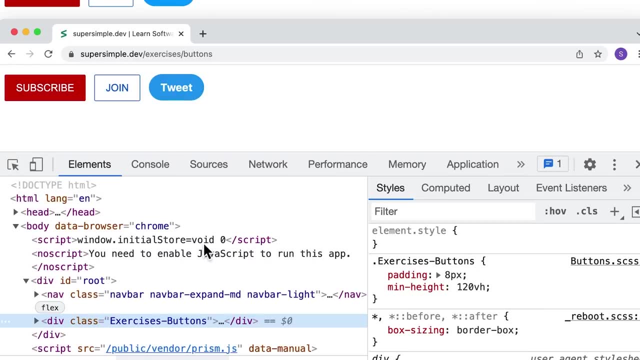 button. So what's even better is that we can open the DevTools in any website that we want. So we can actually open it in supersimpledev and you can see all the HTML that is on this website, as well as all the CSS. 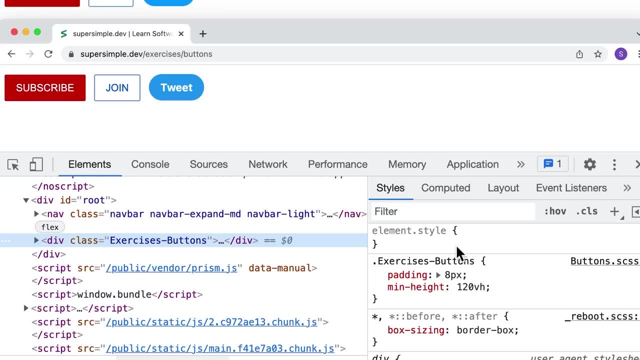 So this is a really great tool where you can open it in any website that you want and see the exact styles that they're using on that website. The next feature I want to show you is this pointer icon in the top left. So, instead of 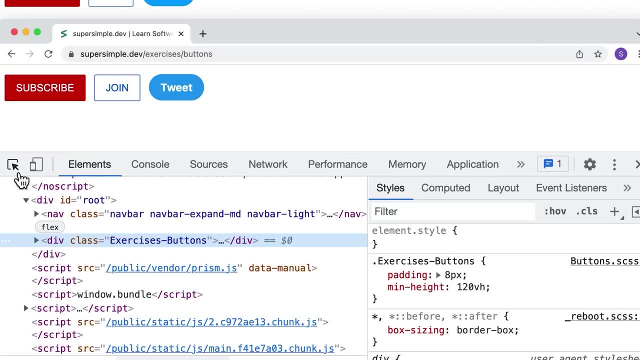 trying to find these buttons in all of this HTML. we can actually click this pointer icon and it will let us hover over any element on the webpage and show it down here. So if we hover over this Tweet button and click it, it will find the element for us. 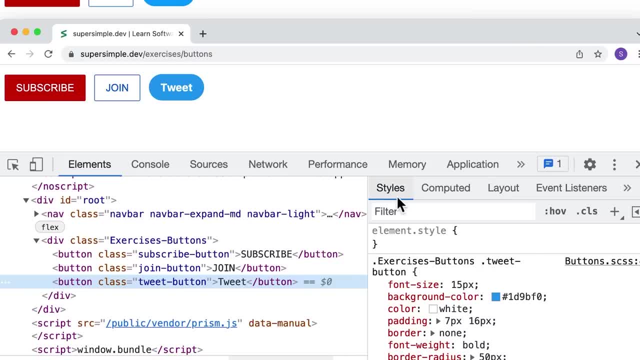 in the HTML, And now we can look at these styles here to see what kind of styles and, more importantly, what kind of background color is set on this button so that we can get a perfect background color. So one thing to note is that this background 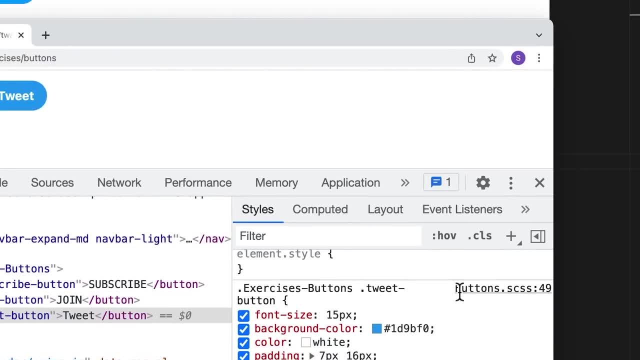 color is actually another way of measuring color. So currently we learned about RGB. now we have another way of measuring color and this is called Hex. It's basically the same as RGB. The first two characters here, 1 and D, represent how much red. the second: 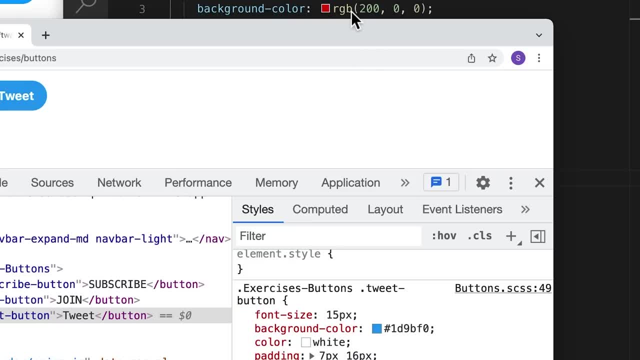 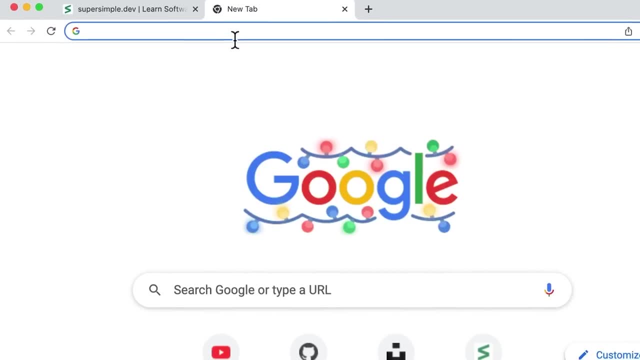 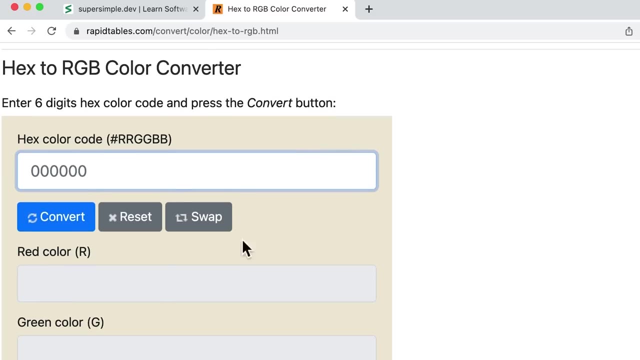 two represent how much green and the third two represent how much blue. So with a little bit of math we can convert from Hex to RGB. So I just Google a Hex to RGB calculator and I find any calculator and then I use it to convert. 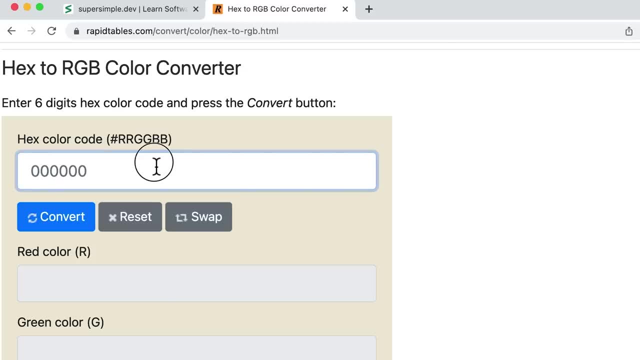 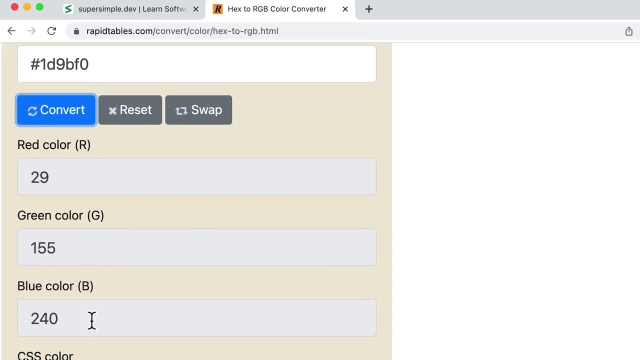 the Hex value. So I'm going to copy this into the calculator and then convert it and it will give me the RGB value. So it'll do that math for me. So that's just another way of measuring color called Hex. The next feature I want: 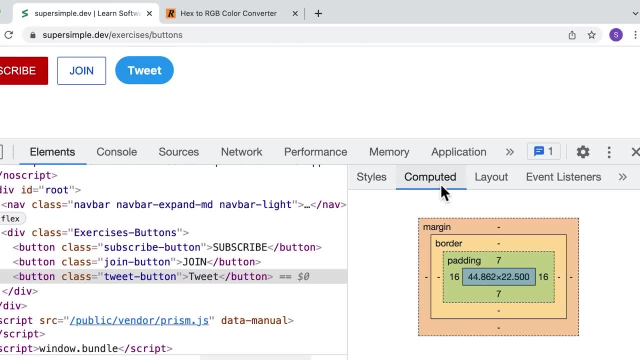 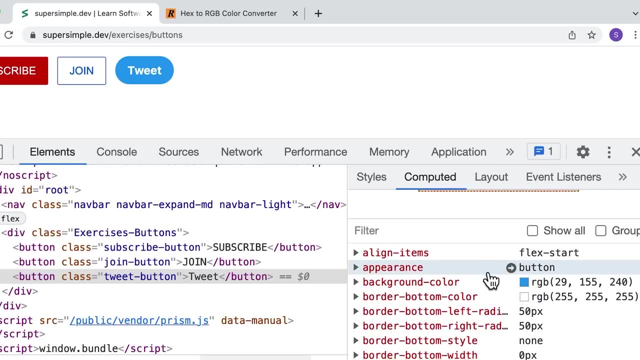 to show you in the DevTools is this computed tab. So this tab actually shows us all the final styles that are applied to this element. So we can actually scroll down here and we can find the background color in the RGB value. We can also find 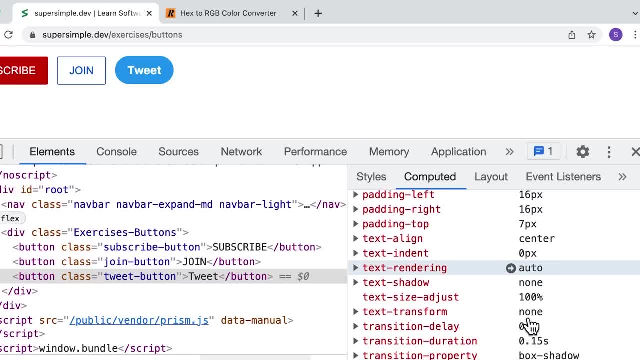 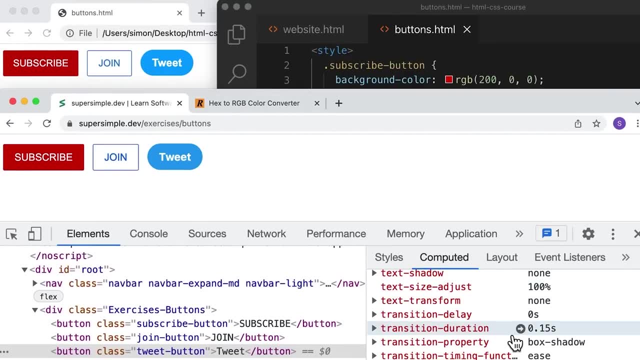 things like the height, the final calculated height, the final calculated width, So that we can get the perfect size as well as the perfect background color. So let's actually just use the background color here, And we're going to copy this and paste this into our code. 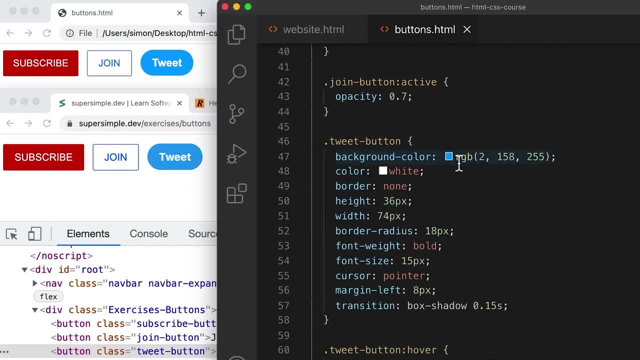 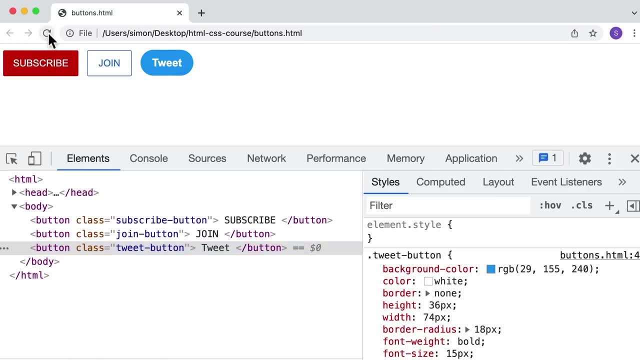 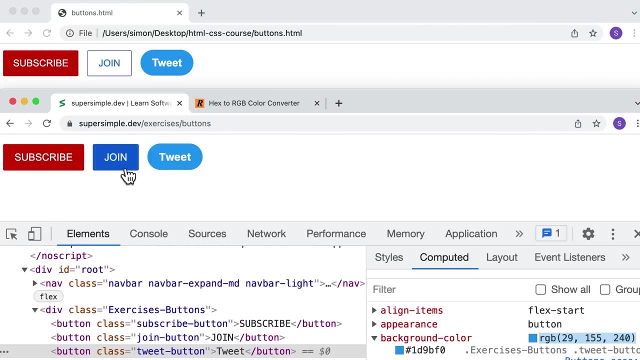 So we're going to get an exact color instead of trying to guess it like we were before. So if I copy and paste here, save it and now I refresh. now our button has the exact same color as what we have here. So the same thing happens for the join button. 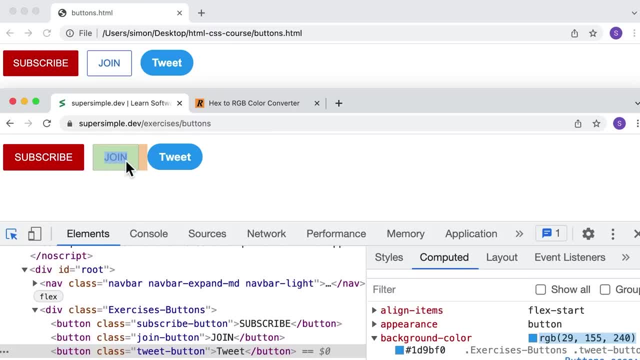 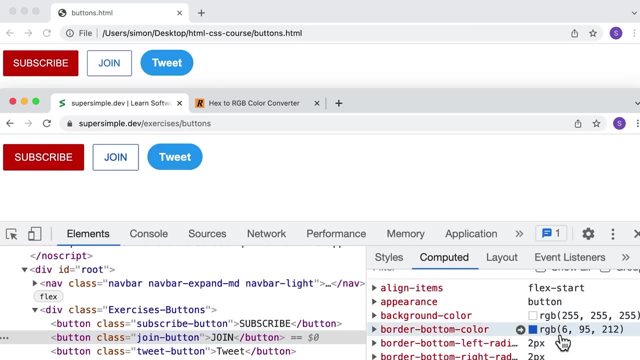 Let's click this icon here and hover over the join button to find it in the HTML click. and now we can see all these styles, all the final computed styles on the join button. So, most importantly, we can find the border color, which is this: 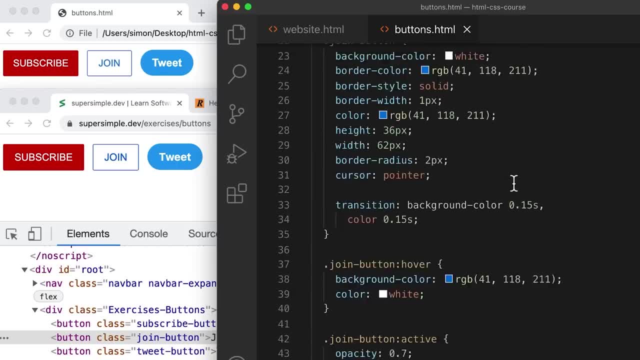 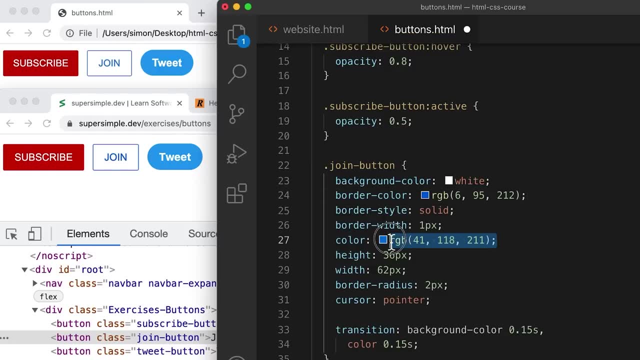 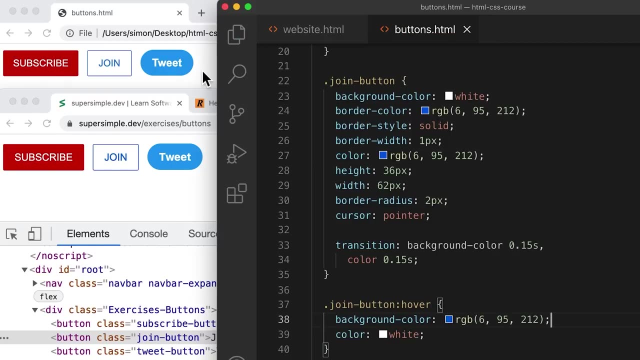 Let's go into. let's copy it and put it into our CSS so that we can get a perfect color. End it with a semicolon to follow the syntax rules. Copy it there and copy it here. Now we're going to save refresh. 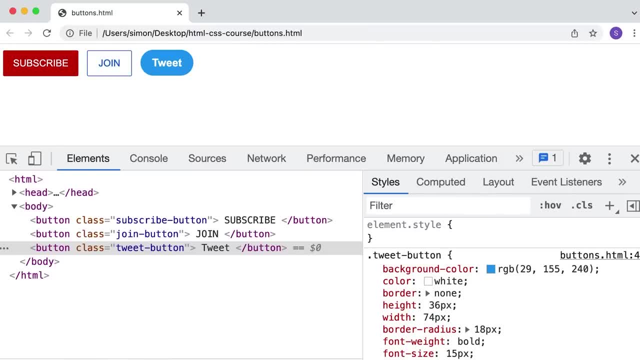 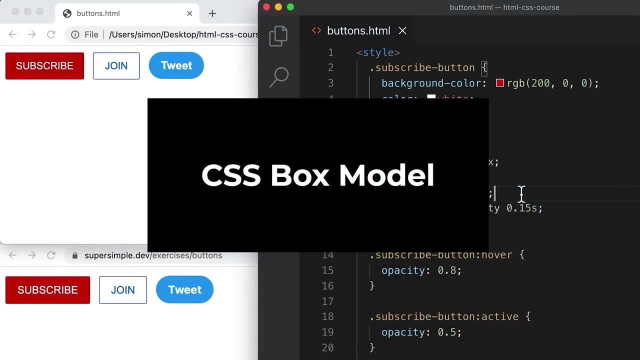 and now our button color is going to match the design exactly. So that's how you use the dev tools to get perfect color for our HTML elements. Now we're going to learn about the CSS box model, which basically allows us to add space between: 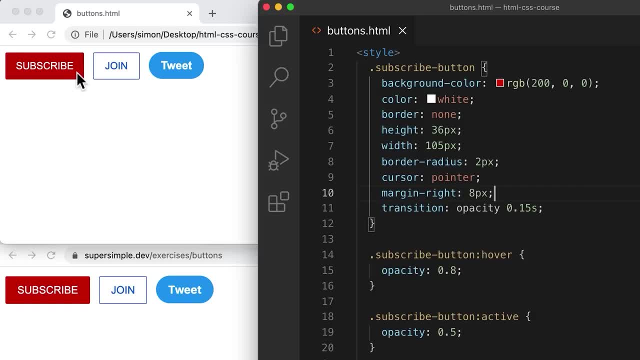 our elements like this, as well as add space inside our element to make it bigger. The first part of the box model is spacing on the outside of the element. This is called margin. If we look at our code, we already worked with margin before. Here we set the 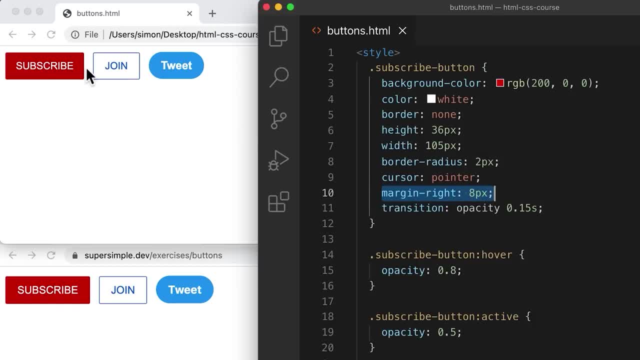 margin right to 8 pixels. That means that we added space on the outside of the button on the right of 8 pixels. If we change the margin right to 30 pixels, for example, and save and refresh, now there's 30 pixels of space. 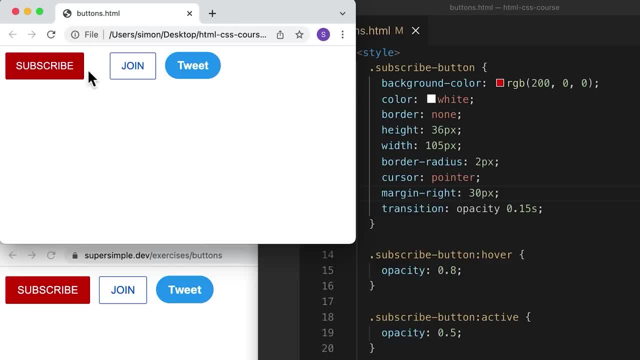 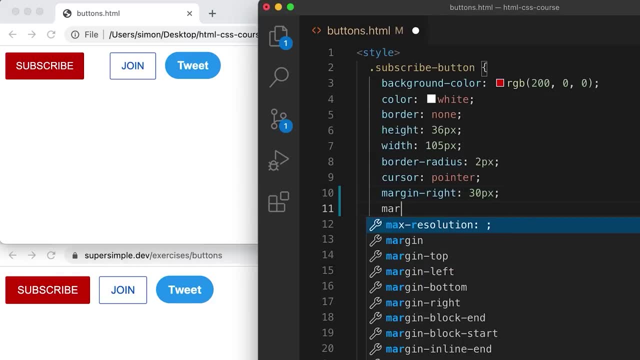 on the outside, on the right side of the button, So we can add margin to all four directions: Top, right, bottom and left. Let's try adding margin to the left side of the button. this time We're going to add margin left of 20,. 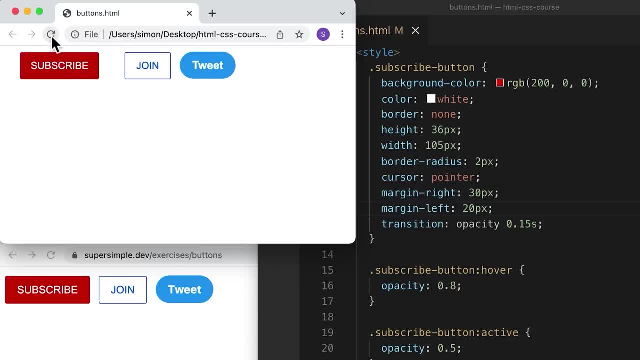 pixels, Save it and refresh, And that adds space on the outside of the button on the left of 20 pixels. So that's basically how margin works. It lets us add spacing on the outside of the element, The second part of the box. 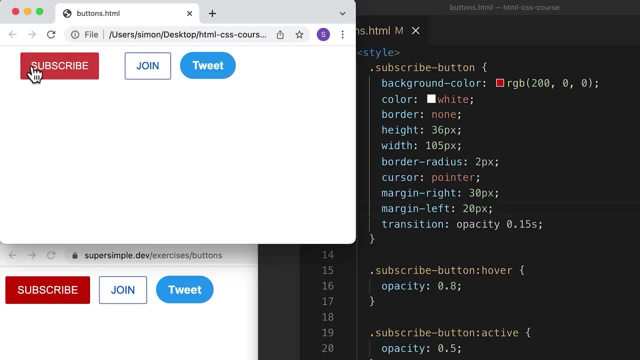 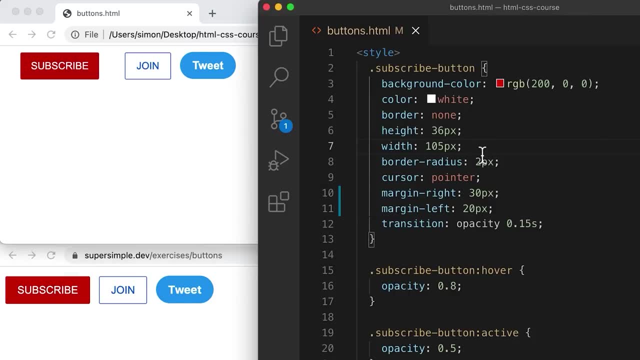 model is spacing on the inside of the element, So basically all the spacing in here around our text. So currently, if we look at our code, we're setting the height and width of our buttons And this is not actually a good idea. I'll show you why. 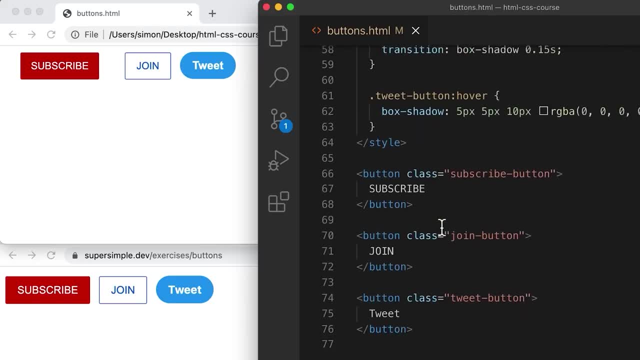 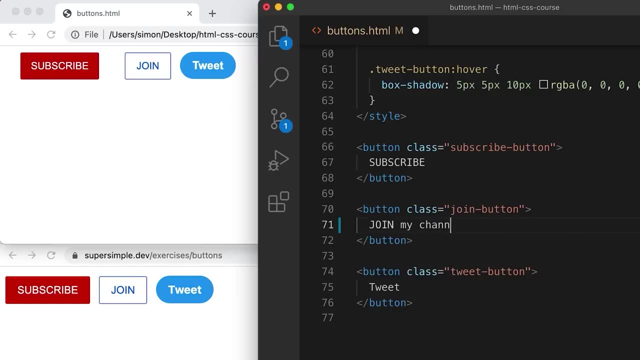 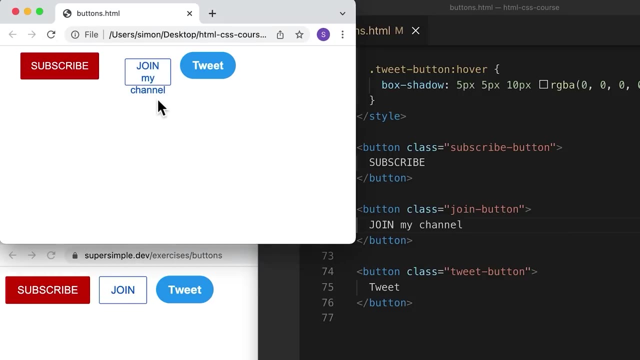 I'm going to scroll down to the join button because it's a little easier to see, And I'm going to change the text to join my channel. Save it and refresh And you'll notice that the text is actually overflowing the button, like this: 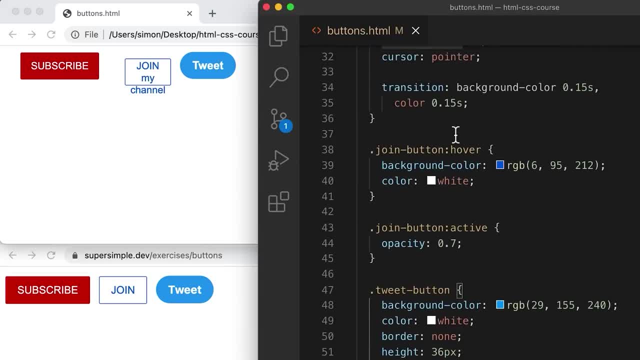 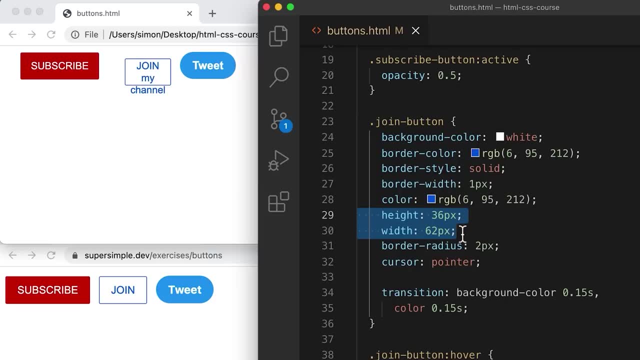 And that's because, if we scroll up, we're setting the height and the width. That means that we're forcing the button to have a height of 36 pixels and a width of 62 pixels. But here notice that our content is too big. 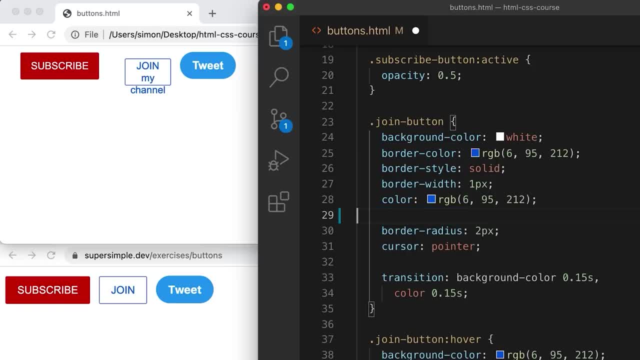 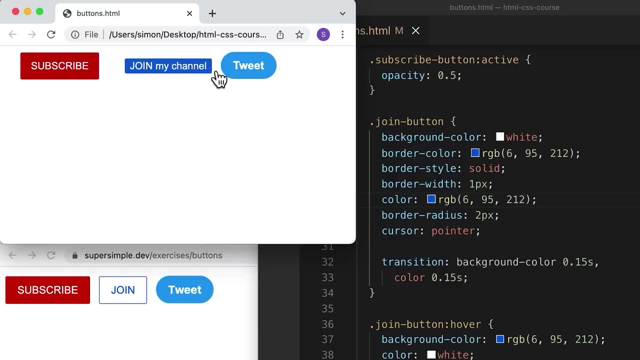 So what we want to do is to remove these lines and save it and refresh the page And, by default, our button actually adjusts the size automatically based on the content. So now, instead of setting the height and the width, we're going to 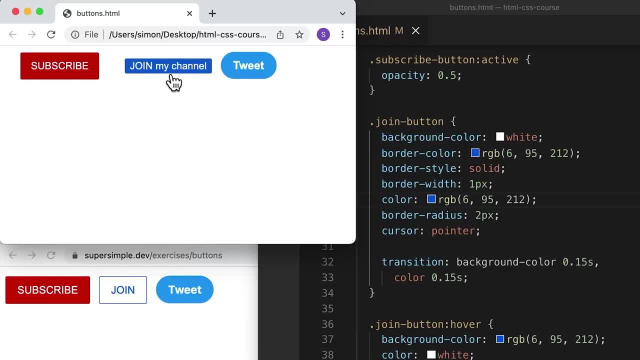 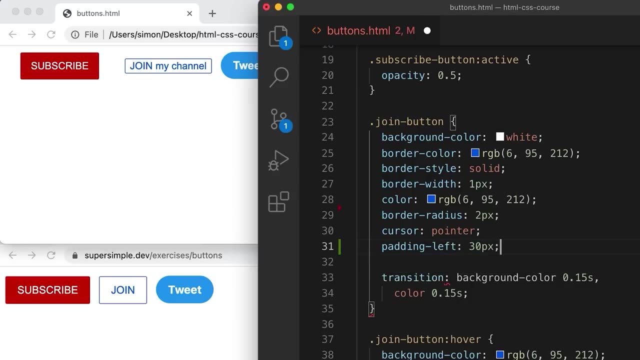 achieve the same thing by adding spacing on the inside of the button. So the spacing on the inside of the button is called padding. Let's go into our code and give it a try. So we're going to add padding. dash left of 30 pixels. 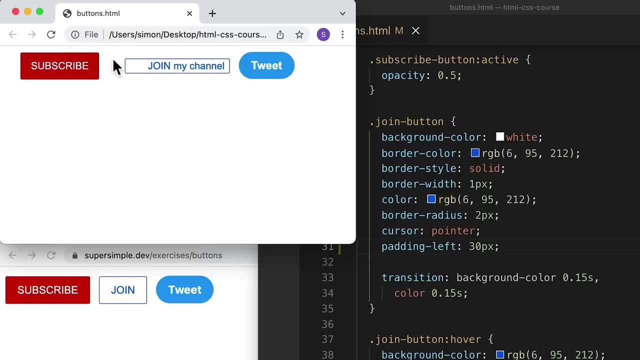 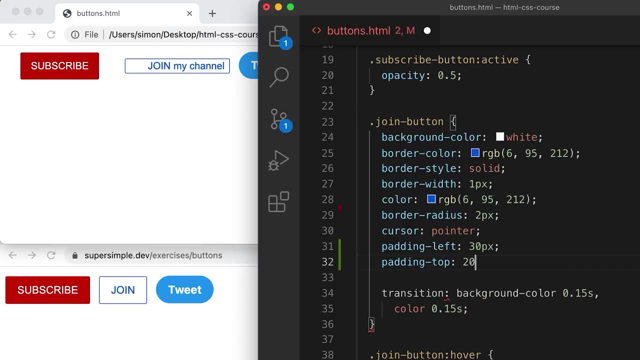 Save it and refresh And you can see that padding adds spacing on the inside of the button And, just like margin, we can set padding in all four directions. So let's try adding padding dash top to 20 pixels. Save that and 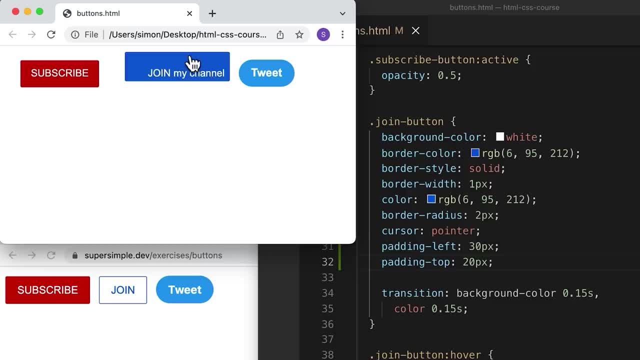 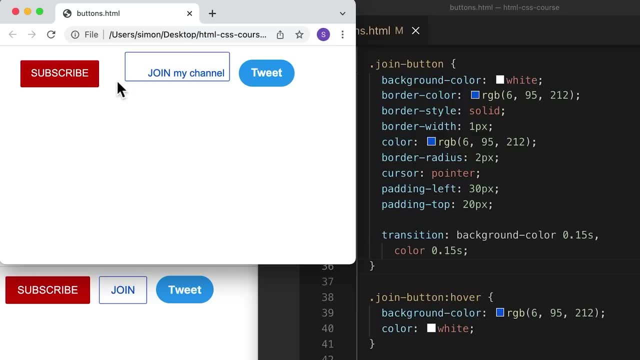 refresh And now you can see that we added padding on the top by 20 pixels, So we can actually use the chrome dev tools that we learned earlier to visualize the margin and padding of our elements. Let's go into a blank area of our webpage. 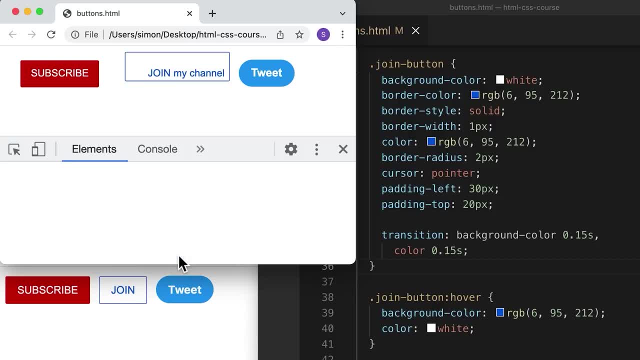 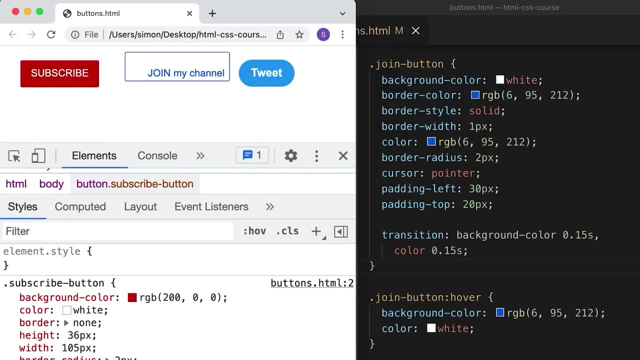 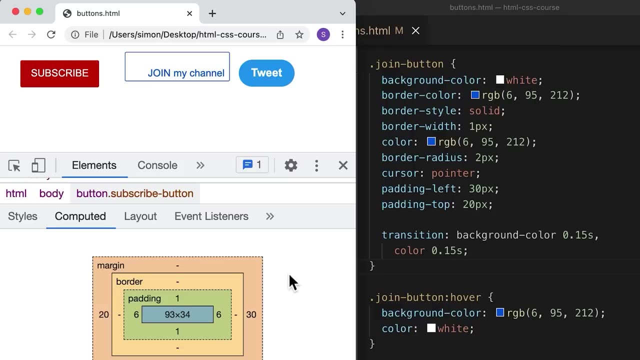 and we're going to right click and inspect and then click this top left icon and then click our subscribe button. So I'm going to drag this down and then we're going to go into the computed tab. So this section is basically. 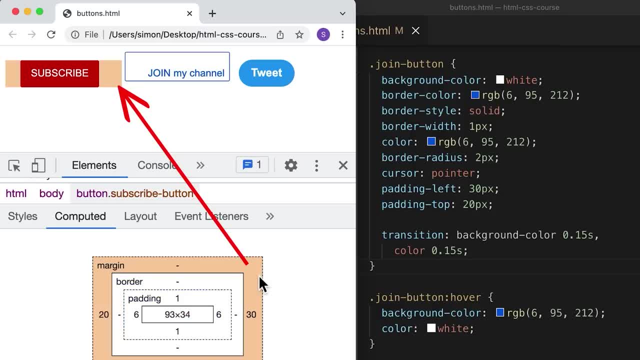 the box model. We have our margin, which is the space on the outside of the element. You can see that highlighted in orange. We have the border, which we learned earlier, And we have the padding, which is the space on the inside of the element. 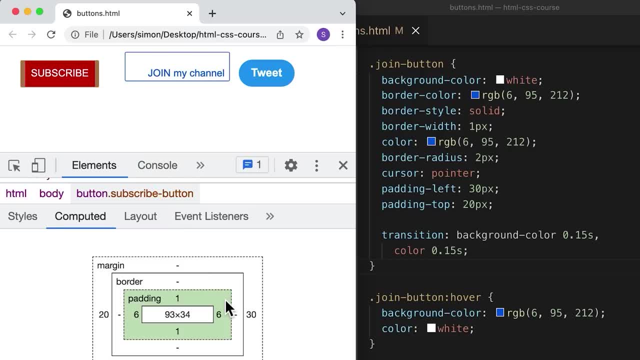 which you can see highlighted in green Buttons, by default have a padding of 6 pixels on the left and right and 1 pixel on top and bottom, So let's click this top left again and go to our join button and click this. 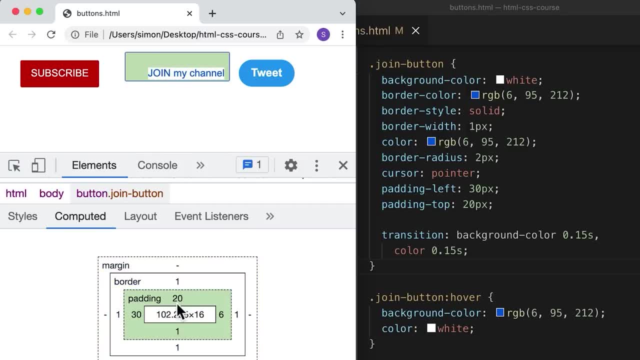 button. In this example, we have padding on the top of 20 pixels, which is what we have in our code. We have padding on the left of 30 pixels, also what we have in our code- And then we have a default padding. 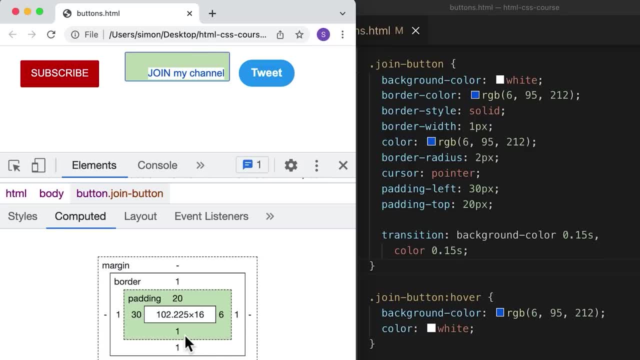 of 6 pixels on the right and 1 pixel at the bottom, And for this button we have a border of 1 pixel wide, which you can see here in our code. So all of these combined make up the CSS box model. 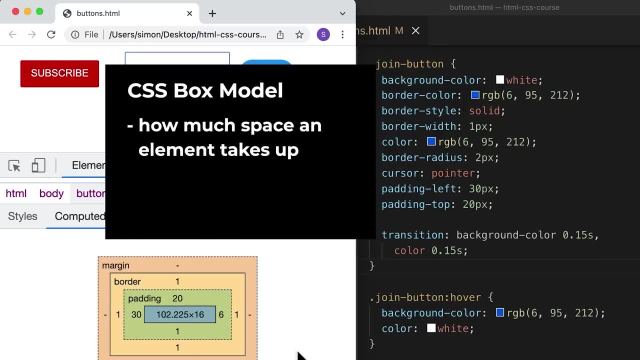 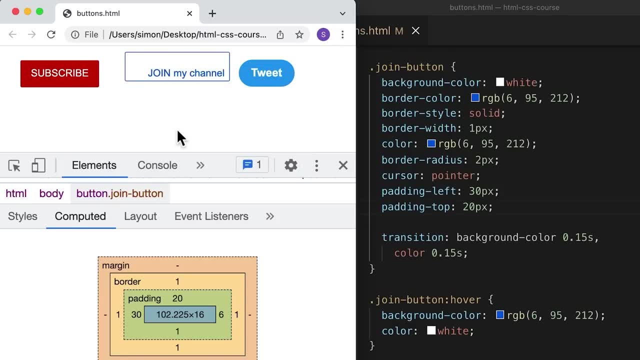 This basically determines how much space an element takes up on the page and how far it is away from other elements. So now that we learned the box model, we're going to use it to recreate our design here. So currently, if we look at our code, 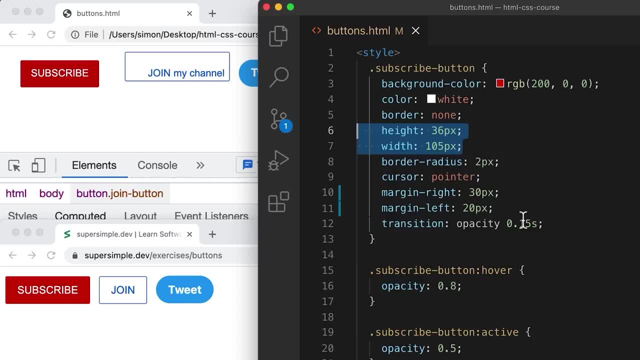 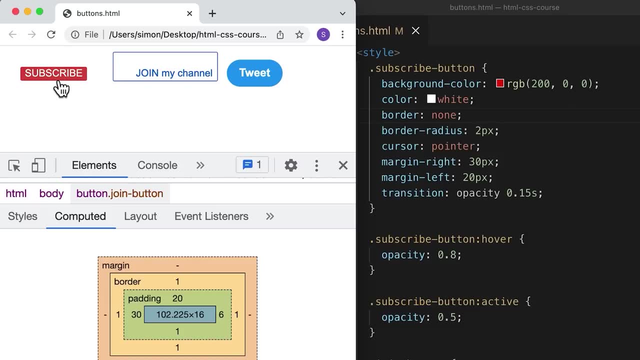 we're using height and width. Let's replace this with the box model. Let's get rid of this and save it and refresh. And now our button's back to what it was before. And now we're going to add padding to this button so that it 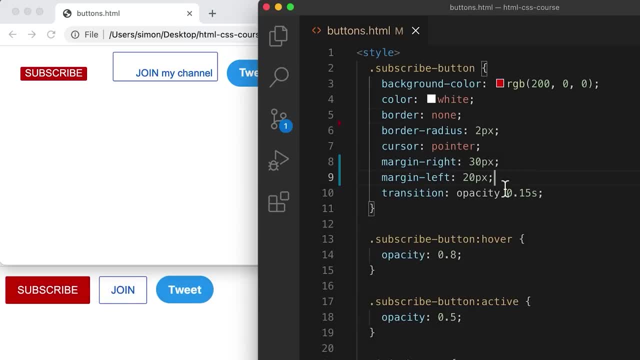 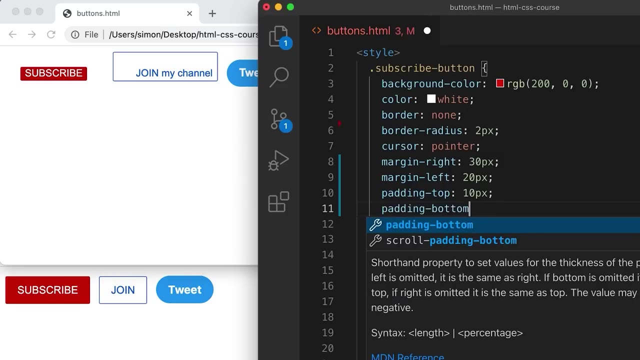 matches the design at the bottom here. So let's add some padding dash top of 10 pixels. So we'll add spacing on the inside of the button at the top here of 10 pixels. We're also going to add padding dash bottom. 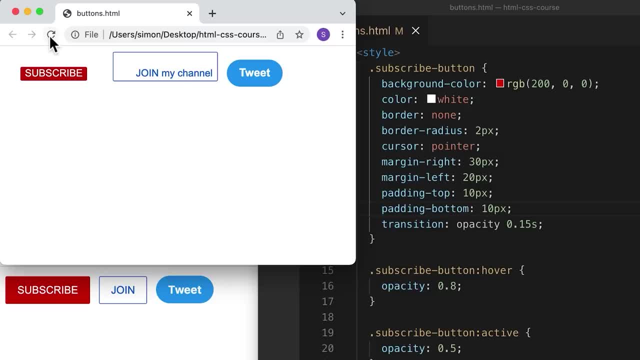 of 10 pixels. Let's save that and refresh. Okay, so now we have space at the top and bottom, So that looks pretty close. We're also going to add space on the inside, on the left and right, So we're going to add padding. 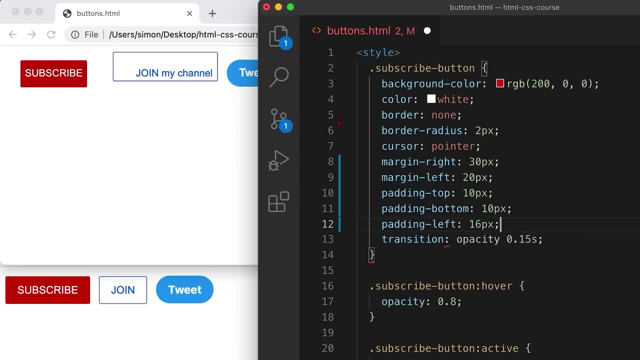 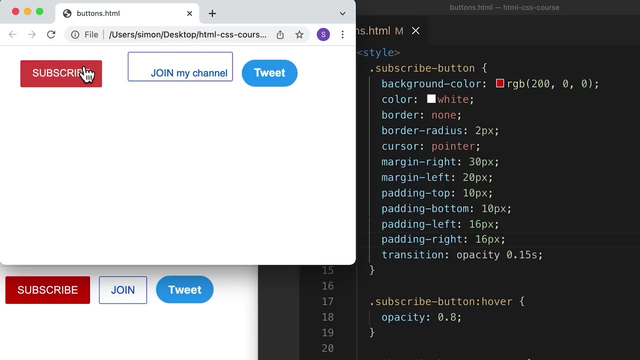 dash left of 16 pixels And padding on the right of 16 pixels, So let's save that and refresh, And I think this looks close enough. So, using padding, we added spacing on the inside of our button And the good thing about this is that if we change, 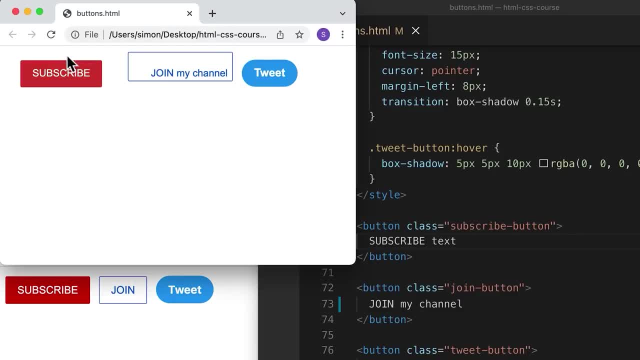 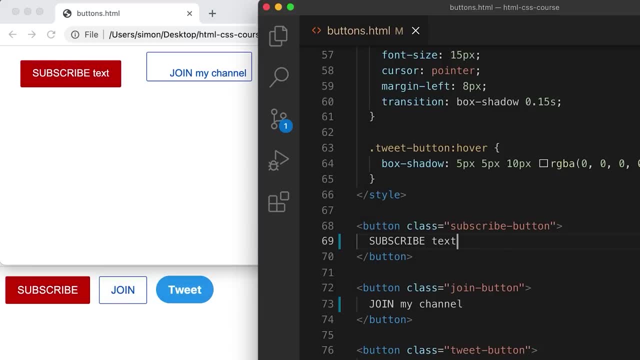 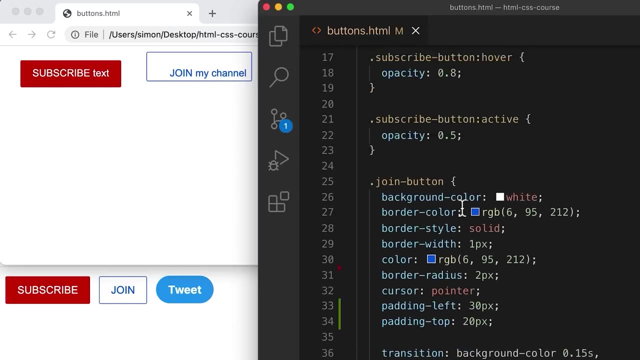 the text like this and save it and refresh. the button will resize with the text, but it will keep the spacing on the inside. So using padding is a better alternative to height and width. So let's save that and refresh the page. 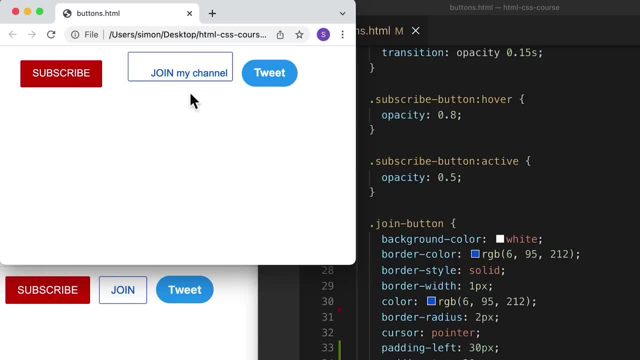 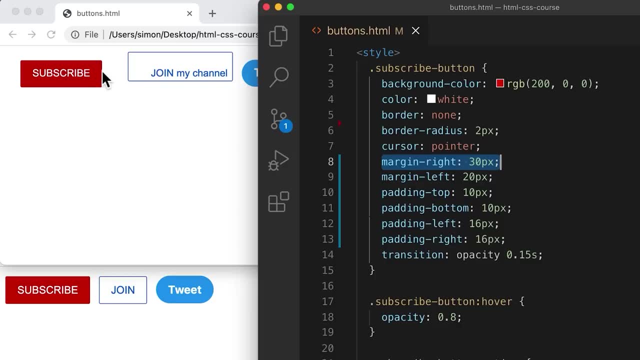 And let's actually move these buttons back closer together. So currently if we scroll up, we have margin on the right of 30 pixels, So spacing on the outside of the button on the right of 30 pixels. We're going to change it back. 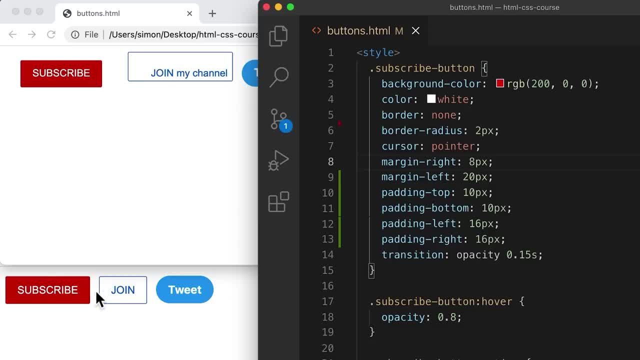 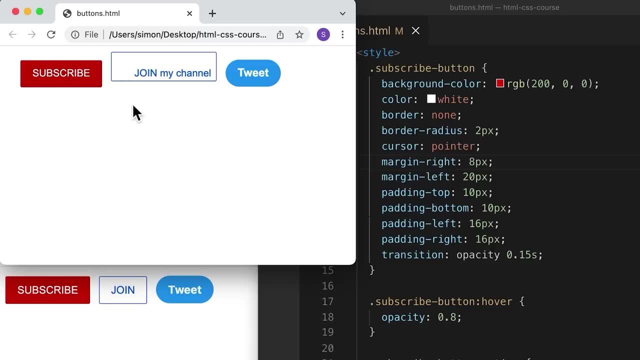 to 8 pixels So that it's closer, like we have in our design. Save it and refresh. Okay, so that looks pretty good. Now, one thing you'll notice is that our buttons are not aligned with each other, So the join button is all the way at the top. 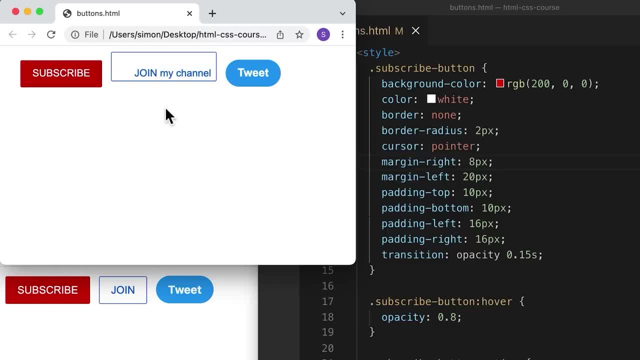 while our subscribe button is a little bit below. So why is this happening? By default, the browser tries to align our buttons based on the text, So notice that the text is in one line like this. So that's the default behavior of the browser. 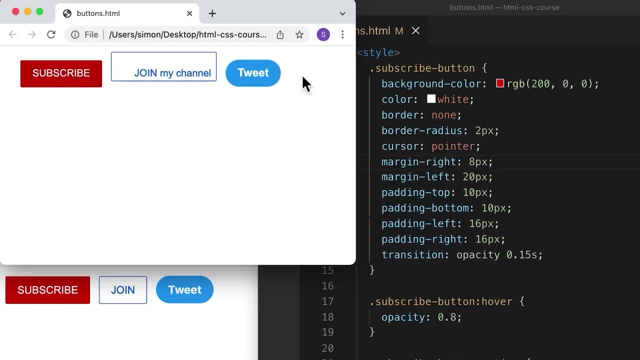 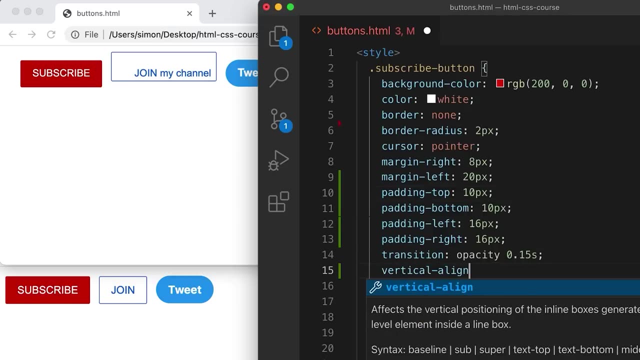 This is because browsers in the beginning were mostly text based. Now, to override this behavior and align everything to the top, like we had before, we can go into our CSS and we're going to add a property called vertical-align And we're going to set this to top. 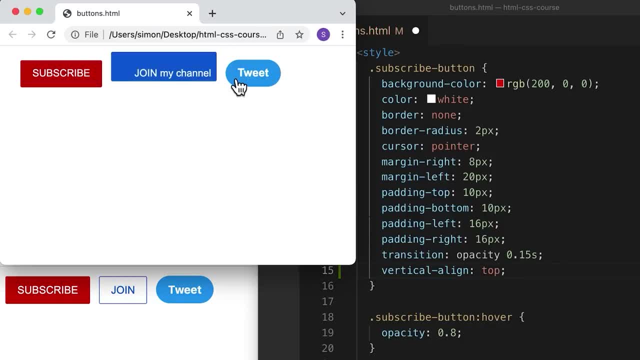 So, instead of aligning the buttons based on the text like this, we're just going to align everything to the top, So let's do that and refresh. Now the subscribe button is aligned to the top, which is right there. Let's do the same thing for the tweak button. 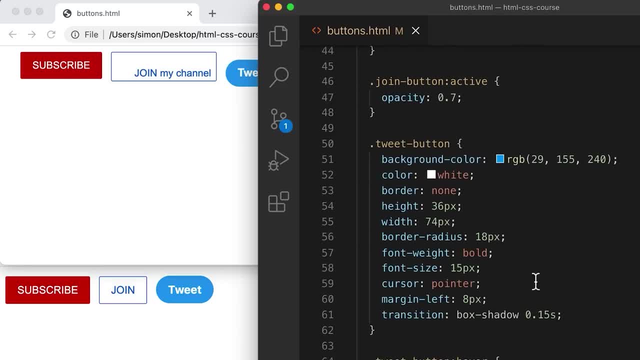 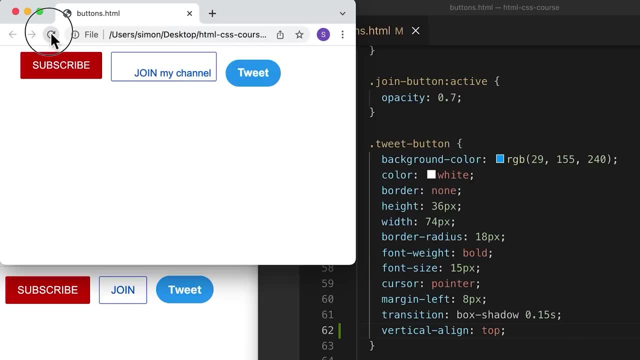 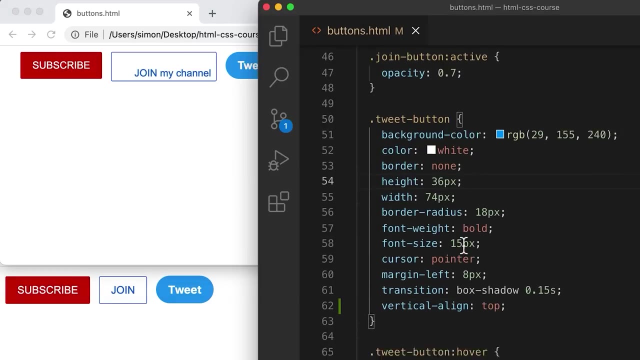 We're going to scroll down and we're going to add vertical-align colon top here as well. Save and refresh, And now everything's aligned properly again. Now let's work on the join button. I'm going to scroll down and remove this extra text here. 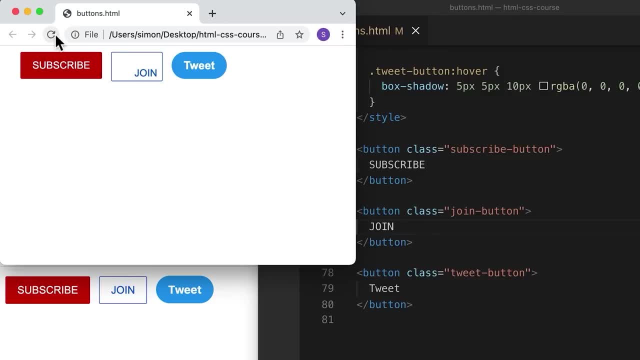 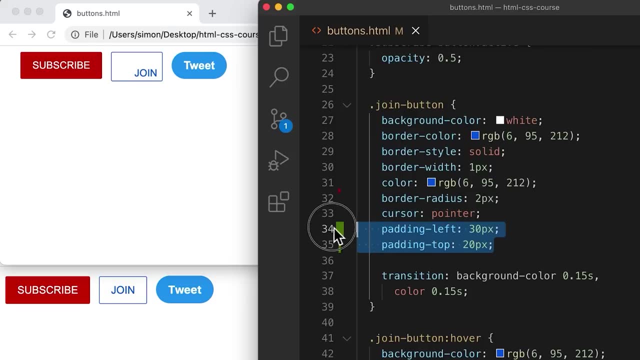 Save it and refresh. And now we're going to go to our CSS for the join button. So I'll scroll up to right here and we're going to adjust the padding. So let's actually just borrow the padding from the subscribe button, because 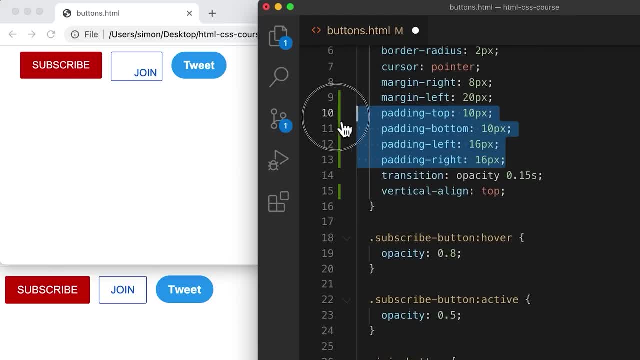 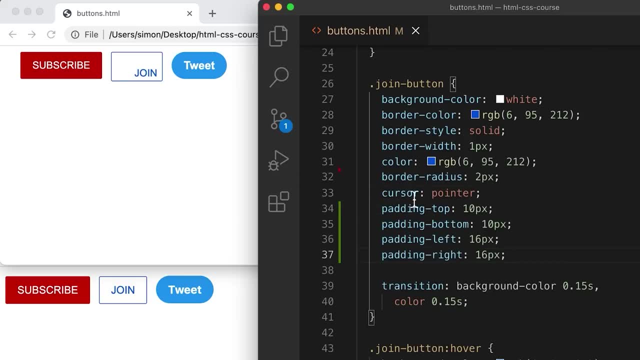 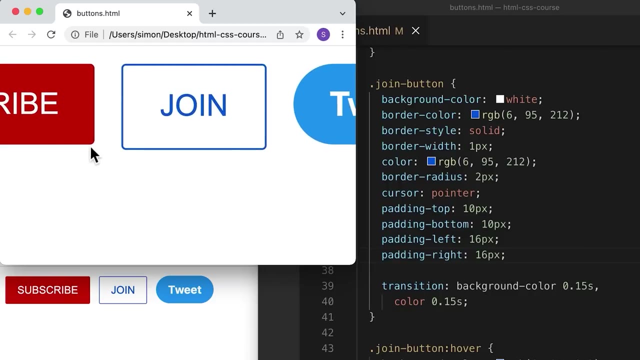 they look pretty similar. I'll scroll up here and copy these and just move them down to the join button Right here, Save that and refresh. Okay, so that looks pretty good, Except our join button looks a little bit off. It looks a little bit taller. 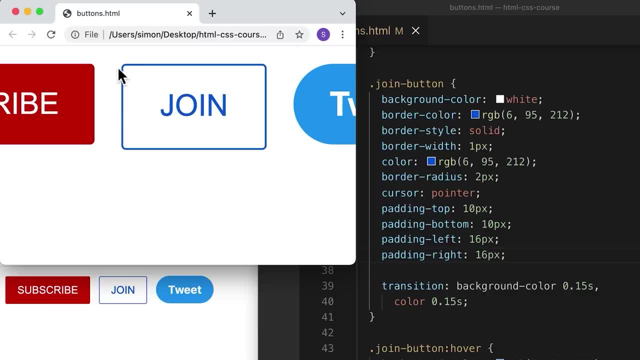 than our subscribe button, And that's because the border actually adds a little bit of size to this button, So it adds one pixel on the top and bottom. That's why this button is taller than the subscribe button. So to compensate, we're actually going to reduce the padding. 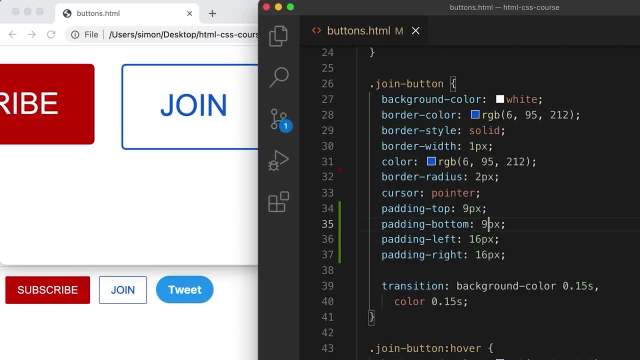 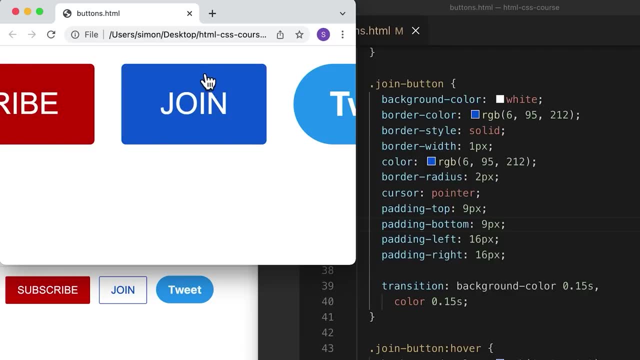 at the top and the bottom by one pixel. Save it and refresh And now they're the same size. We have nine pixels of space on the inside plus the one pixel of the border width, And that matches the ten pixels of space on the inside of the. 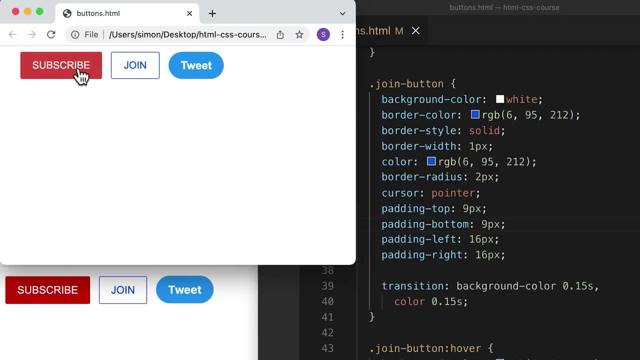 subscribe button And I'll leave changing the tweak button up to you as an exercise. So that is the CSS box model. Every element can have spacing- on the outside called margin space, on the inside called padding, as well as a border, And these properties. 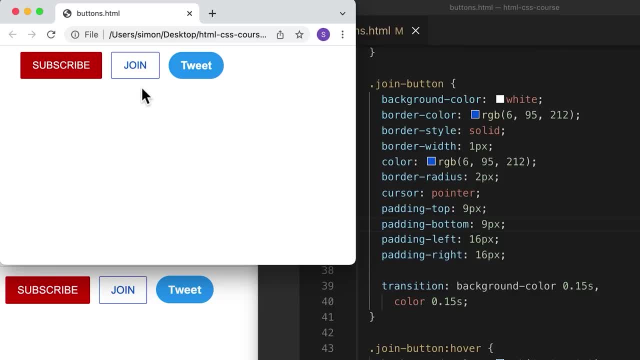 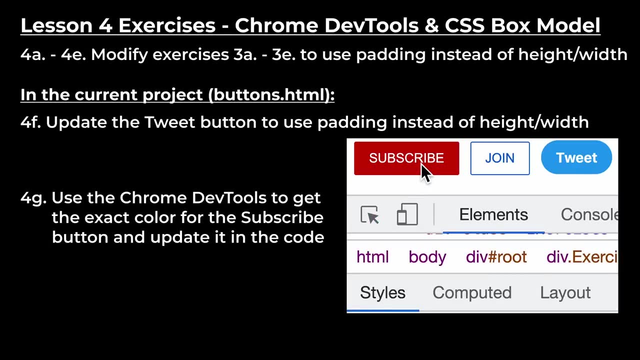 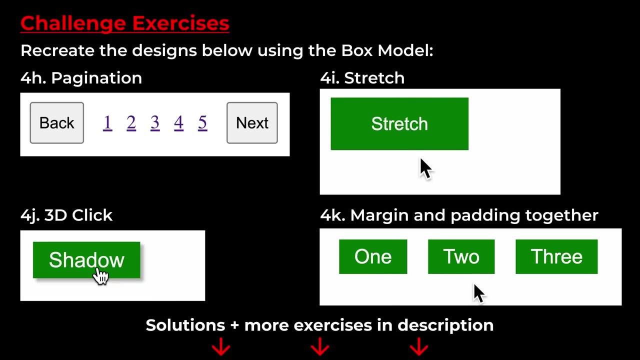 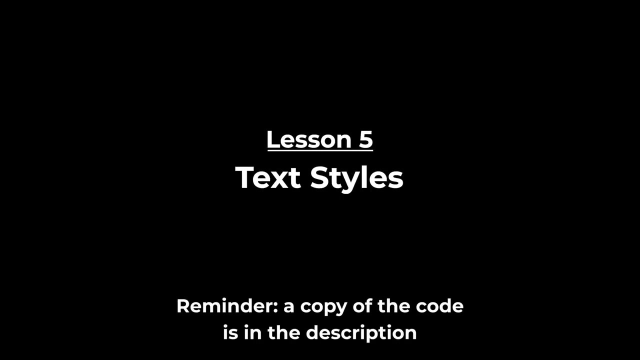 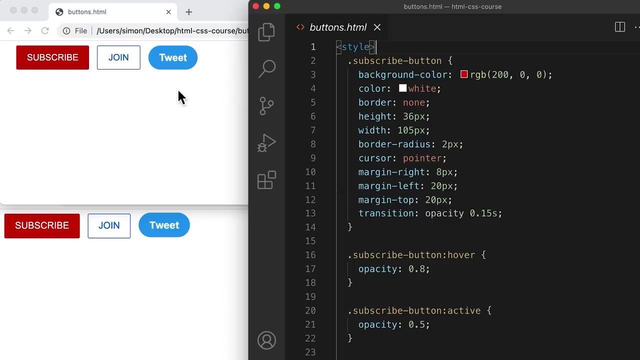 determine how much space an element takes up on the page. Here's some exercises of using the box model to get yourself more familiar with this concept and these properties. For most of the course, we've been working with buttons. In this lesson, we're going to work with text and we're going to 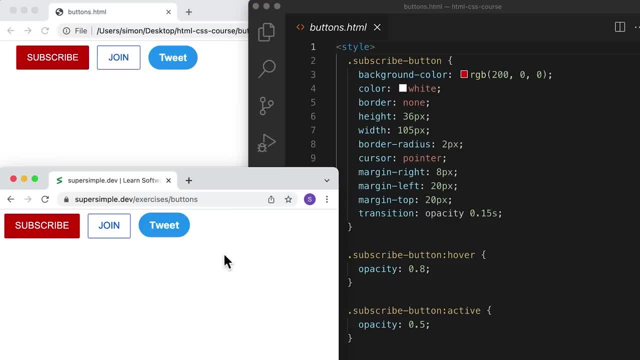 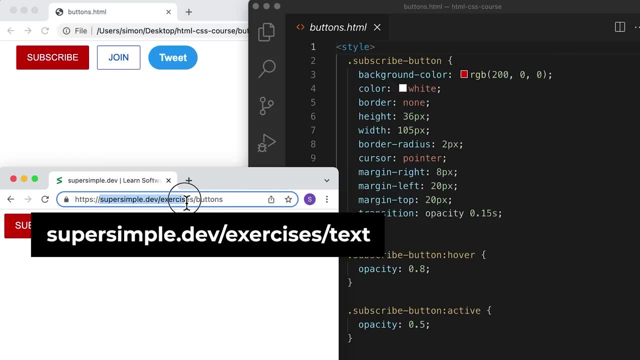 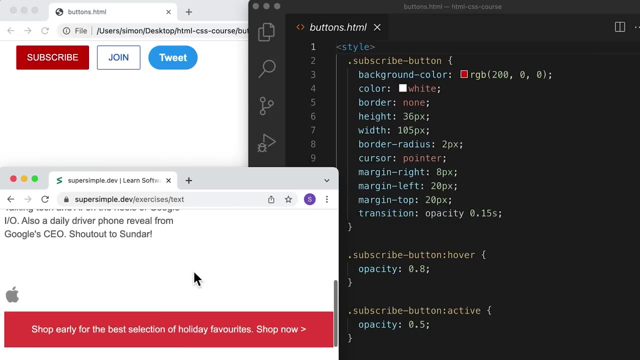 learn how to style text. So, just like our button lesson, I've created an exercise that we can practice with text. So we're going to go to supersimpledev slash exercises- slash text, And now we have some text from YouTube and Apple that we're going to learn how to copy. 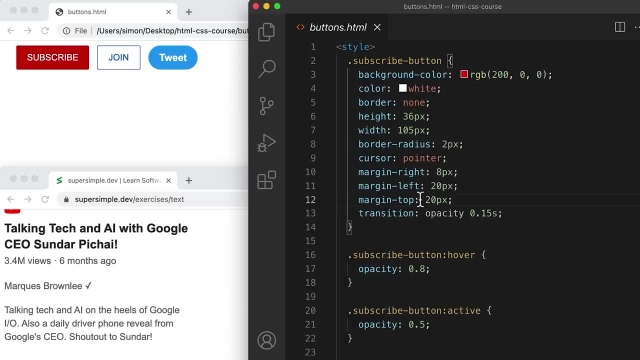 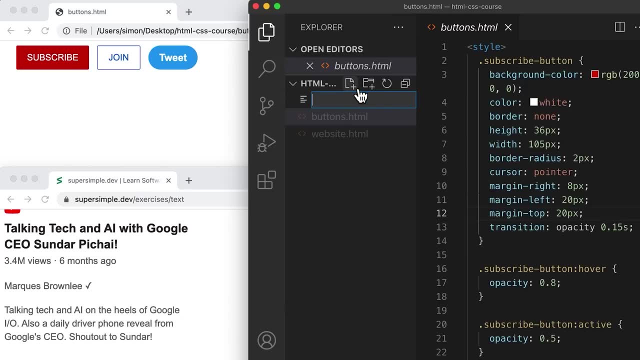 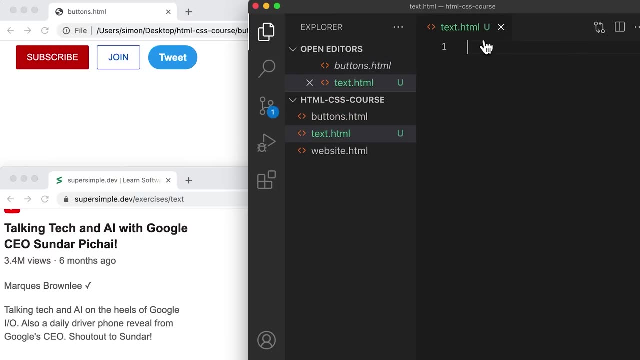 So, first of all, let's create a new HTML file where we can focus on practicing text styles. So I'm going to go here and create a new file And let's just call this texthtml. And now we're going to open this file. 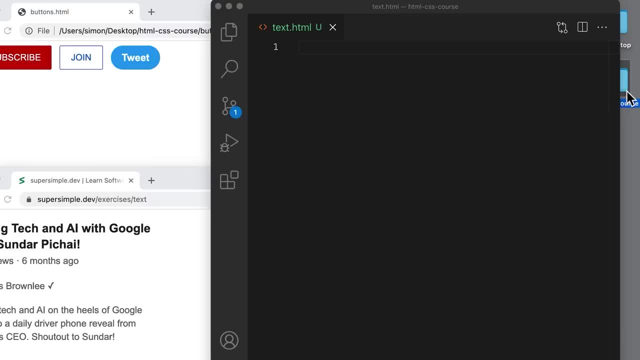 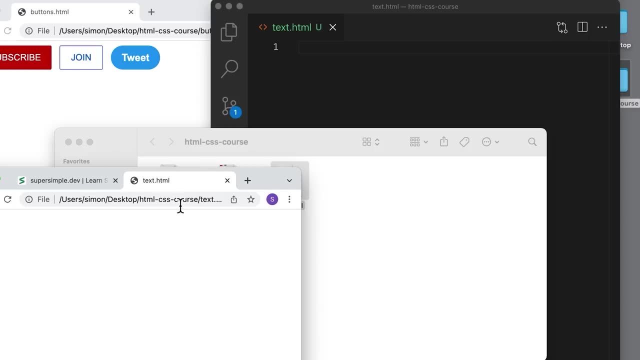 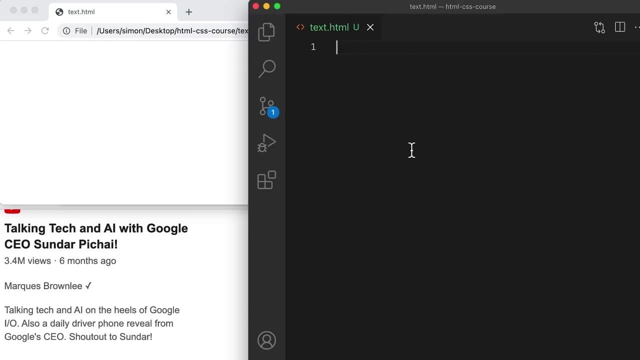 in our browser. So open the folder that contains our code and right-click open with Google Chrome. I'm actually going to put this up here, Alright, so now we're ready to begin. If you've ever written a text document before, 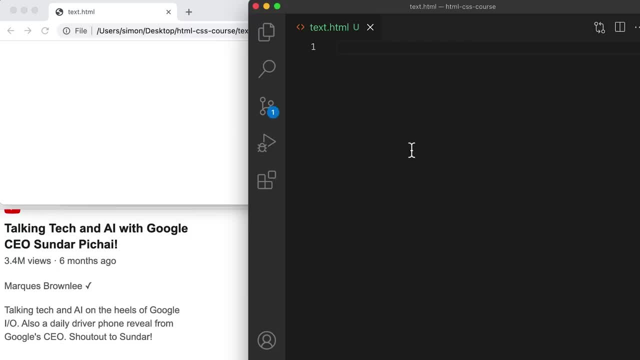 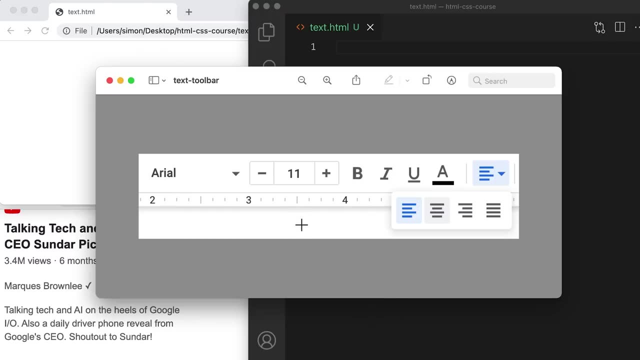 using something like Google Docs or Microsoft Word, you've probably seen something like this. This is a toolbar that allows us to change the style of our text. We can change the font, the text size, we can make it bold, we can center it, etc. 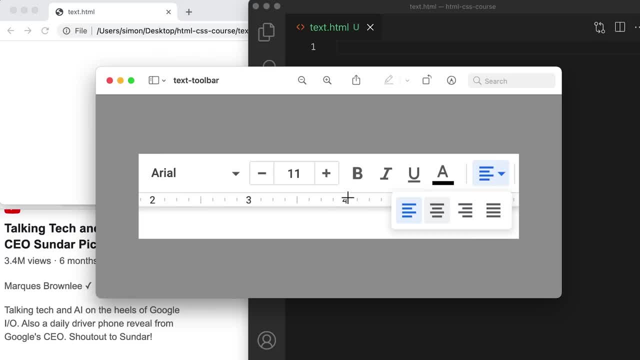 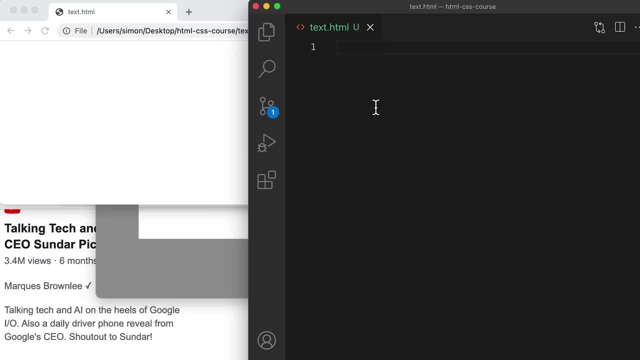 In CSS, we have a style for each of these things. Let's go to our code, and we're going to first start by creating some text on our page. So let's first create a paragraph And then, inside our paragraph, let's start with the text. 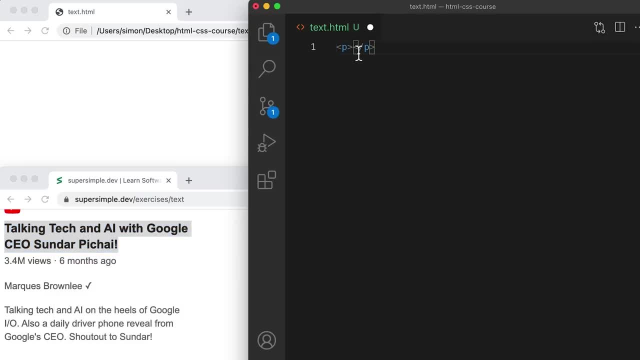 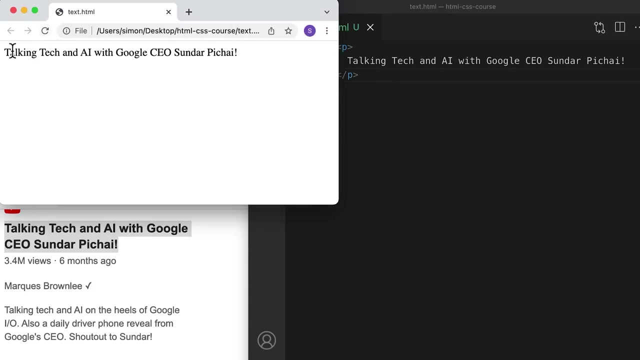 here. So I'm going to copy and paste this into our paragraph and I'm just going to reorganize the code a little bit and save. Remember that in HTML these extra spaces and new lines don't matter. Now refresh the page and we have. 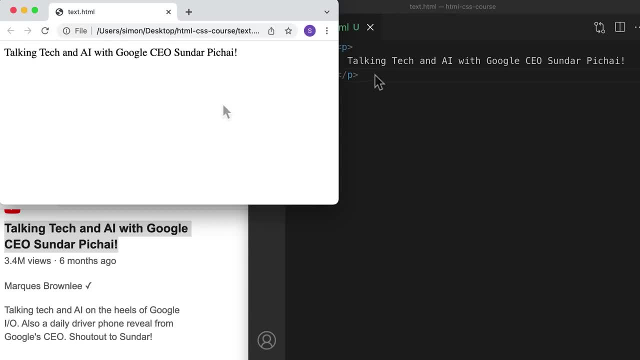 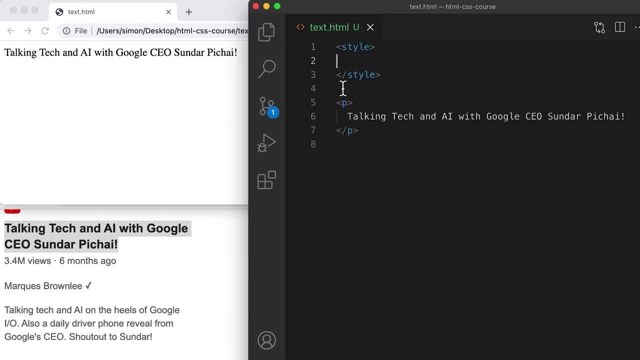 our first paragraph that we can practice with. Next, let's create a style element so we can write some CSS code. Now we'll set a class on this paragraph so that we can target it in CSS class. equals video-title, because this is a video. 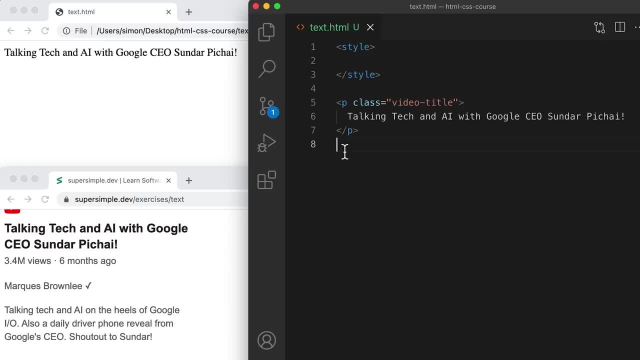 title that I copied from YouTube. So let's save it and refresh, and now we can start targeting this paragraph in our CSS. So remember, we're going to start with a dot to target a class and we're going to target video-title. 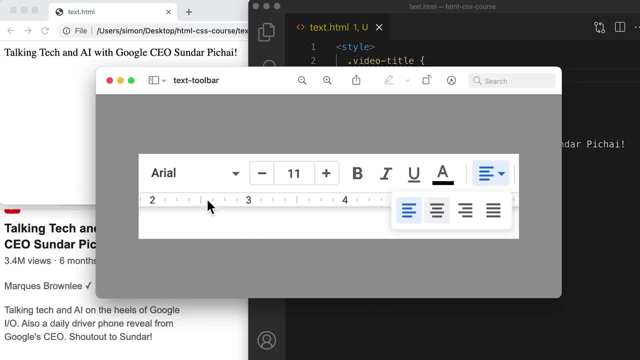 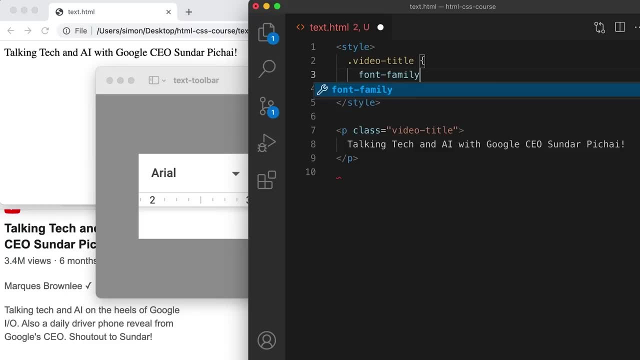 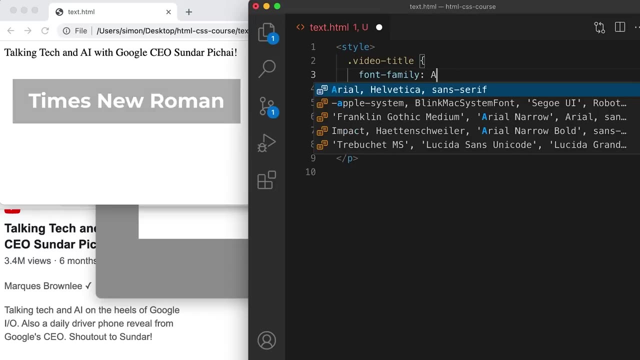 So the first thing we're going to change is the font. To change the font, the CSS property is font-family, So websites by default use the font called Times New Roman. We're going to change the font to a font called Arial. Save it. 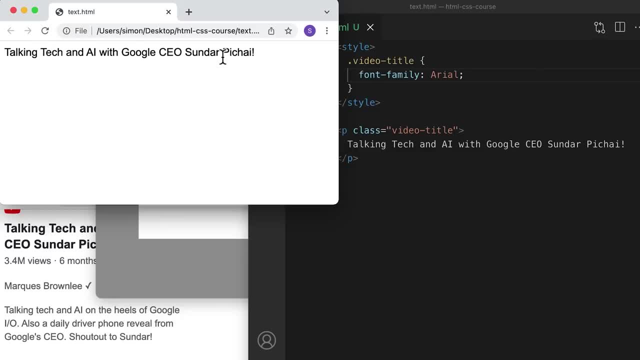 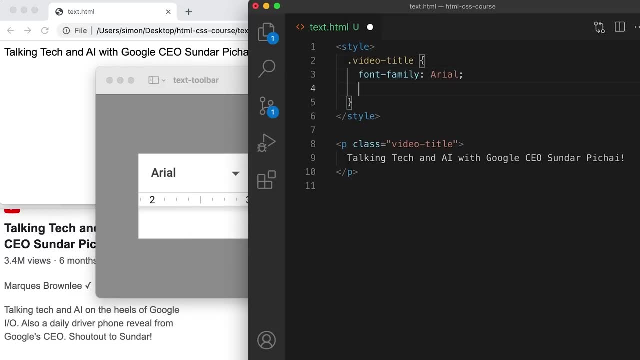 and refresh, and now you can see we changed the font. Let's go to the next one. So this is the font size and we can change the font size using the property font-family- font-size. And let's change it to something like: 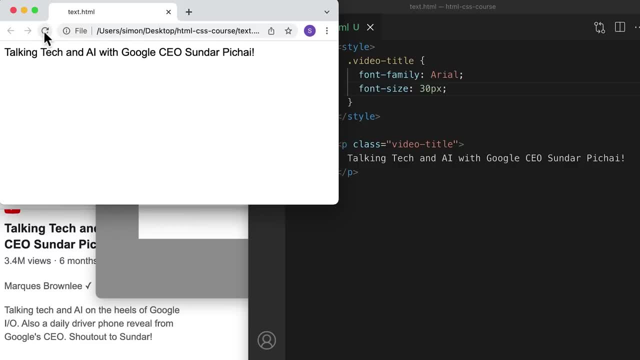 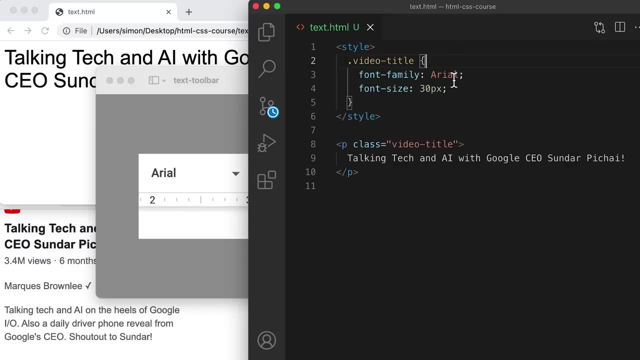 30 pixels, Save it and refresh, and now we have a bigger font. The next example is: let's make it bold. We're going to go here and we're going to set the font-weight to be bold, Save it and. 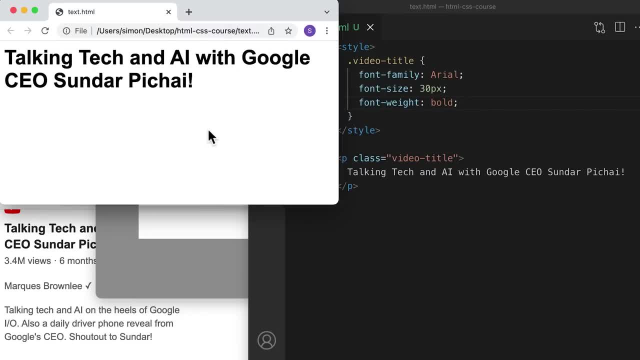 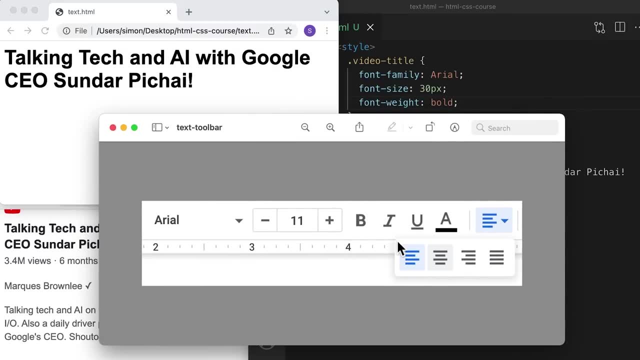 refresh and now we have bold font. So, as you can see, CSS has properties for doing all of these things, And for most of these properties, it's pretty easy to Google them. For example, let's Google for how to make a font italic. 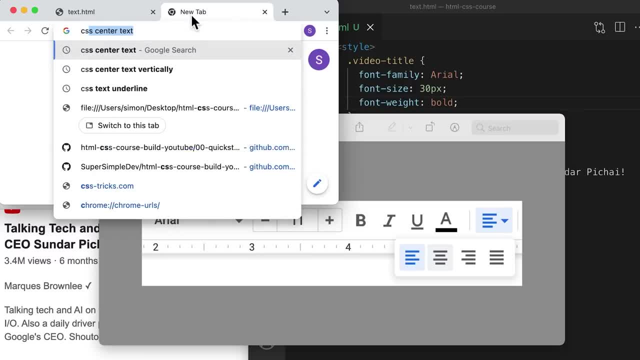 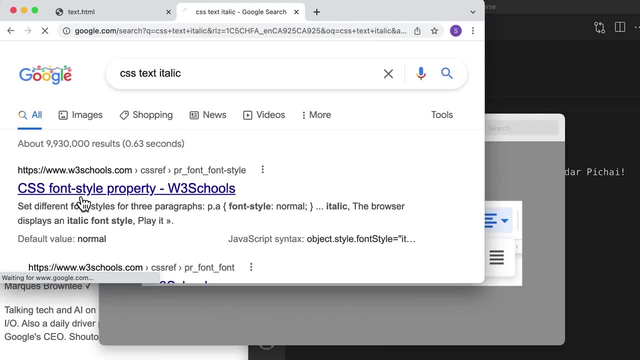 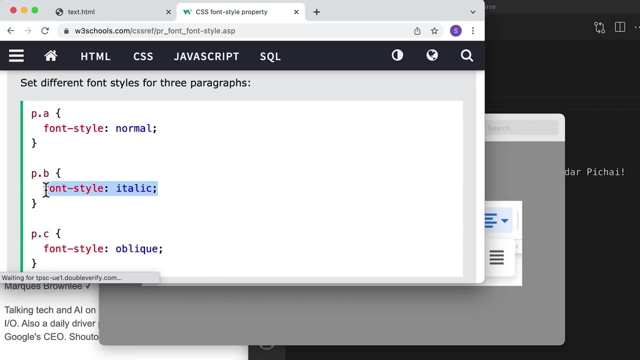 So we'll go to Google and we just need to search something like CSS text italic. And now in the first result we're going to go in here and if you scroll down you can see this CSS font style italic. So I'm going to copy this: 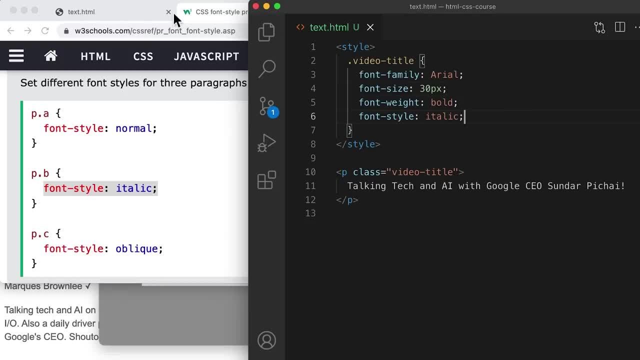 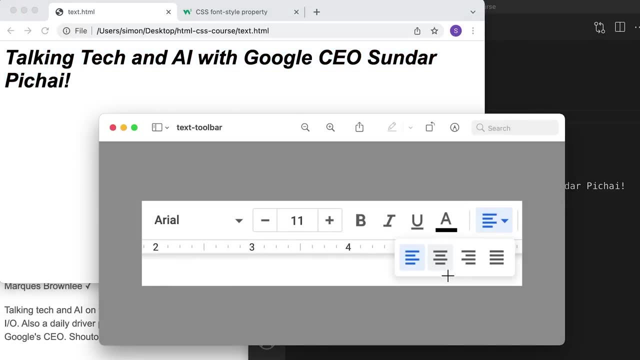 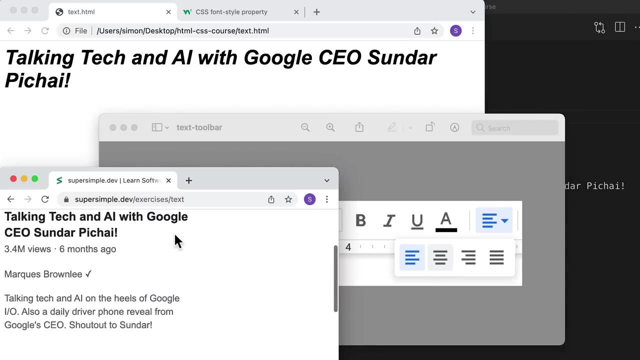 and paste it in my code, save it and refresh, and now we have italic text. The last one I'm going to show you for now is how to center this text, Because in our exercise we have an exercise where the text is centered To center. 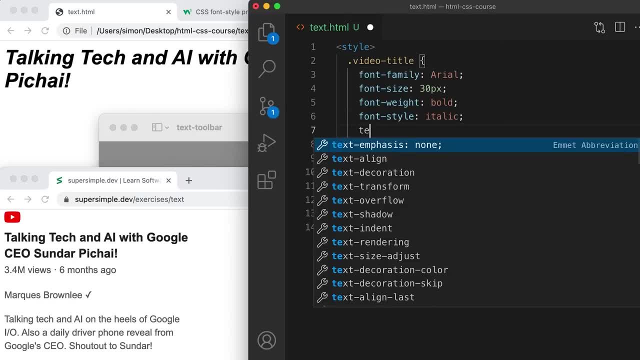 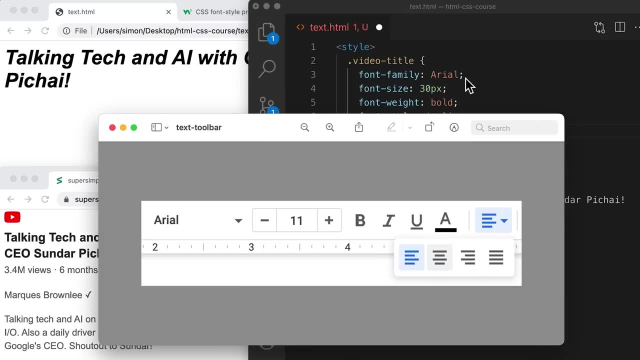 text. we're going to go to our code and we're going to type text: dash align. So this is the property for centering text, or putting it to the left or to the right. Now we're going to give a value of center. 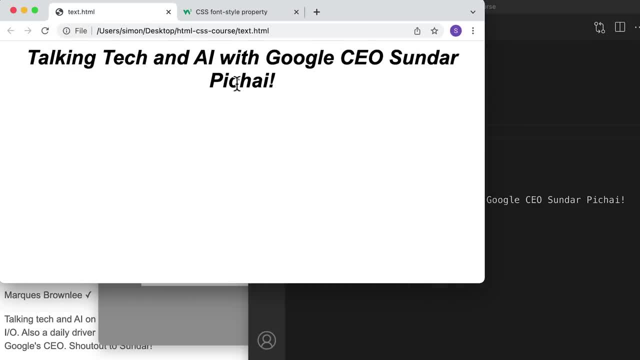 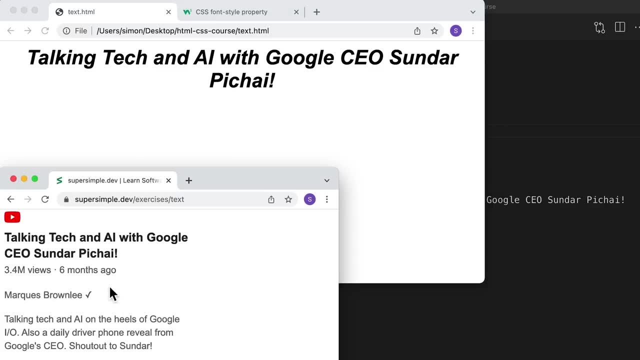 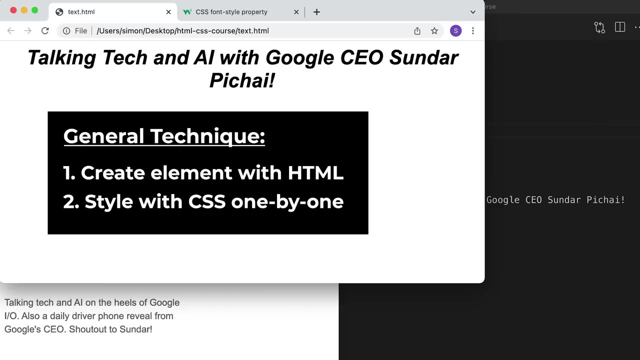 Save it and refresh, and that's how we center our text. So that was pretty easy. right Now, let's go ahead and try to copy this style in our exercise. So, if you remember, the general strategy for creating anything that we see is first: 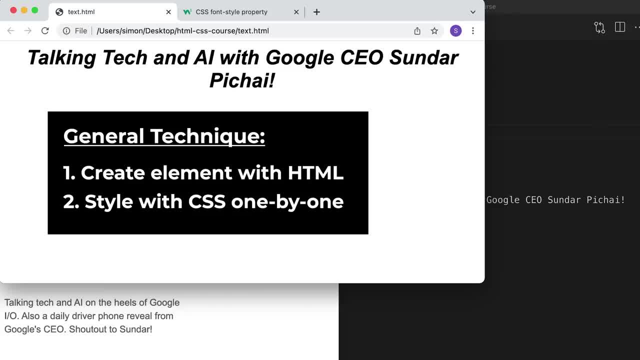 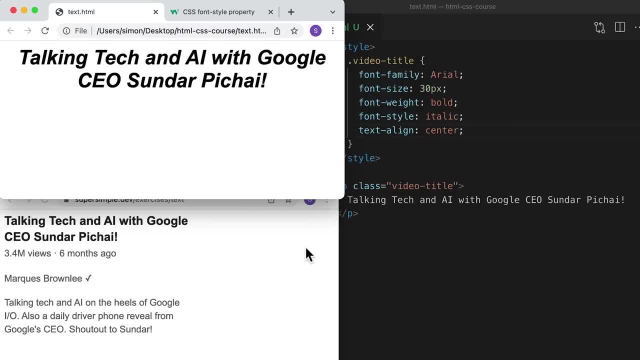 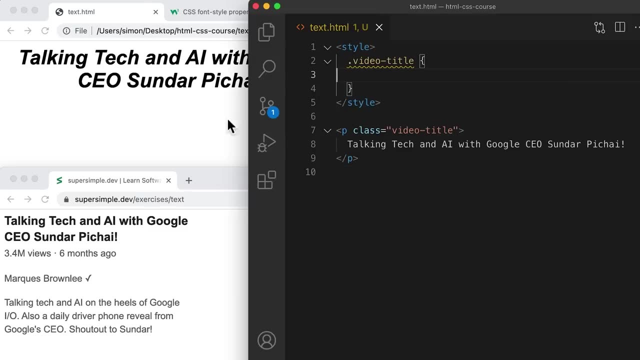 create the element with HTML and then style it with CSS one by one. Let's go ahead and do that for this exercise. I'm just going to resize this back and we're going to start by resetting all of these styles. Save it. 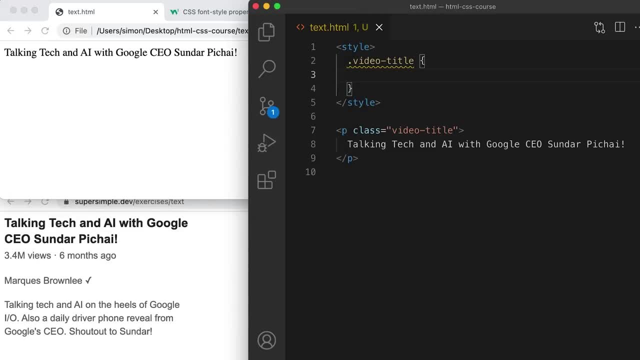 and refresh. First I'm going to start with the font family. So for this exercise I actually used the font family Arial, just to make it easier for us. So we're going to set the font dash family to Arial, Save it. 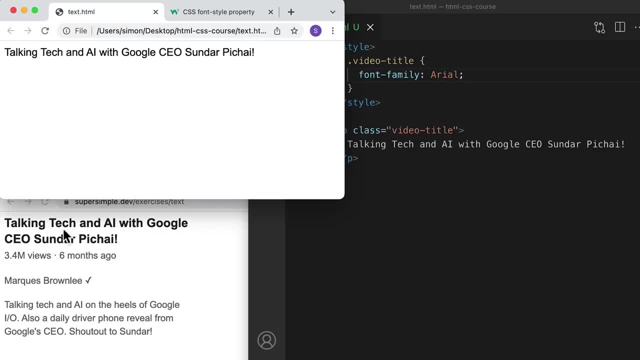 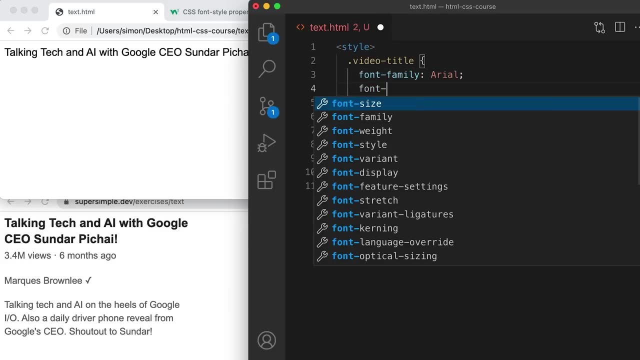 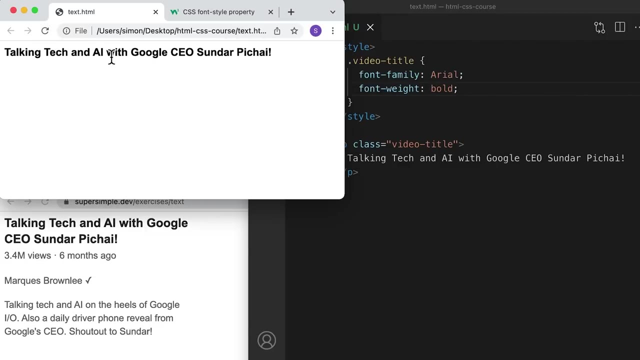 and refresh. Next I'm going to change the font weight. So this font is bold and I want to make my font bold as well. So we're going to add font dash weight bold, Save it and refresh. Next let's change the font. 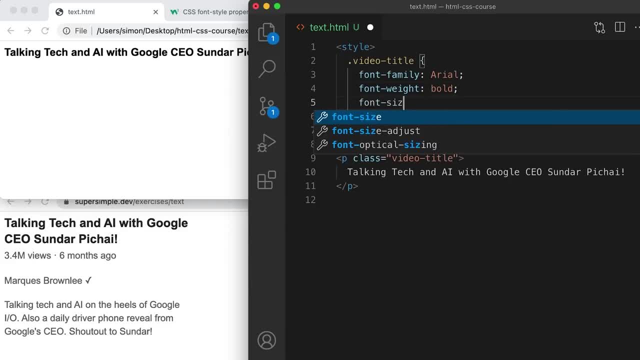 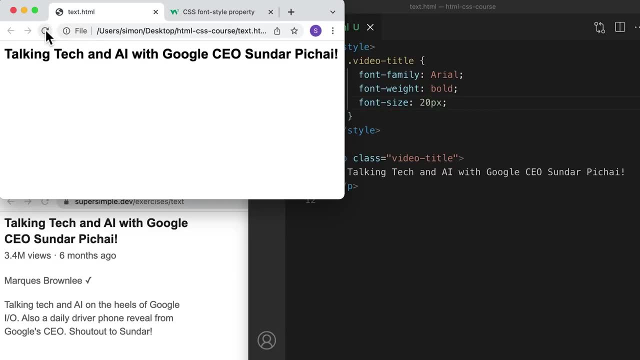 size. So I'm going to change this font size to something bigger, like maybe 20 pixels, Save it and refresh, And it looks a little too big compared to the design, so let's tone it down just a little bit. maybe 18 pixels. 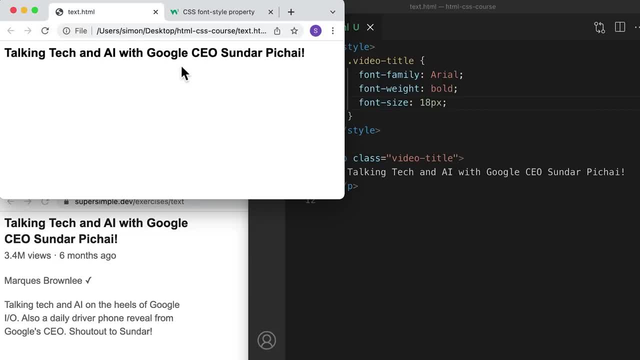 Save and refresh. Okay, so I think that looks close enough. Next, you'll notice that this text sort of wraps around to a second line, while ours doesn't. The way to make this happen is we're going to set a width on this title. 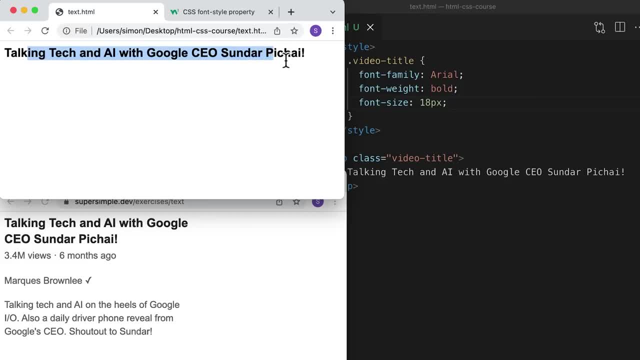 Now I know that in the previous section we said it's bad to set a width, but here it's actually what we want, Because if we set a width we're going to force the text onto a second line. So let's go ahead and set a width. 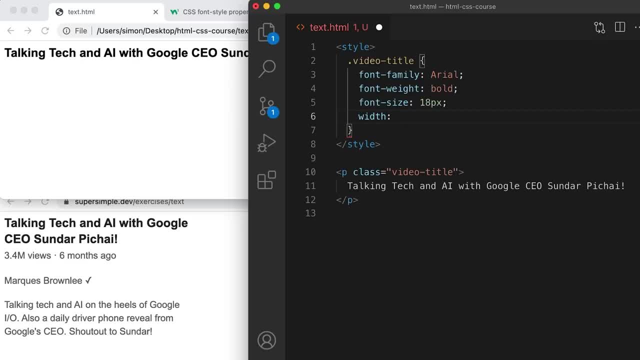 right now and I'll set it to something like 400 pixels. Let's see how that looks. Save it and refresh. Okay, so it needs to be less than that. Let's do 300 pixels: Save and refresh. Okay, so that looks. 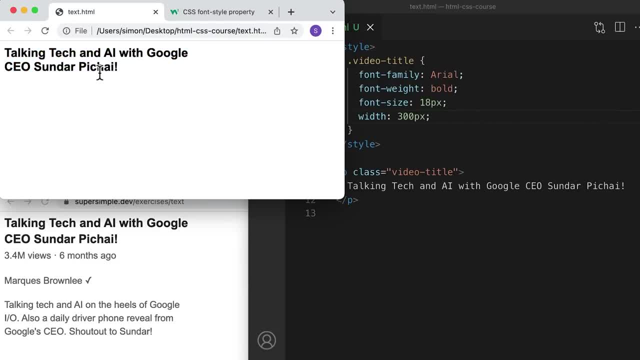 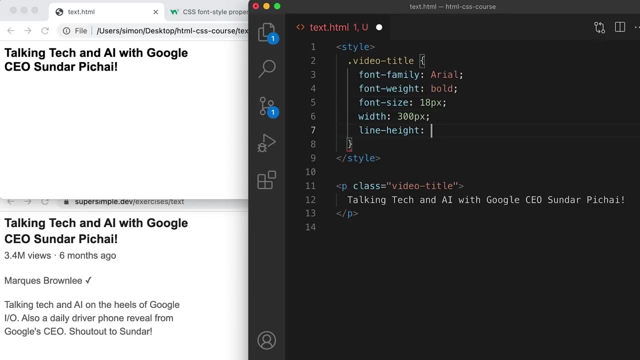 right to me now. And the final thing with the title is: I notice there's more spacing between the lines here than what we have. So to adjust the spacing between lines, the property is called line-height, So don't worry if it seems like we're learning a lot of new properties. 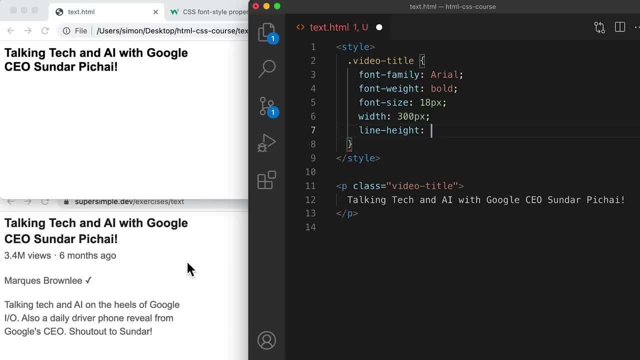 The point of this lesson is for us to go through some complicated examples together, which will prepare you for the exercises that you can practice on your own. So for this line height, let's try something like 20 pixels. Save it and refresh. 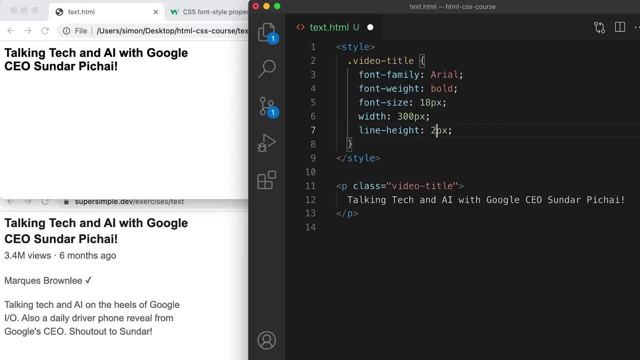 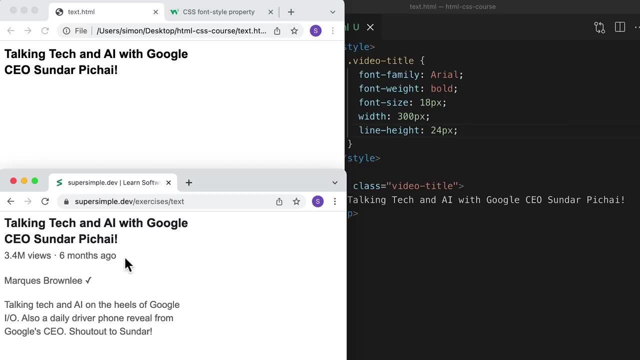 Okay. so it looks like that didn't work. Let's change it to 20, 6, maybe. Save it and refresh. Okay, maybe 24.. Save and refresh, Okay. so I think that looks pretty close. Next, let's work on the. 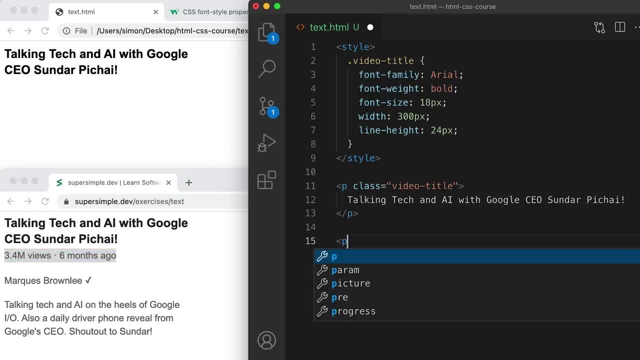 second paragraph. So we're going to create a new paragraph, 3.4 m views. And now to create this dot, we're going to create something called an HTML entity. So an HTML entity lets us type out special characters, For example, this dot, and. 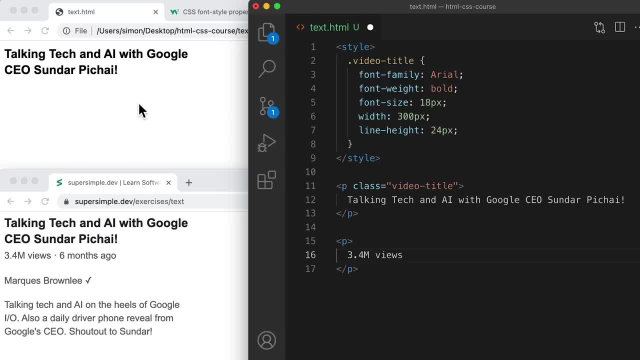 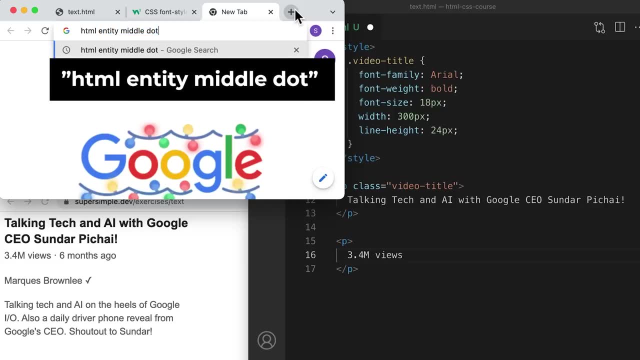 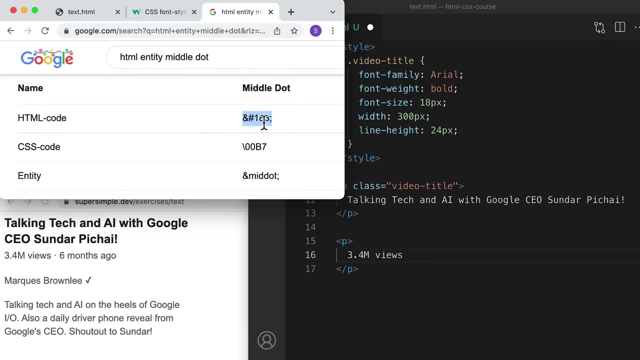 this checkmark To get the HTML entity for this dot. we're going to Google HTML entity- middle dot. And now, if we scroll down, this will give us some HTML code that we can copy into our code. So I'm going to copy. 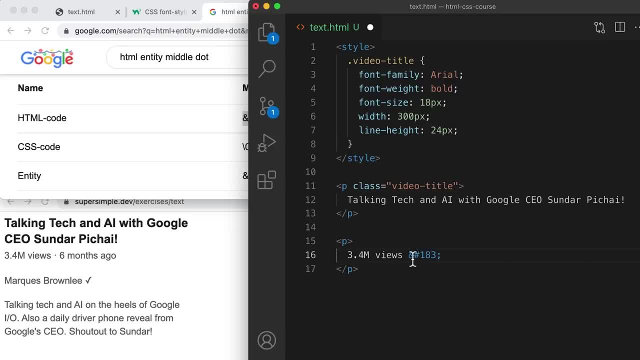 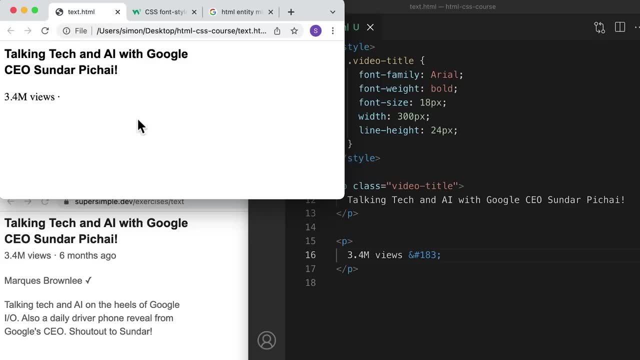 this and then paste it here And that's going to create a dot on our page. So if I save it and refresh, that's what we get. Now I'm going to type out the rest of the text in this paragraph. 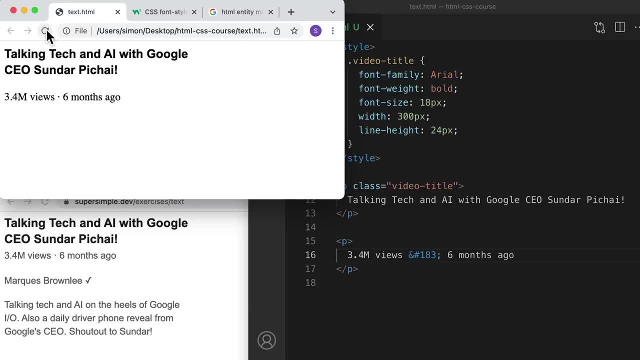 Now let's save that and refresh. So now, remember, the general process is: we created the element with HTML. now we're going to style it one by one. First, let's give this a class So we can target it. Let's call this video: 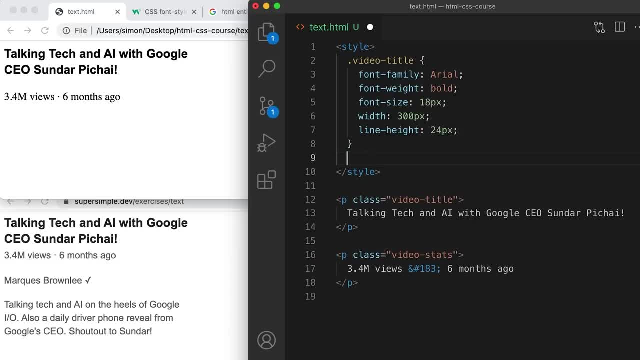 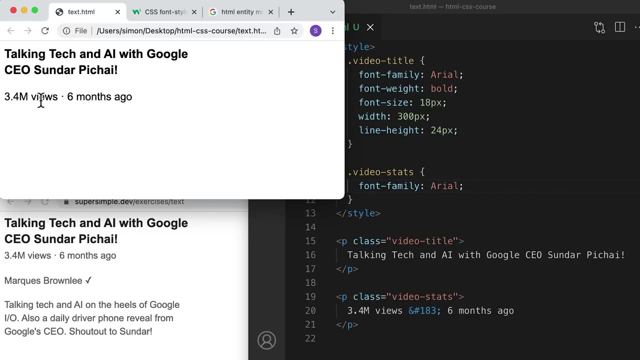 dash stats. And now in our CSS we're going to style this text. We're going to start with font-family, arial, Save and refresh, And then we're going to change the font size. So it looks like our design is a little bit. 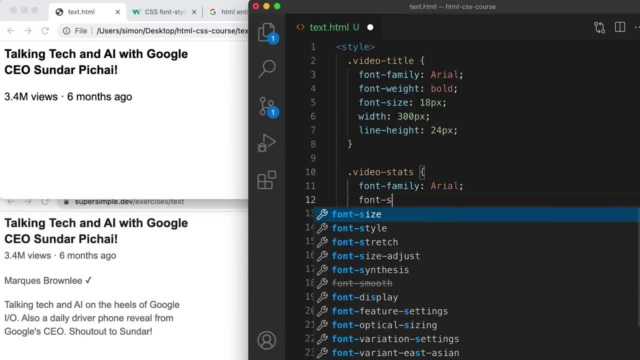 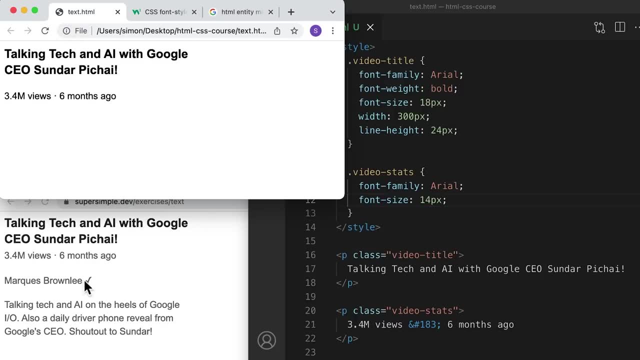 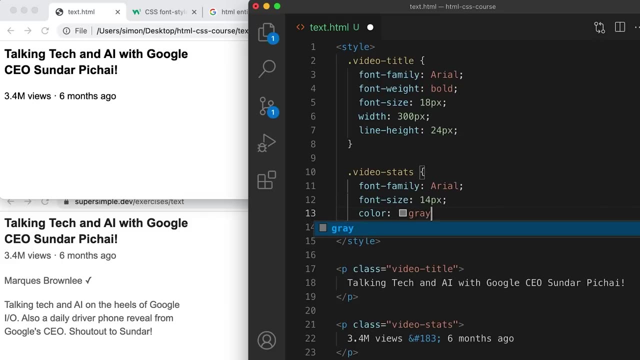 smaller than what we have. Let's change the font size to maybe 14 pixels, Save and refresh, And I think that looks pretty close. Next, let's change the color. So let's set a color of maybe gray And refresh. 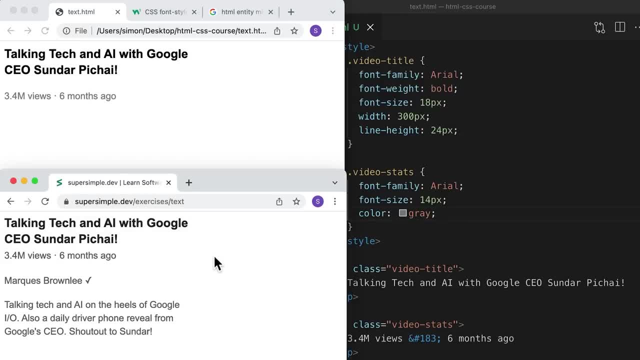 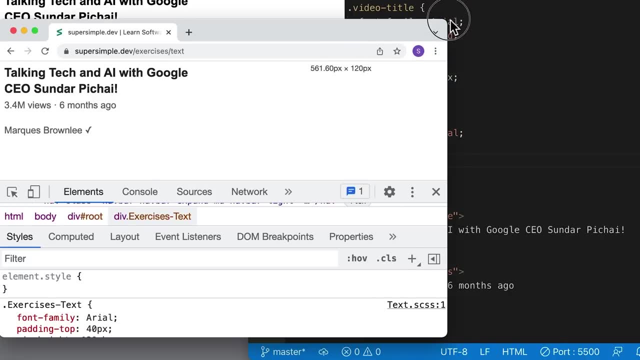 Okay, so that's a little too light. So to get an exact color we can right-click in a blank area of the webpage, click inspect, and then we're going to inspect the styles of this element. So the trick to doing that is we're going to click. 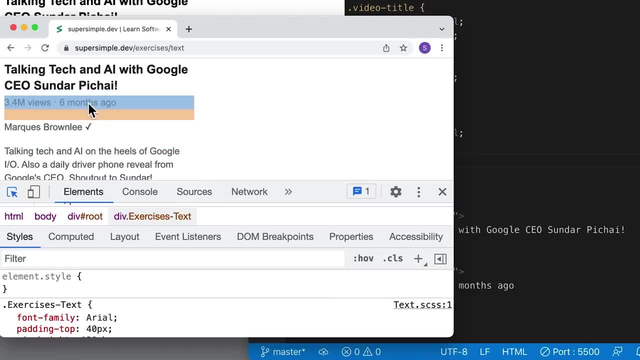 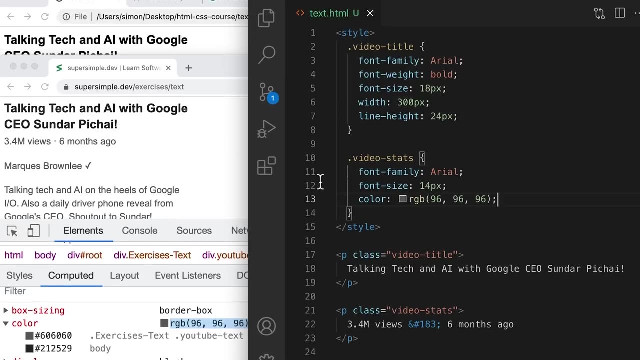 this top left icon. hover over this element and click it, And then we can find all its styles in the computed tab. So if we scroll down, we can get the text color. So let's copy this and save Refresh. 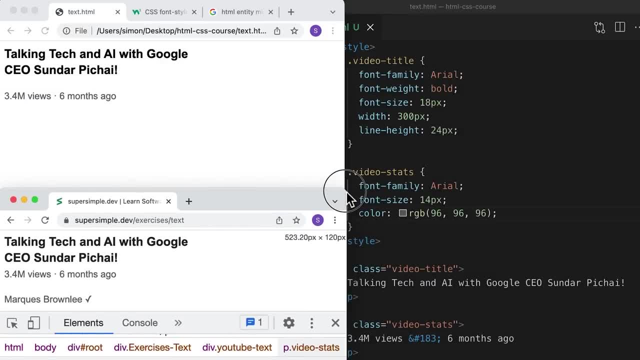 And that looks pretty good compared to the design. Next, let's adjust the spacing between these two paragraphs. So remember from the previous lesson: the spacing outside of an element is called the margin. But if we look at our code, we didn't. 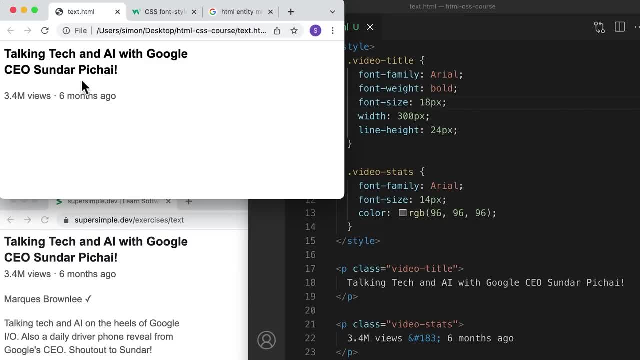 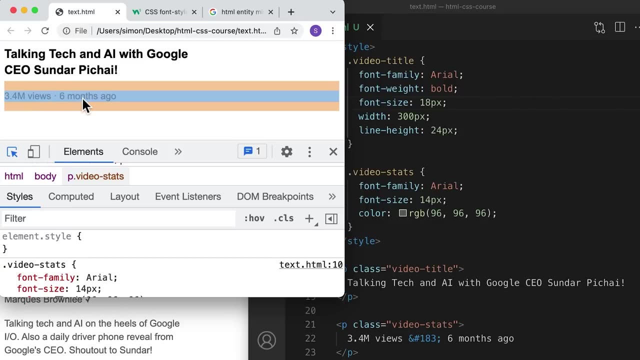 actually set any margin yet. So why is there so much space between these two paragraphs? And the reason is, if we right-click in an empty area of the webpage and click inspect, and we click this icon and hover over this paragraph, this paragraph. 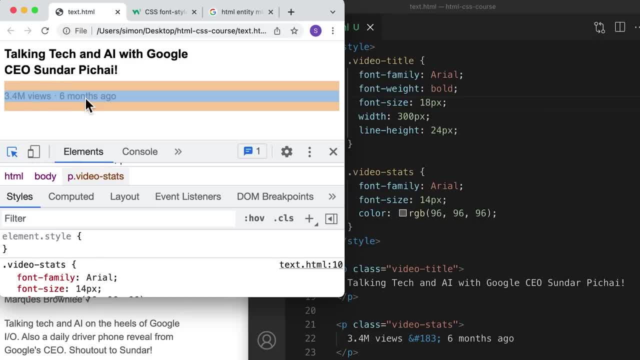 already has margin at the top and bottom. So if we click this go to computed, it has 14 pixels of margin at the top and 14 at the bottom, And the same thing for this paragraph, And the reason for this is because paragraphs by default. 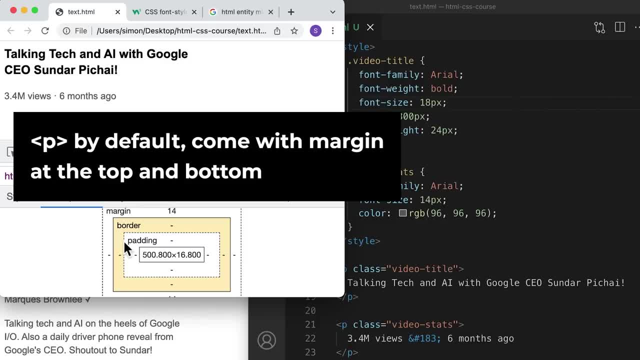 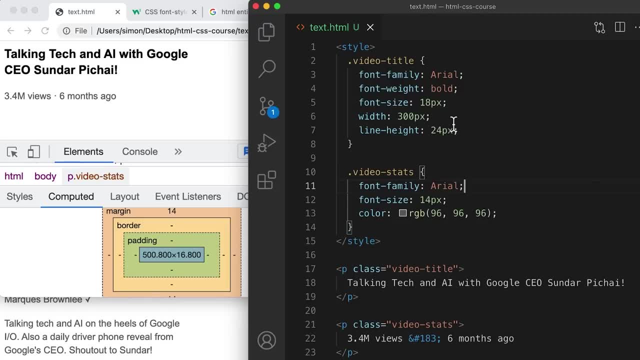 come with margin at the top and at the bottom. So that's why there's all this spacing that we have here, where we didn't set it in the CSS. So the general process is we're going to remove the default spacing and then 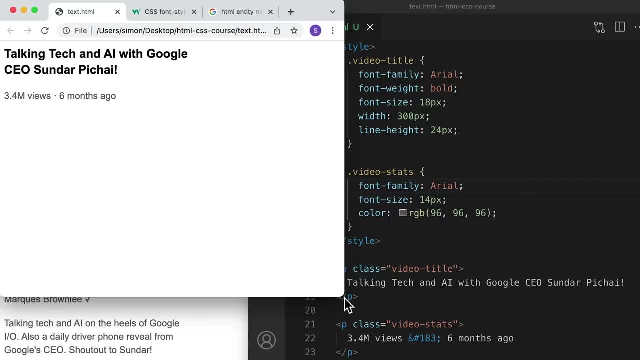 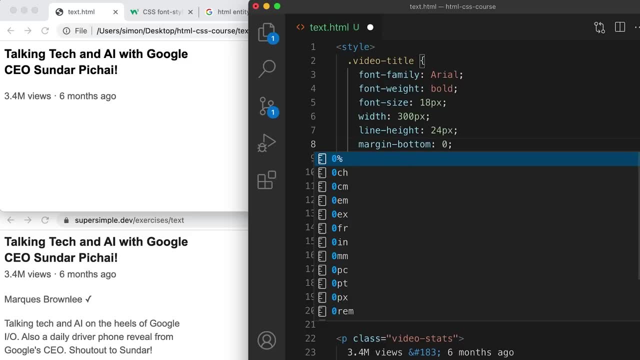 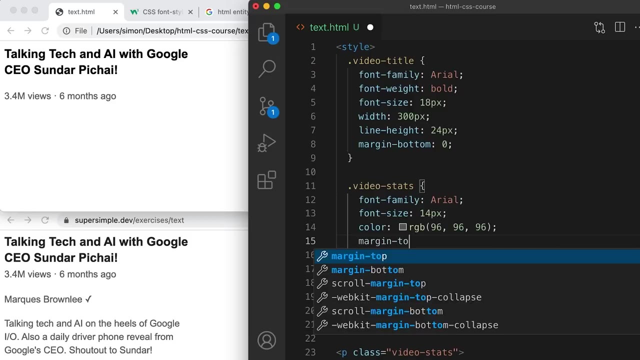 we're going to set our own spacing. So let's go into our code, and first we're going to remove the margin dash bottom of the title, Set that to zero. and we're also going to remove the margin at the top of the second paragraph. 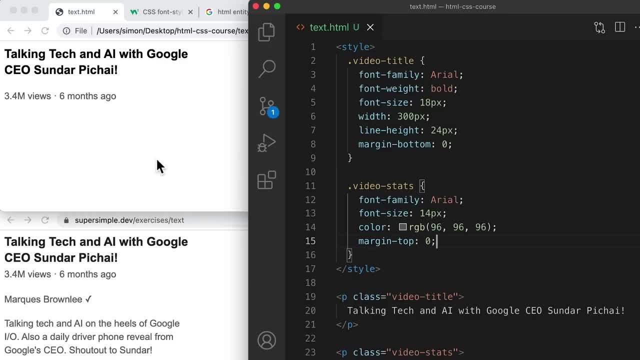 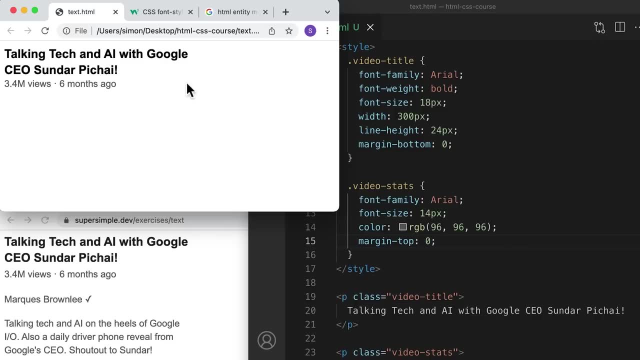 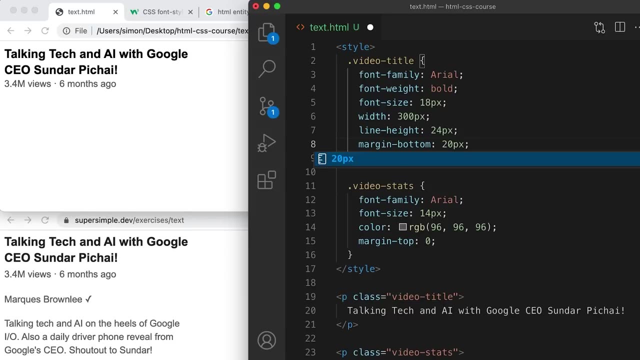 and set it to zero. Save that and refresh. and now there's no default spacing between these and they're really close together. Next, we can set a more precise margin bottom. So let's set it to maybe 20 pixels. Let's see how that looks. 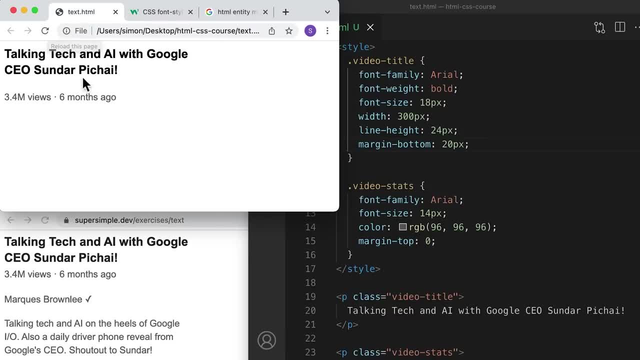 Save it and refresh- Okay. so that's way too much space. let's tone it down to something like maybe 5. Save and refresh- Okay. so I think this looks pretty close to the design, actually. Let's move on to the. 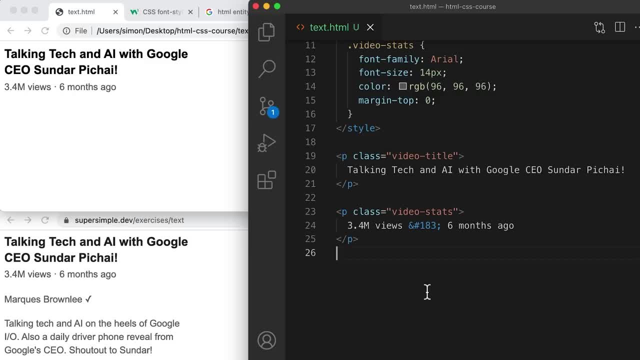 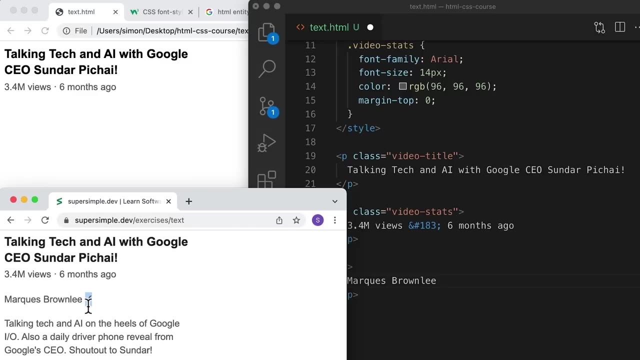 next paragraph. We're going to move all the way down and create a new paragraph element with this text inside. And now for this checkmark, we're also going to use an HTML entity. Now, I know that you can actually copy this and put it into our code directly. 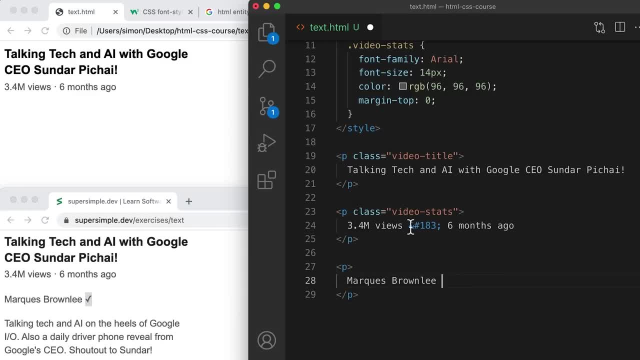 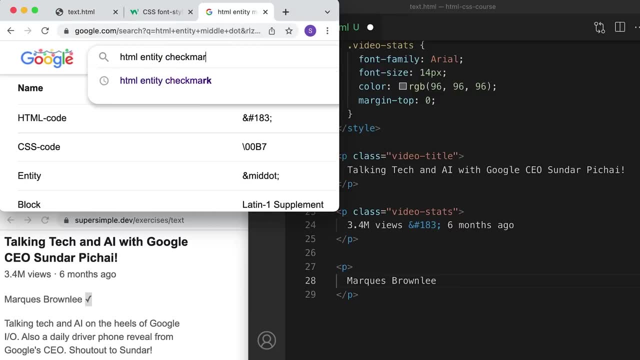 but some browsers might not support this, so that's why we're using HTML entities. We're going to go to Google and we're going to search HTML entity checkmark And I'm going to scroll down and grab the HTML entity here. 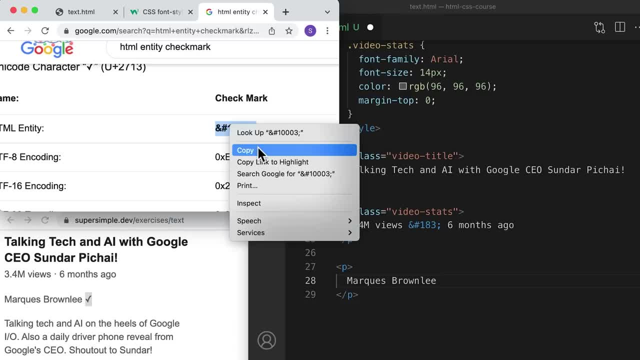 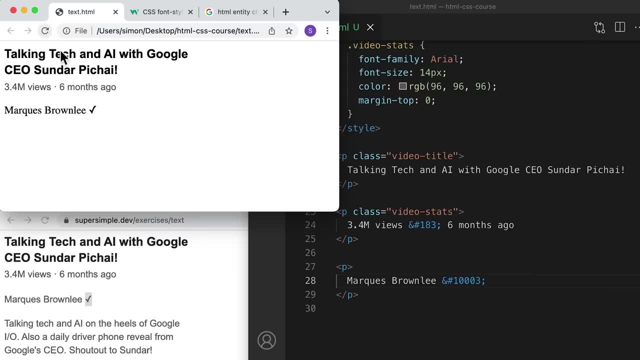 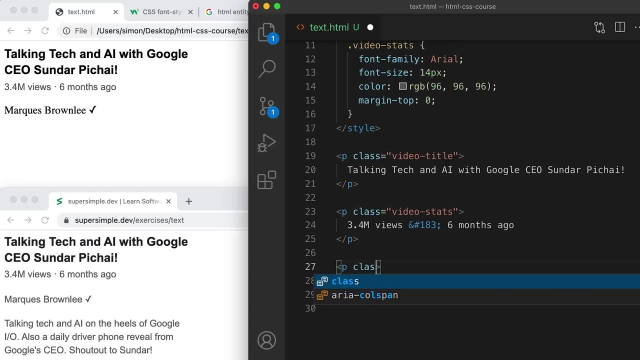 So here we actually have three. I'm just going to take the first one, Copy paste, save it. let's go back and refresh. Okay, so that looks pretty good. Next, let's keep styling these one by one. So I'm going to go a little bit faster here, because 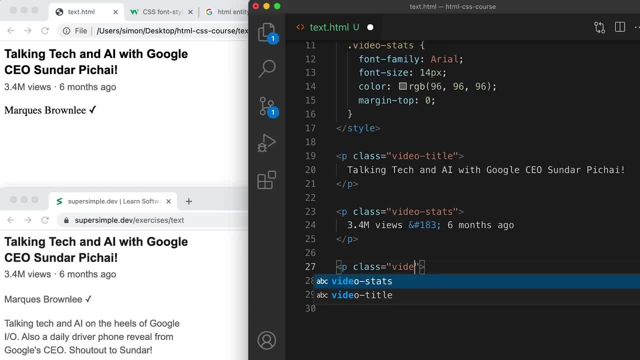 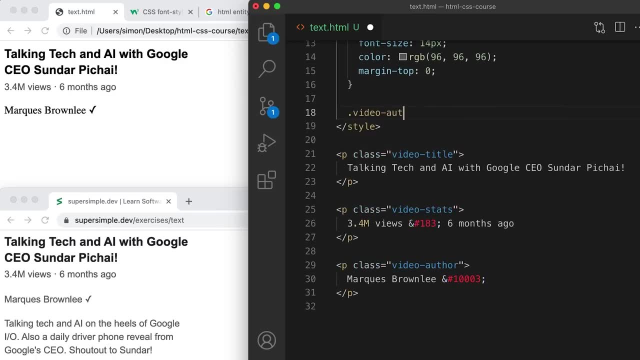 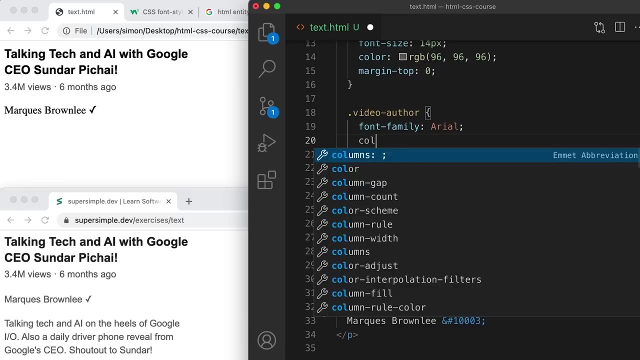 it's basically the same thing that we've been doing for the first two. Let's call this one video author and then we'll style it up here. So we'll set the font family to Arial, like the rest of the paragraphs. I'm going to set the color to the same as. 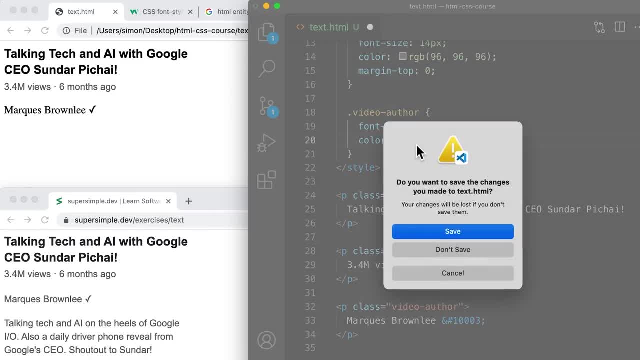 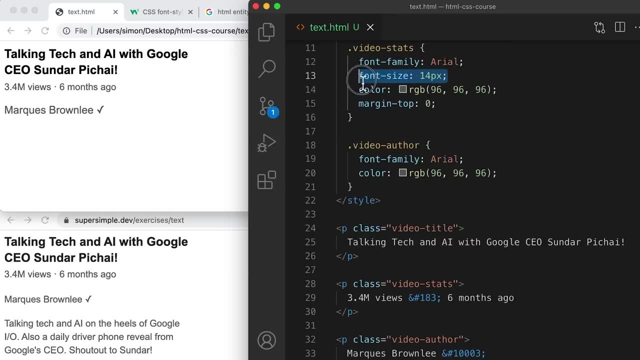 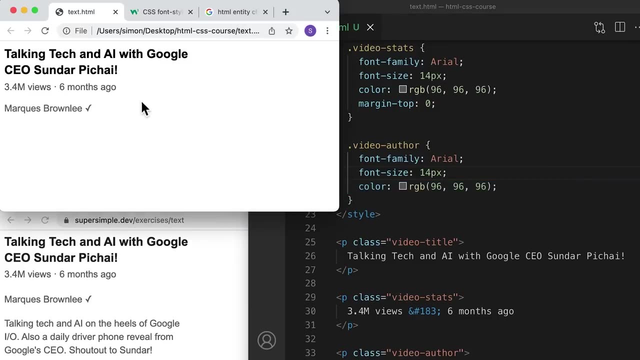 this paragraph, So copy and paste. Okay, that looks pretty good. Oh yeah, we have to set the font size. It looks a little too big right now. Set the font size to 14 pixels. Next we're going to reset the default spacing. 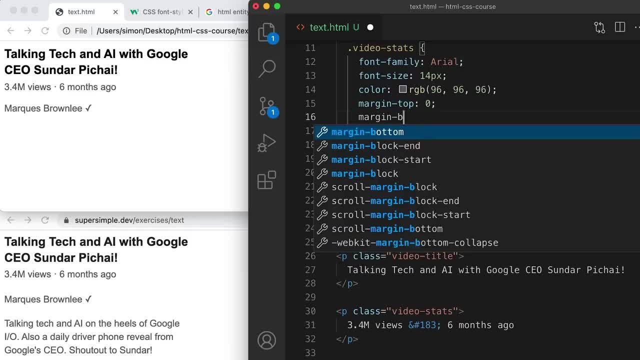 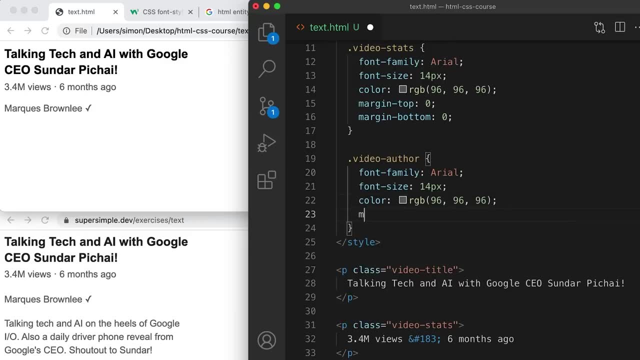 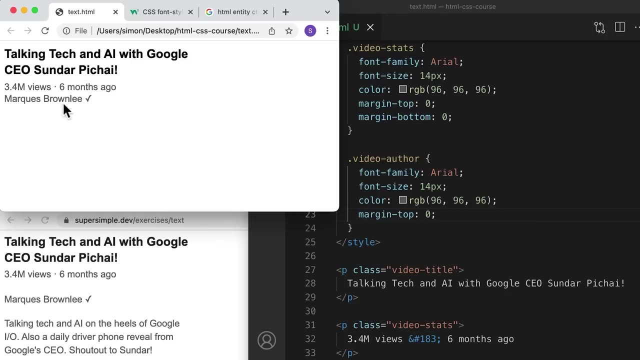 here. So we're going to set the margin-bottom and remove it by setting it to 0.. And also remove the margin top and set it to 0.. Save and refresh, And now we're going to set a more precise margin. So let's try. 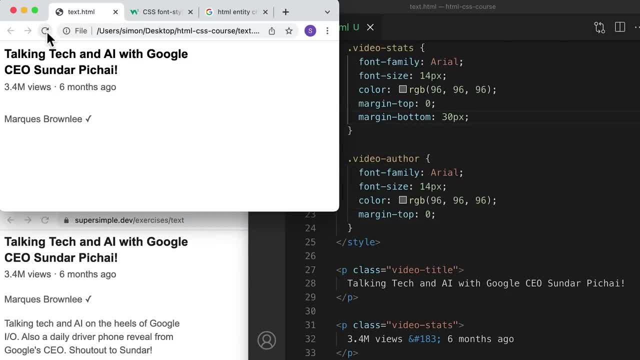 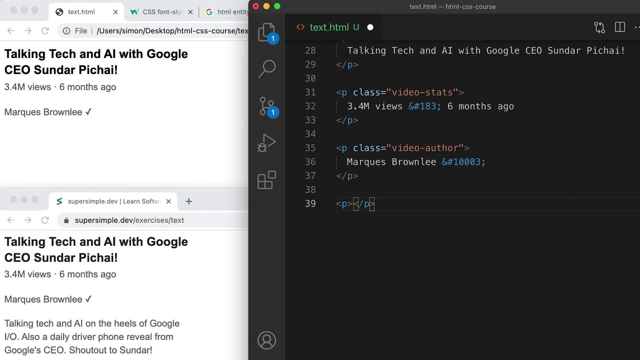 maybe 30 pixels. See how that looks. Okay, that's way too much. Maybe 20 pixels? Okay, I think that looks about right. Then we're going to do the third paragraph. Let's go down here: create the element. 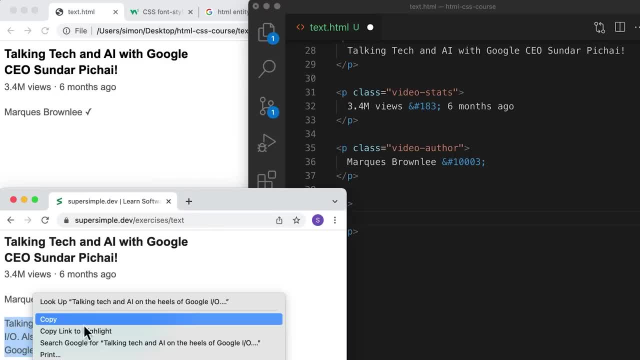 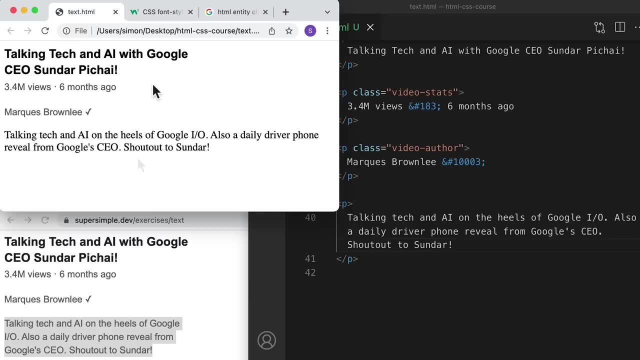 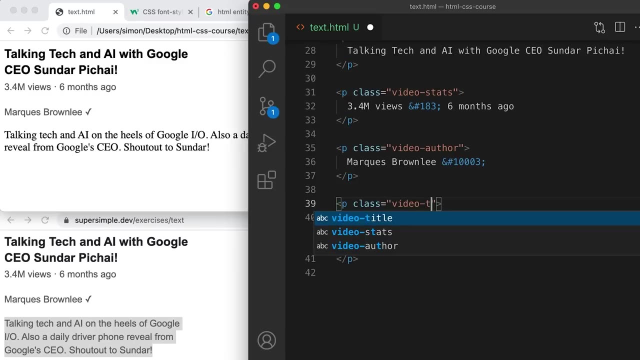 and then style it with CSS. I'm just going to copy and paste this in here: Save and refresh. First, let's give a class to the text so that we can target it. Let's call this video-description: Go up here: 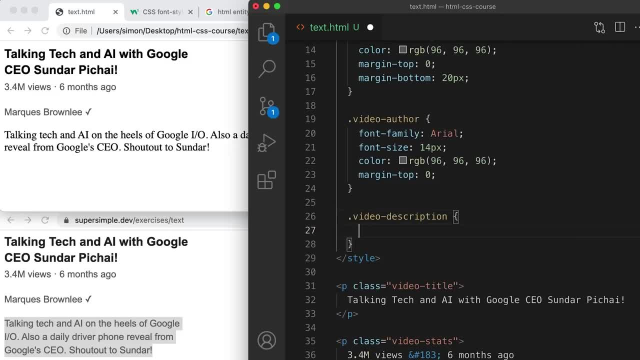 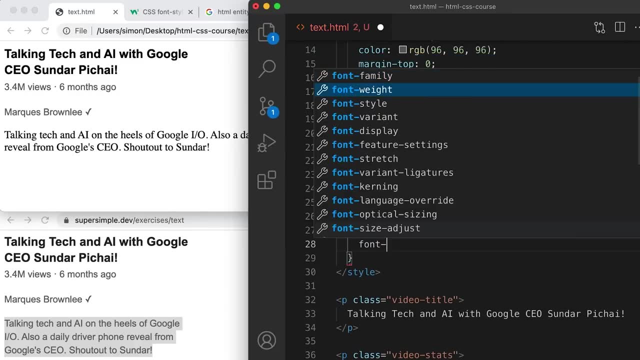 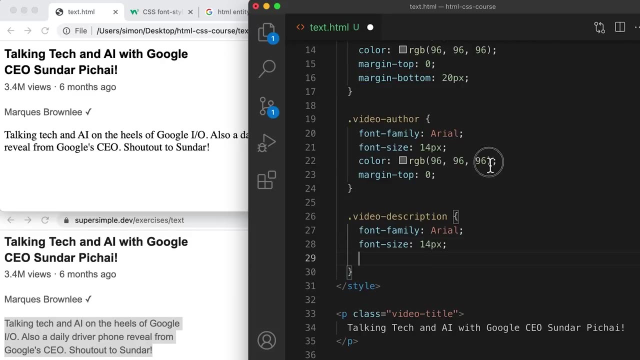 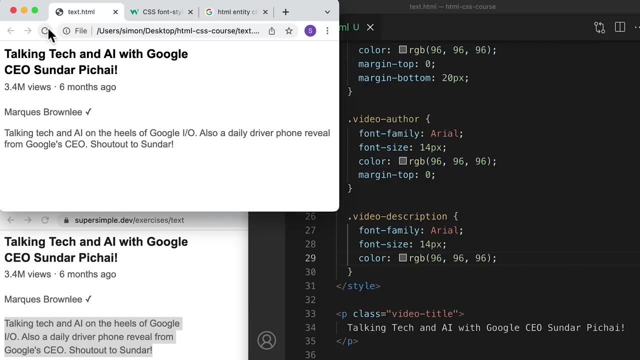 video-description. We want a font family of Arial, a font size of 14 pixels and the same color, And we save it and refresh. Okay, that looks pretty good, And now we want to give it a width to make it wrap around. 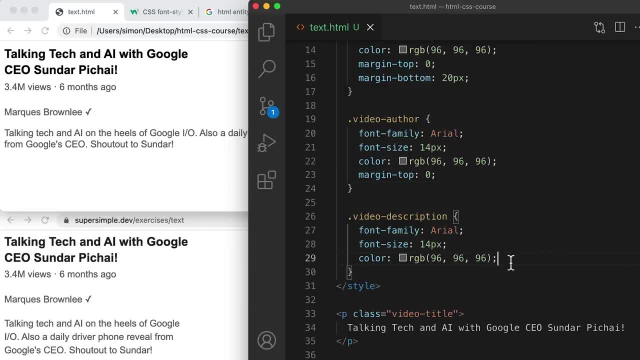 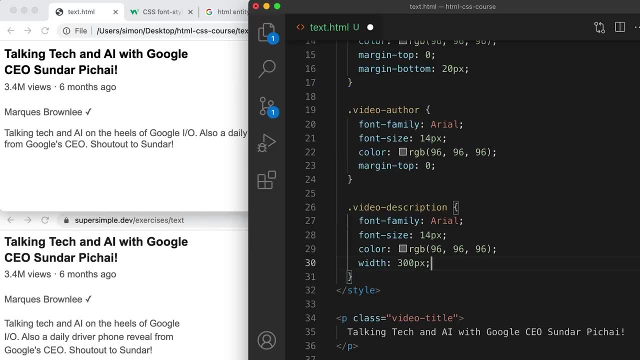 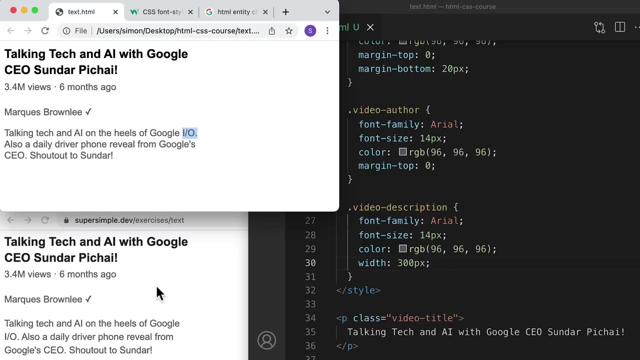 like this. So let's set the width to the same as the title, which is 300.. Width: 300.. 100 pixels. Save and refresh. Okay, so it looks like this IO is actually on a separate line. Let's make it. 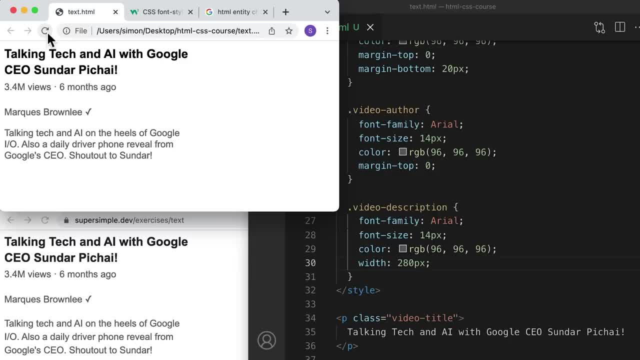 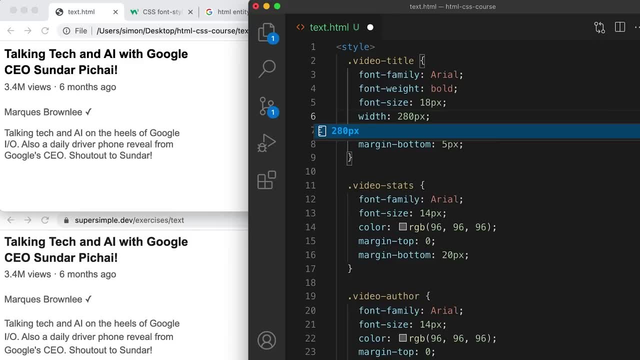 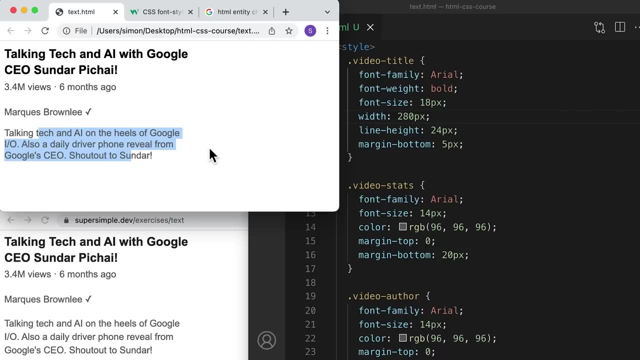 280.. Save and refresh. Alright. so that looks pretty good, And I'm also going to make it 280 up here, just to make sure they're the same. So the last thing I'm going to change is the height or the space between these lines. 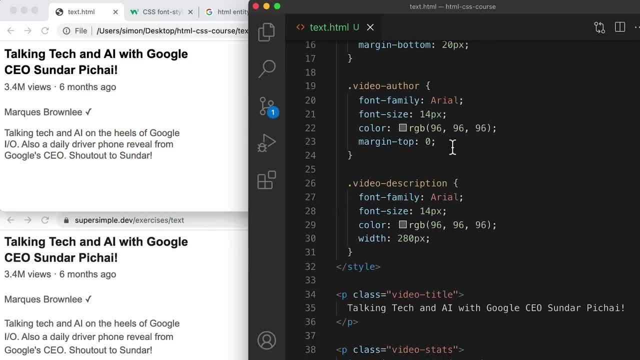 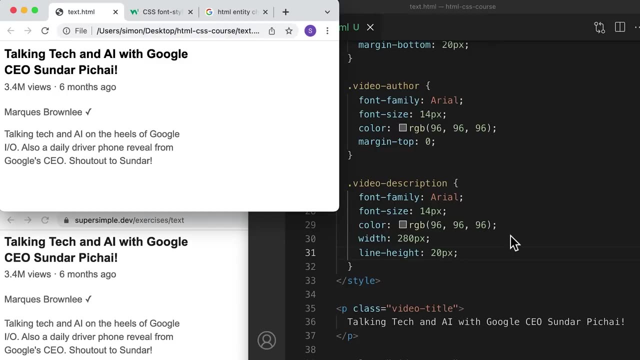 To do that, we're going to use line height. Let's scroll down and then add another property called line-height And let's set this to 20 pixels. Let's see how that looks. Save and refresh And let's set it to maybe. 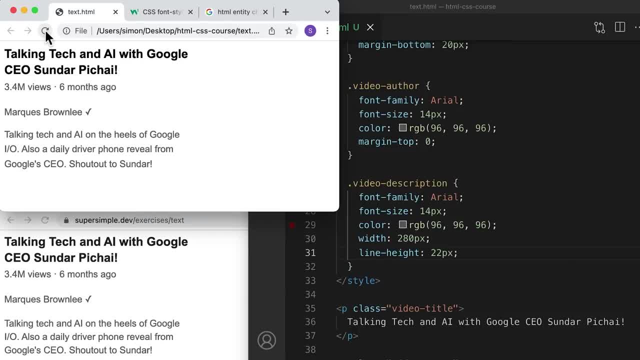 22 pixels. Save and refresh. Okay, so I'm pretty happy with this. And lastly, we're going to modify the space between these two paragraphs. First, we're going to reset the default margin. Let's get rid of the margin-bottom. 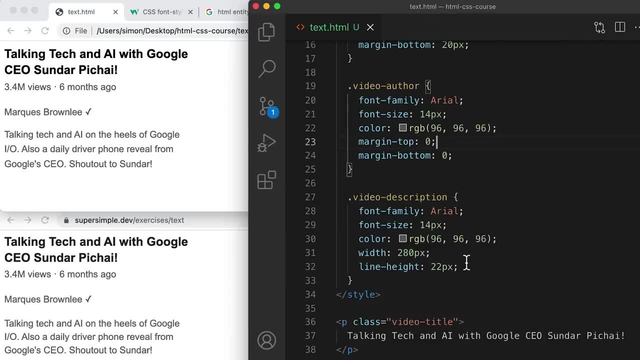 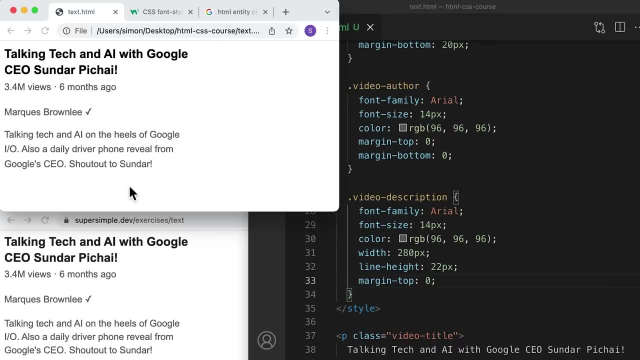 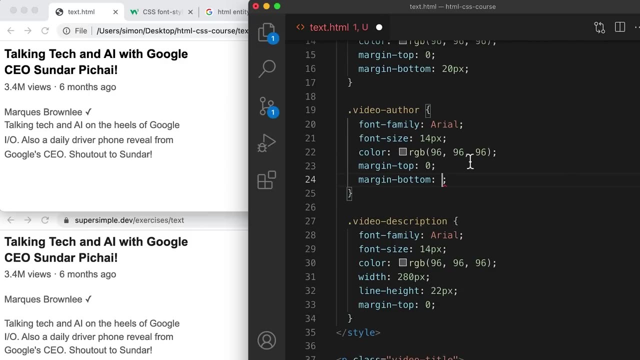 on the first one here and the margin-top on the second one. So, margin-top, I'm going to get rid of it and set it to 0.. Save and refresh And then we're going to set a margin-bottom, Maybe the same thing as up here. 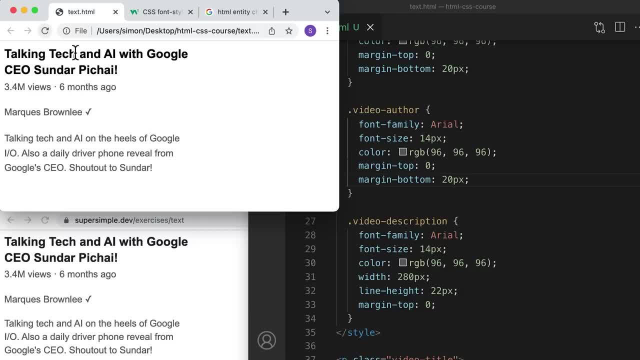 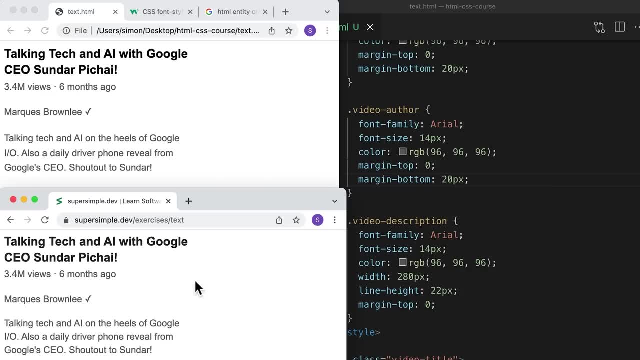 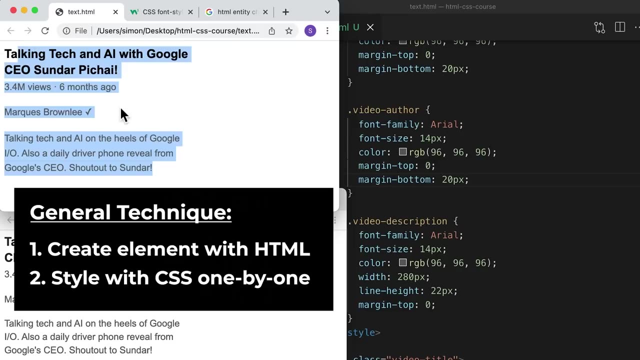 20 pixels. Save and refresh. Alright, so that looks really good to me. We just recreated a really nice looking style that you can find on youtubecom, And the general process that we use is: first we created the elements with HTML and then 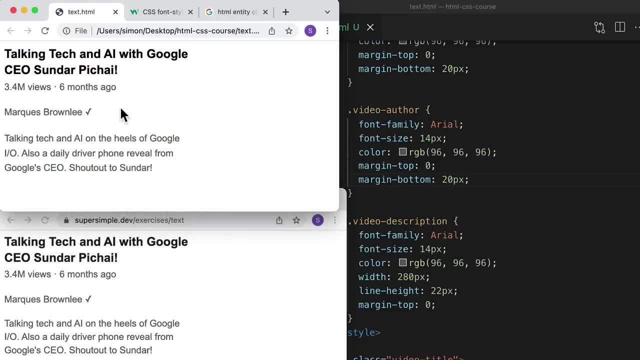 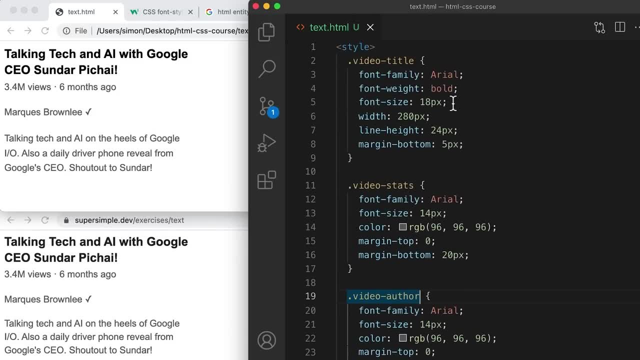 we styled them with CSS one by one. So before we move on to the next exercise, I'm going to show you a way to clean up our code. So, if you notice, all of our styles right now have a line called font-family arial. 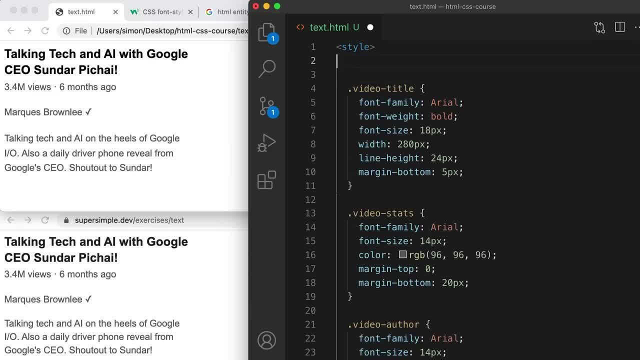 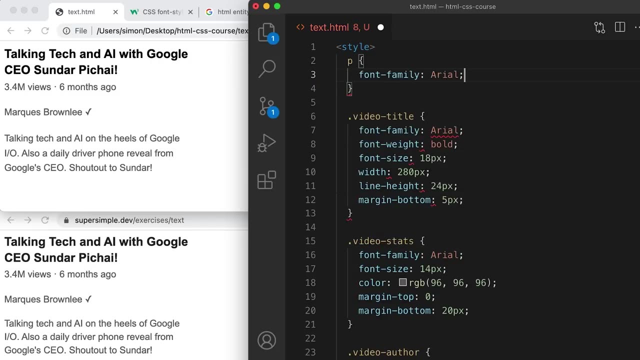 Now we can actually clean this up and remove the duplication by creating a new style. This time we're going to target all paragraphs on the page And we're going to give all paragraphs- font-family, colon, arial, Save. So this style is going to apply. 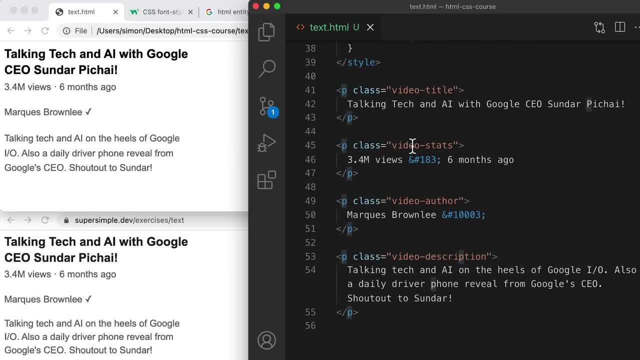 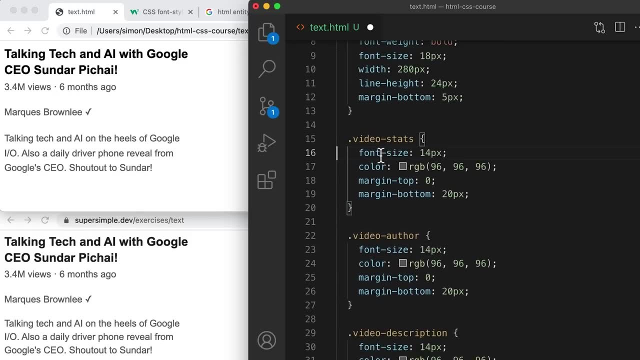 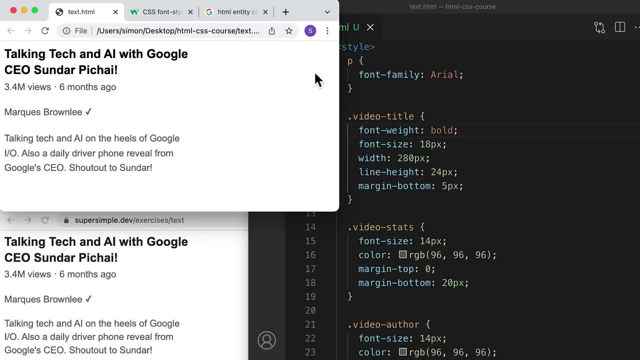 to all paragraphs, which means all of these. That means that we actually don't need this line in any of these class styles anymore, So we can actually remove all of these. Now, if I save it and I refresh, you can see that nothing changes. 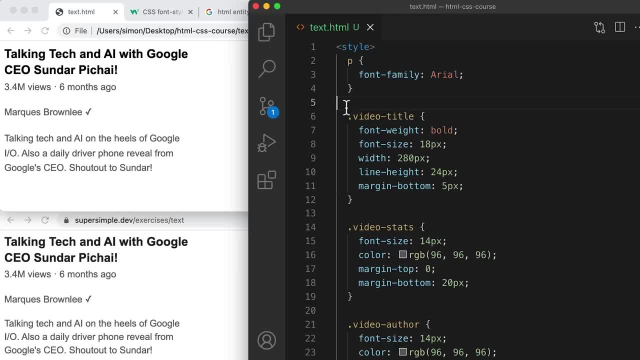 because this is doing the same thing as the code that we had before. So you can also see from this example that an element can be targeted by two sets of styles. For example, for this code, here we're targeting all P elements on the page and 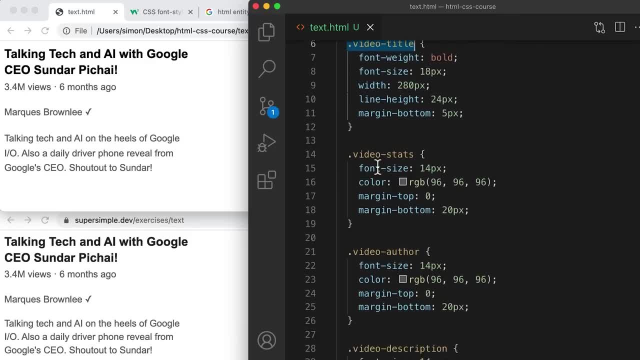 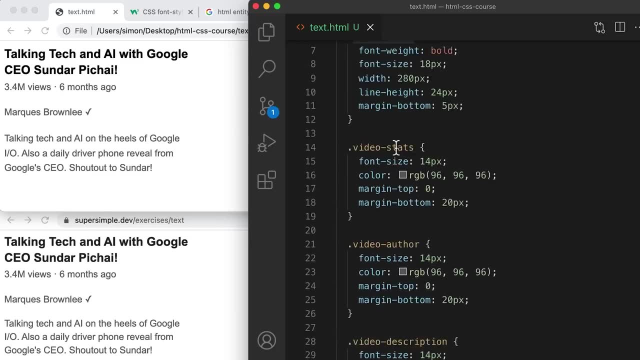 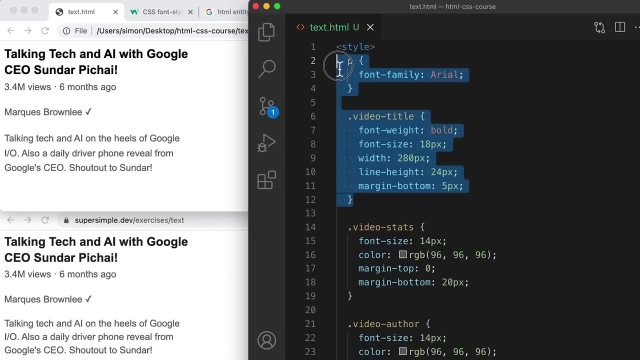 all elements with a class of video-title. If we scroll down here, here we have a P element that has a class of video-title, which means it's going to be targeted by both this set of styles and this set of styles. So it's being targeted by multiple sets of styles. 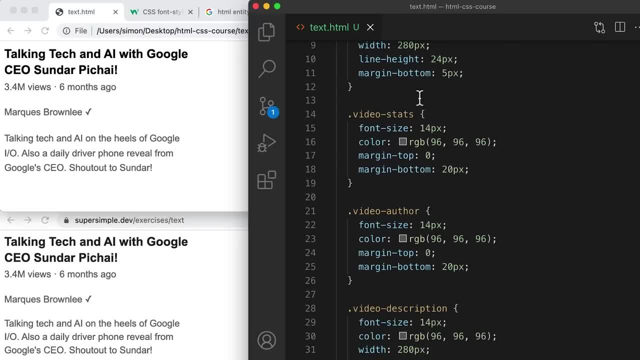 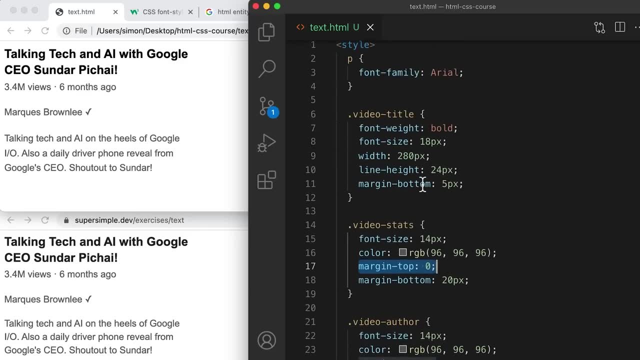 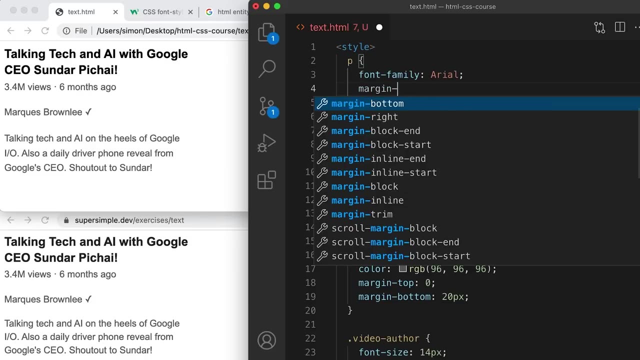 Now, another thing that we can clean up is remember how we reset the margins for all of our paragraphs, Instead of doing it for each one individually. we can actually put it all up here, So, for example, we can set the margin dash top to zero. 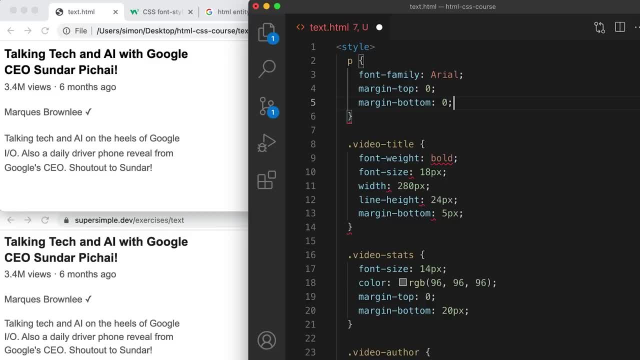 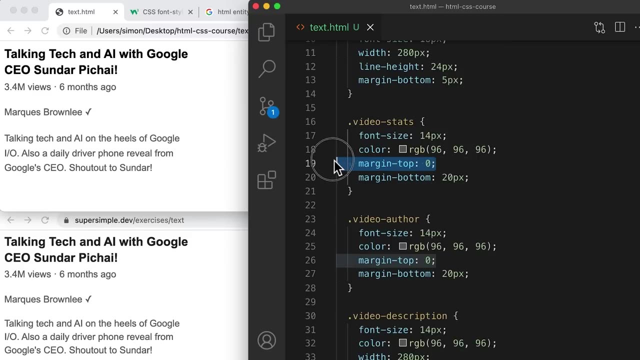 and the margin dash bottom to zero. We save it and we refresh. It looks pretty much the same, except we're now cleaning up all of the default styles up here so that we don't have to do it in our code at the bottom. So we don't need. 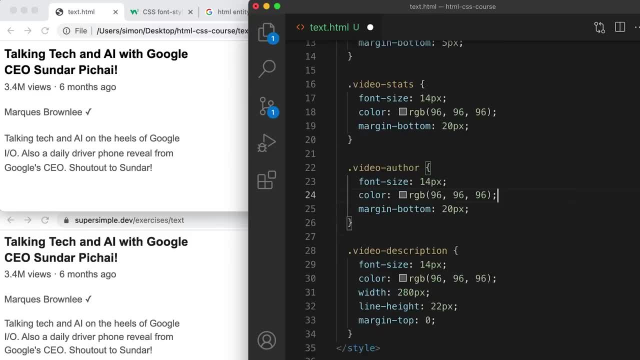 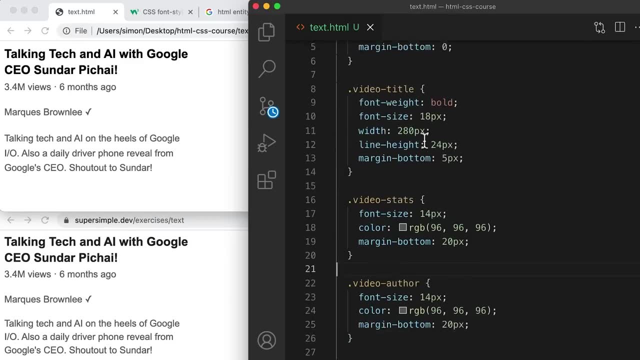 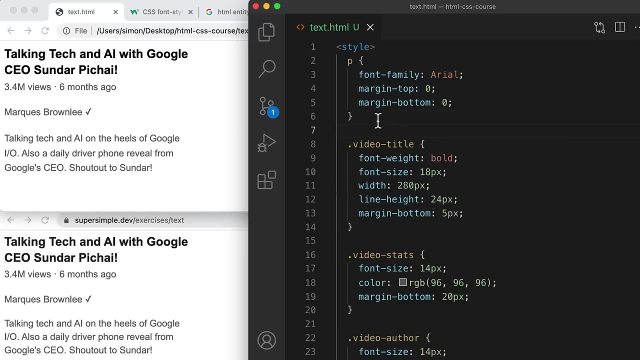 this anymore, or this or this, If we save that and refresh, we still get the same thing, because we've reset all of our styles in this set of styles. Now, the last concept I want to show you before we move on to the next exercise is: 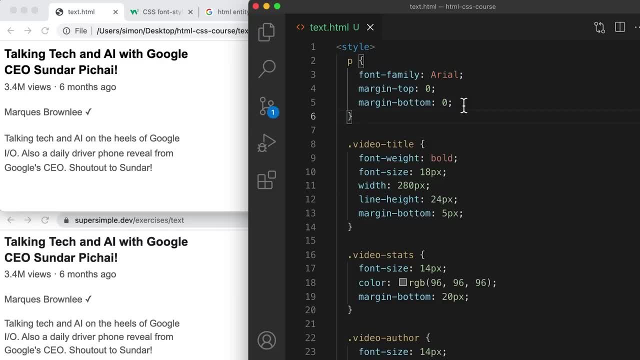 the fact that in this set of styles we're setting the margin bottom to zero, But here we're also setting the margin bottom to five pixels and the margin bottom to twenty pixels. So how does that work? We're setting it to zero here and to five and twenty. 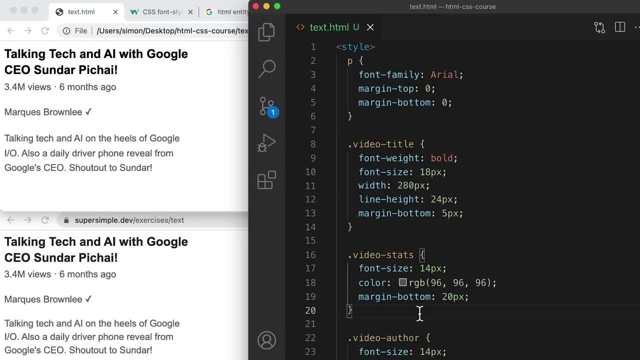 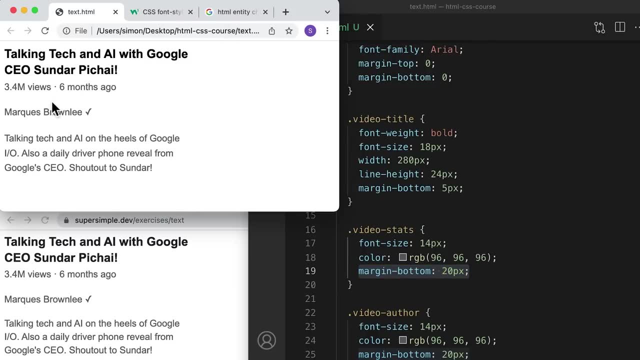 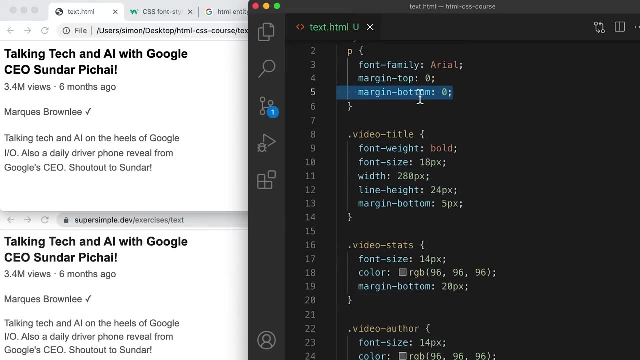 here. Which style does the element actually get? And the answer is: we're getting the style down here. So if we refresh, you'll notice that there's still twenty pixels of space between these two paragraphs. Now you might think that it's because this line is at the top. 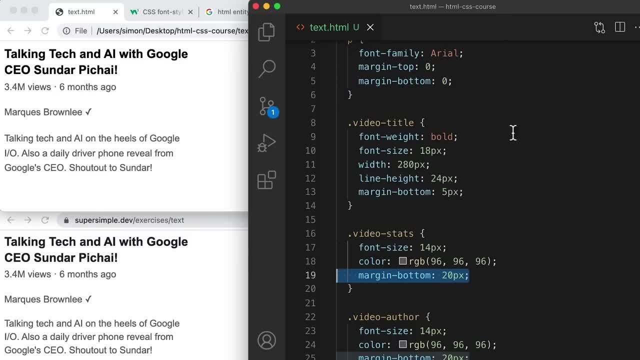 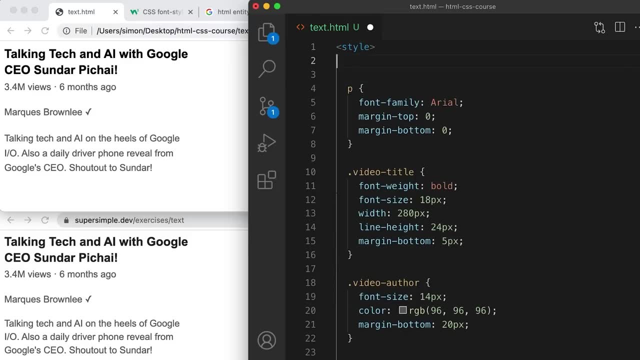 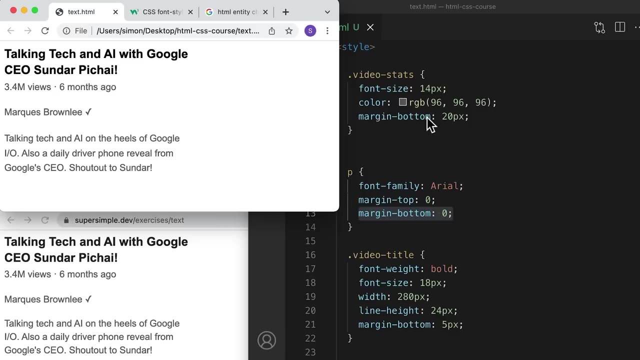 and then, once we get to this line, it overrides anything that comes before it. But if we actually move this to the top and we save and reload, you'll see that we still have twenty pixels of margin bottom. So why is this happening? This is something called CSS. 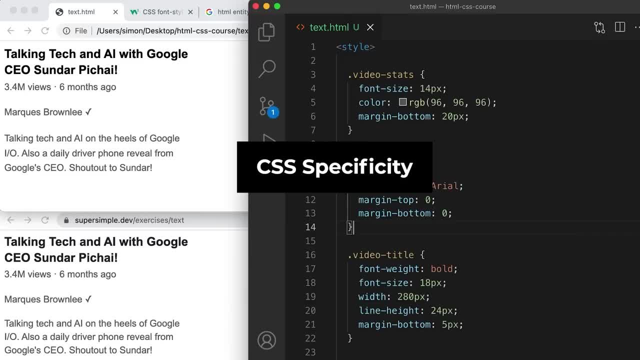 specificity. If we have multiple lines setting the same property, there's actually a priority that the browser follows. So in this situation, this style has more priority than this style, And to determine which one has more priority we have to look at this word before the brackets. 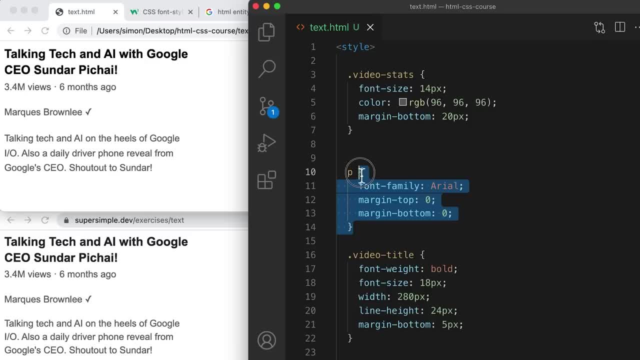 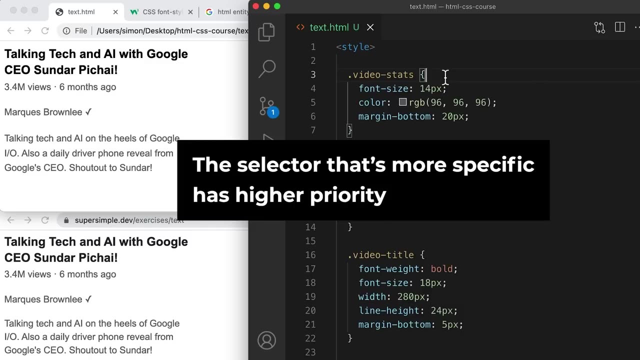 So this word tells us what these styles are targeting. This is known as a selector. This is another selector that targets a particular class. Now, the selector that is the most specific is going to have higher priority, So this selector is actually more specific than paragraphs. 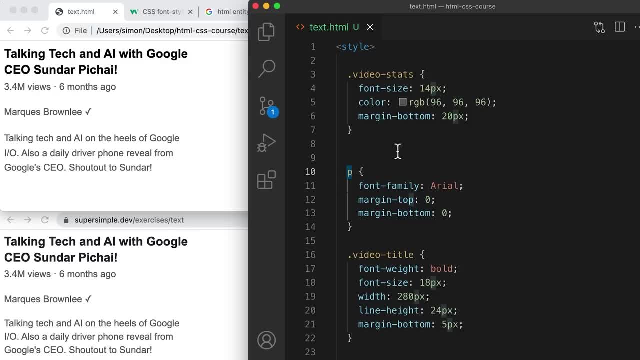 So what I mean by specific is that this targets all paragraphs on the page And this targets a specific class, So not all paragraphs are going to have this class of video-stats, So that's why this is more specific. It targets a smaller group of. 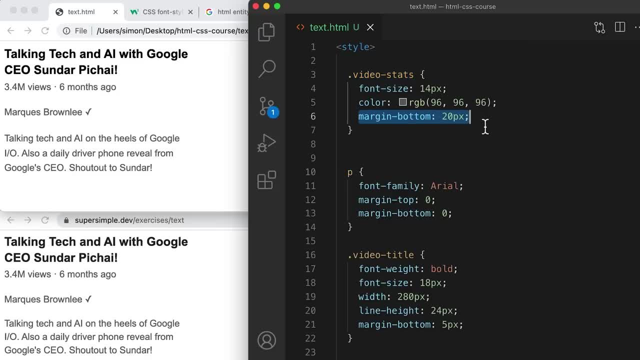 elements than this. That's why this line has priority over this line. So that's just an introduction to CSS specificity For now. just know that a class name like this has more priority than an element name like this, So I'm going to move this code. 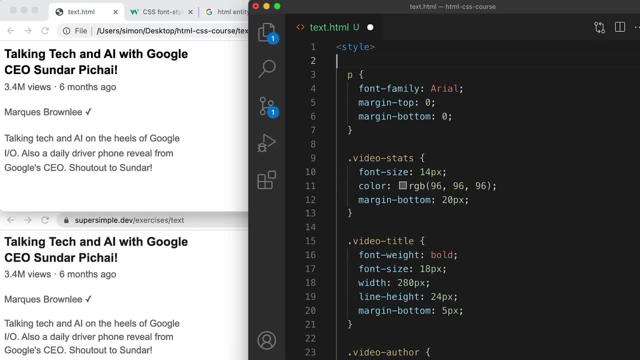 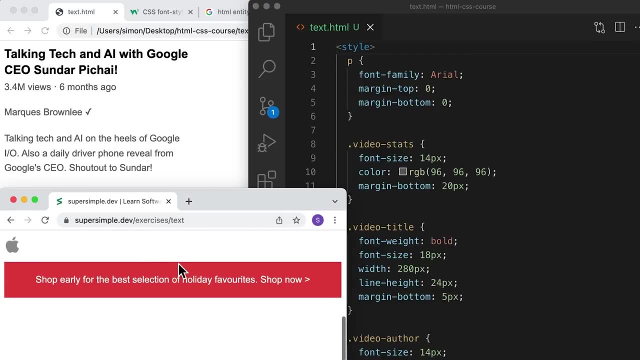 back and we'll continue with the rest of this exercise. Next, we're going to copy this text from Apple So you can see that there is a background color and the text is centered, And also, if I hover over this part of the text, we get a. 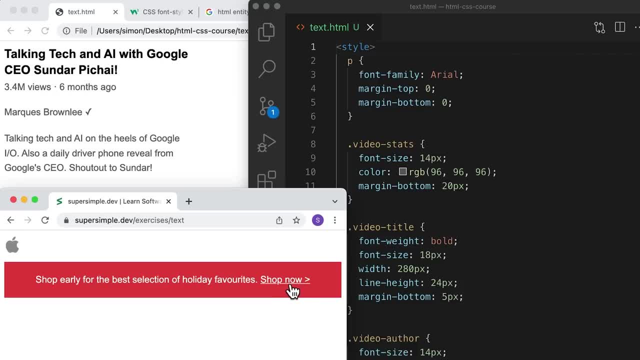 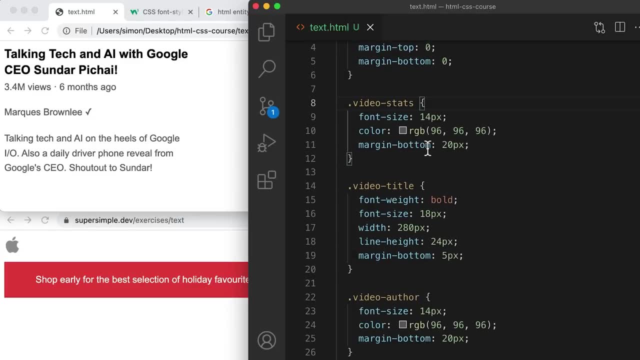 pointer on our mouse and we have an underlined text. So let's see how we can do this. First we'll create the element and then we'll style it one by one. So we'll go down here and we're going to create a new paragraph. 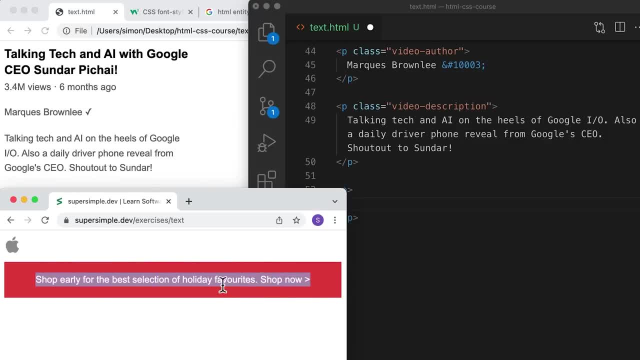 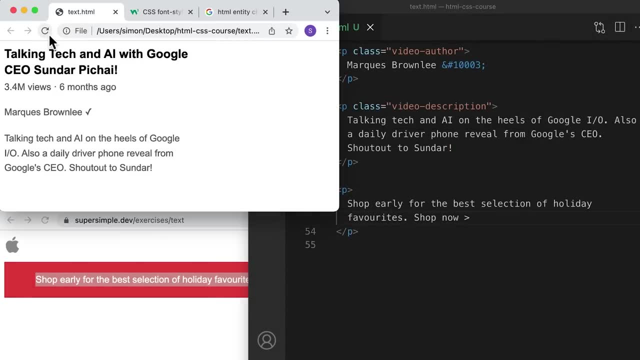 And let's copy this text into that paragraph: Copy and paste, Save it and refresh. Okay, so that looks good. So usually, if you have a greater than or less than symbol, you want to create it with an HTML entity, Because the browser could confuse these symbols. 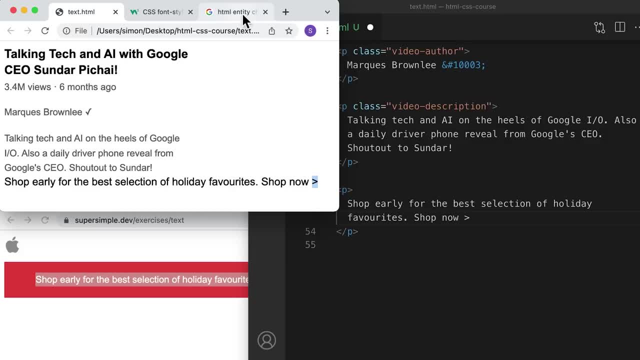 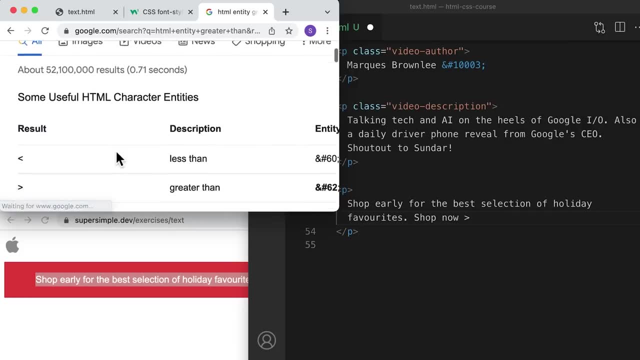 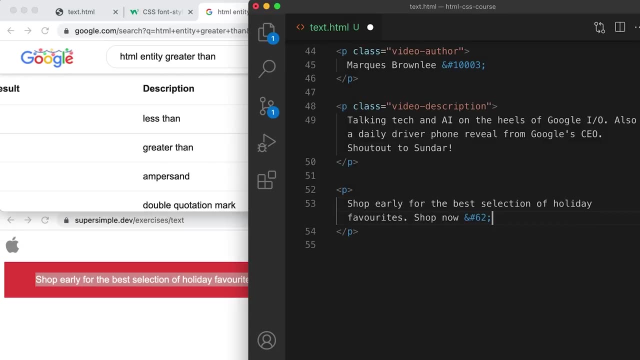 with an HTML tag, So I'm going to search for the HTML entity for greater than So. this is the symbol that we want. I'm just going to copy and paste this into our code, Save it and refresh. Next, let's actually 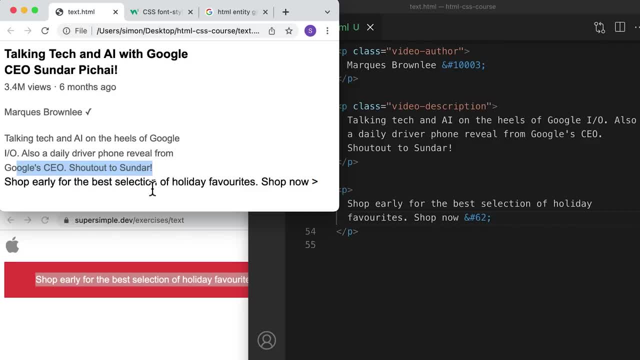 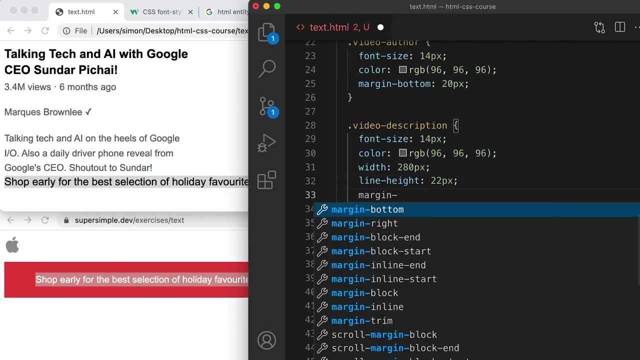 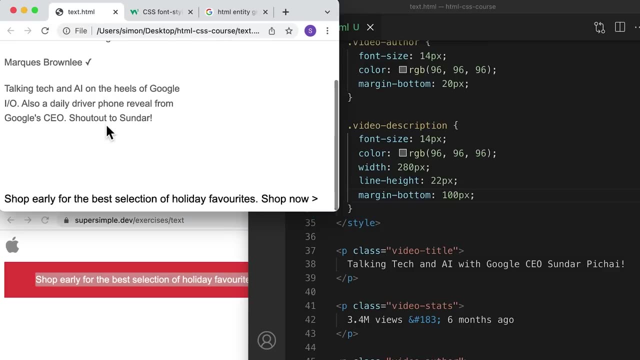 add some space at the bottom of this paragraph so that we can see our new paragraph clearly. So we're going to go here and just add some margin to the bottom, Because it's a little bit too cluttered right now. Alright, so that looks. 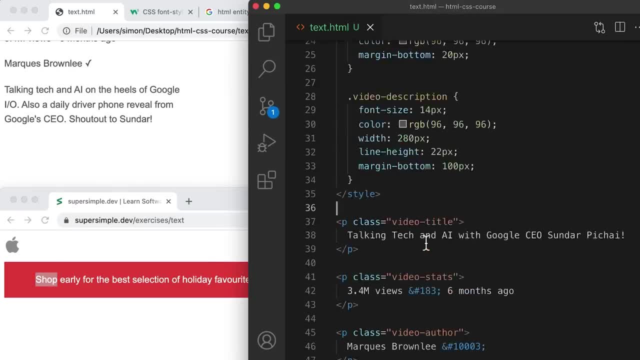 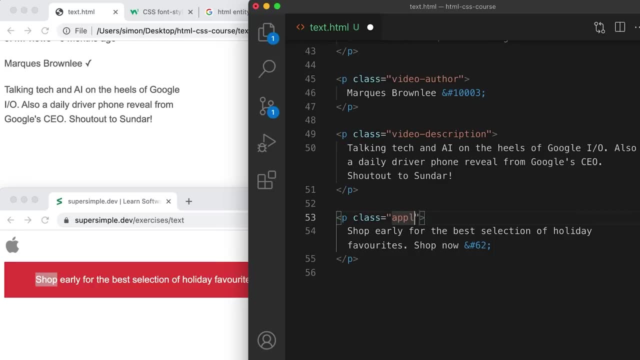 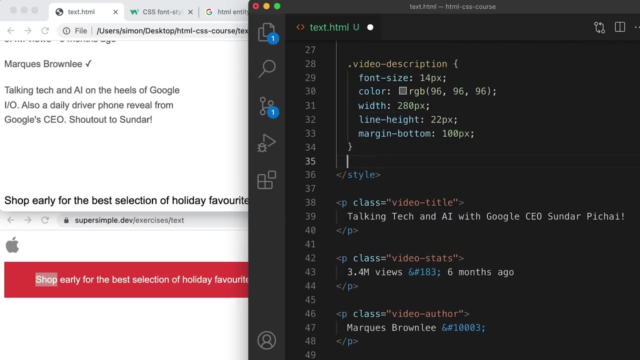 pretty good. We're going to start by adding a class to our paragraph so we can target it in our CSS. Class equals maybe apple dash text, Save it and refresh And apple text. Okay, and first I'm actually also going to give. 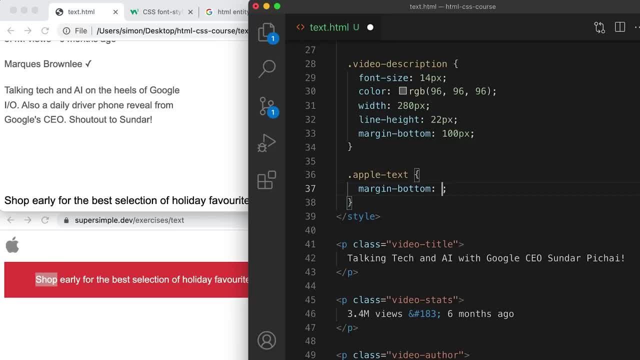 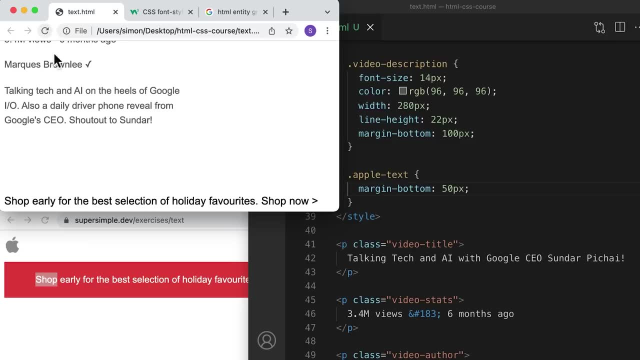 some spacing at the bottom So it's easier for us to see our actual code. So 50 pixels at the bottom: Save and refresh, And now it's a little easier to see what we're working with. So next I'm going to change. 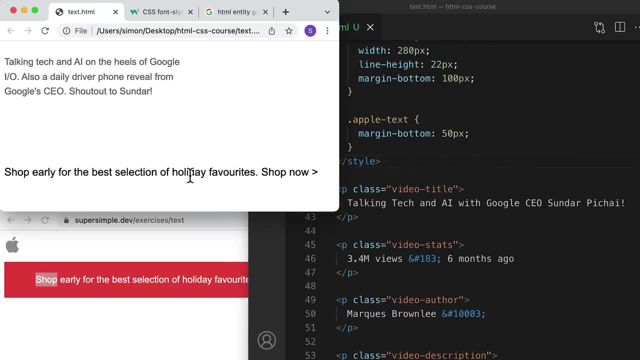 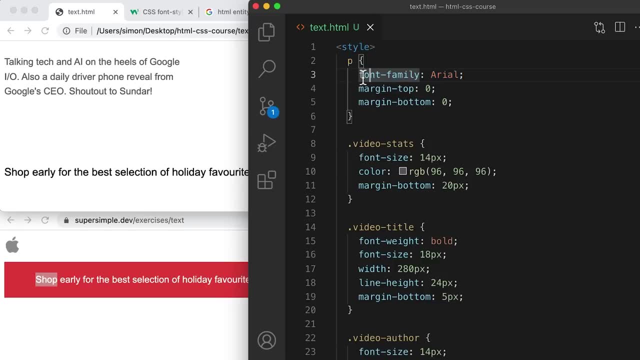 the font size. One thing you'll notice is that the font family is already Arial. If we scroll back up, we have this set of styles that target all paragraph elements, So it's already set our font family to Arial. Let's scroll back down. 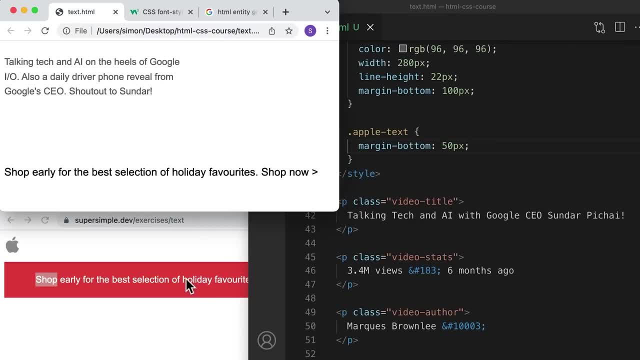 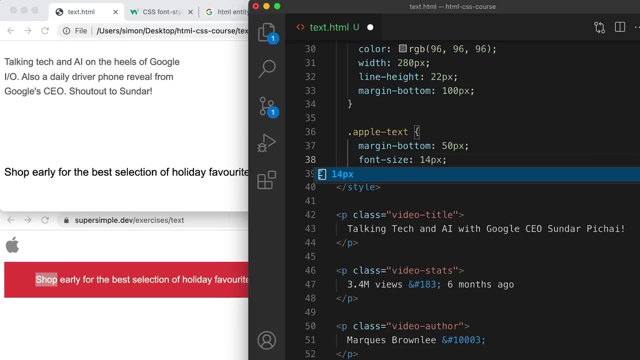 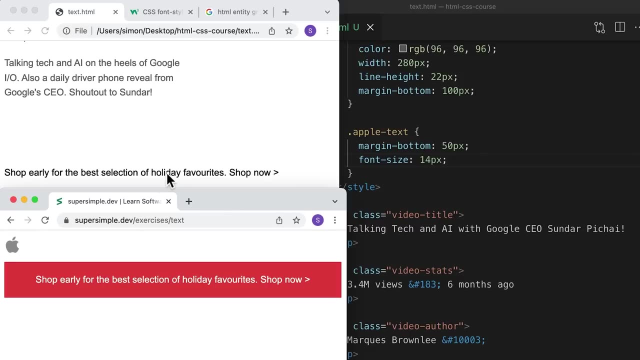 And let's adjust the font size So this one looks a little bit smaller. So let's set it to maybe 15 pixels. Let's see how that looks, Save it and refresh. Okay, so I think that looks pretty similar to the design. 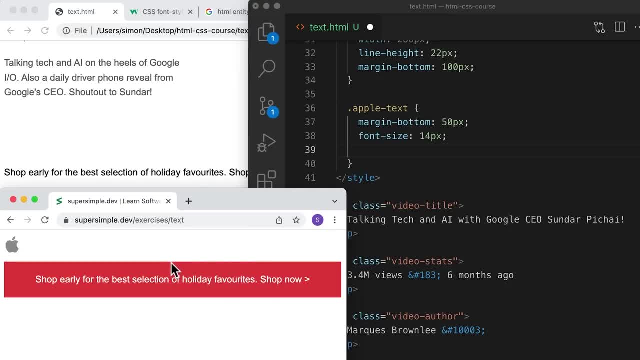 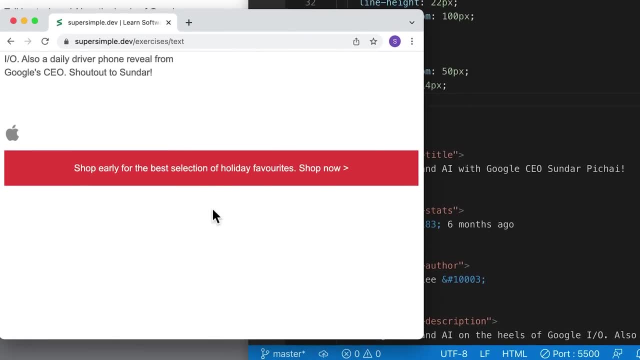 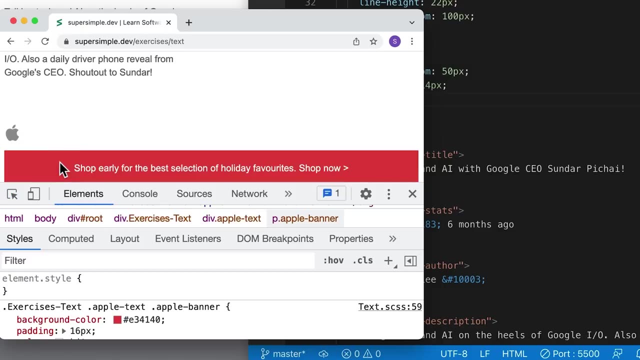 And now the next step is: let's set a background color of red. Now a trick for getting the background color is we're going to right click in an empty area, inspect, click this icon and click the element we want to copy styles for And then go to the computer. 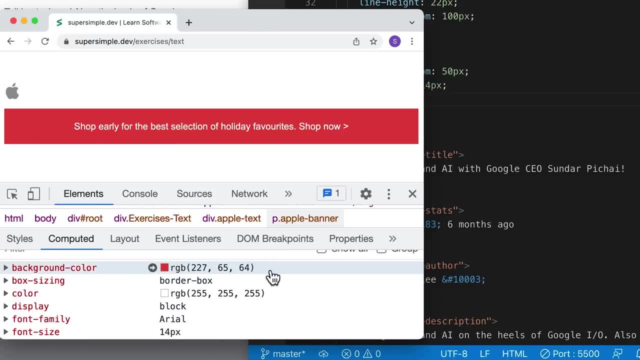 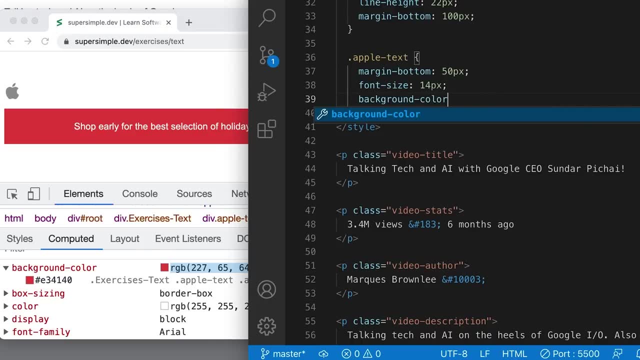 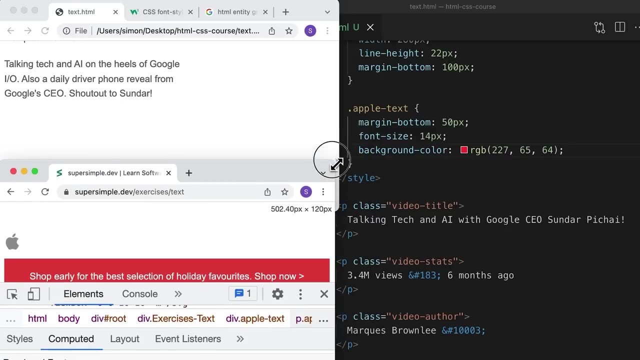 tab and scroll down. Now we have the background color. I'm just going to copy this and paste it in here. So background dash color. I'm going to paste that, Save and refresh. Okay. Next we're going to do the text color. 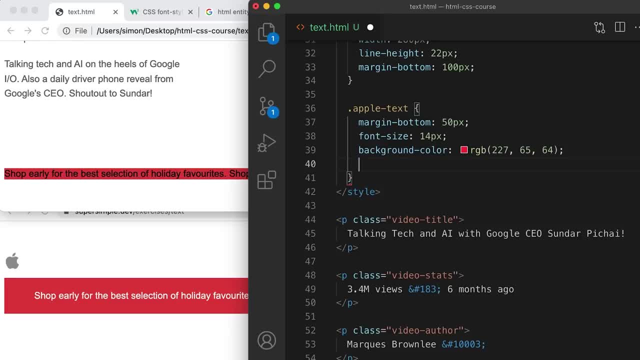 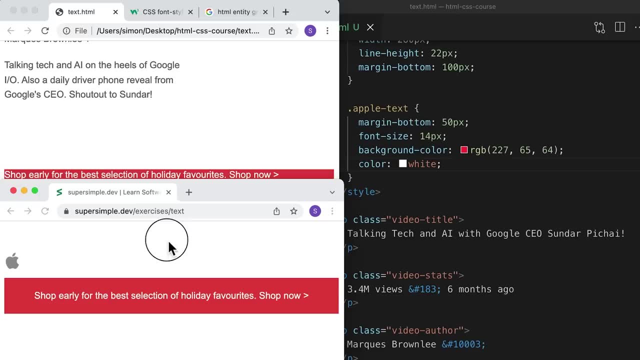 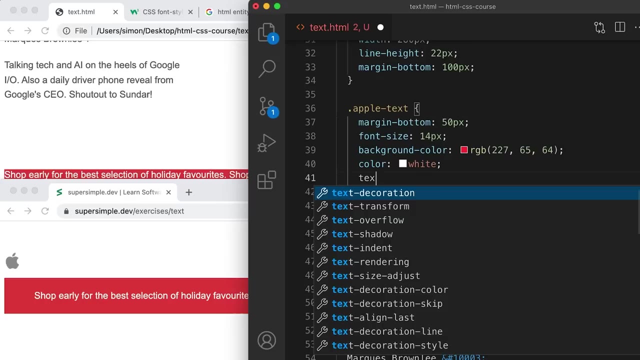 So let's set the text color to white: Color dash white, Save and refresh. And now, if we look at our design, this text is actually centered on the page. So remember, the property for centering text is text dash align center, Save and refresh. 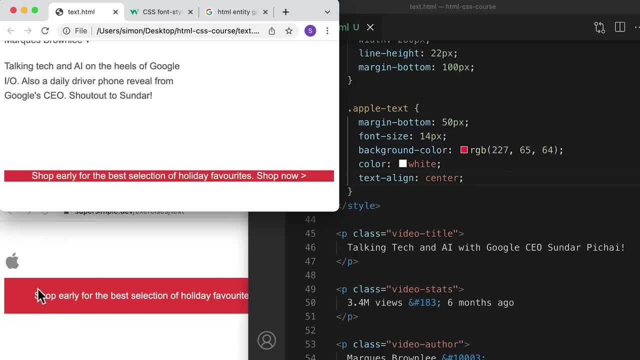 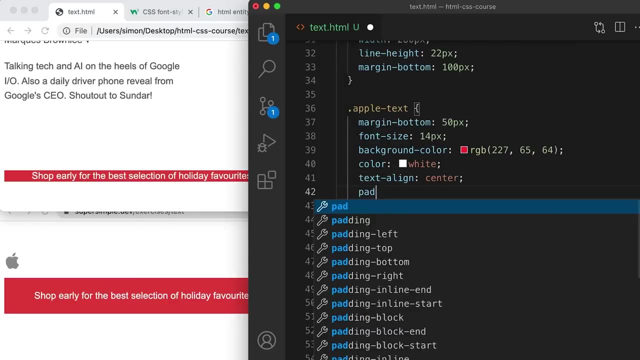 Okay, and the last thing is there's some spacing at the top and the bottom here. So here we actually want to add spacing inside our paragraph And remember from the previous lesson, spacing on the inside of an element is called padding. We're going to add some padding. 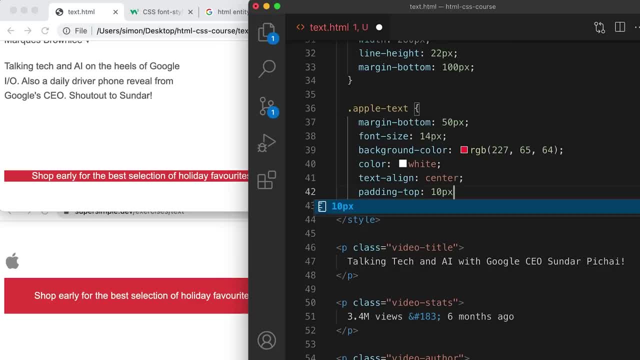 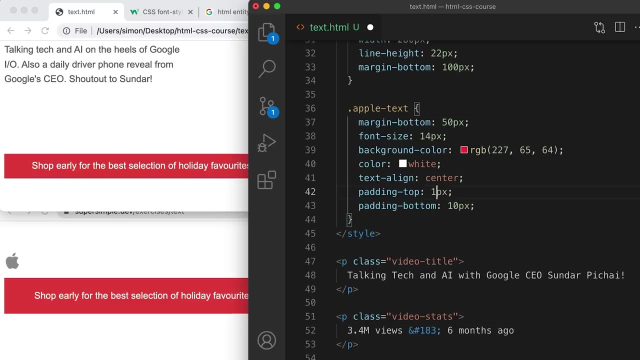 to the top, Maybe 10 pixels, And then padding to the bottom And 10 pixels. Let's see how that looks. Save and refresh. Okay, So I think we could add a little bit more padding, So let's change it to. 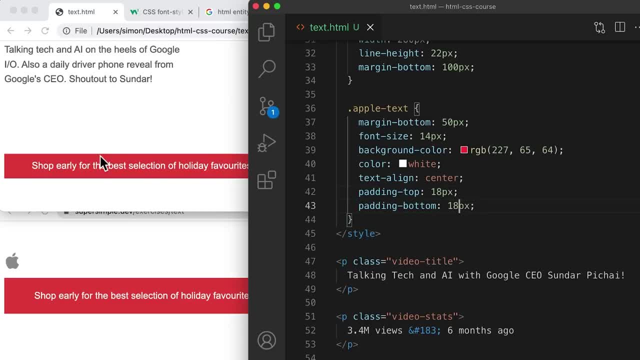 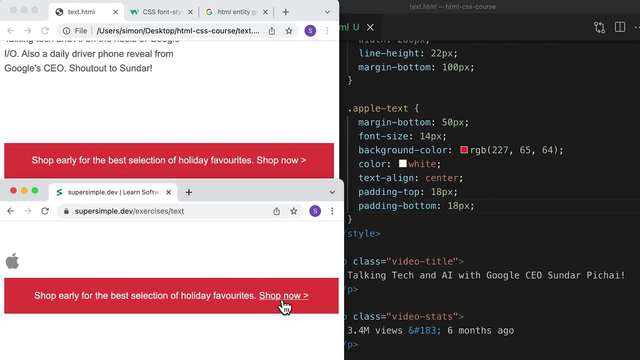 maybe 18 pixels. Save and refresh. Alright, so I think this looks close enough. Now the last thing we're going to work on is this text here that becomes underlined when we hover over it. First, let's learn how to create underlined text. 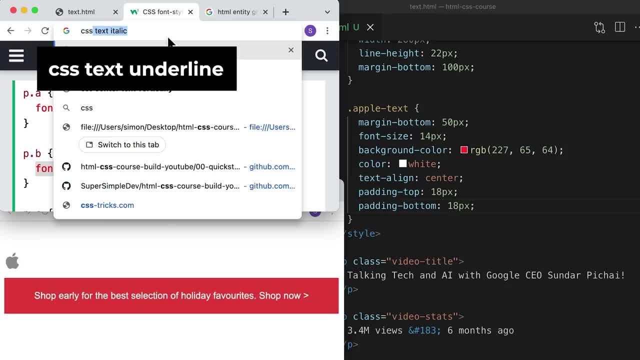 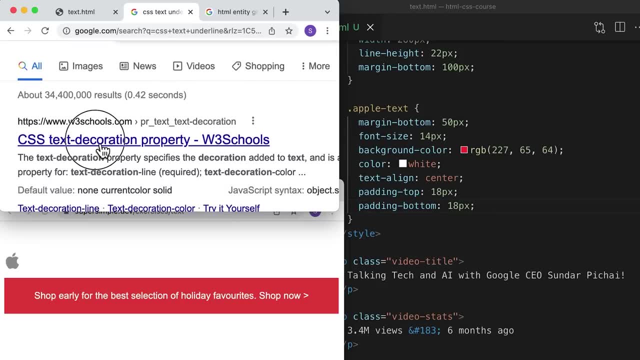 We're going to practice our Googling skills and we're just going to search for CSS text underline. So keep it simple. And then in the first link we have the text decoration property. We scroll down, we have an overline. 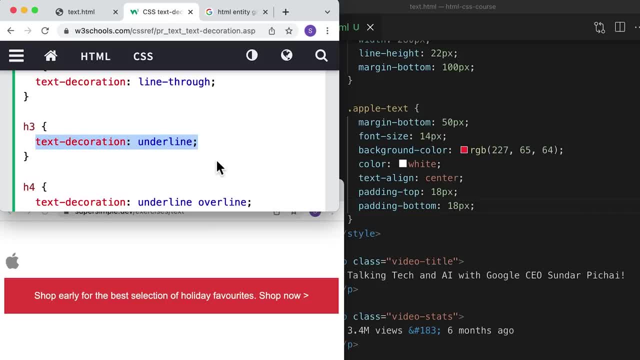 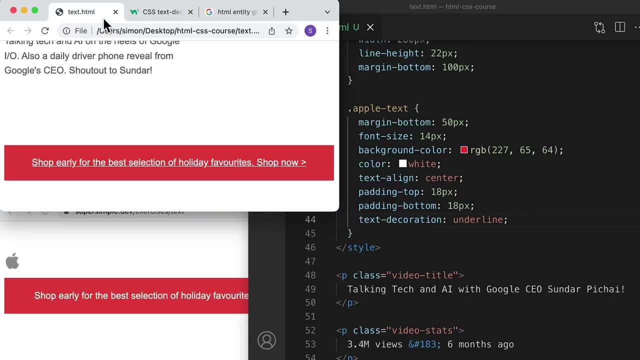 line through and underline. So let's grab this piece of code. I'm going to just copy it in here: Save and refresh. Now, unfortunately, this property actually affects the entire paragraph, But we want it to only affect this part of the text. So how do we? 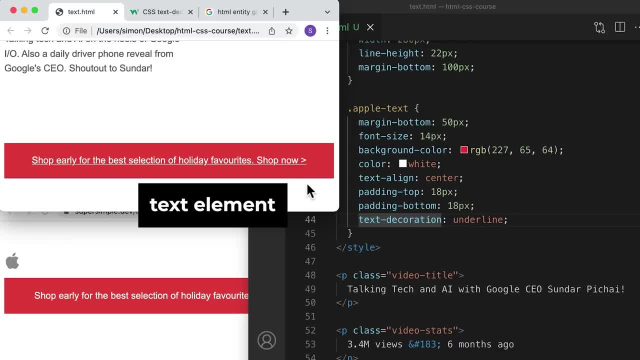 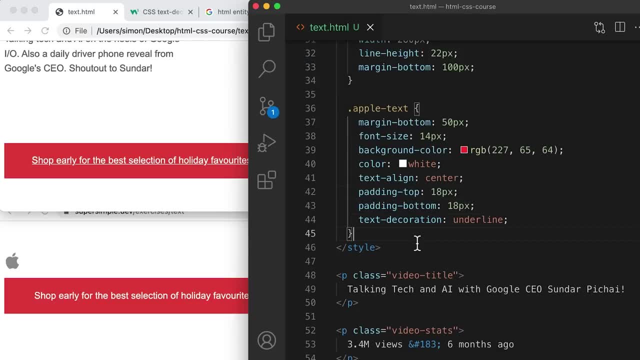 do that, We're going to need to learn something called a text element. So a text element is an element that is inside a line of text. So let's do an example, just to see how it works. We're going to go to the bottom and we're going to create a new. 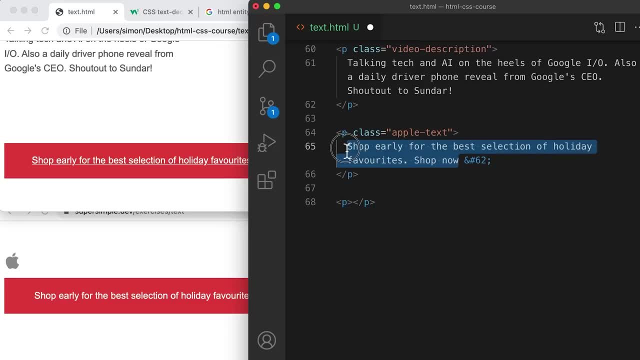 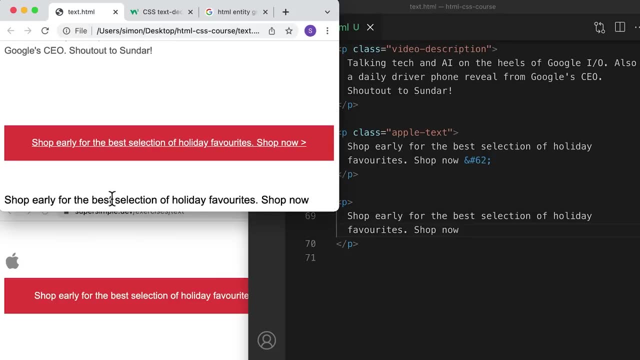 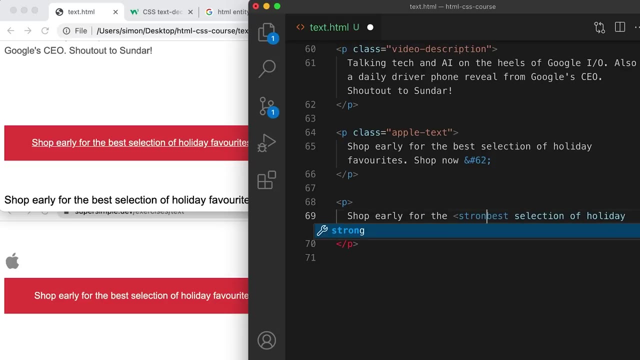 paragraph to practice with, And let's actually just copy this text and put it in there, Save and refresh. And now we're going to create some text elements on this paragraph. So the first text element I'm going to show you is called the strong. 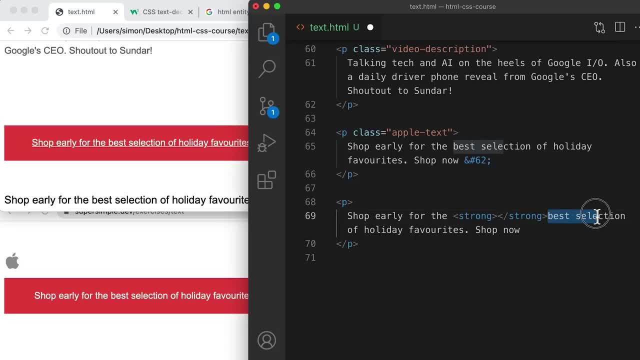 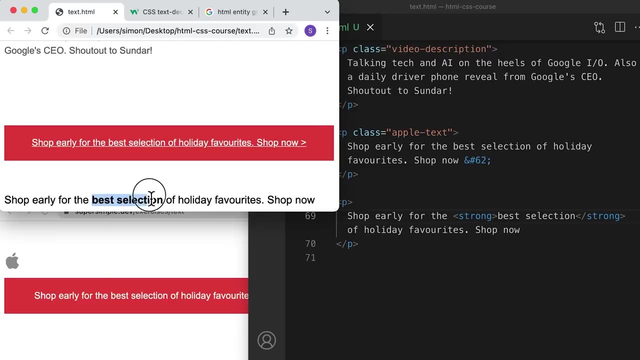 element. So now let's copy, maybe, this text and then put it in there And save And refresh. So the strong element here creates this bolded text that you see on the webpage. So the thing to know about text elements is that they essentially exist inside a line. 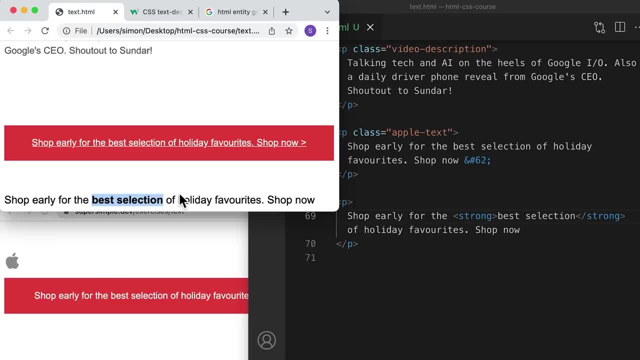 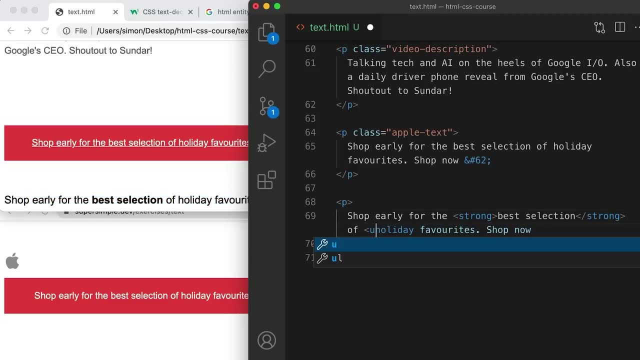 of text, and then they modify that part of the text, So they're not modifying the whole thing. Another text element we can create is the U element. So this one creates some text that is underlined. So if we move this text into here, save it. 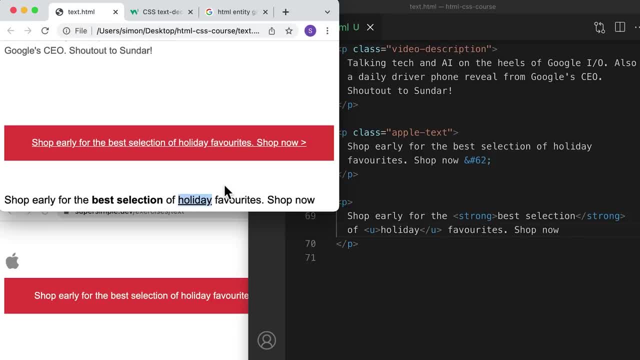 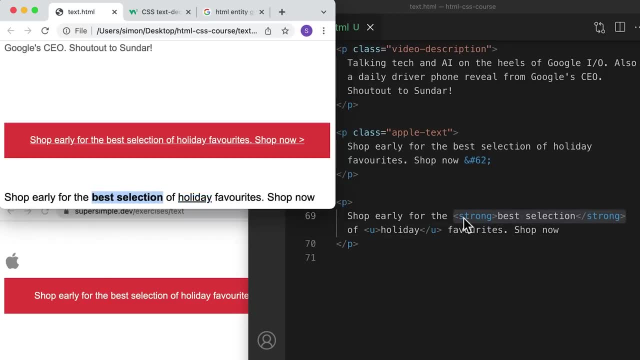 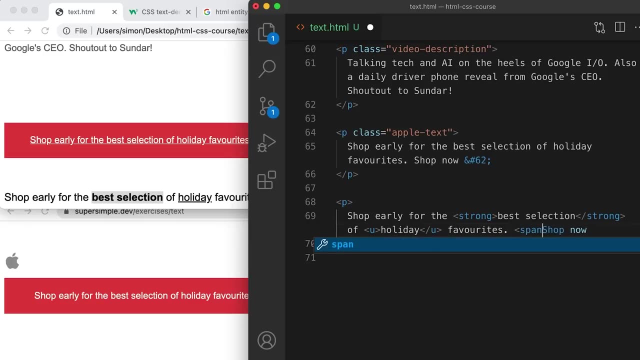 and refresh. we now get an underlined text element. So that is how we style specific parts of a line of text. The final text element I want to show you is called the span. So let's create a span element And we're going to put this text: 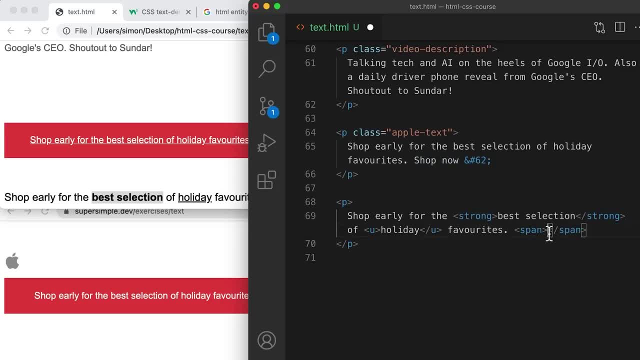 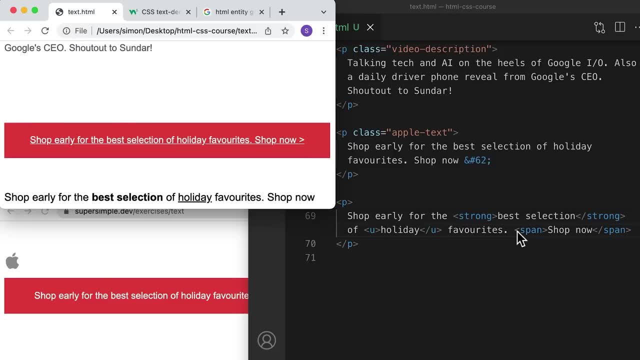 inside, So cut and paste, Save it and refresh. Okay, so the span element is here, but you'll notice that nothing changed, And that's because the span element is the most generic text element. It has no styles, So the span is really. 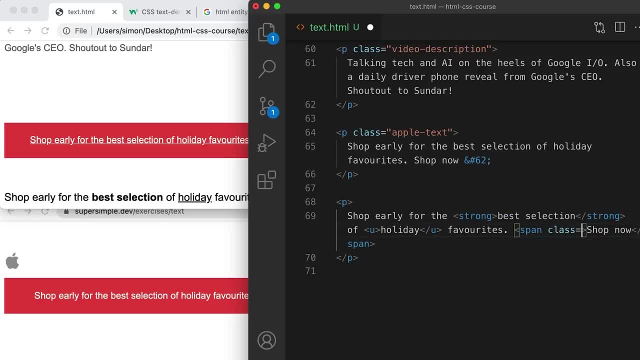 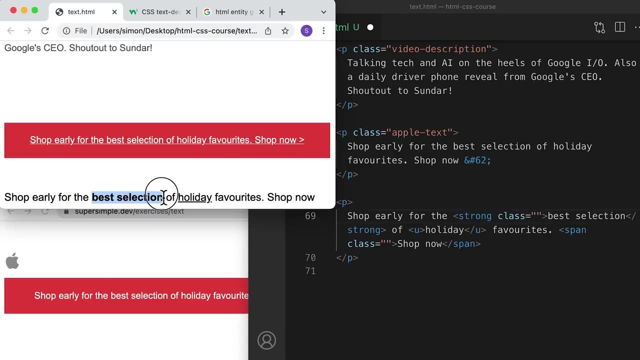 useful because we can actually give it a class and we can style it ourselves and give it any style we want. Now we could add the class attribute to these other text elements, like the strong and the U element, but notice that these text elements come with a default style. 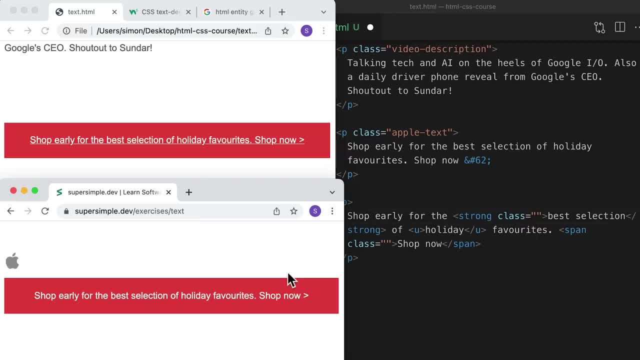 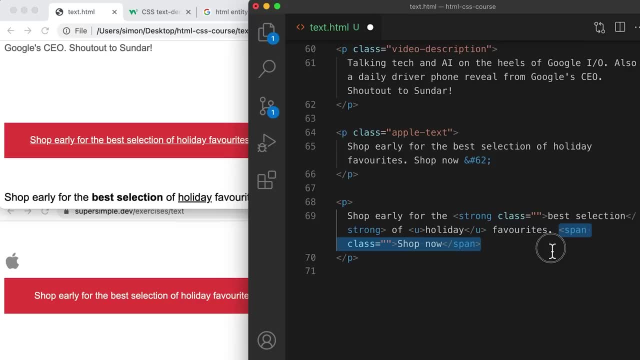 And that may not be what we want, especially in this situation where we don't actually want a style until we hover over it. So that's why we use the span text element. It lets us modify a specific part of the text without affecting the whole thing. 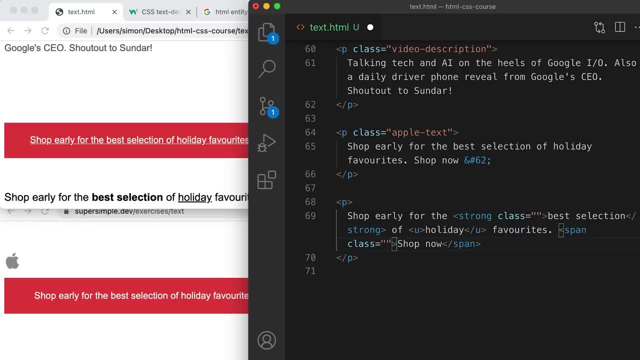 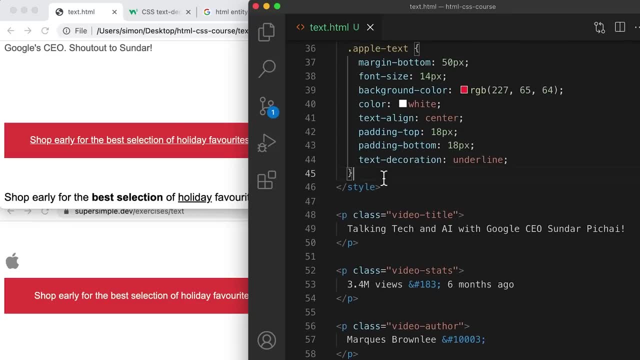 And it's the most flexible and we can style it however we want. So if we give it a class of span example, and then go to our CSS and then we target span example, we can give it any styles that we want. For example, we can set a color of. 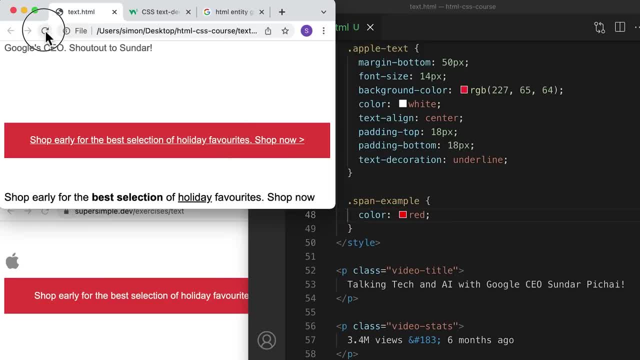 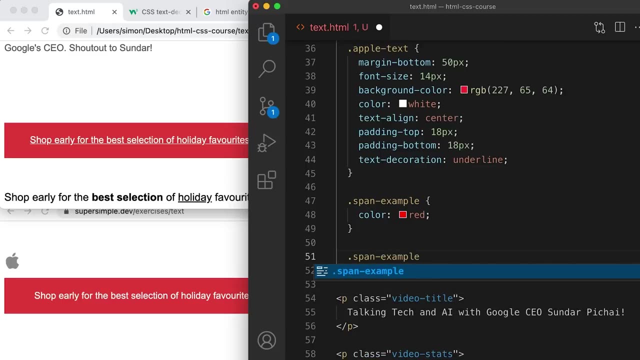 red. Now, if we save this and refresh, the span now turns this part of the text red. The other cool thing is that everything we know about CSS still applies, So we can target span, example colon hover, And these styles will only apply when we hover. 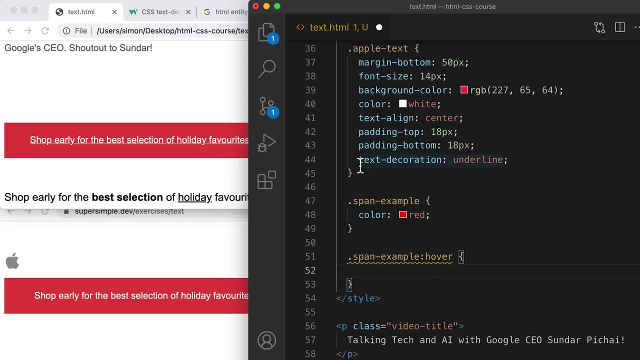 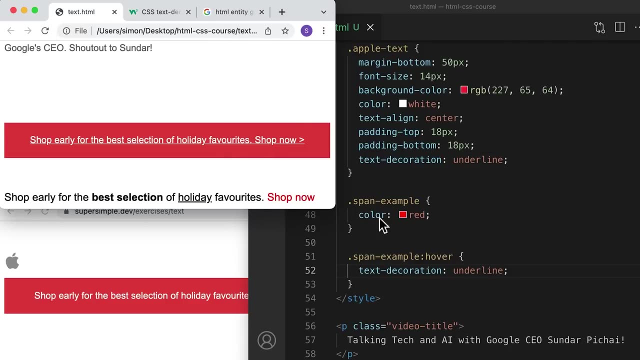 over the span. So in this case let's underline it because that's what we want. So if we do text dash decoration and underline, just like up here, Save it and refresh. Now this span has a color of red here and when we hover over it. 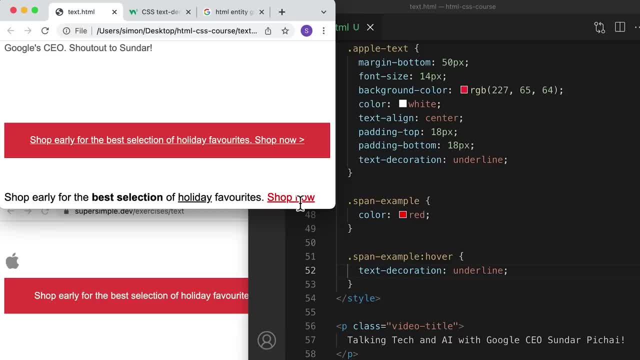 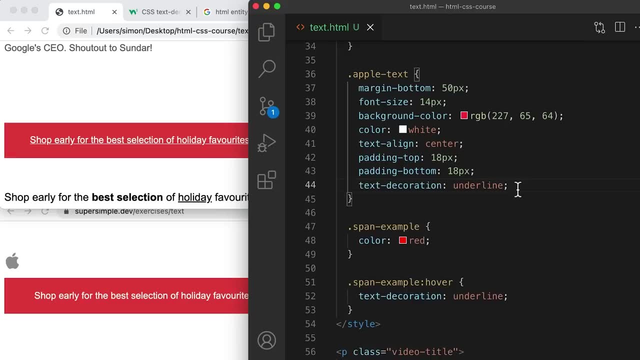 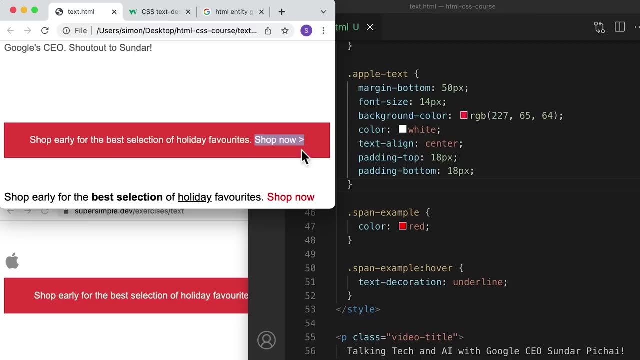 this style apply and it's gonna get underlined. Let's use what we learned here to finish up our example. We're gonna first remove this line because we don't want to underline the whole thing. Let's refresh and we want to create a span so that we only 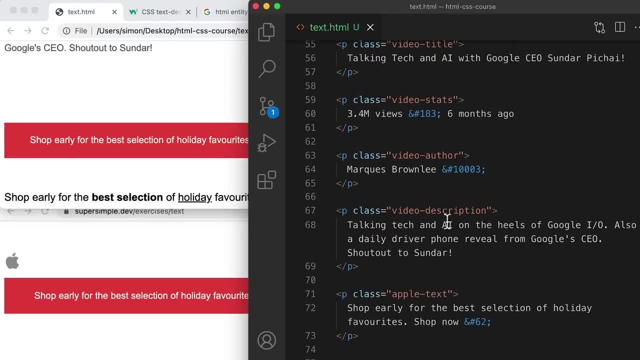 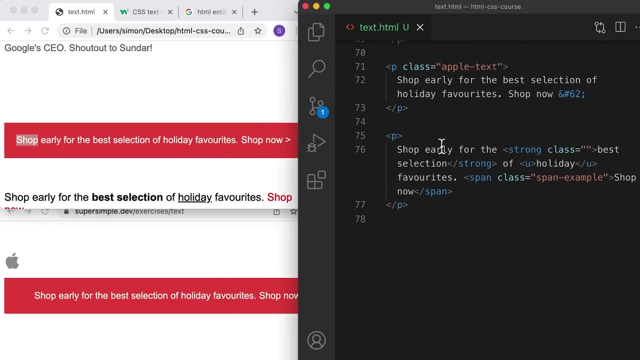 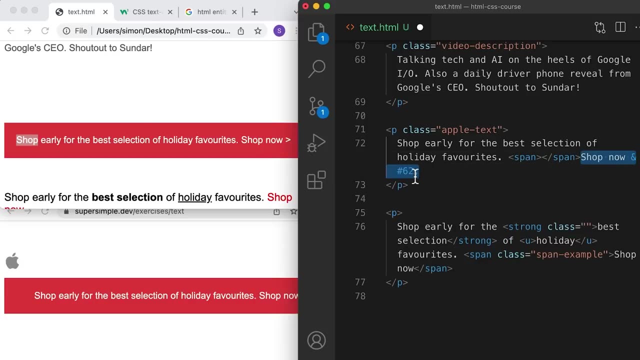 target this part of the text. Let's go back down. gonna resize it a little bit just so that we can see. Okay, so we're gonna scroll down to here. we're gonna wrap this in a span, Just gonna move this into here: Save. 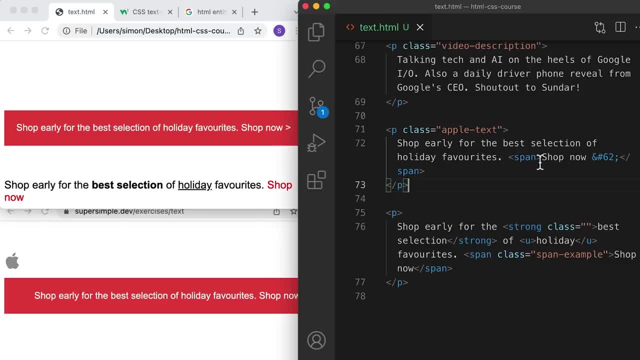 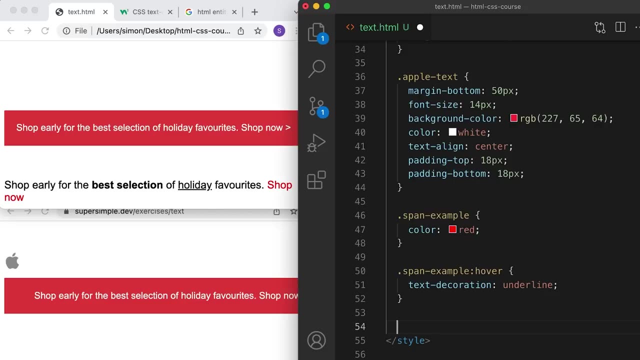 Refresh And now we're going to style this span. So remember, we're gonna give it a class so that we can target it in our CSS. Let's call this the shop link, Save it and let's go here and we're gonna style it now. 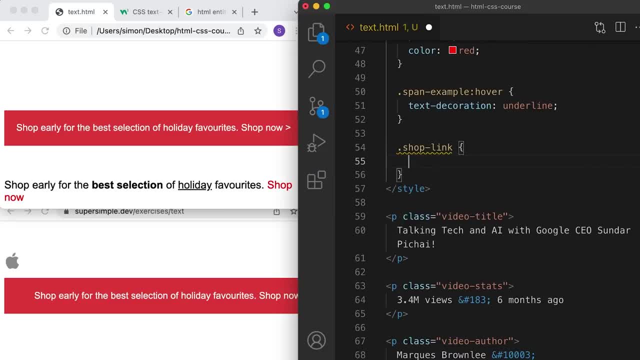 So shop dash link. So remember, the style for this is that the mouse turns into this pointer. So to do that we're gonna use the property cursor dash pointer, Save and refresh. So now, when we hover over it, our mouse is a pointer. 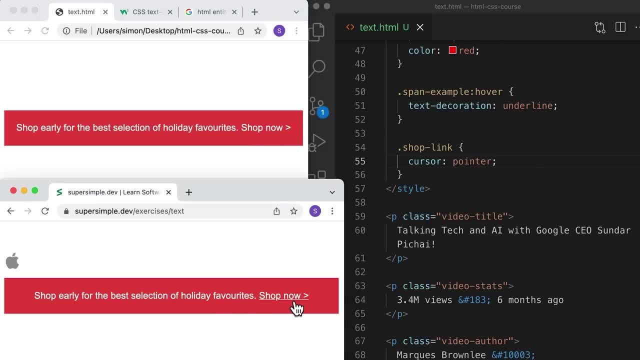 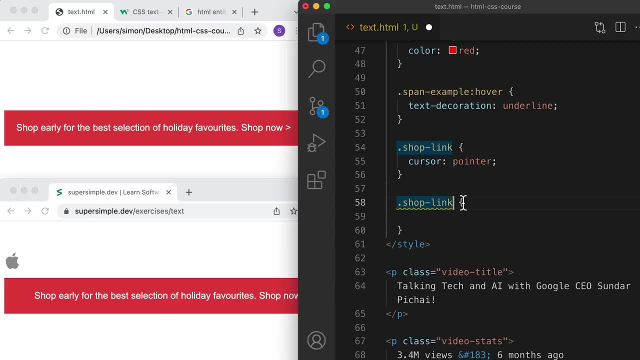 And the last thing is that we want it to be underlined when we hover over it. So let's create a hover style Shop dash link And we're gonna give this pseudo class colon hover And we're going to underline it with text decoration. 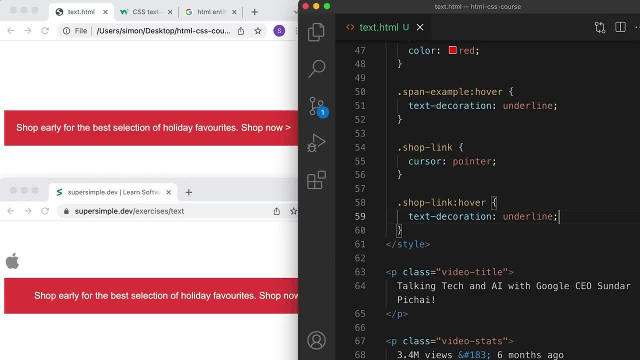 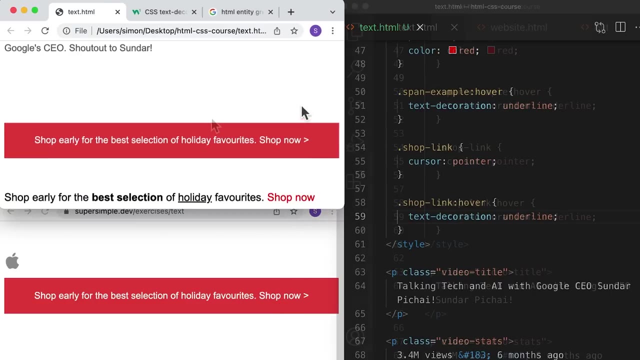 underline, Save it and refresh. And now, when we hover over this, it's going to turn our mouse into a pointer and it's going to underline it. So we've achieved the exact same styles as our design. So there's one last thing I'm gonna show you in this. 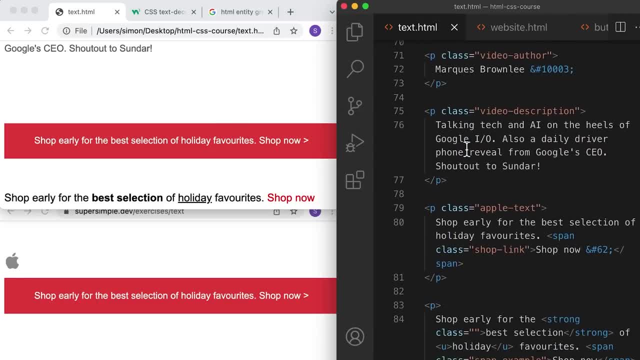 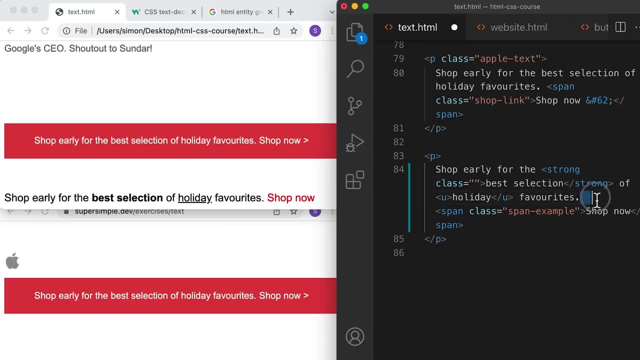 lesson. Let's go back into our code. we're gonna scroll all the way to the bottom And recall that in HTML, if we have multiple spaces like this, it will combine them all into one space. So if I save this and refresh, you'll see that only one space shows. 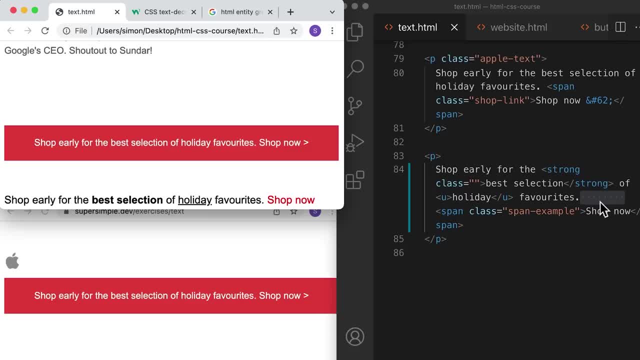 up here. So I'm gonna show you how to get over this problem. Basically, instead of typing out multiple spaces in our HTML, all we have to do is set a margin left on this text element. So we're gonna set a margin left on this element and it's gonna. 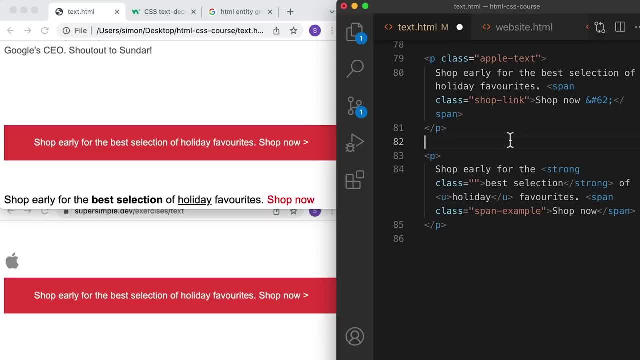 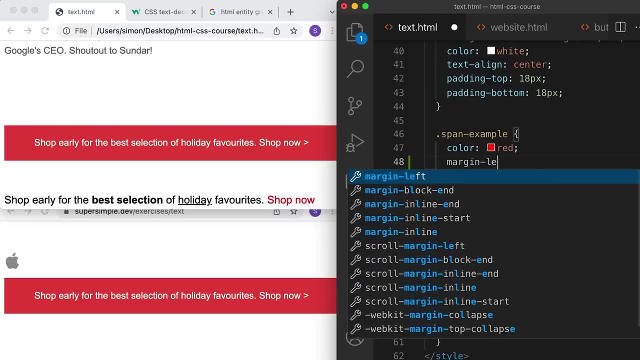 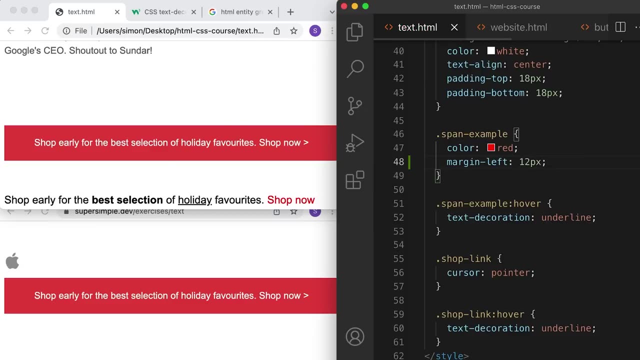 add spaces on the left. So, as an example, let's scroll up and we're gonna add margin dash left to our span element here and let's do something like 12 pixels, Save it and refresh, And now we have spacing between our words. 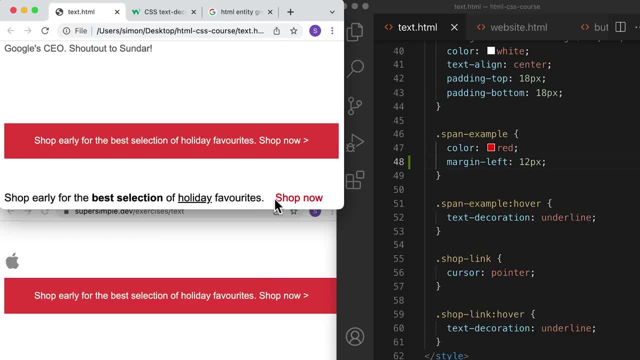 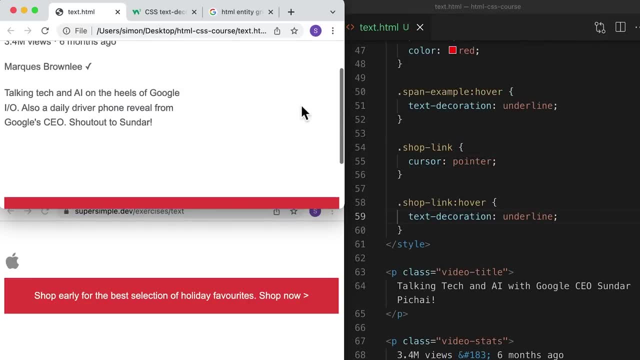 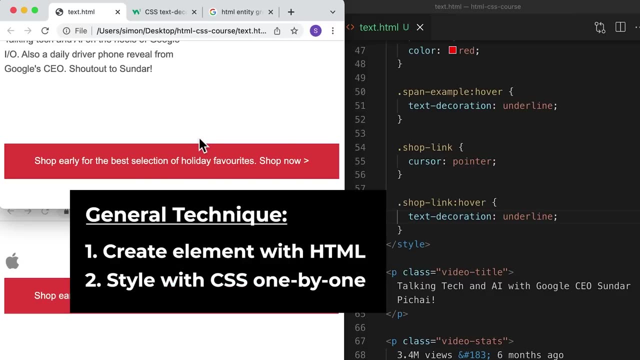 So this is how we achieve multiple spaces between our words, even though HTML combines them. So that is how we create really professional looking text like this and like this: We first create the element with HTML, and then we style it one by one with CSS. 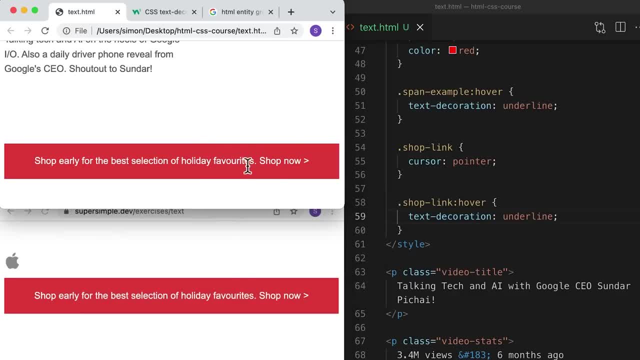 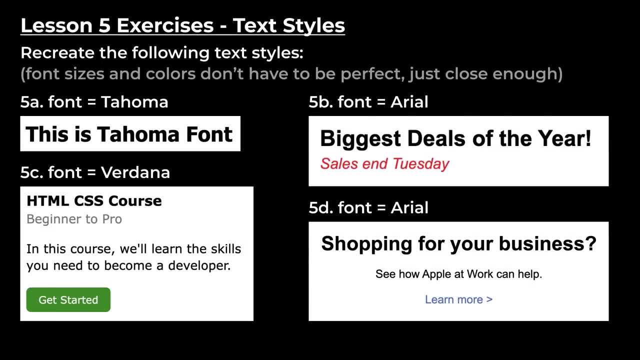 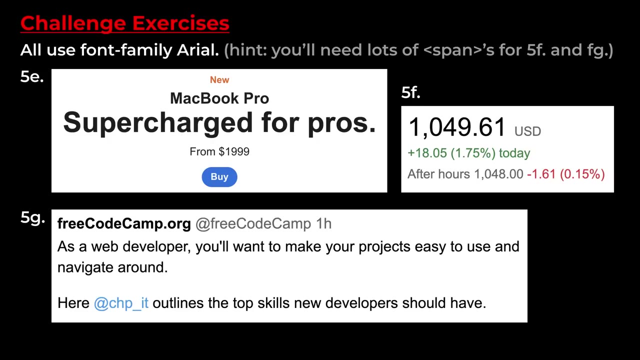 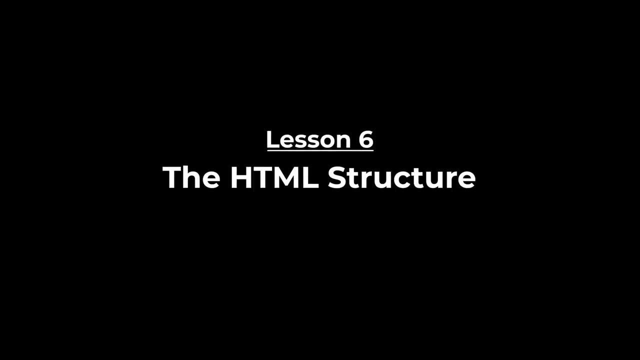 And if we wanna style only just a part of the text, we have to use a text element like a span. In this lesson we're gonna learn the proper structure of HTML and that's gonna give us access to all the features of HTML. So up until this point we've 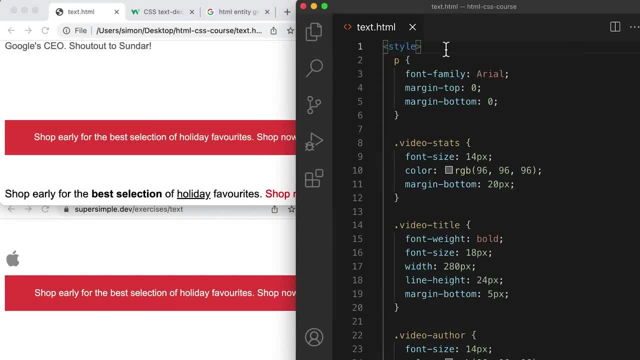 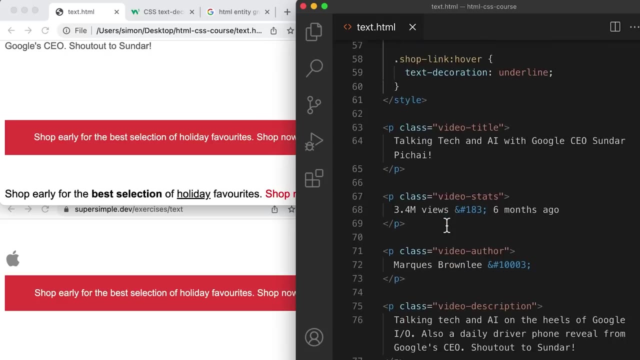 actually haven't been following that structure. For example, if we look at our code, we scroll down, we can see that we're creating elements that we're not following. For example, if we look at our code, we scroll down, we can see that we're creating elements. 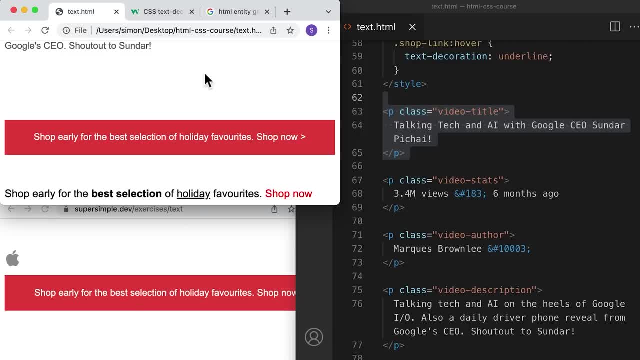 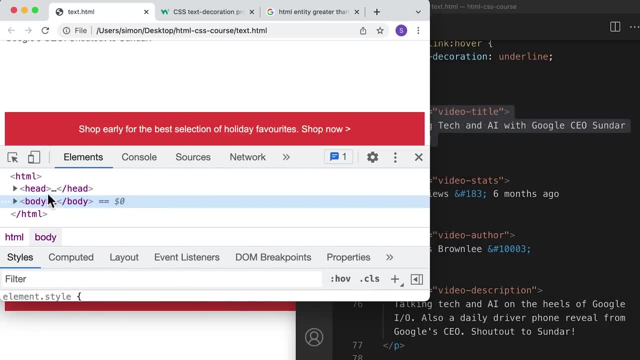 directly like this. If we go to our website, however, and we right click and inspect and we look at our HTML, we can see that we have some elements here called the HTML element, the head element and the body element. So this: 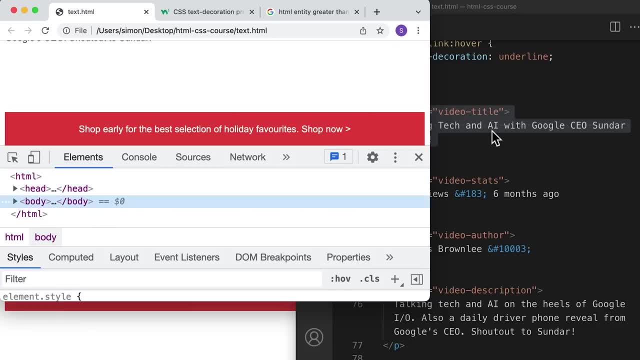 is the structure that we're actually supposed to have in our HTML file, And because we don't have it, the browser is automatically creating this for us. So this was fine in the previous lessons because we're just learning, but it's actually best to. 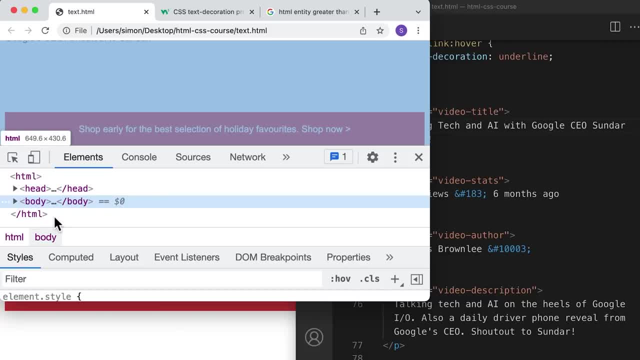 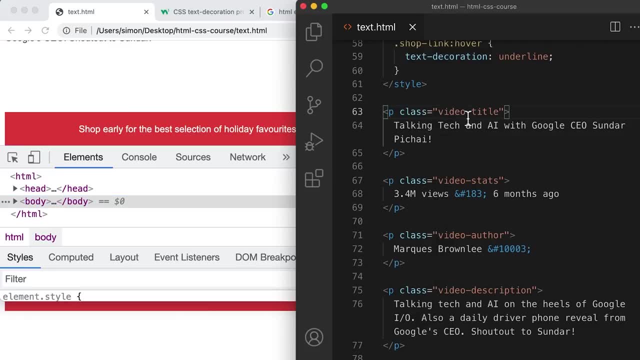 have this structure in our code because we're actually missing some useful features. So let's go ahead and learn what this structure is and add it to our code. So we're going to go back to all of our code and add in this structure. 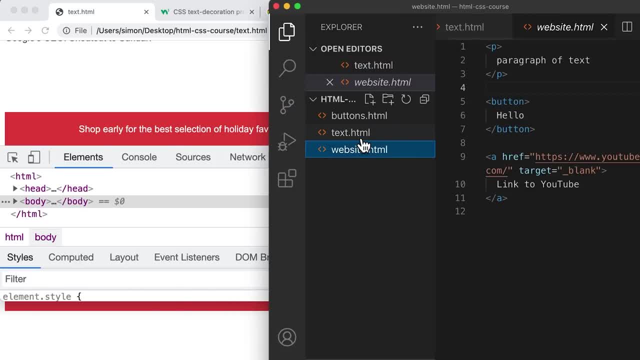 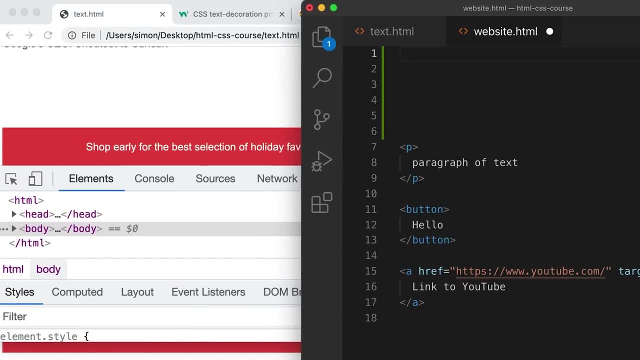 Let's go back to our very first HTML file and at the top I'm going to add some spaces and we're going to learn what the proper structure is. Every HTML file is going to start with less than exclamation: doc. type space: HTML greater than. 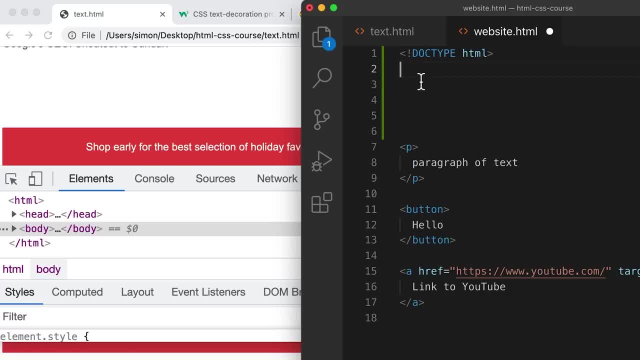 So you just have to type this line out exactly as I have it here. This is not really an element, it's just a special line that has a meaning to the browser. This tells the browser to use a modern version of HTML. If we don't have. 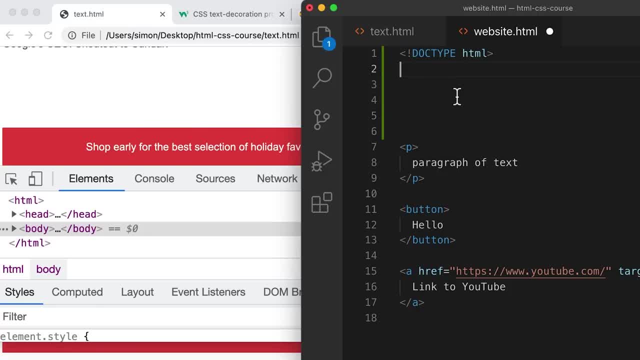 this. it sort of falls back to an older version that has less features. The next part of the structure is to create an HTML element. So this says there's a web page inside this element. There's not much meaning to it, we just have to have. 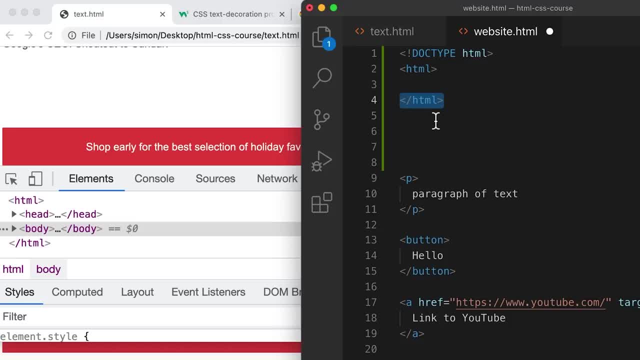 this at the top and the closing tag at the bottom of every HTML file. Next, we're going to create this head element, So head and closing tag. and we're going to create the body element, So body and closing tag. So this is the proper structure of all. 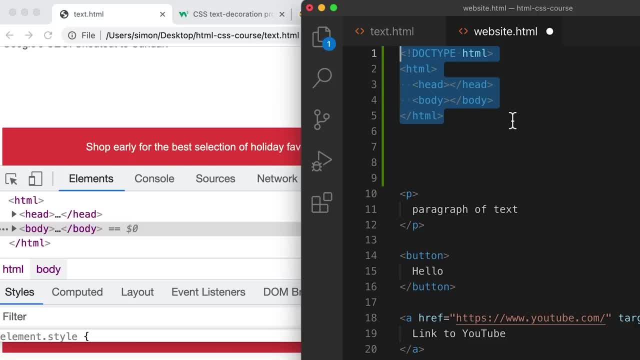 of our HTML files, and this is how we're supposed to start and end our files. So here you can see that we have an element inside another element. This is called nesting. So not only can we have text inside an element, we can have other elements inside elements. 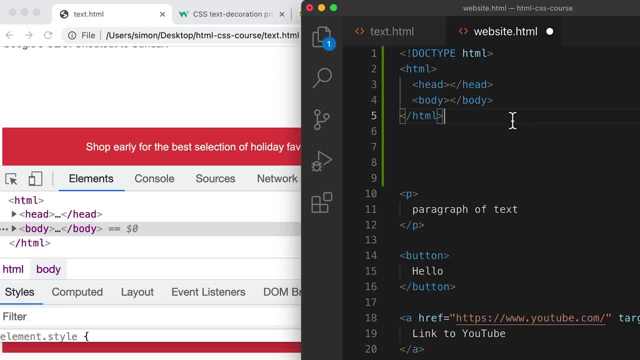 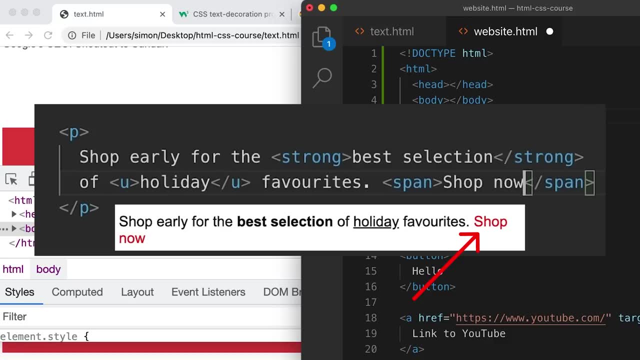 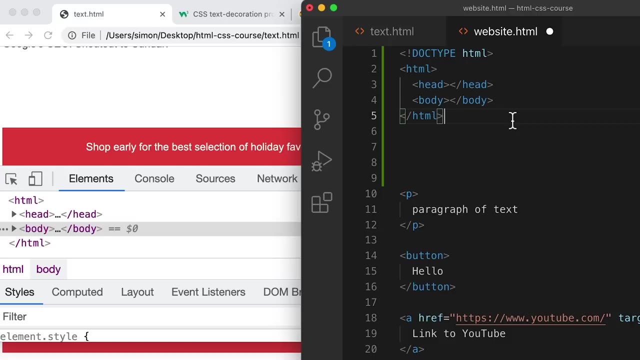 We've actually already seen an example of this in the previous lesson. We put a text element like a span inside a paragraph and that allows us to have some text in the paragraph that was styled differently. Here we have our second example of nesting. We have a head and a body. 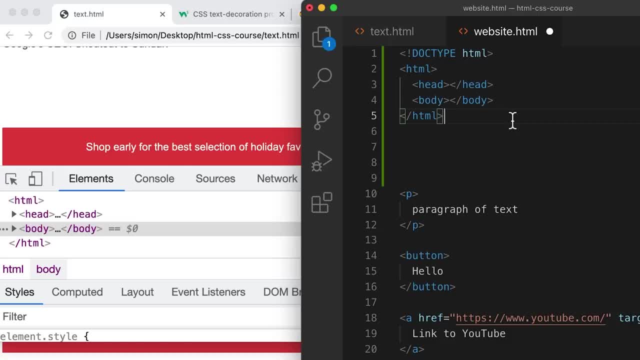 element inside an HTML element, So this doesn't actually do anything visually, unlike our previous example, but it's part of the HTML syntax rules that we have to follow. Every file has one and only one HTML element, and this element represents the entire webpage. 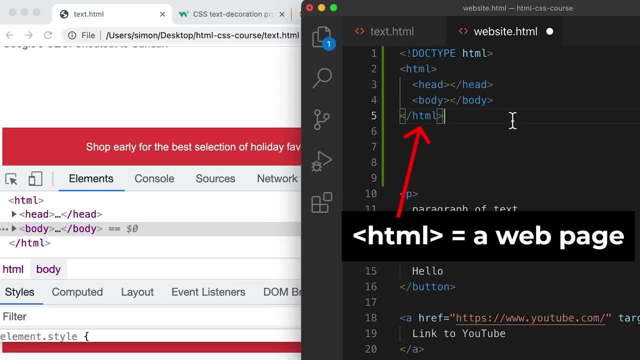 And the HTML element is designed for nesting. It's designed to contain one head element and one body element, And then everything on our webpage is supposed to go either inside the head or inside the body, So both of these elements are also designed for nesting or to have elements. 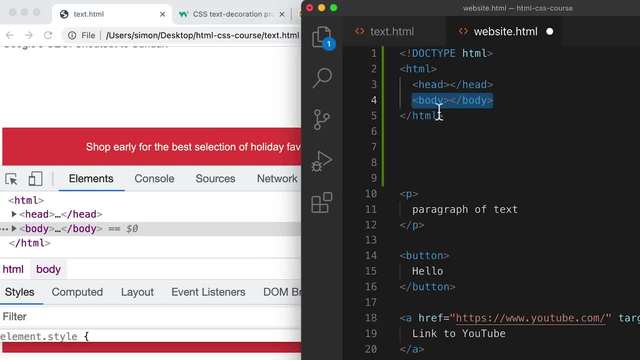 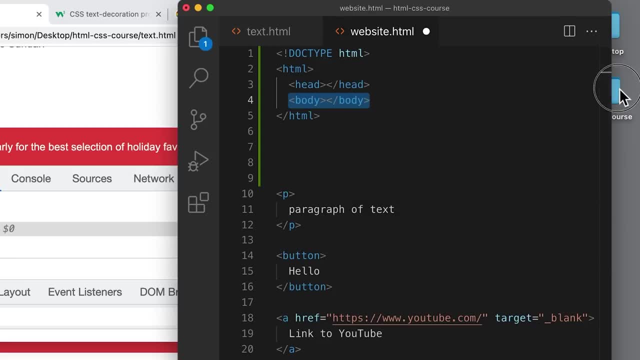 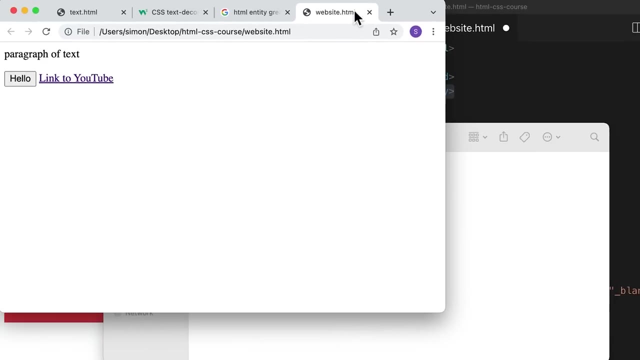 inside The body element here is supposed to contain all the elements that are visible on the page. So let's actually open this website. I'm going to go into our folder that contains our code. I'm going to right click open with Chrome, So on. 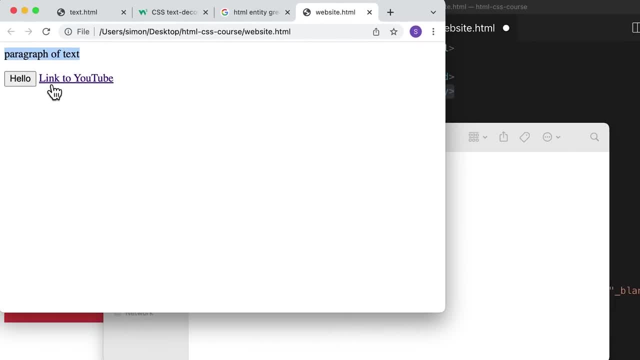 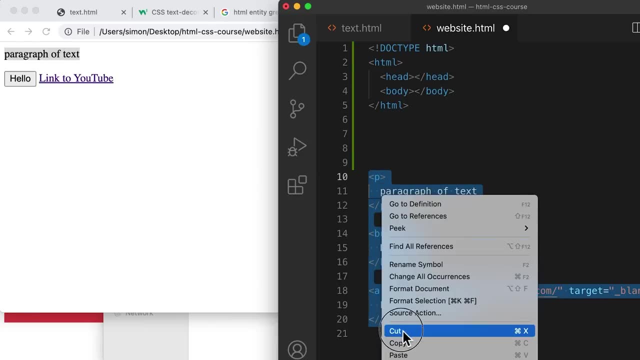 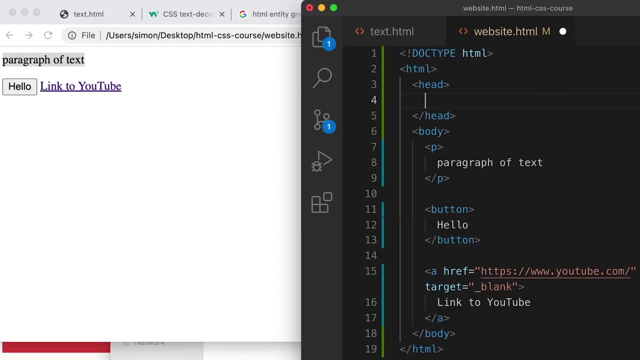 this website, you can see that the paragraph is visible, the button and the link is visible, So all of this is visible on the website. So it should go into this body section. Inside the head element are all the elements that are not visible on the. 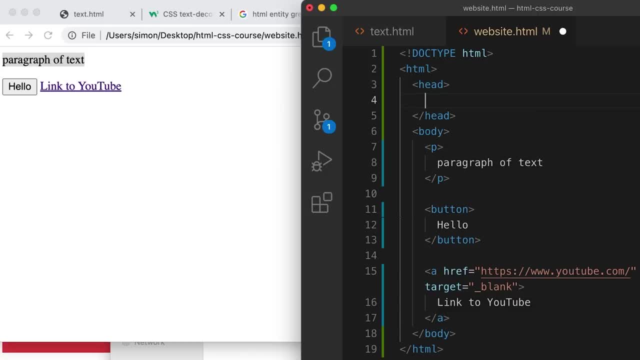 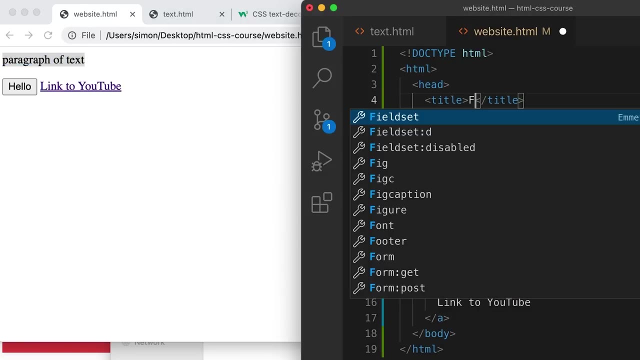 page. So here's an example of such an element. We're going to create an element called title, So the text inside the title here is going to change the text in the tab here. So, for example, if I use the text first: website. 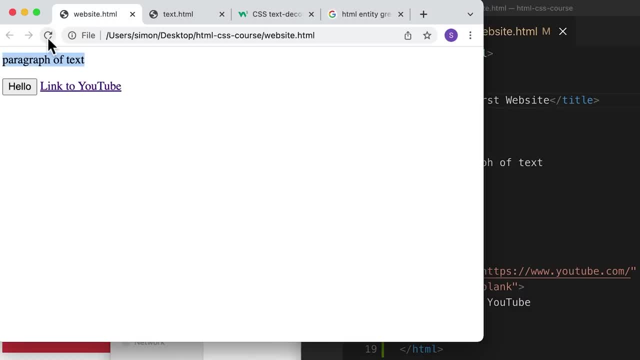 that's going to show up in the tab. So if I save and refresh, that's where the title element shows up. But notice that this title element doesn't actually show up on the page And that's why it belongs in the head section. 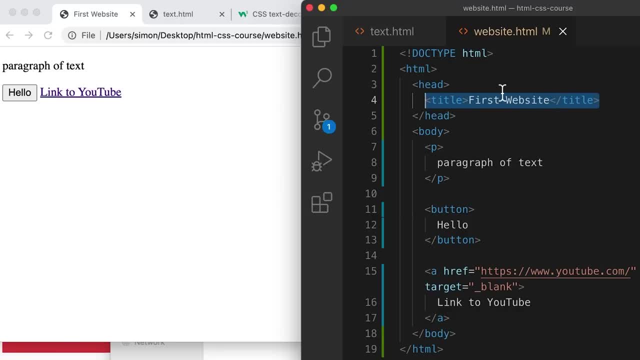 So the title is the first feature that we get from following this structure. The second feature that we get- that's really useful- is the ability to automatically reload our webpage whenever we change our code. So you may have noticed that every time we change our code, we 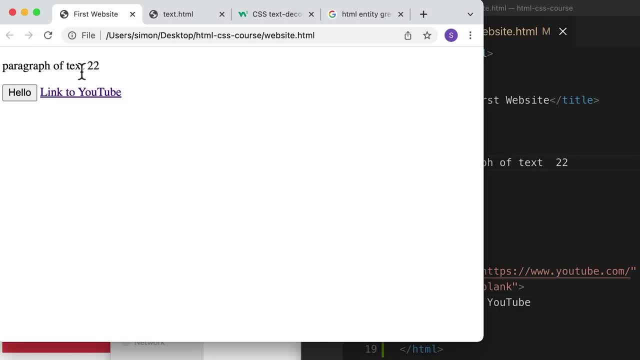 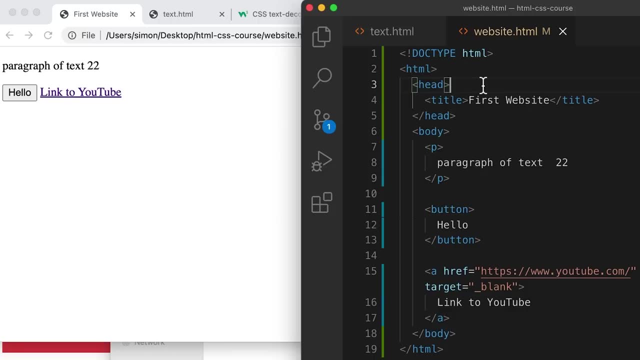 have to go to our website and then refresh the page to see our new code. Now we can actually avoid this by following this structure and then installing a VS Code extension. So let's go to this extension area here And we're going to install the extension. 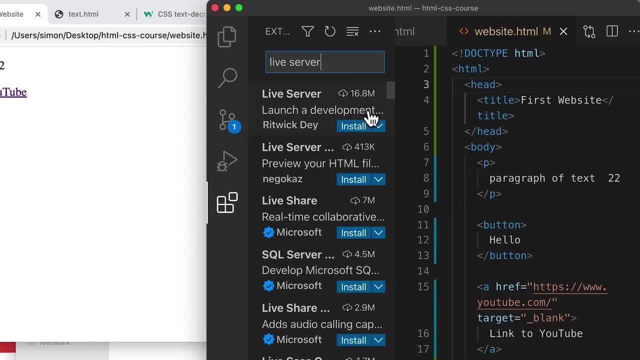 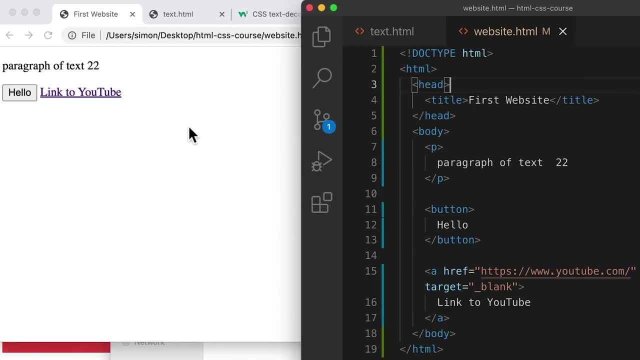 live server. I'm going to install this And now we can use the live server to reload our page automatically whenever our code changes. To open this website in a live server, we're going to right click and we're going to click: open with live server. 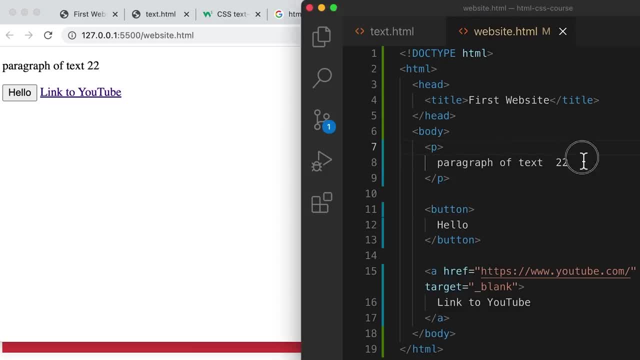 And now we've opened this website and it will automatically refresh whenever we change our code. So if I change the code like this and I save now, it automatically refreshes without having us to go back and forth. So that's a really useful feature. 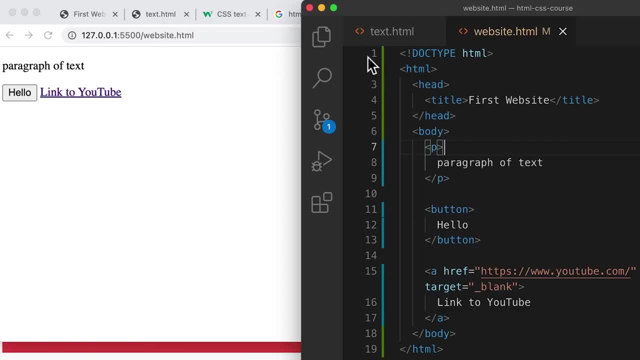 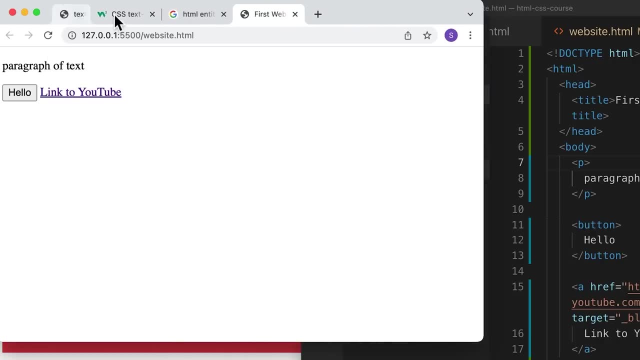 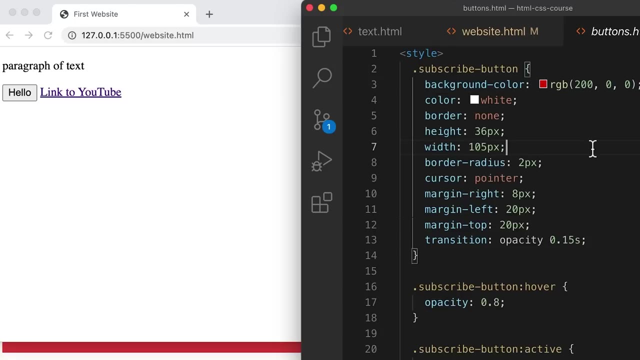 to speed up our development. Now let's get some more practice and we're going to convert both of these HTML files to use the proper structure. First, I'm going to actually just delete all the extra tabs here, And now let's work on the buttons file. 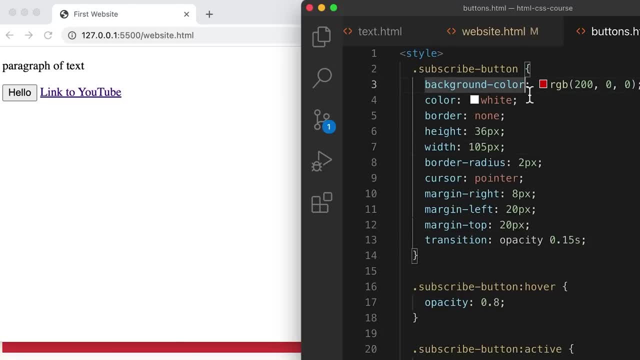 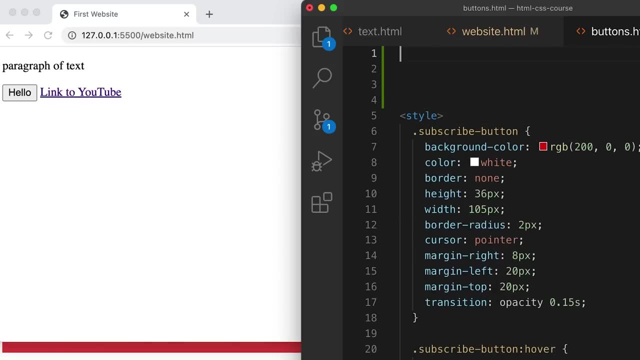 Now, the live server doesn't really work if we don't have that proper HTML structure in our code. So let's add that structure first. I'm going to go up here and we're going to create the structure. So remember we start with a doc type. 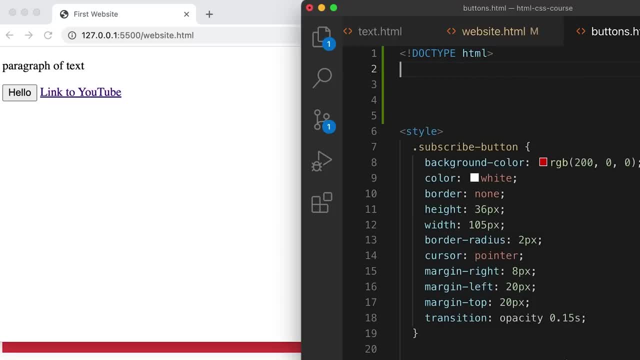 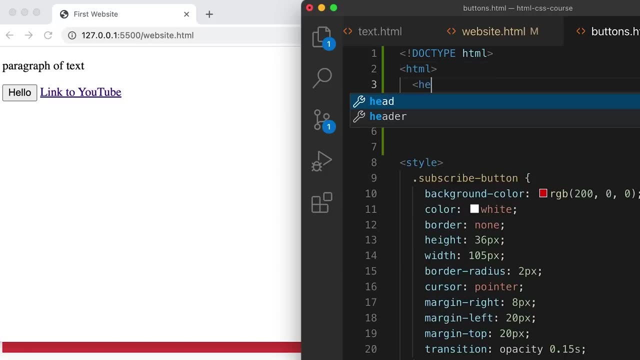 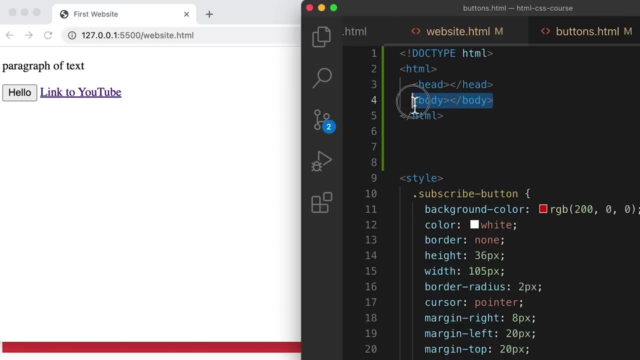 space HTML and then we're going to create an HTML element And then inside we're going to create a head and we're going to create a body element. And remember, the body contains everything that is visible on the page. So if we scroll down, 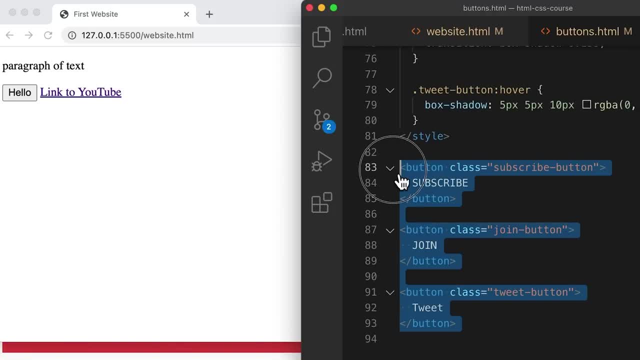 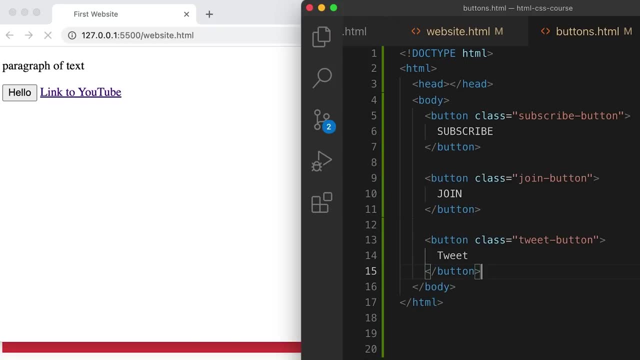 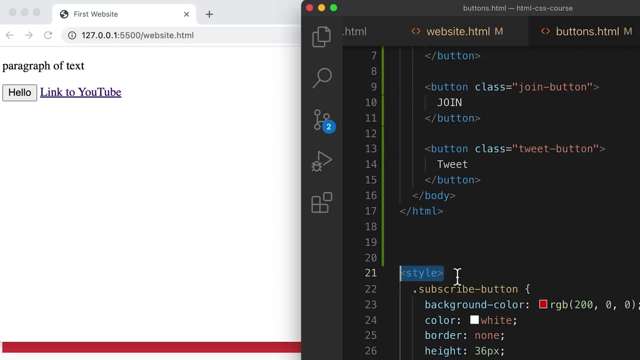 these three buttons are visible on the page, So we're going to move these into the body element And now they're in the right place. Now for this style element. remember that we said: the style element doesn't actually create anything visible on the page. 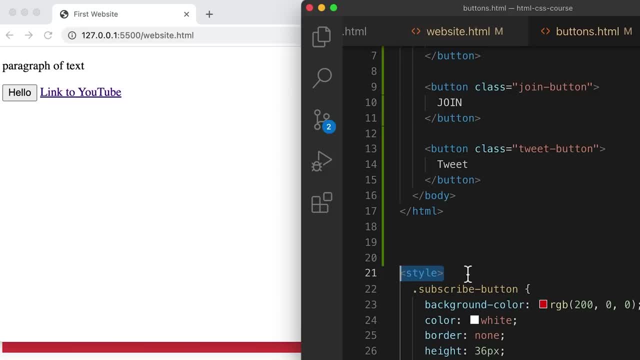 but it could change the style of other elements. So this is a good example of something that should go in the head element, because it doesn't show up visibly on the page. So we're going to copy all of this and put it into the head element. 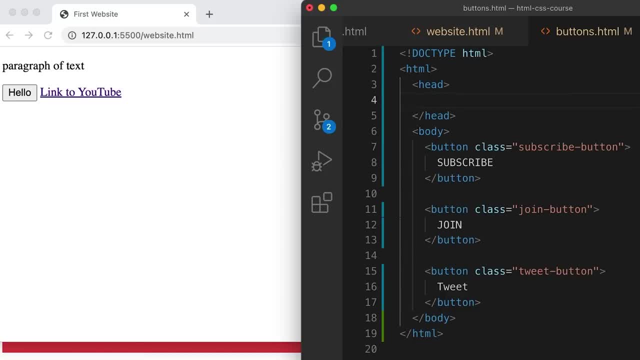 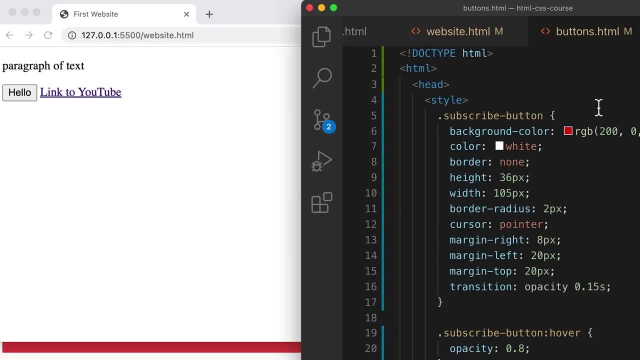 I'm going to go up and we're going to save this in here. So now all of our CSS code is in the right place And now that we have the proper structure, we can open this with our live server, just to make sure everything looks good. 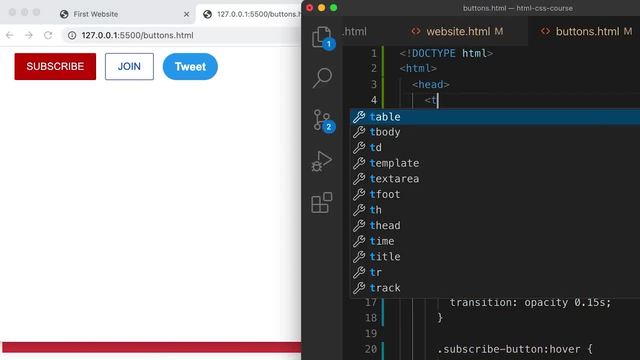 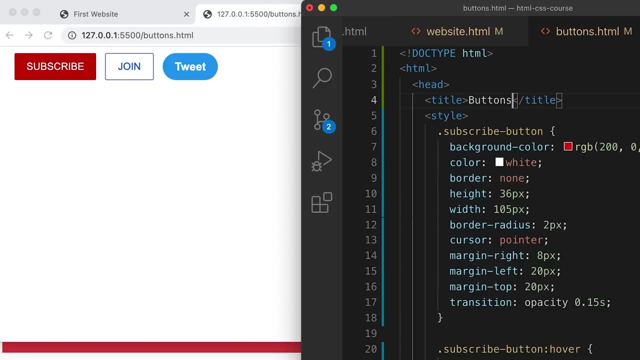 Let's go here and add a title, like we learned, And this is going to change the text at the top of the tab. So let's call this: buttons, practice, Save it and you'll notice that it automatically reloads. Now we're going to. 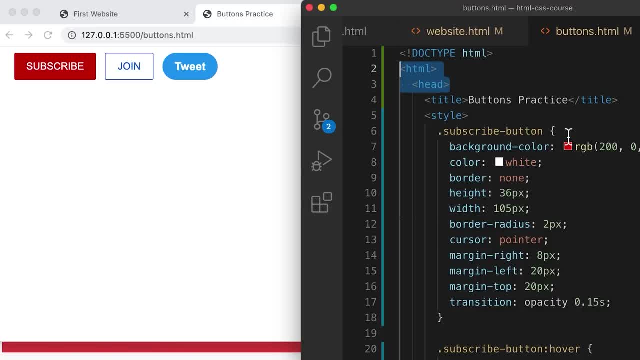 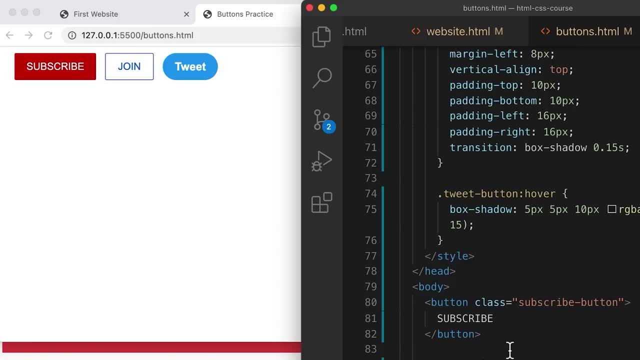 learn another feature that we get from following this structure. If we look at our code, we have all of our CSS code together along with our HTML code. Now this gets confusing because we have a lot of lines of code and we're mixing two different languages. 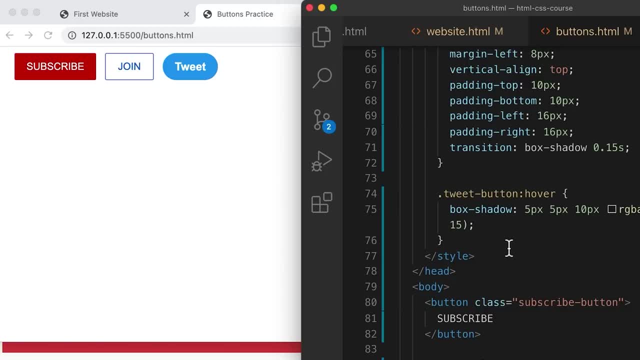 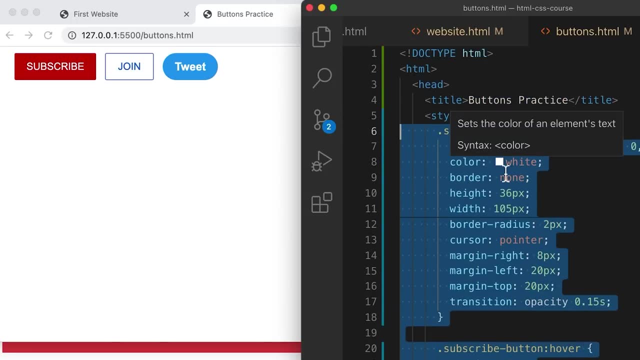 To solve this problem, we can move all of our CSS into a different file. So let's copy all of this and we're going to create a new file to just contain our CSS. We're going to go here and create a new file And let's call it. 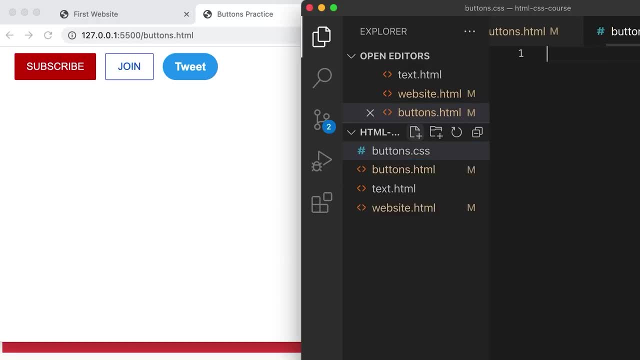 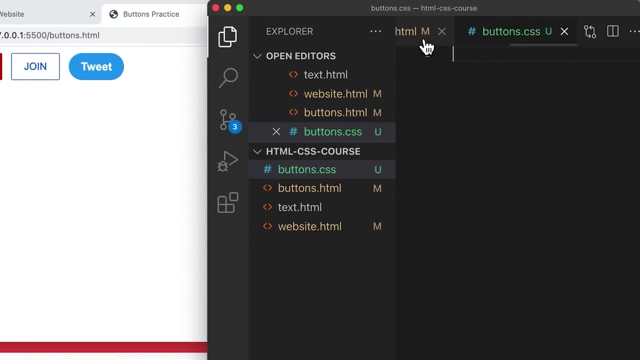 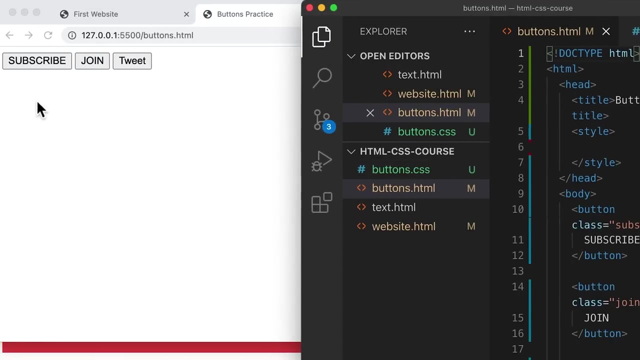 buttonscss- Make sure your file ends in css- to tell the computer that this file contains CSS code. And now we're going to move our code into that file And save And save here. Now you'll notice that we lost all of our styles. 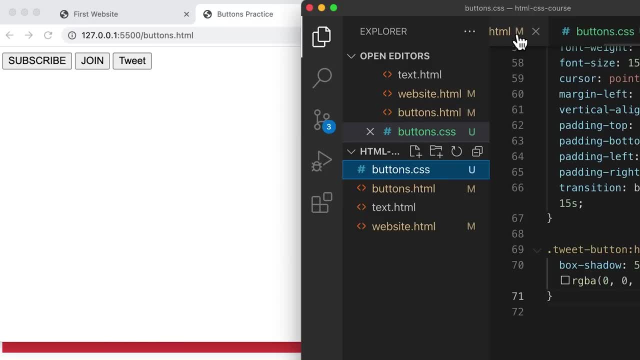 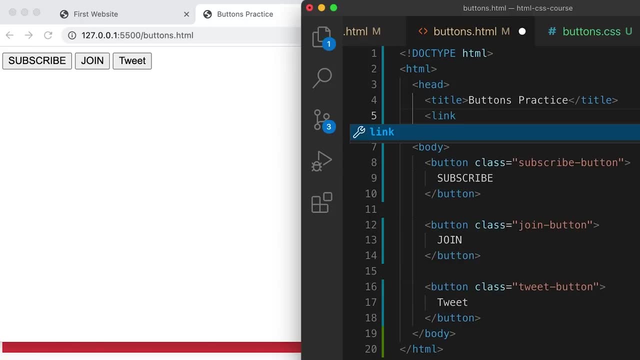 and that's because we now need to load this new CSS file into our HTML. To do that, we're going to learn a new element called the link element. So the link is sort of a special element because it doesn't require a closing tag like we've seen so far. 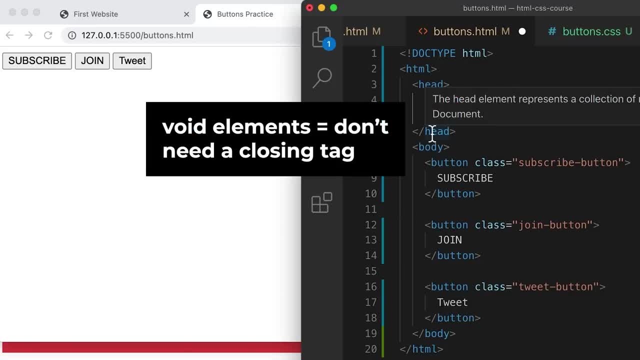 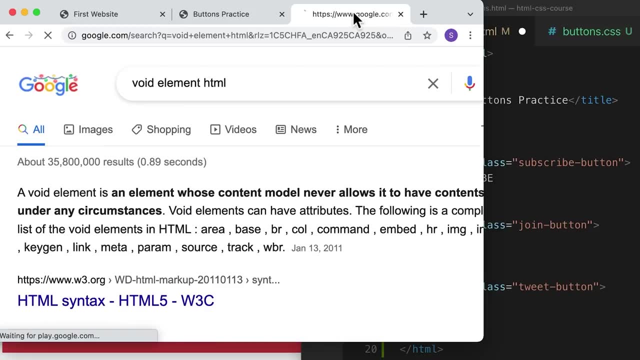 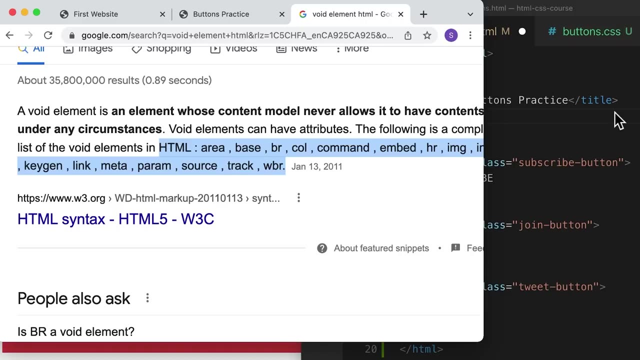 Elements like these are called void elements. So if we search for Google and we search void elements, HTML, this will give us a list of elements that don't need a closing tag. So these are the exceptions to the rule that everything has to have a closing tag. 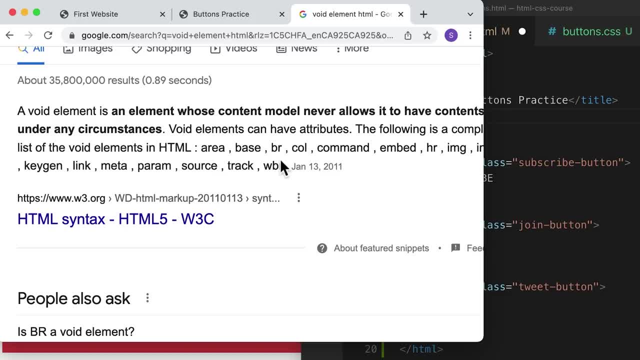 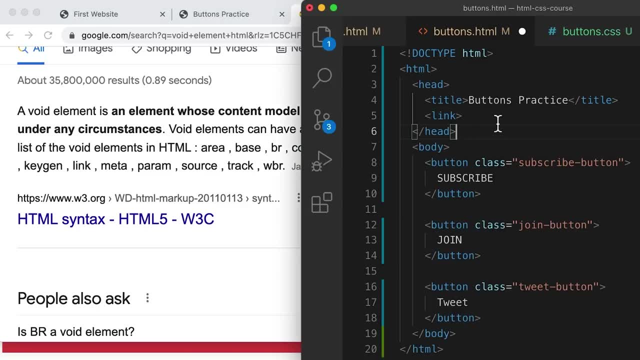 So don't worry too much about memorizing all of these. You'll get more used to it the more that you write HTML, And I'll introduce these elements to you one by one. So here we're going to learn our first void element which doesn't need a closing tag. 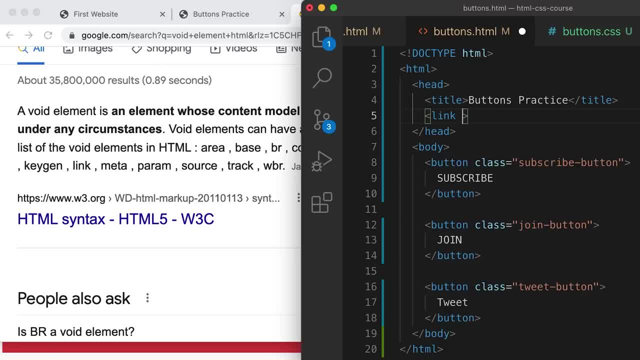 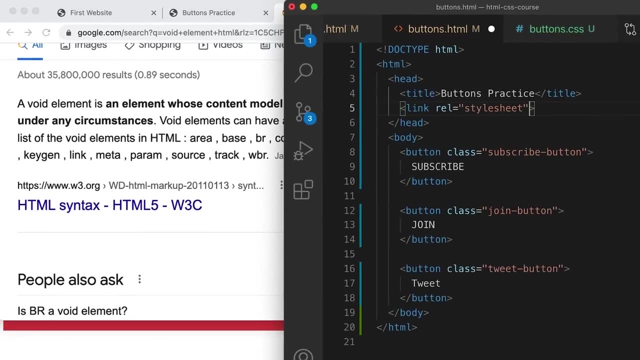 But this element takes two attributes. The first one is called REL, which stands for relation. So what kind of thing are we linking in? In this case? we're going to link in a style sheet And then we have to tell it. another attribute, which is: 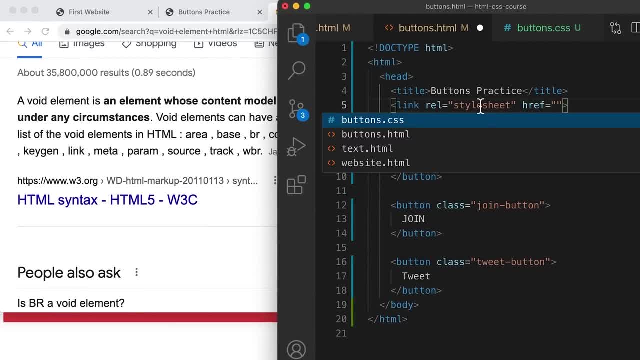 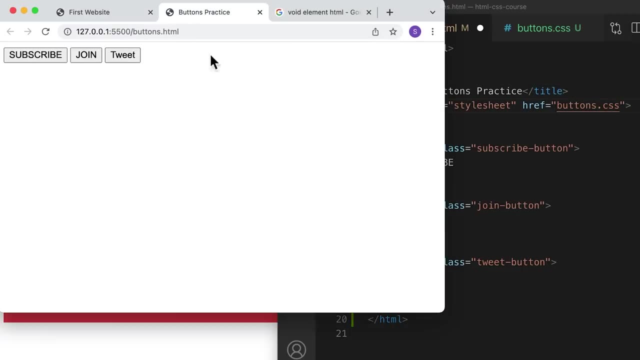 href. So this tells the link what file we're going to link into this file. So here we're going to link our CSS file into our HTML. We're going to link buttonscss. Now let's go back to our page. You'll notice we don't have our styles. 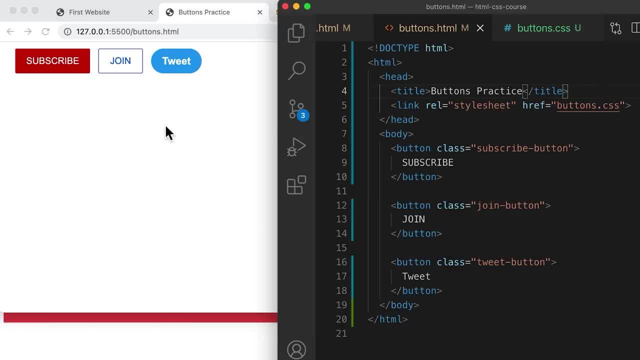 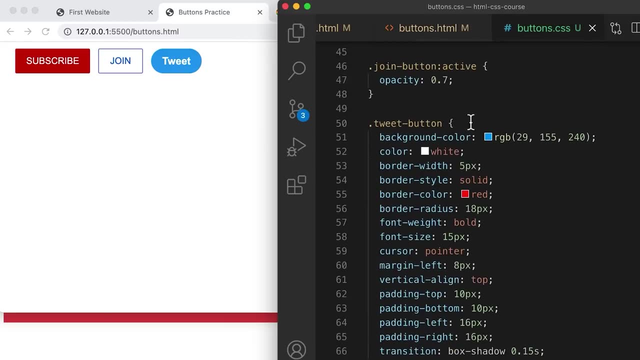 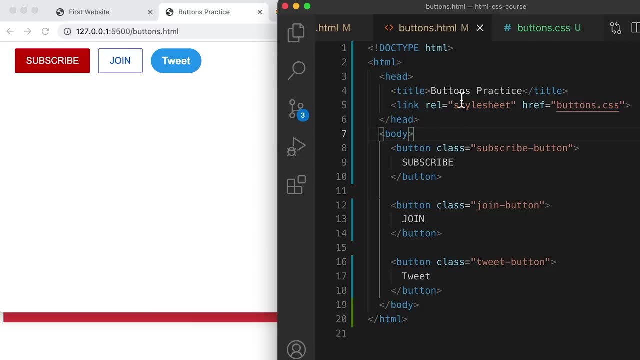 And now, when I save this, we get all of our styles back, And that's because we're loading all the CSS code found in buttonscss- which is all the code we had before- into our HTML. So this is another way to load CSS without having to write it all. 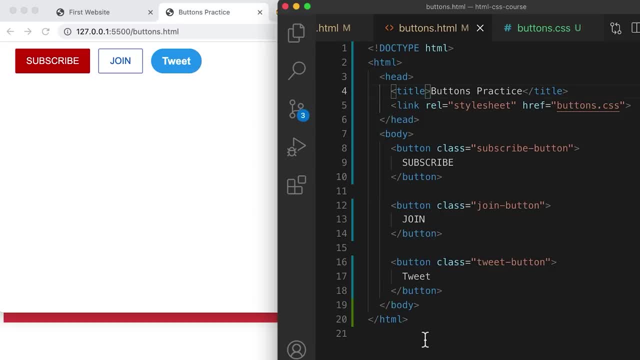 in our HTML file. Now, the big benefit of this is that each file contains less code and each file contains one type of code. So in this file we only have HTML code and in this file we only have CSS code. So it makes the files smaller. 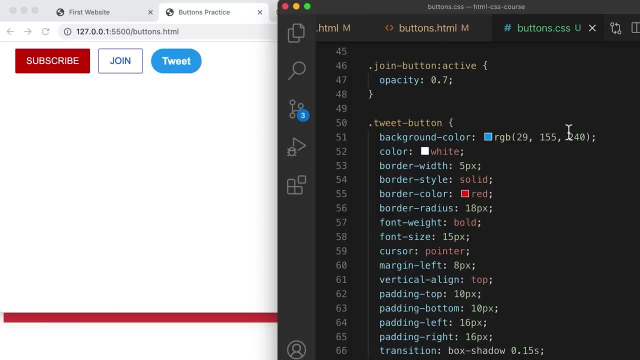 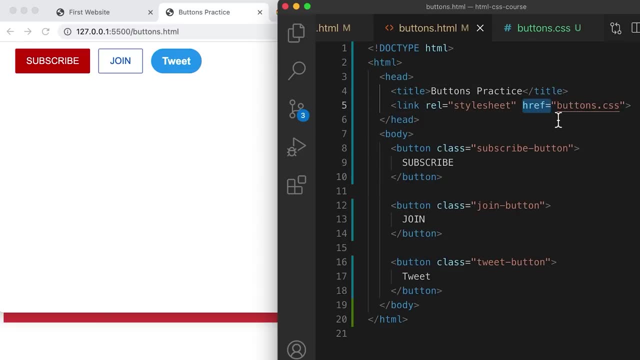 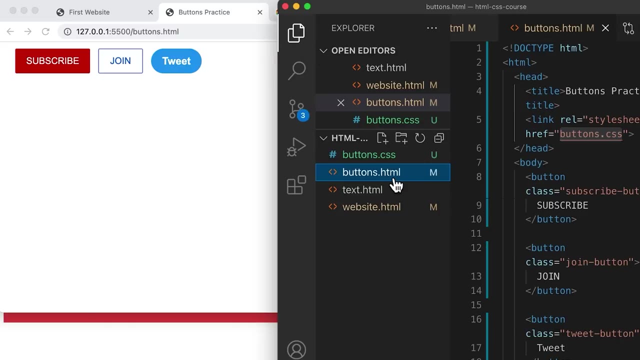 and more focused, And that's going to help us develop easier. Now, before we move on, I do want to talk about the href attribute. So the way that the computer finds this file is that it's going to search right beside our HTML file. 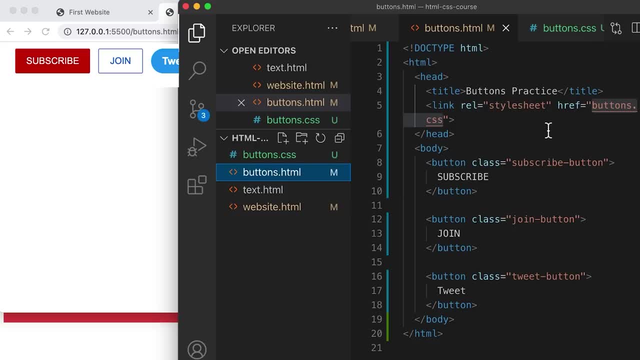 So it's going to search right beside the file that this code is in. So it's going to look for a file called buttonscss. it finds it and it loads it into our HTML. But if this file was in a folder, let's create. 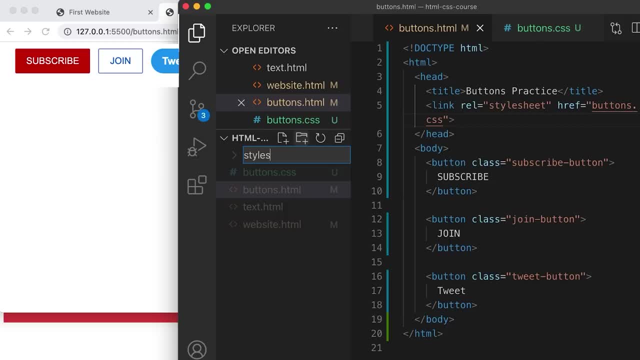 a new folder. let's call this styles. Let's put the CSS file in our new folder And now you'll notice that the styles are gone, And that's because this link can't find buttonscss anymore, What it's trying to do. 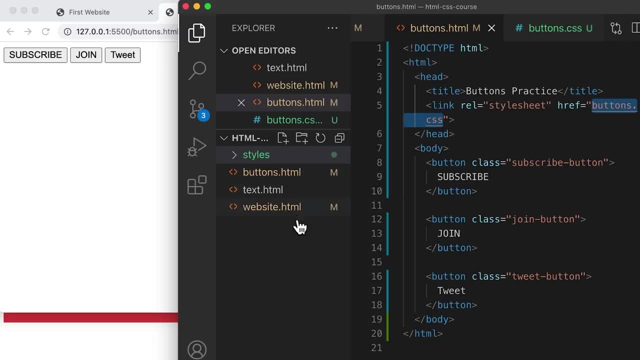 is it's trying to look for a file called buttonscss beside our HTML and there's nothing there. So to link a file that's inside a folder you first have to give the name of the folder that's beside the HTML file In this. 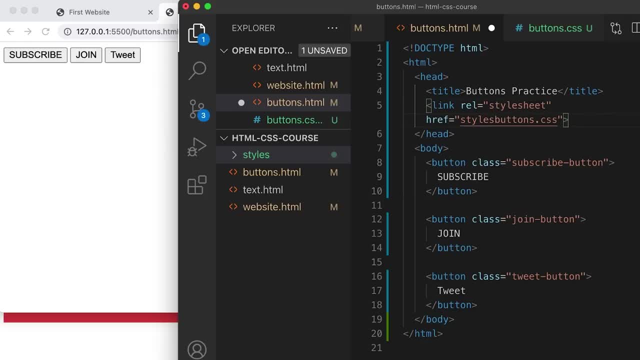 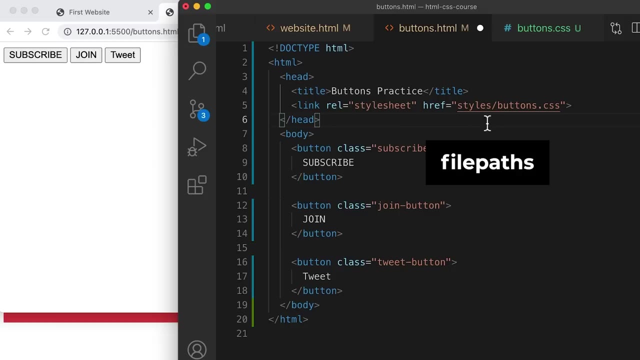 case it's styles. Next we have to type a slash. So this slash means we're going into the styles folder And then inside we're going to find the buttonscss. So this is something called file paths, And this is basically how we locate different files. 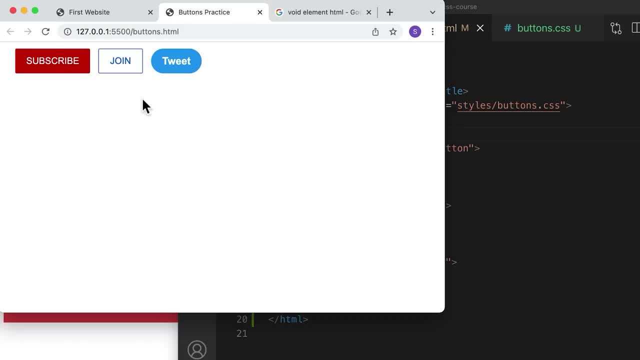 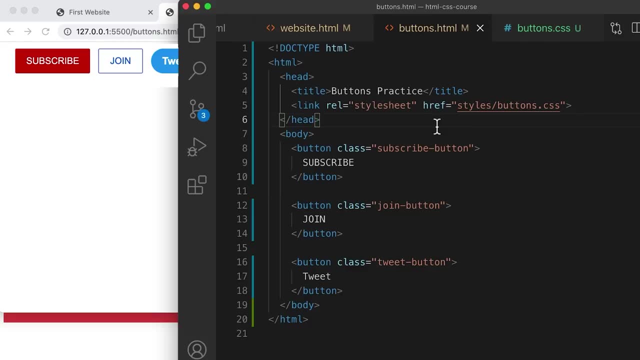 within our HTML code. So let's save this, and now we're able to successfully link our CSS file. So that's a little bit about how file paths work. We're going to need to use this later on in this course when we recreate YouTube. 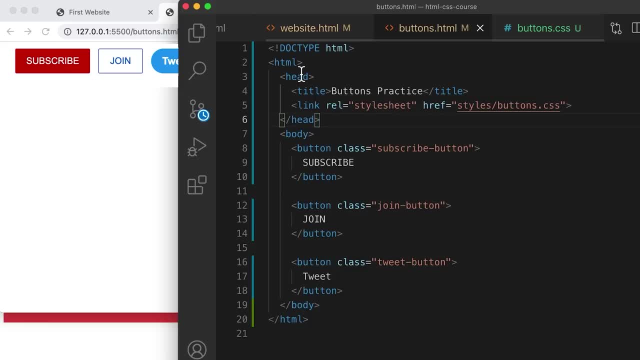 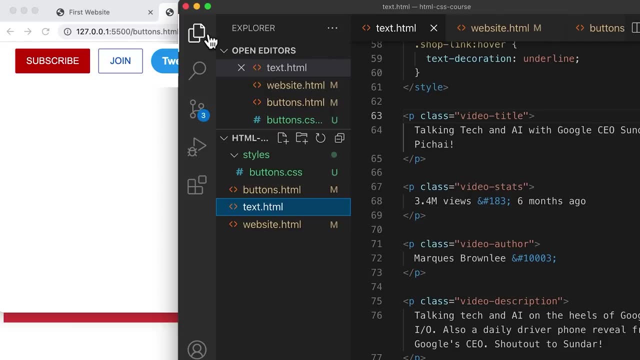 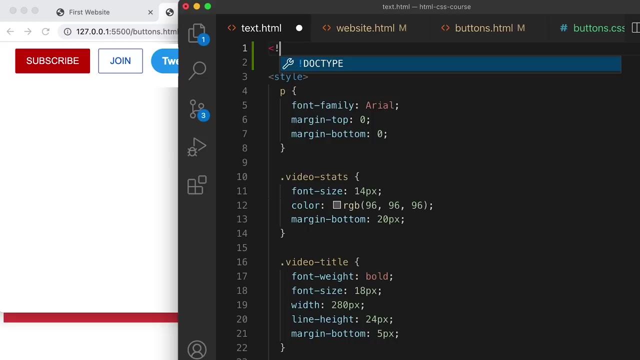 dot com. Now let's get some more practice and we're going to convert our final file into the proper HTML structure. So let's create the structure first, because we can't use live server just yet. We're going to write a doc type space. 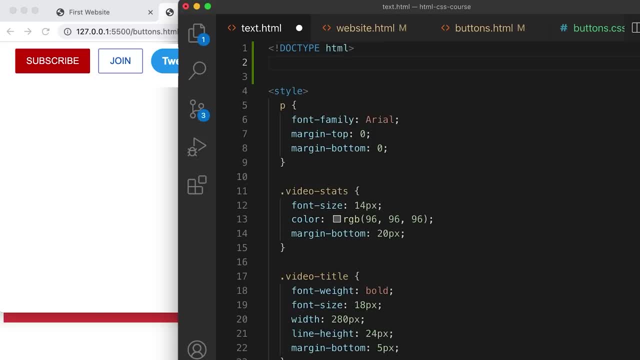 HTML at the top, and then we're going to have an HTML element, and then inside we're going to have a head element and then we're going to have a body element. Now everything that is visible is going to go inside the body. So if we scroll down, 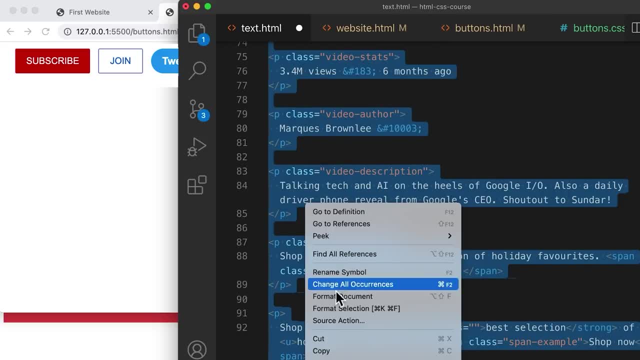 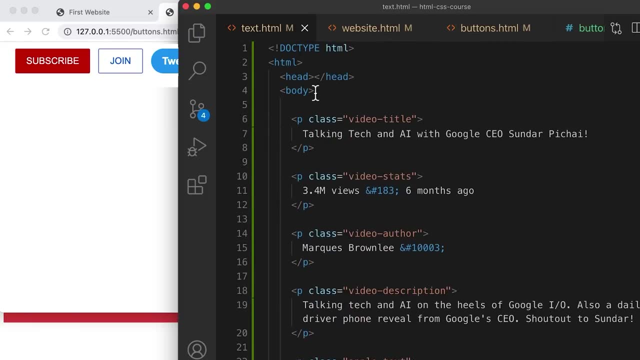 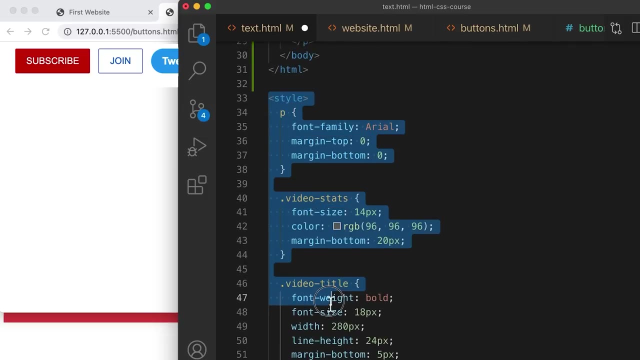 all of our paragraphs are going to go inside the body. Cut and paste, Save it. and now anything that's not visible is going to go inside the head. So if we scroll down, the style element is not visible on the page, so it's going to go inside the head element. 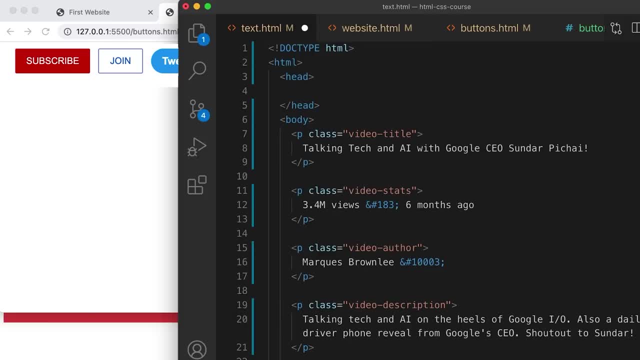 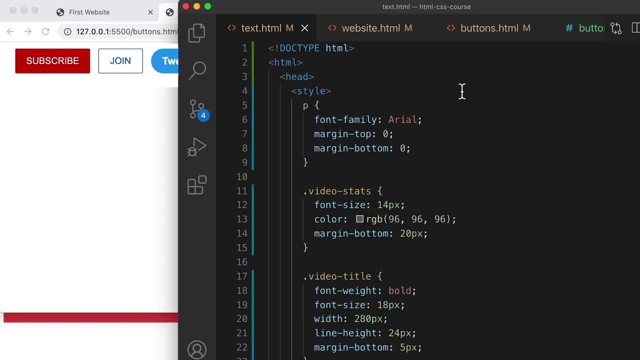 Cut and paste. Alright, So now we have a proper HTML structure. We're going to open this with live server, Move it to the left. here Everything looks good And we're going to do some more practice. We're going to set the title. 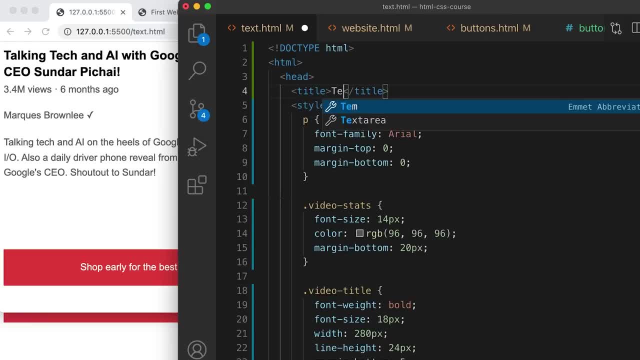 again. just to get more repetition, Let's call this text practice, Save it and you're going to notice that the title is set up here And we're going to move all of this into a CSS file. So let's create a new file. 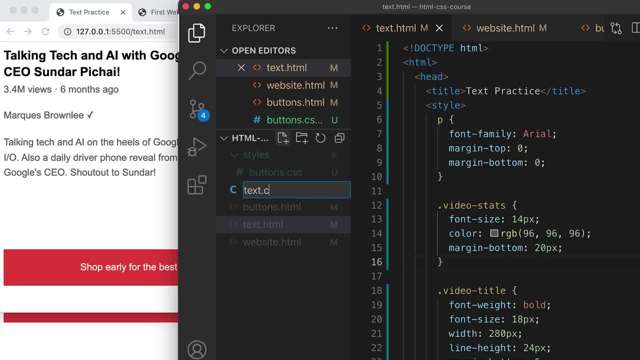 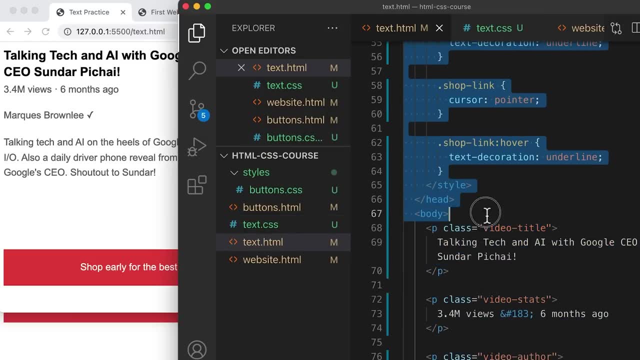 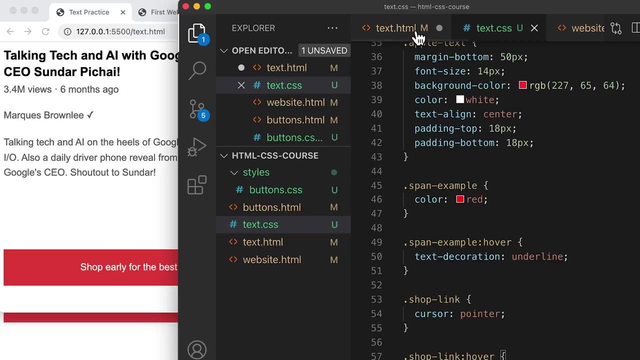 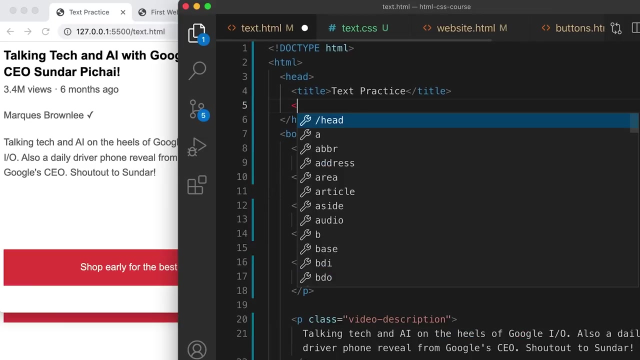 called textcss And we're going to move all of the CSS code into there, So let's cut and paste it into here. Next, we're going to link the CSS file in this HTML file. Let's create a link element. It needs two attributes. 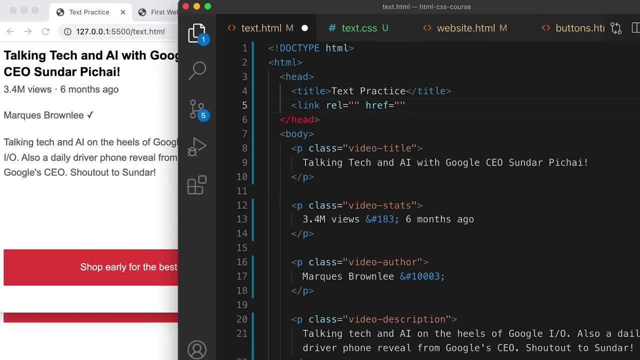 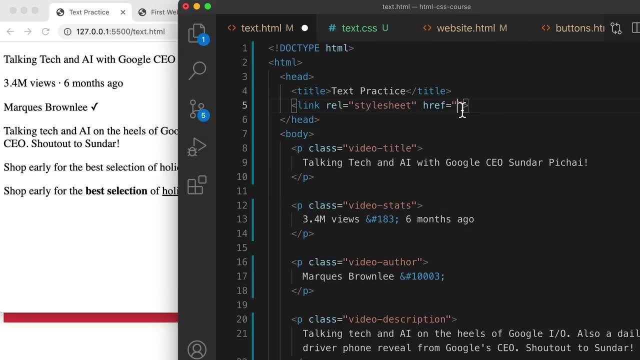 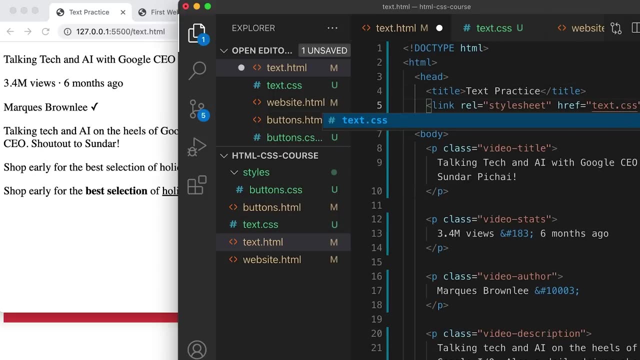 rel and href. So we're going to link a style sheet And the file is located right beside the HTML file. So all we need to do is link textcss, Save it and refresh, And now it's back to where we were. 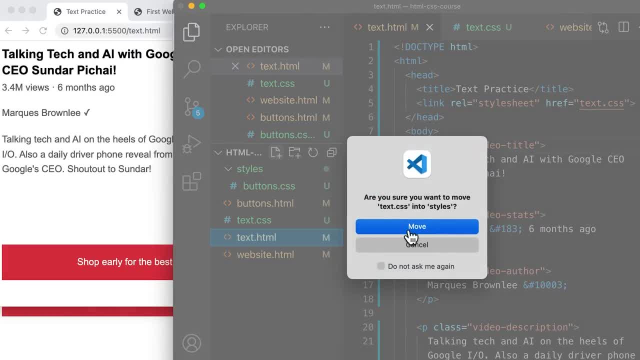 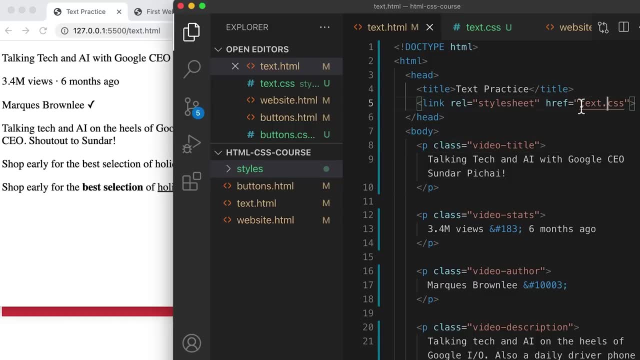 Again, let's practice moving this into a folder. Now we're unable to find textcss beside our HTML file, But there is a styles folder, So we're going to look inside the styles folder. We're going to use a slash to go inside. 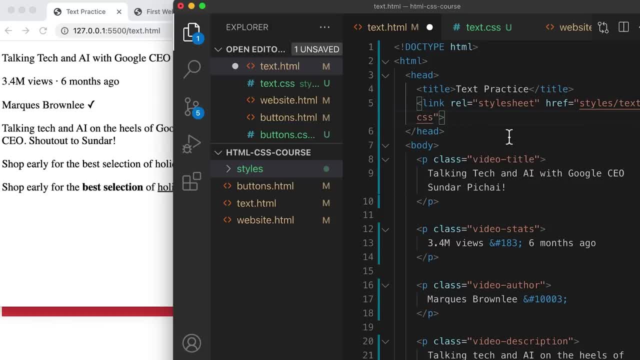 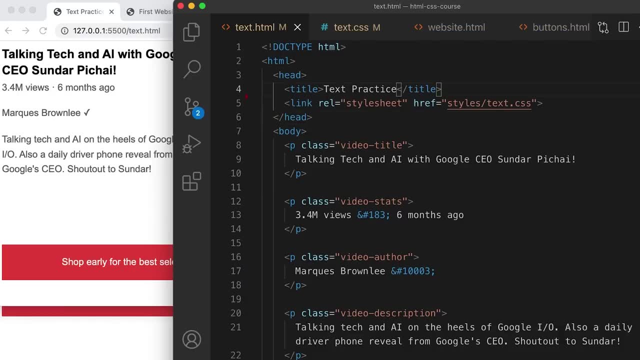 And we're going to link this textcss file, And that is how we use file paths to link CSS files. The last feature we're going to look at that we get from this structure is the ability to add new fonts onto our website. So websites have. 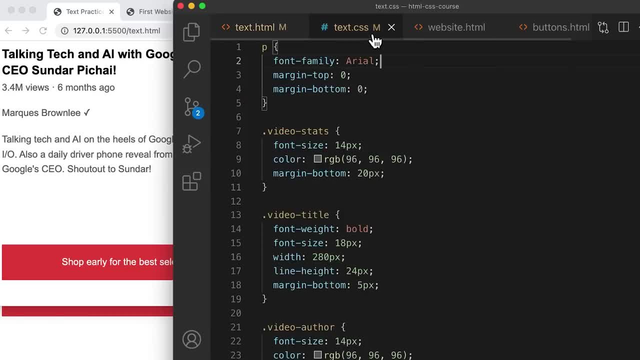 a set of fonts by default that we can use. For example, one of them is called Arial. Another one that we've seen is called Times New Roman. That's basically the font that we get on a fresh website. Now, in addition to these default, 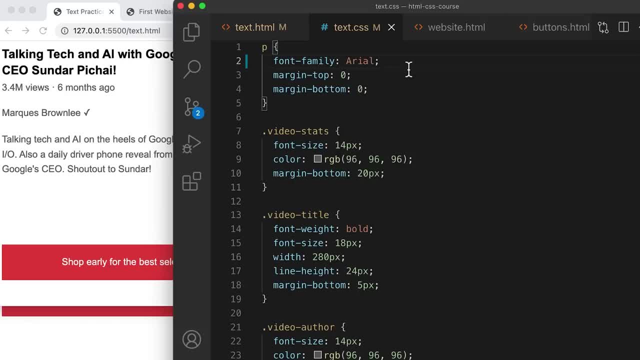 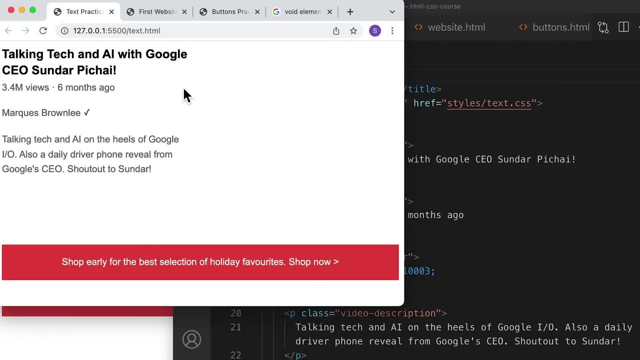 fonts. we can actually load new fonts from the internet, And we're going to learn how to do that within this structure. So let's go to our webpage, And Google actually provides a lot of really great free fonts that we can use, So we're going to open. 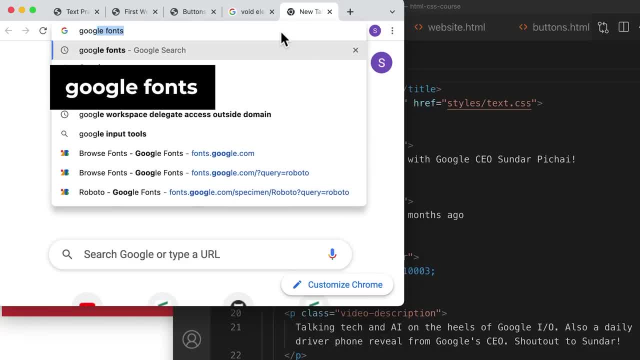 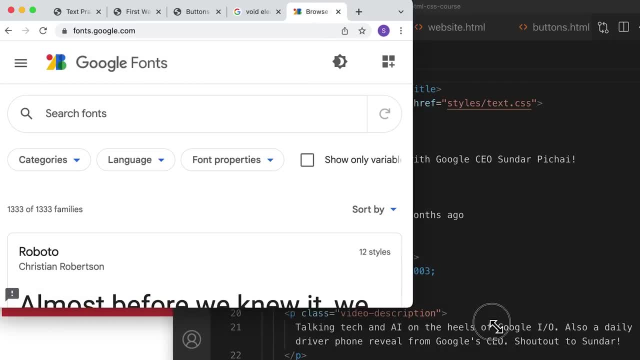 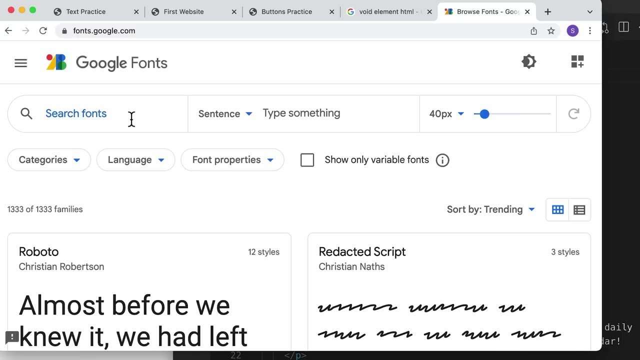 a new tab And we're going to search for Google fonts And we're going to go into this first link. Now this website might look a little different for you, but the general process is the same. First, we're going to search for a font that we like. 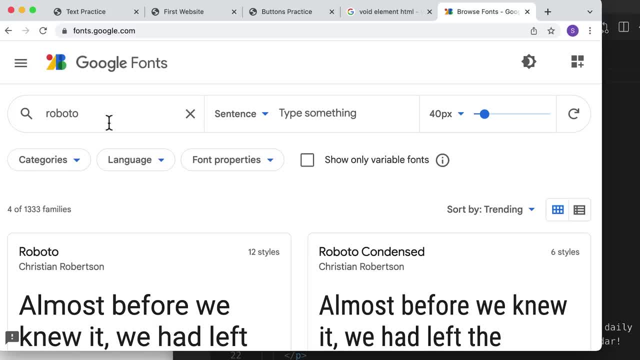 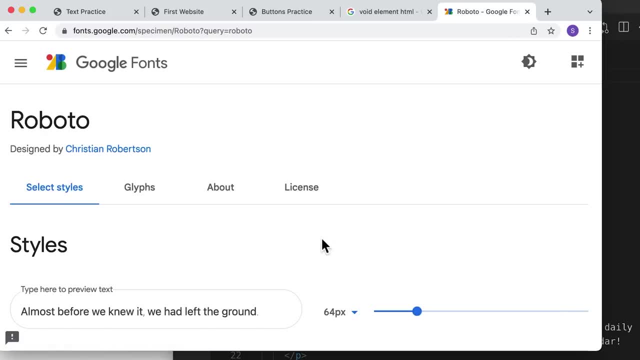 So a good font to use here is Roboto, And this is the font that we're going to use for our final project. We're going to pick this font And then inside here we're going to pick the styles that we want. So for 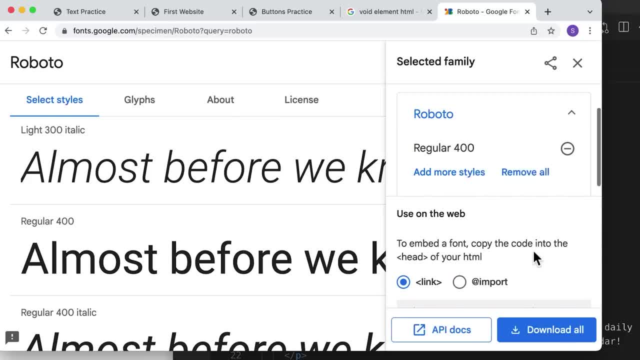 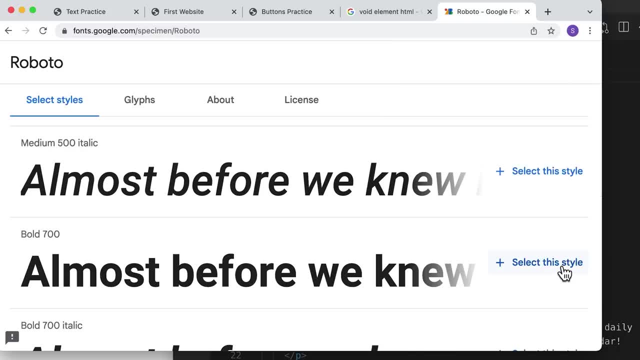 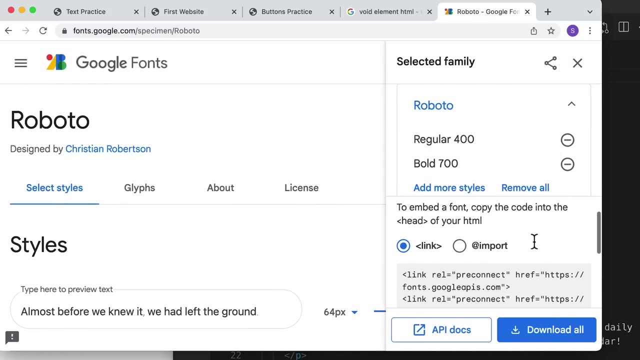 example, I'm going to pick the regular style And I'm also going to pick the bold style here. So I'm going to pick the bold style And then I'm going to go to the basket of fonts that I selected, And then Google is going to. 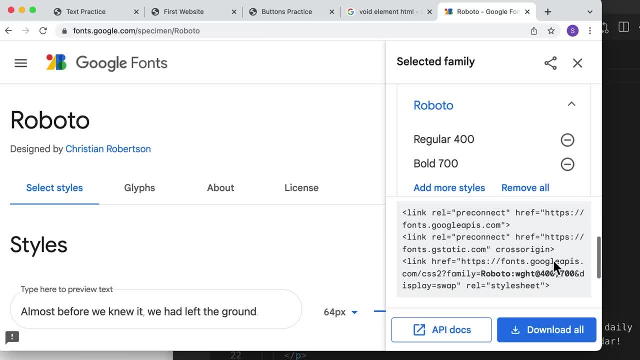 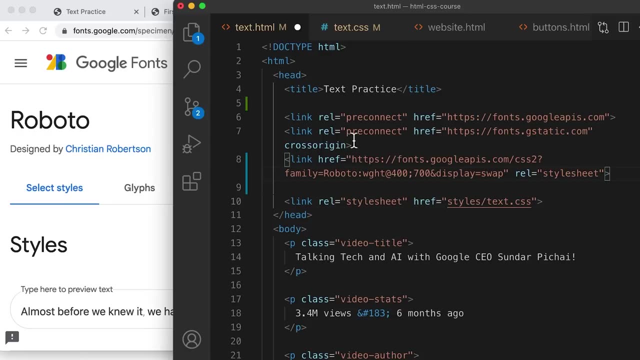 give me the code that I need to load these fonts. All we need to do is copy this code exactly and then put it in our head section of our HTML. So we're going to put it in our structure, in this head section, And now. 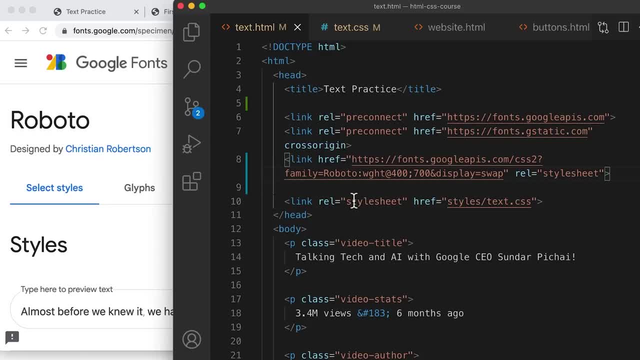 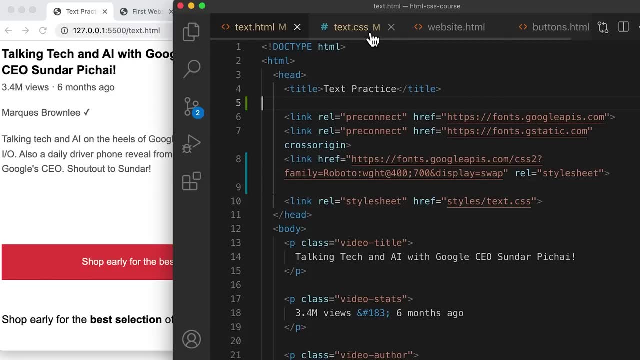 we've loaded a new font that we can use on our website. So now let's go back to our website and we're going to use this new font. So remember that currently we set our fonts to Arial. This time we loaded the font called Roboto. 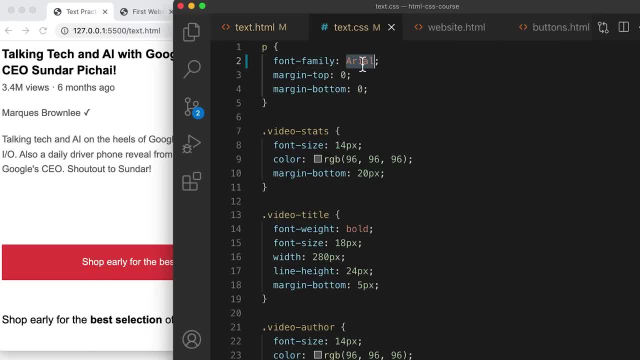 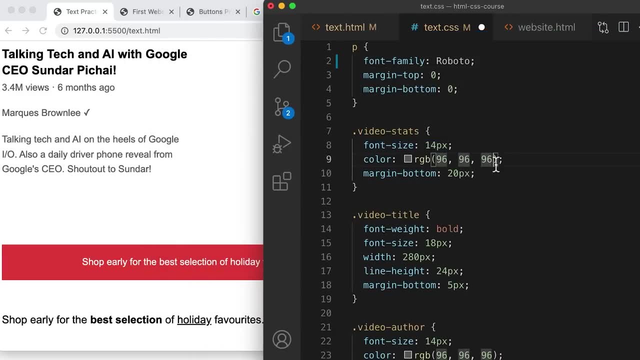 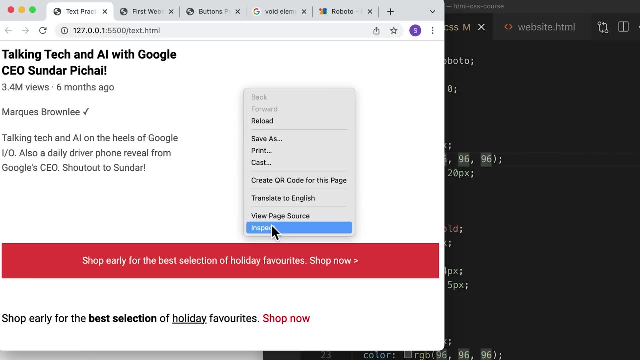 and that's what we're going to use. So let's change Arial here to Roboto. Now, when I save, the font is going to change, And there you go. It might not look that much different because Roboto is very similar to Arial, but if 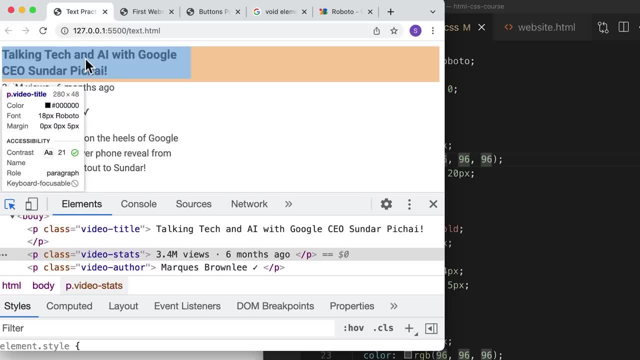 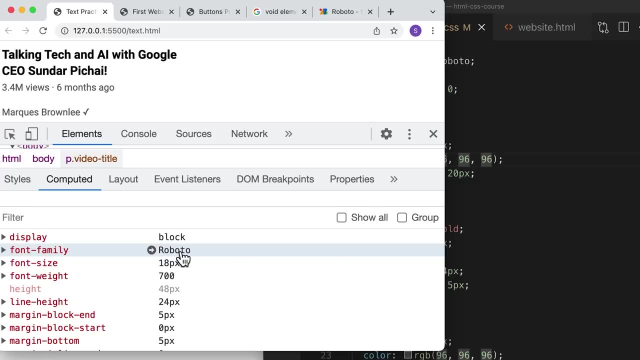 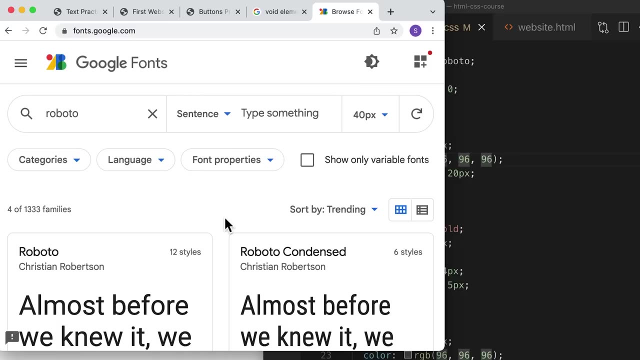 we inspect and we click on this element and go to the computer tab, we'll see that the font family has now been changed to Roboto. So this is how we can load a huge selection of fonts from Google onto our webpage and use them on our website. So those are. 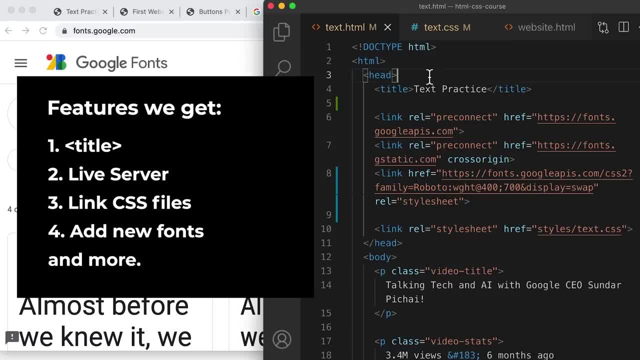 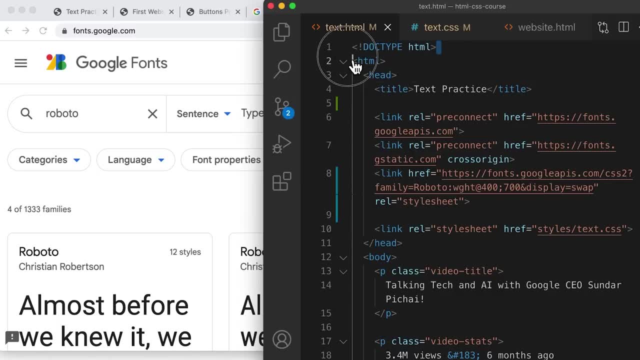 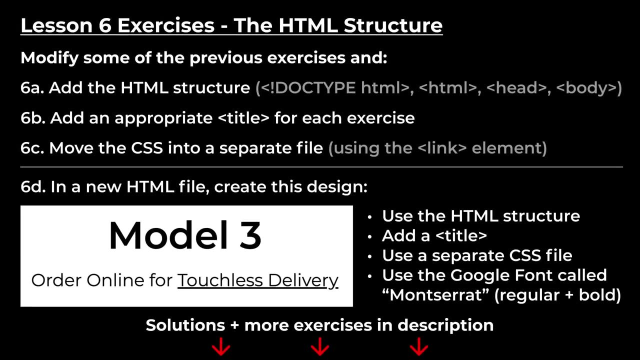 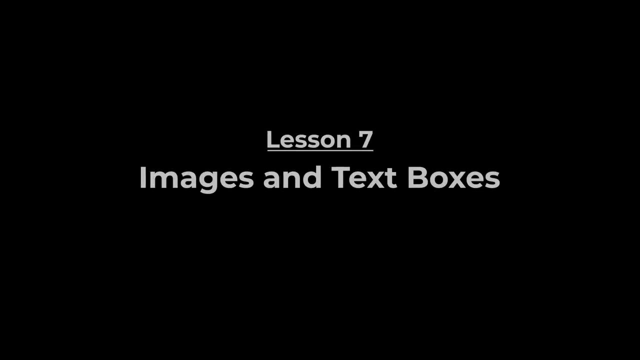 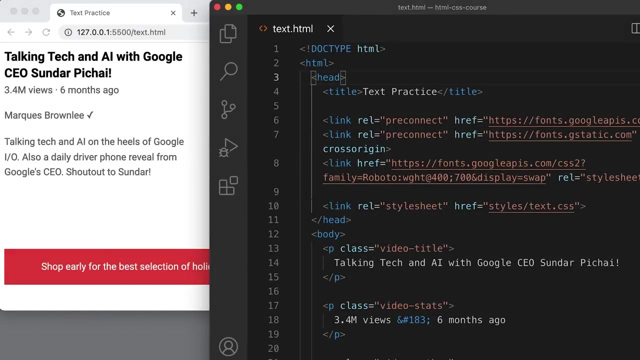 the features that we get from following this HTML structure. Every website that we create from now on will always have an HTML tag, a head and a body and a doctype at the top. Now we're ready to work on the final project of this course: recreating. 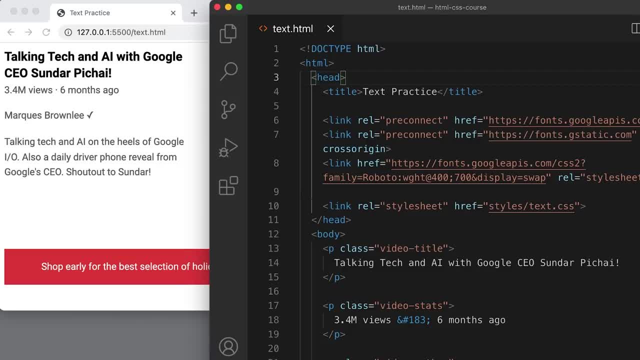 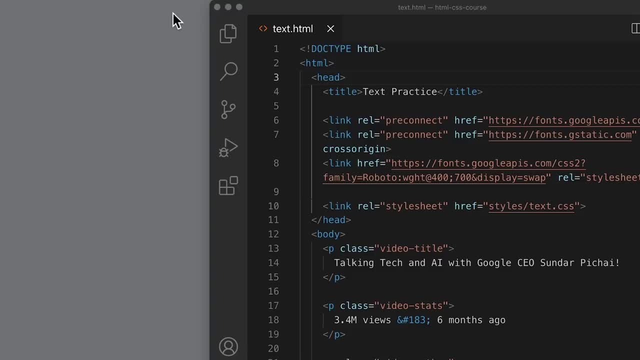 youtubecom. Just like before, I've created a page on my website that'll show us what the final project looks like. So first we're going to close all of our browser tabs because we're going to start over again, and then we're going to open. 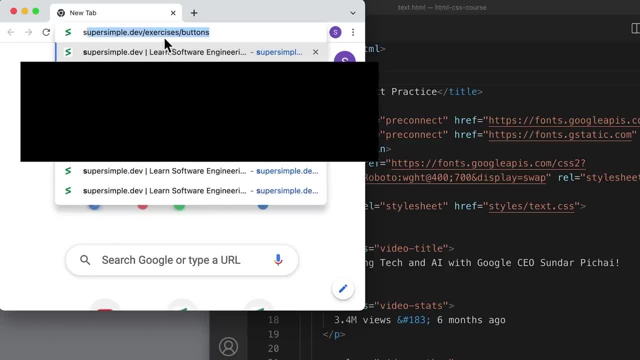 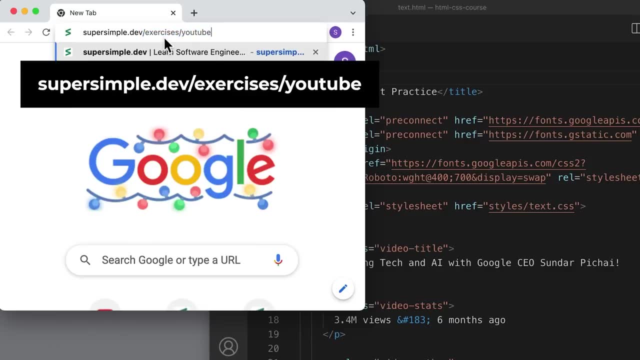 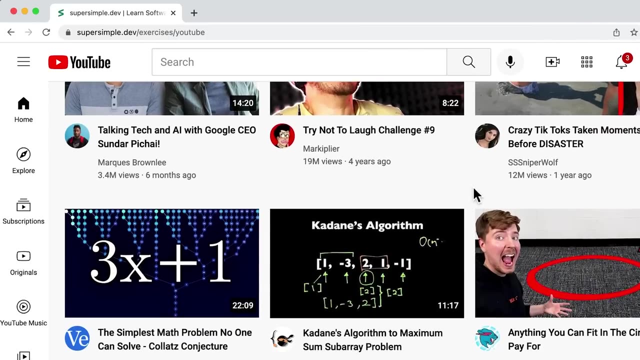 a new page And we're going to go to supersimpledev, slash exercises, slash youtube. So on this page you can see what our final project will look like. So we're going to learn how to recreate youtubecom that you see here. So first, 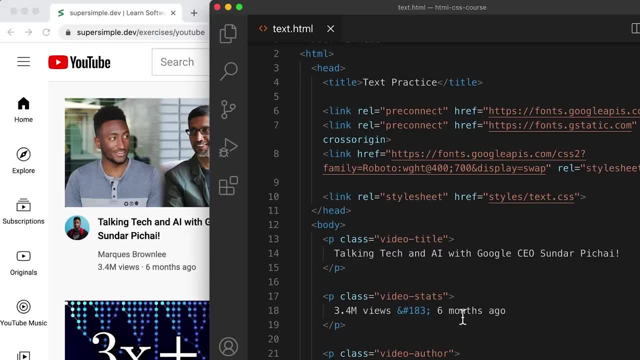 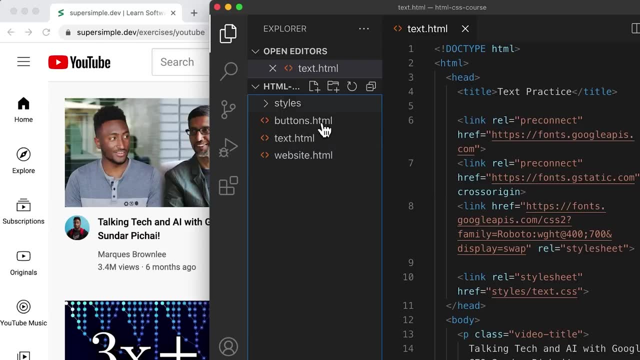 let's set up our project in our code editor, So let's go into here and let's actually create a folder that's going to contain all of our previous code. So the final project is going to contain a lot of code, so we don't want to get it confused. 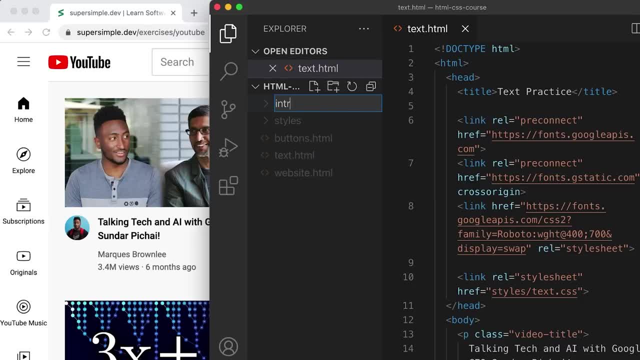 with the previous lessons. So let's call this intro-2 dash html, And we're going to put everything inside this folder. We're going to put this in here and these html files in here as well. Next, we're going to create a new html. 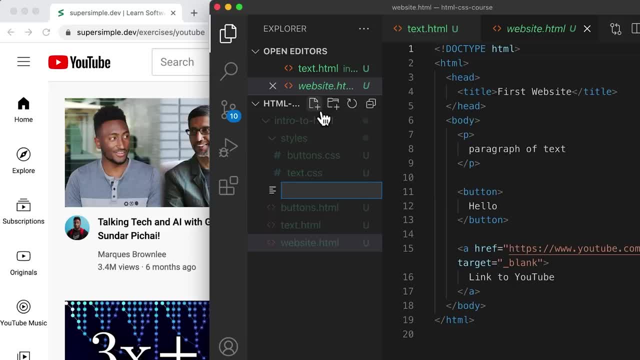 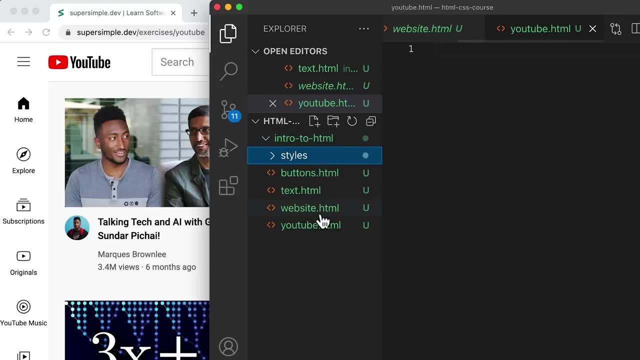 file for our final project. So let's create a file called youtubecom dot html, And I actually put it inside this folder. I'm going to take it out by dragging it down here. So now we have an intro-2 html folder and our youtubehtml. 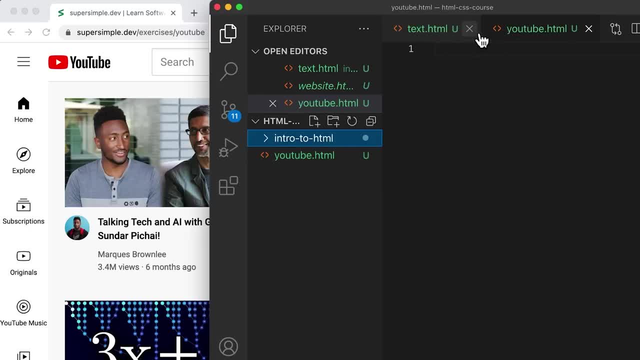 and we're ready to get started. First we're going to set up the proper structure of html that we learned in the previous lesson, So we're going to start off with a less than exclamation doc type And html, And then we're going to create an html element. 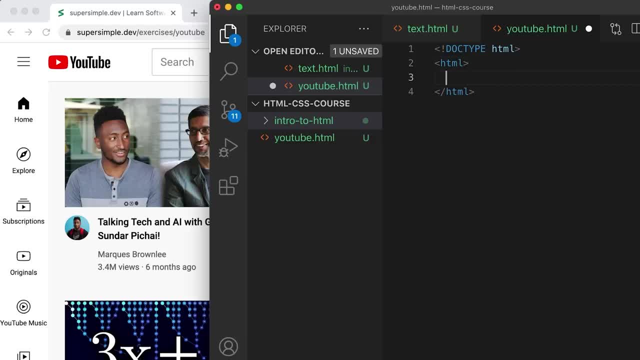 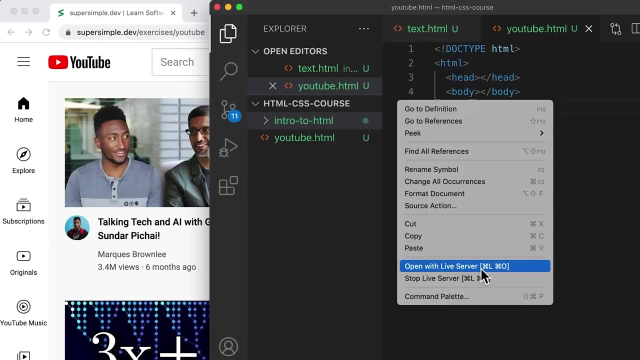 that's going to contain our entire webpage, And inside here we're going to have a head element And we're also going to have a body element. Now that we have this structure, we can open it with live server, And now we have our 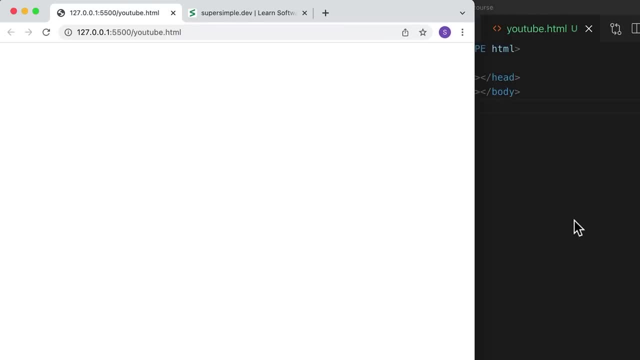 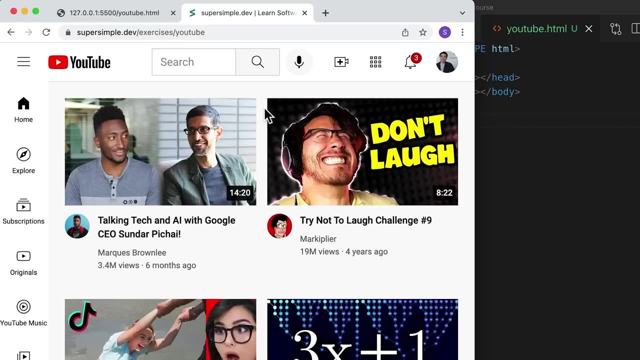 blank page, So this page is going to automatically reload when we change our code. Now, before we can work on the final project, we need to learn two more html elements: How to load images onto our website and how to create a search box. 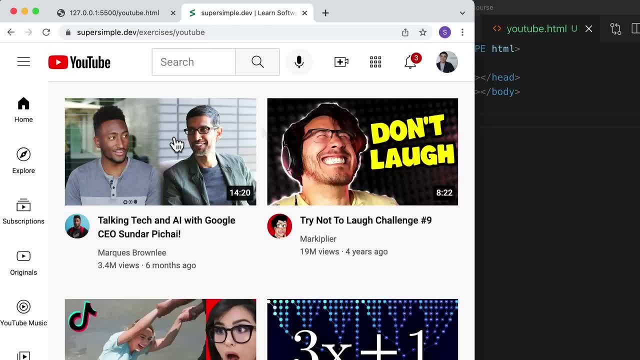 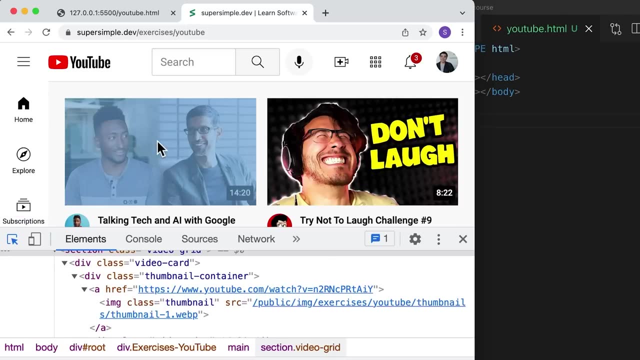 So let's start with loading images first. So I'm going to show you how you can download these thumbnails from my website. We're going to right click in a blank area and inspect, And now, if we click this icon in the top left and hover over an image, 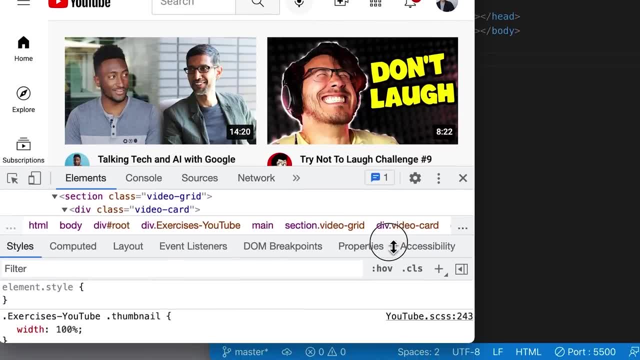 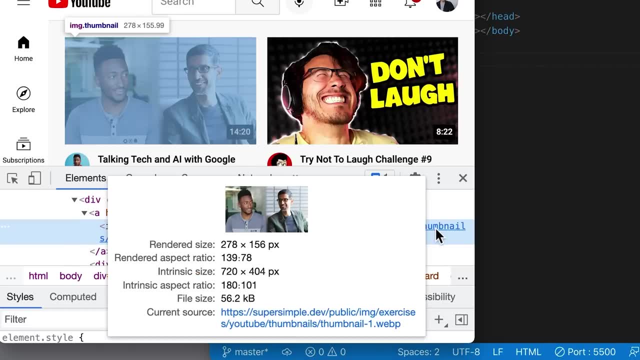 and click it, And you might need to drag this down to see the html. We can find the image in the html and here is the url for the image, So we can actually click this and it will open the image in a new tab. 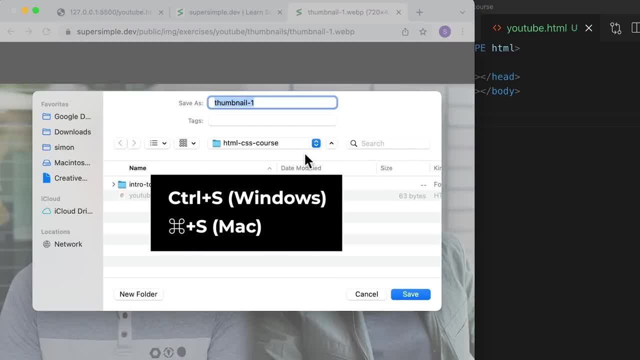 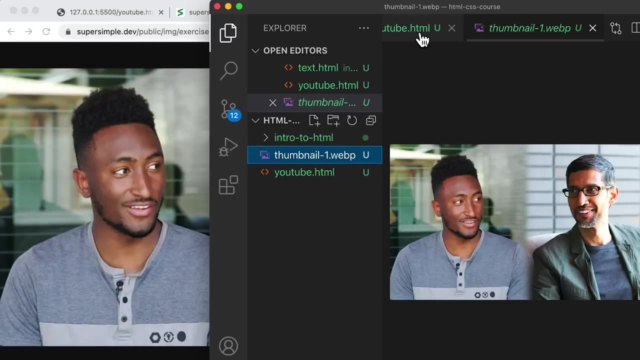 And we can control s to save it. So make sure we save this image in the folder that contains all of our code. So that's this folder for me. I'm going to save it, And now it might take a while, So if I go back to my code editor. 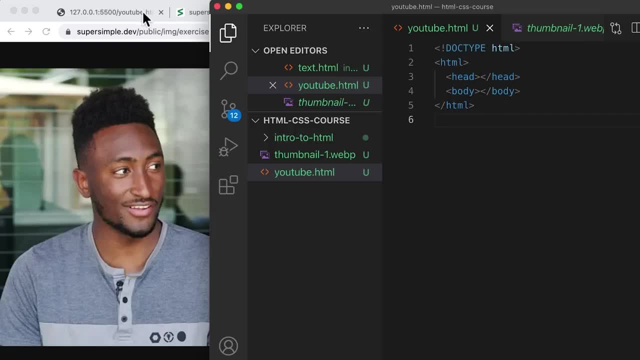 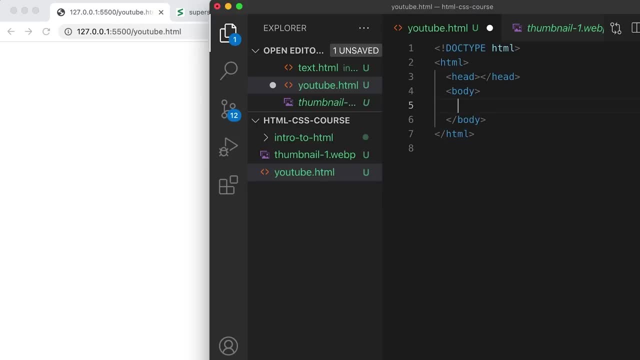 I can see the image. Next, we're going to create an html element to load this onto our page, So I'm going to go back to my page here And then we're going to go into the body and create the image element Which is less than img. 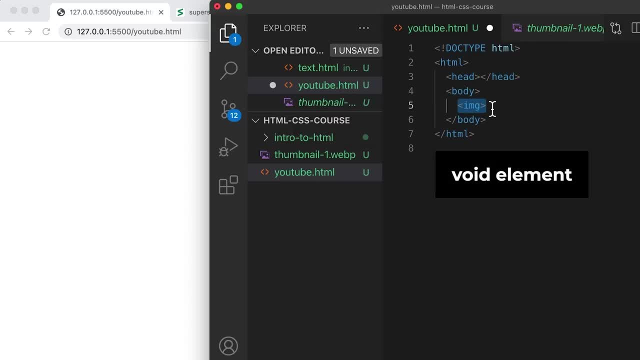 greater than Now. the image element is unique because it's another void element, So we mentioned void elements briefly in the previous lesson. It's an element that doesn't require a closing tag, So we're going to add those exceptions to the rule. 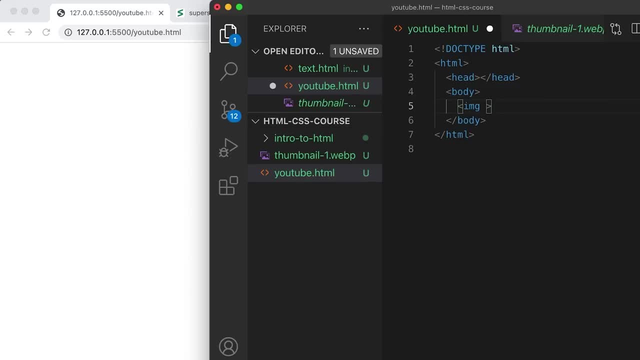 So the image element takes one attribute called src. Now this attribute tells the computer which image to display on the website. So for us, that image is the one we downloaded, called thumbnail1.webp, So we're going to display thumbnail-1.webp. 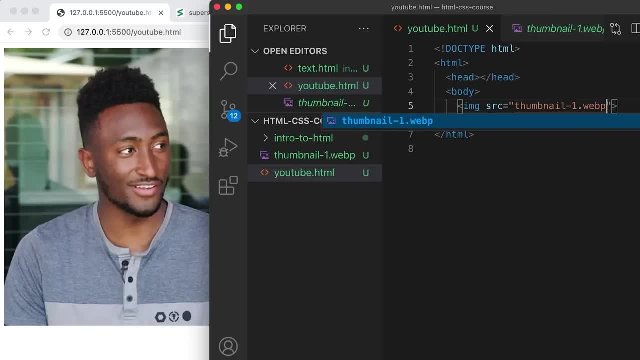 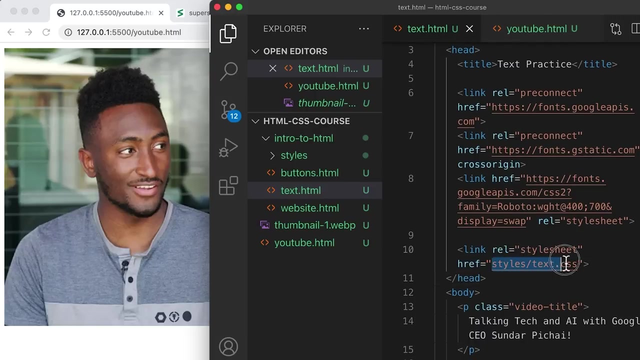 thumbnail-1.webp, And when I save it, the image is now loaded onto our website. So this src attribute works the same way as the link attribute that we saw earlier. It follows the rules of file paths to locate our file. So, just as a reminder, 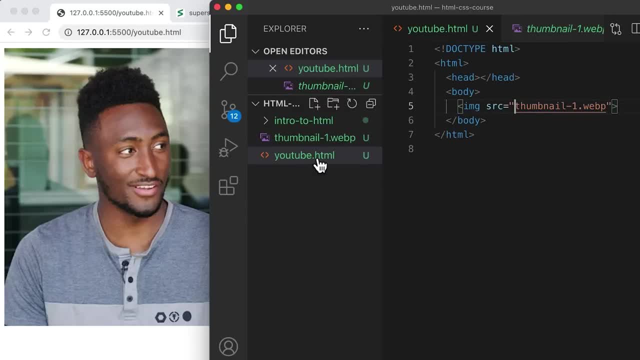 if we type thumbnail1.webp here, it's going to look for a file named thumbnail1.webp right beside our HTML file. It's going to find it and then load it onto our website. But now we're actually going to create a folder. 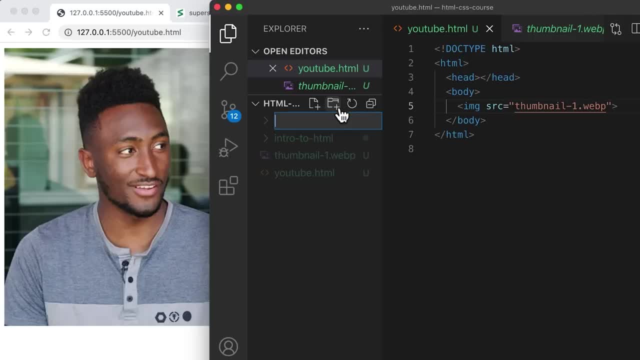 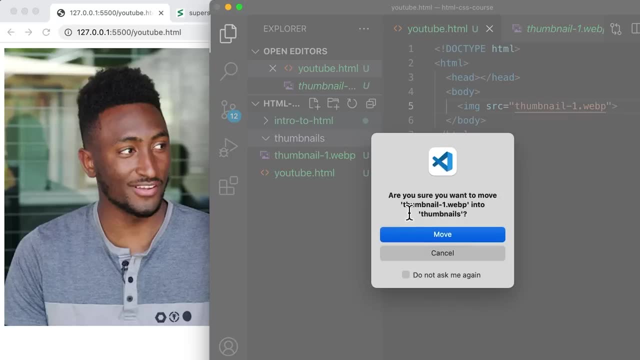 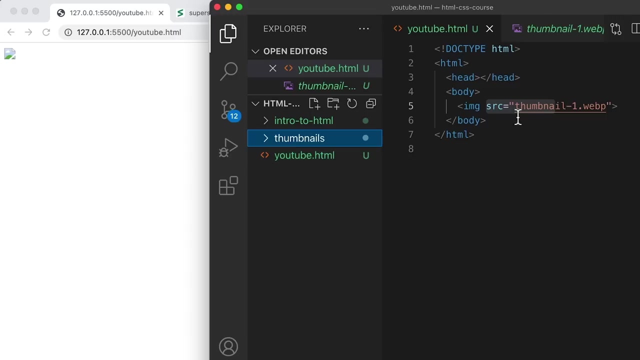 Because we have multiple thumbnails and we want to organize them. We're going to create a folder called thumbnails And we're going to drag this into that folder. So now for this src attribute. we don't have a file beside our HTML called thumbnail1.webp. 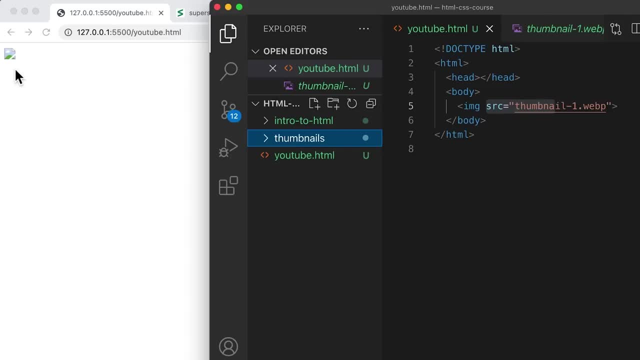 and then you see this error here. So this means that there is an error loading an image. Now, to find it in the thumbnails file, we're going to type thumbnails- slash- thumbnail1.webp. So first it's going to look for a file or folder called thumbnails. 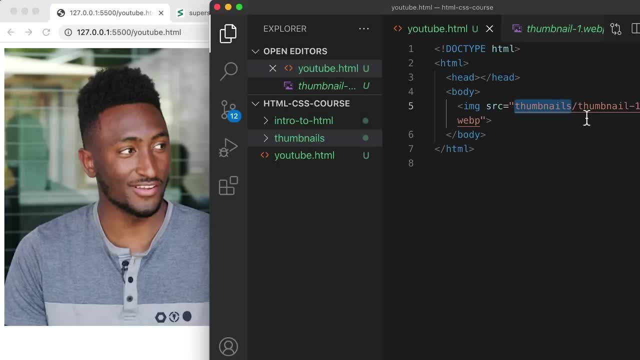 beside the HTML file, It finds this one, and then the slash here means to go inside the folder and then find this file inside that folder, which is here. So that's how we load images onto our page. Now we're going to learn how to style. 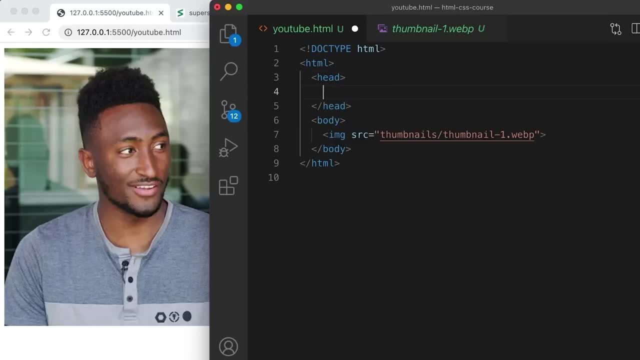 our image elements. So let's go into our head section here and create a style element. Now, before we do that, I forgot to do something, which is: let's create a title for our page So we can call this youtubecom clone. And if we save this, 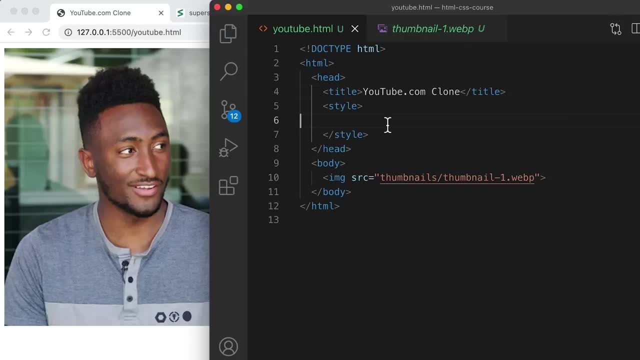 the title will show up in the tabs. Alright, so let's learn how to style our image. So, as always, we're going to give it a class attribute, And let's just call this thumbnail. And now we can target this class in our CSS. 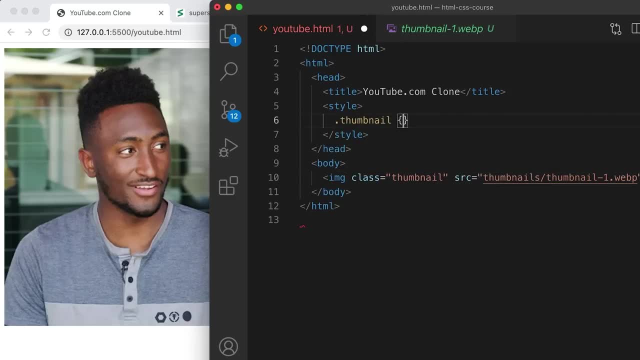 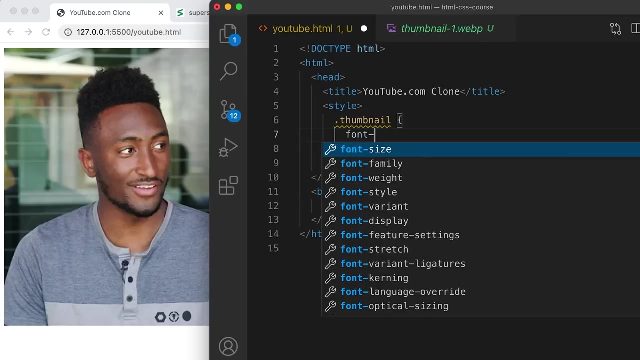 So dot thumbnail. Now, all of the CSS properties that we learned so far apply to the image. Some of them make sense and some of them don't, So one property that obviously doesn't make sense is something like font-size, So if I save it, you'll see nothing changes. 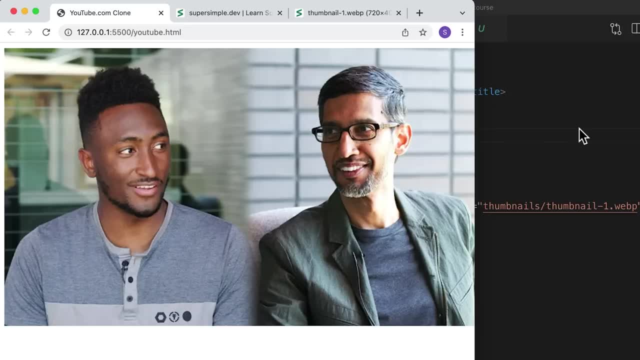 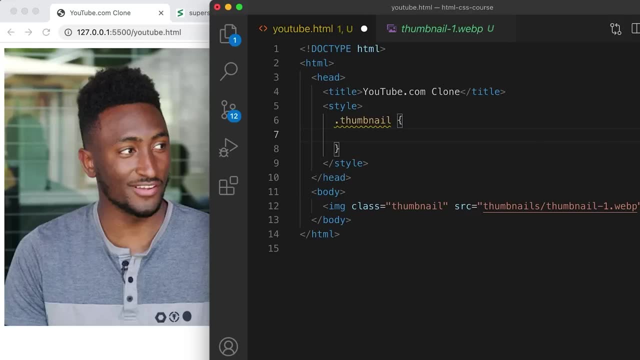 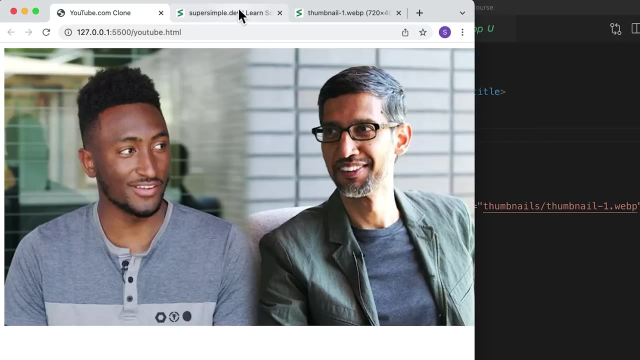 because there is no text inside this element. It's an image. So even though this works, it doesn't really change anything. Now, a property that does make sense for an image is width, So this will set the width of this image. Let's make it smaller. 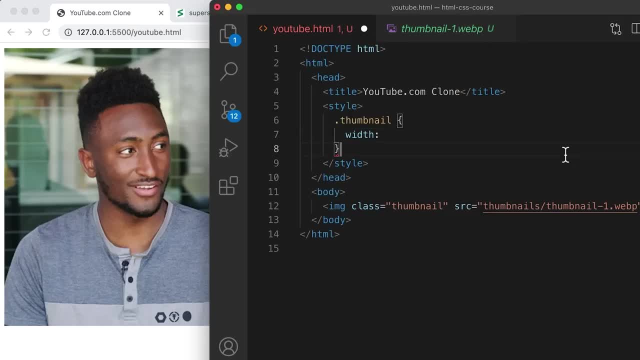 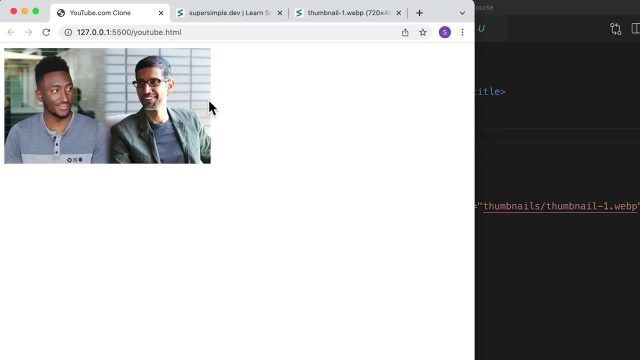 to match what we have here. So let's make the width something like 300 pixels. Now we save it, and now the width of this image is 300 pixels. So one thing you might notice is that when we set the width of an image, 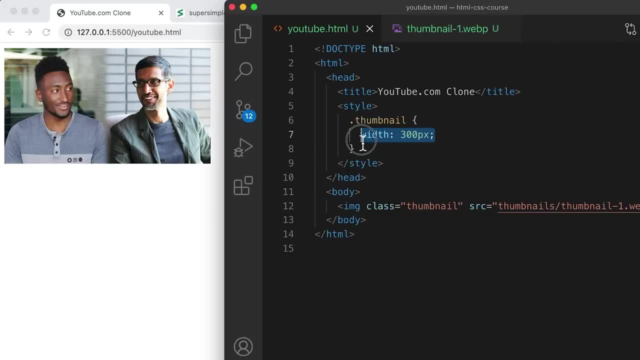 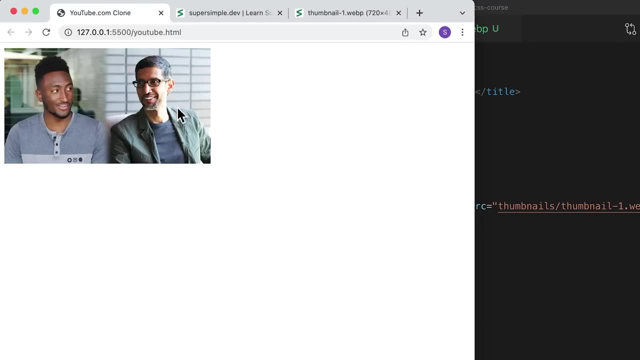 the height also changes. So before we had this notice that the image was a lot taller. But as soon as we set the width, the height also adjusts. So that's one behavior of images that we should know When we set the width. 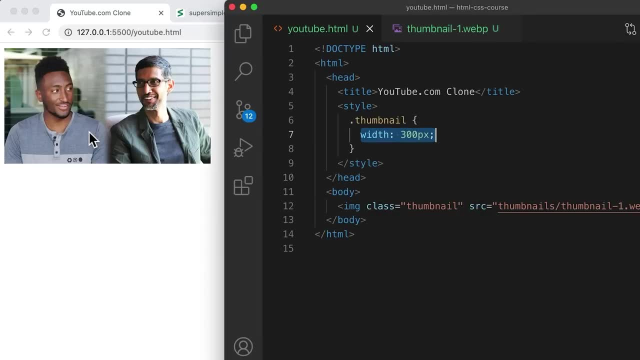 the height will also adjust so that the image has the same dimensions. What I mean by same dimensions is that it keeps the same shape. So, for example, if I set the height as well, this is going to cause the image to lose its shape or lose its dimensions. 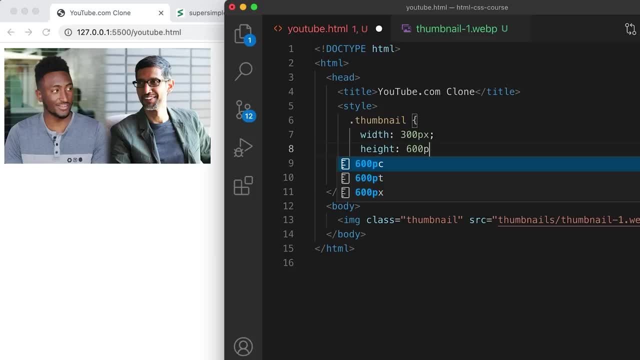 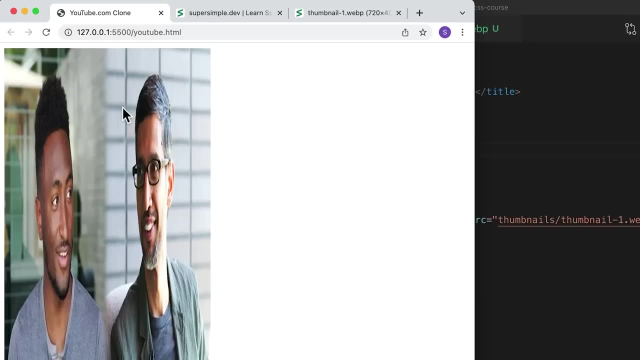 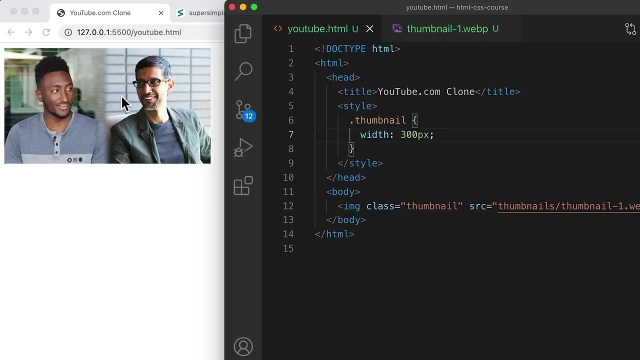 Let's set the height to something like 600 pixels, Save it, And now you'll see that the image is 600 pixels tall, but it's lost its shape and now it's become stretched. So that behavior of an image sort of keeps us safe, So it keeps the image looking. 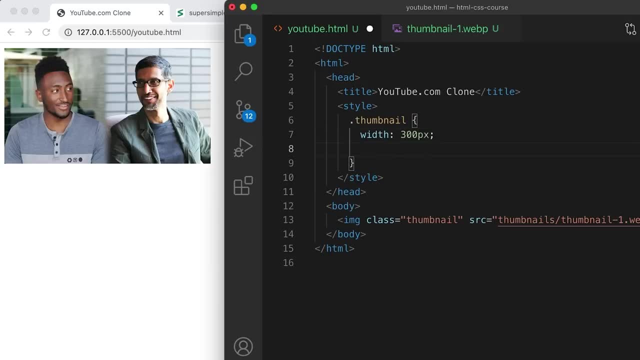 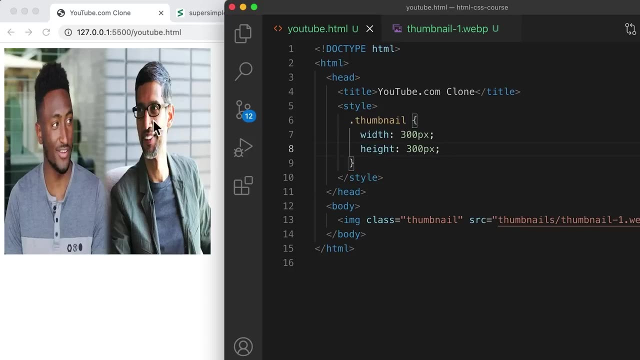 nice. Now, if we really wanted an image that was exactly 300 pixels by 300 pixels, what can we do? So this image, as you can see, is getting stretched out. So, in addition to all the CSS properties that we've learned so far, 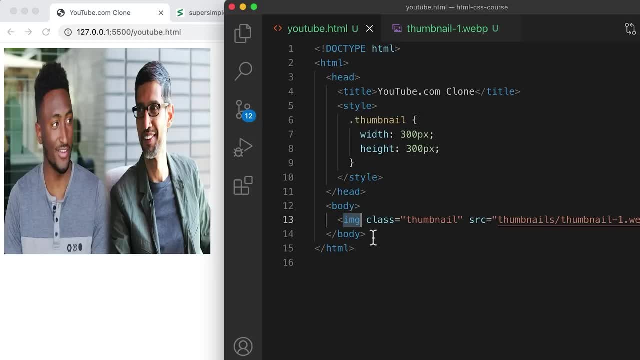 the image element has its own properties that are specific to an image, So one of these is called object fit. So this determines what happens if this size doesn't match the image's dimensions or the image's shape. So, for example, I can set a value. 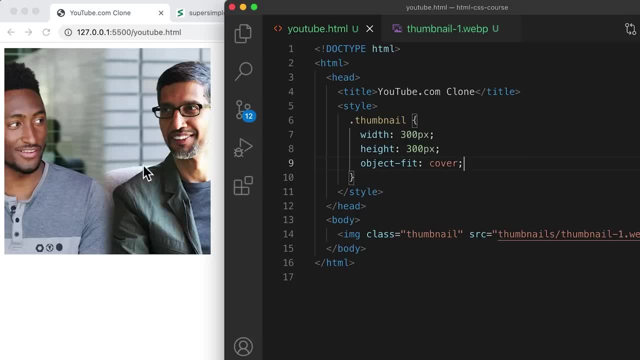 of cover. So this tells the image to cover this 300 by 300 area, but it's also going to keep its shape, So this area might not be big enough to show the whole image, which may or may not be okay, depending on what we want to do. 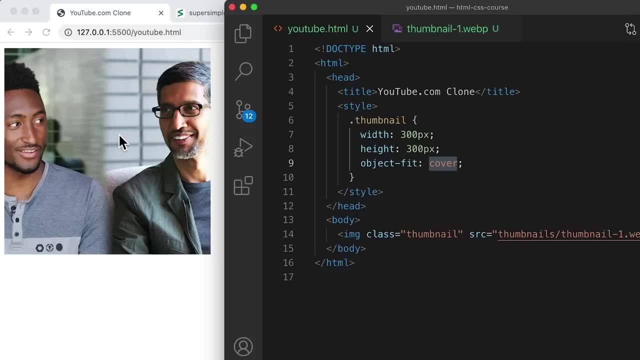 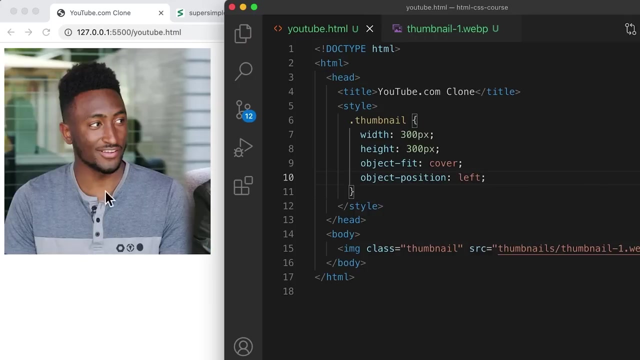 Now we can adjust which part of the image that we see using another property called object dash position. So currently we're looking at the center of the image. We can set the object position to left to view the left side of the image, or we can also set it. 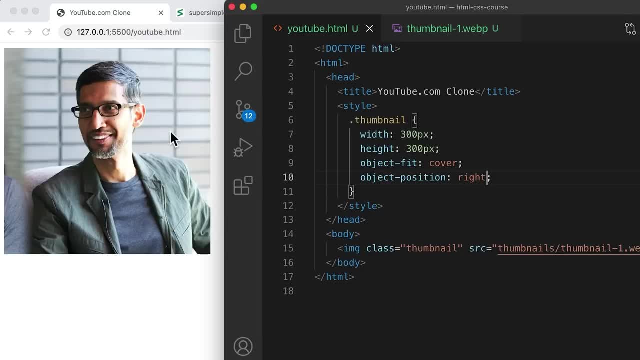 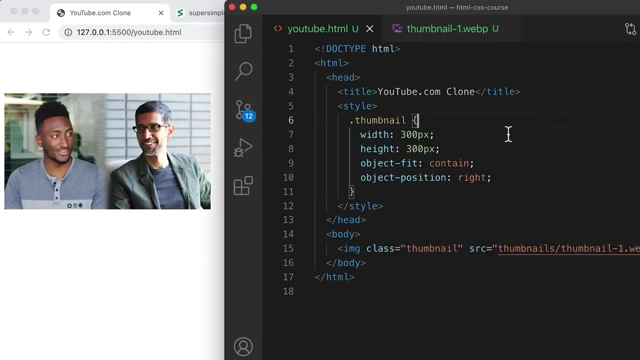 to the right to view the right side of the image in the case that the image doesn't fit in our area. Another value we can give to object fit is contain. So if we save this, the entire image is going to shrink until it is contained in this 300 by. 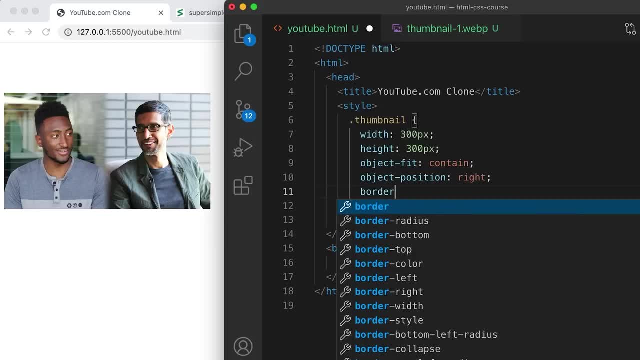 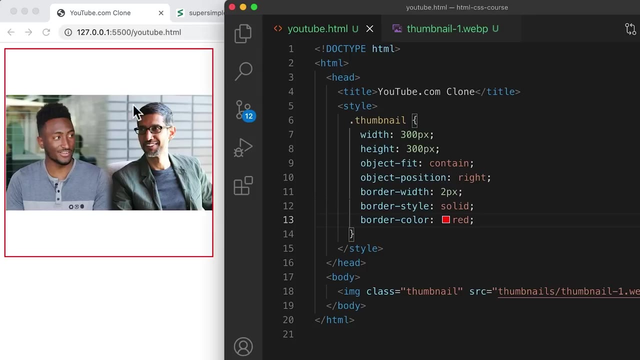 300 area. So I'm going to set a border so that we can see what this is doing. I'm going to set a border of 2 pixels. border width of 2 pixels. border style: solid. border color of red. So here the border shows us our 300 by. 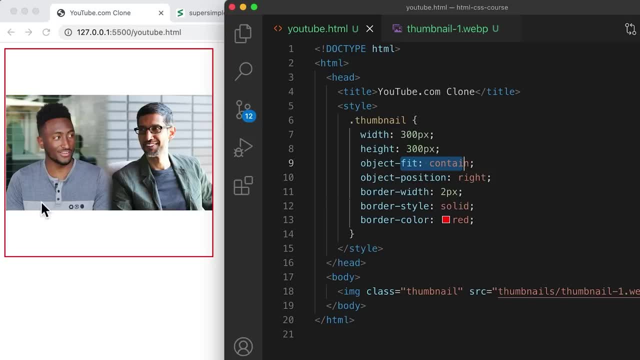 300 area and contain makes the image shrink until it is contained in the area, But that means that it might not be able to cover the entire area if it's not the right shape. So in this case the object position can move the image to the top. 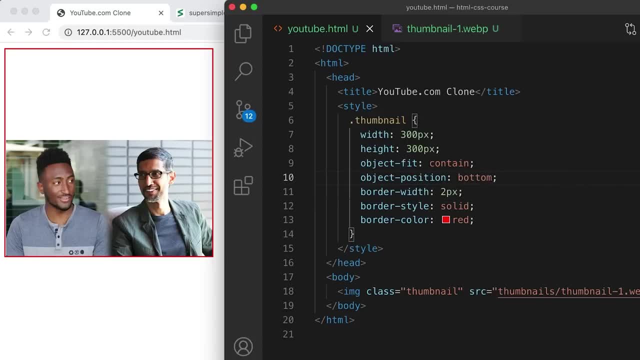 or to the bottom. So that's basically how images work. As you can see, a lot of the CSS properties that we learned before, like width and height and border, can be applied to the image element, and the image element also has some of its own properties. 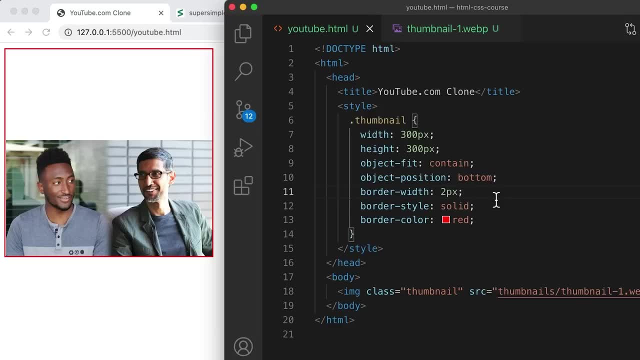 that determine how the image is displayed. So for now, let's create something that's kind of like our final website. So I'm going to set the image width to 300 and I'm not going to set a height, so that the image doesn't stretch and we 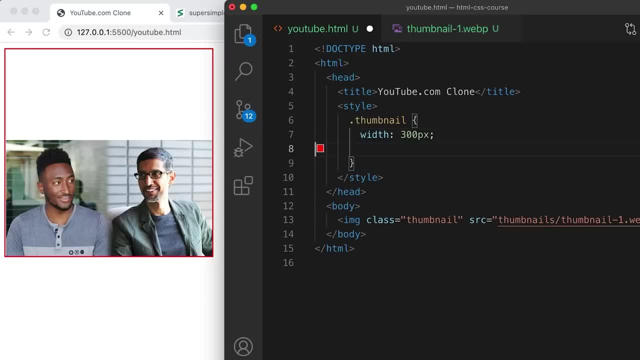 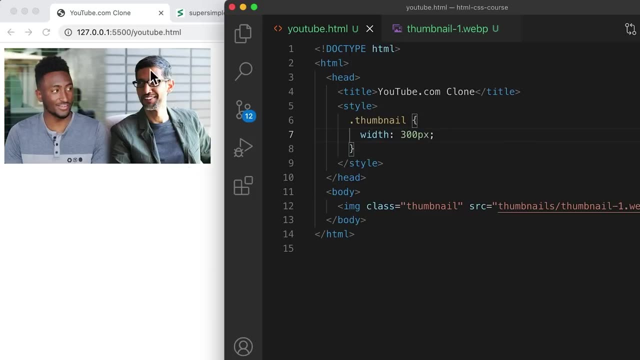 don't have to do all this stuff, And I can actually just remove all of this, So the only thing I'm doing is telling the image to shrink down to a width of 300 and to shrink the height as well, so that the image keeps its shape. 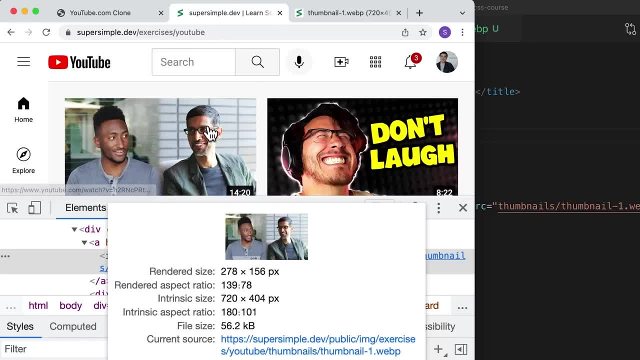 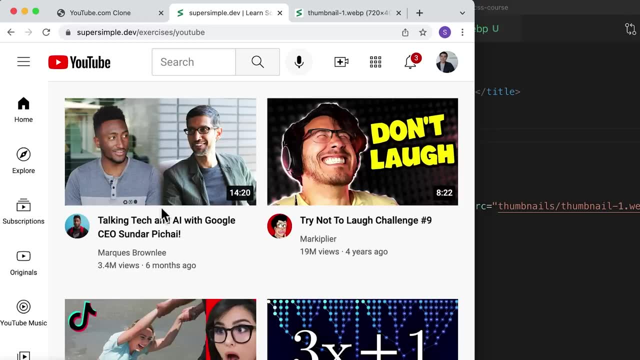 So we're going to stick with this for now- and this is going to correspond to this part of our final project- And we're going to start learning how to build out the entire video preview. The next element we're going to learn in this lesson is how to create. 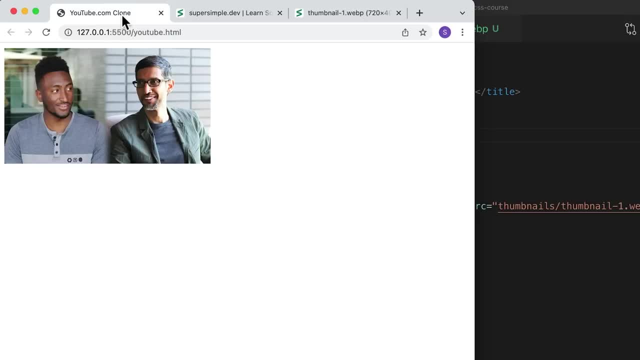 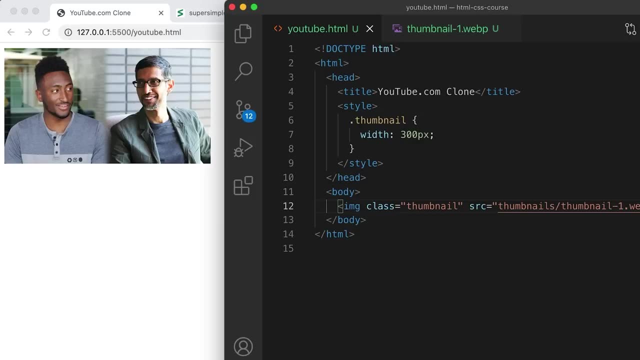 search boxes like the one you see up here. So let's go back into our website and we'll learn the code for creating a search box. The HTML for creating a text box is less than input, greater than So. the input element is a void element. 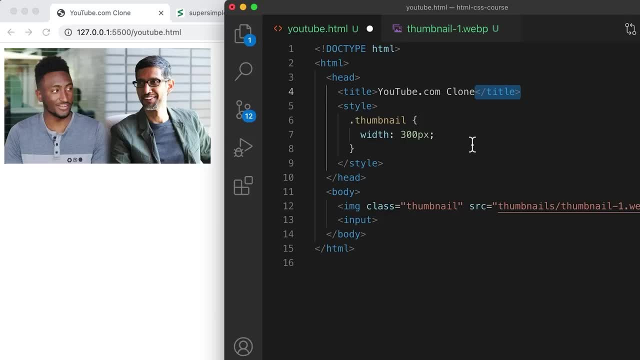 just like the image element, It doesn't require a closing tag. So the input element has several attributes that we can give it. One of them is called the type. So we set the type equals text. It's going to give us a text box. 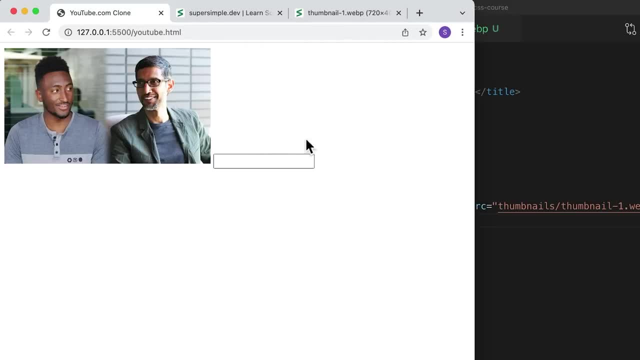 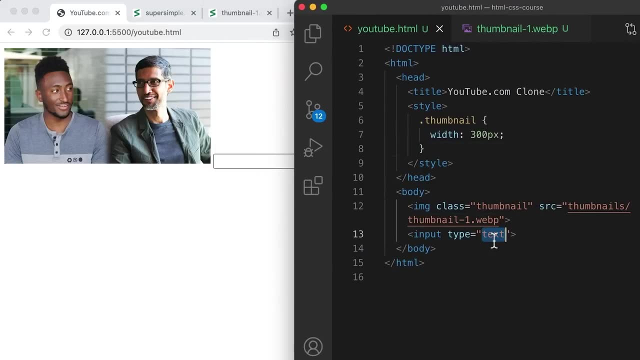 I'm going to save this and now in our HTML you can see we have a text box. Another type that we can give to this input is called checkbox. So if I save this, now we have a checkbox. So for our purposes we're going to set the type to: 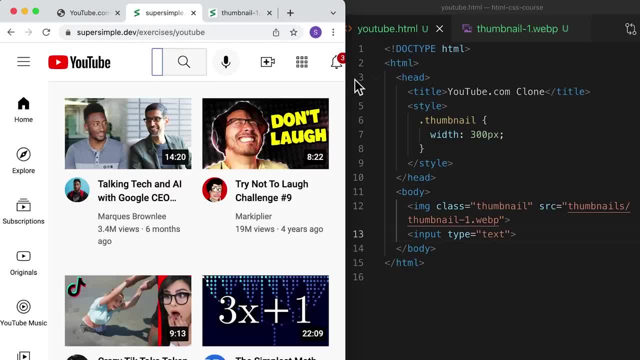 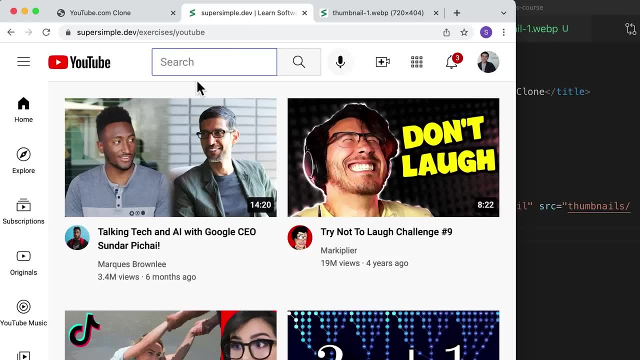 a text box because we want to create the YouTube search box up here. So you'll also notice that this text box has the word search in it, And when I start typing, that search word is gone. So this is sort of like a label for the user. 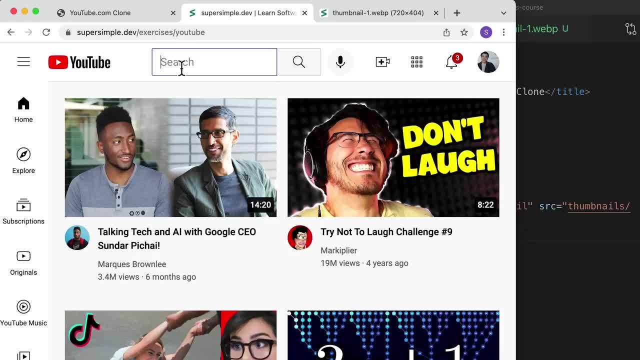 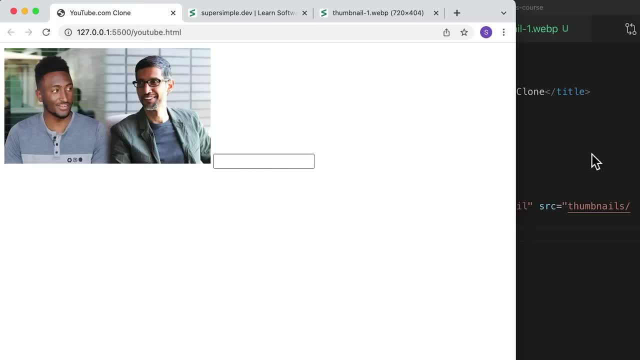 telling them what to put into this text box, And this is known as a placeholder. So if we go back to our website, we're going to add a placeholder to our new text box. To do that, we're just going to give the attribute placeholder. 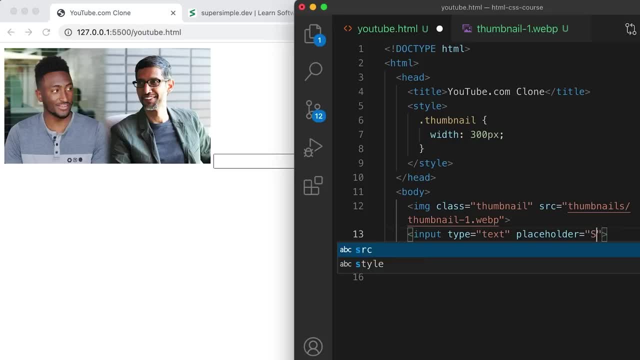 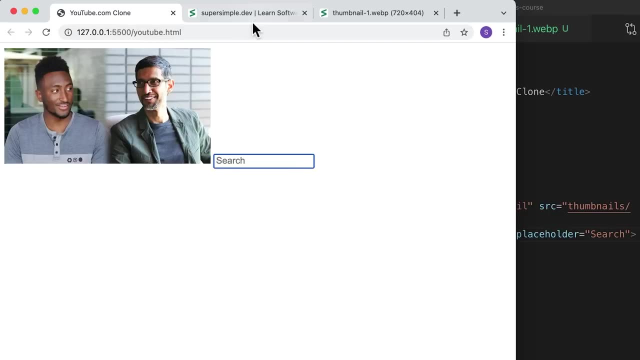 And let's set the placeholder as search. Save it. Now we have a placeholder that disappears when we start typing, So that's how we create what we see on YouTube. So for the text box, all of the CSS properties that we learned so far. 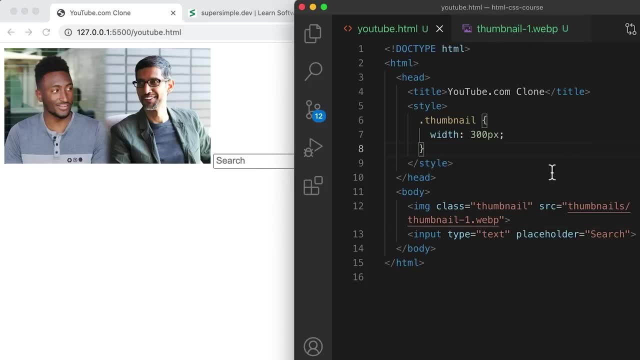 can be used on the text box. So let's look at some examples. Let's add a class attribute first, like always, So that we can target it. Let's call it search-bar, And then, inside our CSS, we're going to target. 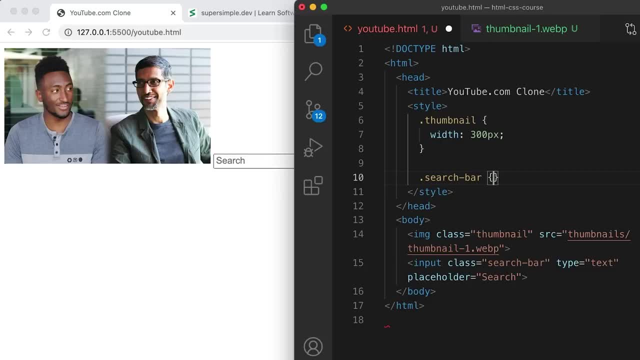 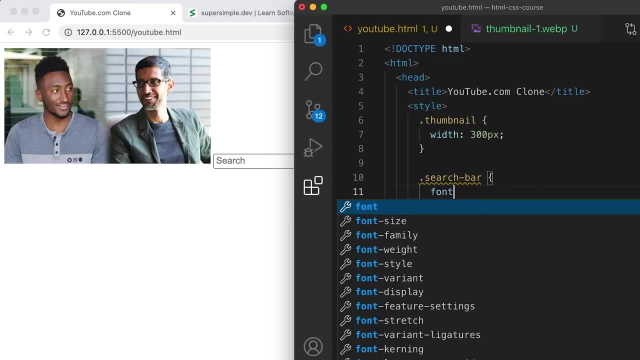 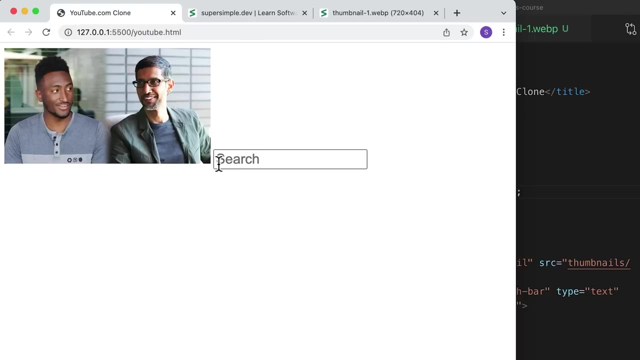 dot search bar class And then inside we can set our usual CSS properties. So, for example, in this case, we can set a font-size, And let's set it to 20 pixels, Save it and reload, And now you can see that the 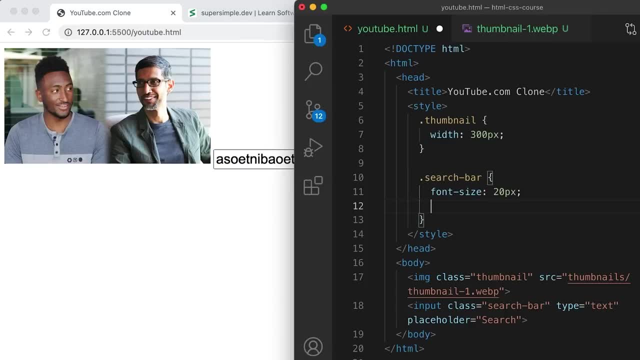 font size has changed. Another thing we can change is margin or the spacing. So let's add some margin to the left of 12 pixels, Save it, And now we have some spacing on the left. So basically everything that we've learned so far about CSS properties. 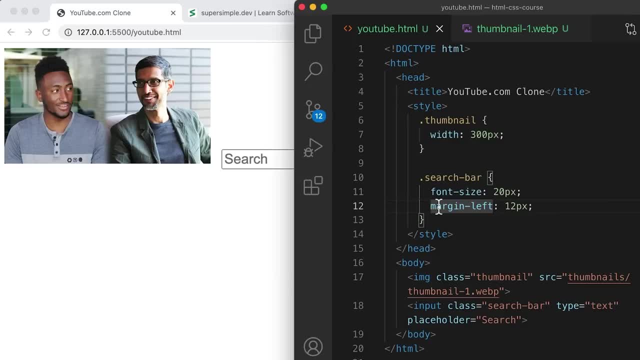 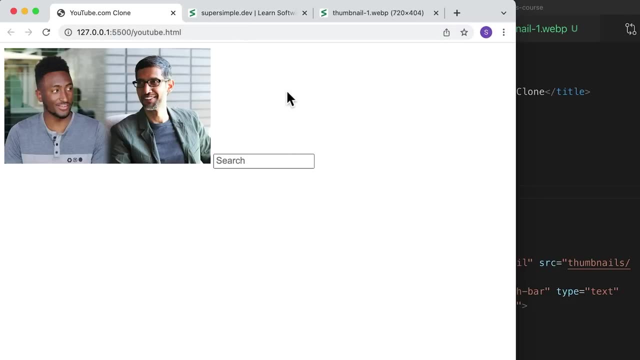 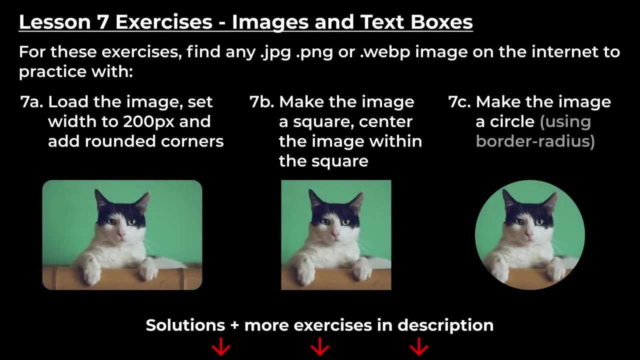 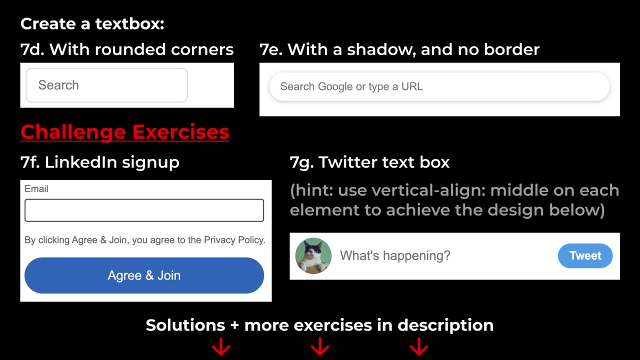 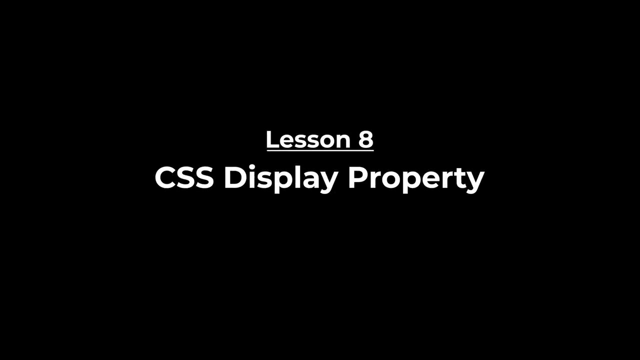 we can use on the search box. For now, let's remove these example styles and we're going to style this search box to look like our final project later in this course. In this lesson, we're going to learn one of the most important CSS properties. 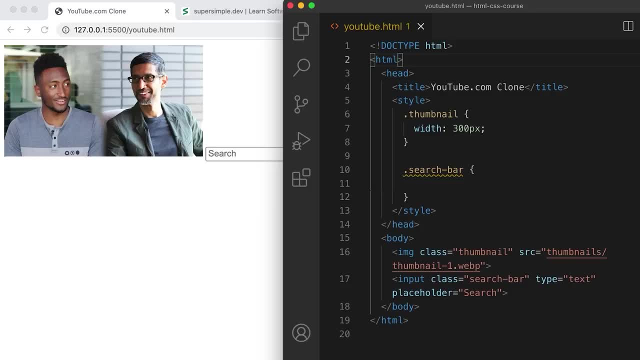 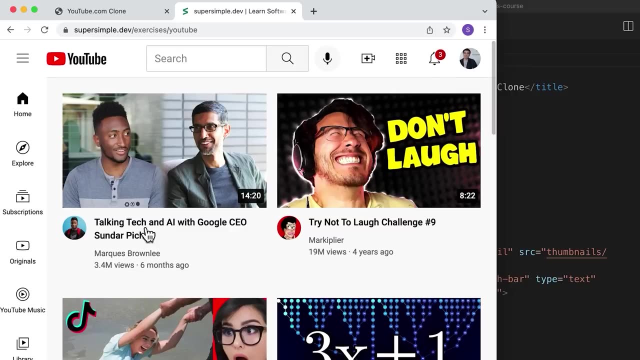 called the display property, And we're going to use this to start building out our final project. We're going to start off by taking a look at our final project And we're going to start building out the text here. So we're going to create paragraphs. 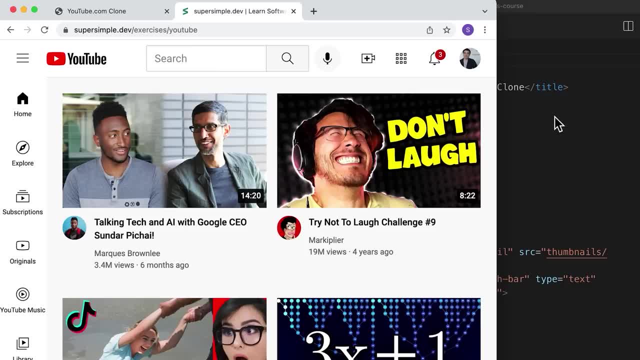 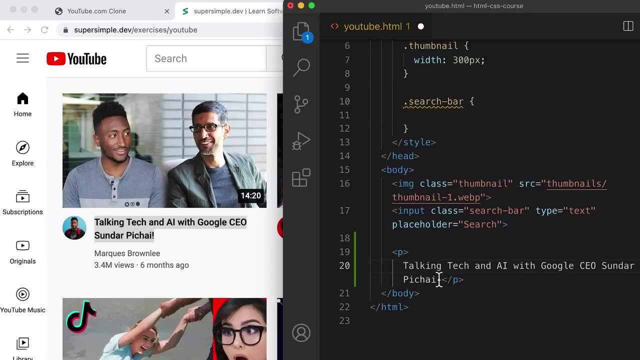 for these texts. Let's go into our code And we're going to create three paragraphs. So here's one of them And we can copy the text: Copy and paste. So here's another paragraph And we're going to copy this. 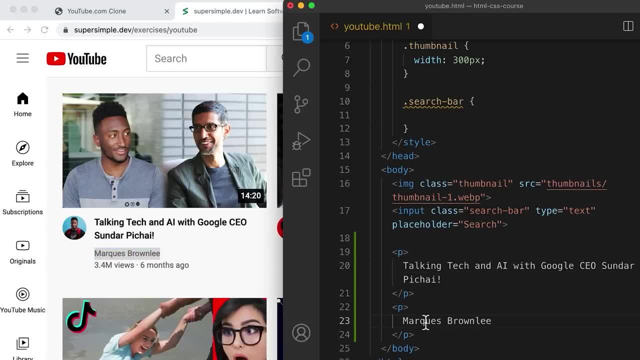 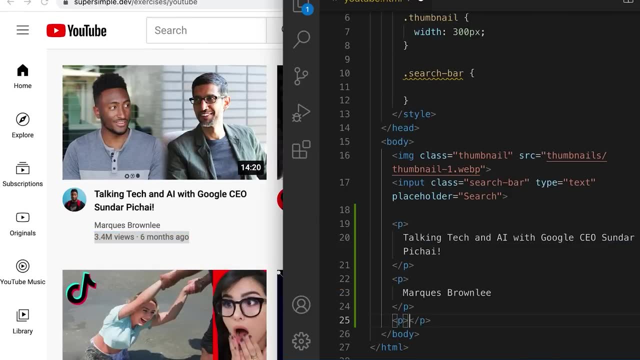 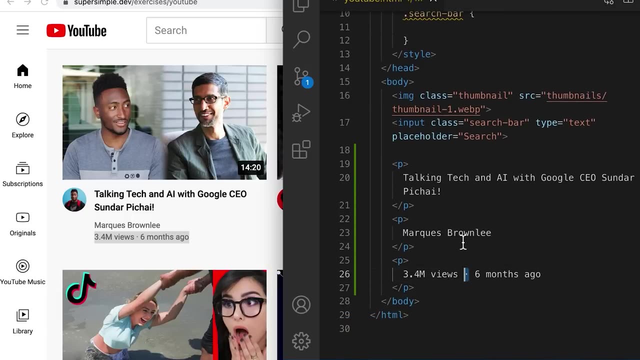 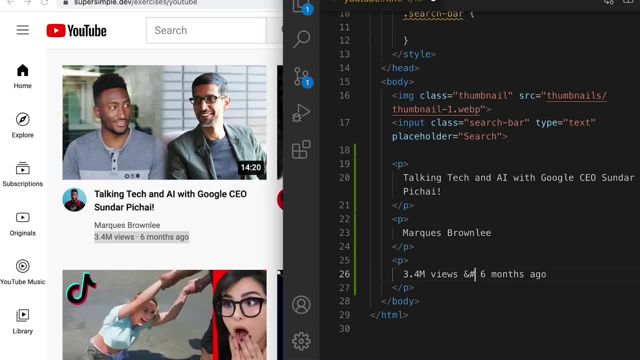 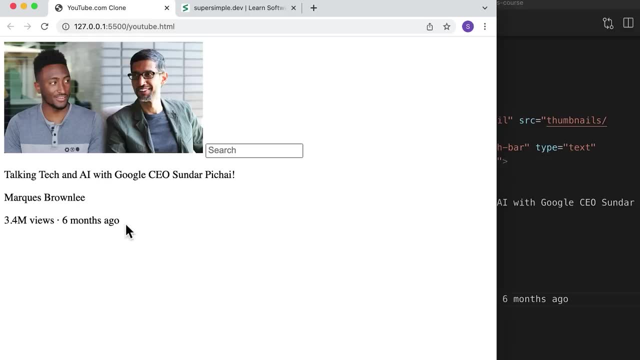 So, to save us some time, I'm just going to type it out here Now. I'm going to save this and go back to my webpage, And now we have the text that we're going to use. But you might notice something weird. 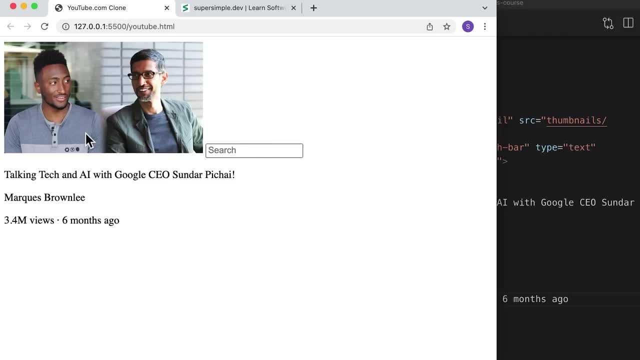 How come this text box is beside our image? If we look at our paragraphs, they are on top of each other, So one after another on each line. How come text boxes and images appear on the same line? So this is due to the display property. 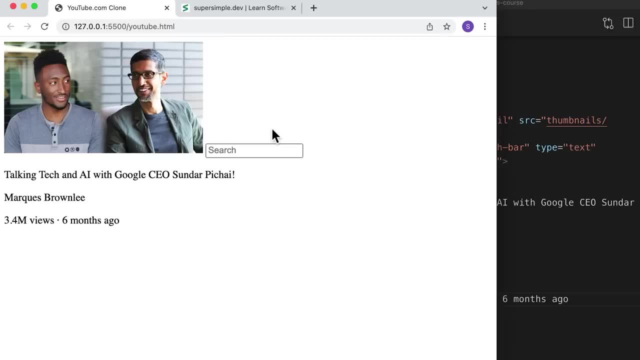 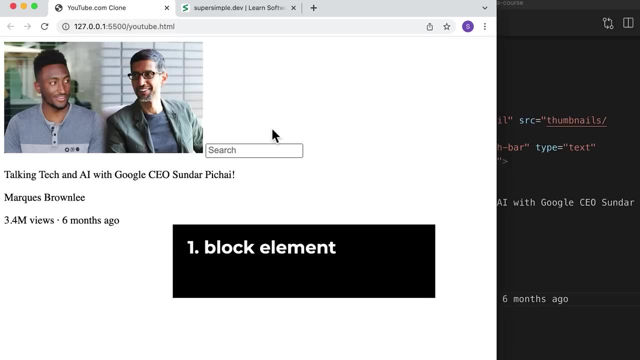 in CSS And we're going to learn what that is right now. In HTML there are three types of elements. The first type of element is called a block element. A block element takes up the entire line, So a paragraph by default is a block element. 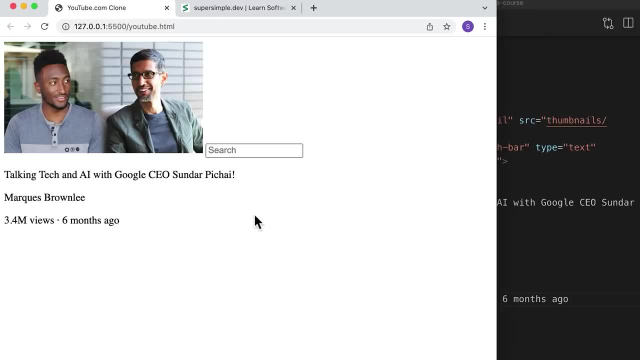 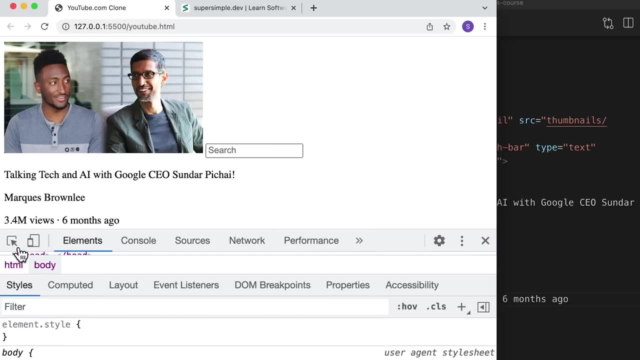 And you can see that in our dev tools by right clicking in the browser and then clicking inspect, And then clicking this icon in the top left Right here And then hovering over our paragraph. So you can see that, even though the text goes to here, 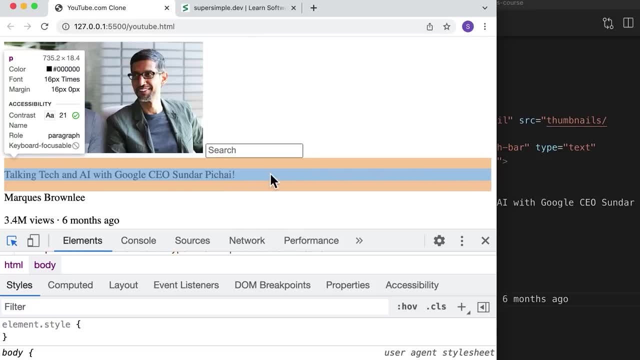 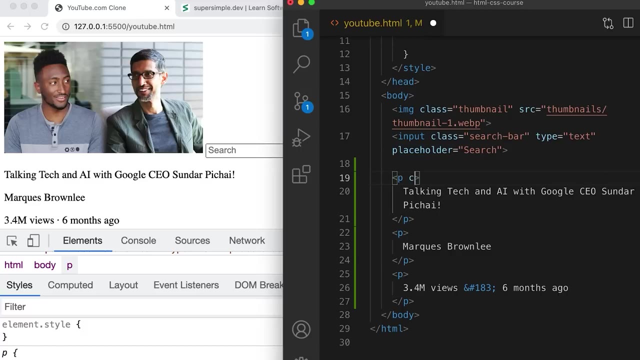 the paragraph extends to the end of the line Because the paragraph by default is a block element. Block elements take up the entire line. So let's go into our code and I'm going to demonstrate another property of block elements. If we set a class, 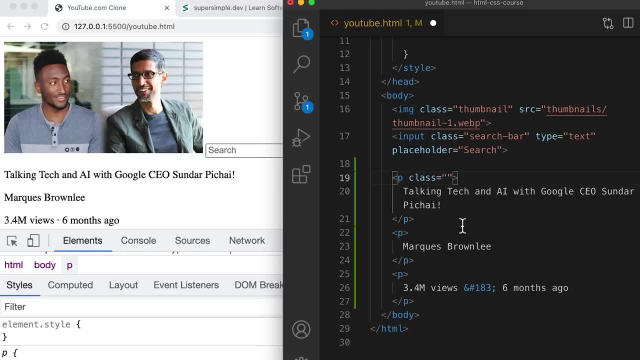 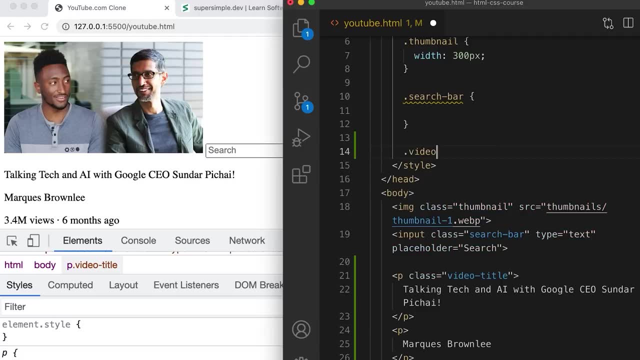 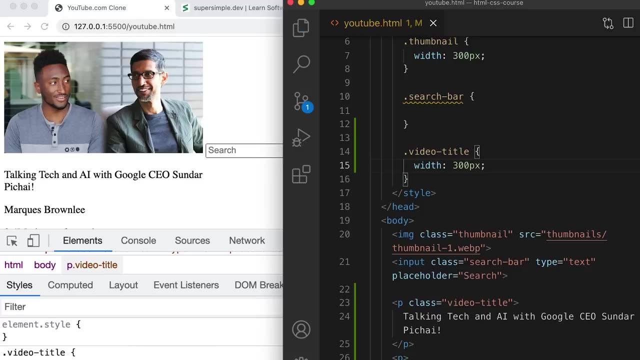 on the paragraph and we style it. So let's set a class of video-title, Let's save it And we're going to style it, And let's give it a width of 300 pixels, Save and refresh, And now this paragraph is only 300 pixels. 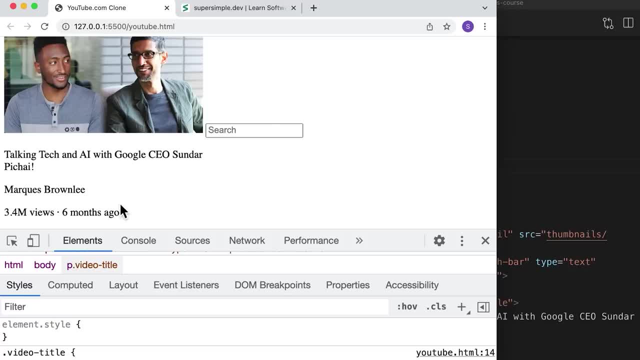 So it's not stretching to the end of the line anymore. So let's verify that using the dev tools by clicking this top left and then hovering over, So you see that the paragraph itself only takes a width of 300, like we set in our CSS. 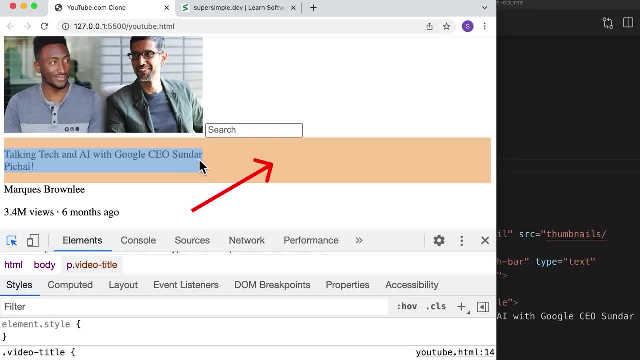 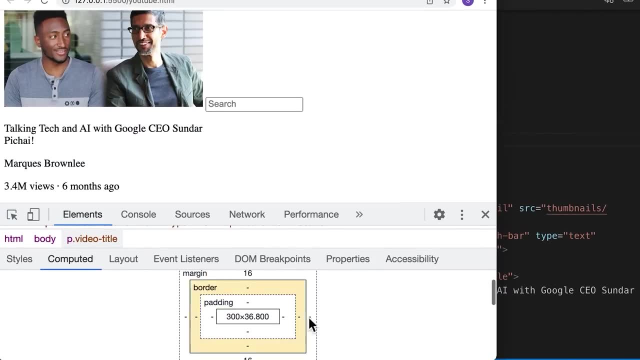 But it still takes up the entire line Denoted by the orange part on the right here. If we click on this paragraph and we go to the computed tab, notice that there is no margin on the right side, But we still have a ton of orange area. 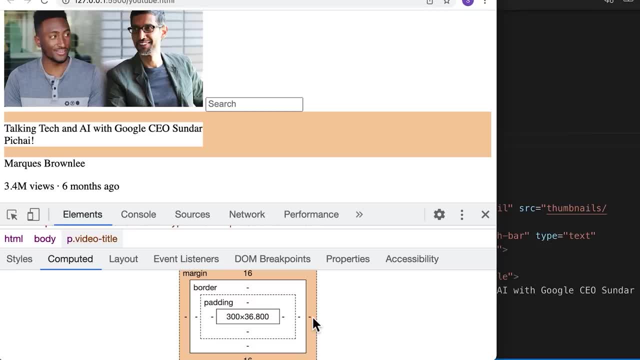 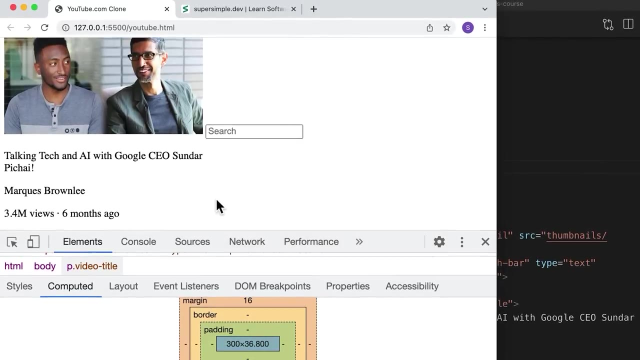 on the right. So it's going to work. Regardless of how much space they actually take up, they take up the entire line. So they're forced to be on their own line, like this paragraph and these two paragraphs. So that's what a block element means. 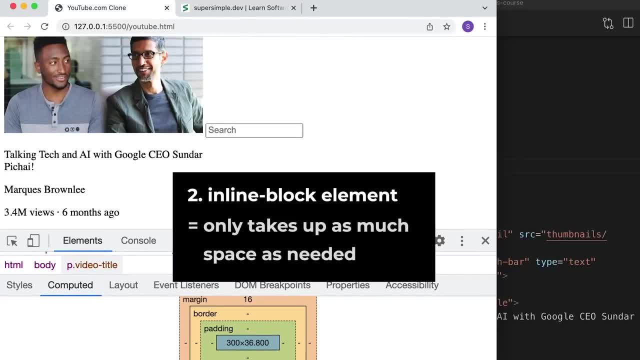 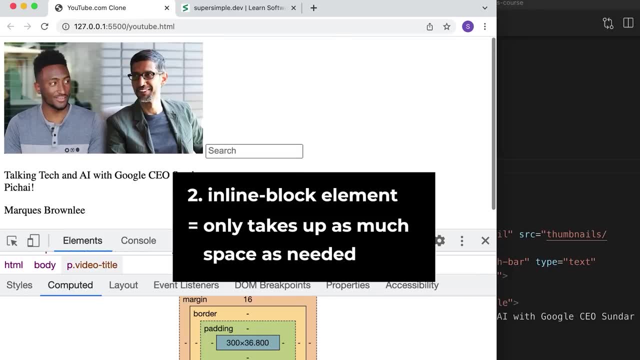 The second type of element is an inline block element. An inline block element only takes up as much space as it needs to and doesn't take up the entire line. An example of an inline block element is the image element or the image element element. 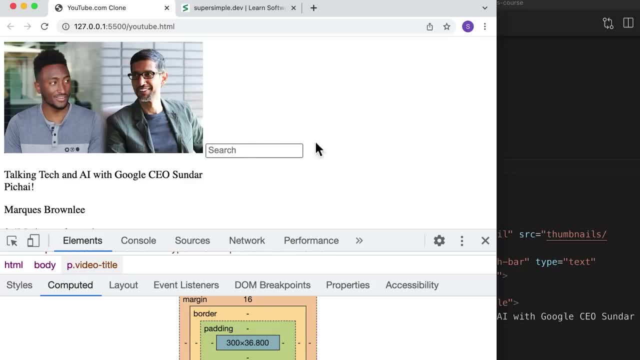 They only take up as much space as they need to and they don't take up the entire line. So another element could appear beside them, like we see here. So that's the inline block element. The third type of basic HTML element is called the inline element. 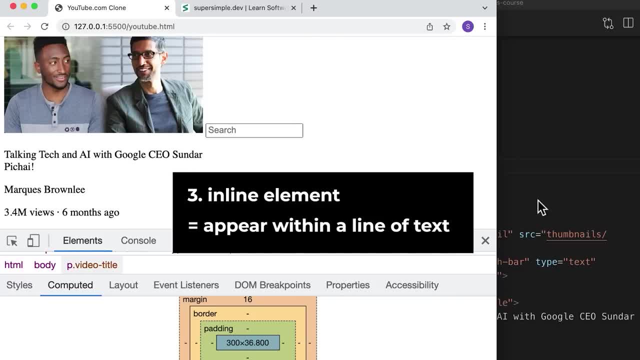 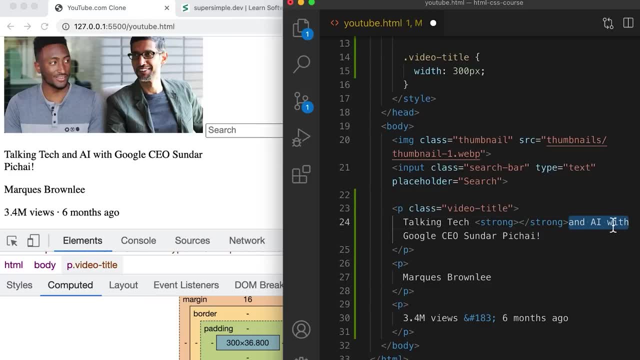 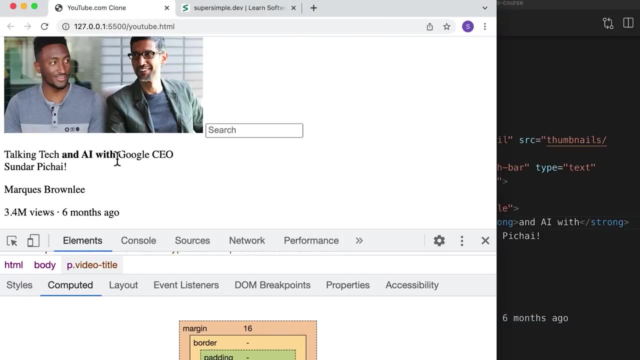 Inline elements are basically just text elements. They appear within a line of text. So, if you remember, we briefly introduced the element strong Like this. So this element makes a part of the text bold and it appears within a line of text. So those are the three. 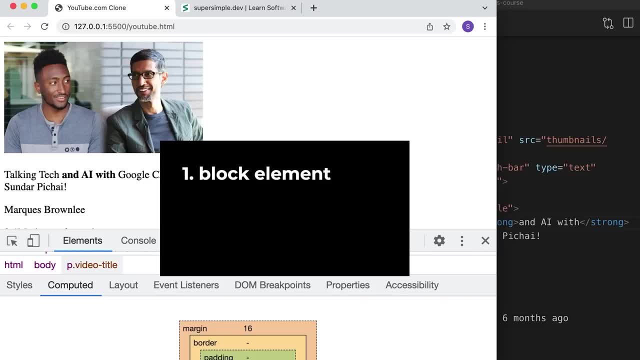 basic types of HTML elements: A block element which takes up the entire line, An inline block element which only takes up as much space as it needs to, And an inline element which appears within a line of text. Now, the most interesting of these three: 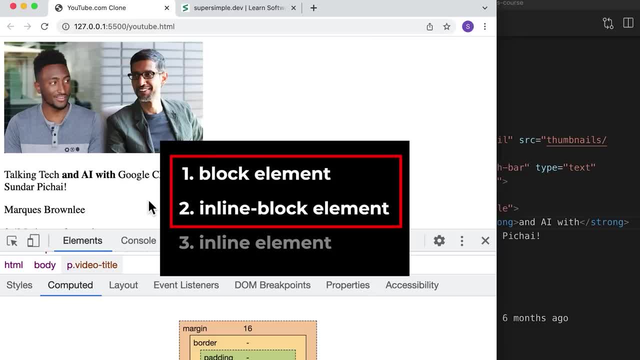 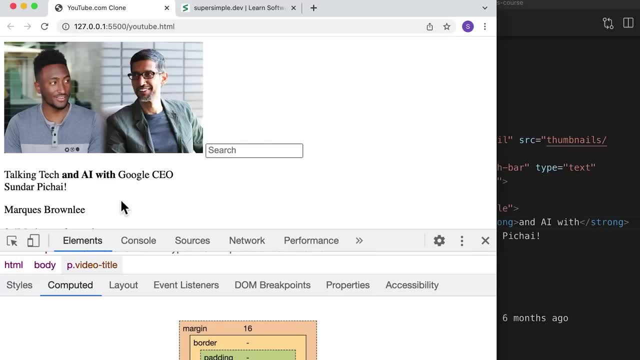 are the block elements and the inline block elements Because they determine how these elements are displayed on the page, Whether beside each other or above and below. In addition, we can use a CSS property called display to easily switch between block and inline block. 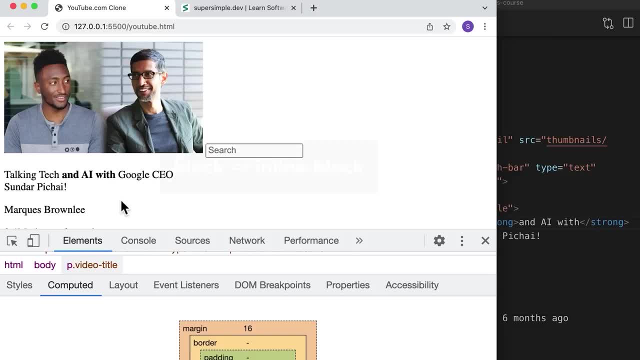 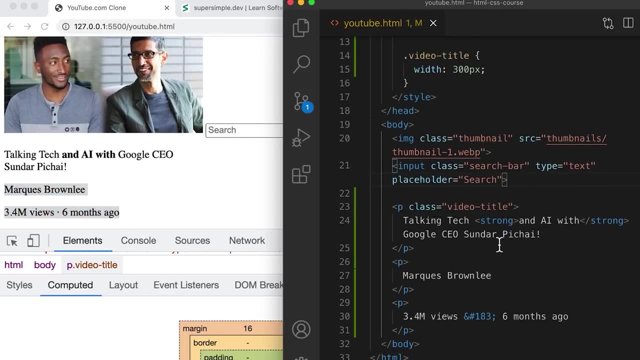 So let's see how that would work. So first let's start by switching from block to inline block. We're going to switch both of these paragraphs to inline block elements. Let's go into our code and we're going to give this a class. 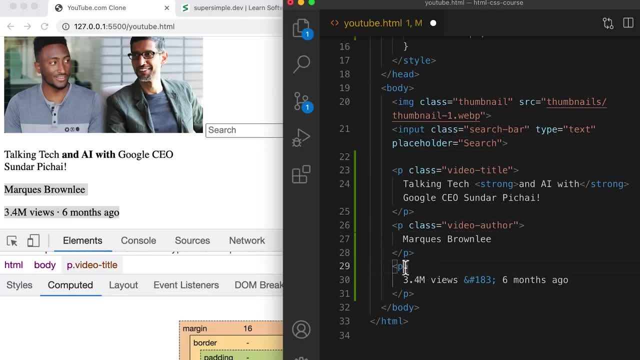 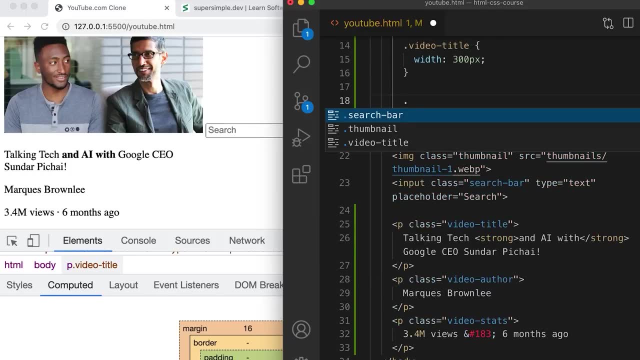 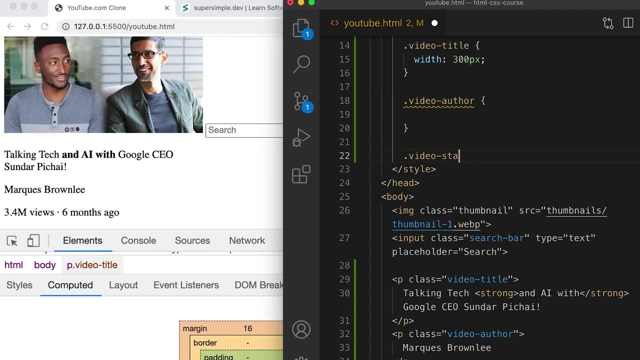 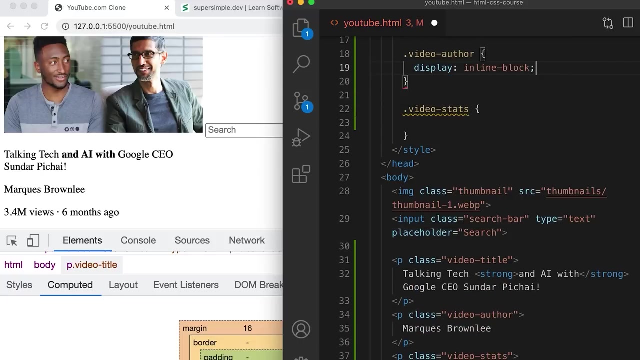 Let's call this video-author and let's call this video-stats, and we're going to style these classes. So we're going to style the video-author as well as the video-stats and we're going to set both of these to display inline-block, and this one as well. 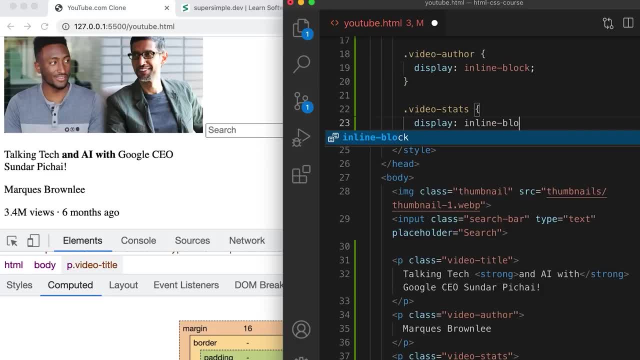 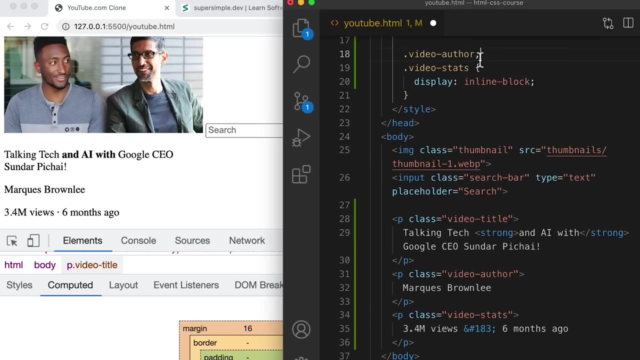 display inline-block. I'm going to introduce a little bit of CSS syntax here. If we have two sets of CSS styles that are the same, we can actually use a different syntax by adding a comma here. So this comma means that we're going to target both. 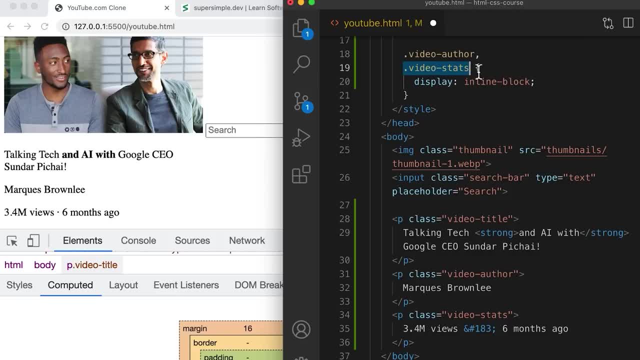 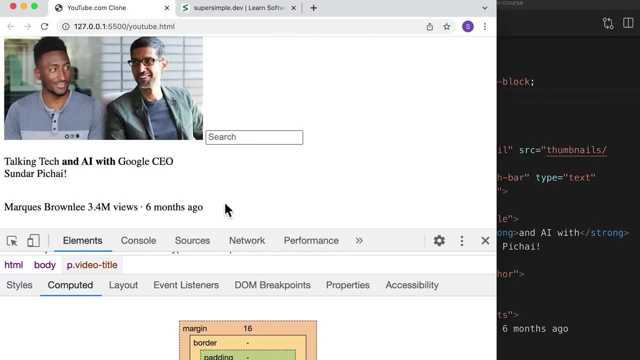 the video-author class and the video-stats class with this set of styles. So this is how we target multiple things in CSS with a comma. So, as you can see, these two elements now appear beside each other. They're both inline block elements and only take up as much space as they need to. 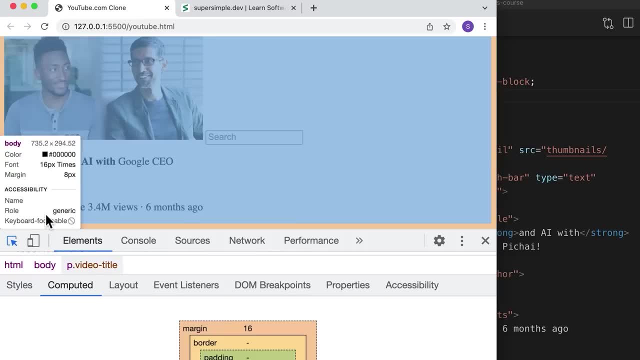 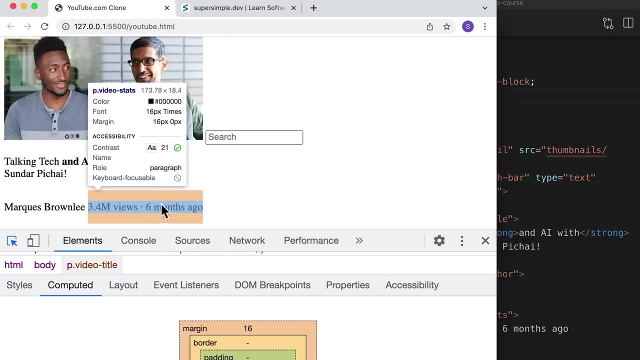 If we click the top left in the DevTools and hover over this, you'll notice that this paragraph is now only taking up as much space as the text, and the same thing for this paragraph. So, as you can see, even though paragraphs by default are, 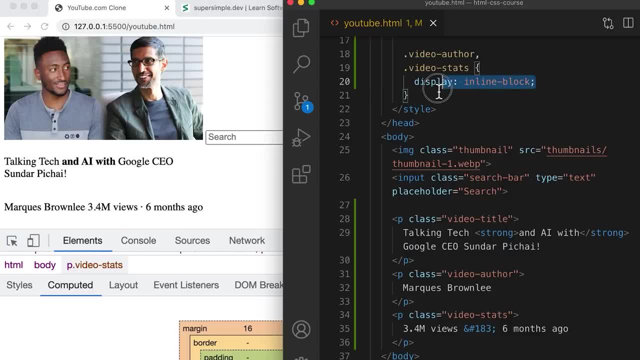 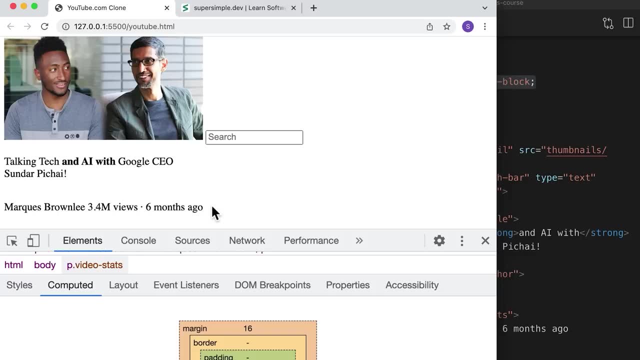 block elements. we can change them very easily to inline-block with the display property so that we can put them beside each other. Next, we're going to try the opposite direction. We're going to go from an inline-block element to a block element. 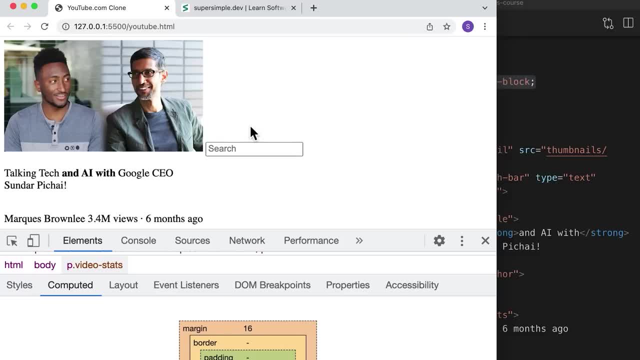 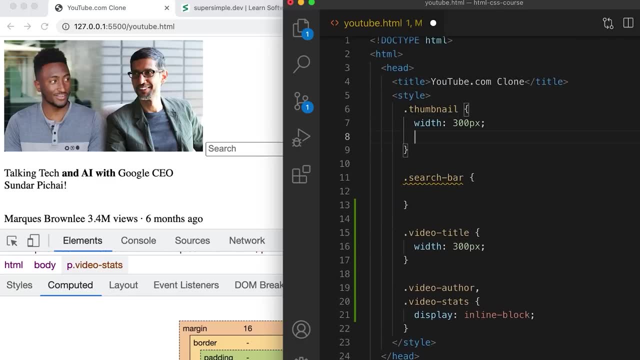 And we're going to put these two on separate lines. So let's go into our code and we're going to style the thumbnail class. So I'm going to scroll up here and I'm going to convert this to display block And now it will turn the image into. 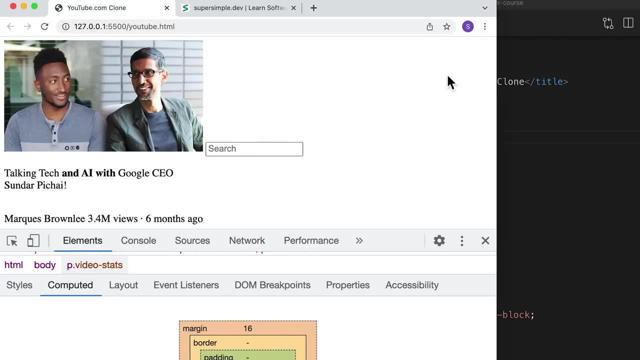 a display block and this will cause the image to take up the entire line, pushing the text box down to the next line. If I save it now, you can see that this image is taking up the entire line. I'm going to verify this by clicking. 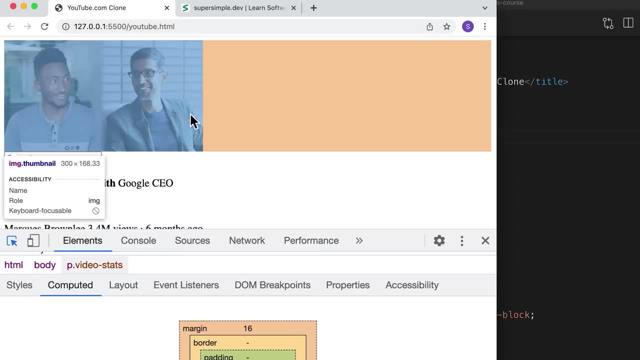 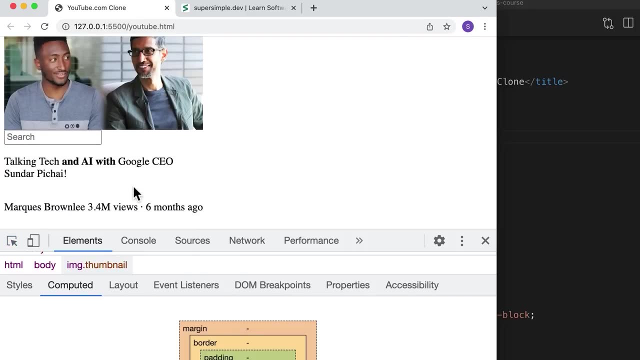 the top left and then hovering over this image. So, using this property, we can control whether an element appears on the same line or on a different line, And that's what we're going to do. to copy this design, The search bar is at the top. 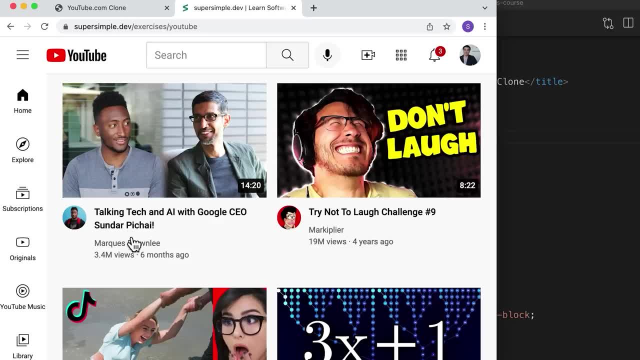 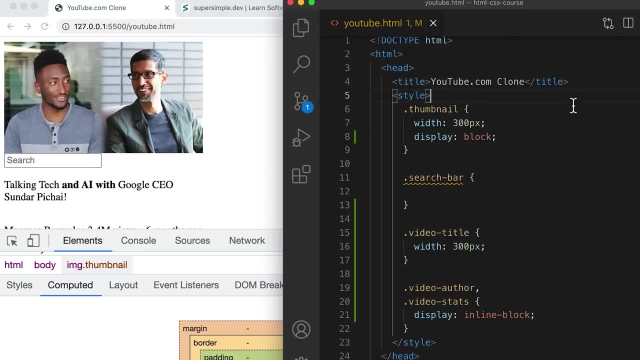 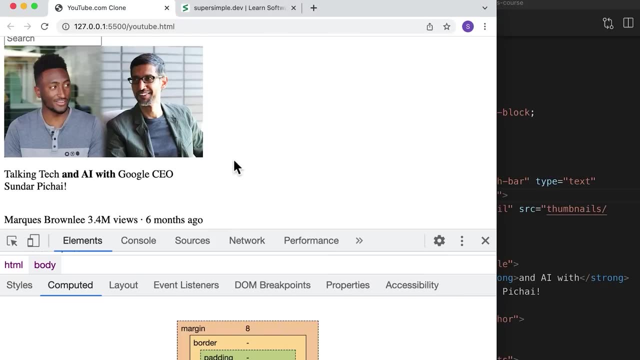 We have an image and then three paragraphs, each on a different line, So we're going to use the display property to achieve this. Let's go into our code and first let's put the search box at the top, Save it And, since our image is already display, 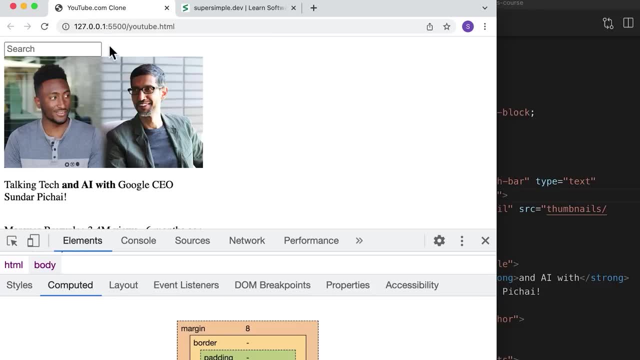 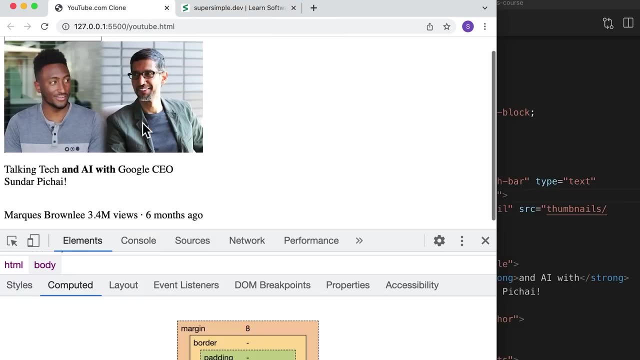 block, it's going to take up the entire line, so it's forced to take up a line below the search box. So I think this is pretty good. As long as the search box is up there, then we're good to go. Next we're going to turn. 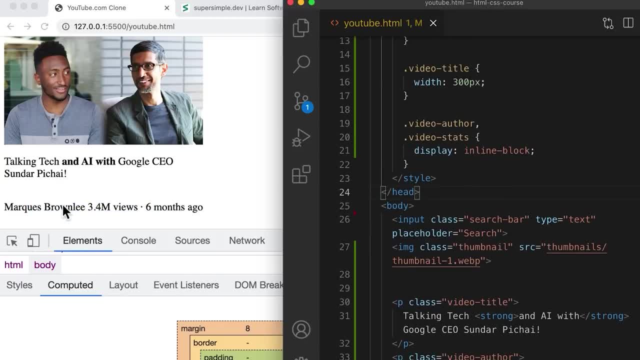 these back into display block because we want these on separate lines, like our design here. So to do that we're going to go into our code and we could change this to display block. But remember that paragraphs by default are display block, So we can just get rid of. 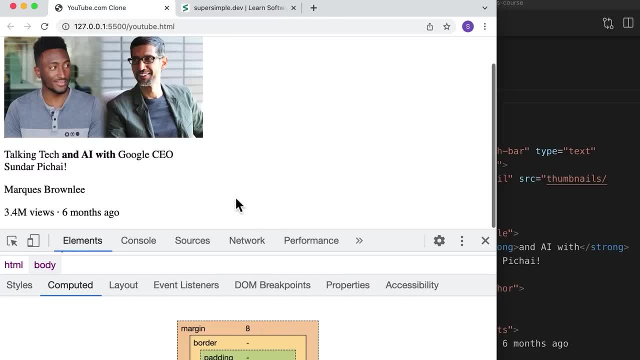 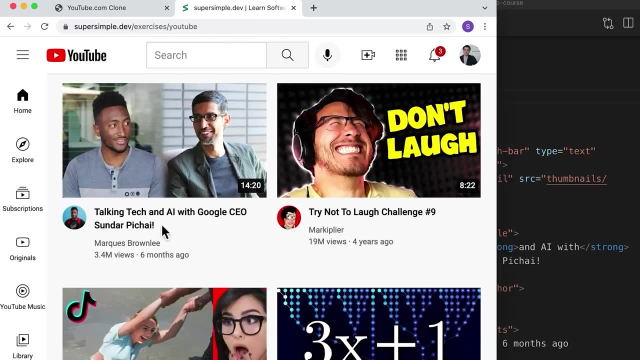 this code, Save it, And now our elements are appearing at least in the same structure as the design, From top to bottom, and each element is taking up its own line. So that is the display property. It allows us to control how an element 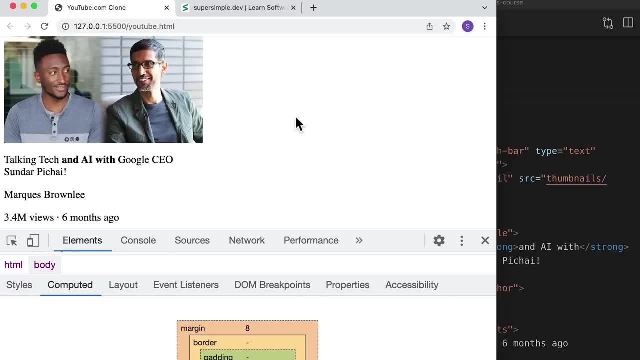 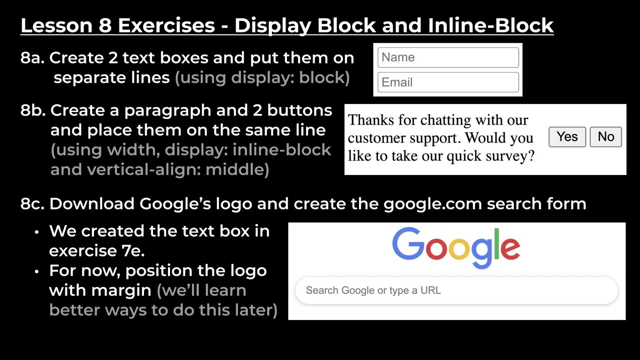 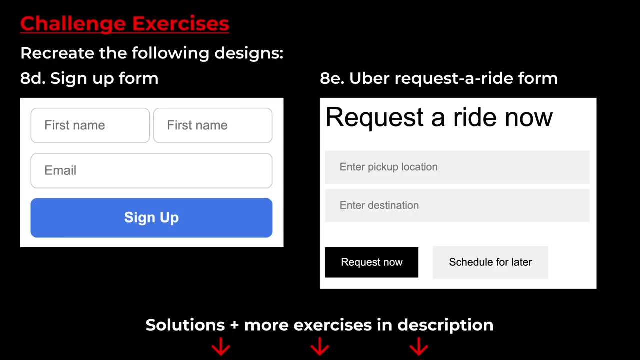 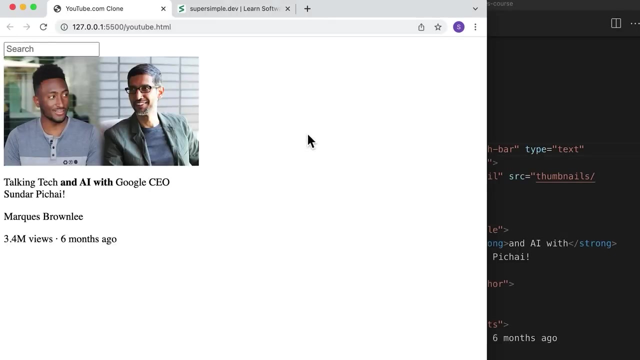 is displayed, Whether they're a block element and take up the whole line, or they're an inline block element and only take up as much space as they need to. In this lesson, we're going to learn about the most important HTML element, called the div element. 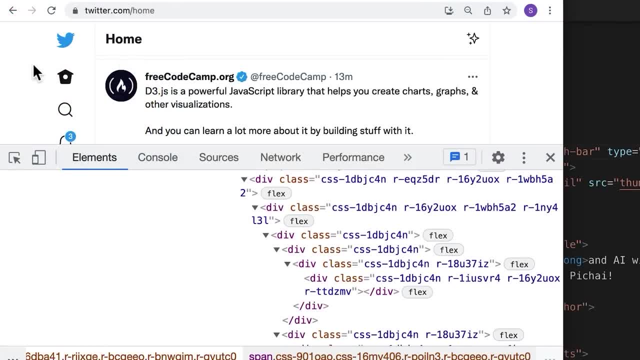 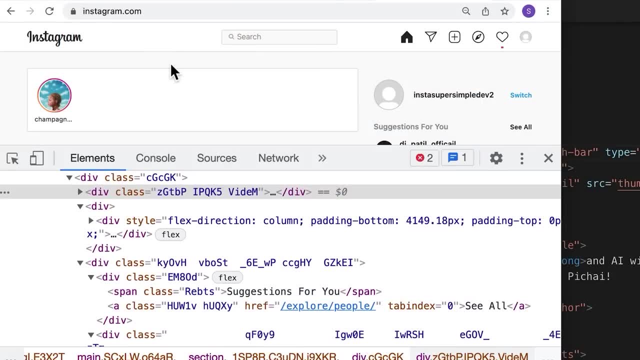 For example, here's Twittercom. If you look at the HTML that Twitter uses, you can see that they're using lots and lots of divs. Here's another example: Instagram. If we look at Instagram's HTML, we can also see that they're using lots. 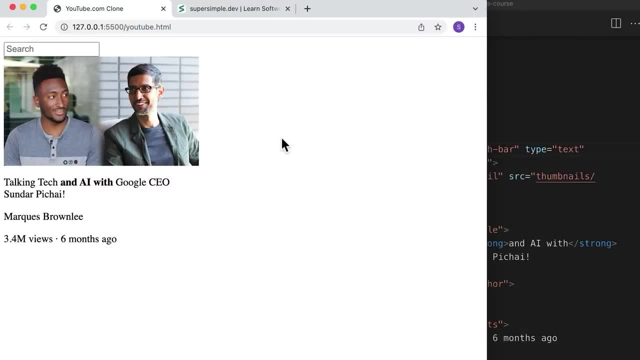 and lots of divs. So what exactly is a div And why is it used so much? So the div element stands for division, But an easy way to understand this is that the div is just a box. We're going to go into our code and look at an. 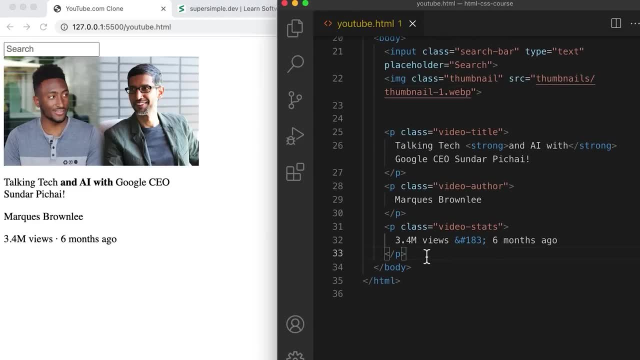 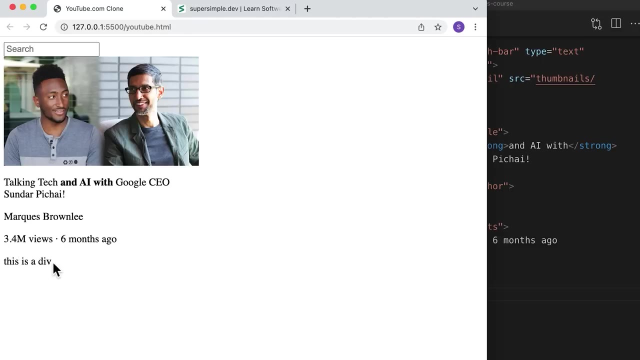 example. So, below our paragraphs, let's create a div element And inside we're going to have some text. This is a div, Save it. And now we have our first div element on the page. To show you that the div is just a box we're going to right click. 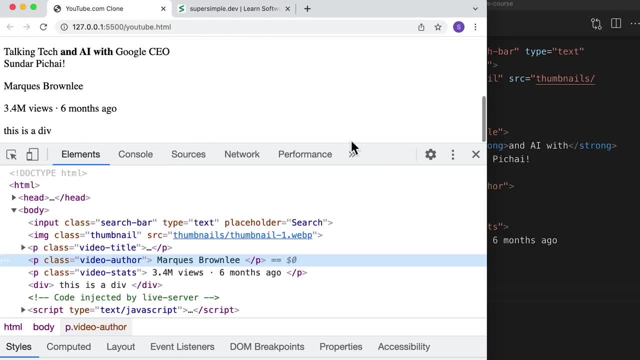 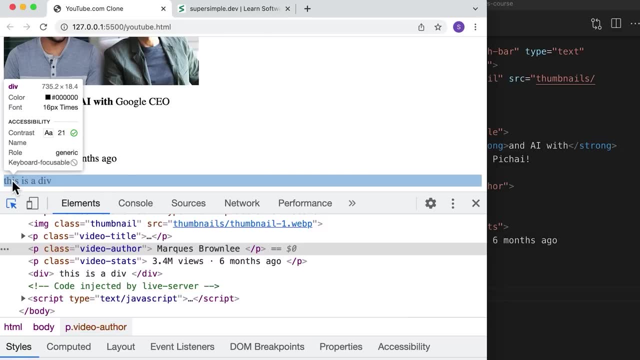 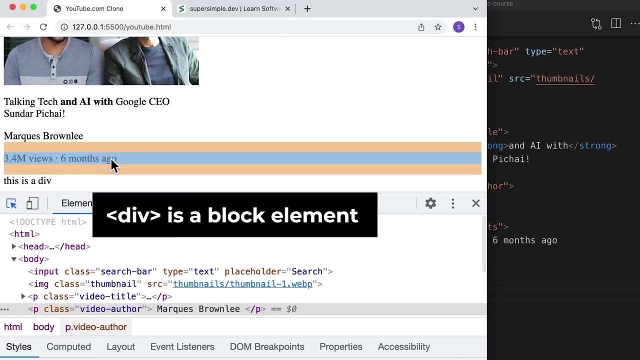 and inspect, And then we're going to click this top left icon and hover over the div. So, as you can see, we created a box around our text. You'll notice that this box stretches to the end and that's because the div like the paragraph. 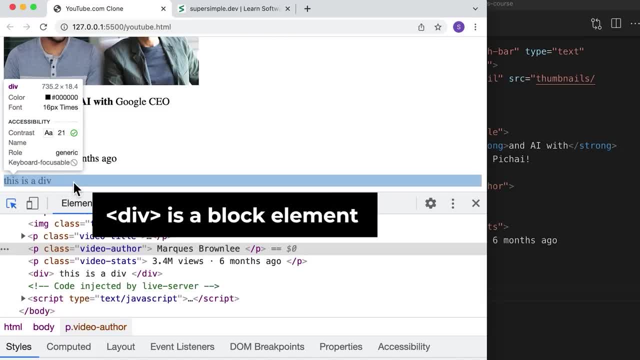 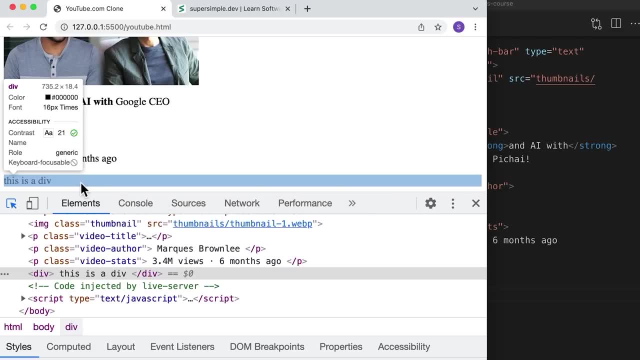 by default is a block element, So it takes up the entire line, But, like we learned in the previous lesson, we can easily change this to an inline block using the display property. So let's go ahead and do that, and it'll be more clear that this. 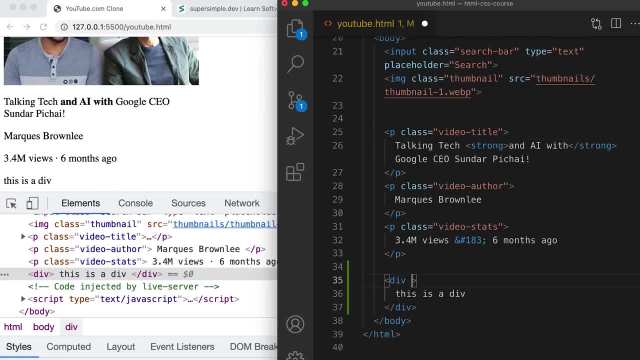 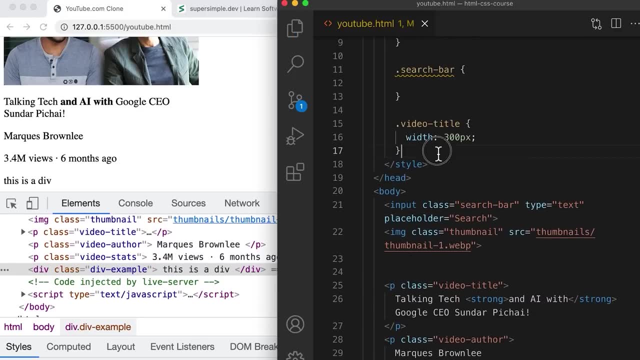 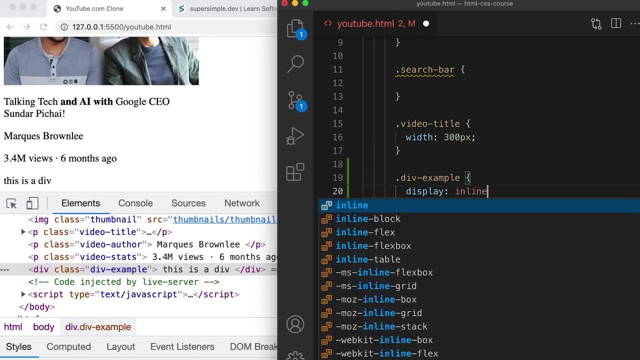 is really a box. So we're going to set a class here, We're going to call this div-example, And now we're going to style it and change the display to inline block So that it doesn't take up the entire line anymore. Save it. 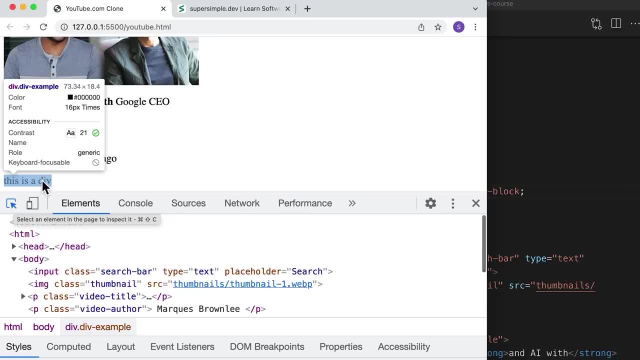 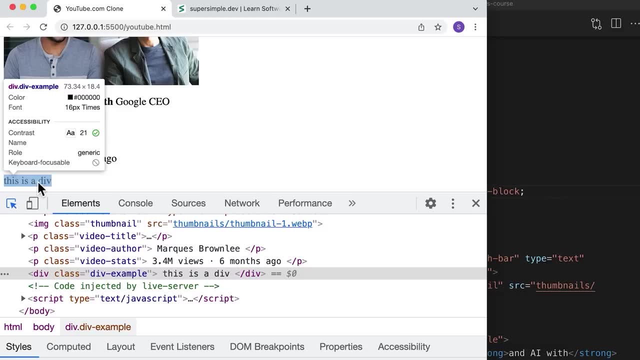 And now, if we go to our webpage, click this icon and hover over, you can clearly see that the div just creates a box around our content. In this case, our content is some text. So that's basically what a div is. Now the second question is why. 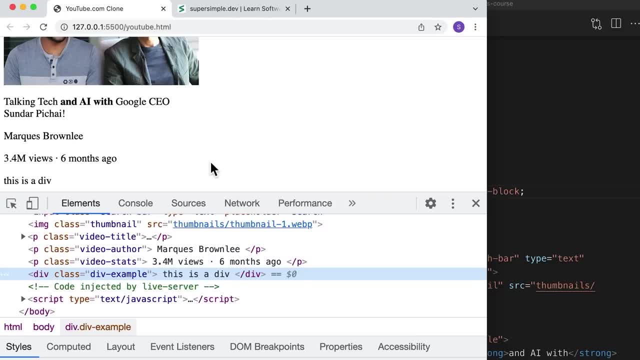 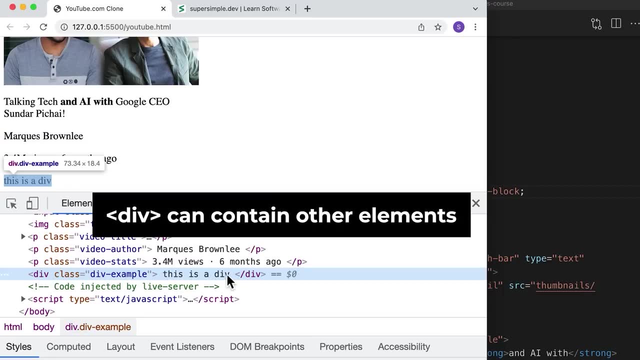 is a div so useful? The key feature of a div is that it can contain any other elements inside. So right now we only have some text inside this div, but we can actually put paragraphs, we can put images, we can put any elements inside. 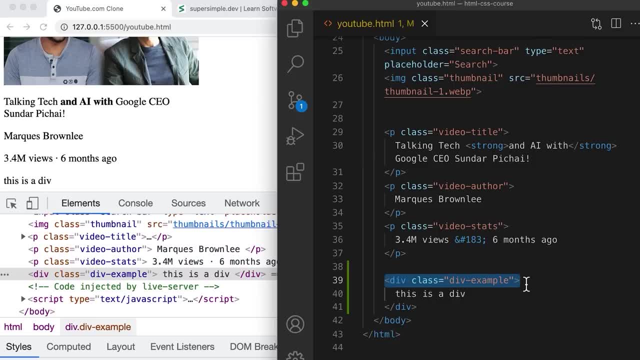 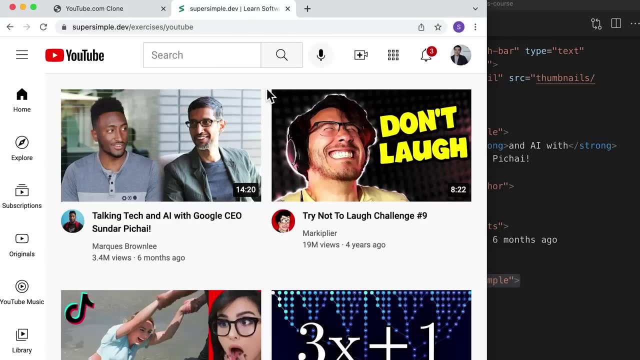 divs as well as other divs. Divs are meant to be containers And if we look at the YouTube design that we have in our project, we use containers everywhere. So here's a container, here's another container and here's. 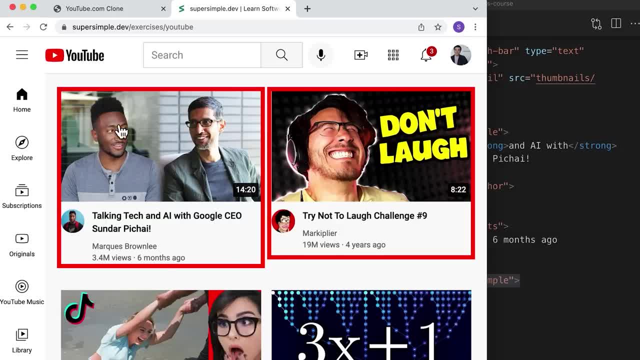 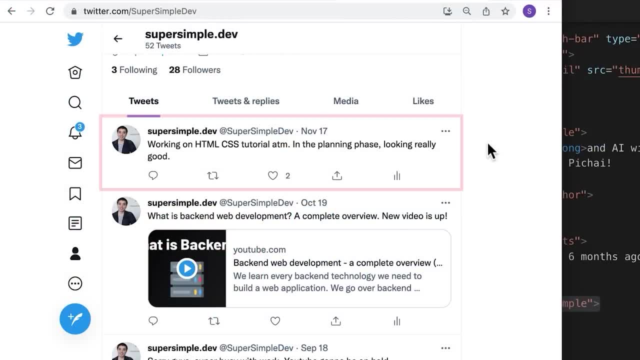 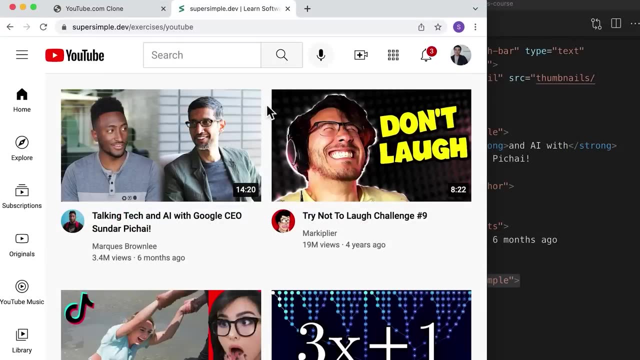 another container. These containers allow us to group all of these elements together so that we can create a layout that looks like this. Here's another example from Twitter. Here's a container, here's another container and here's another container In order to build. 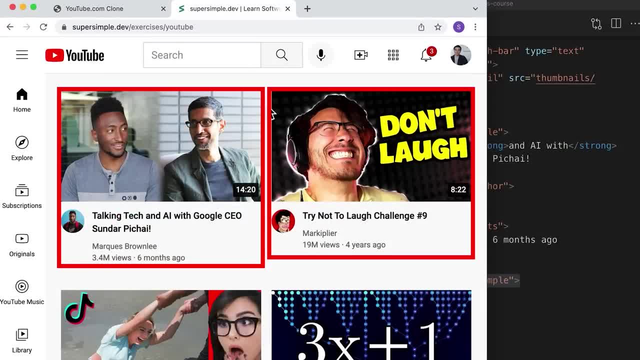 a complex real world website. we need containers to group our elements together and lay them out on the page, And the div is the perfect solution for this container problem And that's why it's used so much. Let's go back to our website and we're going to 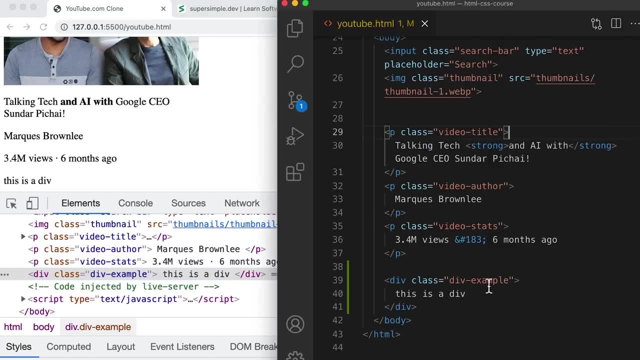 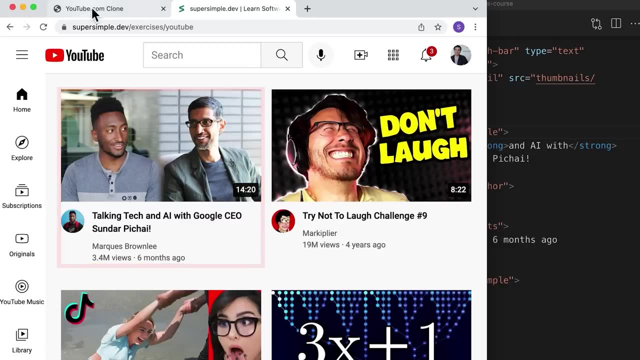 practice using our div as a container. So we're going to create a container, just like our final project, for this entire video preview here. So that means we're going to put all of these elements, this image and all three paragraphs, inside our div. 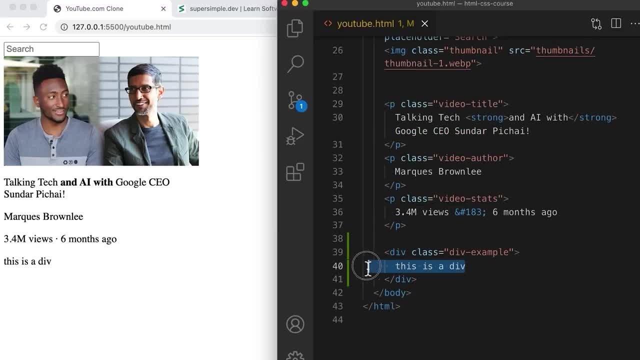 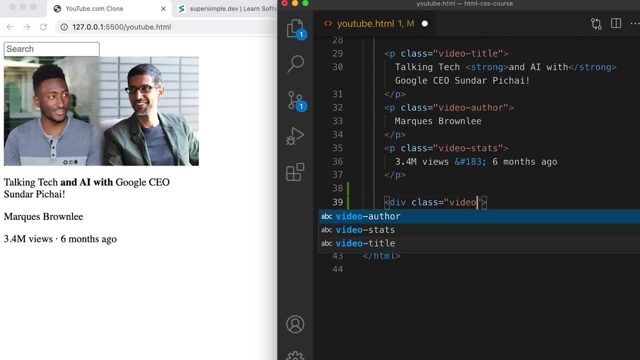 Let's see how that works. So I'm going to get rid of this text first, And then I'm going to change this div to a class of video-preview, Because this is going to contain all these elements that are part of a video preview. 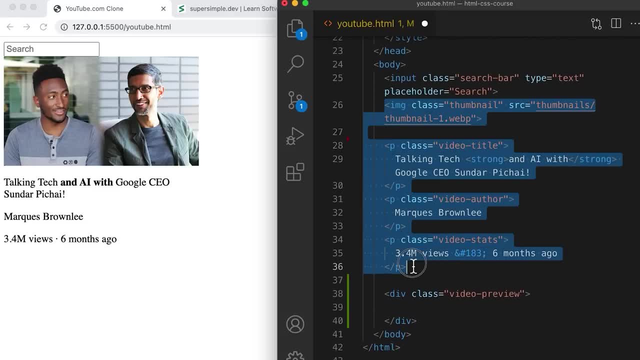 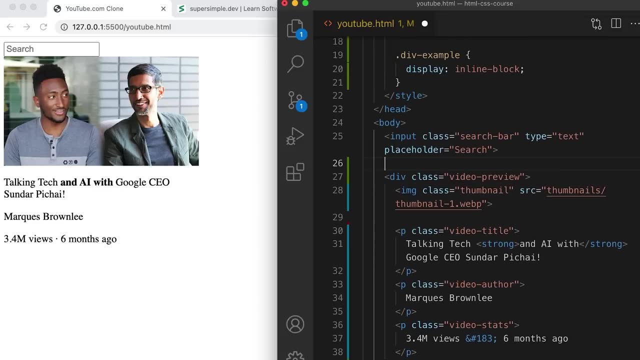 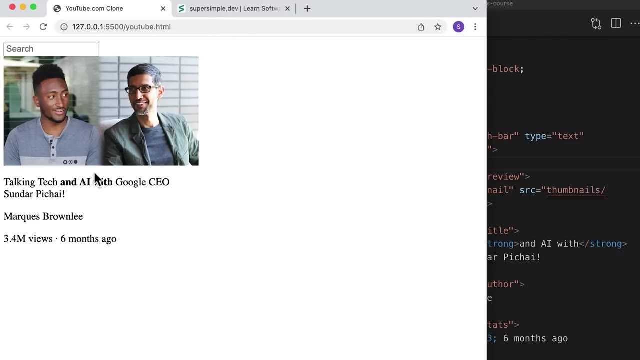 And then I'm going to move the image and the three paragraphs into the div. Now save, And you might not notice any difference because the div is simply just drawing a box around the content inside. But we can right-click and inspect And we can. 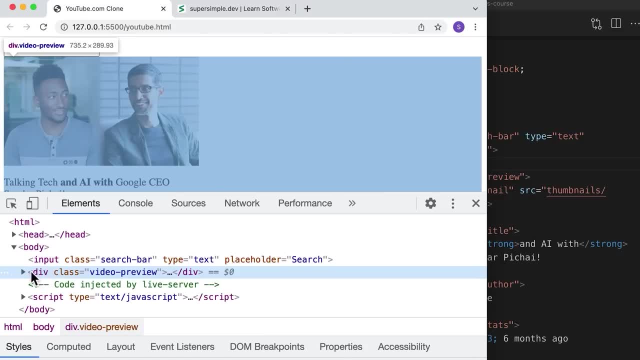 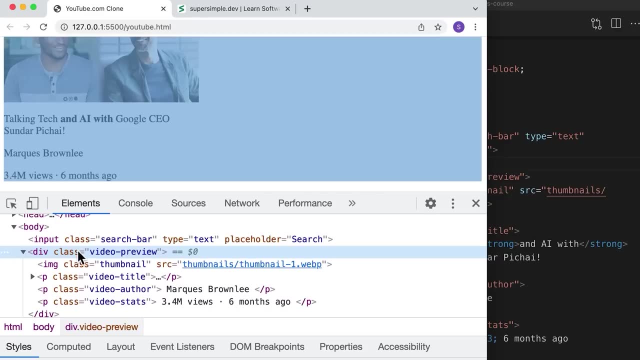 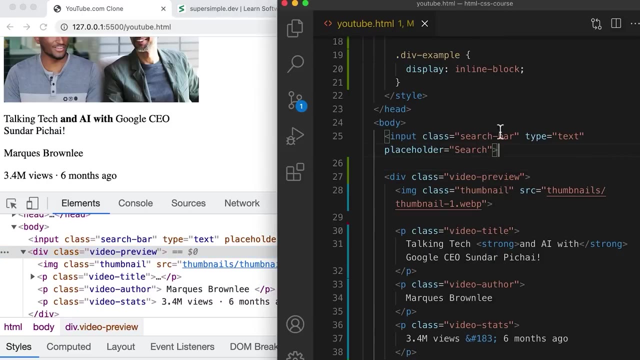 see the div in our HTML here, And inside the div we have our image and our paragraphs. The div is just creating a box around all this content. So now I'll show you why containers are so useful. We're going to go into our code and we're going to 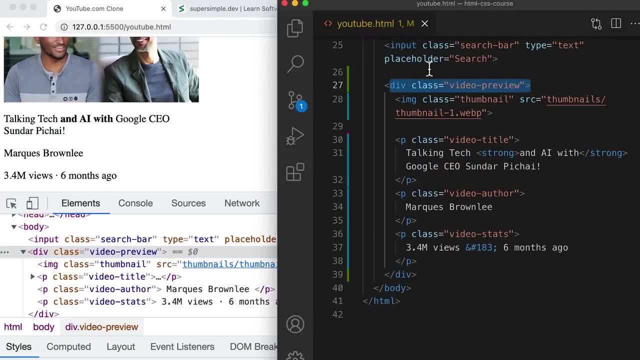 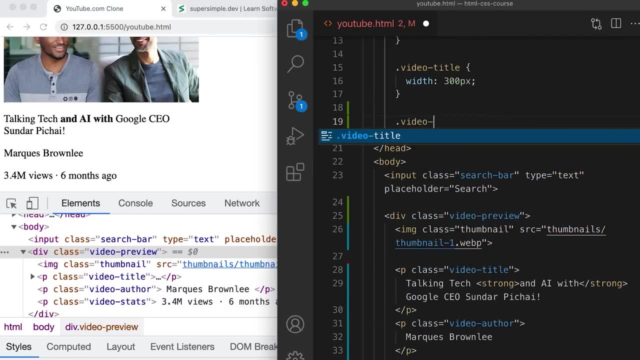 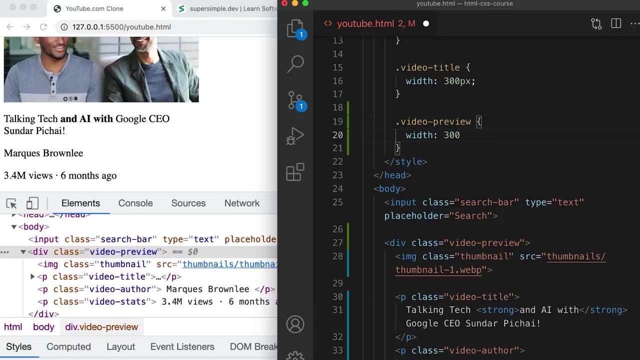 change the width of our div element here, So we're going to go up here and we can remove this. Let's style the video-preview class And we're going to set a width of 300 pixels. Let's see how that looks. 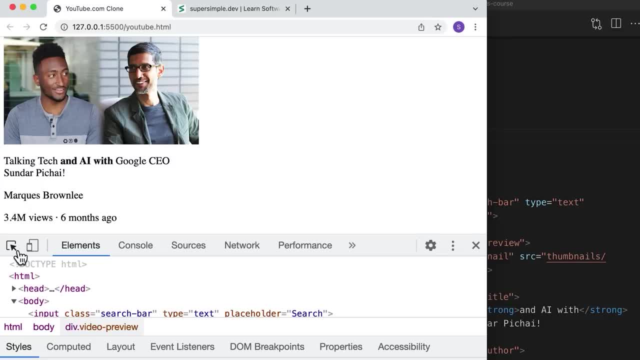 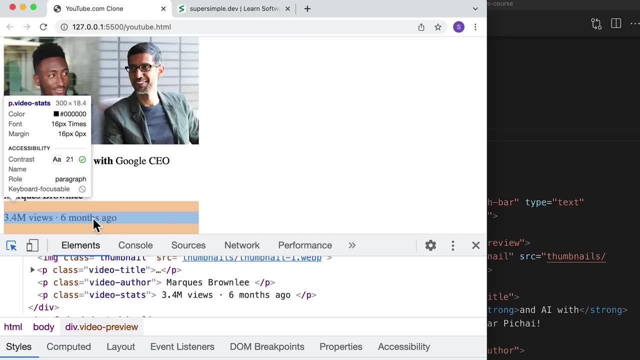 So the page doesn't look any different. but if we click the icon in the top left and then hover over our paragraphs, we'll notice something interesting. This paragraph is a block element, so it's supposed to take up the entire line. But in this 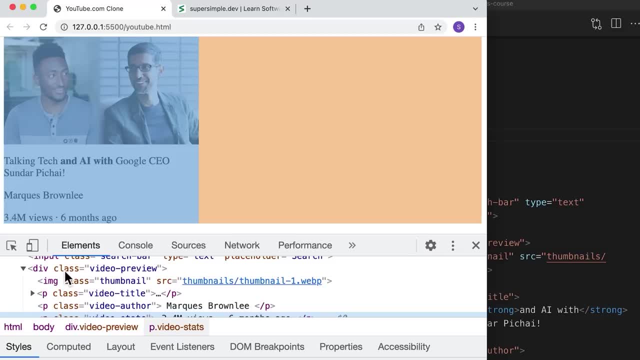 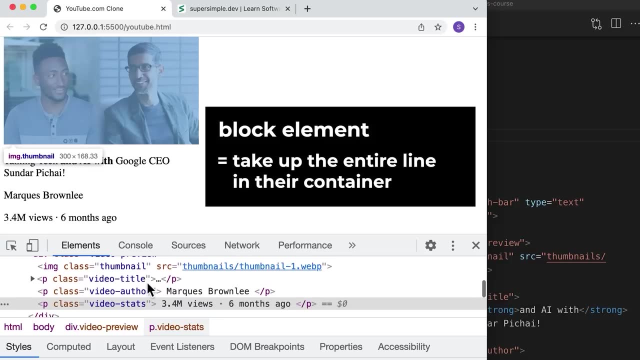 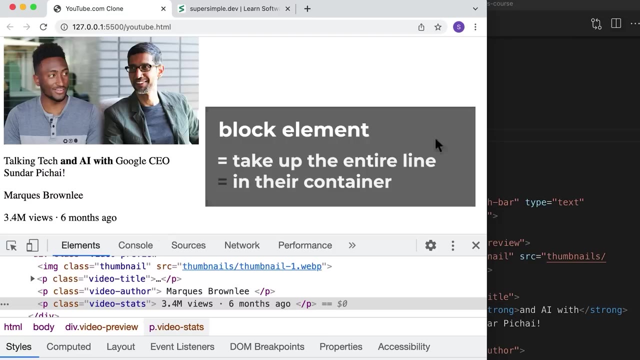 case, because this paragraph is inside a div. it takes up the entire line in the div. So the way that block elements actually work is that they take up the entire line in their container rather than on the page. So that's really useful because if we 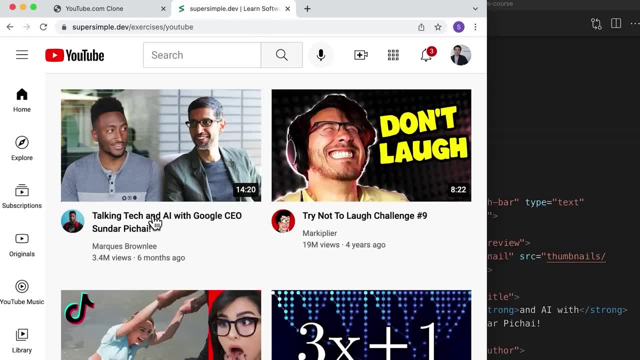 look at our final project. So for these paragraphs we want them to appear on separate lines, like this. So we do want them to take up their own line, But we don't necessarily want them to take up the line on the entire page, because we have some stuff. 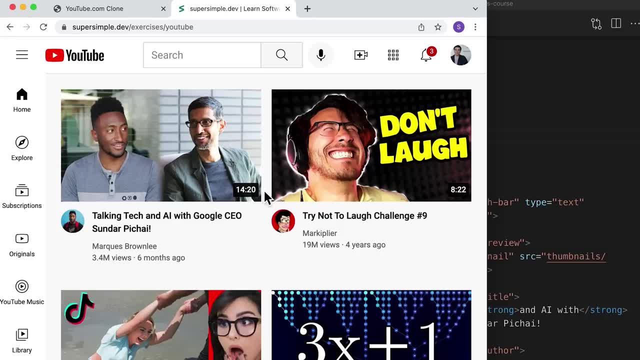 on the right side here. So to solve this problem, we put the paragraphs inside a container so that they take up their own line in the container and not in the page, And that's how we can create a layout like this. Let's go back to our 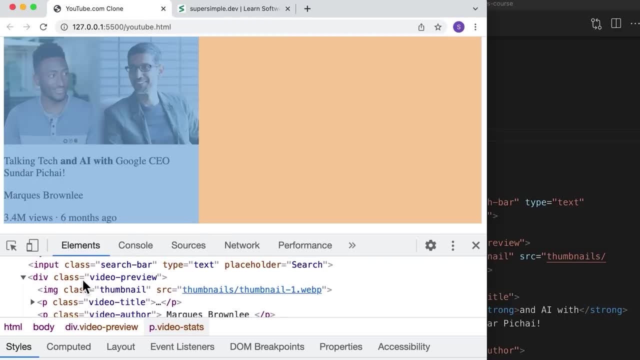 website If we hover over our div now. so this blue box on the left is our container. It groups all the elements together and keeps it within that blue area that you see. Now, a really cool thing about this is that notice that the blue box 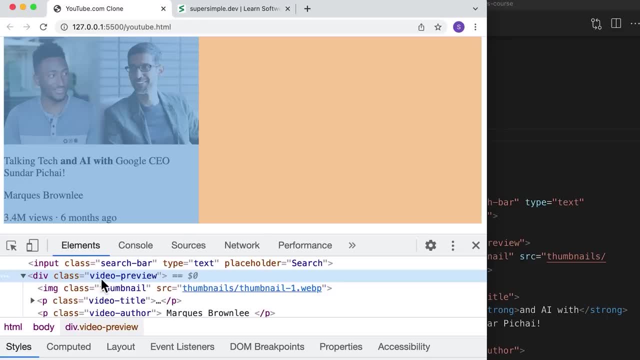 doesn't actually take up the entire page, So we can actually have a second box beside it on the right. So we can add another blue box on the right containing another video preview. So now we're going to do that. But first of all, 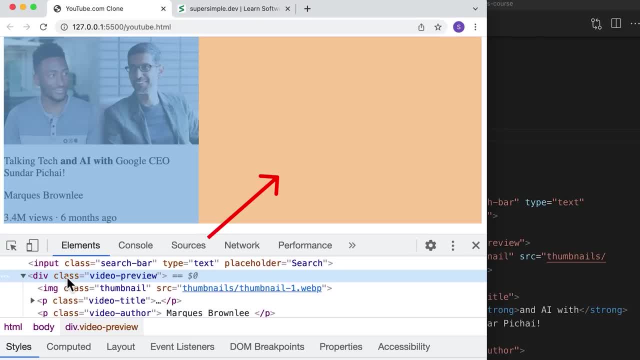 a div by default is a block element. So notice on the right side it's all orange. That's because this div is taking up the entire line. In this case, we don't want it to take up the entire line anymore. That's why. 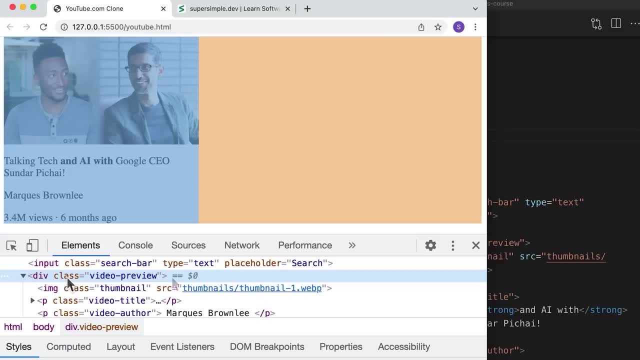 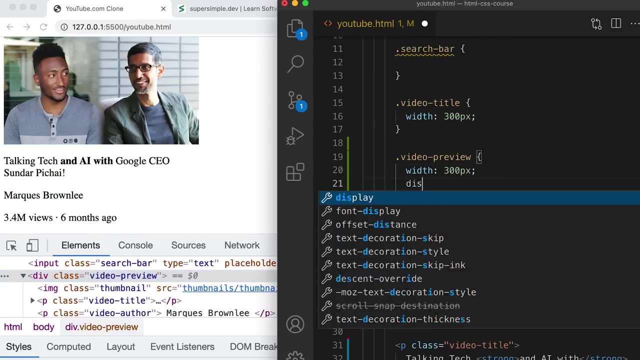 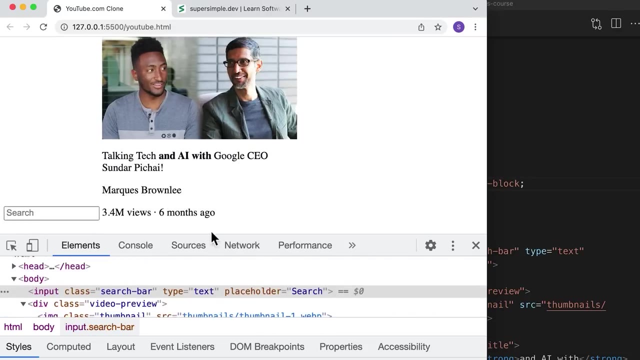 we're going to convert it into an inline block element. So let's go into our code, We're going to go into the video preview and we're going to type display- inline block. Let's save it. And now you can see that our div. 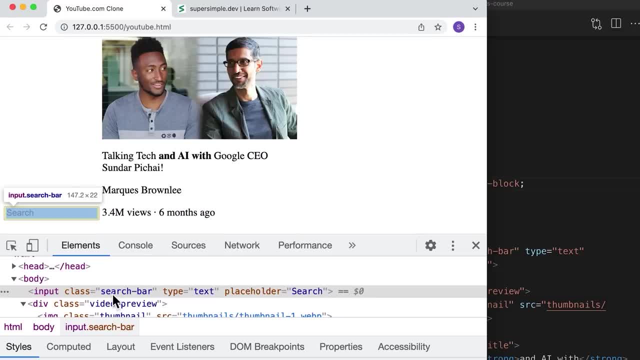 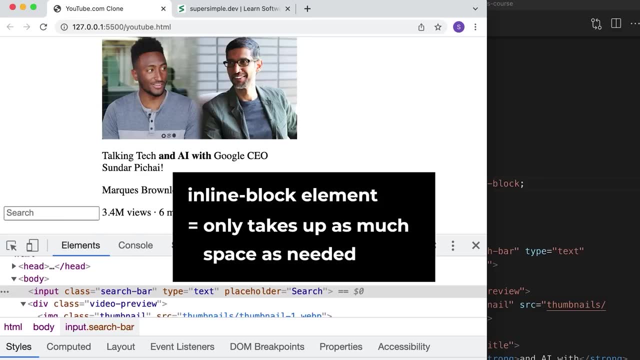 is a display inline block. It's actually appearing beside our search bar because this is also an inline block, So they're both only taking up as much space as they need to, and now they can appear beside each other, However we do. 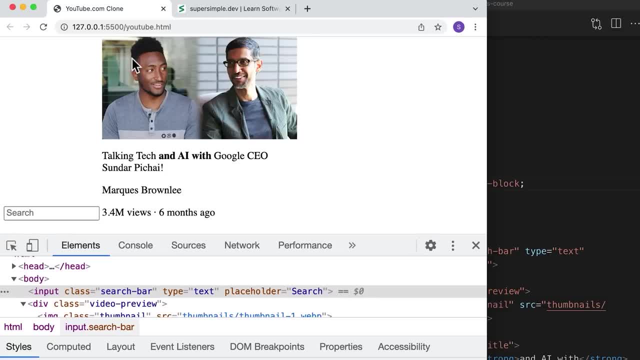 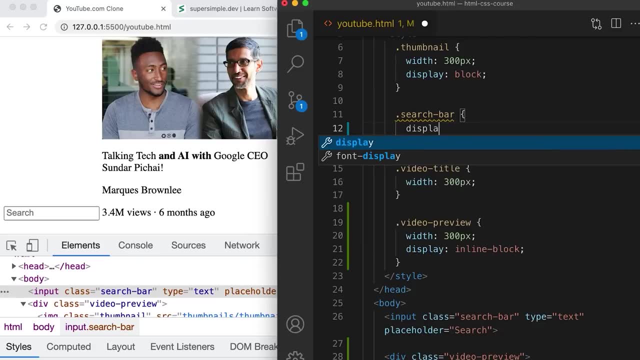 want the search box to be at the top in its own line, So we're going to practice using the display property again. We're going to set the search bar to display block So that it takes up the entire line and everything else is forced below it. 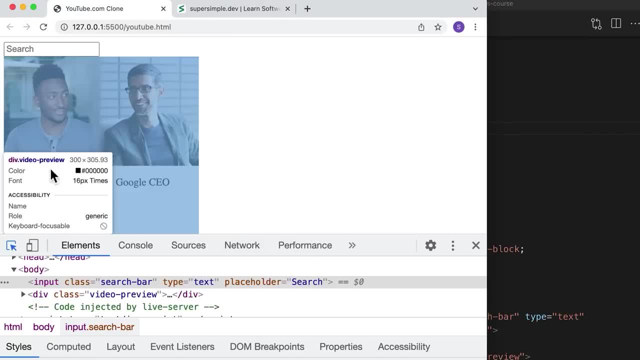 Save it and refresh. And now, if we hover over this input element, we can see that we forced it to take up the entire line. Next, we're going to create another video preview beside this one, Because this is inline block. now we can put another. 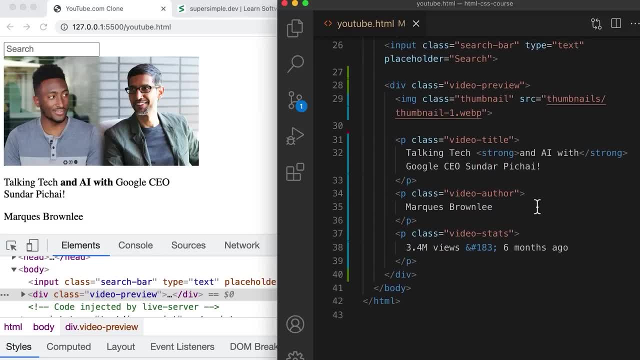 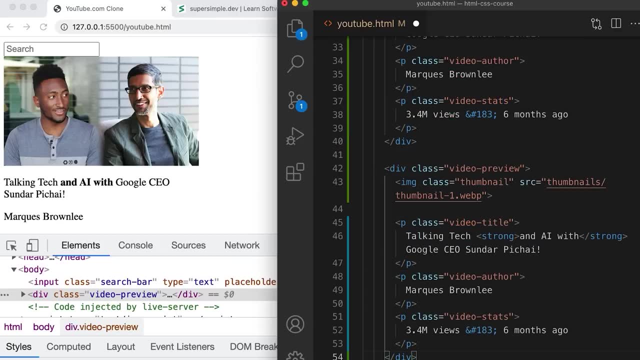 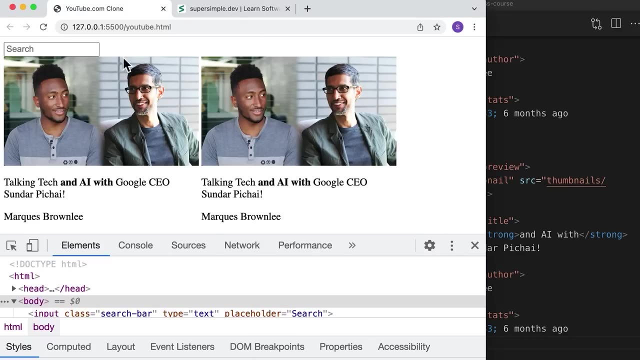 div here. So I'm just going to simplify this by making a copy of our current code. I'm just going to copy and paste And now we have two video previews. Save it and there we go. We now have two video previews beside each other. So 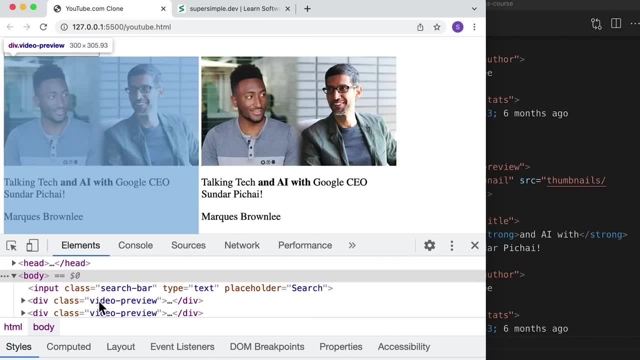 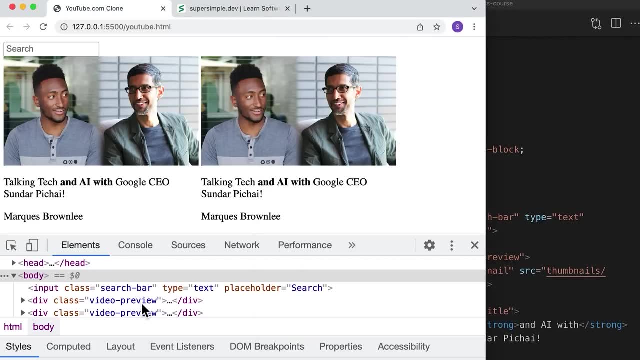 they are two containers right beside each other And, remember, in our CSS we set the width of these containers to 300 pixels, So that's the amount of space that they take, And we set their display to inline block So they don't take up the entire line. 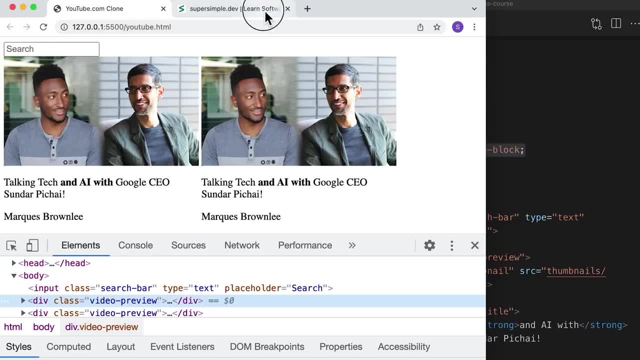 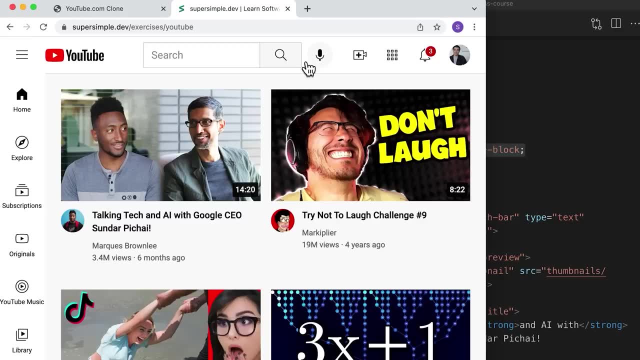 and they can appear beside each other, And now we're on our way to creating a layout that looks like this. In fact, let's actually replace the second video preview here with this content. So to do that, we're going to download the. 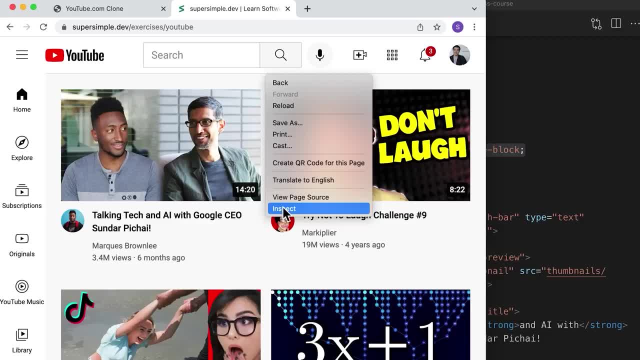 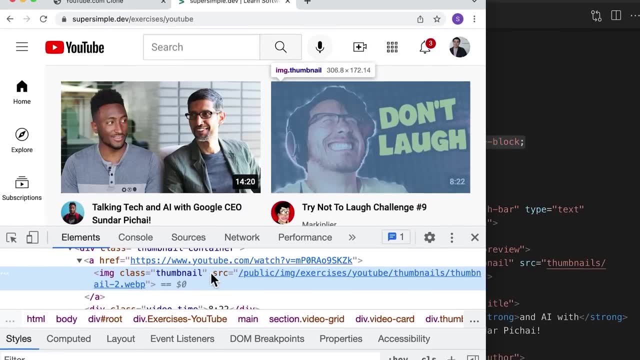 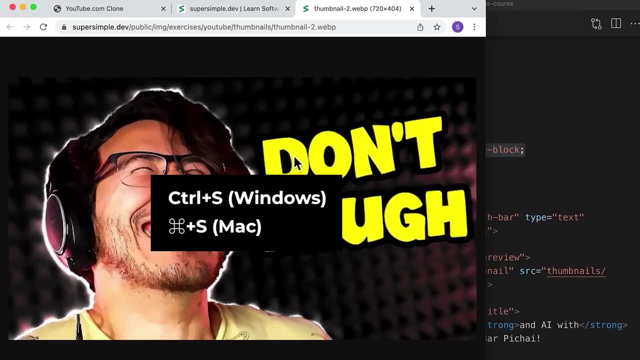 thumbnail and then change the text. So let's right-click and inspect. We're going to click this top left and then click this image. And now I can download the thumbnail by going to this URL and then clicking down here. I'm going to Ctrl-S. 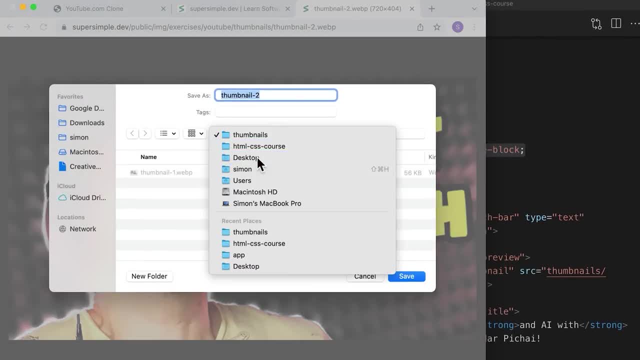 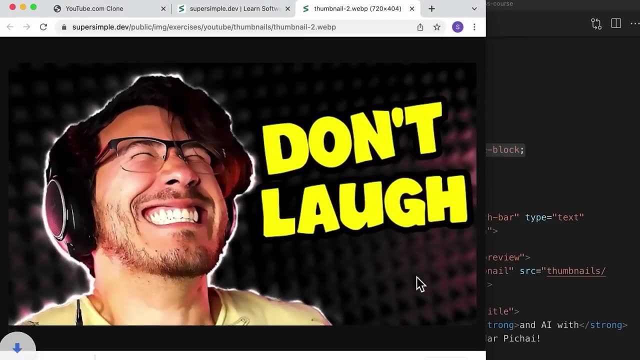 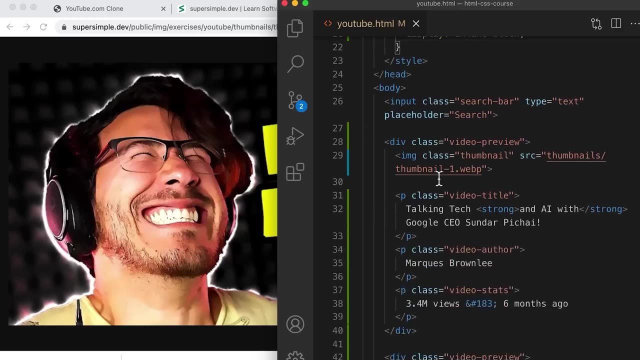 to save the thumbnail. I'm going to save it in the folder that contains my code, in the thumbnails folder, along with our previous thumbnail. So save it here And I should see it in my code editor right there. Next we're going to swap. 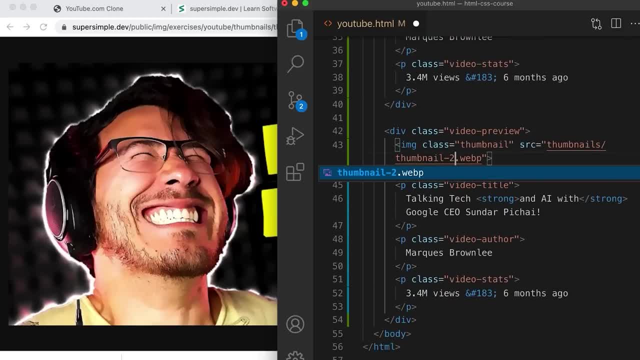 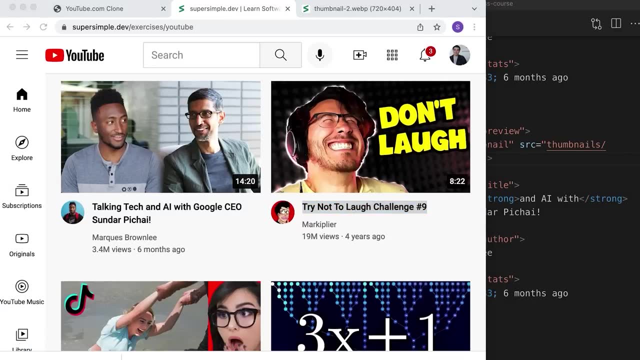 out the thumbnails. So instead of thumbnail 1, we're going to set thumbnail 2. And we're going to change the text. So I'm going to change this text here to be my title, And I notice we're still using the strong element which we can. 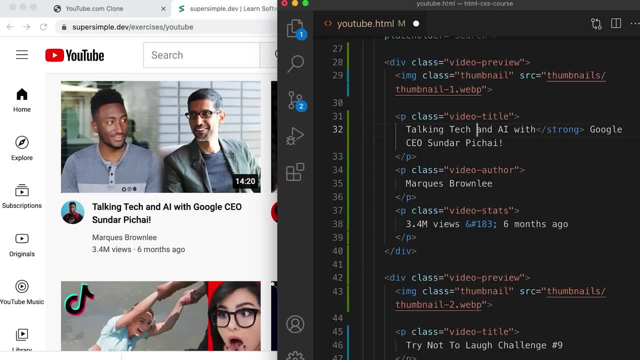 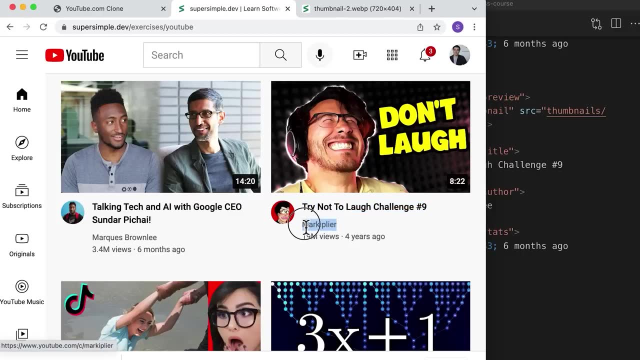 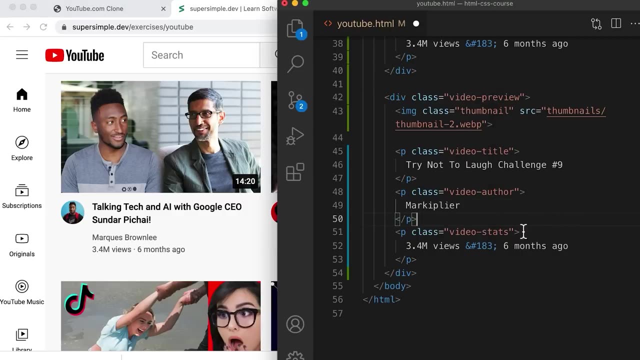 now delete because it was just for an example, And I'm also going to change the channel name here and the video stats, which is 19 million and 4 years And 4 years ago. So now, if I save this, we have: 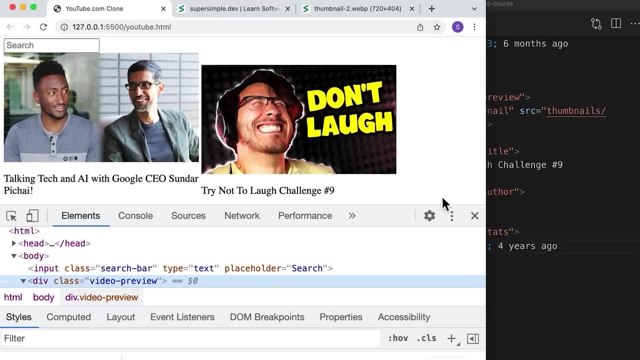 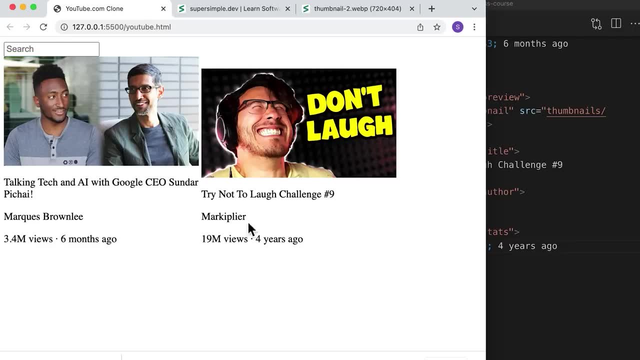 two different video previews, But now we have a problem. You'll notice that these two aren't aligned with each other, And that's because this container is actually a little bit taller than this one. This piece of text here wraps around to a second line. 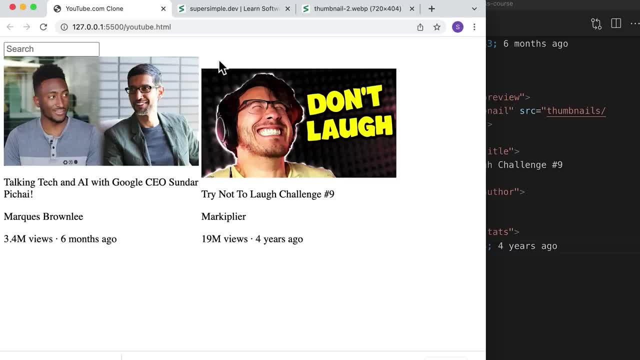 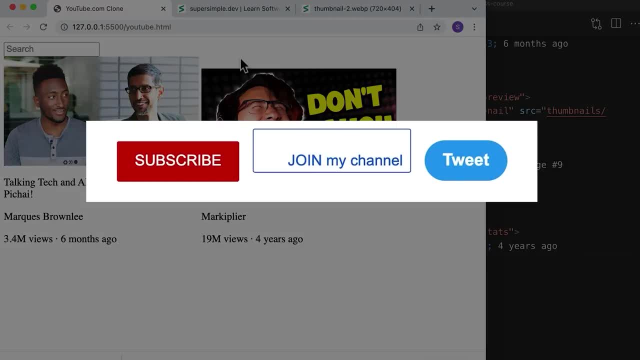 while this one does not. However, to make it look better, we want to align these at the top. So we learned this way back in one of the earlier lessons and we're going to review how to do that. We're going to go into our 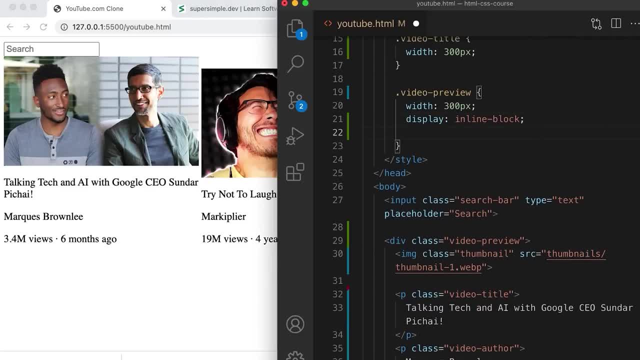 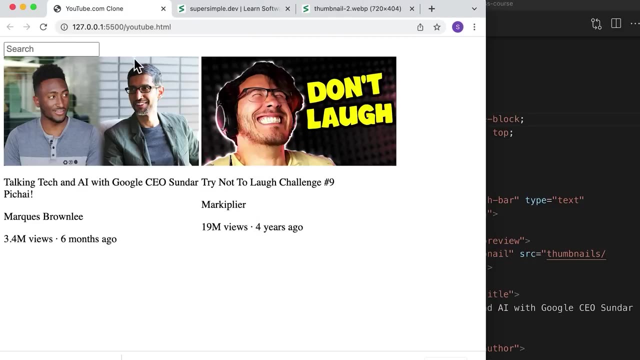 code and we just have to set this property vertical align, And we're going to set it to top So that these elements align at the top. I'm going to save it And now that looks pretty good. We now have two different. 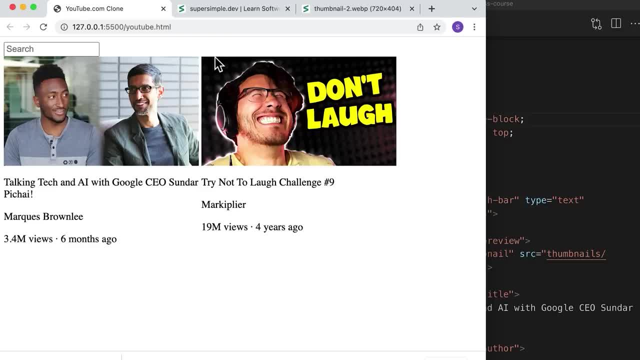 video previews and they are aligned with each other. The last thing we'll do is to add some space between them. So remember, the space outside of an element is called margin, And we're going to add margin to this entire container right now, So we'll go into our code. 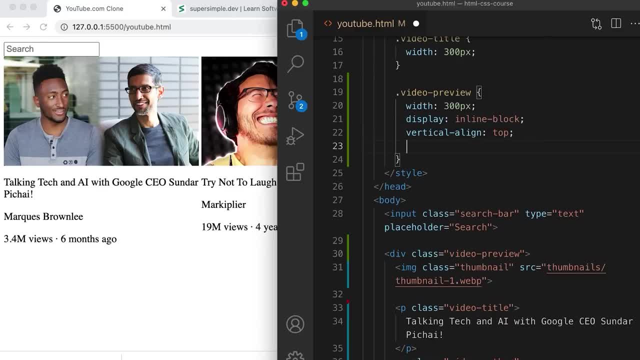 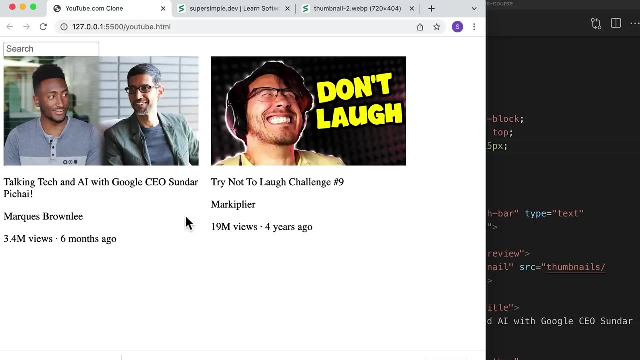 and in the video preview styles we're going to add margin dash right And let's set it to something like 15 pixels, Save it. and now we added margin on the right. And now the interesting thing about this is if we right click. 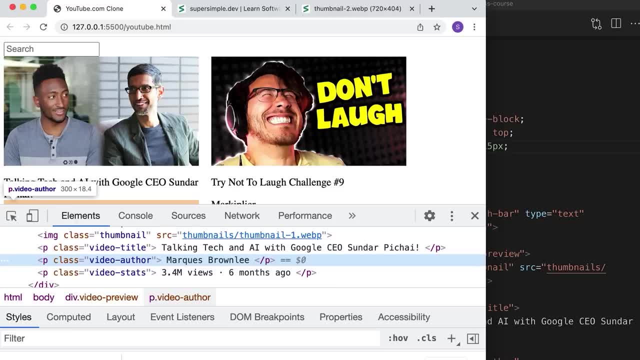 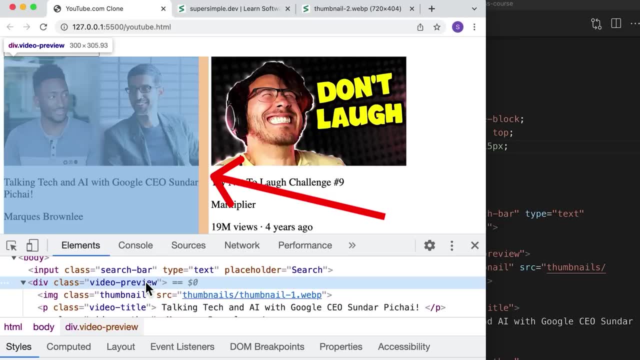 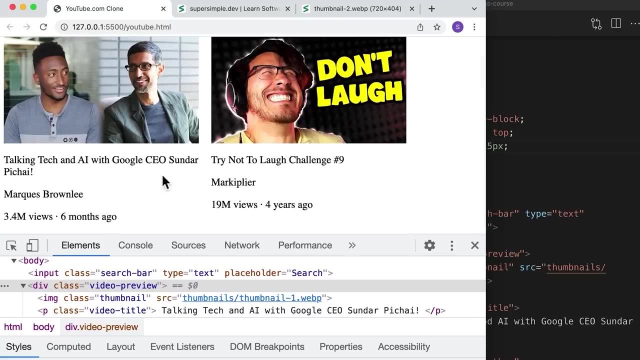 and inspect. and then in our HTML we find our div, which is here. you'll see that the margin is applied on the entire div. So that's how the div element works. It's a container that groups other elements together so that we can create complex. 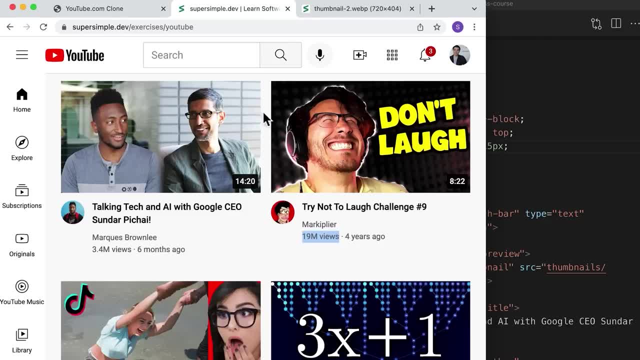 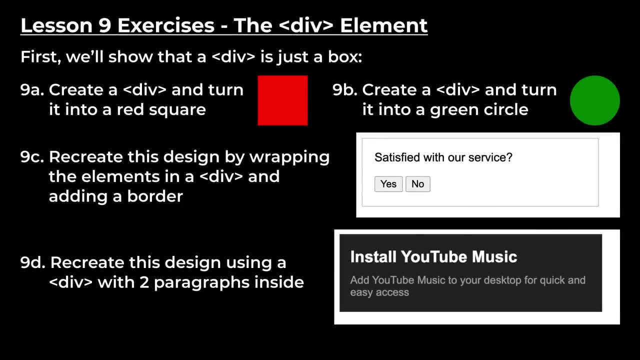 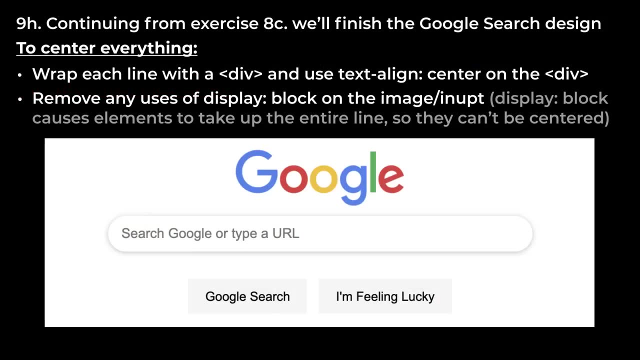 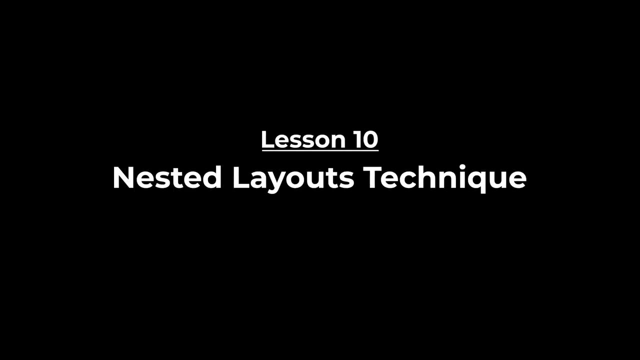 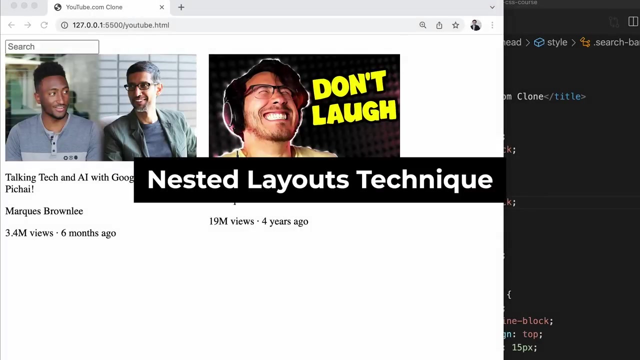 layouts like this and, eventually, our YouTube project. Alright, so this is probably the most important lesson of this course. We're going to learn a technique called the nested layouts technique, and this is going to get us to a professional level with HTML and 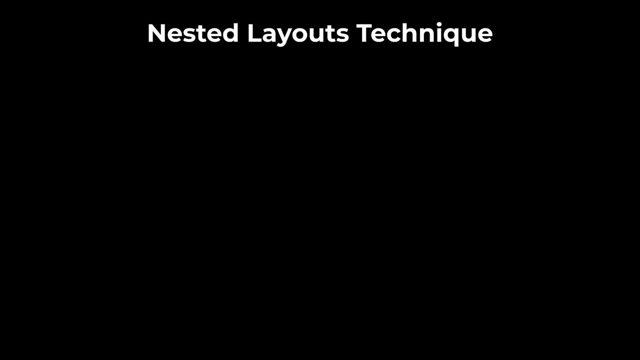 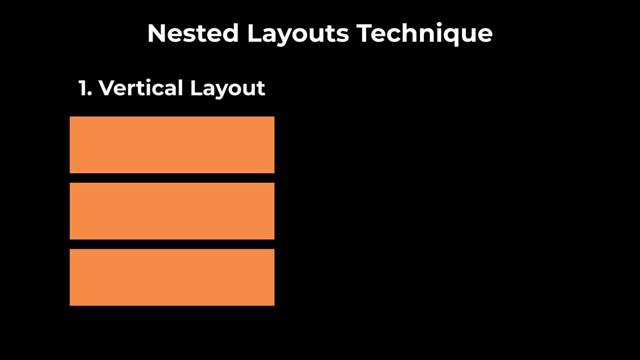 CSS. So what is the nested layouts technique? The basic idea is that there are two types of layouts. The first one is a vertical layout which looks like this, where items are on top of each other, And then the second one is a horizontal layout which looks: 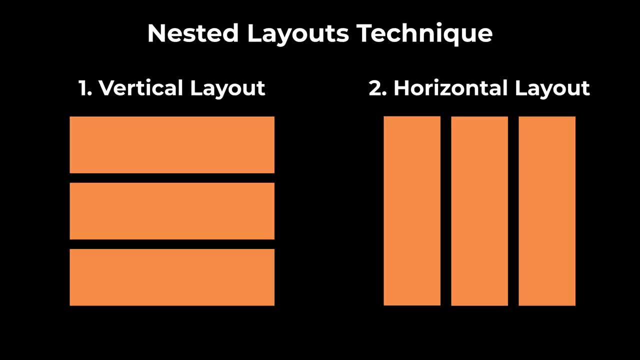 like this, where items are beside each other, And by using a combination of vertical and horizontal layouts, we can create almost anything that we see on a website. So, for example, let's take the YouTube video preview that we've been working on. 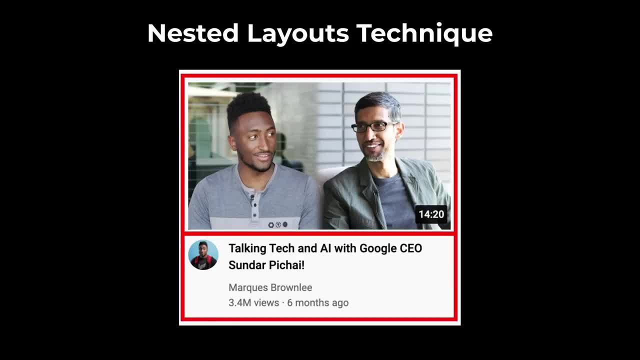 We can break this down by using a vertical layout, and then, inside this vertical layout, we're going to have a horizontal layout, And then, inside this horizontal layout, we're going to have a vertical layout. So, as you can see, we have. 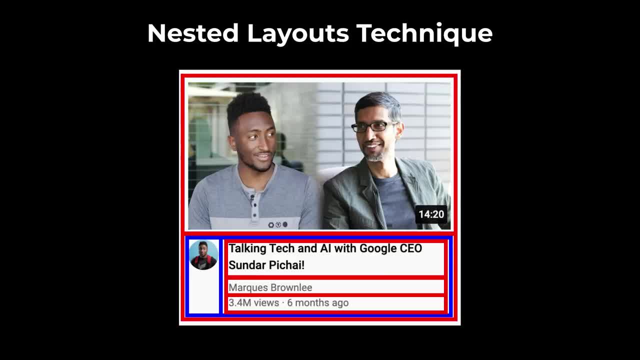 layouts, inside layouts, inside layouts, And that's why it's called the nested layouts technique, And using this we can pretty much break down almost everything that we see on a professional website into a series of layouts and then recreate them using our code. 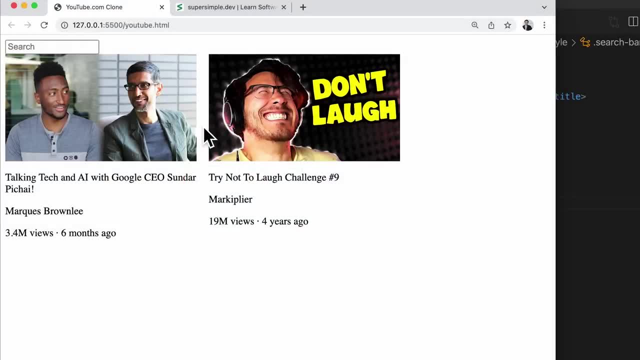 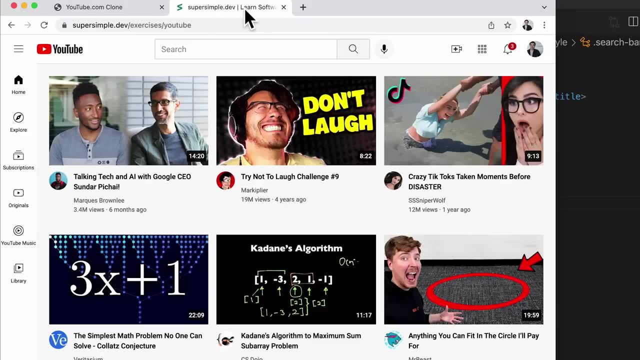 So now we're going to go through together a way that we can practice using the nested layouts technique to break down a design. We're going to go to our final project. If you closed it, you can go to supersimpledev. slash exercises- slash YouTube. 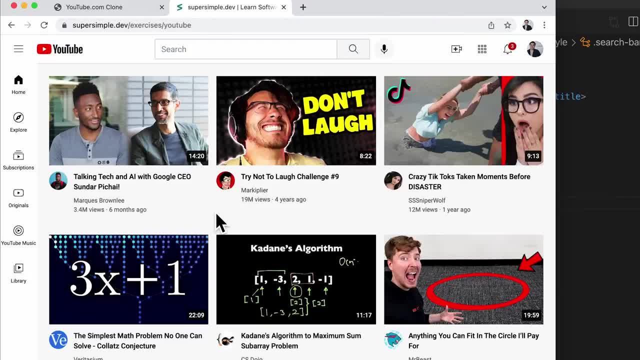 And what we're going to do is we're going to take a screenshot of one of these designs and then we're going to use an image editing software to draw out the layout. So first let's create a screenshot On Windows. 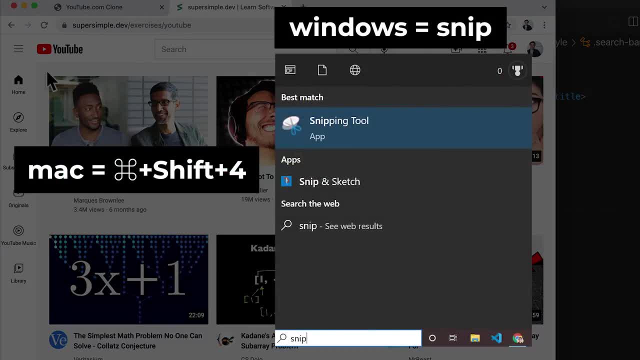 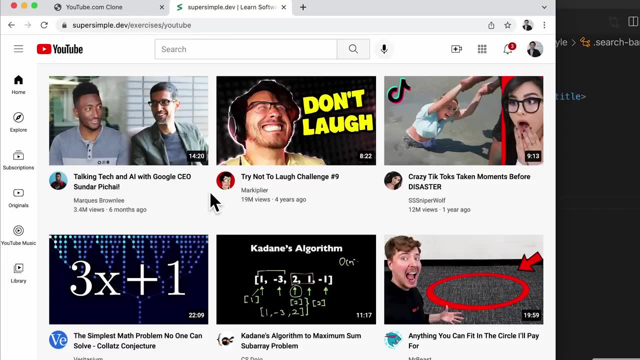 you can use an app called Snip On Mac. we're going to type command, shift and 4 to create a screenshot. So let's take a screenshot of this and then we're going to upload this into an image editing software. Now feel free to use anything. 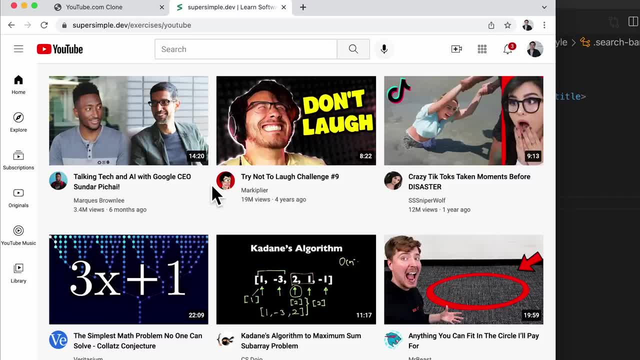 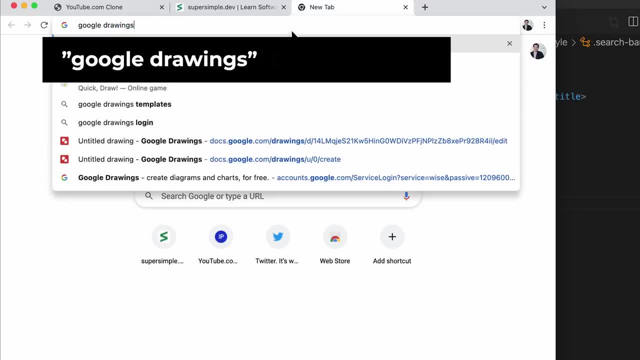 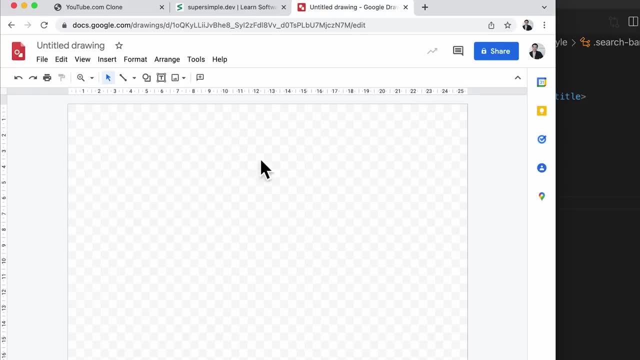 that you're comfortable with. but if you don't know what to use, we can go to a new tab and we're going to search for Google drawings And we're going to use this to practice the nested layouts technique. So once we have this open, 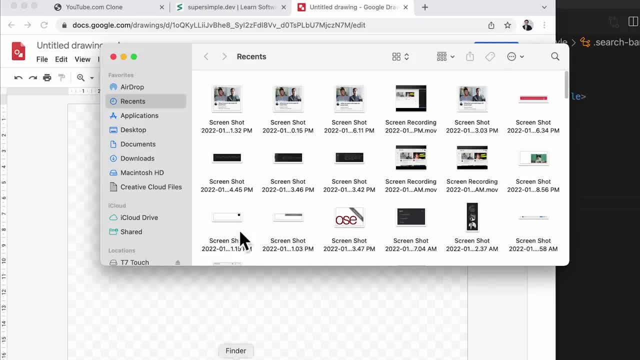 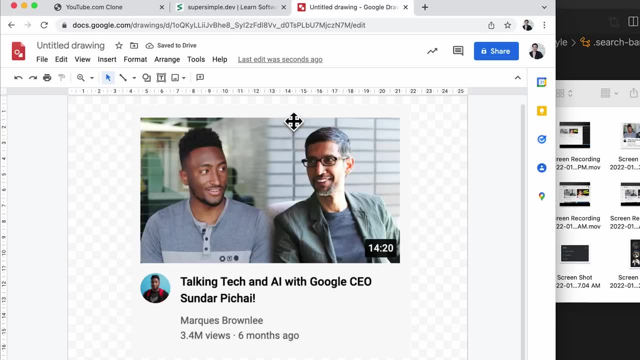 we're going to upload our image. I'm going to go to my computer and upload this screenshot And now we're just going to draw some rectangles to represent our layout. So we're going to go up here to shapes and we're going to create a rectangle. 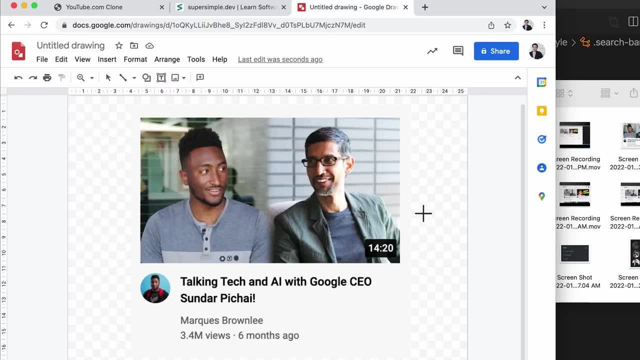 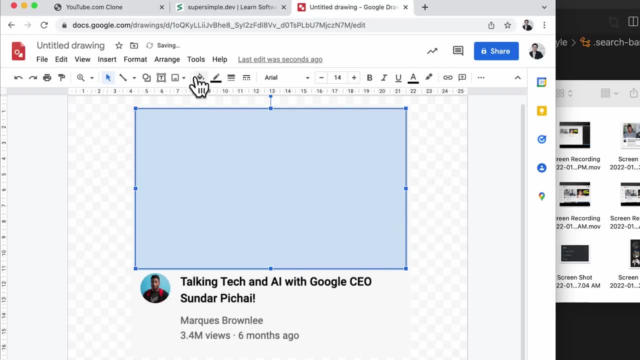 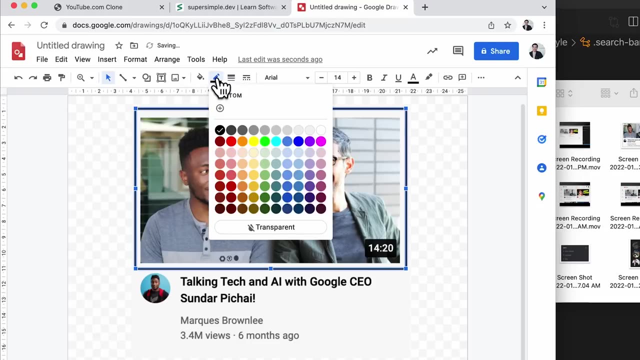 And first we're going to create a vertical layout 1 and 2.. So I'm just going to draw a rectangle here. Let's change the background to transparent so we can see what's underneath, And I'll make the border a little more thick. 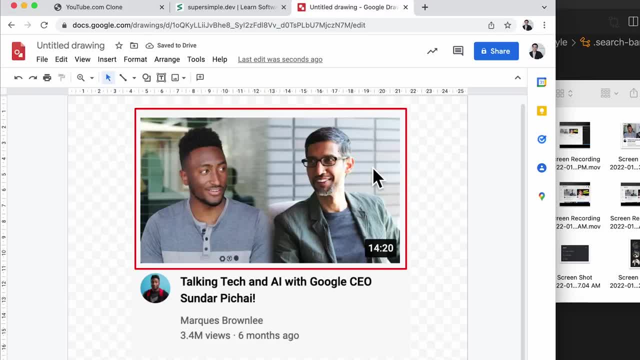 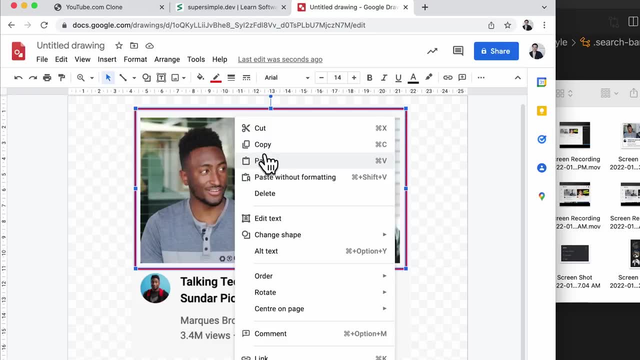 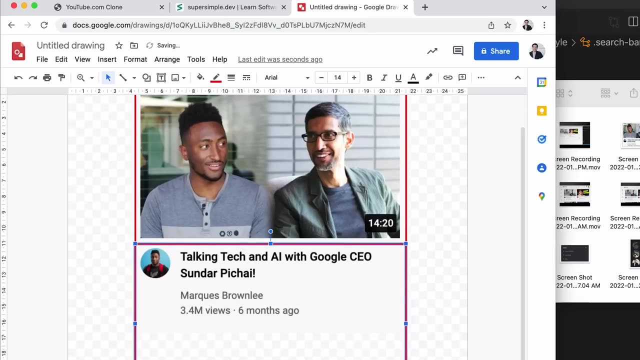 and change it to red So it's easier to see. And now I'm going to copy this and paste it to create a duplicate And I'm just going to move it down here And resize the rectangle like this: Alright, 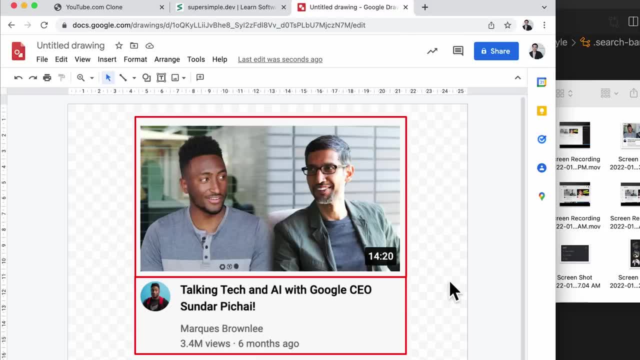 so, just like that, we created a vertical layout For now. don't worry about the video time here. We're going to recreate this later in the course using another feature of CSS. And now, looking at our design, we have a horizontal layout 1. 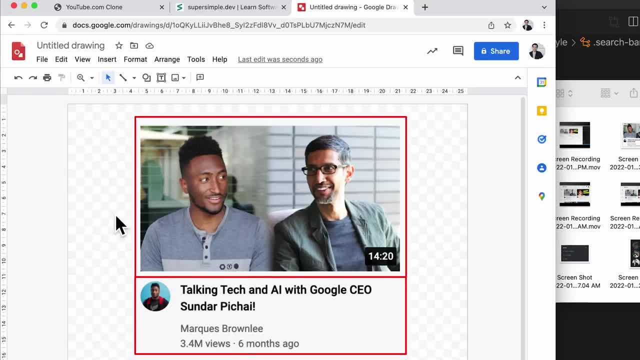 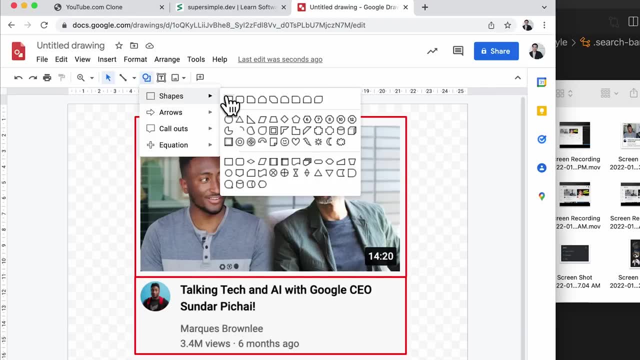 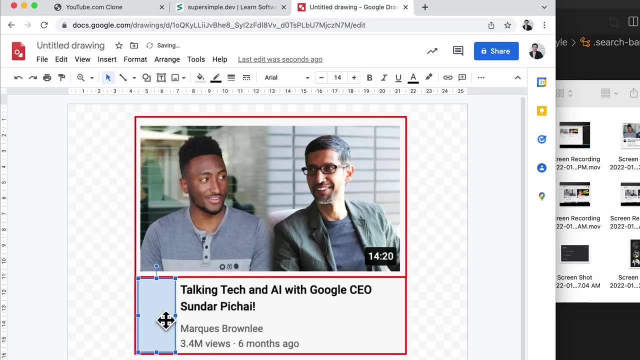 and 2.. So to create a horizontal layout, we're going to draw it out again using rectangles. So let's go in here and we're going to create another rectangle And we're going to draw out the horizontal layout like this. So here's 1.. 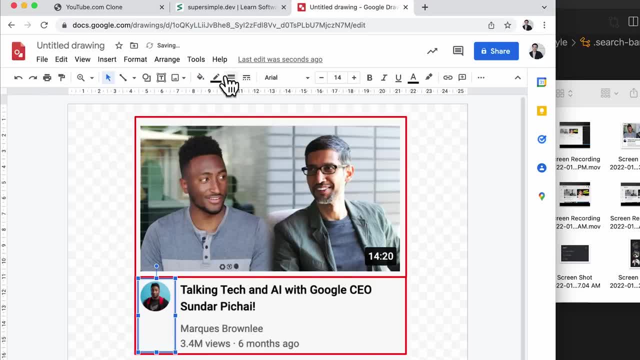 Change the background to transparent, Make it bold, And I'm going to use the blue color to represent a horizontal layout. Now I'm going to copy this and paste it here And resize it a little bit Like that, And now we have our horizontal layout. 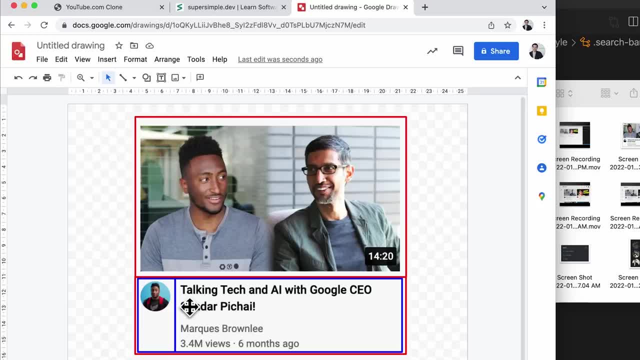 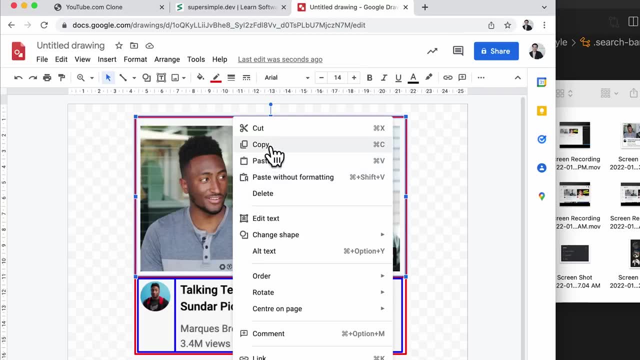 And finally, inside here we're going to have a vertical layout like this. So again, we're just going to keep drawing rectangles. I'm going to copy this and paste it And move it down here and resize it a little bit. 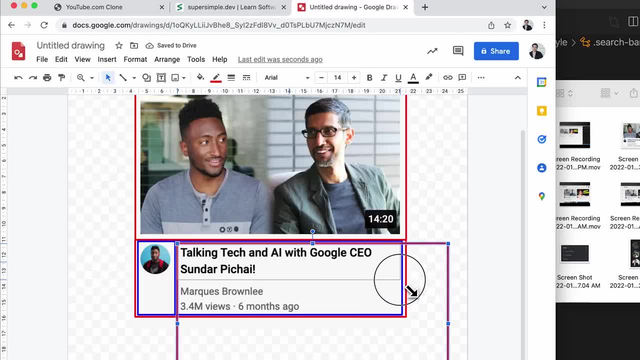 so that we can see it So right here And then copy this And then paste it again. We're going to create the second part of our vertical layout Like that And then copy and paste it one last time Down here. 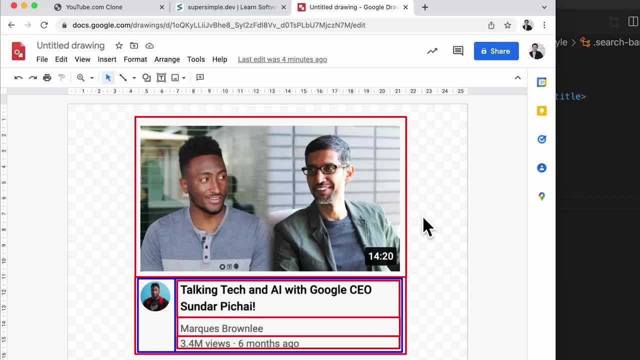 So that's how we use the nested layouts technique to visualize and break down a design into a combination of vertical layouts and horizontal layouts. Now let's do some more practice. We're going to take another design and break that down using this technique. So we're going to open. 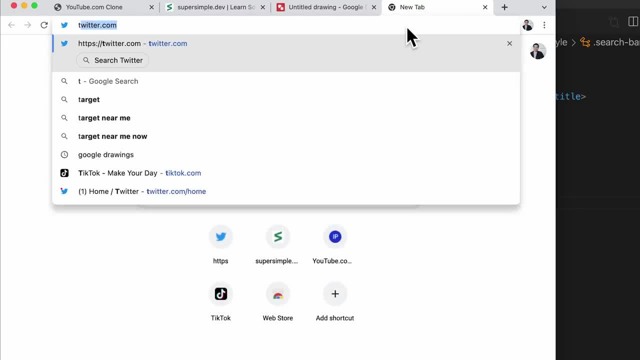 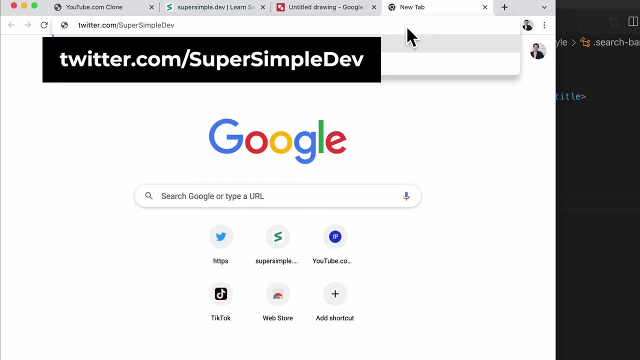 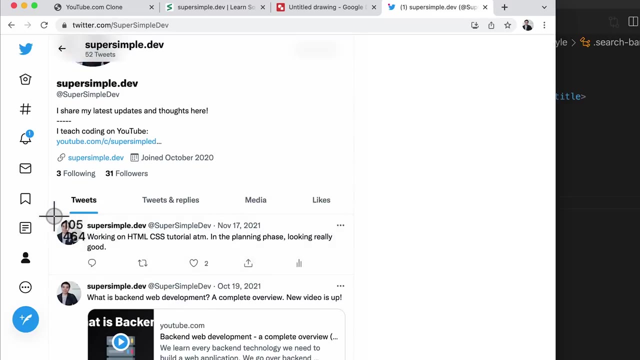 a new tab And we're going to go to twittercom slash, super simple dev And we're going to just take one of my tweets here And take a screenshot of this And we're going to break down this design using the same technique. 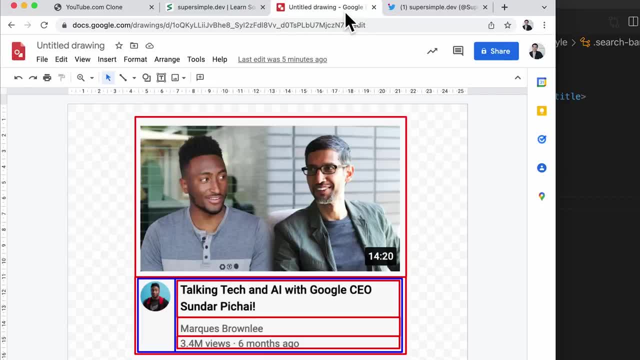 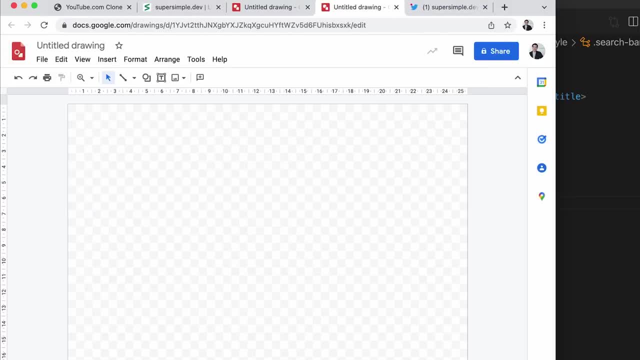 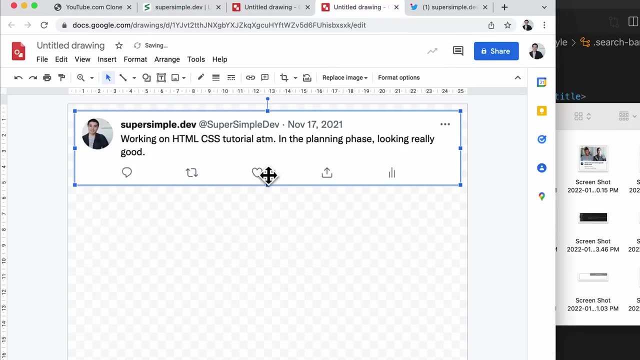 So let's go back to Google Drawings And we're going to create a new drawing to practice with, And let's upload that screenshot that we just took onto this new drawing right here. So now we're going to do the same thing. We're going to draw a rectangle. 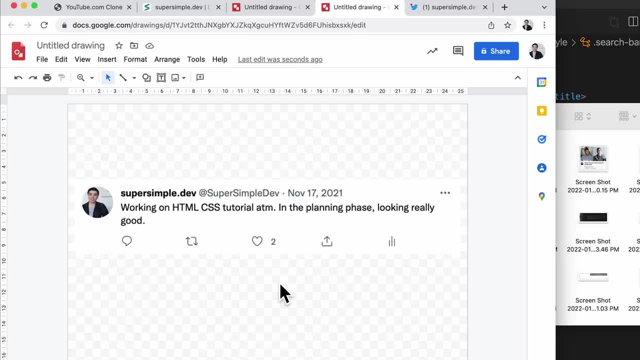 to represent the nested layouts. So let's take a look at this to see how we can break this down Immediately. I see that we have a horizontal layout One and two, So we can break it down into that. first, Let's draw a rectangle. 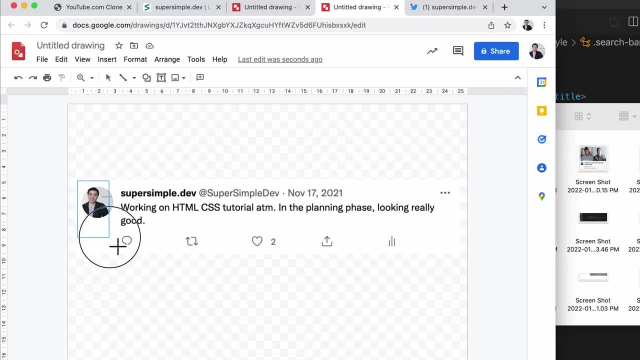 to represent that. So here's the first one, And I'm just going to make it blue to represent a horizontal layout And copy and paste it like this. So that's our horizontal layout. And now looking at the design inside here, I can see that we can. 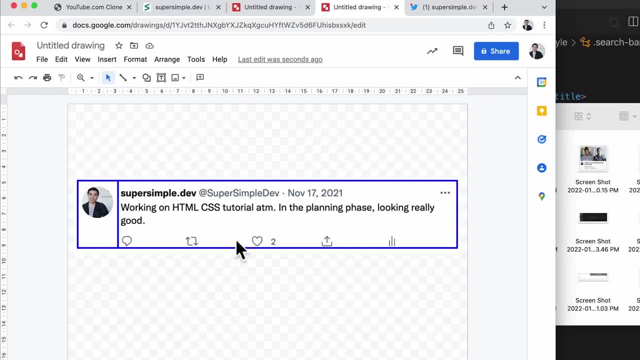 break it down further into a vertical layout. So I'm going to draw some more rectangles And I'm just going to draw it right here And style it a little bit and make it red to represent the vertical layout. So copy and paste. 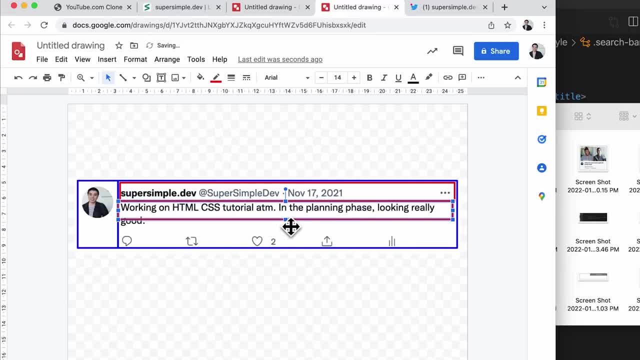 And I'm just going to move it down here. Okay, Okay, so that's two: Copy and paste to get three. So it doesn't have to be perfect. It's just here to help us visualize the design. Alright, so we have a horizontal layout. 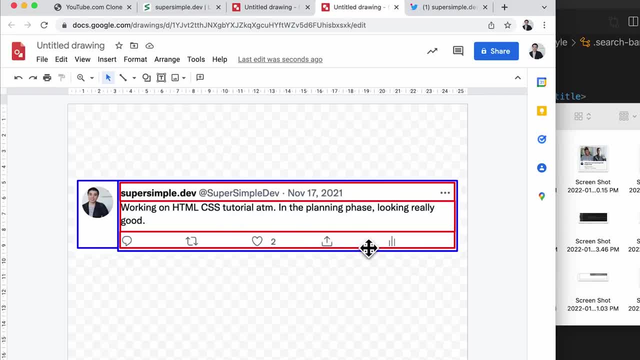 And then inside we have a vertical layout And now, looking at this, we can also break this down into a horizontal layout. Let's draw some more rectangles. Actually, I'm going to just copy this one And paste it And resize it here. 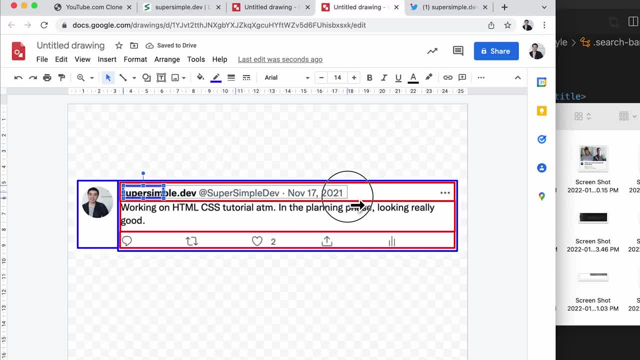 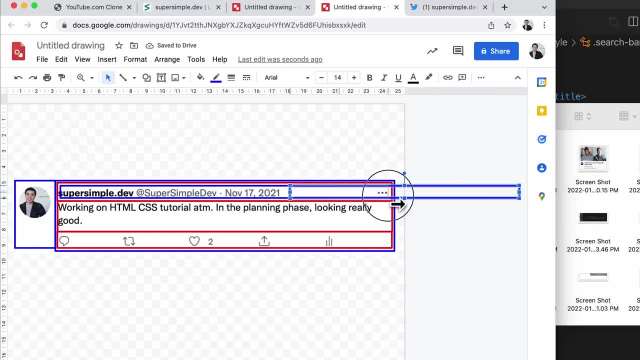 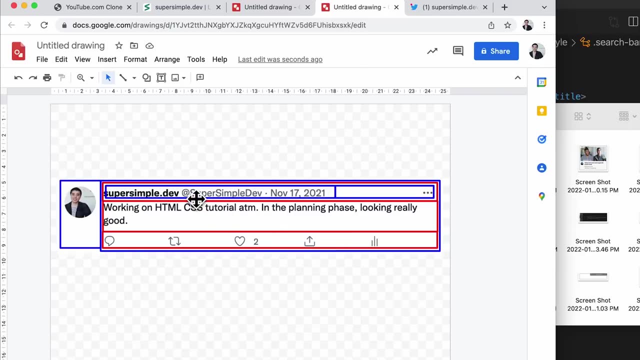 I'm going to break this down further into a horizontal layout inside here. And finally, we can break this part down further into a horizontal layout. So let's copy this again And paste it here, And I'm just going to create a few of them. 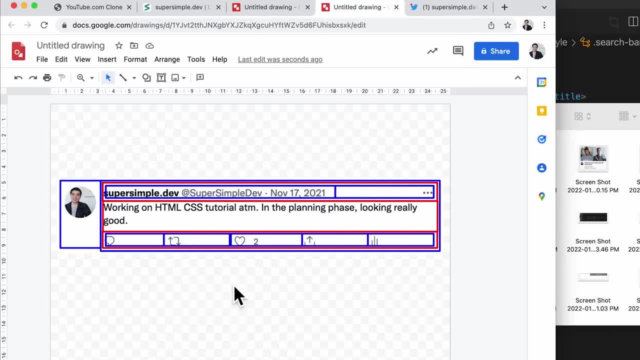 Like this. So, just like that, we broke down this design into a combination of vertical and horizontal layouts using the nested layouts technique. So now that we have a good understanding of how this works, we're going to learn how to recreate this using code. 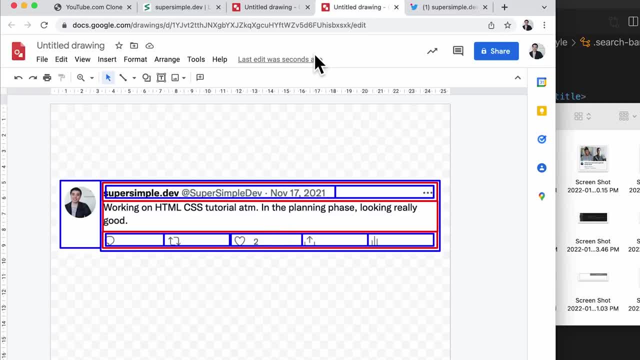 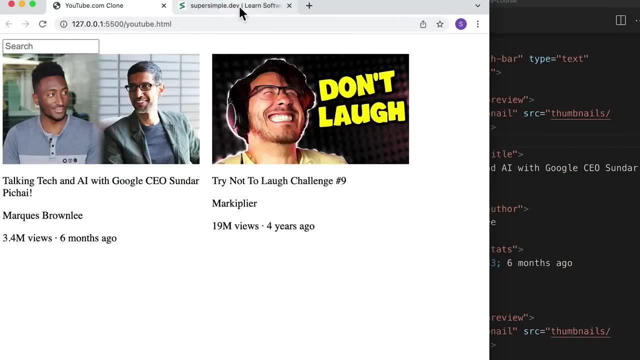 So let's go back into our project. I'm going to delete all these extra tabs here, So we're going to go from something that looks like this to something that looks like our final design here. Now, before we start, we actually need to download this channel profile. 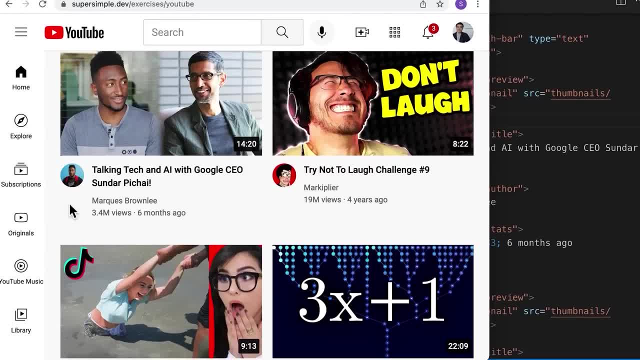 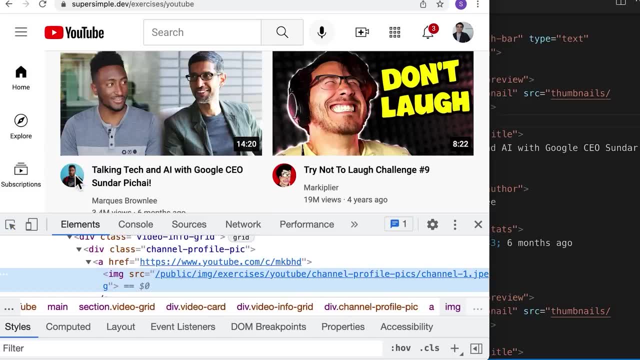 picture. So remember to do that. we can right click and inspect, Click the top left icon here And then click this picture, And we have the URL to download it here. So I'm going to hover over it, scroll down and click. 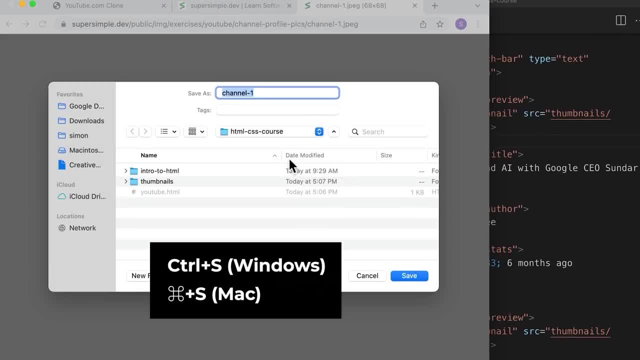 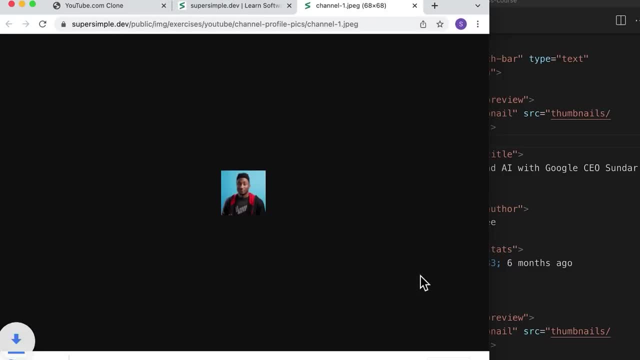 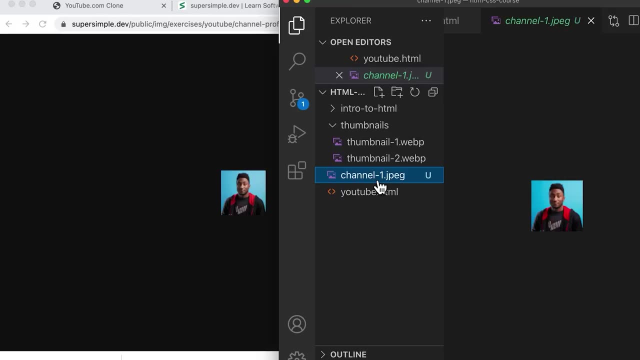 this link Now control s to save, And I'm going to save it in the folder that contains our code, Which is right here And now. this should show up in our code editor. So I'm actually going to create a folder to store all of these channel. 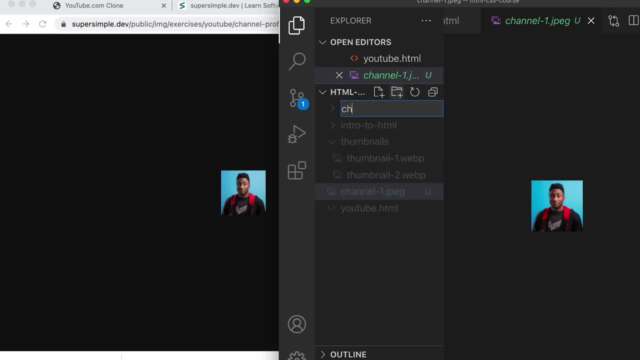 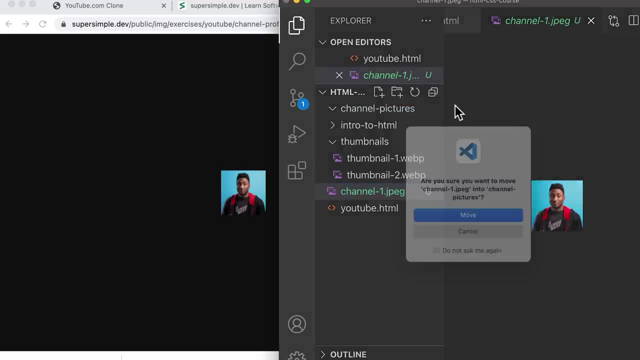 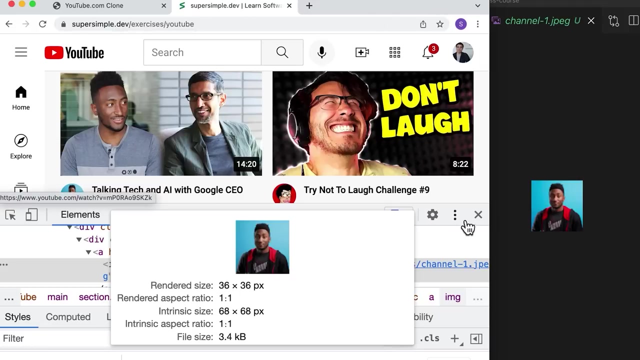 profile pictures, since we're going to have a lot of them, So I'm going to call this channel-pictures And I'll put this in there. Now we're ready to create our layouts, So let's go back to our final design. 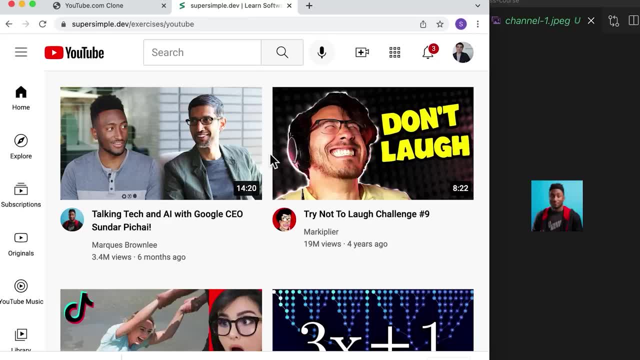 And see what kind of layouts we have. So we're going to have a vertical layout. It's one and two, So two rows, And then, inside the second row, we're going to have a horizontal layout, Which is one and two. Now, inside. 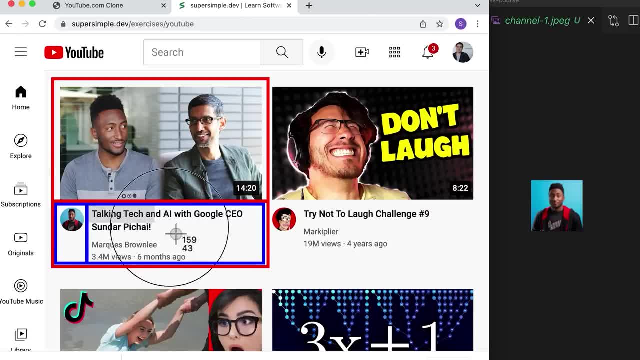 the second horizontal layout. we're going to have a vertical layout: One, two and three. So that's how we're going to break down this design And again, don't worry about the video time here. We're going to recreate this later in the course. 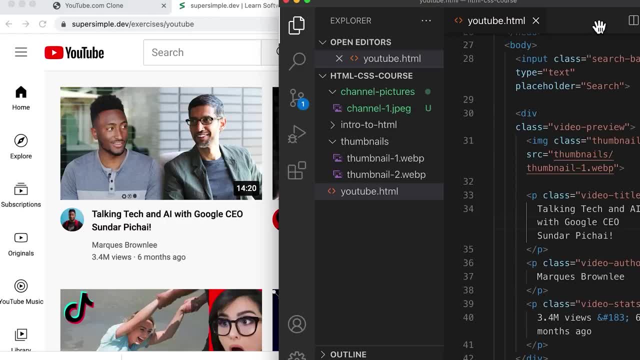 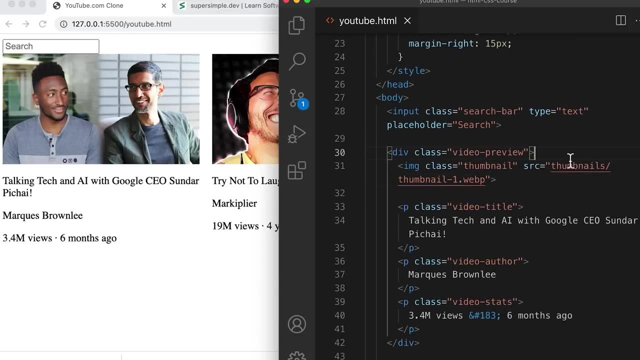 Let's go into our code and we're going to implement that. So make sure that we have our project open on the left here And we're going to start by creating some vertical layouts To create a vertical layout we're going to create. 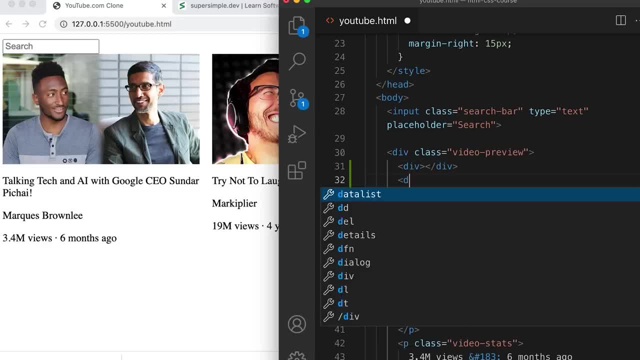 two divs. So this is going to be our vertical layout. Now, remember that divs are block elements by default, So they're going to take up the entire line and appear one on top of another, And that's exactly what we want for a vertical layout. 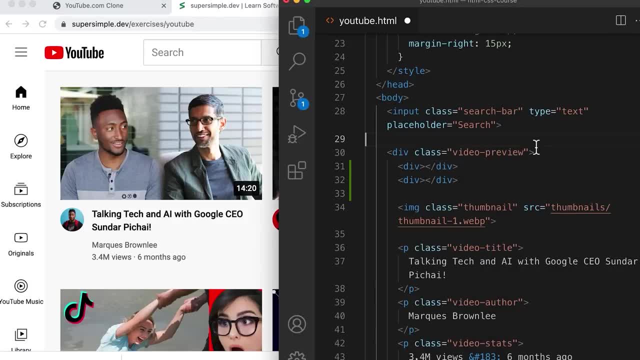 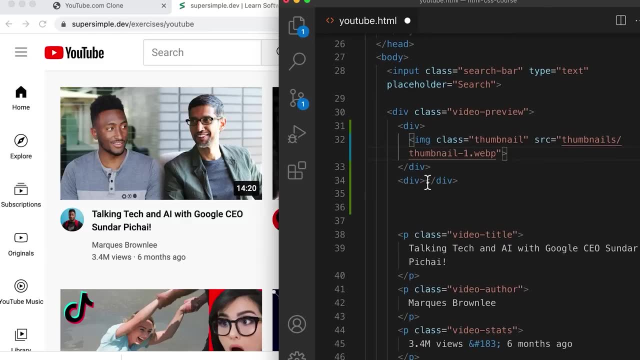 So let's look at our design here. We have the image in the first row, So I'm going to move this up, Cut and paste, And then in the second row, we have everything else, So I'm going to put everything here. 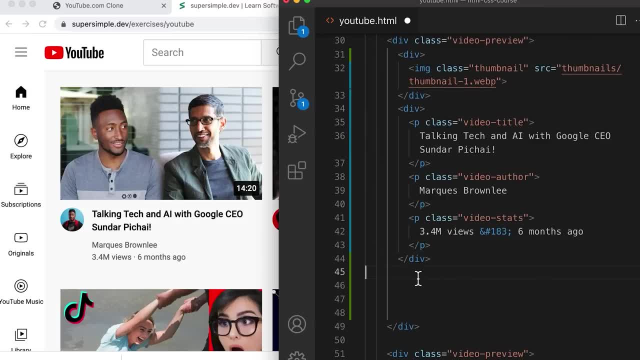 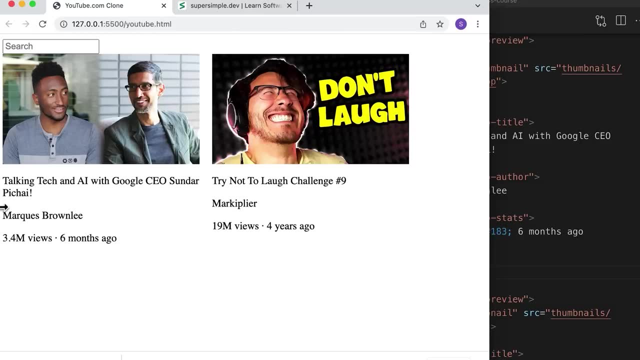 in the second row. So cut and paste. Let's save it and refresh. Now we're going to create a horizontal layout down here. One column is going to have the channel profile picture and the other column is going to have the text. 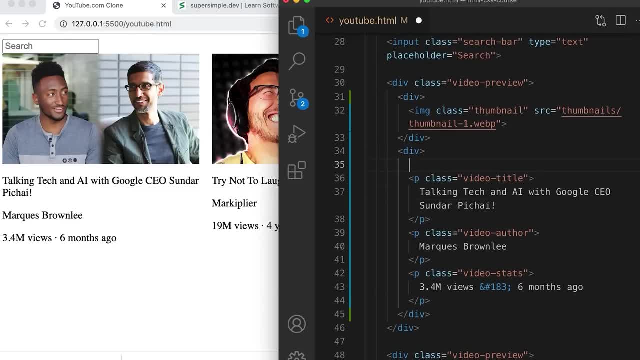 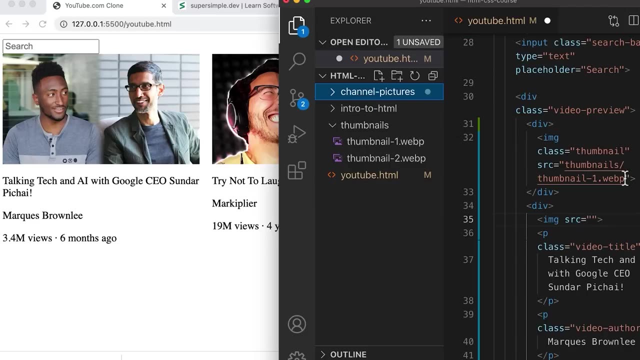 Let's create the channel profile picture first. We're going to create an image element. We're going to give it the source of the picture that we downloaded in the beginning. So that picture is in this folder. So we're going to go into this folder. 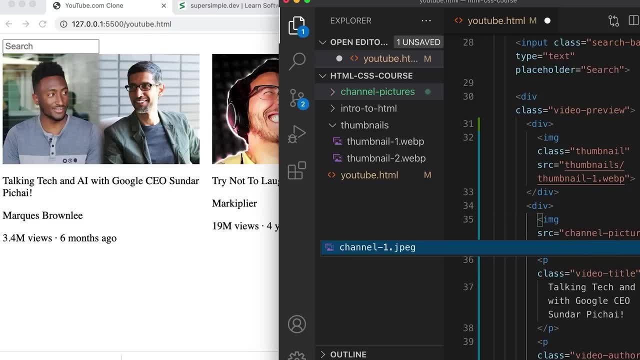 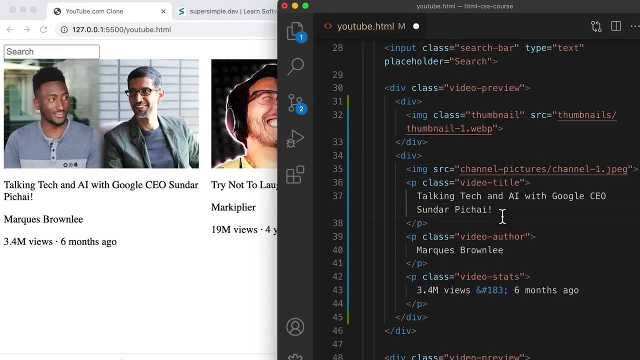 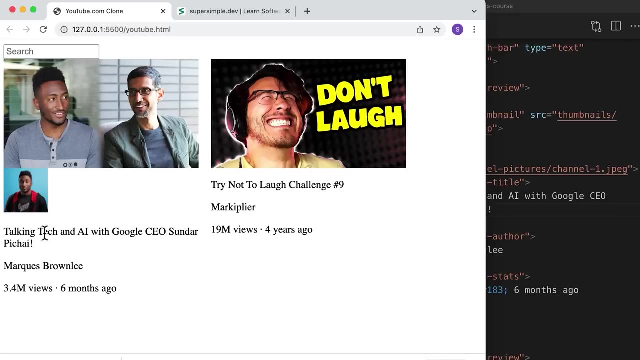 first, which is channel-pictures, and then remember to have a slash to go into that folder, and then channel1.jpg, Save it And now, if we look at our current website, the image is actually in its own row, And that's because 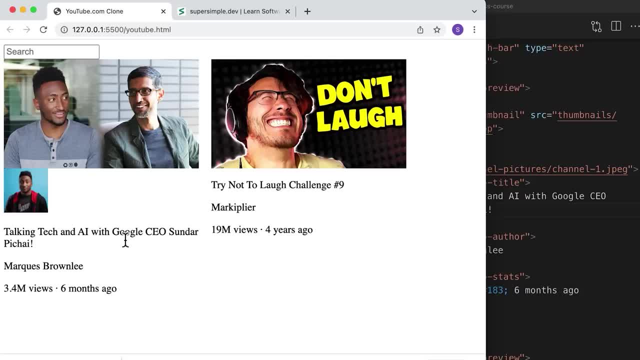 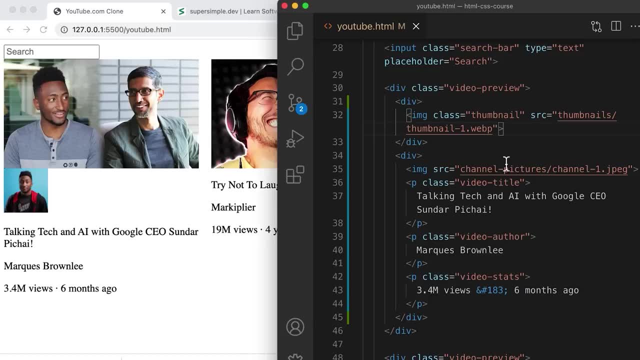 the paragraph is a block element, so it has to appear on its own line. We're going to change this by creating a horizontal layout like 1 and 2.. So to do that, we're going to create two divs. Here's one div. 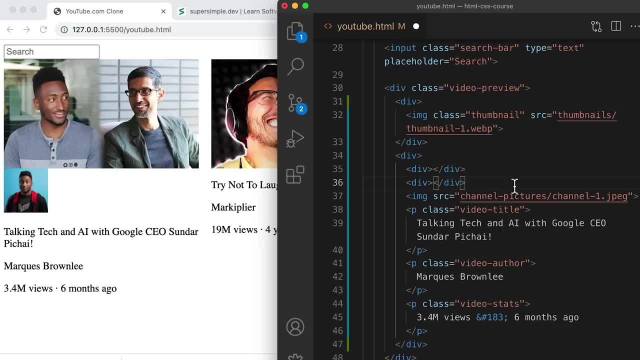 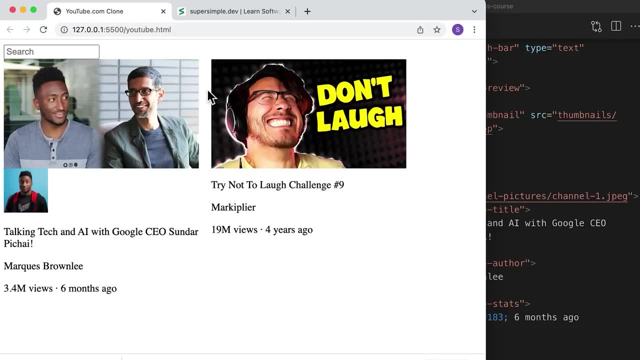 and here is another div. Now, the difference here is that we're going to make these divs inline block elements. So remember that inline block is what allows elements to appear beside each other like this, While block elements force the element to take up the entire line, so they will. 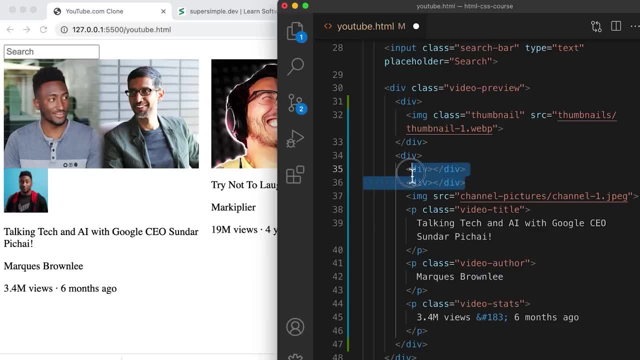 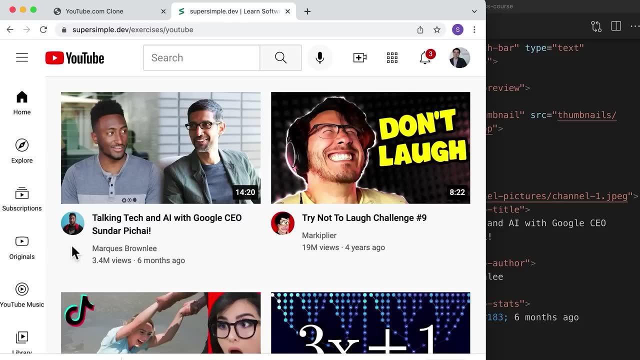 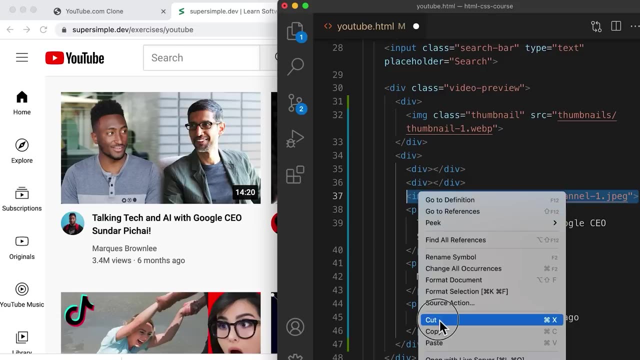 appear vertically. So we're going to make these two divs inline block elements to create our horizontal layout. Let's reference our design first. In the first column we have the channel profile picture, So I'm just going to move this into the first div here. 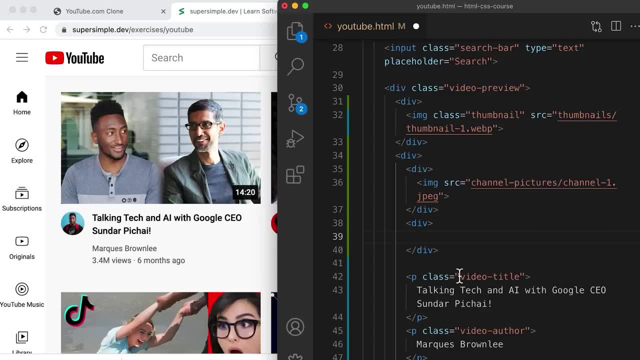 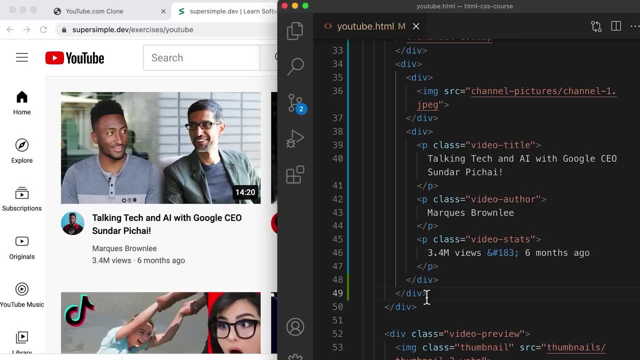 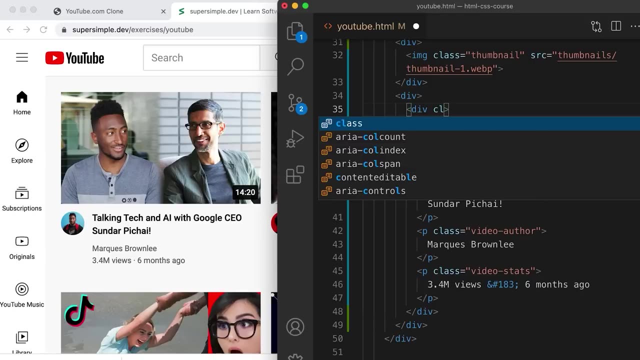 And then in the second div we have all the text. So I'm going to move all of the text here, Cut and paste. Now let's make these divs inline blocks so that they appear next to each other. I'm going to give a class so that. 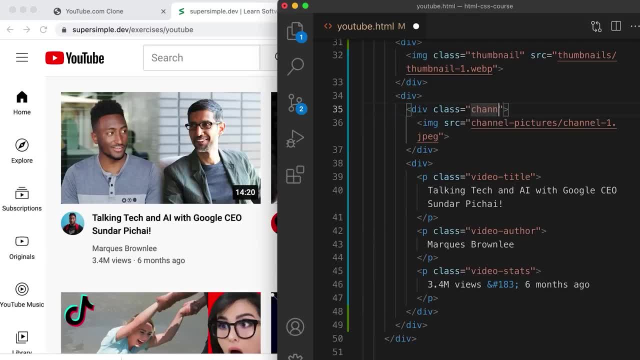 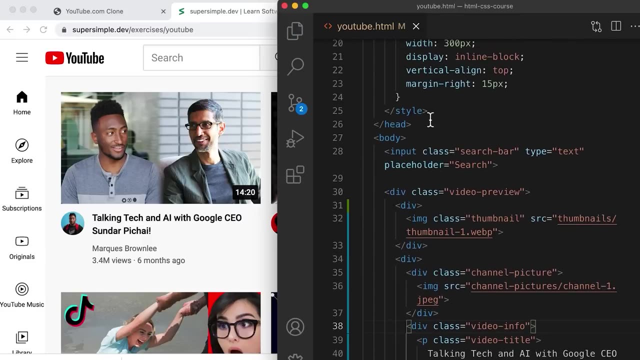 we can target it with CSS. Let's call this the channel picture. And then we're also going to give a class to this div so that we can target it. Let's call this the video-info. And now in our CSS, we're going to make: 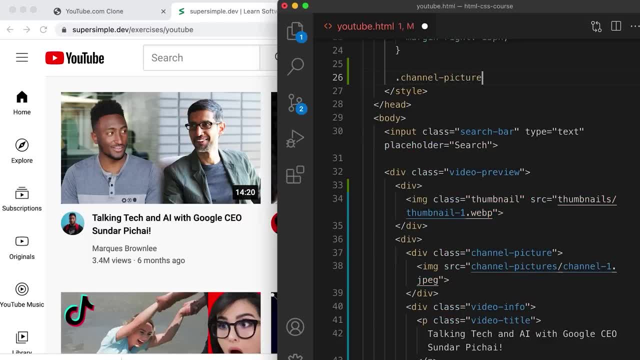 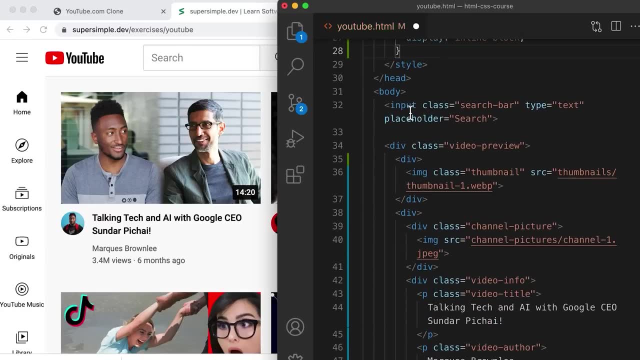 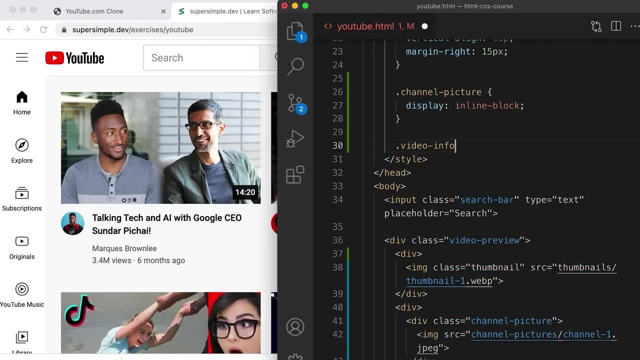 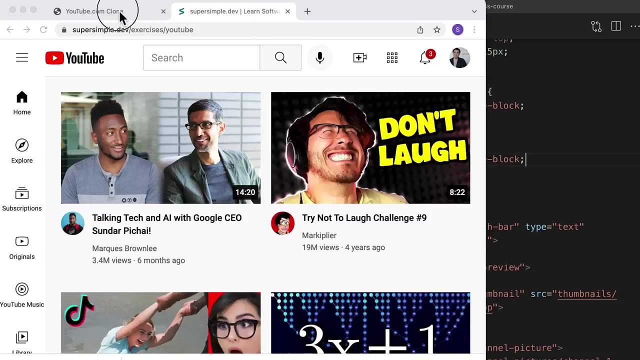 the channel picture picture display inline-block And we're also going to make the video info display inline block, So the two divs appear next to each other. Video-info Display inline-block. Save it and refresh Now you'll notice that they're still. 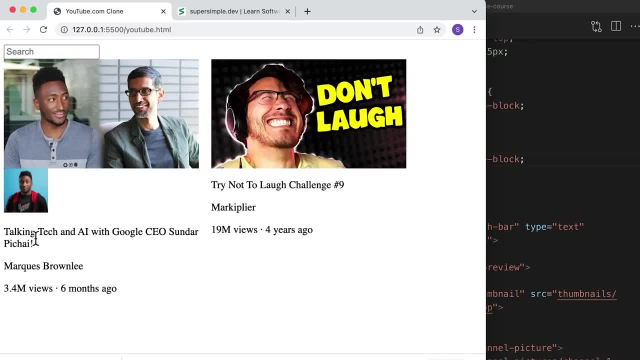 on top of each other, and that's because divs by default have a width of 100%, So we need to decrease the width of these two divs so that they appear next to each other. So remember that for the video preview card. so this whole thing. 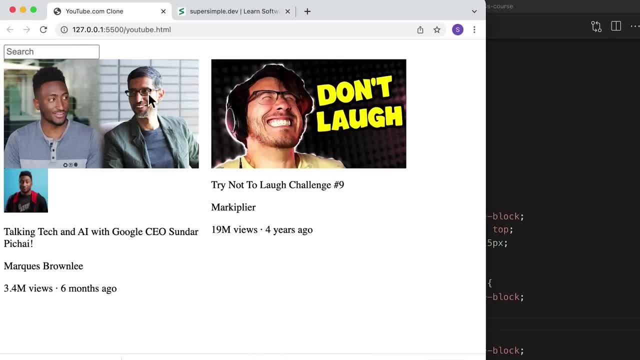 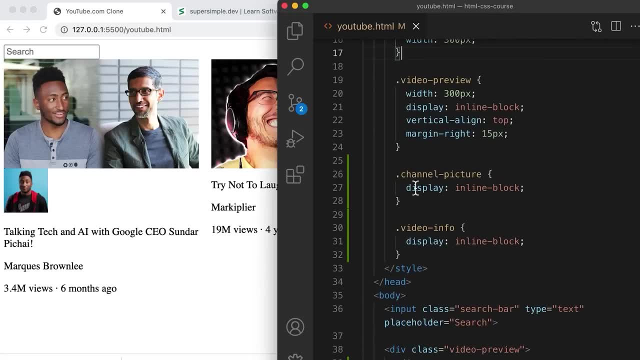 we set the div to 300 pixels And that's how they can appear beside each other. So we're going to do the same thing for our horizontal layout down here. For the channel picture, let's set a width of 50 pixels. 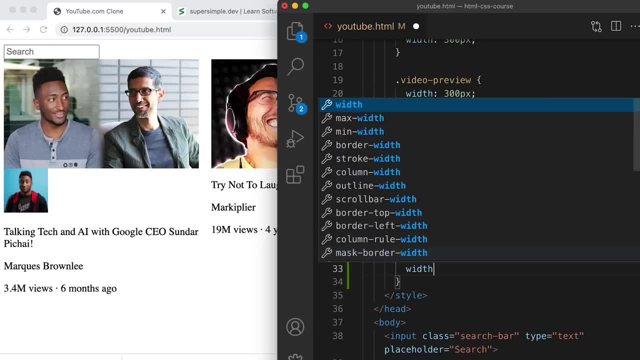 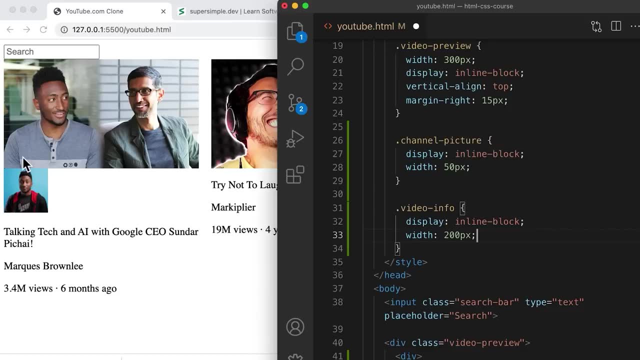 And then for the video info, we're going to set a width to 200 pixels. So this is the first column of our horizontal layout. It's going to take up 50 pixels like this. And then this is the second column. 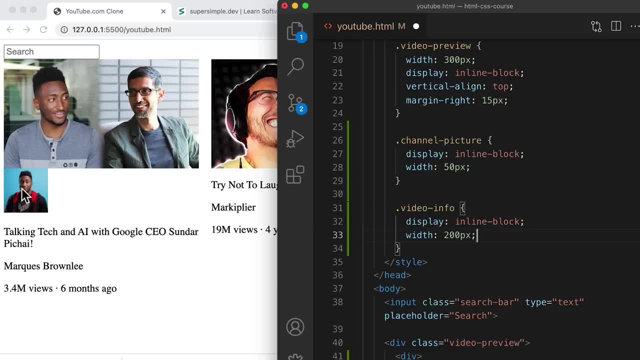 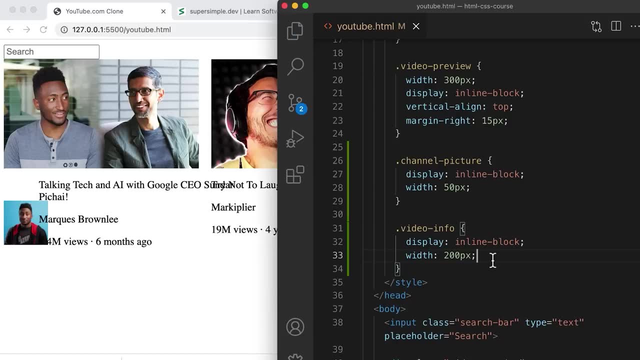 It's going to take up 200 pixels. It's going to appear beside the first column because both of them are display inline block. So let's save this And you'll notice it looks really weird. So let's look at our code and see what the problem is. 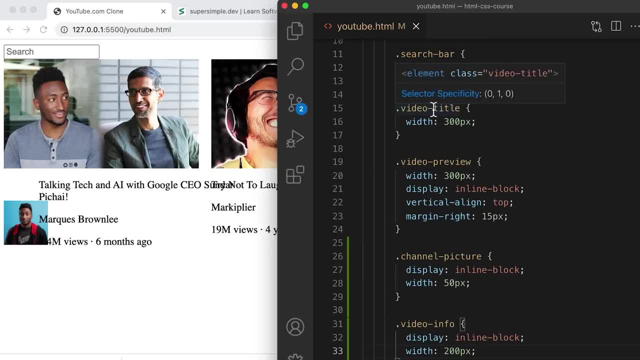 I'm going to scroll up here and you'll notice that we set the width of the video title, which is this text, to 300.. So we're forcing it to overflow here, And that's not what we want. So we just need to remove. 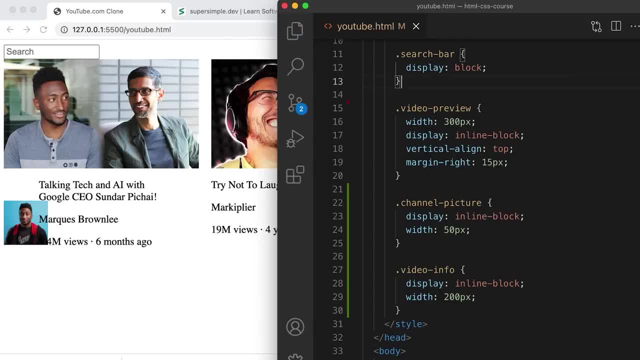 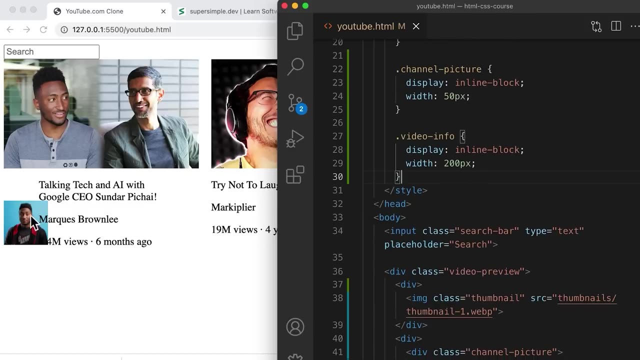 this and not force the width. So if we don't force a width of 300, the paragraph will just take up the entire space of the container, which is 200 pixels. Now, the second thing we notice is that this image is overflowing. 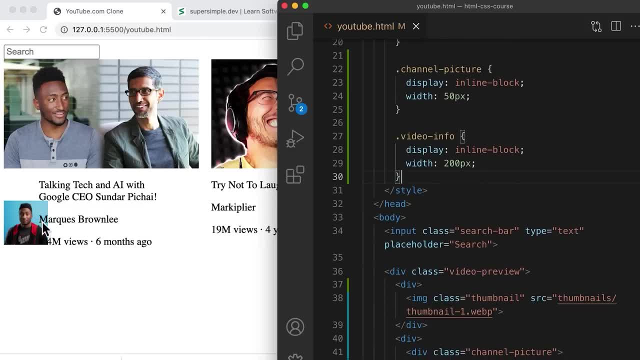 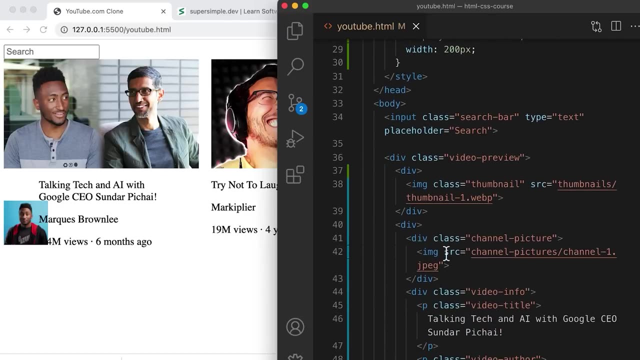 And that's because images, by default, they overflow. So they keep their original dimensions, so they keep their original size, and that causes them to overflow. So we want to resize this image so that it only takes up 50 pixels. Let's go ahead and do that right now. 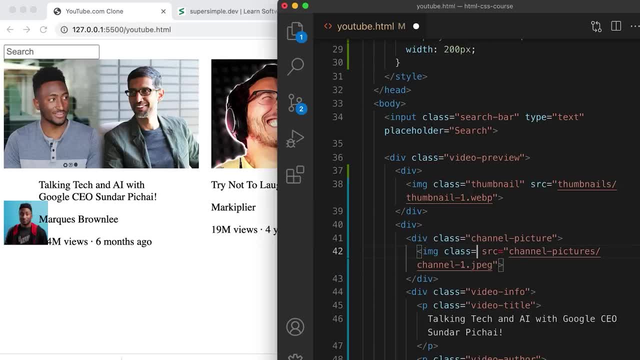 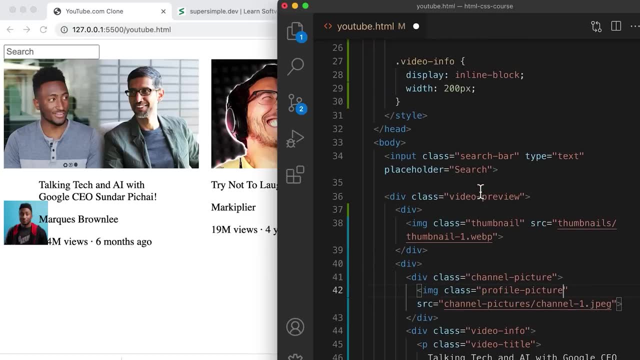 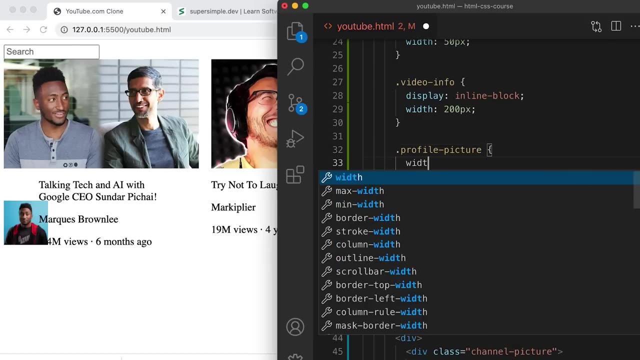 Let's give it a class so that we can resize it, And I'm going to call this the profile-picture, And then I'll scroll up here profile-picture, And then I'm going to resize the width to 50 pixels So that it fits exactly this column. 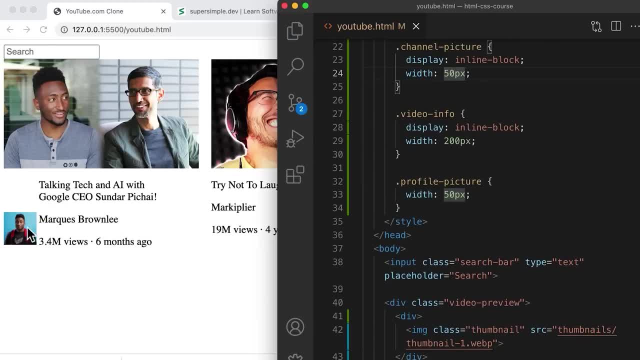 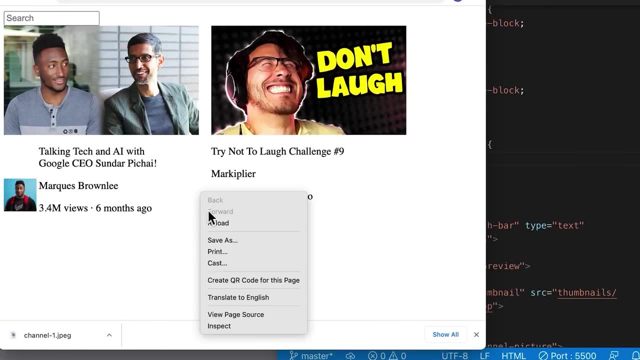 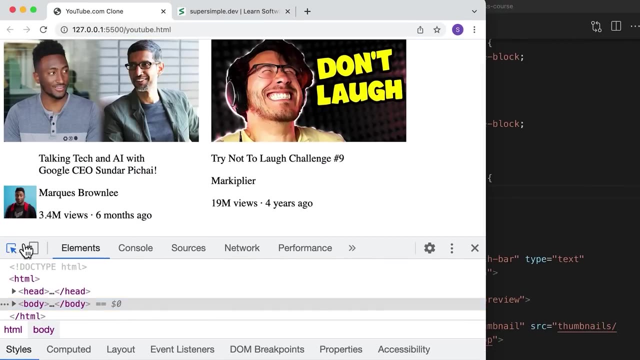 I'm going to save it And now that looks pretty good. We can actually see the layout in our browser by right-clicking inspect and finding this HTML, So I can click this top left icon and just click this picture, So I'll show you what it looks like. 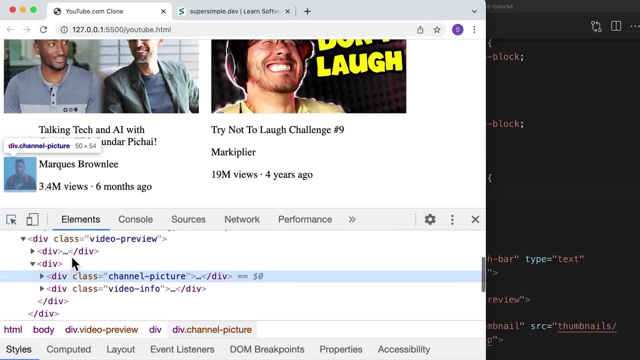 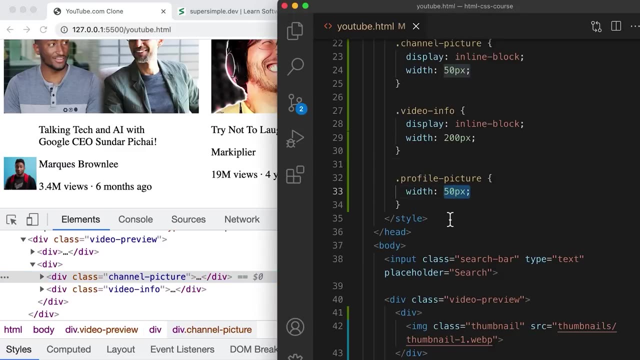 in the HTML. So here we have a vertical layout, so 1 and 2.. And then here we have a horizontal layout: 1 and 2.. Now a better way to do this is actually to set this to 100%. So this means the image. 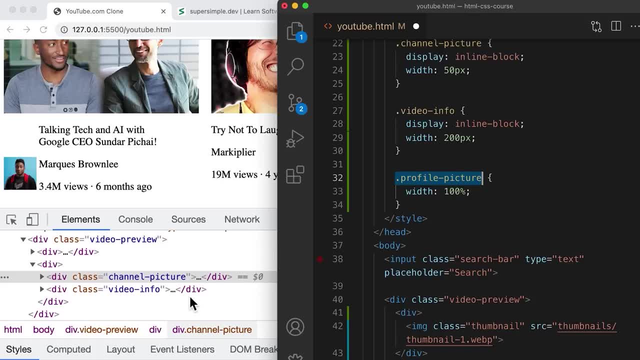 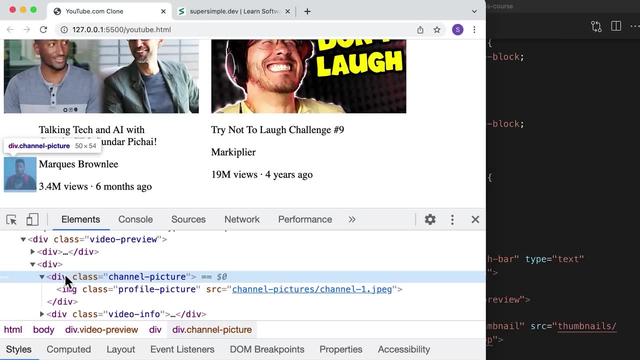 will take up the entire space of its container. So if we look at our HTML, this image is inside this container. If we set it to 100%, it'll take up the space in the container, Which is basically the 50 pixels that we have here. 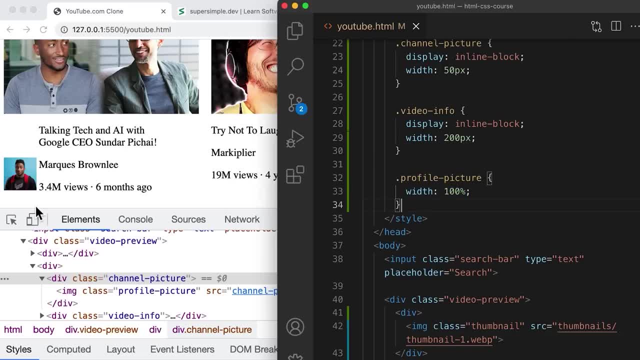 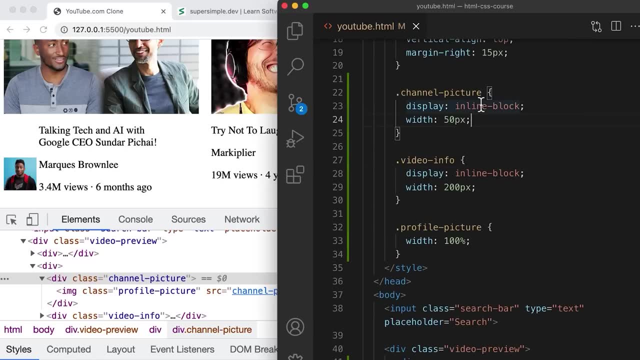 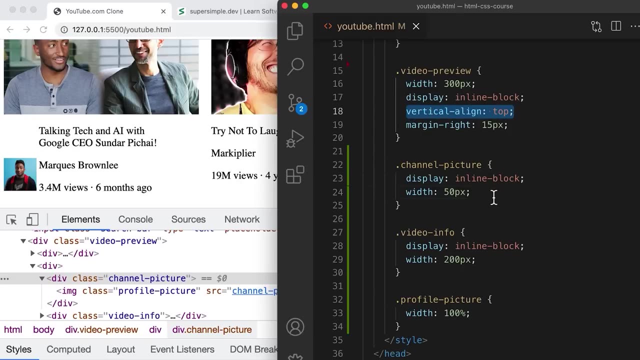 Let's save it. Next, remember that we've seen this problem before: They're not aligned. So we're going to align this inline block element to the top. To do that, we're going to use this property here- vertical align top- that we've seen before. 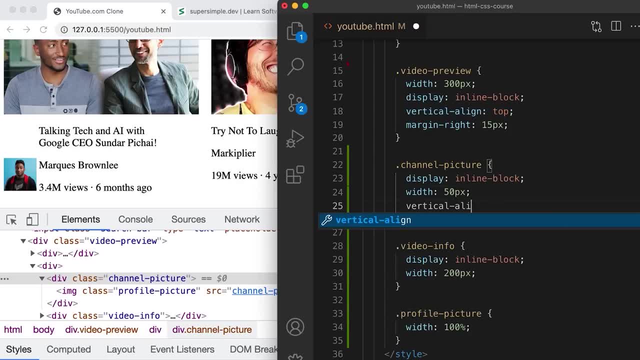 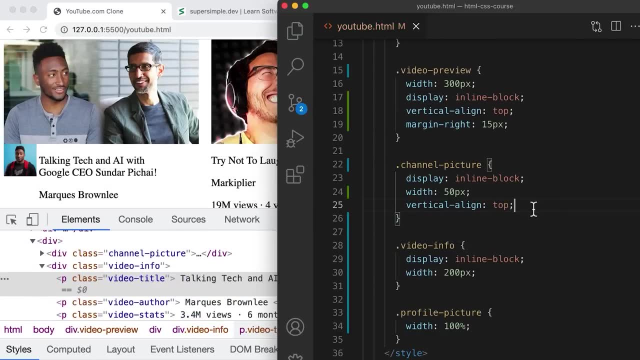 So vertical dash, align top, Save it Alright. so we're almost there, but notice that these two aren't aligned. This paragraph has some margin at the top. Remember that paragraphs by default come with margin at the top and at the bottom. 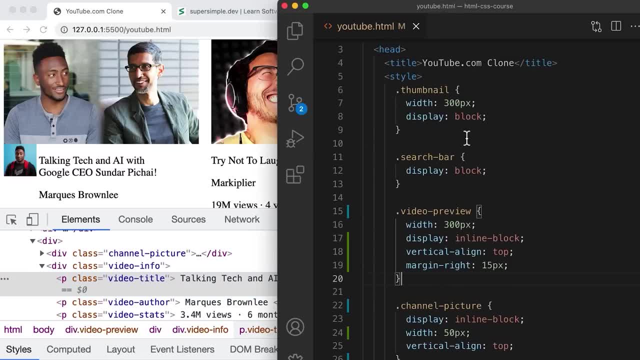 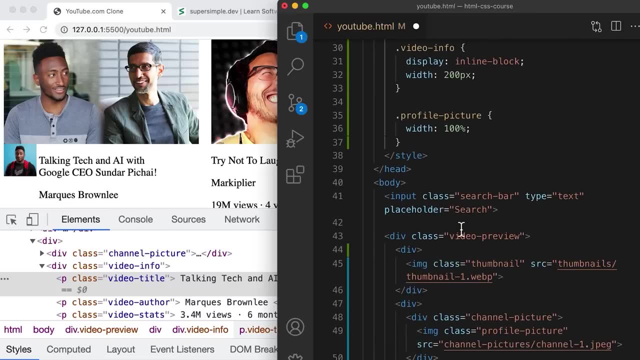 So we're going to go into our code and we're going to get rid of this margin at the top, So let's scroll up. Oh, so we actually deleted that style, so let's create a new style. here We're going to target the 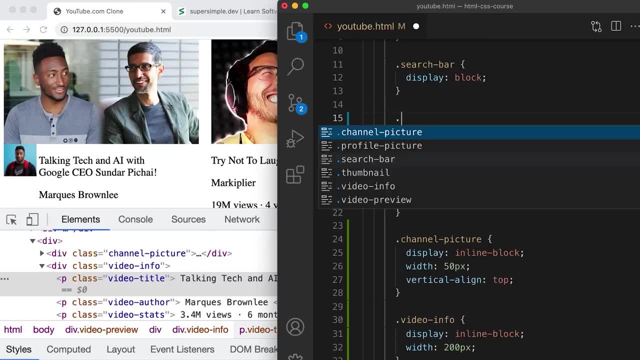 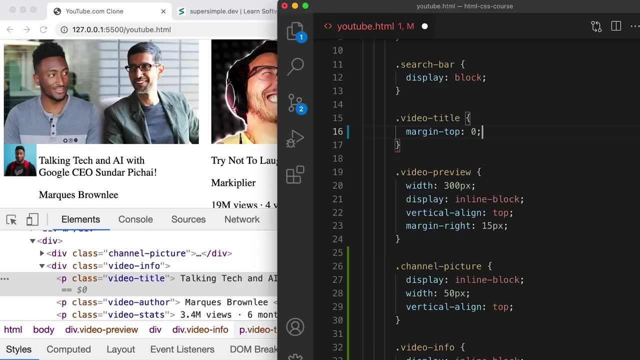 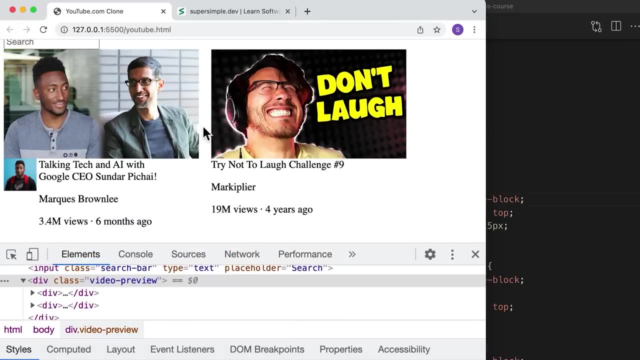 video dash title. We're going to target the class video dash title, Set the margin dash top zero And that's going to eliminate the space up here. So I'm going to pause here because we've actually created the nested layout that we need. 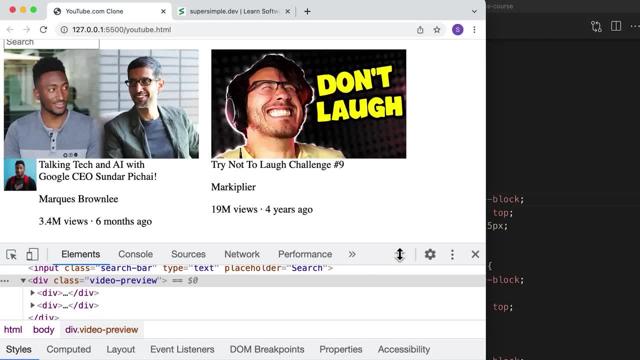 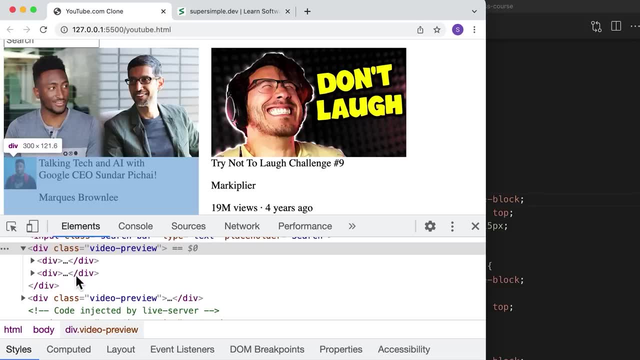 Let's look into our HTML in the dev tools And if we look at this video preview, we have a vertical layout one and two. Inside the vertical layout we have a horizontal layout- one and two, And then inside our horizontal layout we have another vertical. 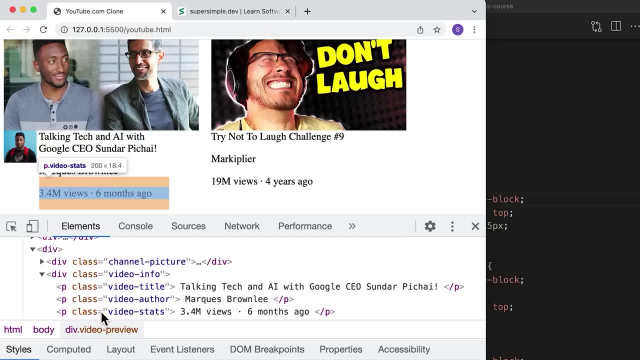 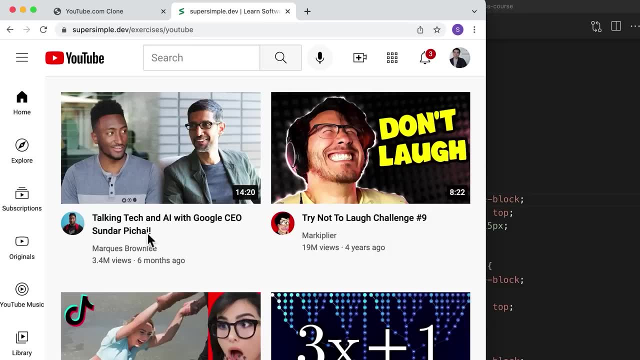 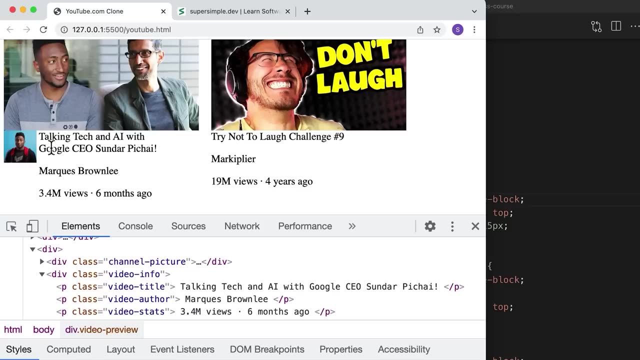 layout one, two, three. So that's a practical example of using the nested layout technique to create a layout that's a similar shape to this. The only thing that's left to do is to style our website with CSS, one by one, until it looks. 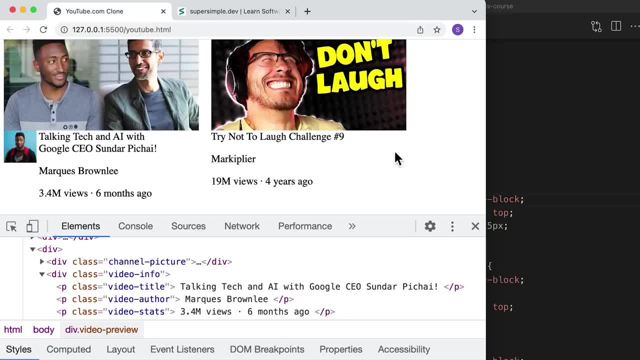 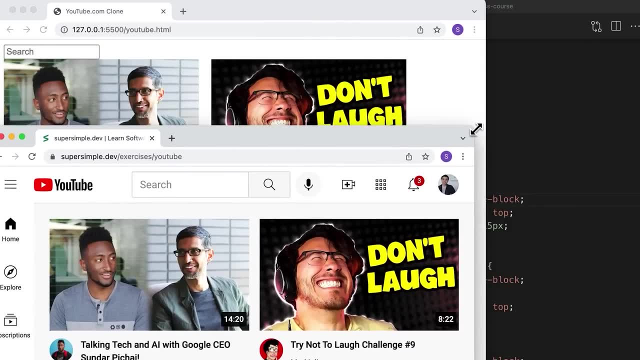 like this. So we're going to do that right now. So let's go into our code and we're going to style these elements one by one. So I'm actually going to move this down here so that I can see it a lot easier. 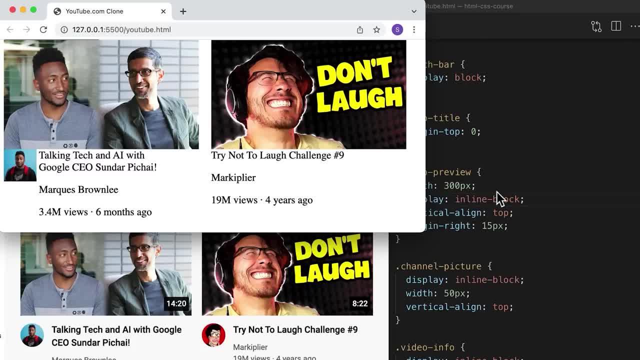 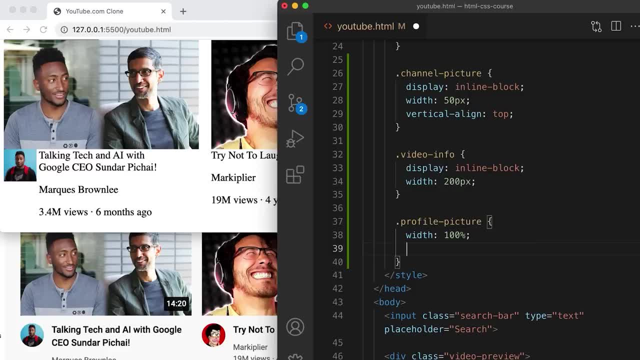 So the first thing I notice is that the image is round. So remember, to create a round image or round anything, we're going to use rounded corners, So we're going to set the border dash radius to, let's say, 20 pixels. 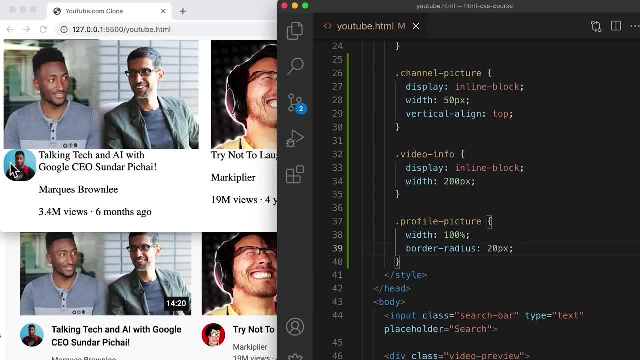 Save it. Okay. so we have rounded corners and it's getting more round, but it's not a full circle yet, So let's set this to maybe 50 pixels, Okay. So now it looks a little too big. Let's set the width to something like: 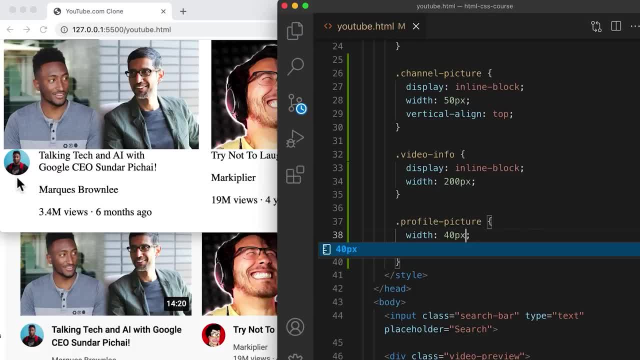 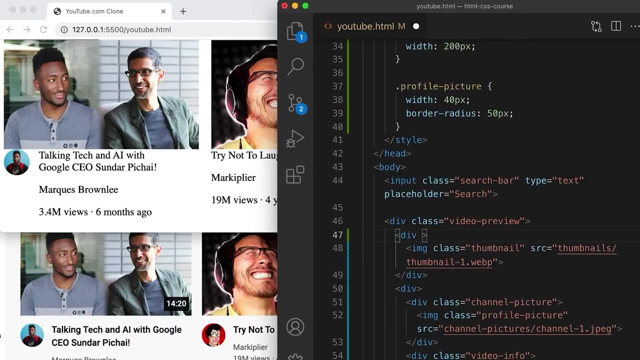 40 pixels. I think that looks pretty close and we can always change it later. Next, there's some spacing between the first row and the second row, So let's go in here. We're going to set a class here. call this the. 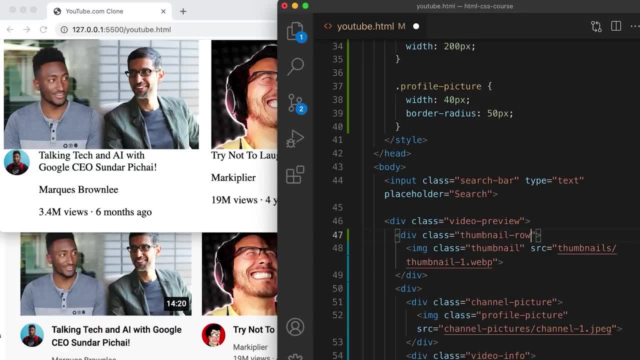 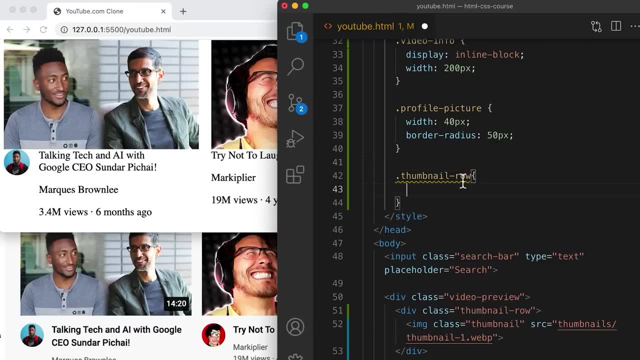 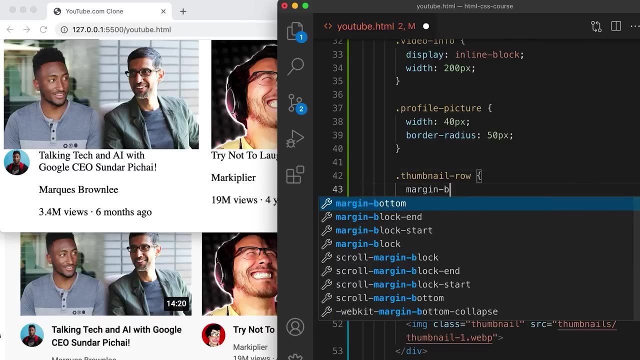 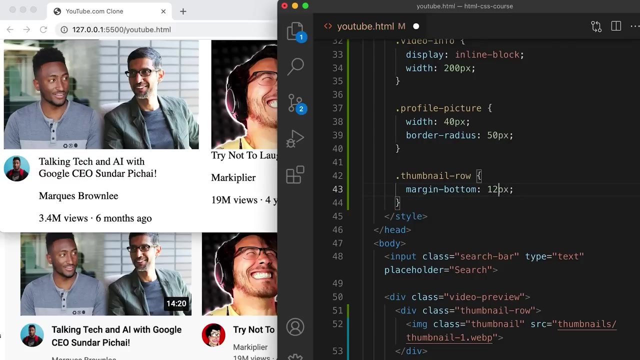 thumbnail dash row. And then we're going to style this thumbnail row And remember to add spacing to the bottom. we add margin dash bottom And let's add a margin of maybe 10 pixels. Save it, Okay. maybe 12 pixels, Okay. 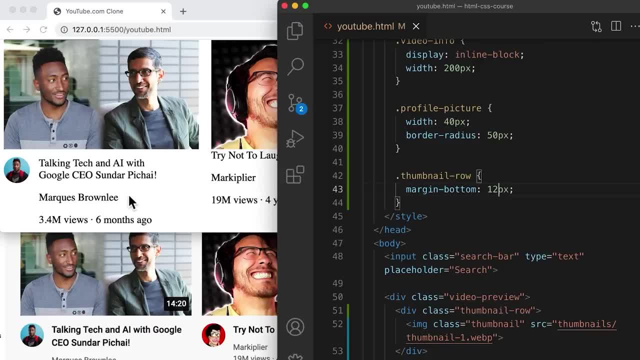 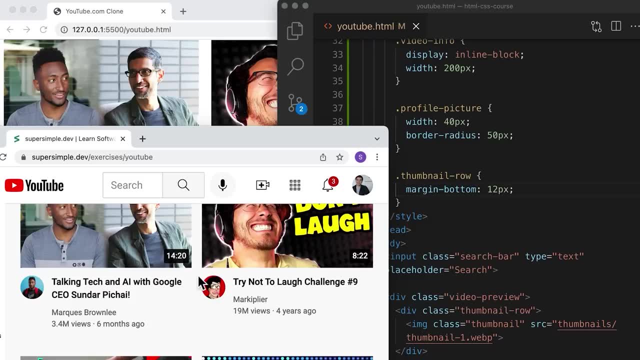 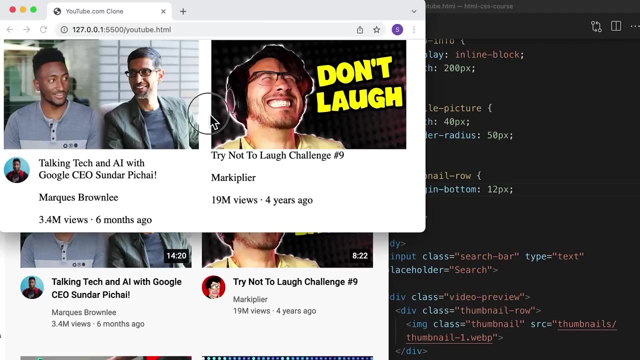 so that looks good enough And finally, we can style the text. So this YouTube project is actually using the Google font called Roboto. We learned in a previous lesson how to load Google fonts and, in particular, how to load Roboto, So we're going to do that again. 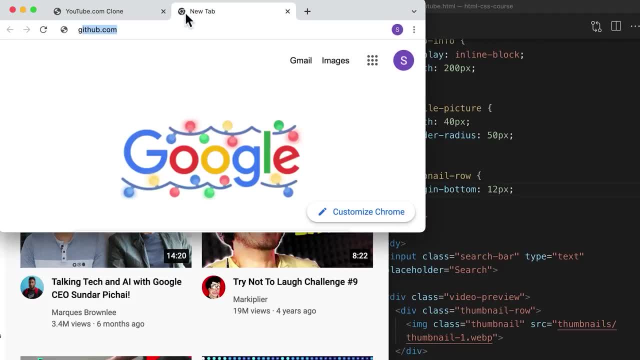 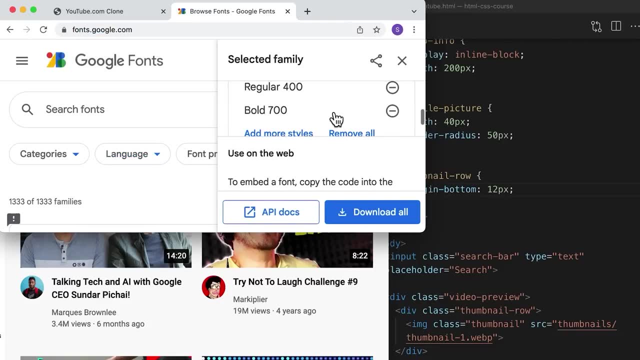 Let's go to a new tab. We're going to search for Google fonts And we're going to load Roboto onto our page. So if you don't have this here, this is from my previous session. We can actually search for Roboto. 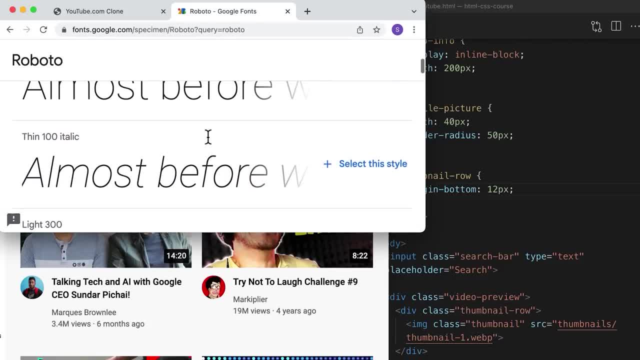 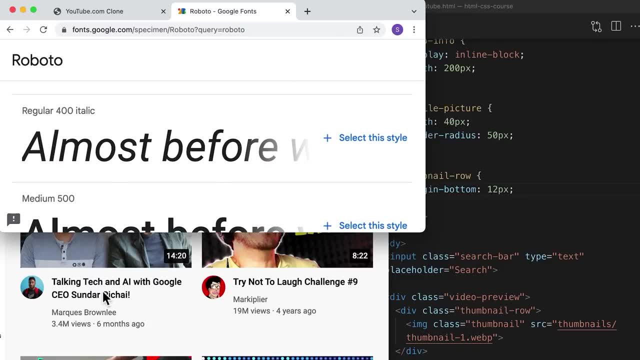 And then just open it here And then we select the styles that we want. So I'm going to get the regular style, And then this seems like a bolded font, so I'm going to get the medium font and the bold font, just in case. 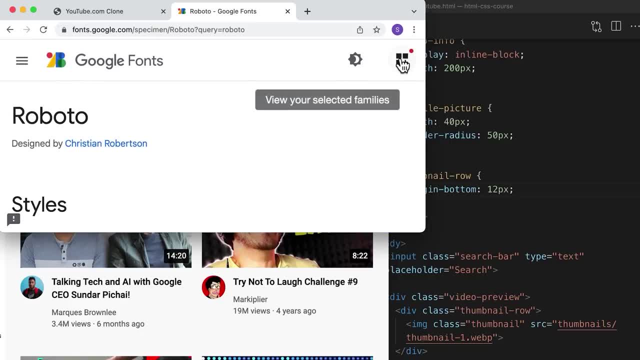 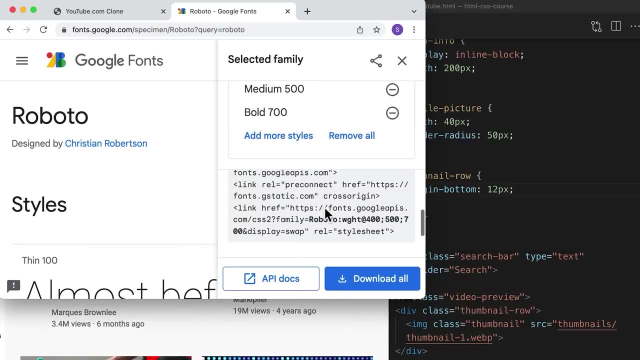 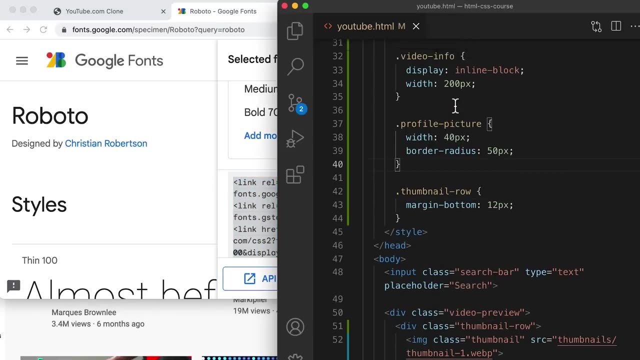 So I'm going to go up to see the styles I selected, And then that looks pretty good And Google will give me the code that I need to load this onto my website. I'm going to copy this and just paste it into my head section. 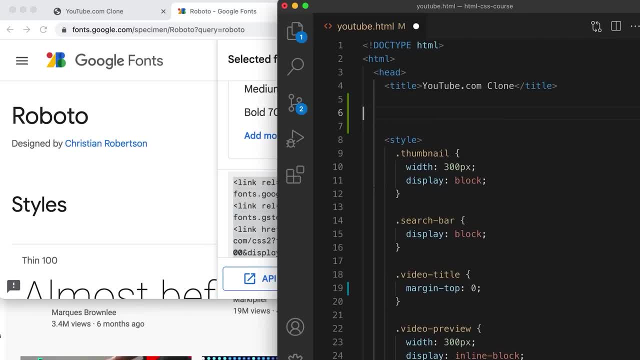 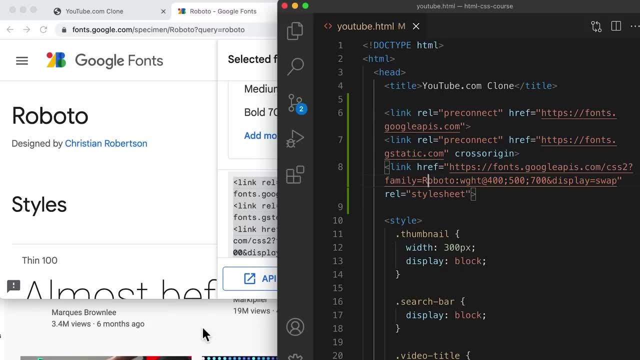 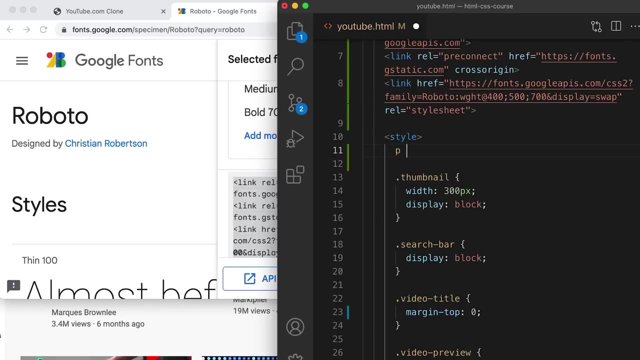 So right in between here, Alright. So now I loaded the Roboto font And we're going to use it in our page. So we're going to target all paragraphs And we're going to change their font family to Roboto And we're also going to 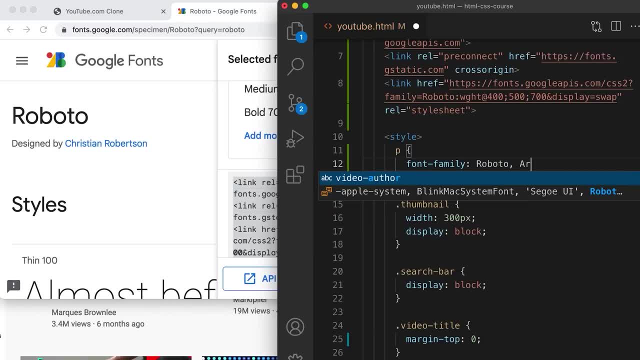 use a backup font with this comma of Arial. So this syntax here with a comma is called a font stack. This basically lets us set up a backup font. If, for whatever reason, Roboto fails to load from Google, then it will fall back to our backup font. 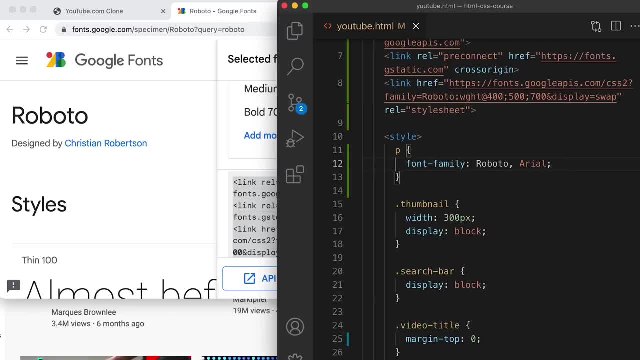 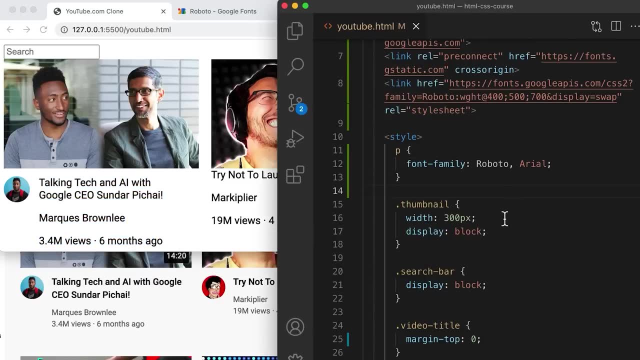 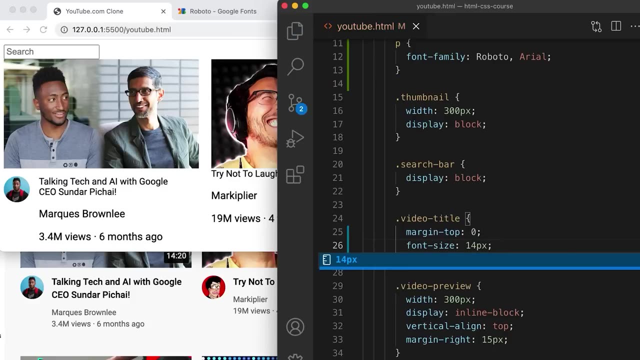 which is Arial. Let's save it. Next I'm going to change the size of the font, So let's change the video title to maybe 14 pixels. Save it. Okay, I think that looks pretty good. Next I'm going to 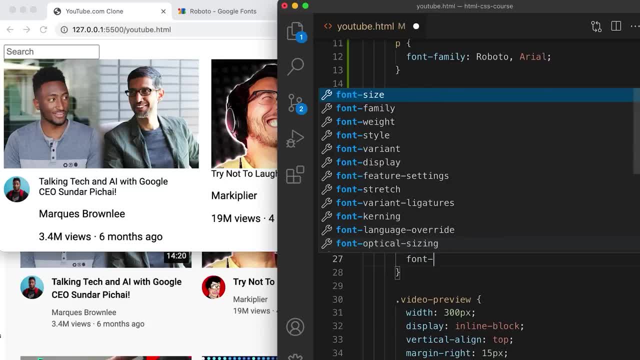 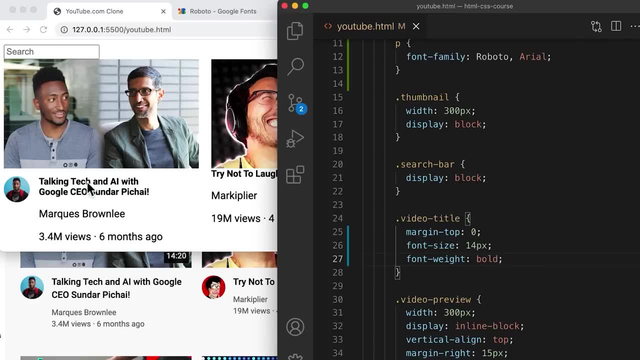 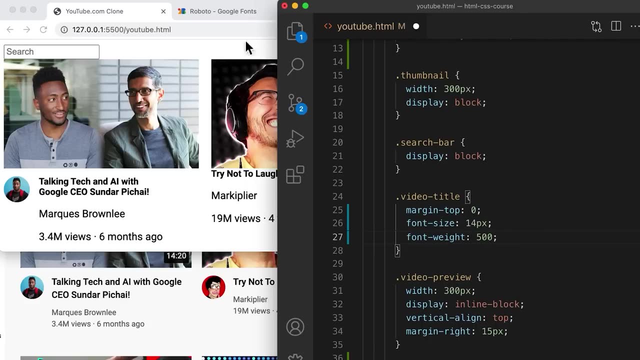 make it bold. So font-weight bold- Save it. So this looks like it's a little bit too bold compared to this font, So I'm actually going to change this value to 500.. So, if you recall, we actually selected three styles. 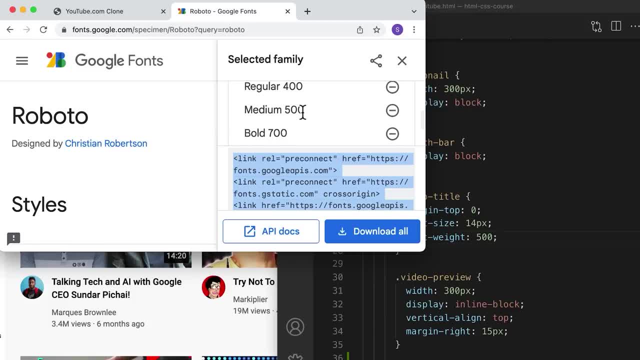 of fonts: The regular 400,, medium 500, and bold 700.. So when we set the font-weight to bold, it actually corresponds to a number which is 700.. A regular font-weight is 400, and a semi-bold. 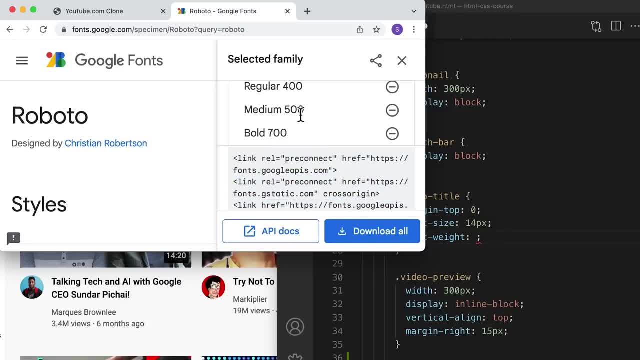 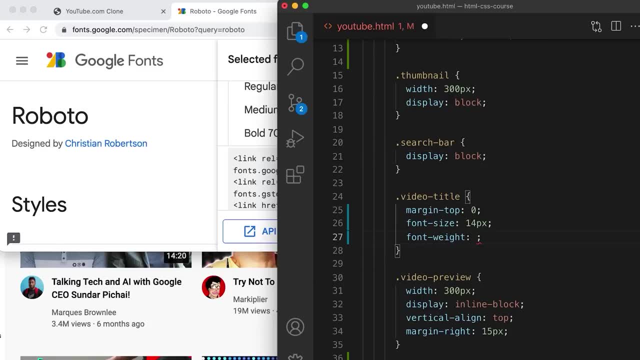 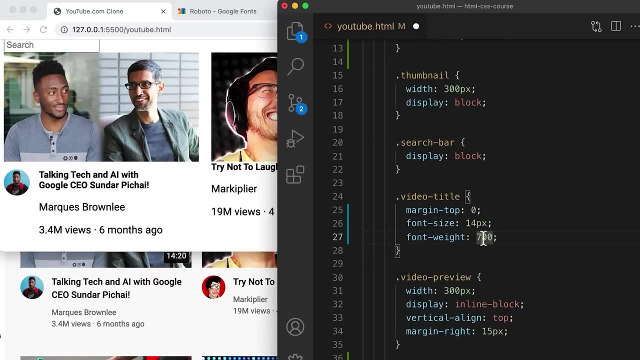 is 500. So usually we use the number value because it's a little more precise. So usually, instead of typing font-weight bold, we would use font-weight 700.. In our case, our font is a little too bold, so we're going to decrease this to. 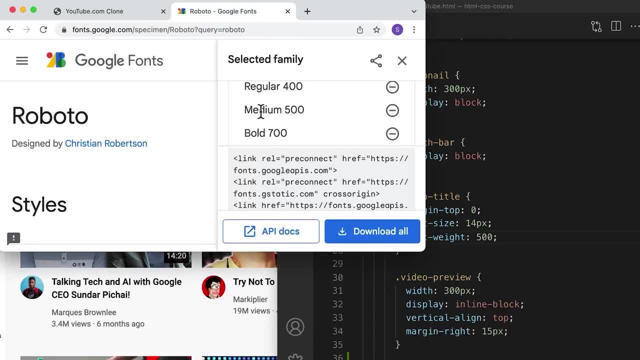 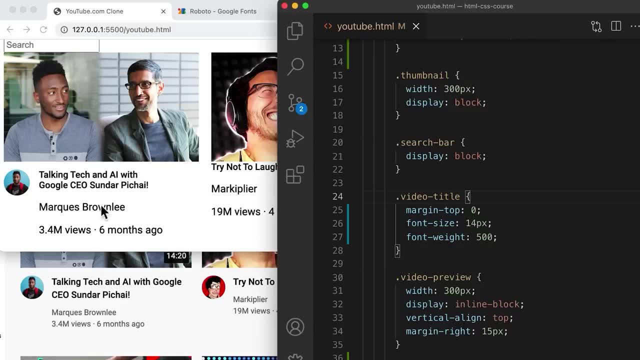 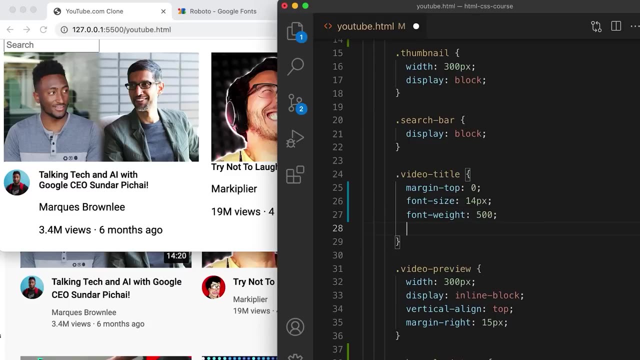 500.. Which is the medium size that we picked on Google Fonts. So let's save this And that looks pretty close. Next, we're going to change the space between the lines, So remember the property to do that is called line-height. 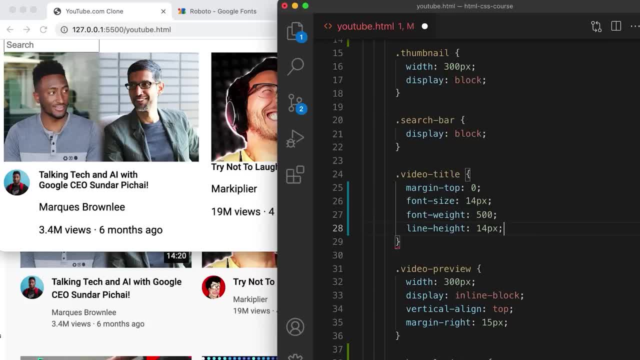 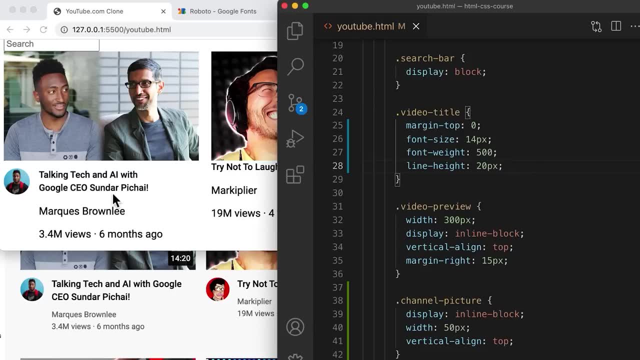 And let's try 14 pixels. That's not enough, Maybe 20 pixels, Alright. so I think that looks pretty good and close to our design. You might notice that the text here is shorter than what we have in the design. You may or may not see this. 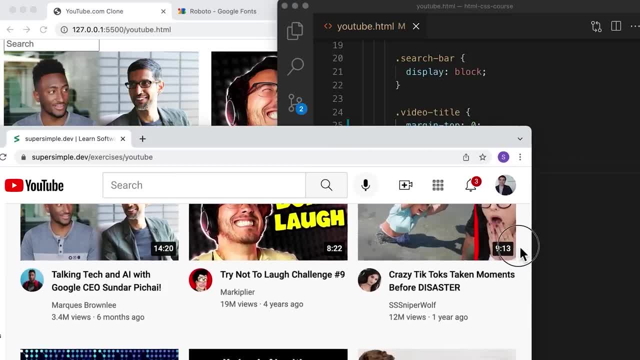 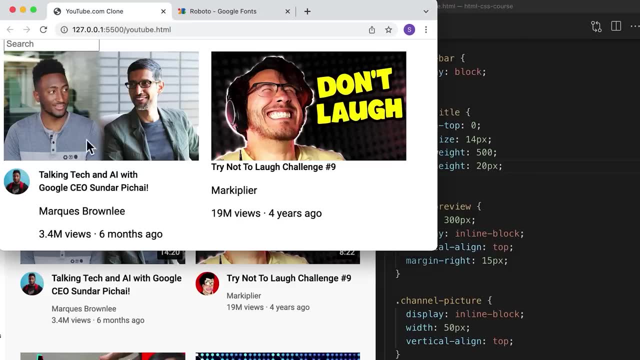 because this text actually depends on the size of the webpage. So depending on how wide your webpage is, the length of this text will change, And in our current website we actually haven't implemented this sizing, So we are going to fix this later. 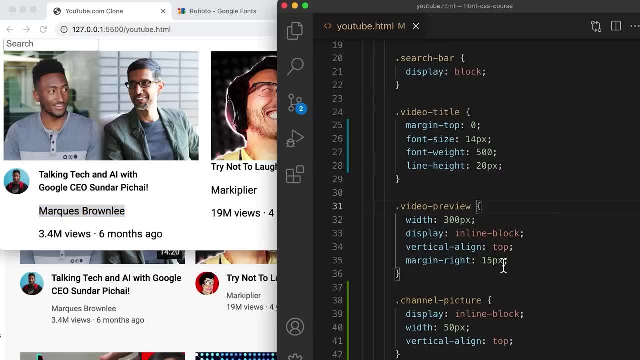 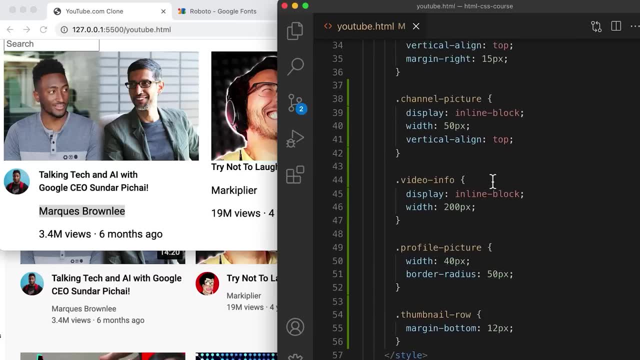 Next, I'm going to style this paragraph, So let's go into our HTML here and look at the class name. so it's the video author, And it looks like we don't have any styles for that yet, So I'm going to write it down here. 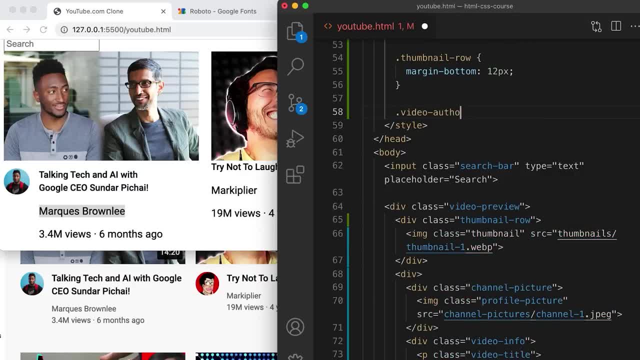 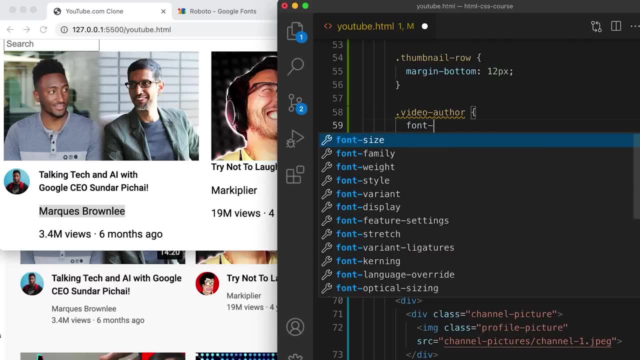 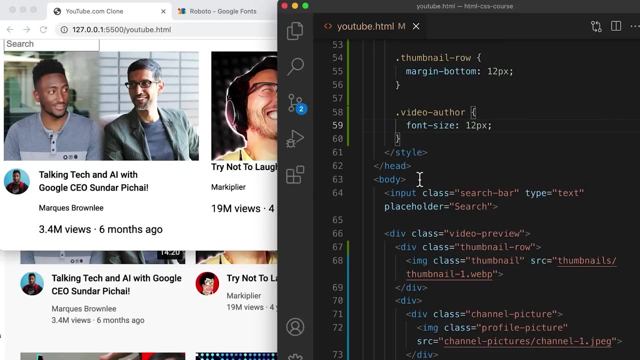 We're going to style the class video-author. The first thing I notice is the font size. so it's a lot smaller Font-size. Let's try 12 pixels. Let's see how that looks. Okay. so I think that looks pretty close. 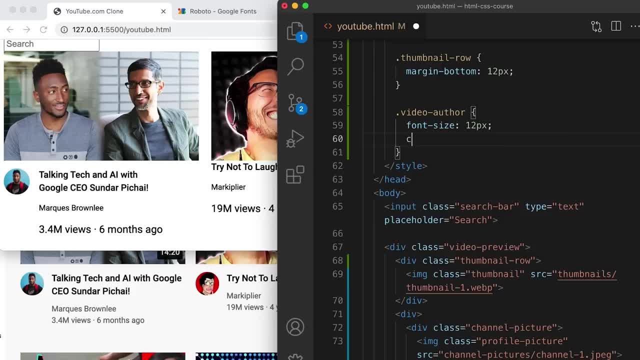 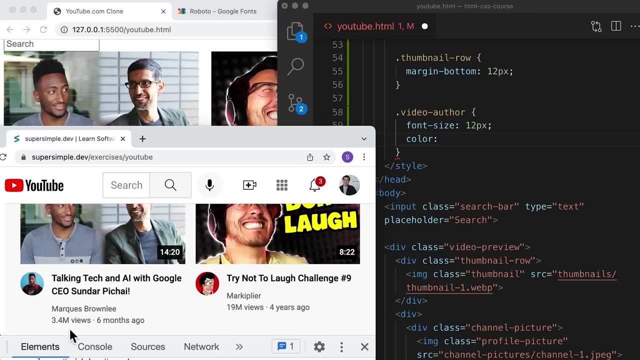 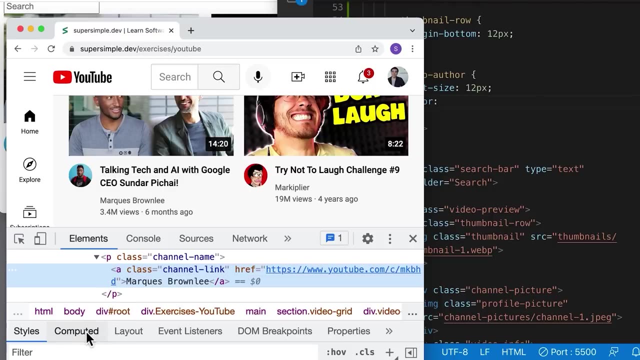 And we're going to change the color Color Now, remember to get an exact color, we can right-click inspect and then click this top left icon. click this text, go to the computer tab and if we scroll down, we should get the text. 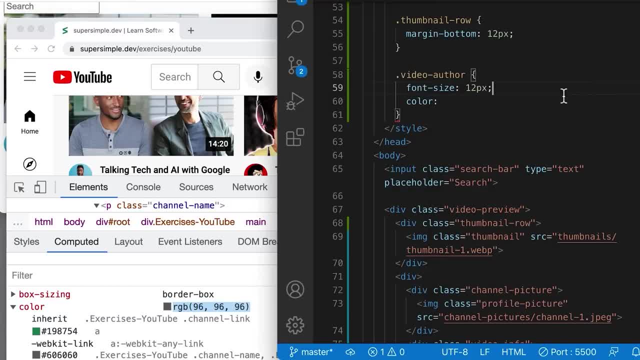 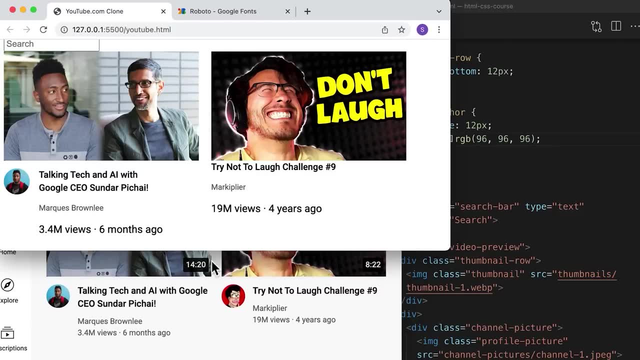 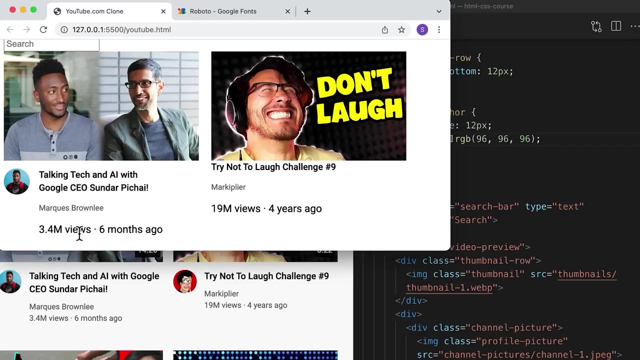 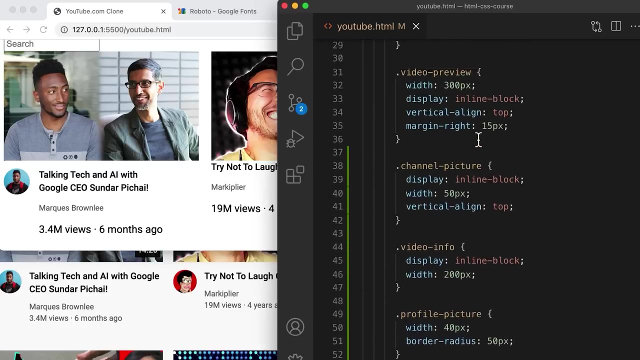 color right here, So RGB 969696.. Save that And if we go back, Okay, that looks perfect. Next, I'm going to style this paragraph. So in our code this paragraph is called video-stats And I'm not sure if we have a style for this. 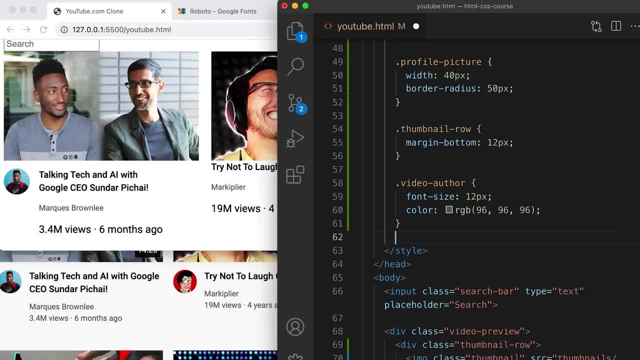 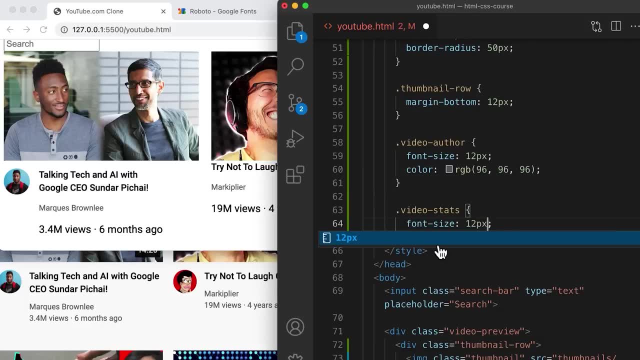 it doesn't look like we do, So I'm going to write a new one: video-stats. We're going to set the font-size to 12 pixels, because these two look the same, Okay, and then we're going to set the. 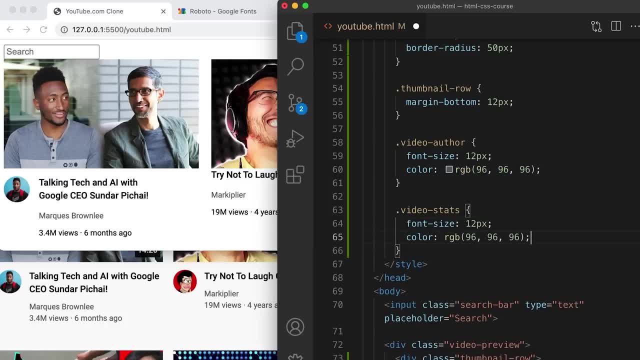 color as well, Since these two look the same. And now remember that whenever we have these duplicate styles like this and this, we can actually target multiple classes by adding a comma. So we're going to target the video-author class as well as the. 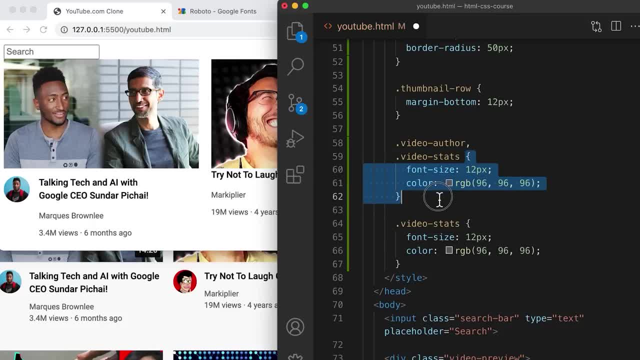 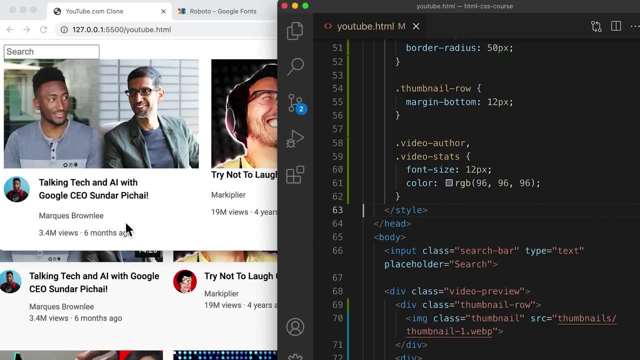 video-stats class. So this is going to help us reduce duplication of our code. So I'm going to delete these lines. Save it. Everything looks okay. And the last thing we're going to modify is the spacing between the paragraphs. So remember that paragraphs by default. 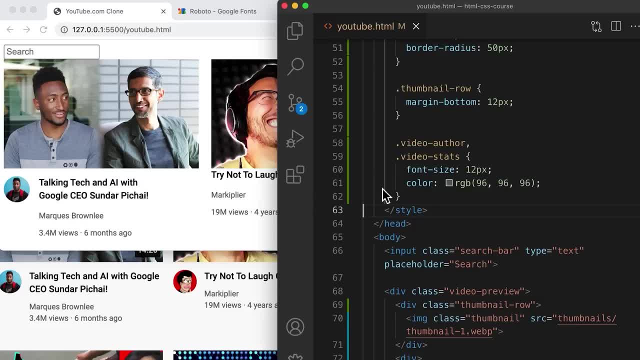 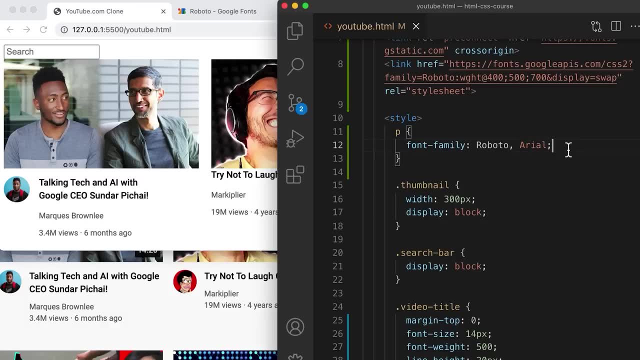 come with margin at the top and at the bottom. Now, instead of removing them individually, I'm actually going to go up to the top of our page, So we did this once before. We're going to get rid of the default margin for all paragraphs. 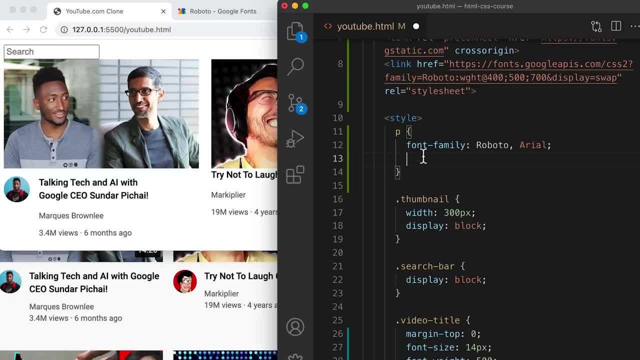 on the page. So to do that, we're going to go into these styles and we're going to set the margin dash top to 0. And we're also going to set the margin dash bottom to 0. And this will get rid of all the default margins. 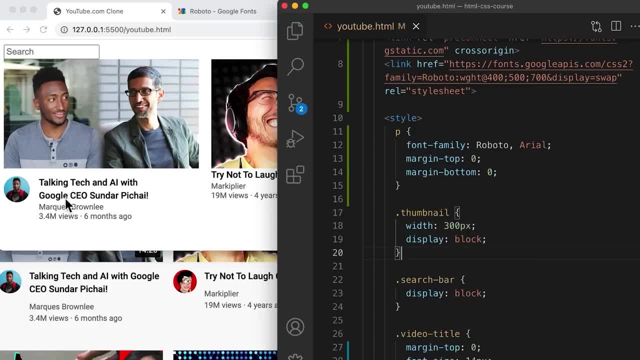 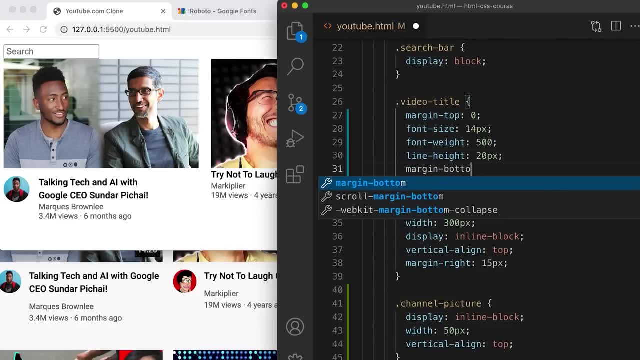 Save it. And now we can set a more precise margin at the bottom here. So under the video title, let's set a margin bottom of maybe 15 pixels. Save it. Okay, looks like it's a little too much. maybe 12 pixels. 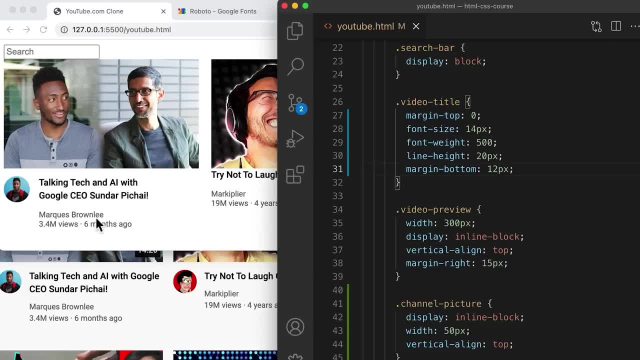 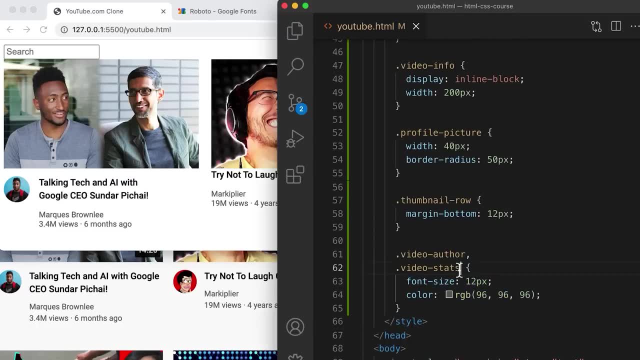 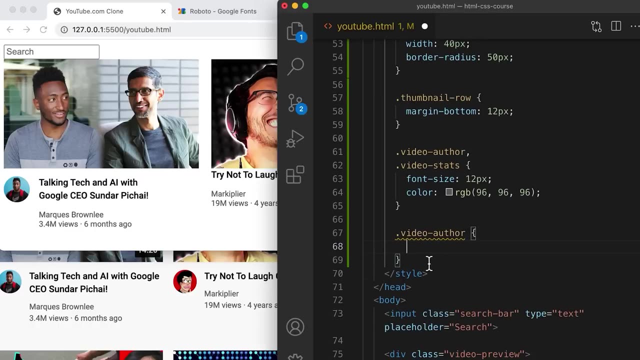 Okay, I think that looks pretty good, And now under the video author, we're going to add some margin. So currently we have some styles that apply to both of these. I'm going to target video-author individually down here. So for the video author, 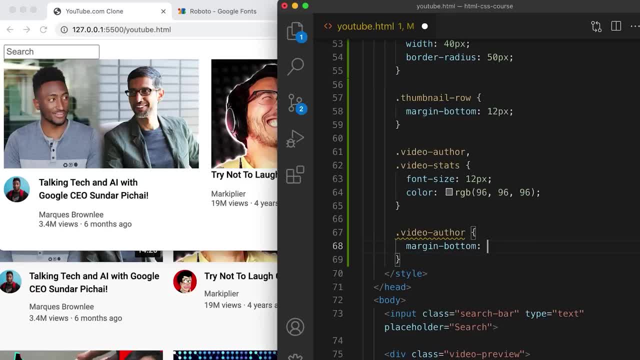 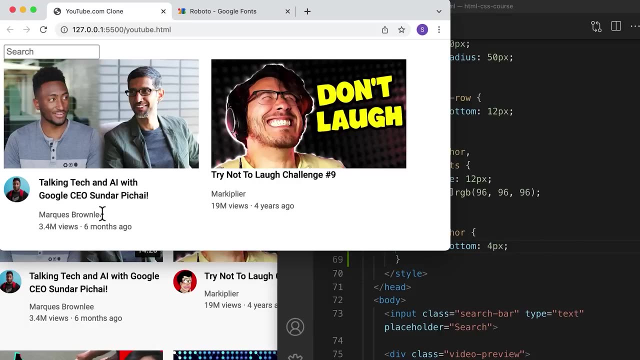 I'm going to add a margin dash bottom of maybe 6 pixels, Save it And maybe 4 pixels Okay. so I think that looks pretty close And now if we look at our website, you can tell that it's actually really close. 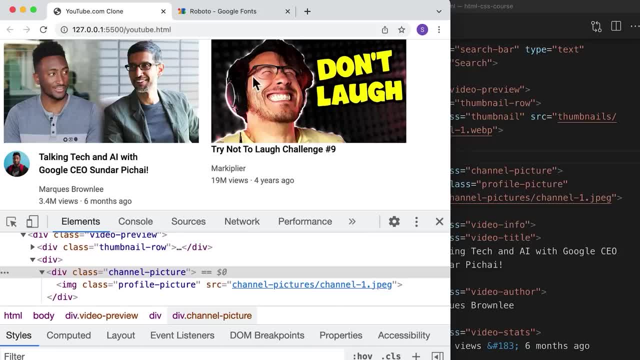 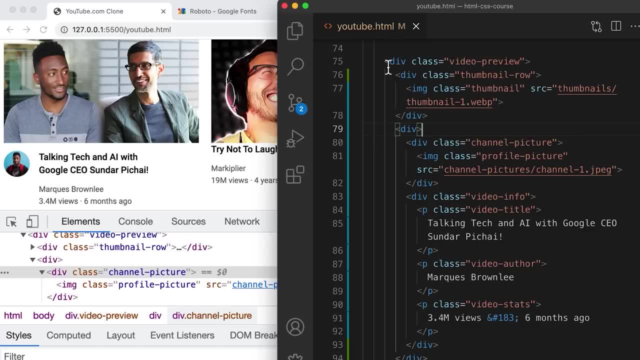 to the final design that we have Now to finish off this second video preview. you have a choice. You can either do everything that we did in the code here to give yourself more practice, or if you want to save time and move on. 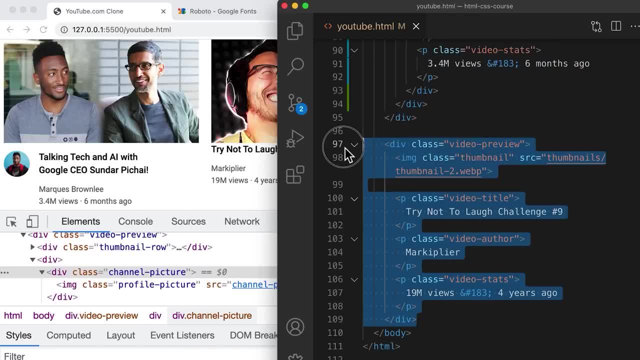 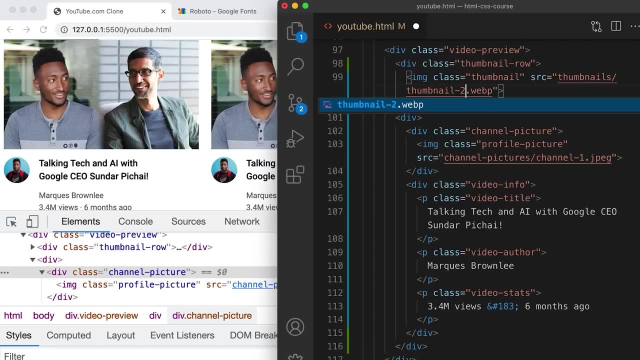 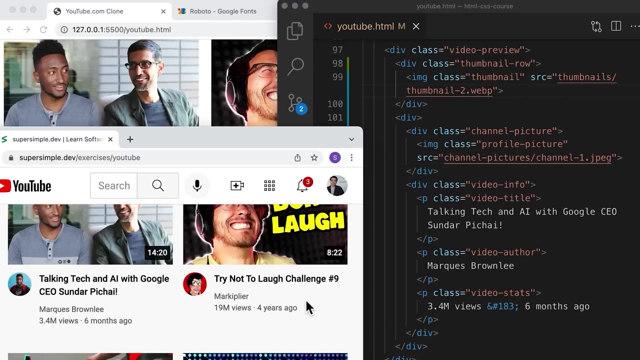 to the next section. we can just copy all of this HTML and replace this part here And then just swap out the thumbnail as well as the channel profile picture, which you will need to download first from here, As well as swap out all of the text. 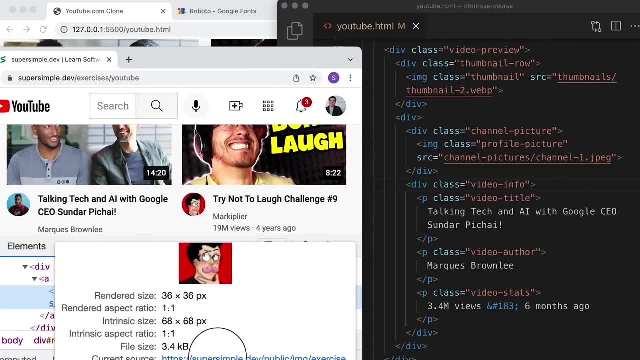 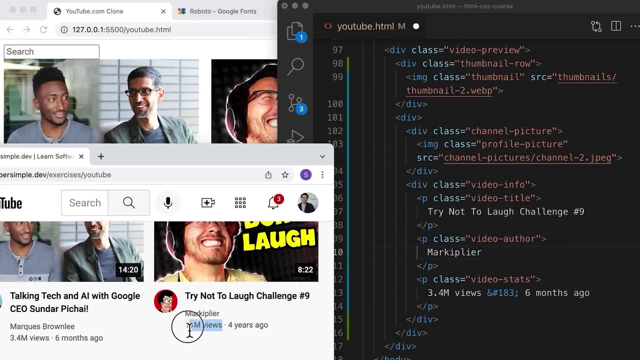 So I'm just going to fast forward this video to finish up this second video preview, But feel free to pause it and try it yourself, to give yourself more practice. And there we go. In this lesson we learned the nested layouts technique, which is one of the most important techniques. 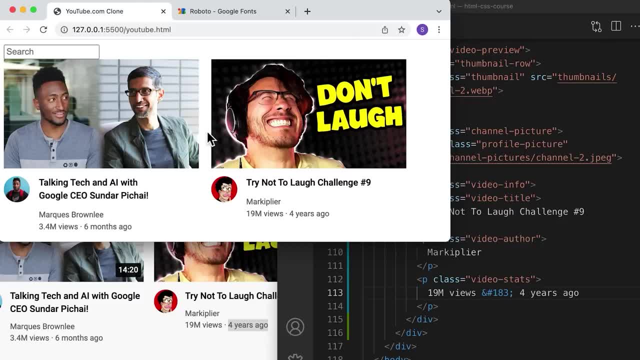 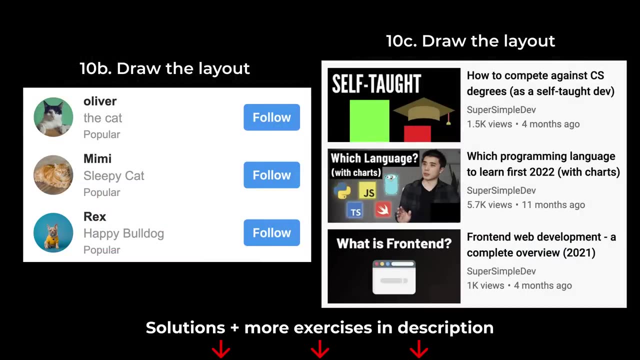 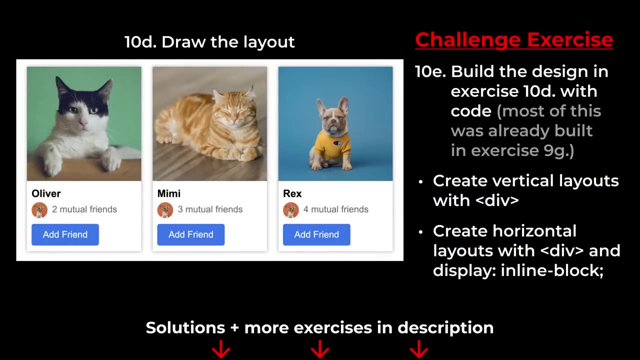 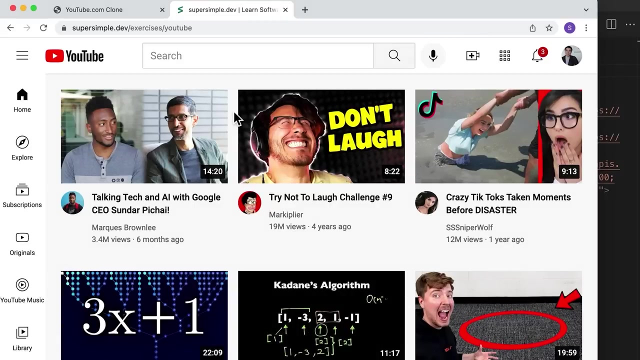 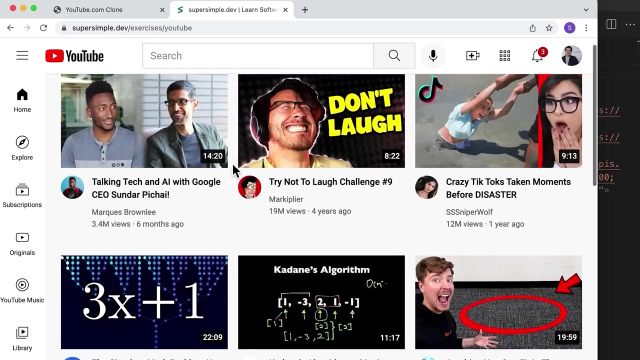 for being able to break down a design that you see on a website and recreate it using code. In this lesson, we're going to learn about CSS Grid, which is a much better way to create these horizontal layouts as well as to create a grid like this. 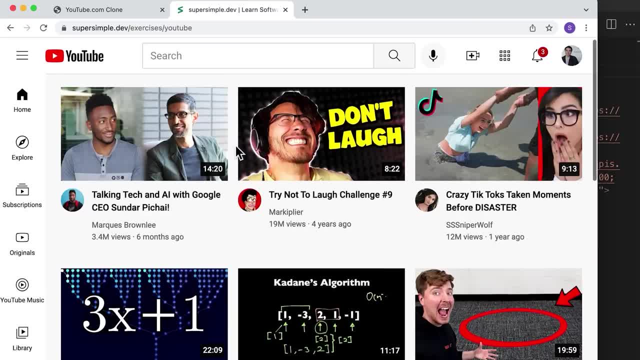 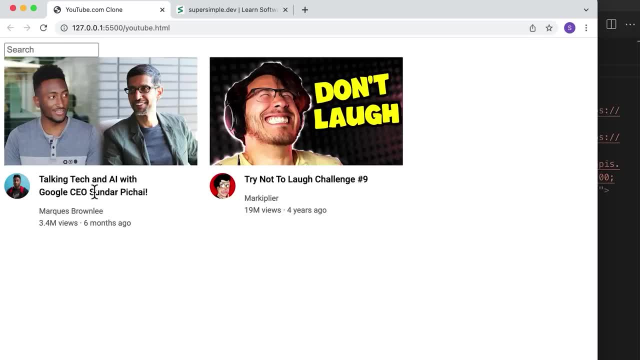 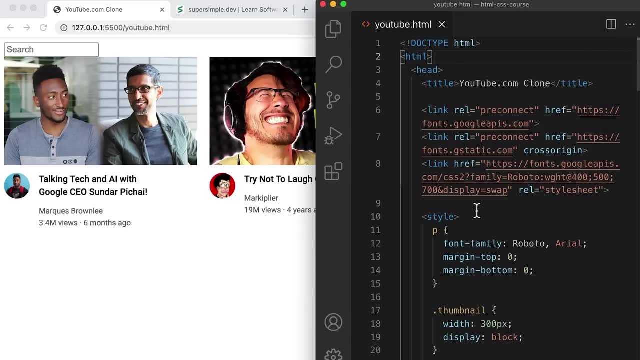 that you see in our final project. First, we're going to open up the website we were working on, So I have it open right here. And remember that for our horizontal layouts we were creating them using something called display-inline-block. So if we go into our code, 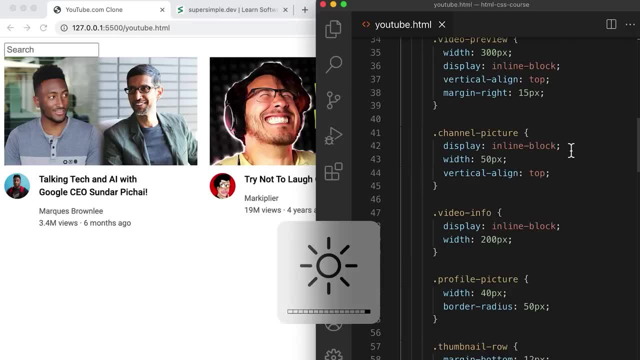 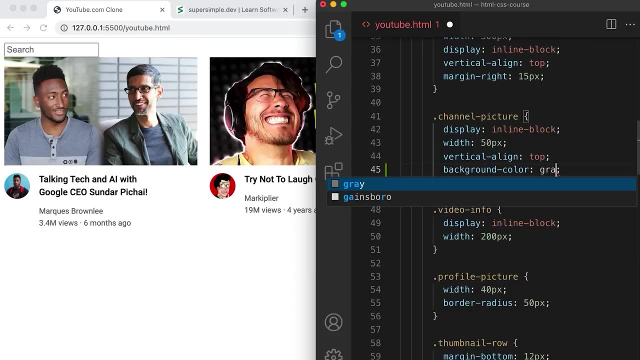 and we scroll down. we were using display-inline-block and a width to put these two side by side. Now there are some problems with display-inline-block that I want to show you right now. We're going to set the background color of these to gray. 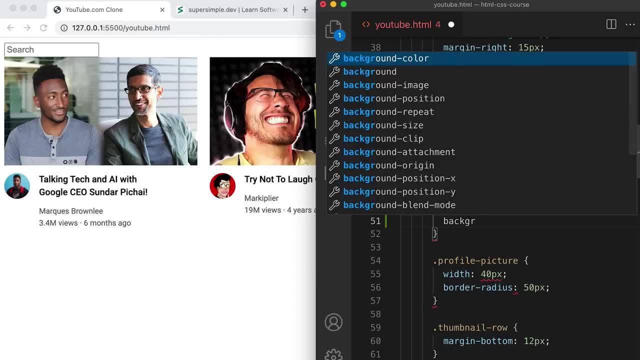 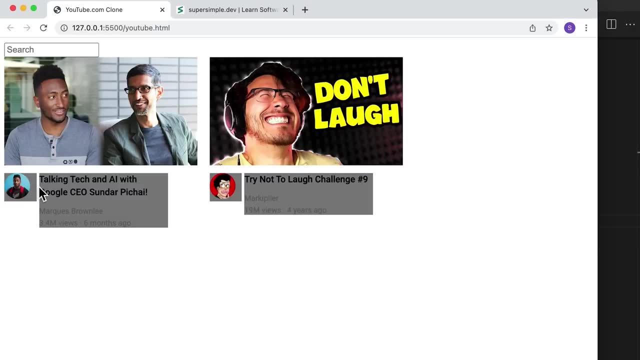 So this will make it easier to see what the problem is. Now let's save it. and now you can see that there's a little bit of space between these two And this causes some alignment problems. So the width of this entire container here. 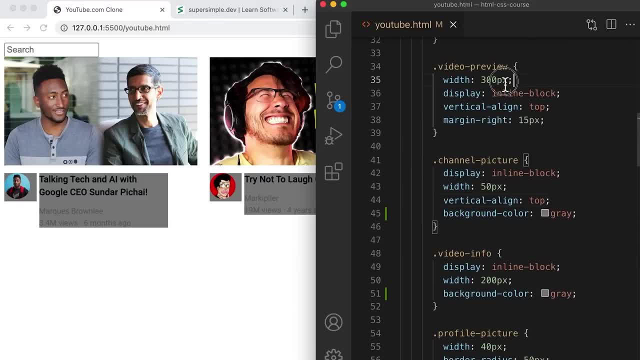 the width: here we set it to 300 pixels, But we set the channel picture to 50 pixels here and the video info to 200. So you would expect that we can actually set this to 250 to take up the entire 300 pixels. 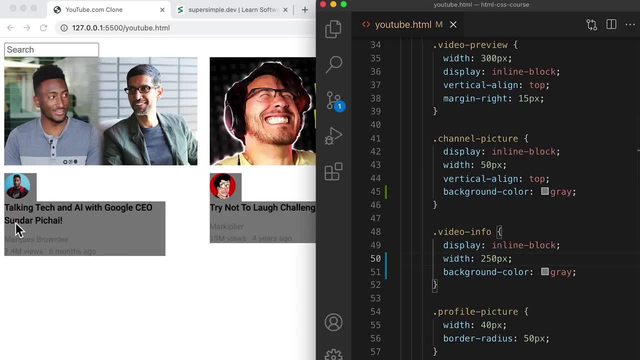 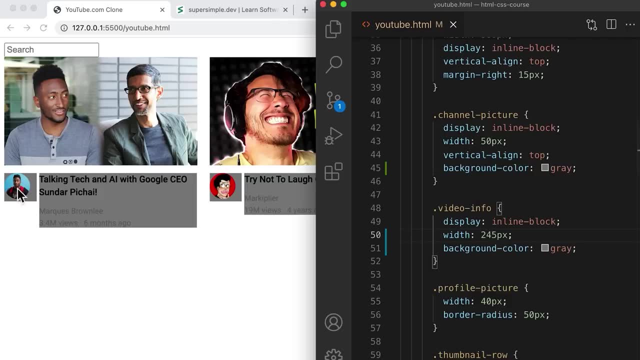 But if I save it, you can see that it's too long and it wraps to the next line. So we have to set it to something like 245. And that will cause it to appear beside each other. So this is one problem with inline-block is that it has. 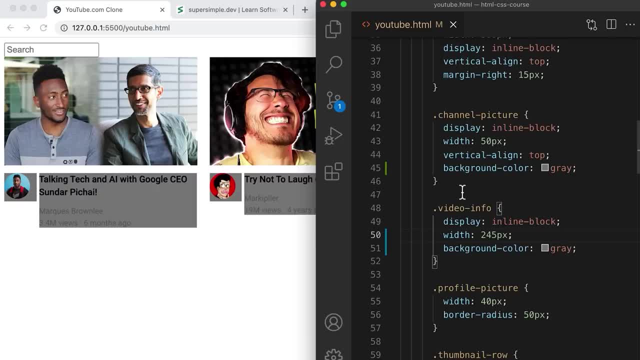 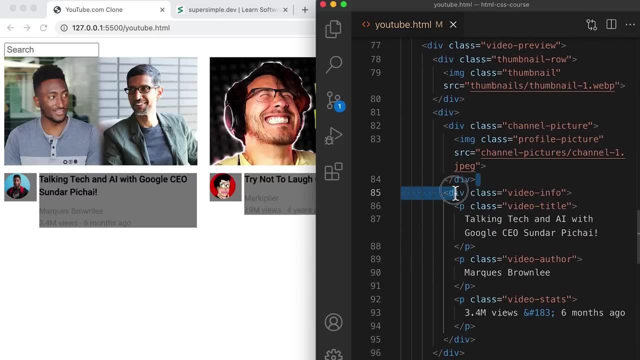 some alignment problems. Now you might be wondering where this space is coming from. If we scroll down to our HTML, we can see that there's actually some space between these two divs, And we learned earlier that HTML aligns multiple spaces together. 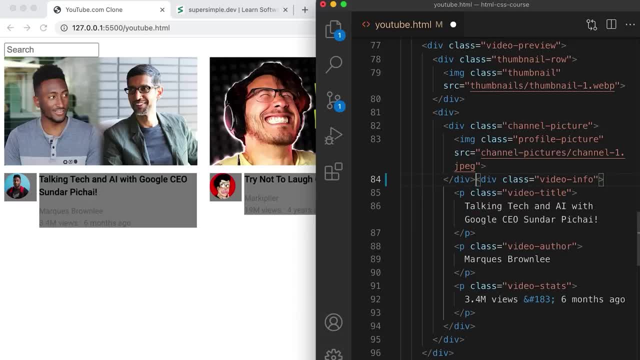 and that's what shows up here. So we could remove this and save and get rid of that space, but that means our code is less easy to read. Now, the second problem that inline-block has is that it's not vertically aligned, like you see here. 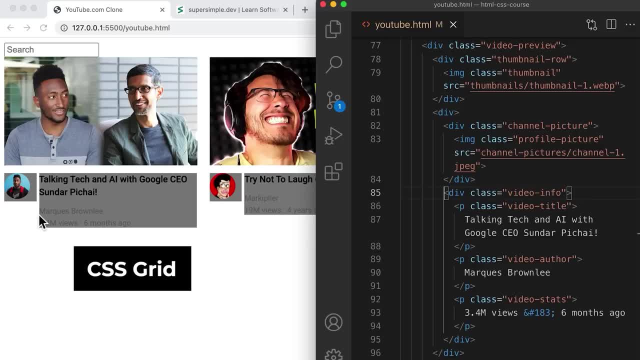 So now we're going to learn a new technique called CSS Grid that's going to help us create perfectly aligned horizontal layouts. To learn grid, we're going to create a new file where we're just going to practice using grids. So let's go into our code editor. 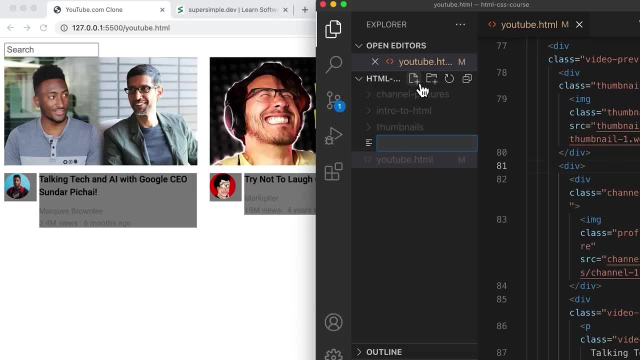 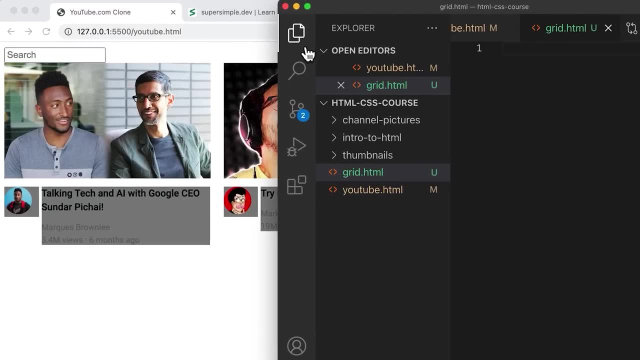 and we're going to create a new file called gridhtml. And remember, for every HTML file we want the proper structure. So at the top we're going to have a doc type and then we're going to have an HTML element. 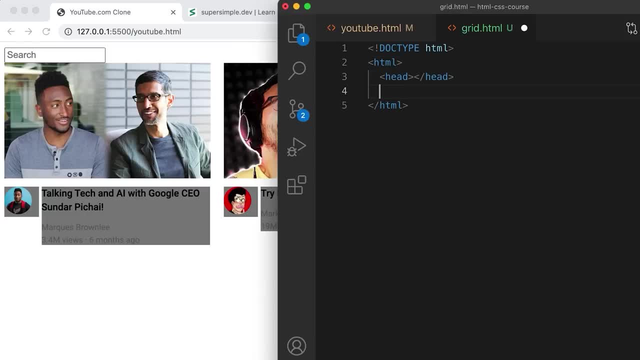 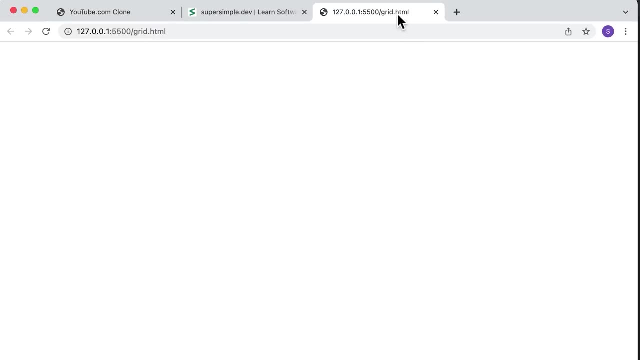 and then inside we're going to have a head element and a body element. Now that we have the proper structure, we can open this file in Live Server. So let's right-click and open with Live Server And then let's set the title. 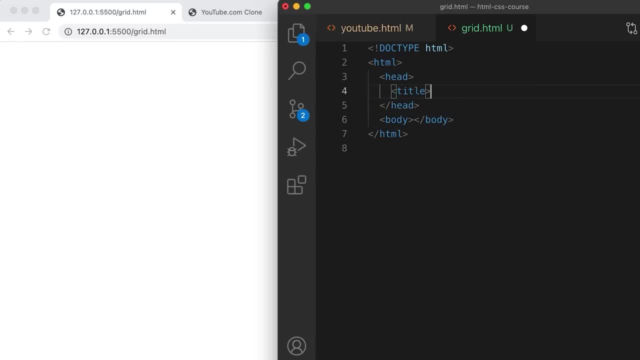 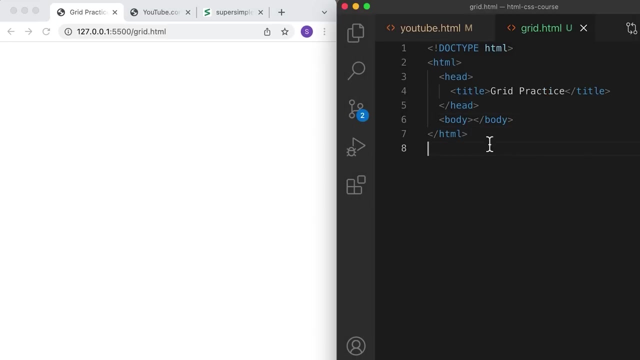 or the text in the tabs here to grid practice. So we know what this file is about. Let's save it. So I'm going to resize my windows here, just so we can see what's going on. We're going to start off. 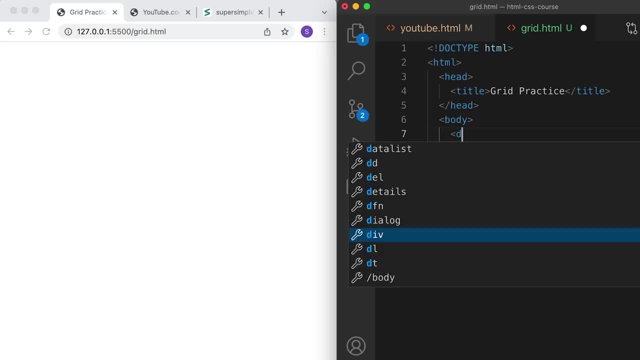 in the body and we're going to create a div, And then, inside this div, we're going to create two divs. So let's call this div1, and let's call this div2.. Save it. And now to help us, 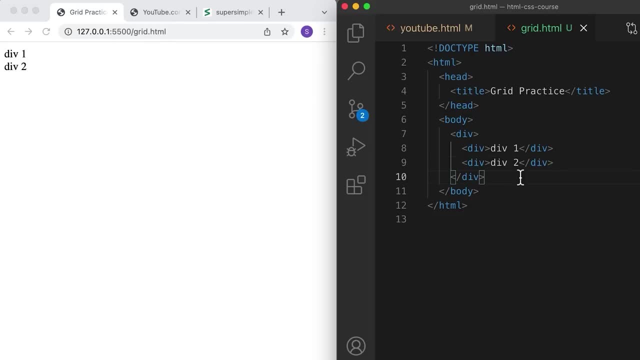 learn. I'm actually going to show you a new way of writing CSS. So if we go to the opening tag here, we can set a special attribute called a style attribute. Now the style attribute is unique because it lets us write CSS code inside. 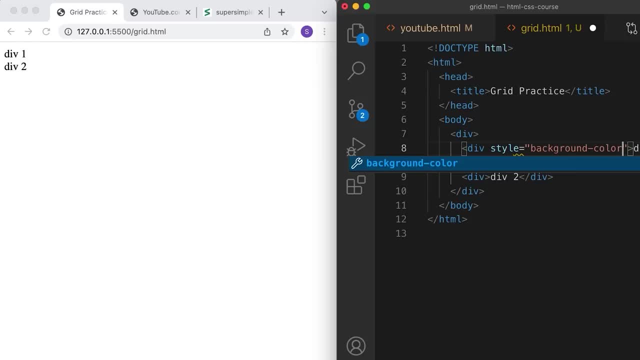 So let's write the code- background-color: light blue- And we save it. We can see that the styles that we wrote here are applied to this element. So this code here is another way of writing CSS called inline styles. We're writing our CSS inside. 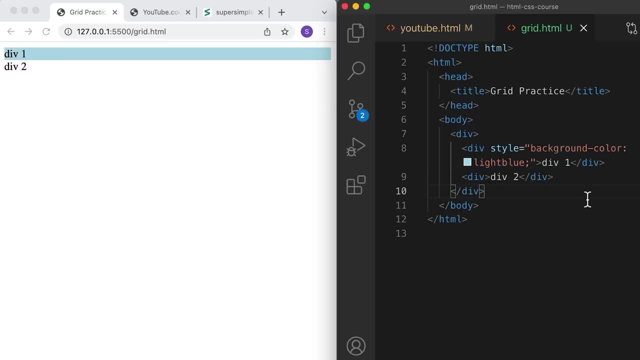 a line of HTML. We've already learned two other ways of writing CSS. One of them is the style element, and the other is to put our CSS in a separate file. This is a third way of writing CSS. Now, generally we don't use this in real websites. 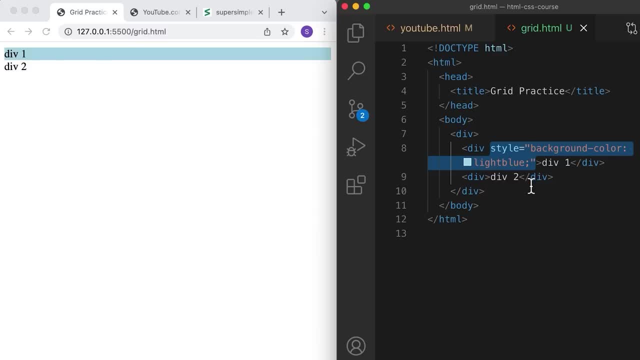 because it makes our HTML harder to read. In real websites, we put our styles in a separate file. But for now, since we're learning, this is pretty useful Because, number one, it only affects the element with the style attribute, And the other thing is that 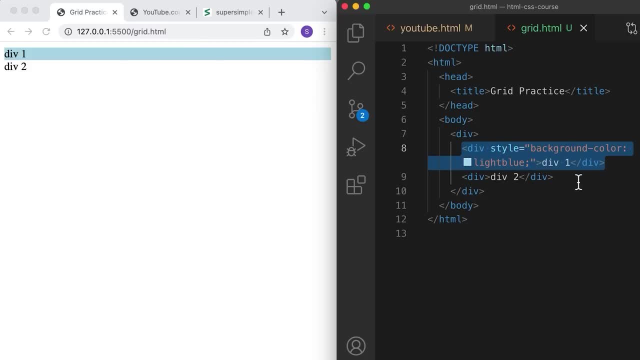 the CSS code is right beside our HTML, So that when you go and review this file later, it's very easy to see what's going on. So let's practice with the style attribute. We're going to add another one to this second div, So let's set. 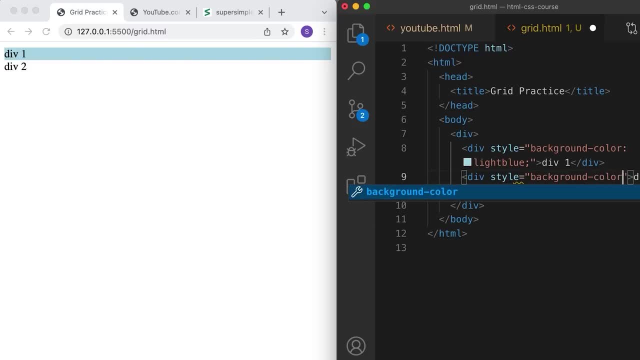 the style to background-color And we'll set a background color of light pink. Let's save it. And now we have the two divs we're going to work with Now. currently, we just have two divs inside another div. There's nothing new going on here. 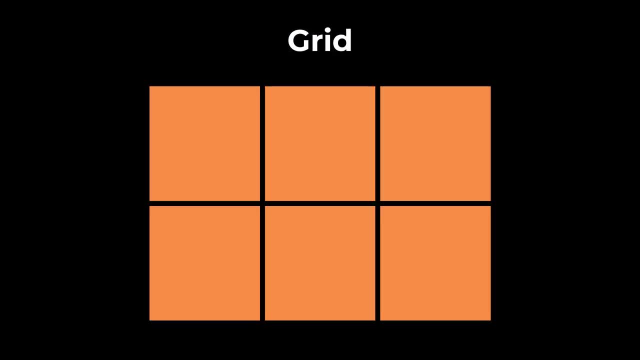 But now we're going to create our first grid. So what is a grid? A grid is a layout that has rows and columns. For example, this is a 2x3 grid. We have two rows and three columns. This is a 1x2 grid. 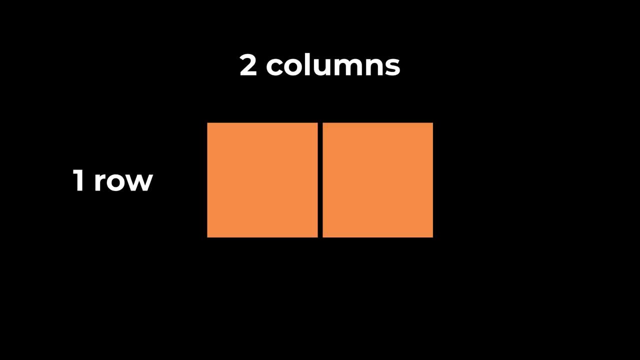 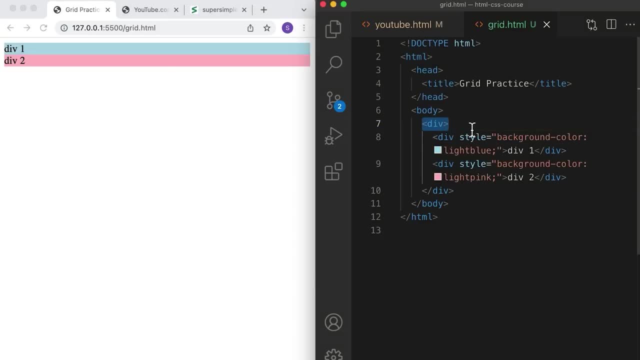 We have one row and two columns, So we're going to learn how to make this kind of structure in our HTML. To do that, we're going to style this outer div or the container. So let's see how that works. We're going to set a style. 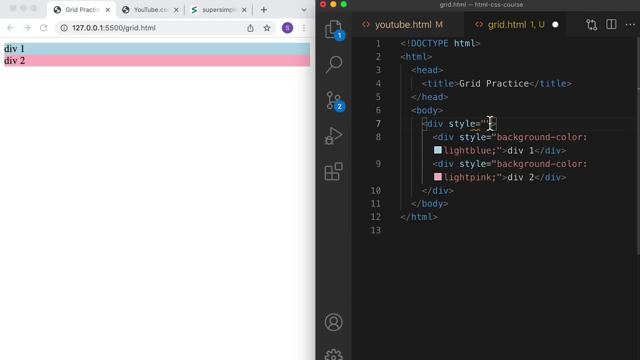 attribute here And to create a grid. we're going to need two steps. The first step is to set the display property And we're going to set display to grid. The second step is we need to set how many columns our grid has. 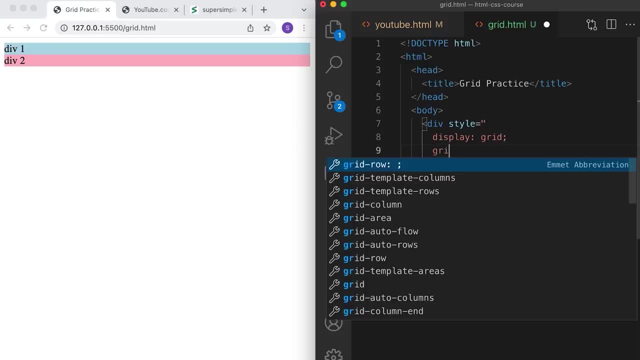 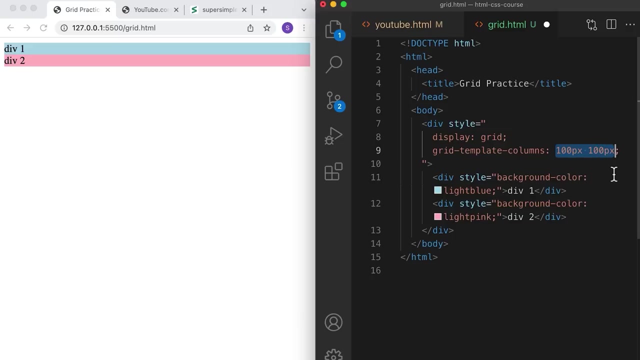 So to do that, we're going to use this property- grid dash, template, dash columns- And we're going to give this property two values: 100 pixels and 100 pixels. So these two values define how wide our grid columns are. The first column is going to have 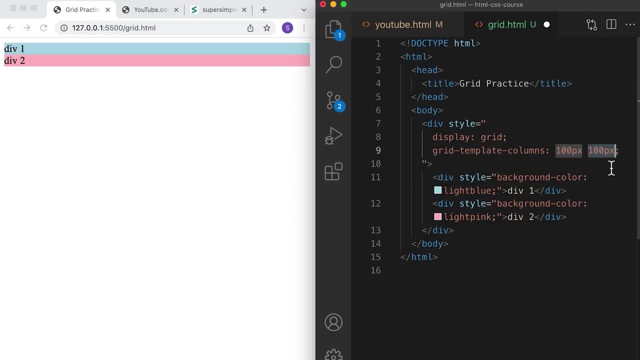 a width of 100 pixels And the second column is going to have a width of 100 pixels as well, And our grid will have two columns. So if we save this, you'll see that we created our first 1x2 grid. 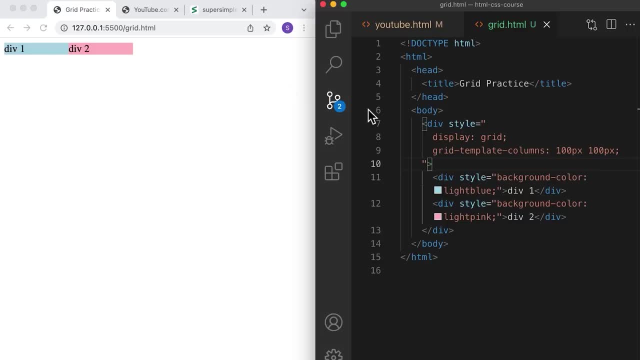 Now I want to point out a few characteristics of a grid. First of all, notice that this div is no longer taking up the entire line, So recall that divs are display block by default. They're supposed to take up the entire line. 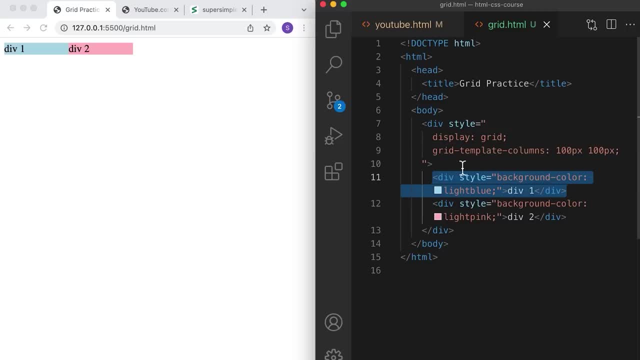 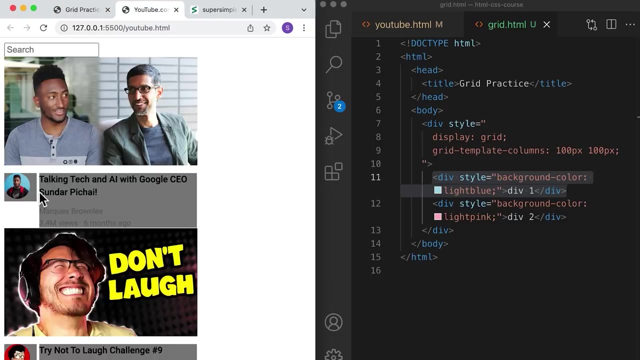 But when this element is inside a grid, it's actually placed into the grid, So it only takes up the entire column instead. The second thing you'll notice is that there's no extra space between these two, Unlike with display inline block. And the third thing to notice: 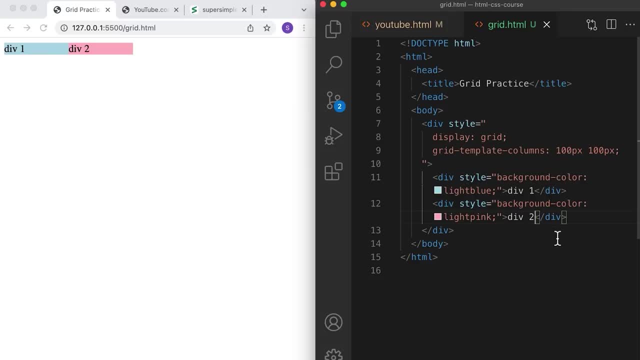 is that, for example, let's add another element into the second div, Let's add a paragraph of text, Save it. When we add more elements, this makes the second div taller than the first one, but they are vertically aligned And that's another difference between grids. 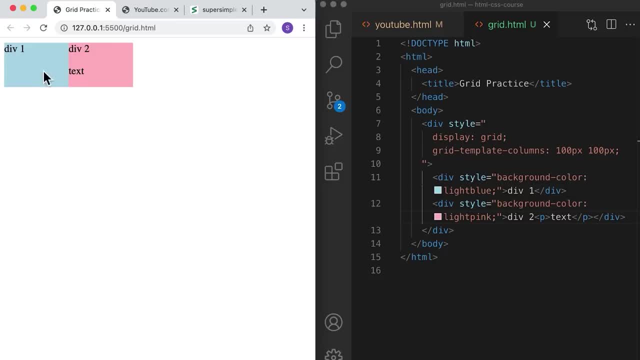 and display inline block Grids maintain alignment much better. Alright, so that is our basic grid. Now we're going to create another grid to practice with. We're going to go into our code, We're going to copy all of this And then we're. 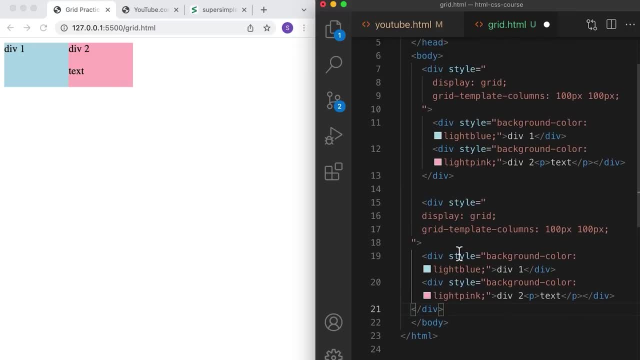 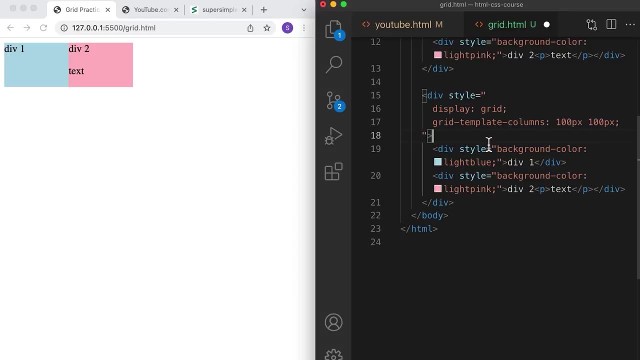 going to paste it below, And it's a little bit weird, the formatting, so we can select this and press tab to move it back into a normal position. Let's save it. And now we have our second grid, But let's actually add. 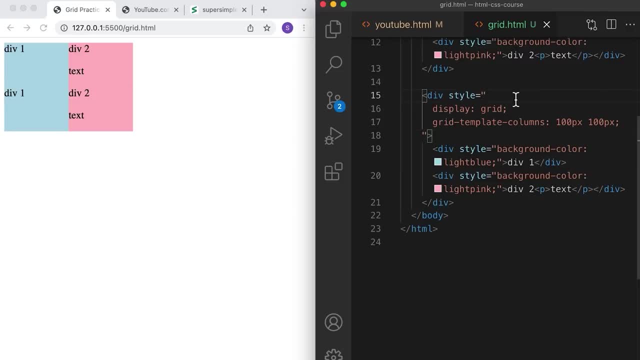 some space to the top so that we can see it more clearly. We're going to add some margin dash top Of 30 pixels. Save it. Okay, that looks pretty good, And this time we're going to add a third column. 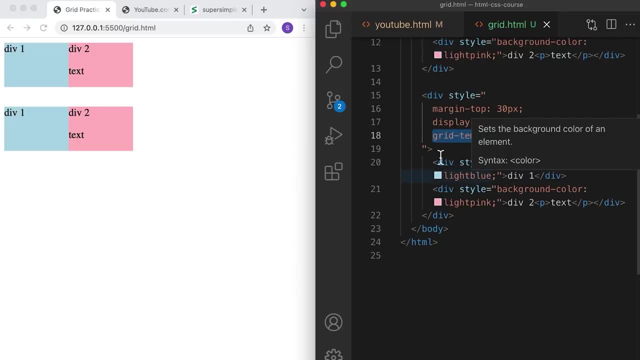 So this property actually takes any number of values that you give it. So if we add a third value here of 200 pixels, it's going to create a third column that is 200 pixels wide. So the number of values determine the number of columns. 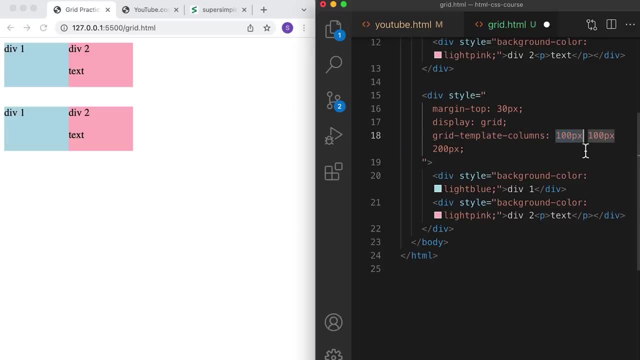 And the value itself determines the width of the column. So if we save it, we do have three columns here, but we only have two divs, So we need another div to fill out the third column. To do that, let's copy our first div. 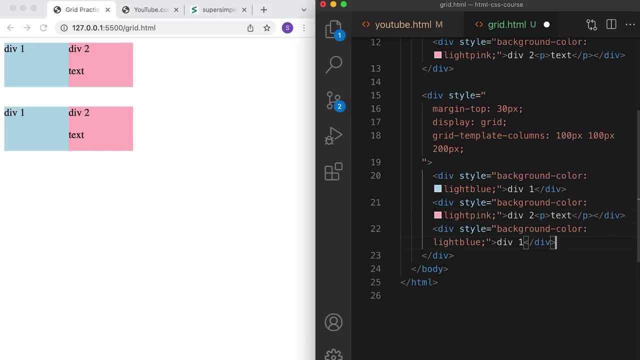 and then we're just going to paste it down here and call it div3.. So now we have three divs to fill out the three columns And you can see that our third column is 200 pixels versus 100 pixels. that we saw right here. 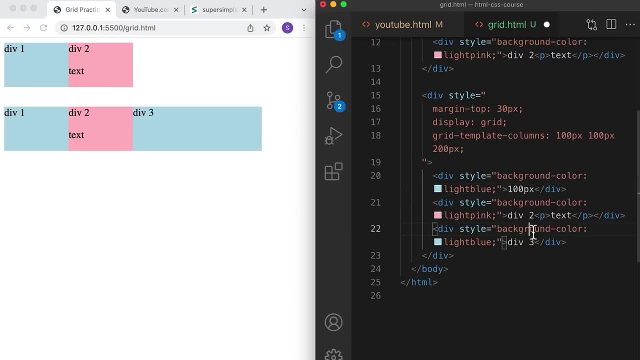 So let's actually change the text here so that we can see what's going on. So 100 pixels, 100 pixels and 200 pixels: Save it. So now let's see what happens when we add another div to our grid here. 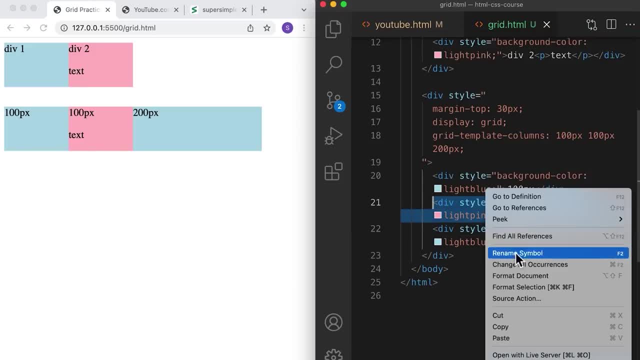 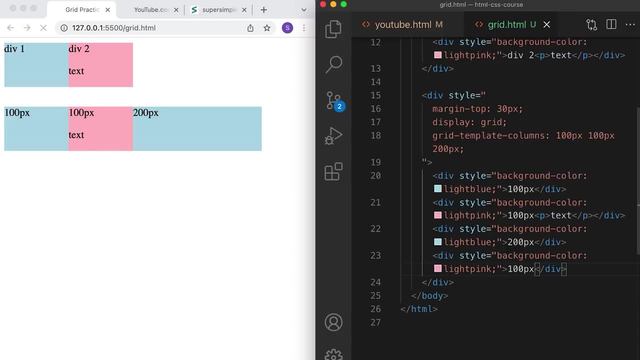 So let's copy this second div and then duplicate it. Copy it and paste. You can actually get rid of this paragraph here And save it. And now you can see that this fourth div wraps around to a second row. So whenever we have more elements than we have, 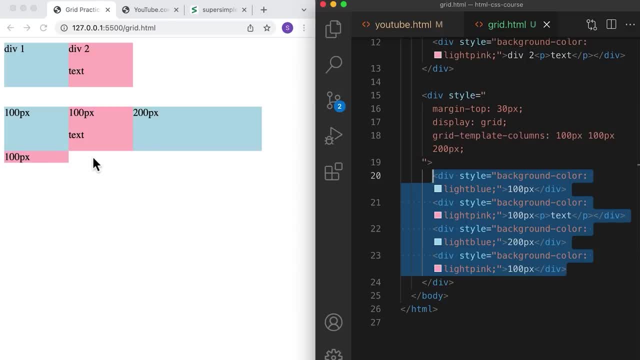 columns. here it starts to wrap around and create new rows. So that's the basics of how grids work. Now I'm going to show you a special value that we can use with grids. First let's copy this and then create a new grid to: 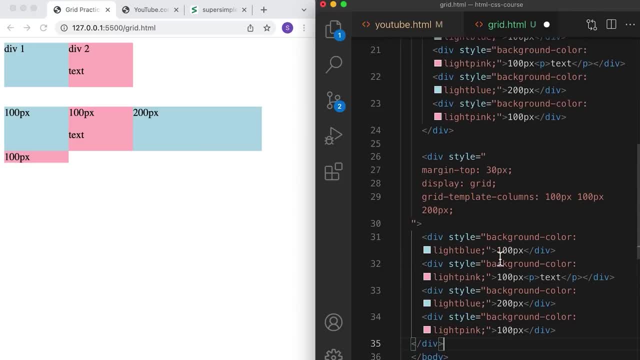 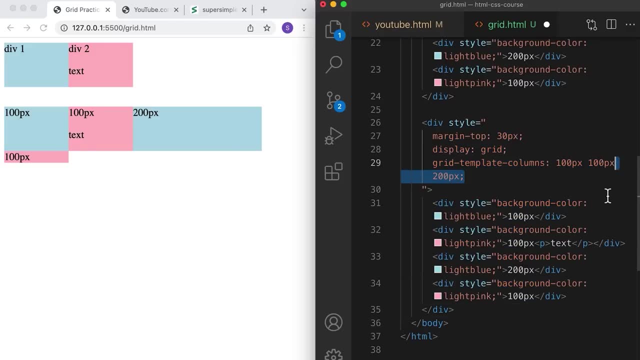 practice with. Let's paste it here And then select this and tab, And this time we're only going to have two columns. So let's get rid of this third column And let's only have two divs here, And we can also get rid of this paragraph. 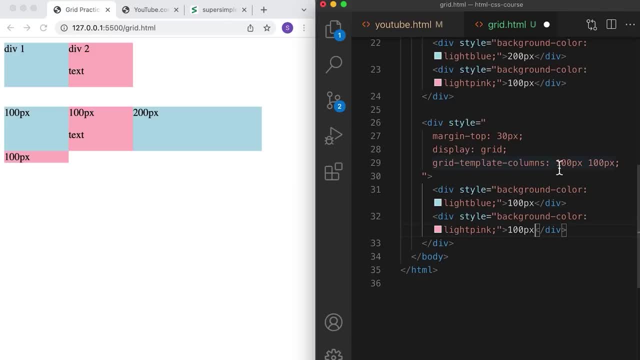 For this grid we're going to have two columns. The first one is 100 pixels and the second one we're going to change it to 1fr. So fr is a special value in grid. that stands for free space. It means to take up the 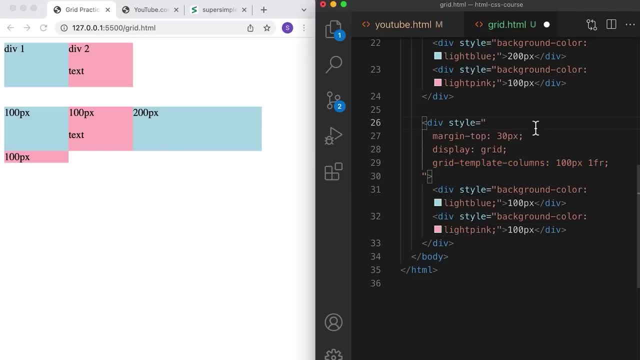 remaining amount of space on this grid. So, if I save it, you can see that the first column here is 100 pixels and the second column has a width of 1fr, so it takes up the remaining amount of space that we have. 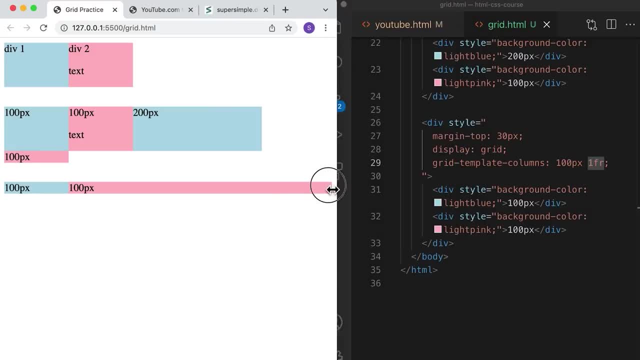 If I resize the page, it'll take up the remaining amount of space. So that's what 1fr means. I'm going to change this to 1fr so that it's easier to see when we review this file. So this fr value is exactly. 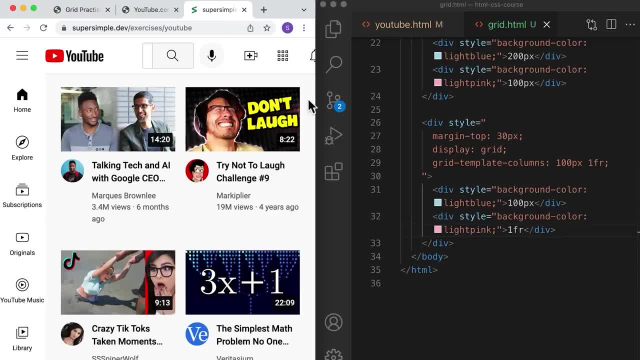 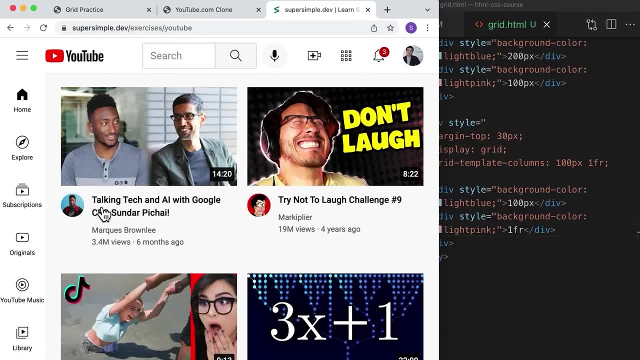 what we need in our final design. If I open my final design, you can see that we have a horizontal layout here. The first column is about 50 pixels and we want the second column to take up the remaining amount of space, which is exactly what we need. 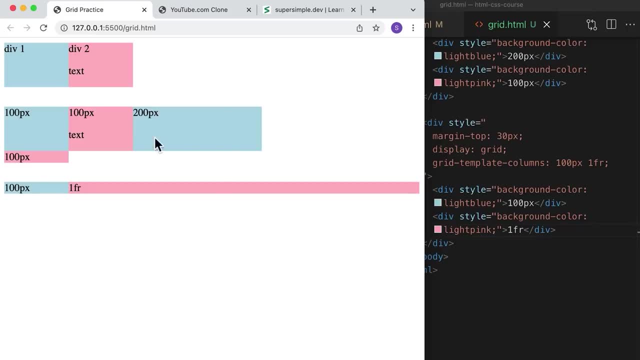 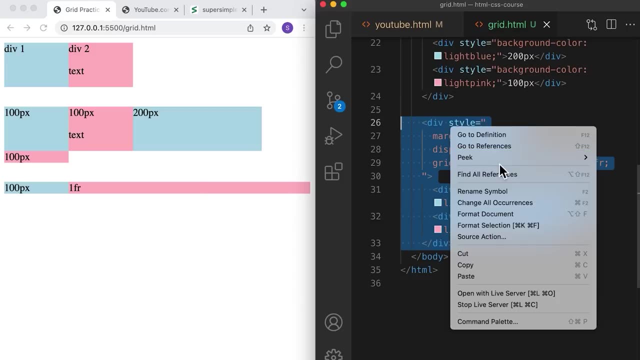 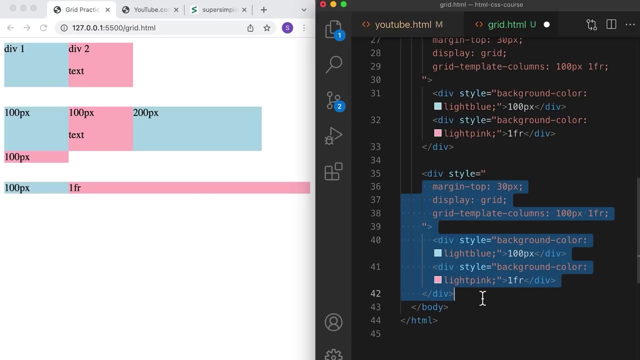 1fr. for Now, before we go and update our project, I'm going to show you another property of this fr value. Let's copy this div and create another grid Below it, And this time we're going to add a third column. 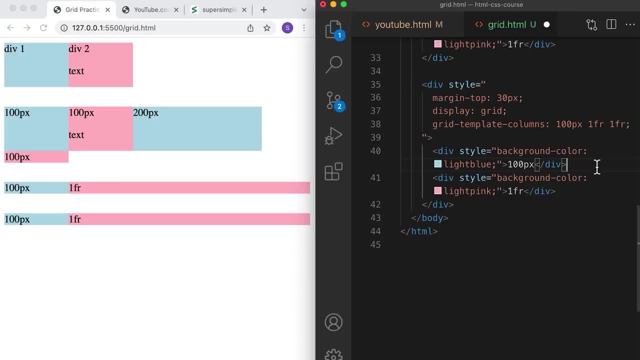 that is also 1fr And we're going to add another div to fill out this third column. Let's copy this and paste it into a third div. This one is also going to be 1fr, So let's save it here. 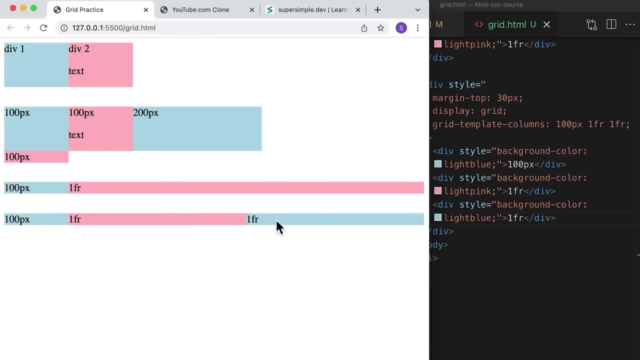 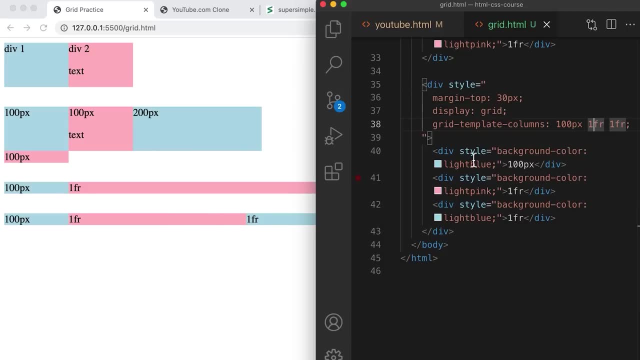 And for this example, the second column and the third column both have 1fr. So 1fr tells the columns to take up the remaining amount of space and the number in front of it tells us relatively how much of the remaining space this column gets. 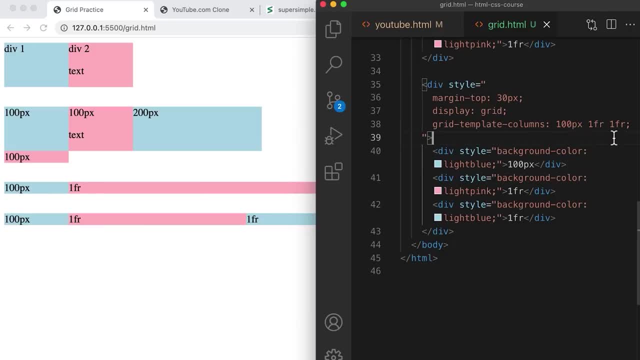 Since in this example both of them are 1, they'll get an equal amount of the remaining space. So here these two are equal and they take up the remaining space If we change the third column to 2fr. so let's change this to 2fr. 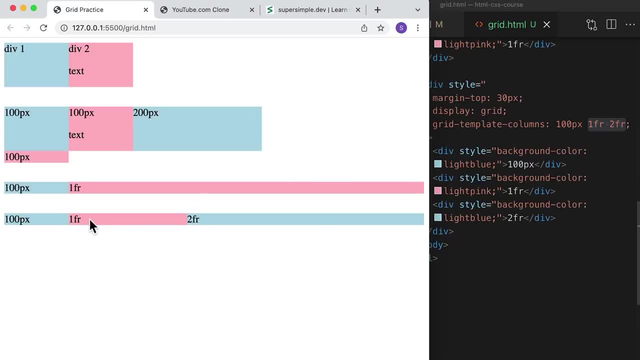 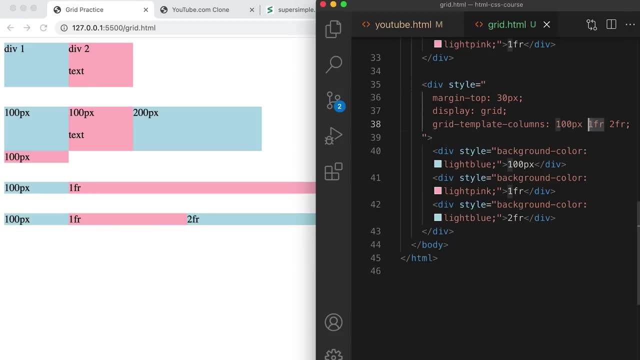 and save. the second and third column will take up the remaining space, but the third column will be twice as wide as the second column, So this number here is sort of like a ratio. This second column will have 1fr of the remaining space. 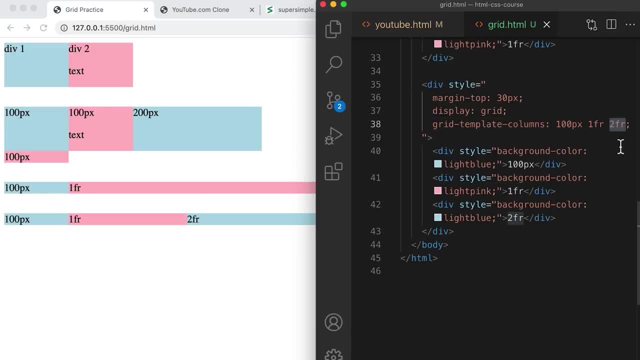 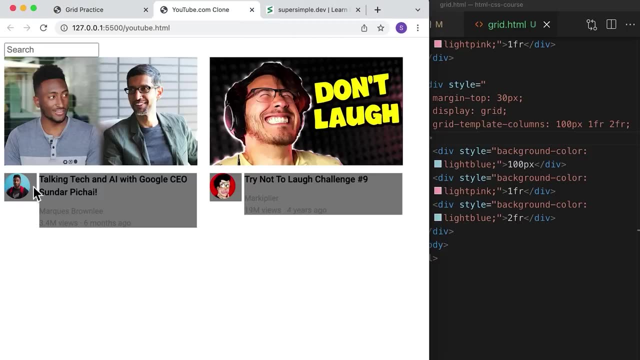 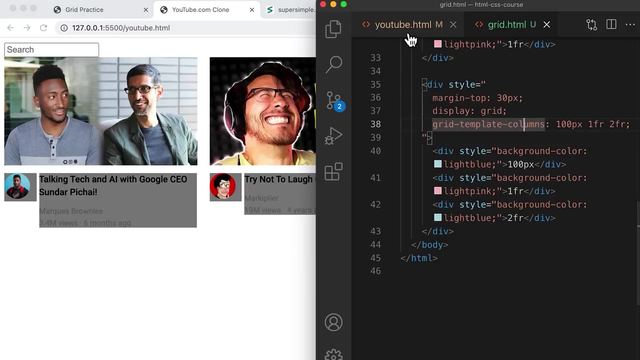 and this third column will have 2fr of the remaining space. Now that we understand that concept, we're going to go back into our project and use grids to create this horizontal layout instead of inline block. Let's go to our code and we're going to scroll down. 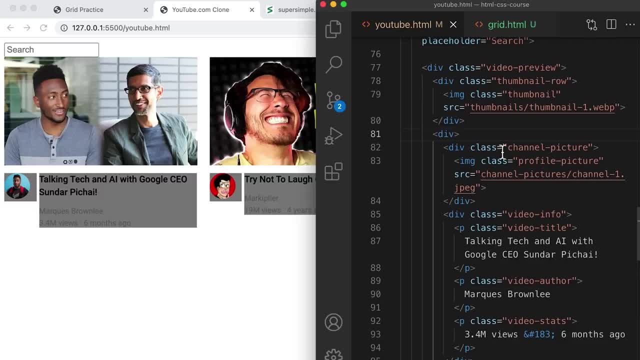 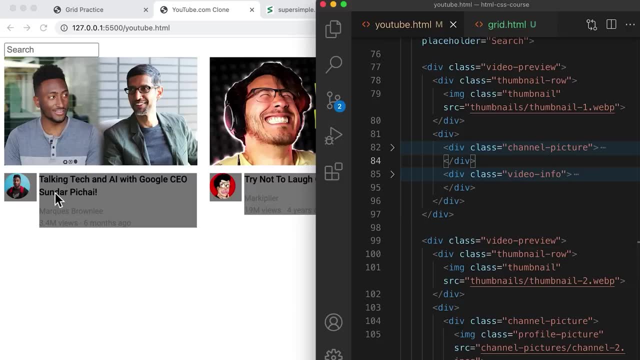 into the HTML for this, which is right here, and I'm going to collapse it so it's easier to see. We have the channel picture and the video info, which is these two. So to create a grid, remember we need to create it on the container. 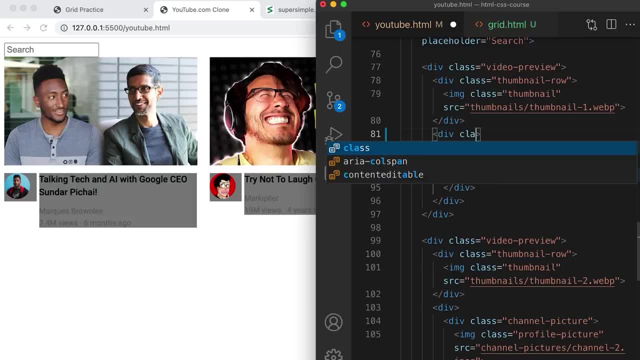 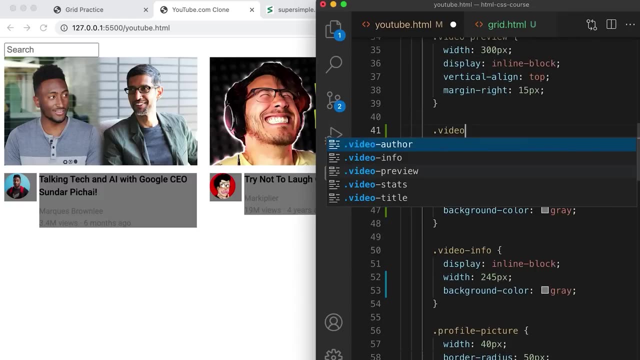 which is this div. So let's set a class name video-info-grid, and then we'll target this class in our CSS above. So I'm going to scroll up and I'm going to actually put it right here: video-info-grid. 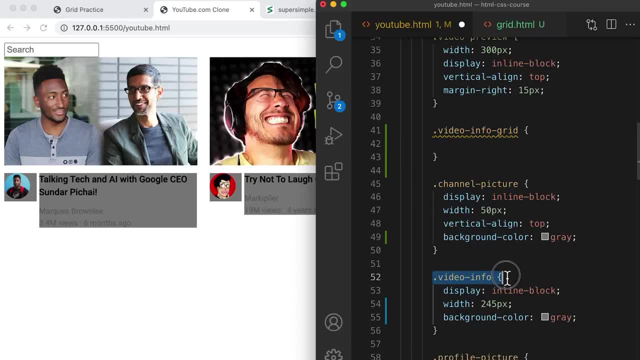 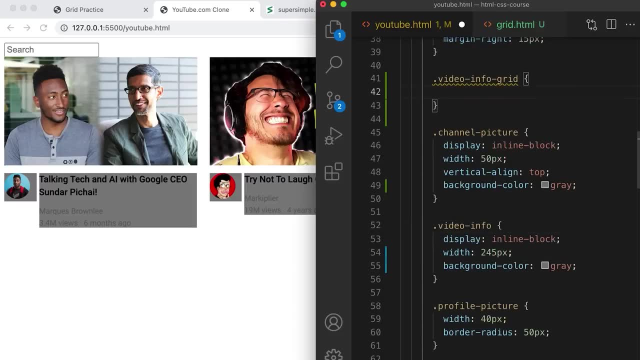 because this is right above the channel picture and the video info, So it's beside other related styles. Now remember: to create a grid, we need two steps. The first one is to set the display property to grid. This creates our grid. and then we need to set 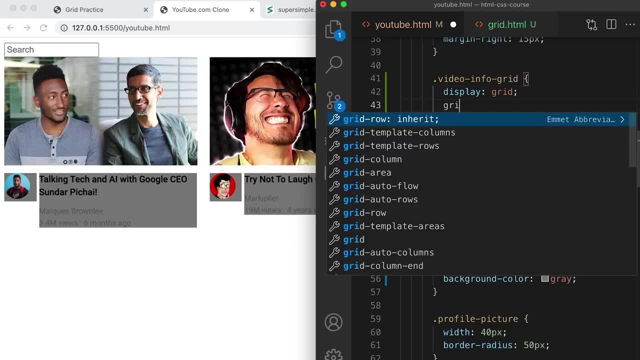 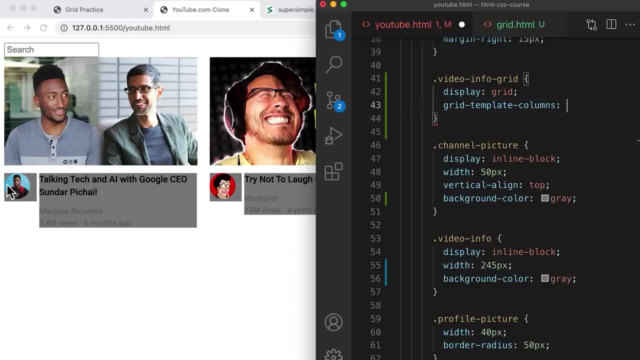 how many columns our grid has. So we're going to set grid-template-columns, grid-template-columns and for our purposes, let's set a column of 50 pixels for the channel profile picture, for the channel profile picture, and then we want the second column. 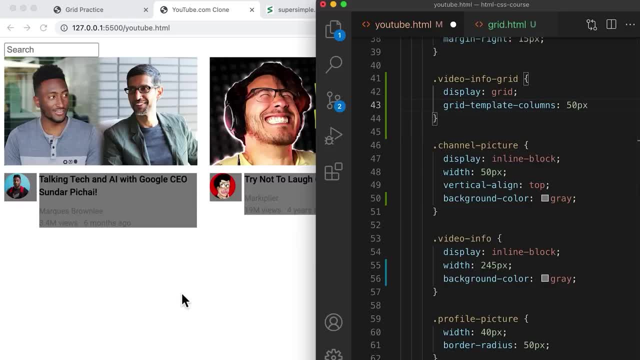 to take up the remaining amount of space. So, as we learned, that is 1fr. Now, if we save it, you'll notice that the space between the inline blocks is gone, so unlike here- And you'll also notice that these two are vertically aligned. 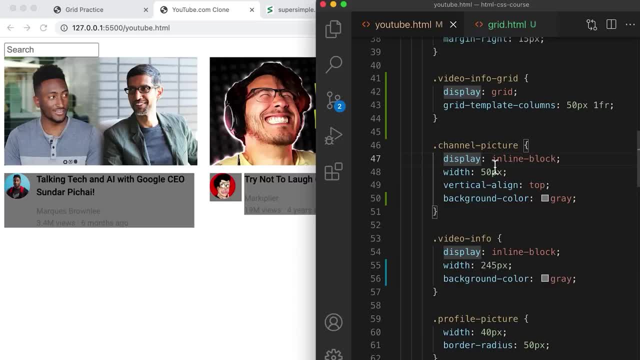 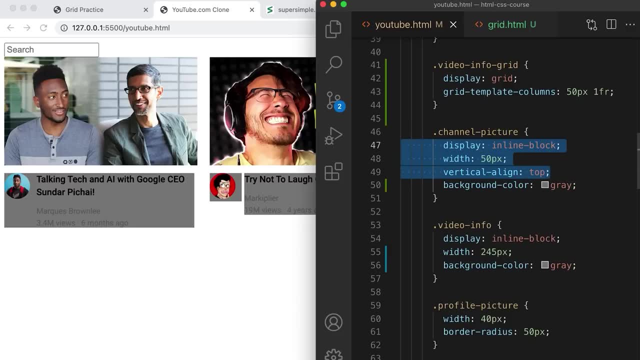 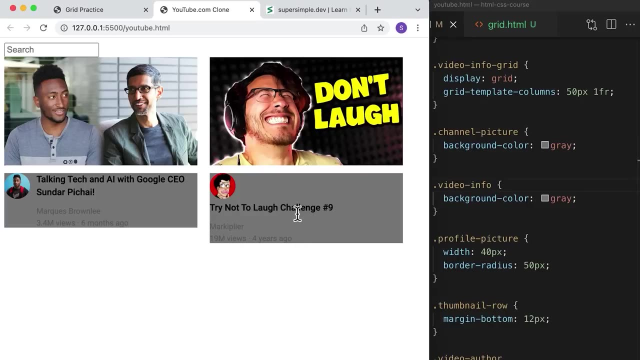 So, now that we have our grid, we can actually remove all of these inline block styles because we're not using them anymore. So we can actually remove all of these and all of these. Let's save it. and now let's set a grid for. 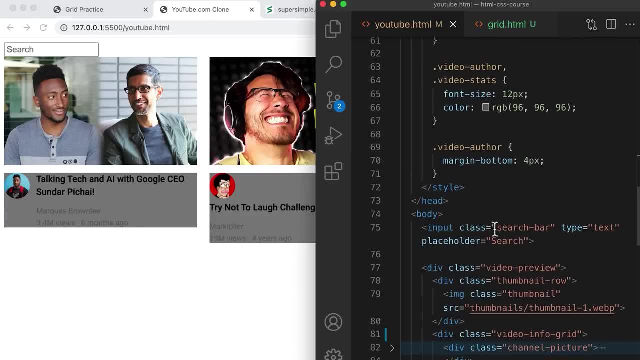 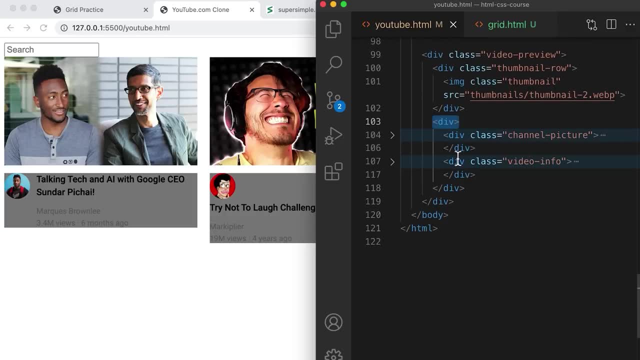 the second video preview. We're going to scroll down, so remember, we're going to set the styles on the container here and then these two divs are going to appear in our grid. So we've already created the CSS at the top. 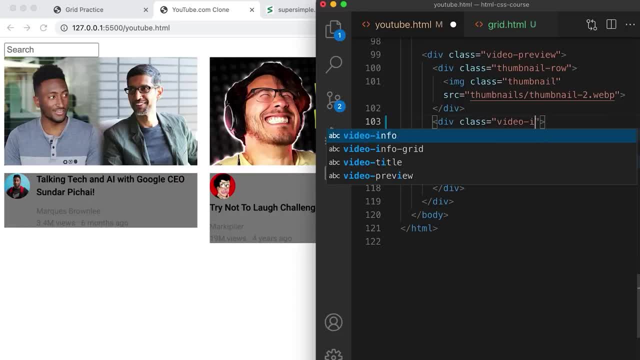 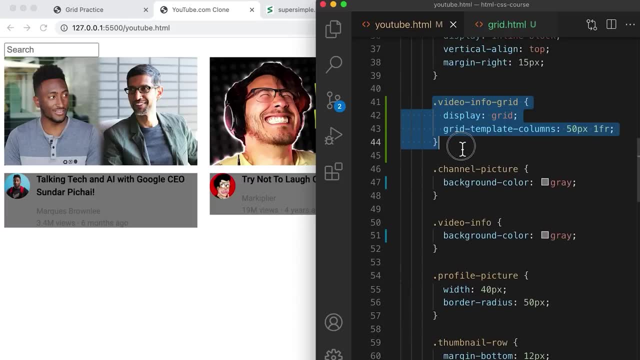 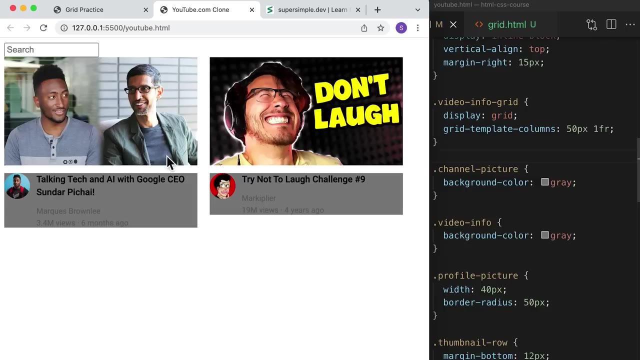 we just need to set a class of video- dash, info, dash grid, Save it and then all the styles that we wrote up here will target that class. So now we have both of our grids and you can see our horizontal layout is perfectly aligned. 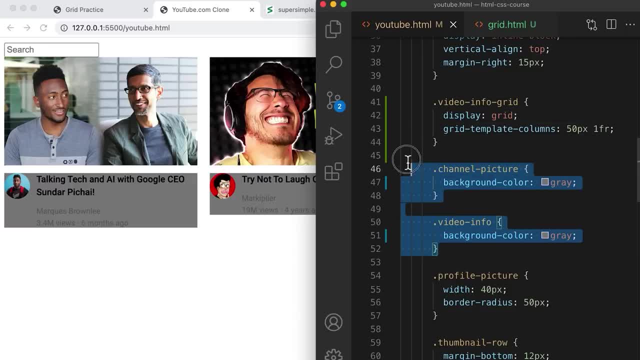 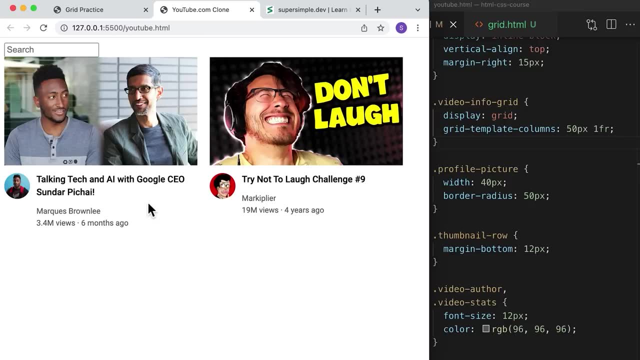 with the rest of our layout And now we can remove this background color and this part of the project is done. The last thing we're going to learn about grids is if we go to our final design, we're going to learn how to build a bigger. 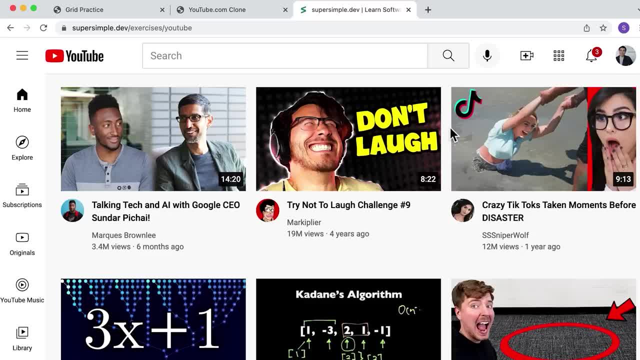 grid like this, So notice that there's a little bit of spacing between the columns as well as between the rows. Now, before we start, you might have a bigger screen and you might see four videos in each row. So for now, let's actually 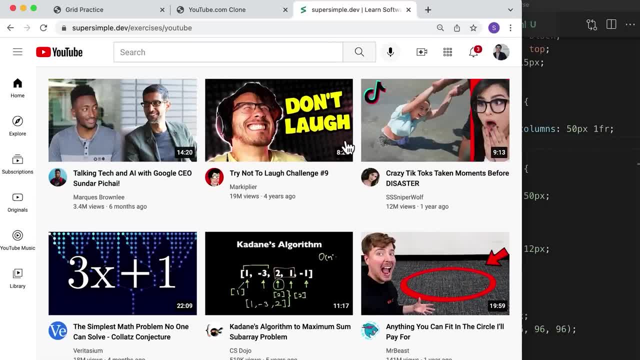 resize the browser so that we see three videos in each row. So I'm doing this because not everyone has a big screen to work with and this will make sure that everyone can follow along. So I'm going to zoom back in and just make sure. 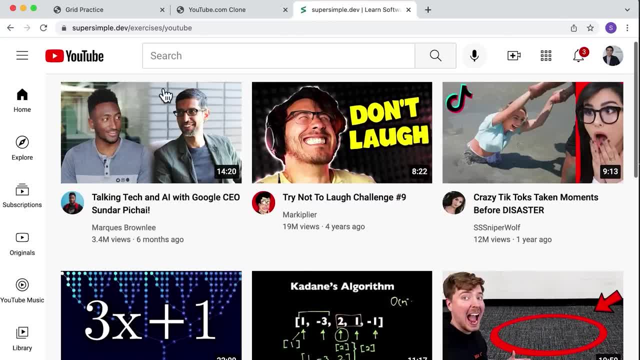 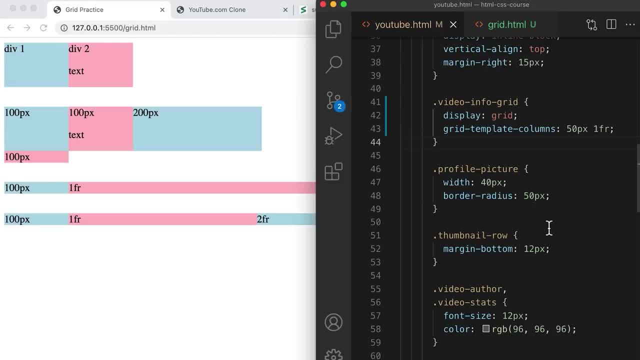 I have three videos in each row and we're going to learn how to create this kind of layout. Let's go into our grid practice file and we'll go back into our code again, and to our gridhtml file and we're going to create. 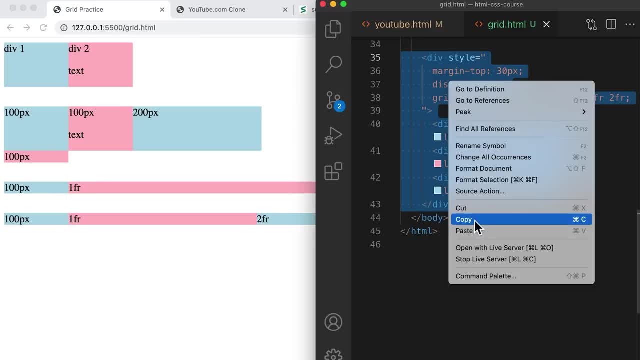 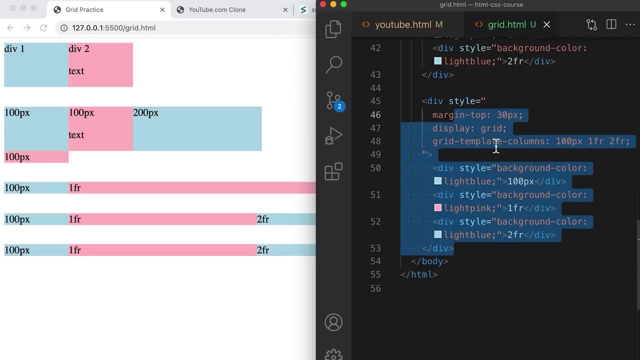 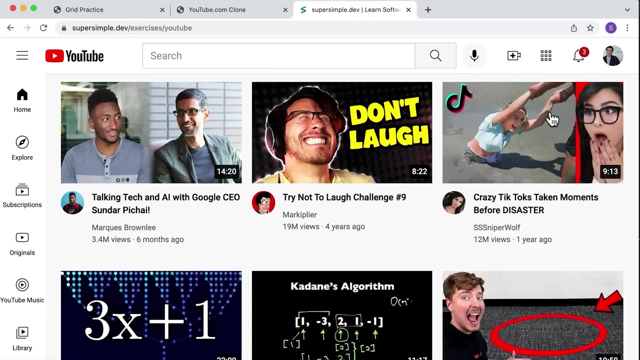 another grid to practice with. So let's copy this and then just paste it down here. And now, for this example, let's look at our final design. We essentially want three columns of equal size, And when we resize the page, notice that the columns resize. 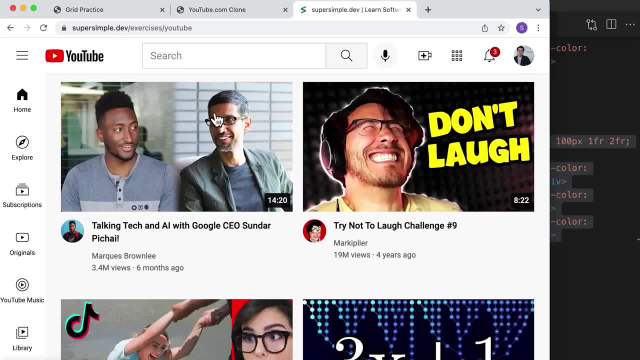 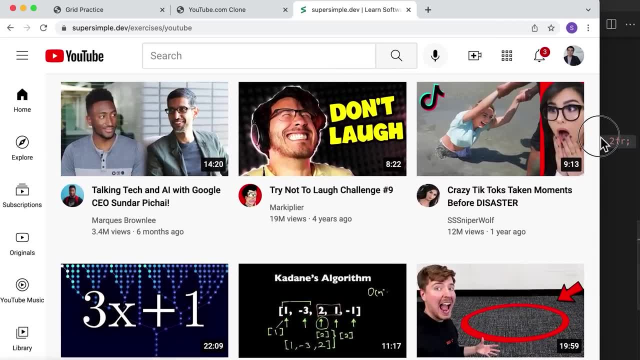 as well. So notice that if I resize too much, it becomes two columns. We're going to deal with this later in the course. We're not going to deal with that, We're just going to deal with three columns that we have here. So for 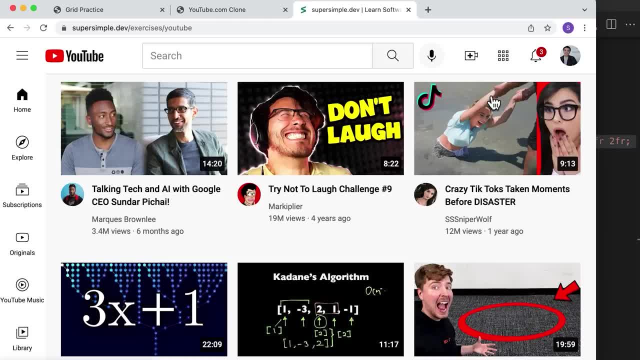 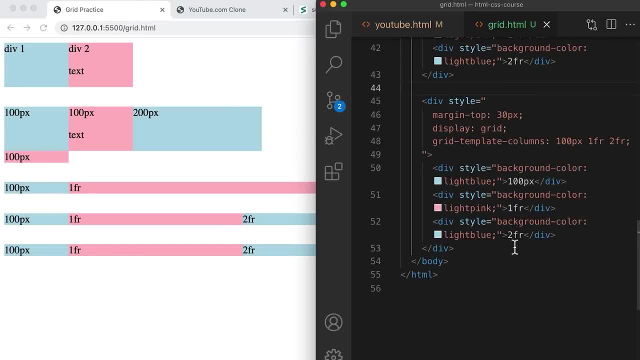 this layout. we want something like 1fr, 1fr and 1fr to divide this space evenly. Let's go into our file here and we're going to set three columns: 1fr, 1fr and. 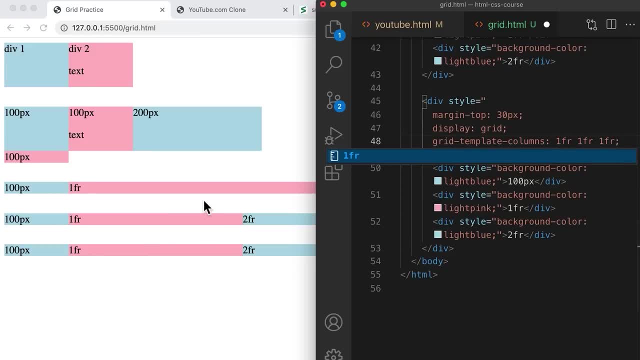 1fr. So this will create three equal columns that will resize with the page. Let's set this to 1fr as well, so that it's clear what's going on. Let's save it, and now we have the three columns we're going to. 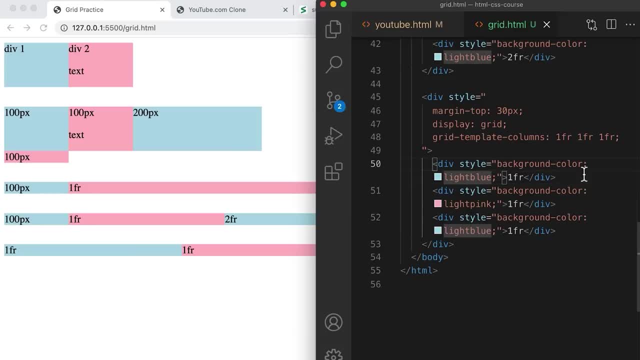 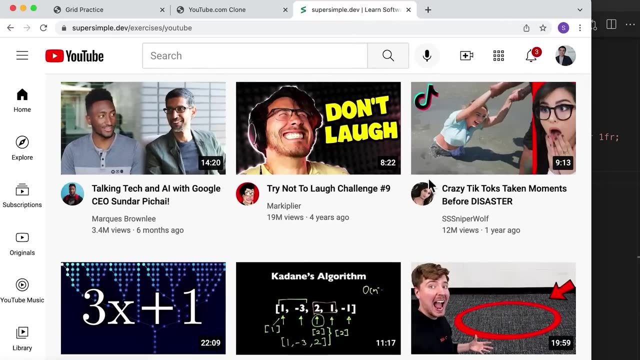 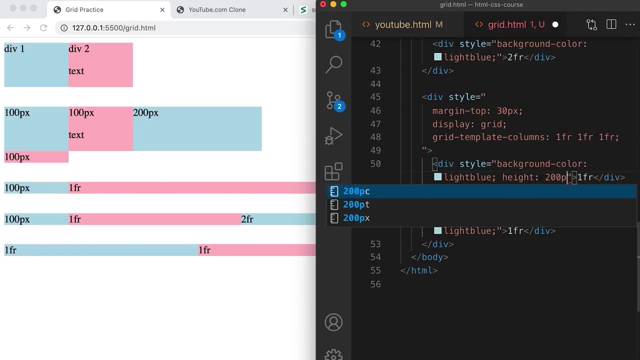 be working with. Let's also set the height so that it looks a little bit like our video previews that we have here. So let's go into our HTML file and we're going to set the height to 200 pixels And let's also set the height. 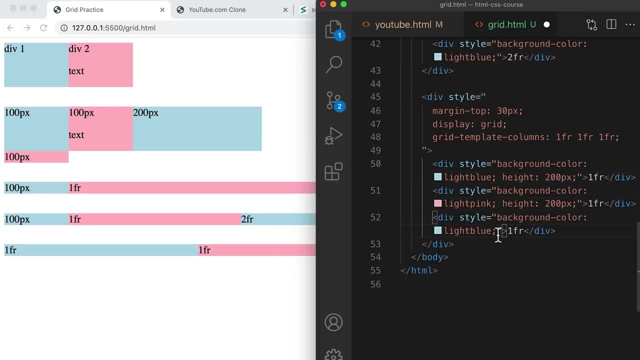 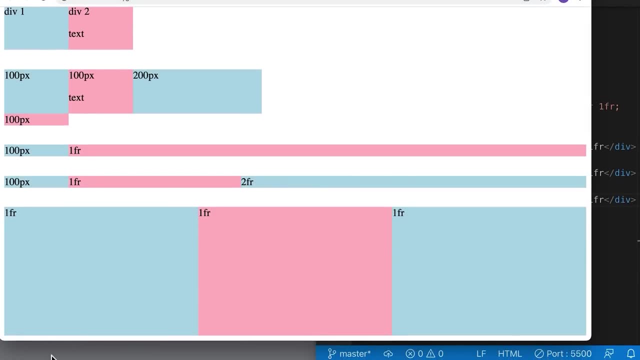 of these other columns as well. 200 pixels and 200.. Save it. Okay, so that looks pretty good, but there are a little bit too much at the bottom of the page. We're going to add some spacing at the bottom of the website so that. 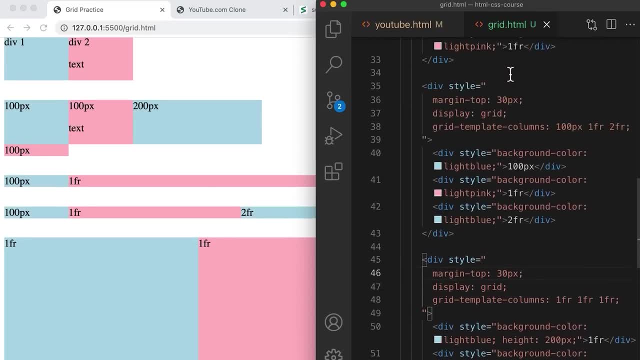 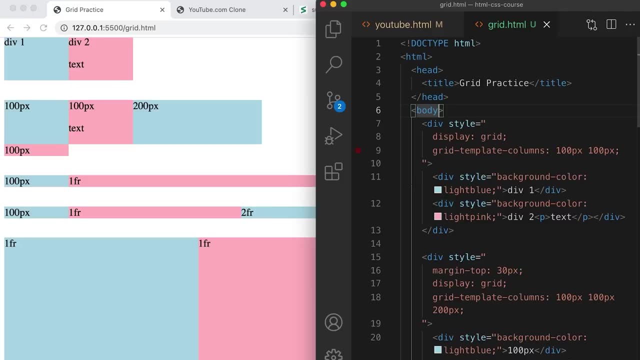 we can scroll these up. Let's go back up into our HTML and we're going to scroll up to the body tag. We're actually going to add some spacing inside the bottom of the body tag, So remember that spacing on the inside is called padding. 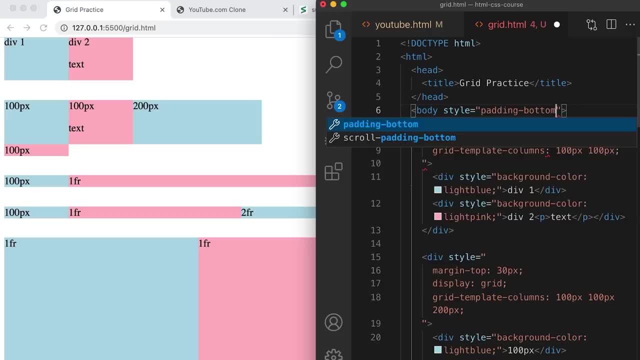 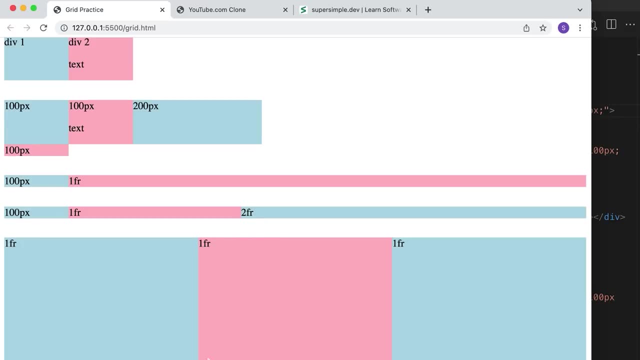 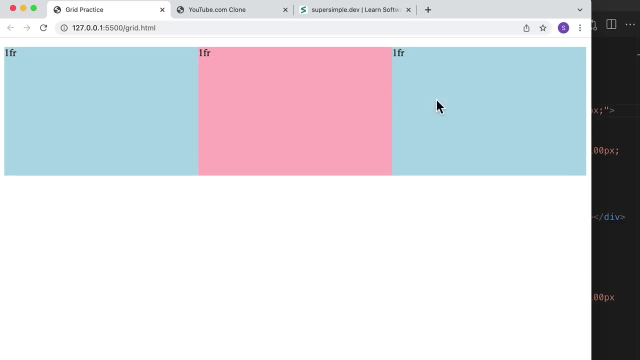 So padding dash bottom and let's set it to something like 1000 pixels So it's a lot easier for us to practice. So now that we have a lot of space at the bottom, we can scroll all the way up And see our grid clearly. 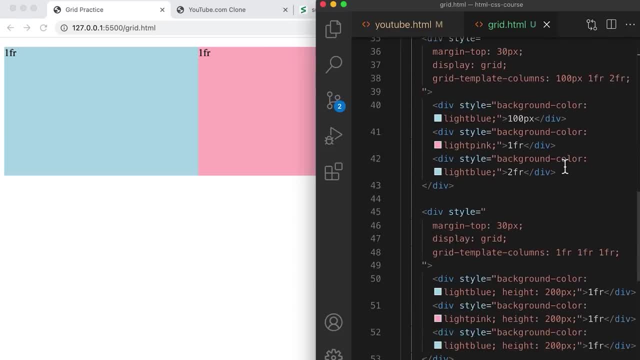 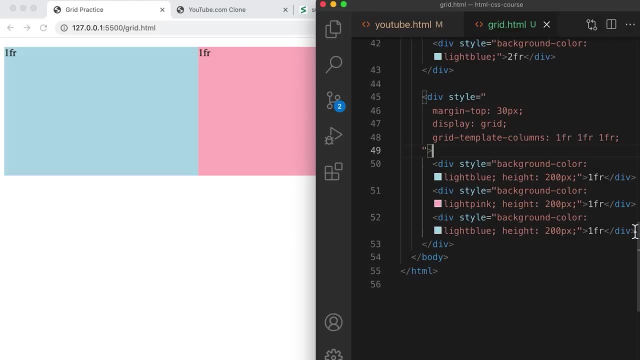 So remember that in a grid, if we have more elements than we have columns, it'll start wrapping around to the second row. So all we have to do is add three more divs. So we're just going to. let's actually copy the pink one first. 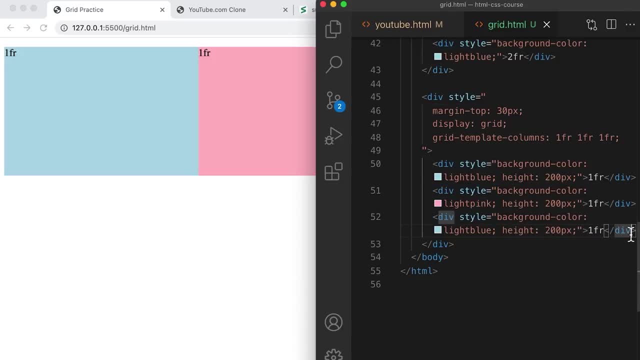 Let's copy it and paste it. And then we'll add a blue and a pink at the bottom. So let's copy and paste it. So we just need six divs to work with that have alternating colors like this. So let's save it. 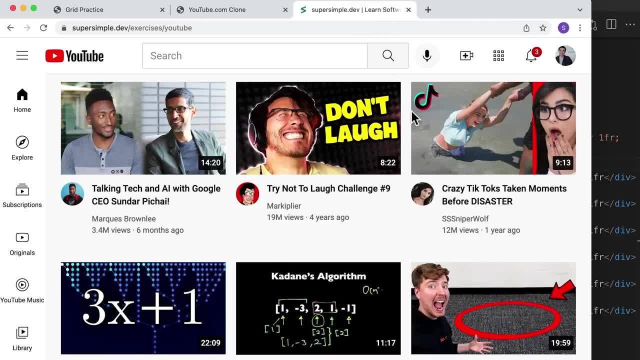 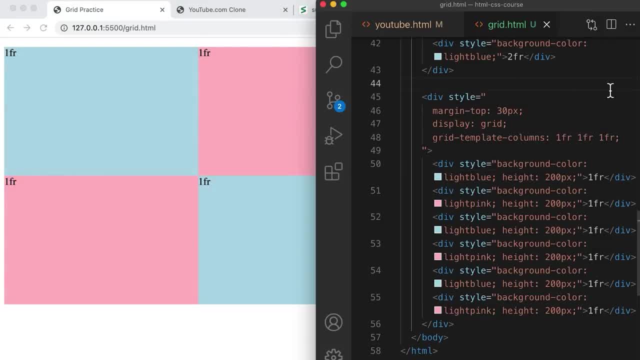 And now we essentially have our video preview that we see here, And we're going to learn how to create the space between the columns and the rows. So it's actually really easy to create this space. We just need two CSS properties. The first one is called: 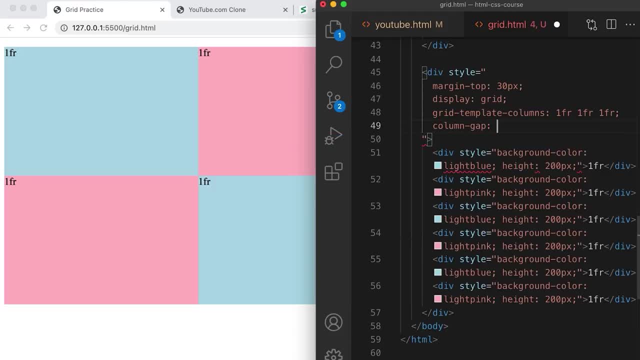 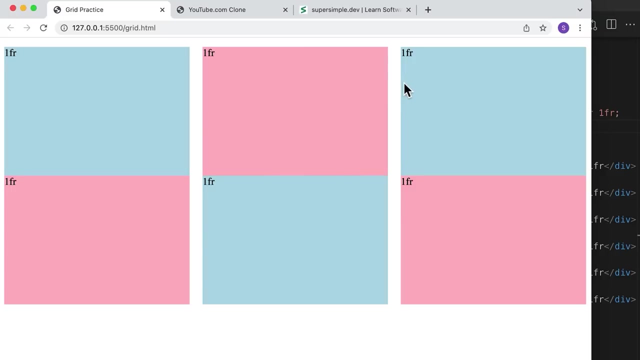 column-gap. So it's pretty straightforward what this means. We're setting some space or a gap between the columns. So let's set a column gap of 20 pixels. Let's see how that looks, Save it And now all of our columns have. 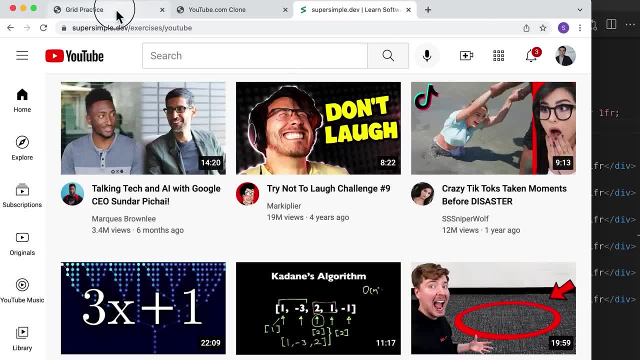 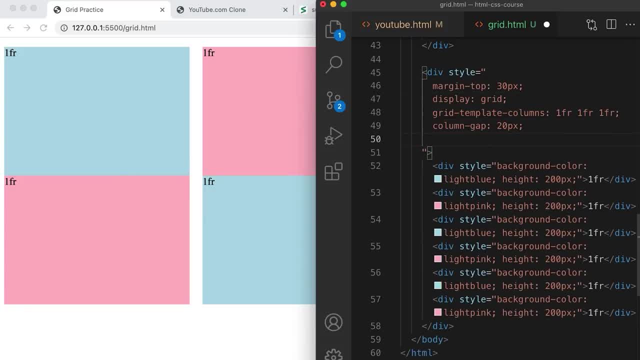 a gap, just like our final design here. Next, we're going to set the space between the rows, And we have a similar and straightforward property for that called row-gap, And let's set this to something like 40 pixels. Save it. 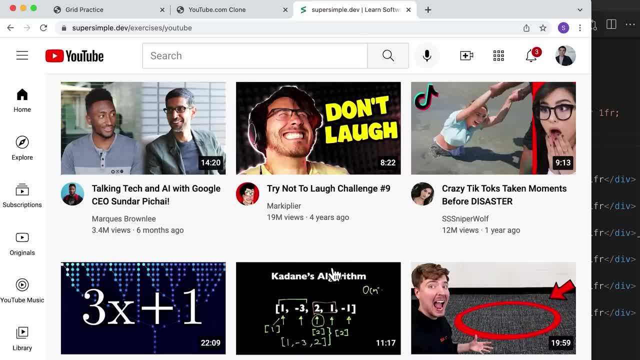 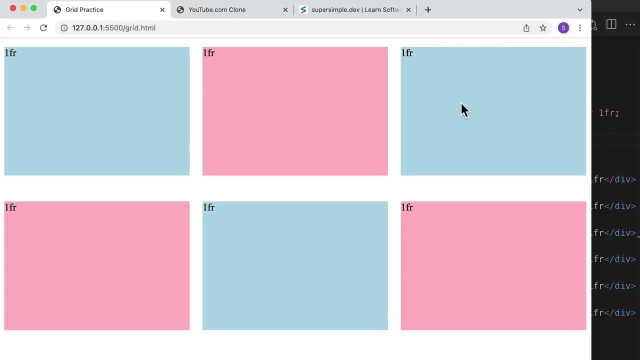 And now we have space between the rows, just like our final design. So that's how we create a grid like this. First, we define our three columns, So in this case, we want to divide it up into three equal columns that resize with the page. That's why we used 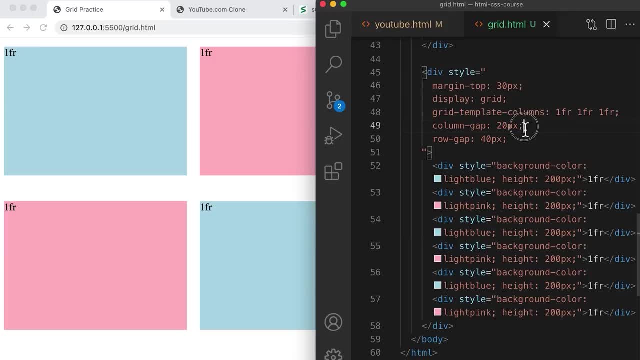 1fr, 1fr, 1fr. And then we just add some space between the columns, using column-gap, which creates this, And we add space between the rows, using row-gap, which creates this. Let's go back into our website. we were working on. 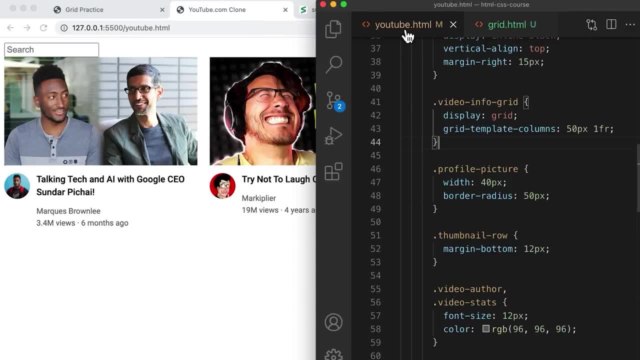 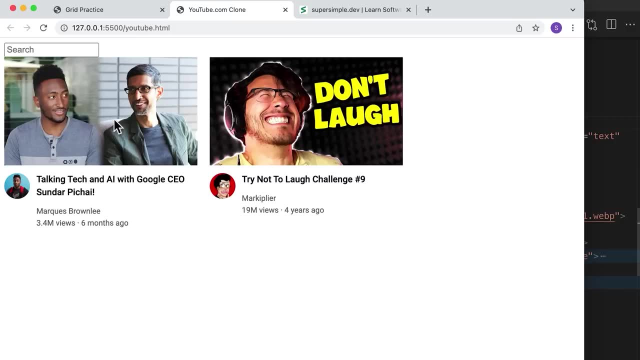 and we're going to apply these skills to here. Let's go back here, We're going to scroll down And first of all, let's just create six of these video previews So we can organize them into a grid that looks like this: Two rows. 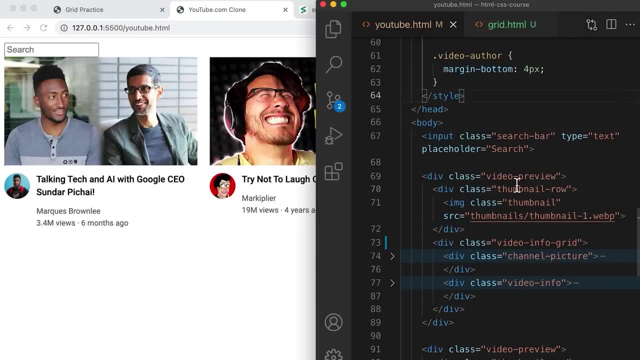 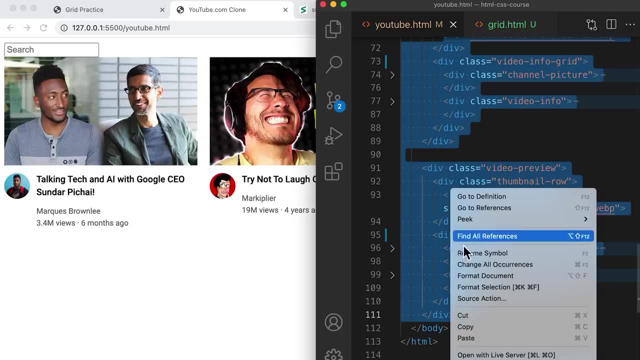 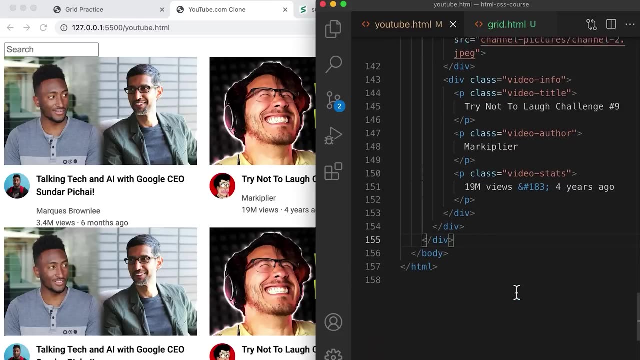 and three columns. So we're going to go into our code and we're going to copy both of these And we're just going to make duplicates. So copy it and paste it. So now, if we save, we have four And we're going to create. 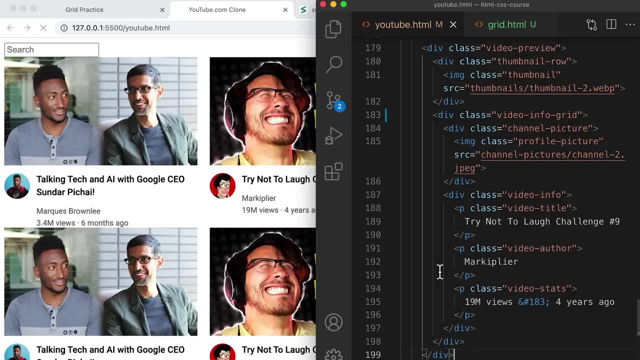 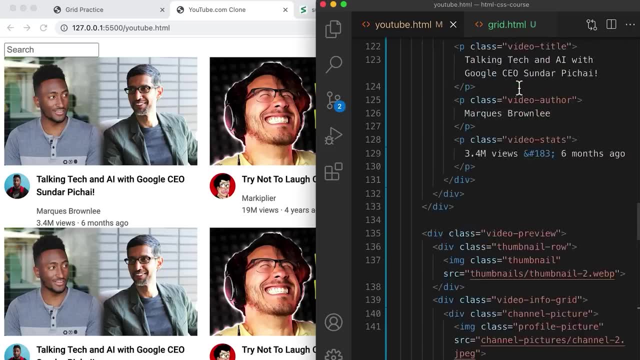 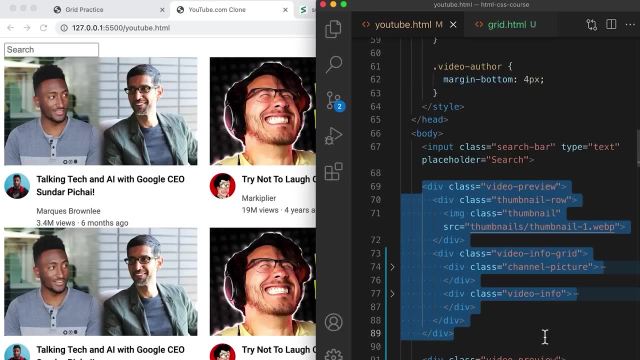 two more, So paste it again, Save, And now we have six. So remember to create a grid. we need a container, So we need a container for all of these video previews, So let's create a div and this is going to be our container. 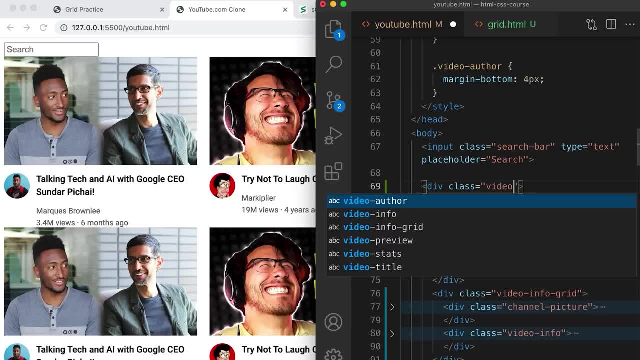 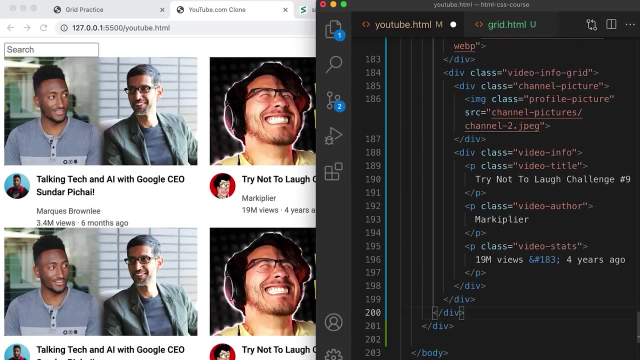 We're going to call this the video dash grid. And now let's move all of these video previews inside our new grid. Just going to move all of them, Cut it And paste it in here. Let's save it. Scroll back up. 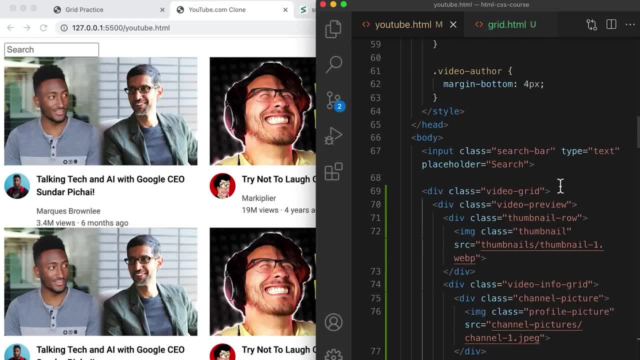 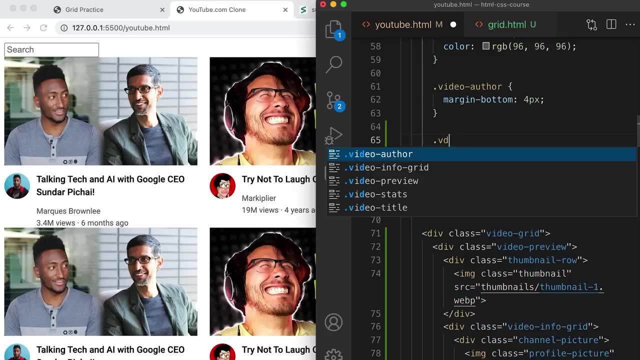 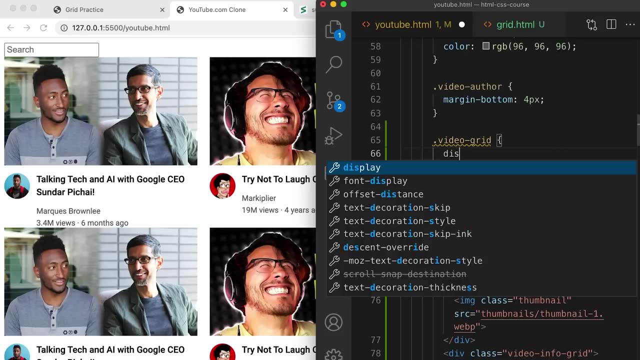 And now to create the grid. we want to set styles on this container element. So let's go into our CSS. We're going to target the video dash grid And remember we have two steps. The first step is to set the display to grid. 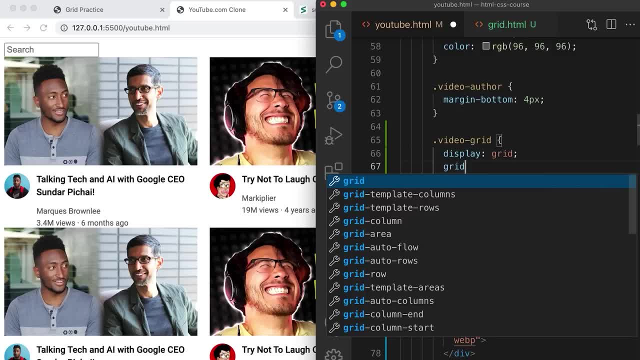 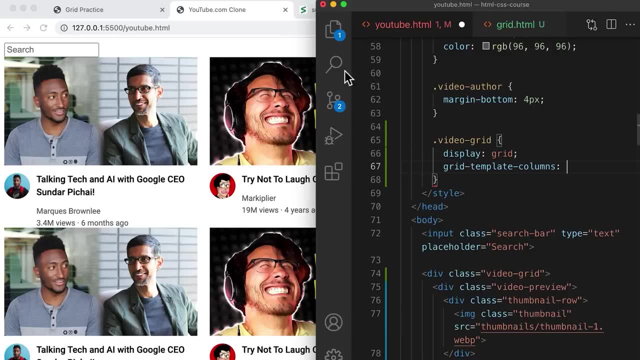 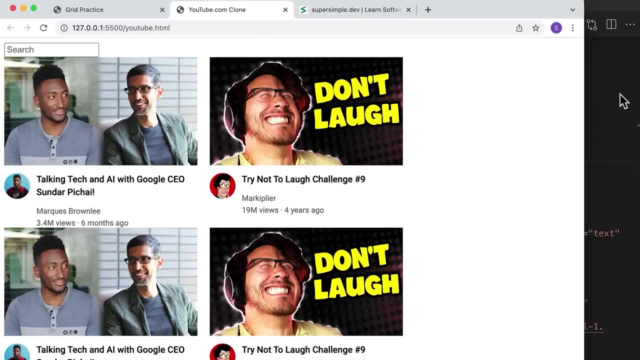 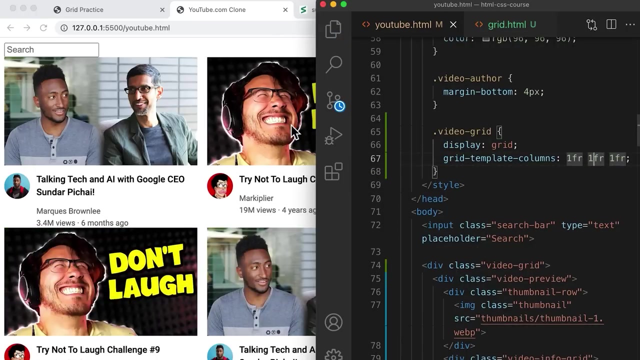 And the second step is to set how many columns. we have Grid dash, template dash columns And, for our example, we want three equal columns that take up the entire space. So let's set one fr, one fr and one fr. Now, if we look at our page, we now have: 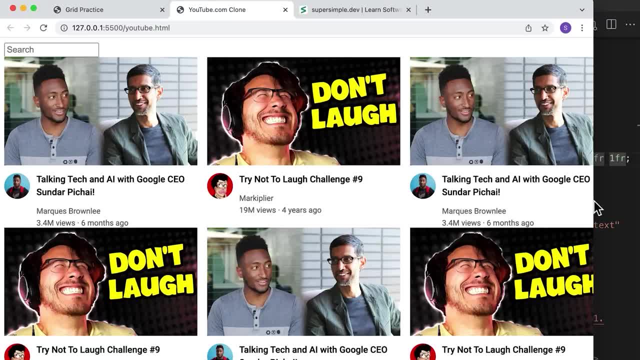 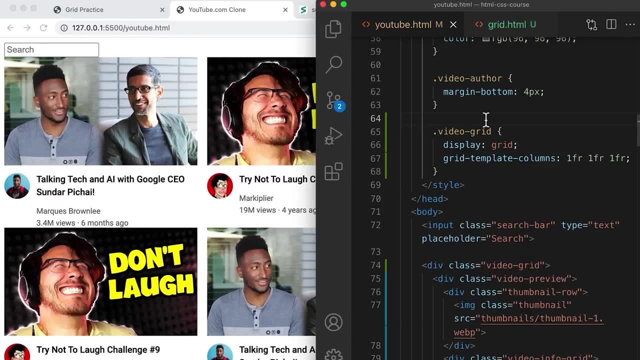 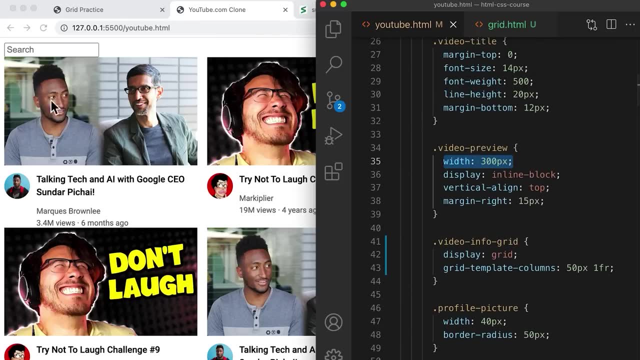 the three columns in our grid. But you might notice that if I resize this down, it actually doesn't resize with the page. So the reason this happens is because if we go and scroll up, we set a width on the video preview. Which sort of forces. 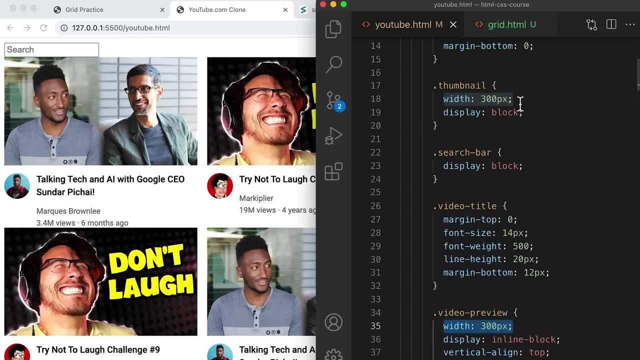 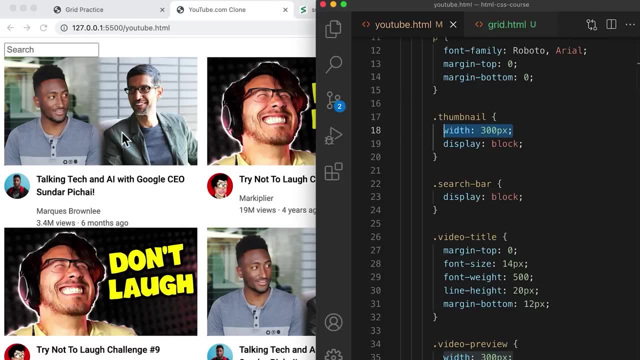 the width to be 300 pixels, And earlier we also set the width of the thumbnail to 300.. So instead of setting the width like this, which will force the width, we actually just want these elements to take up all the space in the columns that they're. 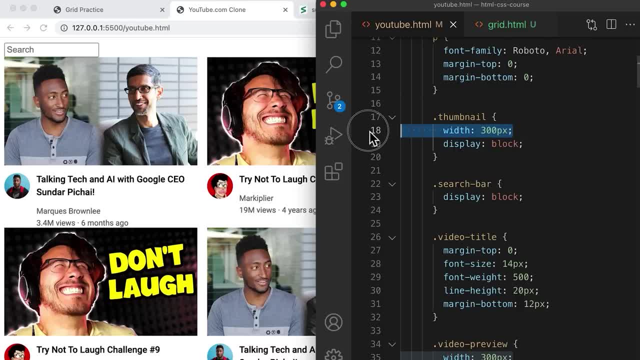 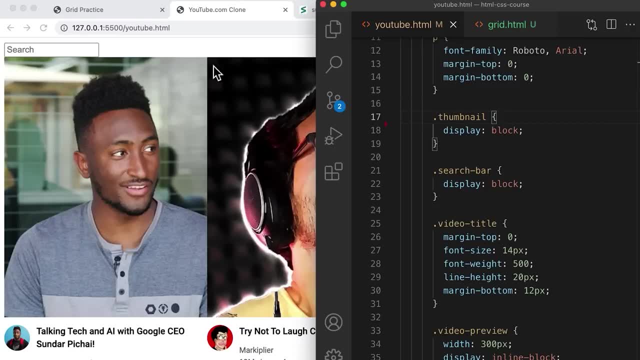 inside of. So to do that, we can remove this property here And let's save it. And for images, a weird behavior is that they always keep their original size To get them to fit inside their container or inside the column of the grid. 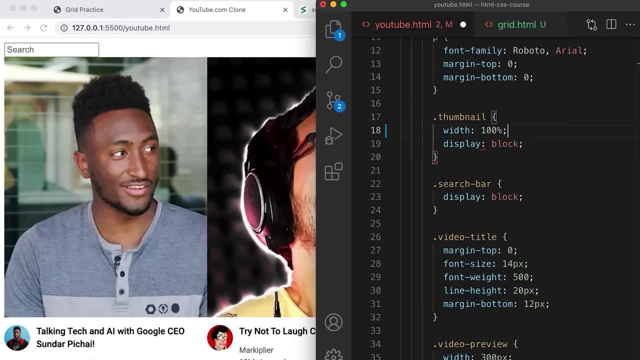 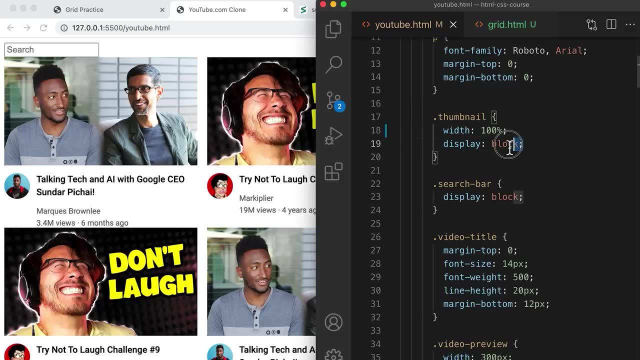 we have to set a width of 100%, Save it, And now they will only take up 100% of their container. Now we also don't need the display block here anymore. This image is taking up 100%. It's already on its own line, so display block. 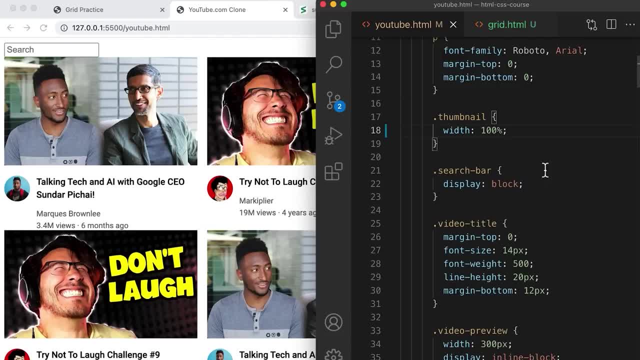 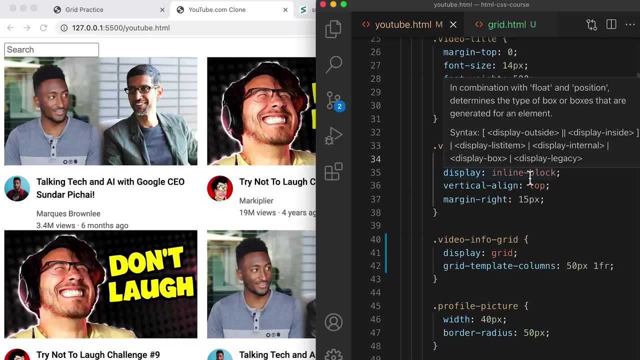 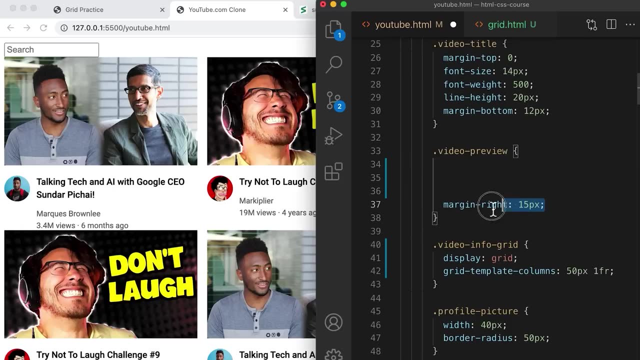 is not necessary. Let's delete that. And now we're going to deal with this video preview width. For this we can just get rid of the width here and the display inline block and also vertical line which relates to inline block, And we can get rid of. 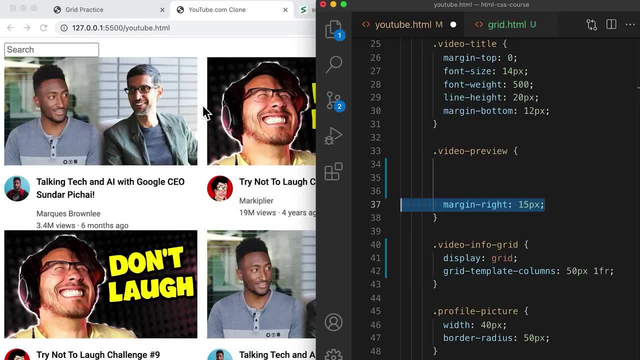 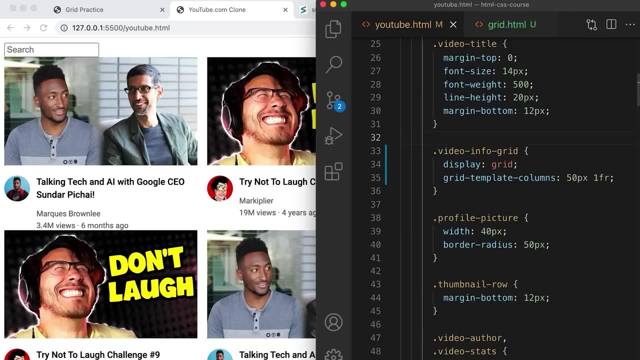 the margin, since we're going to create this space using the column gap property we learned earlier. So let's just get rid of all of these styles. And now, if we save, we can now see that our video previews are fitting perfectly inside of our 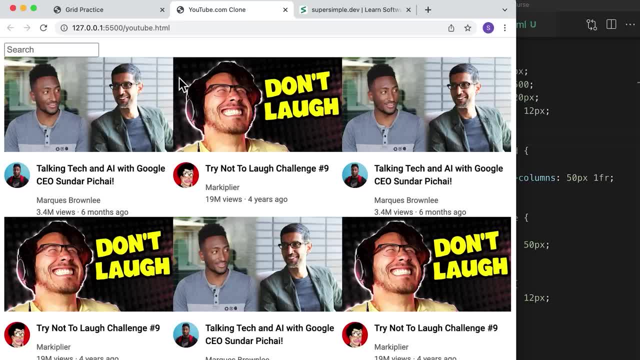 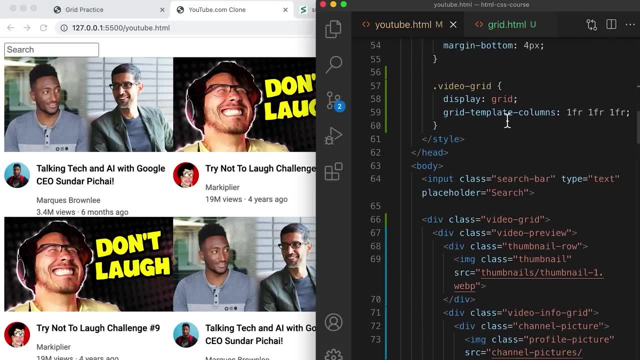 grid. The final step is we're going to add some space to the columns and to the rows, So let's go into our CSS here and remember the two properties. they're pretty straightforward are column-gap, and let's set a column gap. 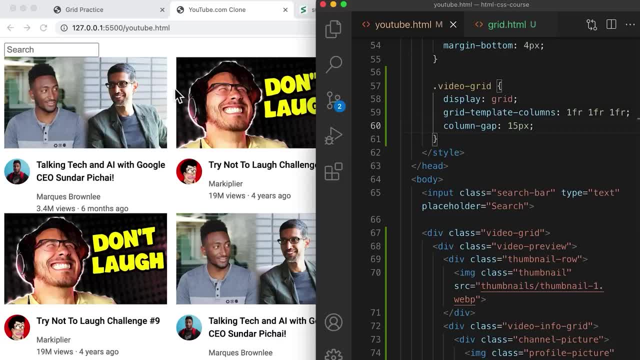 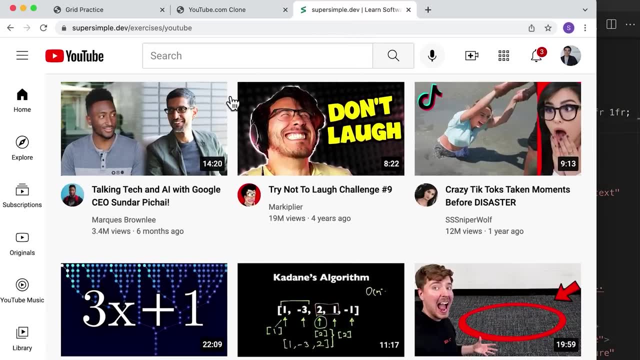 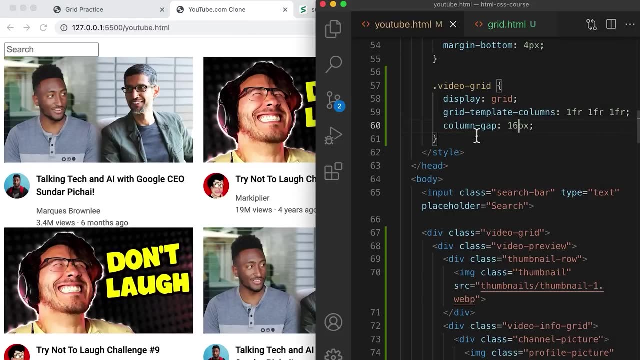 of maybe 15 pixels. Save it. Okay, let's compare that to our design And I'm going to resize it a little bit. So I think this looks pretty close to what we have, Maybe 16 pixels, Okay, and then we're going to set. 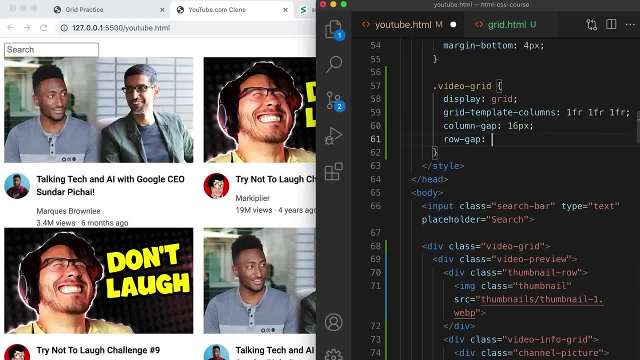 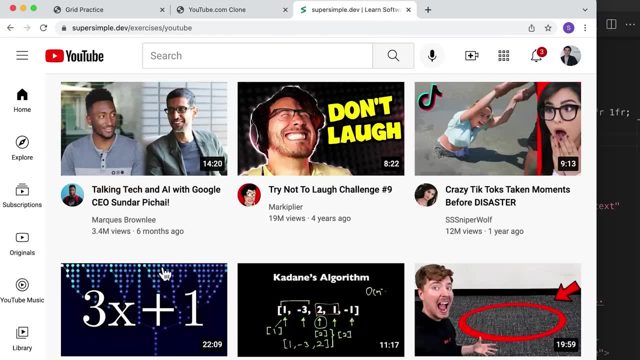 a row gap. Let's set a row-gap of maybe 40.. Save it and compare it to our design. So I think that looks pretty close to what we have Now. the design might look a little bit smaller and that's because we have the sidebar here. 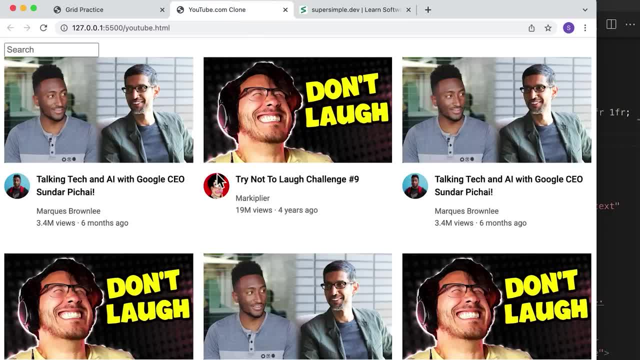 but we're going to deal with that in a later lesson, So for now, this looks perfect. The last thing we're going to do is to swap out the thumbnails, the channel profile pictures as well as the rest of the text to match. 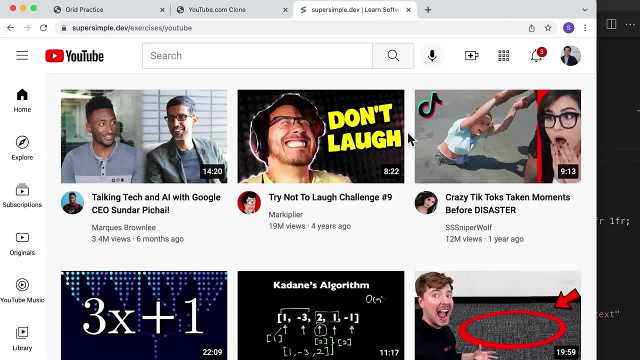 our design, So I'll let you get some practice doing that. Remember, you'll have to download the thumbnail and the channel profile picture first. For now let's just do six of these videos and then we can add the rest of them at the end of the course. 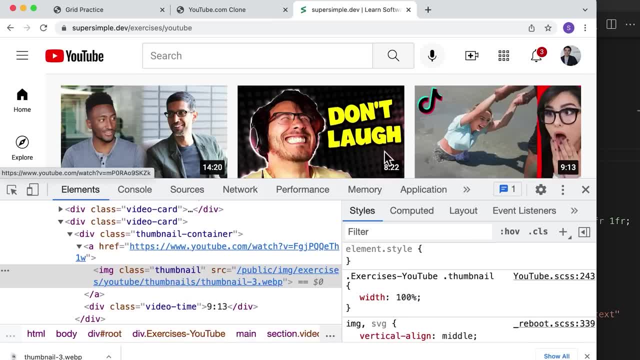 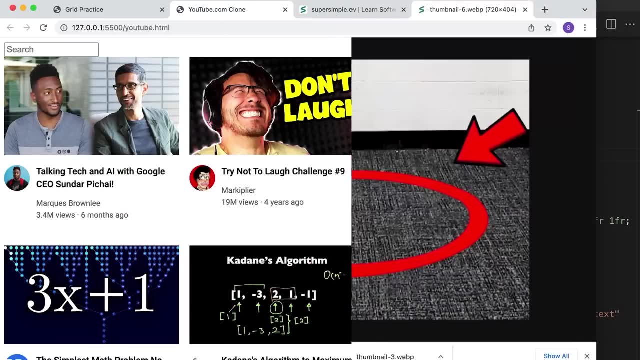 So pause the video right now and swap out all the thumbnails, the channel pictures and the text, And I'll see you back after you've done that. So this is what it looks like after I swapped everything out. So that's the end of this lesson We learned about. 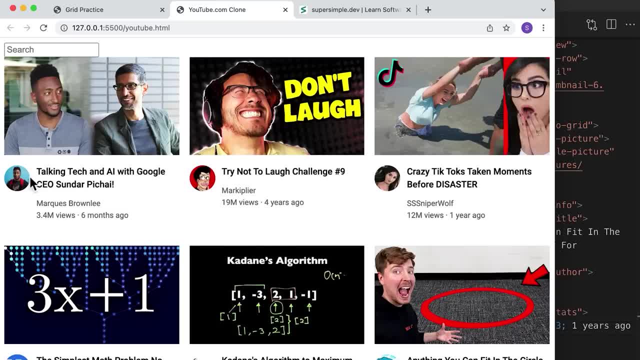 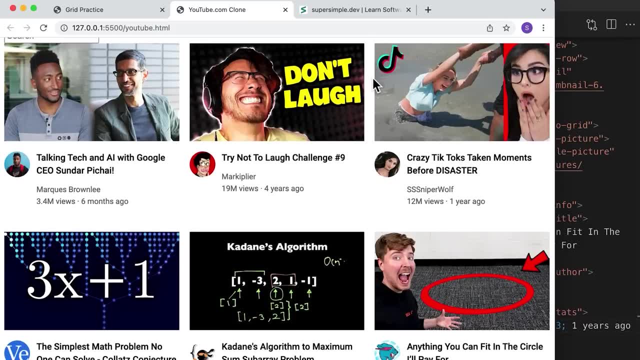 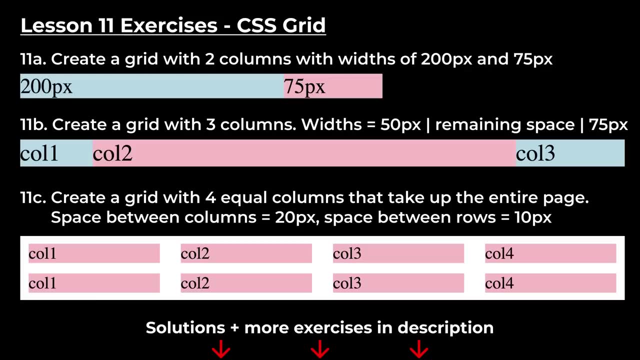 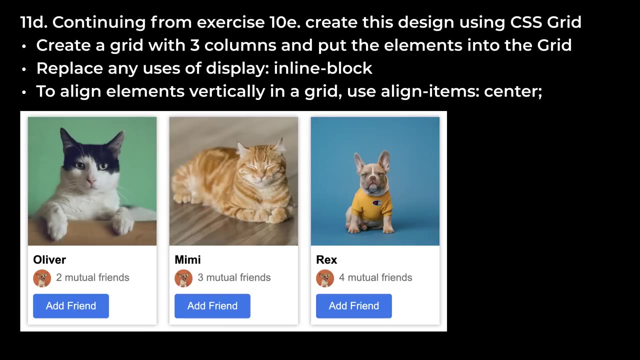 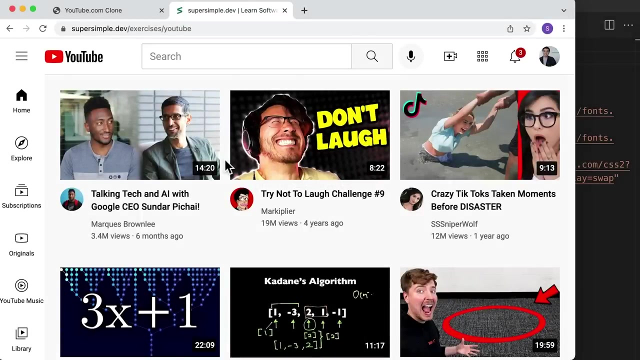 CSS Grid, which is a great way to create these horizontal layouts that are perfectly aligned and to create this bigger grid that we see here. Here's some exercises to get yourself familiar with grids. In this lesson, we're going to learn about Flexbox, which is another way to 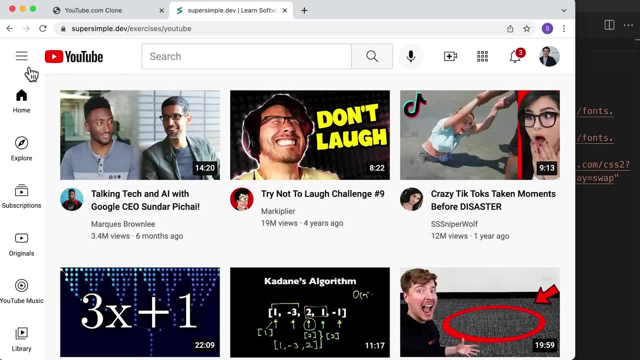 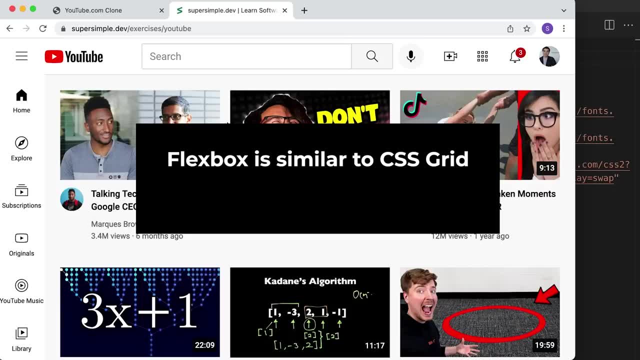 create layouts And we're going to use Flexbox to create the header at the top of the page. So Flexbox is similar to CSS Grid: It can create the same kind of layouts, but it's more flexible. Just like the previous lesson, let's go into our code and create: 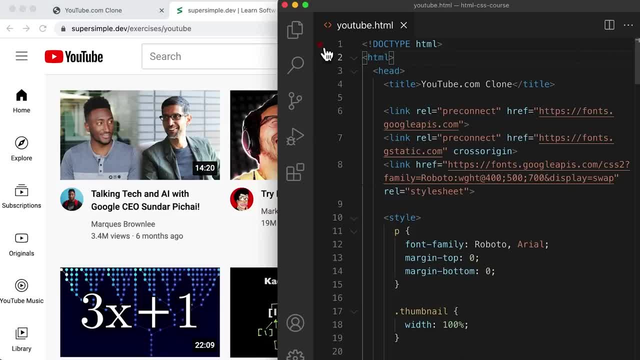 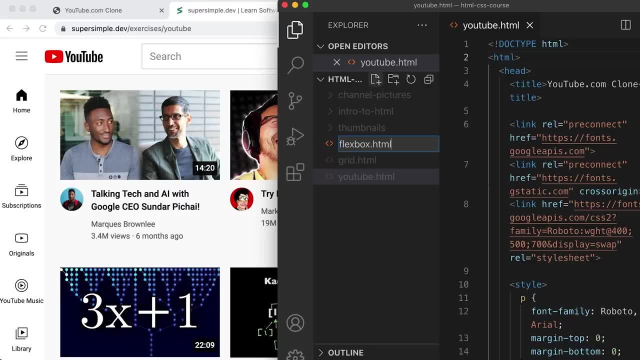 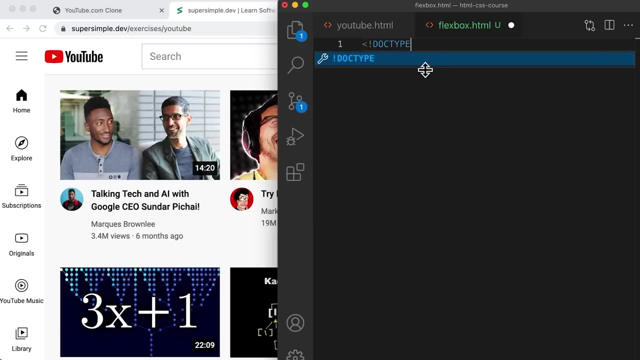 a new file just to practice, Flexbox. We're going to create a new file by clicking this icon and let's call it flexboxhtml. And remember we always start with the HTML structure. We're going to have a doc type at the top. 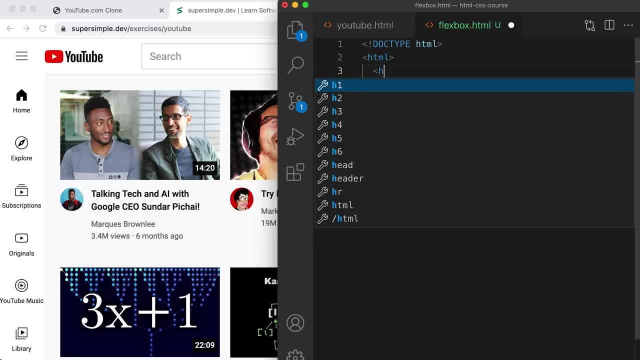 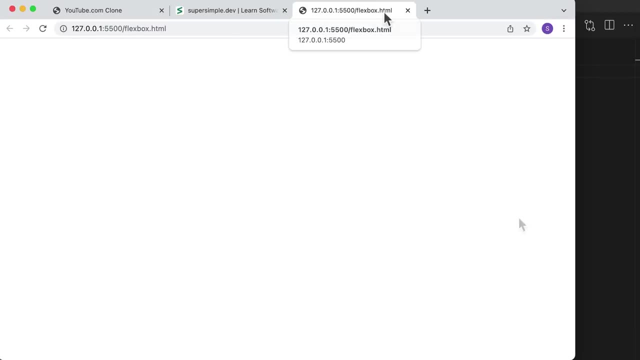 and then an HTML element, a head element and a body element. Let's save it, and now we can open this in Live Server. So right-click and open with Live Server. Now in this lesson we're also going to compare Flexbox to Grid. 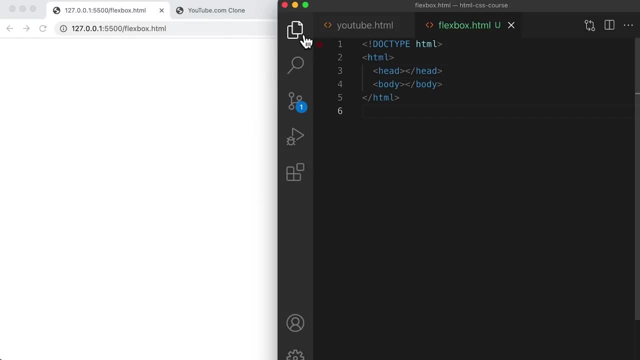 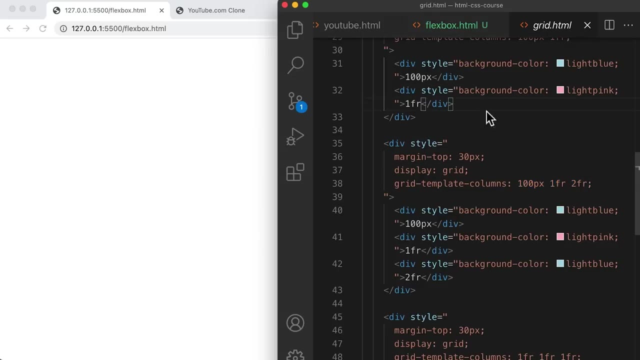 to show what the similarities and differences are. So we're also going to go into our code and open the Gridhtml from the previous lesson, and we're also going to open this in Live Server. So right-click and open with Live Server. 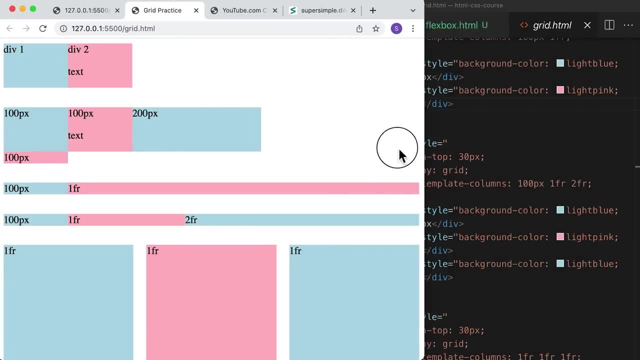 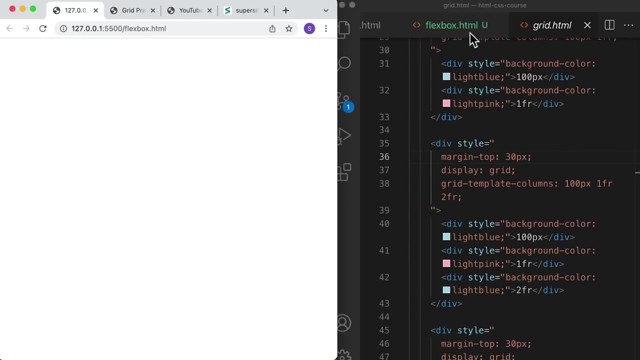 Just going to move these beside each other and resize the page, And now we're ready to be in. So we're going to start off in our flexboxhtml and first we're going to go into the head section and we're going to 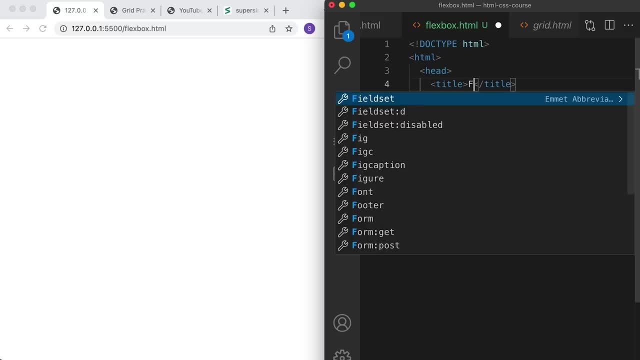 add a title- Let's call this flexbox-practice- and then save. So this is just going to remind us that this file is for flexbox-practice, and it's going to show up here. Next we're going to go into the body. 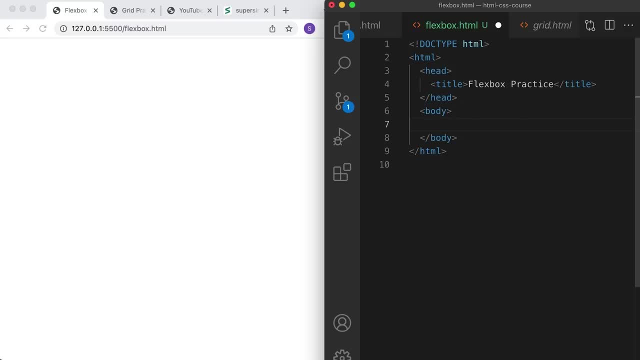 and start creating some flexboxes. So, just like for Grid, we're going to create a div and inside we're going to have two divs, So div1, and div2.. So we're going to use inline CSS, again just like we did for Grid. 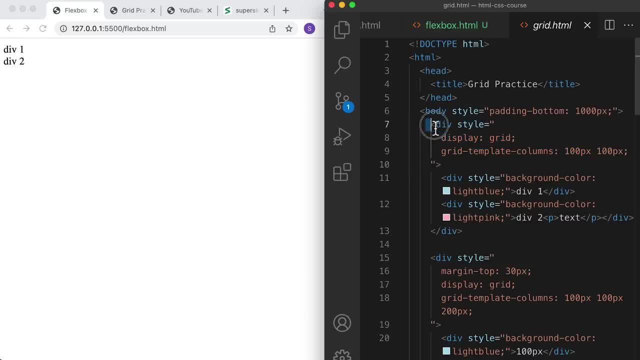 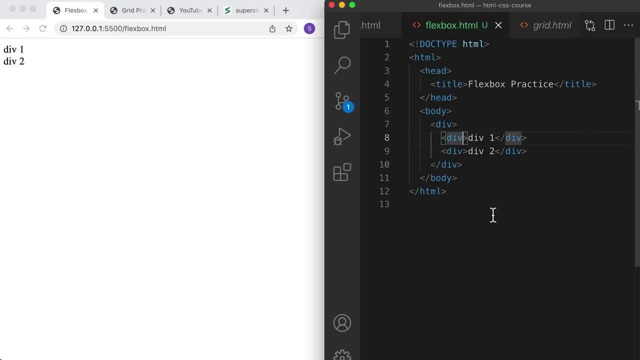 like here, so that we keep our CSS code close to our HTML code and it'll be easier to understand what's going on when we review this file in the future. So inside our div let's set a style and for this div we're going to set the background color. 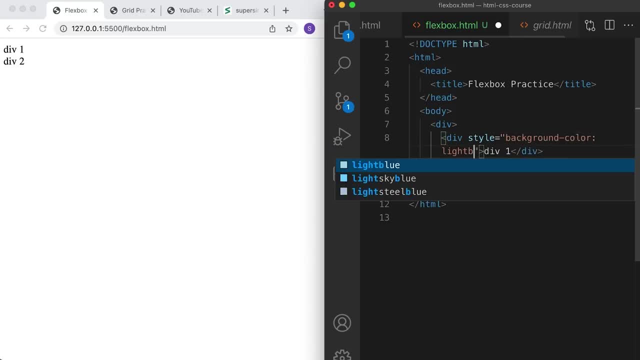 to light blue, like before, And then for the second div, we'll also set it to light pink. So style equals background dash color: light pink, Save it. And now we have the two divs we can work with, So just like with Grid. flexbox requires a. 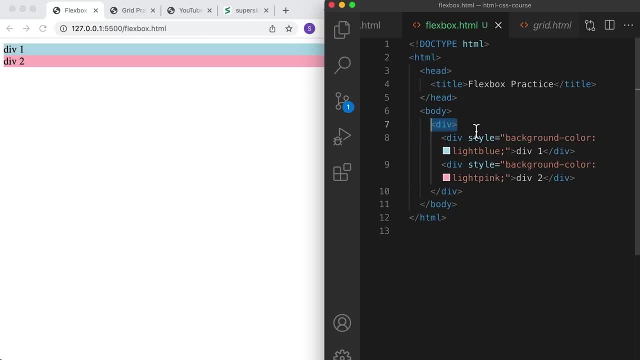 container or this outer div. This container is going to be the flexbox, and then these elements are going to be placed into our flexbox. So now let's learn how to turn our container into a flexbox. We're going to set a style here. 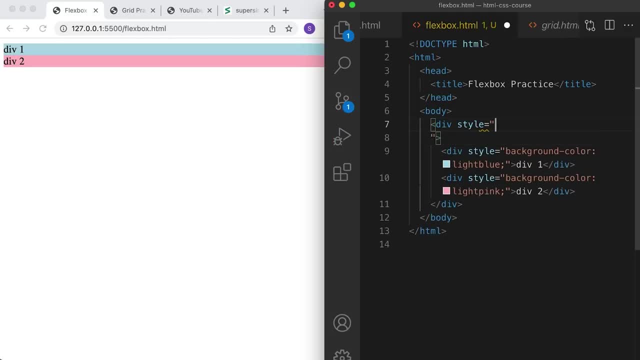 and we're going to do two steps. The first one is to set the display property to flex. This creates a flexbox. And the second step: we're going to set the flex dash direction to row. This means we're going to align these elements horizontally. 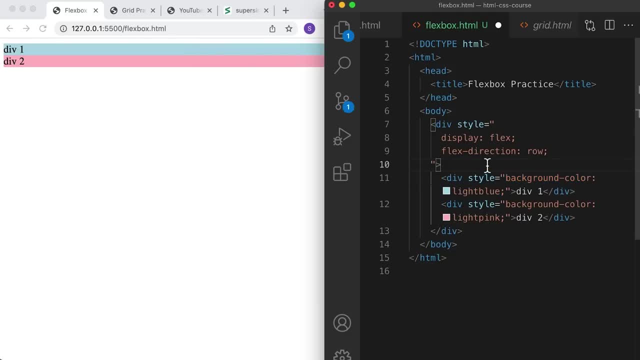 in a horizontal layout. So now let's save this file and we can see the effect that flexbox has. So inside of flexbox, these divs, which are block elements, don't behave like block elements anymore. They behave more like inline block elements. 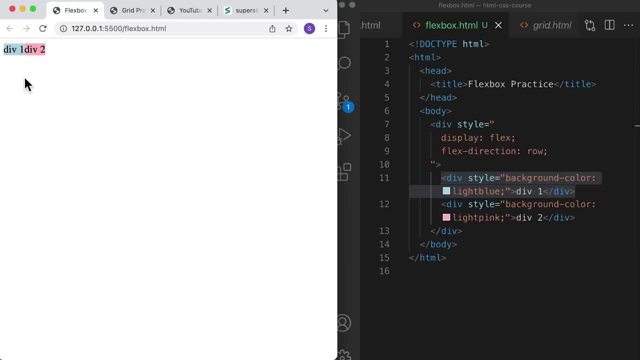 They only take up as much horizontal space as they need to. Now compare that to Grid, where we first set the columns and then the elements went inside the columns. So the layout is a little more rigid for Grid If we go back to our flexbox. 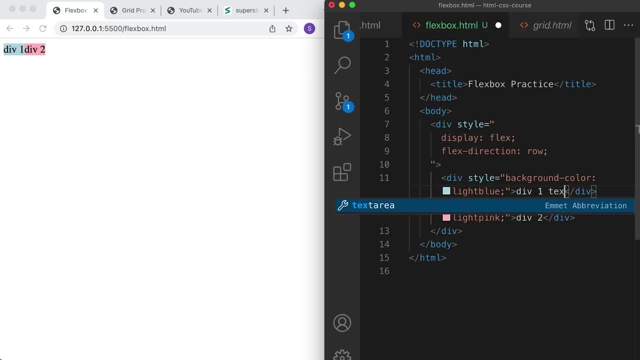 if we add some more text to this first div and save, notice that it expands to take up as much space as it needs to. So this is a flexible box and that's why we call it flexbox. Now there's one other thing I want to point out about flexbox. 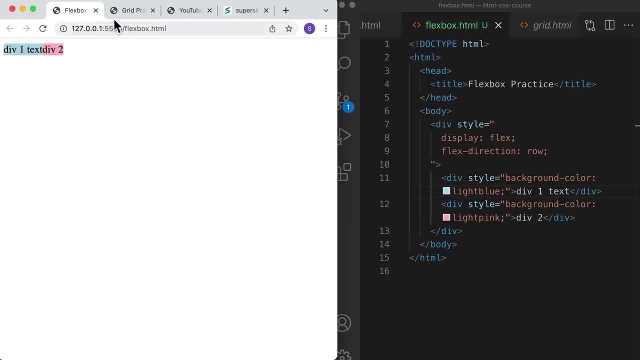 is that if we make this second div taller, just like our Grid example here, the flexbox will be vertically aligned. Let's go into our code and let's add a paragraph to make this div taller. If I save it, you'll see that it got taller, but we still. 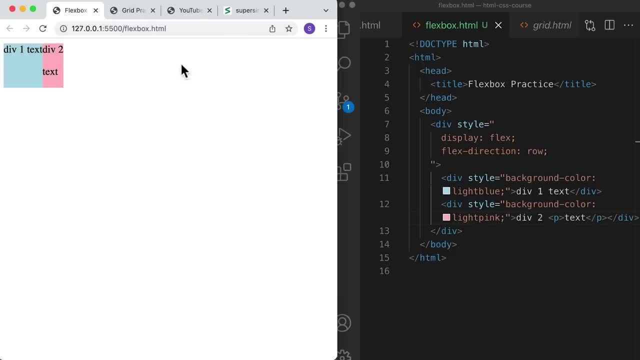 maintain vertical alignment. So flexbox is another way to create these horizontal layouts while maintaining alignment. Alright, let's go through some more examples to see the similarities and differences between flexbox and Grid. We'll start with the similarities first, We'll go into our code and we're going to create. 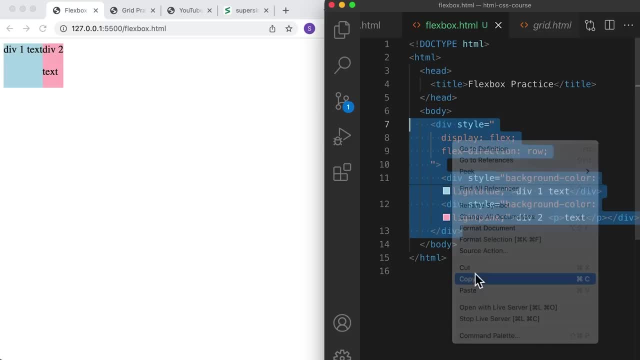 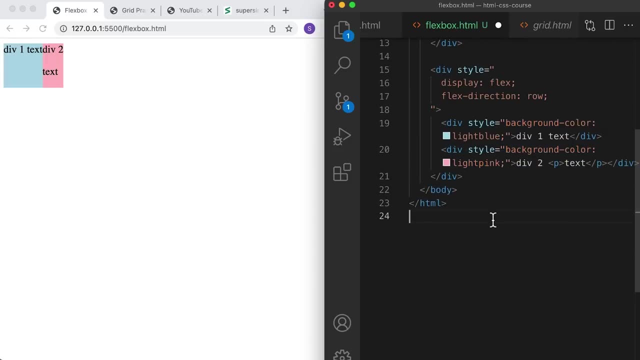 another flexbox to practice with, So we'll just copy this and then paste it down here. I'm going to select this and press tab Now scroll down. So we'll also add some spacing to the top of this, because we want to make it easier to separate. 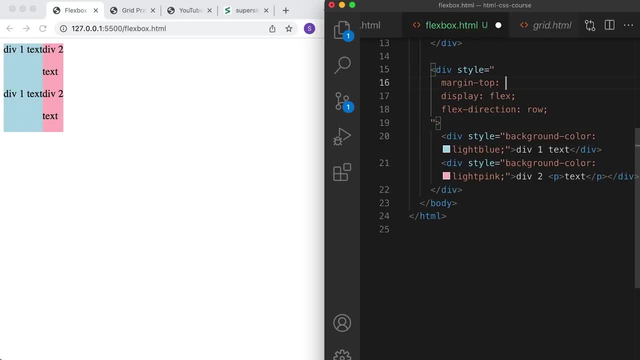 So let's add some margin dash top of 30 pixels. Save it. That looks pretty good. And now for this first div, we're going to set the width to 100 pixels. I'm just going to organize my CSS a little bit here. 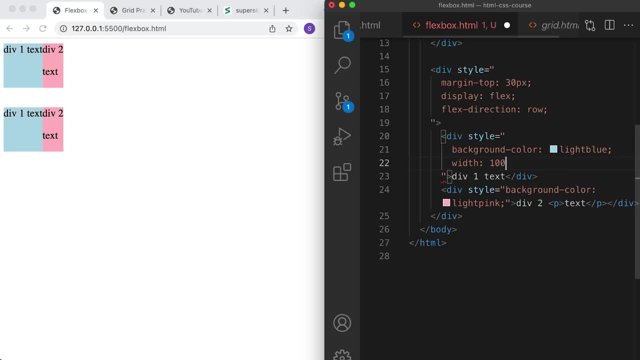 And we're going to set the width to 100 pixels And let's also change the text to 100 pixels so that we know what's going on. So let's save it. So now our first flexbox element is 100 pixels wide. 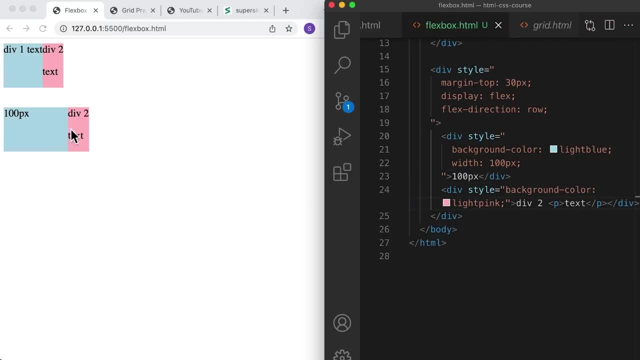 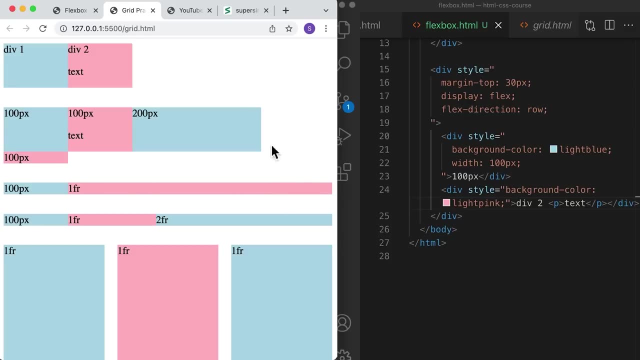 For the second div, we're going to tell it to take up the remaining amount of space. So if you remember, from grid that's equivalent to 1fr. We're going to learn how to do that in flexbox. So for this one, 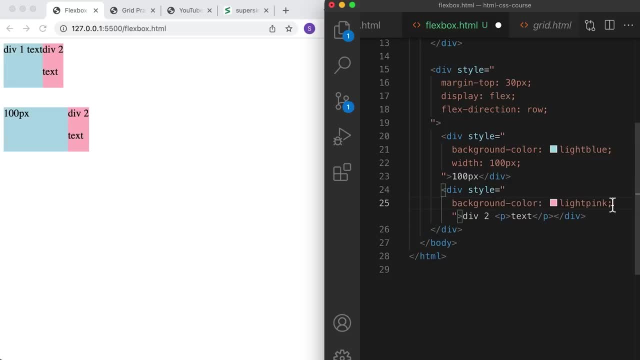 in our code. we're going to add a new style And we're going to add a style specific to flexbox called flex, And we're going to set this to 1.. And we're also going to change this text here to flex. 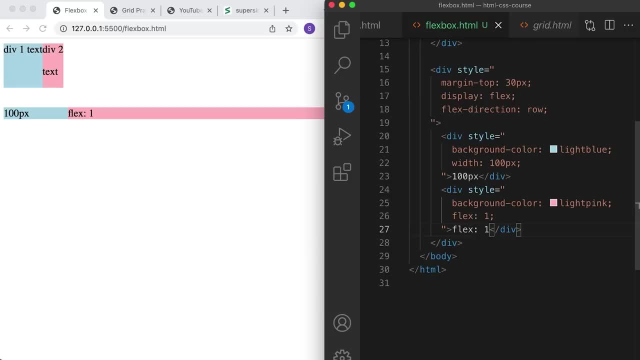 1. Let's save it. And now we can see that flex1 causes this div to take up the remaining amount of space. So flex1 is the flexbox equivalent to 1fr in grid. So let's go through another example. 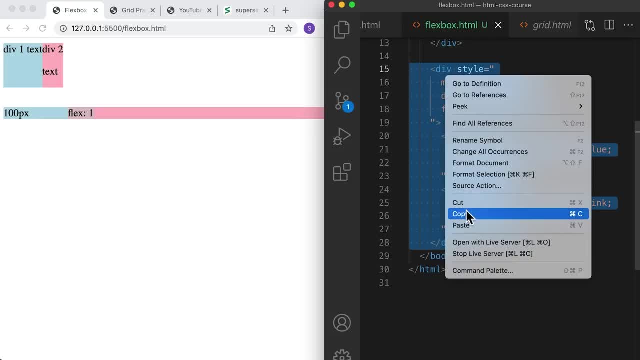 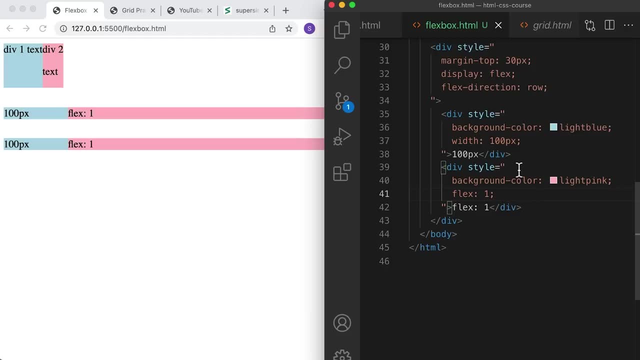 We're going to copy this and then paste it again And for this example, we're going to add another div to the bottom here. So let's copy this first div, Copy it and paste so that we have alternating colors, And then we're going to set the flex on. 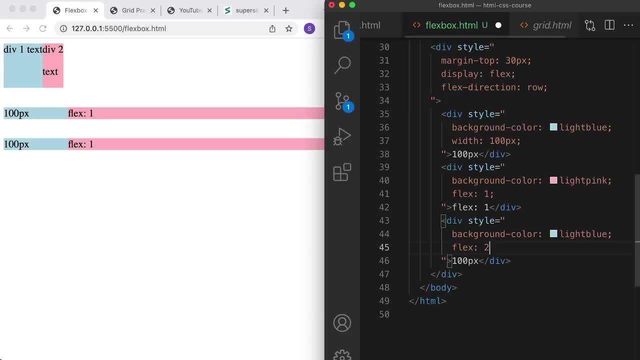 the second div to flex2.. Let's change the text to flex2.. So you can see that flex2 is the equivalent of 2fr in grid. So two items that both have flex are going to take up the remaining amount of space. 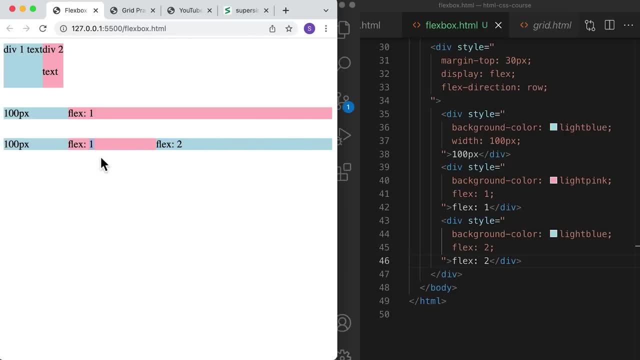 But this number here tells us relatively how much of the remaining space it takes. So this element with flex2 is going to take twice the amount of the remaining space as this element with flex1.. So the value here works the same as the value with fr. 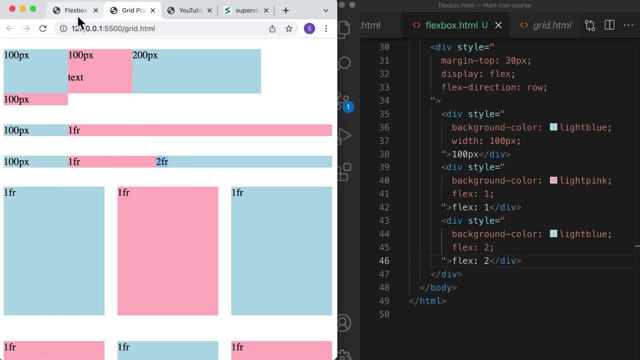 So you can see that the basic things that we do with grid we can also do with flexbox. Now let's talk about the differences. So if we go to our grid examples and we look at this example here, the layout is more rigid for grid. 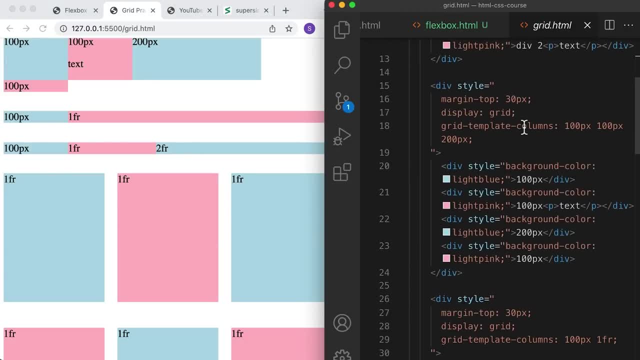 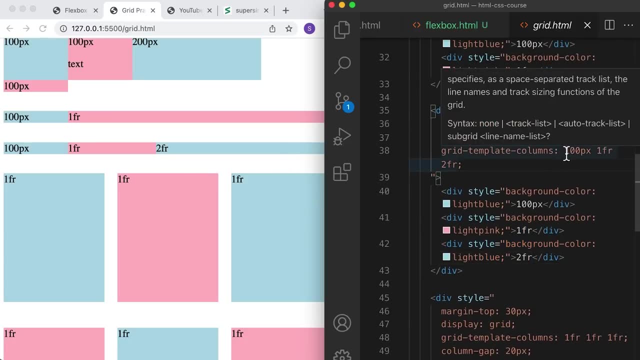 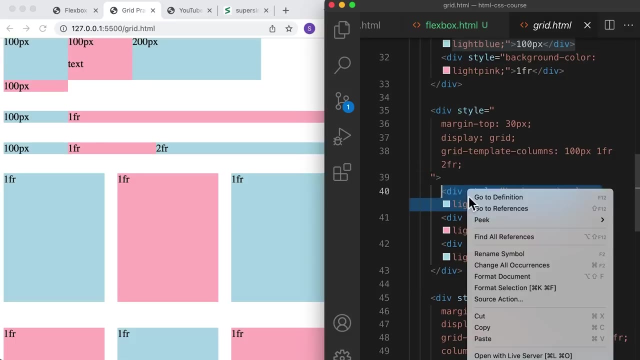 If we go into our grid code and we scroll down to this example which is right here- 1fr and 2fr- you'll see that we first define three columns And then these elements go into those columns. So if I move this element, 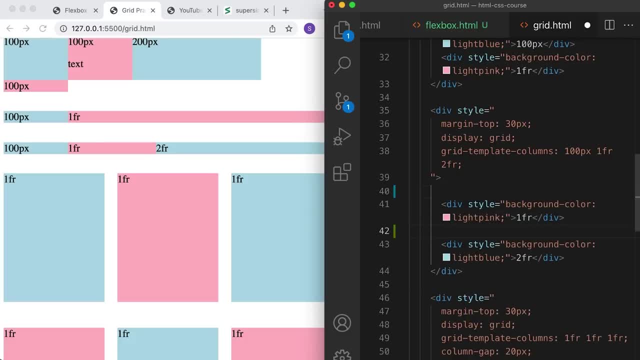 to the second position. I'm just going to cut and move it down here. this item is now going to go into the second column and it's going to take up 1fr of space, even though we wrote 100 pixels here. So if I save this, you'll see that this 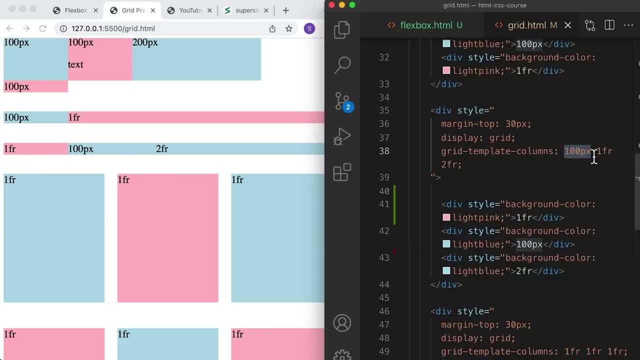 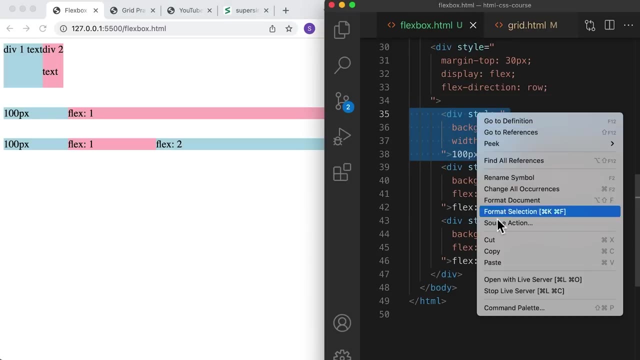 1fr element goes into the 100 pixel column, so it only takes up 100 pixels of space And the layout here is not changing For flexbox, however, if we go to our flexbox example and our code, if we change the order of the elements. so let's cut this. 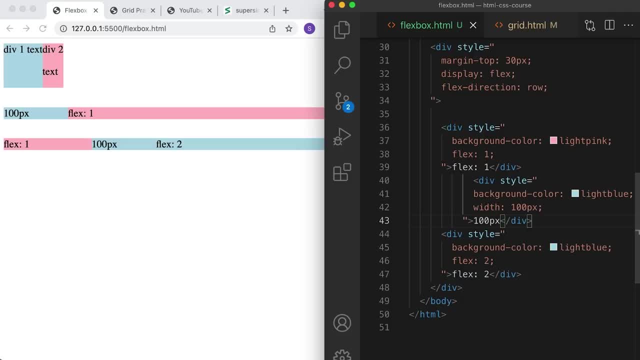 and paste it down here and save it, you'll notice that the layout actually changes. So this element here actually keeps its width of flex1, and then the second element keeps its width of 100 pixels. So the elements take their width along with them if they move around. 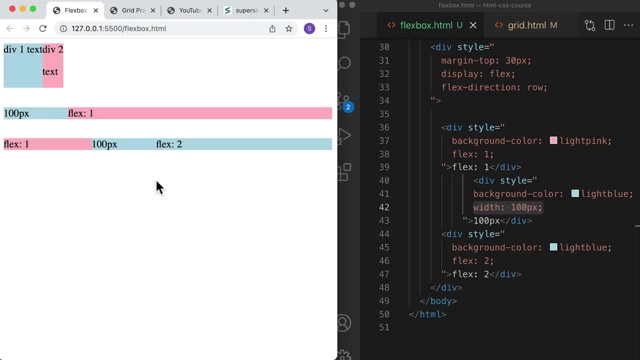 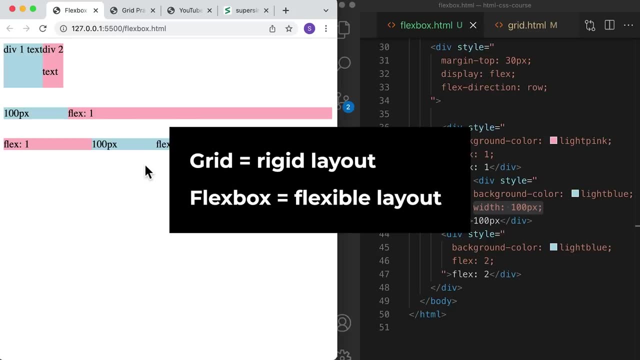 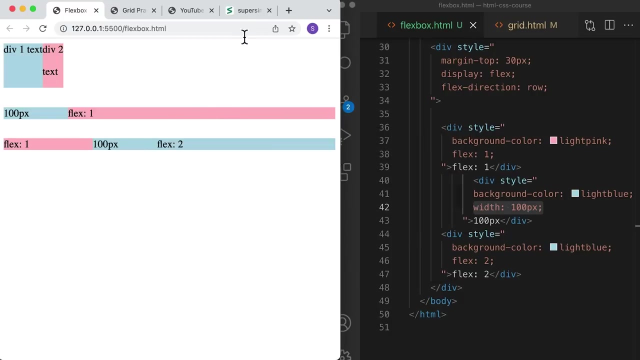 And that causes us to have flexible layouts, depending on how many elements we have and what order they're in. So that's the biggest difference between flexbox and grid. So what's the advantage of having a flexible layout like this? Let's go to our final project. 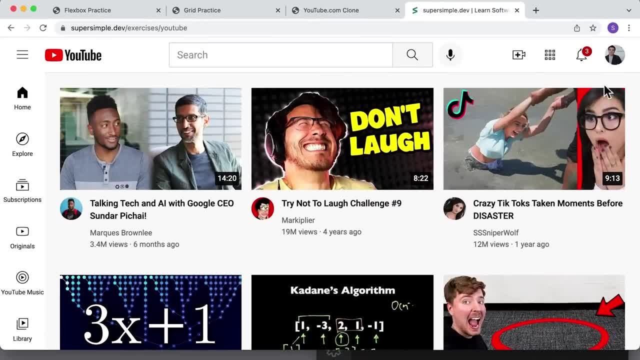 and we're going to resize the browser And you'll notice that in the header, in the right section, we have four icons or images. Now we could create this horizontal layout using a grid. However, when we're logged out of YouTube, you'll notice that we only 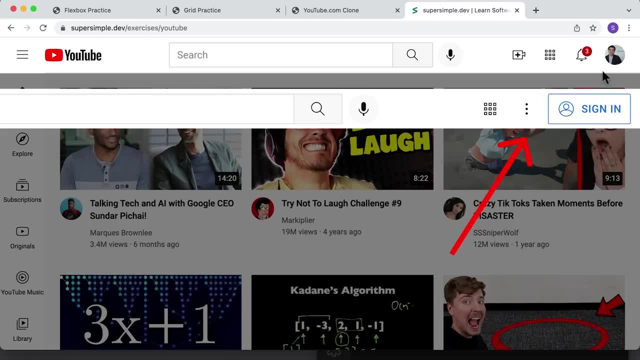 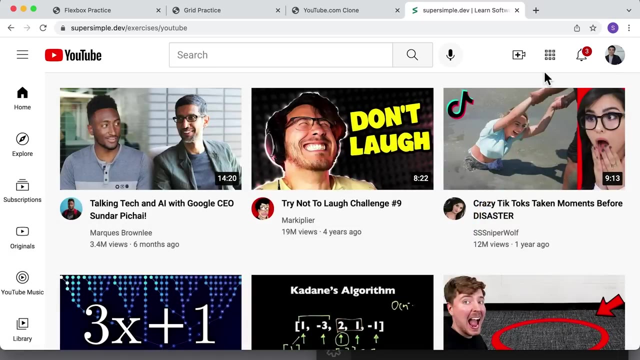 have three icons, So the layout actually changes because we only have three elements now. So this would be a great situation to use flexbox instead of grid when we want a flexible layout dependent on our content. So that's the basics of how flexbox works to create. 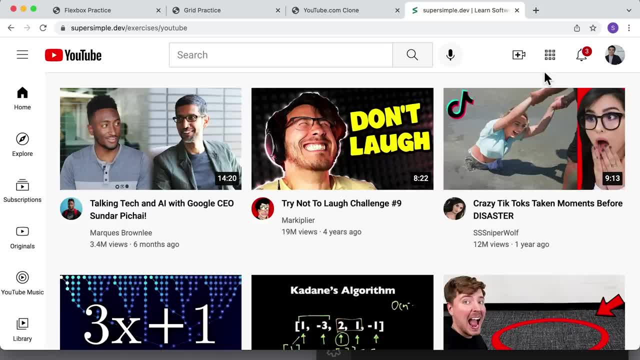 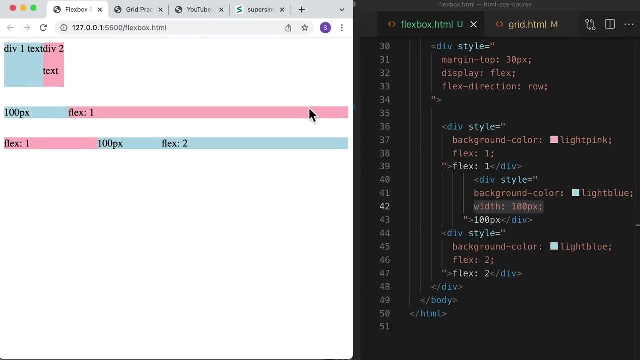 layouts and the main difference between flexbox and grid. We're going to go back to our practice file and we're going to go through some other examples of flexbox to help us build the header of our final project. So first let's actually 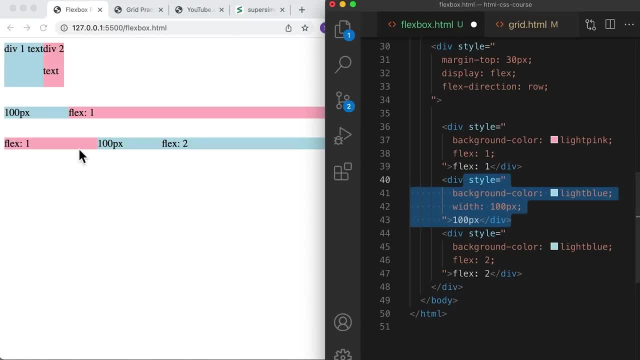 save this as it is so that we get a reminder that the layout is flexible. I'm going to change this to light blue and the other one to light pink, so that we have alternating colors and it's easier to see. Alright, let's go back into our grid code. 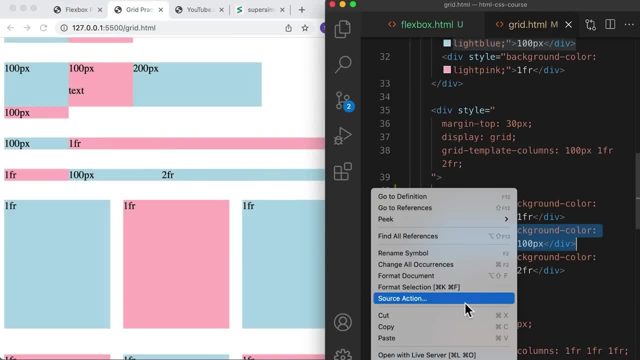 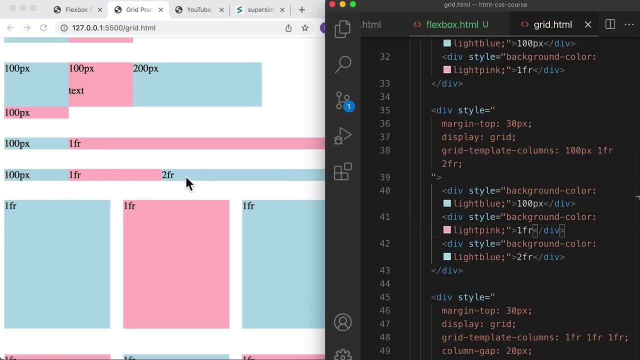 and we're also going to move this back into its original position. So just to remind us that for grid, the layout is more rigid, Save it, and now we're back. So we'll go back to our flexbox file and our flexbox HTML. 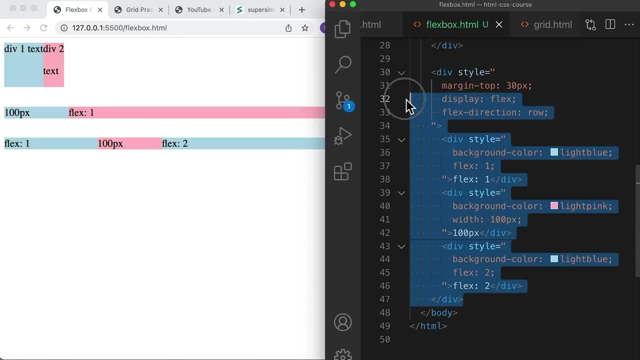 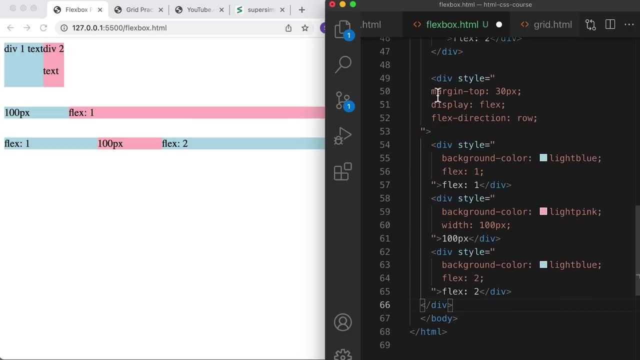 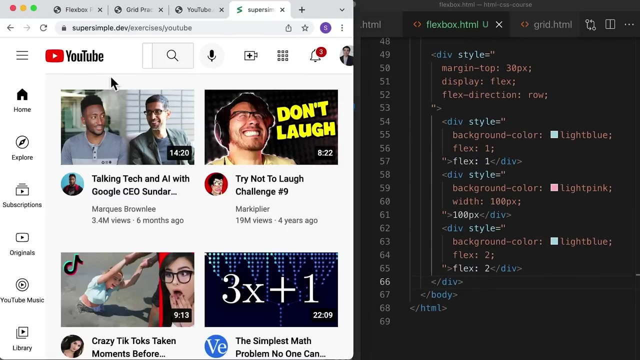 and we're going to do another example. So let's copy this and we're going to create another flexbox to practice with. Now for these next examples. we're going to use them to learn how to create the header up here. So first, let's create something that. 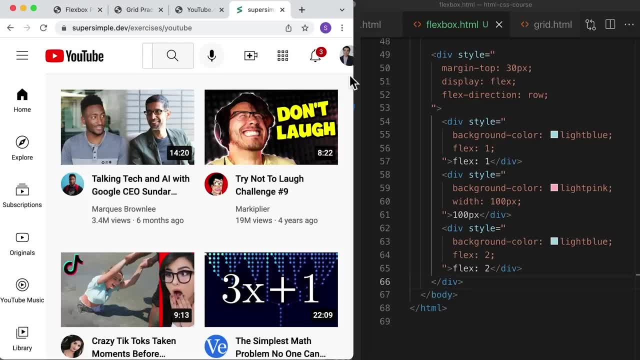 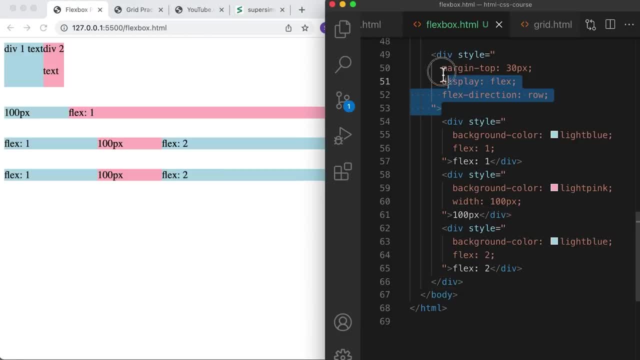 looks like the header. We're going to create a box that has roughly the same shape, So we'll go into our file here and we're going to make this flexbox have the same shape as a header. So let's set the height to 70 pixels. 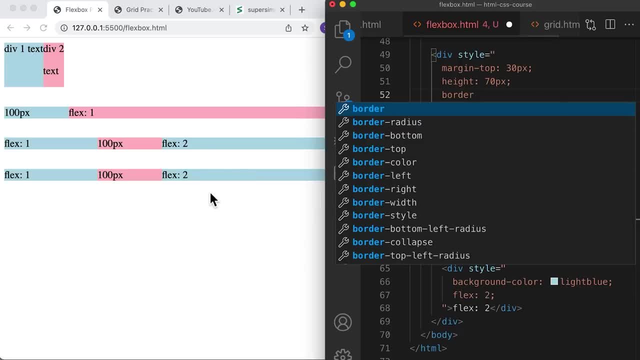 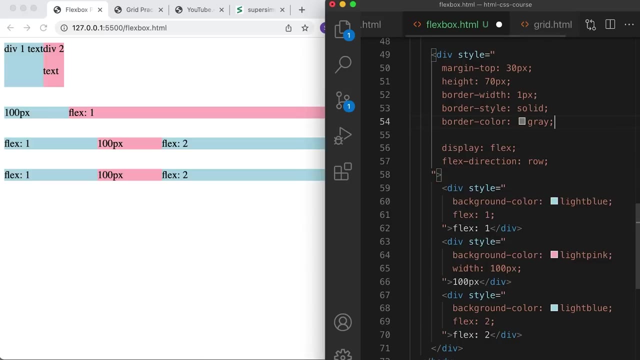 and let's set a border so that we can see the actual box. So we're going to set a border width of 1 pixel, a border style of a solid color and we'll set the border color to gray. And when we save it, 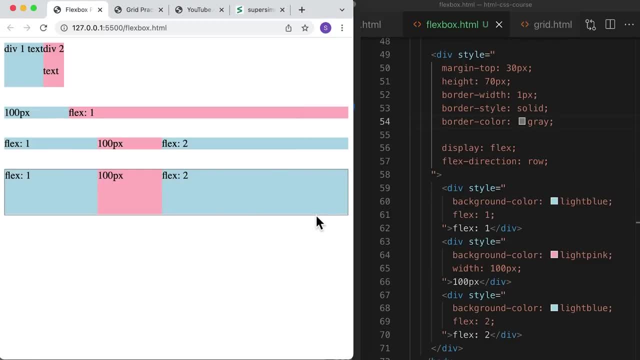 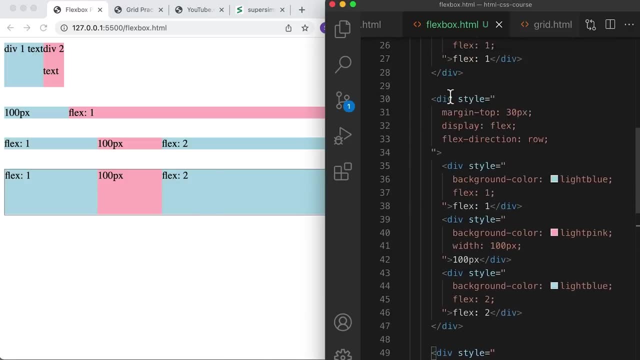 we can now see our flexbox using the border. I'm going to add a little bit of spacing to the bottom of the page here so that we can scroll this up. So remember to do that. we're going to scroll up and add some padding to the bottom. 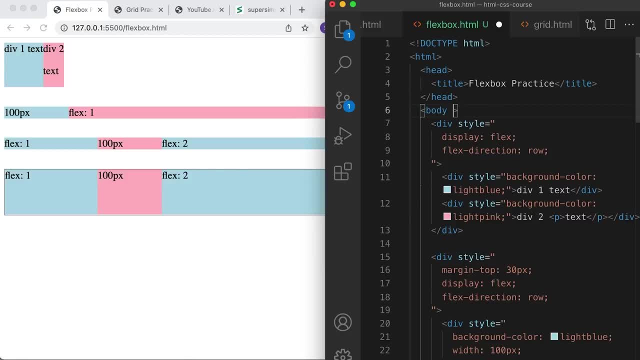 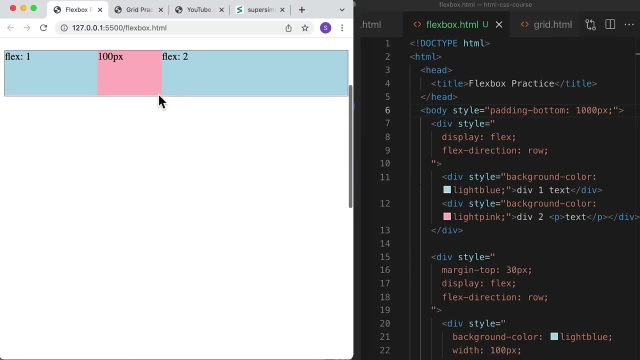 of the body. We're going to add a style to the body and we're going to add some space to the bottom. So padding bottom 1000 pixels. And now we can scroll this flexbox up to the top so that it's easier to work with. 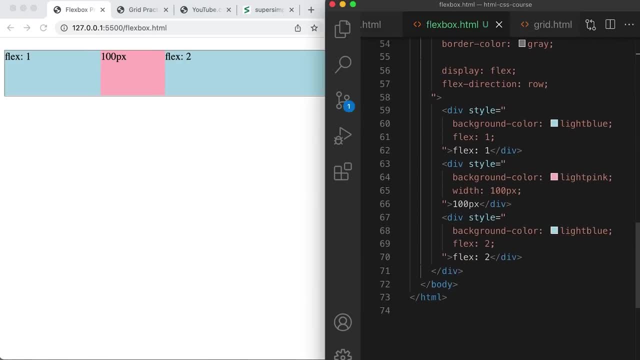 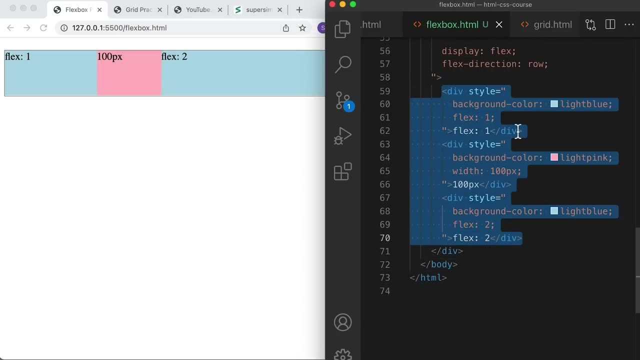 Now let's scroll back down to the example we were working with, which is right here. So, for each of these divs, let's change their width to 100 pixels. So I'll change this one to 100 pixels and let's also change the text. 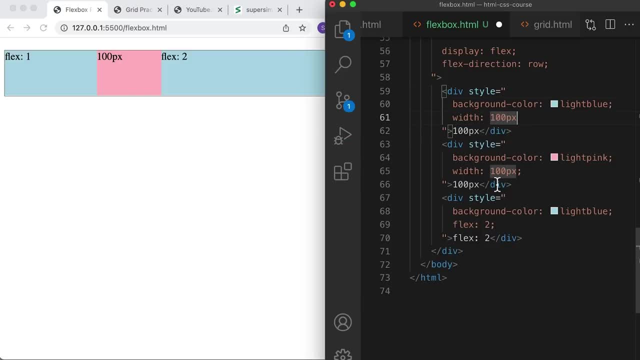 to 100 pixels, But this one's also 100 pixels and the third one to 100 pixels. Now let's save it and we have our three divs here, So notice that these three divs are aligned to the left side, So we can actually change how they are aligned. 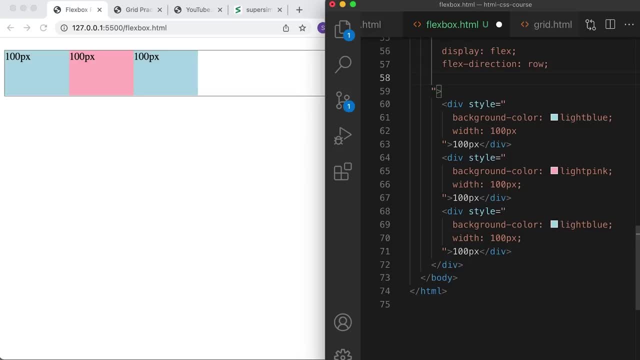 horizontally. To do that, we're going to use a flexbox property called justify-content, So this determines how these elements are laid out horizontally. For example, the default value is start. If we save it, they'll be aligned to the start or the left side. 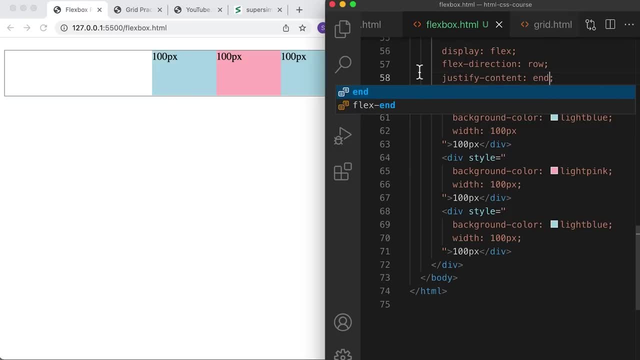 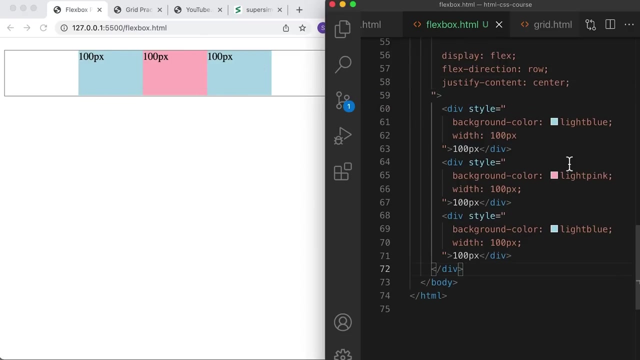 If we change this to end now, they will be aligned to the end or the right side. We can also change this to center to put all of our elements in the center. So that's how we control how these elements are positioned horizontally. We're going to go through. 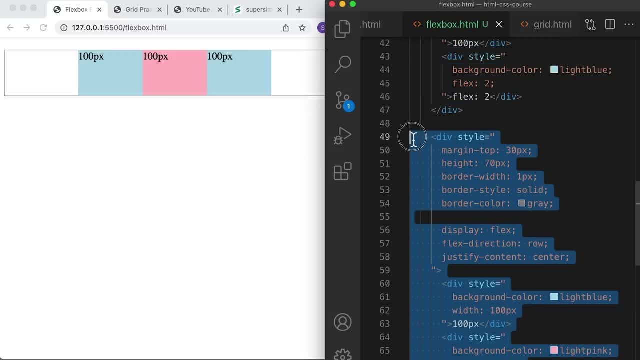 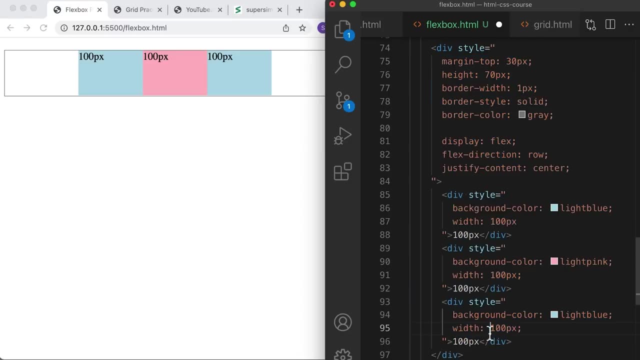 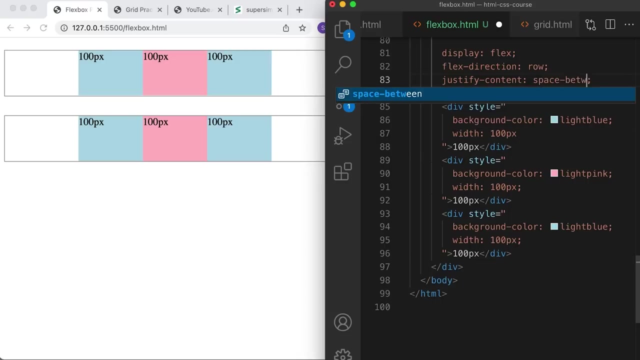 another example here: We're going to copy this whole flexbox and we're going to create another one below it. Let's copy it and paste it, And for this one we're going to set a special value of space dash between. So what space between does. 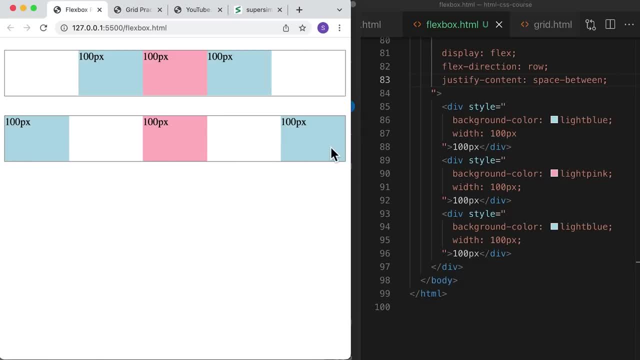 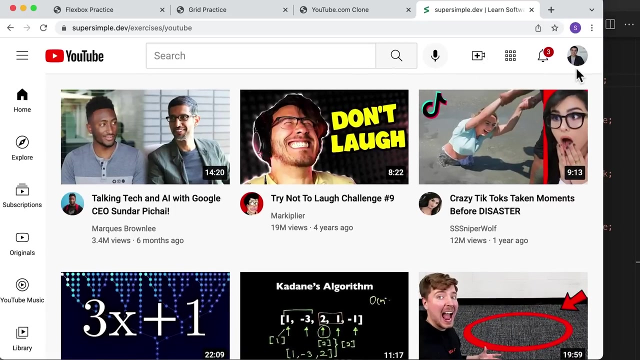 is that it spreads out our elements evenly across this horizontal space And it makes sure that there's equal amount of space between each element. So this is really useful if we go back to our header to spread out these four icons evenly. Now the last example we're going to go through. 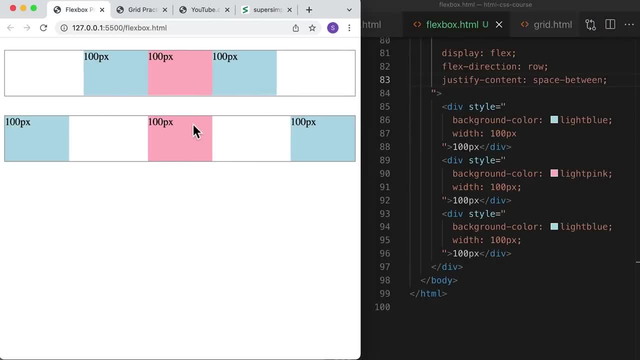 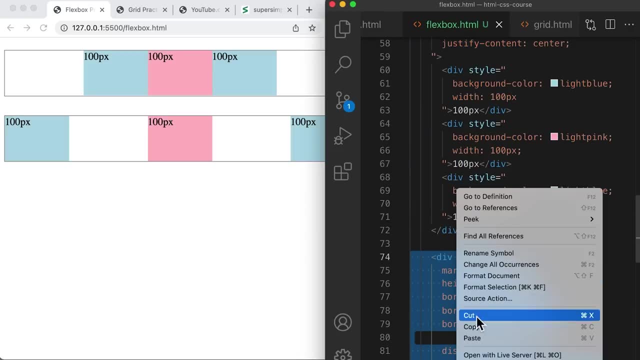 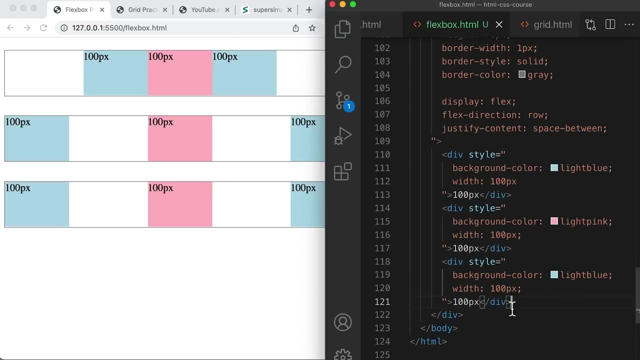 for flexbox is how to align elements vertically. So let's copy this again and create another flexbox. So let's copy this, paste it down here, And for this one we're going to set another flexbox property called align dash items. 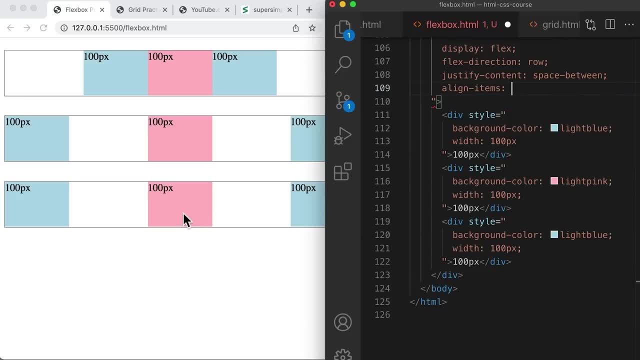 So this determines how these elements are aligned vertically. The default value is stretch, which you can see here. The elements are stretching to fill up the vertical space, But we also have some options. We can align them to the start, so they will no longer. 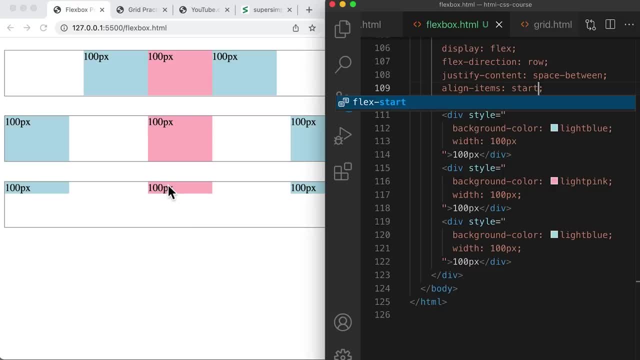 stretch to the vertical space. We can just take up as much vertical space as they need to, and they will be placed at the top, Or we can put them at the end, which will place them at the bottom of the container, And we can. 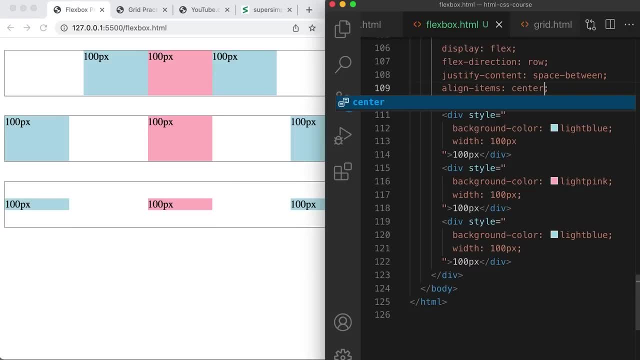 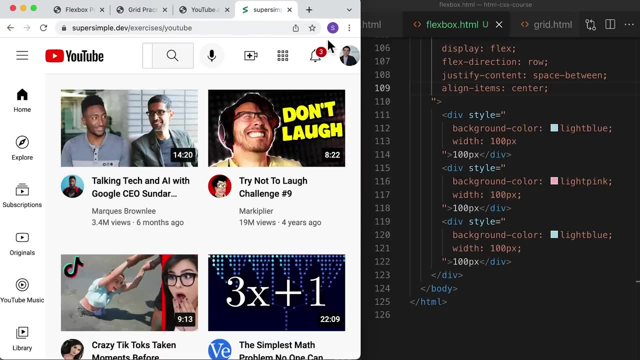 put them in the center, which will place them vertically centered. If we look at our final project again, you'll notice that all of these things in the header are vertically centered. So now we learned all these skills that we need and we're ready to. 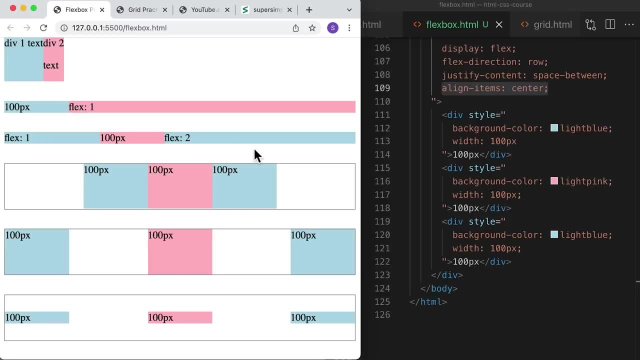 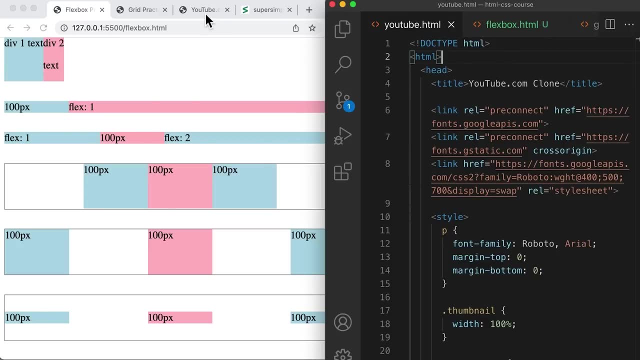 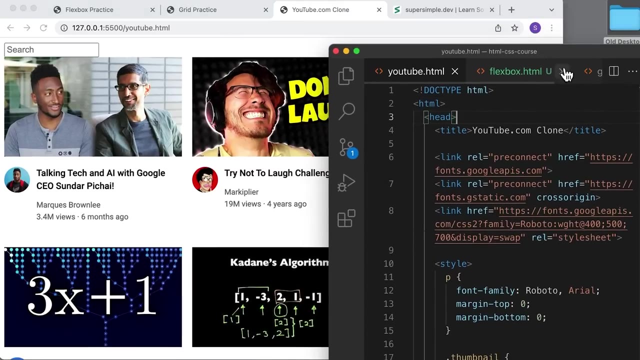 build the header for our project. Let's go to the code for our project we were working on, which was youtubehtml, and make sure you have this open in your browser. I'm going to resize the window here and also the code editor, so that. 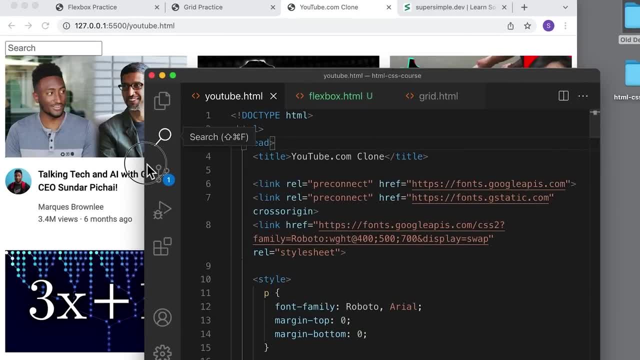 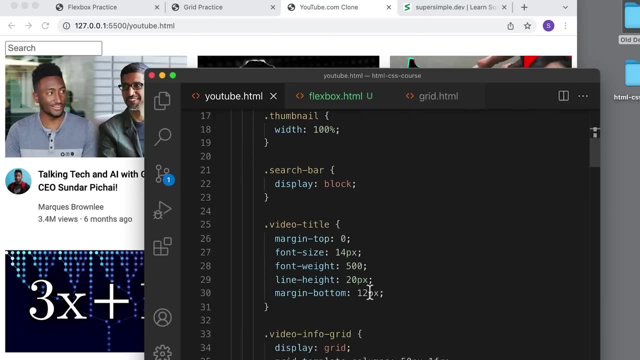 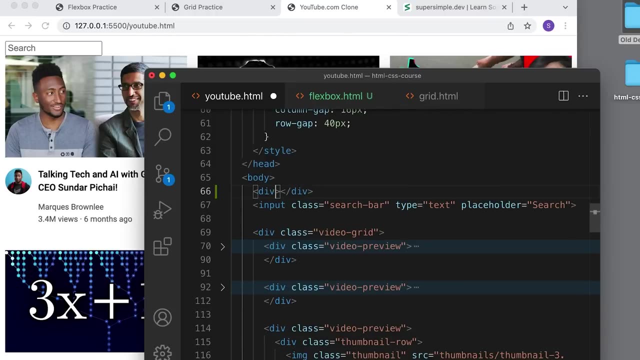 it's easier to see what's going on as we code. We're first going to create an element at the top to represent our header. So let's scroll down and currently all we have is this input. So we're going to create a new div. 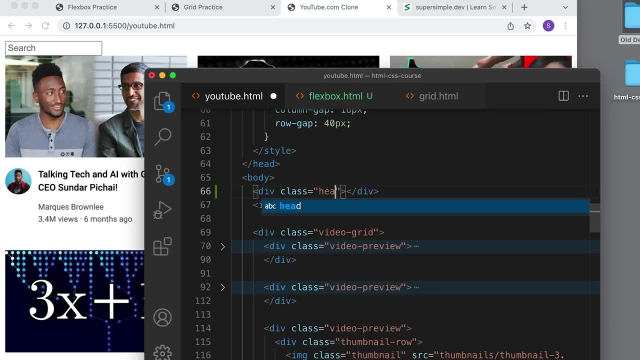 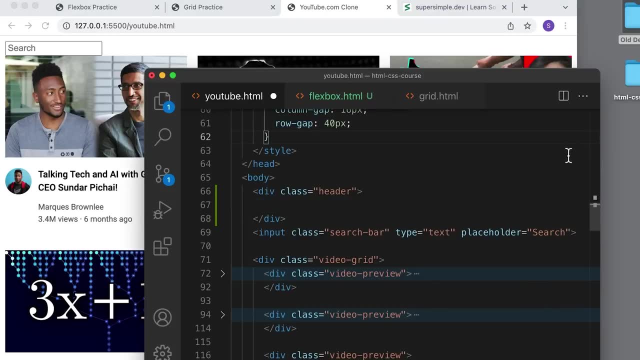 and we're going to give it a class of header. So this div is going to represent the header in the final project. And now let's put our search bar into our new header. So we'll cut this and paste it in here. 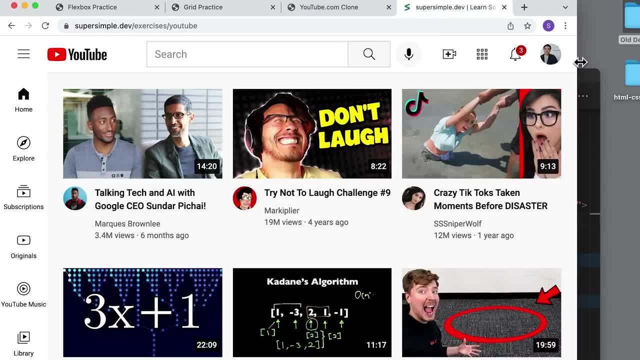 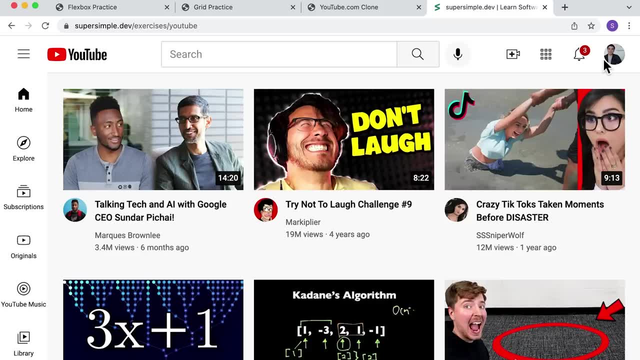 Next, if we look at our final project, the header has three sections. We have a section on the left, a middle section with the search bar and the right section here with some icons. So we're going to simplify this by first creating these three. 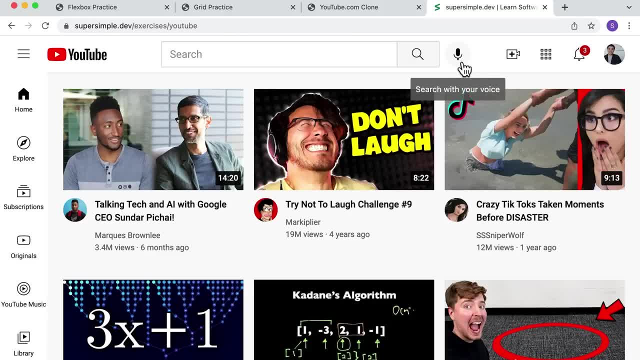 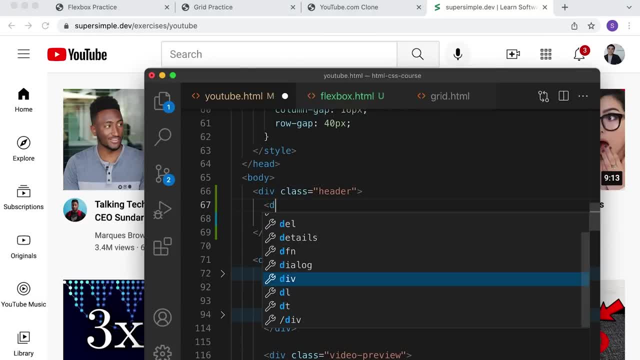 sections and then aligning them and then filling out these sections with the appropriate elements. So let's go back down here and we're going to create three sections, So we'll just use three divs here. So let's call this: 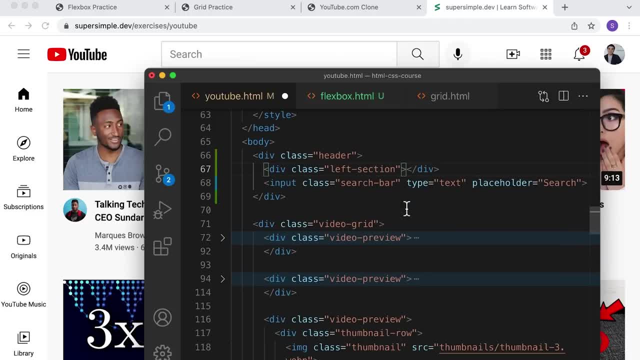 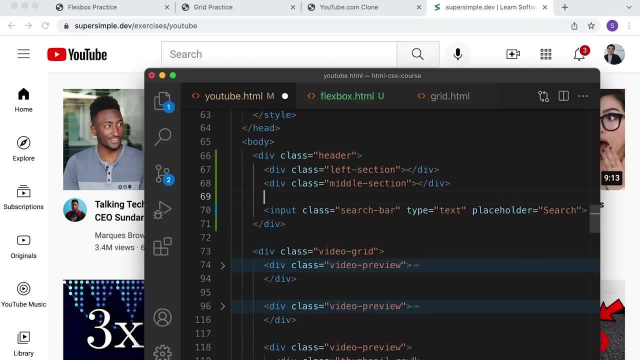 class equals left dash section. We'll create another div and call it: class equals middle dash section. We'll create another div and we'll give it a class of right dash section And we'll put the search bar into the middle section. 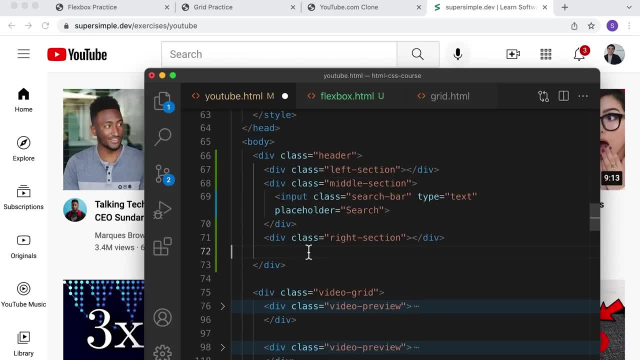 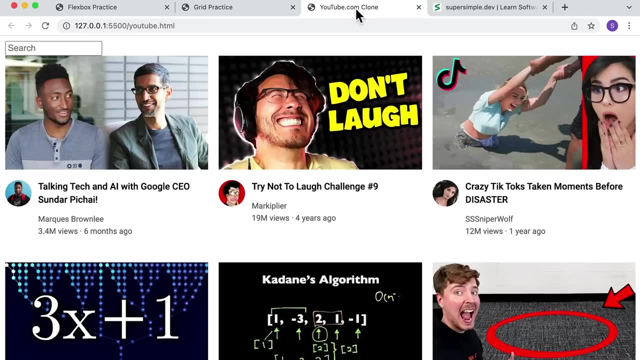 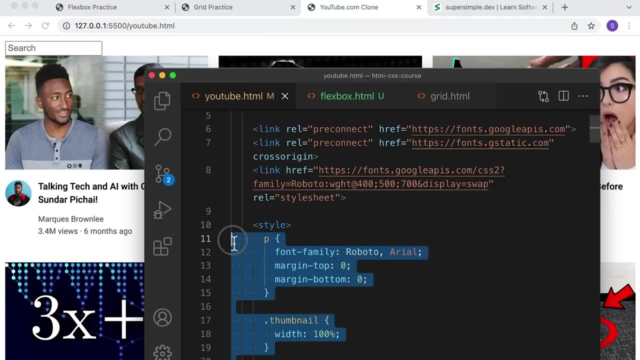 Right here And now. let's style this div so that we have roughly the same dimensions. So before we do that, you'll notice that we already have a lot of CSS code in this file And the best practice is actually to put the CSS. 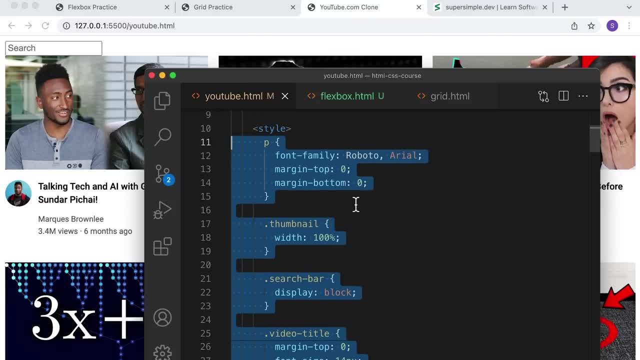 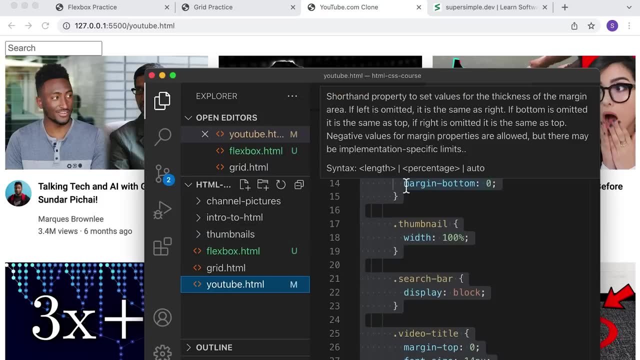 in a separate file. So before we write even more CSS, let's go ahead and put this into its own CSS file. So we're actually going to have multiple CSS files: One file for styles of the video preview and another for every style of. 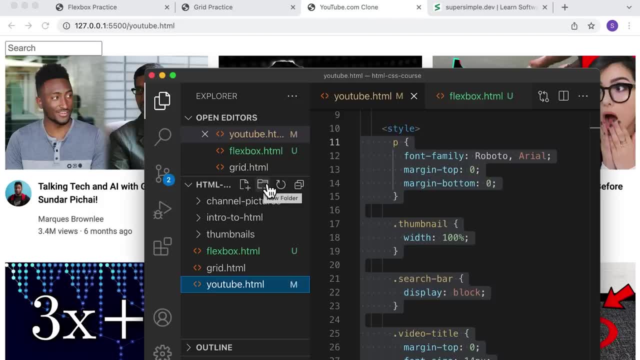 the header. So let's actually create a new folder first to organize all of our different files of CSS. So we'll create a new folder and let's just call this styles. Inside we're going to create two CSS files. The first one is going to be called: 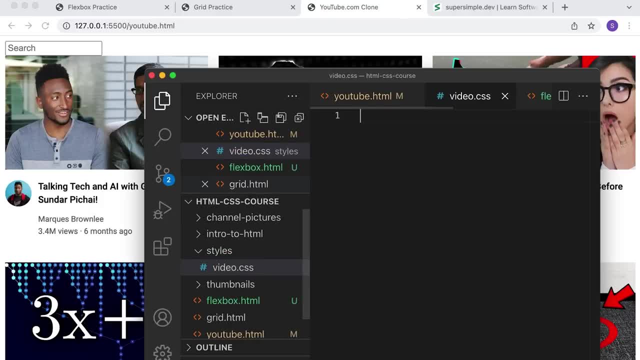 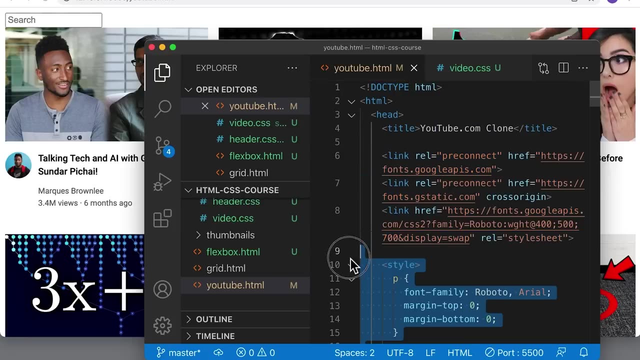 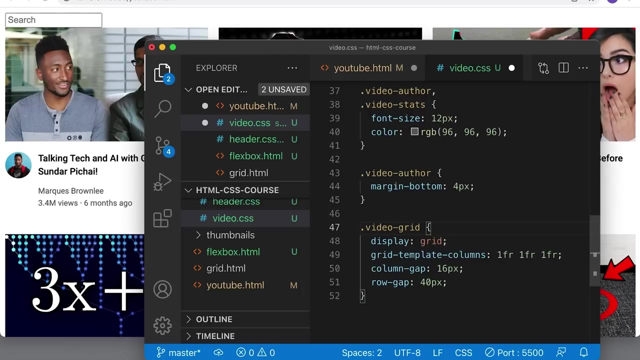 videocss And the second is going to be headercss. So first we're going to go into our youtubehtml, We're going to move all of this into the videocss file, So let's move this into here. Now, all these styles for these videos are separated. 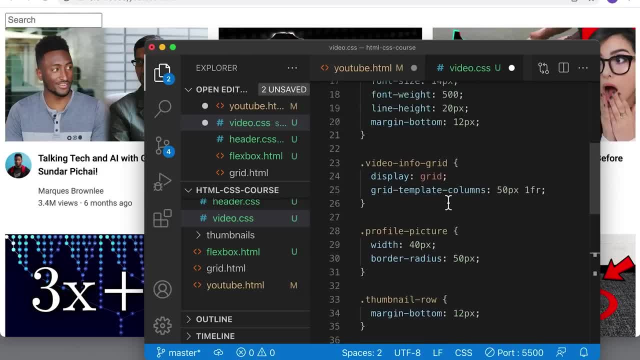 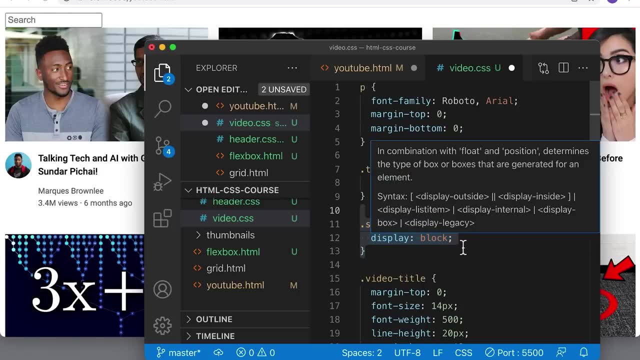 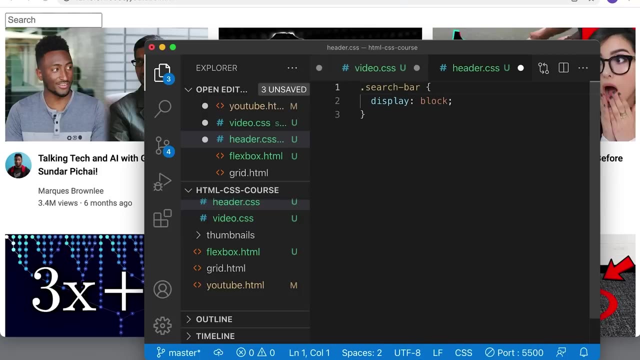 into their own file. Now, if I scroll up to the top here, you'll notice we also have some styles for the header. So this actually belongs in the header And we're going to move this into our headercss file. So we're grouping related styles together. 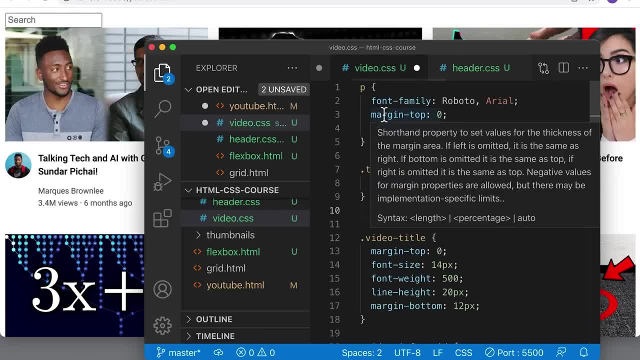 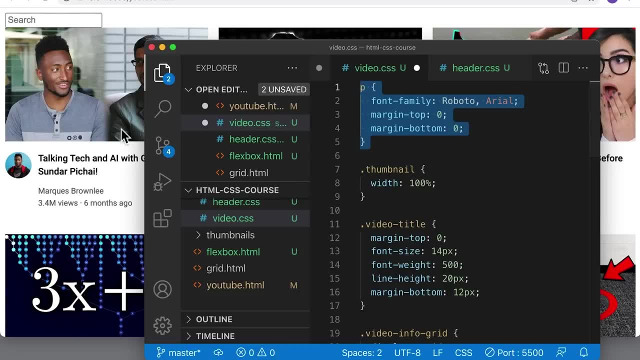 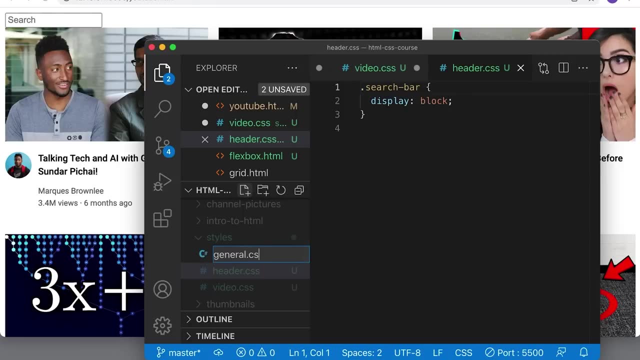 to make it easier to read. Now for the top of this file. again we have this code that targets all paragraph on the page. So this is not actually specific to our videos. So I'm actually going to create another file called generalcss And that's going to. 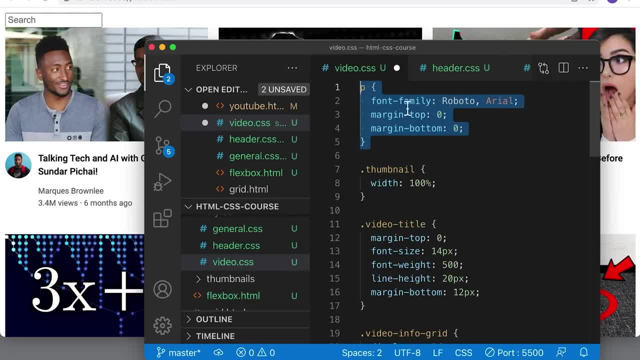 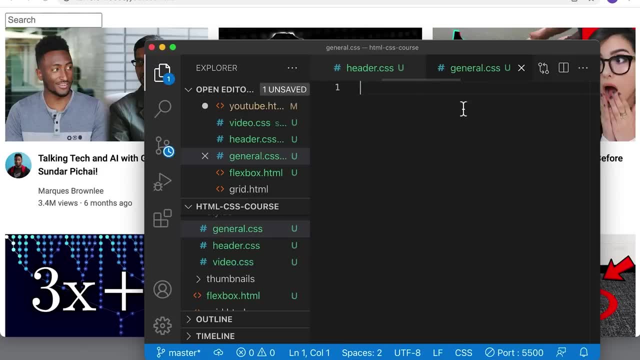 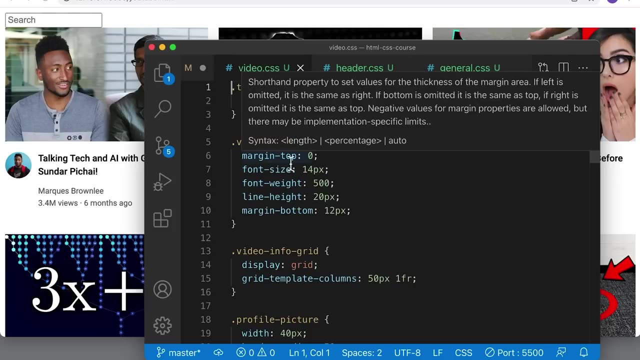 contain all the general CSS code, like this, Where we target all paragraph elements on the page, So move this piece of code into general. So just like that. we have three CSS files and they're all very focused on one part of our web page. 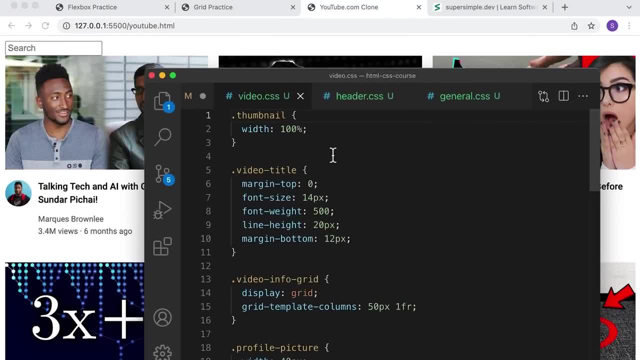 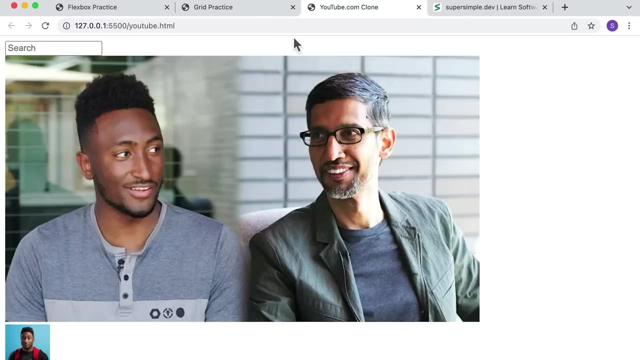 So this is generally what we want to do. We want to organize our code and separate them into different files, depending on what the code does. Next we're going to go into our HTML file and we can remove this and let's save it. But now you can see that all of these styles that we 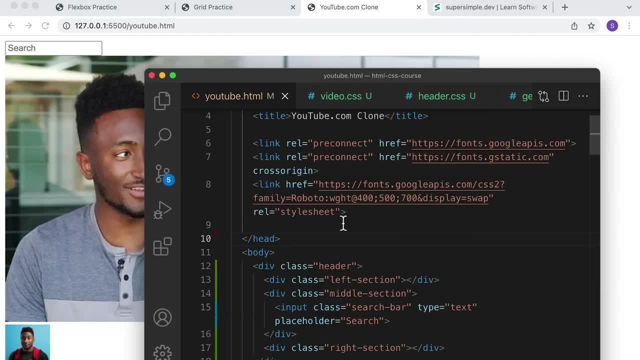 had are gone, So we need to link them back into our HTML. To do that, we're going to create a link element. We'll have an attribute of rel which tells it what we're linking. So we're linking a stylesheet and we also tell it. 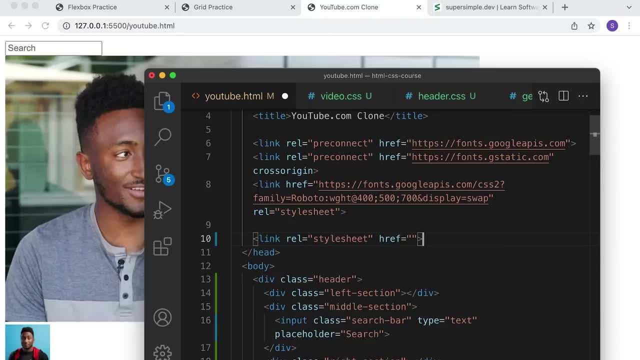 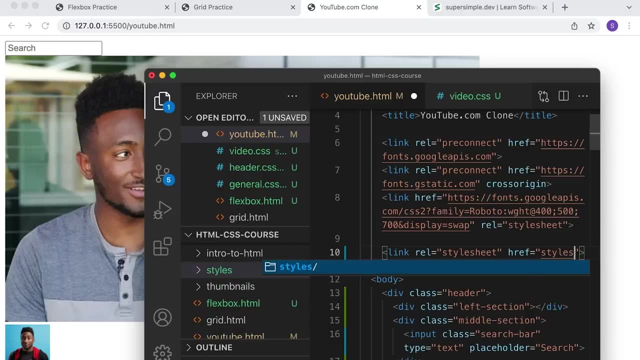 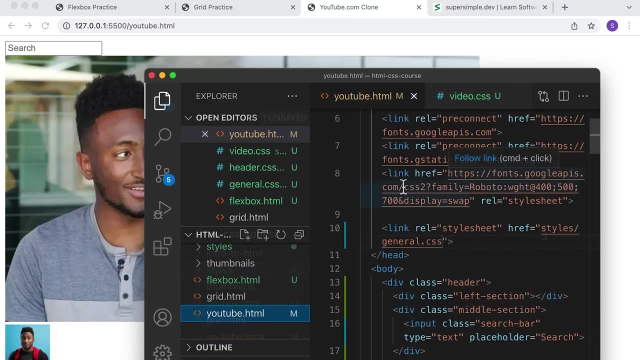 what file we're linking with href. So here beside our HTML file, we have a styles folder. So we're going to first link the styles folder and then we're going to type a slash to go into it and link generalcss, And now we're going to link our other two. 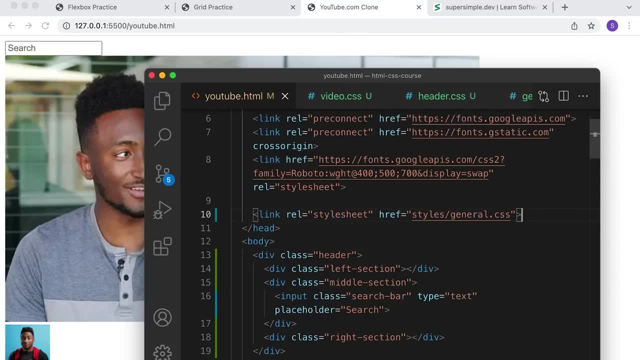 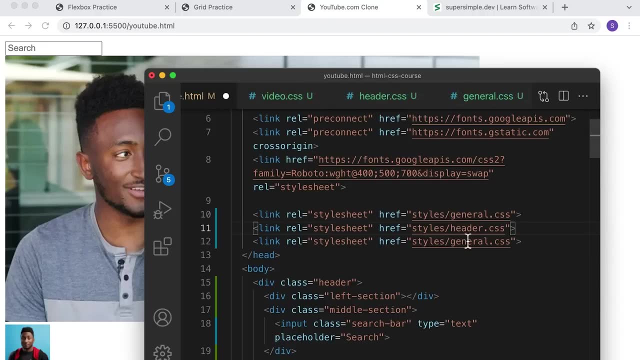 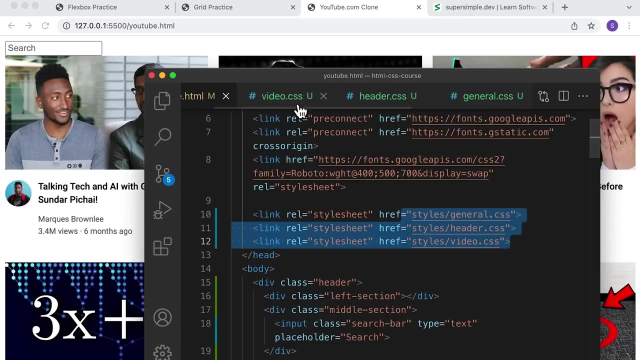 CSS files. So to do that, we just need to copy and paste this, And then we're going to link headercss. And for the third one we're going to link videocss. And if we save it, we linked all of our code in three separate. 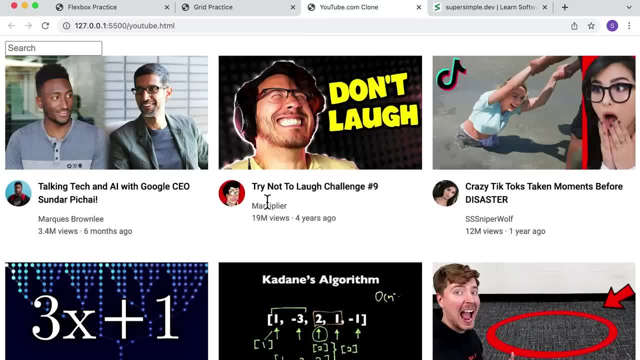 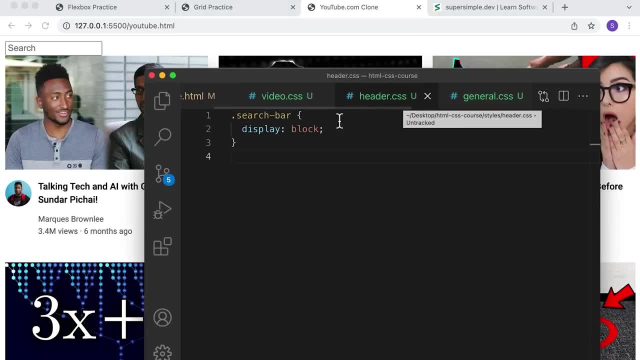 files and we're back to where we were. Next, let's focus on our header styles and create our header. We're going to go into this file and we actually don't need this display block anymore, So we use this to put the search bar on a separate. 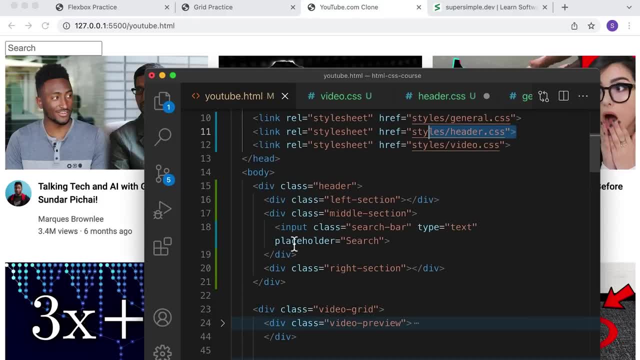 line, but now the search bar is inside a bunch of divs, So the divs will create that separate line for us. Now the one other thing that we had to do is that notice that there is some spacing on the left side, on the right. 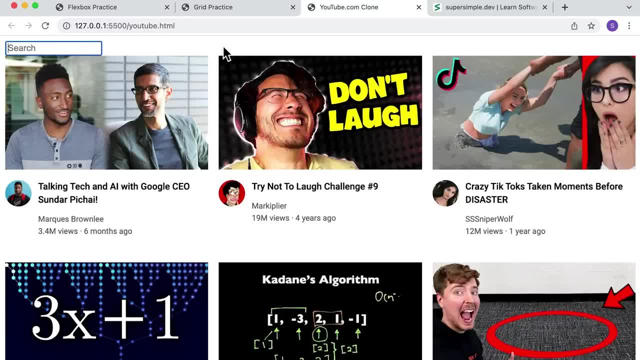 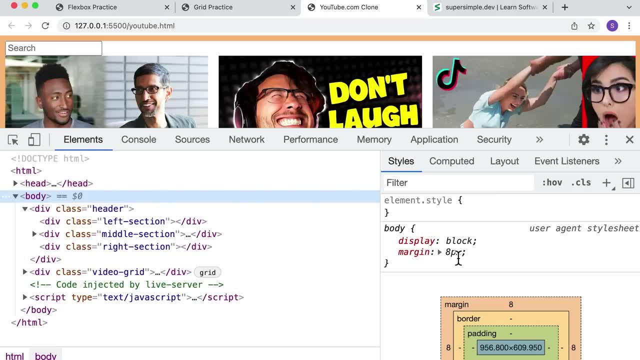 side and at the top, So by default, if we right click and inspect and we look at the body, so the body element has eight pixels of margin on every side, by default. Now, to get a more precise design, we actually want to set this to zero, So we're going. 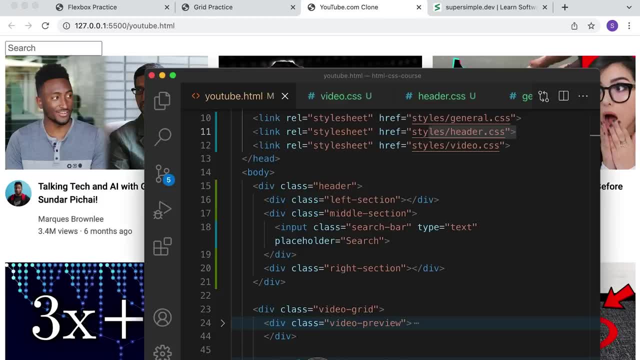 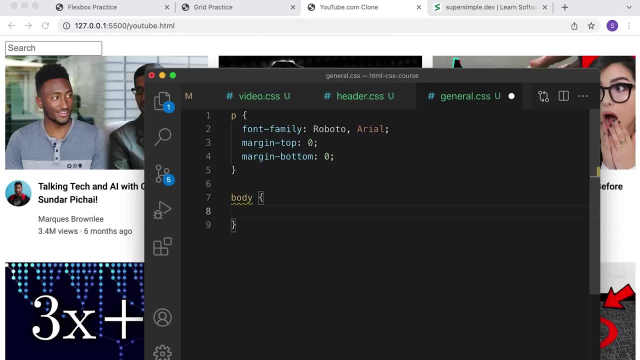 to reset these default styles. So we'll go into our CSS code and we're going to go into the general file And we're going to target the body and we're going to get rid of all margins. An easier way to do this is to: 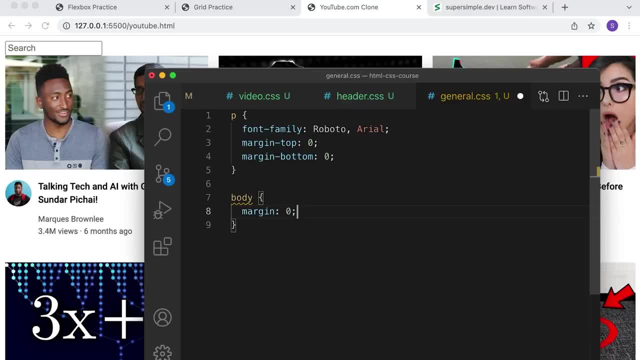 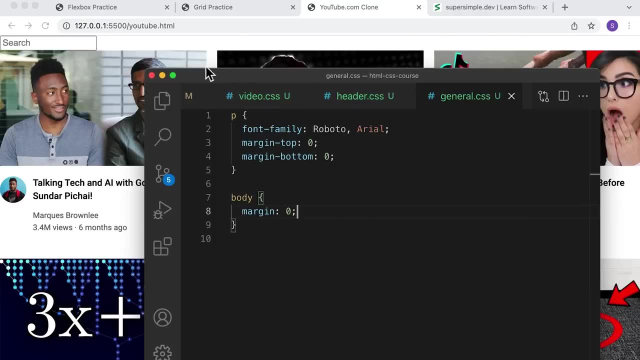 set the margin property and set it to zero. So this will set all margins in all directions to zero. Let's save it. and now our elements are right up to the edge of the page. Next, we're going to work on our header. So I'm actually. 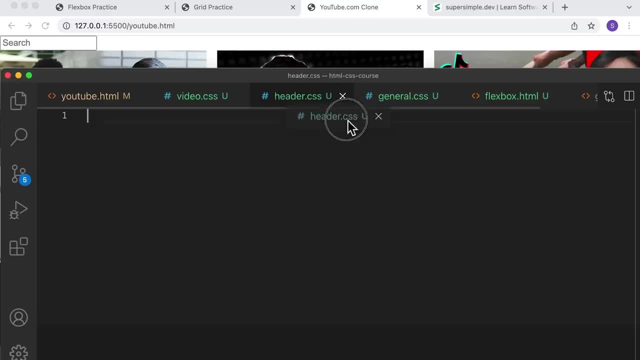 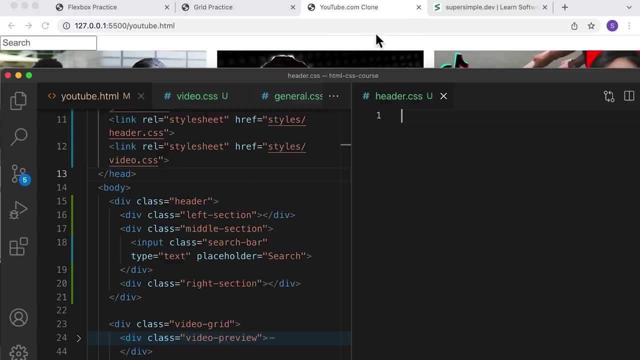 going to make this wider so that we can have both of these files on each side. We're going to have the HTML on the left and the CSS on the right. So the first thing we'll do is we're going to add a height to this header so that it looks: 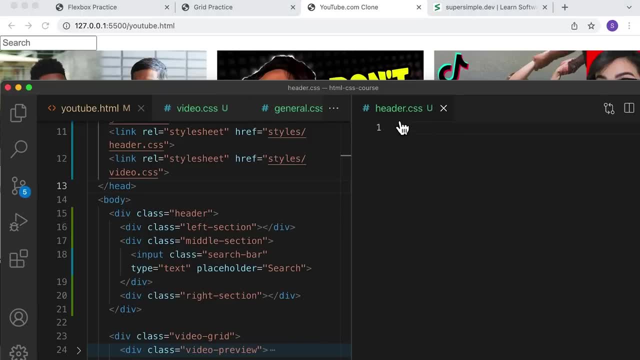 like our design here. So let's go into our header CSS file and remember, we set a class of header, So we'll target that using dot header and we'll set a height of maybe 40 pixels. Okay, so let's compare that to our design. 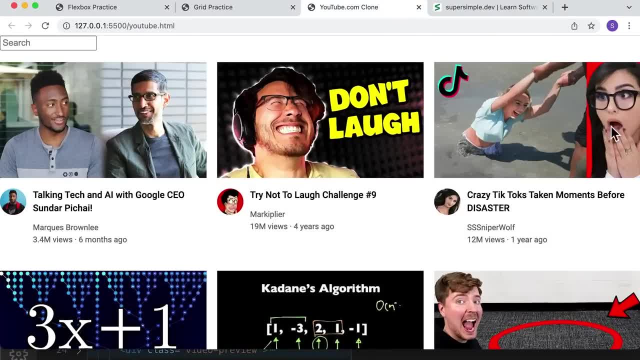 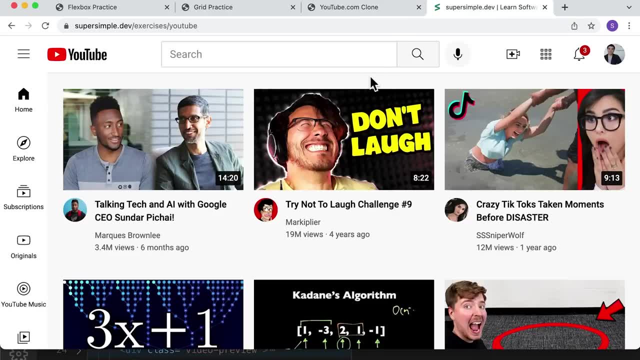 Looks like our design is a lot taller. Let's change it to maybe 55 pixels. Let's compare that. So I'm just comparing this to the bottom edge of here and that looks pretty good. So next we're going to position these three sections. 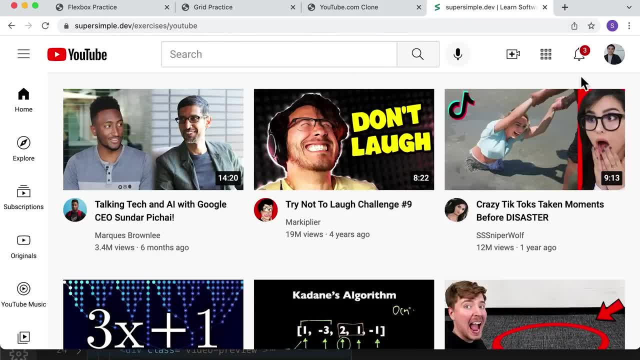 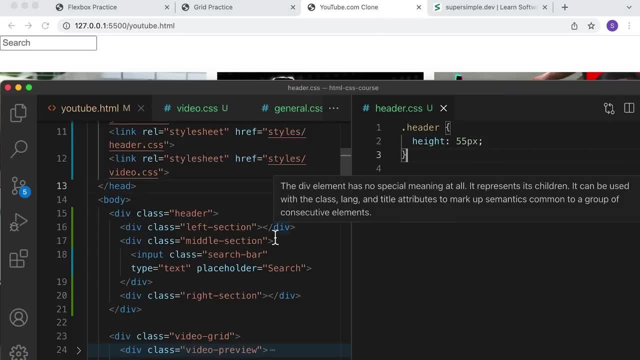 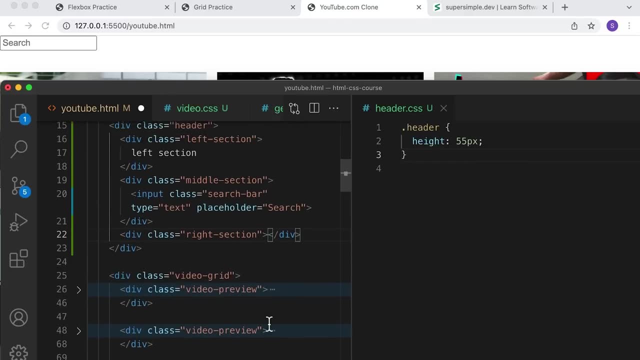 The left section, the middle section and the right section. So in our code we can't actually see the sections right now because they don't have any content in them. Let's just call this the left section and then add the text here as well. 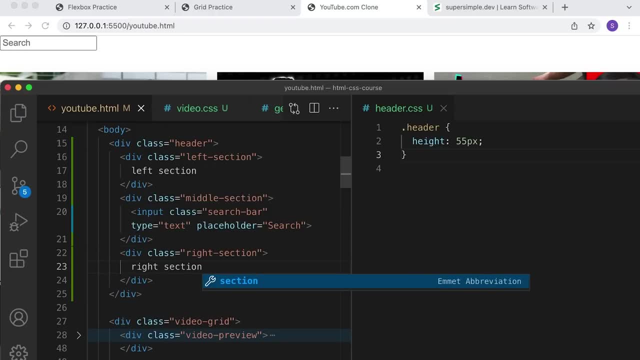 The right section, Save it. and now we have these three. However, you'll notice that they're being aligned vertically and that's because divs, by default, are display block and we haven't made this into a flexbox yet, So to create a horizontal layout. 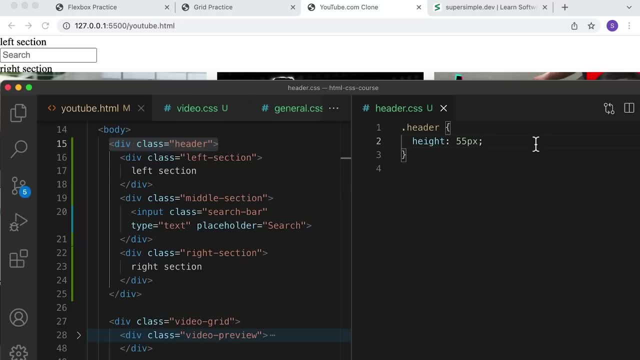 we're going to turn our header container here into a flexbox. We're going to set the display to flex and we're also going to set the flex-direction to row to lay them out horizontally. So let's save. and now our sections only take up as much. 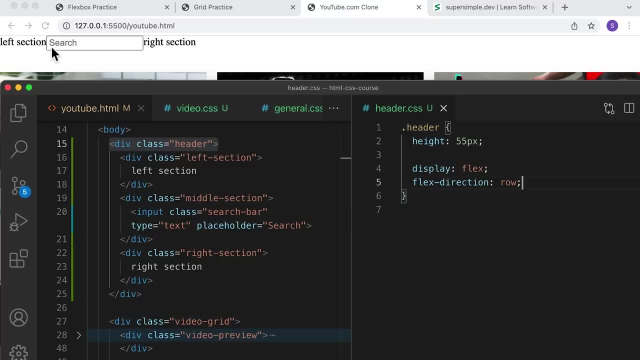 space, as we need to, as we saw in our examples. Next, let's give these a background color so it's easier to see them. So, for the left section, we're going to target it and we'll set a background dash color of light blue. 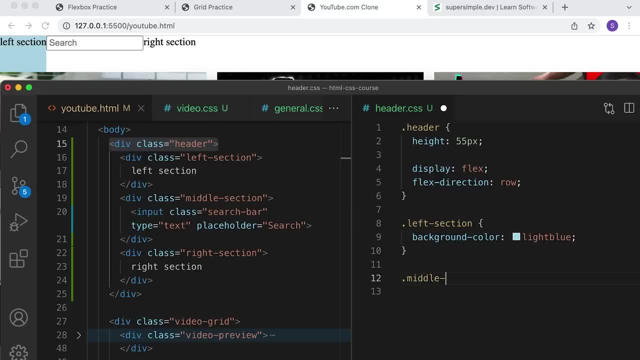 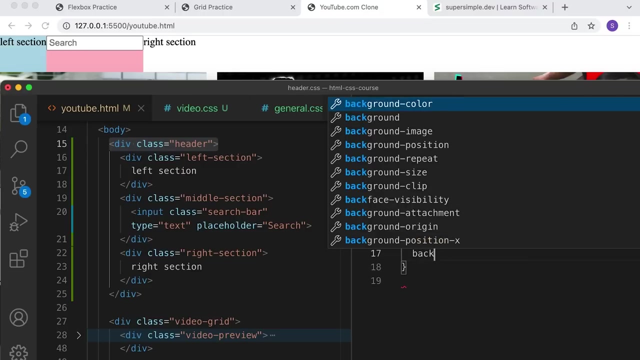 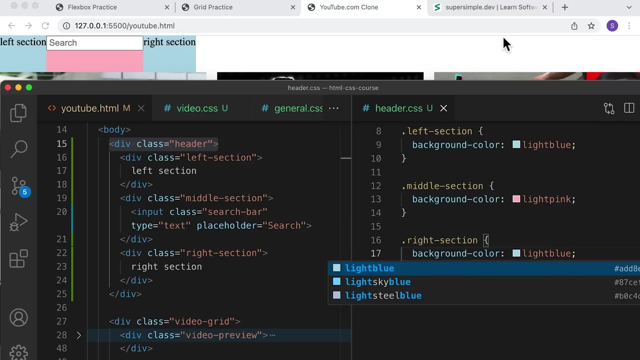 and for the middle section, we'll set a background color of light pink, and for the right section, we're going to set a background color of light blue. Right section: background color of light blue. So now, how do we create this layout? So let's. 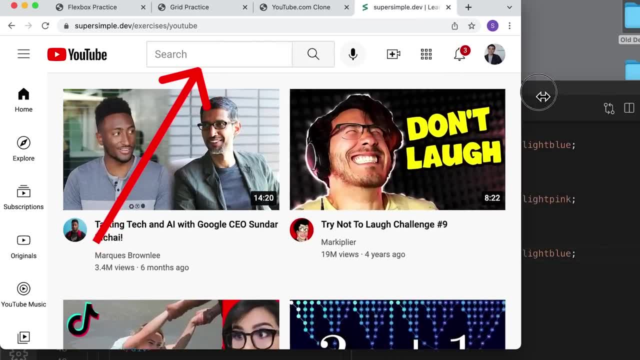 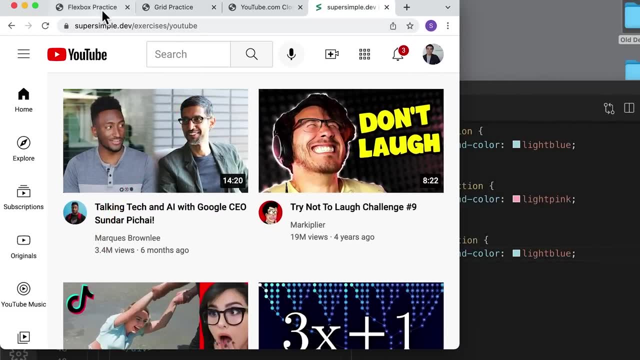 analyze it a little bit. If we resize the page, notice that this middle section is also resizing. So to achieve this, we're going to use a property called flex. So, if you recall, in our examples flex takes up the remaining amount of space. 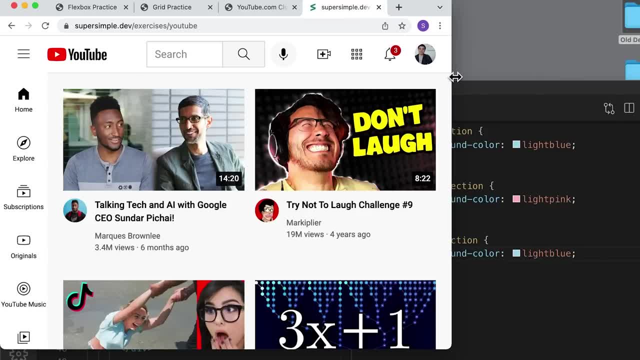 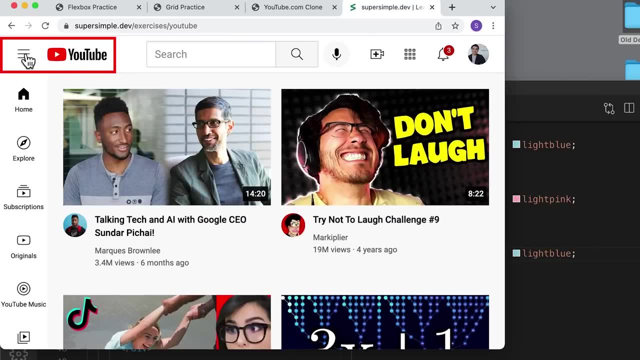 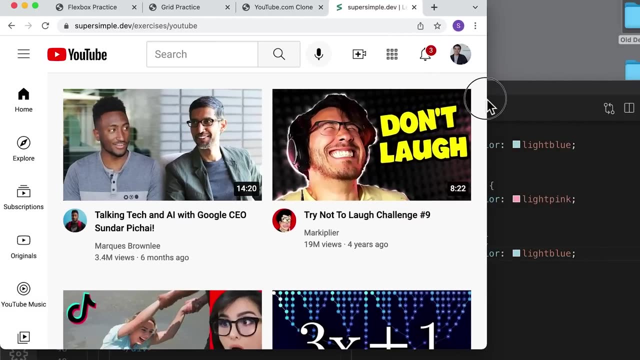 So if I look at the header in our final project, when I resize, this right section is not changing its width and neither is the left section. So these will have a predefined width and then this will be flex Because, as you can see, it's growing as the page is being 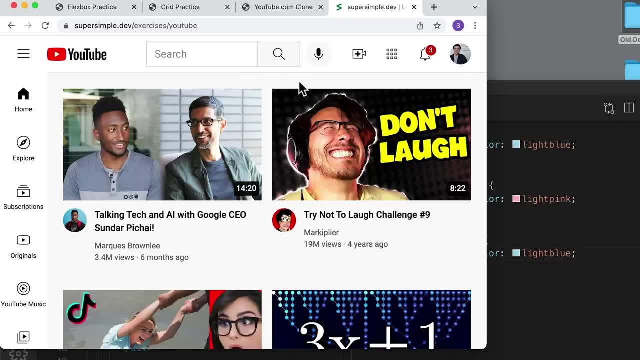 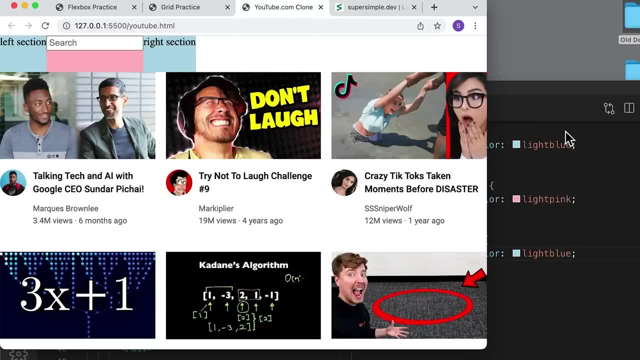 resized. So that's an example of how to analyze these layouts. Don't worry, you'll get better with more practice. For now, we're going to do this example together. On the left section, we're going to set a fixed width. Let's set this to, maybe. 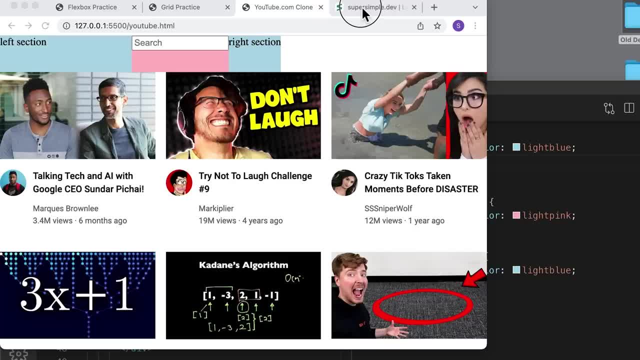 200 pixels. See how that looks. Compare it to our design. So it's actually a little too much. I want it to end right here after the YouTube logo. So we're going to go back and let's change this to 150 pixels. 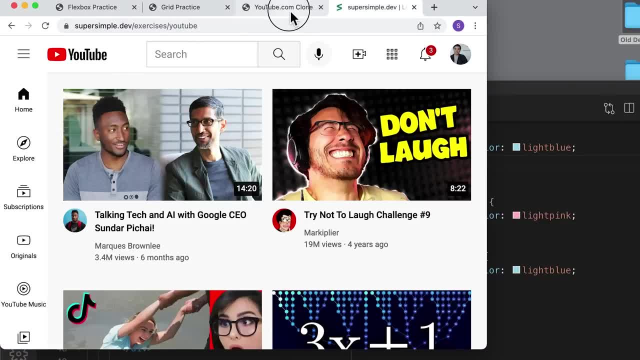 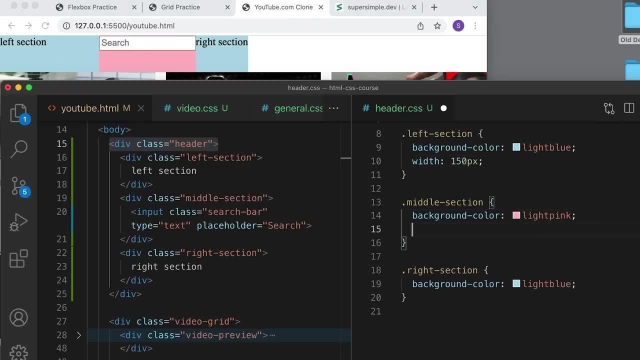 And let's compare it So that looks pretty close. For this middle section, we want it to stretch, So remember the property to do that is called flex1.. So now the middle section is stretching, and for the right section we also want a fixed width. So let's 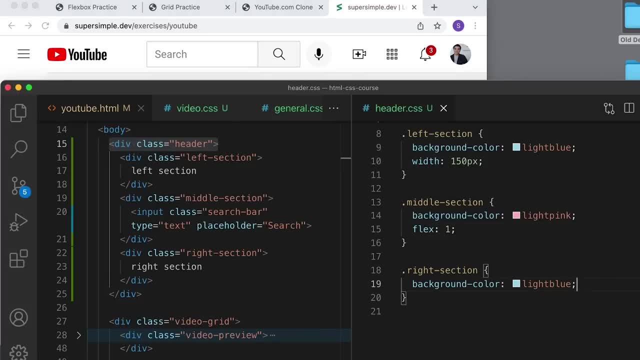 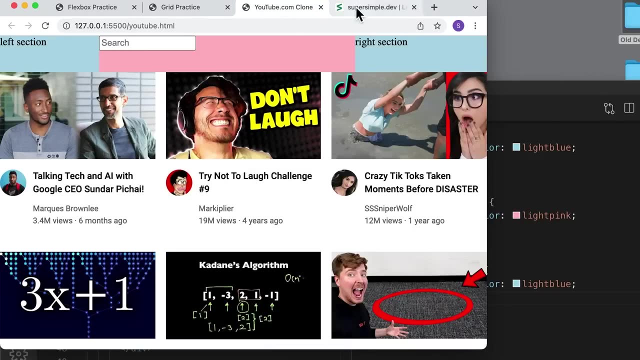 compare it. We want it to be somewhere here. Let's try setting a width of 200 pixels, And then let's compare these two. Okay, so I think this is pretty close to the structure that we have here. So what we're doing is we're just simplifying. 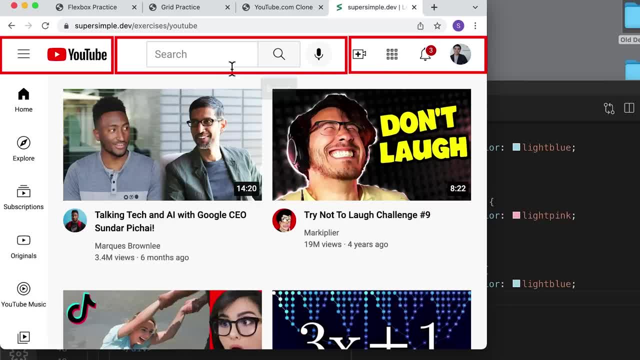 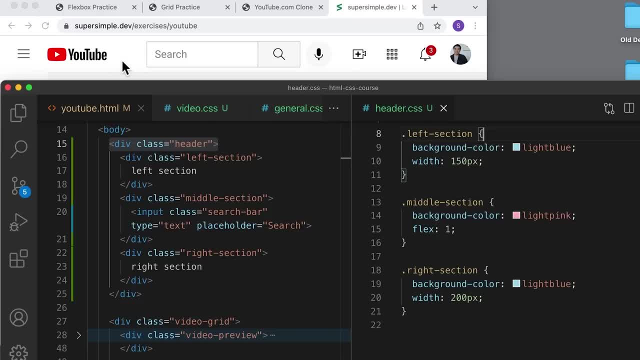 the structure into the bigger picture, and then we'll go in and add these smaller details. Now we're going to set some spacing on the left and the right side of this middle section, So remember to do that. we're going to set our margins. 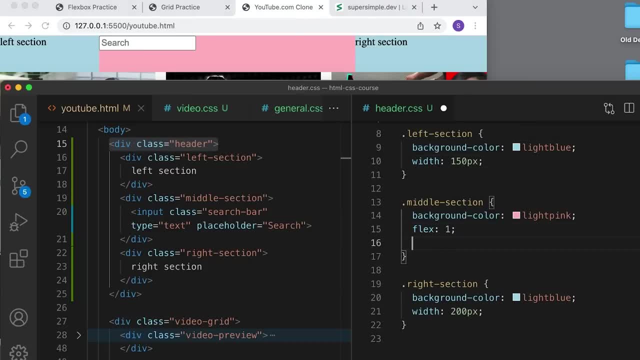 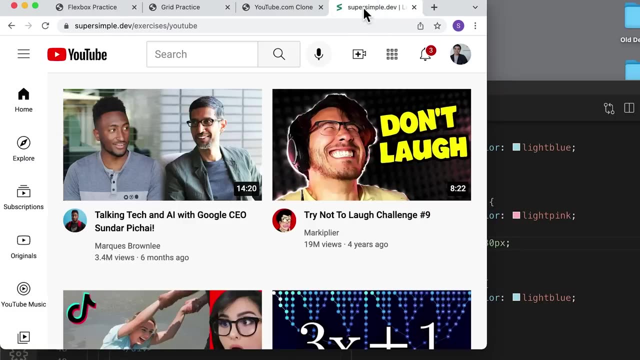 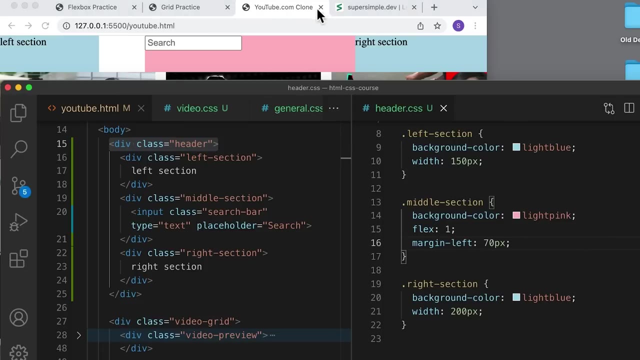 So on the left side, let's set a margin-left of maybe 30 pixels, Save it And let's compare. It's definitely more than 30 pixels. Let's change it to maybe 70 pixels, Save it and compare. So this compared to. 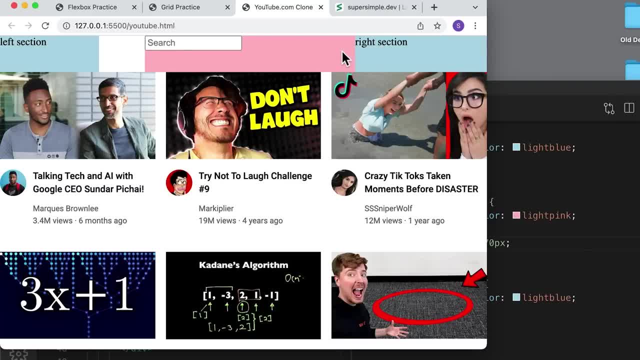 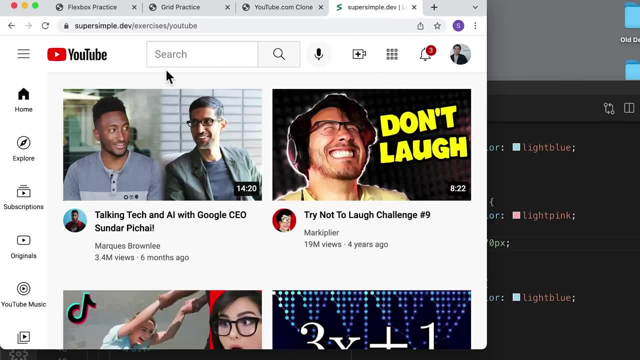 this. I think that's close enough. So now for the right section. we're also going to add a little bit of space. So if we look at our design, So it's less space than we have here, So we're going to add a margin. 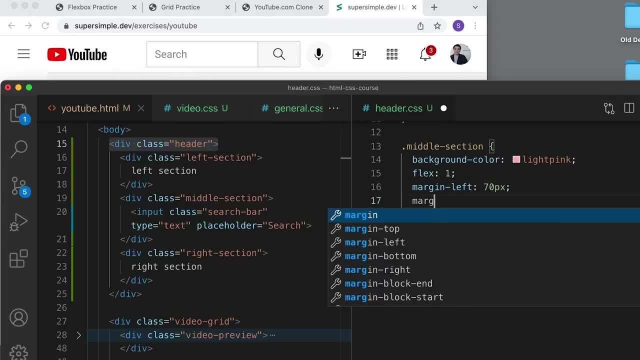 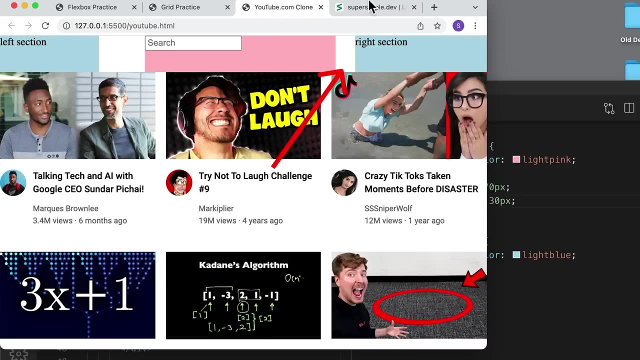 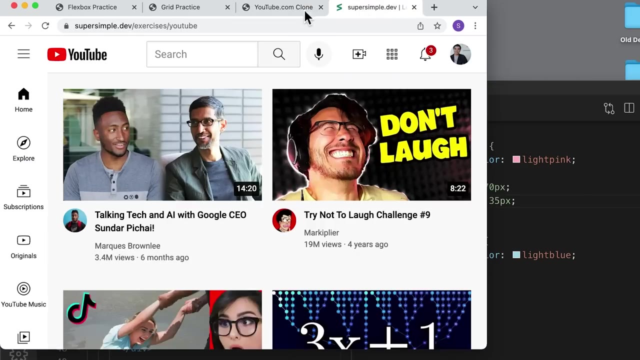 to the right of the middle section And we'll set it to maybe 30 pixels. Save it And that looks pretty close to what we have here, Maybe 35 pixels, Okay. So now, if we resize our page, You'll notice that the 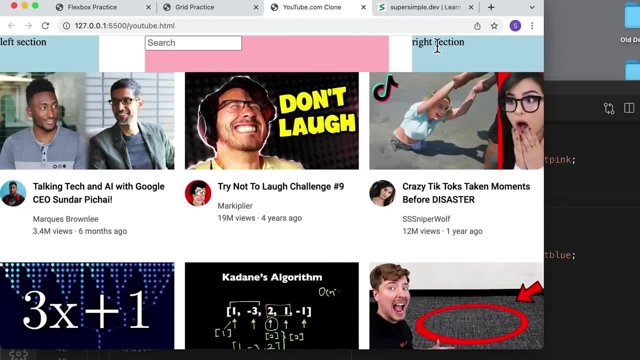 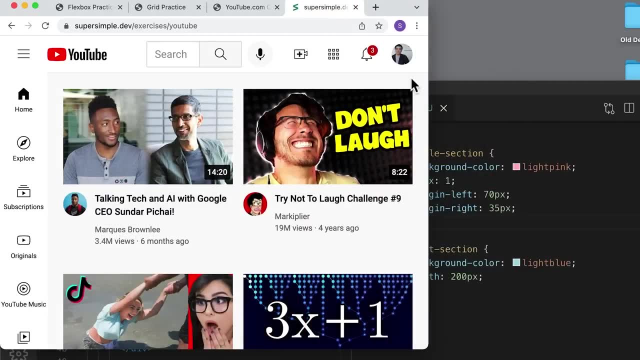 middle section is growing and shrinking with the page, And the right and left are staying the same width, Which is exactly what we have here. So there's one other detail we're going to copy for this middle section. Notice that if I resize the browser and make it wider, 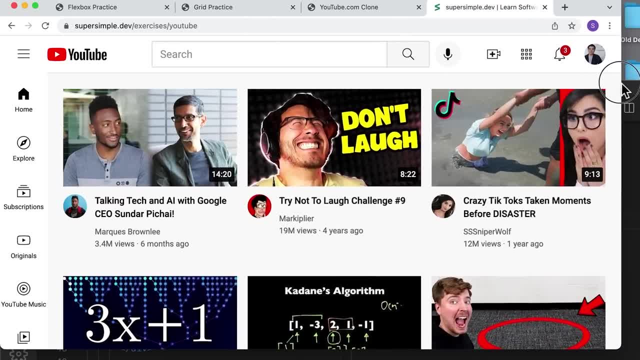 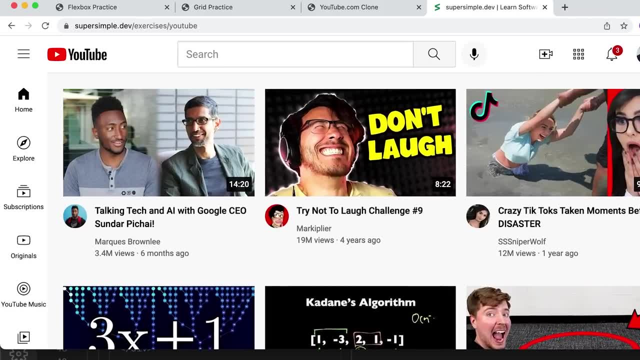 at some point the middle section stops growing. So at roughly this point the middle section will stop growing. if the browser gets wider And it just keeps the same width and is centered horizontally. We're going to learn how to do that. Let's go back into our project. 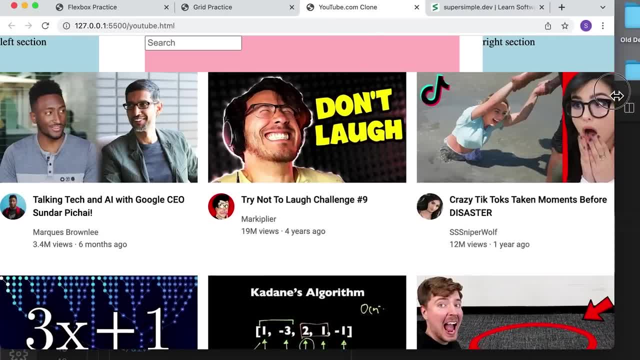 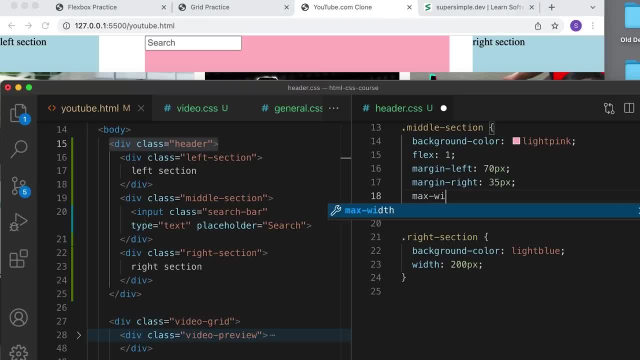 And we're going to limit the width of this middle section first. So we'll go into our code And the property to do that is called max-width And let's set it to 300 pixels. So this property says the width can be. 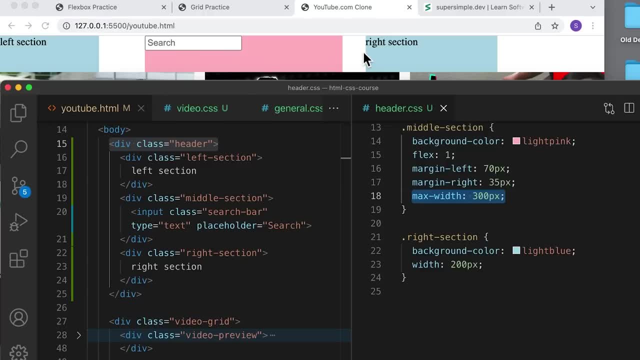 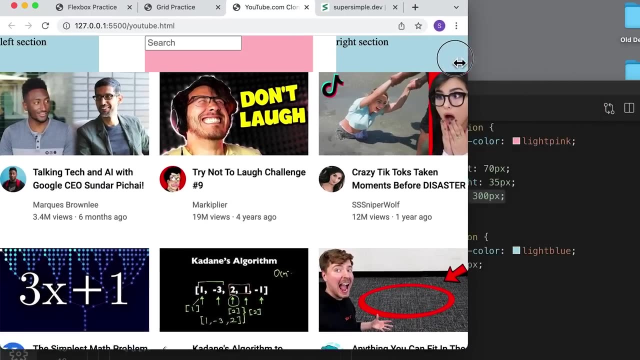 less than 300 pixels, But as soon as it grows to be over 300 pixels, we're going to limit it to 300.. So that's what we see here. Now, when we resize the browser to be less than 300 pixels, notice that it's shrinking and growing. 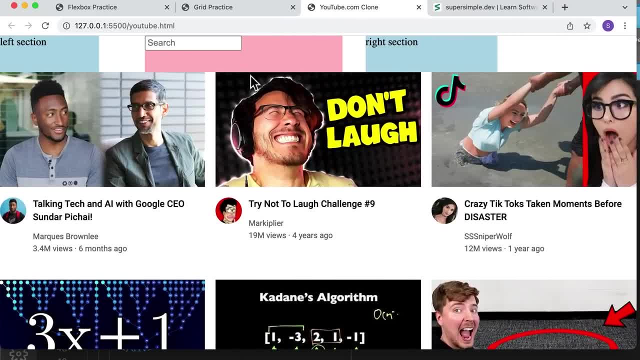 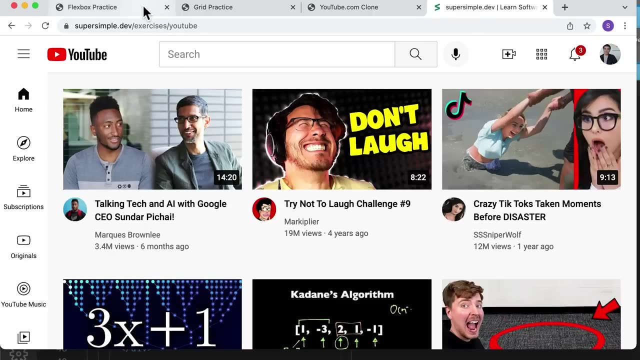 again, But when the browser gets wider, it's limited to 300 pixels because of this line of code. Next, we want to distribute these three sections evenly across our horizontal space, So just like what we have here Now. remember to do that in flexbox. 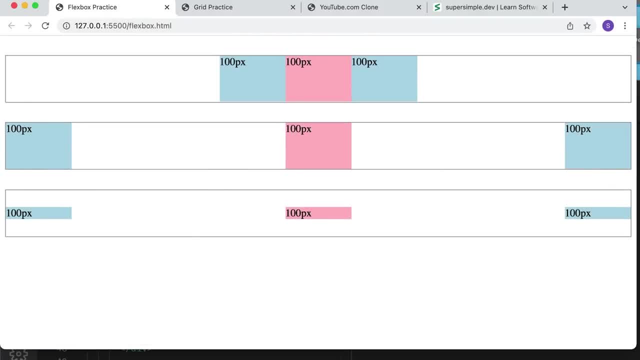 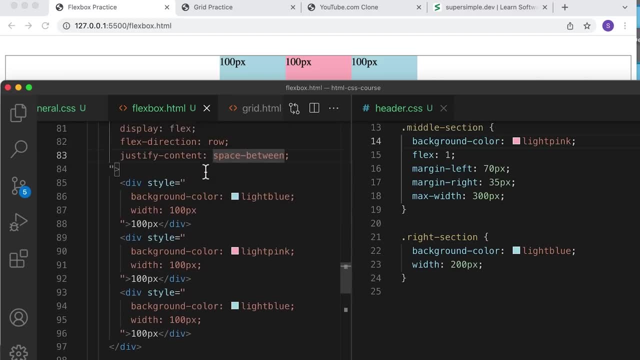 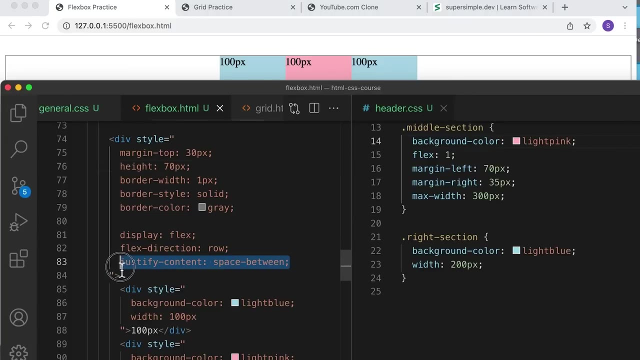 We have an example here. If we go back into our code and go into our flexbox practice file, we can find that example in our code And remember that we achieved this using a property called justify-content space-between And we set this property on our flexbox container. 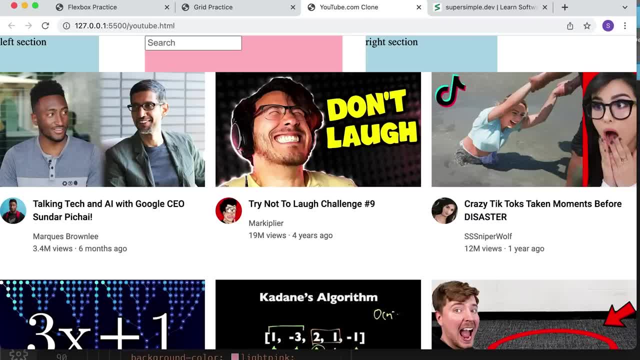 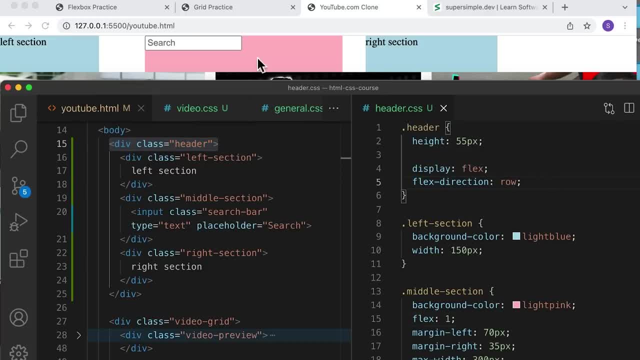 And that's what we're going to do for our project right now. We're going to go up to our flexbox container, Let's go back to our youtubehtml And to spread these out evenly across the entire horizontal space we're going to set. 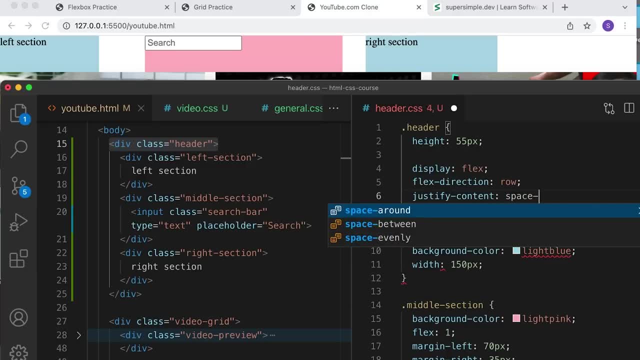 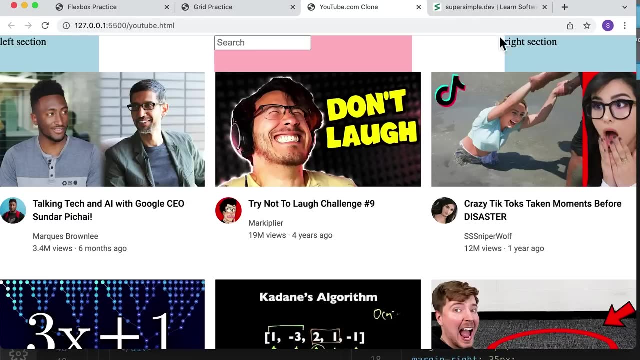 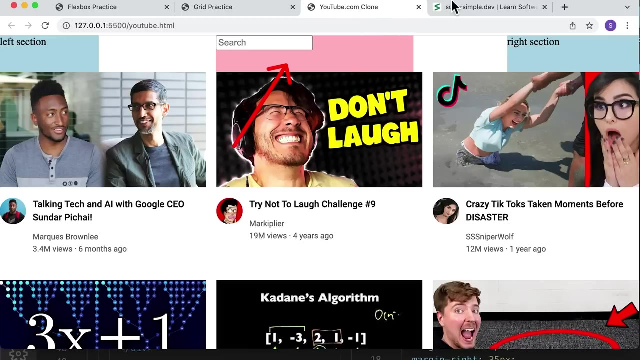 justify-content- space-between. Let's save it. And now they take up the entire space. So if we compare this to our design, we'll notice that the middle section is still a little bit too narrow compared to our design, So let's increase the max width here. 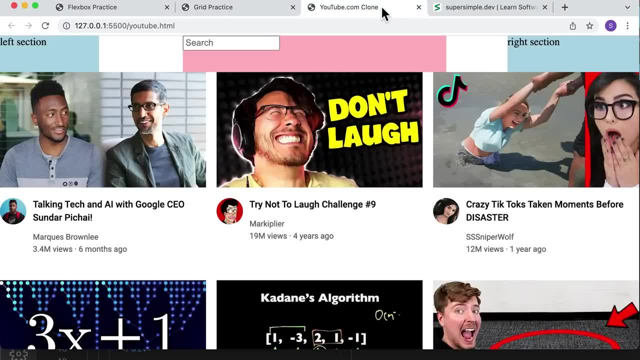 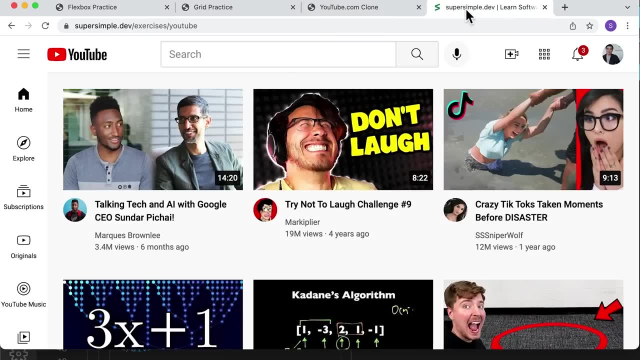 So let's increase it to 400 pixels, Let's see how that looks Okay. so it's still bigger. Let's increase it to 500 pixels, Let's see how that looks Okay. so I think that looks close enough to our design. 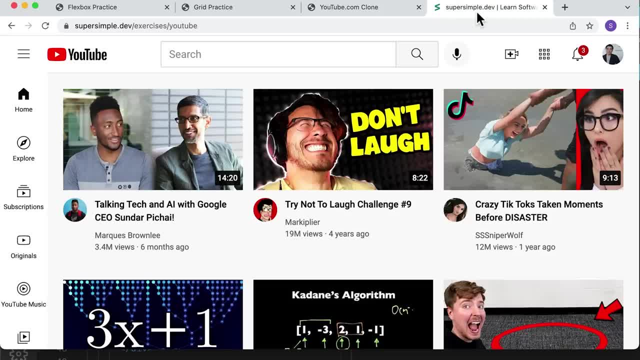 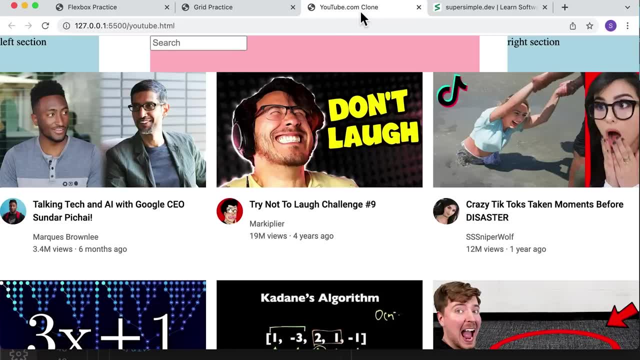 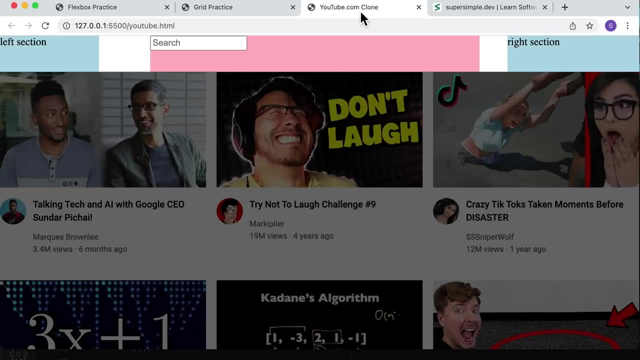 So this middle section in pink is roughly equal to this middle section over here. So that's the end of this lesson. We learned about flexbox and we used it to create the layout for our header. So in this situation, we were mostly focused on our content size. 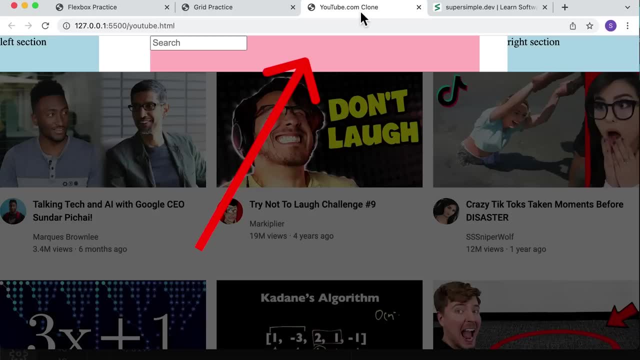 We wanted to make sure the middle section had a max width and at least some space in between. So that's why we used a flexbox, Because we were focused on our content size first, and then the layout doesn't matter as much, We just use a flexbox. 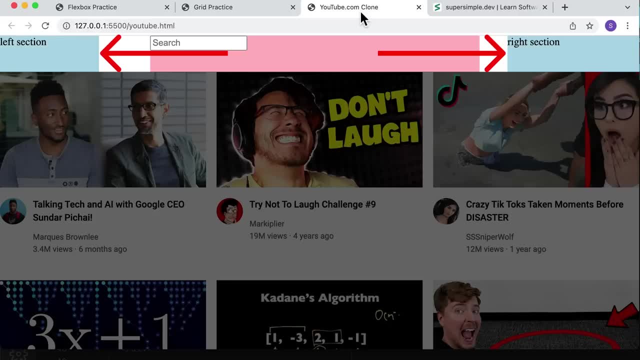 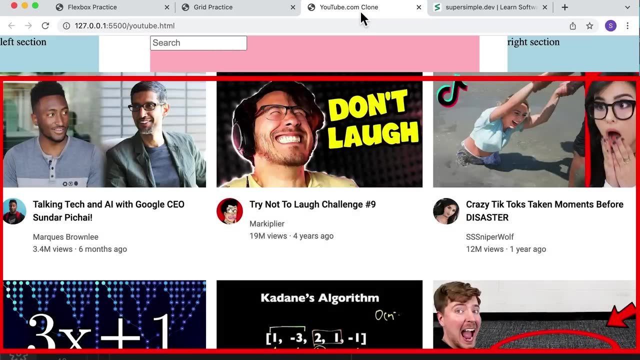 to spread out our content evenly across the horizontal space. So when we focus on content size first, we use a flexbox. When we want to create a grid, we use grid, And for most other situations, for example, this horizontal layout that we created. 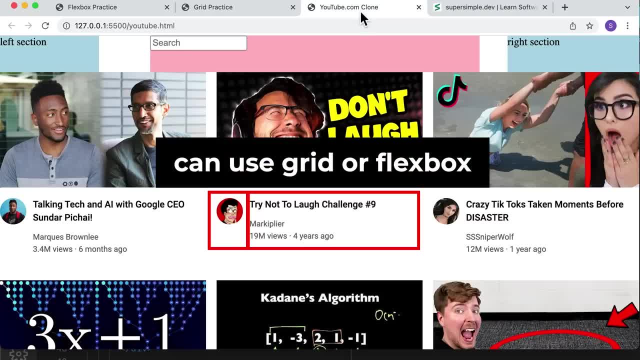 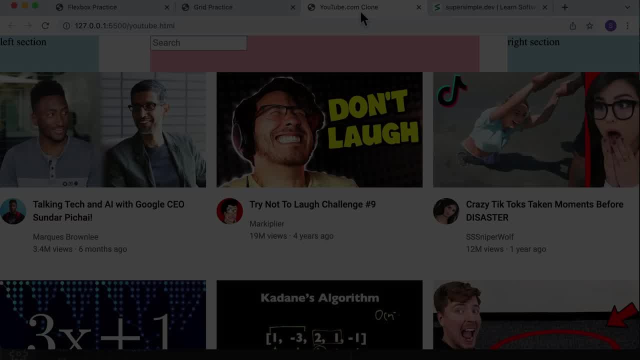 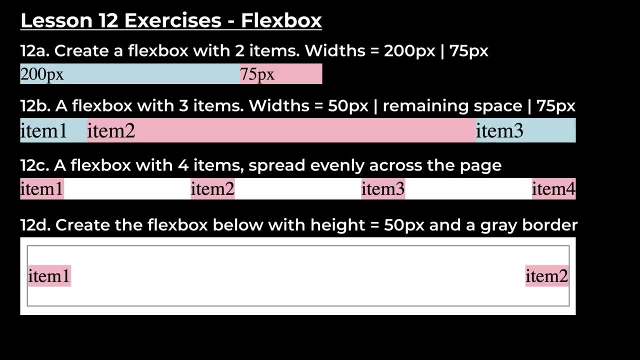 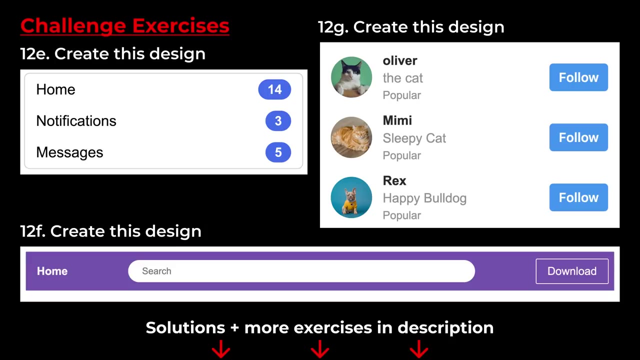 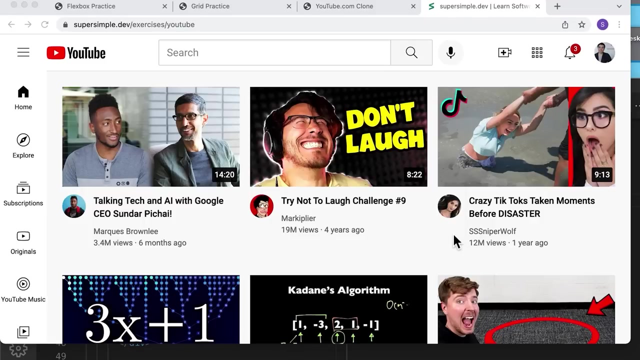 in the nested layouts technique, we can use either grid or flexbox. In most situations they do the same thing. So here are some exercises that you can practice using flexbox to get yourself more familiar with how it works. And now that we have the general layout, we're going to finish. 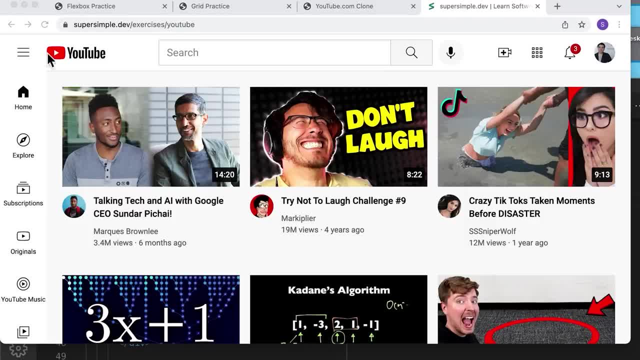 up the rest of the header. Before we do that, we're going to download all of these icons and images that you see here. To do that, we're going to right click, inspect and then click this in the top left and then click the icon we want to download. 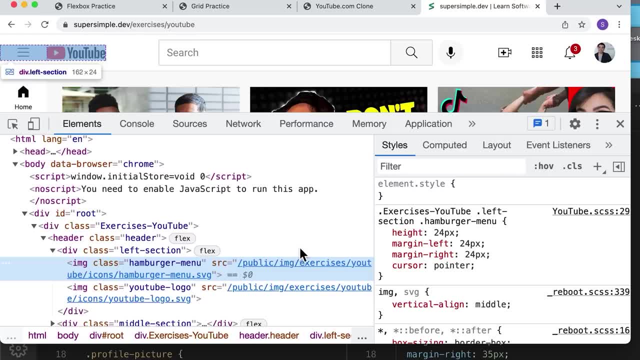 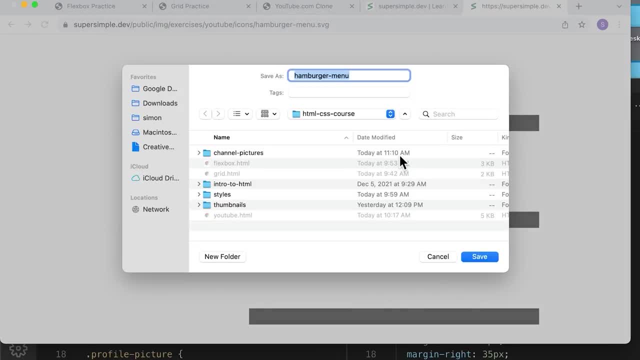 and then we can find the URL down here. I'm going to hover over it and then click this link to open in a new tab and then save it with control s. So I'm going to save this in the folder that contains our code. 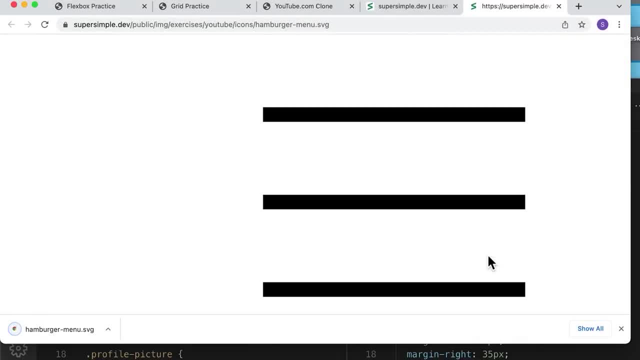 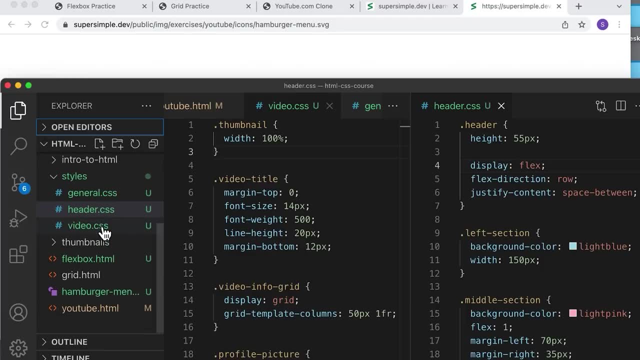 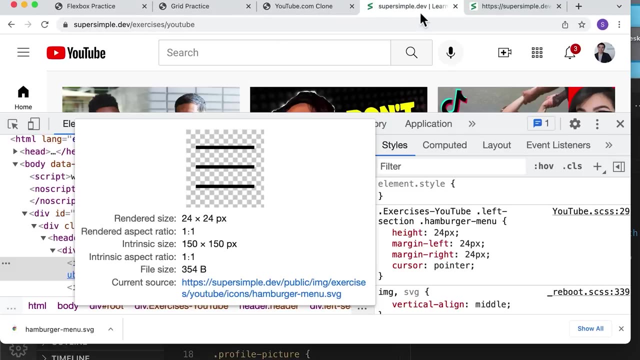 which is this one. So I'm going to save it. and then in our code editor we should see this icon so we can collapse this by pressing that. and then now we have our icon right here called the hamburger menu. Now, looking at our header, we have a lot of 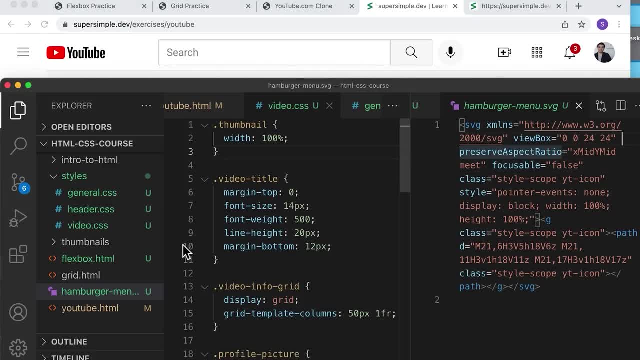 icons to download, so let's organize them using a folder. We're going to create a new folder and let's call this icons. Now we're going to put the icon we downloaded into that folder, So this one right here into this folder. 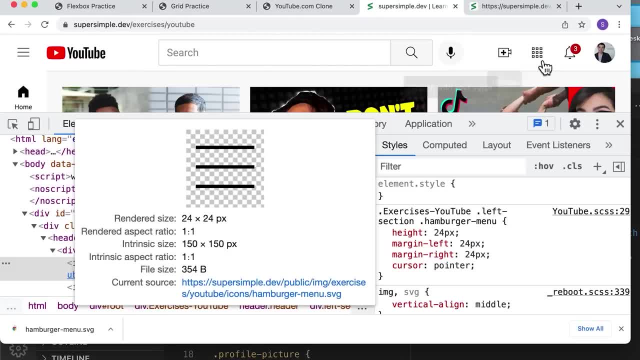 And now we're going to do the same steps: to download all of these other icons and this image that we see here. So we're going to do the same steps: click the top left and then click the icon we want to download, and we can find the link here: 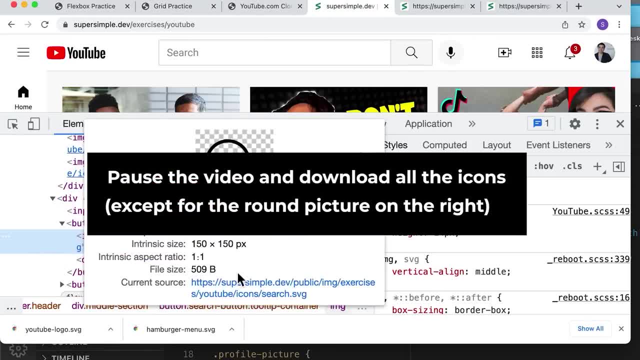 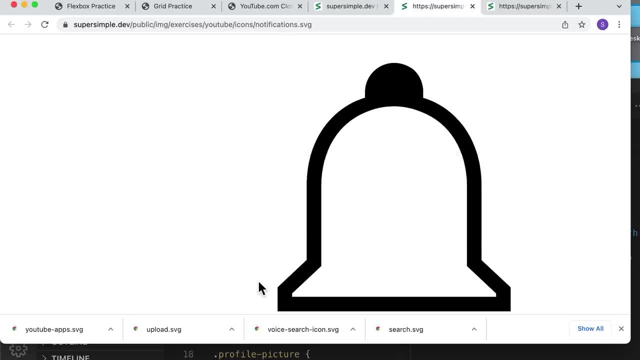 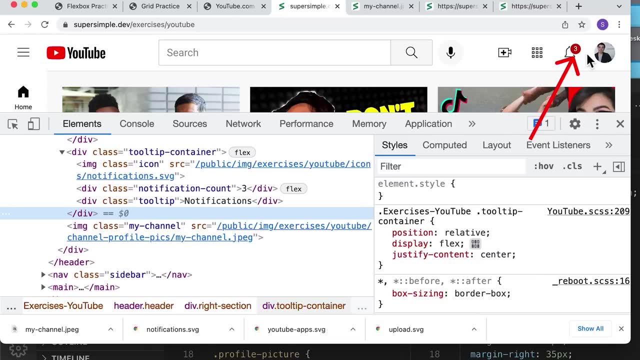 I'm going to fast forward the video here because it's just a bunch of repetitive steps and we'll continue after we downloaded all the icons. So when you get to the notification icon, don't worry about this notification number here. we're going to learn how to do that in the next section. 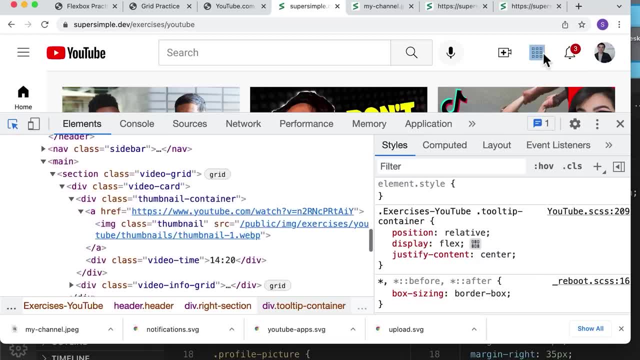 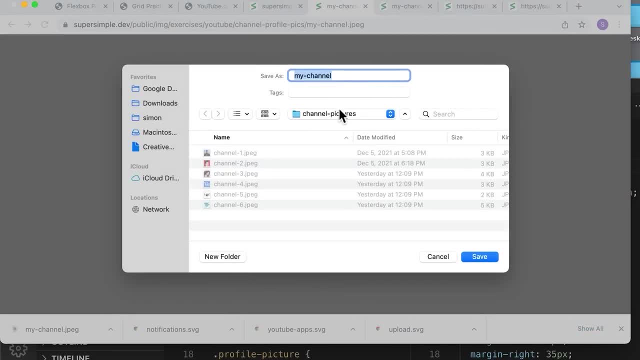 And for this channel profile picture, when I download it, I'm actually going to save it in a different folder from the other icons. So if I download this here and save it, I'm going to put this in the channel pictures folder instead of. 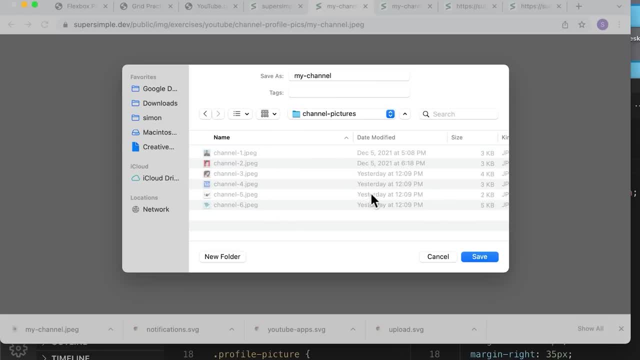 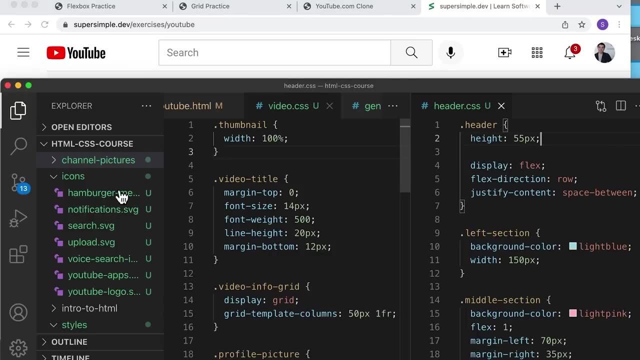 the icons folder Because technically it's a channel picture. So once we have all of that downloaded, let's check in our code editor and we should see all of the icons that we need for the header inside the icons folder, as well as the channel profile picture on. 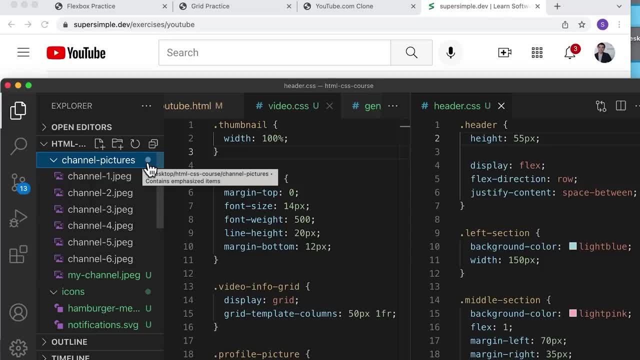 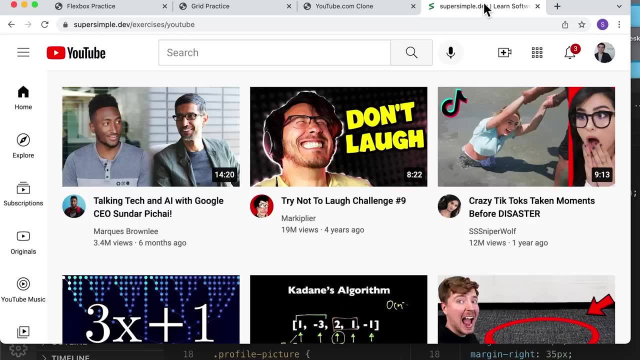 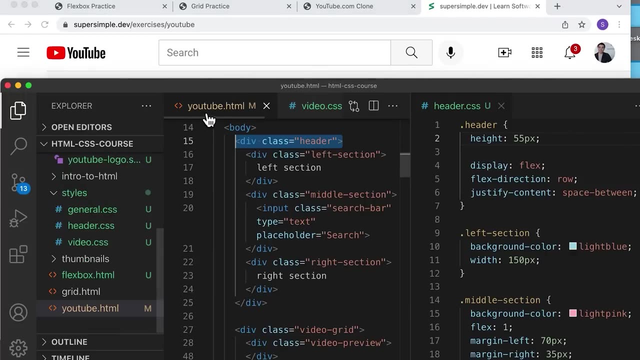 the right in the channel pictures folder, And now we're ready to complete our header in our current project. So in our left section we have this which is called a hamburger menu and the YouTube logo. So in our HTML, in this file in our left section. 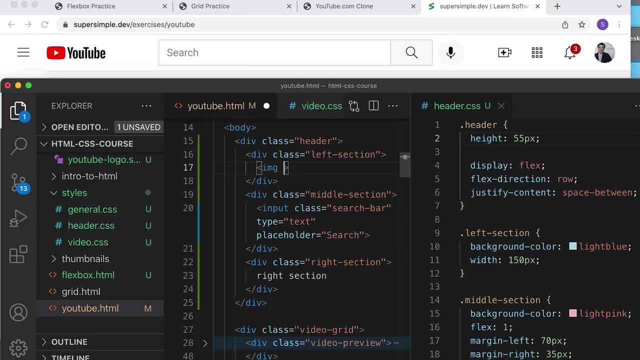 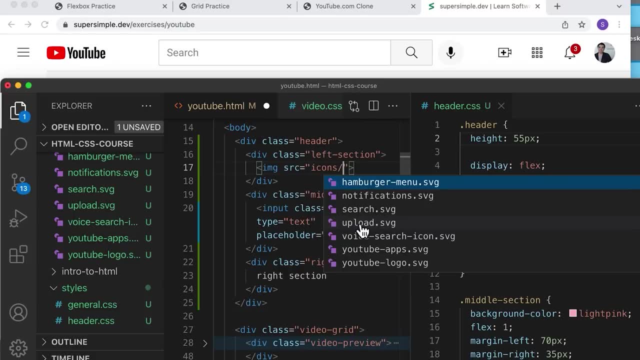 we're going to have an image and we're going to tell it what to load. So loading an SVG is the same thing as any other image. We're going to go into the icons folder and we're going to load the hamburger menu dot SVG. 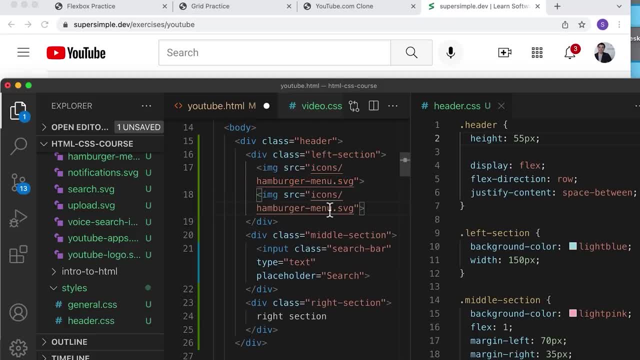 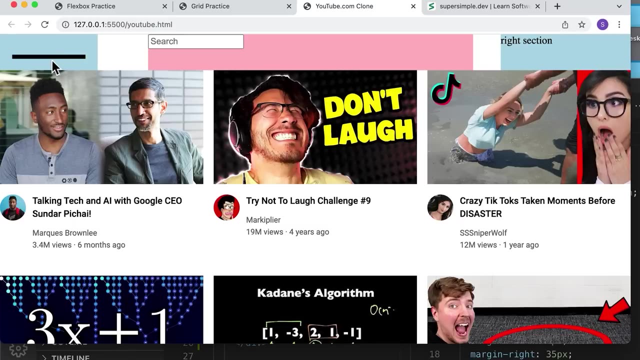 And then we're also going to load the YouTube logo, which is right here. So YouTube logo dot SVG. Save that and look at our webpage and refresh. So the images are loaded, but they're way too big, Let's make them smaller. 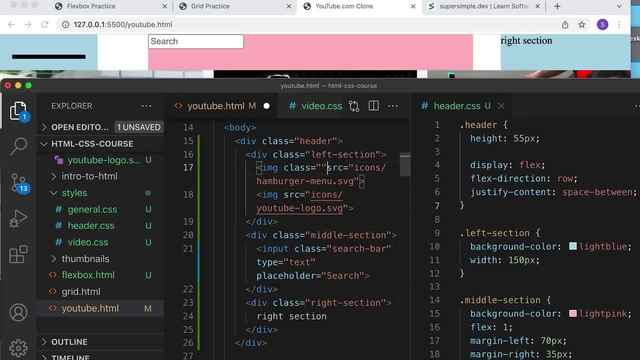 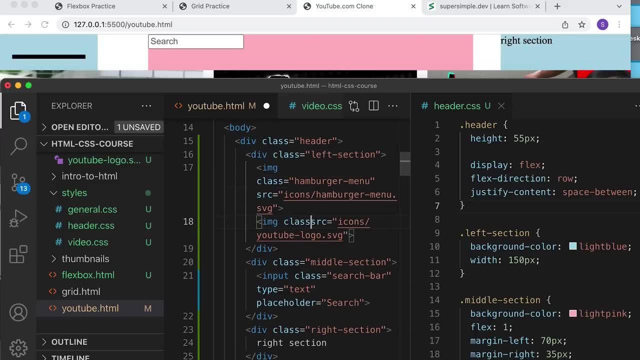 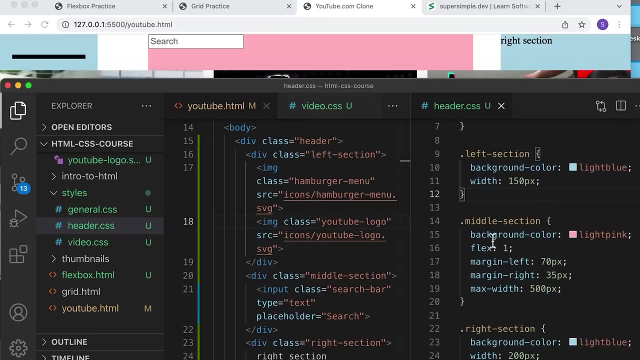 We're going to set a class so that we can target them with CSS. So hamburger dash menu, And for this one let's set a class of YouTube dash logo. And now in our CSS, let's go in here and target the hamburger. 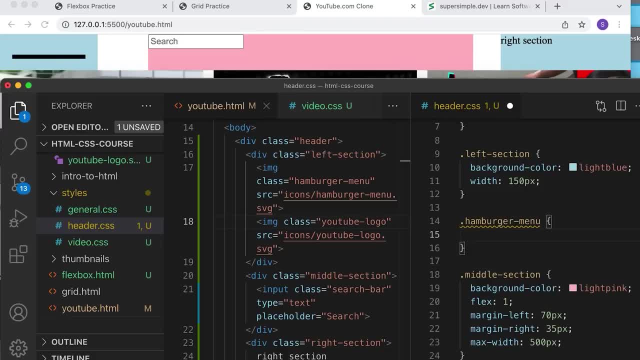 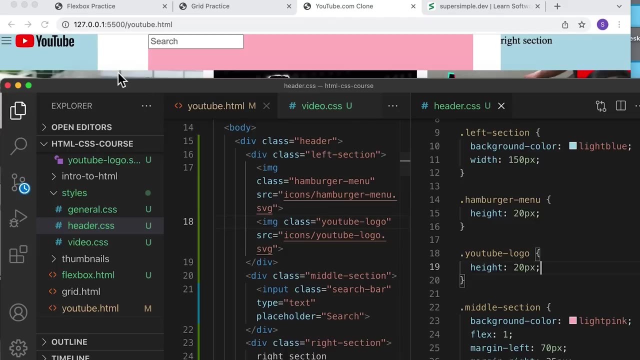 menu class And let's set the height to something like 20 pixels. And same thing for the YouTube logo: We'll set the height to 20 pixels. Okay, so that looks pretty good. Now, if we look at our design, we'll notice that these images are actually. 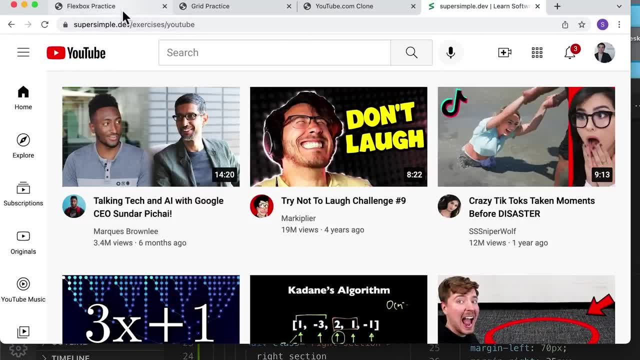 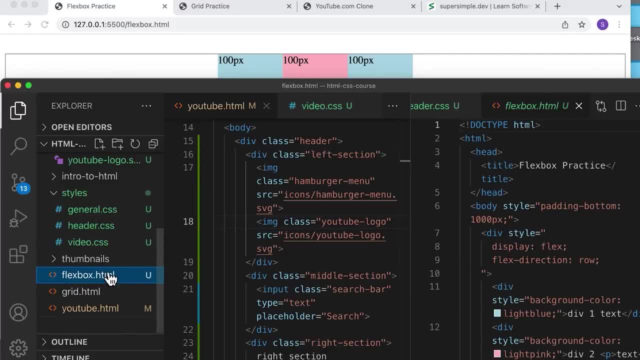 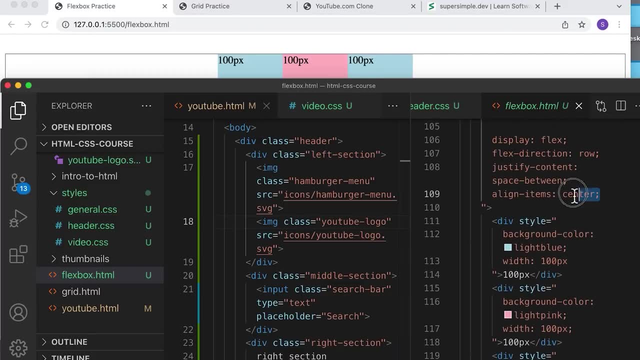 aligned vertically in the center. So in our flexbox practice file we learned how to do this. if we look at our code again, If we look at our flexbox code, let's scroll all the way down to the last example. We did this using align items. 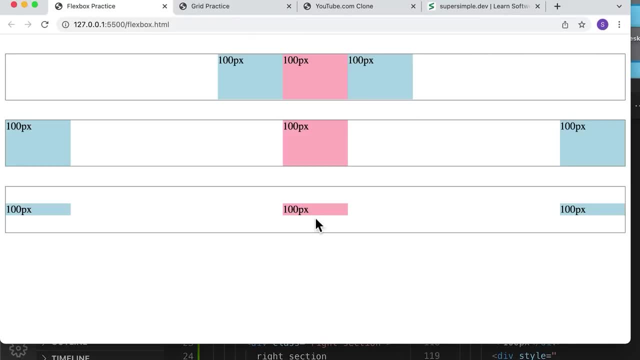 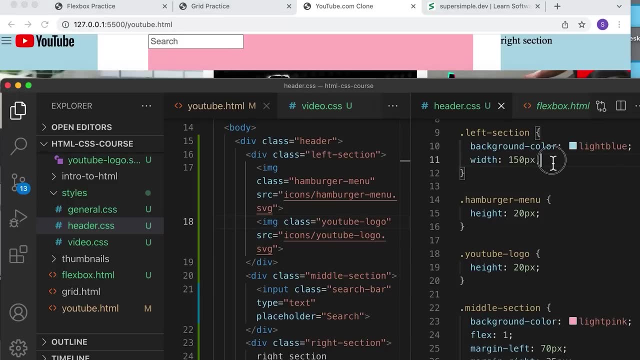 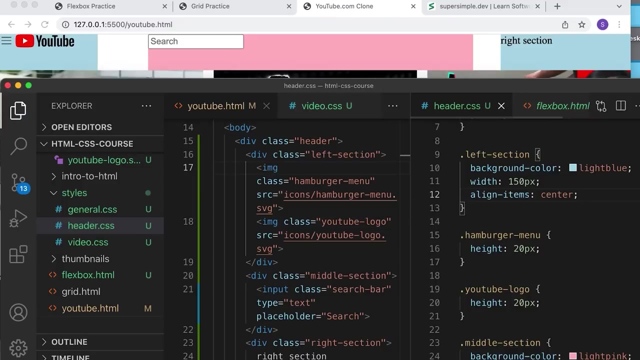 center So that aligns them vertically in the center like this. We'll go back to our header CSS and just have this as a reference. So for our left section, we're going to set align dash items colon center. However, you'll notice that it didn't do. 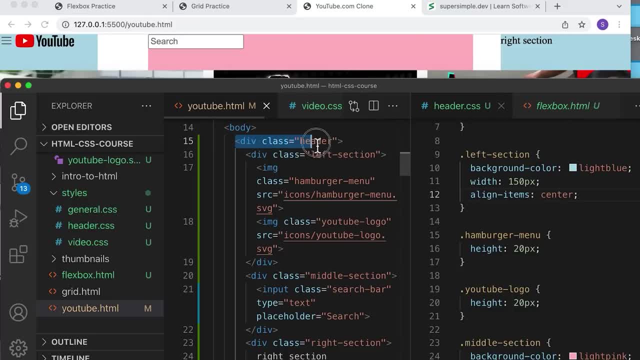 anything, And that's because, if we look at our HTML, the header is a flexbox, But this left section here is still a regular div. It's an element inside the flexbox, but this itself is not a flexbox. So align items doesn't do anything. 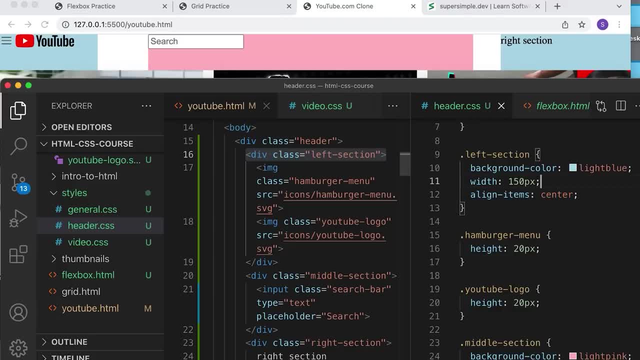 Now to fix this. we can actually turn the left section into a flexbox using display flex And if we save it now, the left section is a flexbox, so align items will align it vertically in the center, So flexbox doesn't actually. 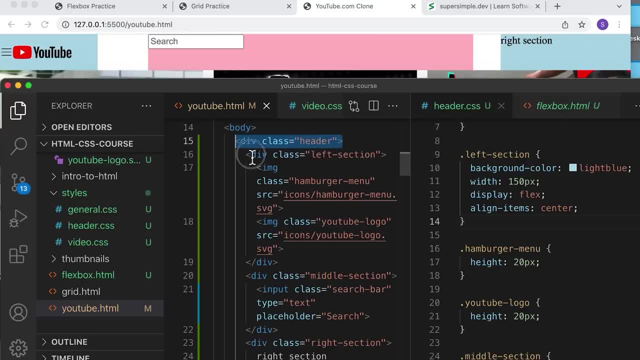 go down two layers, It only affects elements on the first layer, like this div and this div. If we go down another level, like here, flexbox doesn't affect it. That's why we have to turn this into a flexbox as well, in order to use properties like 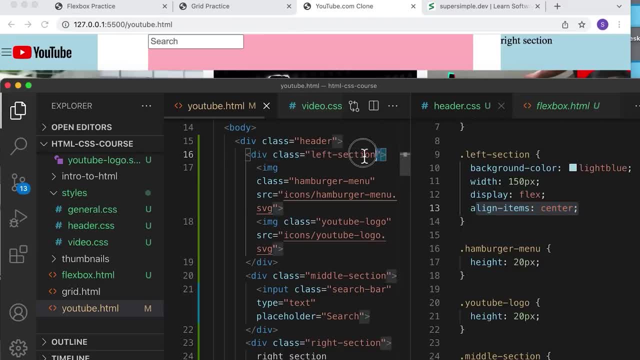 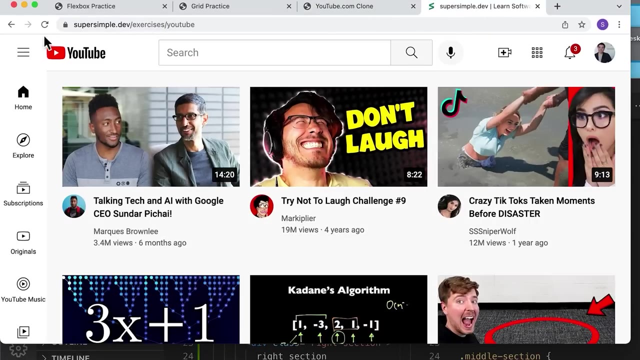 align items center. So this situation of putting a flexbox inside another flexbox is totally valid. If we want to target another level of elements like this, Let's go into our design and compare it And you can see that for our design there, 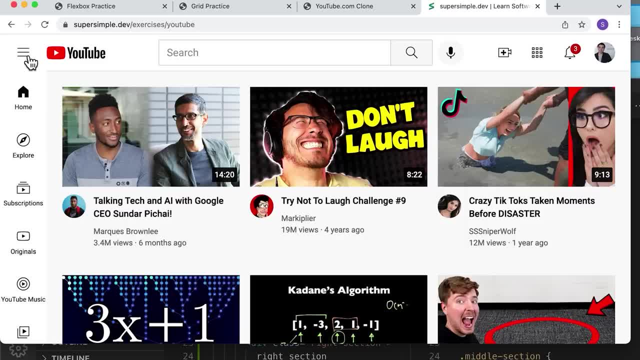 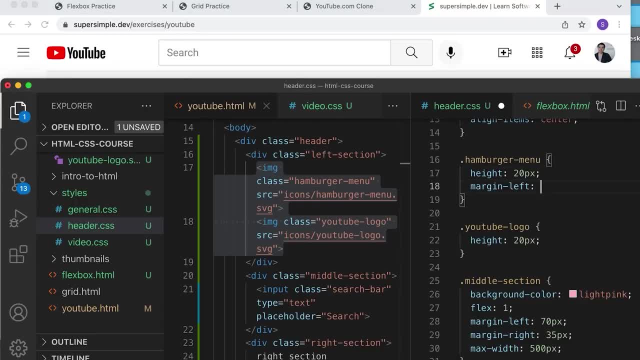 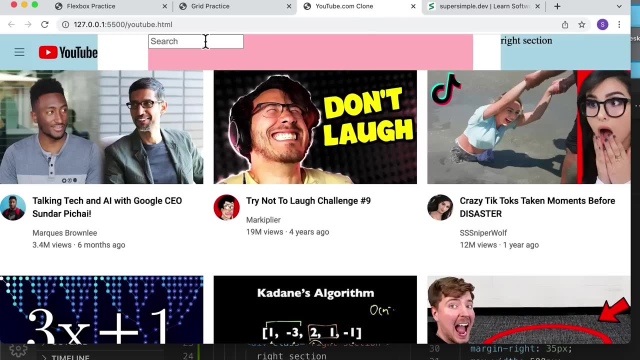 is some spacing on the left and the right of the hamburger menu, So we can create that right now using margin-left- 20 pixels and margin-right of 20 pixels. So we'll add 20 pixels on both of these sides. So if I go back and forth, 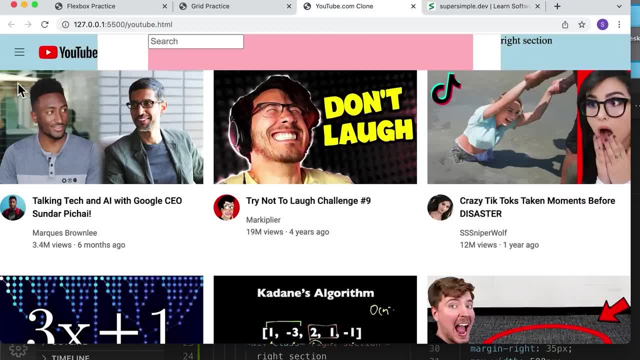 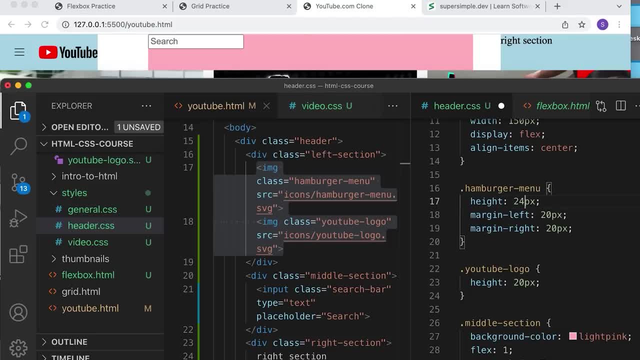 you'll notice that this icon is a little bit bigger than our project. So we can actually adjust our height here to make our icon a little bit bigger. We can maybe set this to 24.. And let's compare it. Okay, so that looks pretty close. 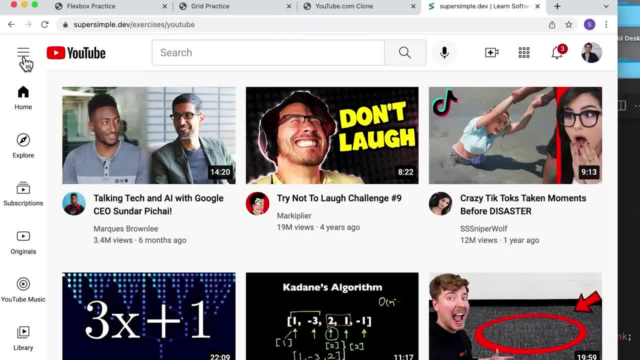 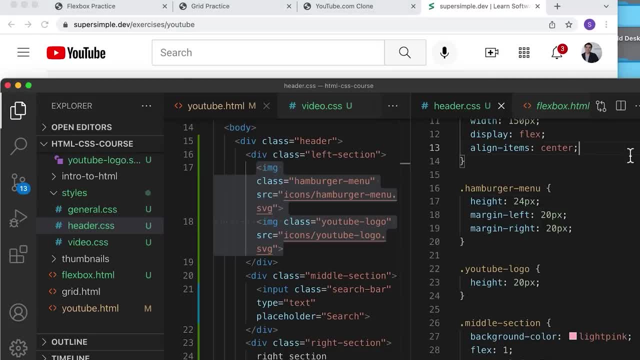 So now I notice that this icon is a little bit to the right of our website, which is here, So you'll notice that it's a little bit to the right. We need to add more spacing, So let's add margin-left of maybe 24 pixels. 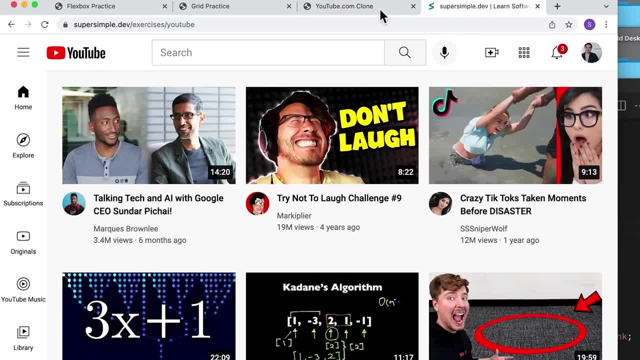 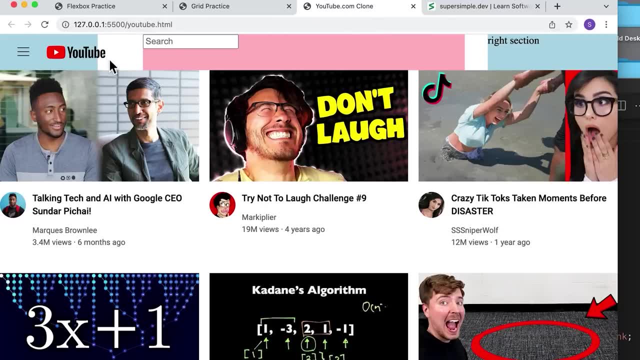 Save it Now. if we compare the two, So that looks pretty much close to what we need, And the YouTube logo is also in the same place, So that's a bonus for us. So now it looks like the left section is pretty much done in our 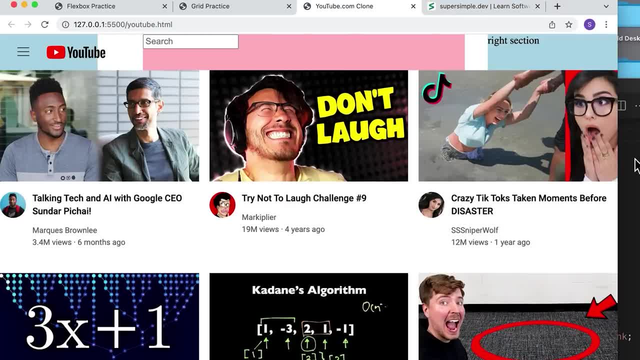 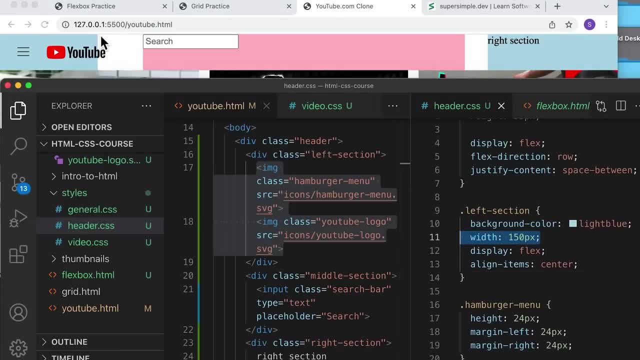 project And we can get rid of this background color that we were practicing with. First, we're actually going to remove the width, So this width of 150 pixels is forcing the left section to only end up here. However, if we remove this, the left 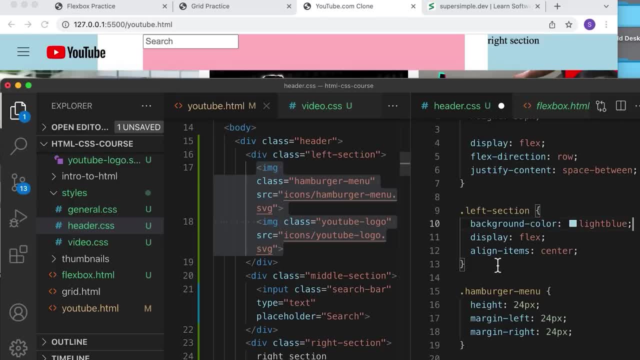 section will stretch to contain all of its content. So if we save it, you can see that it stretches. Now we can remove the background color And that's done. Next we're going to work on this middle section. So for this middle section in our 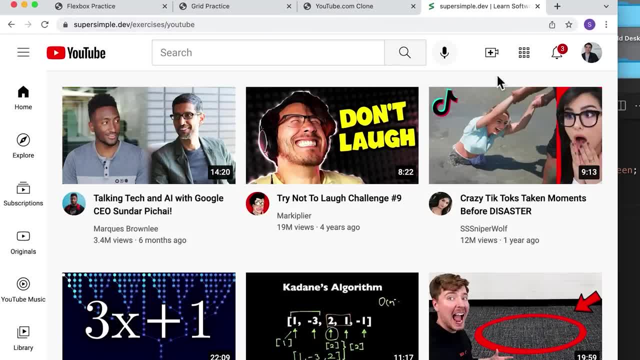 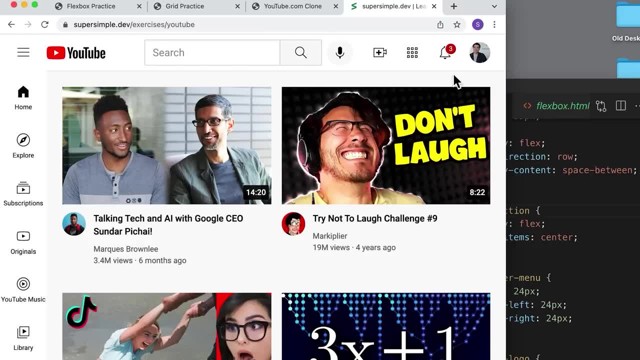 design. we have an icon here, a button here, and if we resize you'll notice that the search box also resizes. So this search box is going to grow with the rest of the page. So we already learned how to do that. As a reminder, 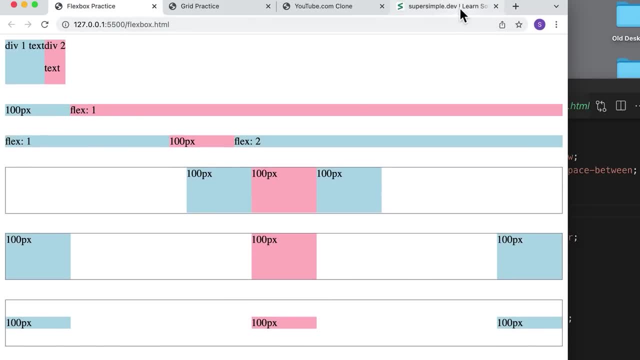 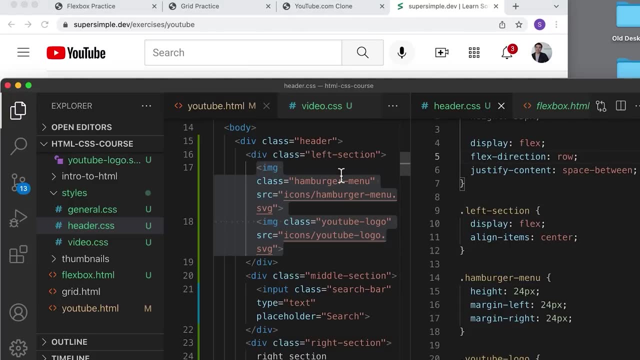 it's flex 1.. So first let's go in and create these two buttons. first, because that's the easy part, Let's go into our code In the middle section here after the search bar, we're going to create two buttons. 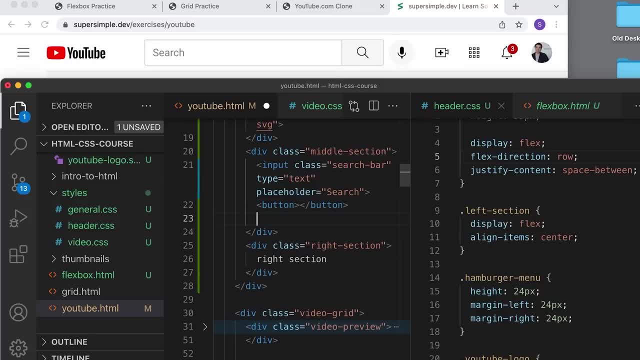 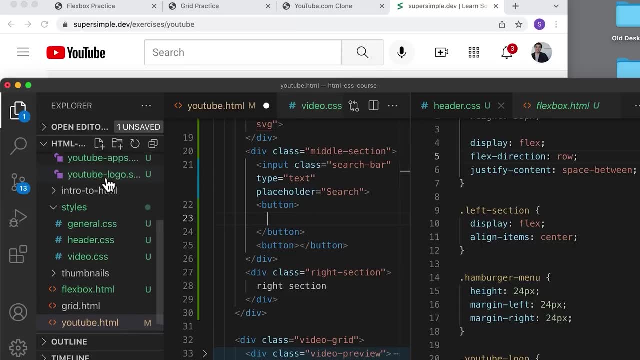 Let's create one button here and another button down here. So inside this first button we're going to have this search icon. So if we go into our icons folder, it's this icon here, searchsvg- So we can create an image element. 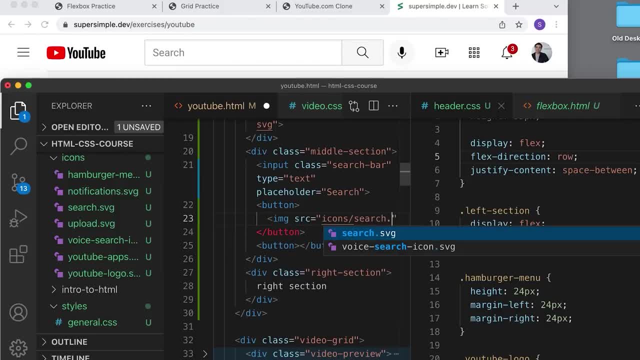 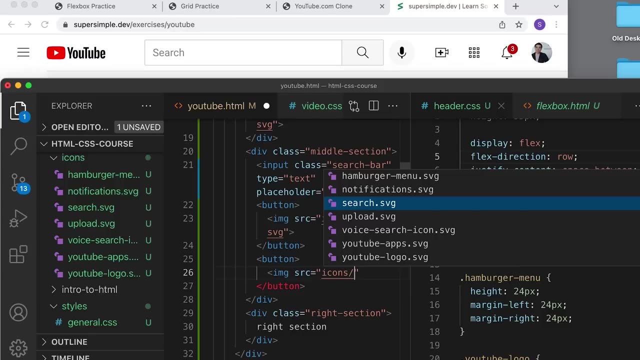 source and icons: slash search dot svg. In the second button, we're going to have our voice search icon, which is this one, And we're going to create another image element and we're going to load icons: slash voice search icon. 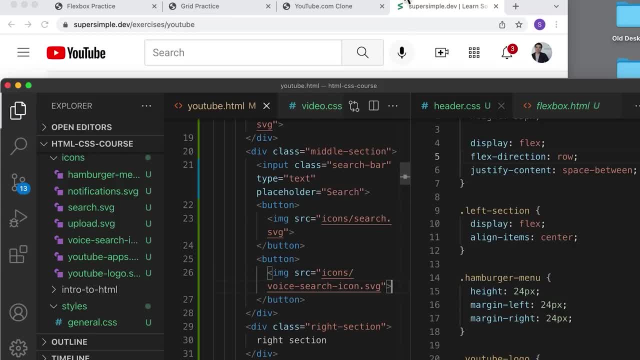 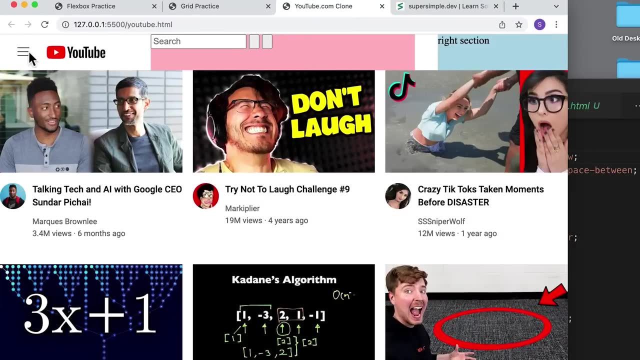 Now let's save it and see how that looks. Okay, so that didn't work out very well, probably because, if you remember, when we loaded this icon here, it was super big, So the two icons we loaded are probably super big and we only see the top. 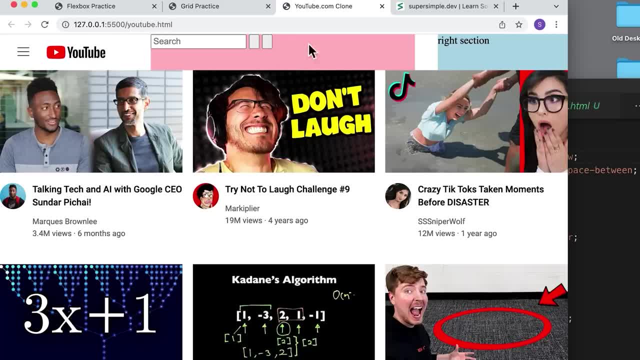 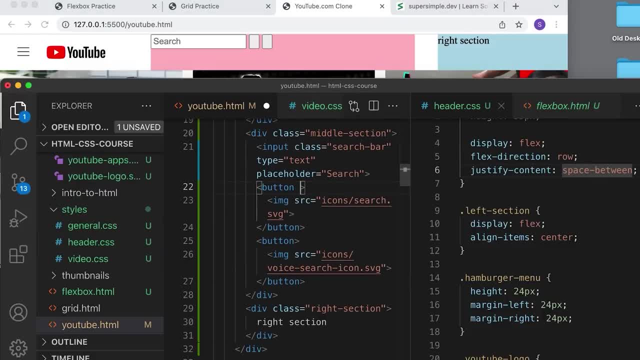 left corner, which is empty. So first let's make our icon smaller and make our buttons a little bigger. Let's go into our HTML. We're going to add some classes so that we can target it with CSS. So class, let's call this the. 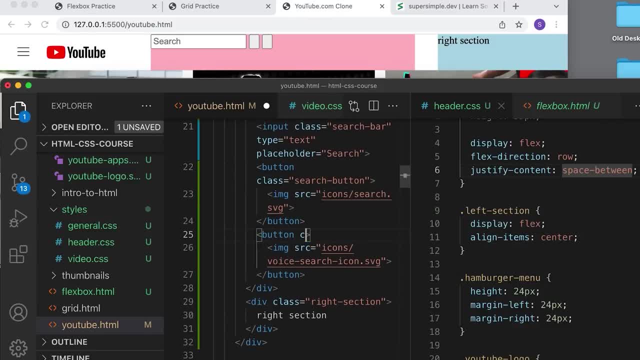 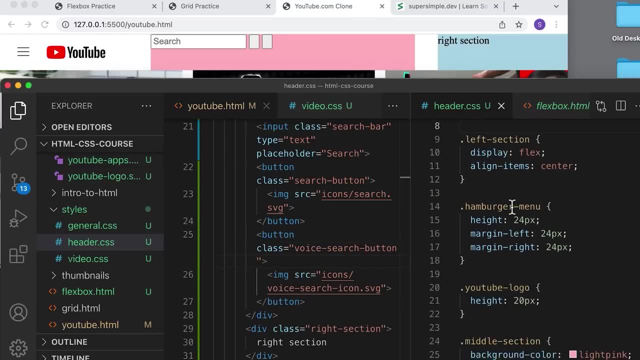 search dash button, And let's call this one the voice dash search dash button. So we're going to go to the middle section here. We're going to target the search button first. Let's set the height to something like 40 pixels and set the width. 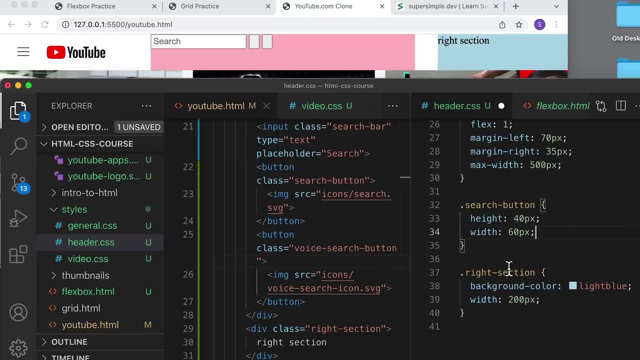 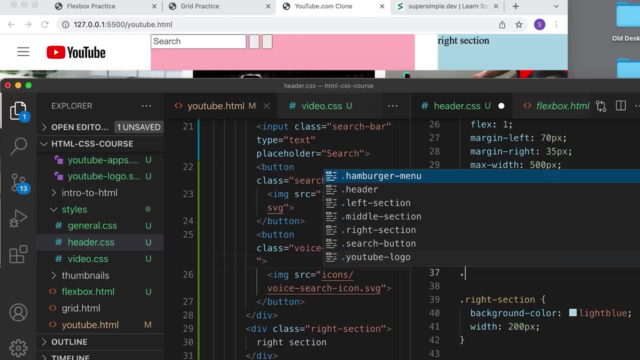 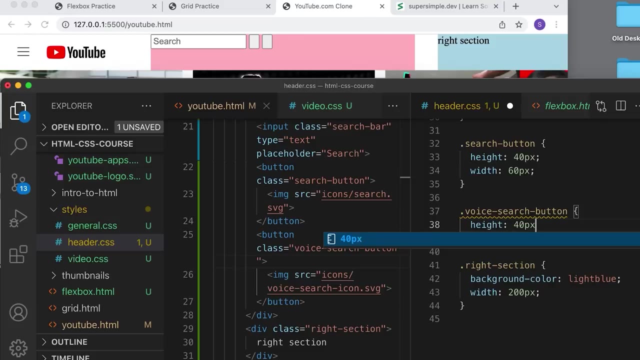 to something like 60 pixels. And for the voice search button, if we look at our design, it's pretty much round. So let's target voice search button, Let's set a height of 40 pixels And we'll set the width. 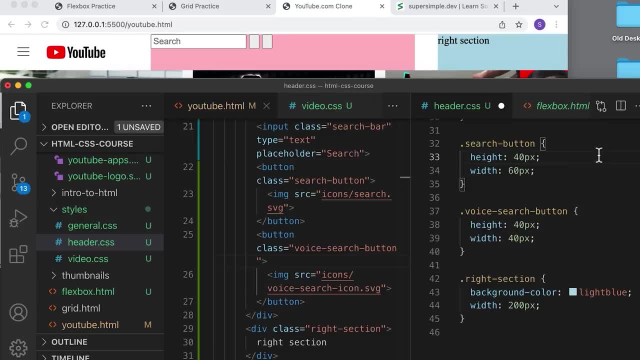 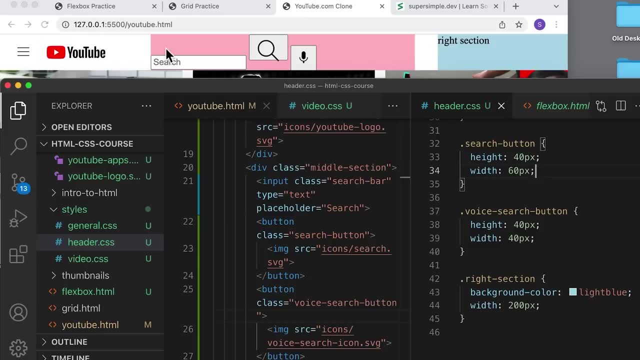 to 40 pixels as well, So let's save it. Okay, so that looks super weird, but we're going to fix this right now, So remember that we want to align these in the center vertically, just like this, To do that. 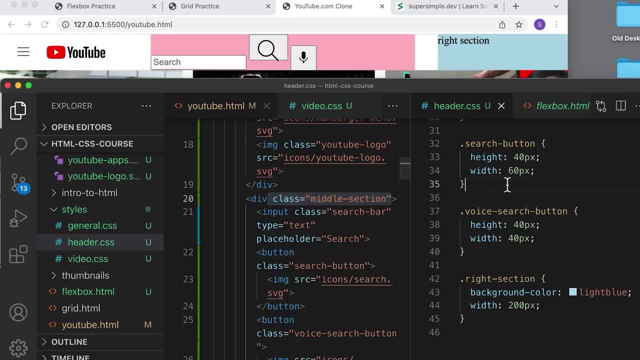 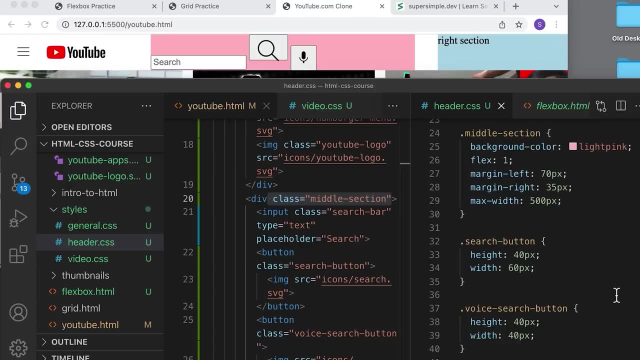 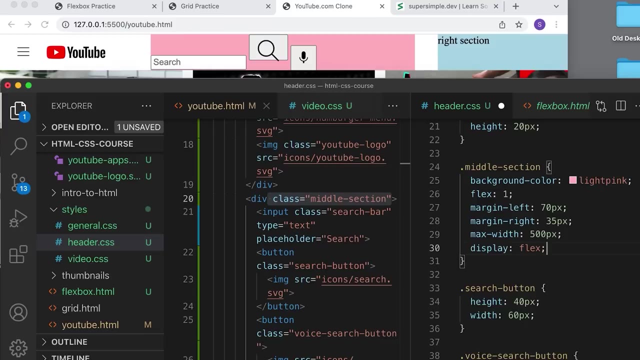 our middle section is also going to be a flexbox And then we can use the align items property that we use for the left section. So let's make this middle section a flexbox And we're going to set display to flex And we're going to set 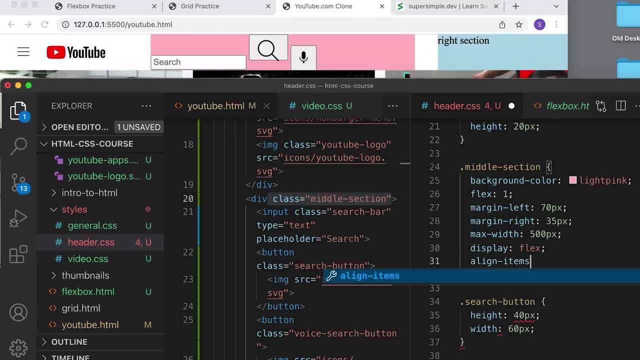 align dash items to center, Just like our left section. So now, if we save, you'll see that everything is aligned to the center and now it's ready for us to style. So there is one thing that I left out, which is: 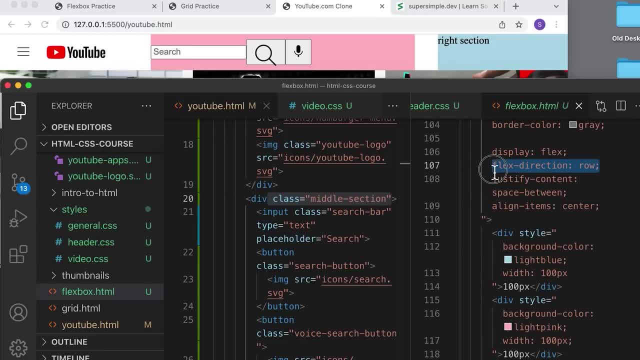 flex direction row. So this tells a flexbox to layout our content horizontally and this is actually the default value, so we don't actually need it. I put it here just for our practice code, But for our header we can be safe actually leaving that. 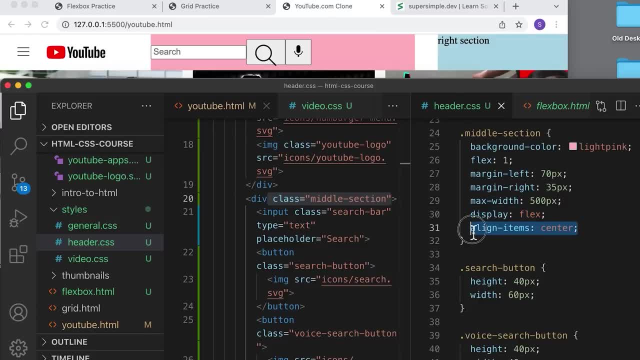 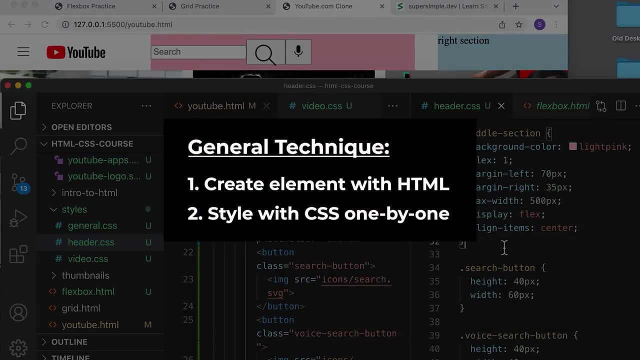 line out and just having display flex and align items center. So now that the layout is good, we're going to go back to our tried and true method of styling this one by one with CSS. The first thing I'm going to adjust is this search bar. 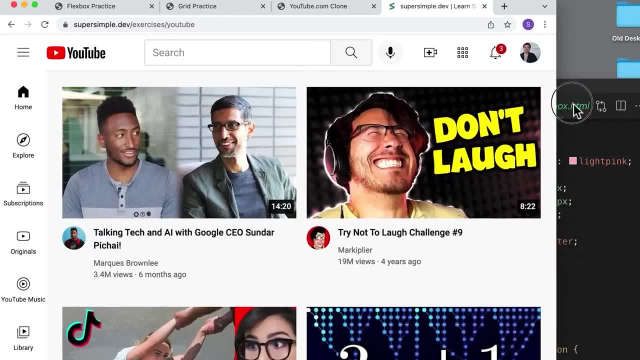 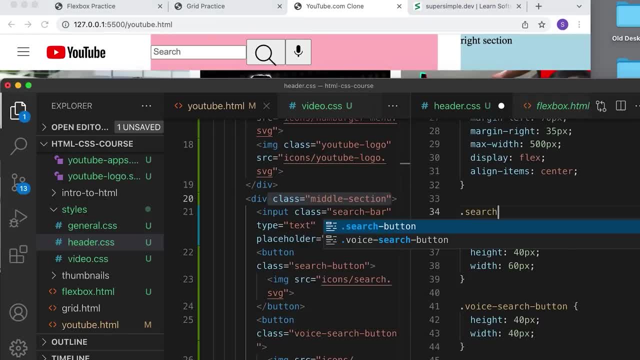 So notice that it stretches to fill up the content when we resize the page. To do that, we're going to go into our code. We're going to target the search bar- search-bar- right here And remember to stretch it to take up the. 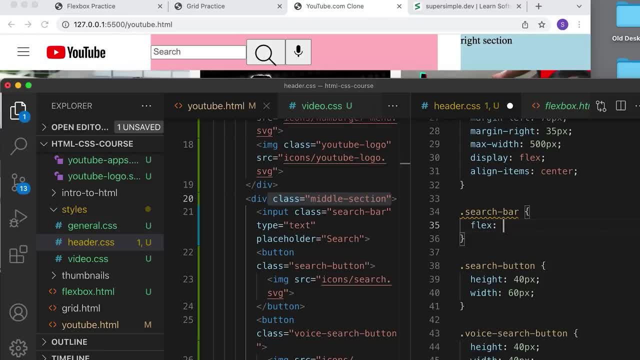 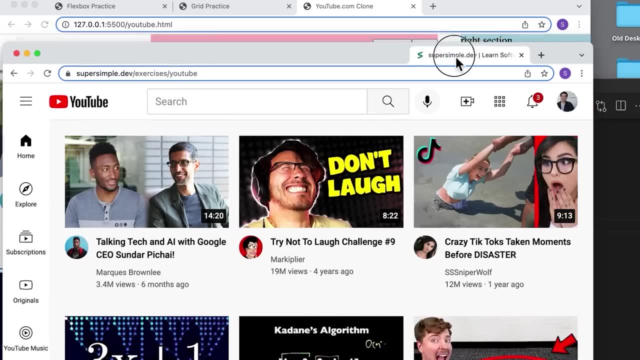 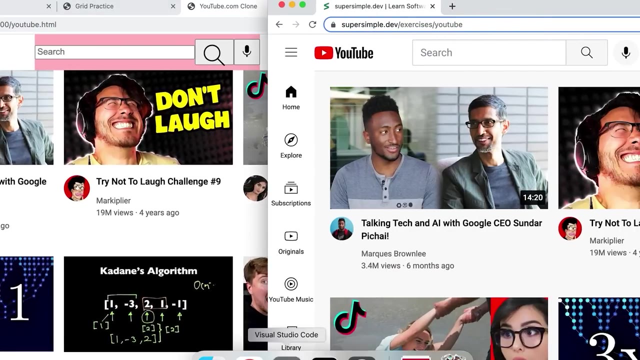 remaining space. We're going to set flex1 and save. Now let's make the search box similar to the design. So I'm actually going to move this here side by side so that it's easier to copy from. So I'll go back into my 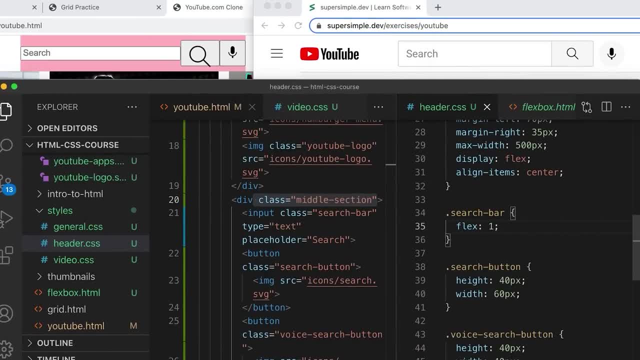 code, and the first thing I'll adjust is the height. So let's set a height of 40 pixels. Okay, that looks a little too much. Let's set the height to 36.. See how that looks. So I think it's still a little too much. Let's set it to 34.. 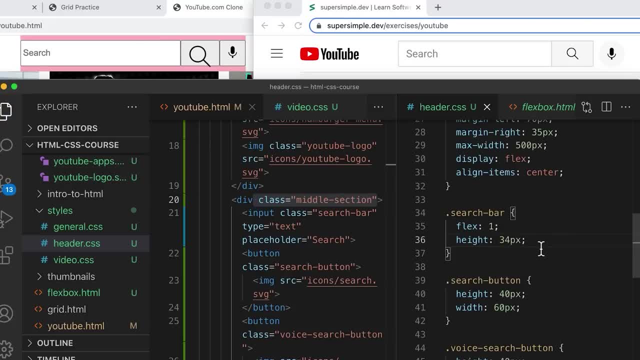 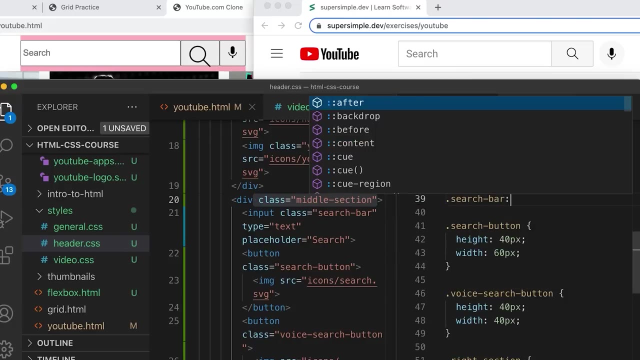 And that looks pretty good to me. Next, let's adjust this placeholder text. So to adjust the placeholder we actually need another sort of pseudo class. So we're going to type search-bar to target the search bar, And then we're going to type: 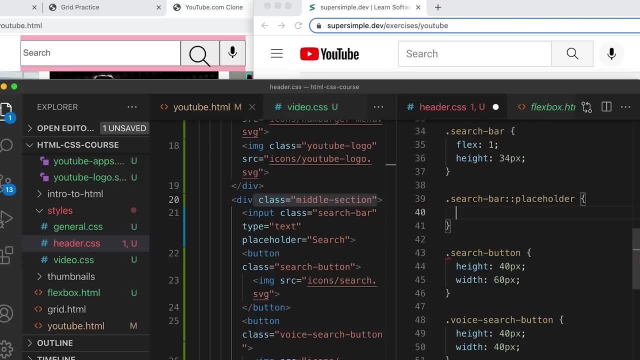 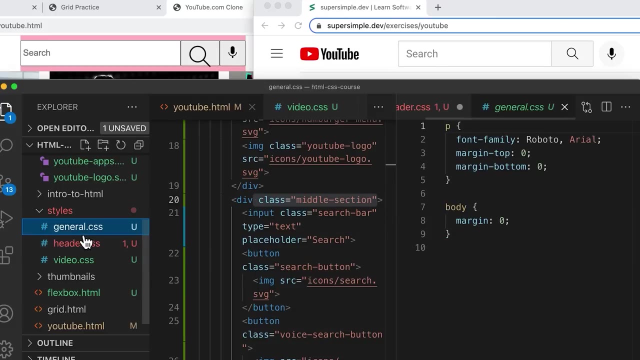 colon, colon placeholder. So this is how you target the placeholder on an input element like this. So first let's set the font-family to the one we're using for this page. If we go to generalcss, we're using Roboto comma. 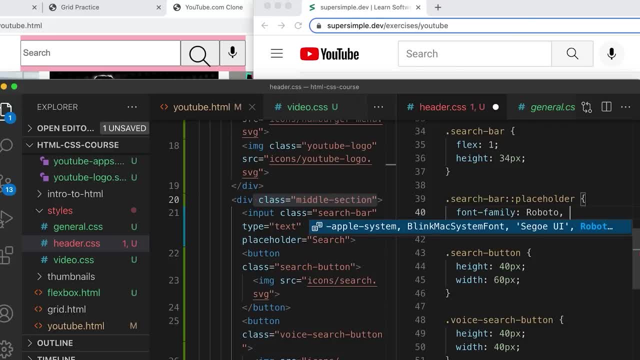 Arial. So we're going to set that to Roboto comma Arial, Save it. So the font changed a little bit. We're going to change the font size to make it bigger Font-size to 16 pixels. let's say, Okay, I think that looks a little bigger. 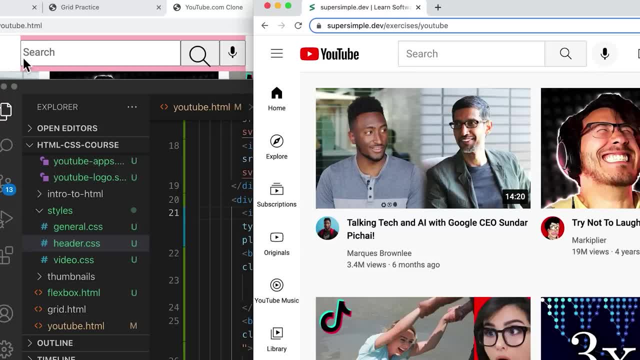 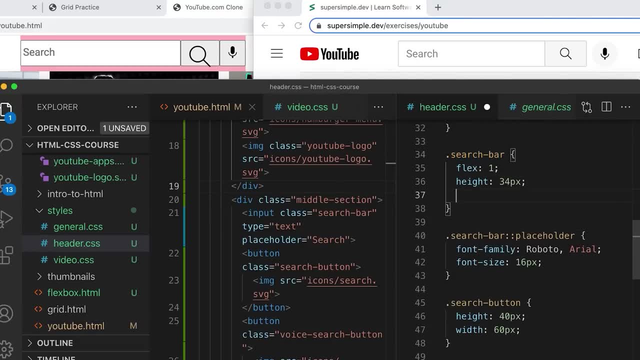 And then next we'll notice that on the inside of this input we have a little bit of space. Well, we don't have that much space here, So we're going to set some padding on the left of our search bar. So let's set the padding. 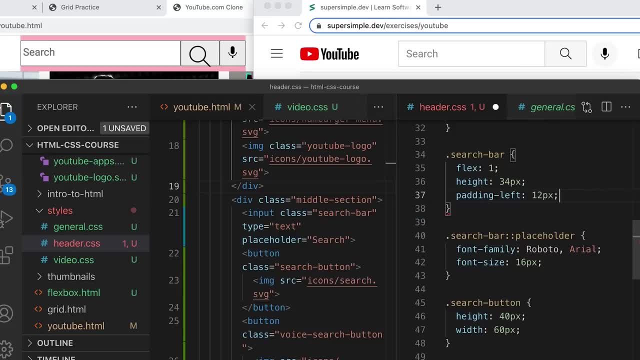 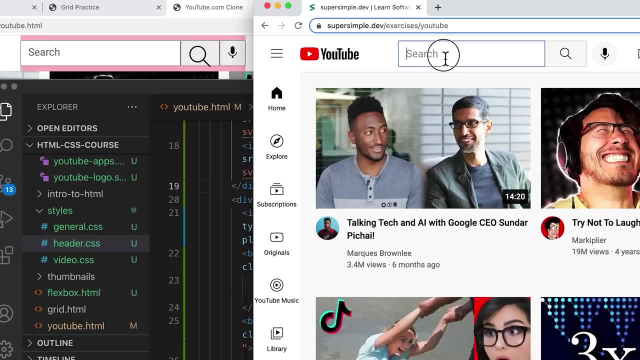 dash left to 12 pixels. Save it. Okay, that looks okay. Let's actually set it to 10 pixels. And then, when we start typing into the search bar, notice that the font is bigger, But for here we still have the small font. 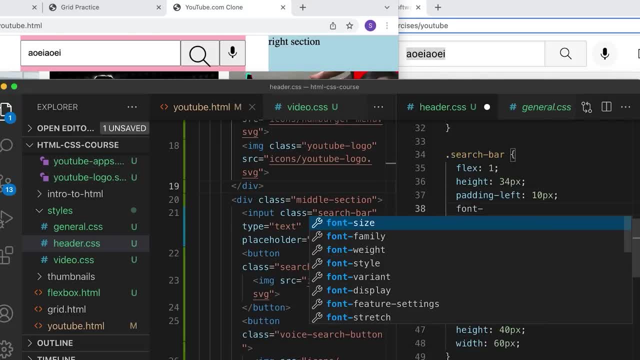 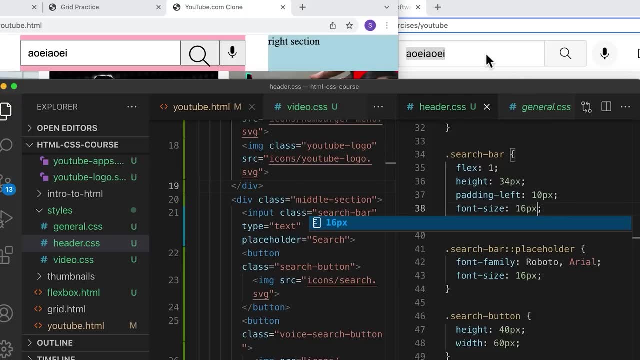 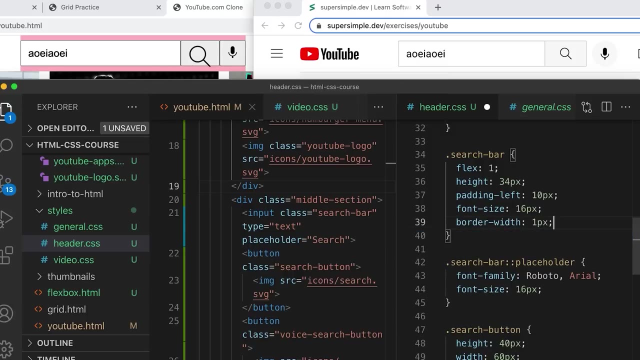 So we can set the font size to 16 pixels. See how that looks. Okay, so that looks pretty close to what we have. And next I'm going to change the border. So I'll set the border dash width to 1 pixels. 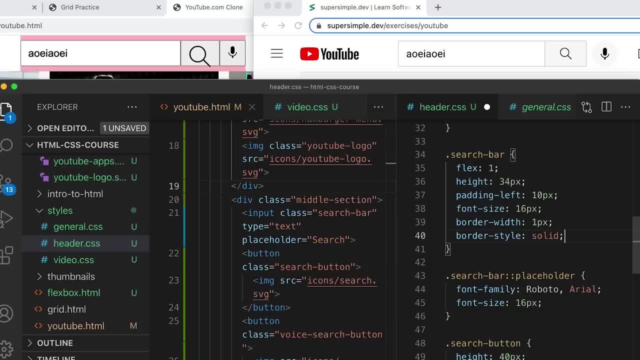 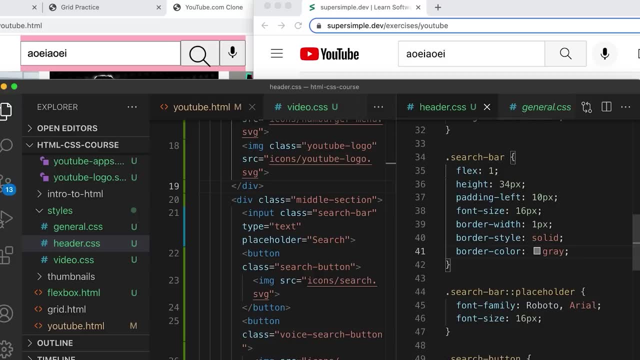 The border style. we want it to be solid And finally, I'm going to set a border dash color of gray. Let's see how that looks. Okay, so I can't really tell the color because of the background. We're going to remove this. 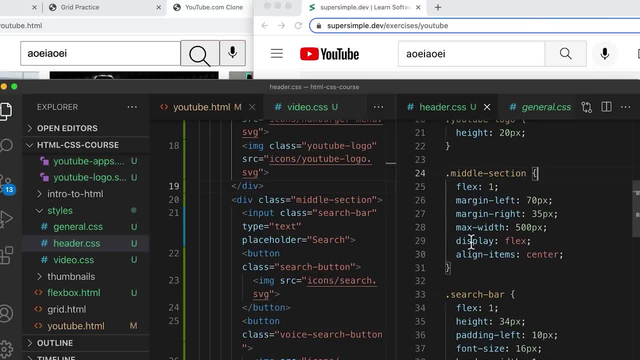 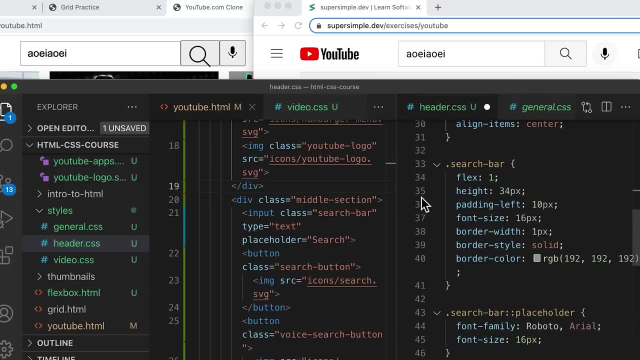 light pink background, because we don't need it anymore And that looks a little too dark, so I'm going to pick something lighter, Maybe something like this: Save, And I think that's close enough to that. Next, let's adjust the height again, because when we 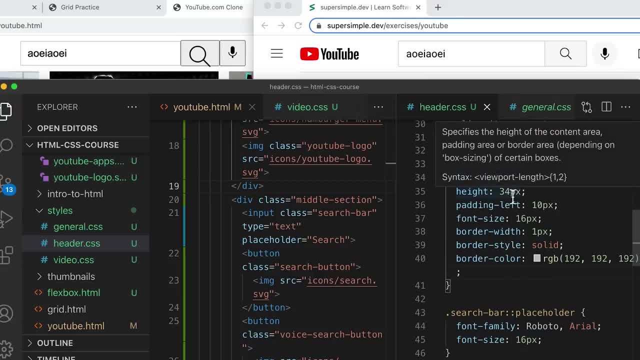 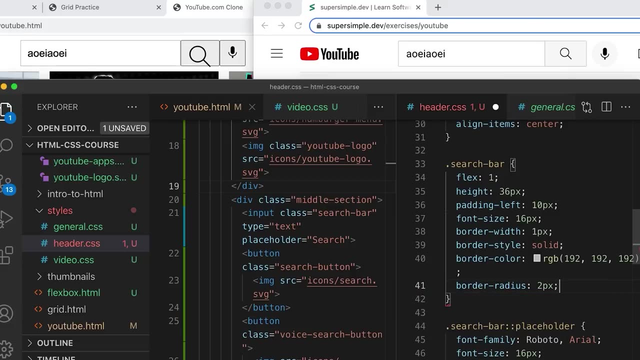 set the border. it actually made it a little bit smaller. So we'll set the height to 36.. And now it aligns with the buttons And I'm also going to create rounded corners So that property is border. dash radius: Set it to 2 pixels. 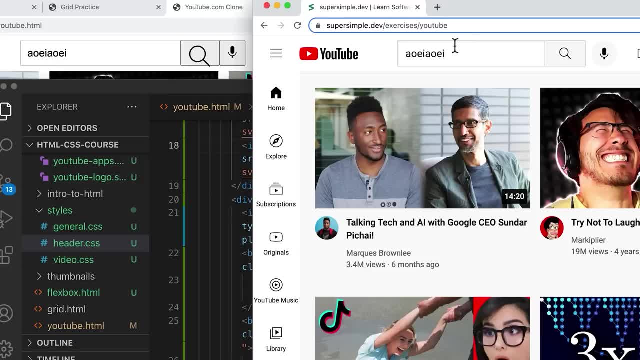 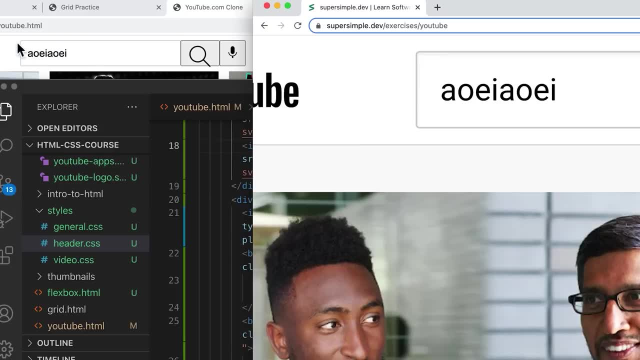 Now the last style we're going to adjust for this is the shadow. So if we zoom in to this search box, there's actually a little bit of shadow in the inside, While our search box does not have that. So we'll go back into our code. 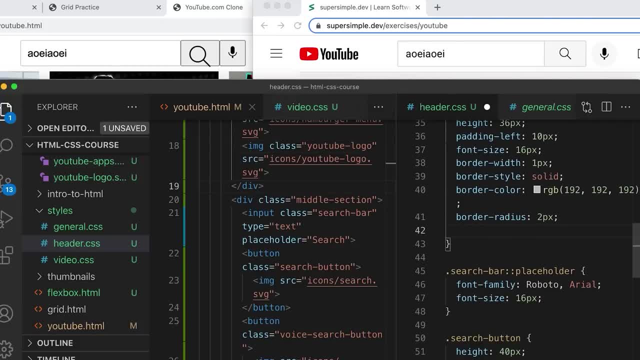 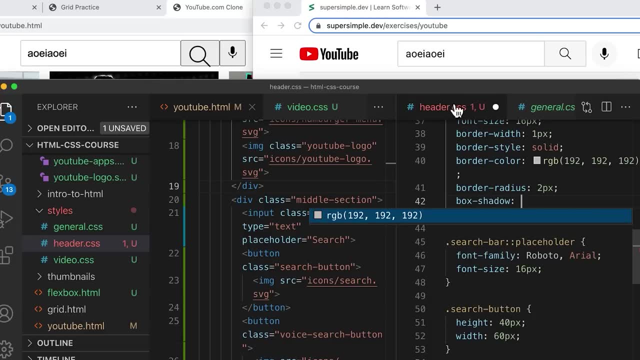 And we're going to add a shadow. We're going to use this from one of the very early lessons- Box dash shadow- And if we want a shadow on the inside of the element instead of the outside, we just need to set inset at the beginning. So this will put this: 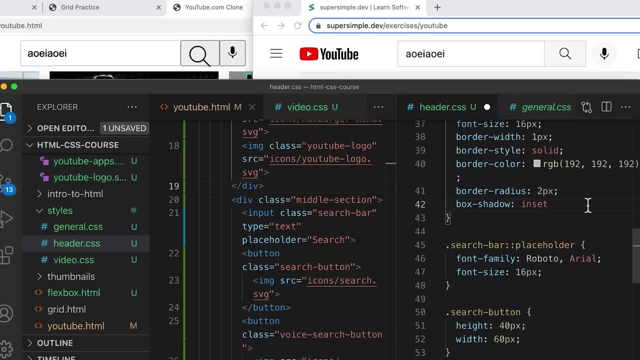 box shadow in the inside. Now we have our usual values, which is the horizontal position, So let's set it to 1 pixels, So it's going to be moved 1 pixels to the right, And the vertical position- let's set it to 2. 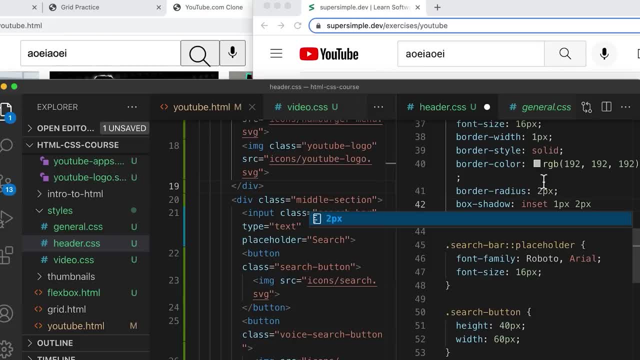 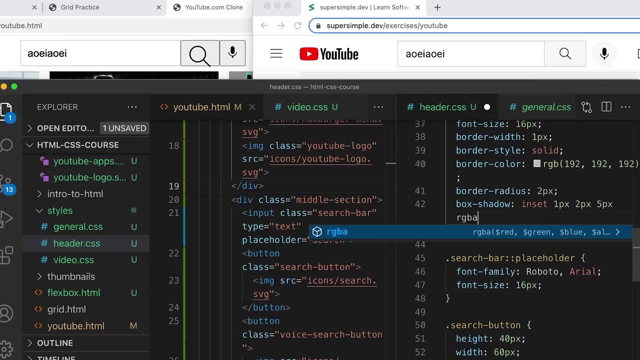 pixels. The shadow will be moved 2 pixels to the bottom. Let's set a blur of maybe 5 pixels And we'll set the shadow color to RGBA 000,, which is black, And then transparency set to only 0.15. 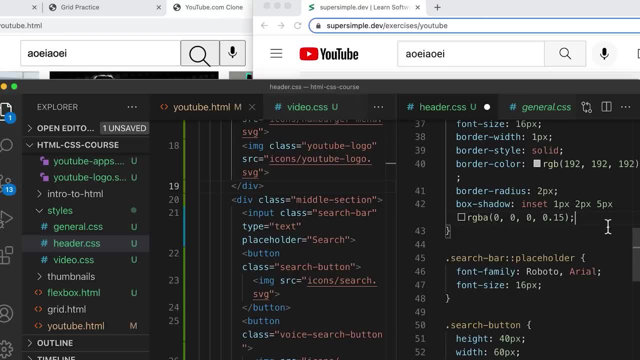 To get a very transparent black. So let's save this. That's way too much. Let's actually reduce the blur to 3 pixels maybe, And then change this to 0.05.. So we're doing a lot of trial and error. 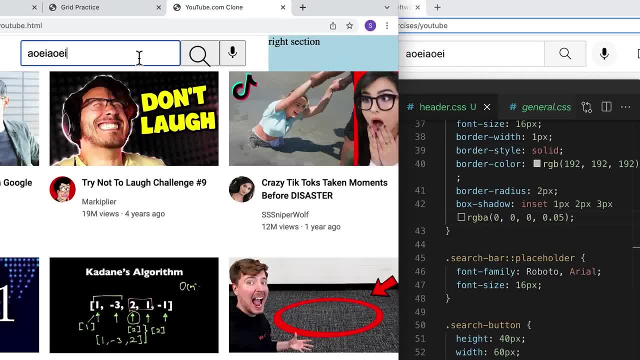 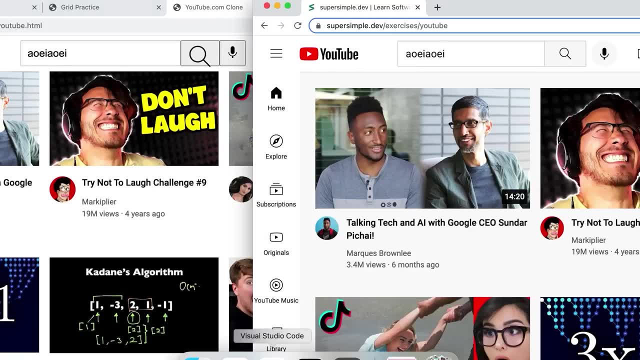 with CSS, which is normal. Okay. so I think this looks pretty close to our design. I think it looks close enough For now. we're going to move on and style the buttons. So first let's resize this icon inside the button. 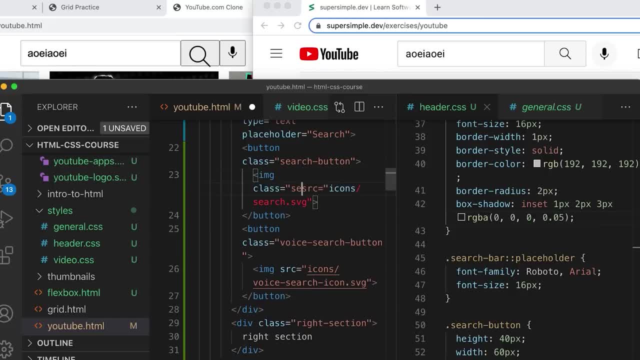 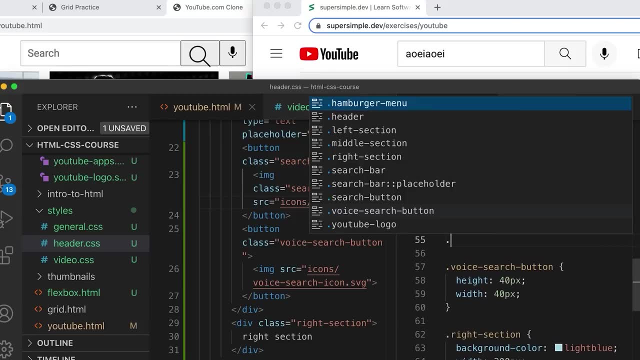 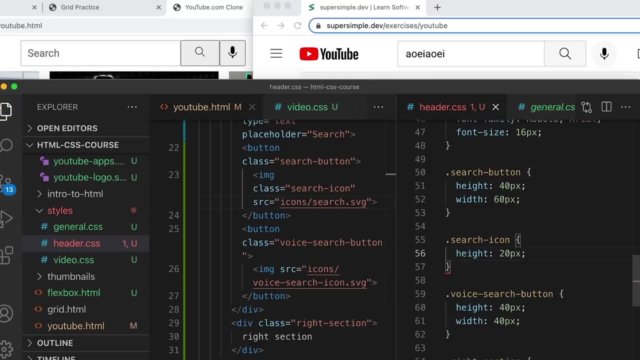 So let's give this a class of search dash icon, Save it And then in here in the search icon. we're going to make it a little smaller, So let's set the height to 20 pixels. See how that looks. 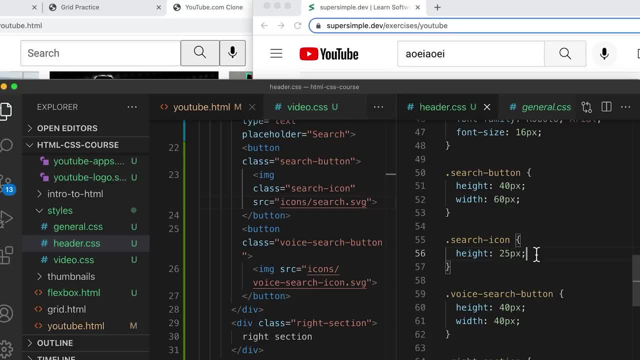 Okay, so that looks too small. I'm going to try 25 pixels. Alright, so that size looks pretty similar. Now you'll notice that this one is vertically aligned, while ours is not, So we can either turn the search button into a flexbox or 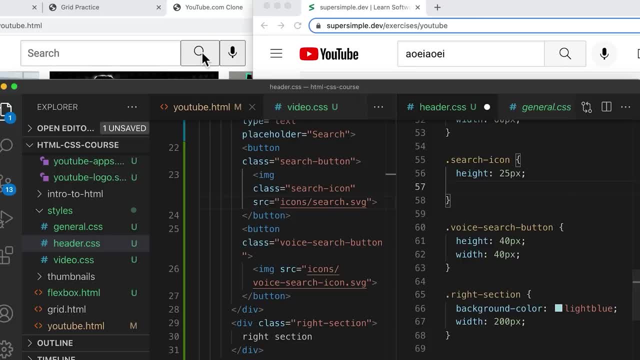 we can just do a simpler solution. We're going to add some spacing to the top of this icon to push it down. So margin dash top of maybe 4 pixels to push that down just a little bit. Okay, so I think that looks close. 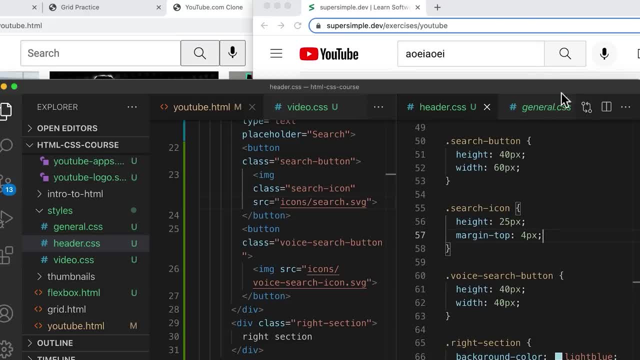 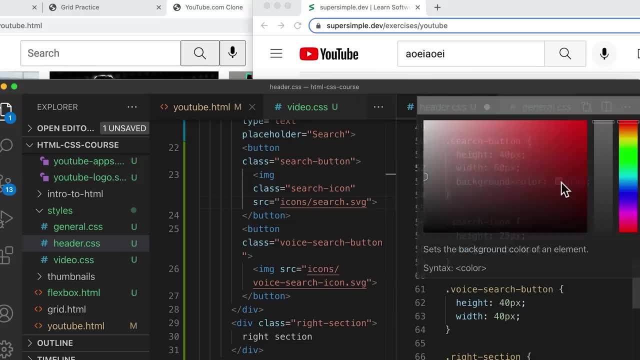 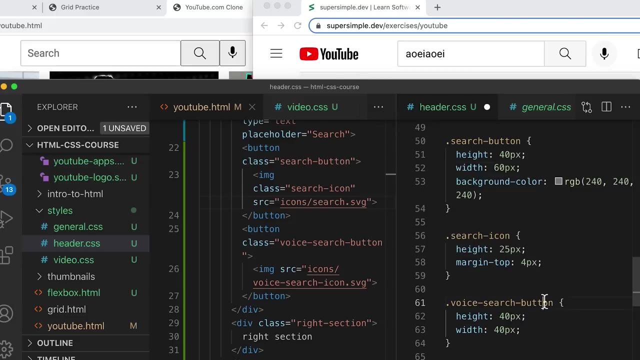 enough. Let's finish off this button. We're going to set a background color of gray and then I'm going to adjust it to match that. So I'm going to pick something like this: maybe 240.. And then save it. 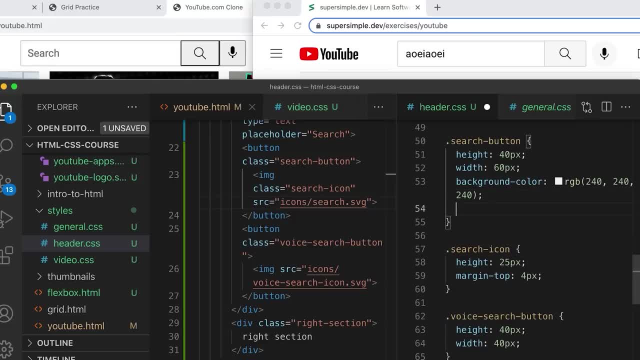 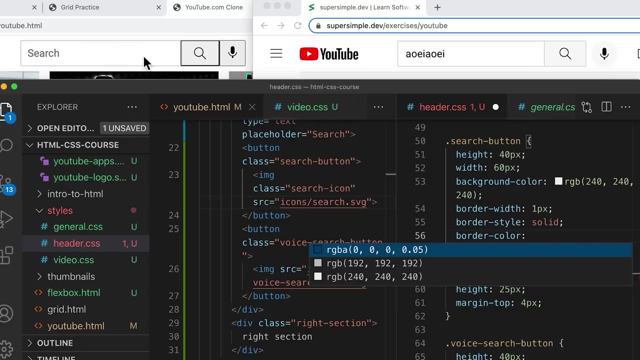 That looks pretty good. but now our borders are messed up, So we're going to set the border border width of 1 pixel. Border dash style of solid color And border color is going to be the same as our textbox So we can go up here. 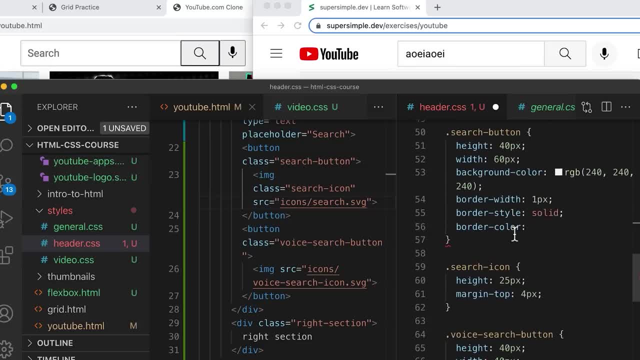 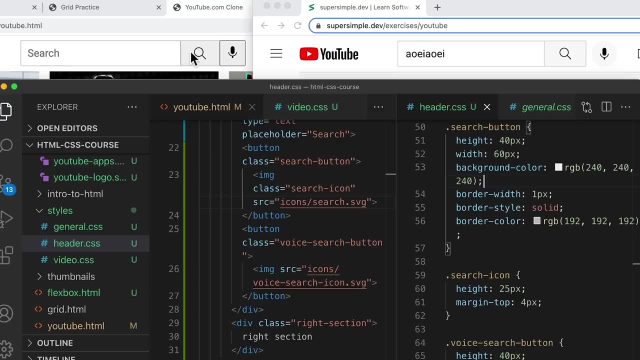 and just copy that And right there, Save it, and there we go. That looks pretty close right now. So now we want to move this button into this input element a little bit like you see here, So that we only have one edge. 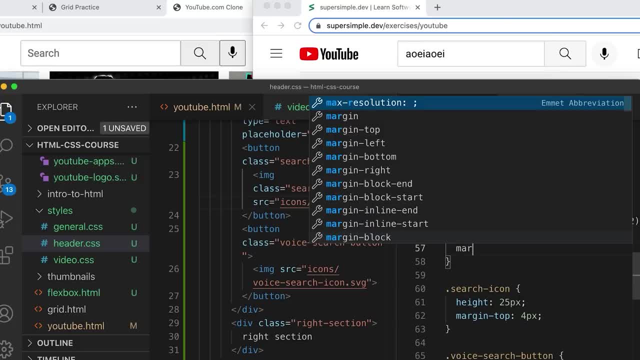 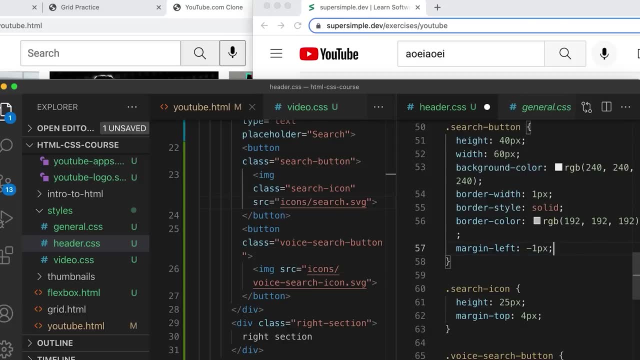 To do that, here's a little trick. We can set some spacing on the left, so margin left. Except this time we're going to add negative spacing. So we're going to add negative 1 spacing. Normal margin adds space and it pushes the element. 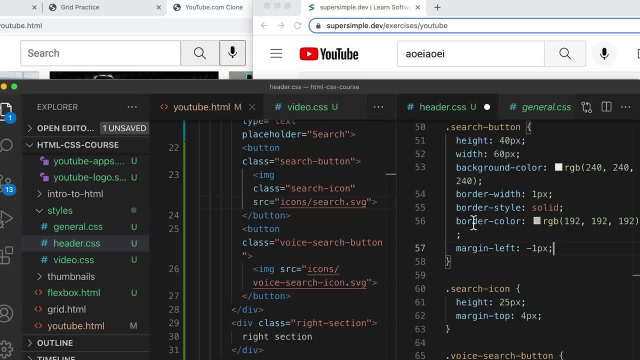 Negative margin subtracts space and pulls the element to that side. So margin left of a negative number will pull it to the left. So let's pull it to the left by 1 pixel, Save it, And that looks really good. Now we're going to make our button a little bit longer. 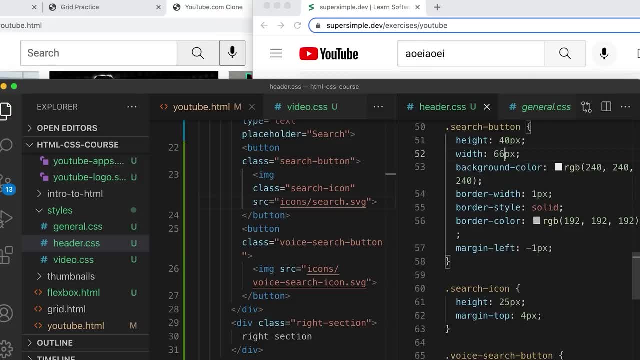 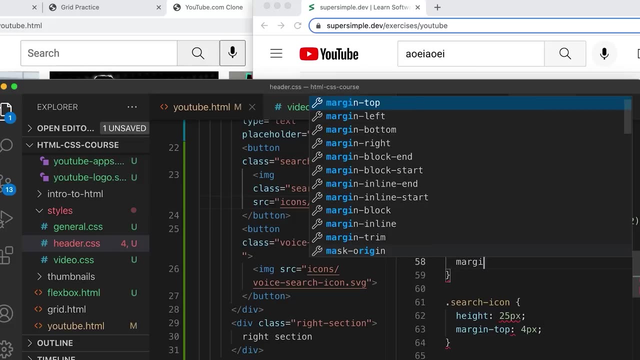 Let's change it to 66.. Finally, we're going to style this voice search icon First. we notice that there's a little bit of space between these two, So let's set a margin on the right side of the button. So this time it's normal margin. 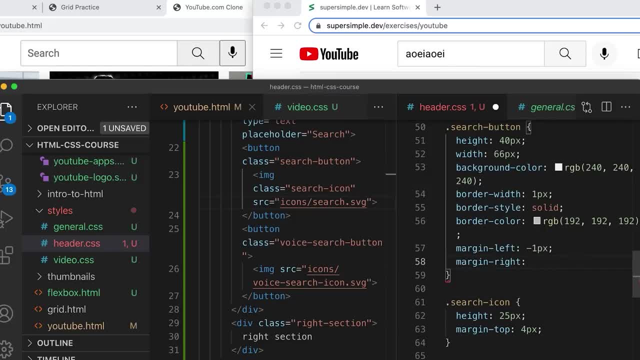 Margin right of maybe 8 pixels. I think that looks pretty close. I'm actually going to set it to 10.. Okay, and then for this button. I'm first going to make it round, So let's go into the styles of this button. 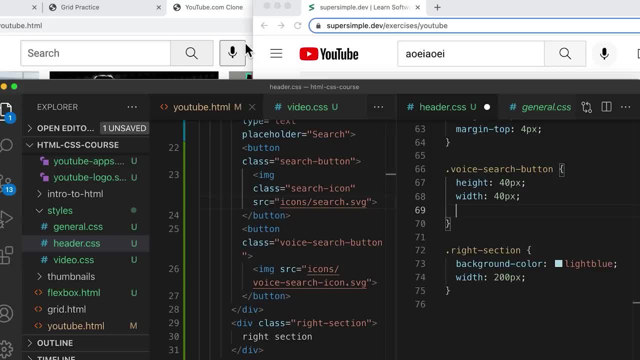 And to make it round, we just have to make the corners as round as possible. Let's set the border radius, and I'm going to set it to 20 pixels. So the trick here is that if you set this to half the width or the height, 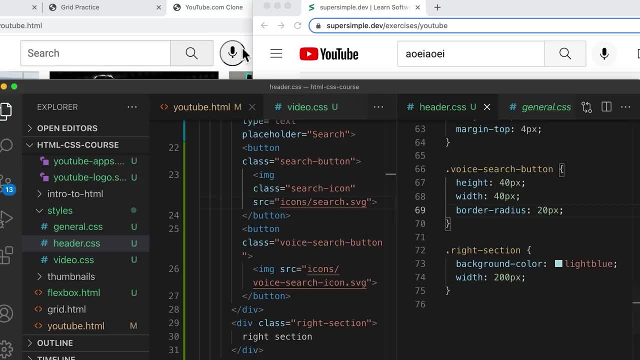 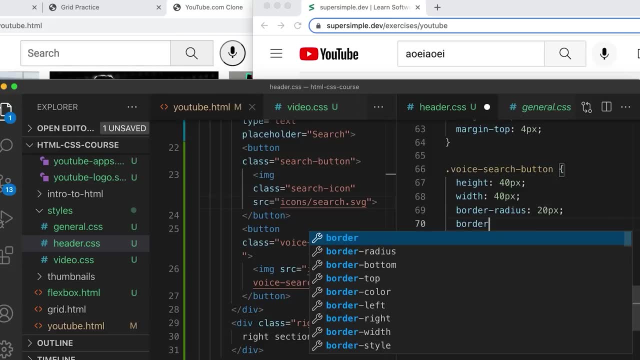 it will make it round. So let's save this. And now we have a round button, but we have a weird border. Let's actually get rid of it because it's not in our design. So border and none To get rid of the border. 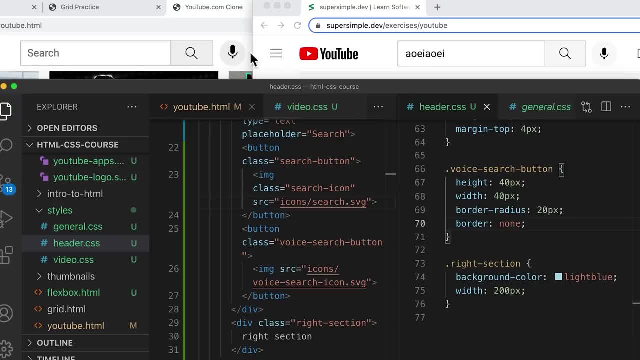 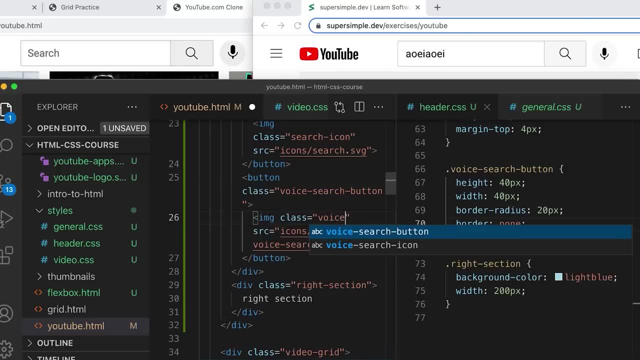 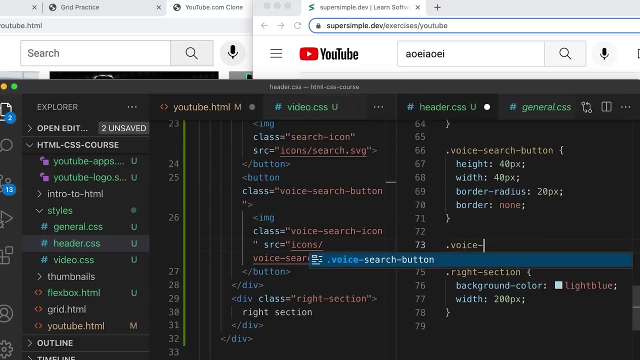 So it's looking really close. Our icon is a little bit bigger than this one, So we're going to target it in here. Class equals voice-search-icon And then in our CSS we'll target that, So voice-search-icon. So for this let's set a. 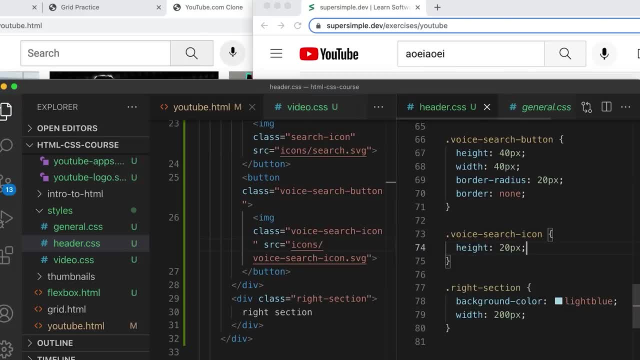 height of maybe 20 pixels. See how that looks. It's a little bit small. Let's increase it to 24.. I think that looks pretty good, And next we're going to try to vertically align it. We're going to add a little bit of margin on the. 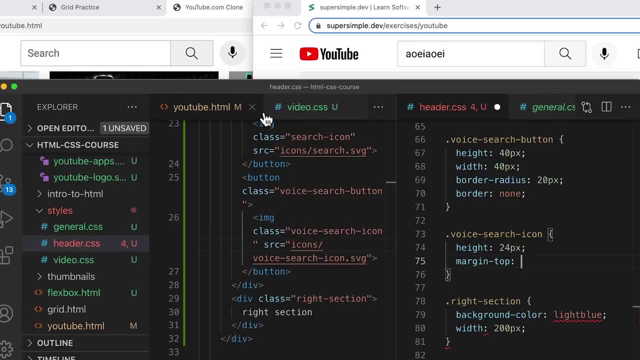 top to push it down. So margin-top and 4 pixels. Okay, That looks pretty good. The last thing is to change the background color. So we're going to change the background color to, let's say, gray, and then I'll pick another color. 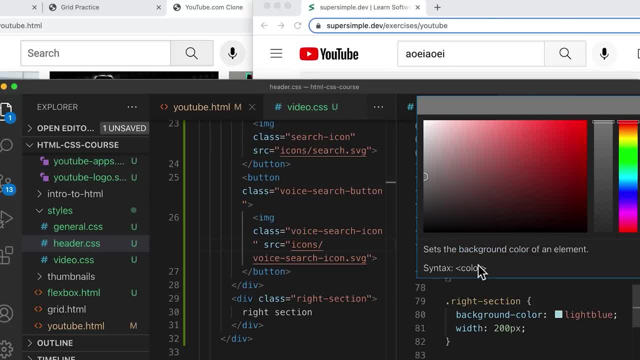 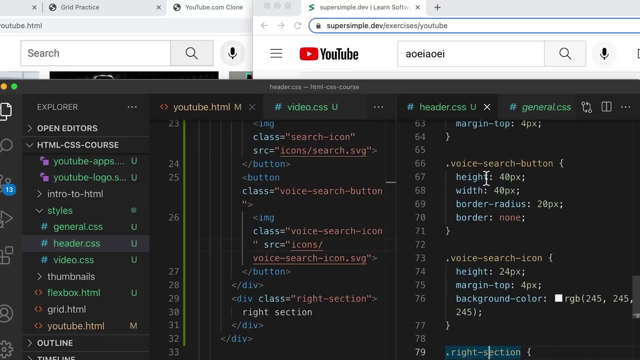 So this time let's pick maybe 245.. And then save. Oh, So I accidentally put it on the icon. We actually want to put this on the entire button, So I'm going to cut and paste this onto the button styles. Let's save. 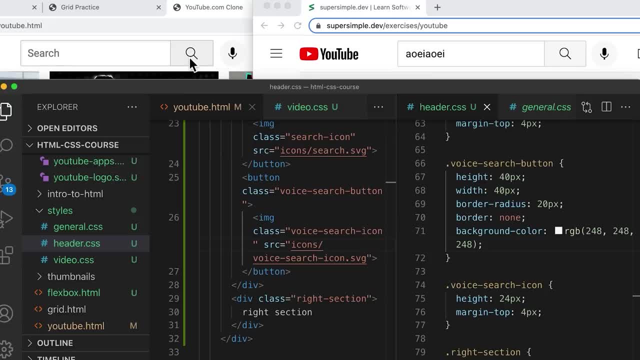 And I think that looks pretty close. So this color is a little bit off from this, but I think it's okay if we look at the bigger picture. So now we've completed the middle section And you can compare it here To here. 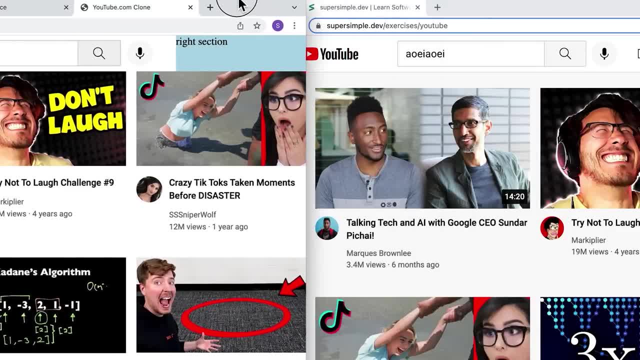 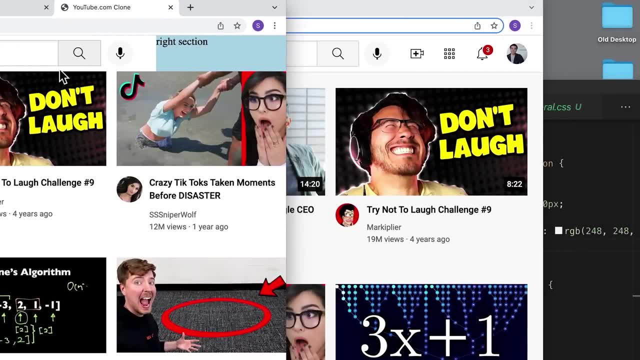 So we're looking really good so far. Next we're going to finish the right section, So I'm going to put them side by side again So it's easier for us to copy. So the right section has three icons and an image. 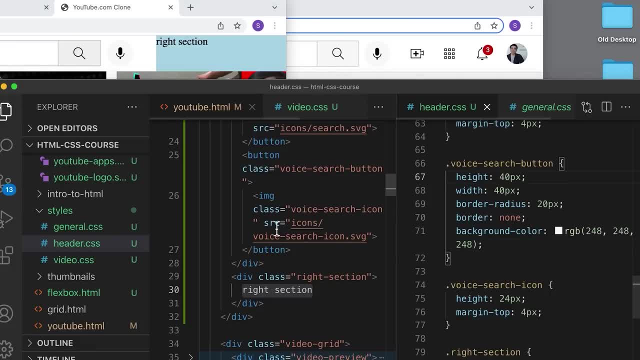 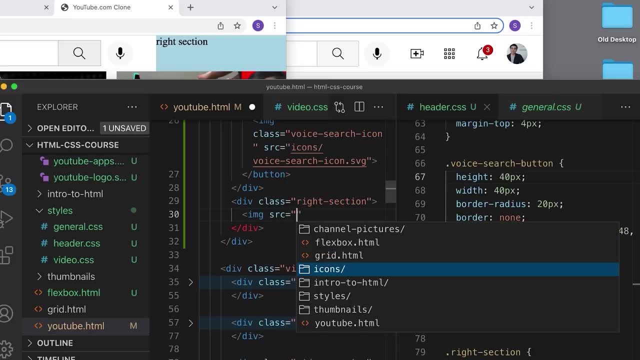 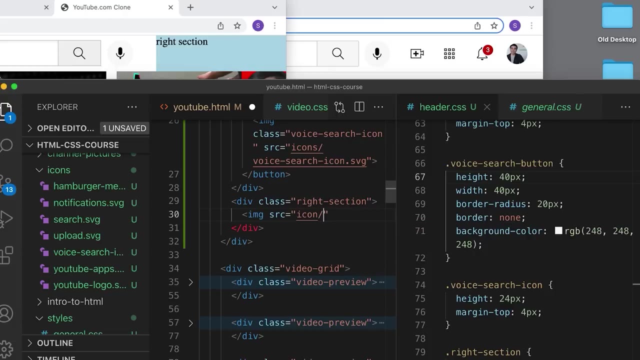 So we're going to add them to our HTML first. So let's go into the right section here And we're going to create an image And we're going to load this, which is the upload icon. So icons slash- upload dot svg. 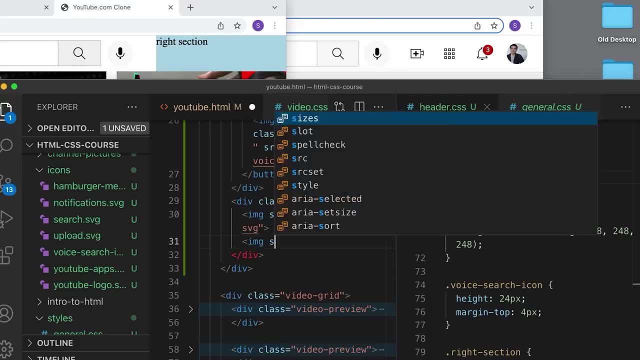 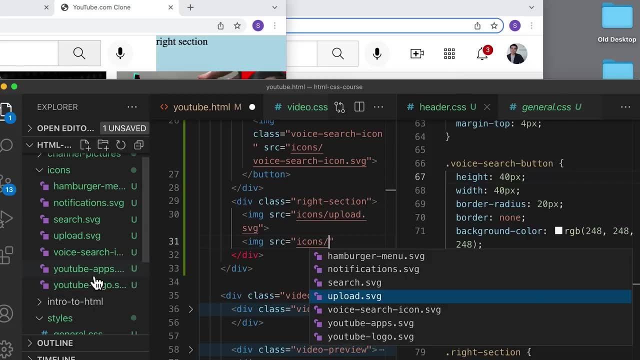 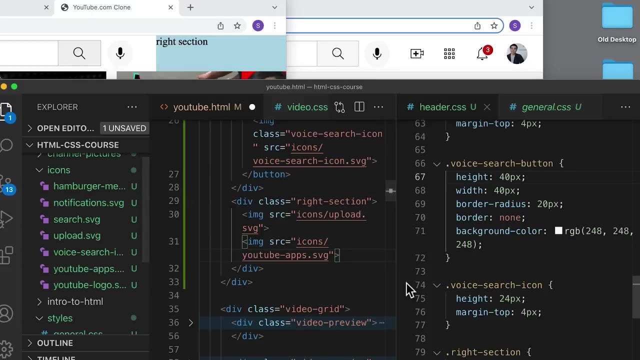 And then we'll add another one, So image, And this one is going to be icons slash. this one is called YouTube apps, dot, svg. And then the last one is the notification icon which is here, So image element, And we're going to load icons slash. 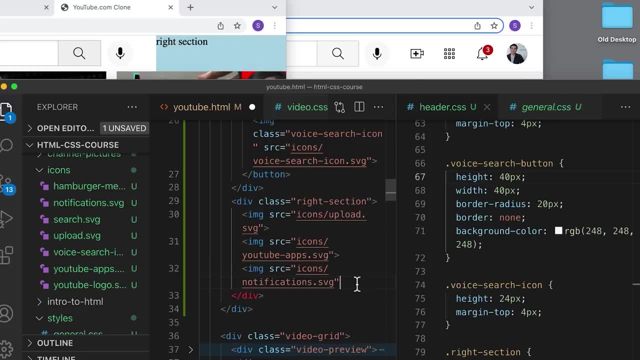 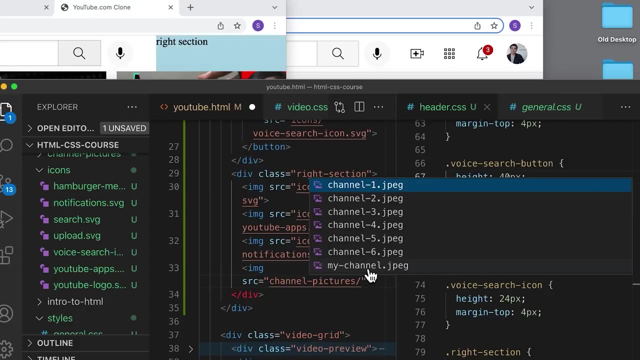 notifications- dot svg. And finally, we're going to create another image And we're going to load this channel profile picture. So source: And this one is located in a different folder, It's in the channel pictures folder And it's called my. 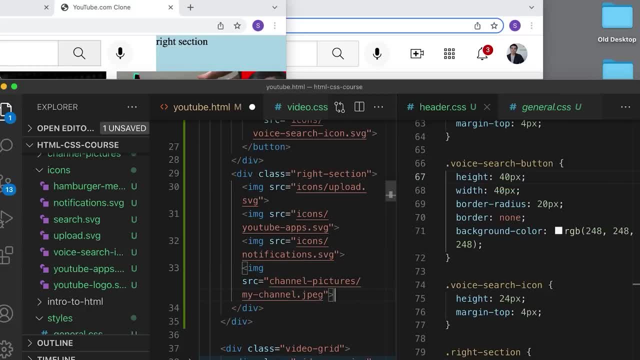 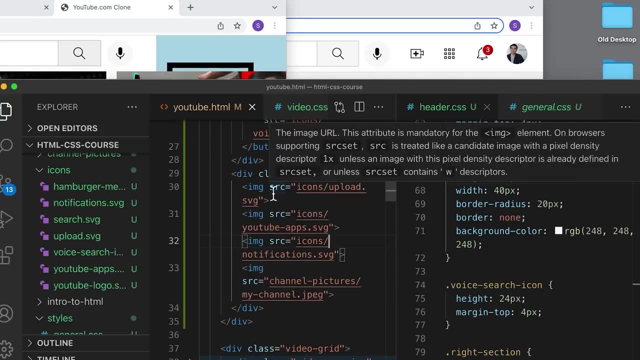 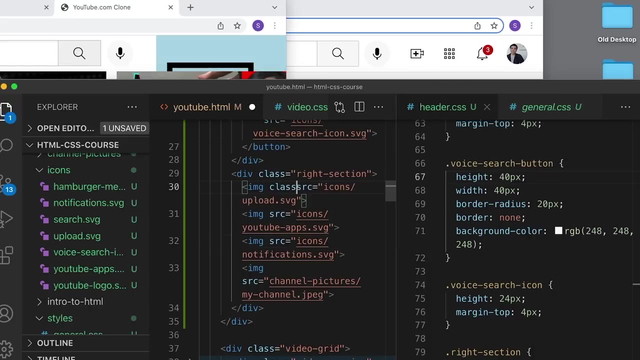 channel dot jpeg, So let's save it. Refresh And again, our svgs are massive, So let's go ahead and resize them in our CSS. So first let's add classes to all of these images, So we're going to set this one to upload. 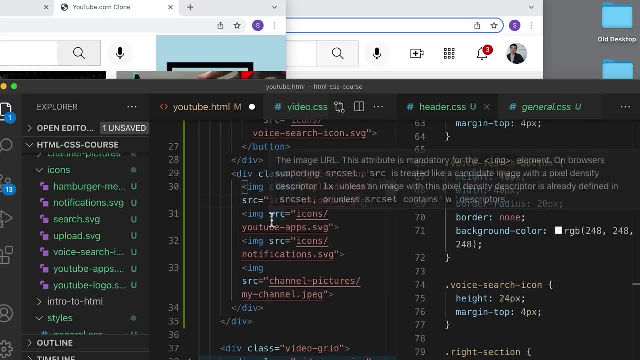 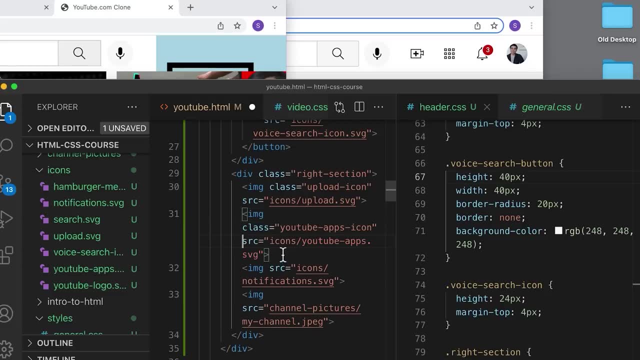 dash icon, So upload dash icon. The next one is going to be YouTube apps icon. Class equals YouTube dash apps dash icon. Next one: we'll do notifications dash icon, So class equals notifications dash icon. And lastly, we're going to name this a little. 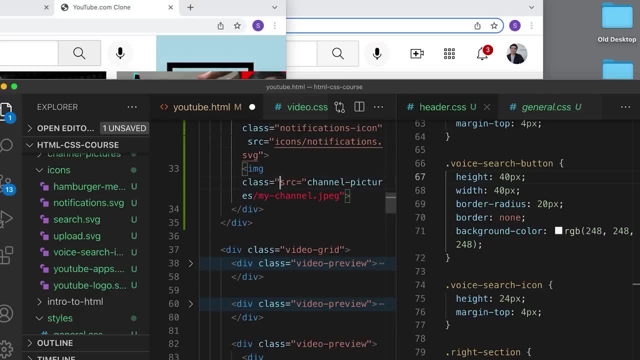 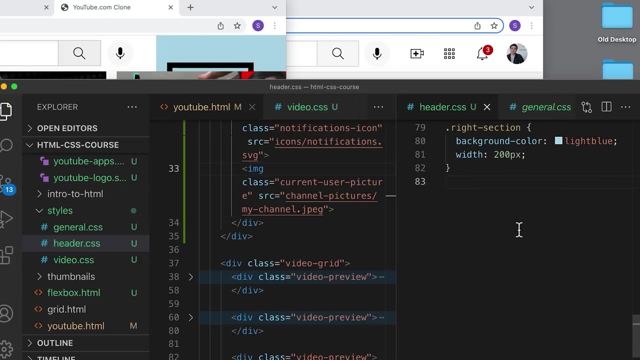 bit different. Let's give it a class And let's call this one: current dash user dash picture. So it's a little more clear that this is different And we can target it with CSS. So let's go down into this right section here. 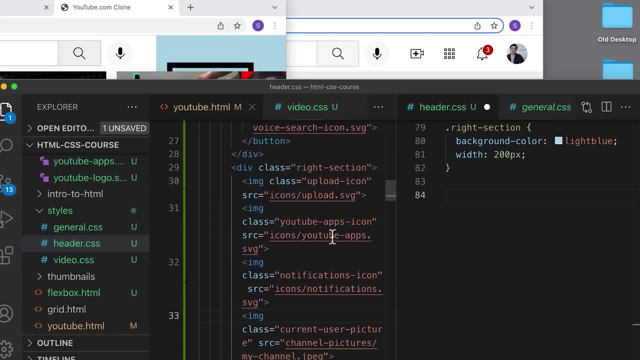 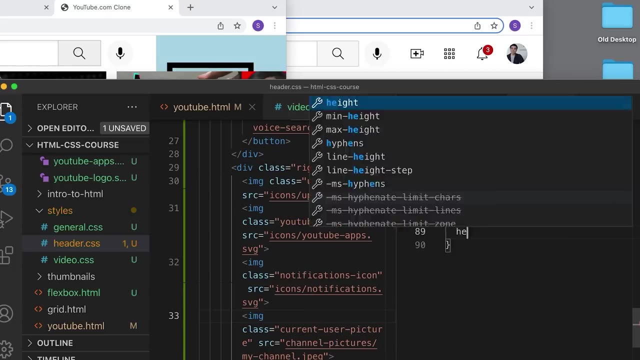 And we'll scroll up and we'll first resize the icons. Let's resize the upload icon. Let's set a height of 24 pixels, And then we'll do the YouTube dash apps icon. Let's set a height of 24 pixels. 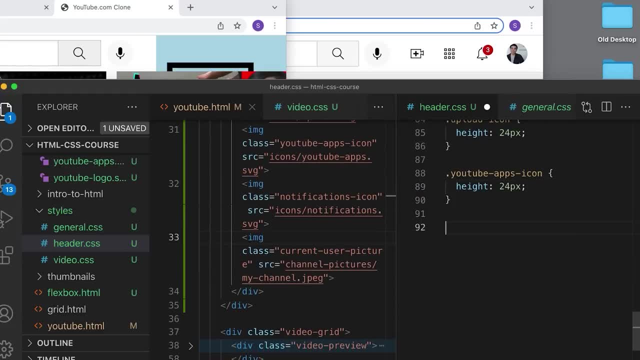 And then the notifications icon, which is right here. Icon, Let's set a height of this 24 pixels again. And the current user picture. So notice it's a little bit taller. Let's target that Current dash user dash picture. 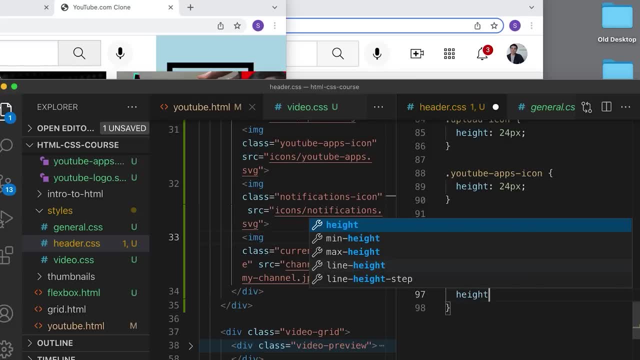 And we're going to set a height of 32 pixels To make it a little bit taller. So let's save it. And now we have the icons we're going to use. Again, we want to align these vertically in the center, Remember. 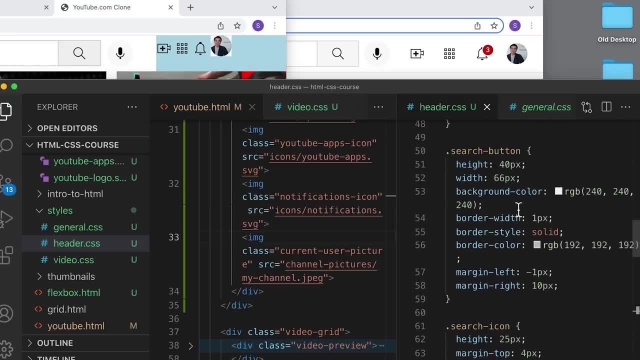 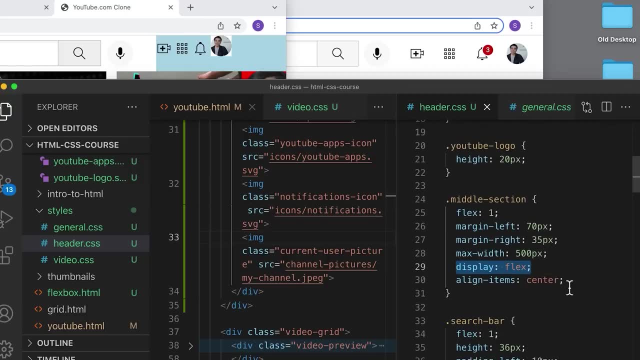 to do that, we're going to scroll up to our middle section, which is all the way up here. We first have to turn this container into a flexbox And then we can use align item center. So inside our HTML we have to turn this: 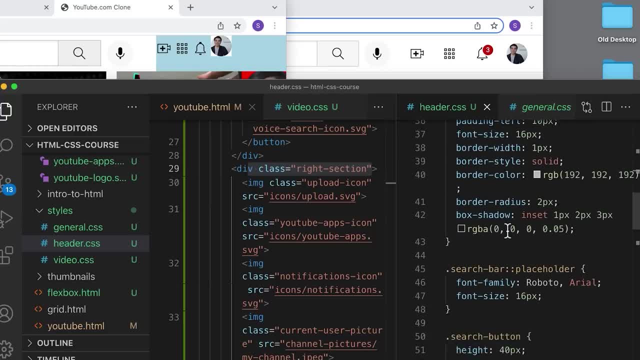 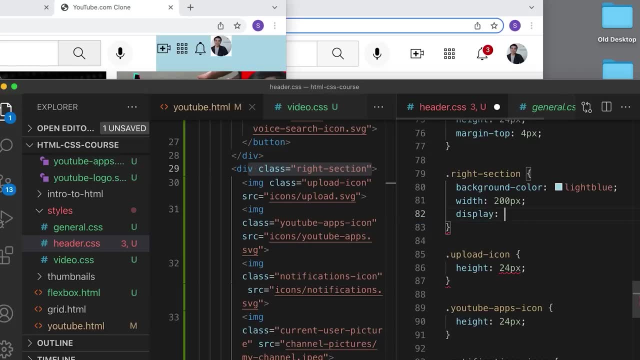 into a flexbox. Let's scroll down To the right section styles. here We're going to turn this display, colon flex, And then we're going to set align dash items, colon center, To align them vertically. Let's save it, Okay. next we want to distribute. 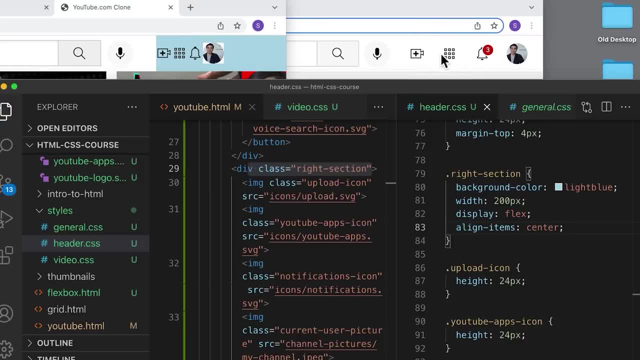 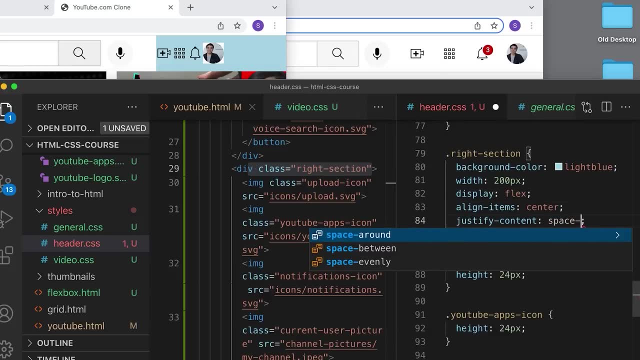 them evenly across the horizontal space, And remember from our practice code that one's called justify dash, content, space dash between Let's save it. And now these icons are spaced evenly across the space, So it looks like they're a little bit too far. 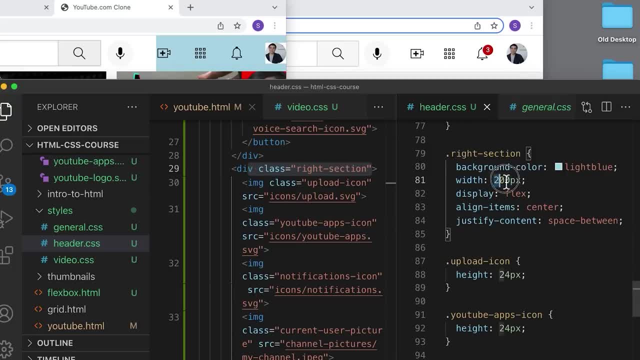 apart from each other. We can adjust that by adjusting the width. So let's decrease the width to bring everything closer together to match our design, And I actually think this, like all the icons, look good enough. The only last thing we're going to change is this picture. 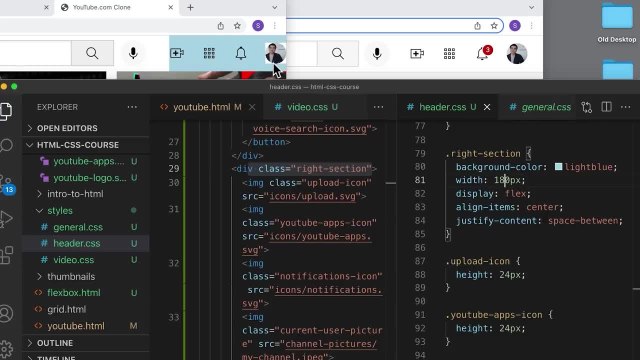 here. So notice, it's still a square. We want to make it a circle. As a review, we're going to use border radius to make it a circle, So let's set it to border dash radius And the trick we learned is half. 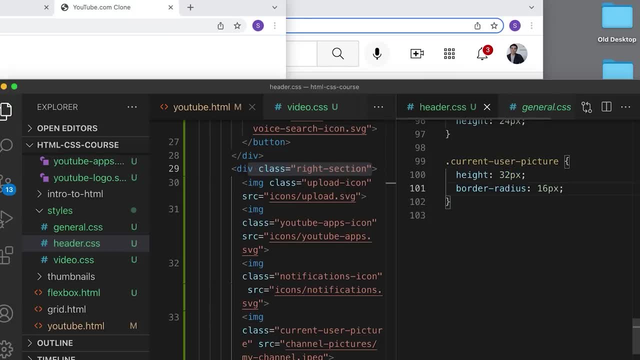 of this will make it round, So 16 pixels, Save it And now we have a round channel profile picture. Lastly, we're pretty much done with this, so we can get rid of the blue background color. So we'll scroll up. 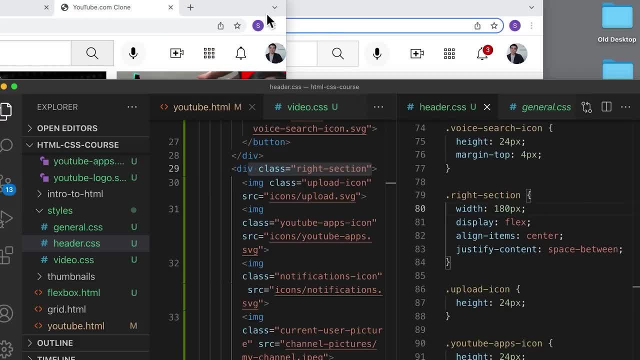 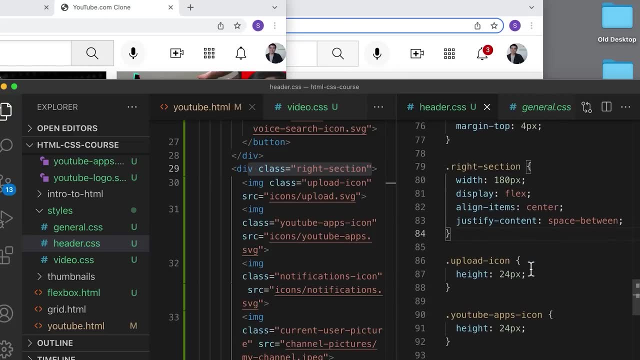 And get rid of this. Now. I actually noticed that we have spacing to the right here in our design, So that's one thing I missed. So let's add that right now. So we're going to add margin right to this section of maybe 24 pixels. 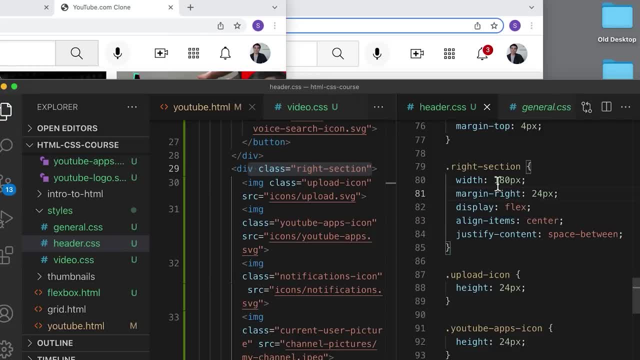 Save it, And I think that's a little too much. I can't really tell. Let's set it to 20, just to be safe. Okay, so I'm happy with how this looks. Alright, so that's basically the content in our header. 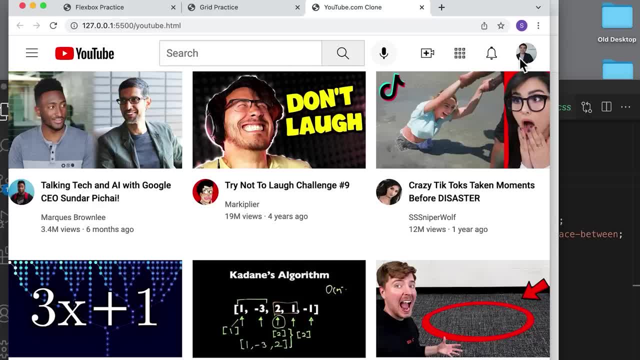 If we look at it right now, it looks really professional. So I know that while we were working on it it looked a little bit weird, It looked unfinished, But you just got to trust the process And at the end we have a really professional result. 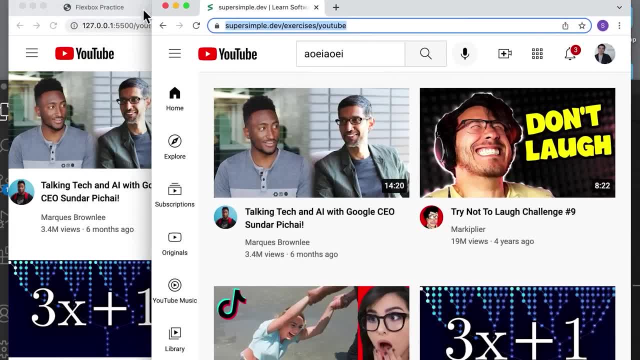 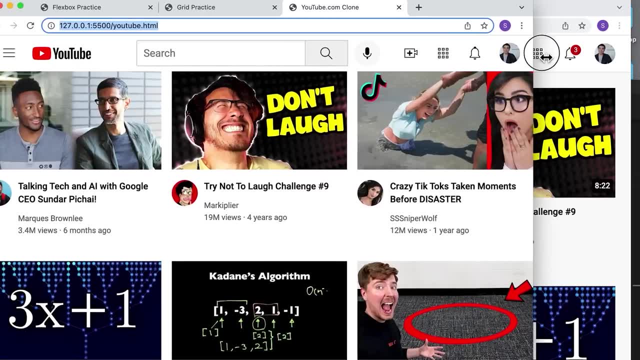 that looks like our design. Now there's going to be one last case I'm going to show you, And this is a weird behavior of Flexbox. So if I resize my browser and I make it smaller, notice that these icons start to get. 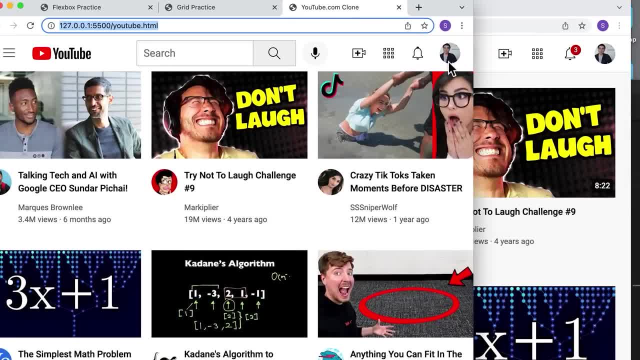 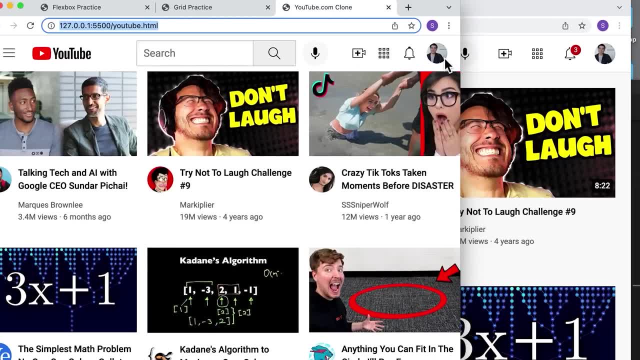 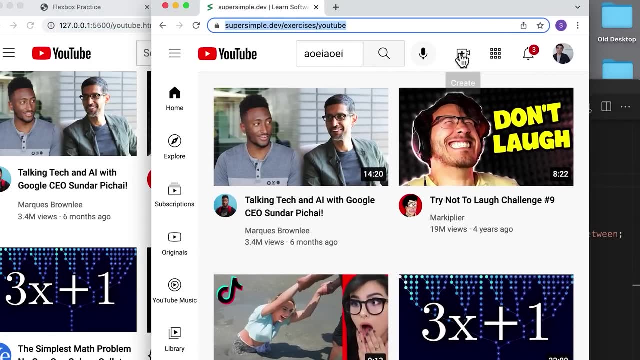 closer to each other. So this happens because Flexbox is flexible. When we start not having enough space, it'll start shrinking the items inside. But if we look at our final project and we shrink the browser, notice that this doesn't shrink And we sort of forced only. 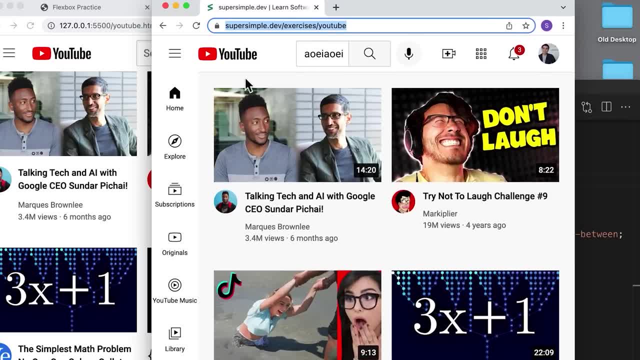 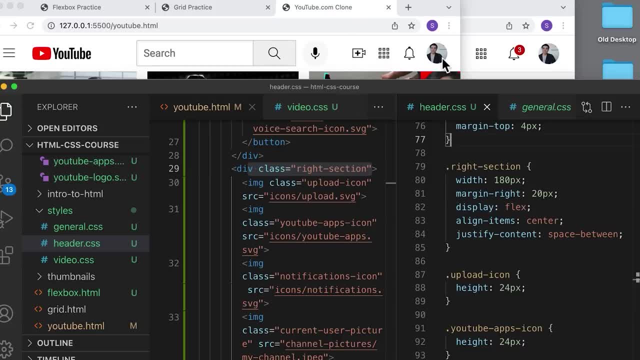 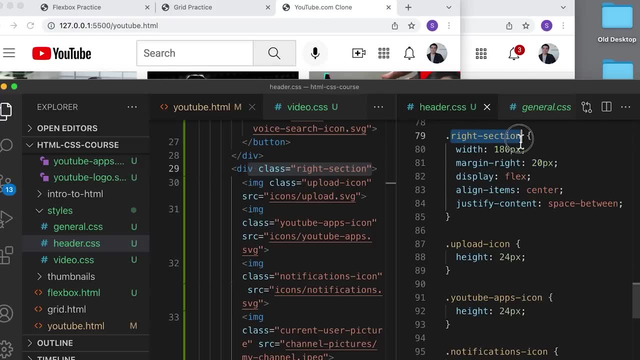 the search bar to shrink. So let's go back into our project and into our code. And Flexbox has a special property to prevent certain items from shrinking. So we're going to scroll down to the right section here And to prevent the right section from shrinking. 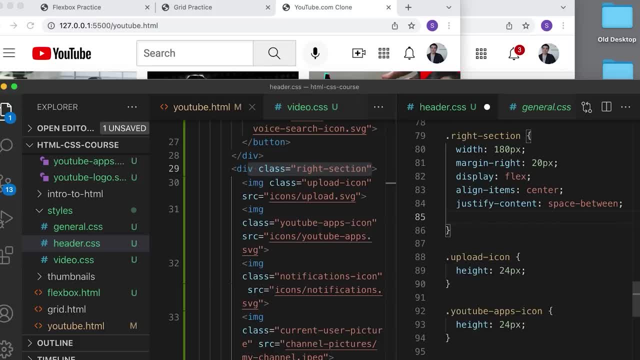 we're just going to set this property flex, dash, shrink, colon zero. So this means that no matter what happens, we're going to keep this width and we're not going to shrink. So zero means don't shrink If we save it. 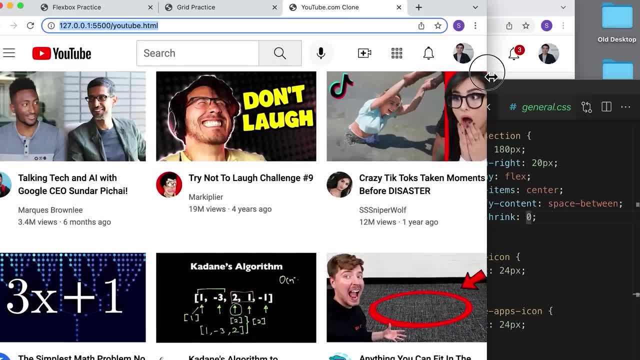 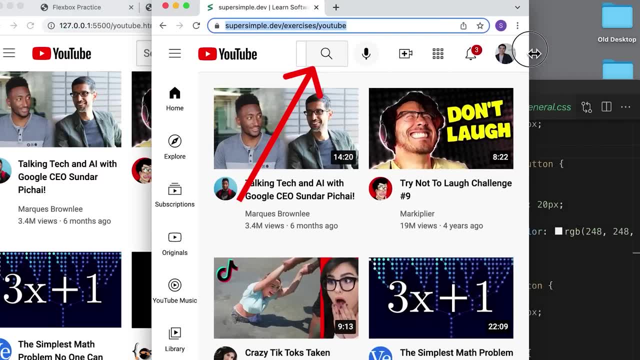 now you're going to see that it doesn't shrink. But now when we resize it, notice that the search bar doesn't actually shrink all the way like our design. So the way to achieve this is to go into our HTML, and then we're going to. 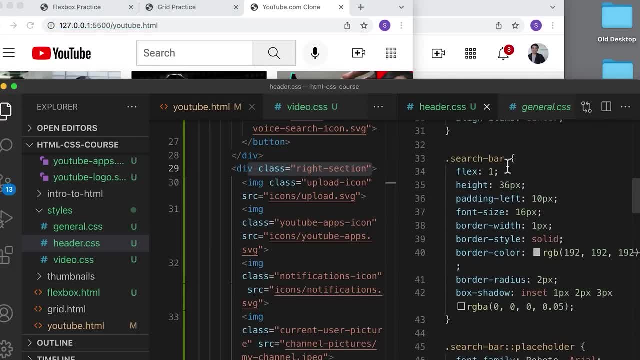 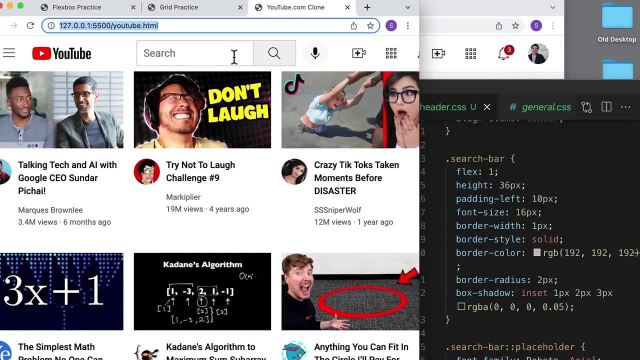 go into our search bar, which is right here. So normally search bars have a default width And we can't really see that because we set flex to one. So it's sort of growing with the page, but as soon as it hits that default width it's not going to go down. 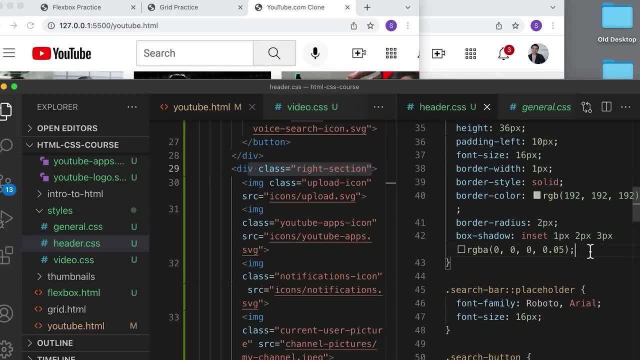 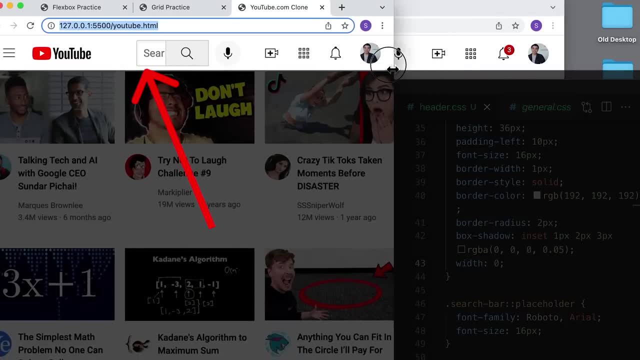 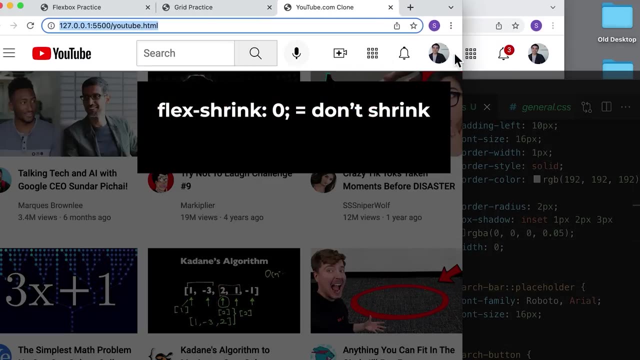 anymore. So to remove that default width, we can just set width to zero. We save it and now you can see that the search box will start shrinking as much as possible. So to recap, we set flex shrink of zero to this right. 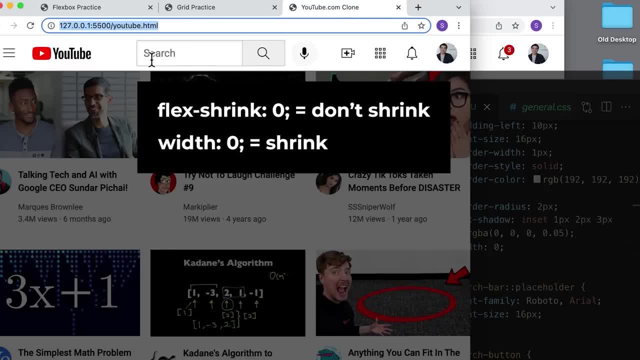 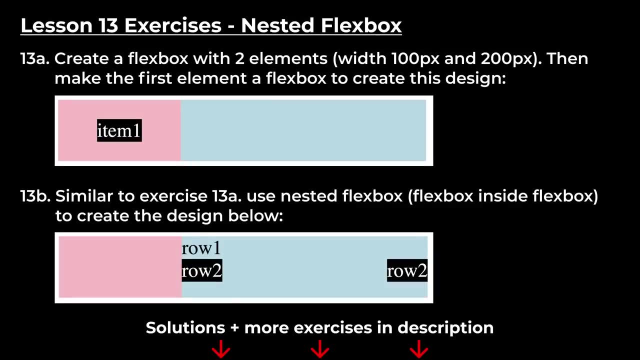 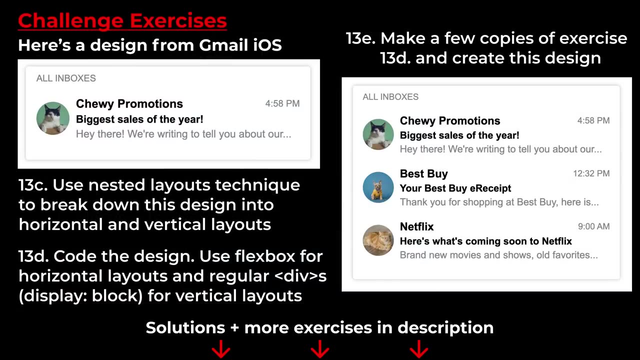 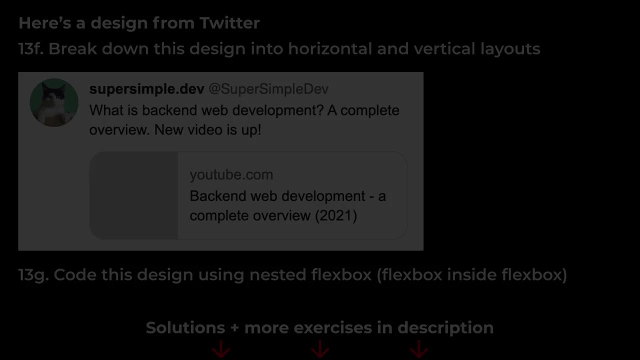 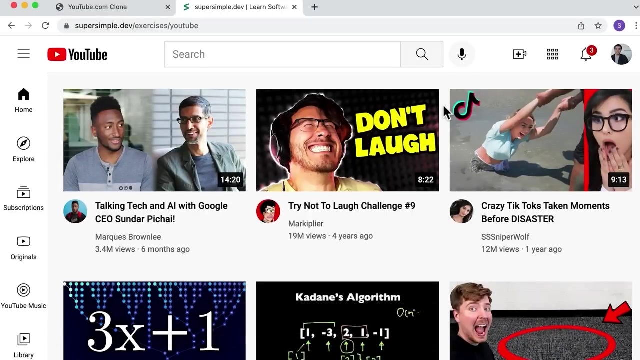 section so it doesn't shrink. And then we set a width of zero to the search bar so that it does shrink. Here are some exercises to get yourself familiar with using Flexbox to create flexible layouts. Now we're going to learn the last major skill that we need to finish off. 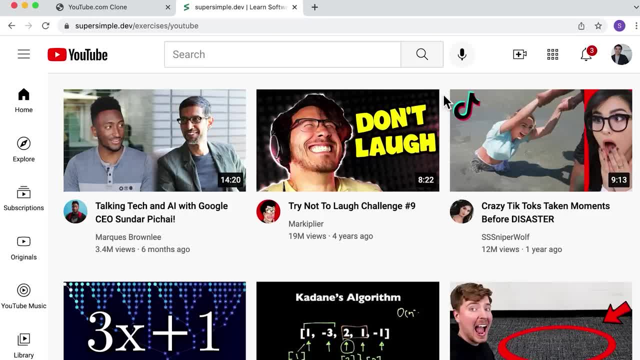 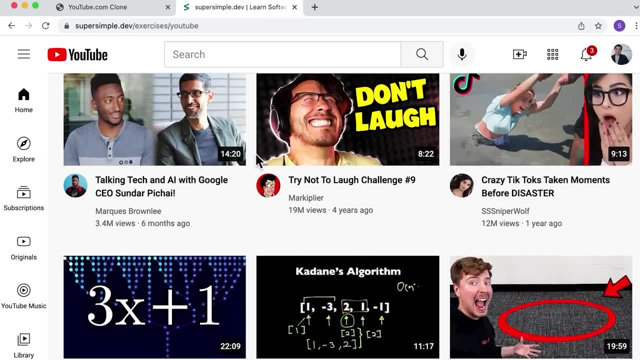 our project We're going to learn CSS position, So position helps us do things like keep the header at the top of the page while we scroll. It also helps us keep the sidebar at the top of the page And, lastly, whenever we see an element on top of. 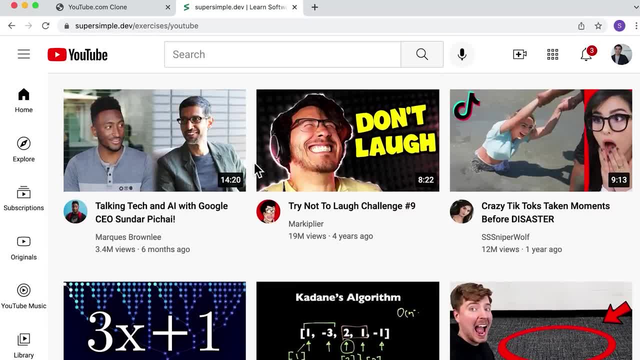 another element that's using CSS position. For example, here the video time is on top of the thumbnail, the notification number is on top of the icon and when I hover over this, we have a tool tip on top of the page. 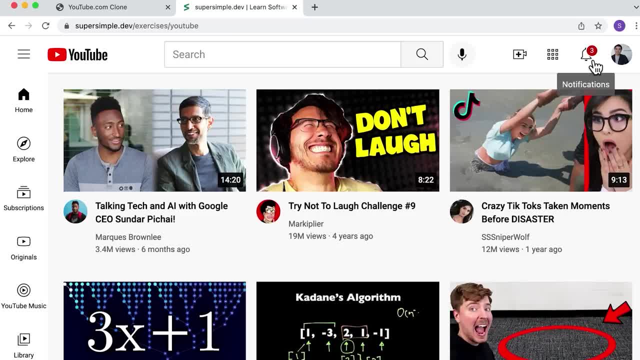 So CSS position adds another dimension to our page. So, just like the previous lessons, we're going to create a new HTML file. just to practice position, I'm going to go into my code editor and we're going to create a new file and 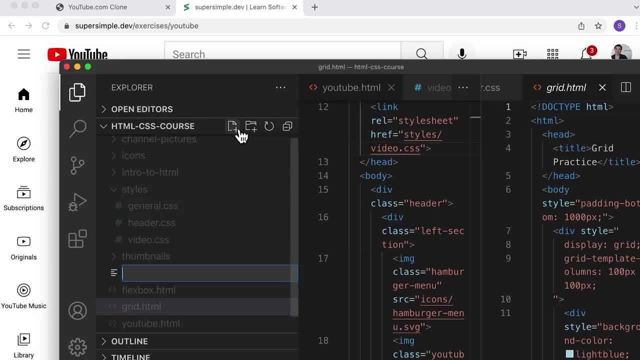 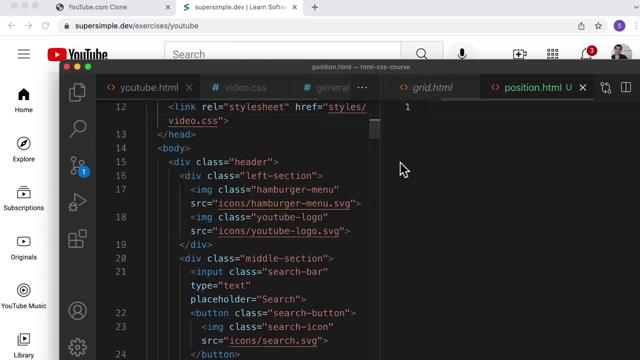 let's put it right here, beside the other ones: New file. let's call this position dot HTML. Now, as always, we're going to start with the HTML structure, So we're going to have doc type at the top and then an. 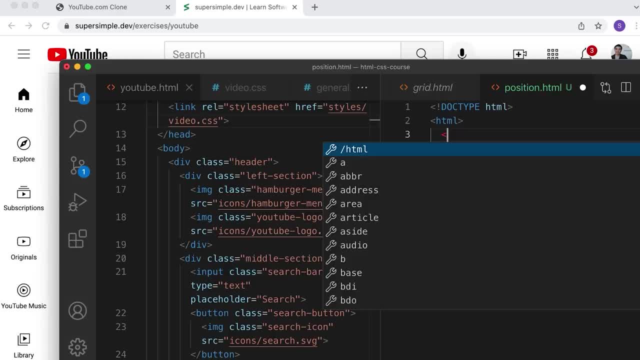 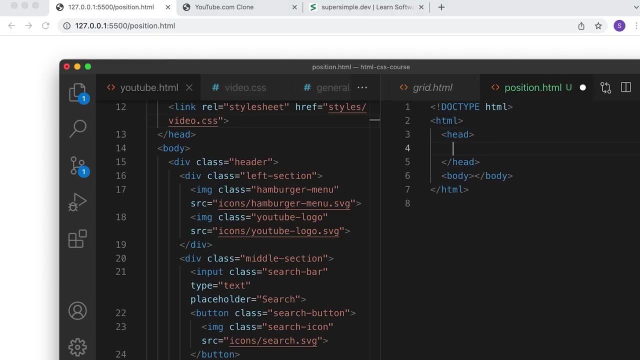 HTML element. Inside we have a head element and then we have a body element. Now we can right click and open with live server and we're ready to begin. So first let's add a title, so that we know what this. 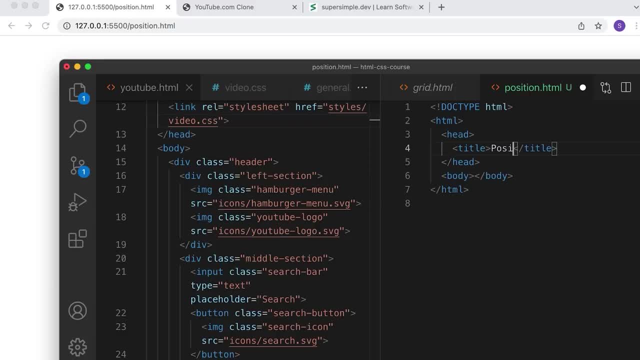 HTML file is for. Let's call this position practice, Save it and then it should show up here. We're going to start in the body again and we're going to create two divs. Let's call this div one and another div div. 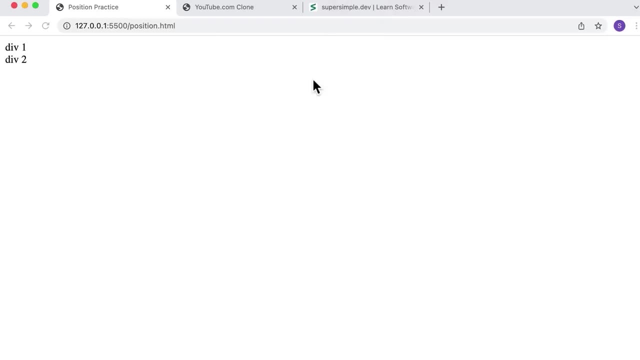 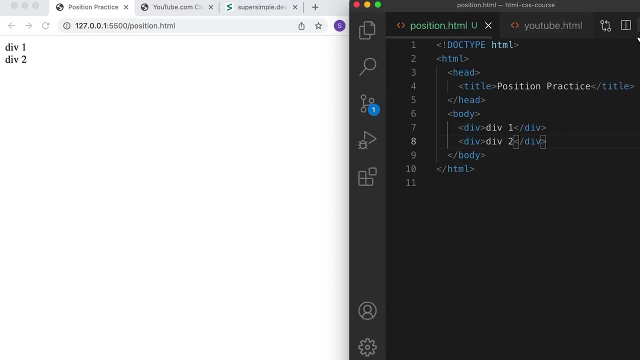 two, And I'm just going to resize this a little bit so we can see it side by side. So, just like before, we're going to use inline styles so that our CSS is close to our HTML code. I'm going to set a style. 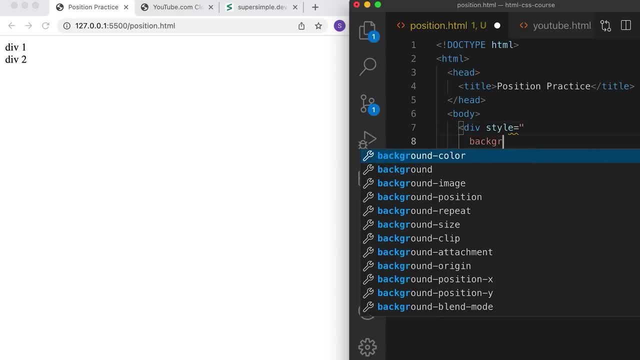 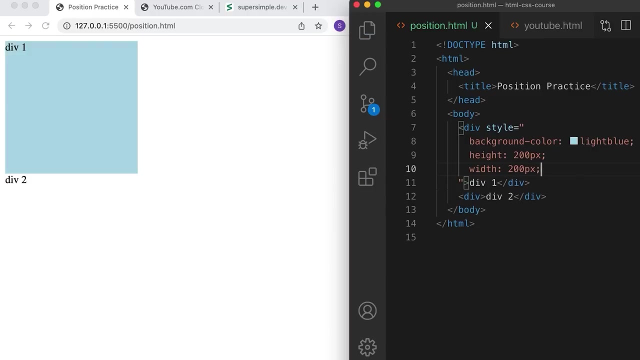 and then we're going to set this one to background dash color and light blue And we're going to set the height and the width to 200 pixels. So height, 200 pixels and width, 200 pixels. Next we're going to set the second div to be: 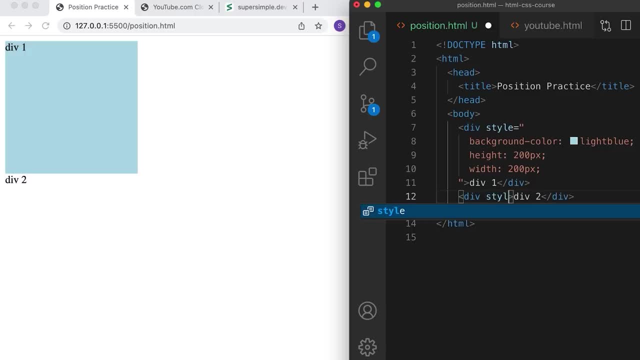 the same size, but with background color light pink. So again we set a style and then we set a background dash color of light pink, height of 200 pixels and width of 200 pixels. So CSS position is just the position property. 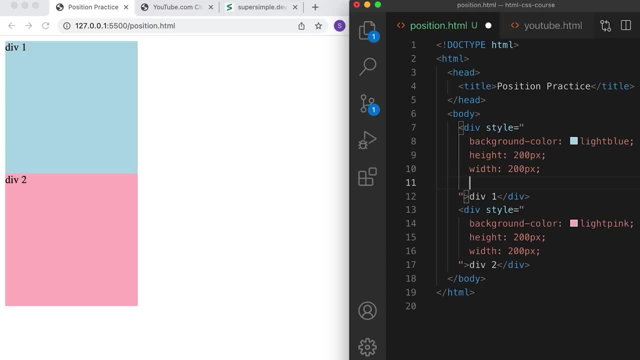 So let's go into our first div and we're going to set the position property to static And then save. So position static is the default position. It's the same thing as if you don't have this line at all. Now we're going to learn a second position. 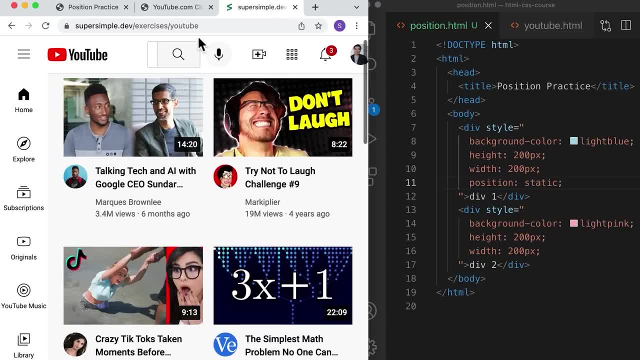 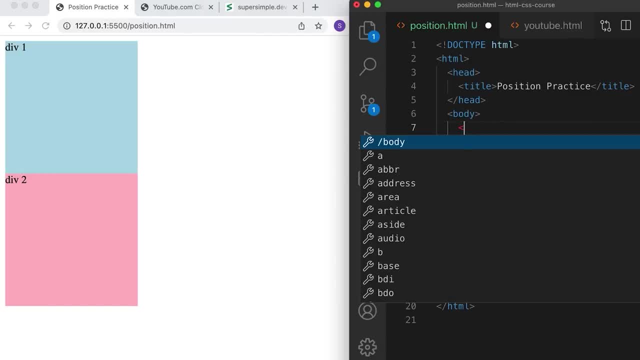 property that allows us to stick an element to the top of the page like this while we scroll, And that is called position fixed. So we're going to create a new element at the top here And let's call this our header. So we're going to learn how to create. 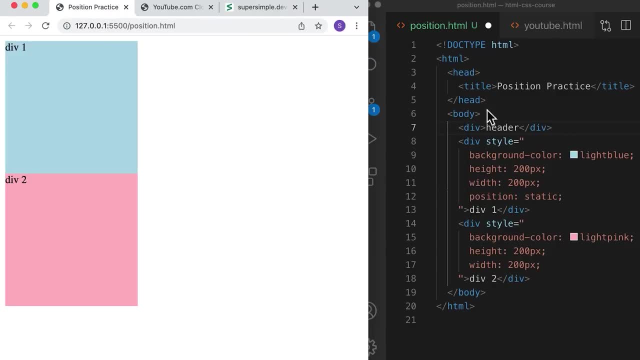 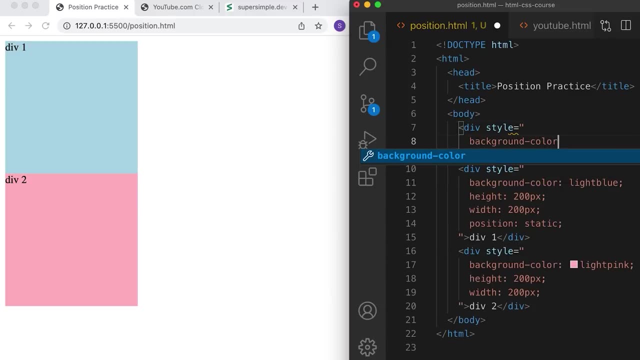 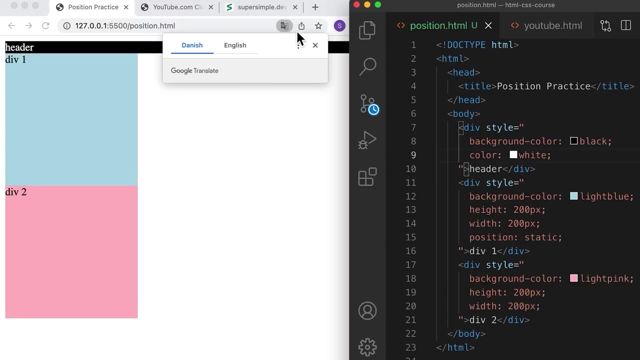 something that works like this. So for this div, we're going to set a style of background color- black- and a text color of white, And now we're going to learn how to stick this to the top of the page. So first of all, we need to be able. 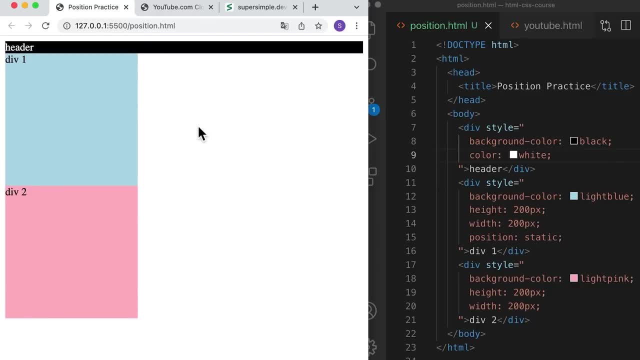 to scroll, And right now I don't have enough content to make the page scroll. So what I'll do is we'll go to the body here and we're going to set a style, And then, inside the body, we're going to set a. 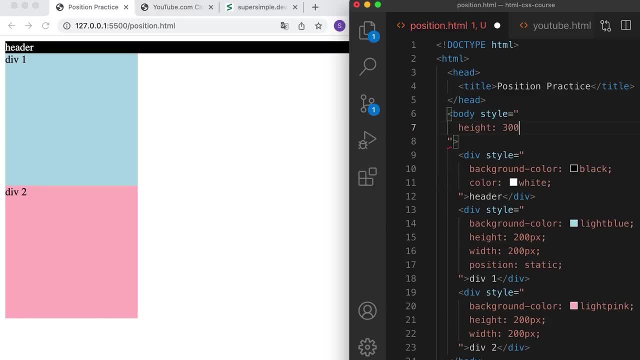 style of height and something really big like 3000 pixels. So we just need to make sure that we're able to scroll this page. Next, we're going to make this header stick at the top. To do that, we're going to use the position property. 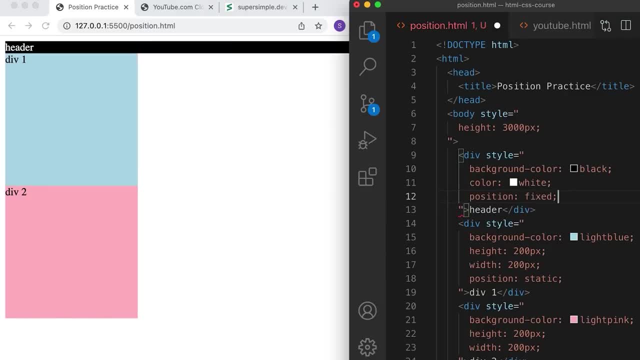 and this time we're going to set a position of fixed. Now, when I save it and I start scrolling, notice how the header element is sticking to the page when I scroll. So that's how we make it stick. So the first thing, 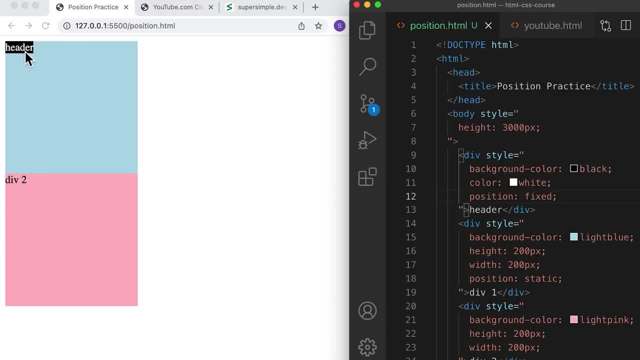 to note is that when we set position fixed like this, it doesn't take up space on the page anymore. So before we had this, and if I save it, so notice that it takes up the top of the page and then these two divs appear below this header. 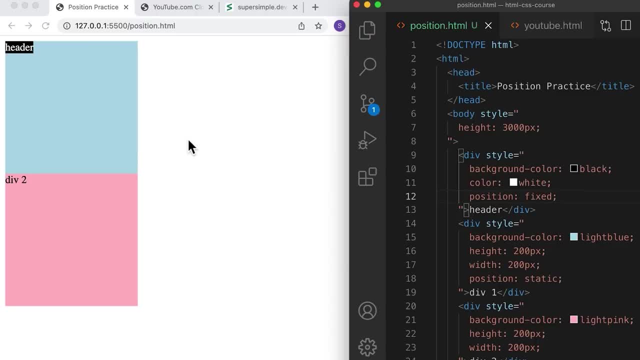 But when we add position fixed it no longer takes up that space at the top of the page because it's sort of floating above the page now. So that's one way to think about it. So the position property has four special properties we can use to: 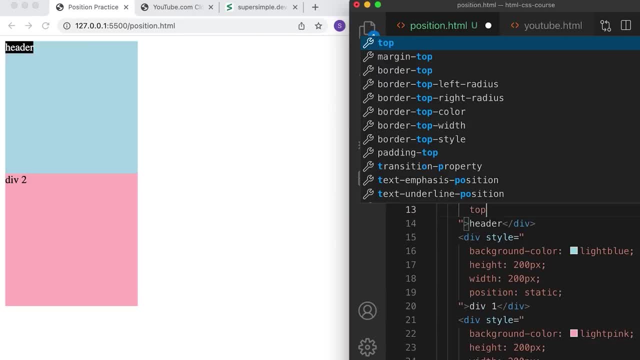 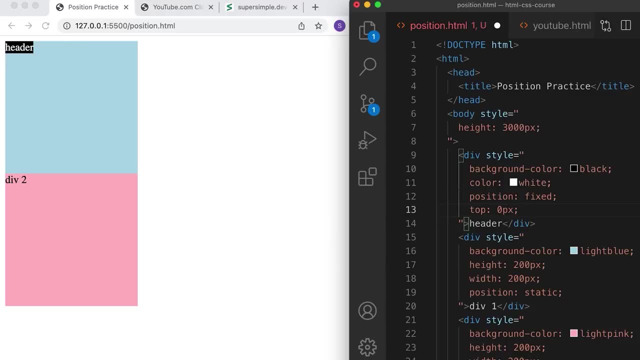 move this element around. The first one is called top. The way that top works is that we can set a pixel measurement. For example, if we set 0 pixels, this is going to make the top of our element 0 pixels from the top of our 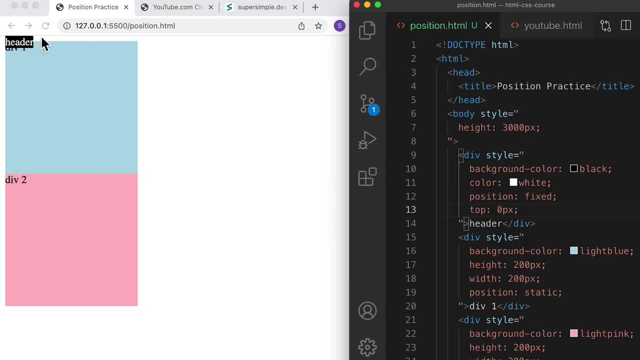 browser window here. So if I save it, notice that the top of our element is right on the top edge of the browser window. If I set top to 10 pixels, the top of our element is now 10 pixels from the top of the browser window. 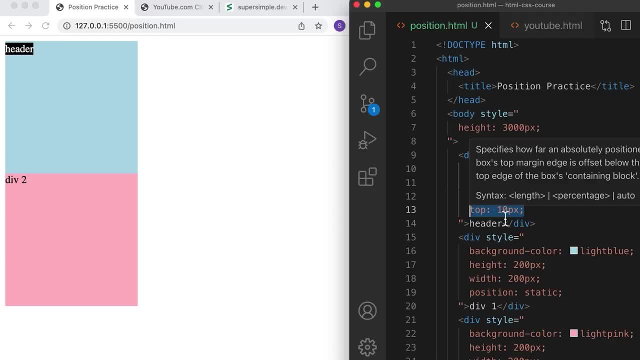 So top specifies how far away our element is from the top of the window. The next property we can set is left. So if we set left to 0 pixels, then the left side of our element will be on the left edge of our window. If we set left to, 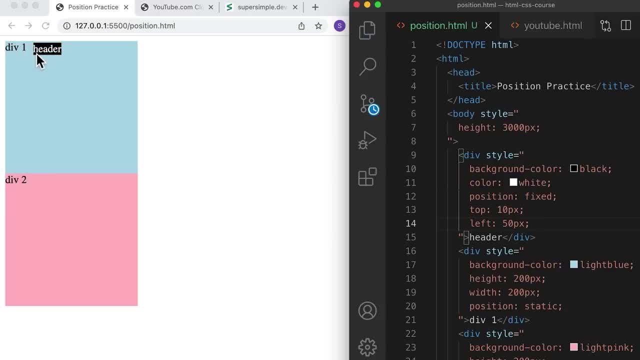 50 pixels, for example. now the left side of our element will be 50 pixels from the left of our window. So left tells us how much space is between the element and the left edge of the window. So we can set this in all four directions. 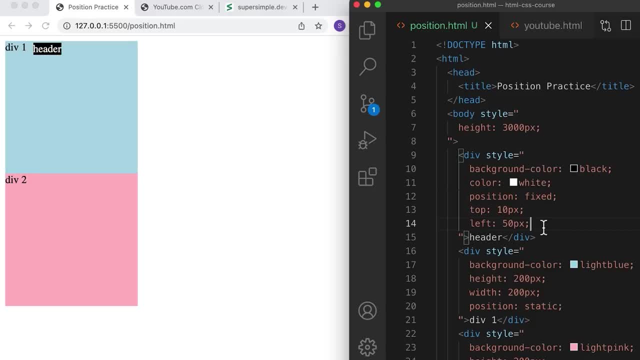 We've seen top, left. we can also set bottom and right. Now, a special feature of these properties is that if we set it in opposite directions, the element will stretch. So, for example, if we set it to left and right. so these two are opposite directions. 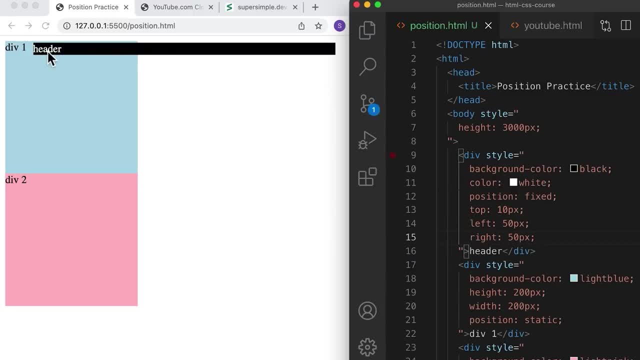 and we set the right to 50 pixels, notice that the element stretches. So now this element is 50 pixels from the left of the page, right here, and it is also 50 pixels from the right of the page, So it will stretch the element to meet. 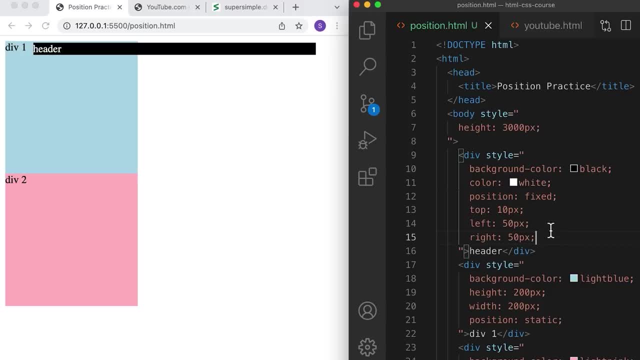 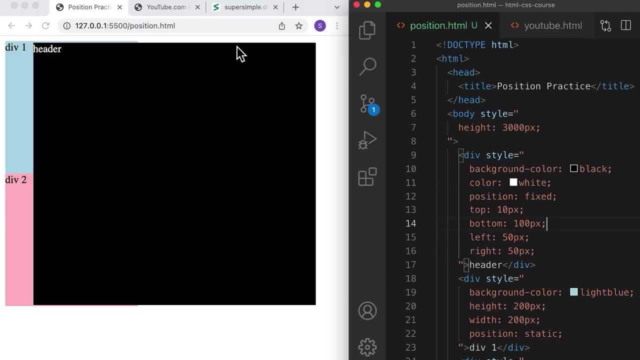 these two conditions Same thing with top and bottom. So if I set bottom to 100 pixels and save it, the element will stretch so that it is 10 pixels from the top and it is 100 pixels from the bottom. So this is. 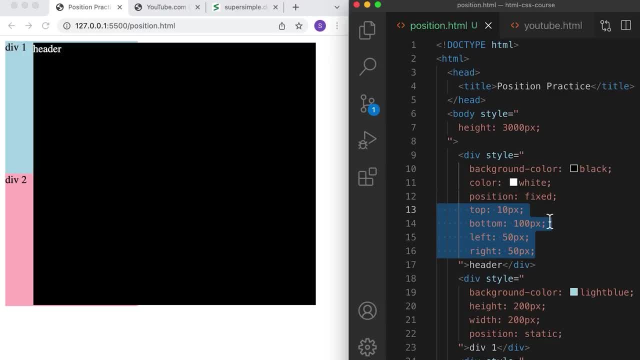 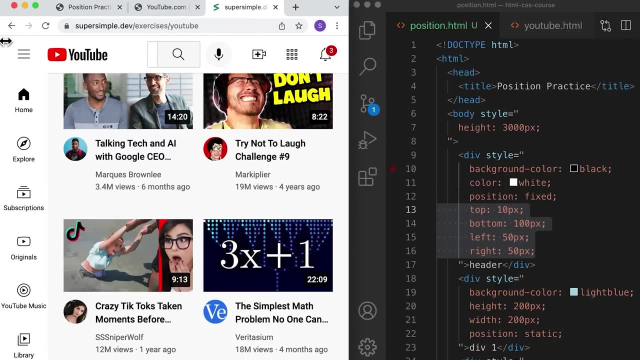 how we move this element around and resize it with position fixed. Now let's try creating the header that we see here. So, as you can see, for this header, it's at the top edge of the page. it's also on the left edge and on the right edge. 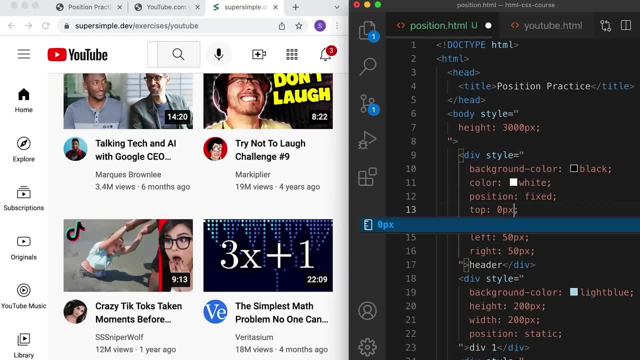 So that means that it's 0 pixels from the top. as a shorthand, we can just write 0, it's 0 pixels from the left and it's 0 pixels from the right. Now for the bottom. we might first try to calculate. 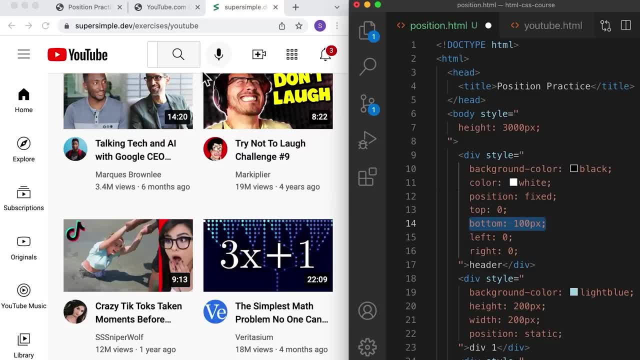 how far the bottom of this element is from the bottom of the page. Now that's not going to work if we resize the page, so we need a different approach. So first let's save this file and go into our practice file. So now you can see. 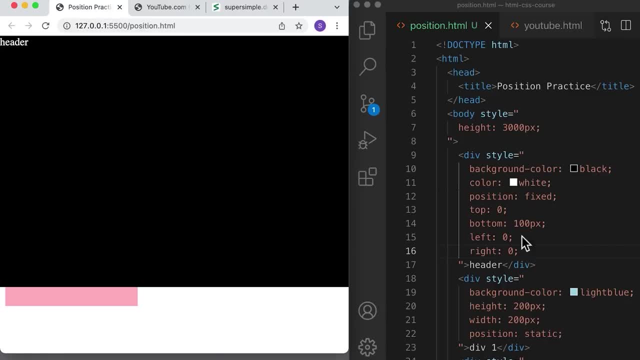 that this element is sticking to the top, the left and the right, which is what we have in our code. Now we have to figure out the height of this div. So, in this case, instead of using bottom, because remember the bottom- 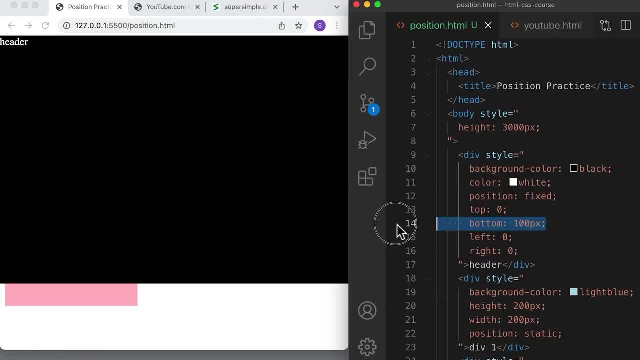 can resize. we want to use simply height. So, in addition to these properties, we can simply use height and width to also resize this element. It all depends on what situation you're in. If you want this fixed element to resize with the page, then 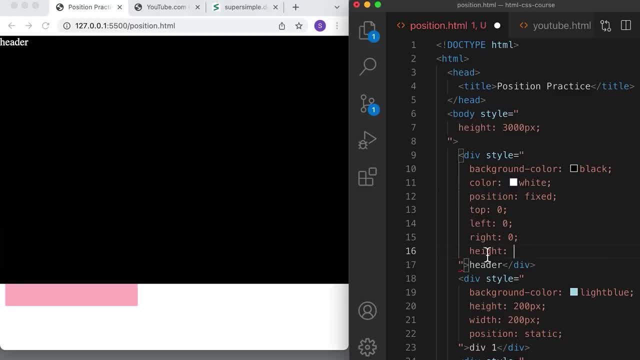 you would use top, left, right and bottom. If you just want it to have a specific height or width and you don't want it to resize, then you use height and width. So here we're going to set the height to 50 pixels. 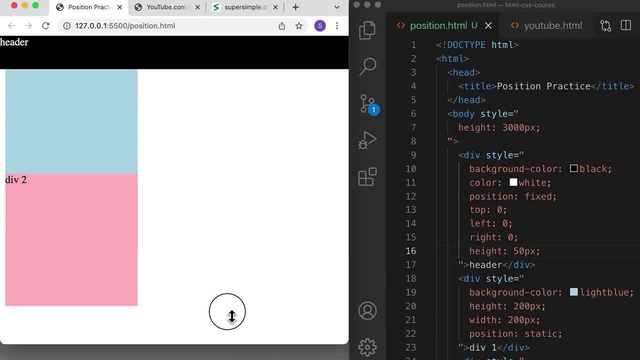 and we don't want it to resize with the page. So that's exactly what we have here Now. when we start scrolling, you'll notice that our header sticks to the top of the page. So that's how we create something like the YouTube header. that. 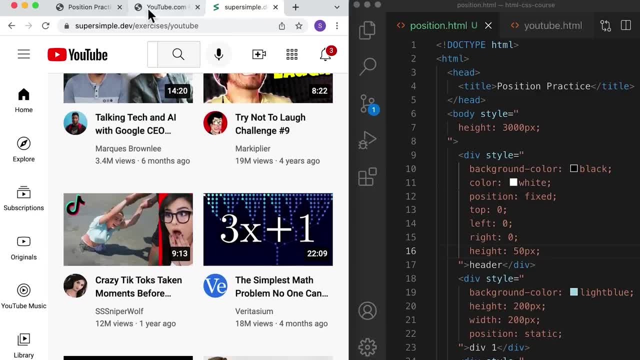 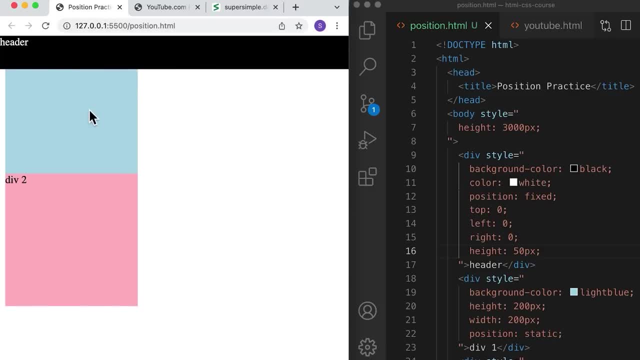 we see here Now. one last problem is that if we go to our practice file, notice that if we scroll right to the top, the header is covering our first div. So we need to add some spacing at the top to push our content down below the header. 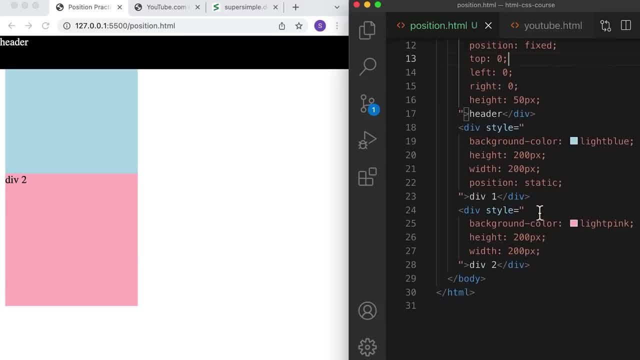 To do that, we can go into our code and the first thing you might think to do is to add margin to the top. So we're going to add spacing to the top and let's add a little more than 50 pixels, so 60 pixels. 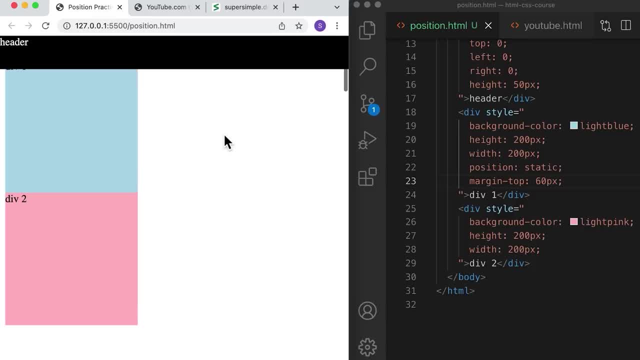 So if we save it and make sure you scroll up all the way to the top of the page, you'll notice that we have 60 pixels of space at the top and now our content is not covered by the header. Now, this is not the best solution, because if 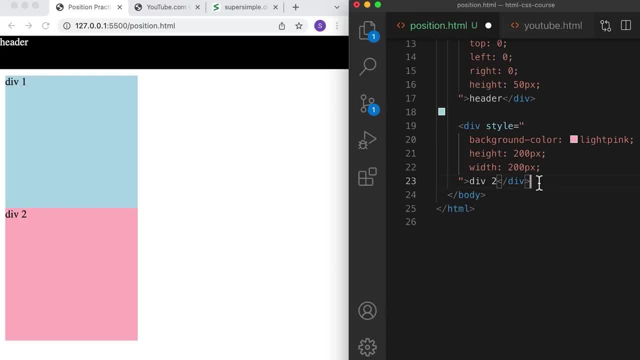 our content order changes. for example, if I move this div down here, notice that it doesn't work anymore. So what we want instead is to always have space at the top of our page, regardless of what the content is. So if I move this to the top, 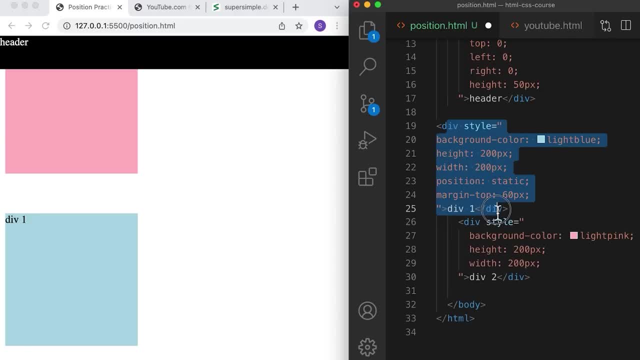 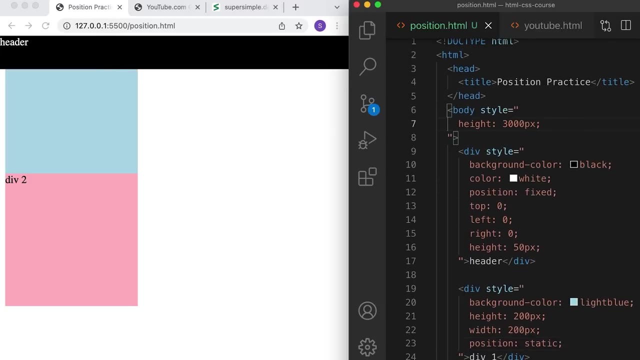 here and remove margin top. I'm going to show you the proper way to do this. So, to properly handle this situation, we need to add spacing to the body element. So let's scroll up to the body. So we have two choices. 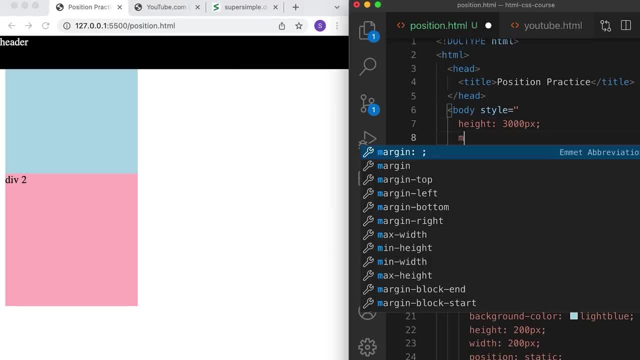 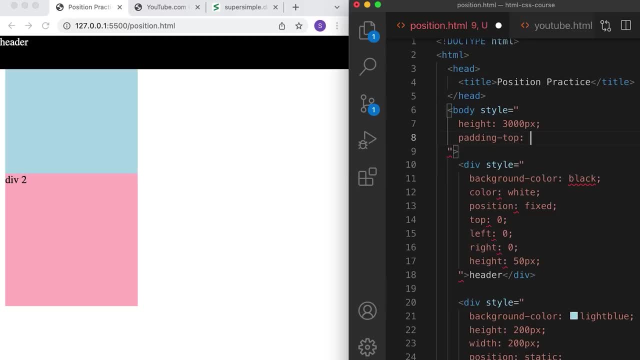 for adding space to the top of our page. We can either use margin or we can use padding. Generally, the best practice is to use padding at the top. So we're just going to add spacing on the inside of our webpage, at the top. 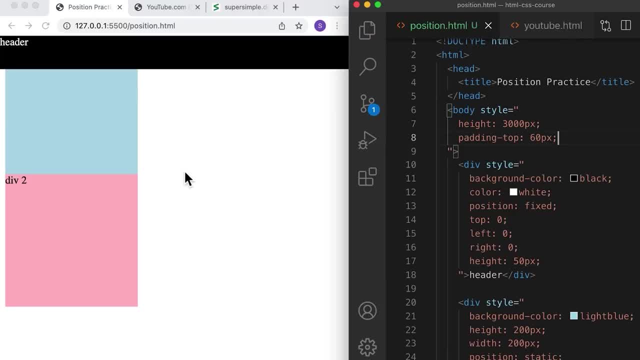 of 60 pixels, Save it and scroll all the way up, And now we have plenty of space at the top of the page and our header is not covering our contents. So now that we learned position fixed and how to move this, 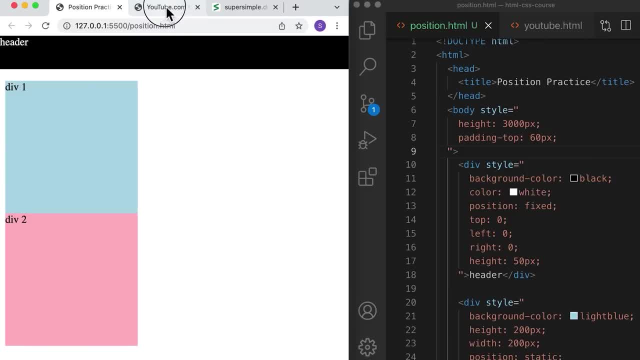 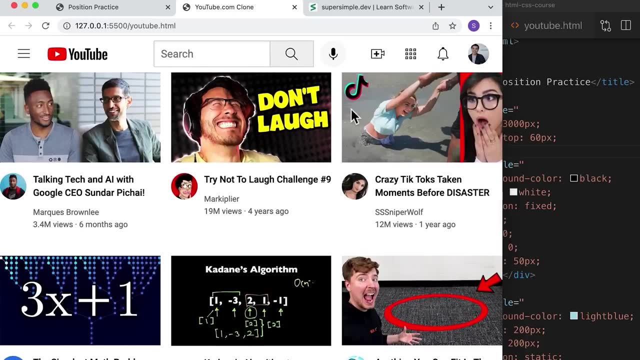 element around and resize it. we're going to go into the project we were currently working on and we're going to put our header and stick it to the top of the page. So let's learn how to do that. First, I'm going to resize my windows. 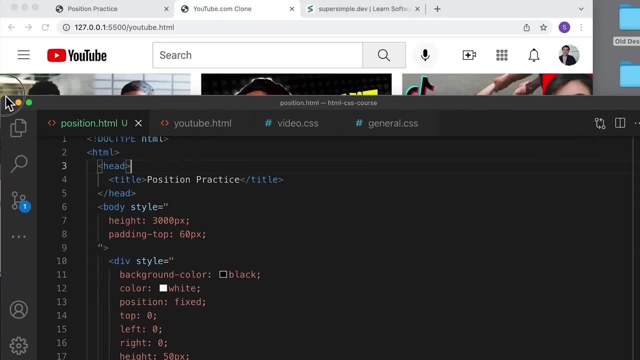 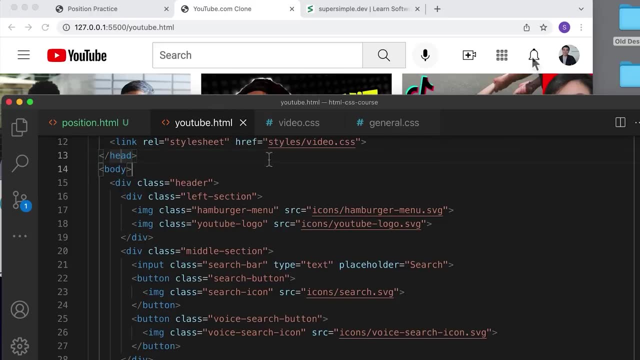 a little bit so it's easier to work with. I'm going to put it right here, And then we're going to open the youtubehtml file, which is our project. So remember, we put our CSS into separate files, so I'm going to open the headercss. 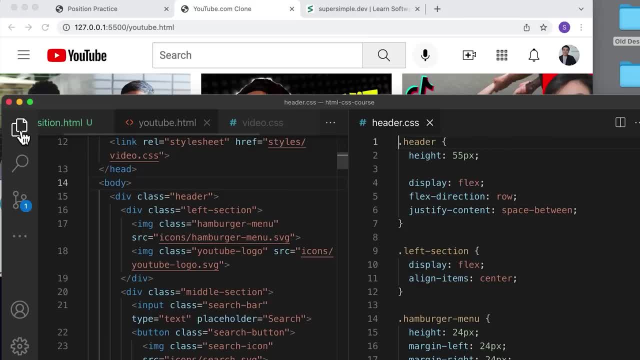 file and I'll put it on the side so you guys can see it side by side. So, just like we learned, we're going to go into the header here. We're going to set a style of position fixed And remember to move this we're going to use 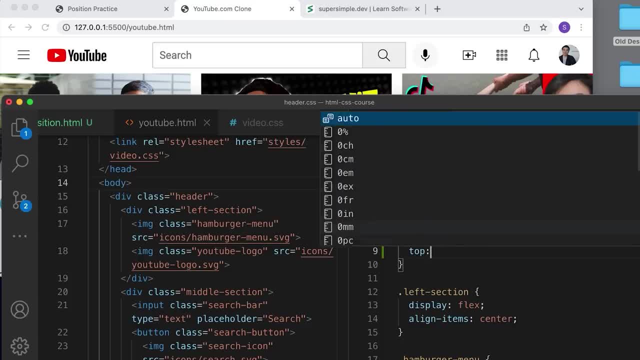 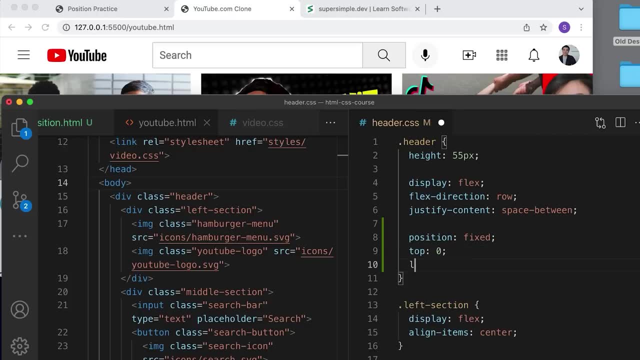 top, left, bottom and right. So top, we want our header to stick to the top of the page. We're going to set that to 0.. We want our header 0 pixels from the left, so on the left edge of the page. 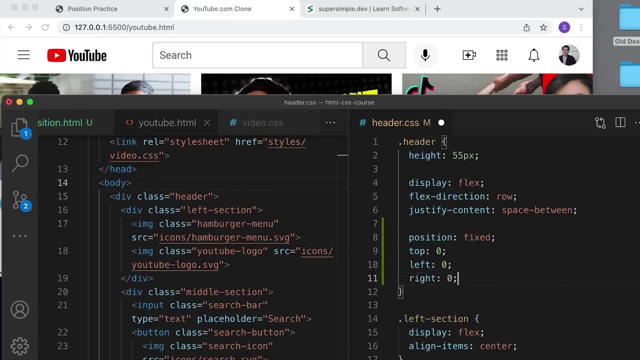 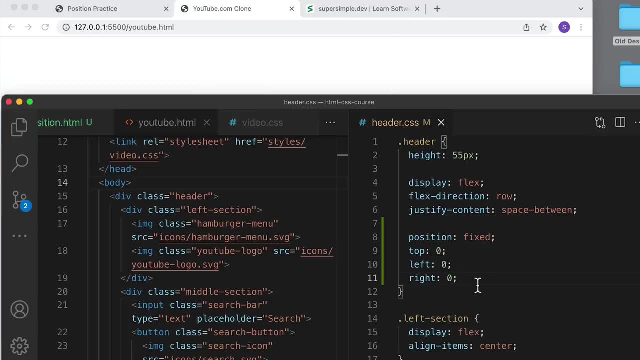 And also 0 pixels from the right. And finally, we're going to set a height. So we already have it up here, So let's save it and see how it looks. So the first thing we notice is that we lost our background color. 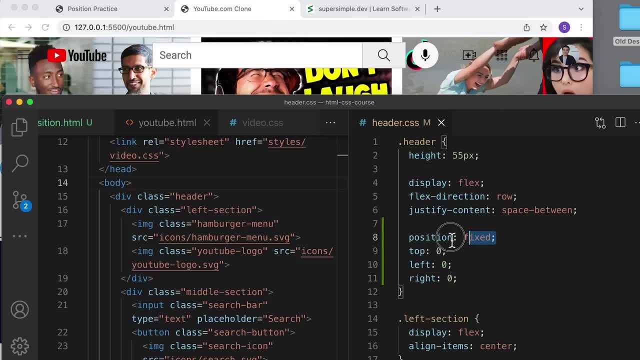 Now, the only reason we had a background color was because, if we didn't have position fixed, this header takes space on the page And the page just happens to be white. so the header appears to be white, But now that it's floating above the page. 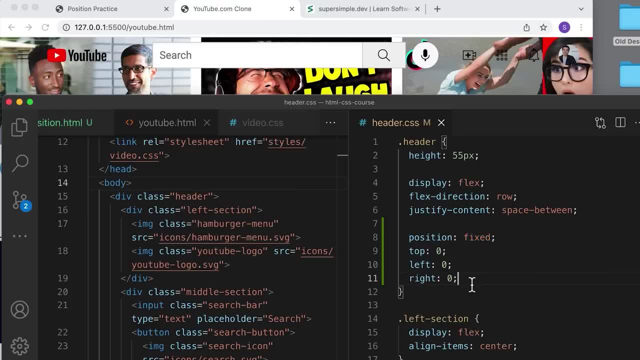 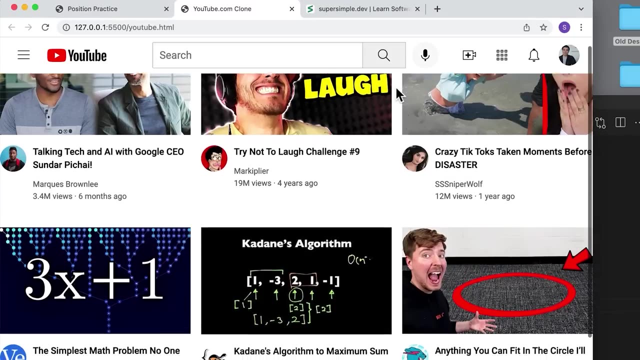 we'll notice that it's actually transparent. So to add our background color again, we just need to set the background color property. So let's set this to white, Save it, and now we're back to where we were. Now, if we go to our project and we start scrolling, 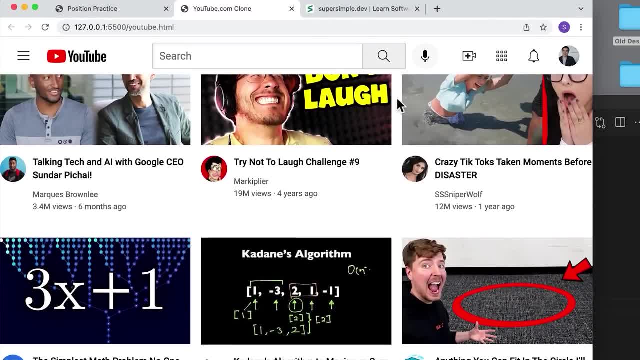 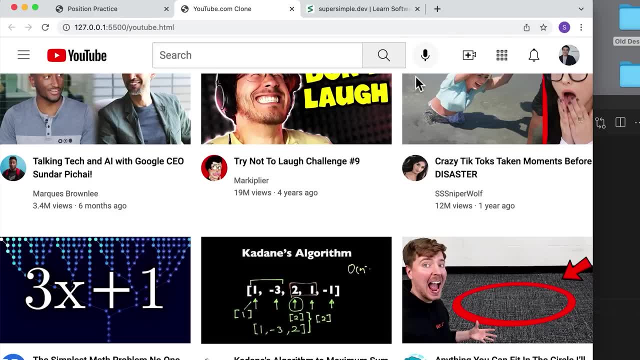 you'll notice that our header sticks to the top while we scroll, So that's exactly what we want. Next, we have this problem where the header is covering our content. So remember, the way to fix this is to add padding to the top of our body. 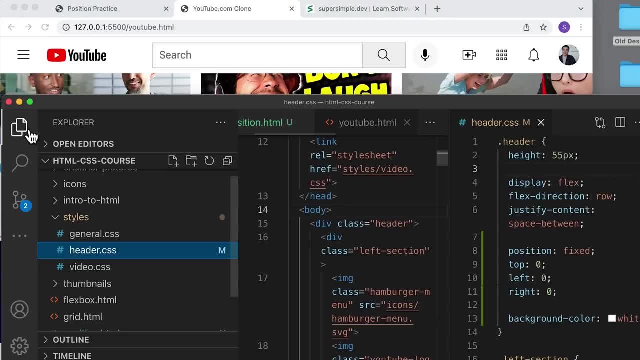 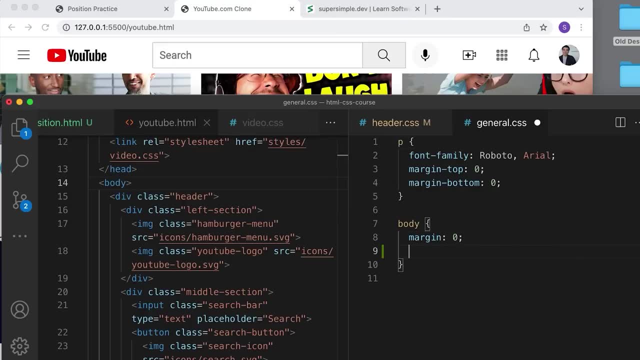 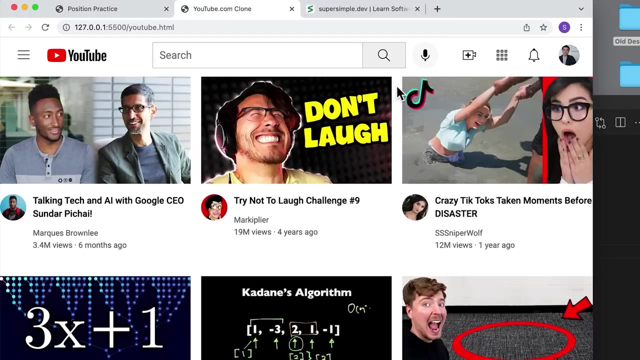 We're going to go into our code and we're going to go into this file, generalcss- That's where we have styles for the body, And then we're going to set a padding dash top of maybe 60 pixels. Let's take a look. 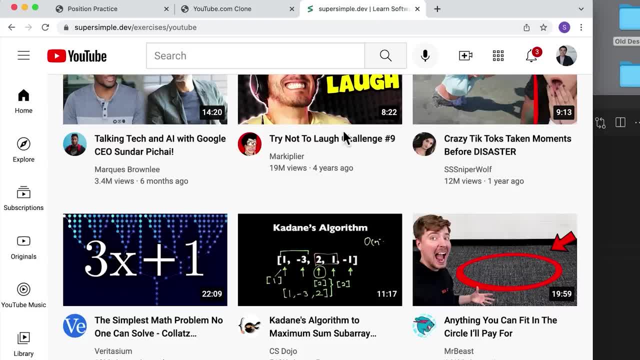 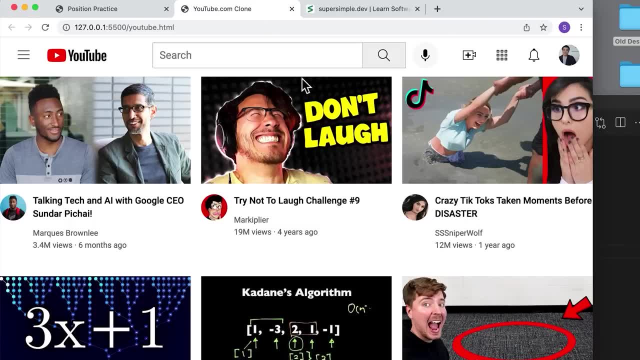 Okay, so that looks pretty good. Let's compare it to our design. If I scroll to the top here and just compare it a little bit, I notice that our videos are appearing at a higher position than our design, So we're going to push them down a little more. 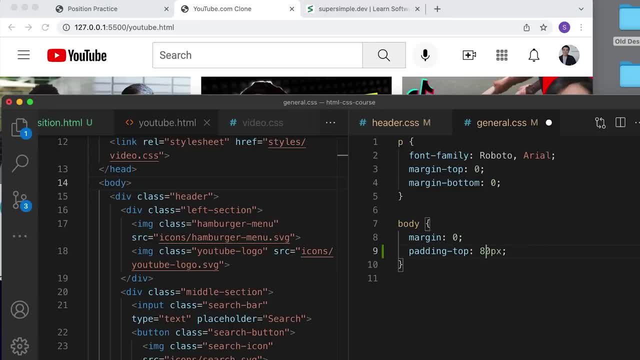 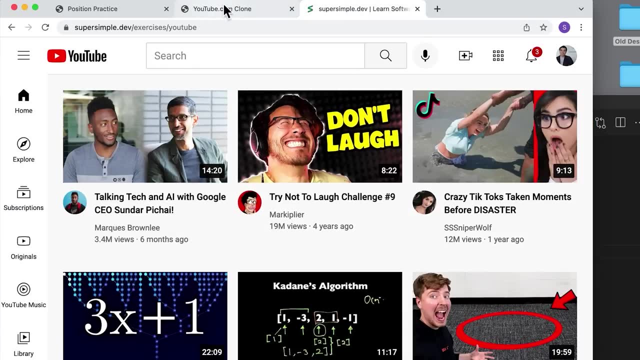 Let's set this to maybe 80 pixels, Save it So we push them down even more, And I think that looks close enough to our design. So the last thing I notice is that we're missing the border at the bottom of our header here. 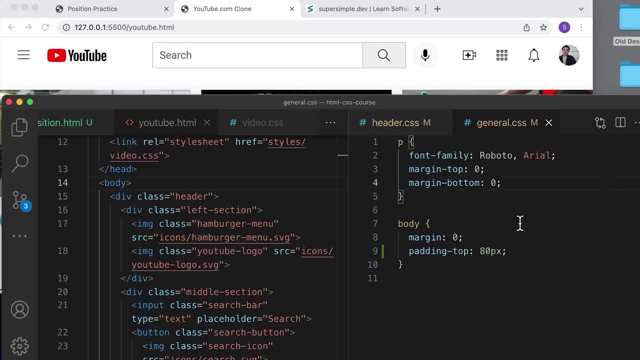 So let's go ahead and add that. So let's go back into our headercss. We're going to add a border to the bottom So we can actually add borders to one side at a time. We don't have to add borders to all four sides. 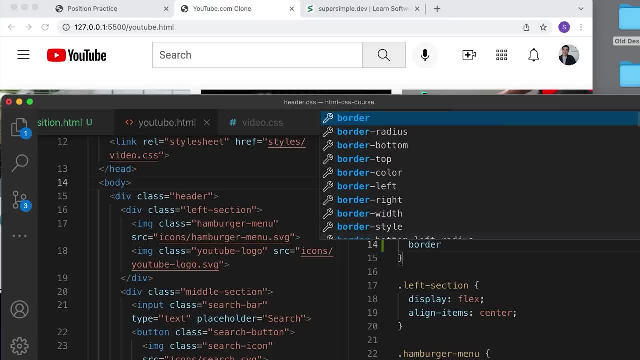 To do that? we're going to set the same border properties we had before. So we're going to start with border-width, But in the middle we're going to tell it a direction So we can tell it bottom, We can also tell it. 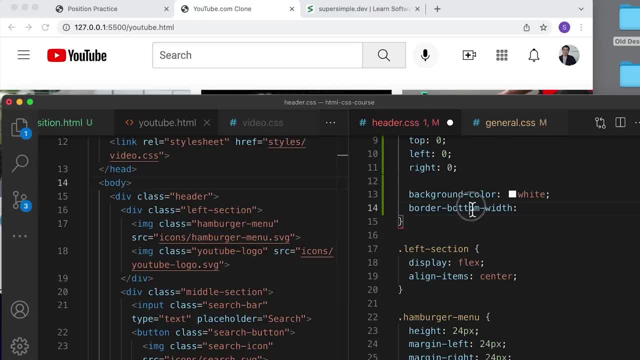 top, left and right, So we have all these four directions. In this case we want a border at the bottom And we're going to set it to one pixels And the other border properties are the same. So border style. 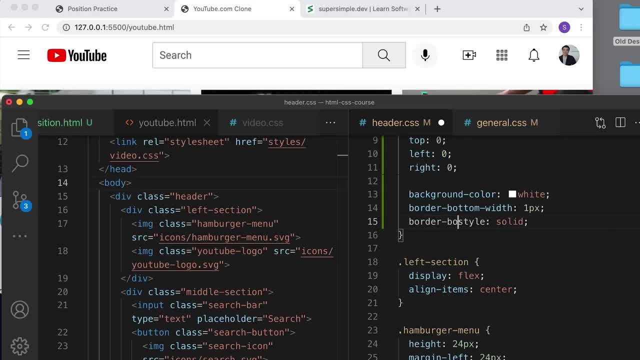 It's going to be solid, but we only want it at the bottom, So it's going to be border-bottom style, And then, lastly, border-bottom-color, And let's set it to gray, And I'm going to pick a lighter. 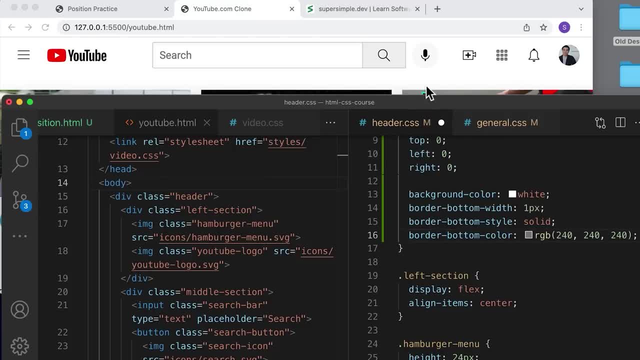 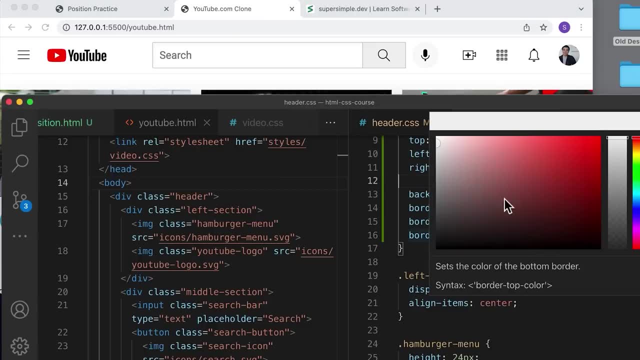 shade of gray, So maybe right there, Save it. Let's compare it to our design. It looks like it's a little darker than what we have Just going to adjust the color to match our design. It's not going to be perfect, but remember you can. 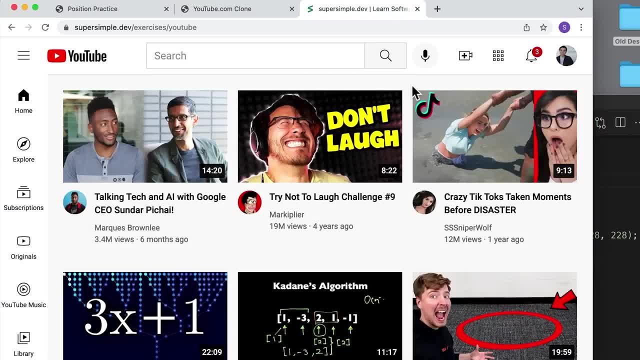 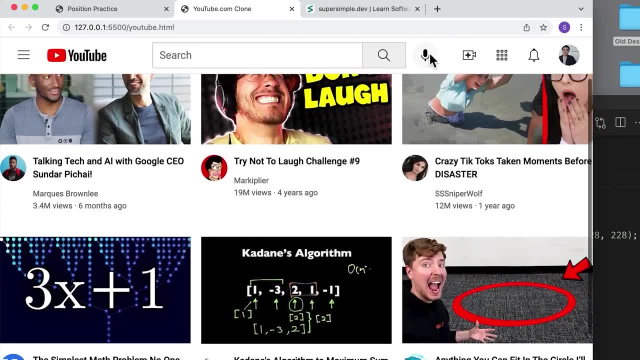 always inspect the design and then make it perfect. Okay, so now if I compare it, I think that looks pretty close enough. And now, if I scroll, you notice that the header is sticking to the top, which is exactly what we want. 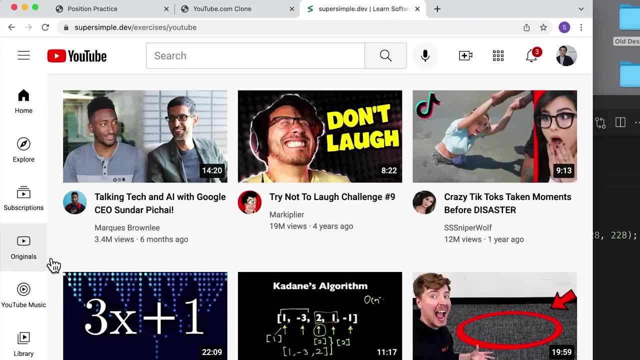 Next we're going to learn how to create this sidebar. So the sidebar is just like the header: It sticks while we scroll. So this is another example of position fixed. We're going to go back to our practice file And I'll resize my. 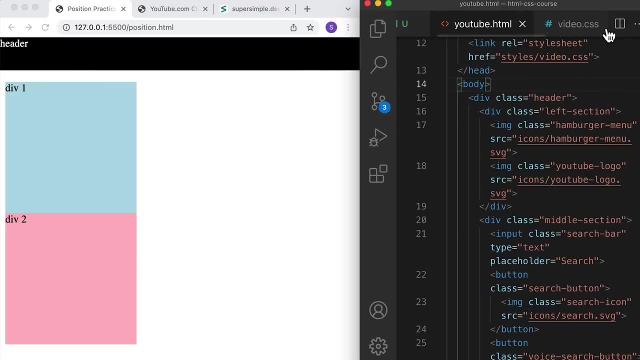 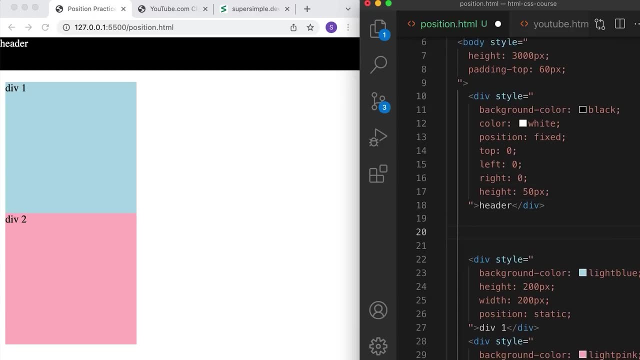 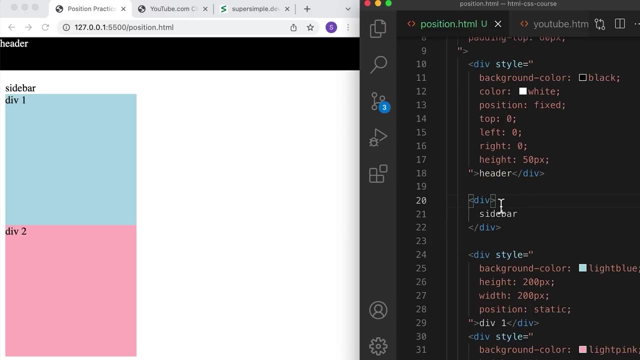 images here And I'm going to open positionhtml we were practicing with, And this time, below the header, we're going to create our sidebar. So let's create a div, And this div is going to be our sidebar. Now for the 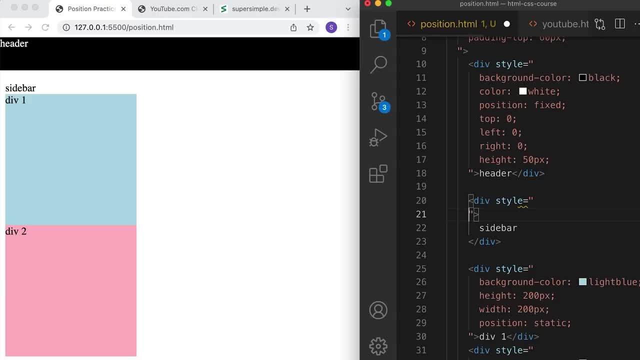 sidebar. let's set a style And then, inside, we're going to set a background color of green this time, So background-color green and a text color of white, So that it's easier to distinguish between all of these different elements. Next, we're going to stick the sidebar. 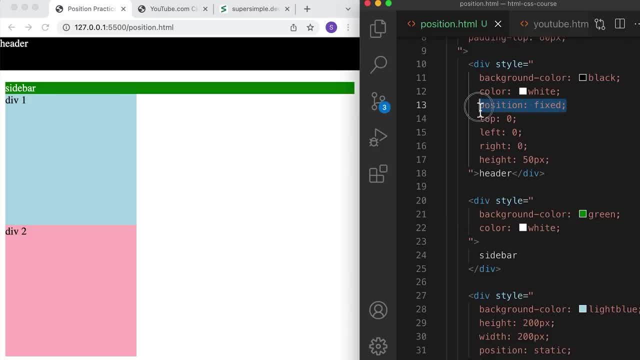 to our browser. So remember to do that. we're going to use position fixed. So position fixed And save it. And now, when we scroll, you'll notice that the sidebar is sticking to our browser while we scroll. Lastly, we're going to put the sidebar 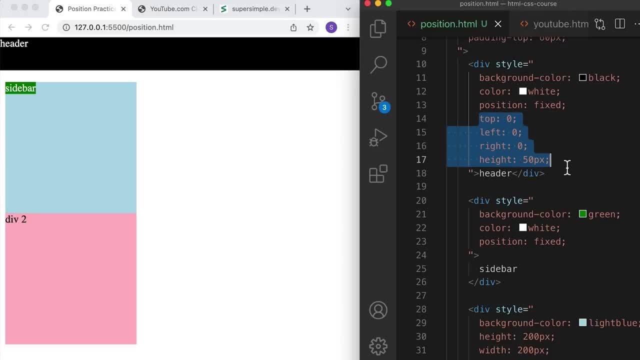 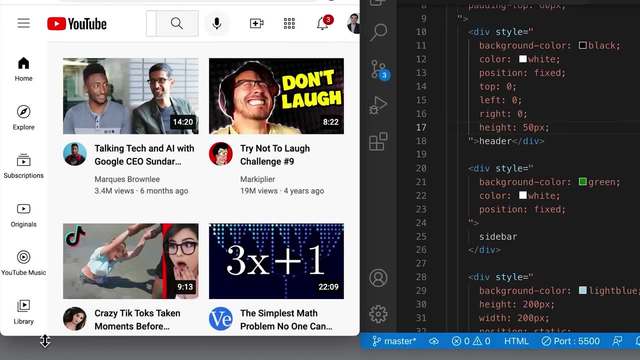 in the right place using top, left, right, height or width. So let's look at our sidebar. in our design, We notice that the sidebar is sticking to the bottom, so we want bottom 0.. It's sticking to the left, so we want left 0.. 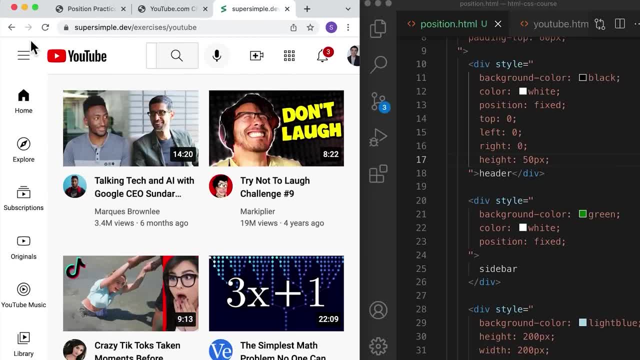 And for the top. it's actually not reaching to the top of the page, Otherwise it would cover up the header. So there's quite a difference between the sidebar here and the top of the page. So let's go back into our practice file. 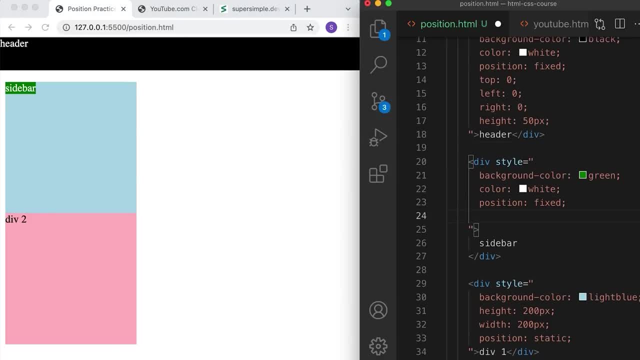 and learn how to position that. Let's start with left. We want the sidebar to stick to the left side of the page, So we're going to say 0 pixels from the left. Save it Now. we want our sidebar to stick to the bottom of the page. 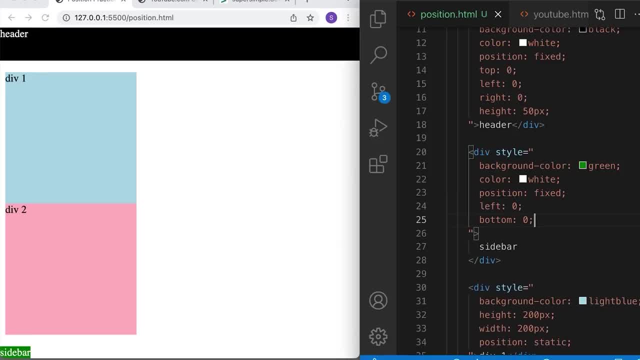 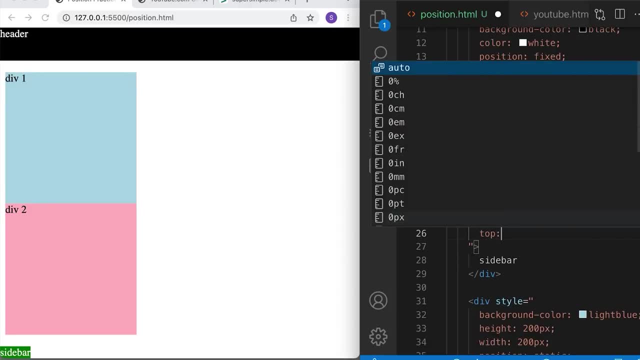 So we're going to say bottom and 0 pixels from the bottom, And finally we want it to be at the top of the page but not cover the header. So let's set the top to 50 pixels, So it's going to meet right where. 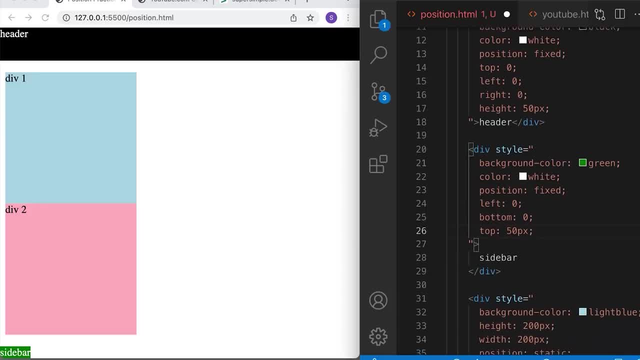 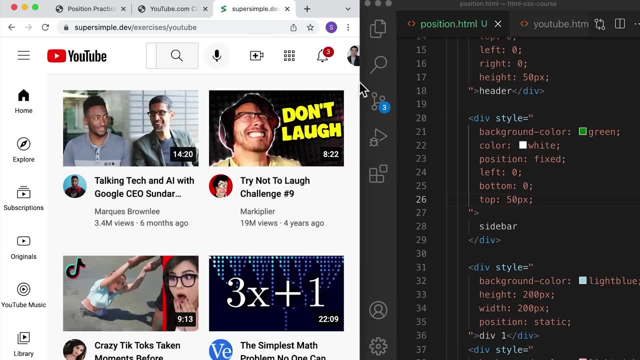 the header ends. We're going to set this to 50 pixels And then save. And finally, we want to set the width of the sidebar. So, for the sidebar, we don't want it to resize with the page, So that's why we're going to use the 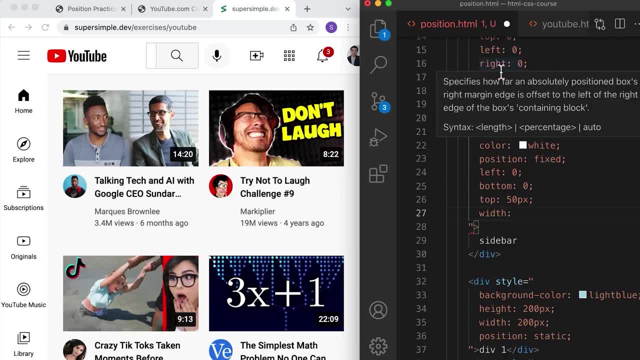 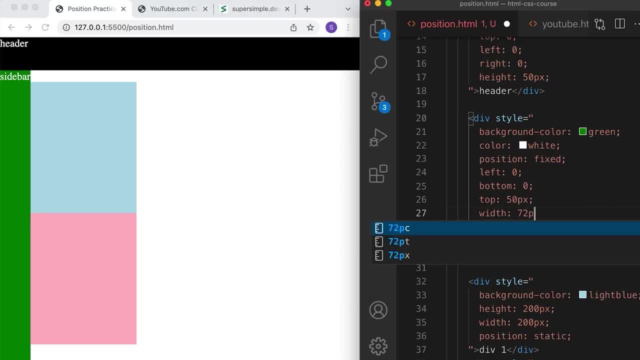 width property instead of something like right. So let's go back into our practice file And we're going to set the width to maybe 72 pixels, Save it, And that looks like what we have in our design. So that's perfect. 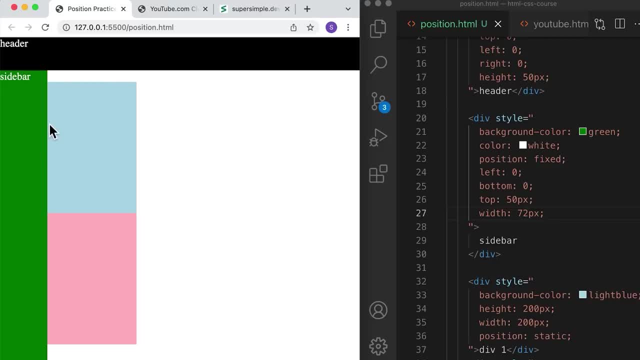 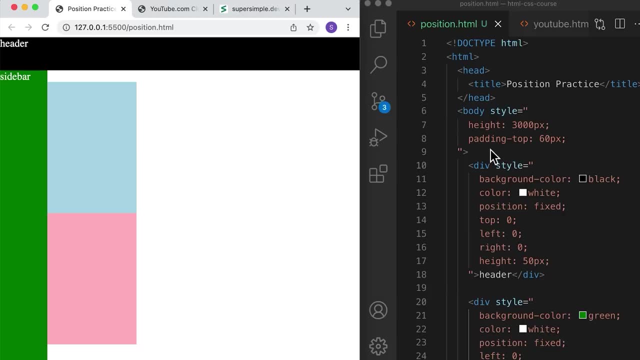 Now we have the same problem again, where our fixed element is covering our content, So let's scroll back to the top. We're going to add padding to our body so that these elements are not covered by the sidebar, So in this case we want extra. 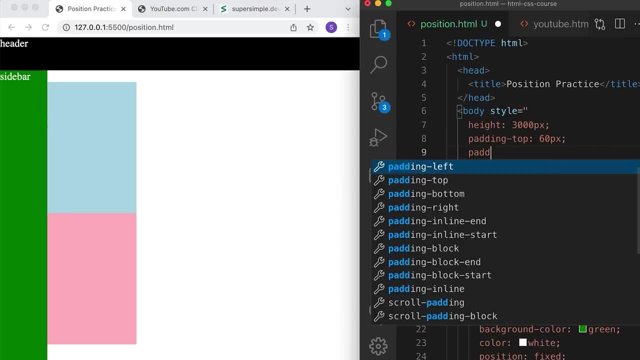 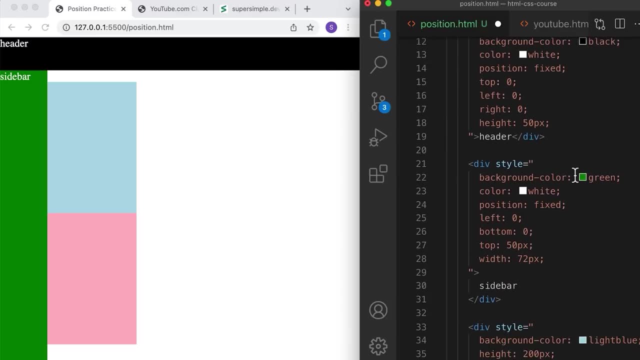 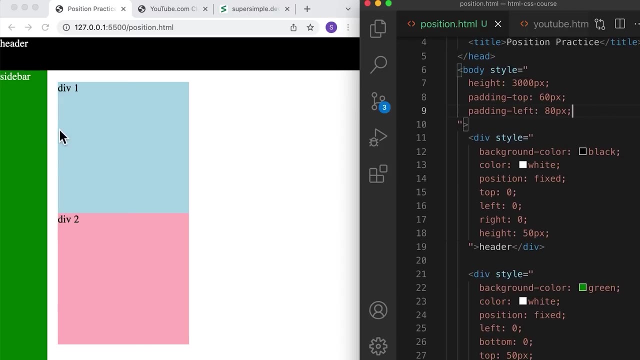 space on the left side. So we're going to set padding dash left And let's set it to 80 pixels, Which is more than the sidebar's width of 72 pixels. So now, if we save this, we have 80 pixels of padding. 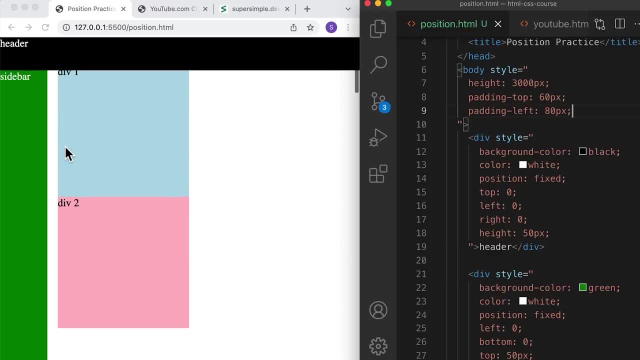 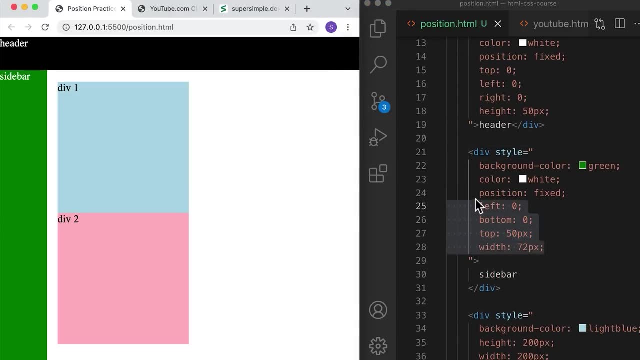 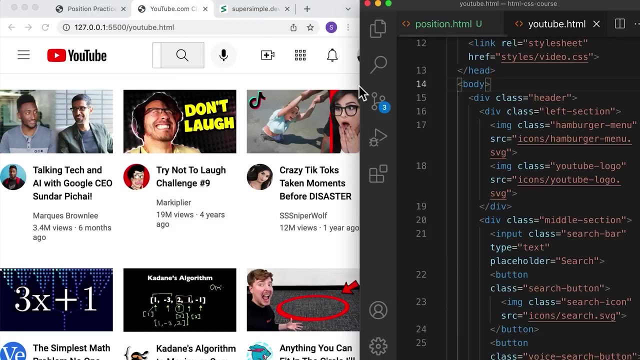 on the left side of the page, And now the sidebar is not covering our content. So that's how we position a sidebar. Now we're going to create the sidebar in our project here. So let's go back into youtubehtml. I'm going to resize my page. 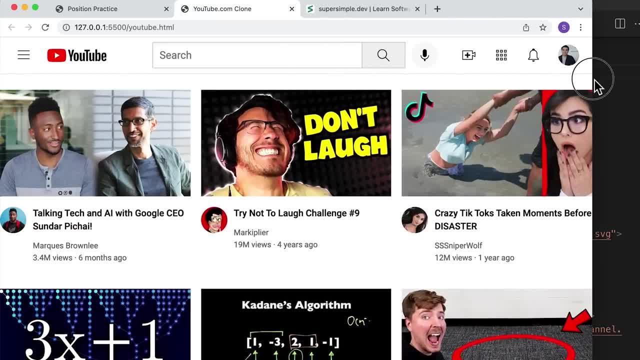 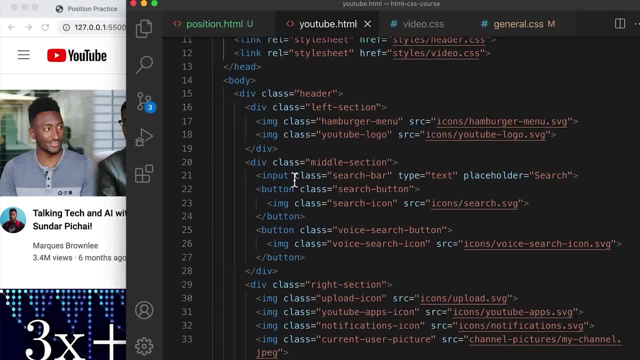 so that we can see it better, And we're going to create a sidebar on the left. So let's go into our code And we're going to put the sidebar right below our header. Let's scroll down below our header. here I'm going to create a div. 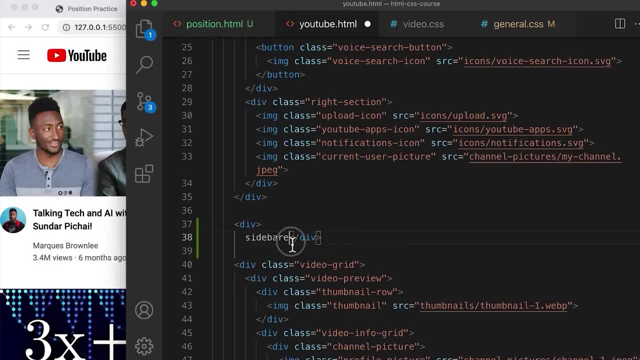 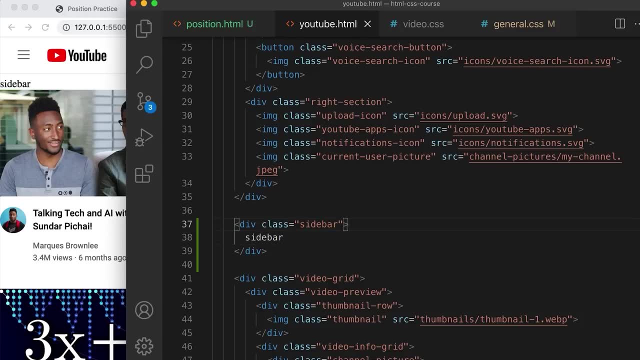 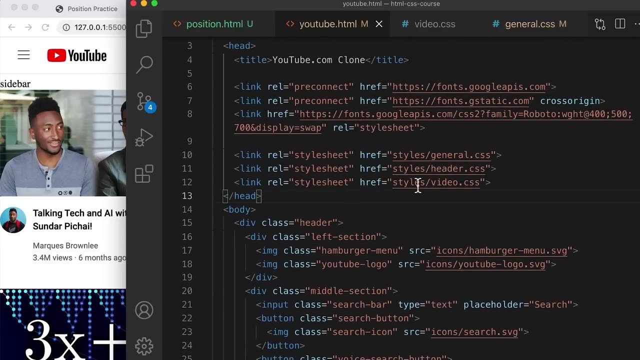 This is going to be our sidebar, And I'm going to give a class of sidebar So that we can target it in our CSS. Now for these styles: let's actually put them in a separate CSS file. So if we scroll up to the top, we have CSS. 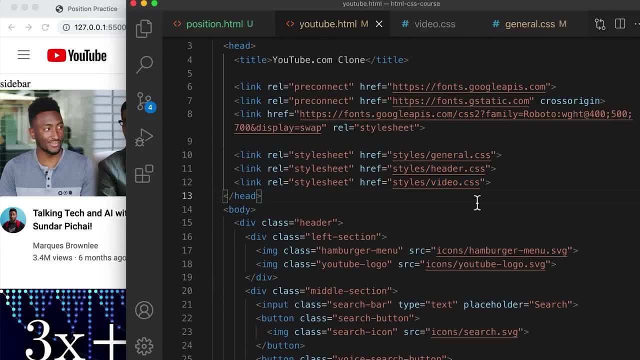 files for our header, for our videos. So it makes sense to split up our sidebar styles into their own file so that we organize our code better. We're going to go into our code editor and then go into the styles folder here. 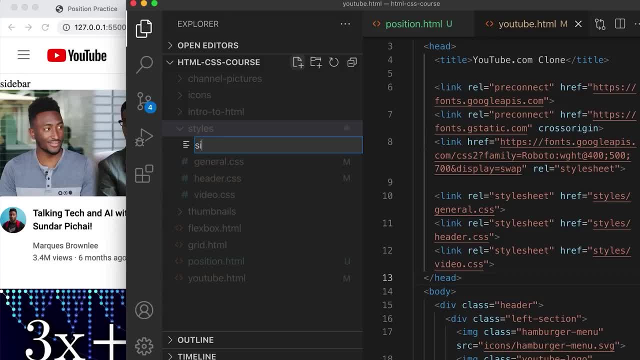 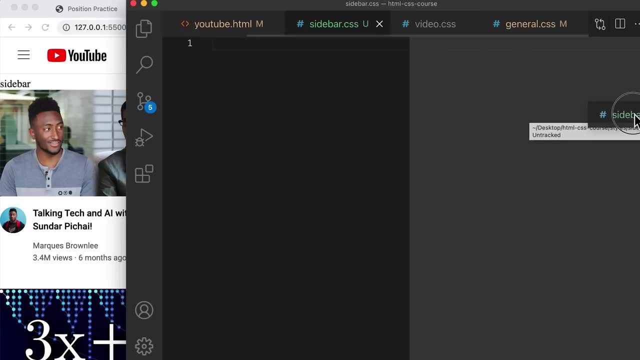 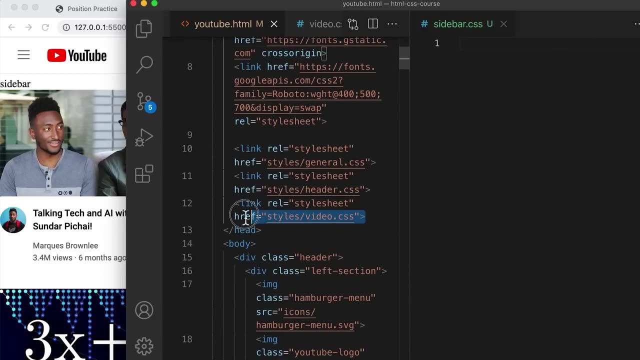 And we're going to create a new file And we're going to call it sidebarcss And I'm going to put it on the side like this: Next, we're going to load sidebarcss into our HTML. So we're just going to do one of these again. 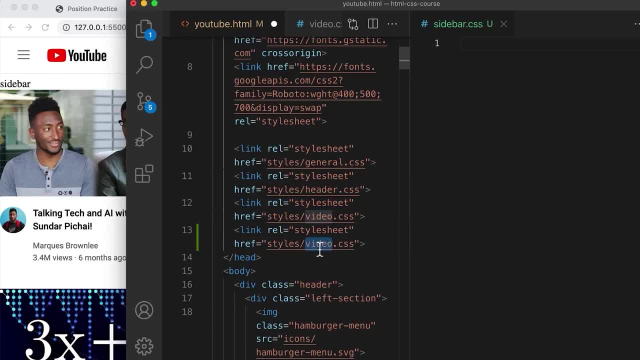 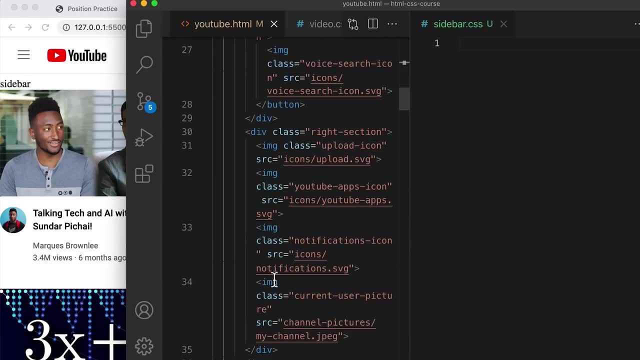 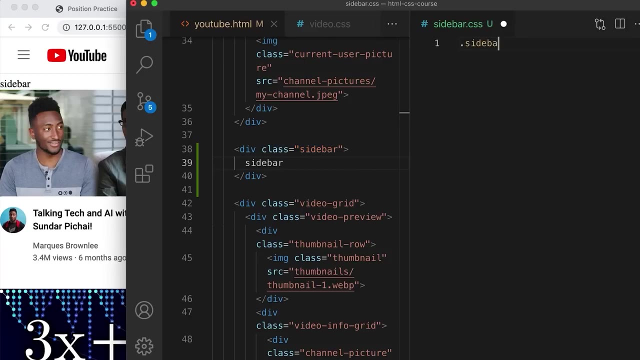 Just going to copy them And then, instead of videocss, we're going to load sidebarcss, And now we're ready to style this sidebar that we just created. So let's target the sidebar class And we're going to set position to. 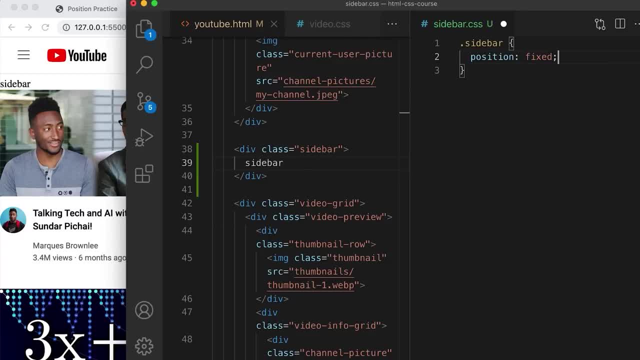 fixed to make it stick. Now for the sidebar. we want it to be 0 pixels from the left of our browser, So let's set left to 0.. And we also want it to stick to the bottom of our browser, So bottom. 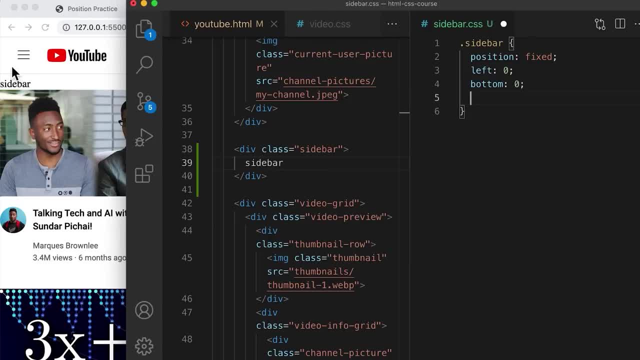 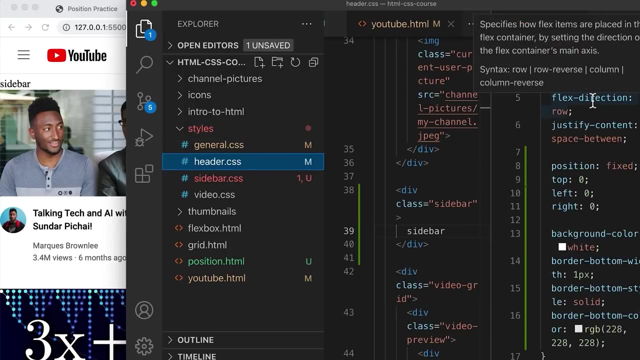 to 0.. And finally, we want it to stretch to the top, but we don't want it to cover our header, So let's set the top to whatever the height of our header is. So if we go to headercss, which is here, we can check the height. 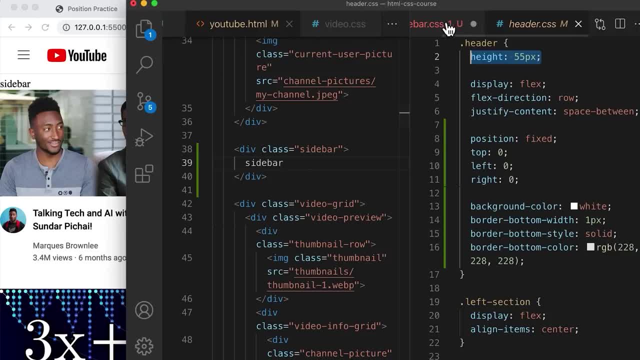 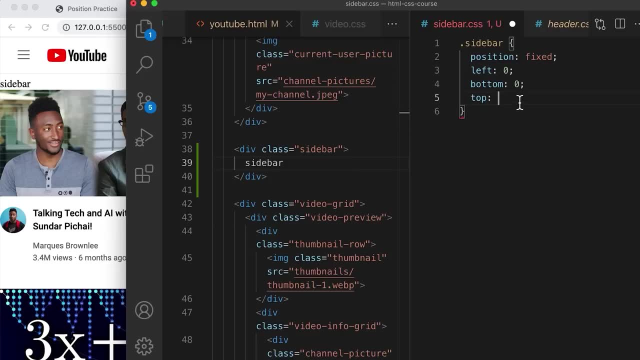 of our header is 55 pixels. So we're going to go into our sidebar here And we're going to get the sidebar to end 50 pixels or 55 pixels from the top. So let's set that to 55 pixels, Save it. 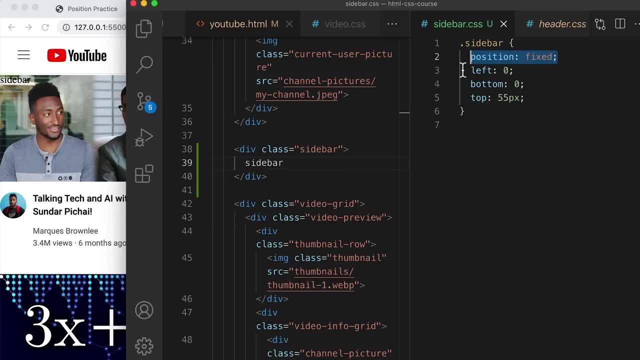 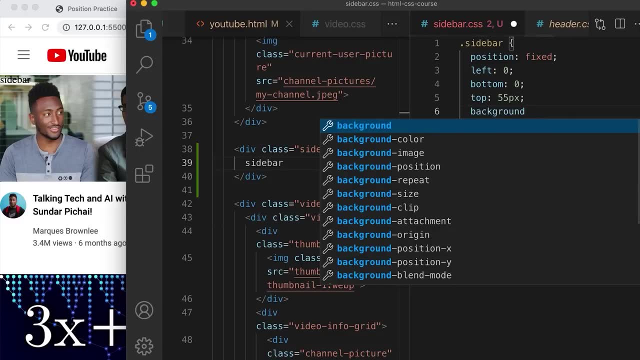 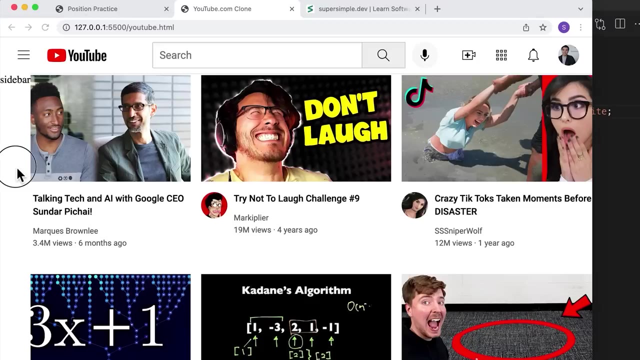 So remember, with position fixed, the element is no longer on the page anymore and it doesn't have a background color. So we just have to set that again background-color. We're going to set it to white, Save it. And now we have our sidebar. 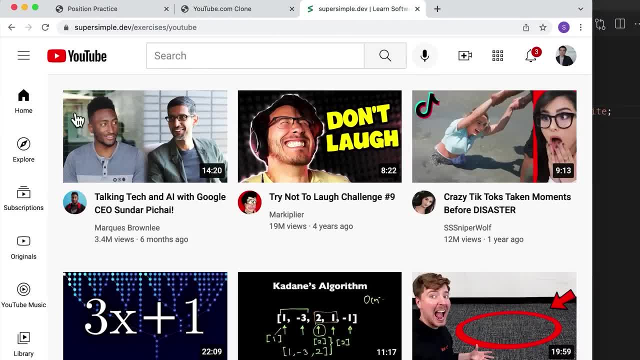 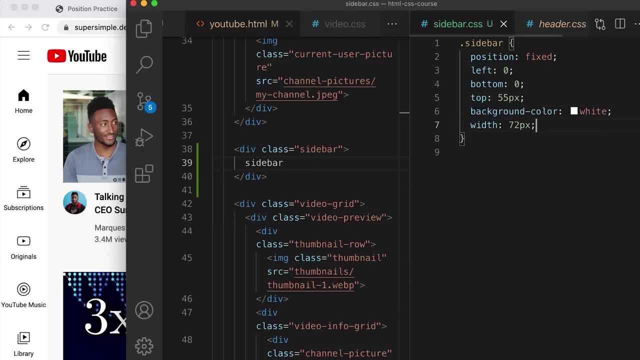 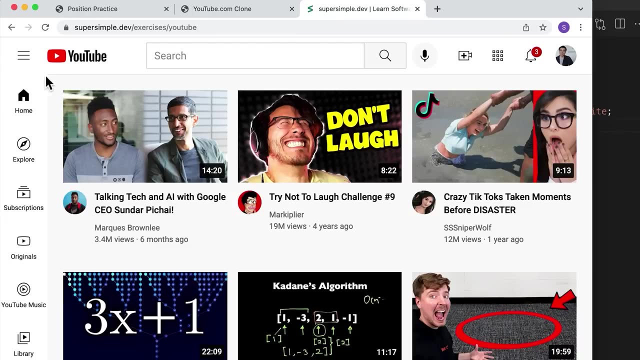 The final thing is to make our sidebar as wide as our design, which is right here. So we're going to set the width to 72 pixels, Save it And let's compare it to our design, And I think it's hard to see because it's white here. 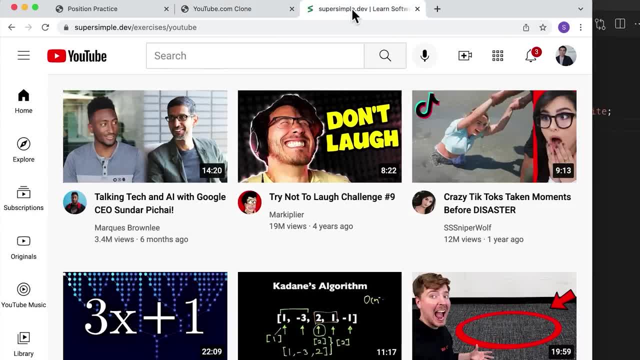 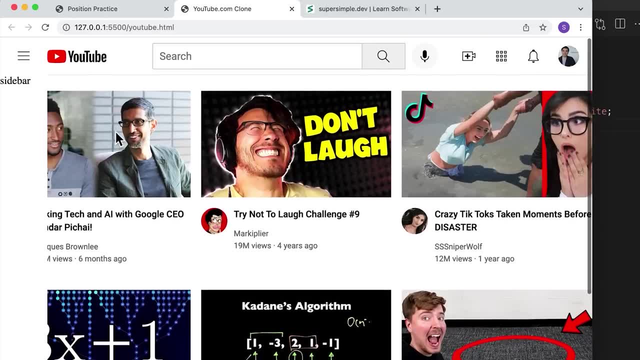 and it's a little bit gray here, but I think that's close enough. Now the next problem we have is that the sidebar is covering our content. So, as we learn, we're going to add some padding to the left to push our content. 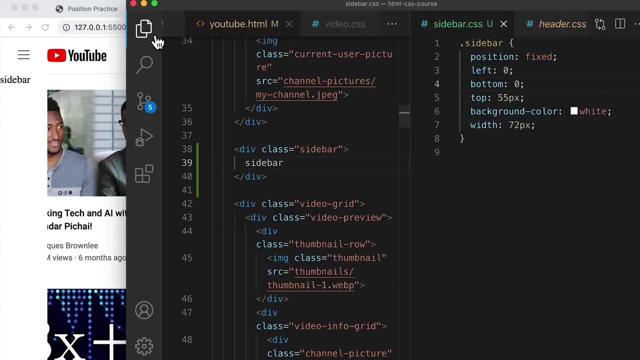 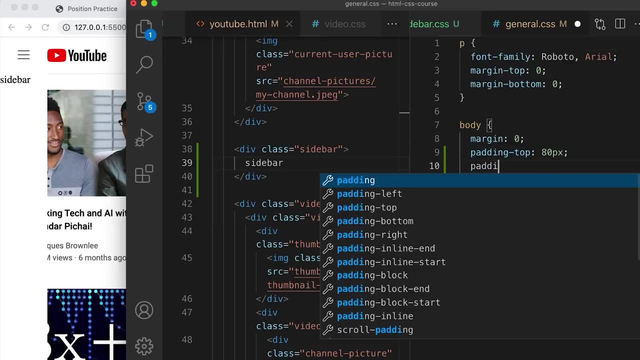 over. So let's go into our general styles, So generalcss, And we're going to style the body, We're going to add padding to the left of our body And let's add padding of 80 pixels again. And now our sidebar is: 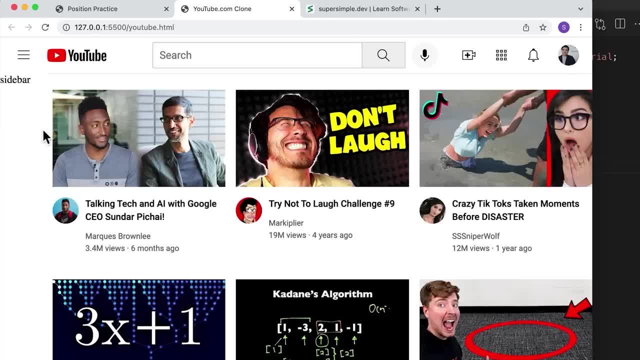 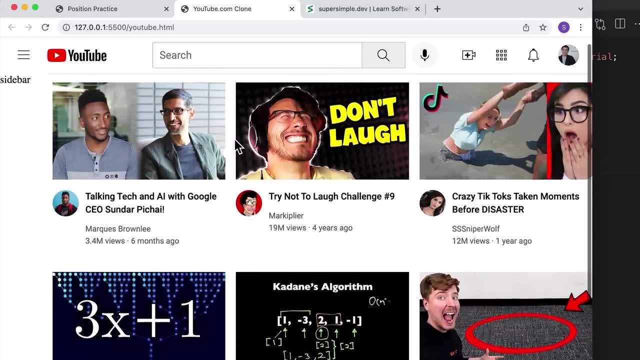 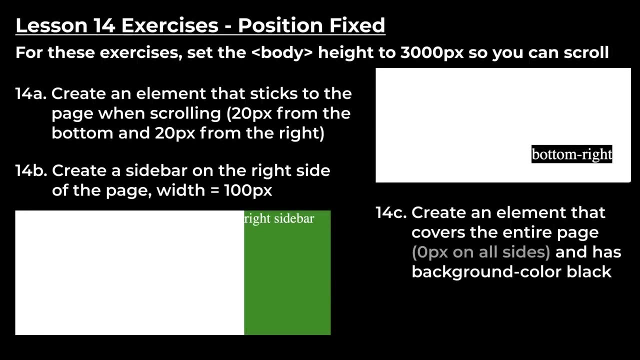 no longer covering our content because we added a bunch of padding to the left of our page. So that's how we use position fixed: to create elements that stick to the page while we scroll, like our header and our sidebar. For now, here's some exercises that you can do on your 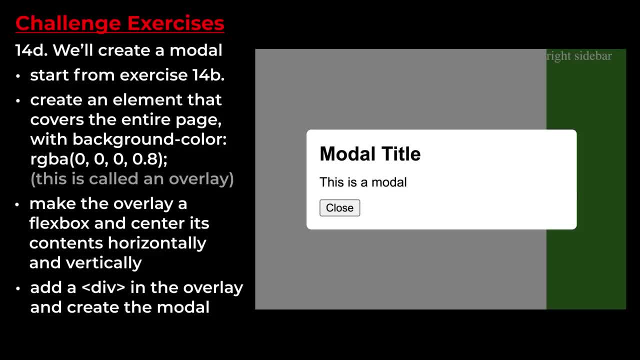 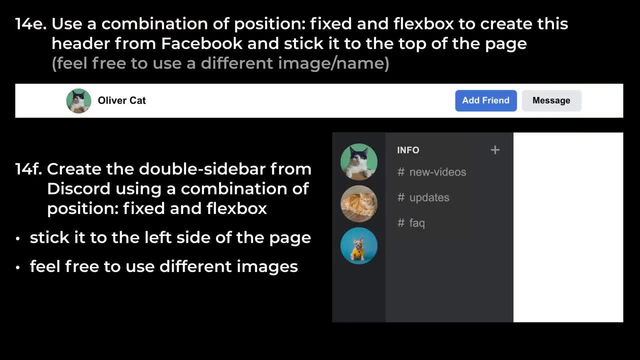 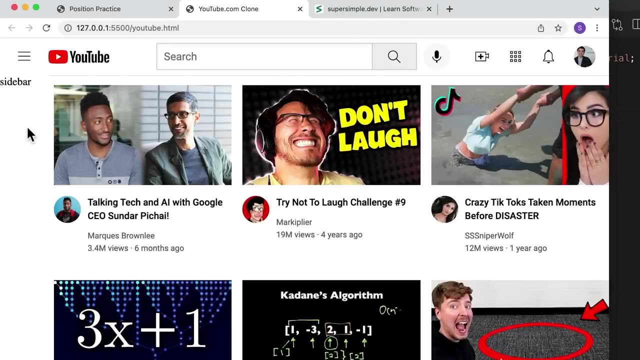 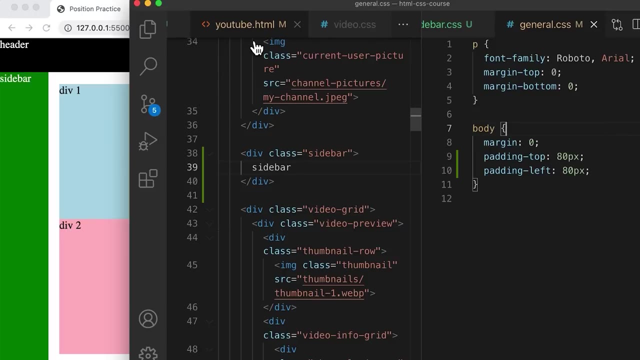 own to get a better understanding of CSS position. Now we're going to learn another position property that we can use. Let's go into our position practice file and the same in our code editor. We're going to open up positionhtml and then close all of these files. 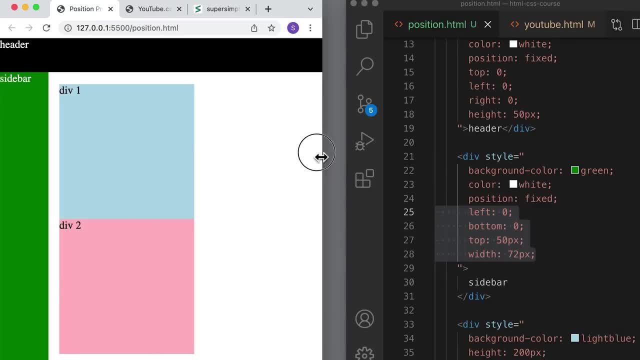 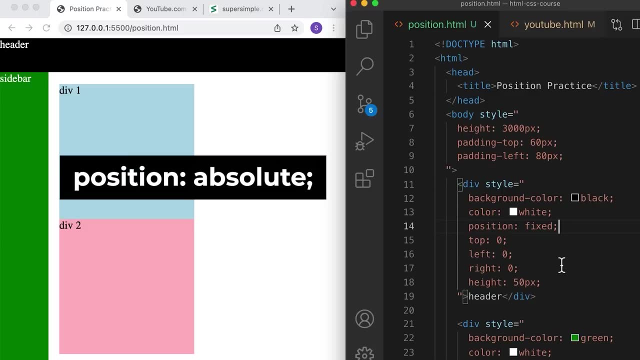 I'm going to resize it so that we can see it better. So this time we're going to learn position absolute. Let's do an example to see how it works. So let's scroll down and we're going to create a div below our sidebar. 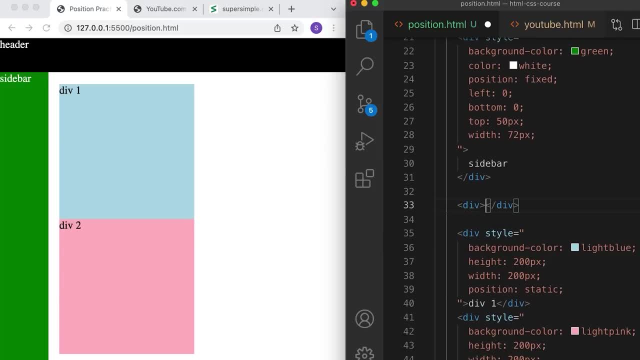 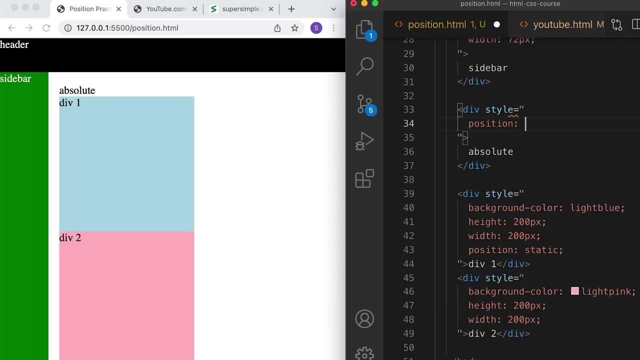 to practice position absolute. Let's create a div and then let's call this absolute, And now we're going to set some styles on this div, So style equals, and then inside here we're going to set position with a value of absolute. 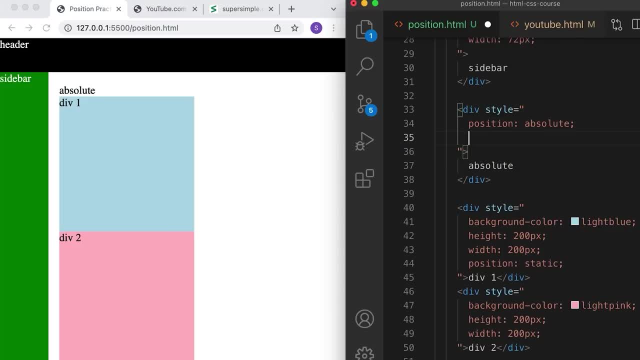 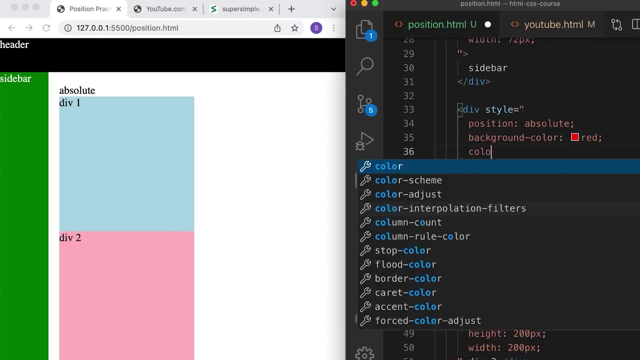 And we're also going to set a background color of red so that it's easier to see. So background color of red, and then the text color is going to be white. So color of white. Save it. And now we have our position. absolute element. 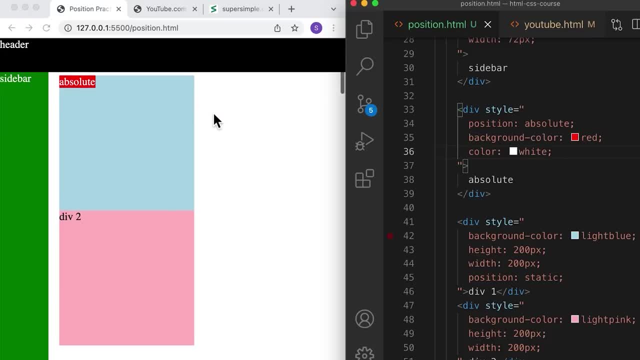 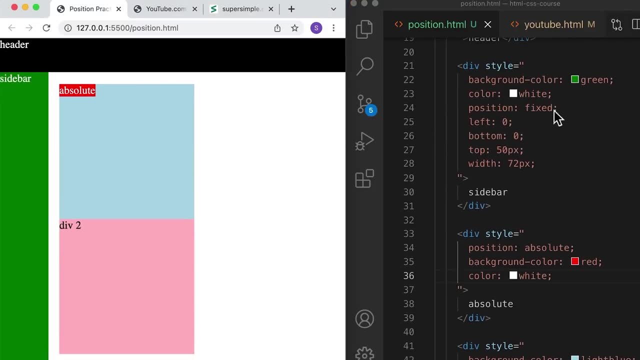 So, before we continue, make sure we scroll all the way up to the top of our page. Now. position absolute also takes the same values as position fixed. So top, left, bottom and right, as well as width and height, But they behave a little bit differently. 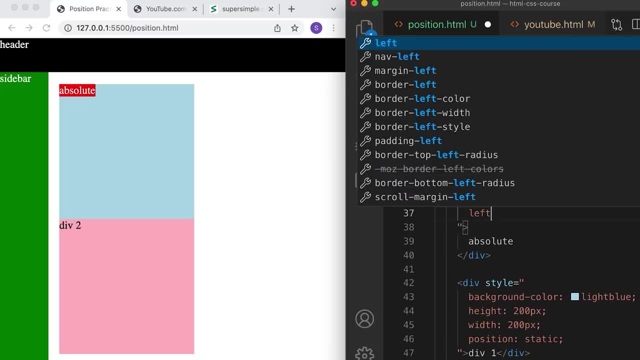 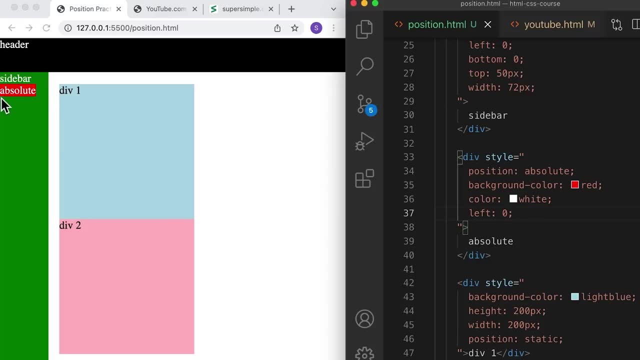 So first we're going to set left, So let's set the left property to 0. And let's save it. And now the left side of our element is 0 pixels from the left side of our page. So this works the same way. 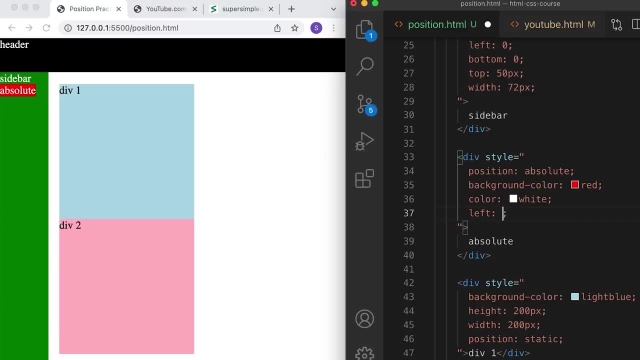 as position fixed. If we set left to 10 pixels now, there will be 10 pixels between our element and the left side of our page. Now let's try setting top. So we're going to set the top to 10 pixels. 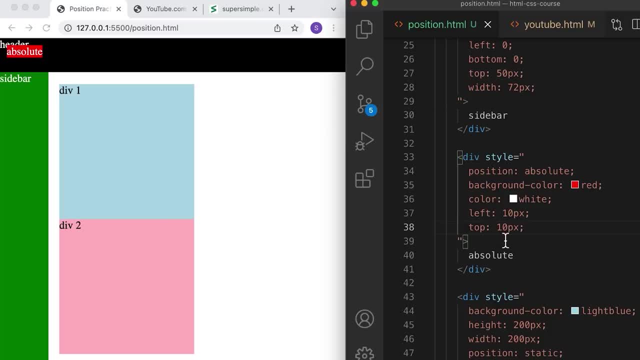 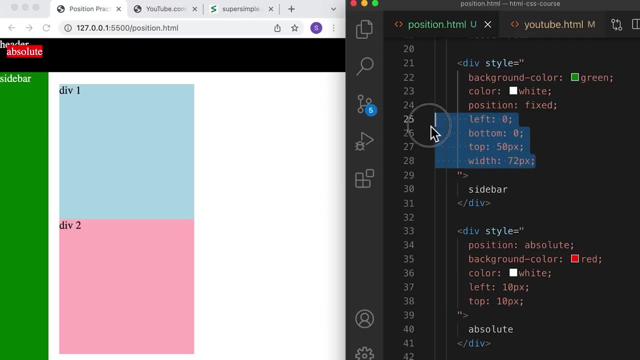 Save it and make sure you scroll all the way up So you'll notice that our element is now 10 pixels from the top of the page. So mostly these properties work the same as position fixed, but with one key difference. For position fixed, the elements are: 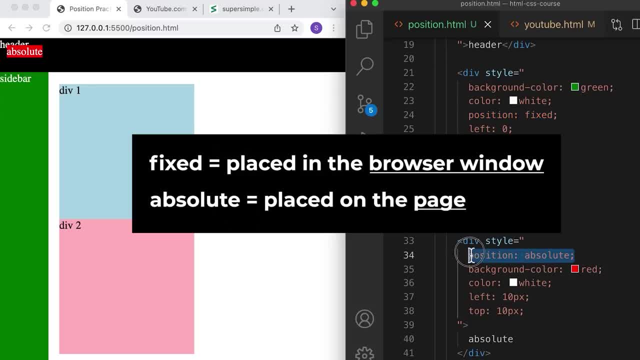 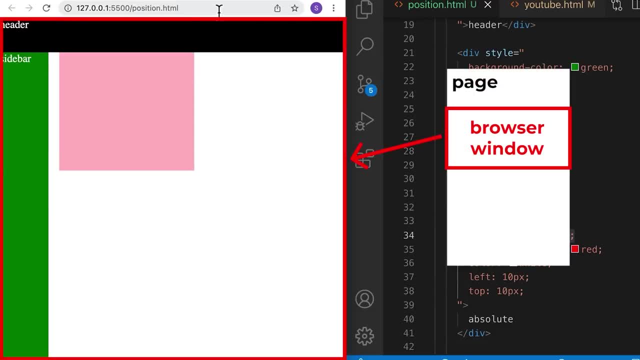 placed in the browser window, While for position absolute, the elements are placed on the page. Now, what I mean by this is that when we scroll the browser window, or just this visible part is not moving, Only the page is moving up and down. 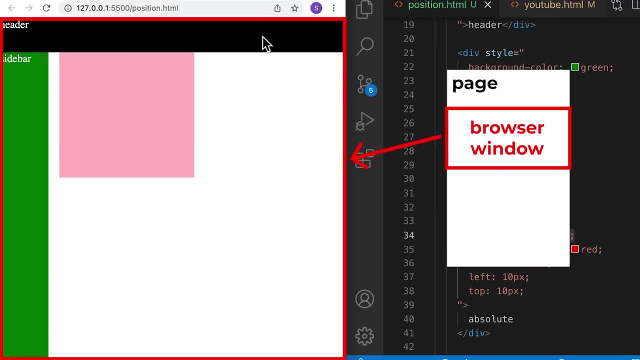 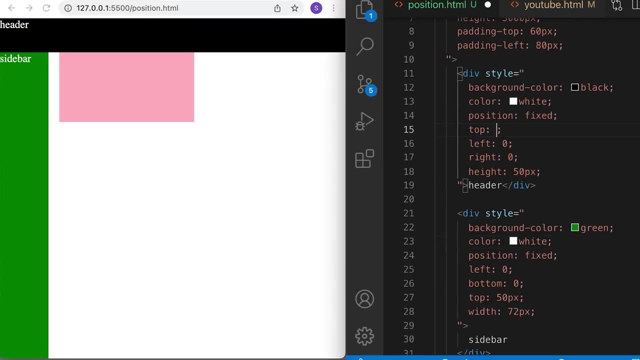 So for position fixed, we're going to put these elements on the browser window, which doesn't move when we scroll. So if we scroll up to the header, if I say top and 10 pixels, this puts the header 10 pixels. 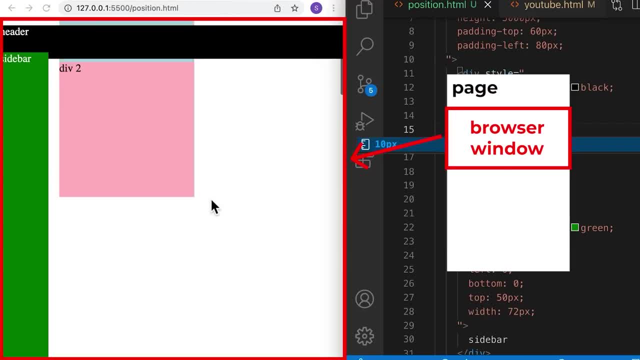 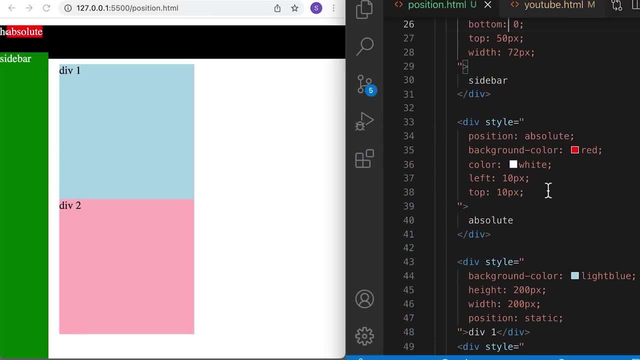 from the top of the browser window, not from the top of the page which is constantly moving up and down, But for position absolute. if we scroll down to there, we're putting it 10 pixels from the top of the page, which scrolls up and down when we move. 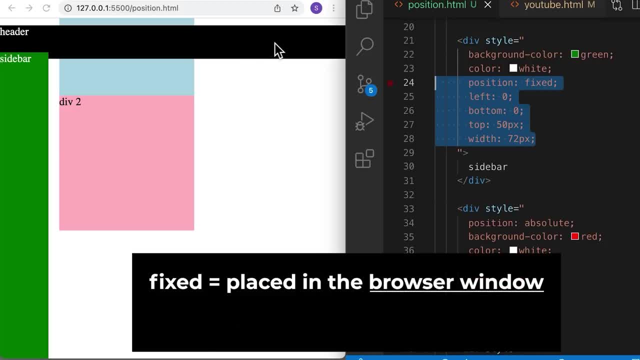 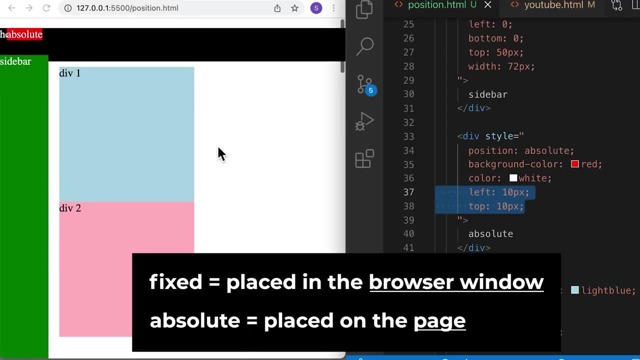 So that's the key difference between the two Position fixed positions, the element in the browser which doesn't move when we scroll, and position absolute positions, the element on the page which does move when we scroll. So let's go back up and 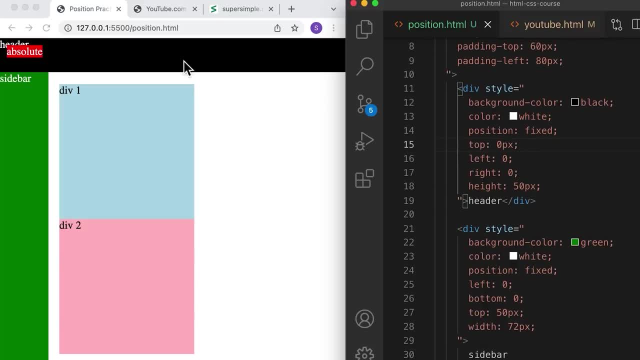 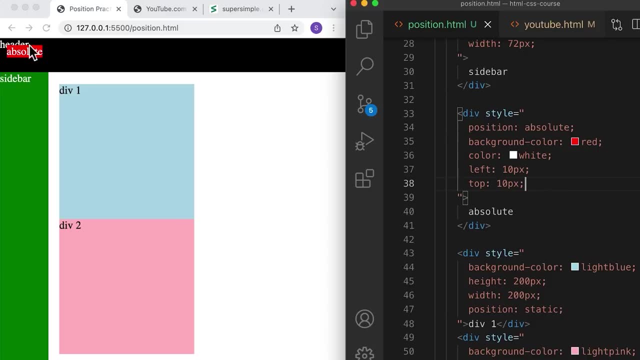 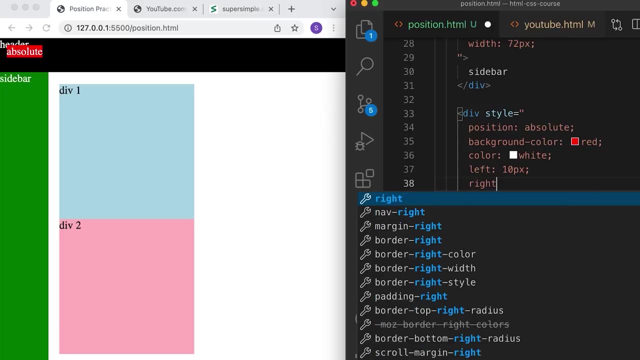 reset this to 0, so that we have our proper header again and do some more practice with position absolute. So, for example, if I wanted to put this absolute element in the top right corner here on our page, we can do something like write: 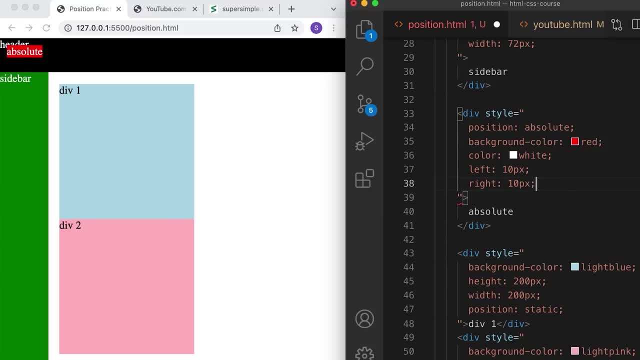 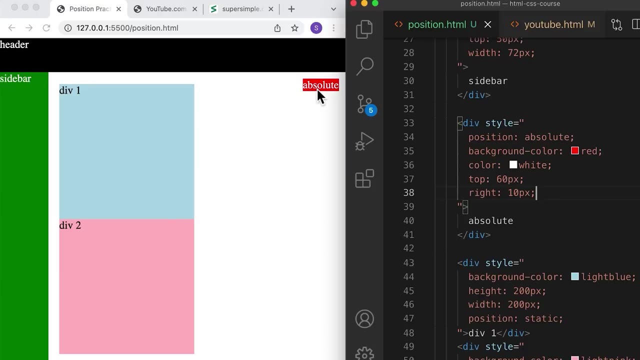 and we'll put it 10 pixels from the right and then top. we can put it maybe 60 pixels from the top, So 60. Save it and we scroll all the way up and that's how we place an element on a precise. 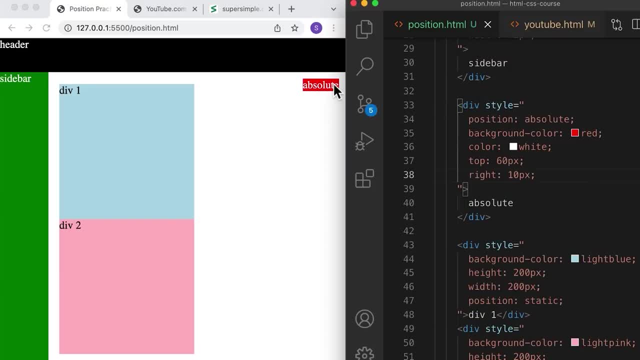 location on our page like this, And because it's on our page, when we scroll, the page will move up and this absolute element will move up with the page. Now, one thing that's weird is that this element is appearing above our header. 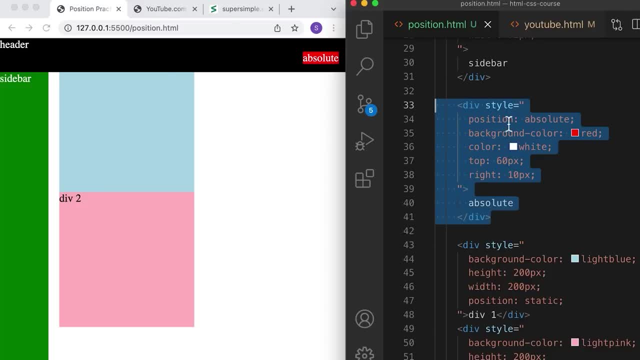 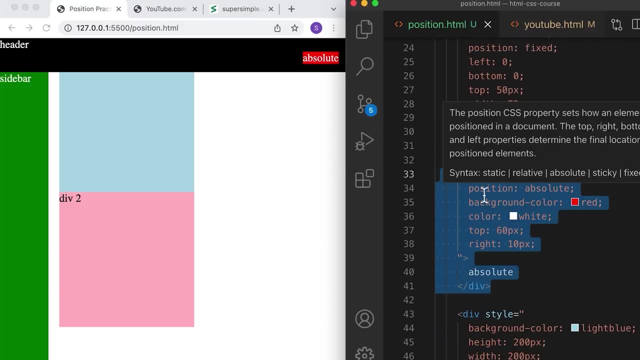 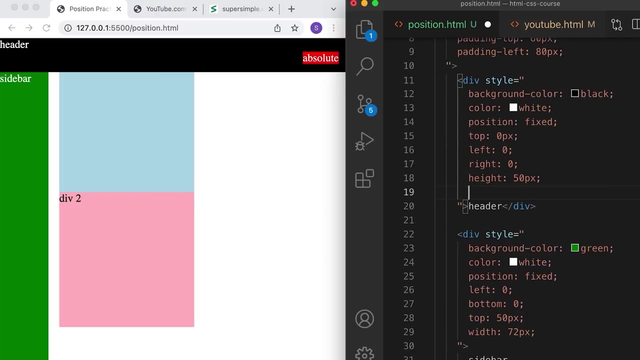 And that's because this element was written in our code below our header. So generally, an element that is written below is going to appear in front of elements that are written above it. Now we can actually override this if we scroll up, by adding another property called 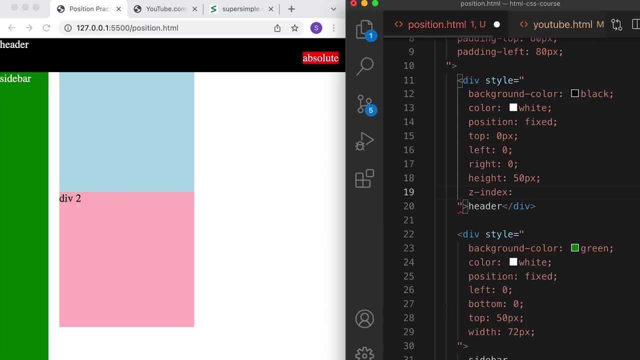 z-index. So z-index determines which elements appear in front and which elements appear behind. So the default z-index is 0. This is the same thing as if you didn't have this at all, But an element with a higher z-index will appear in front of elements. 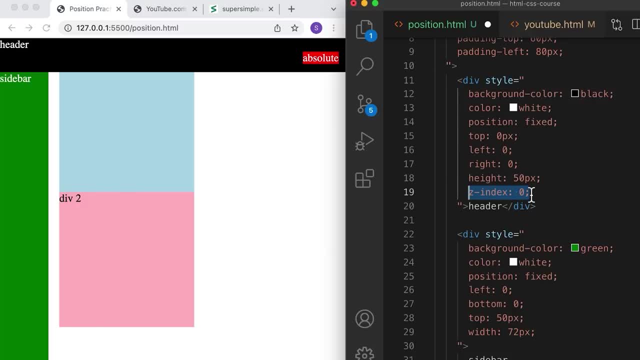 with a lower z-index. So if we set the z-index of the header to 1, it's going to have a higher z-index than the absolute element, which has a default z-index of 0.. If we save it now, the header will appear in front. 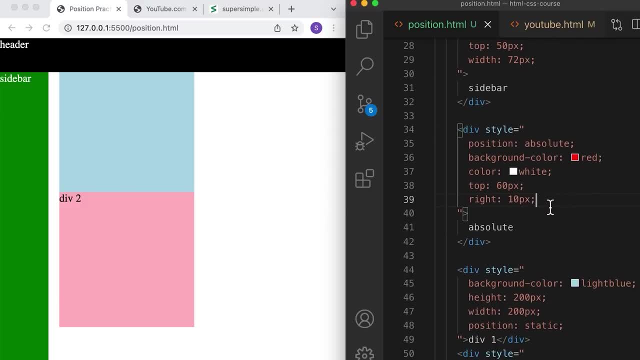 Just as an example, if we scroll down and we set the z-index of this absolute element and we set it to 2, now it's going to appear in front again because our z-index here is greater than our z-index here. 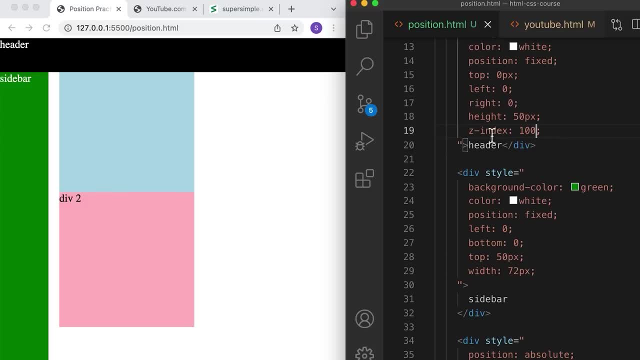 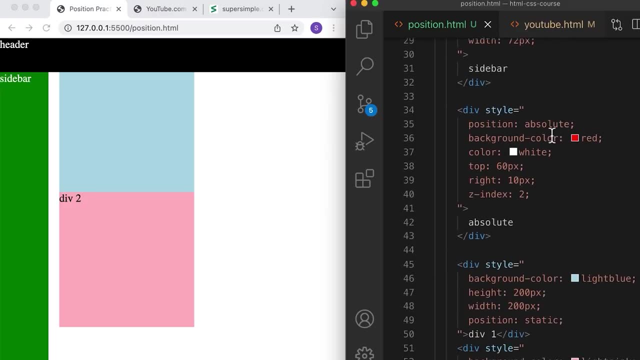 So usually we set this to something like 100, so that we can have a lot of elements in between. if our page has a lot of layers, And usually if we don't care about the z-index, we can just remove it and have a default of 0.. 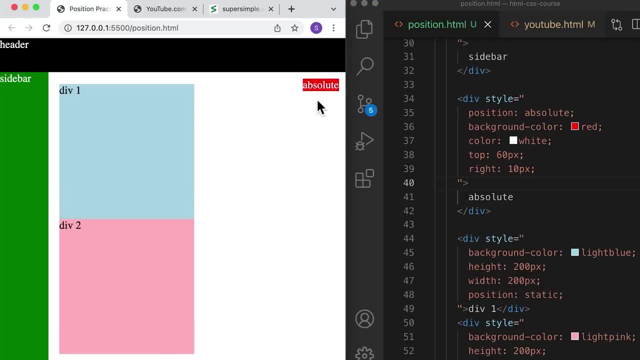 Now that we learned position absolute, where do we use this? The truth is, we don't use it like this very much. This is not a common situation that we run into when we're creating websites. However, position absolute has another key feature that makes it really really useful. 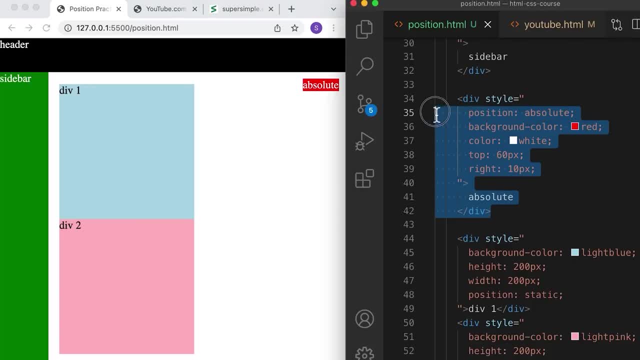 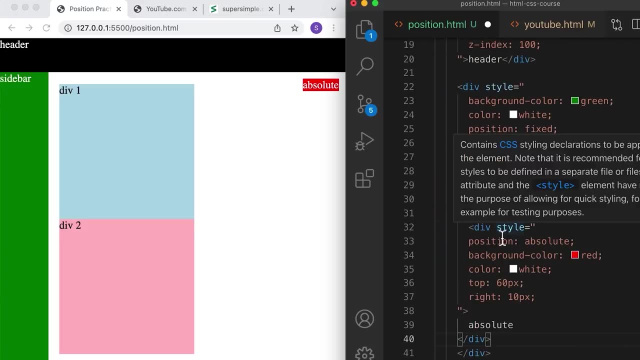 To demonstrate, we're going to take this element and we're going to make a copy of it and we're going to put it inside the sidebar, So like right here. So we're going to put a position absolute inside a position fixed. 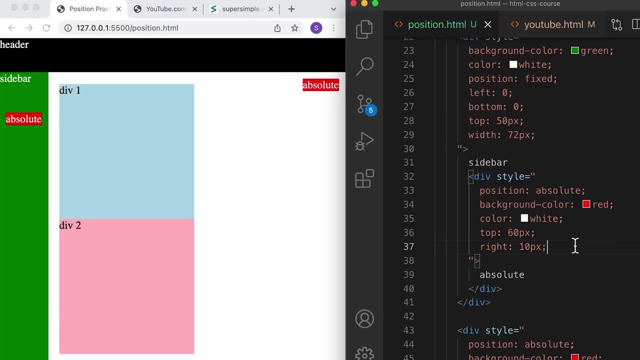 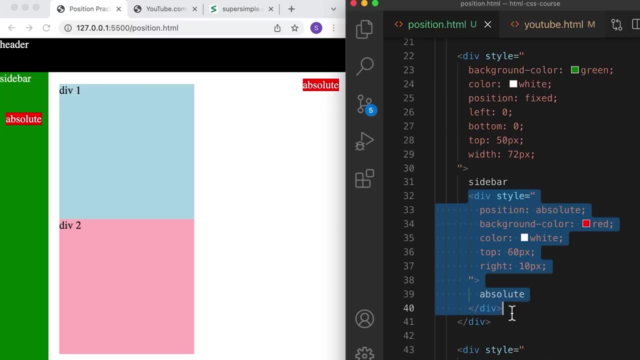 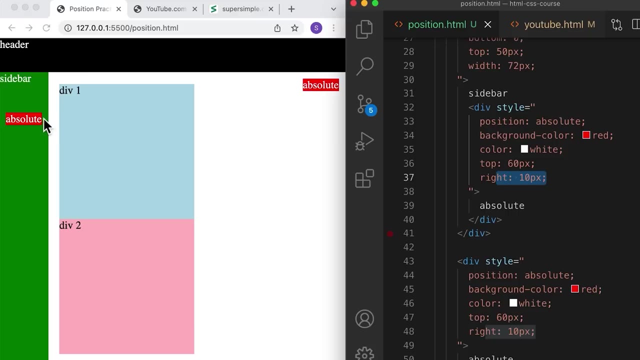 So now, when we save, you'll notice that this element is not being placed on the page anymore. What it's actually doing is placing this element relative to this position: fixed element. So now, right of 10 pixels is actually 10 pixels from the right. 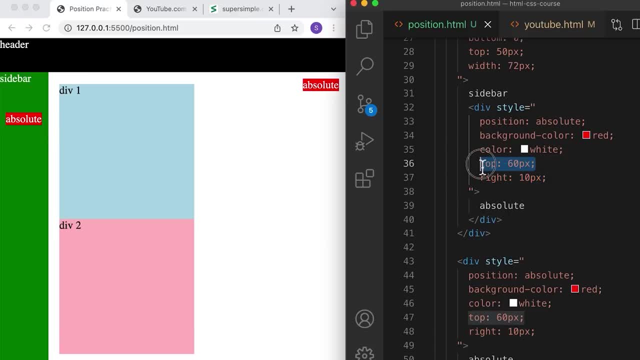 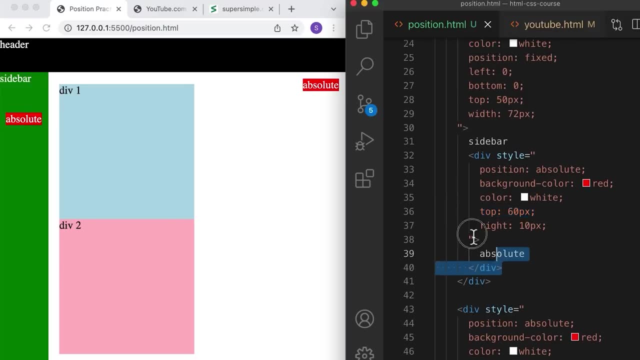 of the fixed element, which is the sidebar Top of 60 pixels is 60 pixels from the top of the sidebar, not from the top of the page. So whenever position absolute is inside a position fixed element, it's going to be placed relative. 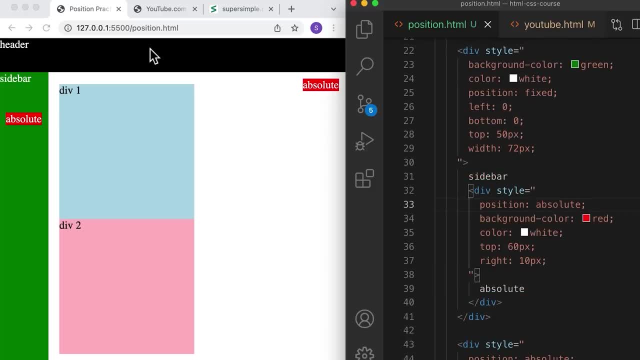 to this position fixed element. So this is the most important feature of position absolute. So let me show you why it's so useful. Let's say that we wanted a close button on the top right of our sidebar. We want to be able to. 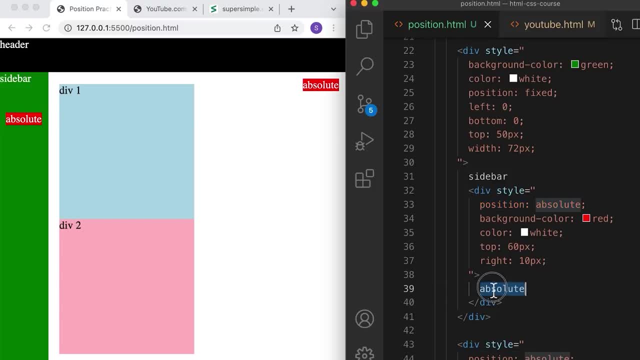 close our sidebar. if we want to, I'm going to change this to an X so that it's kind of like a close button, And then to put it in the top right of our sidebar. we just have to set the top to 0 and the. 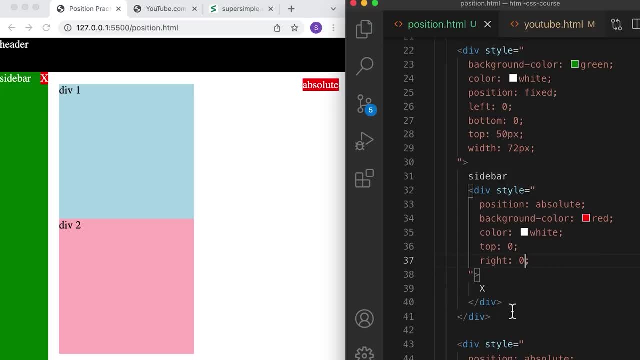 right to 0. So if I save that now this element is in the top right And that's because if position absolute is inside position fixed, top 0 means 0 pixels from the top of the position fixed element Right 0. 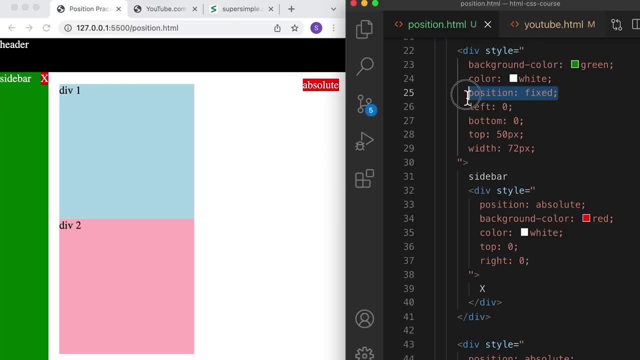 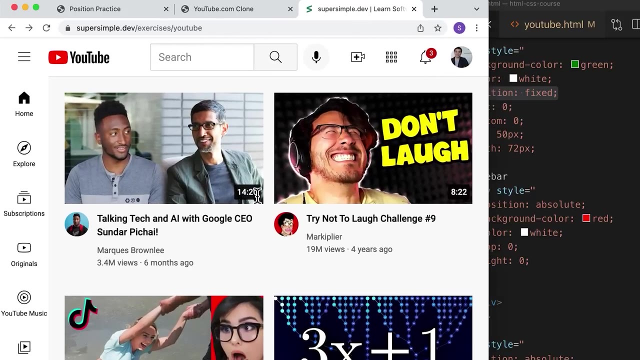 means 0 pixels from the right of the position: fixed element. So this is how we attach elements to the corners or the sides of other elements. If we look at our final project, we can see that going on in our videos. Here we have the video time in the. 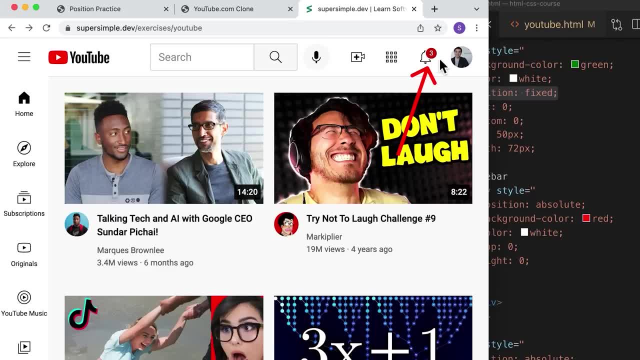 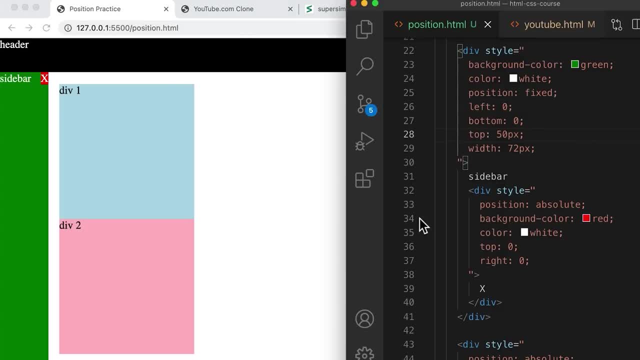 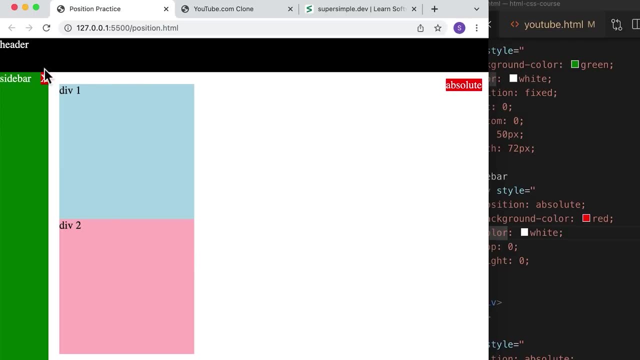 corner of our thumbnail. Here we have the notification count in the top right corner of this icon And, using position absolute, it allows us to put elements in the corner like this. So there's one last thing we need to learn. Here we have 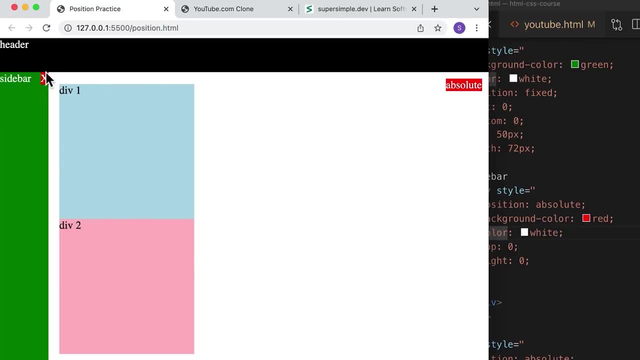 a position absolute inside a position fixed element. That's why we can put it in the corner But notice that this is still a position fixed element and it sticks to the page. But in our final project these videos are not sticking to the page. 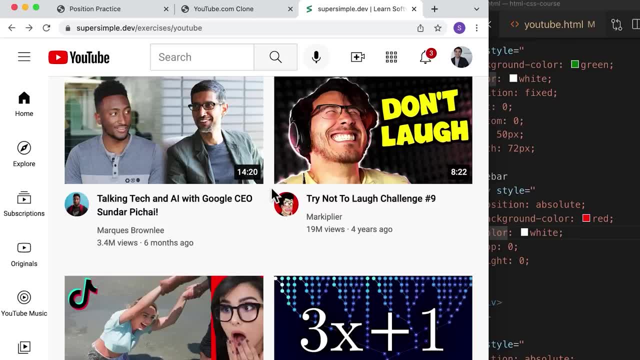 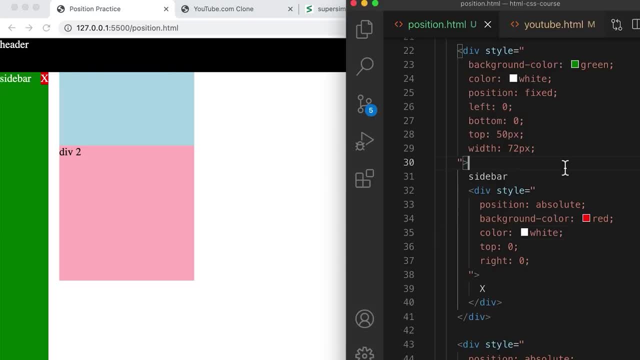 They're scrolling with the page and we're still able to put stuff in the corners. So how do we achieve this? And to do this, we're going to learn another value for the position property, called position relative. We're going to scroll down. 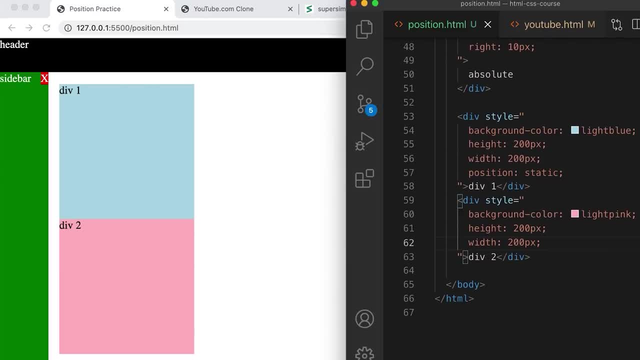 to our two divs at the bottom, and for our second div, we're going to set the position to relative and save it. Now, if we go back to our page, we'll notice that nothing actually changed, And that's how position relative works. 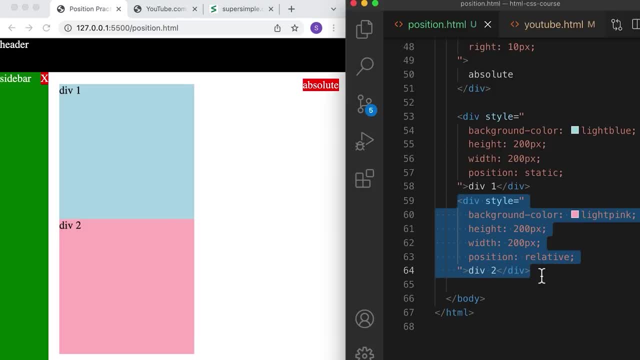 It still displays the element as normal, except if we put position absolute in here, it will position it relative to this element instead of relative to the page. So let's go through an example to see what I mean If I scroll up here. 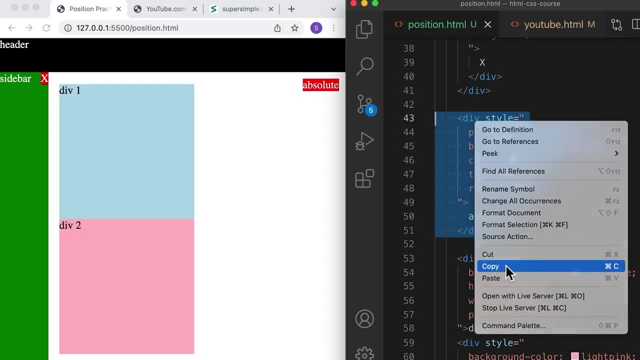 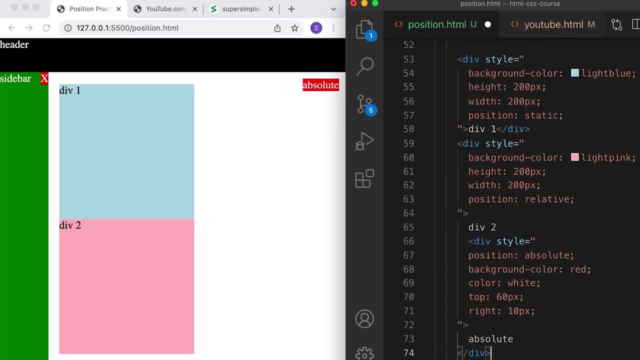 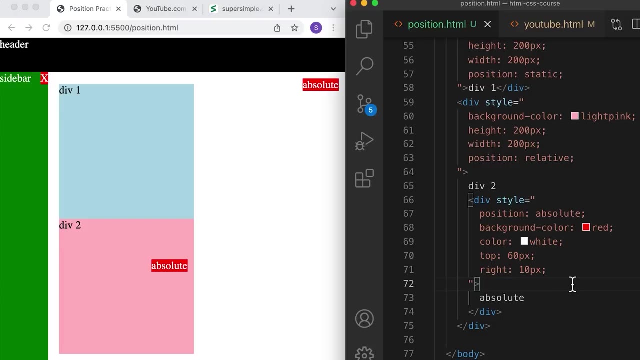 let's copy this absolute element. Let's copy it And then paste it inside this position: relative element. Save it And then reformat it a bit. Press tab, And if we save this, you'll notice that we get the same effect. 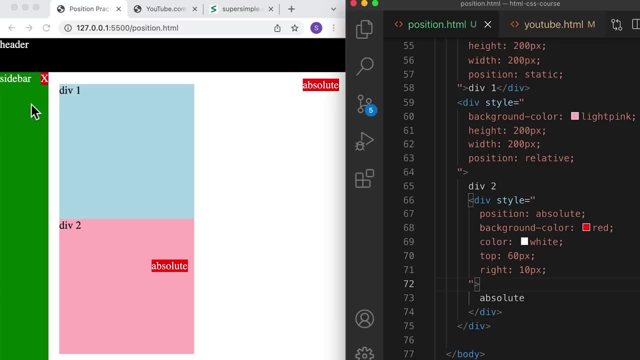 as when we put position absolute in position fixed. Right of 10 pixels now means 10 pixels from the right of the position relative element, Not 10 pixels from the right of the page. Top of 60 pixels means 60 pixels from the top of the. 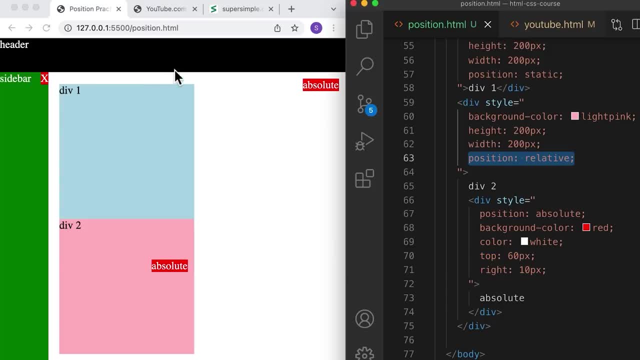 position relative element, Not 60 pixels from the top of the page. So two things are happening here. When position absolute is inside position relative, this will be positioned on the element, not on the page. So that's what we just talked about. 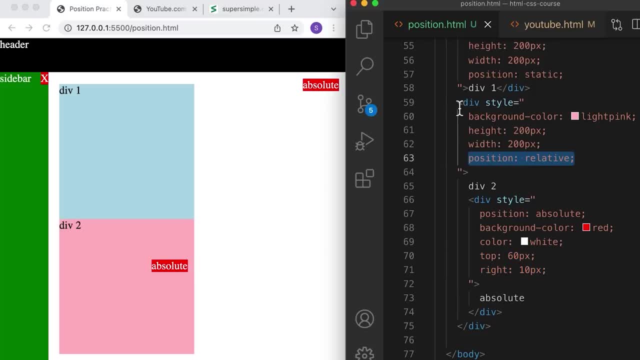 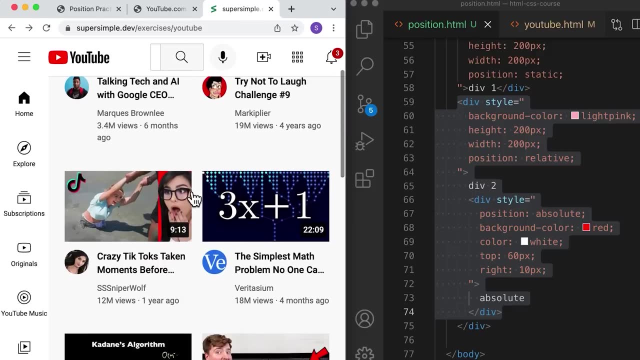 The second thing that happens here is that position relative causes this whole element to display normally. So that's what we get in our final project. Notice that these videos are displayed normally. They scroll with the page, But we have something in the bottom right corner. 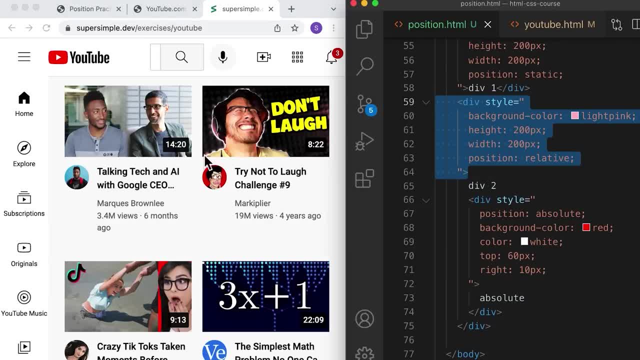 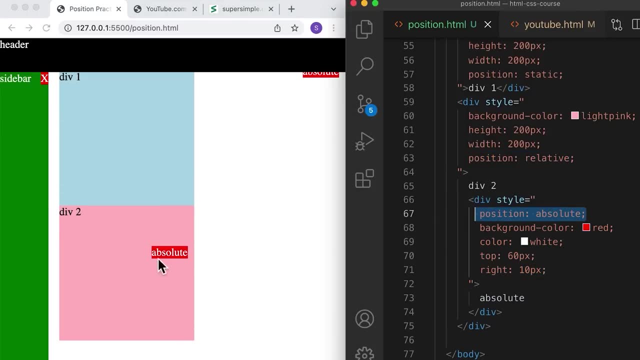 So these are all position relative, And then to put something in the bottom right corner, we're going to put a position absolute inside. So let's actually go through an example here. So we have our position relative element, We have position absolute inside. I'm going to put this: 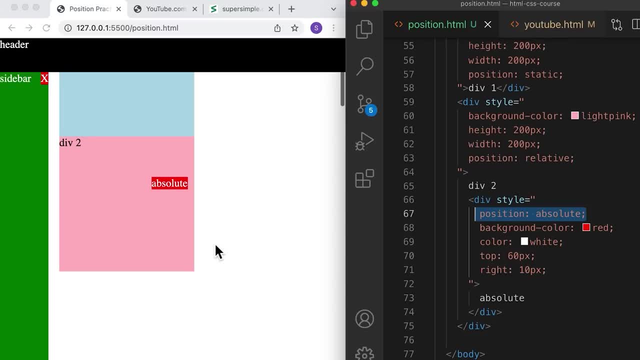 in the bottom right corner, just like our design. So let's change this to 5 minutes And pretend this is like our final project. Let's change the background color to black, And now we're going to put this on the bottom right corner, So let's. 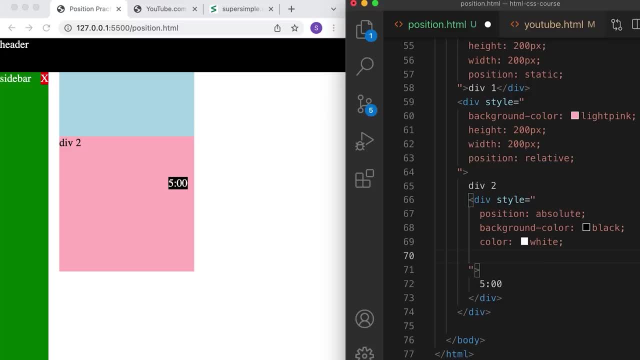 get rid of this first And we're going to put this 10 pixels from the bottom of the position, relative element. So we're going to say bottom 10 pixels And we're also going to put it 10 pixels from the right of this position relative element. 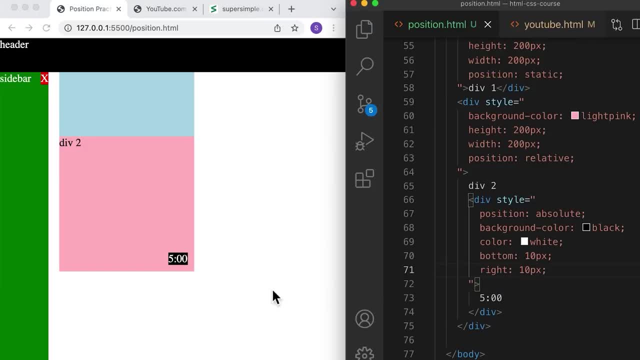 So right of 10 pixels, And that's how we position this in the corner. And because this is position relative, if we scroll the page it acts like normal content. So now that we learned the technique of position absolute, inside position relative, we're going to apply 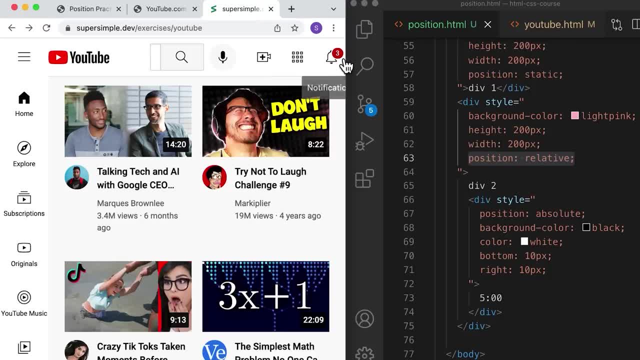 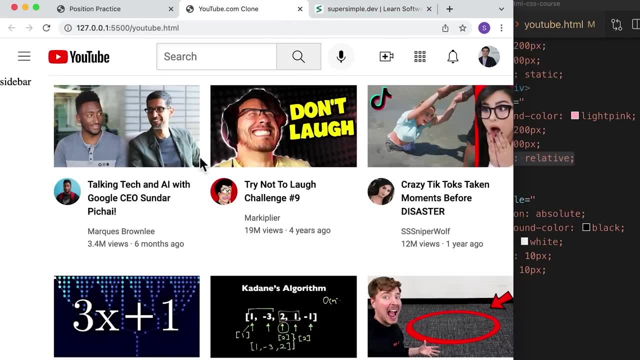 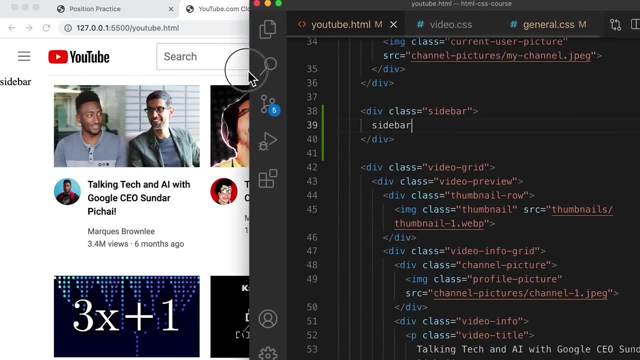 that to our project and create the video time As well as the notification number here. So let's go back to our project And we're going to add video times first. So let's go to youtubehtml And we're also going to open. 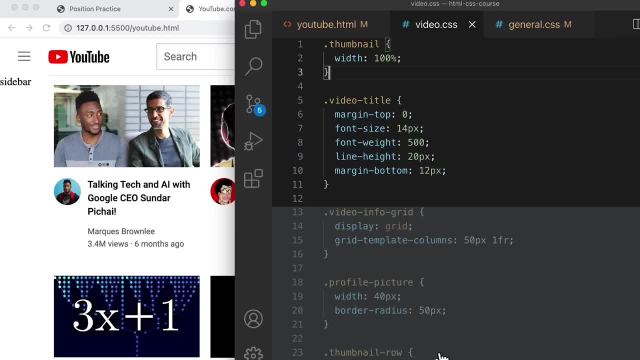 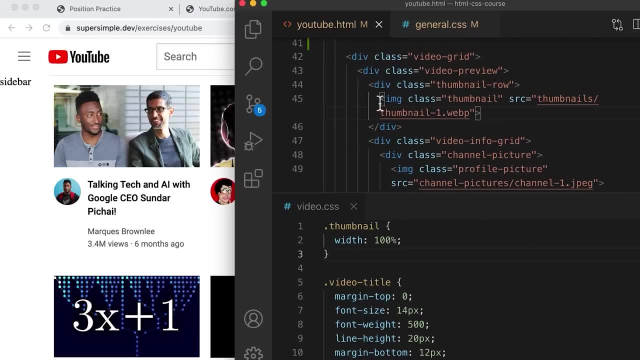 the videocss file. I'm going to put it down here Because we're working with styles for the videos. So first we're going to find our thumbnail, Which is right here, And now remember to put something in the corner We're going to need. 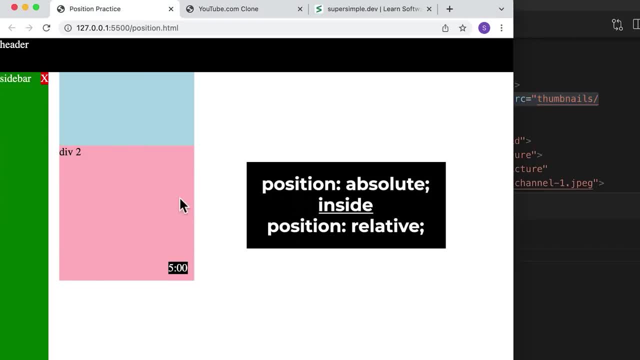 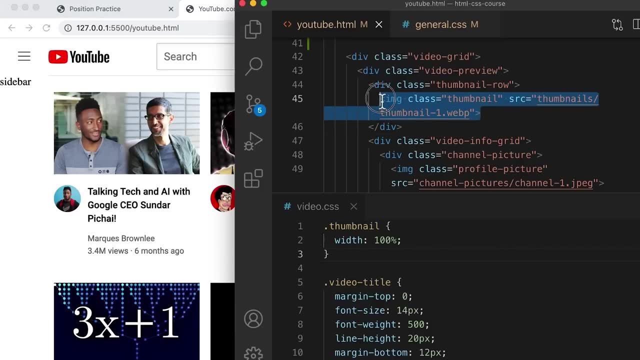 position absolute inside a position relative element. So if we look at our code, what could be our position relative element? Well, it can't really be the image element, because image elements aren't really containers. We can't put something inside it. So what we could use is this thumbnail: 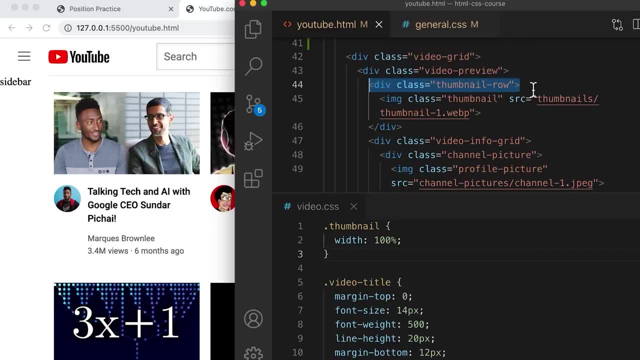 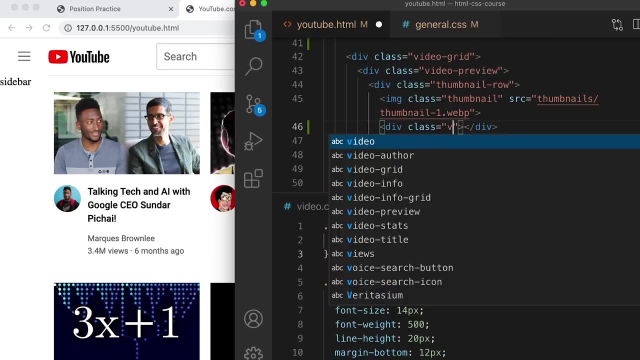 row element. This could be our relative element, And then the video time will be the absolute element inside of here. So first let's create our video time. We're going to create a div And let's give it a class of video: dash time. 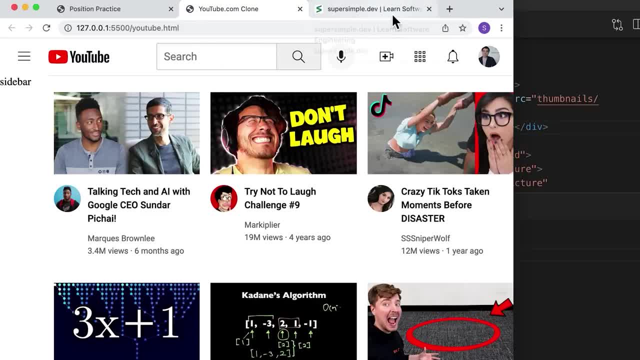 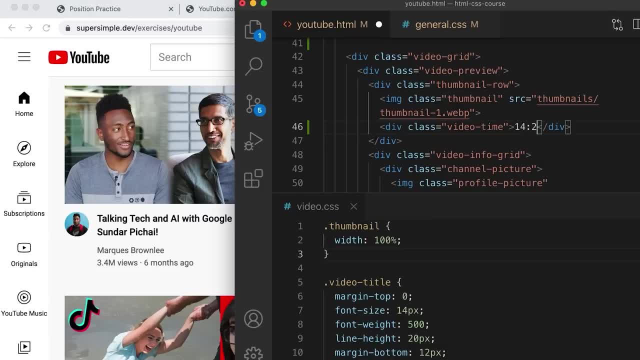 And then inside we're going to put a video time. So let's go to our final project And we're going to copy one of these, So 1420.. And inside I'm going to put 14, colon 20.. Let's save it and go back. 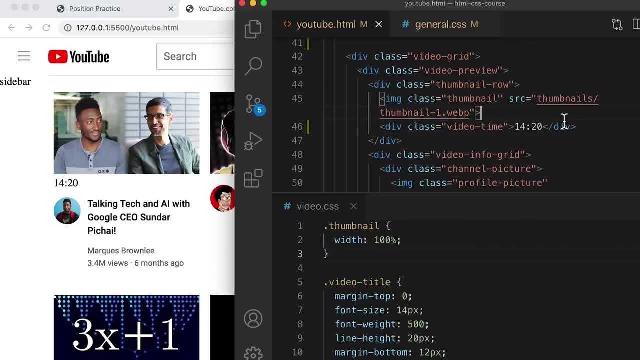 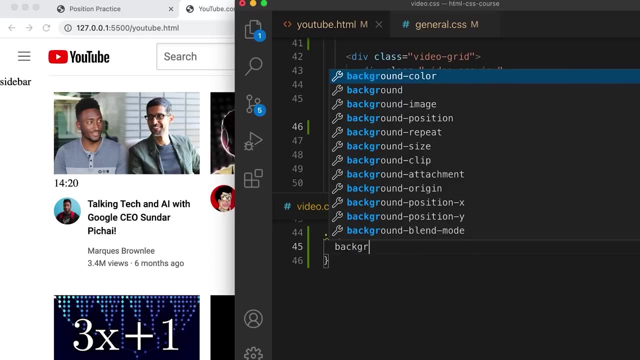 So right now it's just a normal div. Let's go to our css file And we're going to style this Scroll all the way down And we're going to target video dash time class And let's set the background dash color to black. 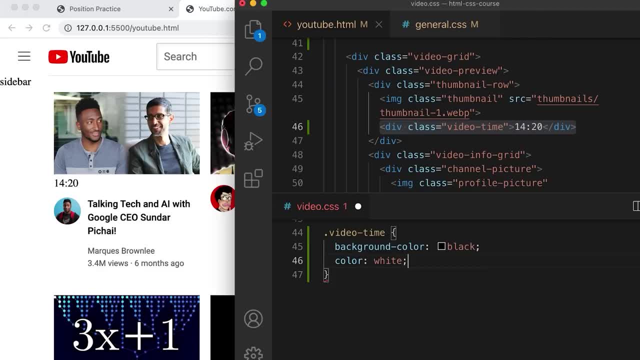 And the text color to white. So just like our final project. So now we're ready to position it properly. We're going to need position absolute inside position relative. So first let's set the position relative on here We're going to scroll up to. 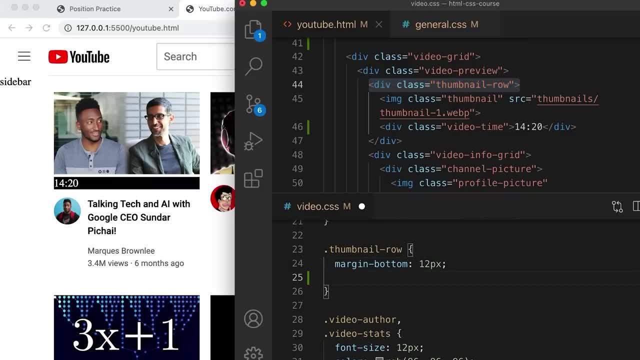 thumbnail row Just right here We're going to set position relative. And remember, position relative doesn't really change anything. Everything appears normal. That's one of the benefits of it, And if we scroll down, we're going to change this to position. 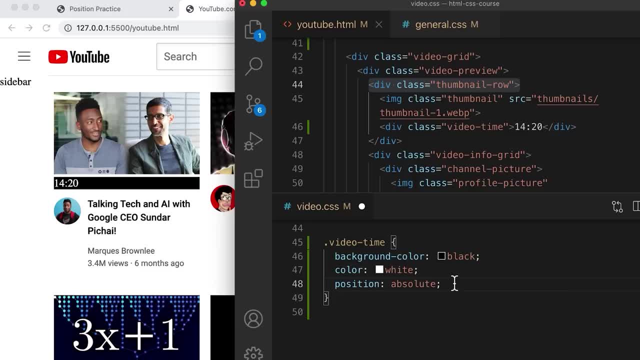 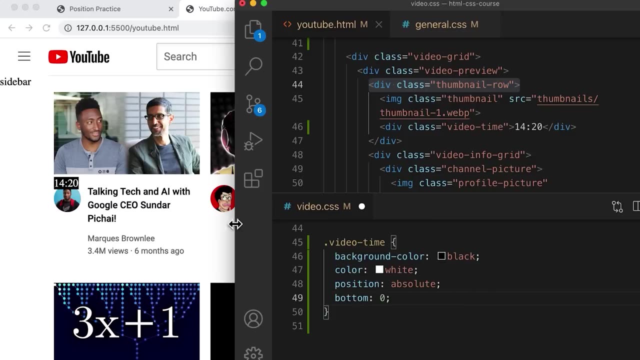 absolute. And now top, bottom, left and right will be placed inside our position: relative element. So if we save it, And now, if we want to put it in the bottom right corner, we just have to say bottom, 0 pixels from the bottom. 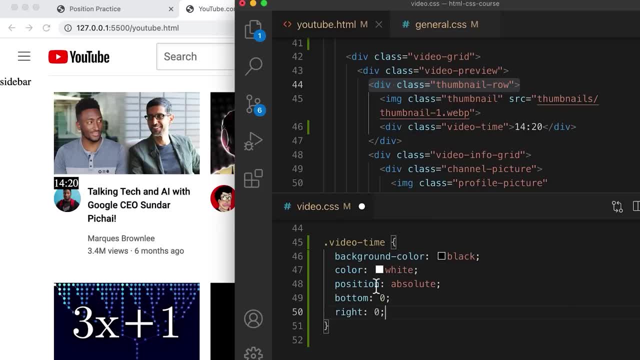 and also 0 pixels from the right. So let's set the position from the bottom to maybe 10 pixels- Save it. And let's set the position from the right side to maybe 5 pixels- Save it. Let's change this to maybe 8 pixels. 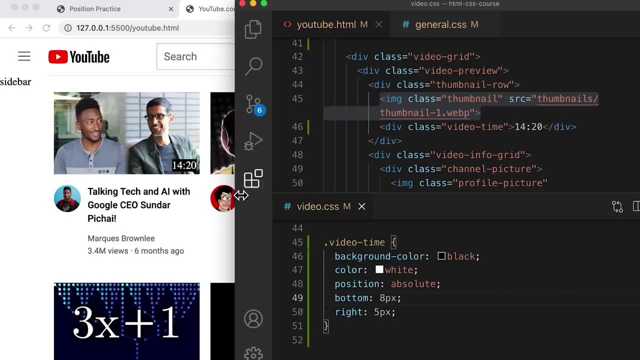 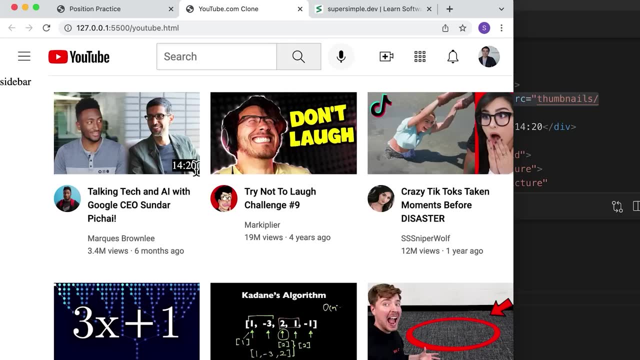 Okay. so I think that looks pretty good And if we compare it to our final design, it's in the right position. So that's how we put an element in the corner of another element. We need a position absolute inside a position relative. 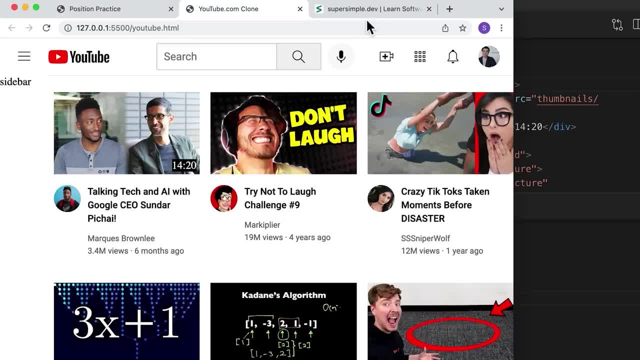 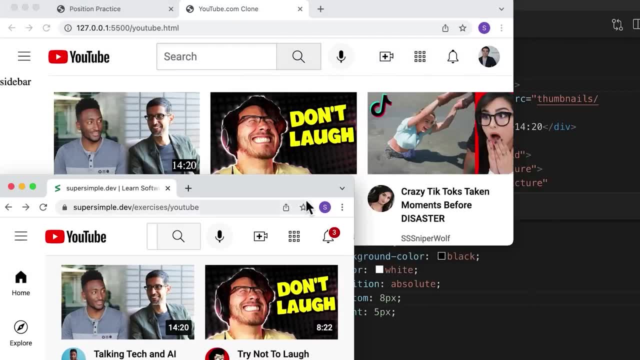 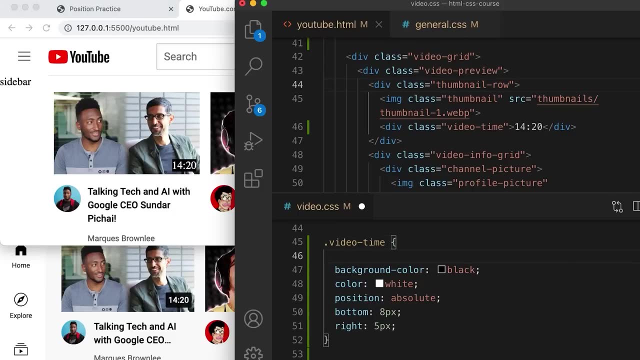 So, finally, let's style this one by one until it matches our design. I'm actually going to move this to the bottom here so that it's easier to compare. The first thing we're going to do is to change the font, So we're going to set. 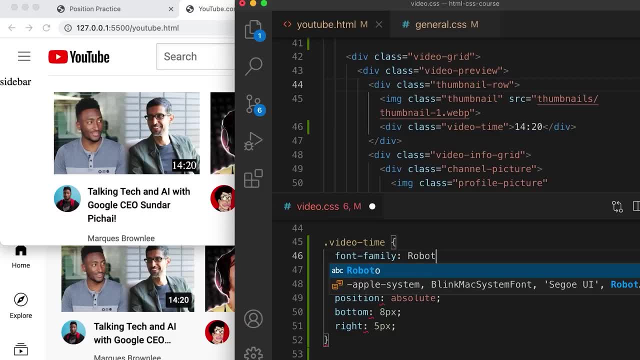 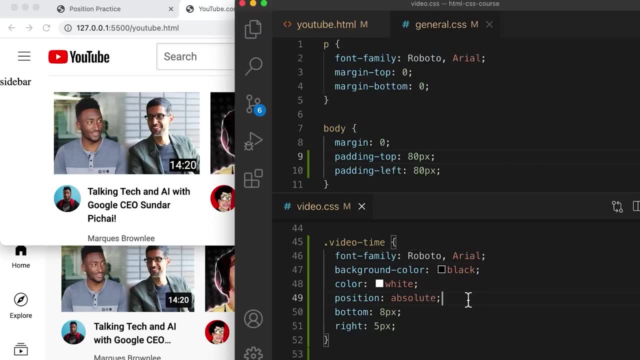 font-family to Roboto comma Arial, like the rest of our fonts. And next let's change the font size. Let's change it to font-size of maybe 12 pixels. Okay, that looks pretty good. Let's make it a little bit bolder. 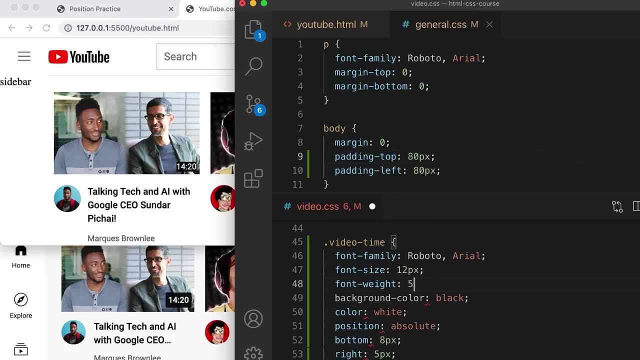 Let's change the font-weight to 500.. And remember, a font-weight of 400 is normal, 700 is bold and 500 is semi-bold. Let's save that. That looks pretty good. And next we need spacing on the inside. 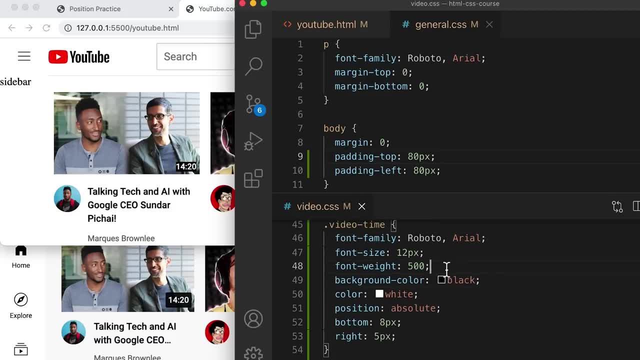 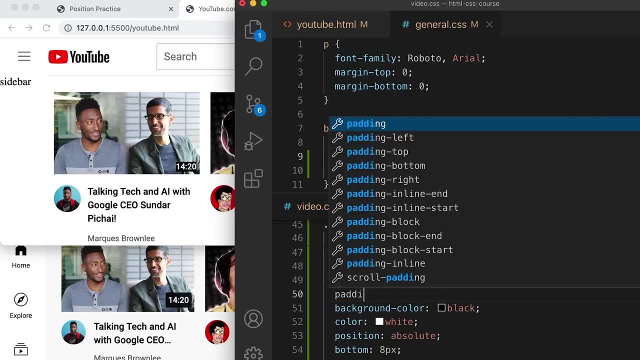 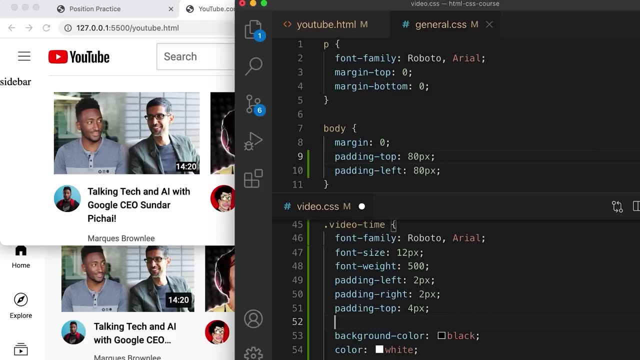 of this element. So that's padding. So let's add some padding on the left of maybe 2 pixels, And same for padding on the right- 2 pixels- And then padding on the top of 4 pixels And then padding on the bottom. 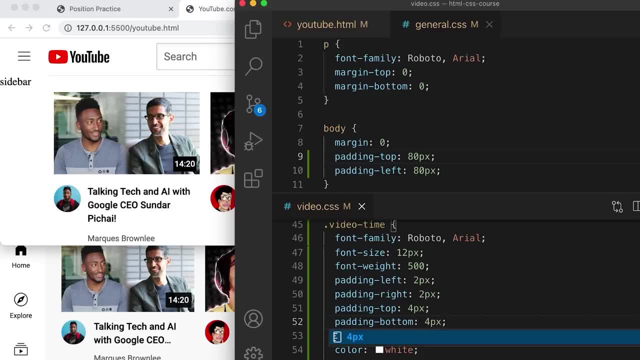 of 4 pixels. Save that. That looks pretty good. Let's add some more padding on the left and right. Change this to 4 pixels and 4 pixels. Okay, so I'm pretty happy with that. Next, we're going to make our corner rounded. 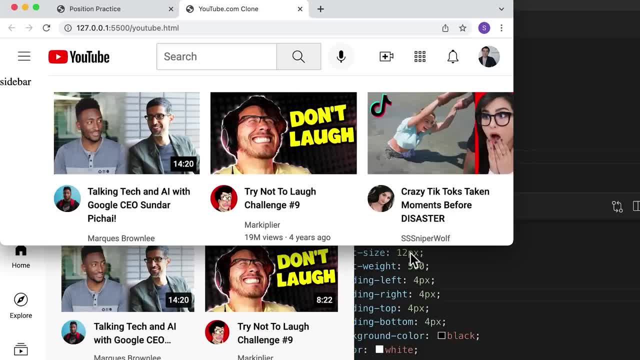 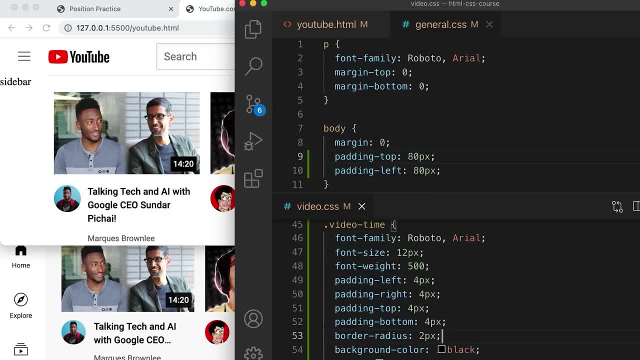 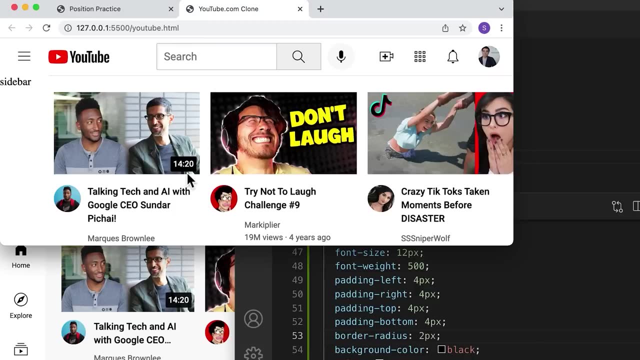 Kind of like this. So to do that, we're going to use border-radius, Change the border-radius to 2 pixels, Save it, And I think that looks pretty close to our design. And there we go. We created the video time in the bottom. 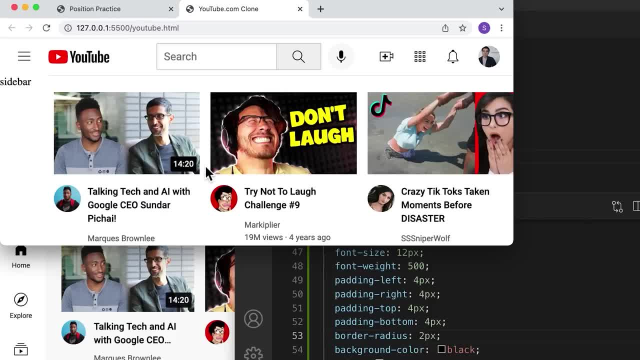 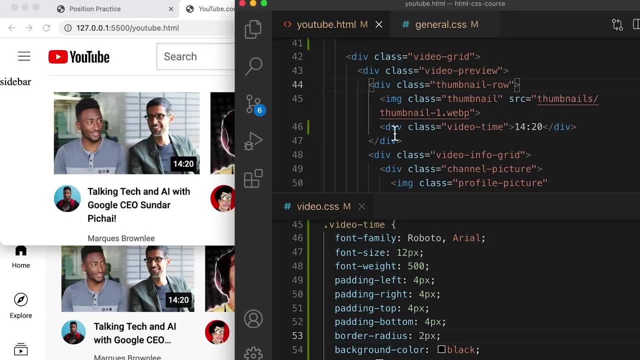 right corner of the thumbnail. Now, to give you guys a bit more practice, I'm going to get you to add the video time to all of our other videos. So inside our HTML, you're going to add this video time to the next video here. 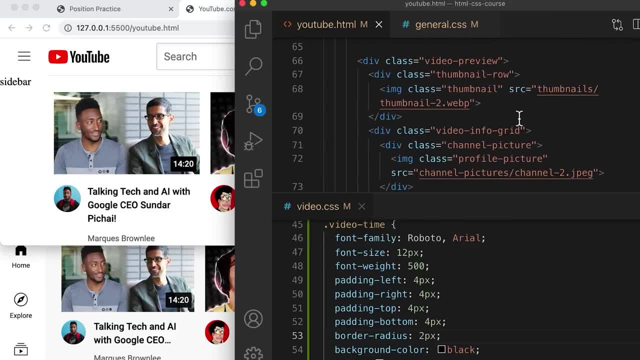 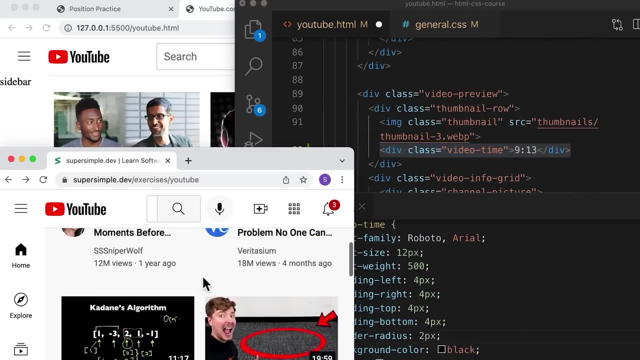 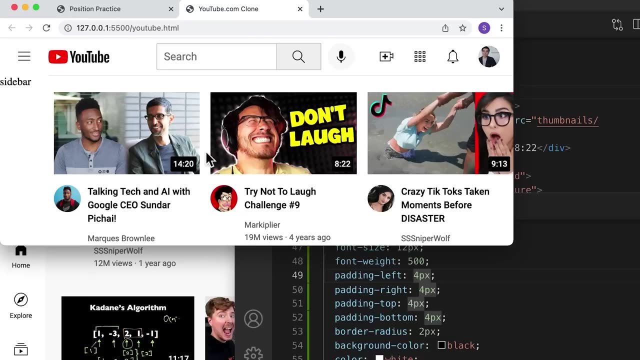 and all the videos in the HTML. So take some time to complete that and then we'll continue the lesson. So now that we have the video time for all of our videos, we're going to run into another problem If we start scrolling up. 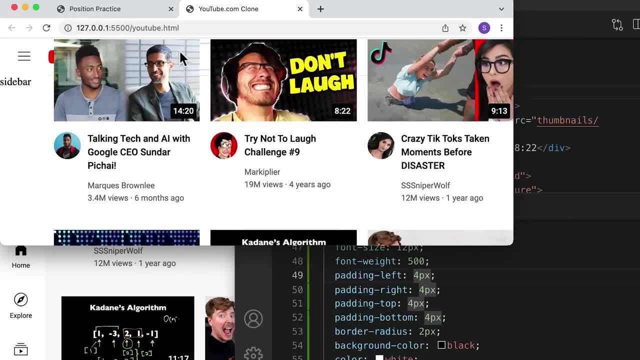 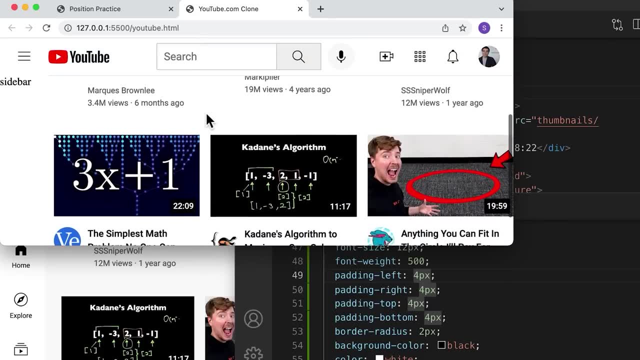 on this page, you'll notice that the thumbnails appear above our header, But another thing is that the other content, like this text and the channel image, will appear below our header. So what exactly is going on? So we mentioned this briefly in the practice file. 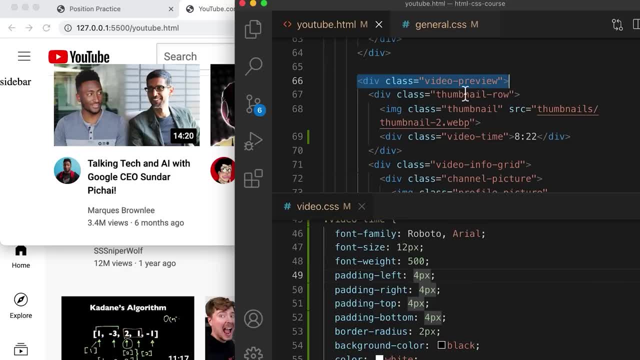 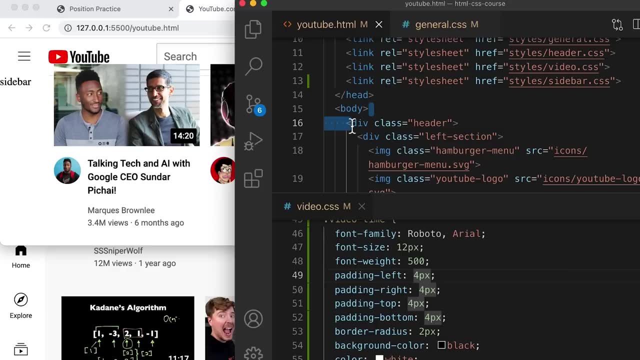 If an element like this video preview is written below another element like the header up here, the element that is written below will appear in front. That's what's happening here: We have a header and then below that we have the thumbnail which is going to appear on top of the header. 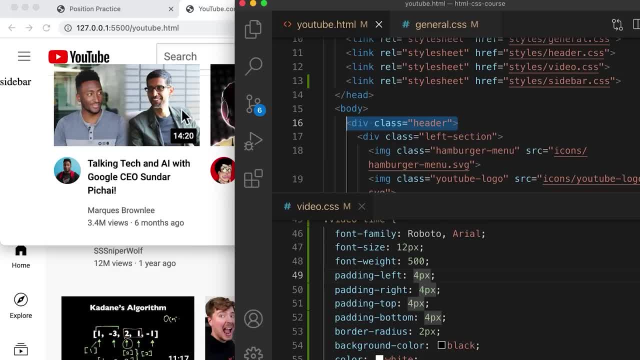 However, what I didn't mention is that this rule doesn't apply to position static or these elements with the default position. Position static will always appear at the back, So that's why you see that these always appear at the back As soon as we set it to something. that's. 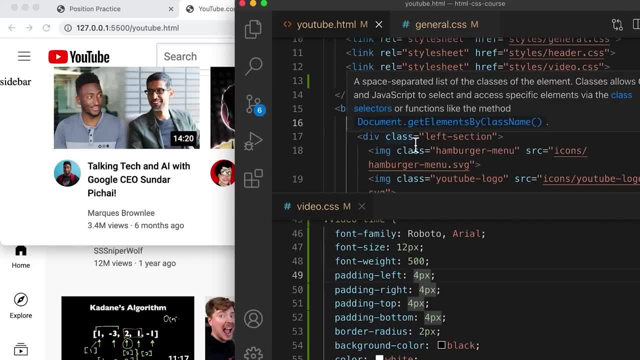 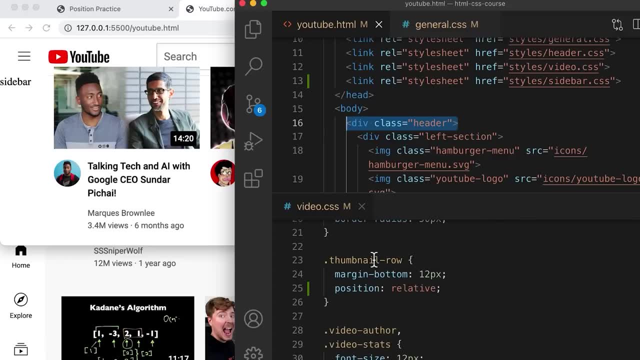 not position static. like position relative, the rules of which element was written first start to apply. So in this case, because if we scroll up the thumbnail row is position relative and it's written below the header in the code, it's going to appear on top of the header. 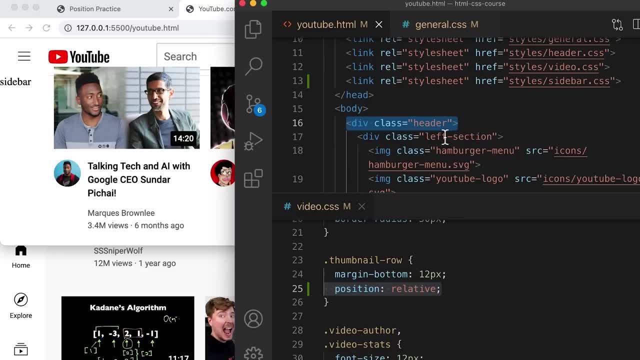 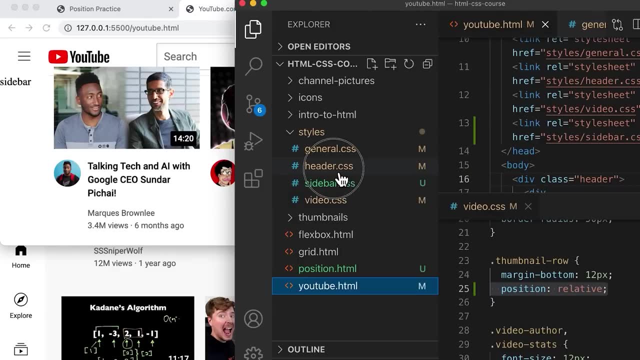 which is what we see And remember. to fix this, we need to set a property of zindex. Let's go into our header CSS file. We're going to open this file here And then, inside the header, we need to set a. 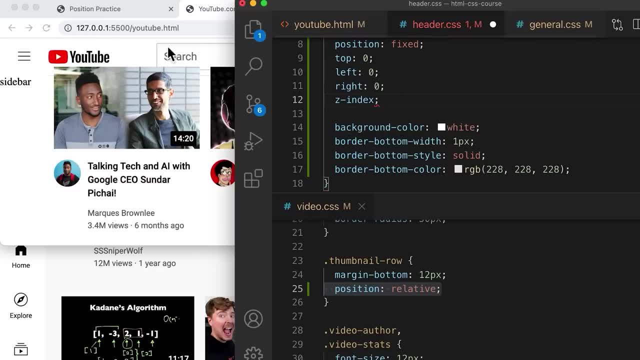 z-index to make the header appear above the thumbnails. So let's set a zindex of 100 so that we have room if we want to put stuff between these two. Now, if I save it, the header has a zindex of 100,. 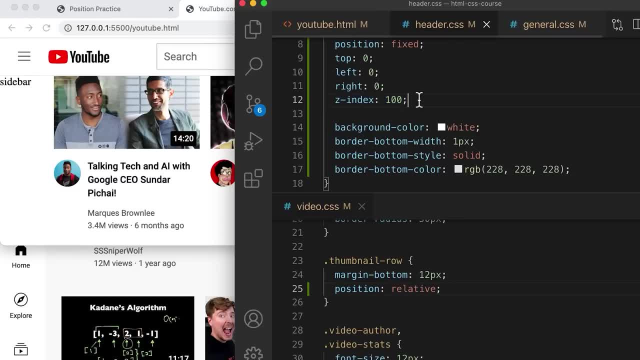 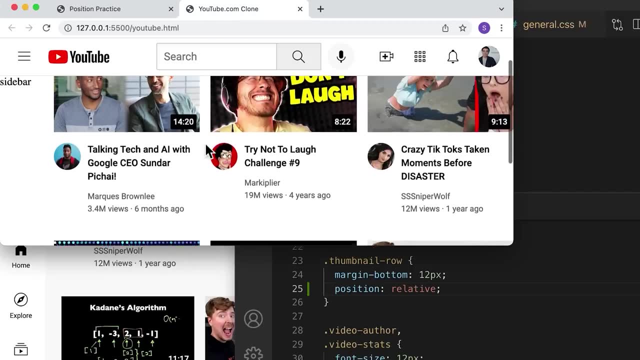 the thumbnail row has a default zindex of 0.. 100 is greater than 0, that means the header will appear on top of all the thumbnails. So we go back and we start scrolling. you'll notice that we're now all good. 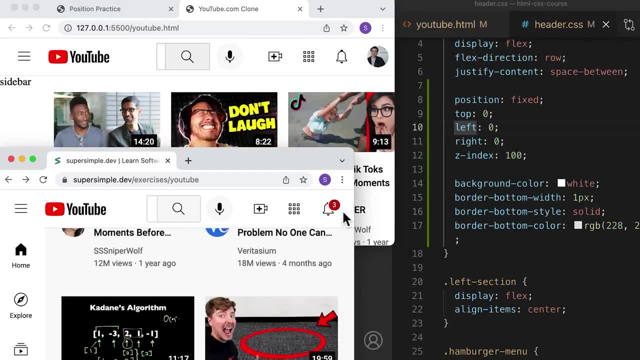 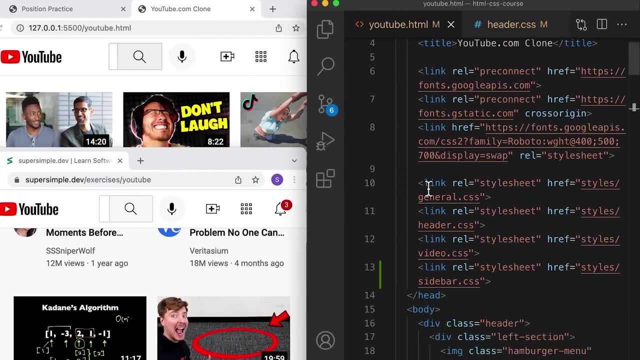 The last thing we'll learn is how to create this notification count in the top right corner of this icon. So let's go into our HTML, so youtubehtml, and find where the code for this notification is. So we scroll down to the header and then scroll down. 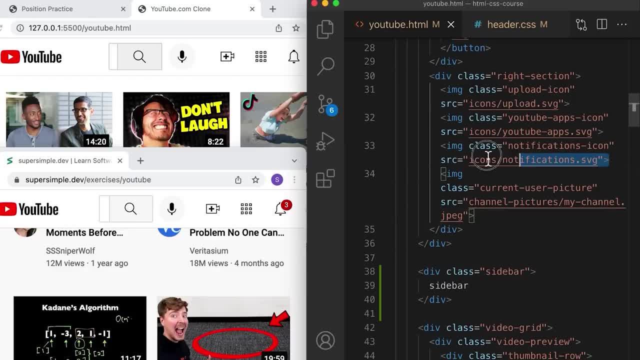 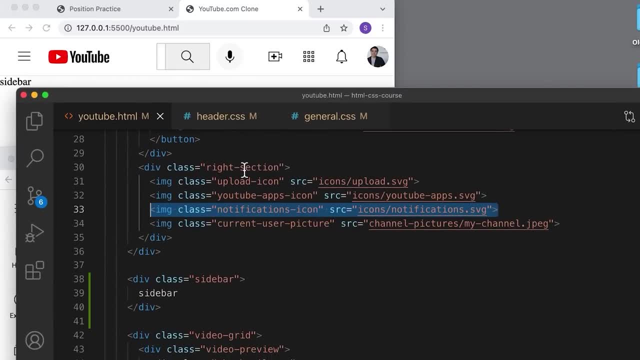 to the right side. that's this code here: notification icons. So I'm going to resize my windows so we can see it properly here And now. we want to put a notification number in the top right corner. So remember, like we've been doing, we need. 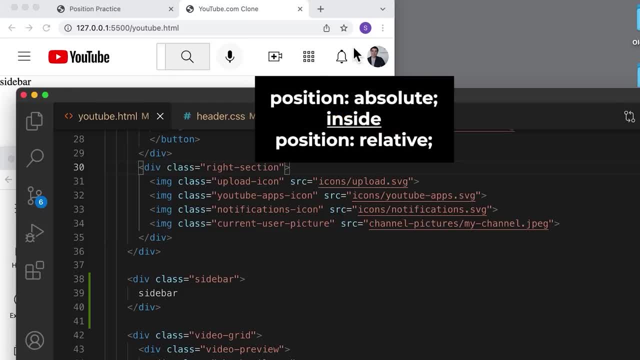 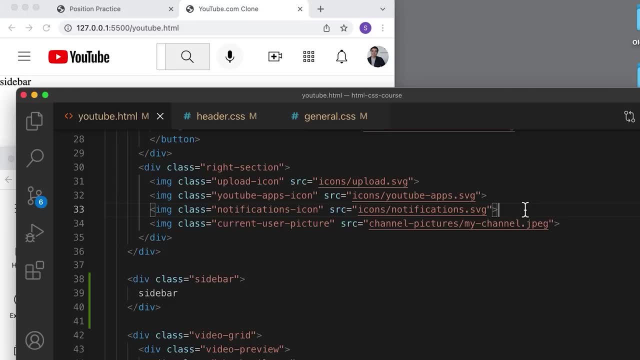 a position absolute inside a position relative. So if we look at our HTML, what could we use as our position relative element? So it can't really be this image, because we can't put stuff inside an image element. So one option is this div up here, But 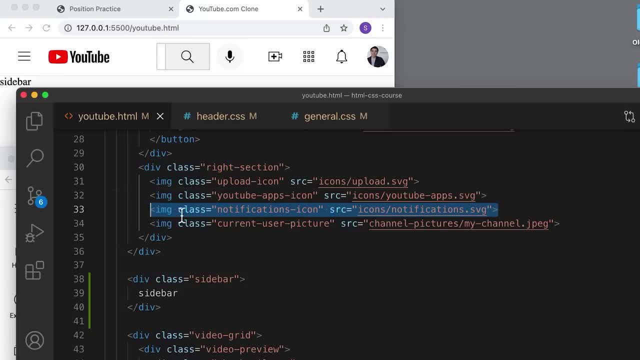 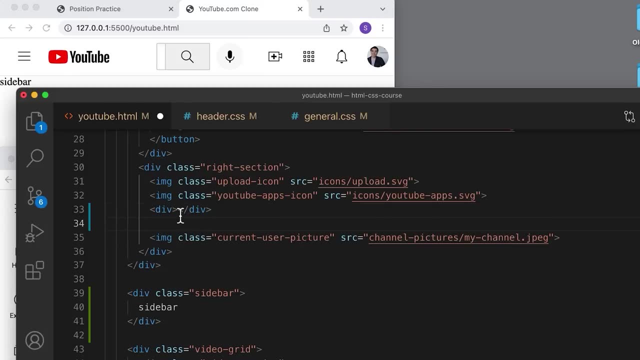 a better option is actually to wrap this image element inside a div. So we're going to create a div here and we're going to put this image inside this div. So remember that the div just creates a box around whatever's inside, So it's not going to change the appearance. 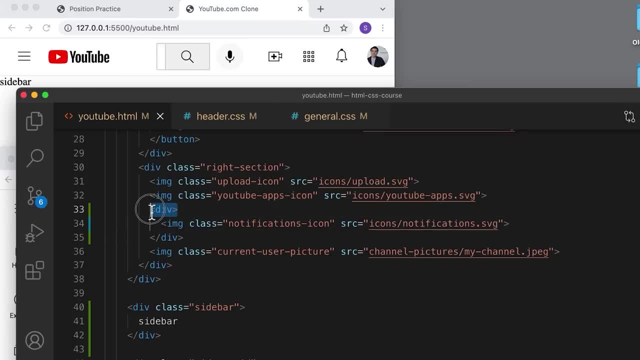 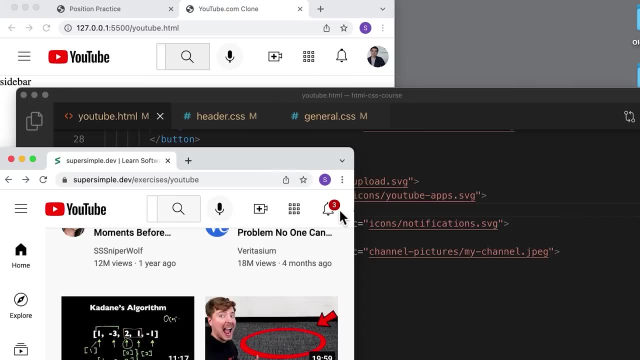 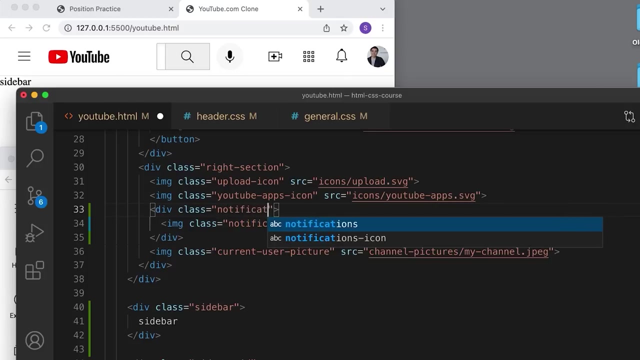 of this image. However, by creating this div, we can now make this position relative, And that's going to help us add stuff to the top right corner. So let's give this div a class so that we can style it later. Let's call it notifications. 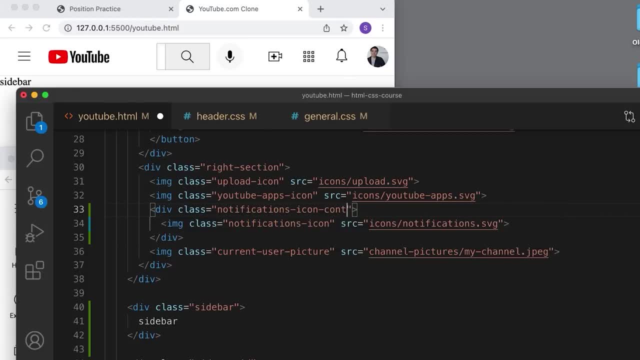 dash icon, dash container, And inside we're going to have our notification count. Let's create a div for our notification count. Let's give it a count of 3. And let's set this class equals notifications with an s dash count. And now we're ready. 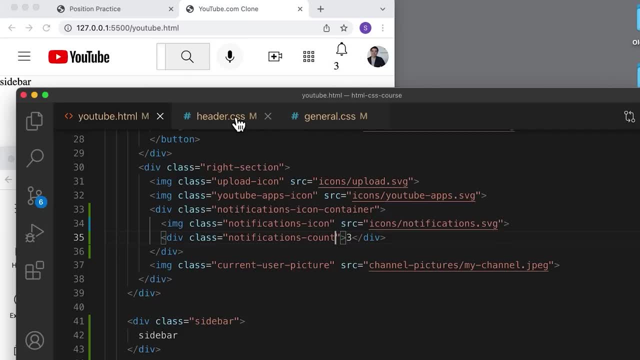 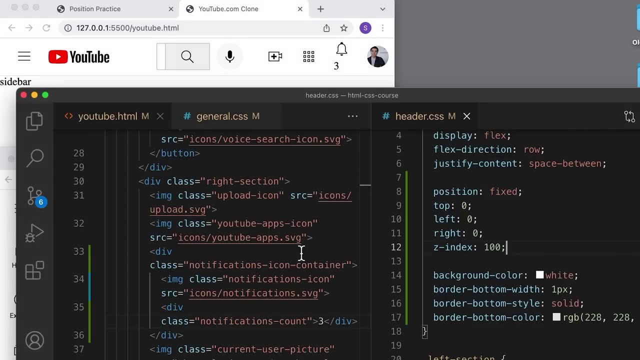 to style this and put it in the corner. So let's go into headercss. I'm going to put it on the side so we can see it more clearly. And now, to start off, let's scroll down to where we have our notification code. 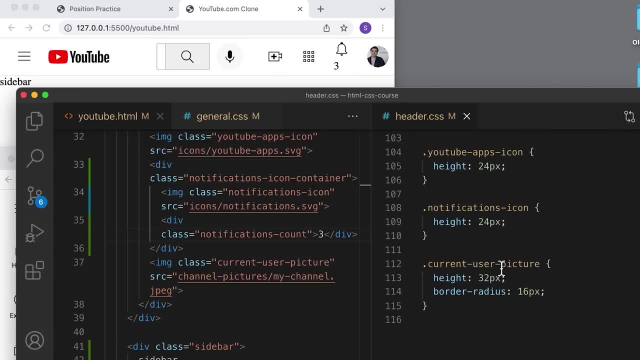 Let's scroll all the way down And we'll find it right here And now. remember we're going to have position relative and then inside we're going to have position absolute. So let's style the dot notifications: dash icon, dash container. 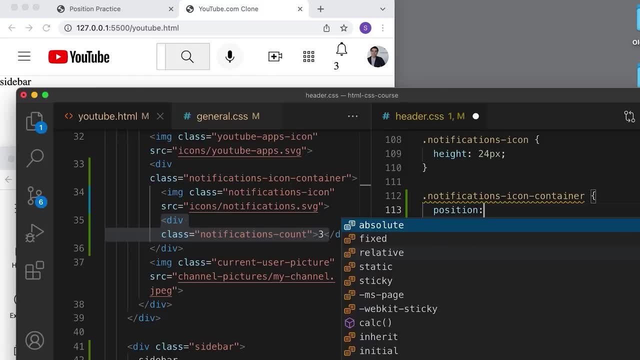 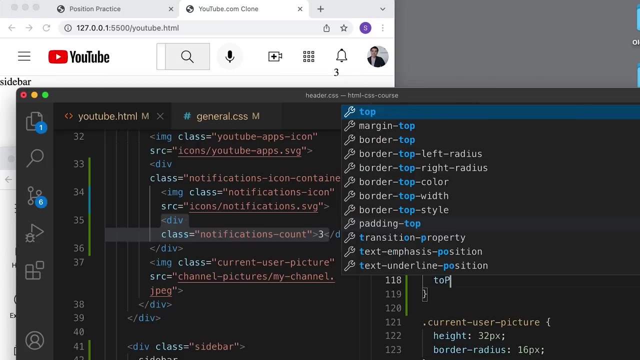 And set this to position relative And then the notifications count, dash count And we'll set this to position absolute. So we want to put this in the top right corner. So let's set the top to zero pixels and the right to zero pixels. 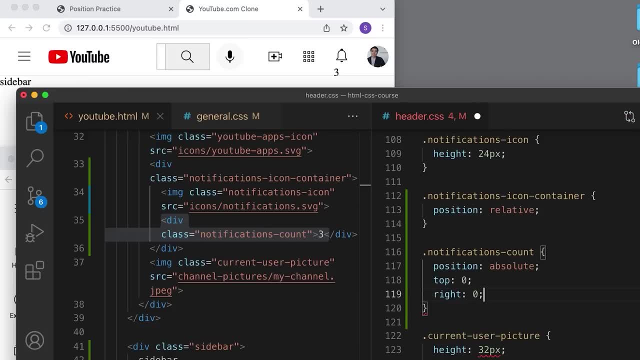 And to see it better, let's set a background color, So background dash color of red And a text color of white. And now, if we save that, it's sort of in the top right corner, but it's a little bit too wide. 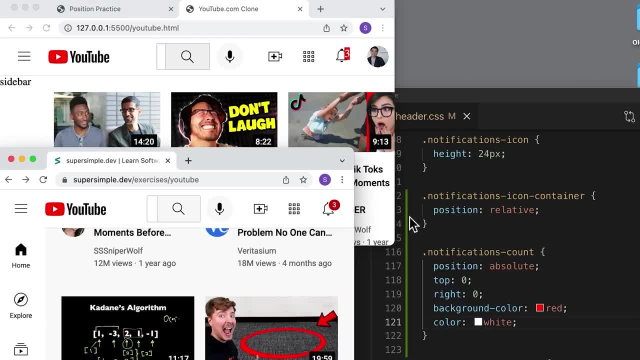 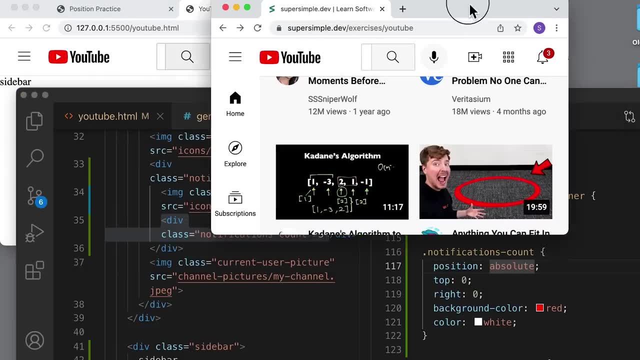 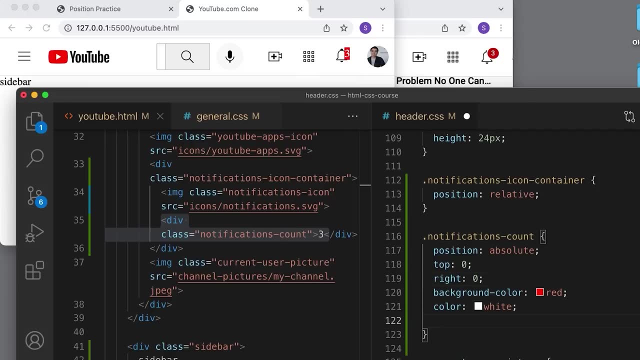 So we're going to style it just like our design here. So I'm going to move this up here, actually, so that we have a better reference, And now we're going to style it by first changing the font. Let's change the font: dash family. 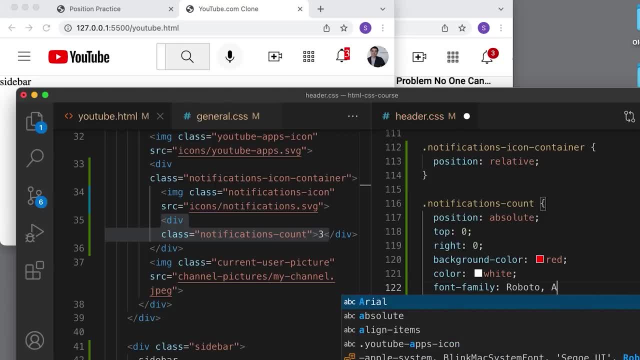 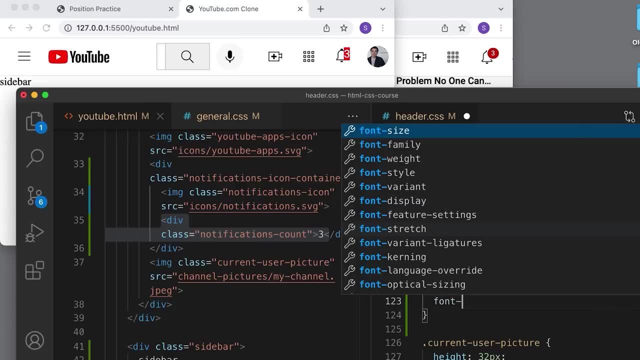 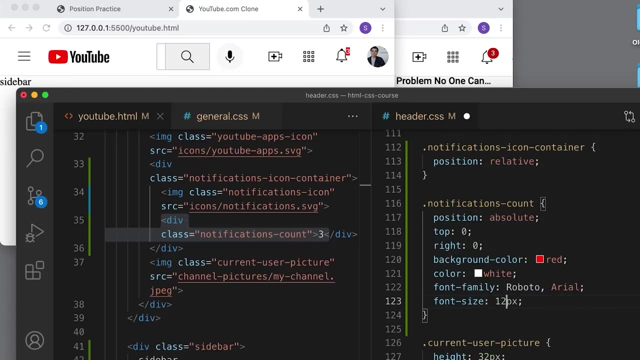 to Roboto comma Arial, like before. Next we'll change the font size. So this is pretty small. Let's change the font dash size to maybe 10 pixels. Okay, it should be a little bit bigger. Let's set it to 12 pixels. 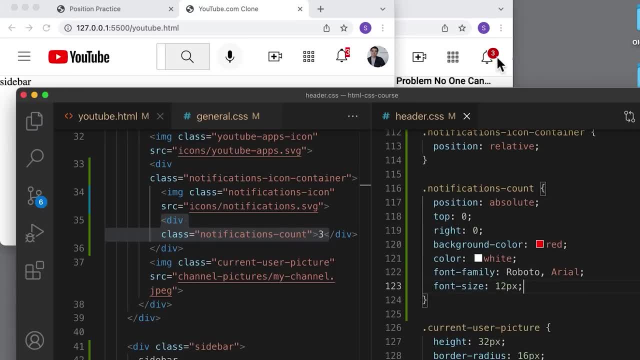 Okay, that looks pretty good. And let's add some spacing on the inside of the element. Let's add some padding Left of maybe 4 pixels. Padding right of 4 pixels, Padding top of 2.. And padding dash bottom of 2 pixels. 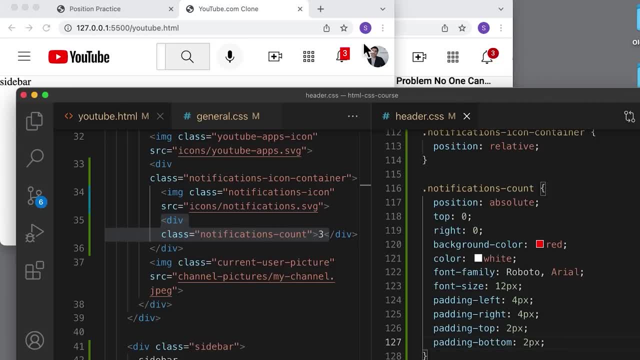 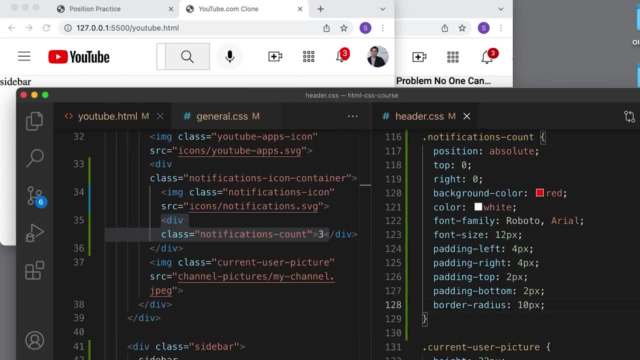 And remember, to make this a circle, we're going to give it round corners, So let's set the border dash radius to 10 pixels, So it looks like we're a little bit too tall here. We're going to stretch out the sides by adding more padding. 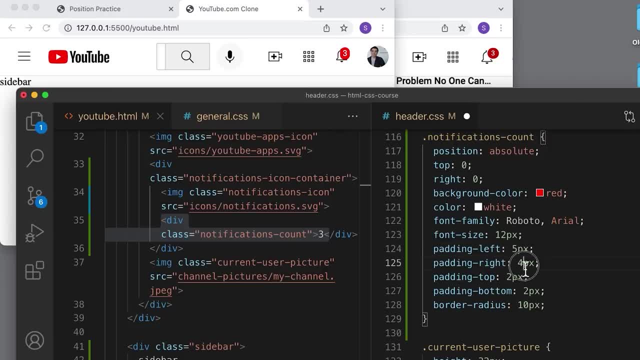 to the sides. Let's change this to: maybe 5 pixels Left and right- Save it Okay. maybe 6 pixels Left and right- Save it Okay. that looks like a pretty good circle. Next we'll change the background color to: 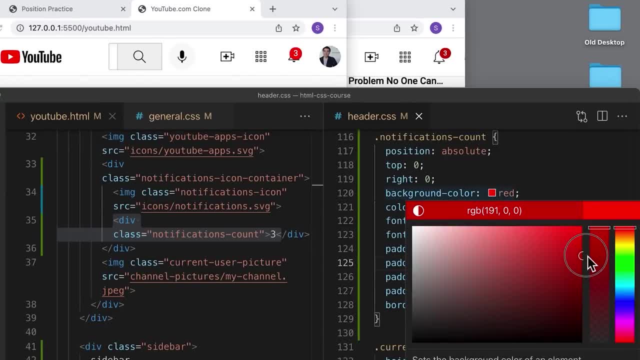 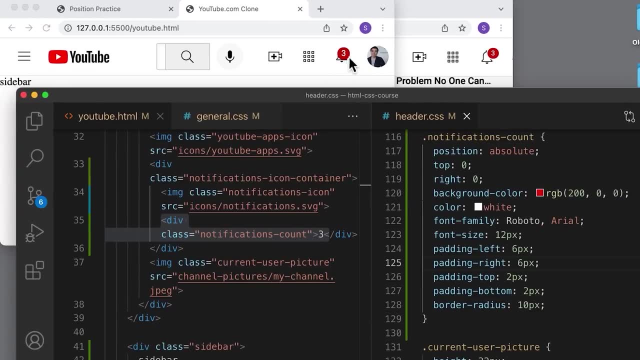 something that looks like that. So I'm just going to pick something like this, maybe Save Perfect, And I'm going to change the font size down just a little bit more because this is pretty small. Let's change this to 11. Save that. 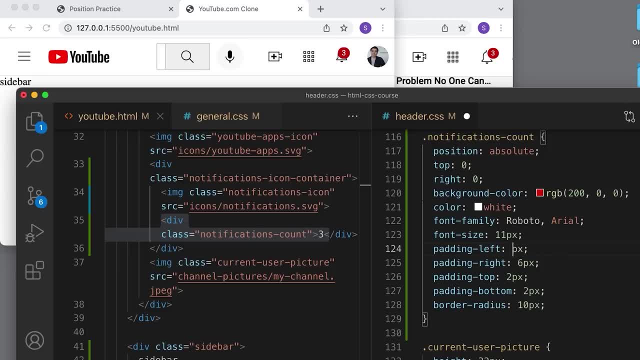 And let's change the padding left and the right, because it's a little bit long on the horizontal side And now we have a circle again. So notice that we put this element in the top right corner using these two properties, But it's not enough. 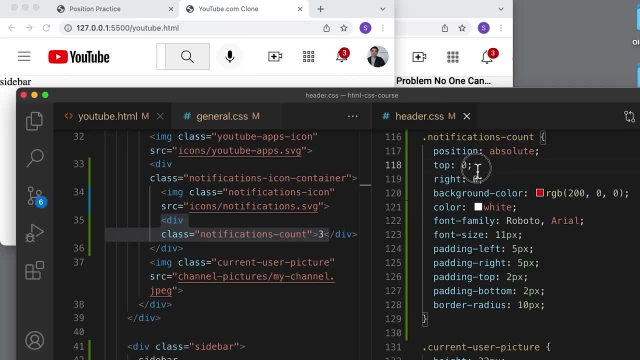 We actually want it out even more. So we're already at the top edge of our position: relative container. How can we go even higher? So the trick here is to use negative numbers. So now this will be positioned beyond the top edge of our container. 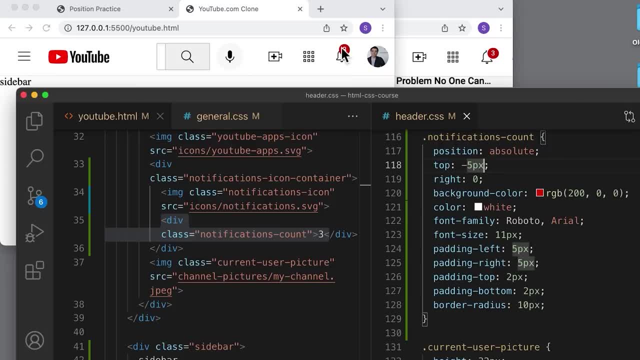 So if I save it here, this is now 5 pixels beyond the top edge of our relative container. Same thing with right. If we set it to negative 5 pixels here, it's now 5 pixels beyond the right edge. So I'm just going to adjust the values here. 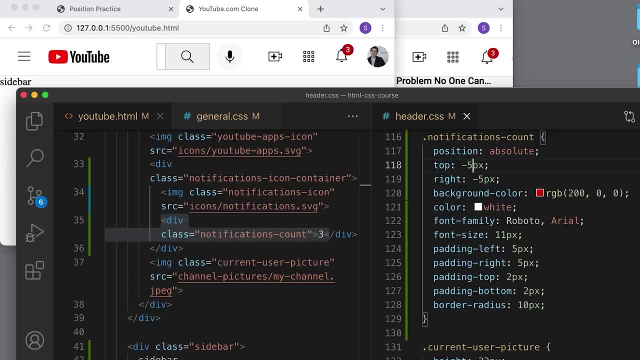 so that it matches our design. So let's set the top to something like negative 2.. Okay, so I think that looks pretty close to our design. I'm pretty happy with it. So in this lesson we learned CSS position, which is one of the most important. 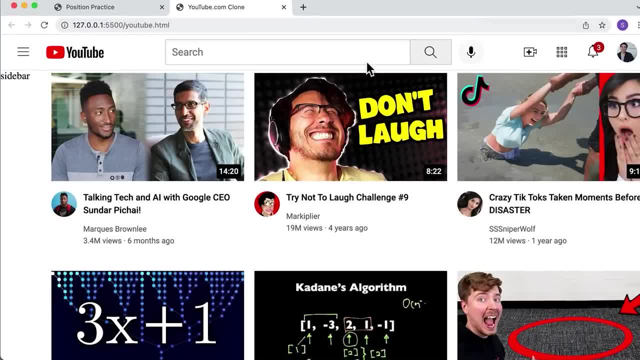 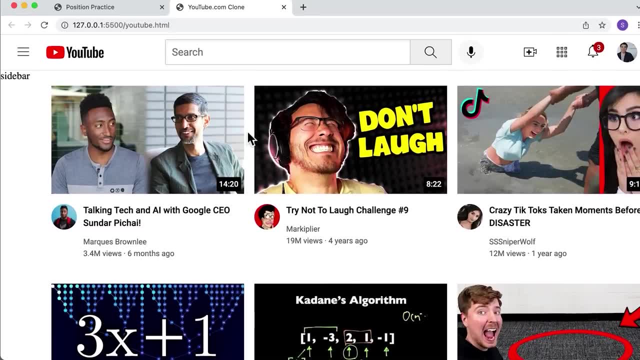 skills in CSS. It allows us to create elements like this header and sidebar that stick to the page while we scroll, And it allows us to add elements on top of other elements, For example, the video time on top of the thumbnail and the notification count on top of the. 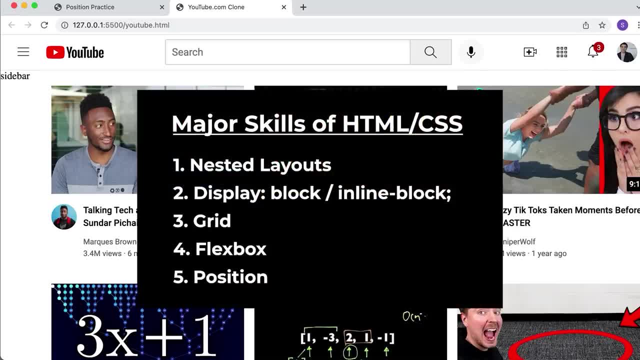 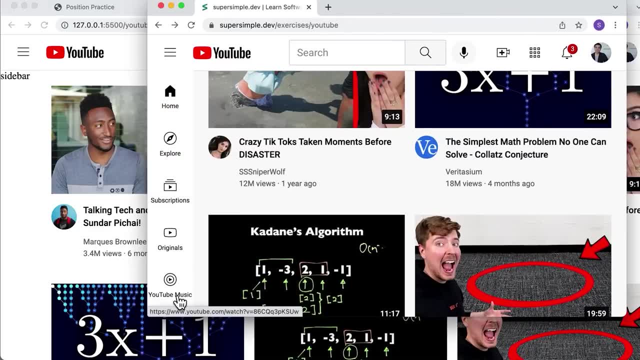 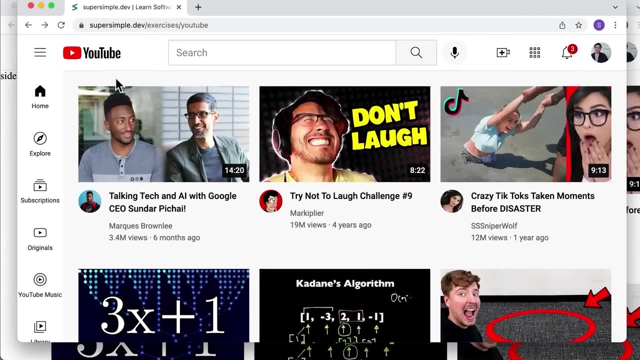 notification icon. So with that, we learned all the major skills that we need in HTML and CSS to complete our project. In the last lesson we're going to create all the other features that we're missing, including the sidebar, the tooltips and making our 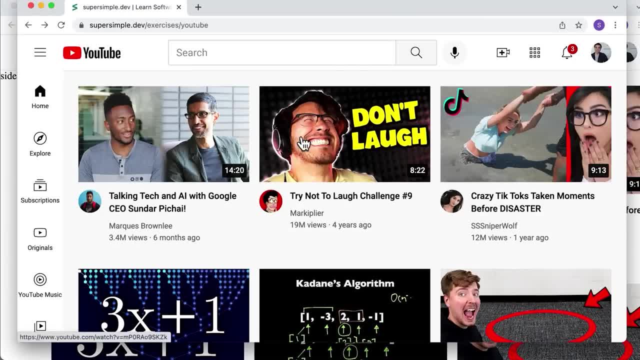 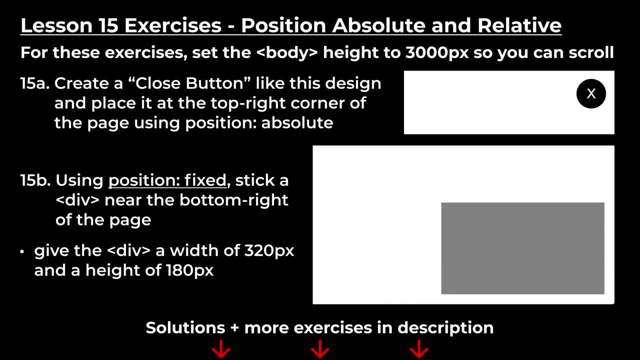 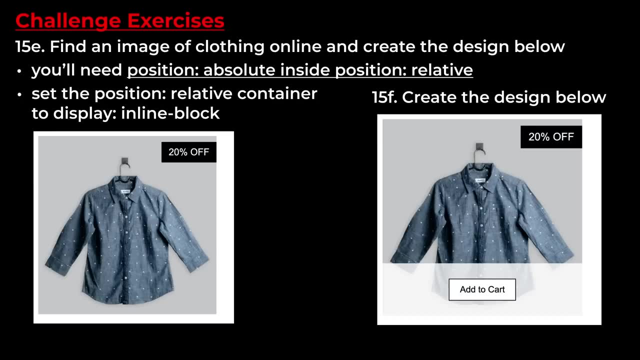 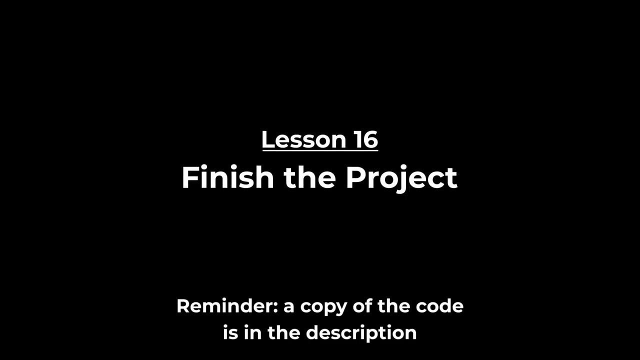 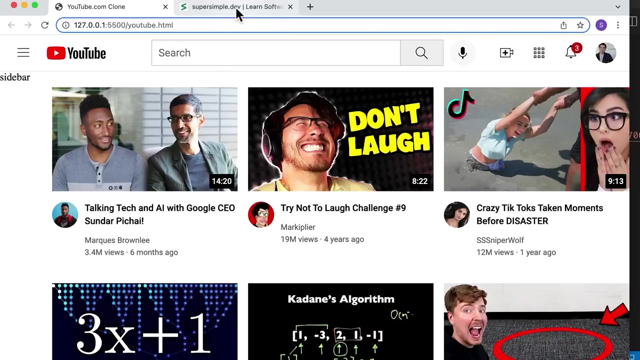 current project look like the final design here. In this lesson, we're going to finish our final project. We're going to create the sidebar. We'll resize our video so that it looks like our design here And, lastly, we're going to create the tooltips when we 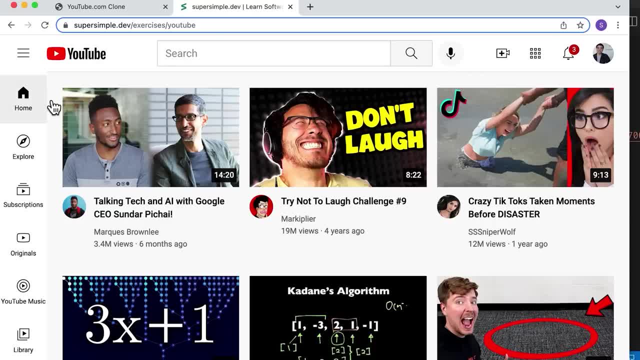 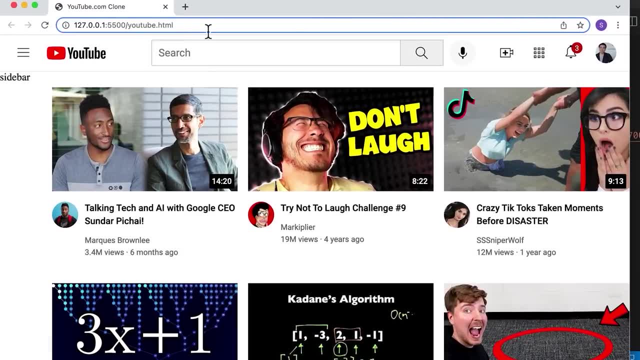 hover over these icons. We'll start off with the sidebar. So I'm going to rearrange my windows here so that it's a little easier to copy. So I put the design on the left. I'm going to put our current sidebar on the right here. 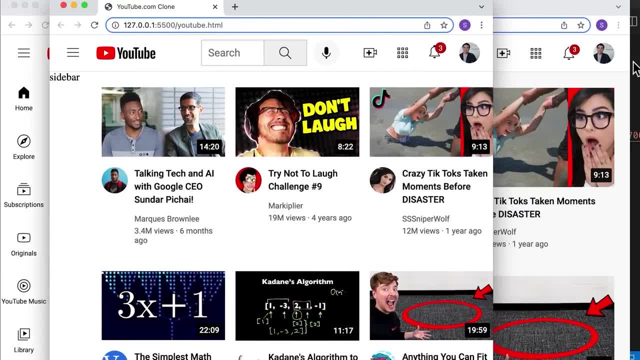 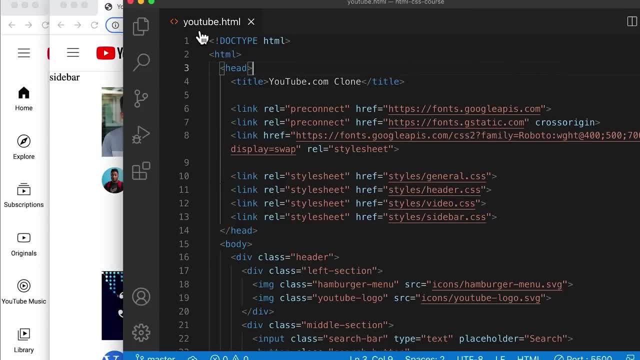 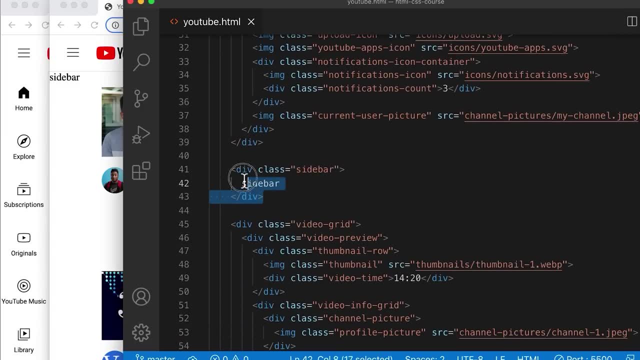 And I'll resize my windows so we can see it better. And now we're ready to begin. So let's open our code editor And we're going to open youtubehtml, And then we're going to scroll down to the sidebar code, which is right here. 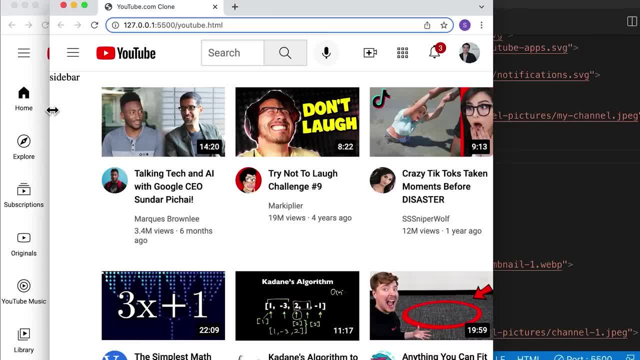 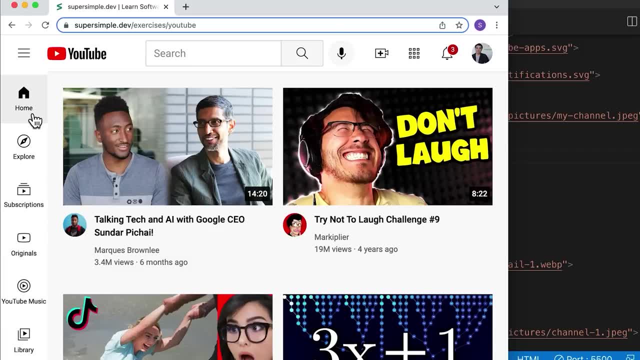 So let's take a look at the design of this sidebar, Our reference design. If I hover over it, you can see that it's just a bunch of boxes, And inside each box we have an icon, some text, and they're centered horizontally. 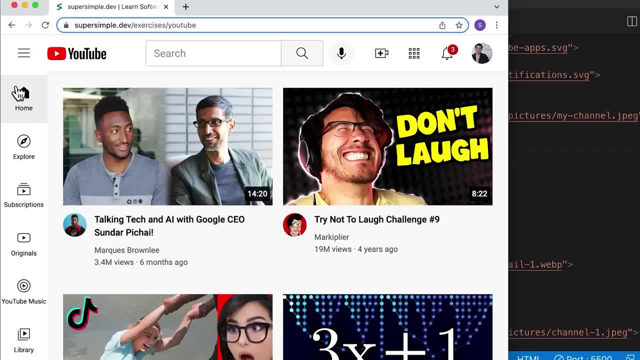 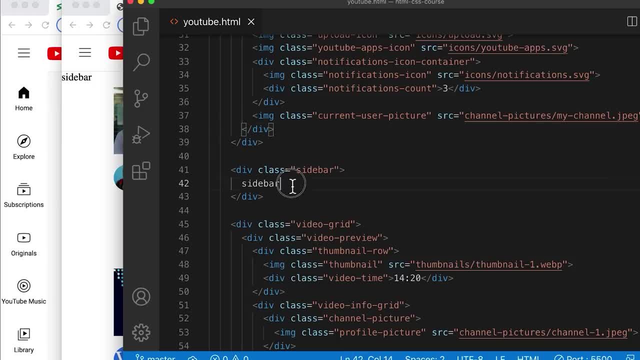 and vertically. So we're going to start step by step. We're first going to create the box. Let's go into our code And instead of this text, we're going to create six boxes. We're going to use a div to create each box. 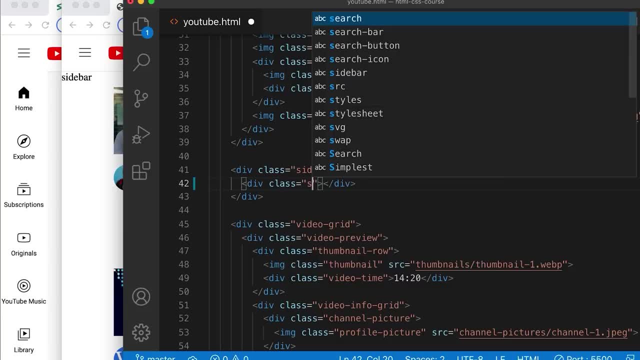 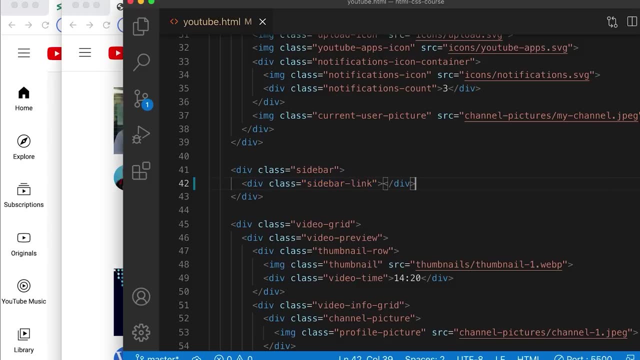 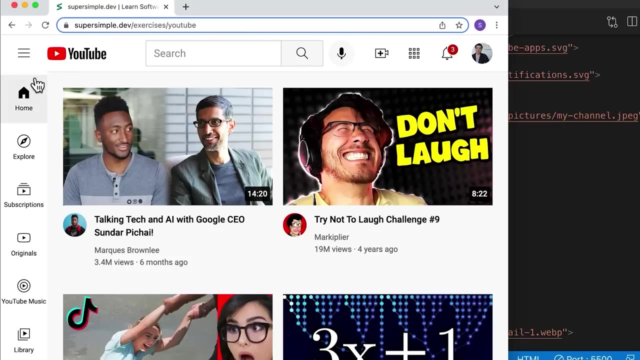 Let's give this div a class of sidebar-link And I'm going to copy and paste this six times: Four, five, six. Next, we're going to style these so that they have the same size as these boxes. We're going to go into our CSS. 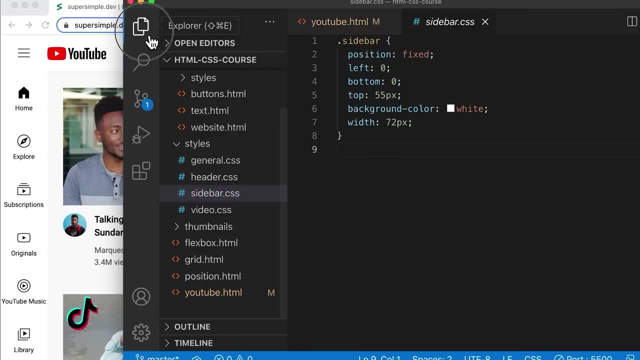 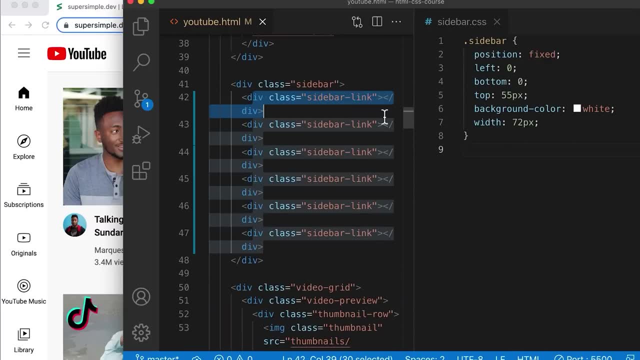 So let's go into sidebarcss. I'm going to put this on the right side here so we can see it better. And now we're ready to style these. Let's target the class sidebar link And for each of these, let's give it. 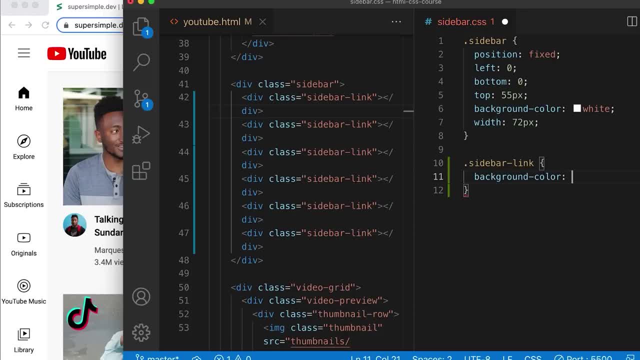 a background color So that we can see them, And let's set it to light gray, And we'll also give them a height, Because without any content in the divs they have a height of zero. So let's set a height. 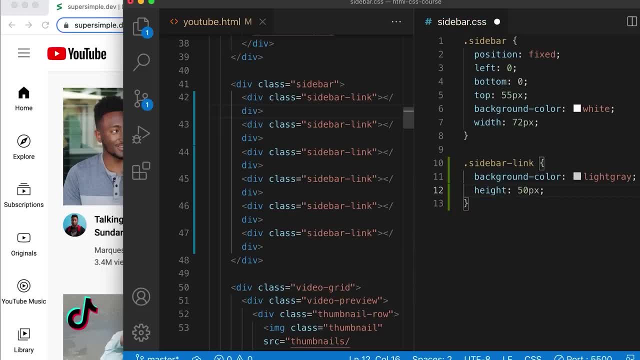 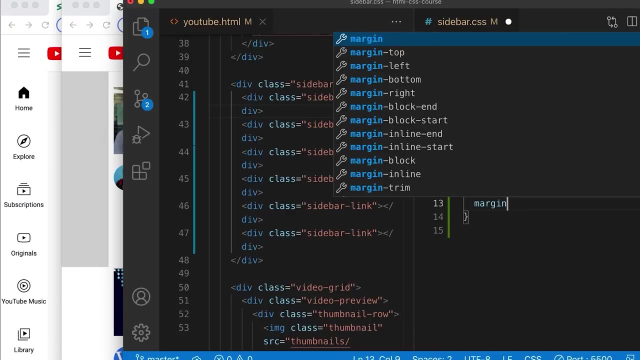 of 50 pixels And let's save it And let's see how that looks. It's hard to tell the difference between them, So let's add some spacing at the bottom of each div so that we can differentiate them And margin dash bottom. 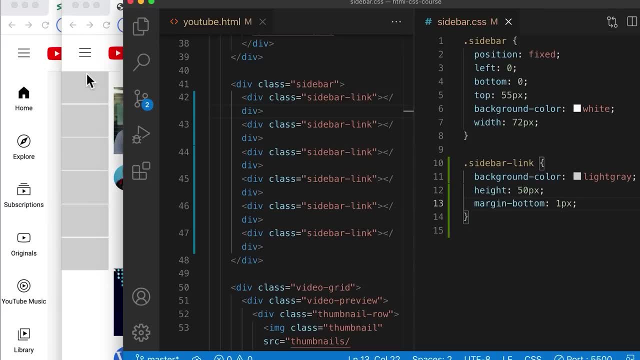 of one pixel, Save it. So from this it looks like our boxes are a little bit too short, So we're going to make them taller. Let's try a height of maybe 75.. Okay, so I think that's pretty close. 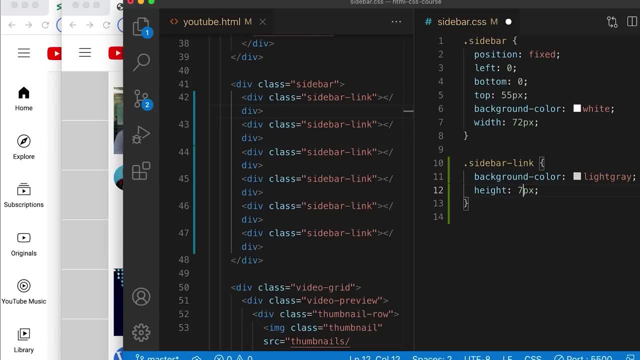 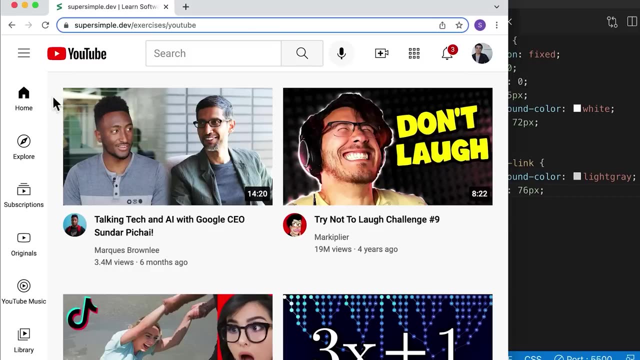 We can get rid of this margin at the bottom And actually increase this to 76 so that we compensate for the margin that we removed. And next, when we look at the design, these boxes are usually white, but when we hover over them they turn gray. 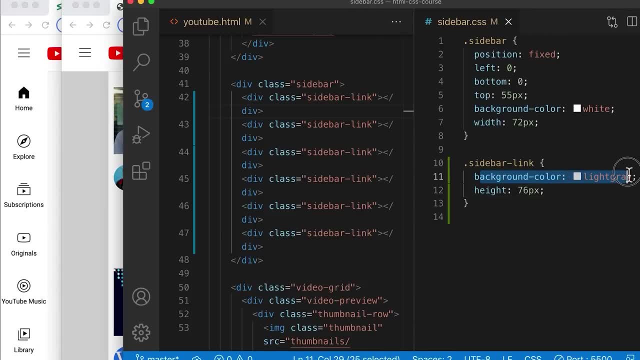 So instead of having this background color gray here, we're just going to set the background color when we hover over this. So let's set a hover style dot side bar, dash link, colon hover And when we hover we're going to set the background color. 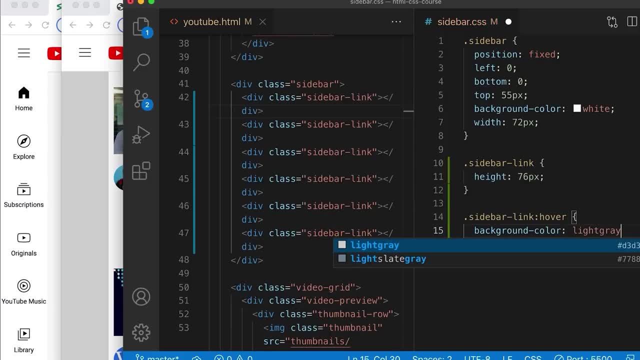 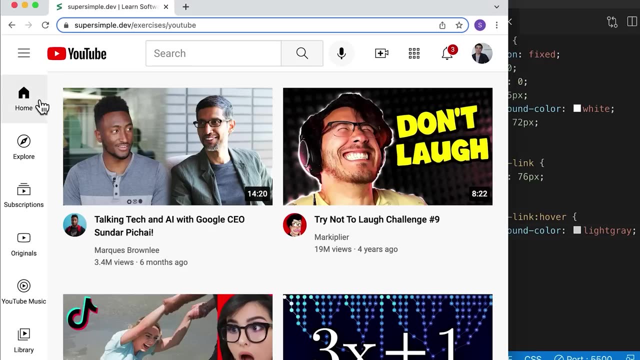 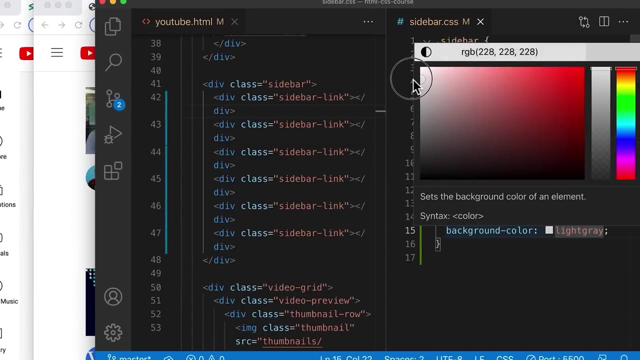 to light gray. Let's save it. Now. when we hover it's light gray, But our design is actually a lot lighter than that, So I'm going to change the color here. I'm going to pick something a little lighter than this. 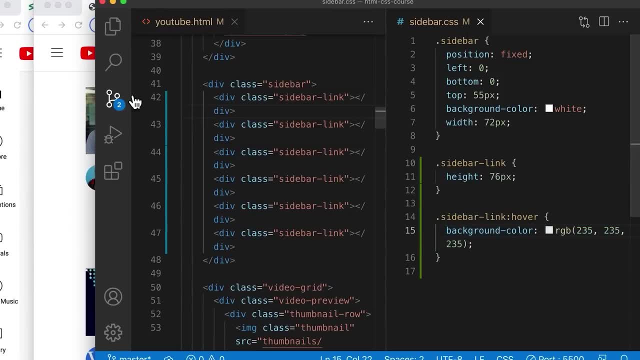 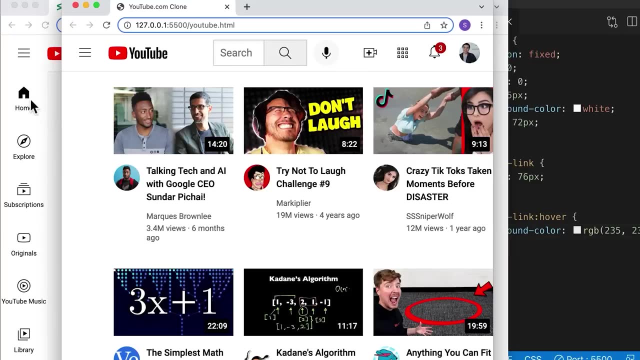 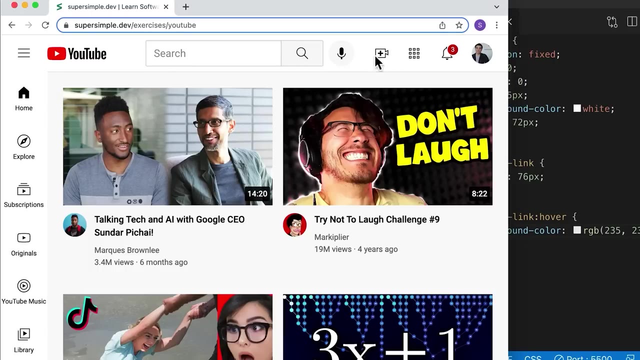 Maybe something here. Save that And check it out, And yep, I think that looks pretty close. Next we're going to add the content in each of these boxes, So first we actually need to download all of these icons, So we did it before for 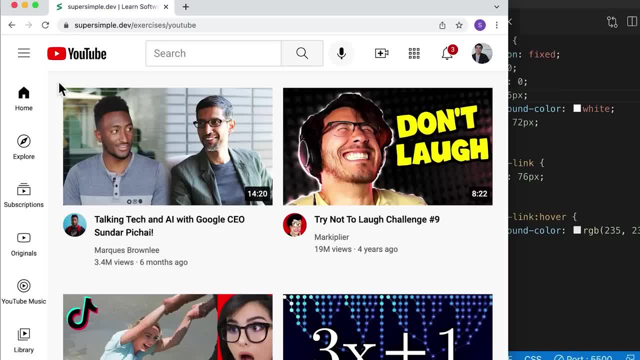 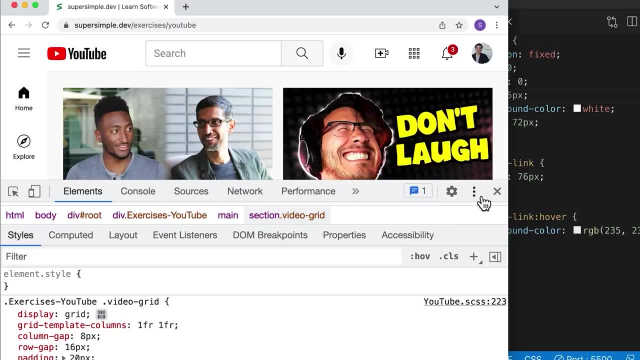 these icons And just a reminder to do that. we're going to right click and inspect, So you'll see that this actually covers up the side bar. What we can do is click these three dots in the top right and then we can. 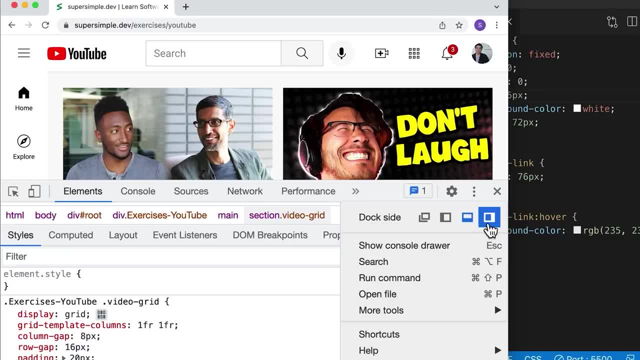 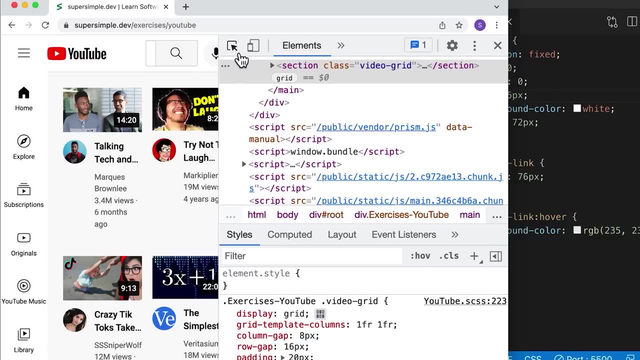 move the dev tools to another side of the webpage. I'm going to move it to the right side here And now we can see the full side bar. Then we're going to click this in the top left. Click one of these icons. 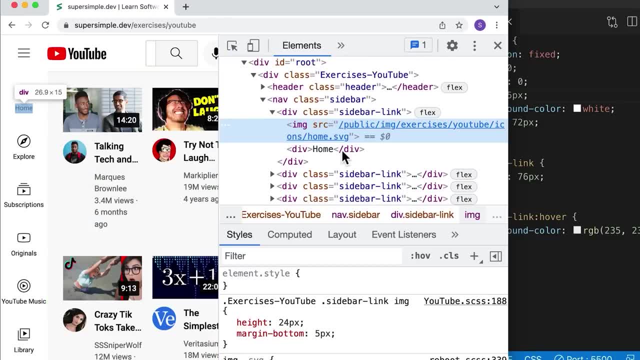 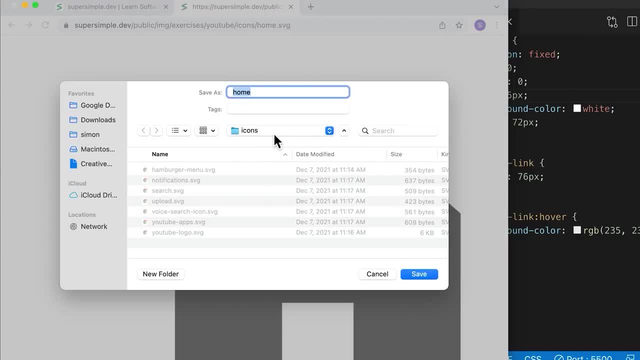 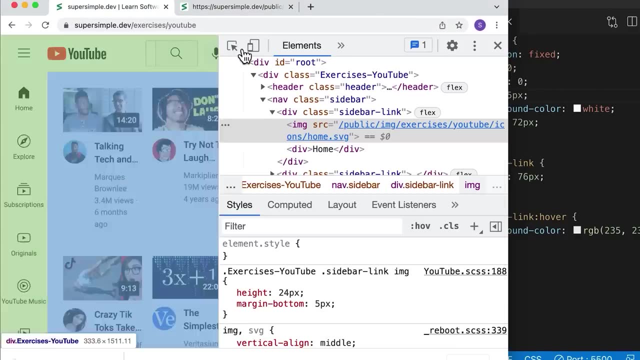 And you'll get the URL to download them here. So hover over this URL and then click this, And now we can control s And I'll save it in the folder that contains my code, in the icons folder. So make sure you do this for. 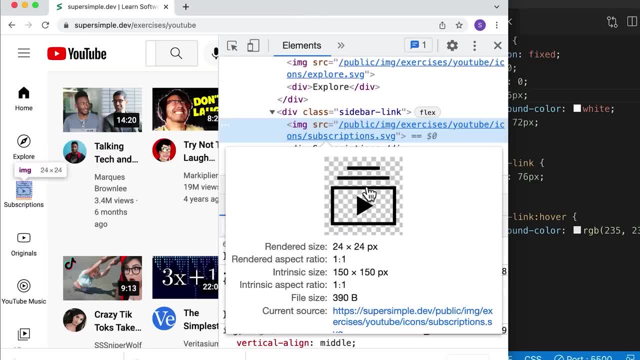 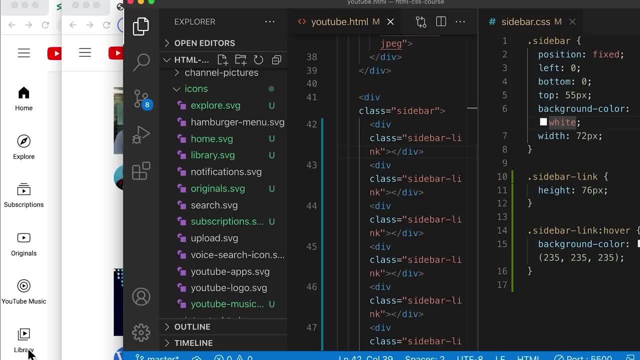 all six of these icons and I'll see you back after you're done. Alright, so once we've downloaded all of the icons from the side bar here, we're going to add them to our HTML. So let's go into each of these and add our icons. 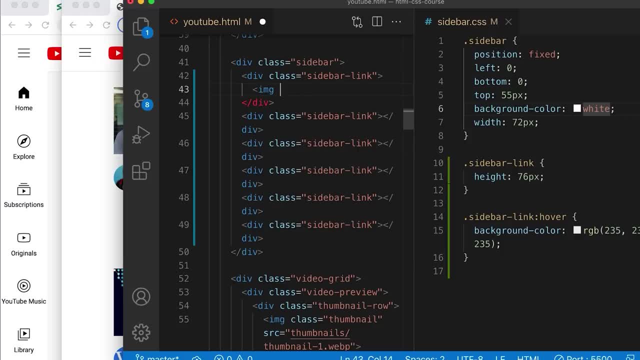 Inside this first div, we're going to add an image element And we're going to set a source attribute And we're going to load the icon Icons slash- homesvg, because this is the home icon And let's save it. 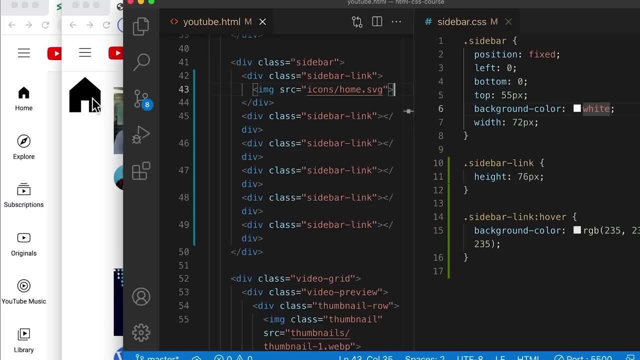 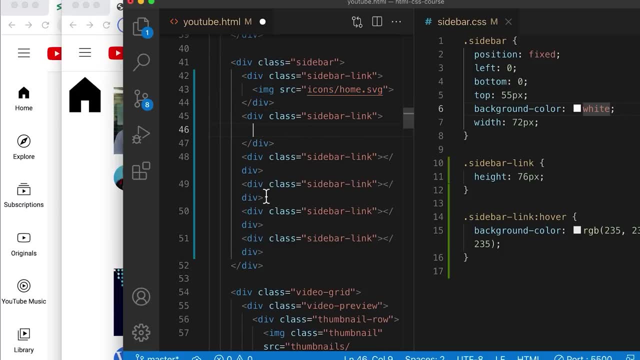 And now we have our icon. It's a little bit too big, but we're going to resize it after. For now, let's copy this and add the icons for all of these other boxes. So we're going to add for this one. we're going to 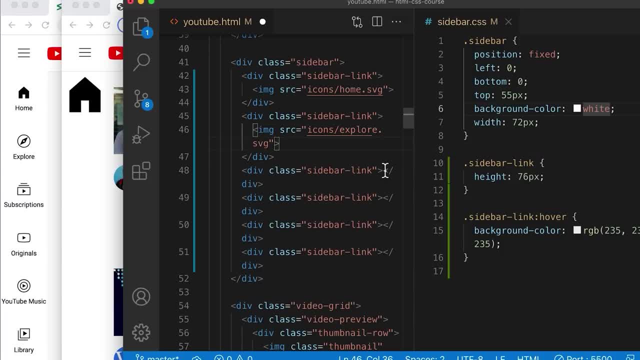 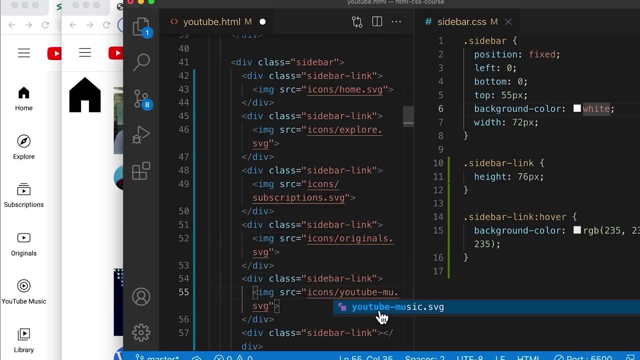 add the explore icon, So exploresvg, And for this one is the subscriptions, And then for this one it's originals, And then for this one it's youtube-music, And the last one is library. I'm going to go down here, change this to. 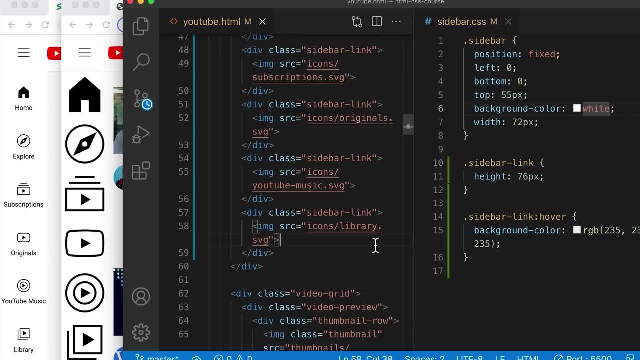 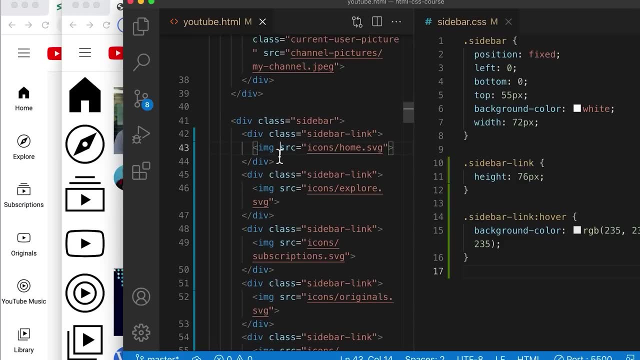 library Perfect. Next, we're going to make these icons smaller. So usually we would set a class on these images so that we can style them with CSS, But for this lesson I'm going to show you another way that we can target. 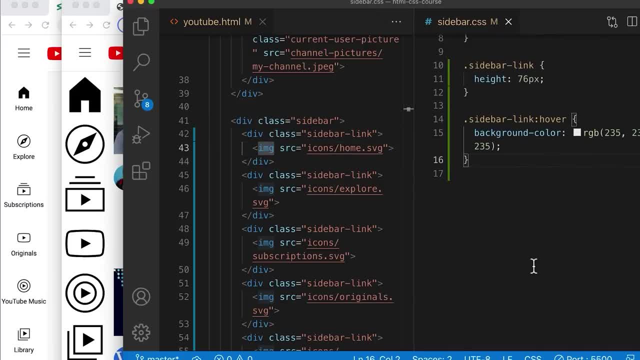 these images. So let's go into our sidebar styles. We're going to learn a new CSS technique, So we already learned that. this text before the brackets here: this tells the computer which elements we're styling. In this case, the dot means we're targeting. 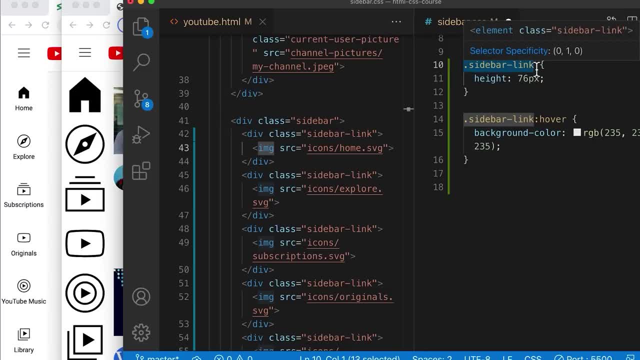 a class and we're styling all elements that have the class sidebar link, which are these elements? So this bit of text is called a CSS selector, And there's actually a lot of different selectors that we can use in CSS, So we already learned the class. 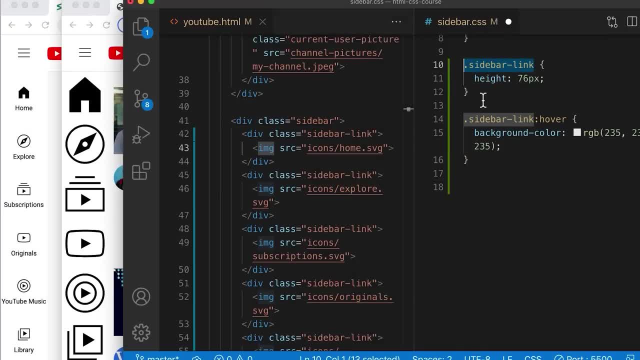 name selector, which looks like this and starts with a dot, and we learned the element name selector, which just starts with the element's name. Another thing we can do with CSS is to combine selectors together. For example, if we said dot, sidebar dash link. 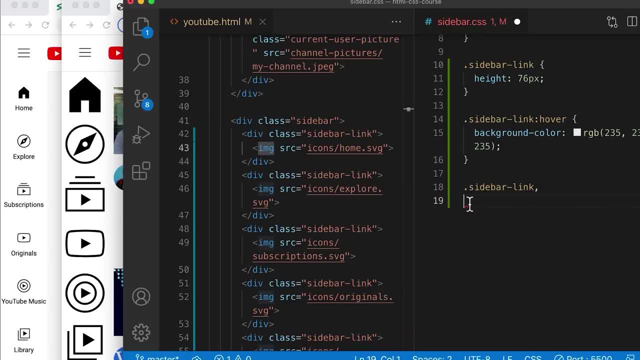 and then wrote a comma down. here we can add another selector. So let's say we also want to target dot header. So now all of the styles inside the brackets will target all elements with the sidebar link class and all elements with the header class. 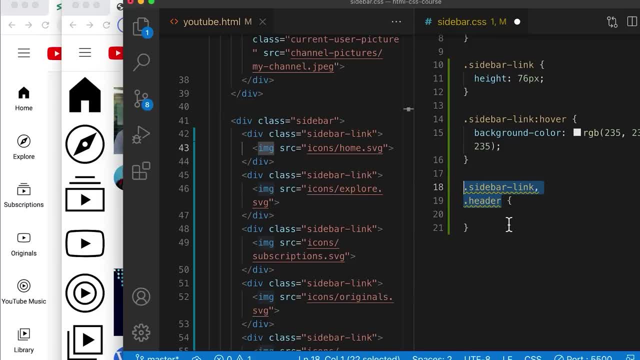 This is an example of a more advanced selector. Another selector we can use is: instead of a comma, we can use a space And then type another selector like image. So when we have a space between these two, this means that we're targeting all images. 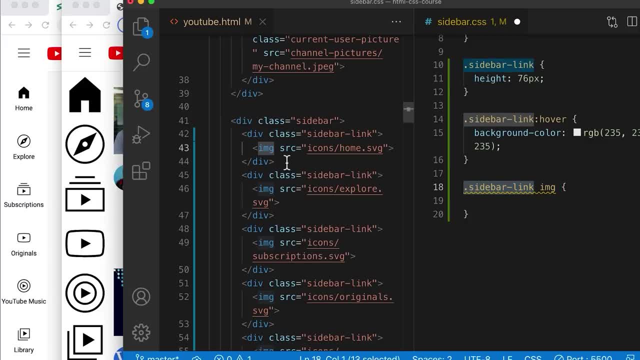 inside all sidebar links. So we're going to target these images inside sidebar links only. We're not going to target all images on the page. So let's style these images and make them smaller. We're going to set a height and let's try 24. 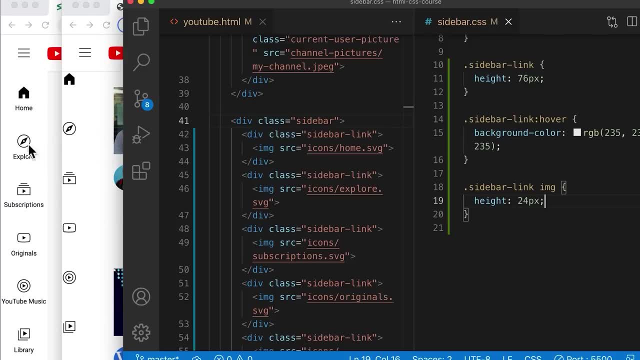 pixels. Let's see how that looks. Okay, so I think that looks pretty close to what we have in the design. Next, we're going to center these horizontally and vertically and finally add the text. So to center something vertically is actually challenging in CSS. The best way to 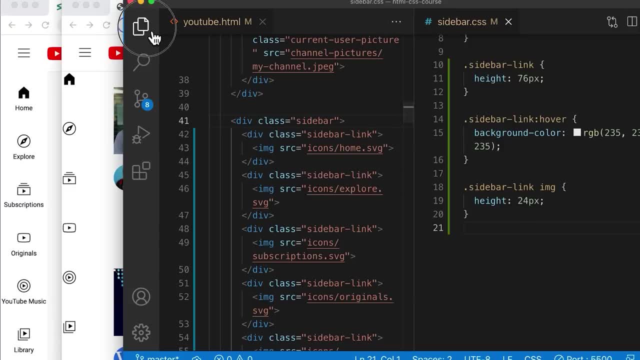 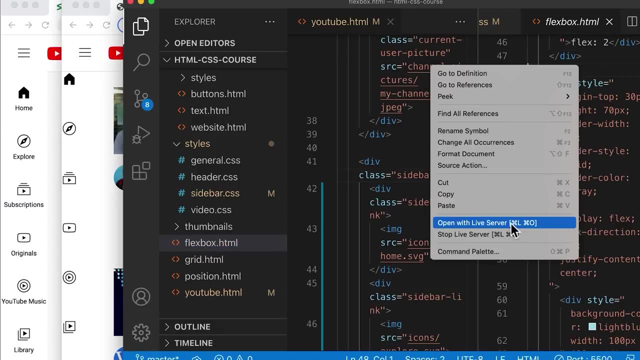 do? it is to use a flexbox. If we look into our code editor and open our flexbox example- so flexboxhtml- and then we right click and open with live server, we have a bunch of examples of using flexbox In the. 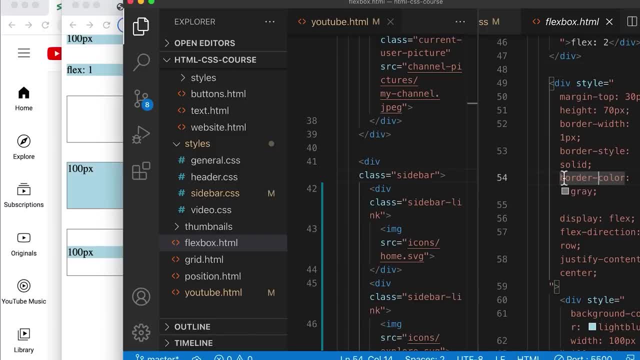 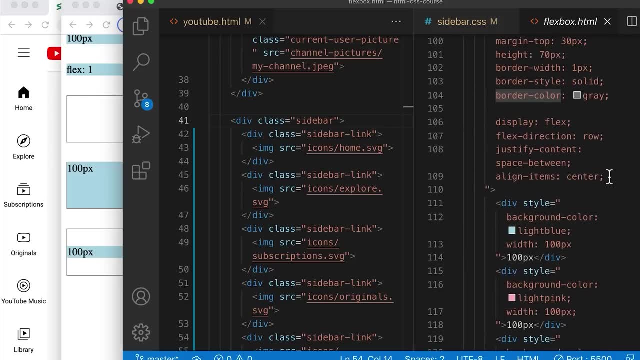 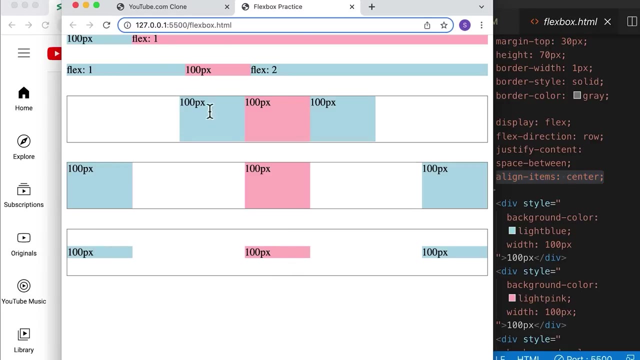 last example: here we're doing vertical alignment. If we scroll down to our example, in our HTML we have this property called alignItemsCenter, So this vertically centers our content. Here we also have an example of horizontal centering If we scroll up. 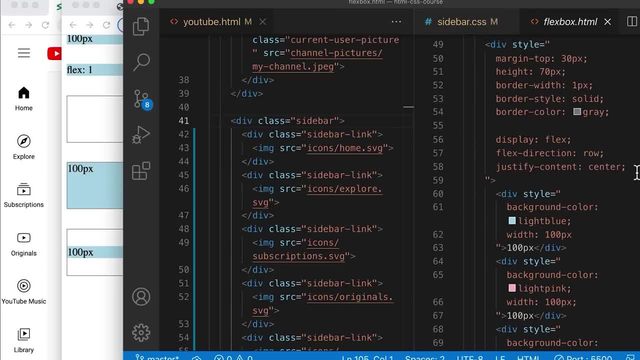 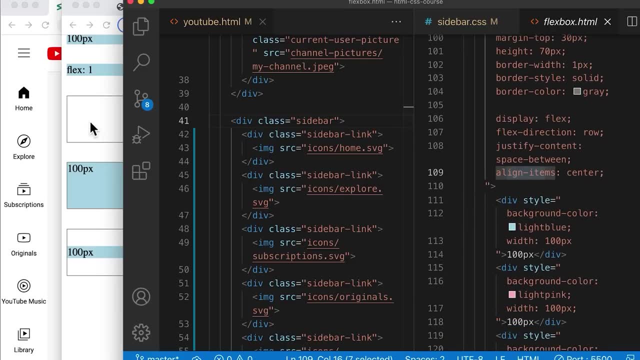 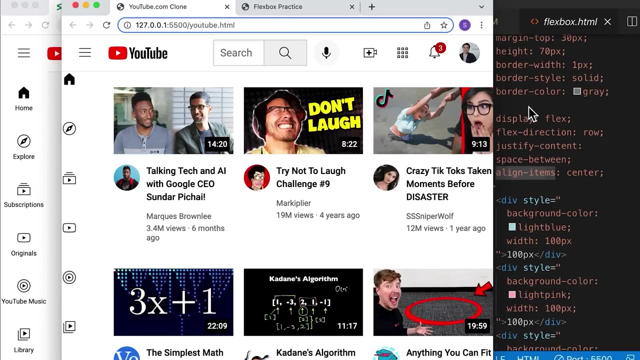 to that example, which is this one. we have the property justifyContentCenter, So using justifyContentCenter and alignItemCenter, we can put it both horizontally and vertically centered. So let's go back into our project and use a flexbox to center these. 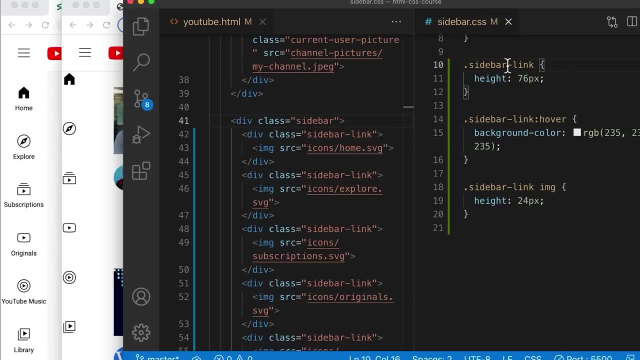 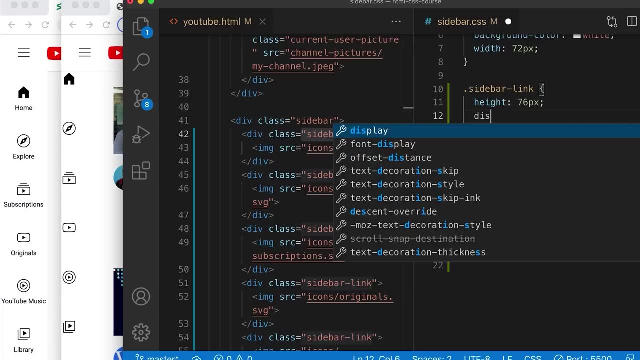 We're going to go back to our CSS and we're going to make each of these sidebar links a flexbox, So let's set the display property to flex And we're going to set justify-content to center, So this will center horizontally. Let's save it. 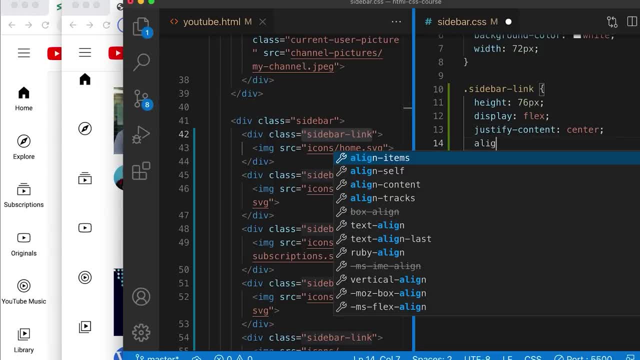 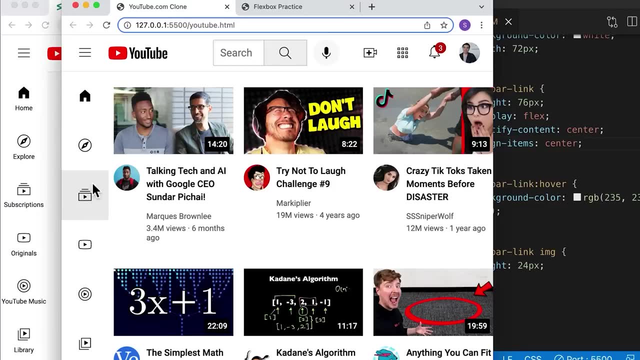 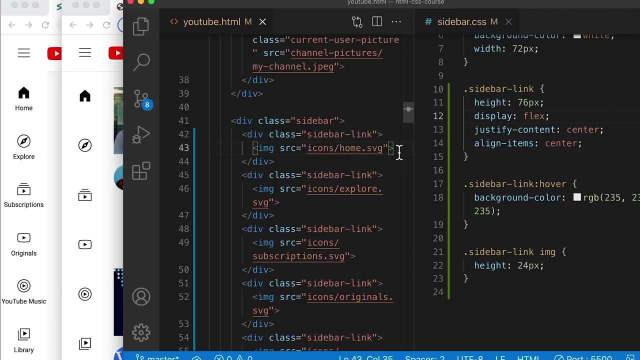 And now they're horizontally centered, And then align-content items center for vertical centering. So this is coming along great. Next, we're going to add the text. So underneath each of these, let's add a div. So for this first one, 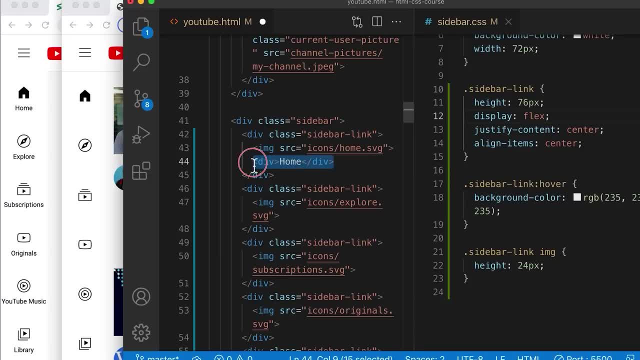 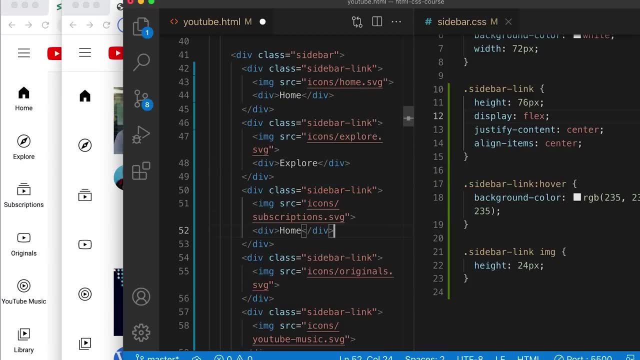 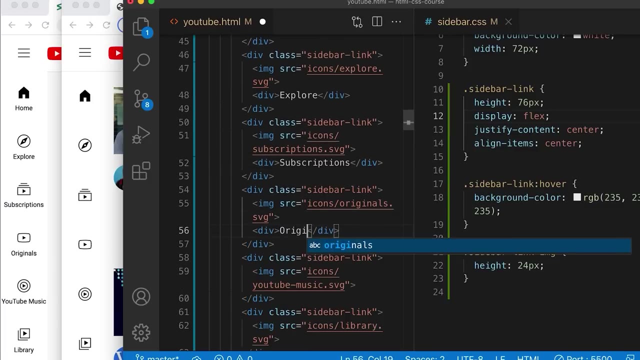 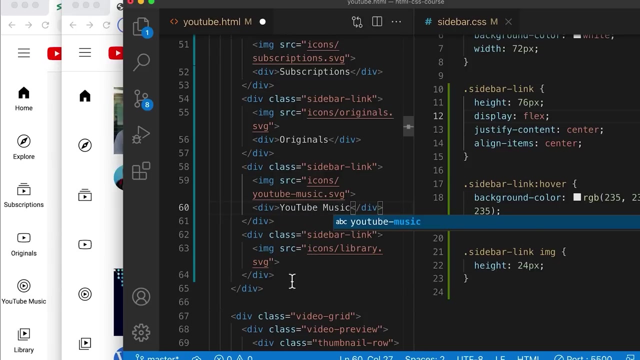 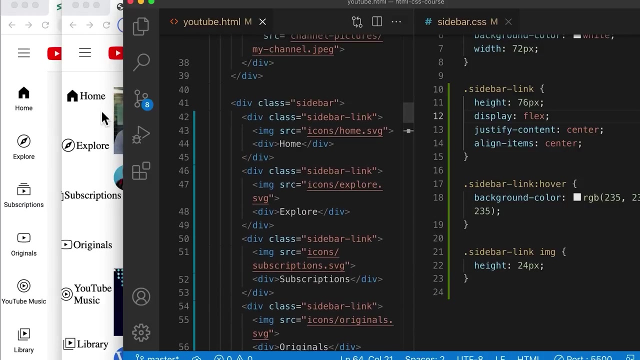 it's going to be called home And I'm just going to copy these and replace it with each of these texts, So explore. this one is subscriptions, originals, YouTube, music and library. Now let's start styling this text a little bit. I'm going to use 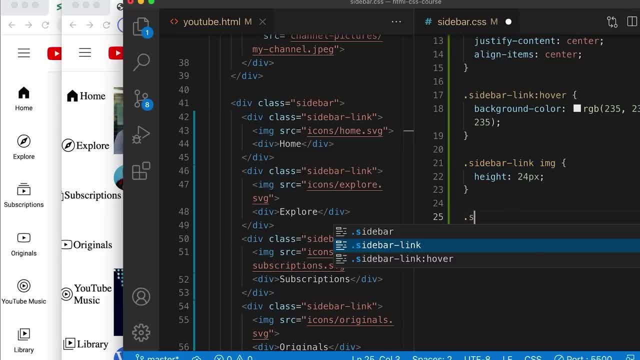 this advanced CSS selector. again, We're going to go into the sidebar link class and then we're going to target all the divs inside sidebar link. So we're going to target divs, So this is not going to target all divs on. 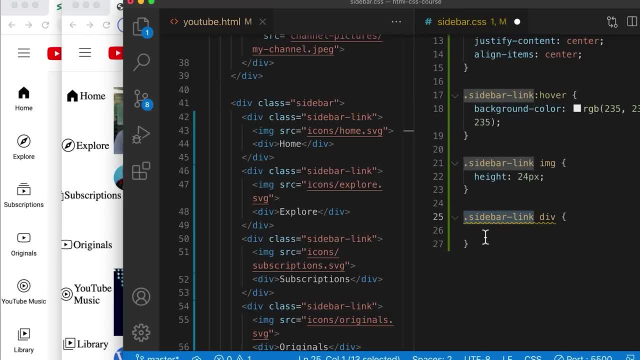 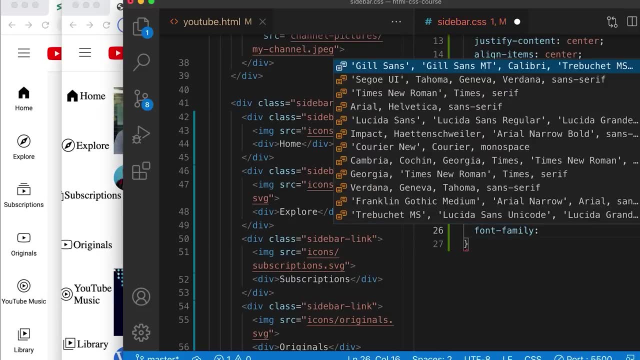 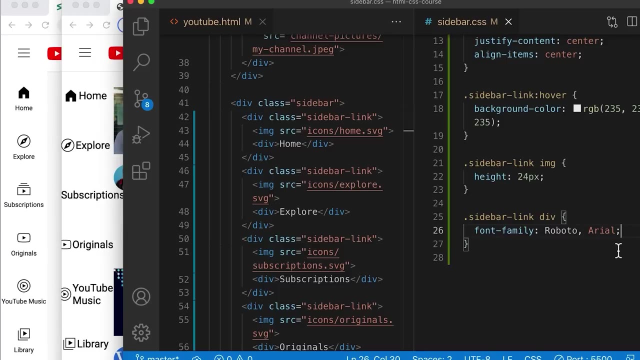 the page, only the divs inside sidebar link. Let's change the font here first, So we'll set the font dash family to roboto comma ario, like before, And let's make the text smaller. next We're going to set the font dash. 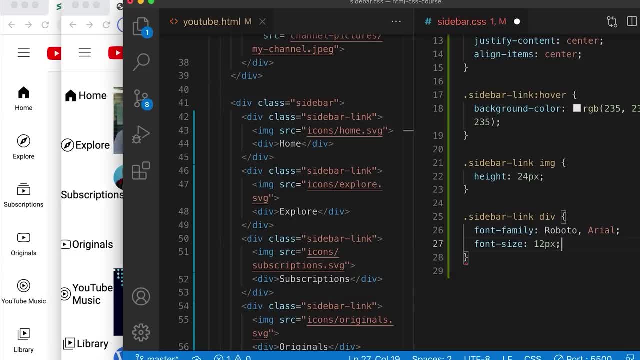 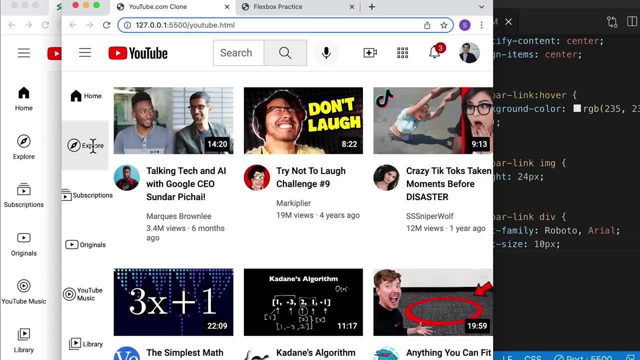 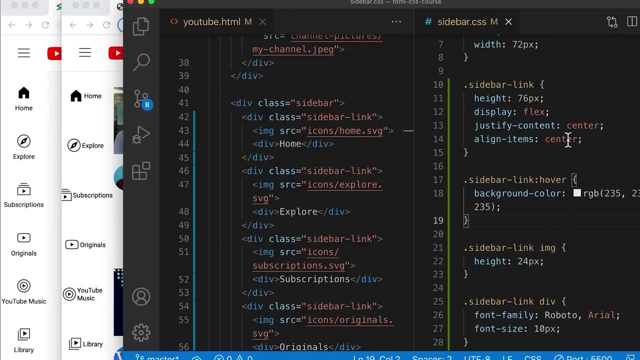 size to maybe 12 pixels, Okay, maybe 10 pixels. Save it. And now the next problem we have is that our elements are appearing beside each other, not on top of each other. So why is this happening? So remember that we can set a property called. 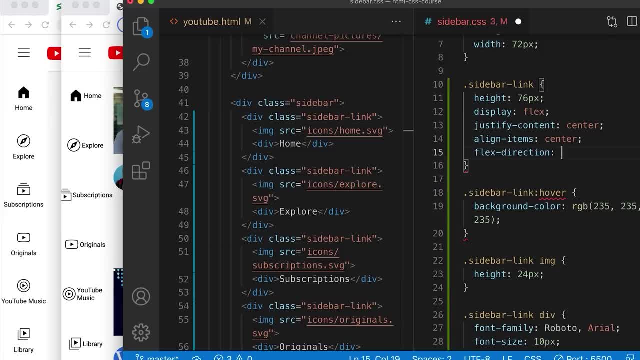 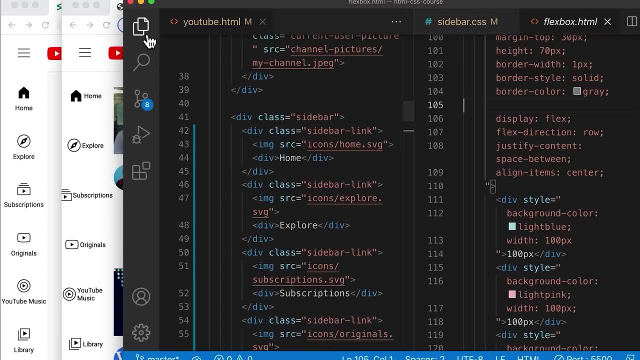 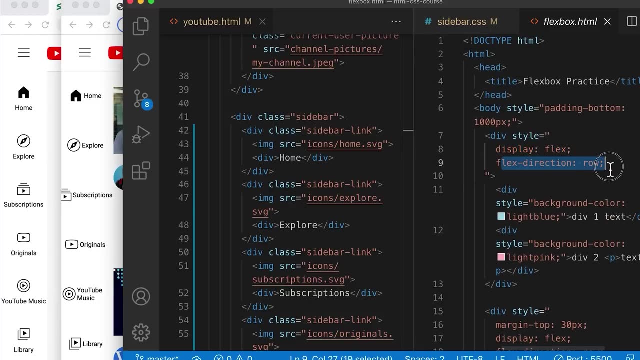 flex dash direction colon row. If we go into our flexbox example flexbox dot html and we scroll all the way to the top, this was the first thing that we learned: Display flex and flex direction row. So if we open this in our browser, 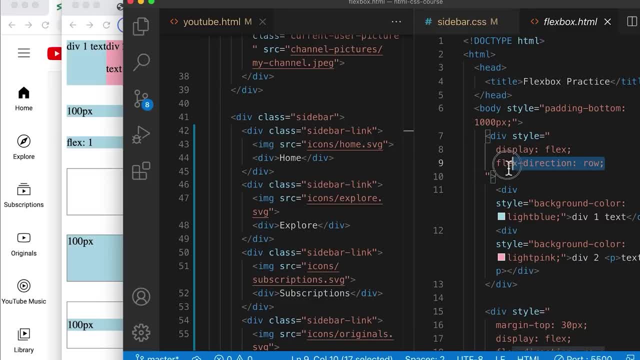 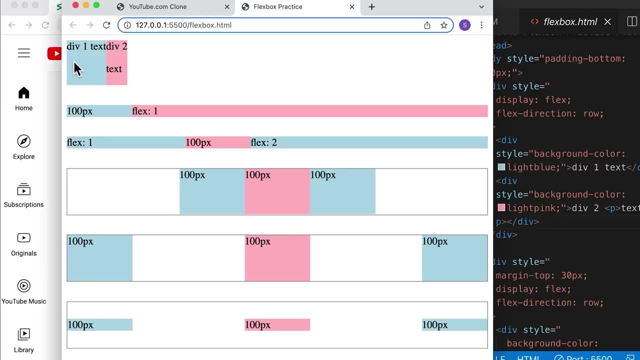 and we scroll to the first example. flex direction row causes our elements to be displayed horizontally, So notice that these two are divs, but they're displayed next to each other, not on top of each other. Now, to change this, we're actually going to go. 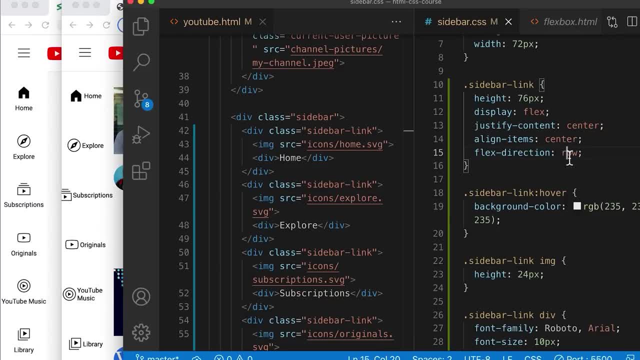 back and we're going to use flex direction column. So where flex direction row displays them horizontally, flex direction column displays our elements vertically. So if we save it now, it's displaying our elements one on top of each other. So this is another direction. 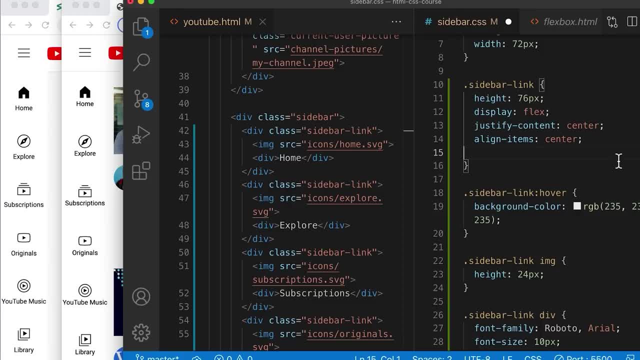 that we can use for our flexboxes. By default, flexboxes are flex direction row, so they will appear horizontally, but we can set flex direction column when we don't want that behavior. So for flex direction column, these two properties are actually. 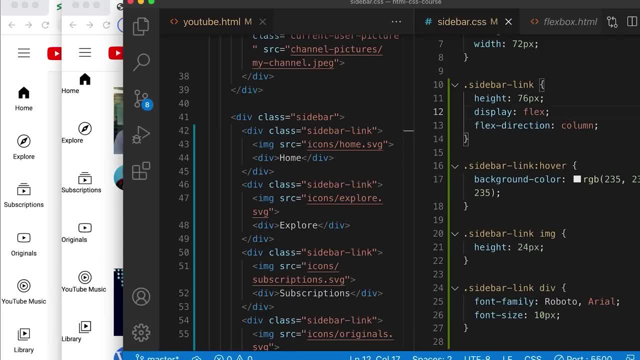 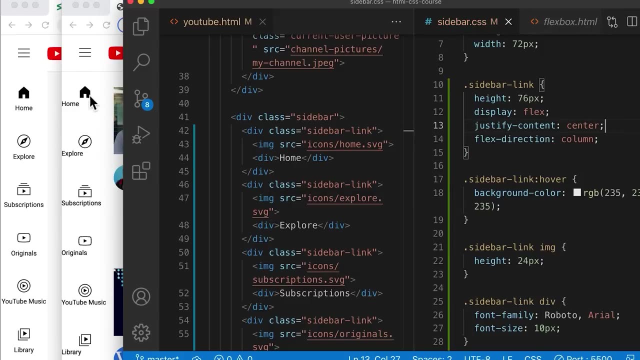 switched. So if I remove both of them first and I first use justify dash content colon center, save it. justify content now affects the vertical direction instead of the horizontal direction with flex direction row. And if I use align dash items center, align items now affects the horizontal direction. 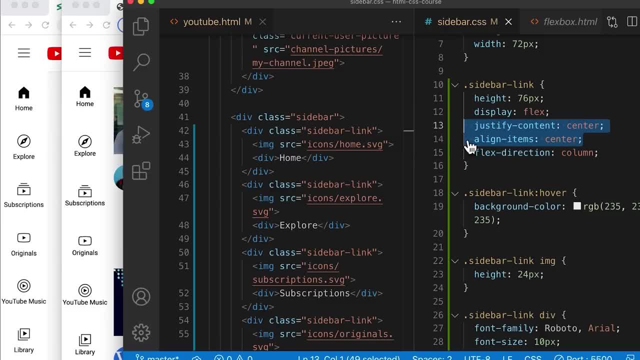 So for flex direction column, these two are reversed. It's a little bit confusing, but the more you use flexbox, the more you'll get used to it. Alright, so we're almost done. We're just going to add some space between these two. 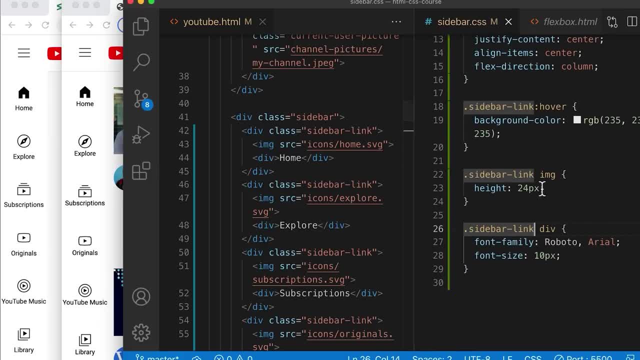 To add some space. let's add some margin bottom to the image. So margin dash bottom maybe 4 pixels. save it. ok, I think that looks pretty close to me And it looks like our elements are a little bit too tall. So I'm actually going to scroll. 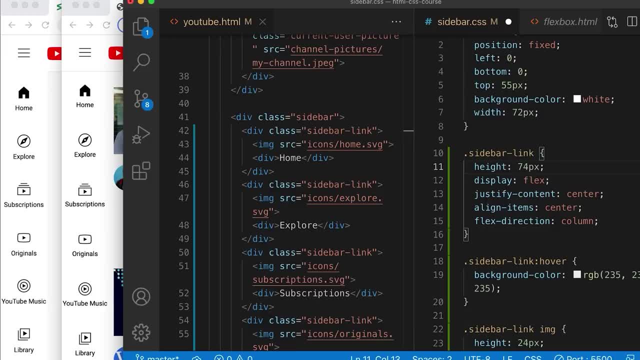 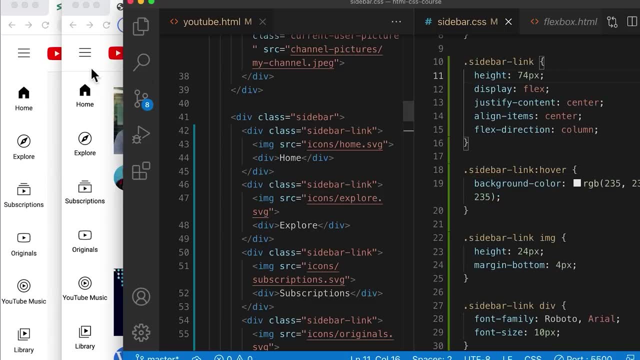 up and adjust the height here to maybe 74. Save it and ok, that looks pretty good. So one last thing with the sidebar is that I noticed in our design it kinda covers the header while ours does not. So to change that, 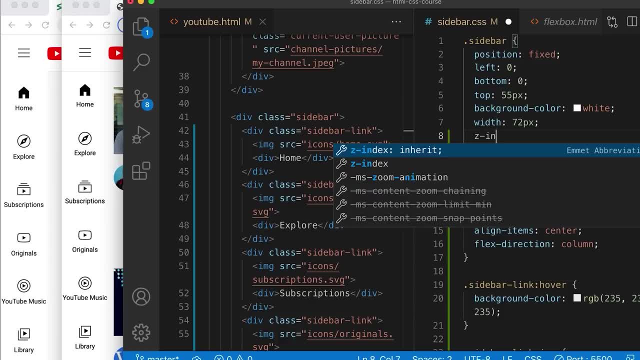 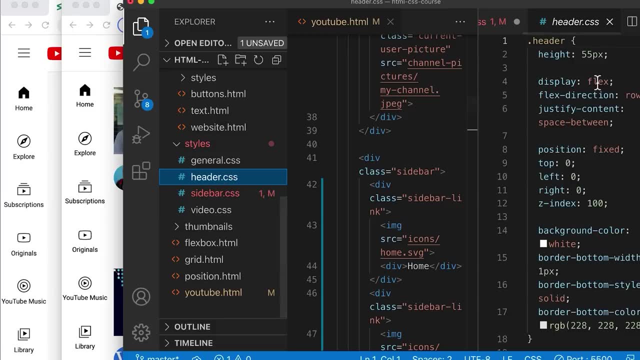 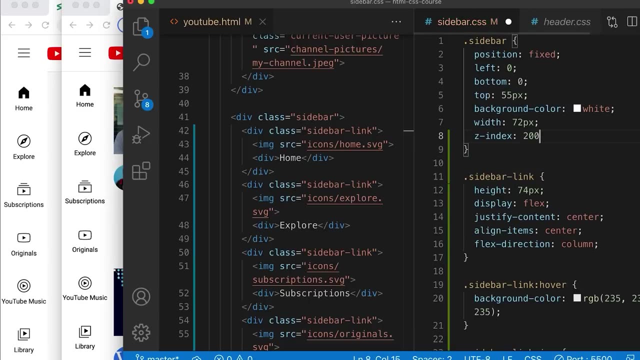 remember we can change the z dash index to be higher than whatever the header is. So if we go into our header styles, headercss, notice that the z index is 100. So we're going to change our z index to bigger than that, so 200. 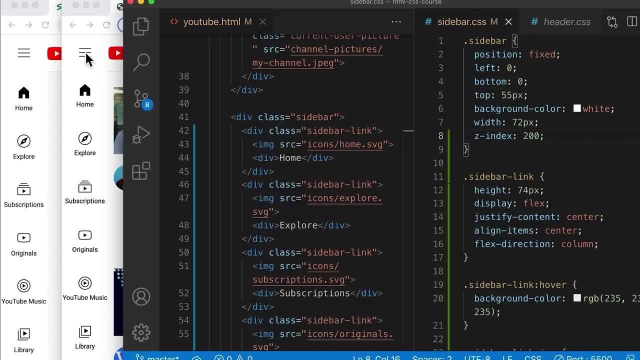 save it. and now our sidebar is covering our header. Next, I want to move all of these icons down a little bit more so that it's aligned. So to do that, I'm going to add some padding or space spacing to the top of this. 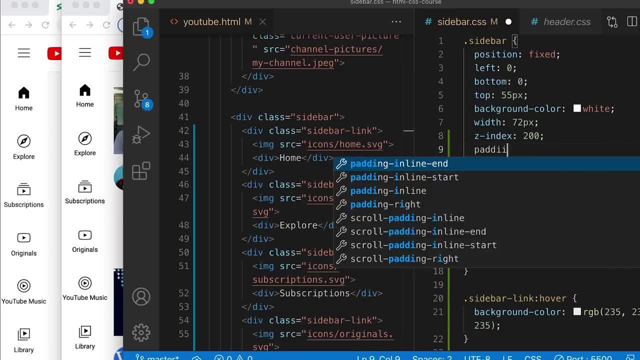 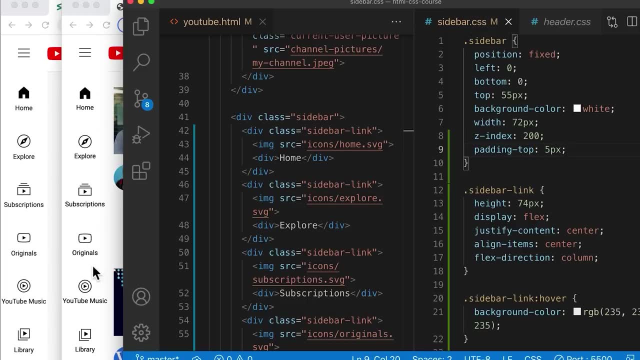 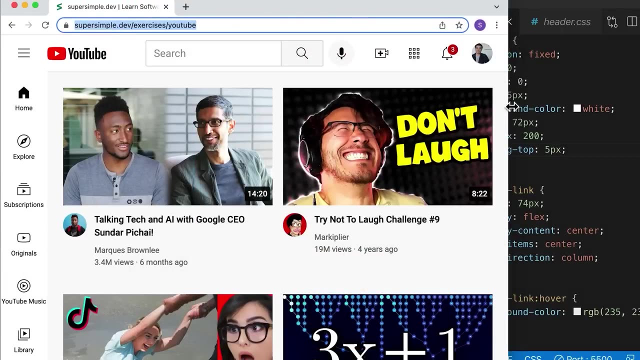 So we're going to add some padding dash top of maybe 5 pixels. see how that looks. Ok, so that looks perfect. And actually one last thing is: I'm going to make the cursor a pointer when we hover over it. So let's go into our sidebar link. 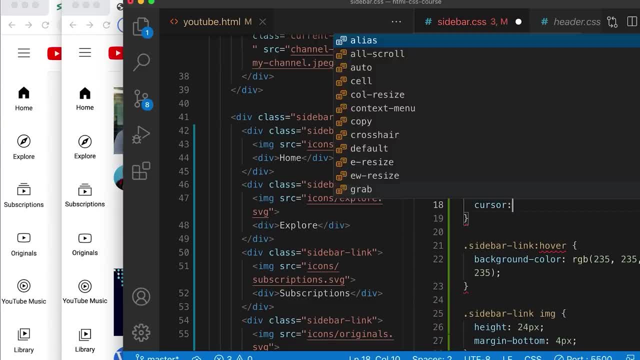 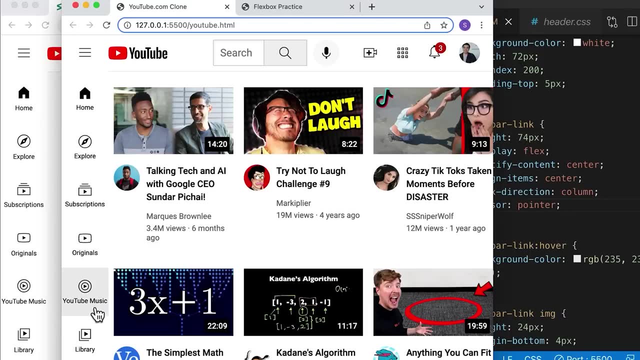 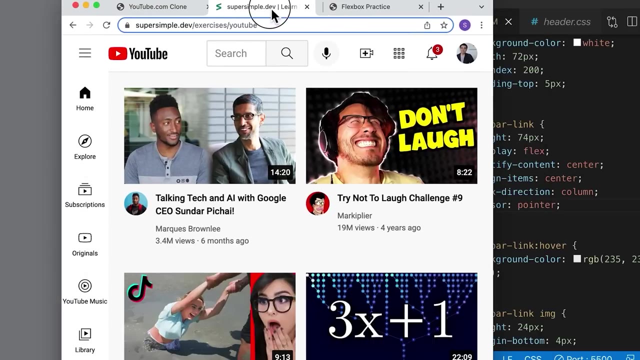 and we'll set the cursor to a pointer, Save it. and now this looks good to go. Next, we're going to resize these videos to match the design, So I'm going to move this back into one window and we're going to resize. 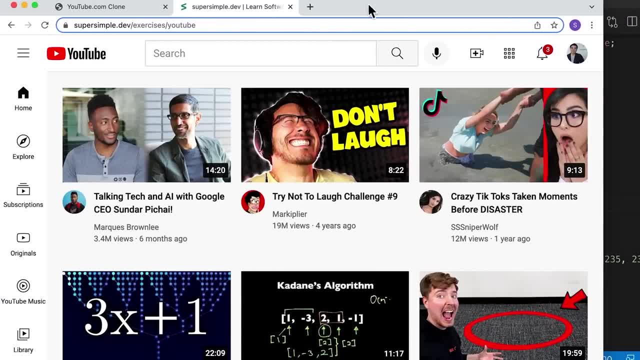 this so that we have 3 videos in each row And now we can properly switch back and forth to compare. So as I switch back and forth between these, you can see that there's a size difference between the videos. So we're going to fix that. 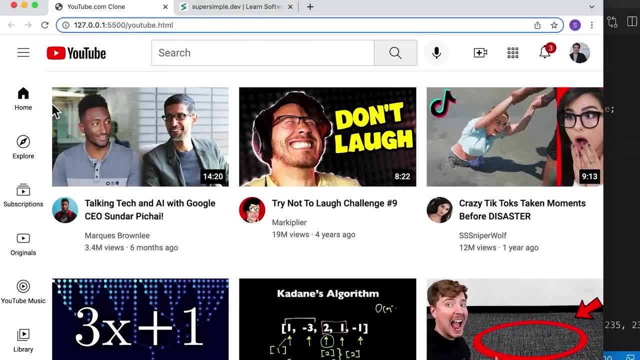 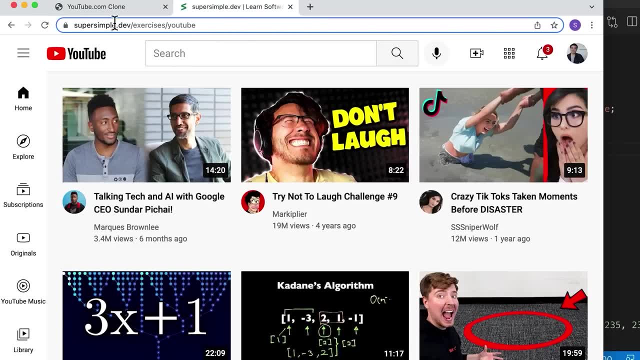 So for our website. I noticed that the left edge here can be moved to the right a little more. So if we look at our design, it's more to the right. Go back to our current project design. more to the right, So to. 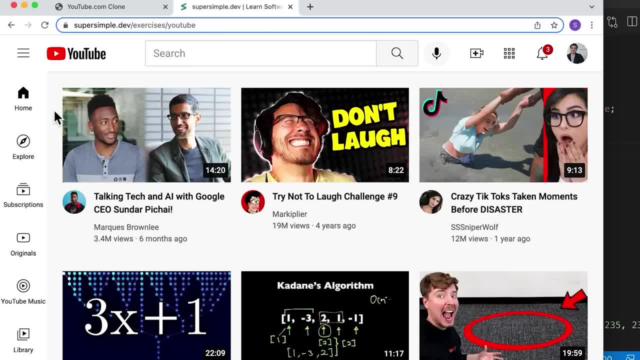 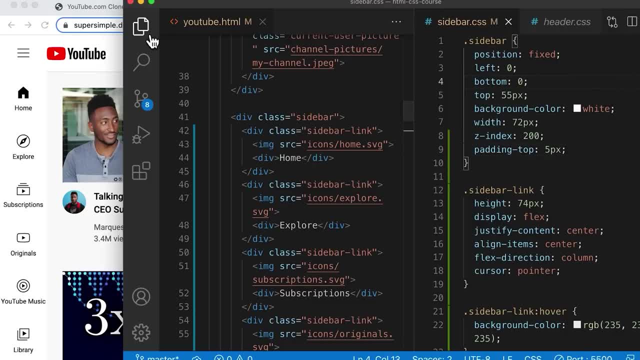 move this to the right. we're actually using padding, So we have to increase our padding on the left side of the page. Let's go back into our code and we're going to find the padding which is in generocss. So remember, we added padding to the. 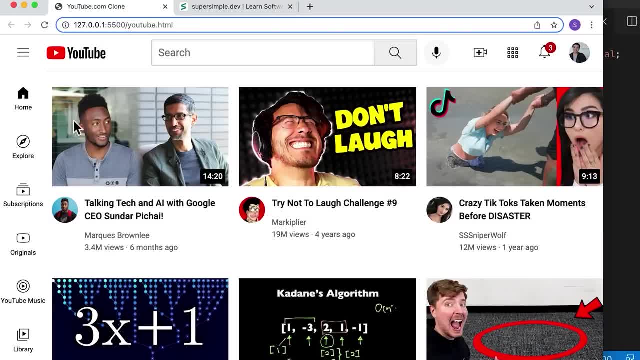 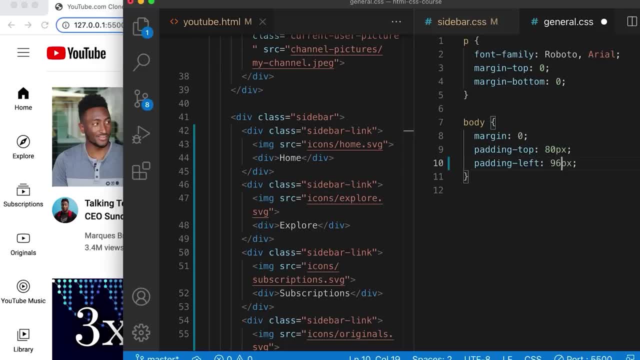 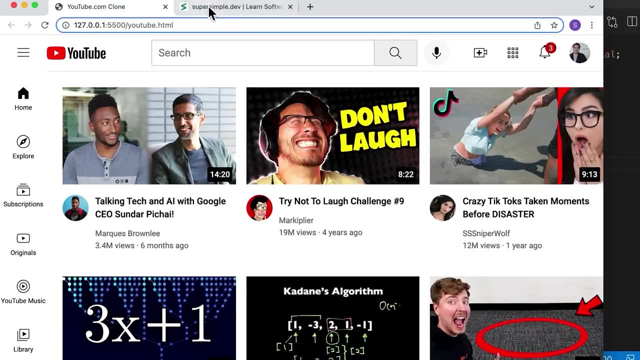 left side of the body. That's what's pushing these elements over here. So let's increase the padding to maybe 96.. Save it And let's compare it to the design. Alright, so I think that looks perfect And we also have padding. 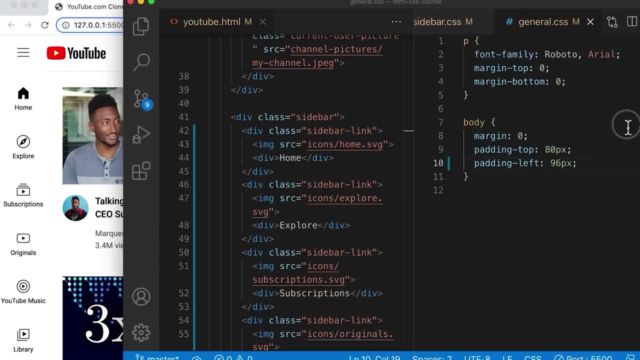 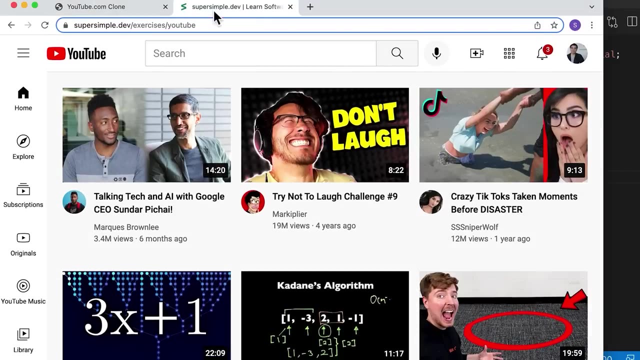 on the right, while our website does not. So let's actually also add padding dash right of 24 pixels. Now, if we save that there and compare it to our design, our videos are now exactly the right size. So that looks great to me. 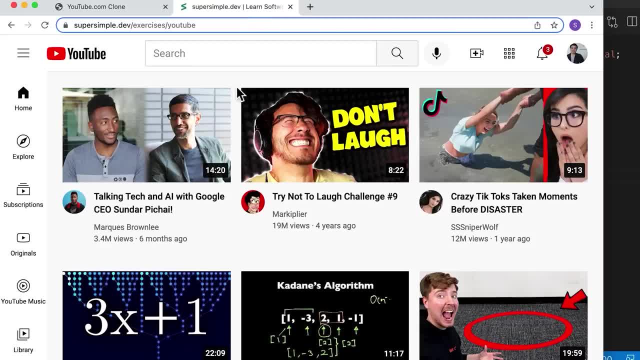 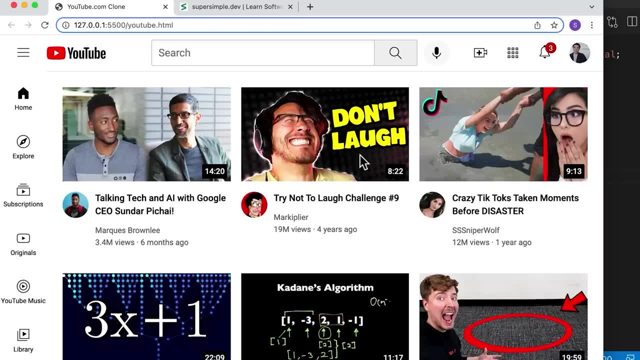 The next thing we're going to tweak is, if we look at our design, the background color here is a light gray, While our background color is white. So we're going to make the background color of our entire page a shade of gray, like this: 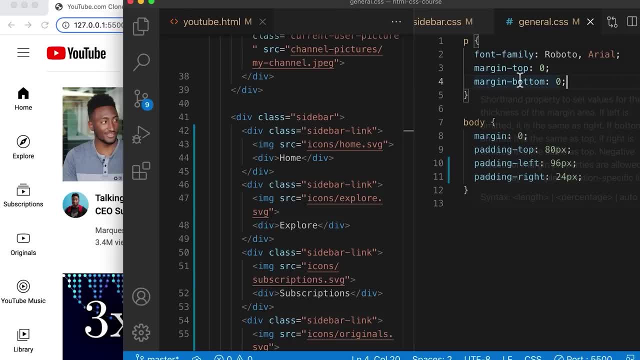 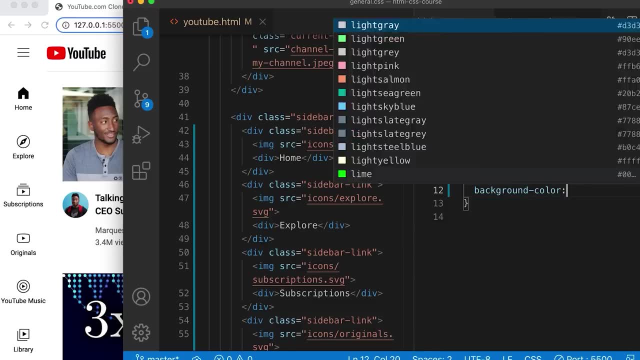 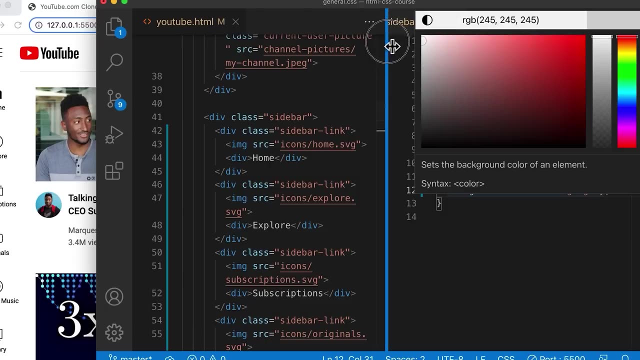 So let's go into our css and in our body styles in general. css: let's set the background dash color to light gray- And I'm going to hover over this- and select a lighter color, Maybe 248.. Save it And let's compare. 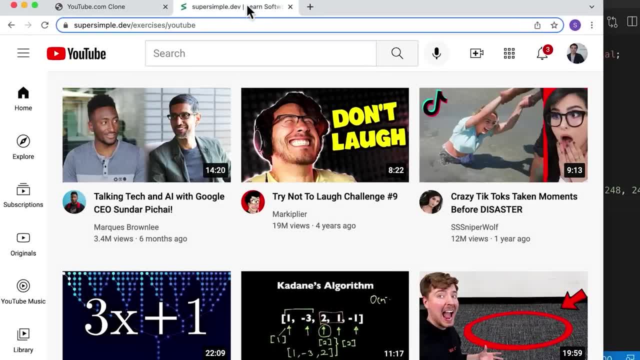 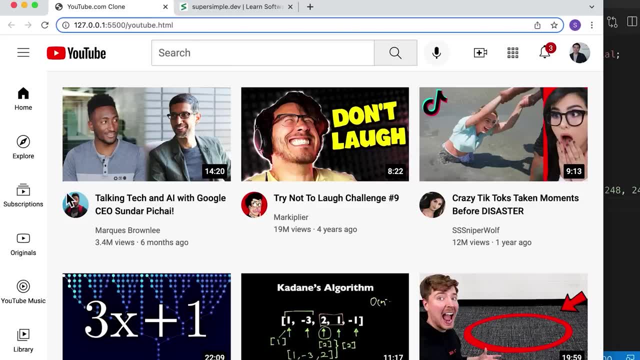 it to our design. So this is our website, This is the design. I think that looks pretty close, And the last few details I want to adjust is this part. So if I look at my design and I compare it to my website, 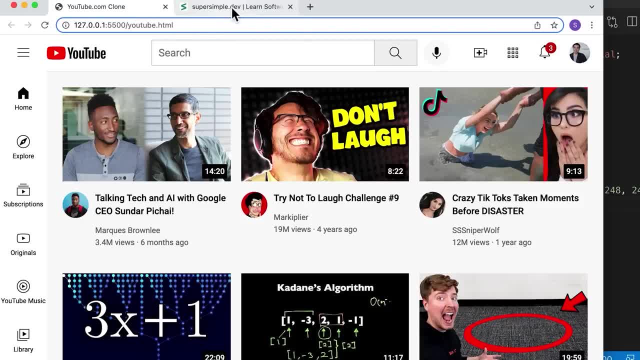 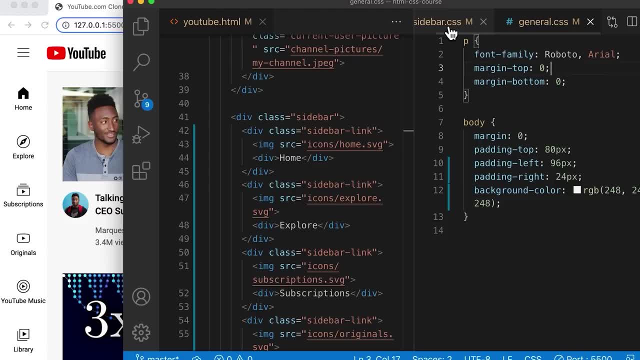 it looks like our channel pictures are a little bit too big, So if I look at the design here, we could make them a little smaller. So let's go into our code And we're going to go into the video styles. Let's open. 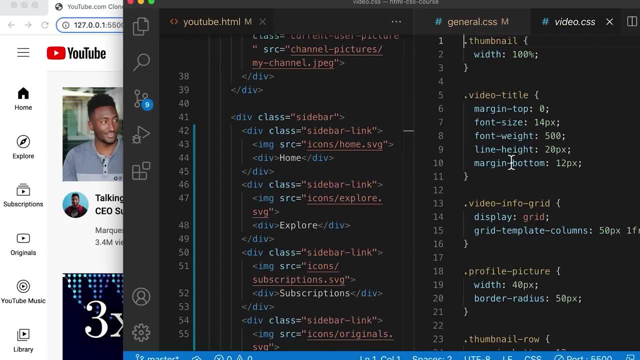 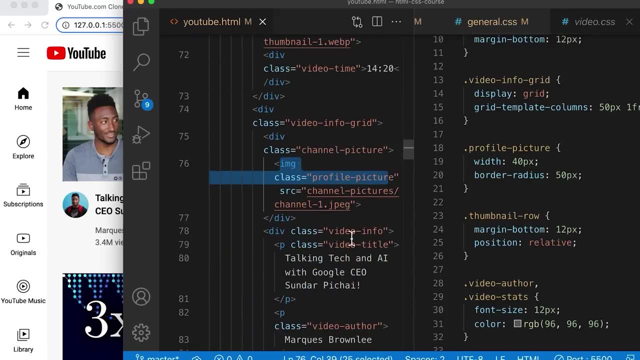 videocss. We're going to find the profile picture, So if I scroll down. so this image here is the channel picture. It has a class of profile picture. We're going to decrease the width to maybe 36.. Save it. 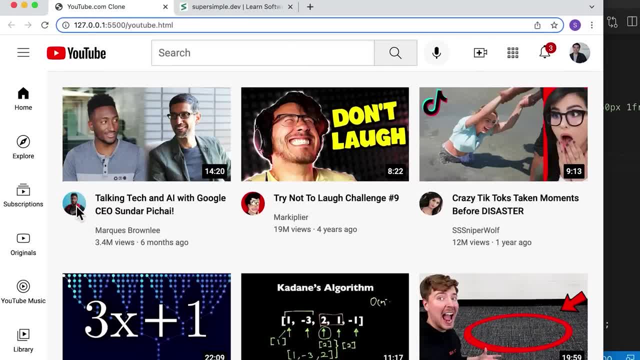 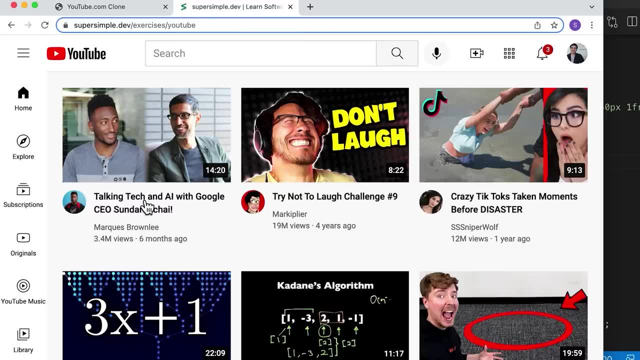 Compare it to our design. Okay, so I think that's the right size. Next, I'm going to adjust some of the spacing here. So if I compare it to the design, there's actually a little bit less spacing here than our website. 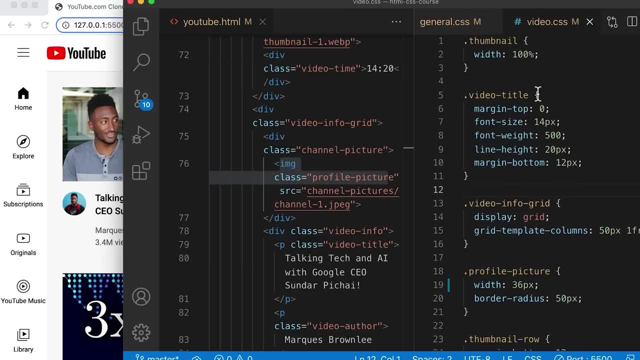 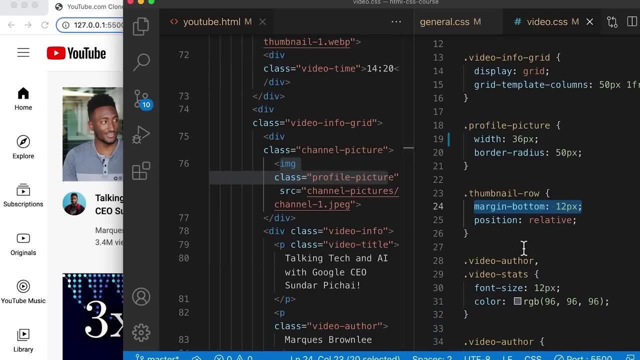 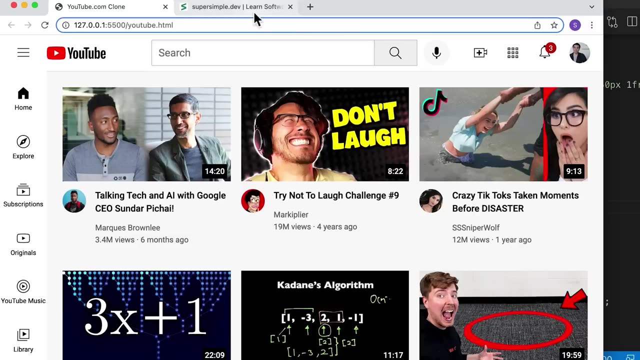 So I'm going to decrease that. So for our website, we're adding some margin bottom to the thumbnail, The thumbnail row. I'm going to decrease this to maybe 8 pixels. Let's see how that looks, Then compare it to our. 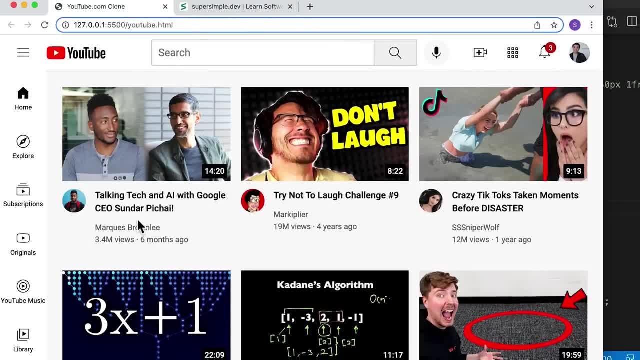 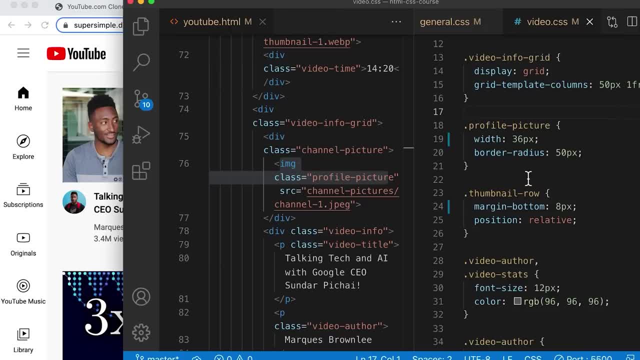 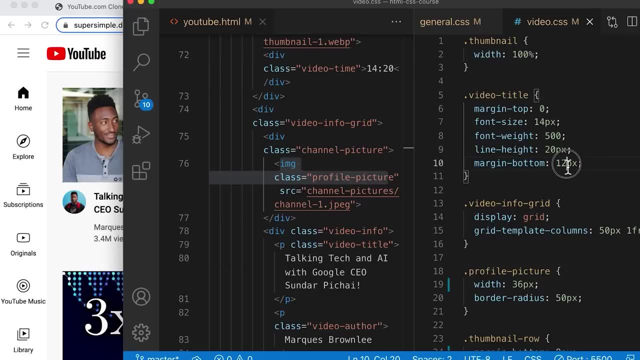 design Okay, so I'm pretty happy with that. And finally, I'm going to adjust the spacing between these two. So for our video title, we go into our code And scroll up here. It has a margin bottom of 12.. I'm going to decrease it. 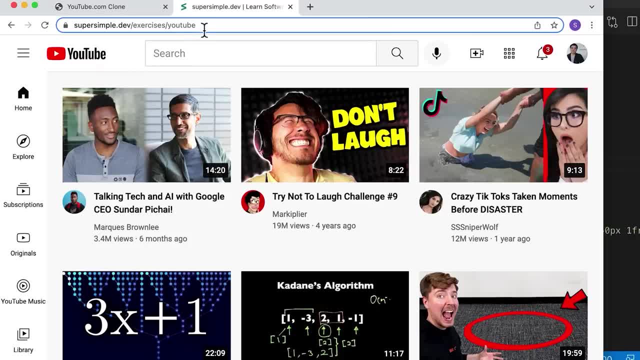 a little bit to 10. Save it And compare it. Okay, so I think that's good enough. It doesn't have to be perfect, It's a little bit off, But I think that our current website here looks really good to me anyways. 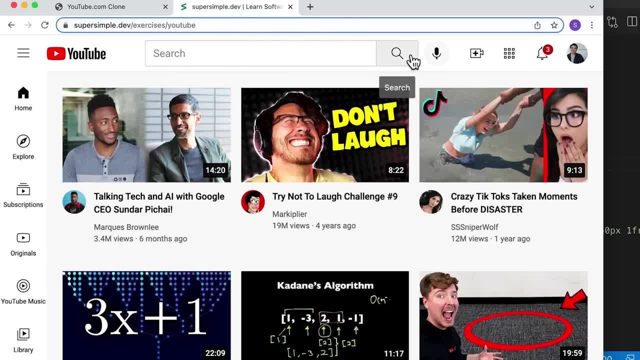 The final thing we're going to do in this lesson is we're going to create these tooltips when we hover over these icons. So, before we learn how to make these appear when we hover over, let's just create these tooltips and place them below each icon. 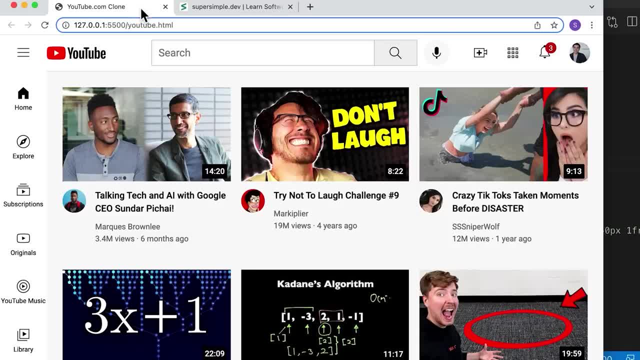 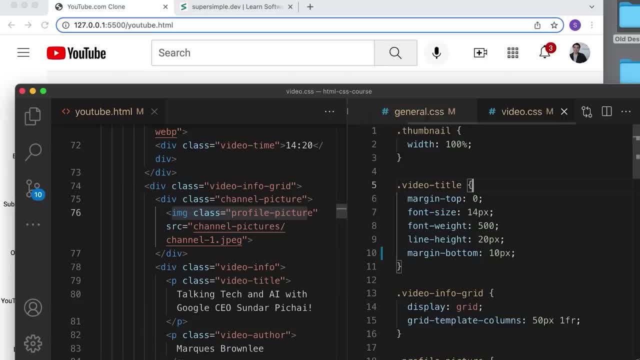 So let's go into our website And we're going to add some tooltips to these, So we'll go into our code And I'm going to resize the windows so we can see better. So we're going to go into our HTML. 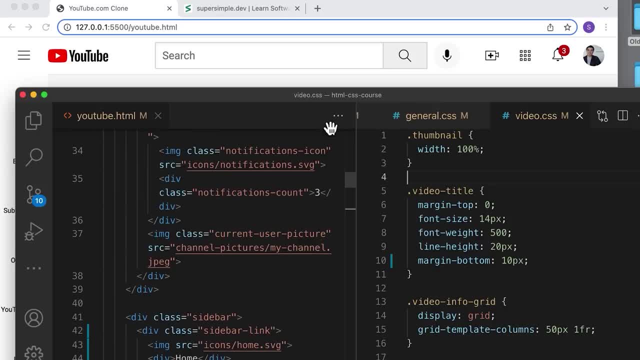 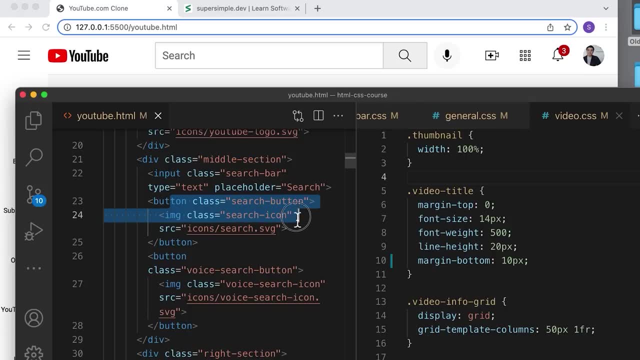 We're going to scroll up to our header And let's first find the search icon here, Which is in the middle section, and then the search button here, So to create the tooltips, we're actually going to use the position property that we learned earlier. 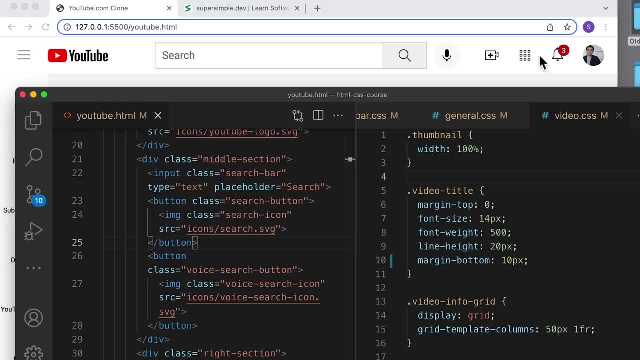 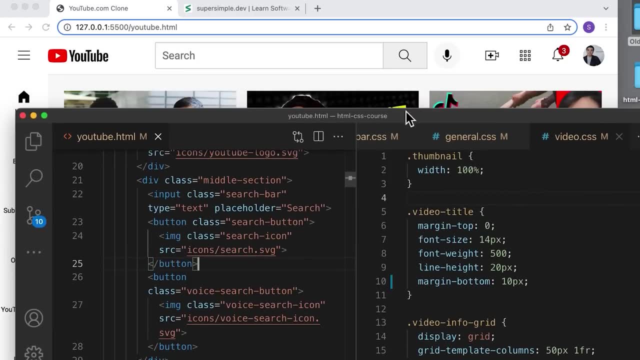 So remember that we used position to put this number in the top right corner. We're going to use position to put a tooltip below the element right here, So let's first add a tooltip inside the button. So we're going to create a div. 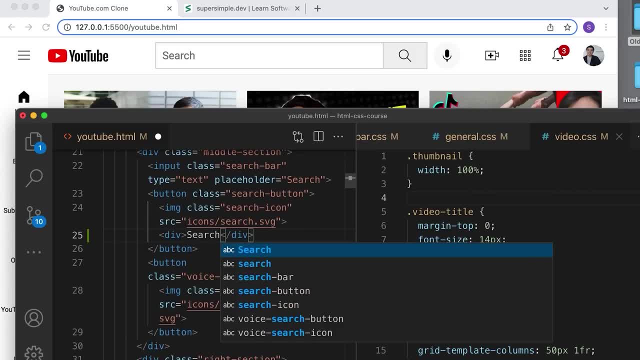 And let's call this search, Let's save it, And now that's our tooltip. And now we need to position this tooltip relative to our button. So remember from the previous lesson: we need position absolute, inside position relative. So let's first, 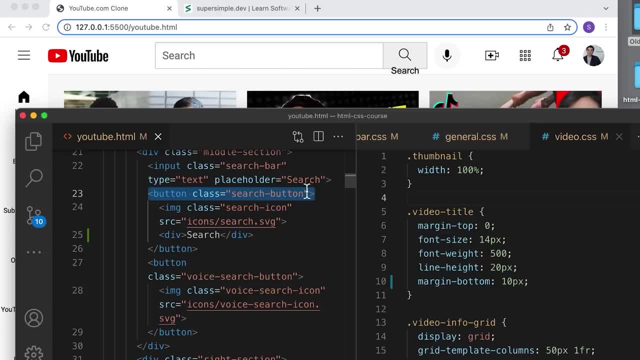 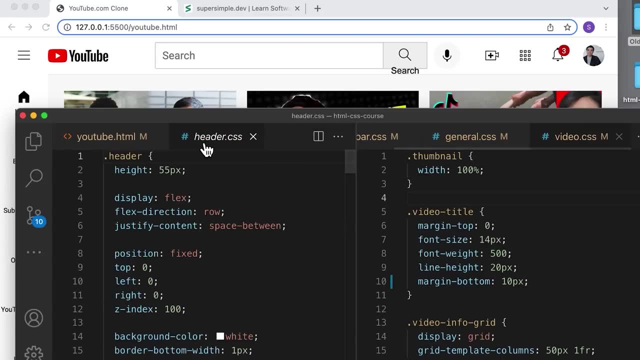 add those position properties. We're going to go into the header CSS file because we're working with the header, So let's open that up And I'm going to move it to the right side here And now we're going to scroll down. 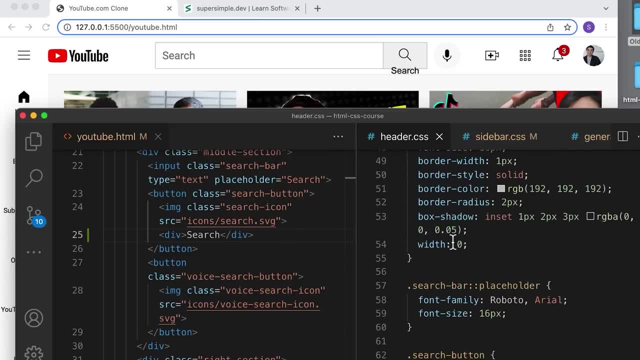 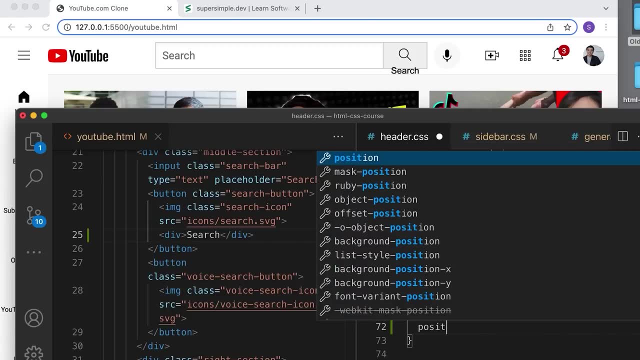 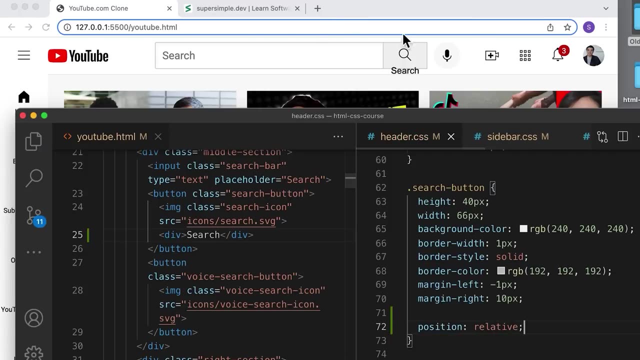 until we find our search button. So I'm going to scroll, scroll, scroll And it's right here. So we're going to set this search button, which is our container, to position colon relative, Save it And nothing happens, because that's how position relative. 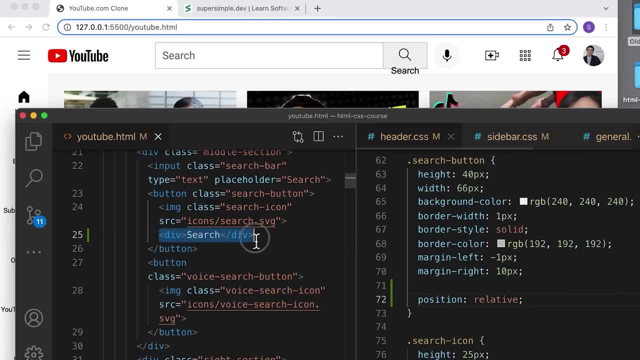 works. And now the magic comes when we set this to position absolute. So we're actually going to set a class here so that we can target it a little easier. We're going to call this tooltip And we're going to use that advanced CSS. 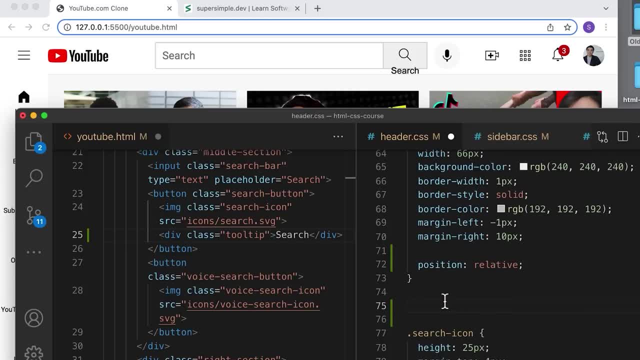 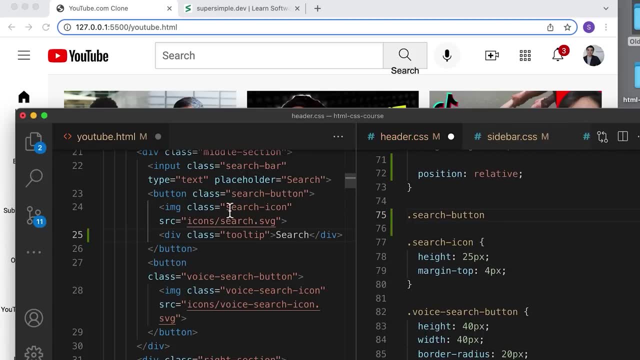 selector. we learned earlier. So we're going to target search-button first, And then we're going to type a space, And then we're going to type tooltip. So this means that we're targeting the tooltip class not on the entire page, but only inside. 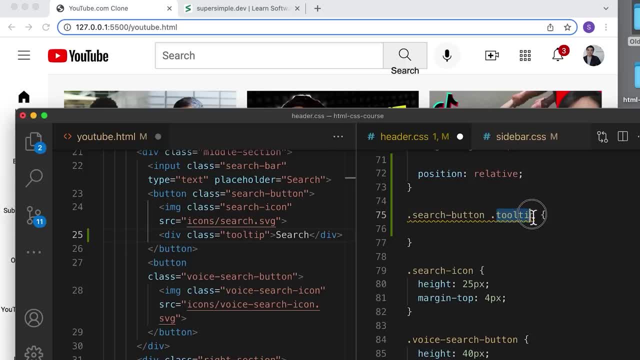 the search button. So now we don't have to come up with a unique name for this specific tooltip. So if we save it, we're going to set this to position absolute, And now we have an absolute element inside a relative element. So if we save, 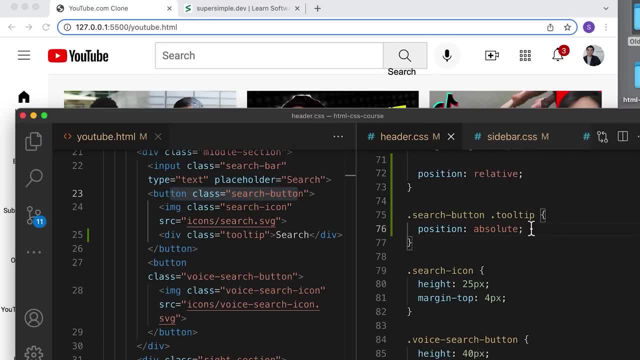 that now we can start positioning this. Let's give a background color so that we can see it better, So background-color of, maybe gray, And let's set the text color to white, So color colon: white. Let's give it some padding on the inside. 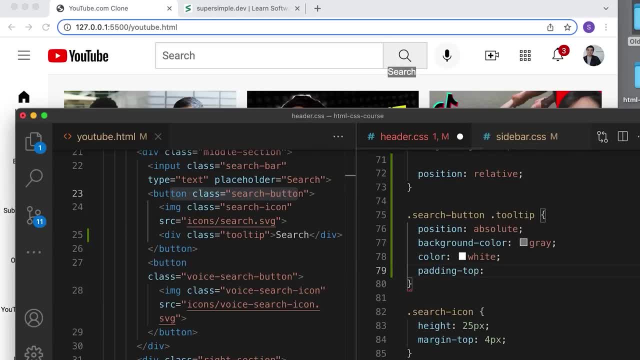 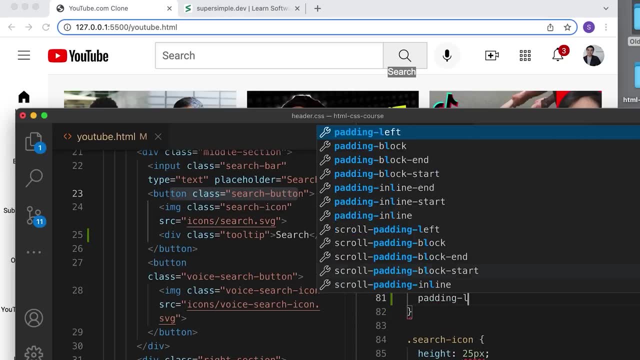 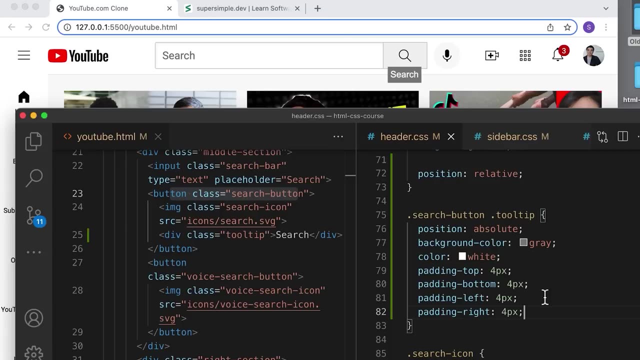 So padding-top of maybe 4 pixels, Padding-bottom 4 pixels, Padding-left 4 pixels And padding-right 4 pixels, Save it And let's actually increase the padding on the left and right to 8.. See how that looks. 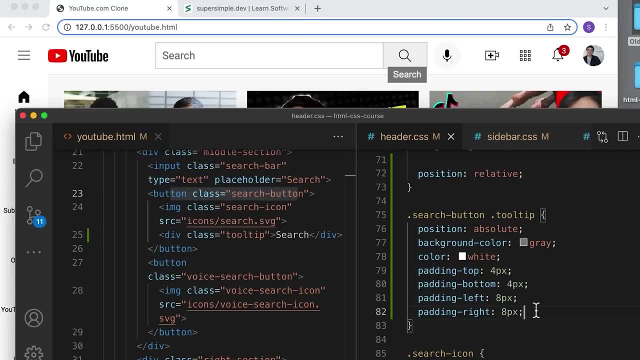 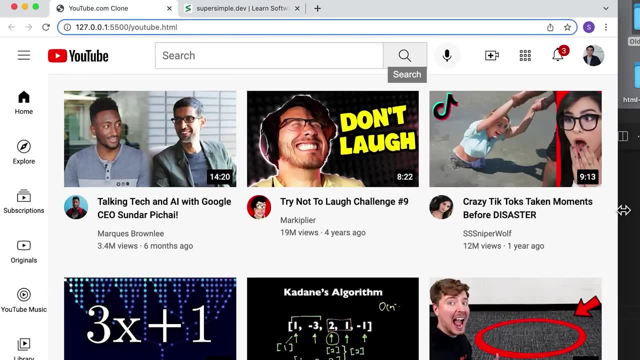 Okay, I'm pretty happy with that, And now I'm going to set some rounded corners, So we don't have to exactly match our design. We can make it close enough So we can set some rounded corners. Border-radius of 4 pixels. 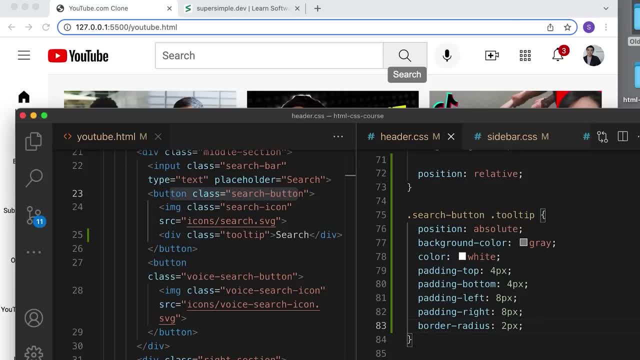 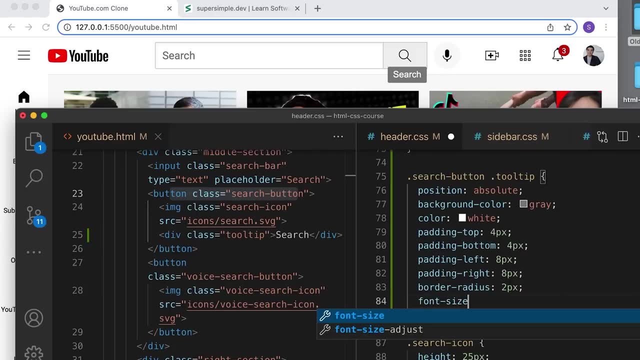 It's a little too much for me. Set it to 2 pixels, And I'm also going to make the font a little bit smaller. So I'm going to set the font-size to 12 pixels. Save it. I think that looks. 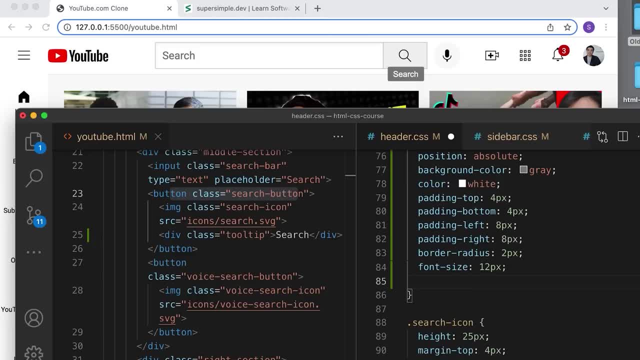 pretty good to me. Next, we're going to use the properties top, bottom, left and right to position this within the relative element. So for our cases, let's start with bottom 0.. So this means that the bottom of our tooltip will be at the bottom. 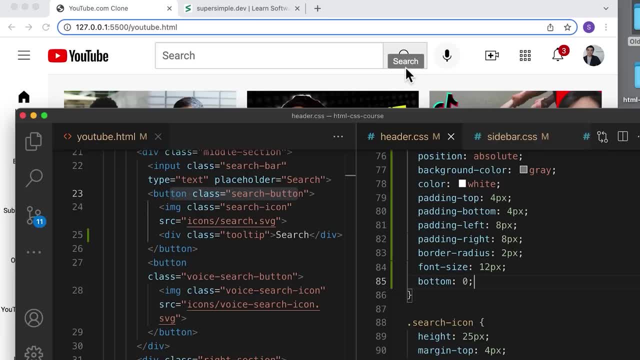 of the button. If I save this, that's exactly what we have Now. to move it even further to the bottom, we're going to use negative pixels, So let's set negative 20.. Save it, Okay. so I think that's looking pretty good. 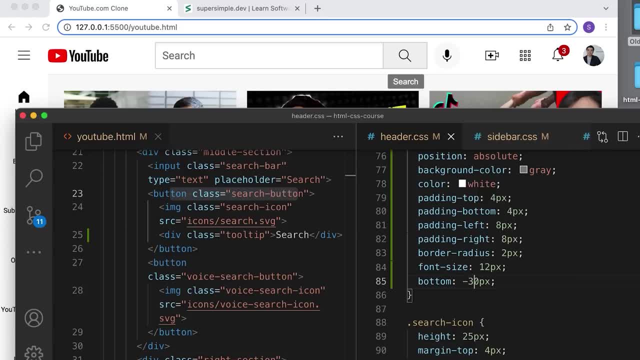 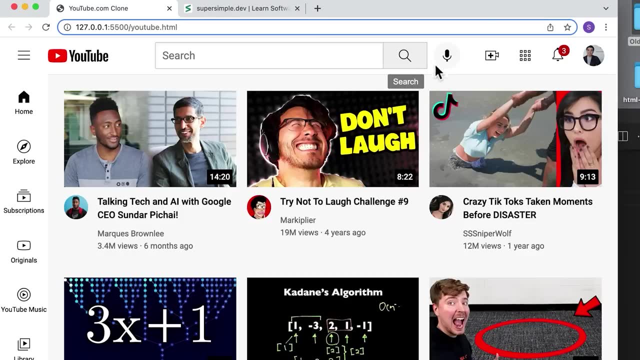 Let's increase it a little bit more. Let's increase it to 30 pixels, Save it Okay. so I'm happy with that position. Now we're going to learn how to make this tooltip appear when we hover over this button. So the trick here is we're going to 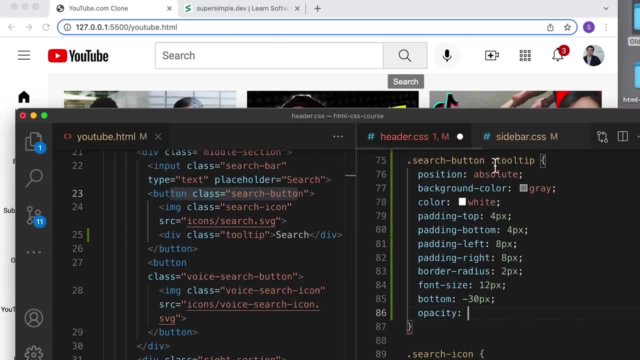 set the opacity- or how see-through the tooltip is- to 0,, which is completely invisible, And then, when we hover over this button, we're going to set the opacity to 1.. So how do we actually change this when we hover over the button? So we're actually 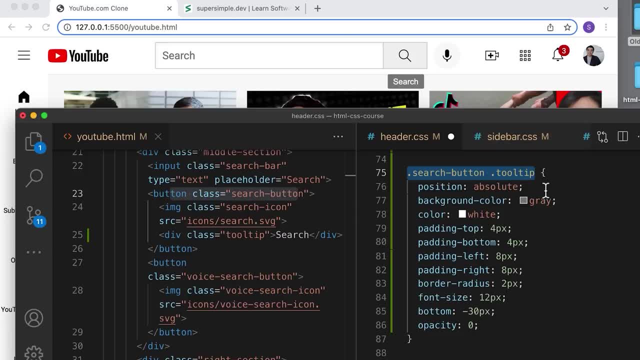 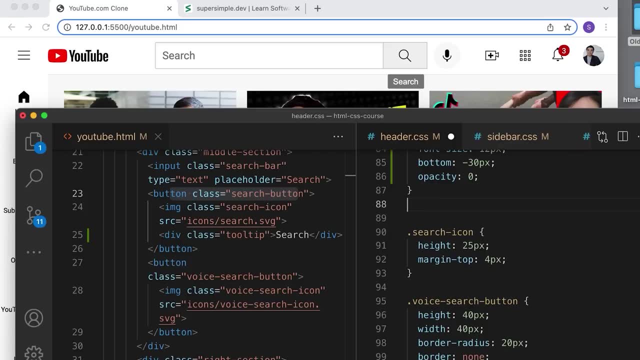 going to use a combination of this advanced CSS selector and pseudo-classes which are like hover. So first we're going to target the search-button class and we're going to add a pseudo-class, colon hover. And now we're going to type another selector. We're going to 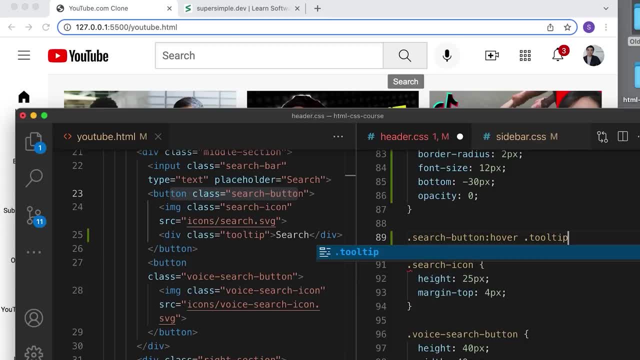 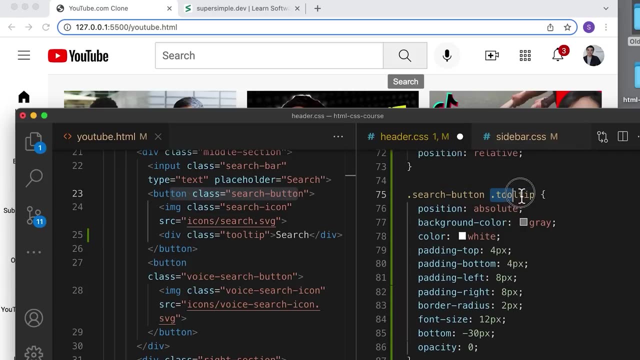 type tooltip And we're going to set some styles here. So what this does is that we're going to target the tooltips only when we're hovering over this search-button. So up here, notice that we're targeting the tooltips inside the search-button regardless. 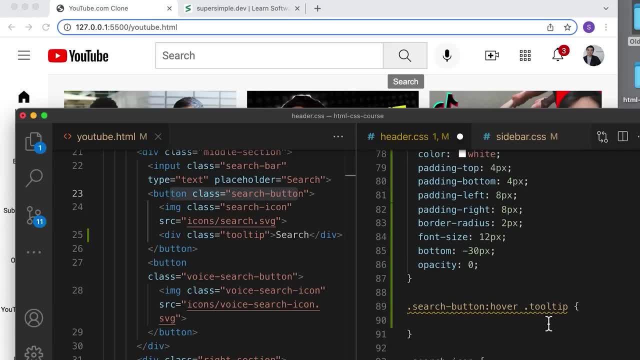 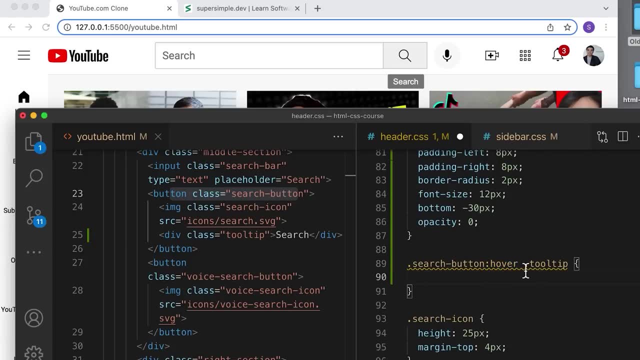 of whether we're hovering over it or not. In this case we're going to target all tooltips inside the search-button, but only when we hover over it. So when we hover over it, we can set the tooltip opacity to 1.. 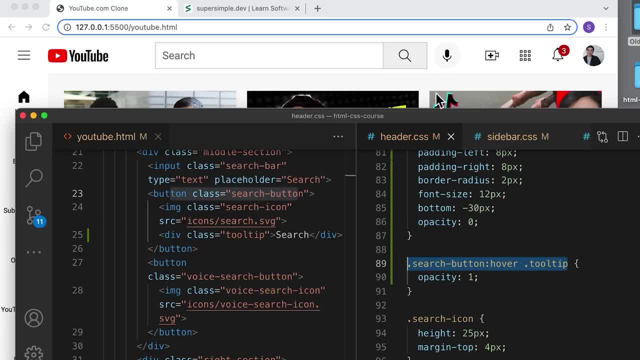 So this is a neat trick that you can do to create tooltips like this. So if we go into our webpage when I'm not hovering over the button, you'll notice that the opacity is 0, but when I'm hovering over the button, this tooltip will have an. 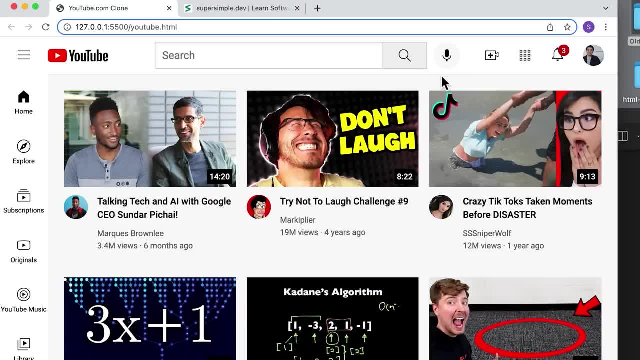 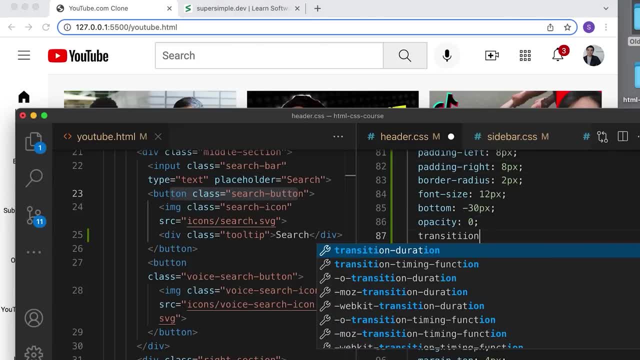 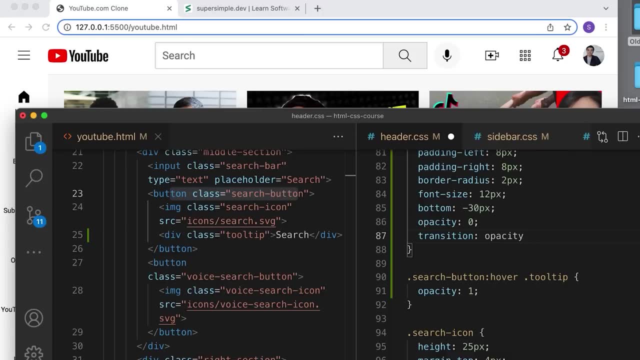 opacity of 1, which looks like this: And now, because we're changing the opacity, we can set a transition. So let's set a transition. We need to tell it what to transition, which is opacity, and how long the transition will take. 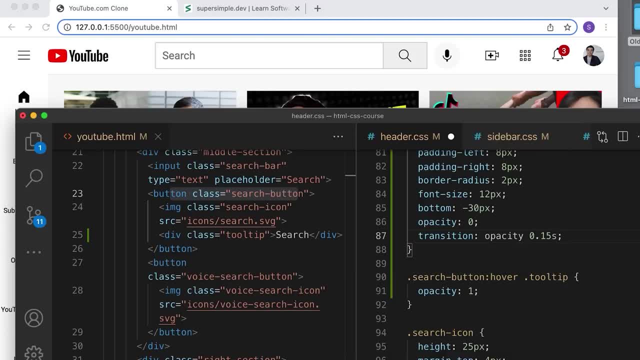 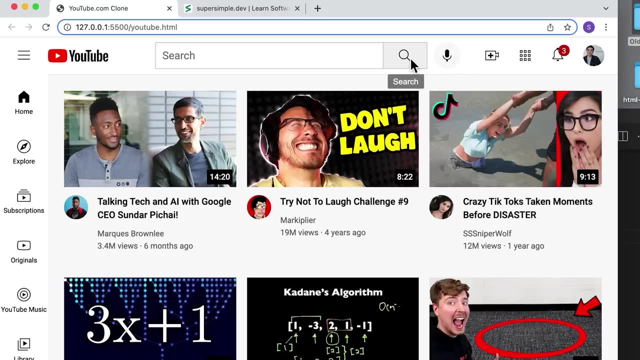 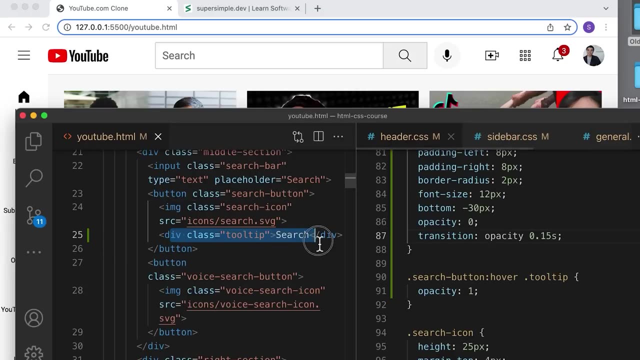 Let's say 0.15 seconds, Save it, and when we hover over this now, we get our tooltips. Now the last thing I want to show you is, if we hover over the actual tooltip, you'll notice that because it's inside this button. 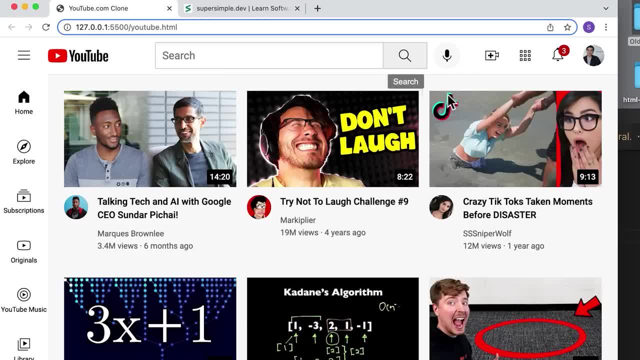 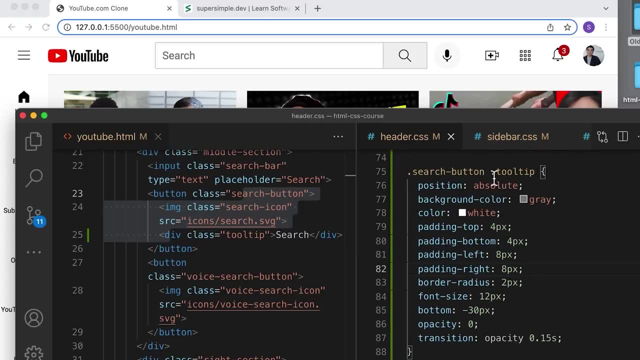 when we hover over the tooltip with our mouse, it also counts as hovering over the button. We can fix this by disabling hovers on the tooltip and only allow hovers on the button. So to disable the hover on this tooltip, we're going to use another CSS. 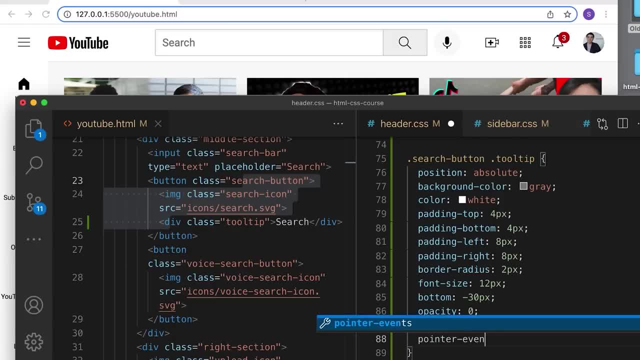 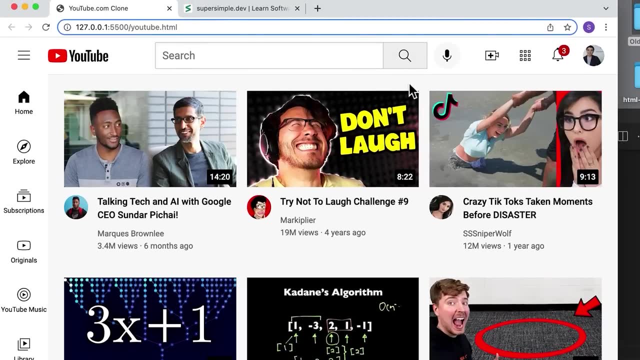 property called pointer-events, colon none. This means that when our mouse hovers over the tooltip, it's not going to do anything. So that's how we create these tooltips on our webpage. Let's do the same thing with this voice search button. 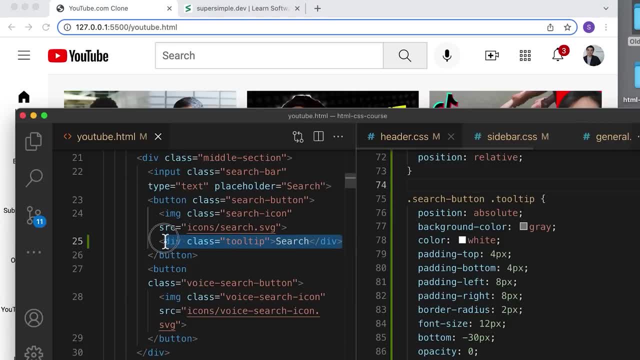 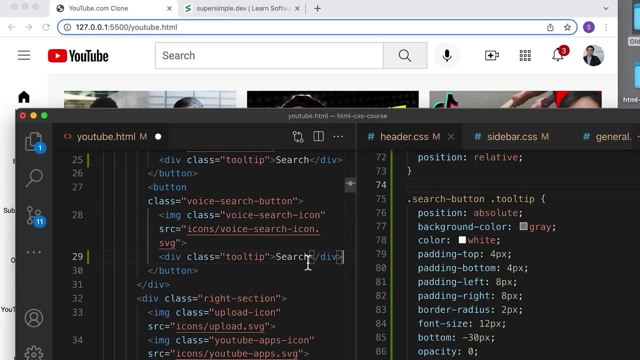 We're going to go into our HTML and we're just going to copy this tooltip and just move it down here into the voice search button, Just like that, And let's change the text to search with your voice. Save it and now remember to position this: 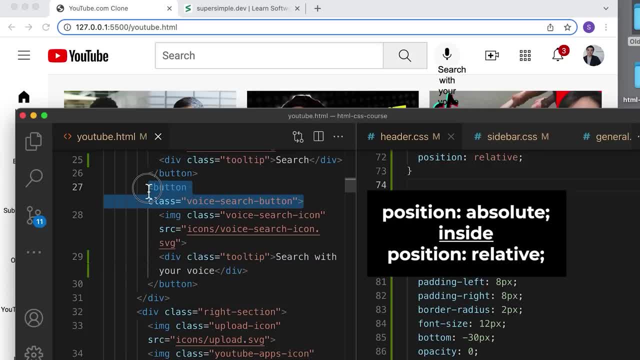 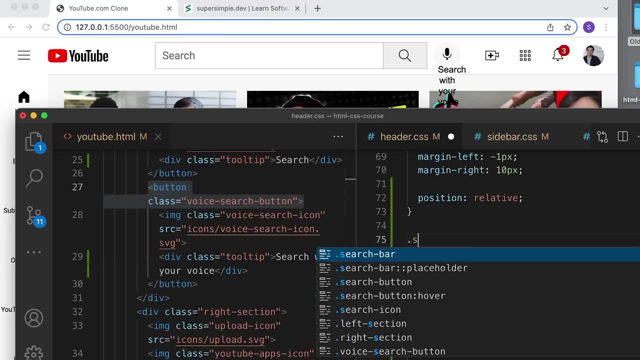 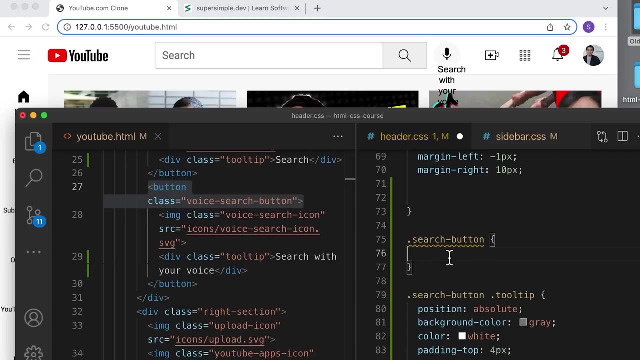 We're going to have position absolute, inside position relative, So let's turn this to position relative first. I'm actually going to make it easier for us. I'm going to first target the search dash button And I'm going to put this inside here. 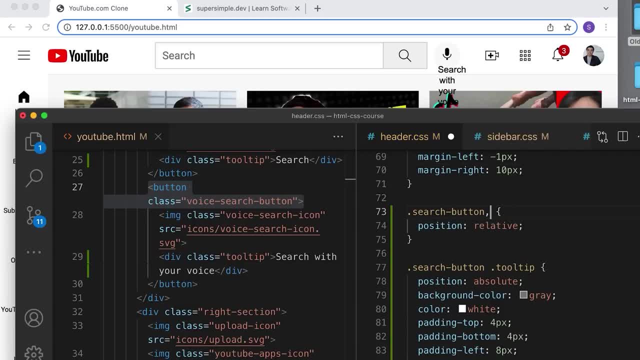 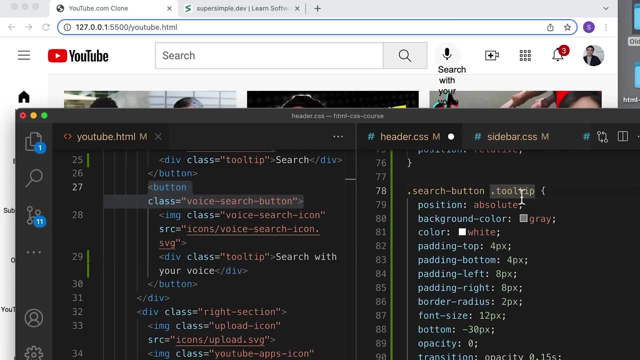 And I'm also going to target with a comma the voice search button. So it's this one. So now this code is going to apply to both of these, So it saves us a little bit of coding. Same thing down here. We're going to apply all of these styles to the. 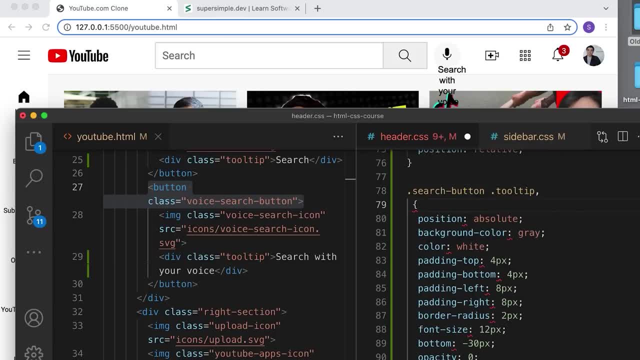 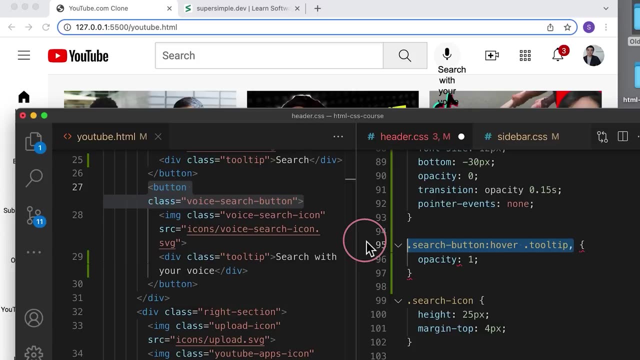 search button tooltip and comma. the voice search button dot tooltip. So using these advanced CSS selectors can save us a lot of code. I'm going to scroll down all the way here too and use a comma and set this to the voice dash search button. So make sure you don't have a comma. 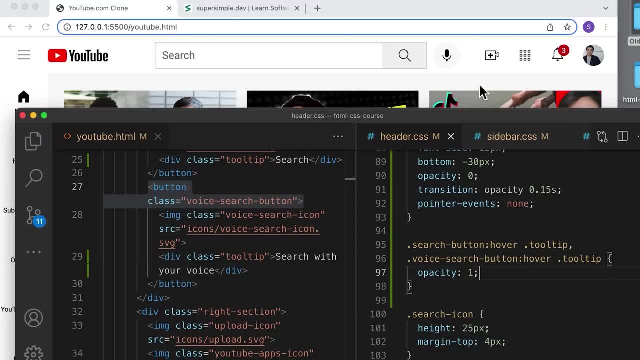 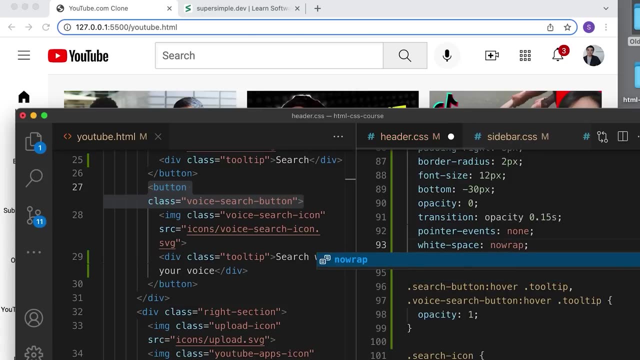 at the end there: Save it. Now, when I hover over this, you'll notice that it doesn't really work because the text is sort of wrapping around. We're going to fix that by setting this property: whitespace, no wrap. Save it And this will prevent. 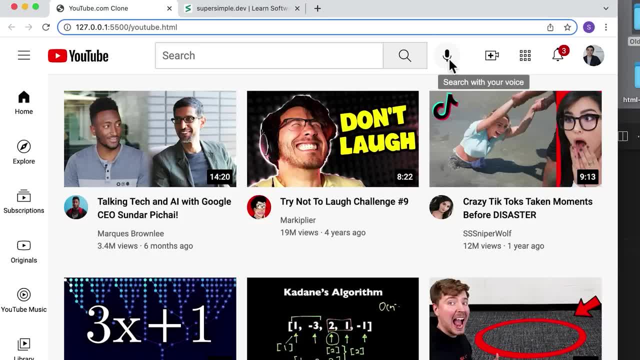 the text from wrapping around. Now, the last thing I want to do is to center this tooltip with the button. To do this, we can use a flexbox, Because, remember, with flexbox we can center horizontally and vertically. In this case, we want to center horizontally. 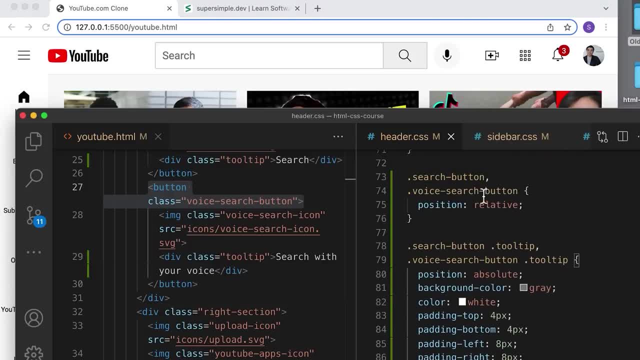 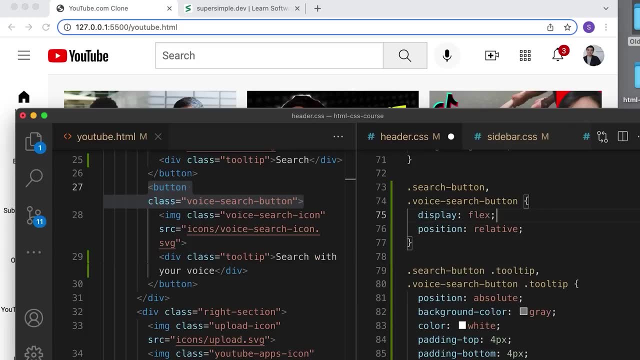 So we're going to make, we're going to scroll up and we're going to make these buttons flexboxes. So let's set display flex by default. it's flex direction row. So justify content is going to center horizontally. Justify content center. 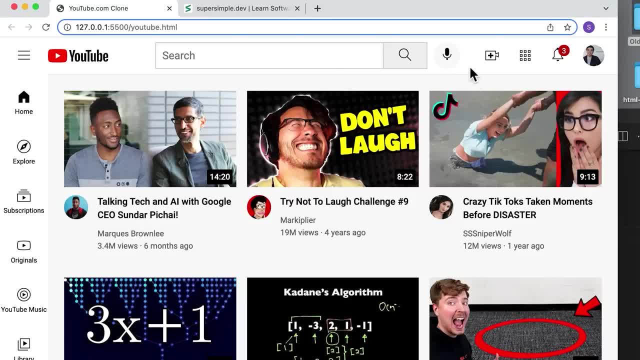 Save it. So now, if we hover over our buttons, you'll notice that the tooltips are aligned horizontally, But you'll also notice that our icons are not vertically aligned very well. So let's go back into our code and we're going to align them in the 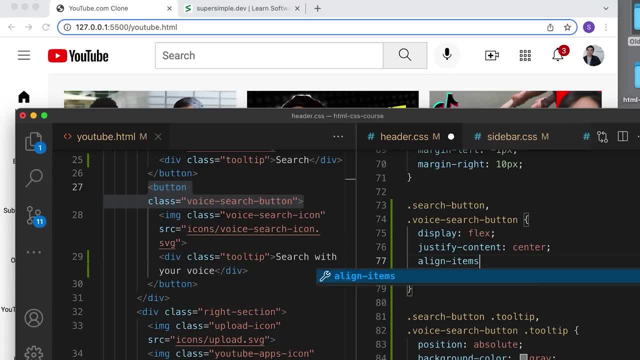 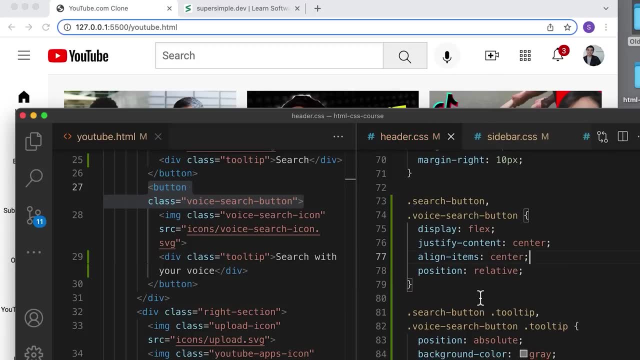 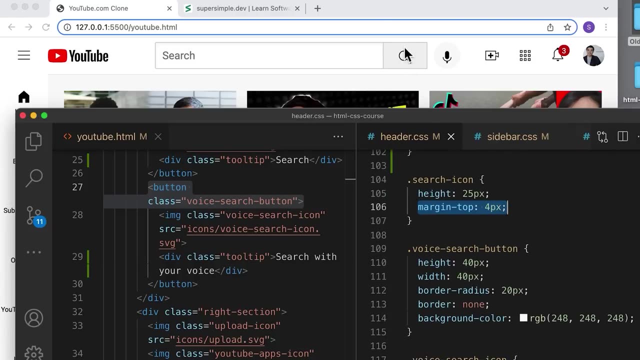 center with align-items colon center, Save it. So that didn't seem to work, but if we scroll down into our code, so way earlier in the course we actually added margin top to the search icon as well as the voice search icon. So we just need to get rid of this margin top. 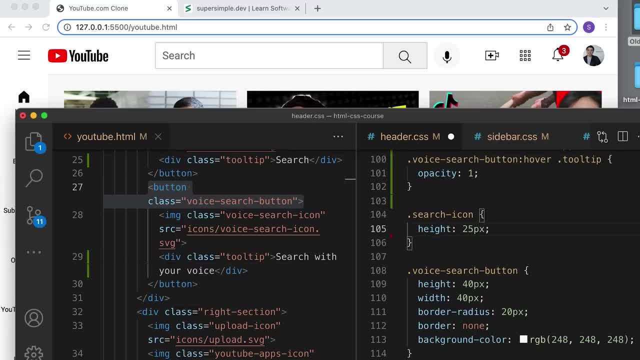 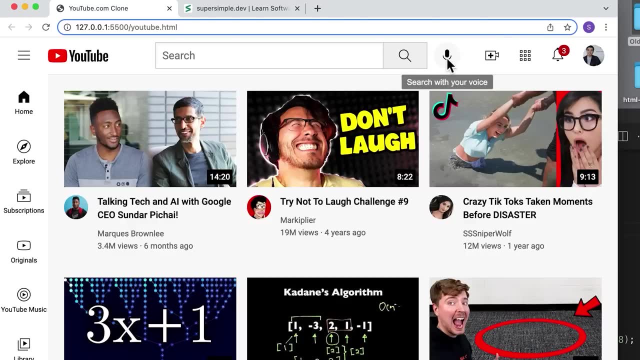 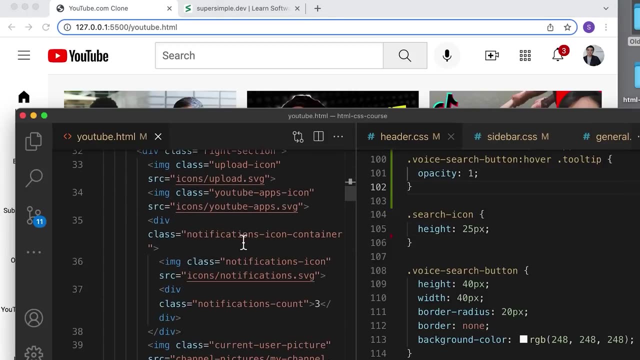 and let the flexbox handle the vertical centering. So if we save that now, the icons are perfectly centered and if we hover over, we have a centered tooltip. The tooltips for these icons are the same thing, except if we scroll down. we currently just have an image. 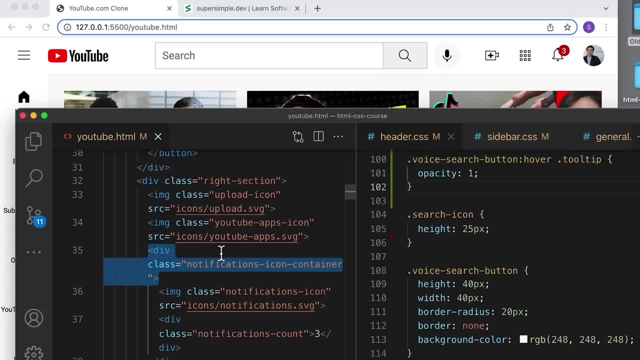 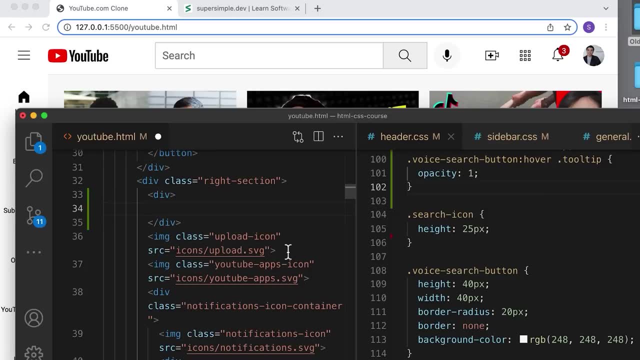 We're going to need a container like this that's going to act as our position relative container. So let's create a div that's going to contain our upload icon. Let's cut this and then paste it in here. Let's give a class. 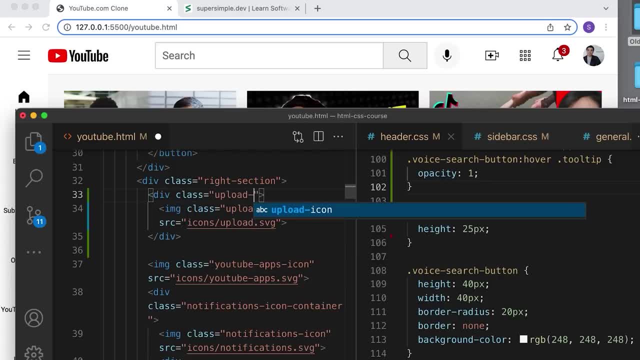 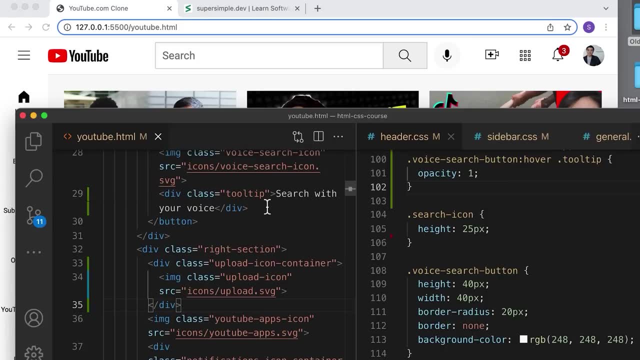 of upload-icon-container and then inside this container we're going to have our tooltip. So let's copy this and then paste it in here And let's call this: let's look at our design: create. So our tooltip is going to have the text: 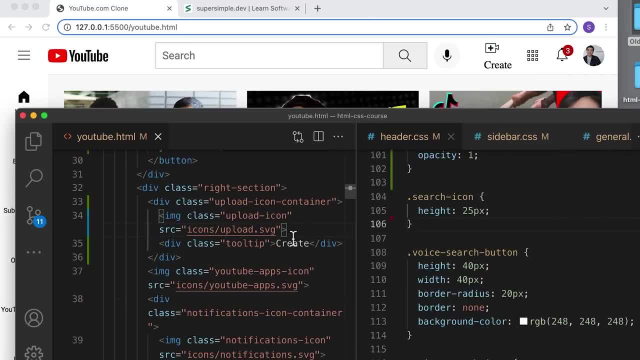 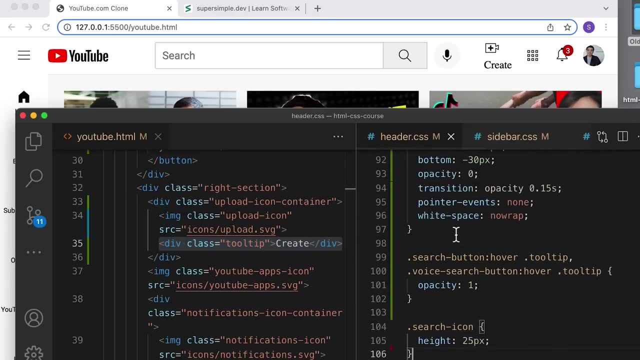 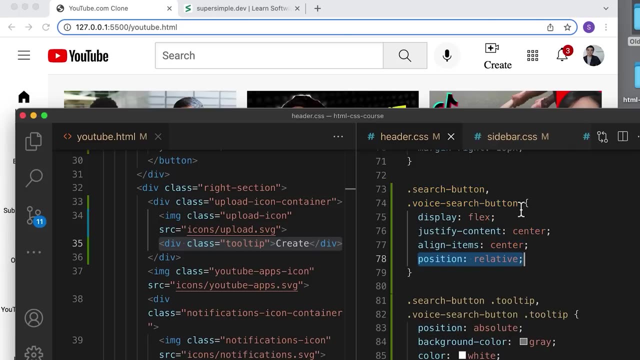 create. Next, we're going to change this to position-relative and position-absolute-inside, So let's scroll up and we already have this code here that sets to position-relative and centers everything. We're going to add to this the upload-icon-container. 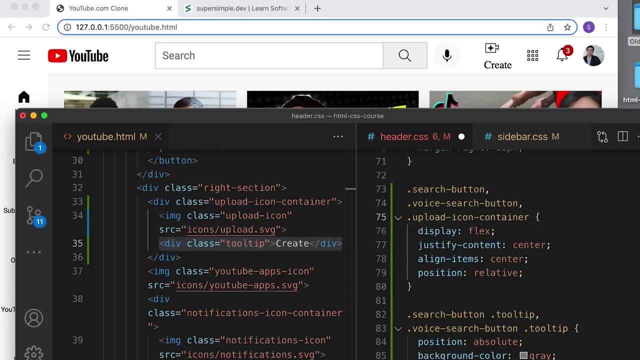 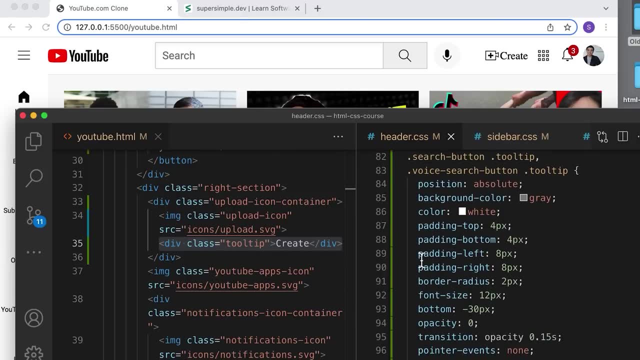 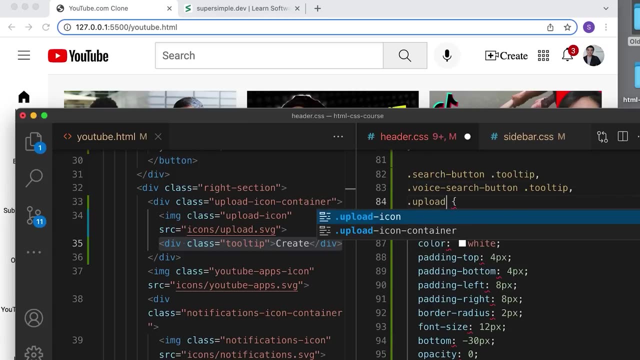 upload-icon-container, Save it, And then we need a position absolute on this tooltip. So again, we can just add it in here, so we don't have to copy all this code again With a comma: upload-icon-container, upload-icon-container, upload-icon-container. 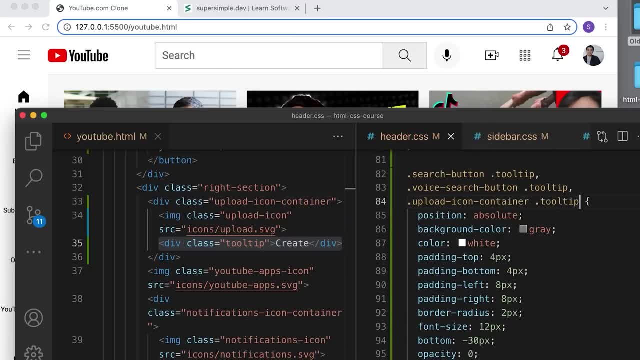 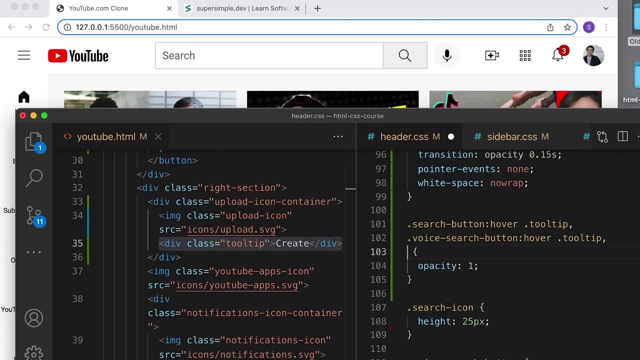 tooltip, Save it And, lastly, we're going to scroll down and add it to here So that appears when we hover. So let's set upload-icon-container, upload-icon-container, upload-icon-container, And when we hover over it, the tooltip 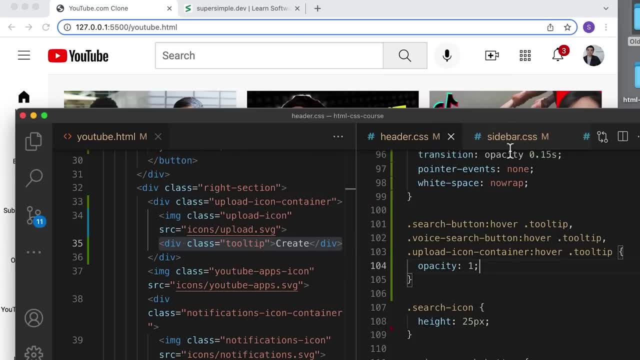 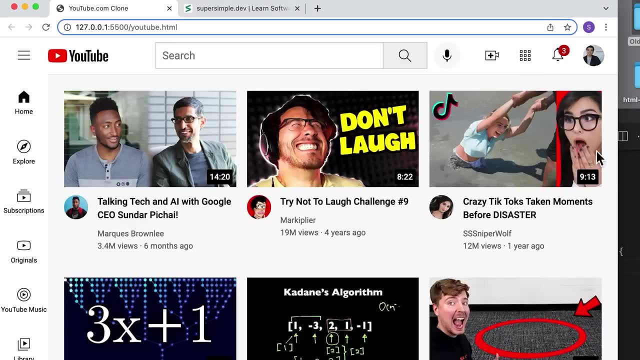 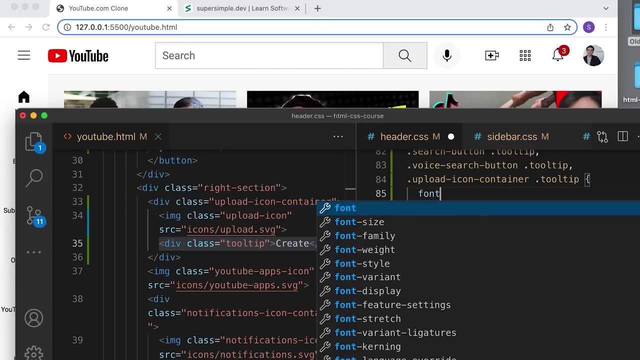 is going to have opacity of 1.. Let's save it and hover over, Alright, so that looks pretty good, But let's change the font here. So let's go into this code which sets our tooltip styles, and let's set the font dash family. 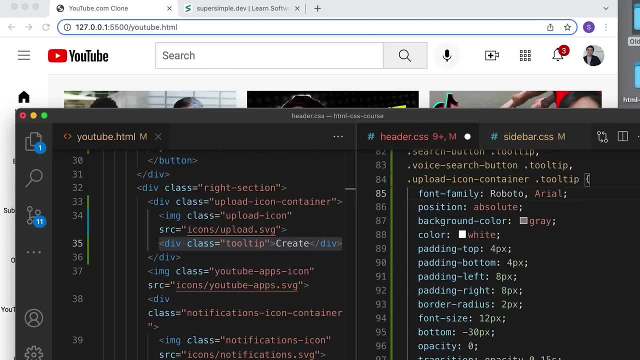 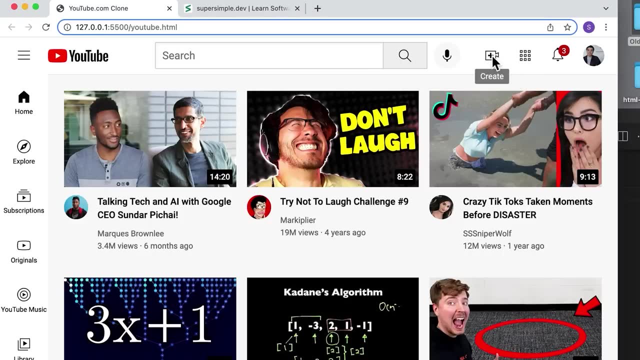 to Roboto comma Arial like before. We save it and we hover over it. Now we have a nice looking tooltip on our icons. So that's how we create these tooltips when we hover over these icons and these buttons. Creating tooltips for these two other icons are the same thing. 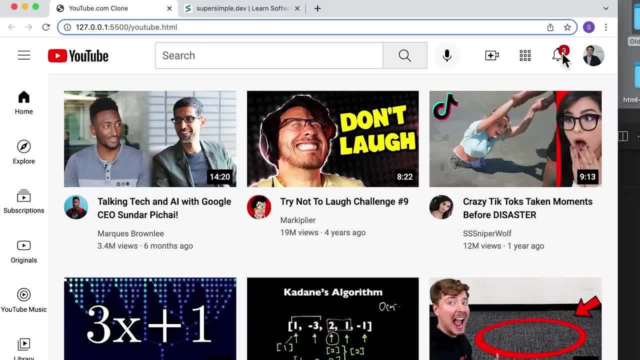 and I'm going to leave it as an exercise for you to do on your own. So in this lesson we finished up our final project. We created the sidebar, resized our videos, created the tooltips and now, if we compare it to our design, our project looks pretty much perfect. 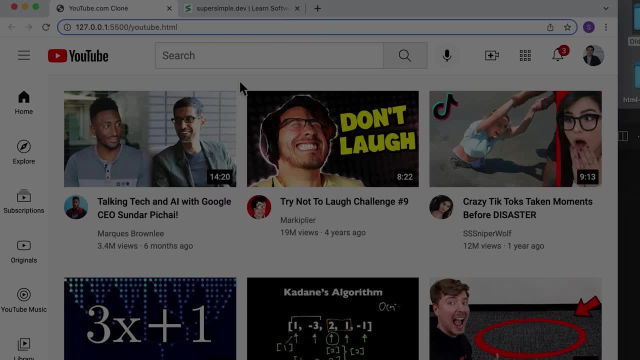 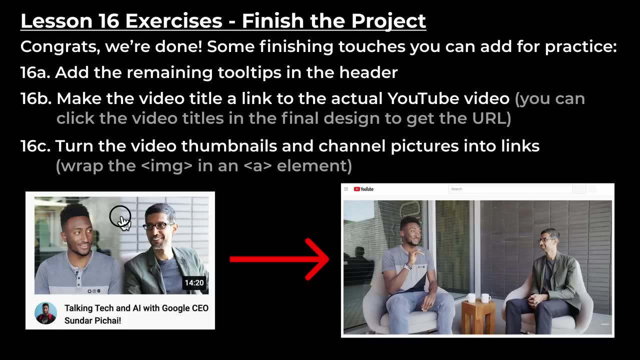 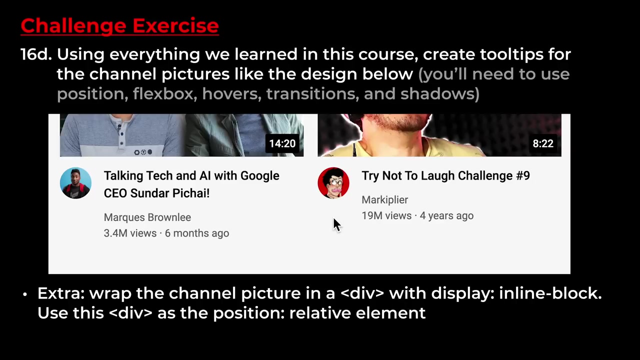 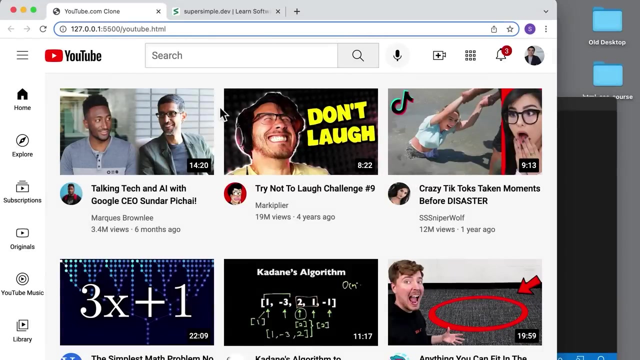 and ready to go. So here's some exercises you can try on your own to wrap up everything that we learned in this course. In the previous lesson, we finished our final project, which is this. In this lesson, I'm going to show you some more. 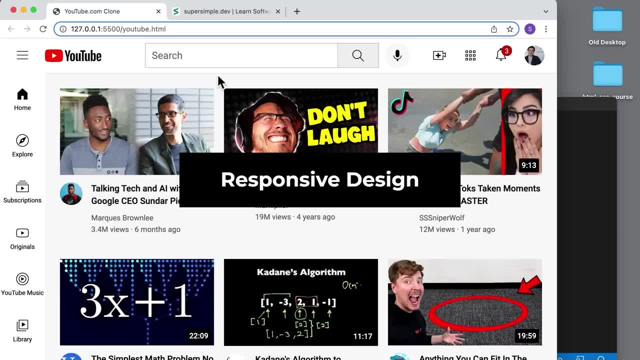 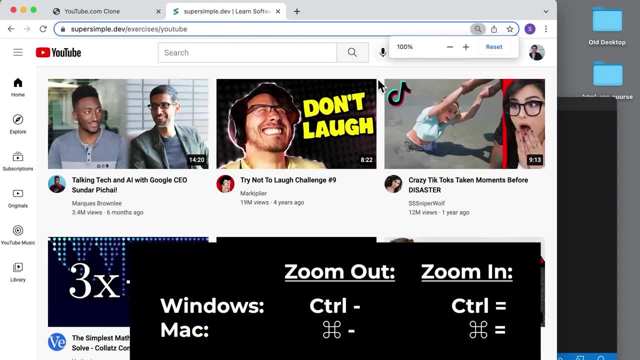 useful features of CSS. We're going to start off with responsive design. If we go to our reference design here- and I'm going to zoom out a little bit so you can see If I make the page smaller- you'll notice that we now have two videos. 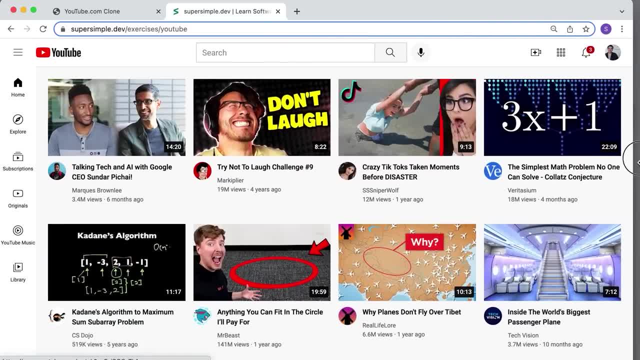 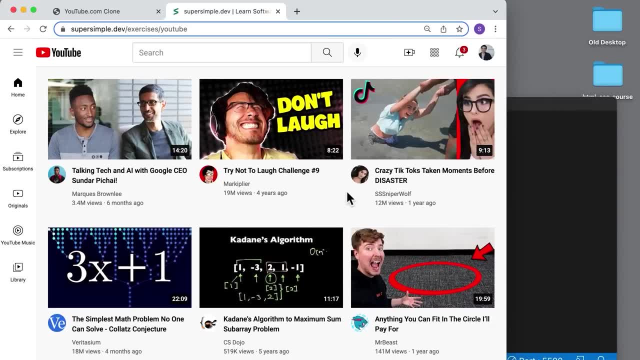 in each row. If I make the page bigger, we have four videos, So notice that at every screen size the layout adjusts so that the website looks good. So that's the idea of responsive design: Making the website look as good as possible on every screen size. 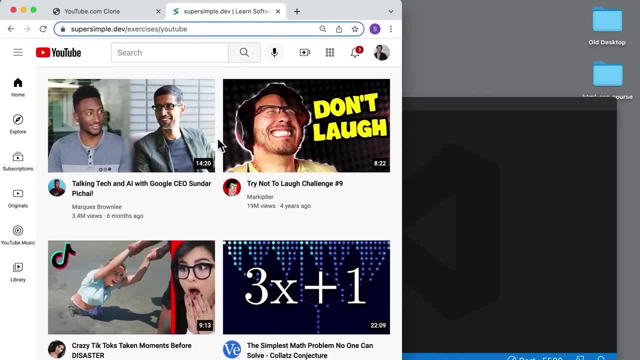 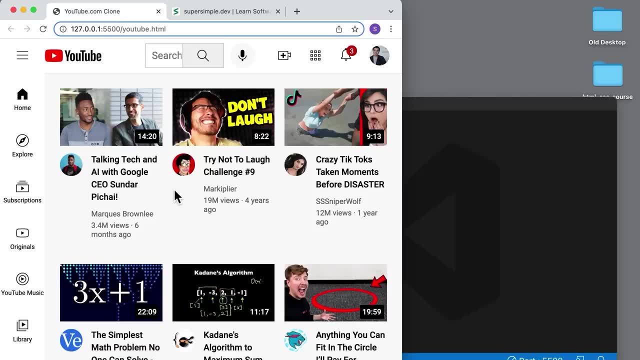 Now, if we make this a little bit more narrow and we switch to our current project, you'll notice that all of our content is sort of squished. So we're going to learn how to implement responsive design into our project. Let's go into our code. 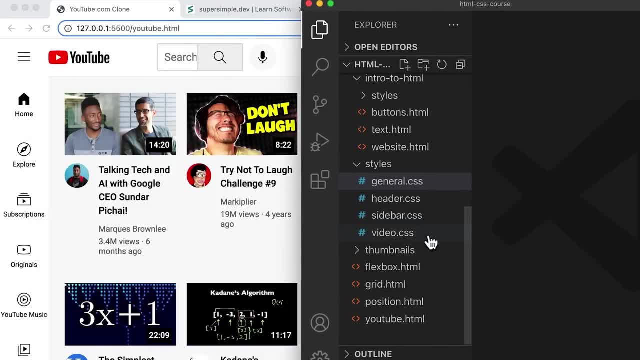 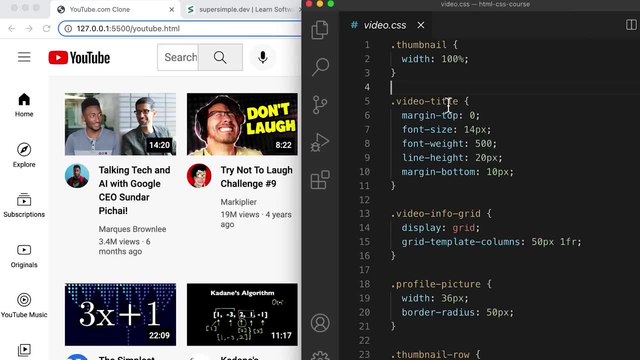 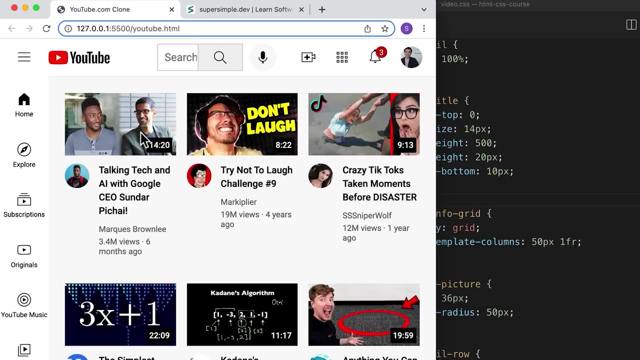 and we're going to open the file called videocss, which controls the video grid styles. Let's open that. And now inside, we're going to adjust our video grid so that when the screen size is small, we only have two videos per row, and when the 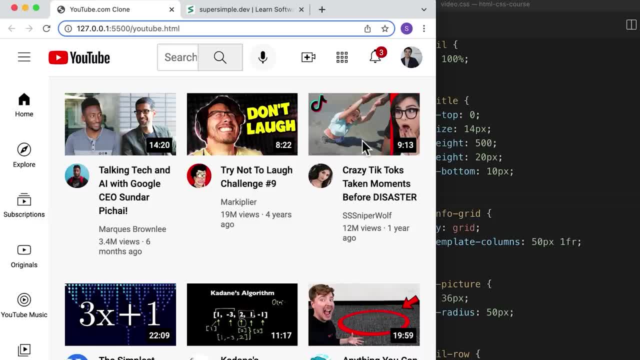 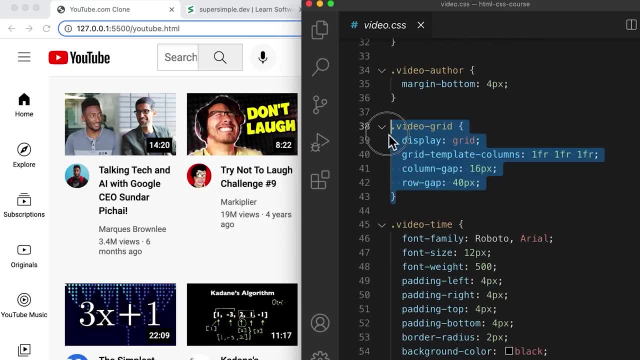 screen size is big. we have more than three videos per row. So let's go into our code and we're going to scroll down and find the video grid styles. So notice that for these styles we set three columns of equal size. Now to make this responsive. 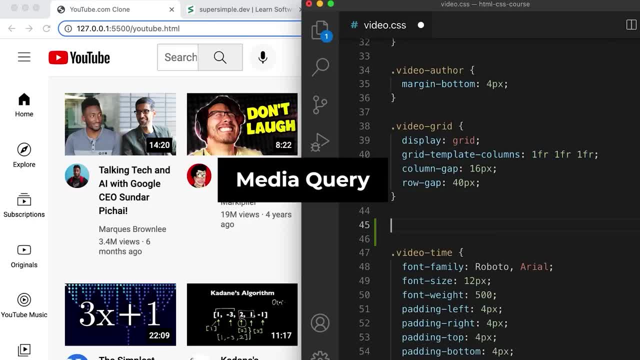 we're going to use something called a media query. So to create a media query we're going to type at media and then we're going to give it a screen size. So we're going to say max dash width colon maybe 600 pixels. 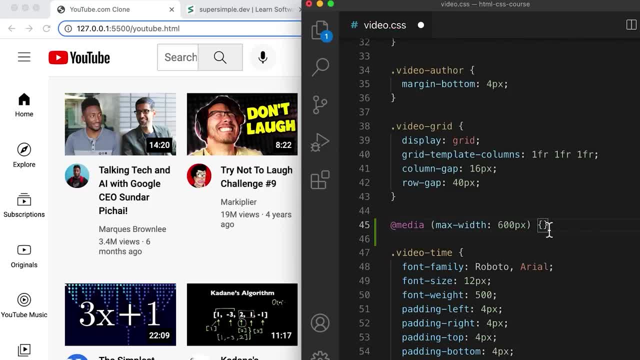 And then we're going to type open squiggly bracket and then close squiggly bracket. So the way this works is that we're going to have a bunch of css in here and this css will only activate if the screen size is 600. 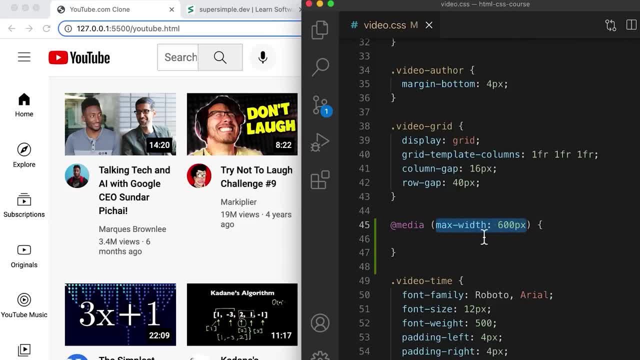 pixels or less. That's what this max width means. So, for example, let's target the video grid class inside here and let's set the grid dash template, dash columns, to 1fr. That means from a screen size of 0 to 600 pixels. 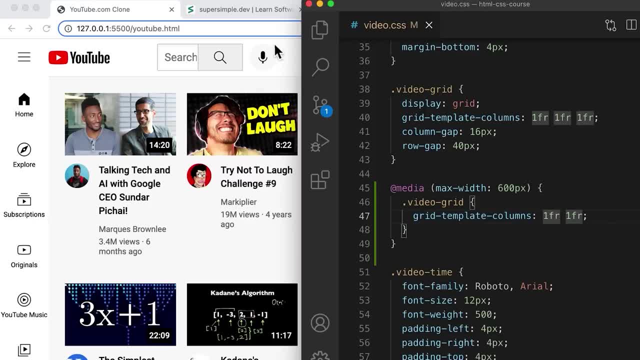 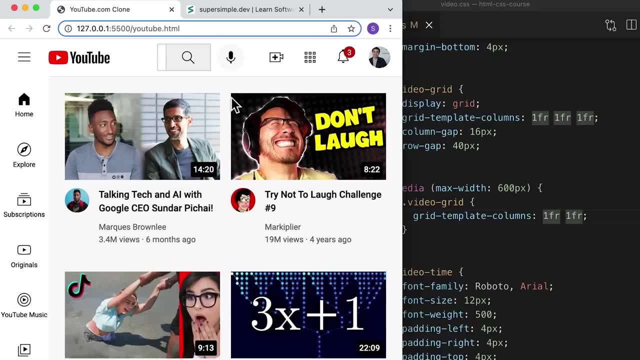 we're only going to have two columns, So we save it and we start to resize. Notice that once we get to 600 pixels, we now have two columns in our grid. Now, to figure out how big our screen size is, we can right click. 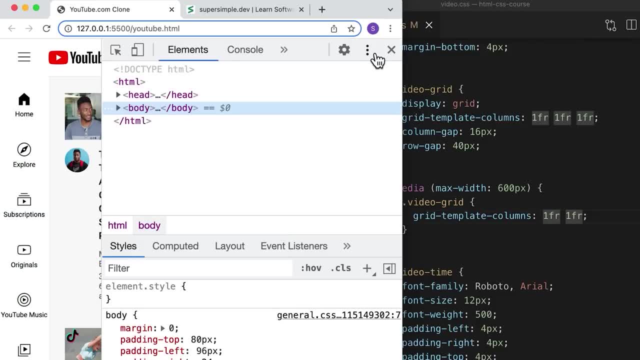 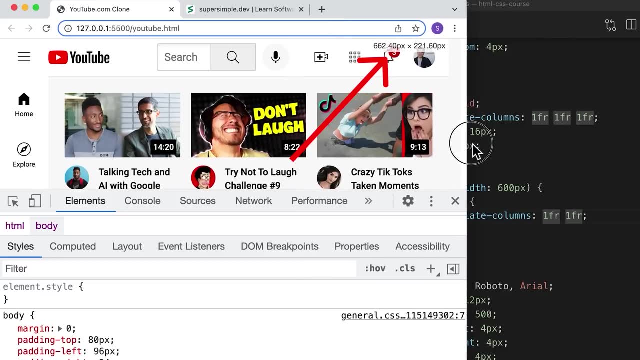 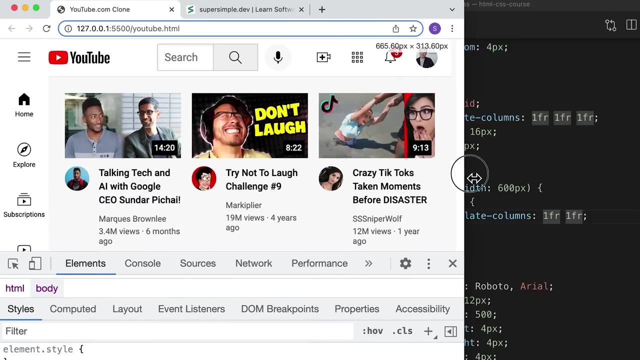 and inspect, and I'm going to click these three dots and move it back down to the bottom like this. And now when we resize, you should see the screen size at the top right of the page. So it's really up to us to pick a screen size. 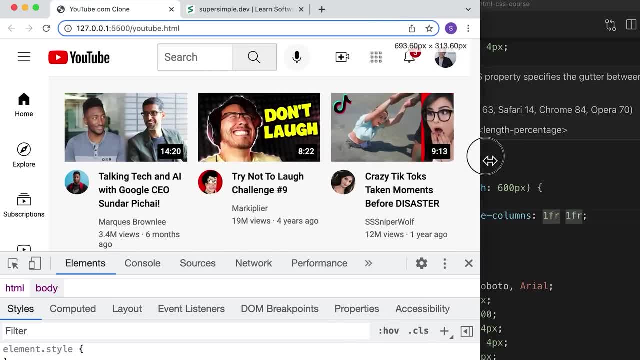 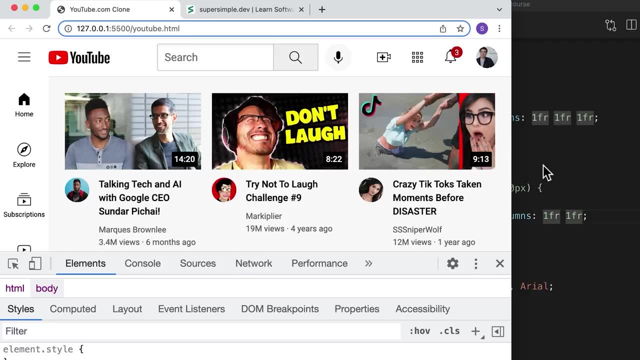 where we're going to go from three columns to two. So I think even at this screen size- maybe at 750- it looks a little bit squished. So I'm going to increase this to 750 pixels, Save it. and now, once we get to 750, 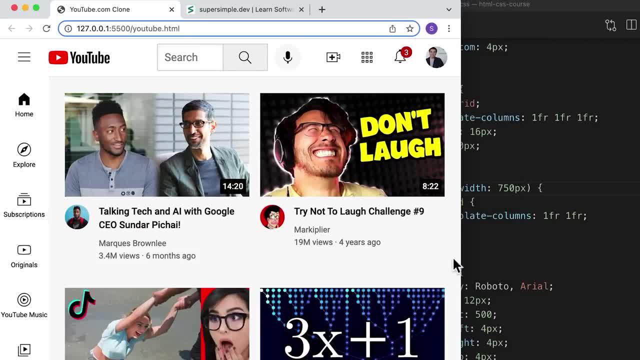 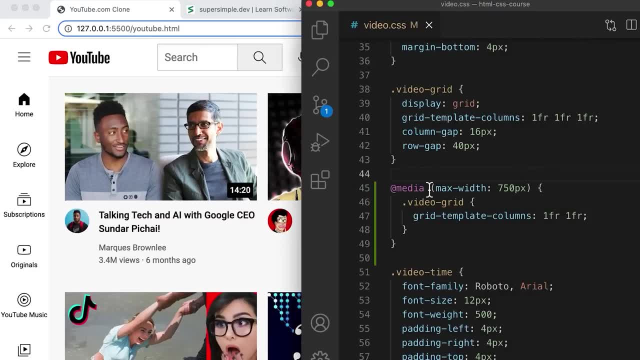 we're going to have two videos in each row and it's not going to be as squished anymore. So that's the basics of how to create responsive designs using these media queries. Let's do another example. We're going to have four videos. 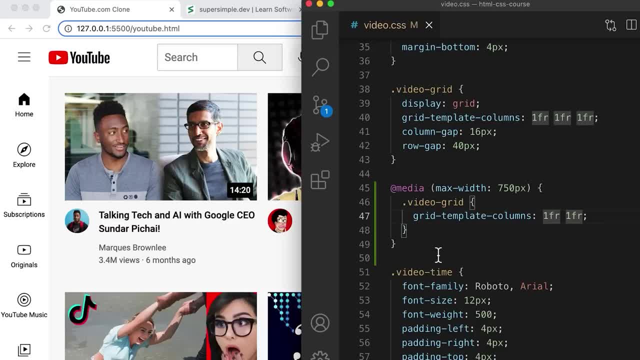 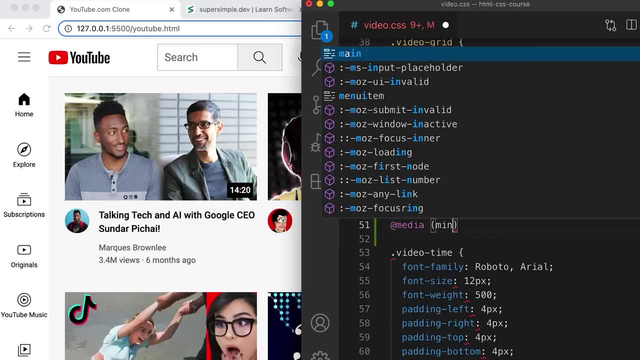 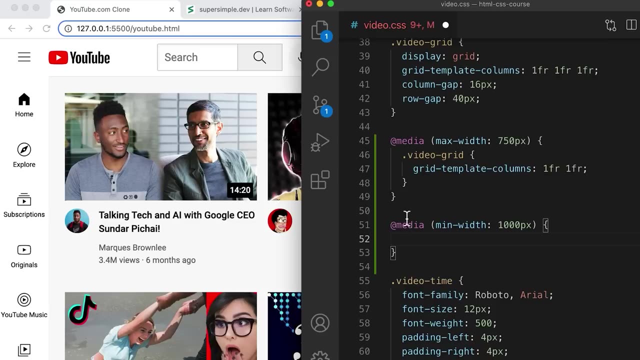 per row when our screen size gets really big. So let's set another at media, at media, and for this time we're going to set a minimum width of maybe 1000 pixels, And then inside here we're going to copy this and paste it here. 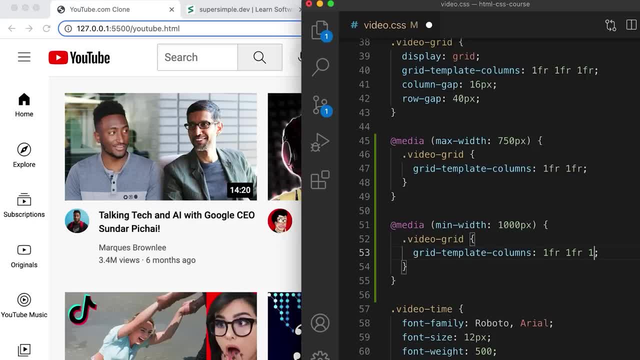 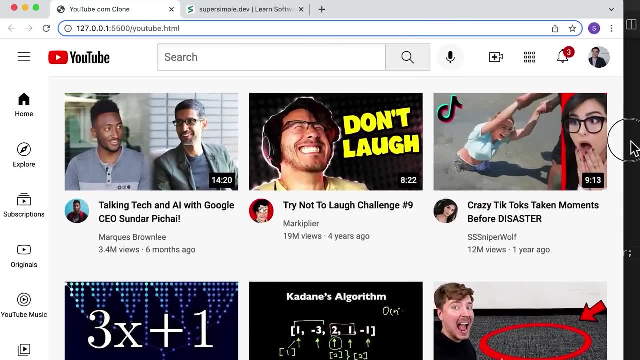 We're going to change grid template columns to four columns, So 1fr, 1fr. Now, if we save it and we resize the browser to 1000 pixels, it's going to become four videos per row. Now you might need to press. 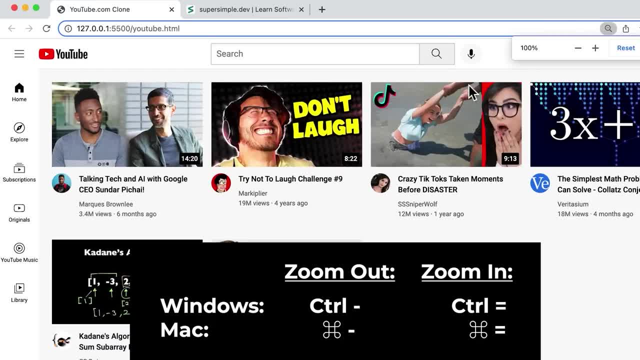 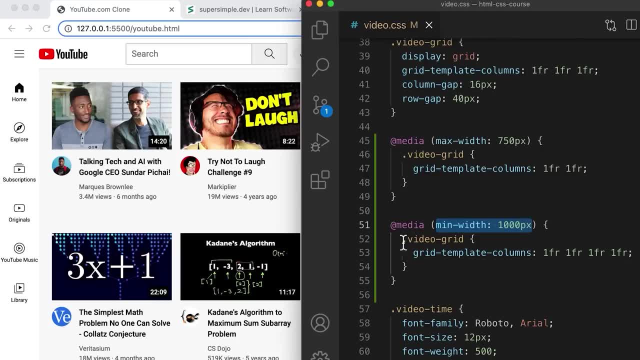 command or control minus to make the webpage smaller, to see this. But basically the way this works is that once the screen size hits 1000 pixels, this will activate and we have four columns instead of three. So the last example is that we can actually combine these two. 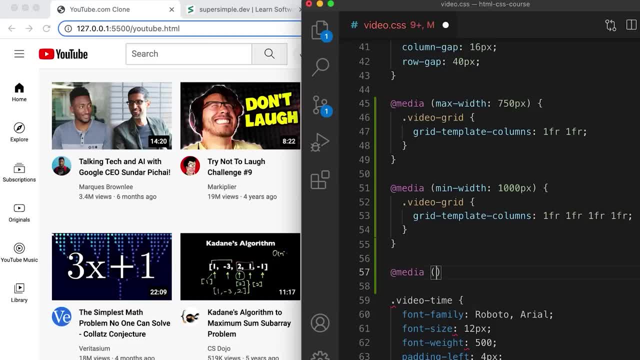 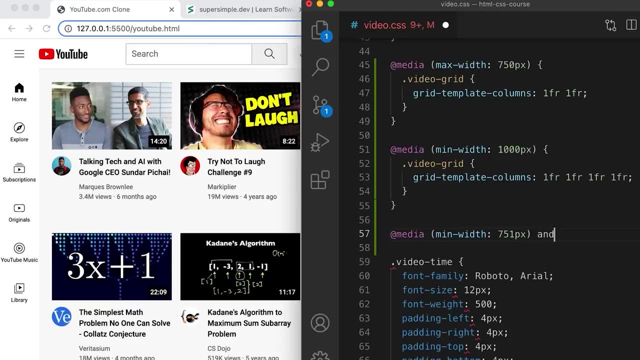 So we can set at media and we can set the min dash width to 751 pixels and the max dash width to 999 pixels. So this will cover the space between these two measurements here. So let's actually put this in the middle. Okay, so from. 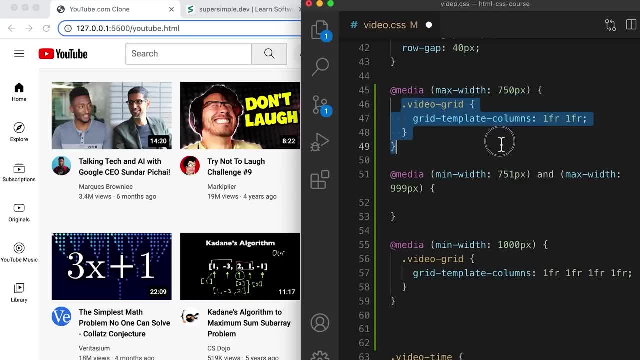 0 pixels to a max. of 750, we're going to have these styles, And then from 751 to 999, we're going to have these styles. We're going to set this to three columns, And then from 1000 and up, we're going to have 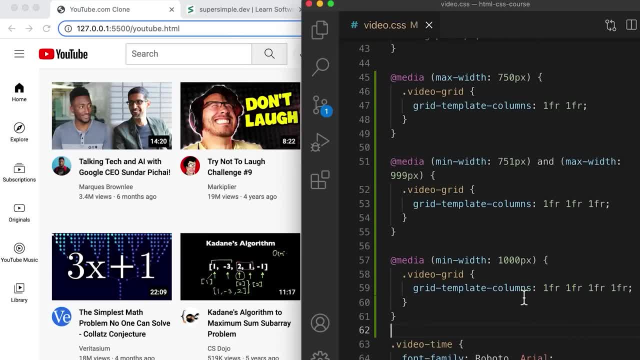 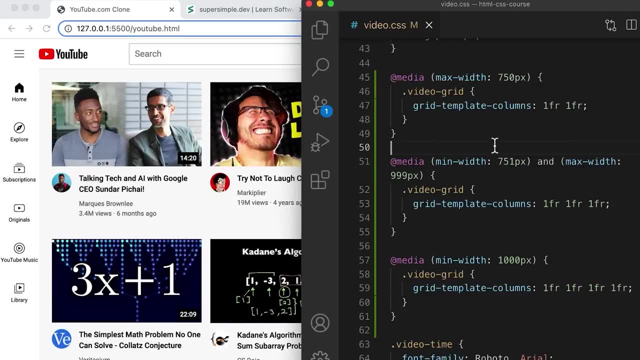 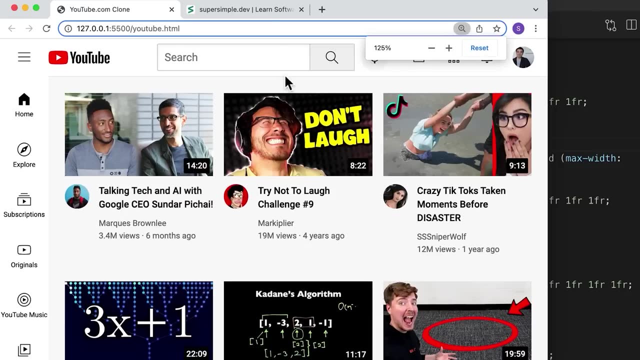 four columns. So this is the basics of how to create a responsive design like this. You just have to write a lot of media queries, Alright. so that's the basics of responsive design. We're going to go back to our webpages. 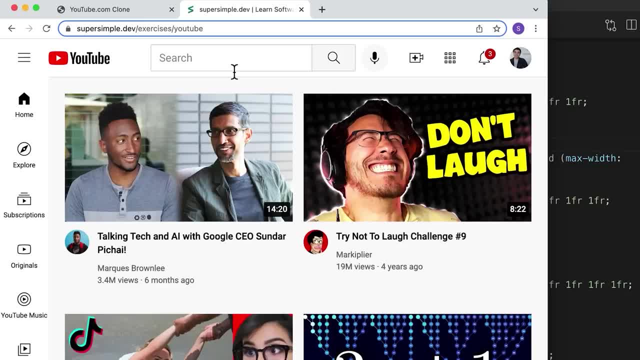 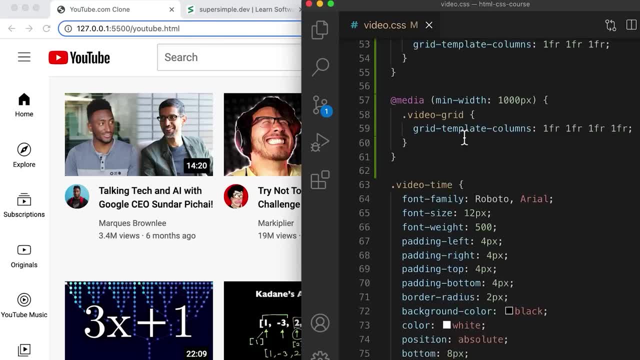 I'm just going to zoom back in And we'll learn the next feature of CSS. So let's go to our project here and open our code And let's scroll down to this style: the video time. So the next feature we're going to learn. 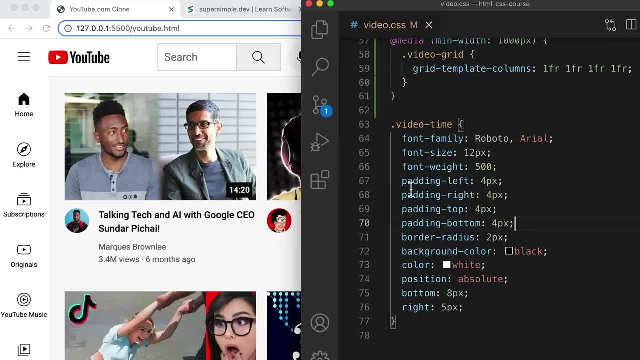 is sort of like CSS shortcuts. So instead of setting padding on the left, right, top and bottom separately, like this, we can actually use a property called padding, Which is sort of like a shortcut for all four of these. So if we set the padding to 4 pixels, 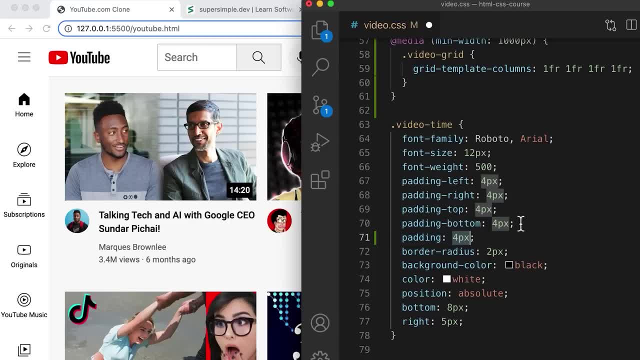 this is the same as setting padding on all four sides, So we don't need this code anymore. So it makes it a little cleaner for our code to use these shorthand properties. So another thing we can do with this is we can have two values. 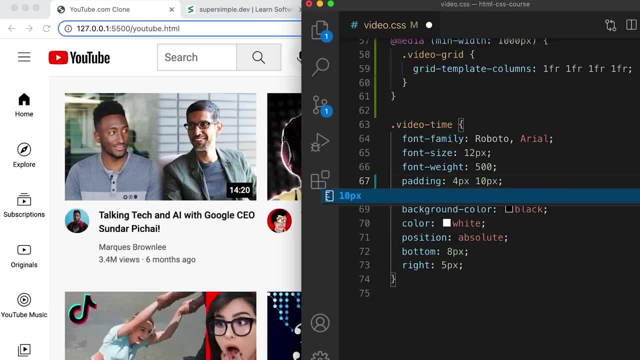 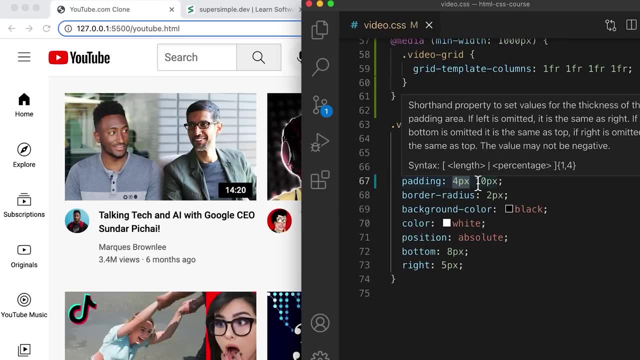 Let's say 4 pixels and 10 pixels Save it. So this first value is going to be the vertical padding, So padding top, padding bottom, And the second value is horizontal padding, Padding left and padding right, The next thing we can. 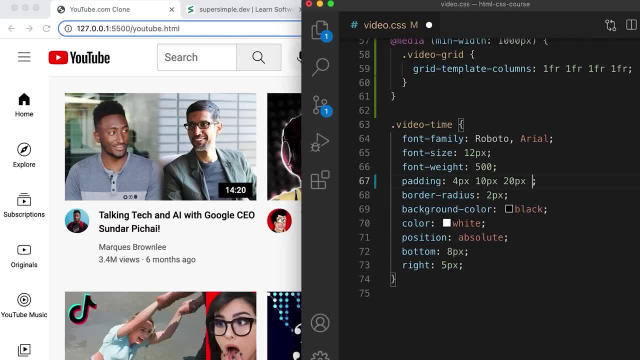 do is have four directions, So 20 pixels and 30 pixels. Let's see how that looks. So this is how we can set padding in all four directions using one line of CSS. This first value is the padding top. Second value is the padding right. 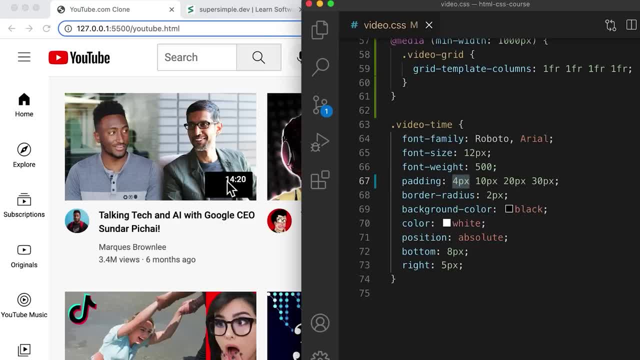 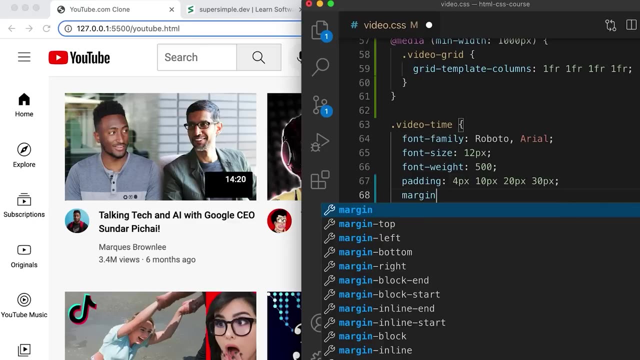 Third value is padding bottom And fourth is padding left. You can think of this as first you start from the top and then you work your way clockwise around. So that's what these four values mean. Another shorthand property is margin, And this is a substitute for. 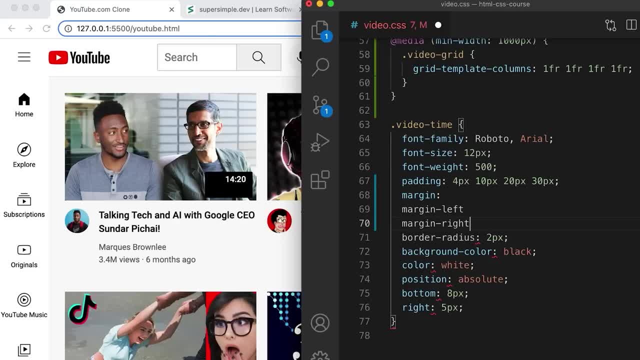 margin-left, margin-right, margin-top and margin-bottom. So this margin shorthand property works the same way as padding. If we have one value, this is all four directions. If we have two values, this first value is the vertical direction. 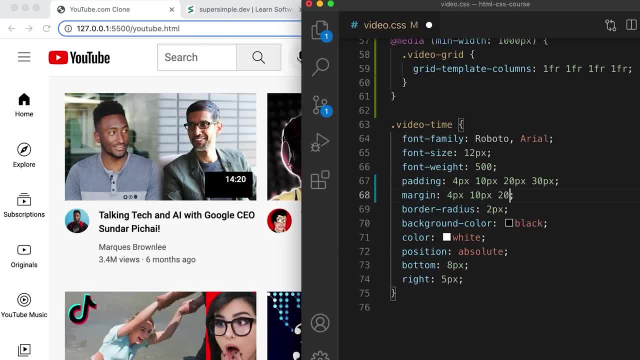 Second is the horizontal direction, And if we have four values of margin, this is the top, right, bottom and left. So these are just examples. We're going to move our styles back to four pixels of padding on every side And we're going to look at one final. 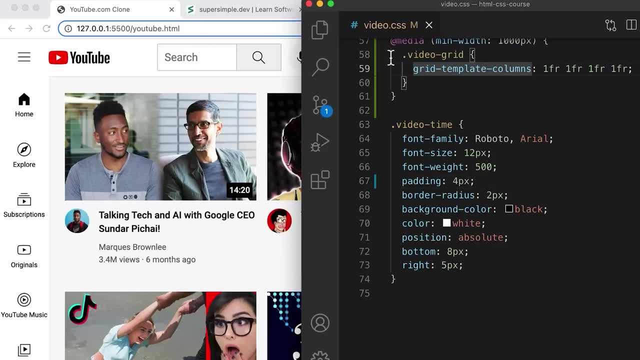 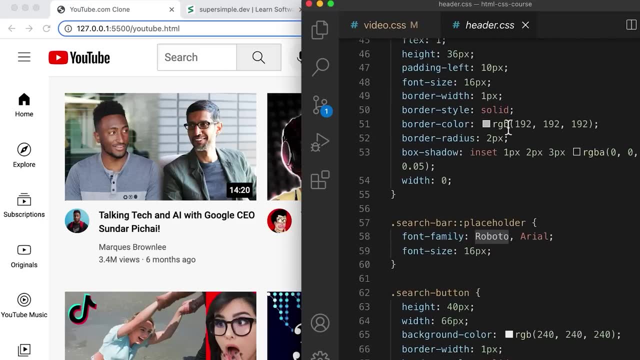 shorthand property, which is the border. So let's go into our header CSS file and find these styles for this search bar. So we're going to scroll up until we find our search bar, which is here, And notice, for our borders we always set a width. 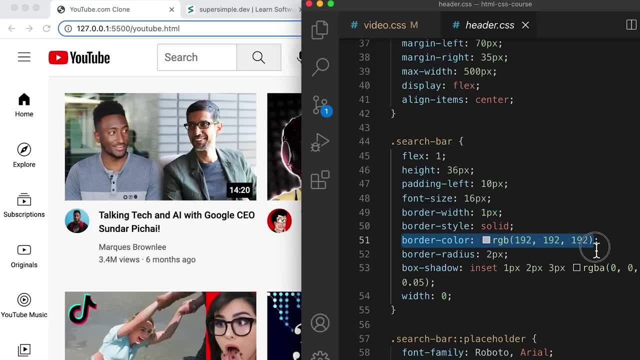 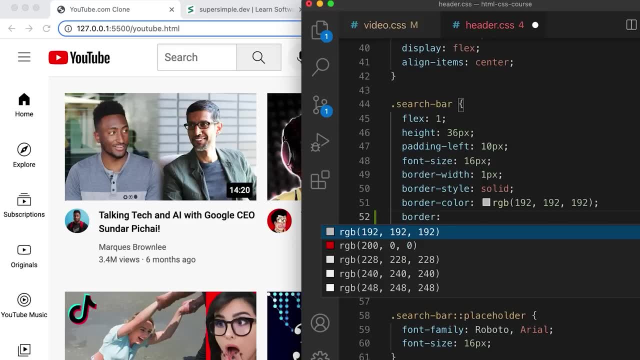 a border style and a border color. So instead of setting these styles separately, we can use a shorthand called border. So for border, we can set one pixel. This is going to be the width. We can set another value of solid. This is going to be the border. 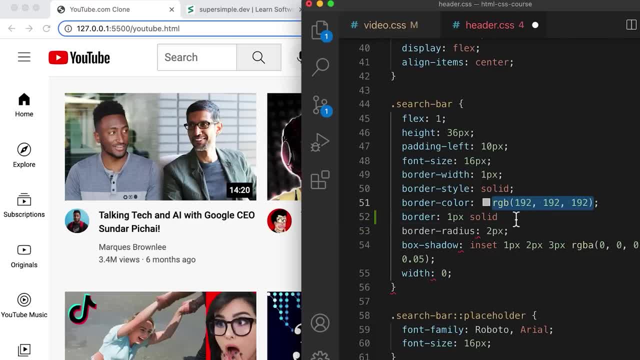 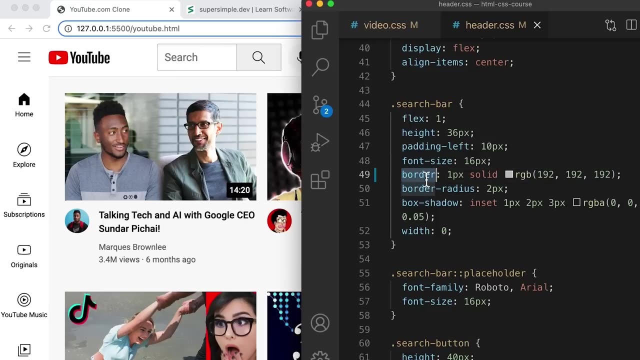 style And we can set the third value of color, And so this one line of CSS can replace these three. If we delete that and we save, you can see that everything still appears normally, And that's because this border property is a shorthand for the other three. 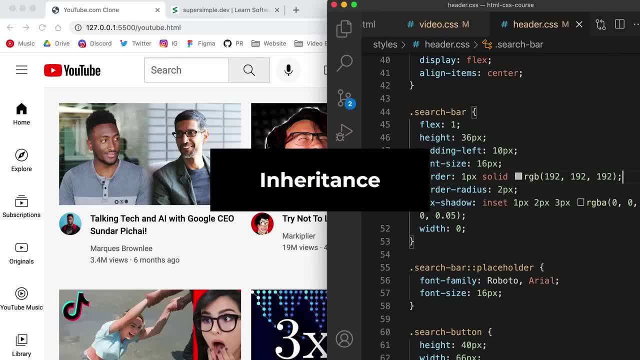 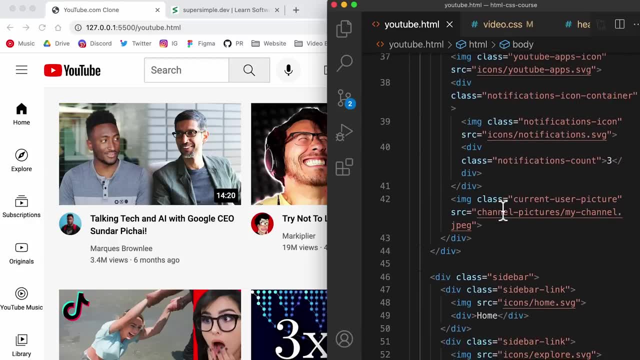 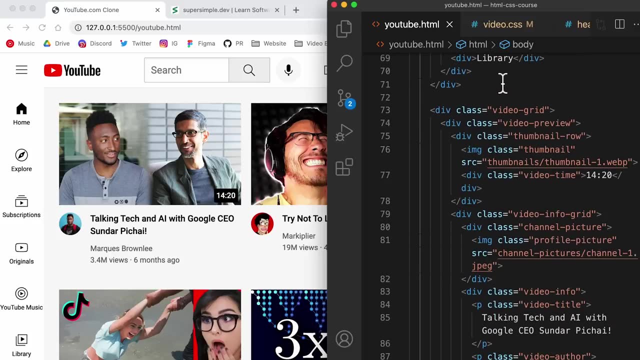 The next thing we're going to learn is called inheritance. Let's go to our youtubehtml file And we're going to scroll down to the video grid which is right here. So inheritance means that for certain CSS properties, if we set the property on the outer- 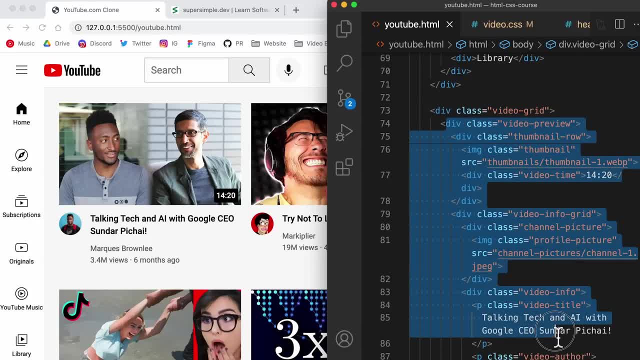 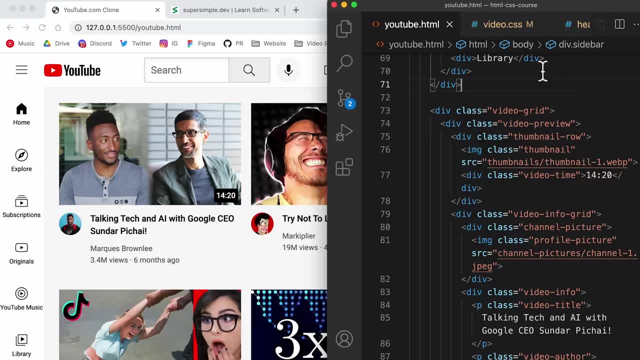 element, it will get passed down to the inner elements like these. Let's do an example. We're going to set a property on the video grid, We're going to go to the videocss file And we're going to find the video grid styles. 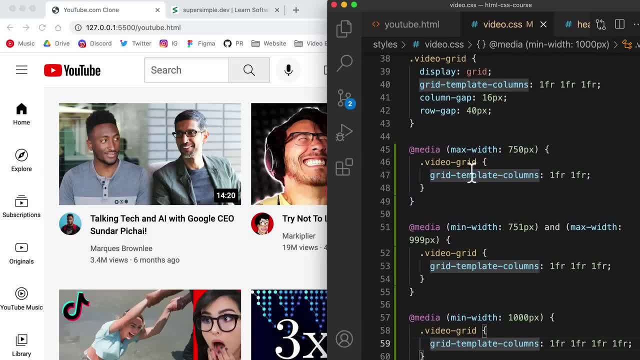 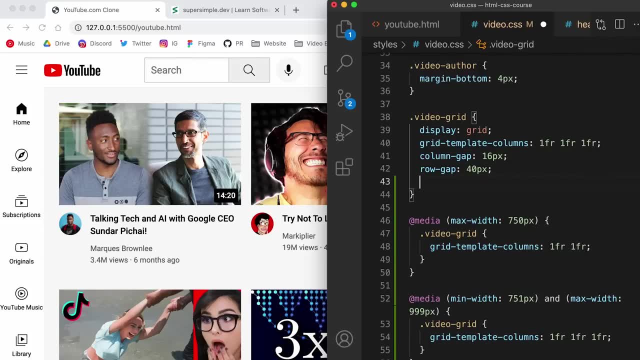 which is all of these. We're going to set it on this style here, So we're going to set it for all screen sizes. Let's add a style. We're going to make the text underlined. To do that, we're going to use this property. 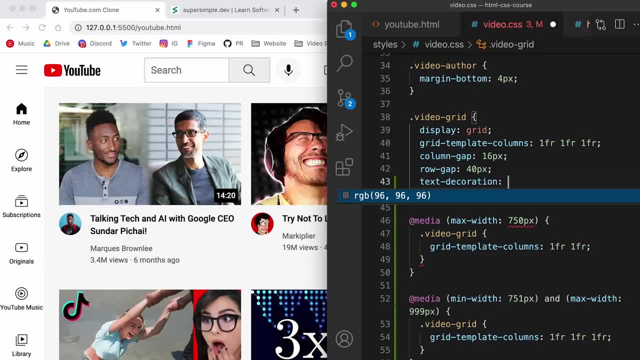 text-decorate decoration underline. Now, if I save this, you'll see that even though I set text-decoration underline on the video grid, all of the paragraphs inside have been underlined. So this is called inheritance. If we set this style on the outer element, which is 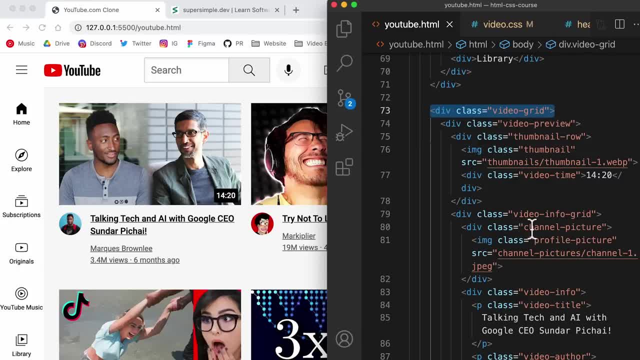 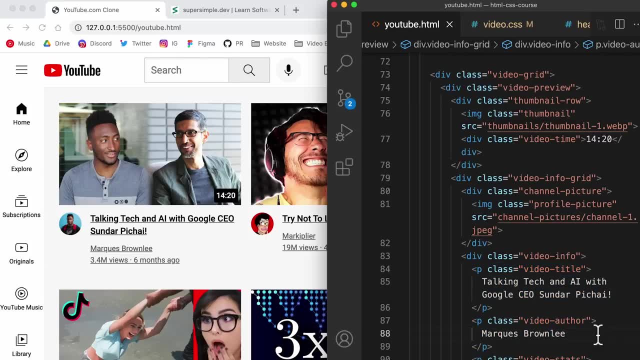 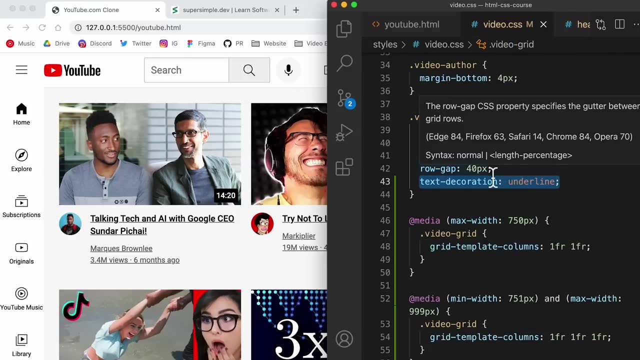 the video grid, it gets passed down to all the inner elements, which are the paragraphs here. However, not all properties are affected by inheritance. For example, if we go back to the videocss file and we're going to add a border this time. 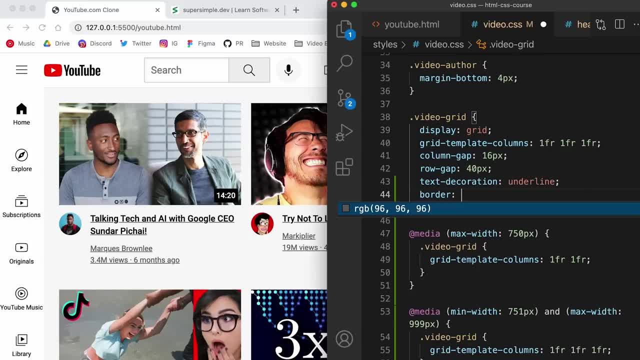 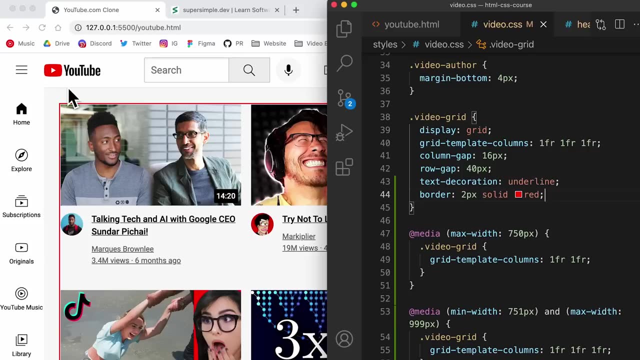 So let's add a border, and we're going to make it 2 pixels wide, a solid color and let's just make it red. If I save that, you'll see that the video grid has a border around it, but this border is not passed down to. 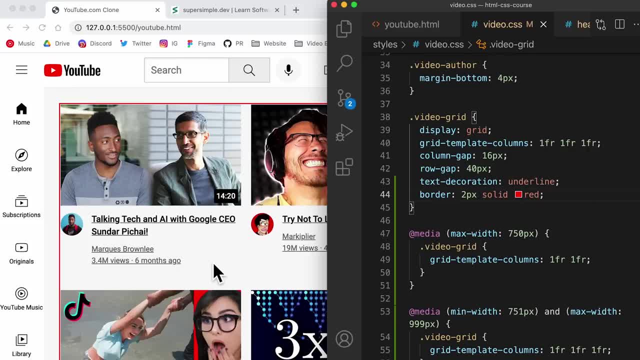 the inner elements here. So inheritance mostly just works with text properties like text-decoration-underline, color, font-weight and font-family. It doesn't affect things like border padding or margin. So that's what inheritance means: Certain properties. 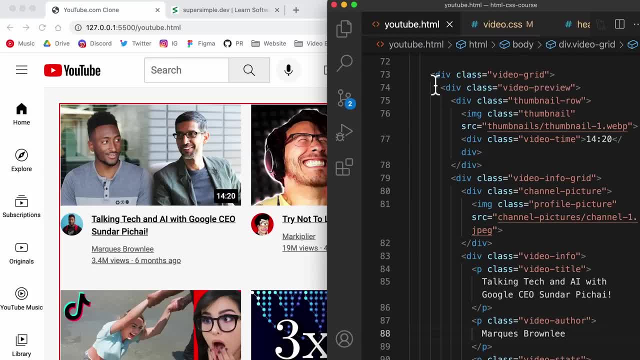 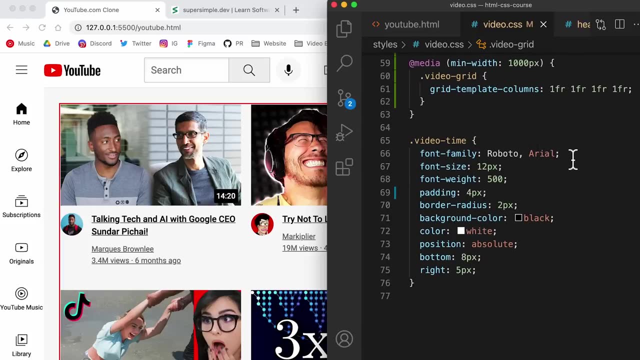 mostly text properties will get passed down from the outer element to the inner elements. Now this can save us some code. For example, if we go back to the videocss file and we scroll down, you can see that the video time uses a style called font-family. 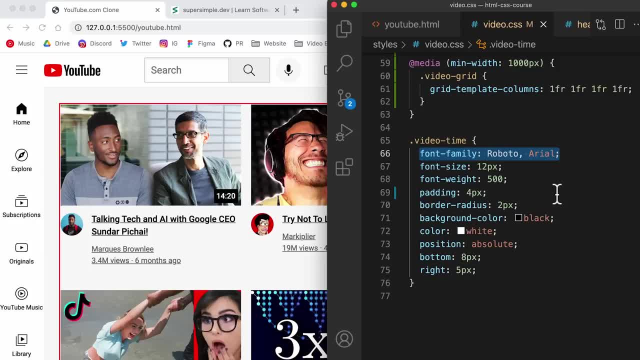 roboto-aerial. So this changes the font of our text And instead of putting it on the video time, we're just going to put it on the entire grid And then it will get inherited by all the elements inside, which includes the. 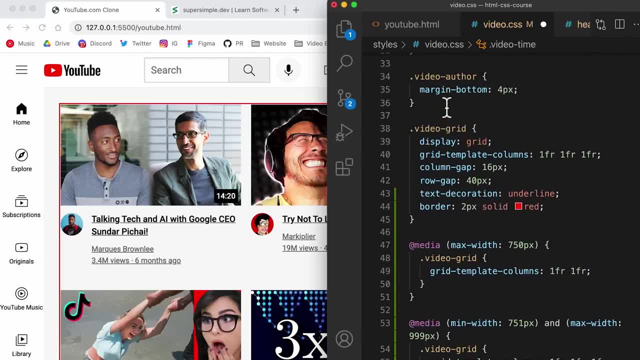 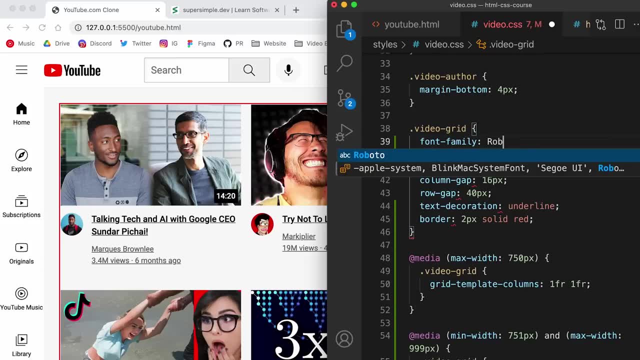 video time So I can scroll up to the video grid and I can set the font-family font-family up here So I can set roboto aerial. If I save this, you'll see that nothing changed with the video time, because 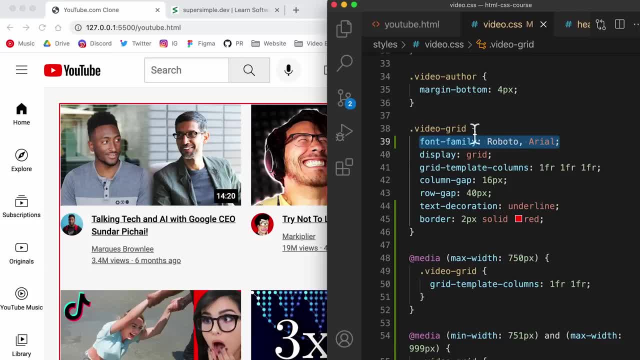 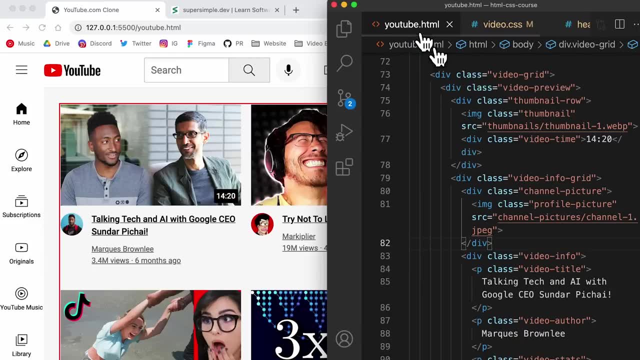 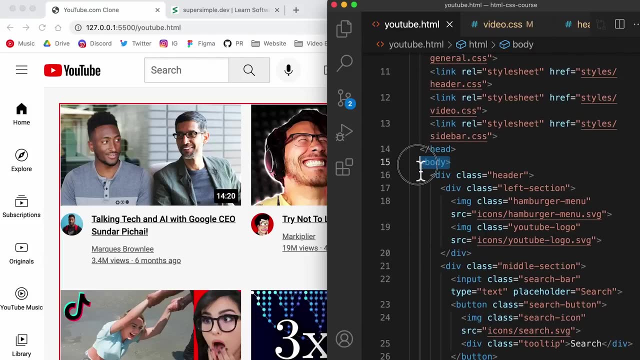 this style is being inherited from the video grid. Now we can actually take this even further. If we go to the youtubehtml file, you'll see that this video grid is actually contained within the entire body, So all of our elements on the page. 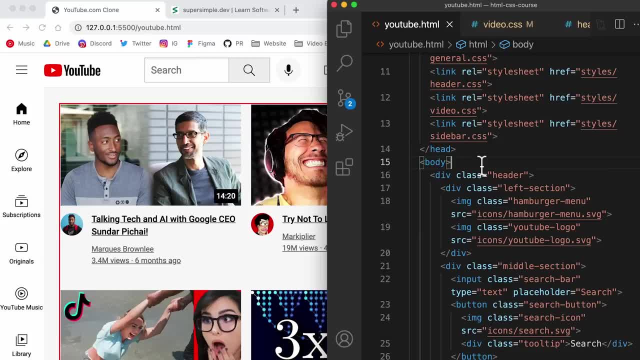 are contained within the body. So if we want to set a sort of default text style on the entire page, we can actually just put everything in the body, and that'll save us a lot of code. So let's actually go back to the 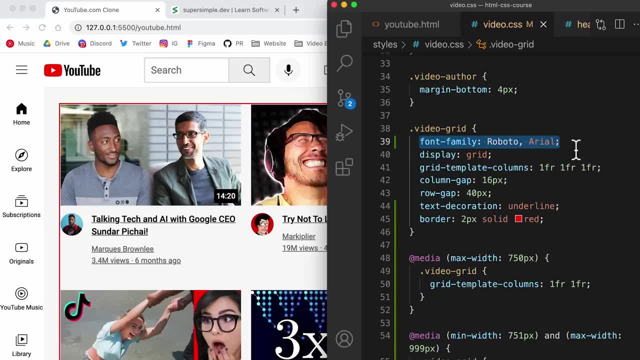 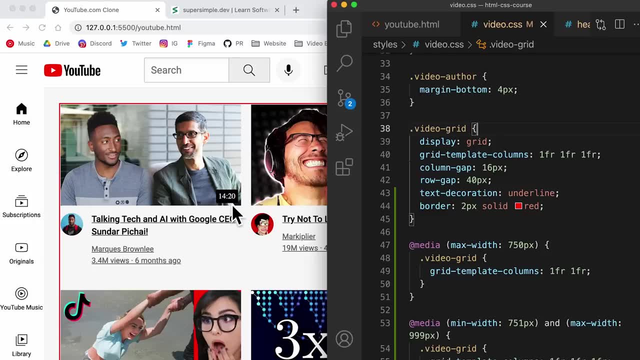 videocss file. We're going to remove this and save it. You'll see that the video time now goes back to the default font, which is Times New Roman, And these paragraphs actually use a different set of styles. So if we go to the file called, 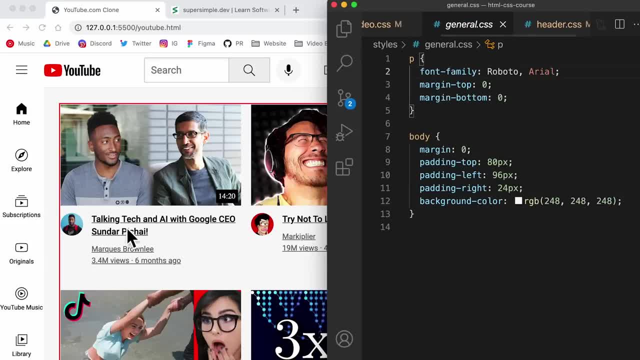 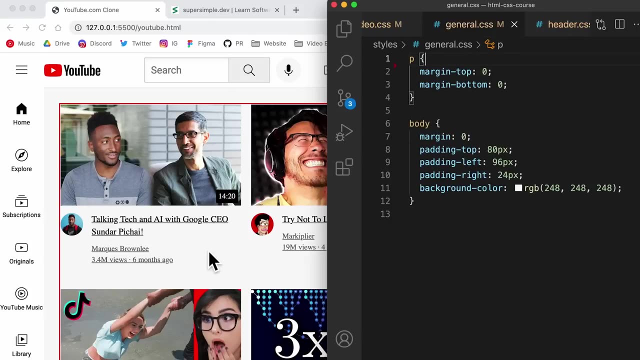 generalcss, we set the font family for these paragraphs using just a P selector here. If we remove this and save it, you'll see that it goes back to the default font of Times New Roman. Now we're going to set this style on the body, so that 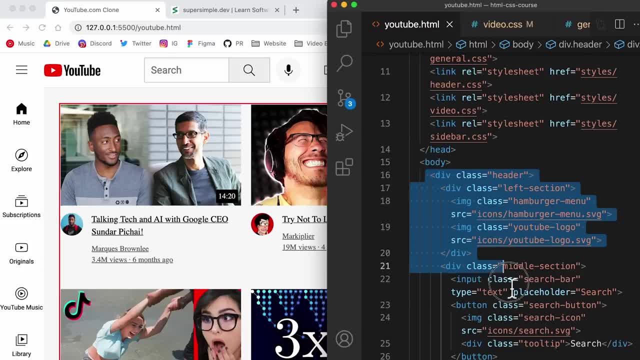 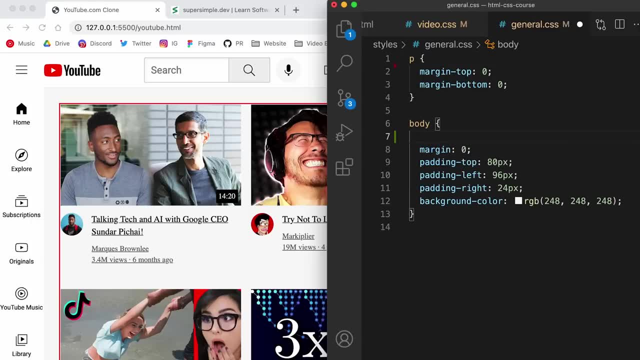 it gets inherited to the entire webpage inside. So we'll go to generalcss and we're going to set font-family to Roboto Arial to take advantage of inheritance. If I save this, you'll see that all of the fonts went. 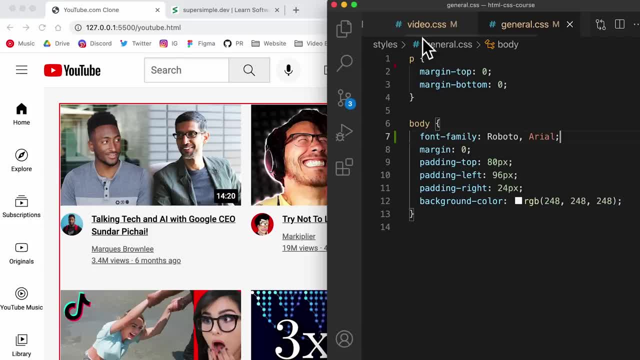 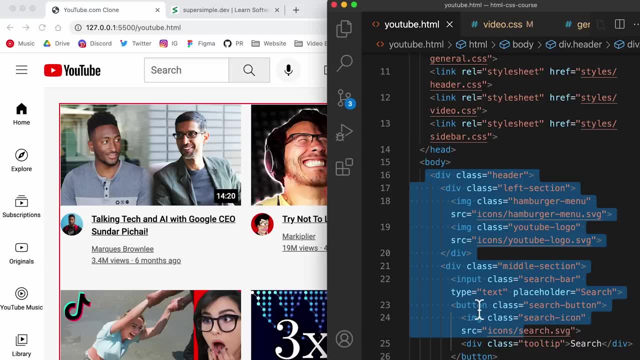 back to Roboto, And that's because we set it on the body and all of our elements are inside the body, so this style gets inherited to the inner element. So, using this, we can save more code If we go to our sidebar. 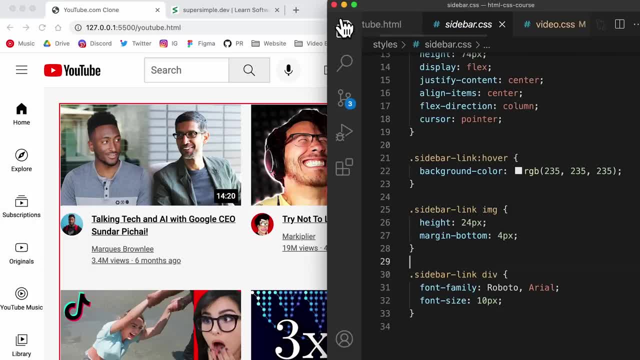 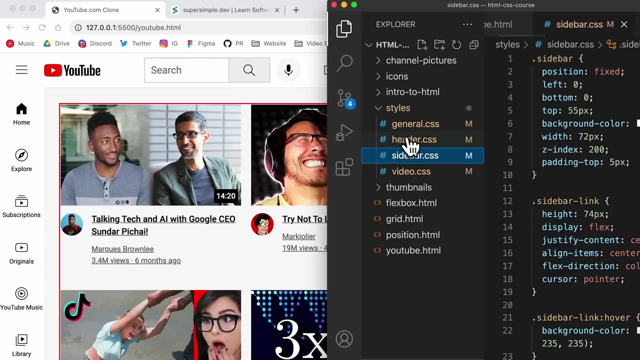 and our header. if I go to the sidebar first, you'll notice that we're also using font-family Roboto Arial, So we can simply get rid of this, because this style is being inherited from the body. And if I go to the headercss, 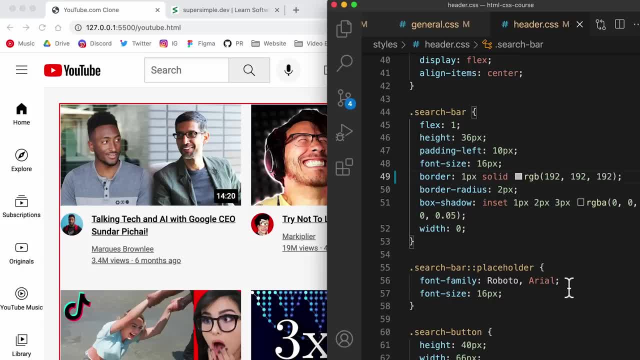 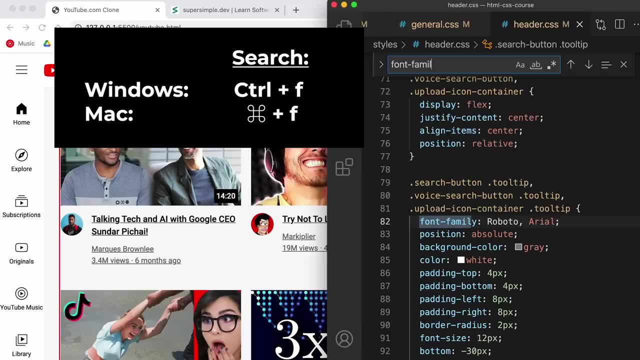 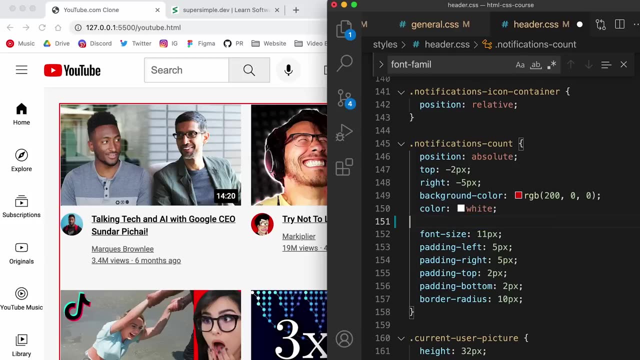 you'll notice that we're also using font-family Roboto Arial in a bunch of places, So we can just get rid of all of these and take advantage of inheritance to save us some code. Alright, so there's one last thing about inheritance that I want to show you. 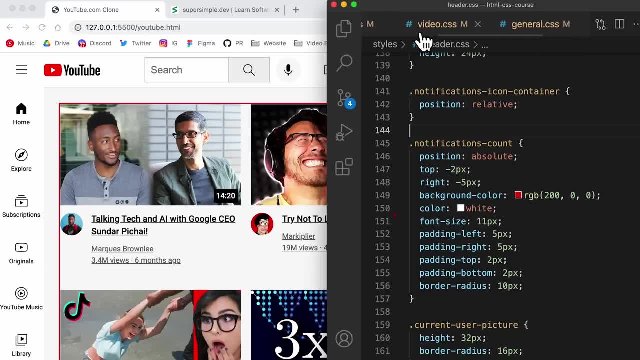 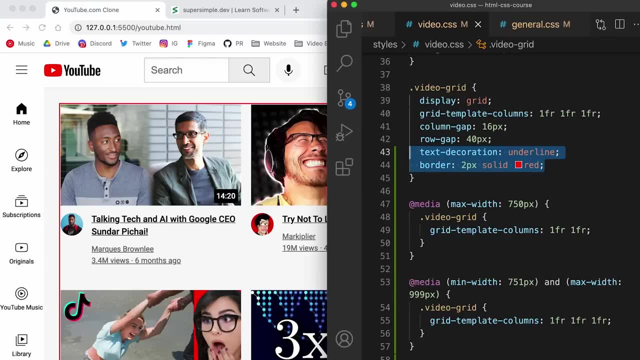 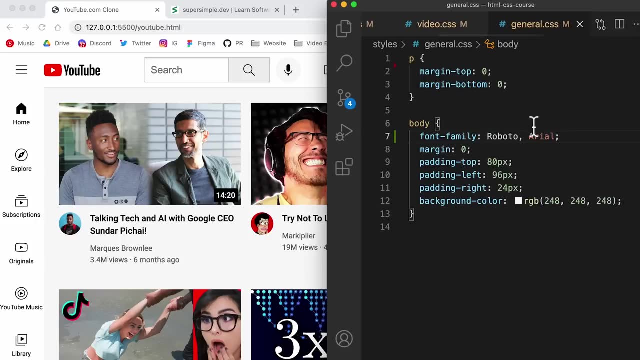 We're going to go back to our videocss file, which is right here And now. let's get rid of these properties that we're using to test with Save it. This time we're going to go to generalcss. we're going to set another style in the body. 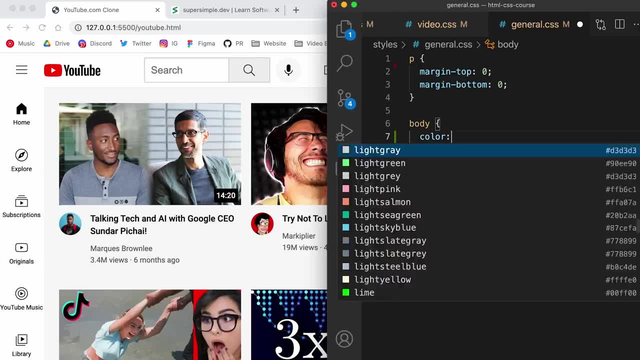 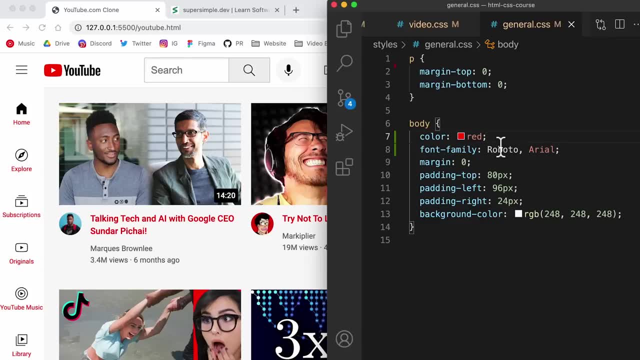 and we're going to set the property color red to change the text color of the entire page to red. If I save it, you'll see that a lot of the text is now red, like the sidebar and the video titles, But not. 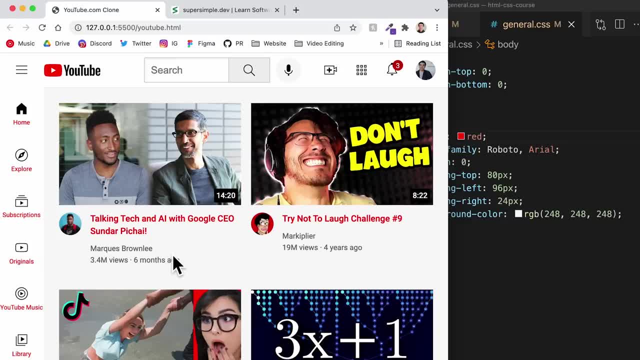 all of the text has been turned to red. So why is this happening? We mentioned this in one of our earlier lessons. CSS follows a sort of priority when you set the same style on the same element. So for these video author and video stats: 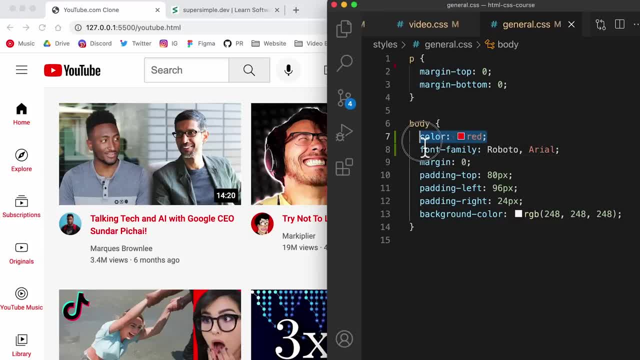 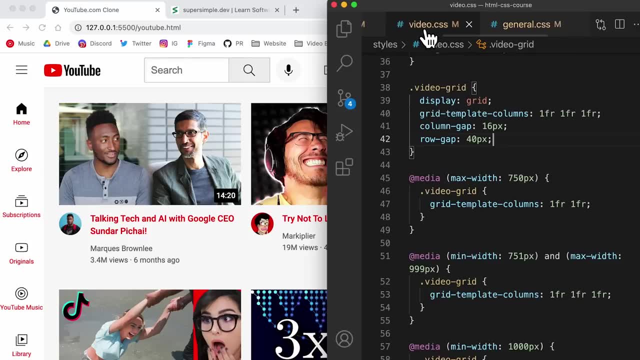 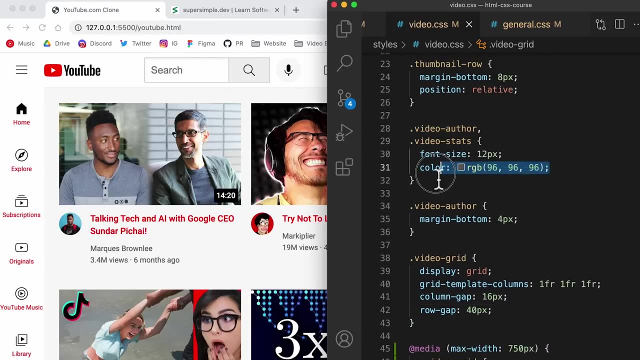 paragraphs. first we set a color of red from the body so that gets inherited down. But then if we look at the CSS for these in videocss and go into the video author- which is right here- you can see that we also set the color. 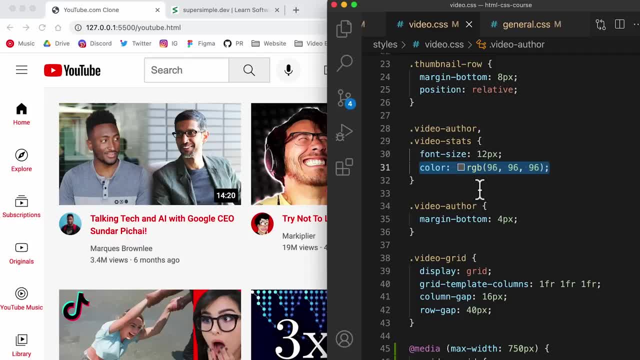 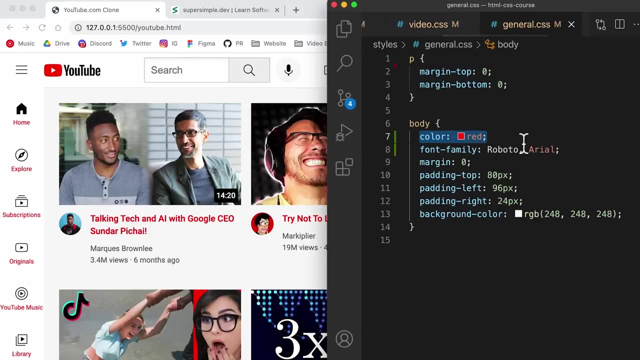 to this gray color. So the color is being set both by these styles and by the styles that are inherited from the body. However, this style is more specific because it only targets the video author and the video stats, while the style in the body 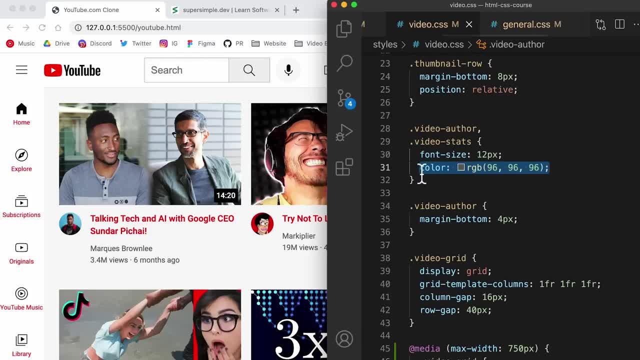 targets the entire page, So that's why this style has higher priority than the inherited style. This is called CSS specificity. Generally, if we set the same style on the same elements, like we have in this situation, the style that is more specific. 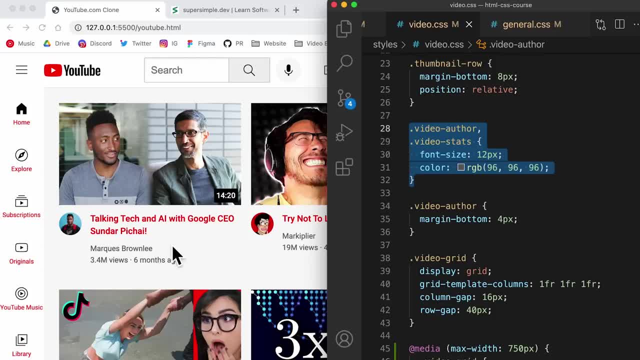 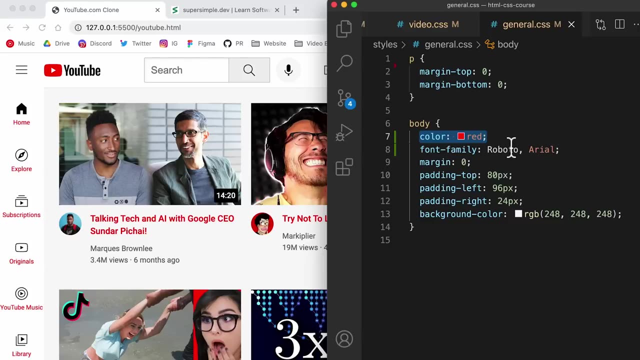 for example, this style targets only the video author and video stats. the style that is more specific has higher priority and it will override a more general style, which is what we have here. So, using inheritance and specificity, we're able to both set a default. 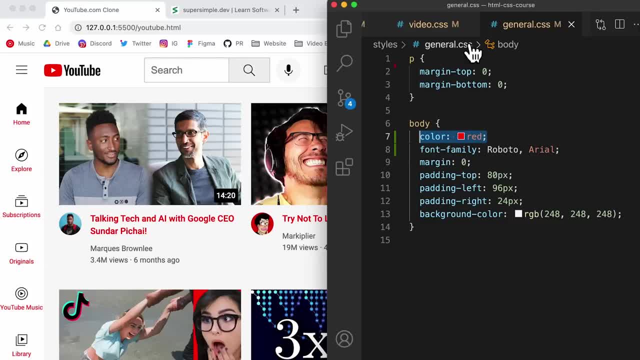 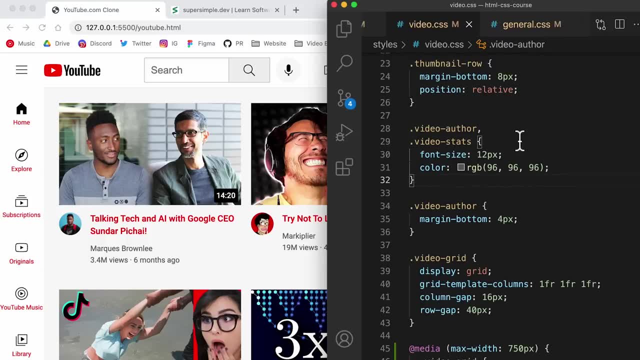 style on the outer element and then, if we need to, we can go to the inner element and then override that style. Now, in this course we didn't go through a lot of detail about specificity and its rules, and that's because we were mostly focused on 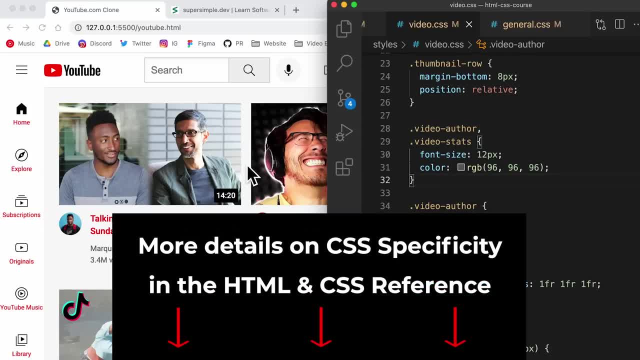 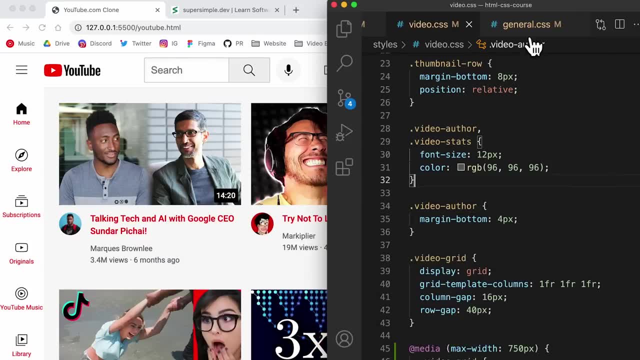 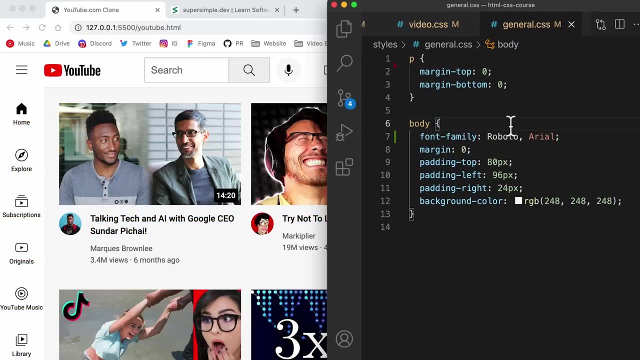 building out this project, But you can find all the details about specificity in the HTML and CSS reference below the video. For now, let's go back into generalcss and let's get rid of this practice style that we were using, And now we're. 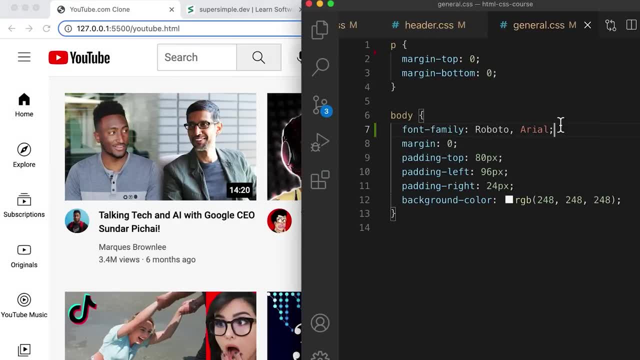 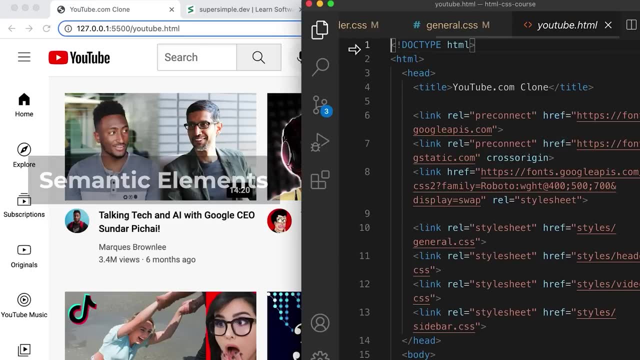 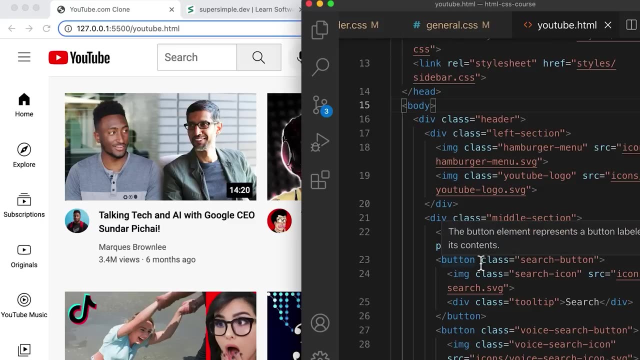 ready to move on? Next, we're going to learn about semantic elements. If we go back to our youtubehtml file, so we learned about a bunch of elements like the div, the image and the button. There's also another set of elements called semantic. 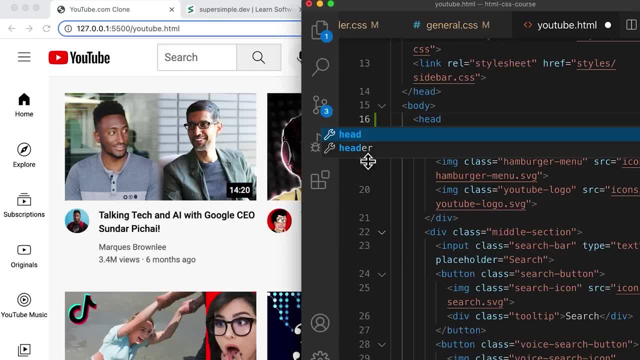 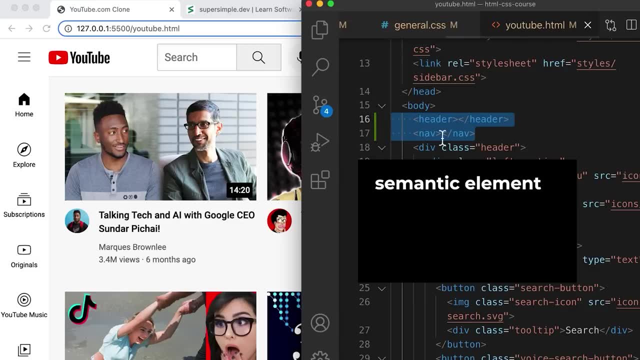 elements. So, for example, header is a semantic element and another example is the nav element. So these elements actually work the same way as a div, except they have a special meaning to screen readers, search engines and any other kind of device or 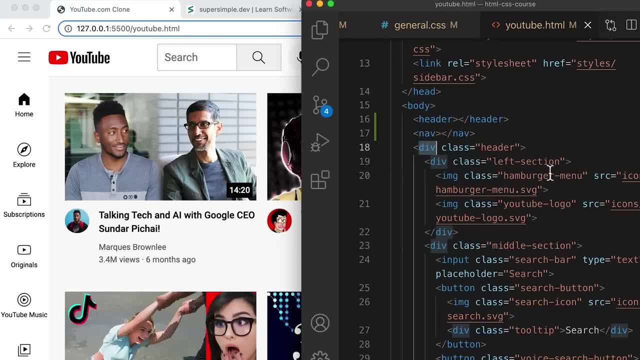 robot that is reading our webpage. So to have the structure of our webpage recognized correctly in a screen reader, we should actually replace some of our divs with semantic elements. So, for example, we can remove this div and replace it with a header. 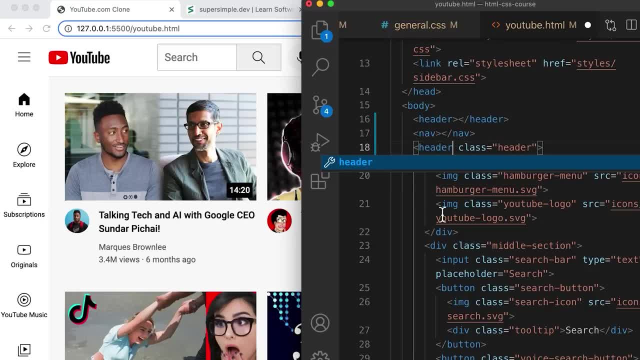 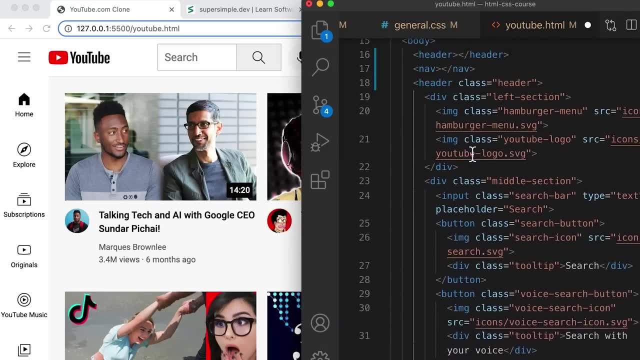 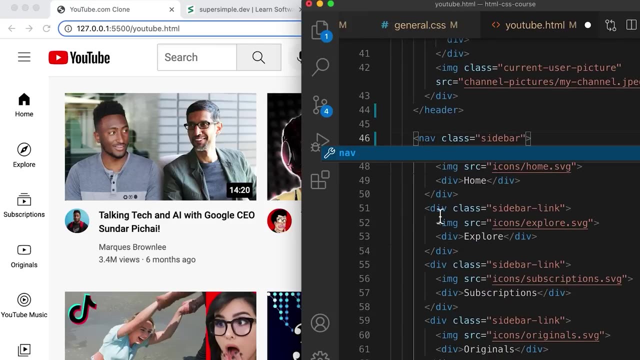 So it works the same way as a div, except it's for the robots. Let's scroll down. we can turn this into a header and then we can also scroll down to our sidebar, and we're going to change this to a nav element. 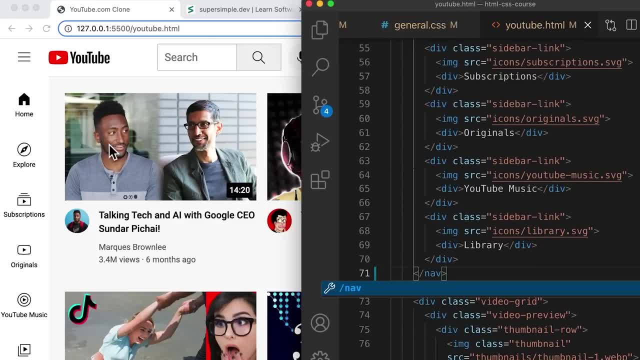 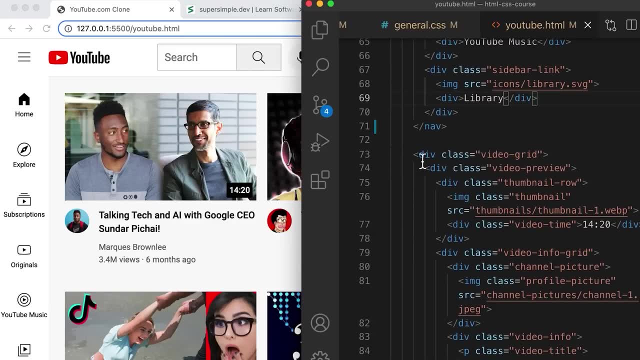 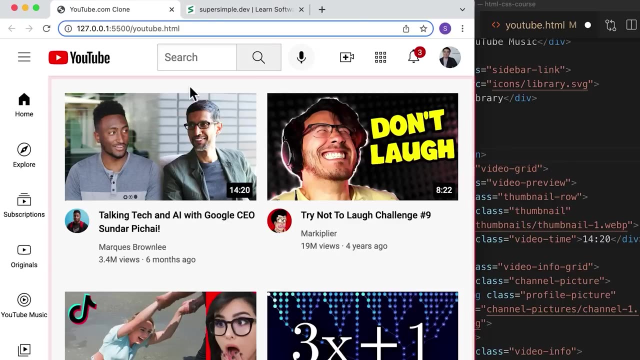 Because the sidebar on the real YouTube should help us navigate through the website. Another semantic element we can use is called main, So this should contain the main contents of your website, which, for us, is this part. We're going to move everything inside here. 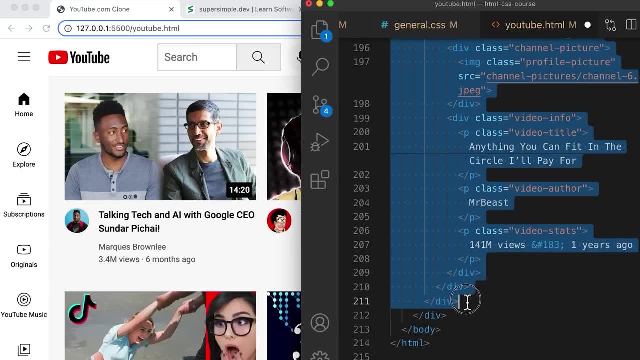 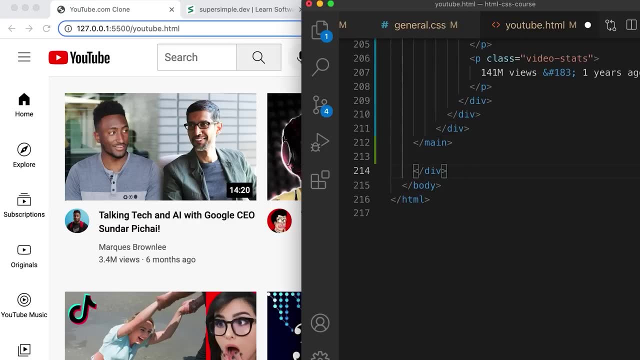 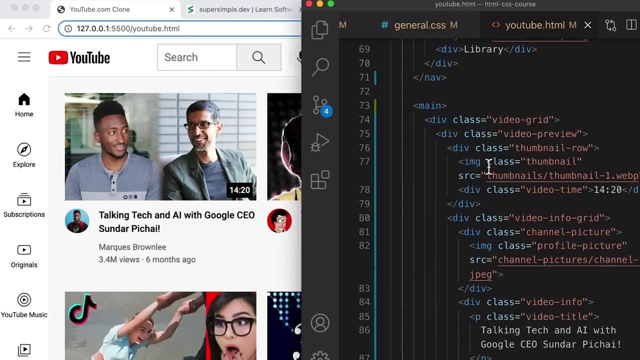 to the main element. So I think it's this I might be missing, Okay, So move all of that into main And let's scroll back up Now. inside main, we're going to have a video grid, but we might also. 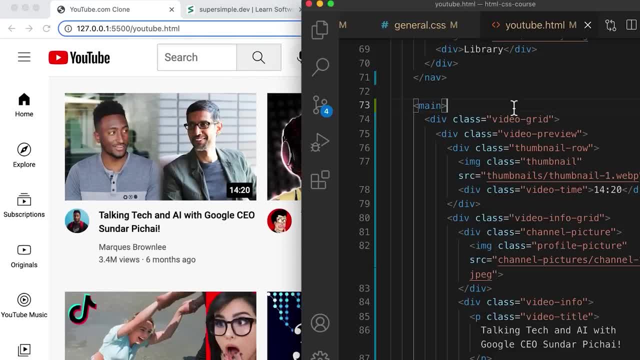 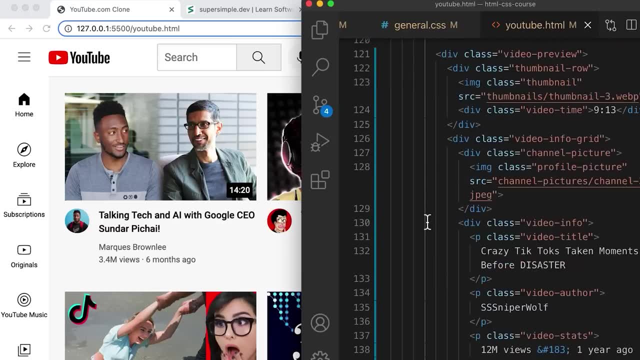 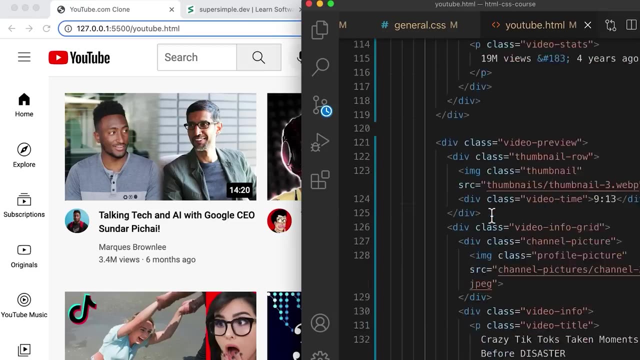 have other things below the video grid. So the video grid is known as a section of our main content. Let's save that and scroll all the way down to the end of our video grid and remove this with section. So that's how semantic elements work. 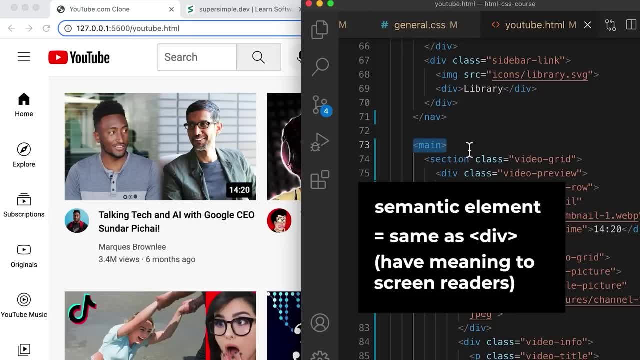 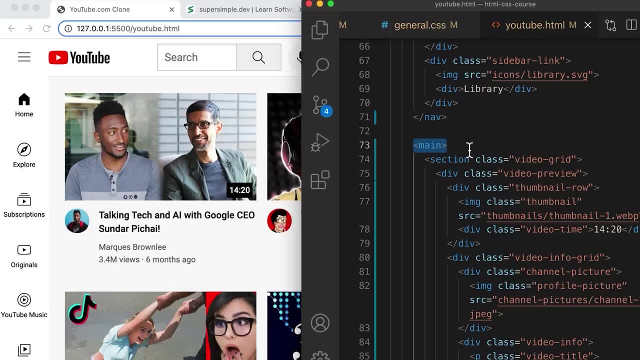 They're just the same as divs, except they give a special meaning and structure to our page for search engines and screen readers. Now the final thing I want to show you in this course is how to write comments. So comments are pieces of code. 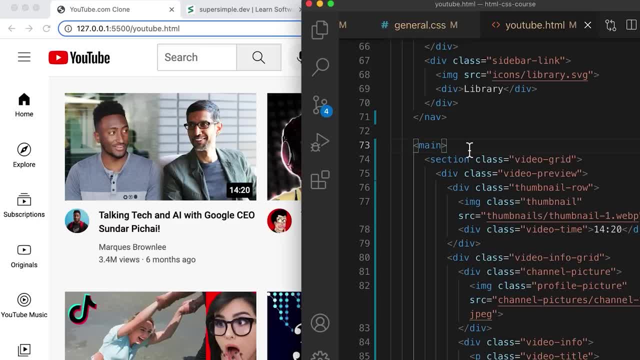 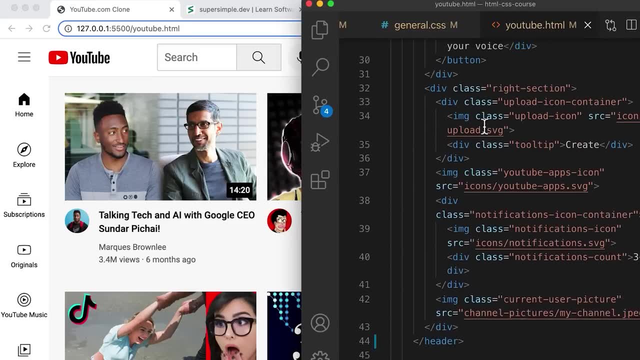 that the computer ignores, but you can read yourself to remind you of information or to tell yourself what's going on in the code. So, for example, if we scroll up to our header- maybe I forgot how we created this tooltip So we can actually add- 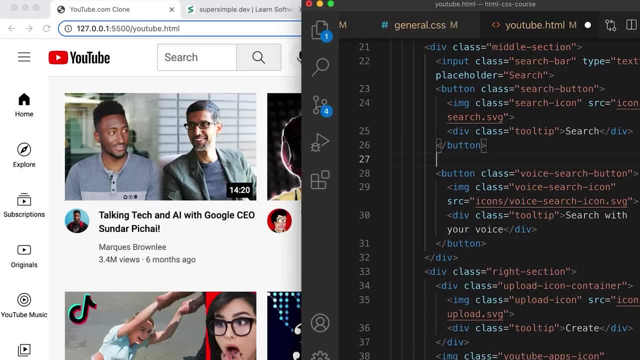 a comment in the code. that reminds us. So let's add a comment here. We're going to type "-" And we're going to end the comment with "-" like this. So this is a comment. If I save the webpage, you'll see that this text appears. 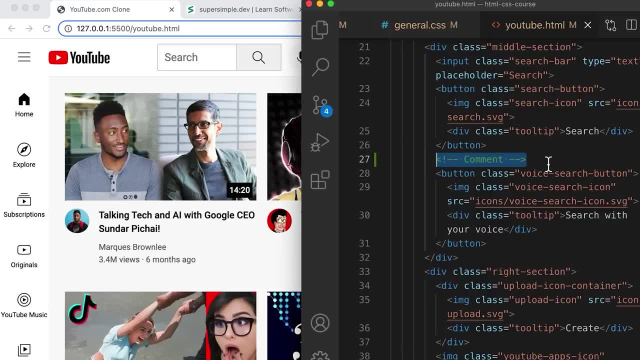 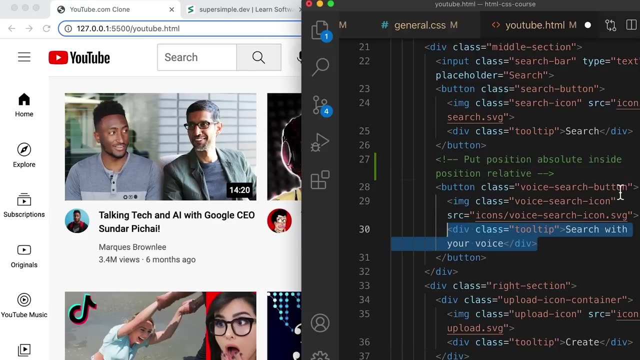 nowhere on the webpage And that's because the computer basically ignores comments. So we can add comments like: put position absolute inside position relative to remind us that we need to put a position absolute inside a position relative to create this tooltip In CSS. we also have 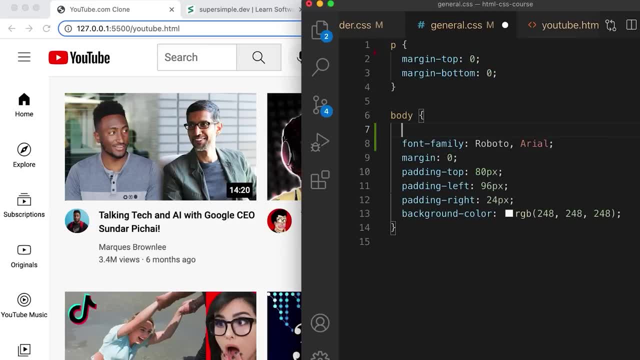 comments. So, for example, we go here We can write a comment by writing "-" with star slash. Now, everything in between here is a comment. So we can say this style below will be inherited, So, as you can see, comments add. 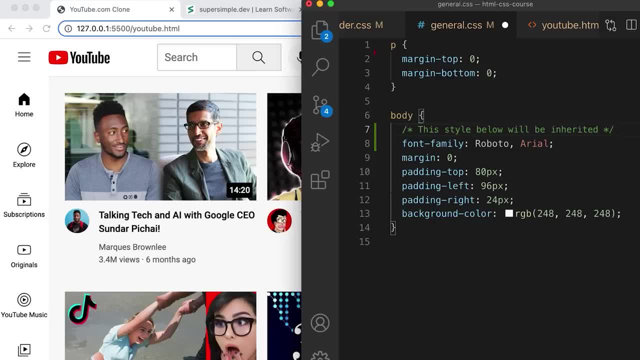 extra information into our code without affecting our webpage, So it's a really useful tool when you're working on a team to document how your code works. And now for everything in this course. if you ever forget, remember that you can always google it, For example, 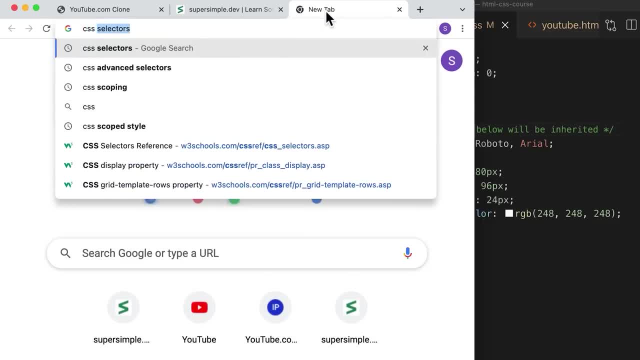 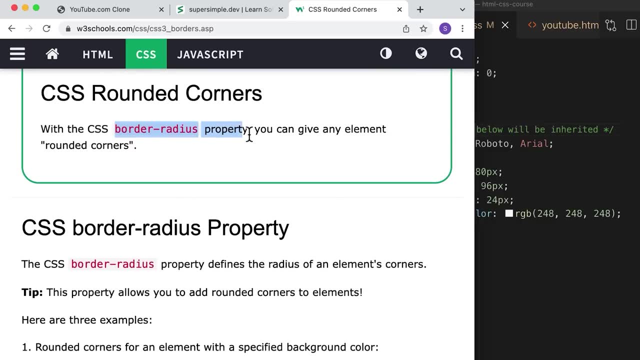 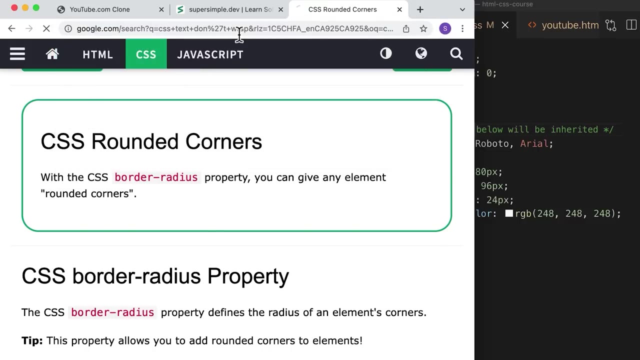 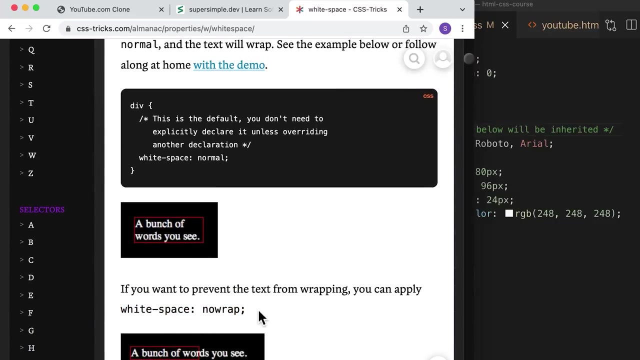 if I go to google, I can search things like CSS rounded corners, and it will give us the border radius property. I can also search for something like CSS text don't wrap, and it will give us the whitespace property and the value whitespace, no wrap. 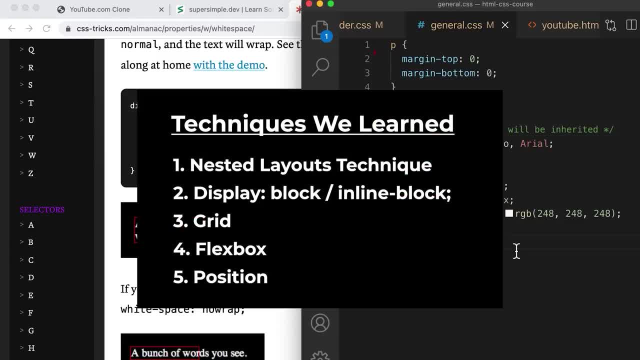 So this is how you learn from here. You take the techniques that we learned in this course, such as the nested layout technique, using grid, flexbox and position, and then you try to recreate things that you see on the internet And, if you ever, 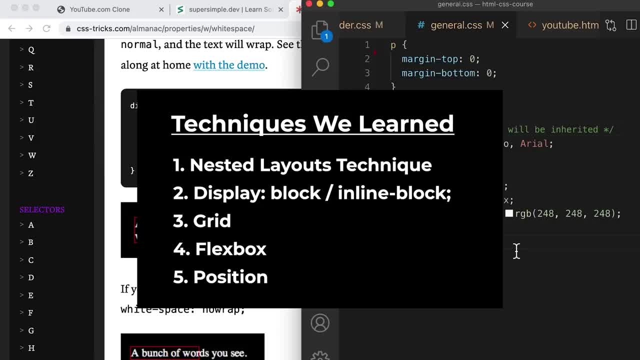 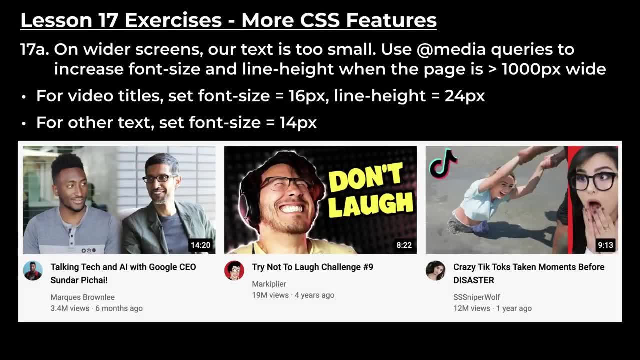 forget, you can google and get the exact code that you need. So, now that we learned all the major skills that we need to build complex websites like YouTube, here are some challenge exercises that you can do to create other popular websites on your own. 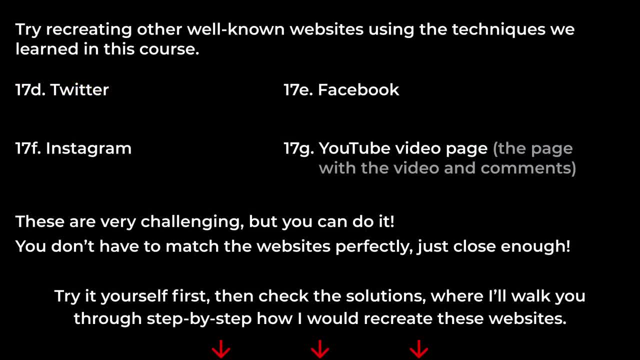 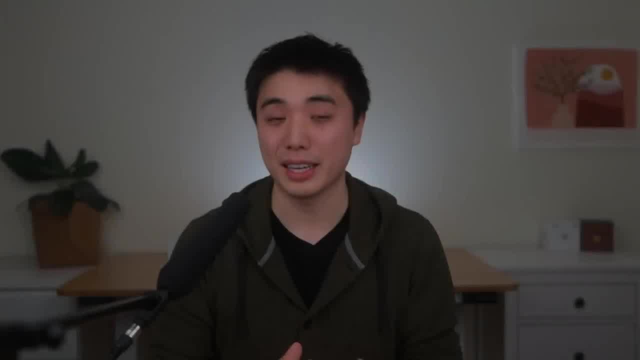 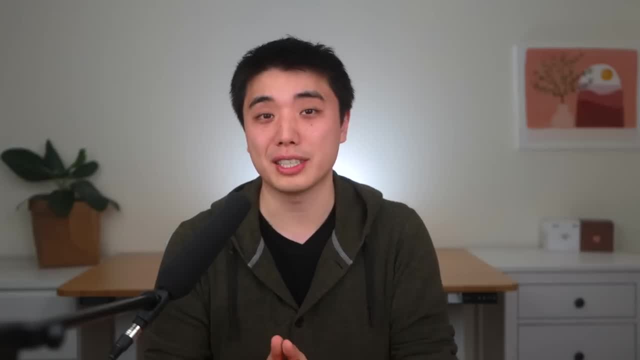 Thanks so much for taking this course with me. I hope you now realize that creating websites is not as intimidating as it seems. We just need to create each part of the website step by step, using the major features of HTML and CSS that we learned in this course. 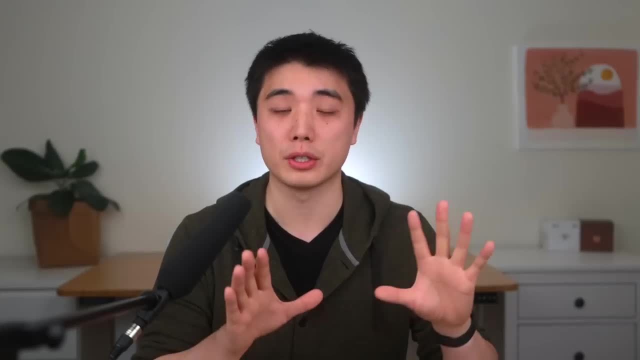 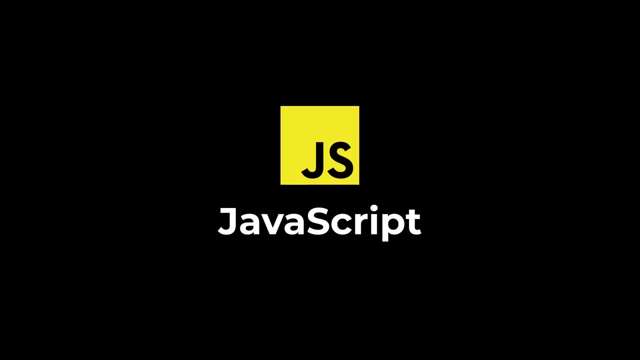 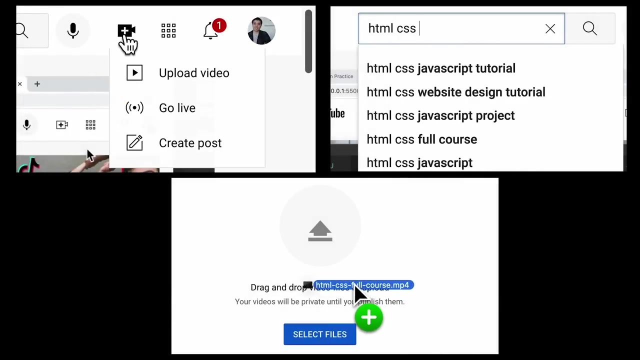 Now, where do we go from here? As the next step, I recommend learning the javascript interface, The javascript programming language. Javascript is what makes our webpage interactive, For example, if we click something, type some text or drag something onto the page. 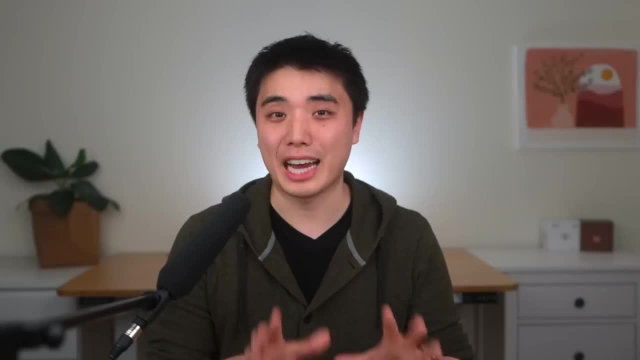 javascript is what updates our page, So it's a natural progression from HTML and CSS. Now, if you want to learn javascript, I have a full javascript course for absolute beginners that you can find by clicking this link. Again, thanks so much for watching. My name is. 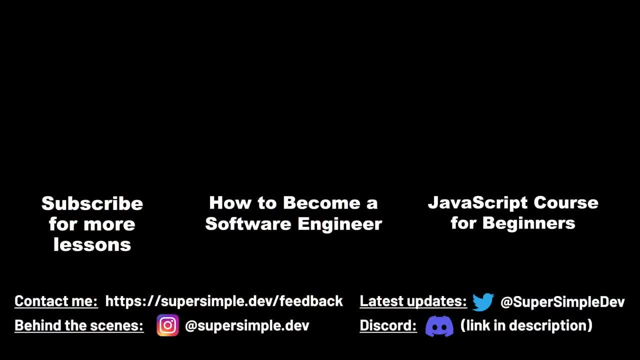 Simon from supersimpledev. I want to make a tech career possible for anyone. If you have any comments, questions or feedback, please leave them down in the comments section below, If you want to support this channel and you want more courses. 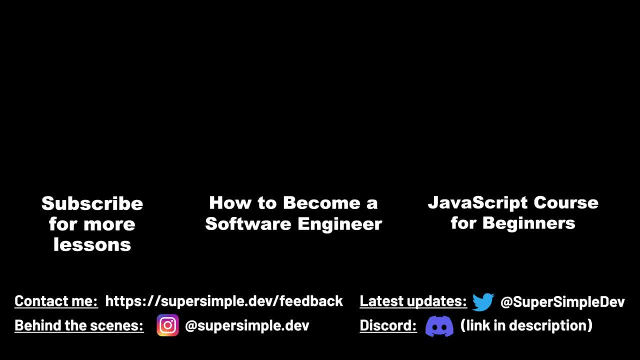 like this. please click the subscribe button. Thanks so much and I'll see you in the next one.